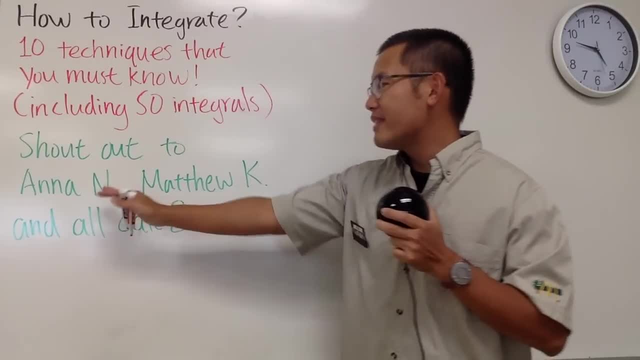 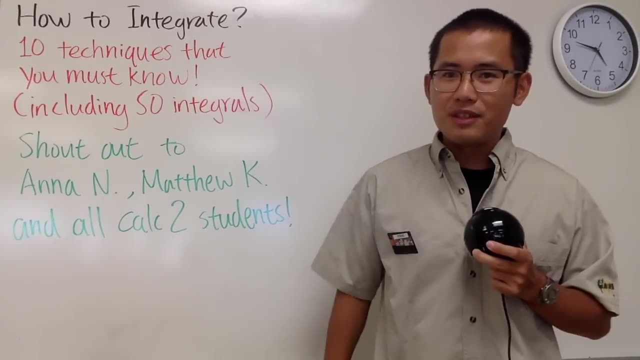 already. Before we start, I just want to give a big shout out to Anna and Matthew. They are my current students And I know you two have been subscribed to my channel for a while And you guys have been watching my videos. Thank you guys for the support And, of course, 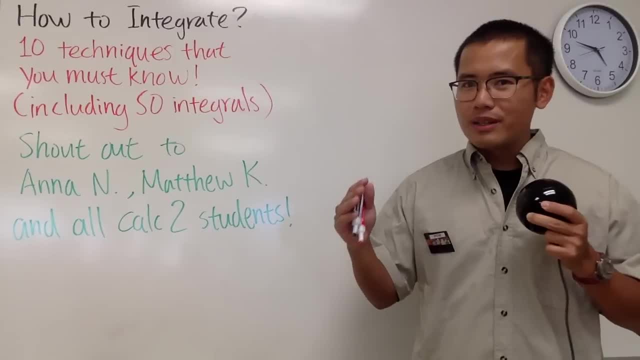 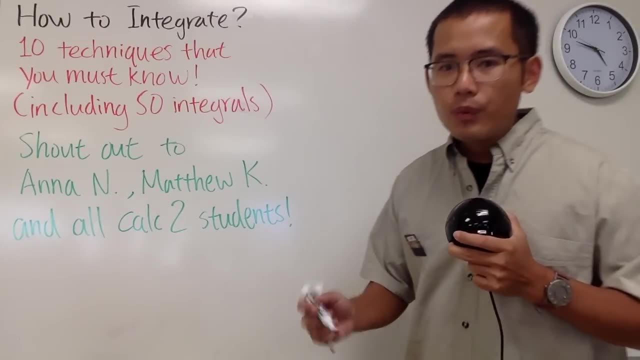 for all the calculus 2 students. Either you are taking my class right now or maybe later in the future, or maybe you are taking with somebody else. Best of luck to you guys. So here we go. Of course you guys can go download the file, The link to the file with some notes. 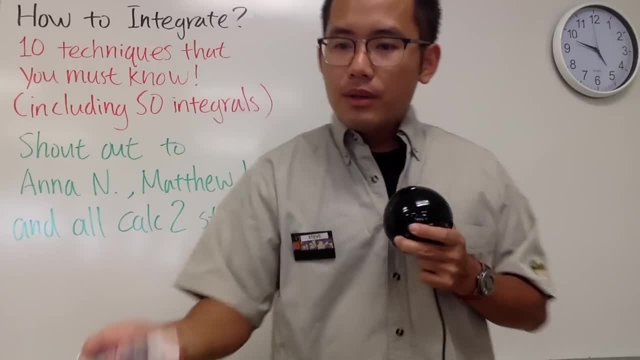 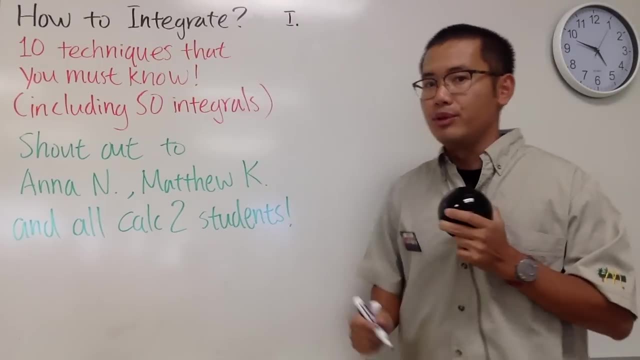 is in the description for you guys already. Okay, so here we go. This is the first part. Well, I'll just call this the first category or the first technique, Up to you. Here's the idea, Before you want to do any like a real legitimate technique. 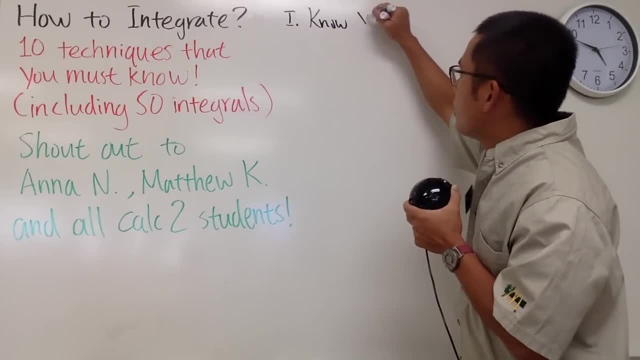 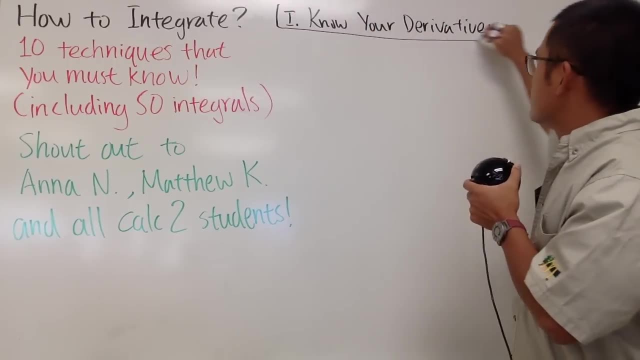 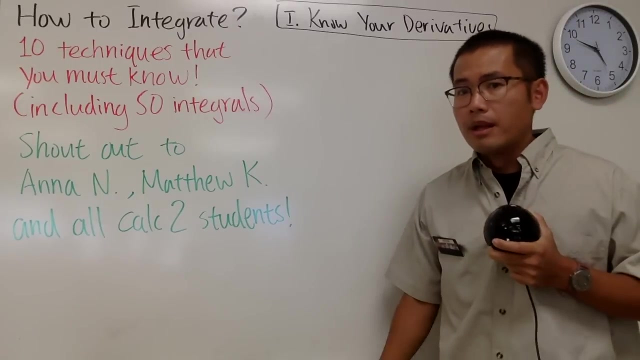 before you want to do any other integrals, you must know your derivatives really, really well, Right? So the first thing that you have to know is all the derivatives. And you might be wondering: why Aren't we talking about integrals? Why am I bringing up derivatives? Well, because some of 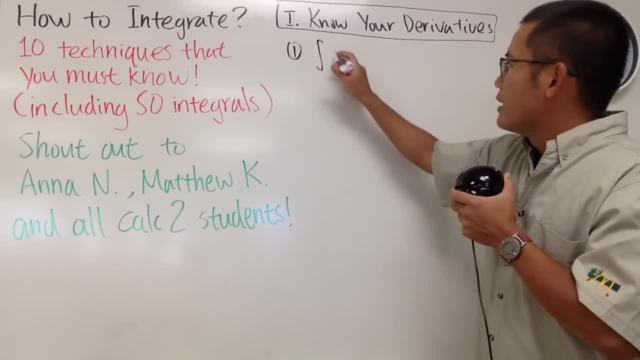 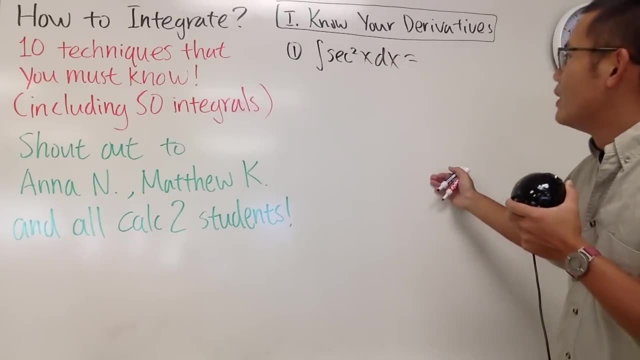 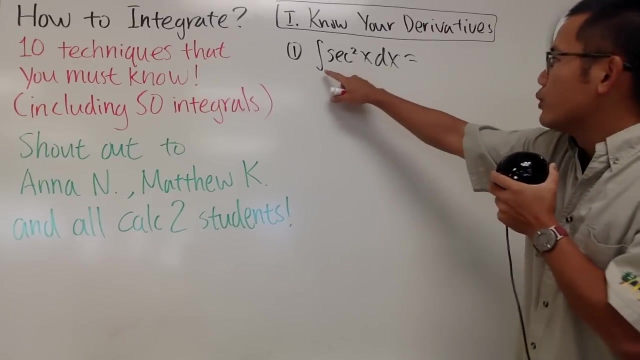 the problem. let's look at the first one. For example, if we have the integral of secant squared- x, dx- Well, to do this, all we have to do is ask ourselves the derivative of what will give us secant squared. That's all, Because, keep in mind when we are trying to do an indefinite integral. 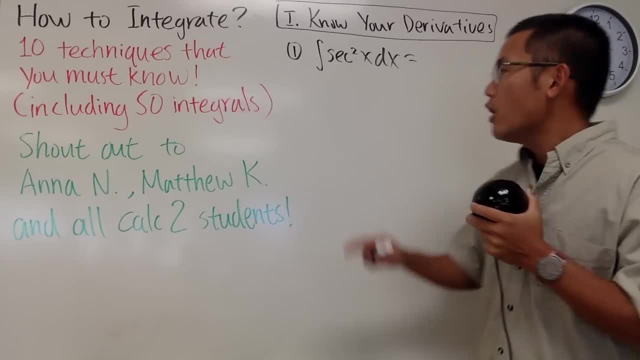 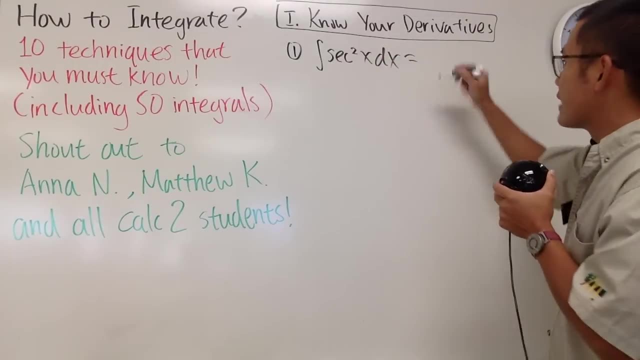 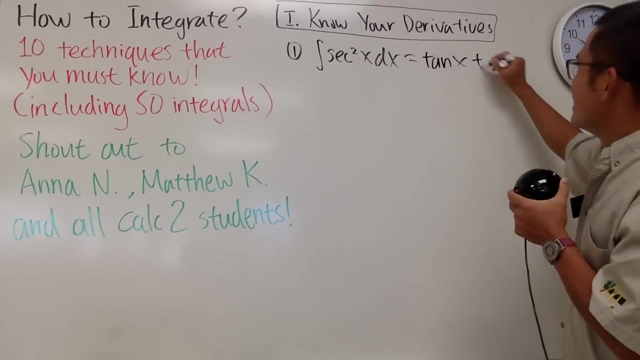 we are pretty much just doing the entire derivative. So if we can think about derivative of tangent x will give us secant squared and that's it. So the integral of secant squared x is equal to tangent x. And don't forget your plus z, Because if you differentiate this, you get that. 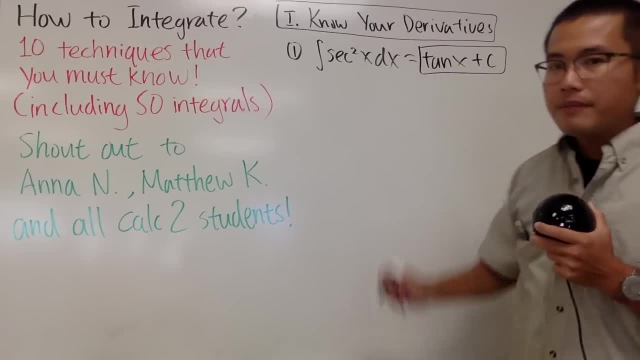 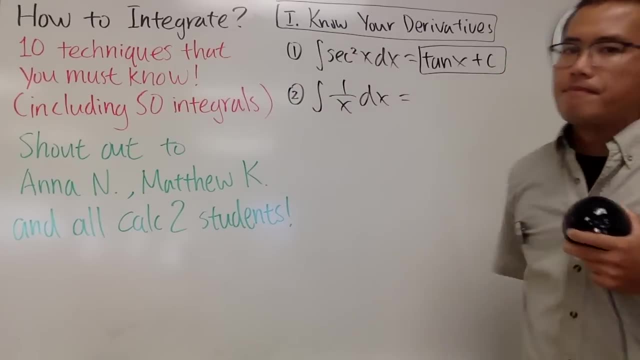 So that's it: No more to be show. This, is it Right? And let me just talk about another one. Let's look at number two. We have the integral of one over x, dx. hmm, the derivative of what will give us 1 of x. 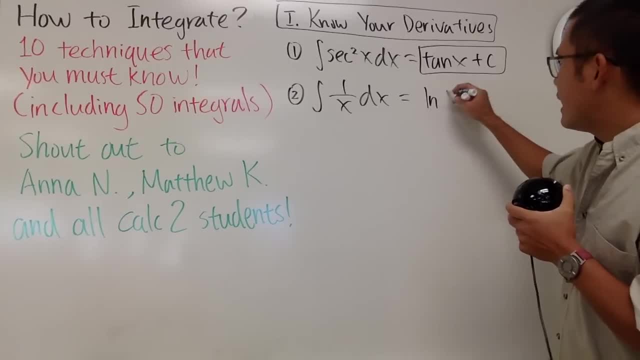 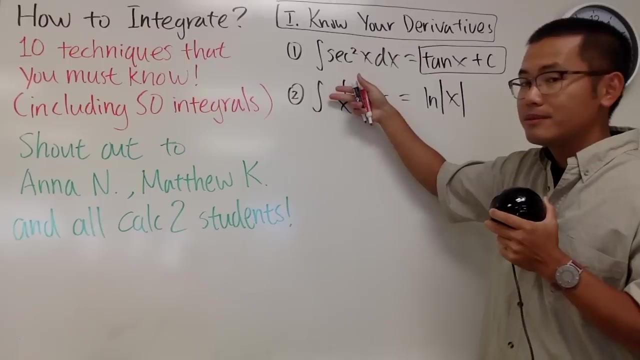 The answer to that is natural log of x. And here's the deal: When we go from the integral of 1 over x to natural log of x, be sure you attach the absolute value, especially when we have some numbers right here, If we have negative numbers. 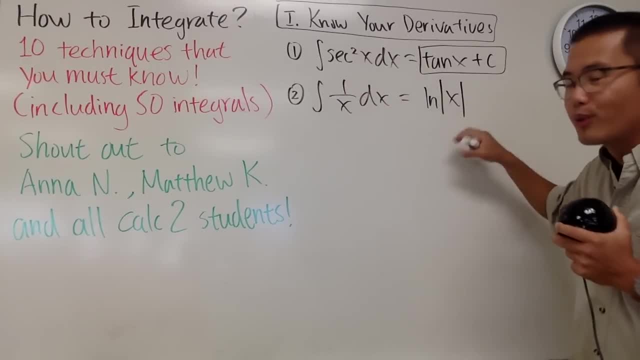 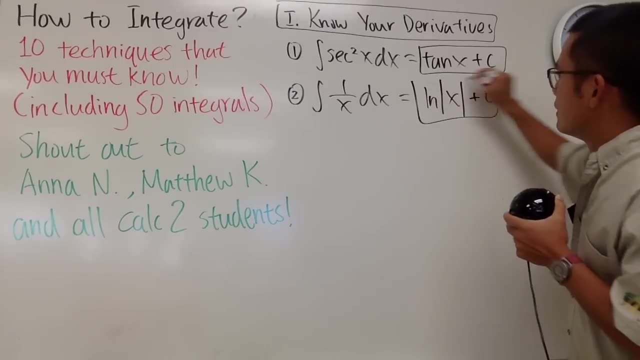 well, you have to make sure that we have the absolute value. so that log of absolute value of negative numbers, that makes sense, right? Okay, so that's it Then, number 3.. So I have these examples prepared for you guys. 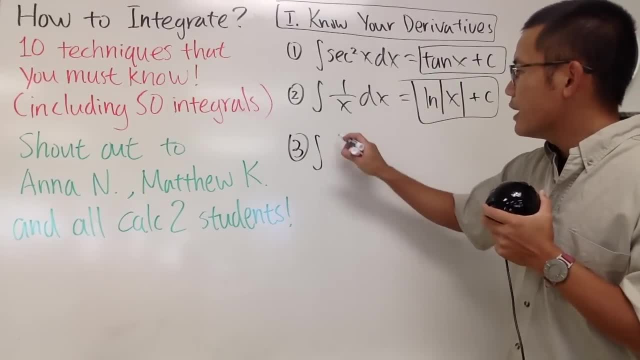 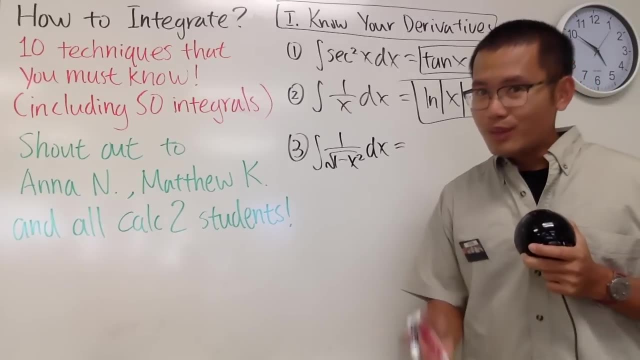 and we'll just go over them. Let me talk about the other one for you guys. Let's look at the integral of 1 over square root of 1 minus x squared dx. Hmm, this one is slightly harder, but it's not so bad either. 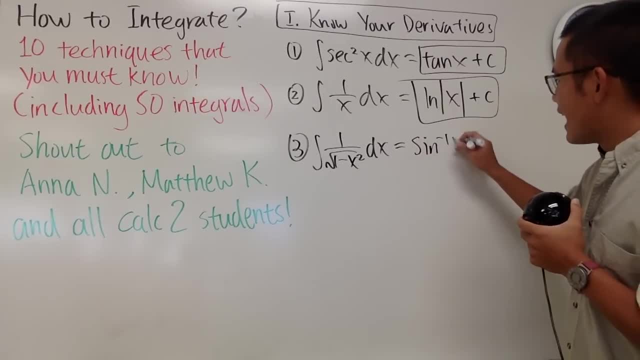 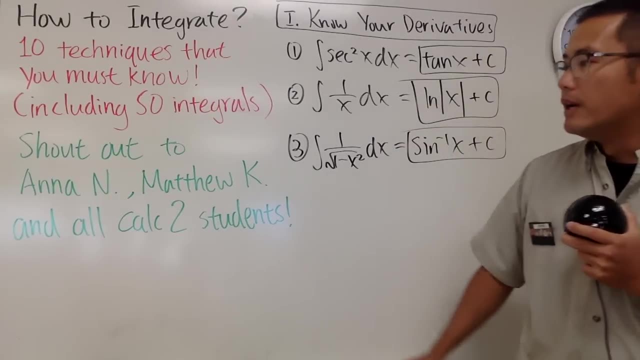 This is just going to be inverse sine x plus c. Again, all this right here. you just have to know your derivative. You just have to know your derivative really, really well. And now I'm just going to erase this. I'll give you guys five more for you guys to think about. 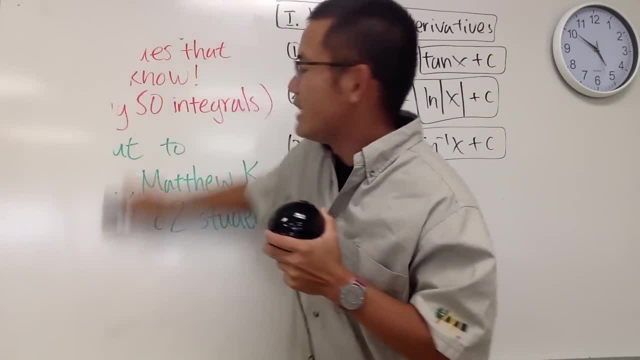 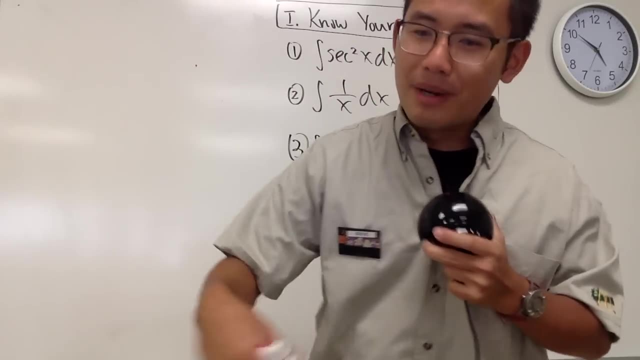 and then we will go over them real, real quick. So that's the idea. And if you haven't done calculus, if you haven't done derivatives or integrals for a while, well, we better just go back to review all the things. 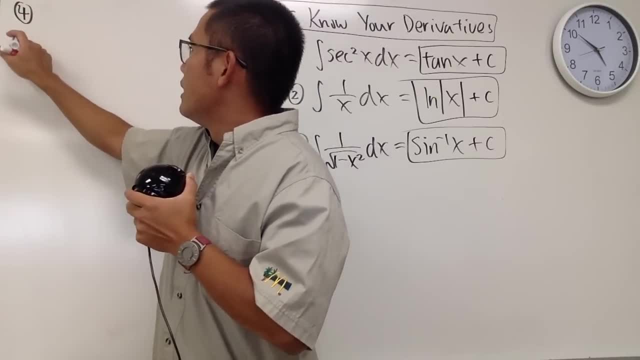 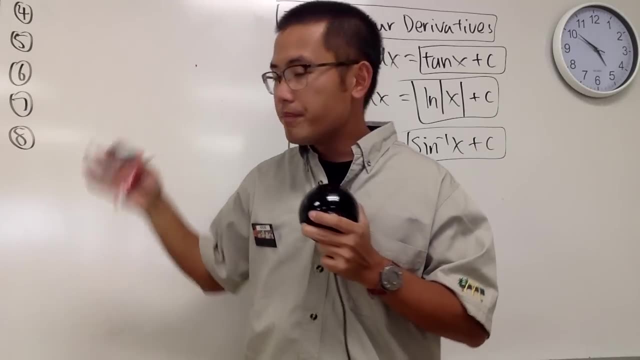 maybe from Calc 1, from your previous class, etc. etc. So, anyway, let's look here: Number 4,, 5,, 6,, 7, and 8. And I think these are the eight most common ones that you definitely have to remember. 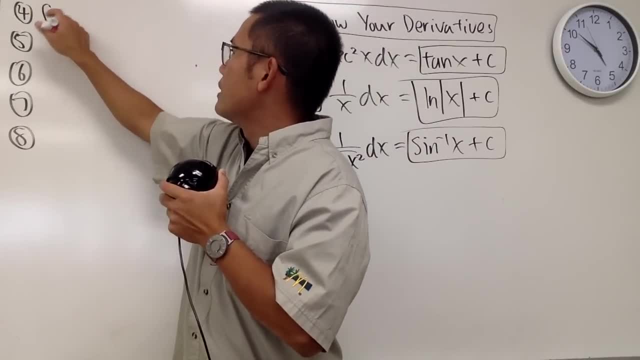 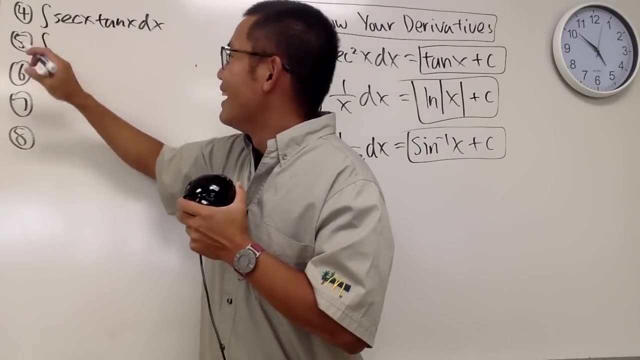 and I have it right here. Let's look at the first one right here. Here is the integral of secant x times tangent x dx. And let me just put on the questions. first, Number 5, the integral of 1 over 1 plus x squared dx. 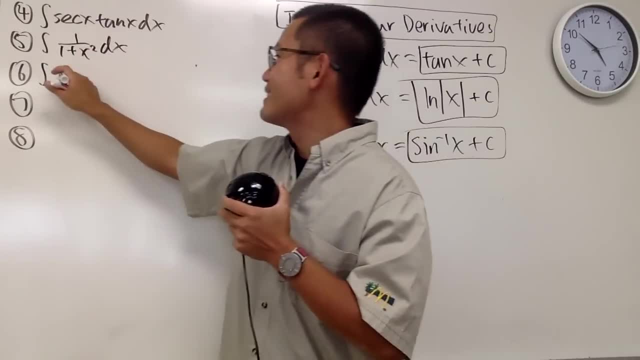 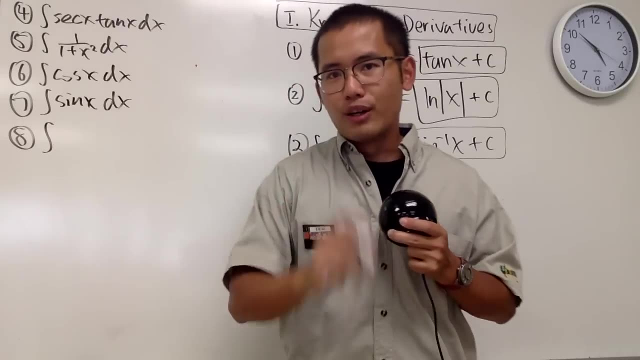 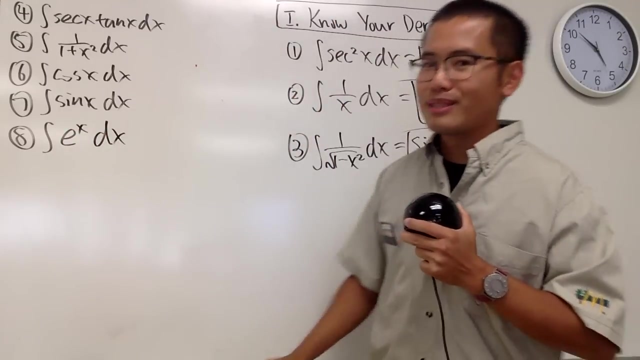 And then number 6, we have the integral of cosine x dx And, of course, integral of sine x. And number 8 is the hardest one: The integral of e to the x dx. Anyway, pause the video real quick and just think about the answers to here, right? 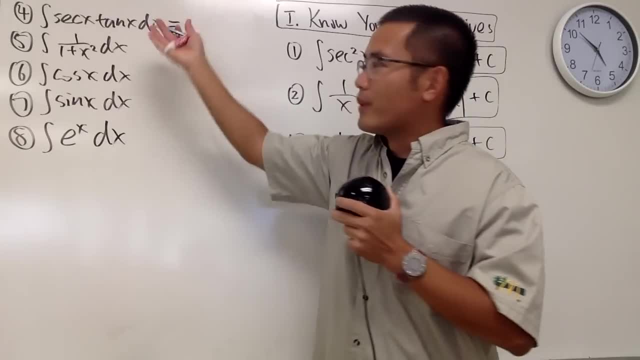 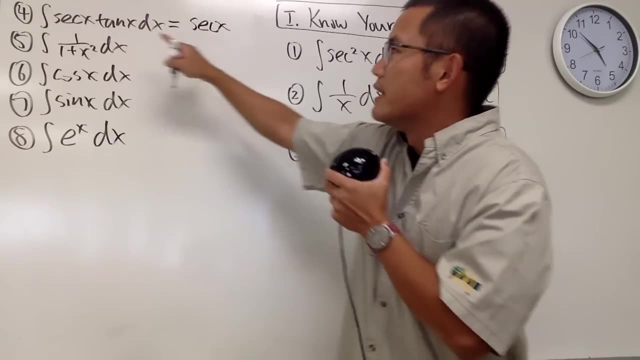 Okay, so I trust you guys. Now let's go over this together. For this one, well, we just need secant x. Yes, because the derivative of secant x will give us secant x times tangent x. That's it, right. 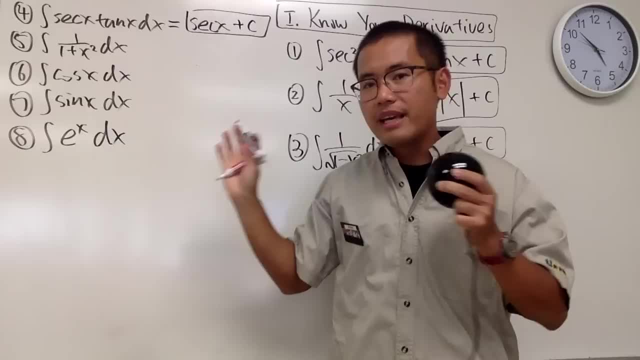 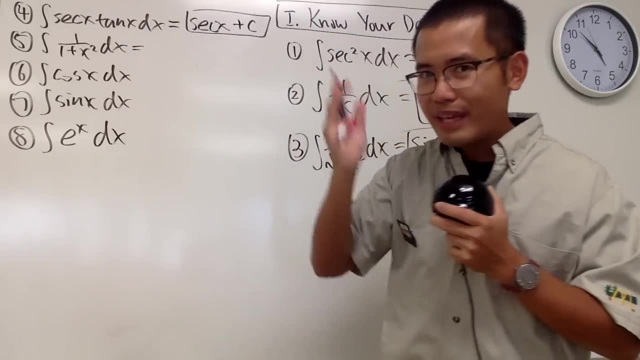 So secant x plus c. Again, we don't have to do any work, It's just by knowing the derivatives And number 5, this is going to give us inverse tangent x. Very good, And this is how we write the inverse tangent x notation. 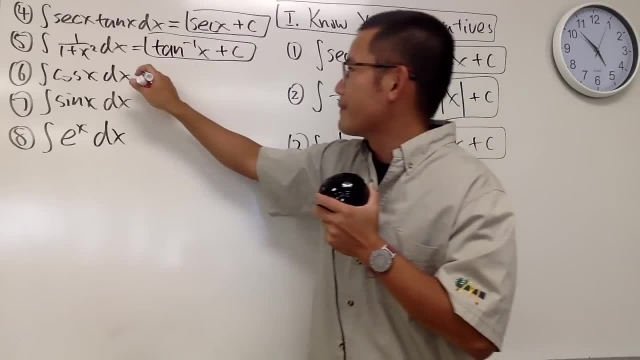 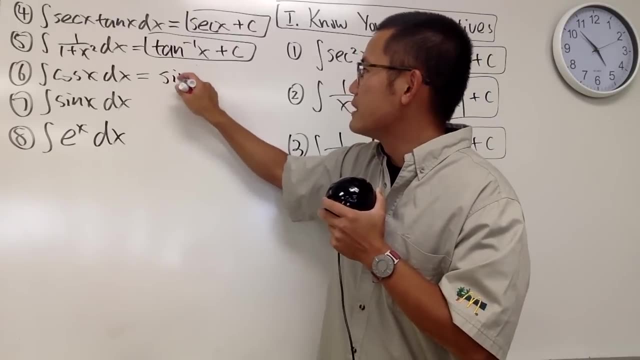 And I'm going to just discuss this after we finish this right here. Number 6,: what's the integral of cosine x? Well, the answer to this one is positive sine x, Because the derivative of positive sine x will give us positive cosine. 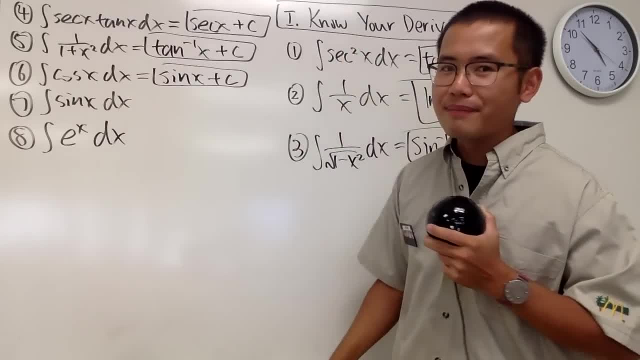 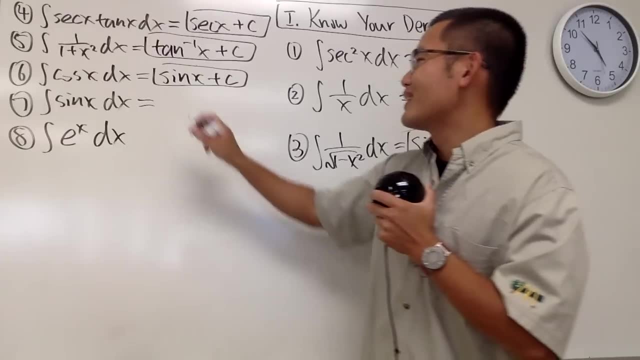 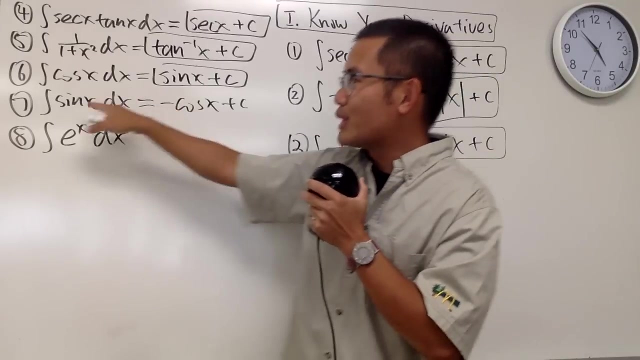 So the integral of positive cosine will give us positive sine. However, if we are integrating sine x, we will have to get negative cosine, Because the derivative of cosine is negative sine. we must have another negative so that we can end up with that positive right. 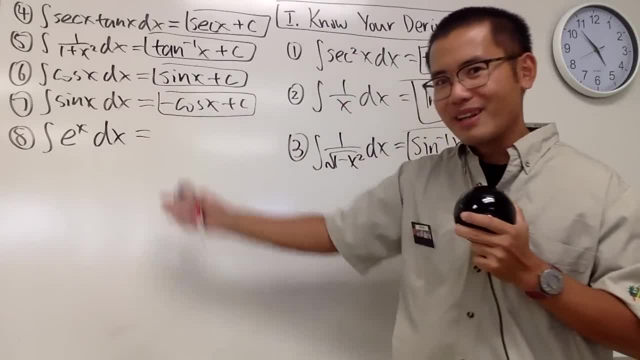 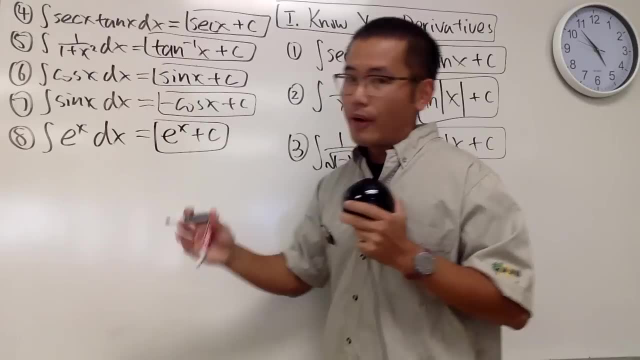 So this is the answer for that. And lastly, the hardest one, the integral of e to the x is just e to the x, Yeah, Plus d, Alright. So that's pretty much it. And now, before we continue, let me just tell you guys that we will do a lot more like other questions, okay. 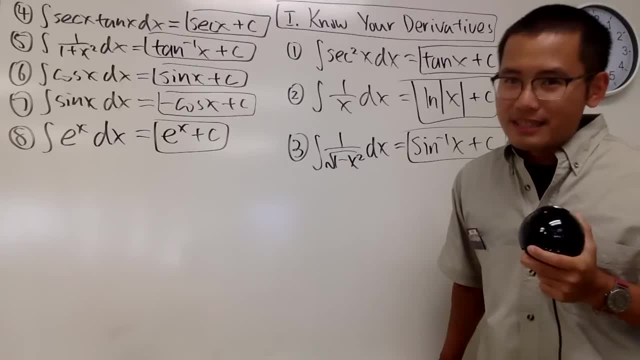 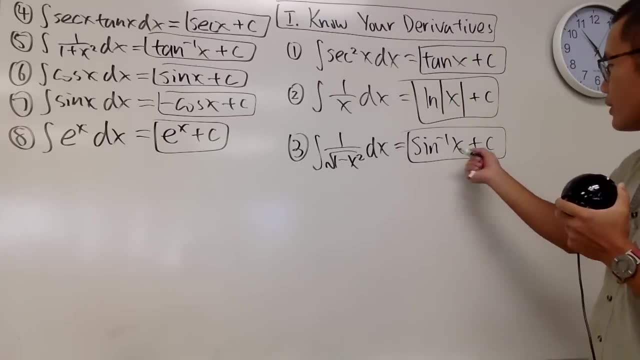 So I know this first 8 questions. I didn't really show you guys any technique, But again, this is like the default that you really really have to know really well. alright, And let's talk about the notations right here. 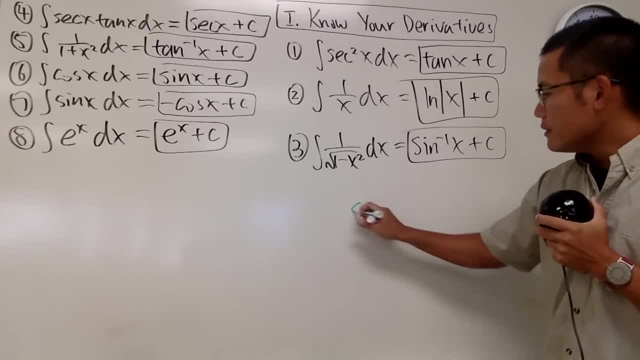 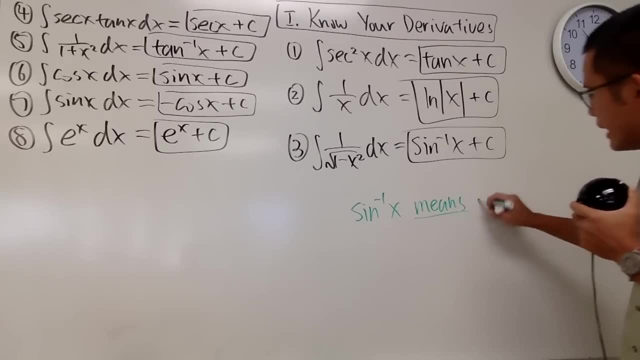 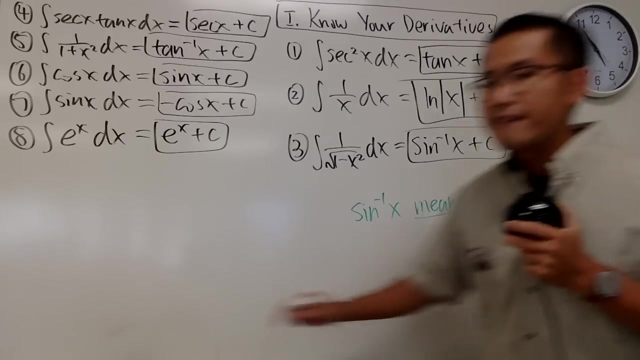 Let me pick this one. for example, When we have sine with a negative one right here, x. this means alright, This means the inverse, The inverse sine function, right, The inverse of the sine function. So what I mean by this is the following: for you guys, right? 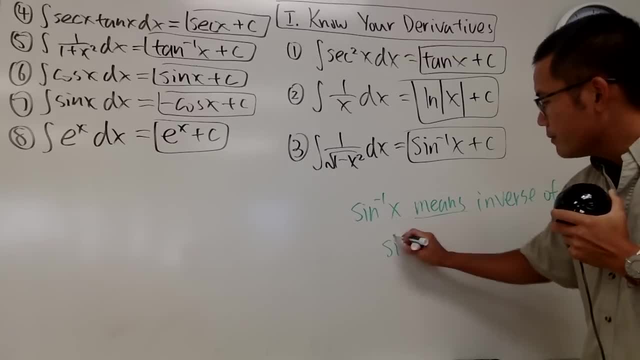 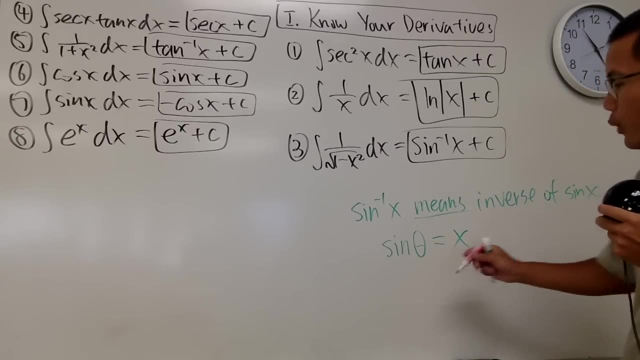 Suppose, today we have sine of an angle- and this is the original Sine of an angle is equal to x, for example. Well, what we can do is we can do the inverse on both sides like this, And in another word, we will be able to say: alright, this is the inverse of the sine function. 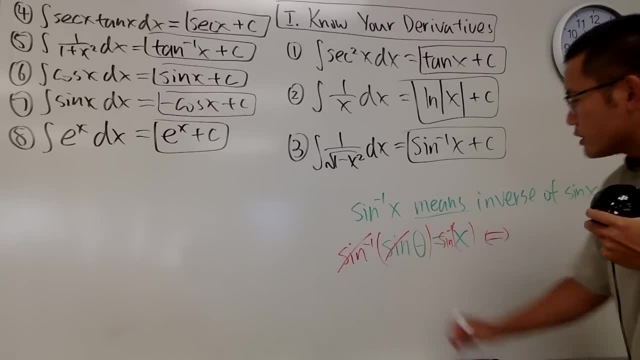 We will be able to see that the angle theta- because this and that will be cancelled here- the angle theta is equal to the inverse sine x, like that. So this is the idea of the inverse function, just like the inverse tangent right here as well. 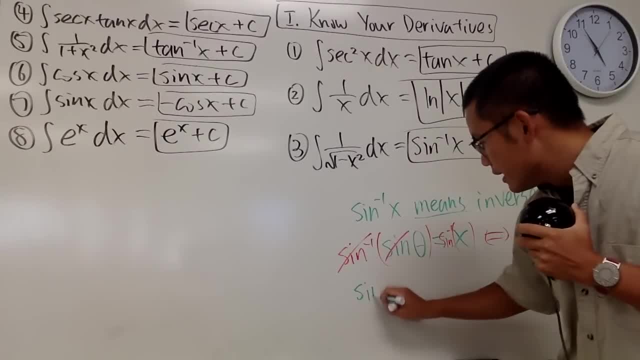 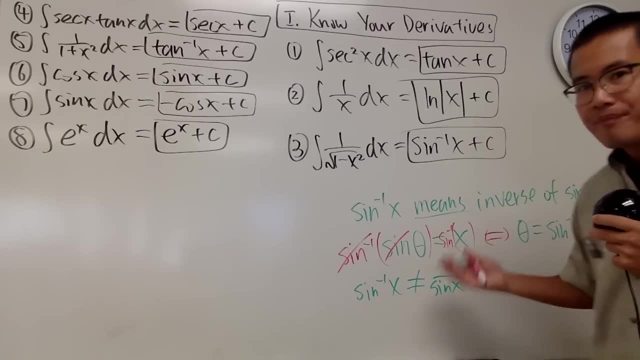 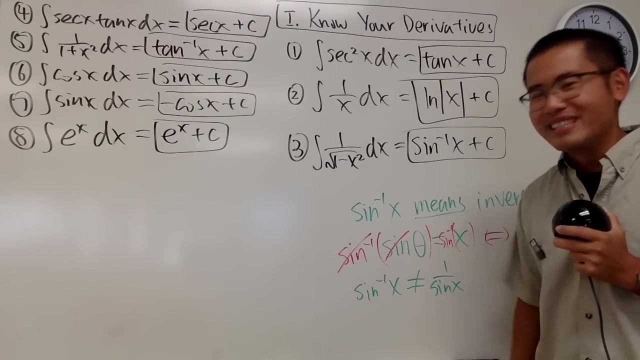 Notice the following notation: When we have the inverse notation like this, do not interpret it as 1 over sine x. Unfortunately, this is not the case When we have the negative one right here. I know this is the most heady notation, but we just have to live with it. 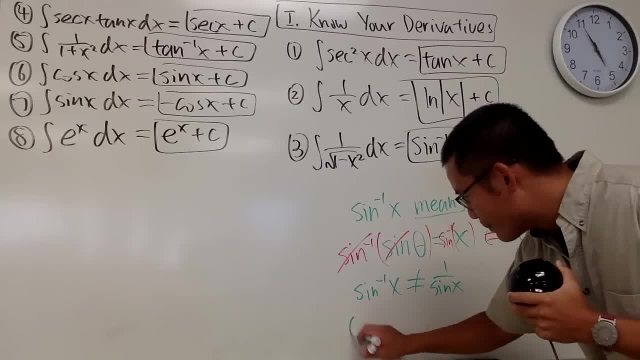 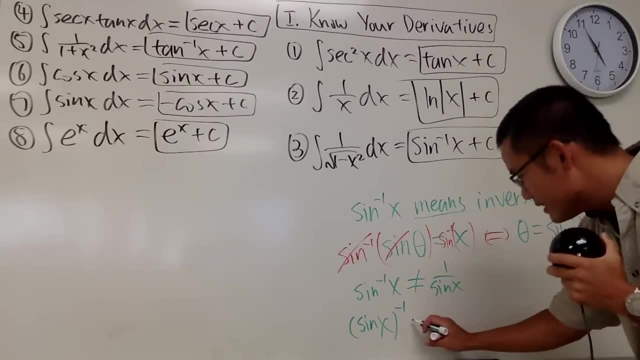 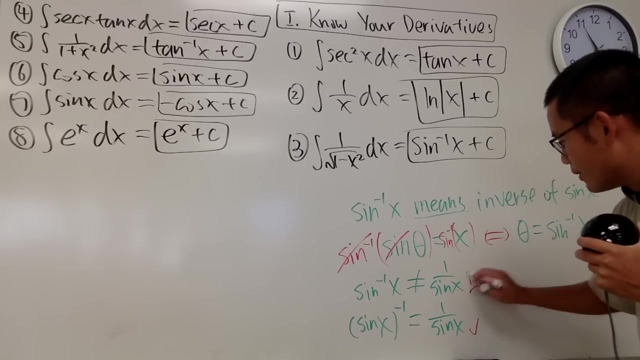 Sorry, Yeah. However, though, if you have a parenthesis with sine x inside and then raise to the negative one power right here, this does mean 1 over sine x. This is okay. This right here is no Right, I know. 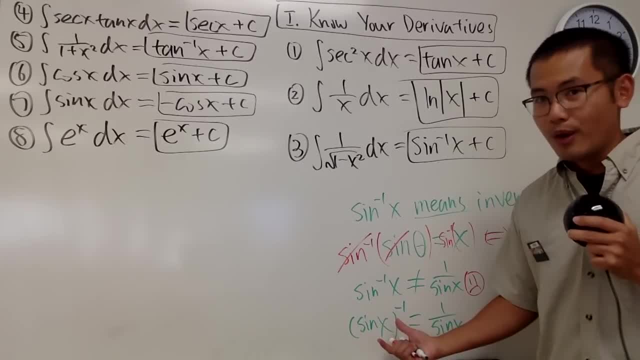 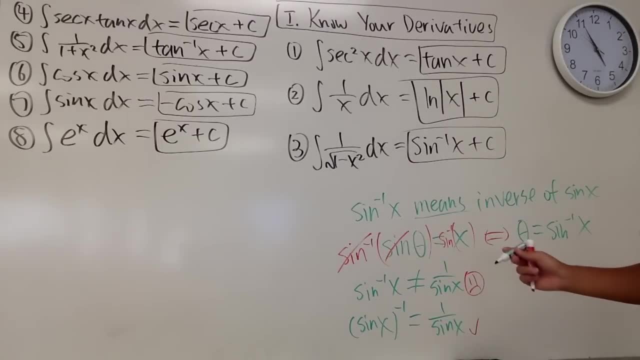 I know this is just so bad. So you have to use parenthesis really, really well, And please just don't ever put the negative two right here. Seriously, that's just a horrible thing to do. And another notation that people might prefer is if you have sine inverse x like this right here: 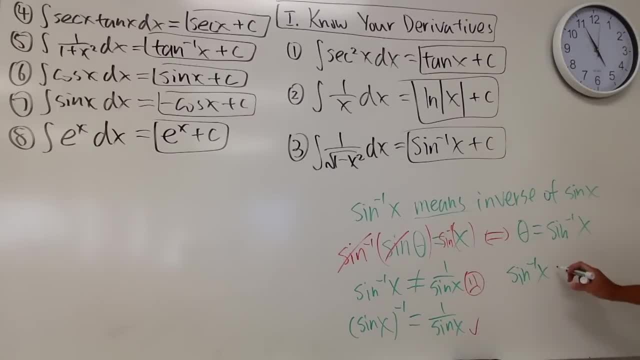 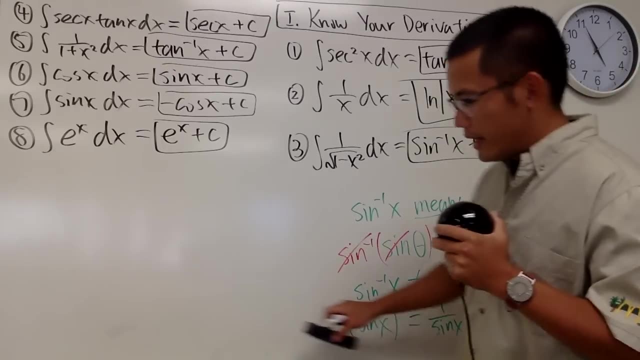 If you really don't like this notation, some of the people will actually just write it as the arc sine notation, Arc sine of x, like this. So this is just a notation issue and we just have to kind of get used to it, because I know it's not the ideal notation. 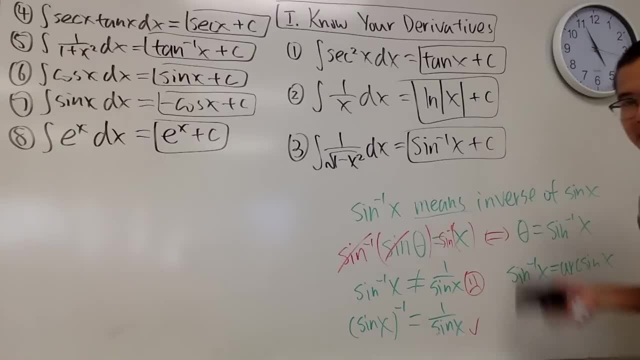 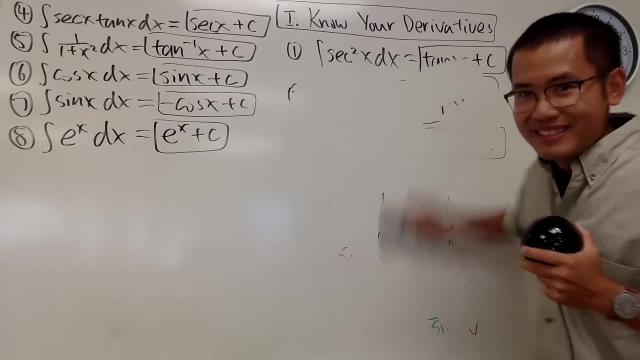 But again we just have to deal with it, That's all. So this is the first category right, And again we will have the harder ones coming up. So, yeah, this is just like a warm-up right. 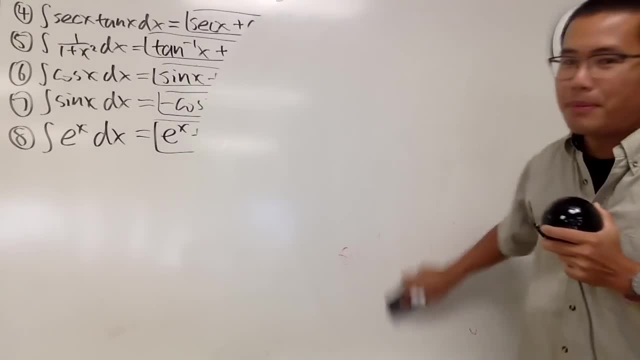 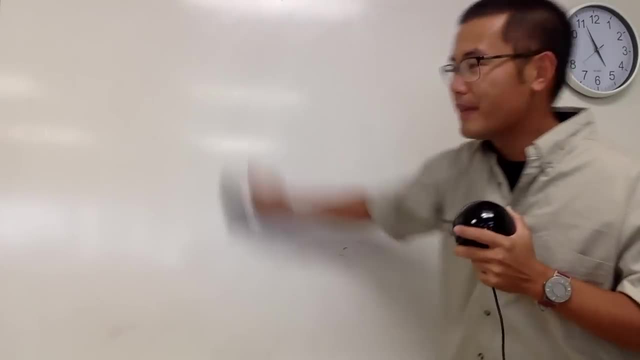 And be sure you guys go download the PDF, because I spent a lot of time to type out all the notes for you guys, So be sure you guys just utilize it And let me know if you guys are taking Cal 2 right now in this semester. 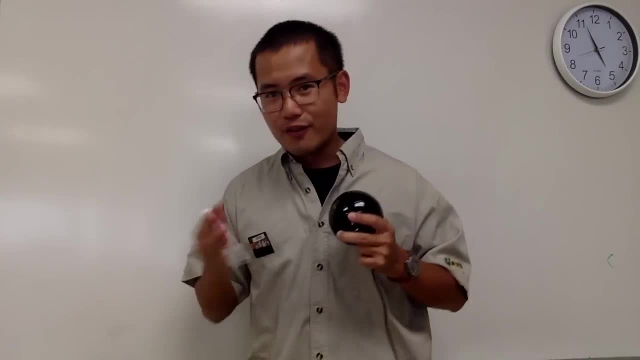 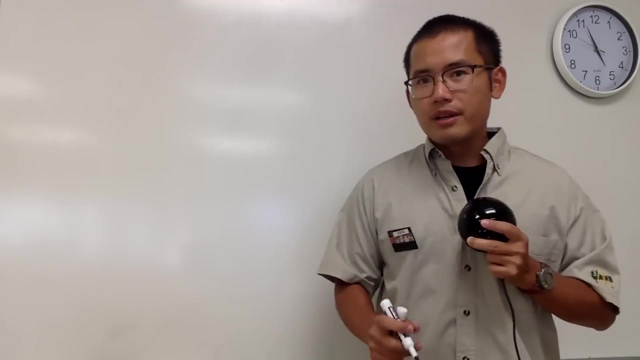 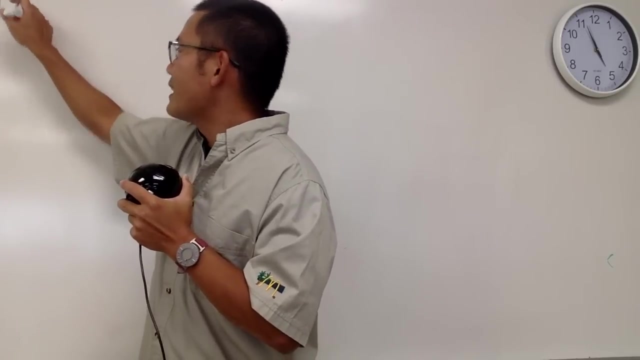 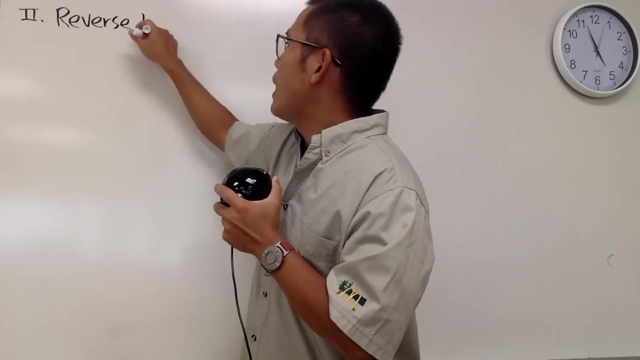 And hopefully the video right here will be really helpful for you guys. Okay, Now we're going to get serious. Now, perhaps this right here is actually the first technique and I will put it down right here for you guys. Well, for category number two, I will call this the reverse power rule. 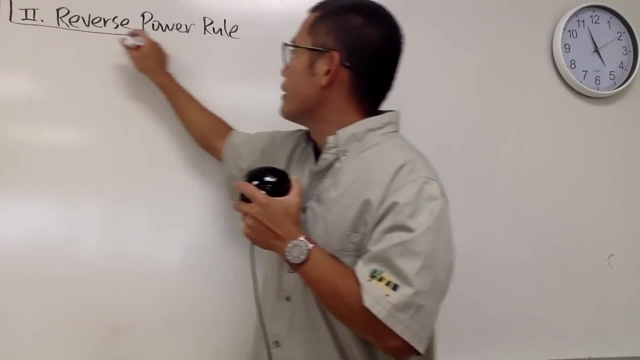 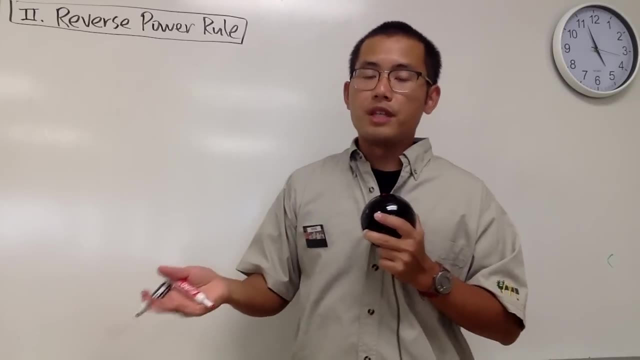 And let me tell you guys what I mean by the following right here. Well, remember, when we are doing integrals, we are trying to find the anti-derivative. That's pretty much the idea. And, of course, if we want to do the anti-derivative, we should talk about how to do the derivative first. 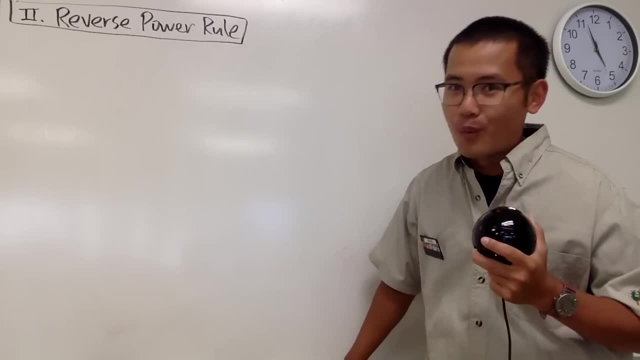 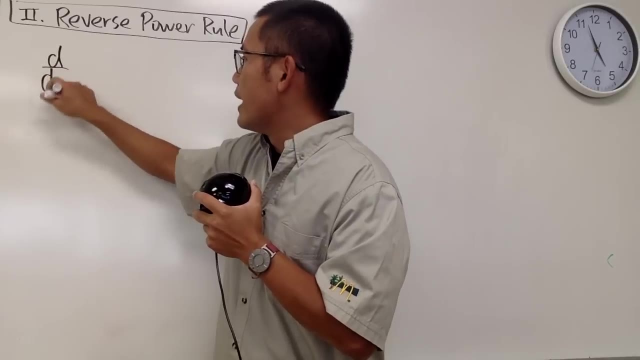 And of course, just like the Google days in Calc 1, we have the power rule to take the derivative. And let me just put this down right here for you guys: If we want to differentiate a function in the form of x to the nth power, like this: 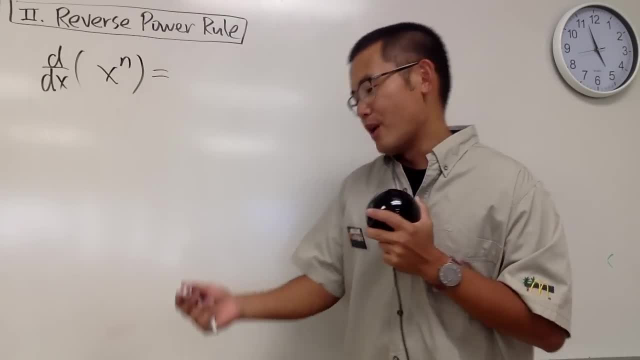 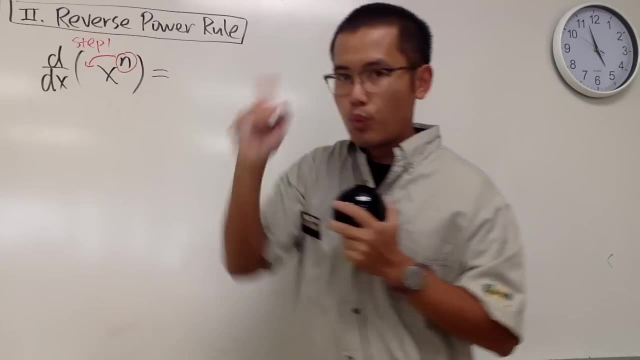 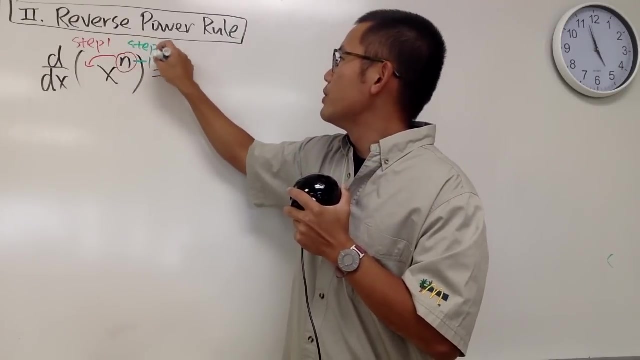 this is everybody's favorite derivative question, right? Well, because we can just go ahead, put the exponent in the front and notice this right? here is step one. And then we are going to subtract one from the exponent, and this is step two. 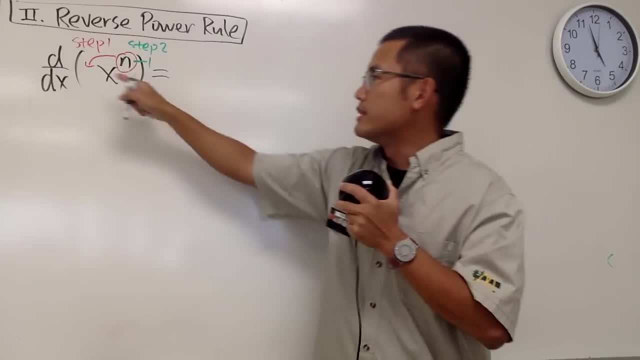 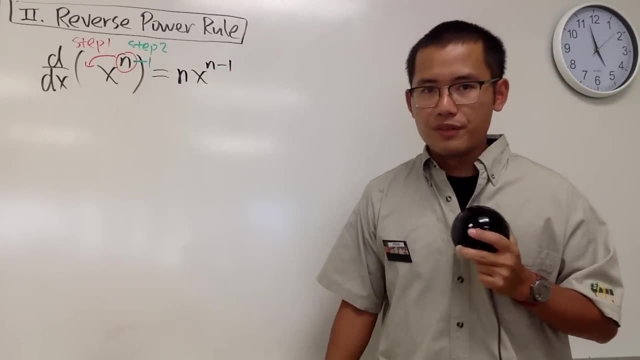 That's all, Step one, step two, And in the end we end up with n times x to the n minus one power, And this is the power rule when we are doing the derivative. Now for integral, we just have to do this backwards. and let me show you. 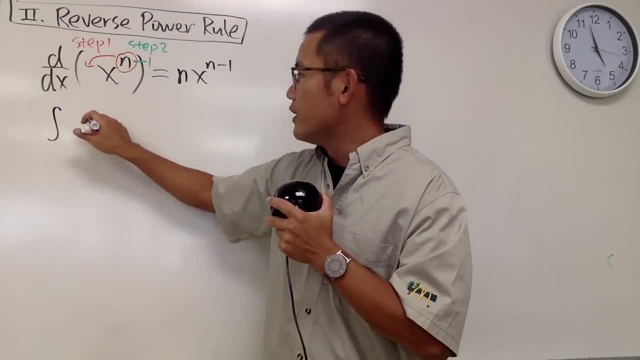 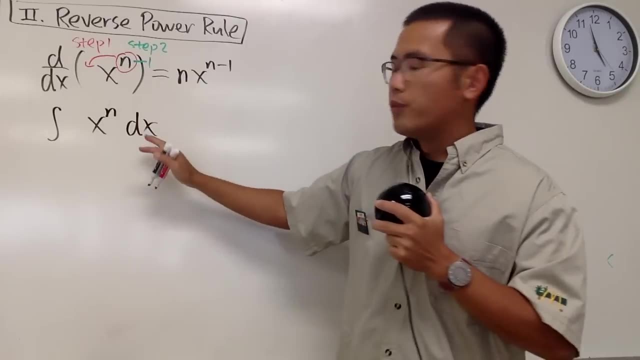 And the idea is that we will be integrating a function in the form of x. This right here has to be just x raised to the nth power. and don't forget, when you have the integral, always write down the d-whole-ever, like this: okay. 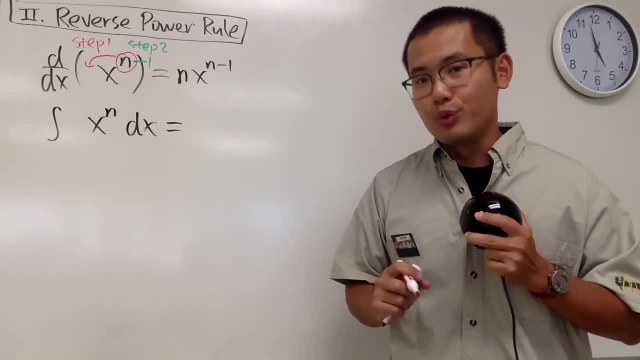 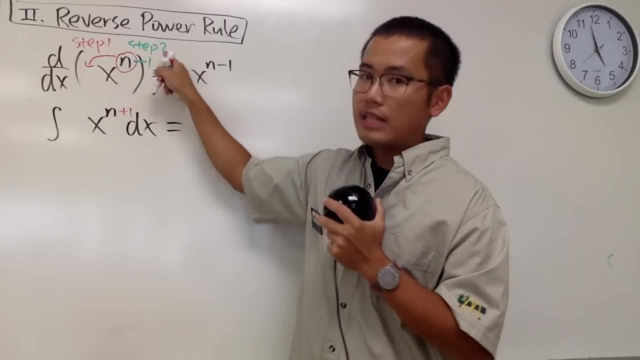 Now we are going to reverse the power rule, and this is how we do it. First of all, we are going to add one to the power because, you see, earlier we took away one from step two. Now we have to do the power first and we have to reverse the operation. 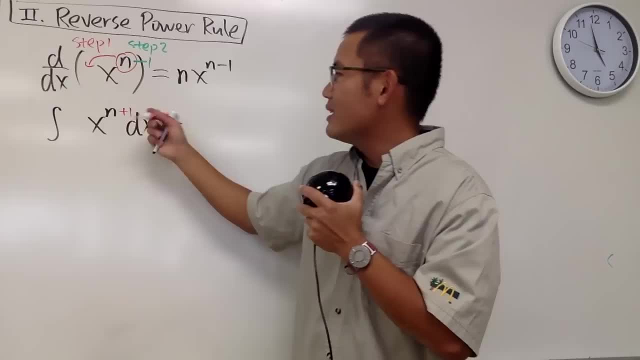 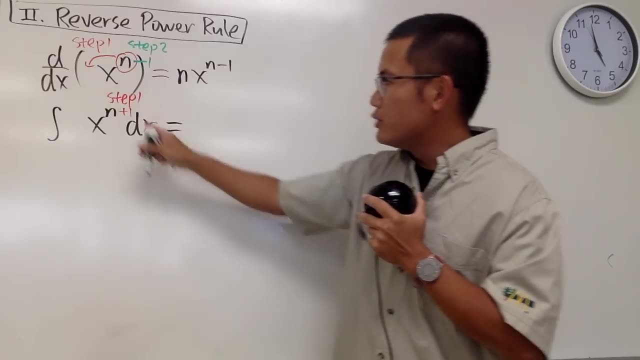 We subtracted one, now we have to add one to it And as you can see- let me just indicate this for you- This is step one. now we add one to the exponent and then we look at what this new power is divided by it, because earlier we multiplied it. 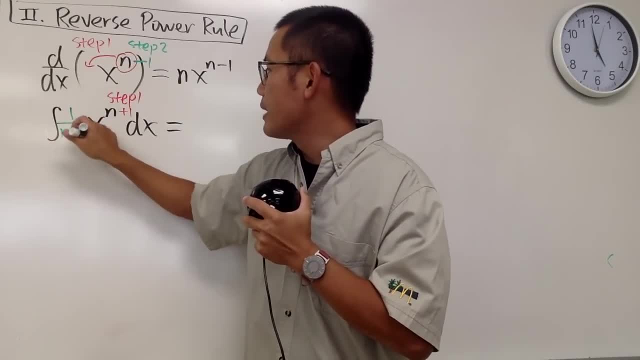 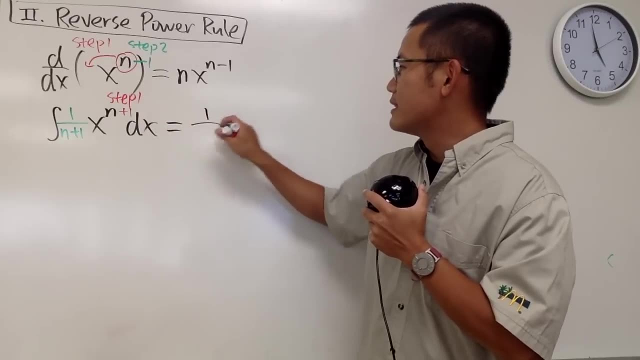 So we will just put down one over n plus one, just like how we divide the exponent, like this. That's pretty much the idea And I will just put this down for you guys: One over n plus one times x to the n plus one power. 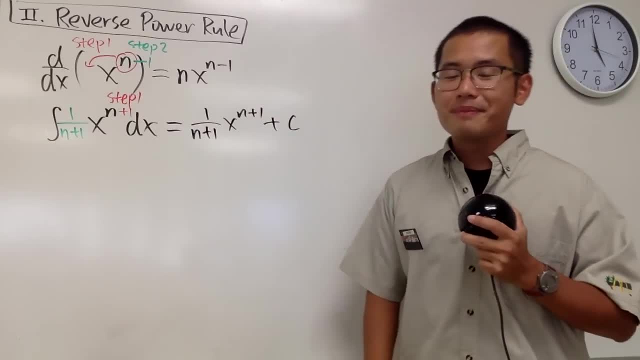 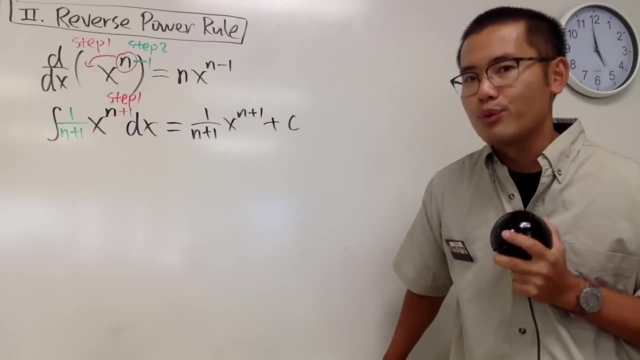 And, of course, you guys were late to tell me the plus c, okay. However, this formula is unfortunately not good for one particular n value. What is it? Well, hopefully you can all see that Right here we have the n plus one in the denominator. 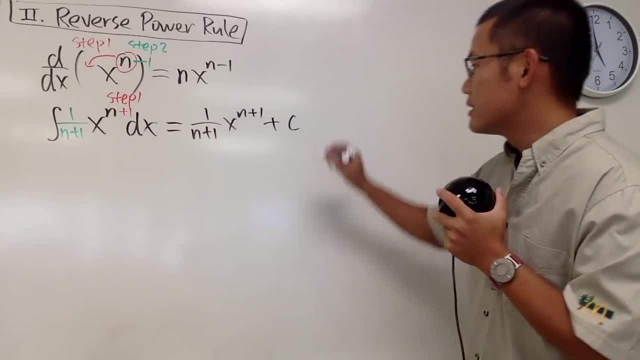 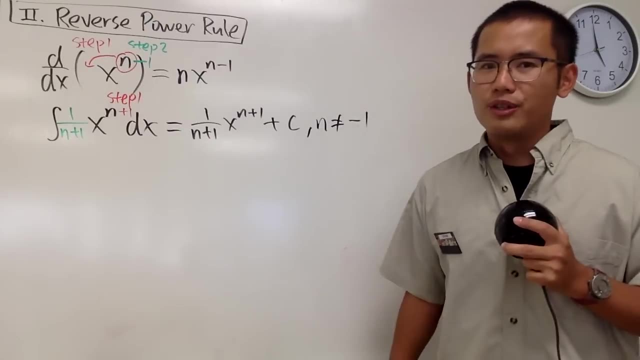 So, unfortunately, this is only good if n is not equal to negative one, because if n is negative one, we will be dividing by zero. That's no good. Well, what is it If n is equal to negative one? let's take a look. 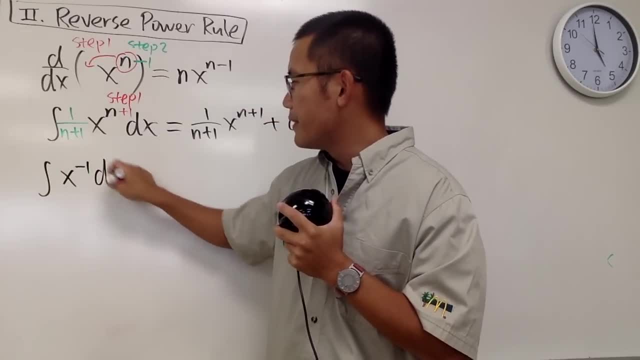 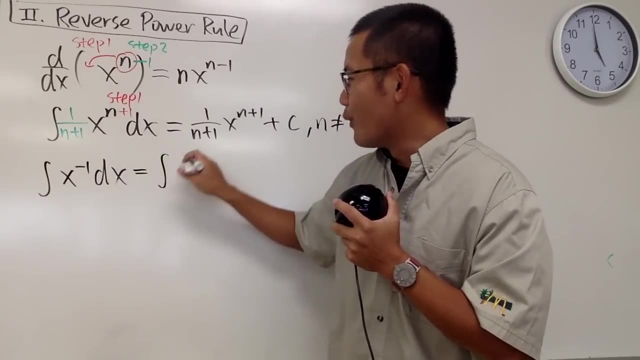 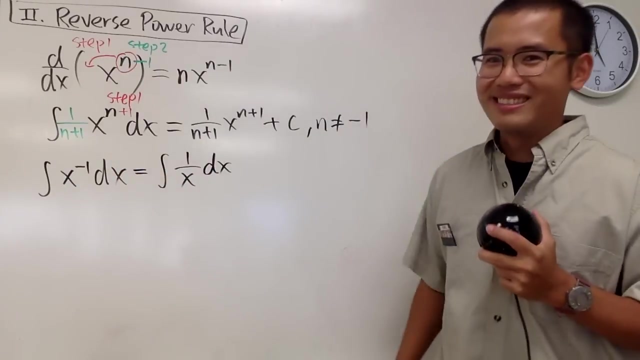 Here we have the integral x to the negative one, power dx. Of course, when we have the negative one notation, in this case, this does mean the integral of one over x. This does mean just the one over x. I know the negative one notation is perhaps the most disliked notation. 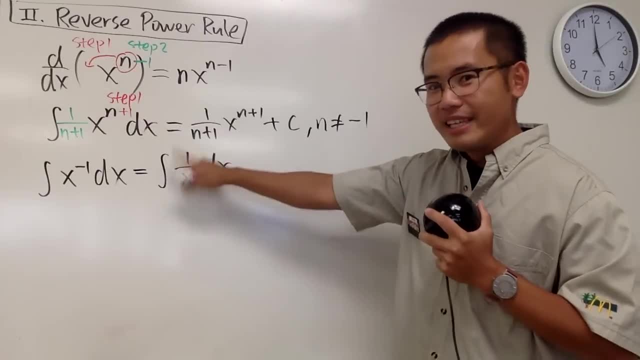 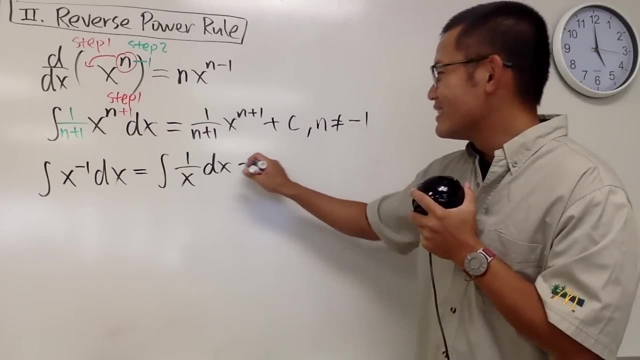 but again, we just have to deal with it. And now the integral one over x, based on what we talked about earlier. example number two: right Question number two: This right here is just the natural log of x. and don't forget, you attach the absolute value. 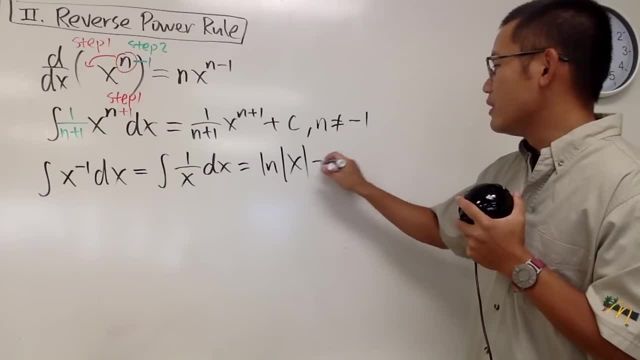 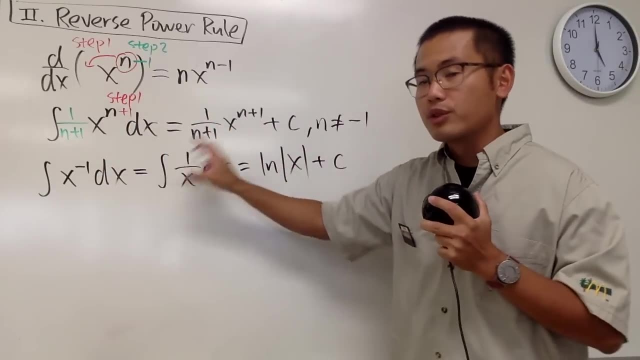 because again x could be negative. So this right here is the deal. So this right here is the complete version of the power rule. right? This is the reverse version. right, This is the original. This is the reverse version. 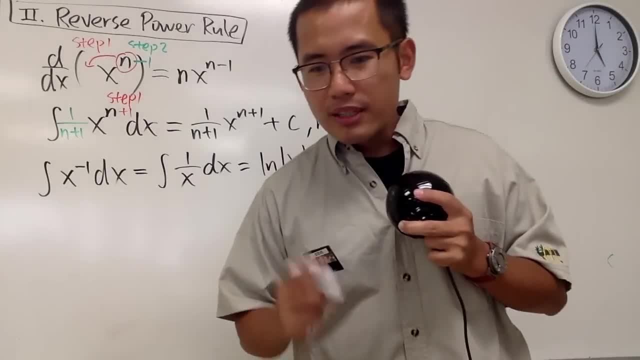 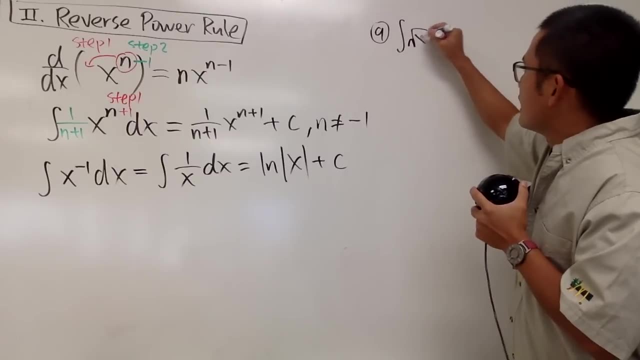 So this is, of course, what we will have to know. Now let me show you guys two examples on the reverse power, rule Number nine: right here. Here we have the integral of the square root of x times x plus four. 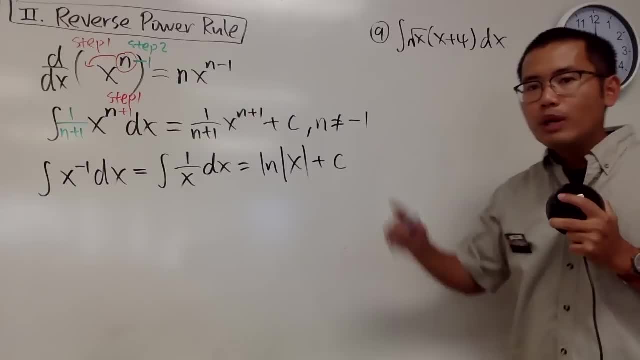 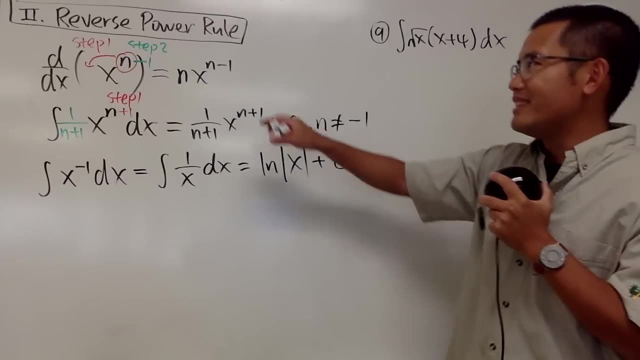 And again we have the dx right here. First thing first. whenever we have the square root in calculus, we almost always look at the square root as the one-half power, because we can either use the power rule or the reverse power rule for derivative or integral right. 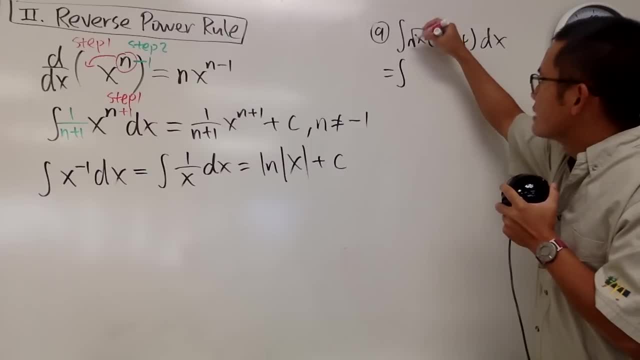 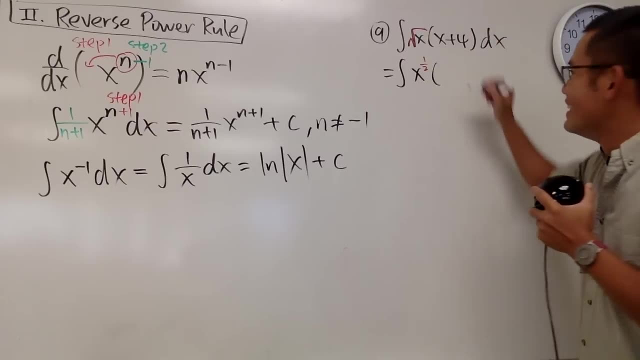 So, with that being said, let's look at this as the integral And the square root right here, which is just x to the one-half power, and we have the x plus four. So let me just put that down right here for you guys. 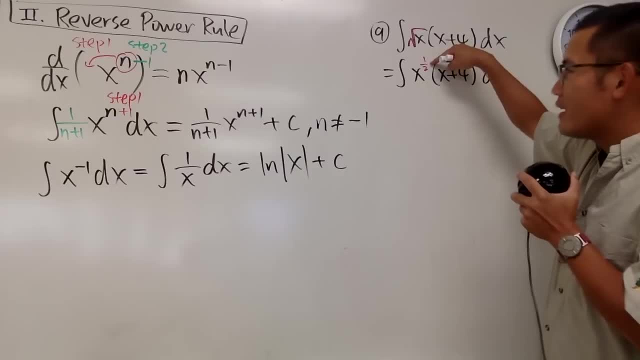 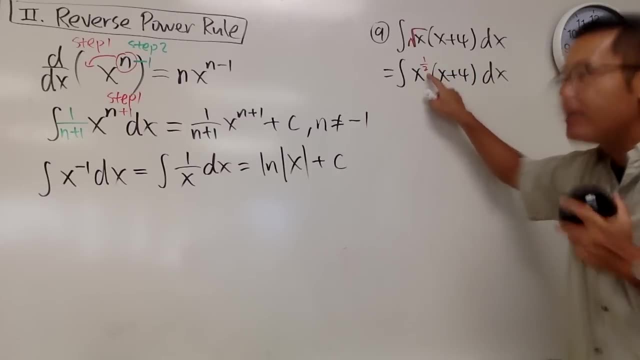 Now, unfortunately, we cannot just add one to the power here and then divide it by the new power yet, because this x to the one-half power is going to be affected by this x to the first power, because this and that are multiplying. 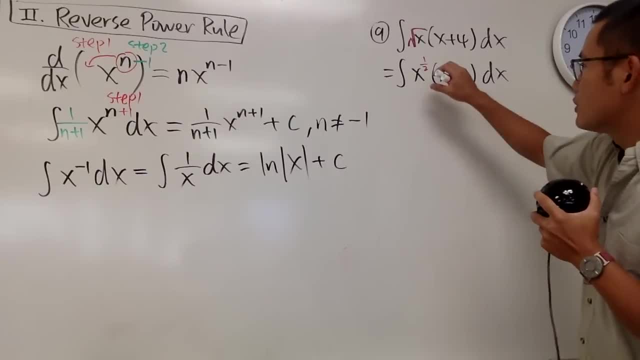 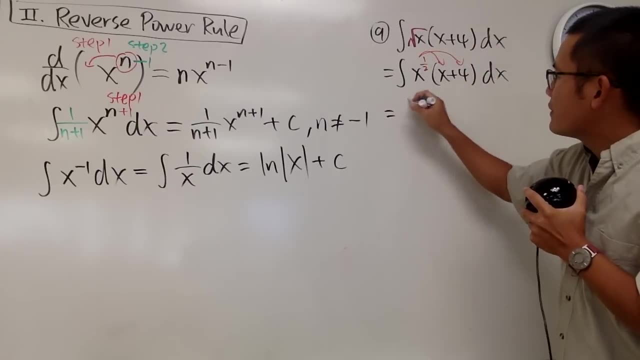 So we have to do the algebra first to make sure that we just have x to a power term right? Well, of course, let's go ahead and just distribute. Here we have the integral. This is x to the first power. 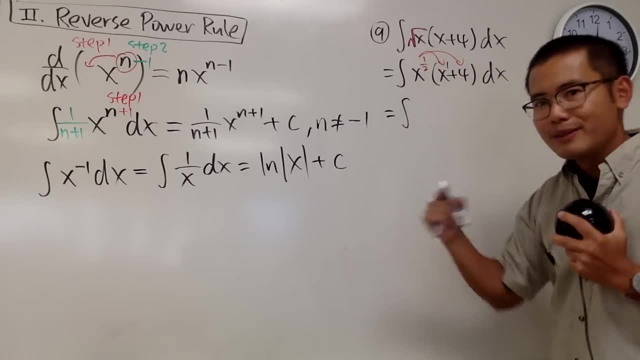 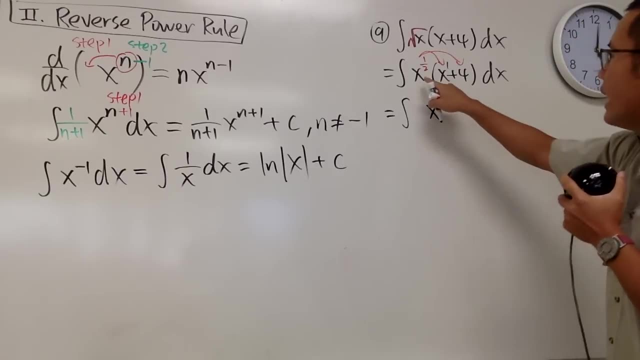 x to the one-half times, x to the first. We just add the exponent One-half plus one is just three-half, and that's the first term. x to the three-half power, And then we do this times that, and that's a plus in between. 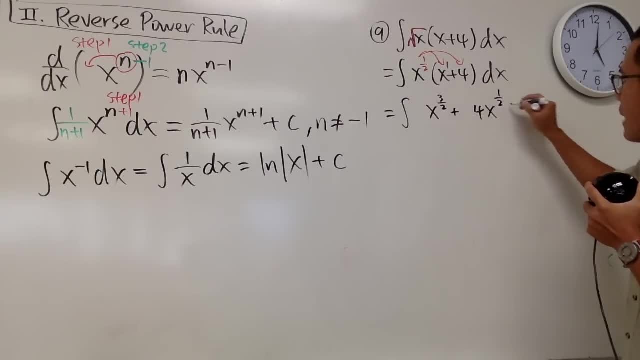 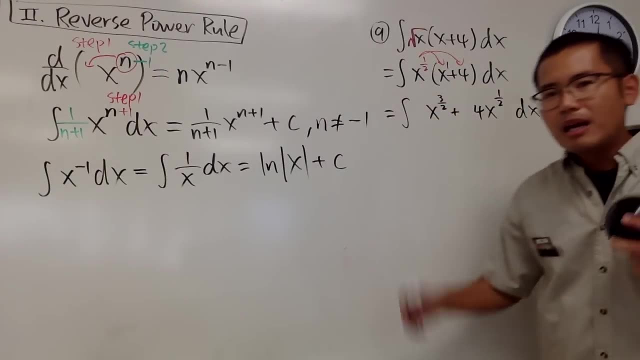 So we have plus four x to the one-half power. In the end we have that dx. And some people may want me to put a big parenthesis like this. In my opinion, as long as you read it clearly, I think it should be okay. 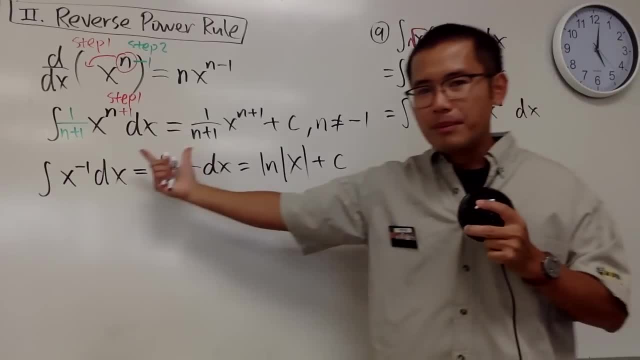 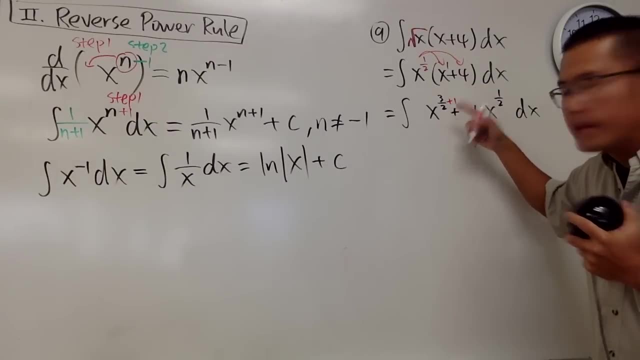 Now x to the three-half power. we can legitimately use the reverse power rule. Let's go ahead and add one to the power We have, three-half plus one, namely three-half plus two over two, which is going to give us five over two. 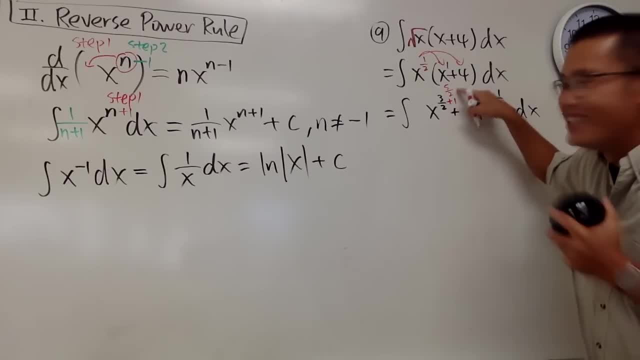 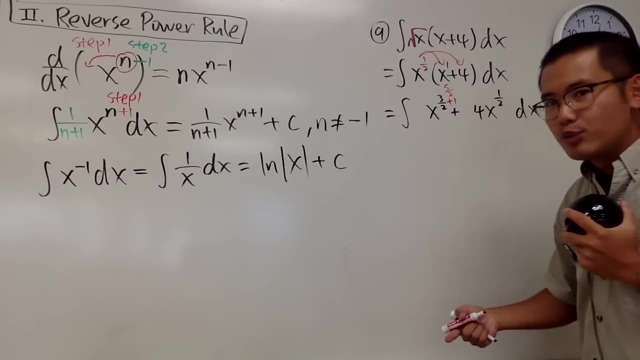 And then- by the way, this is how I recommend you guys to show work- Just put a new exponent right here, And then we have to divide it by the new power. Divided by the fraction is the same as multiply by its reciprocal. 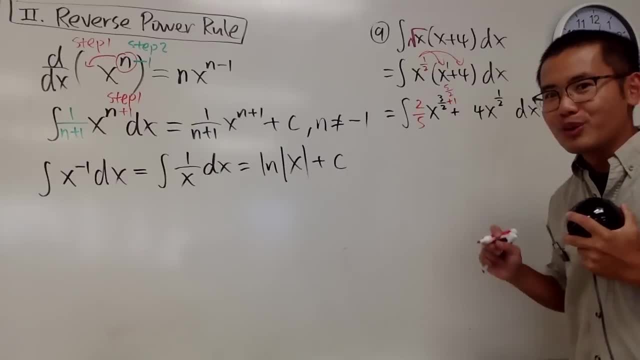 So we multiply by two over five right here. So that's how you can show work. Don't worry, we'll do another example right here. right now, Add one to the power. One-half plus one is three-half divided by the new power. 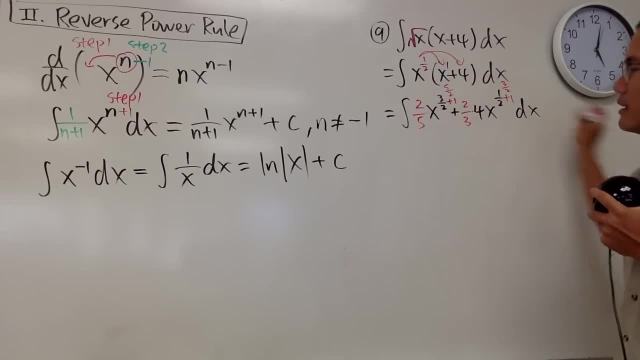 So I just put down two over three like this And keep in mind these are multiplying This and that, this and that, And then we are just adding them up And whenever we have an integral of a sum or a difference, if it's adding or subtracting- 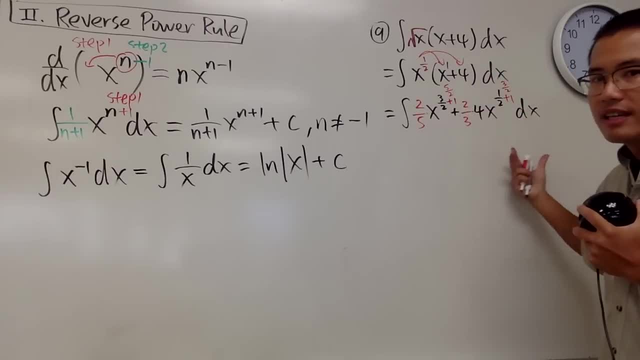 just do the integral of the first and then you add or subtract the integral of the second and then put the answers together. That's the idea, Anyway. here we have two over five And we can write it as x to the five over two power. 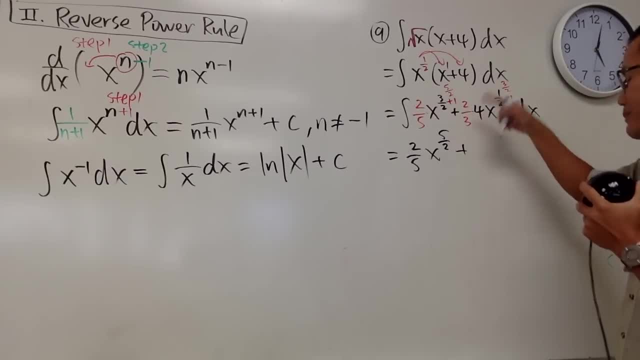 And then we add two-third times eight. That's the answer. Two-third times four is eight over three, And then x to the three over two power. In the end we're done. So just put a plus c. 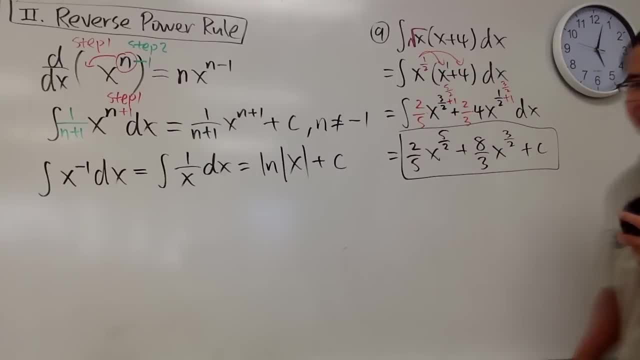 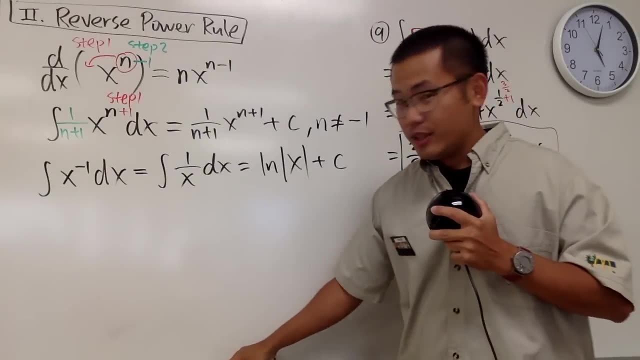 This is it all right. So this is perhaps the first technique that I will really say that's a technique. The first one is: just know your derivatives really, really well. Let's do another example. Here we have number 10.. 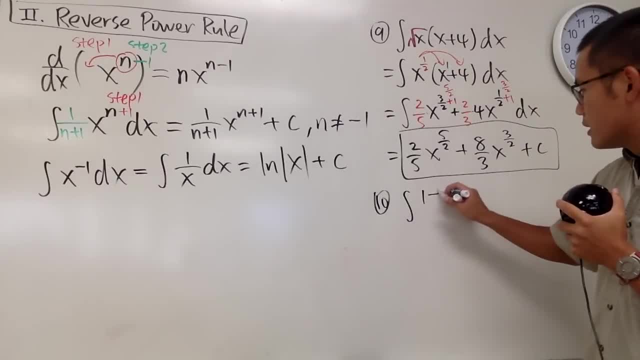 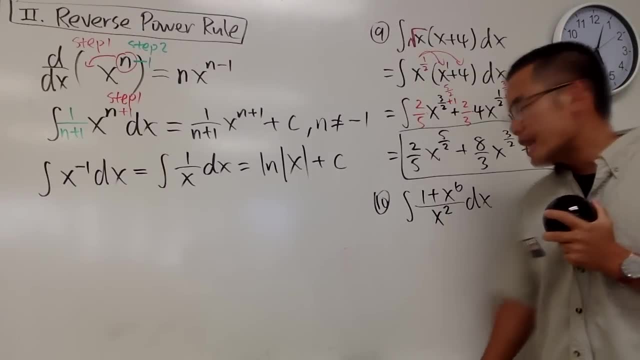 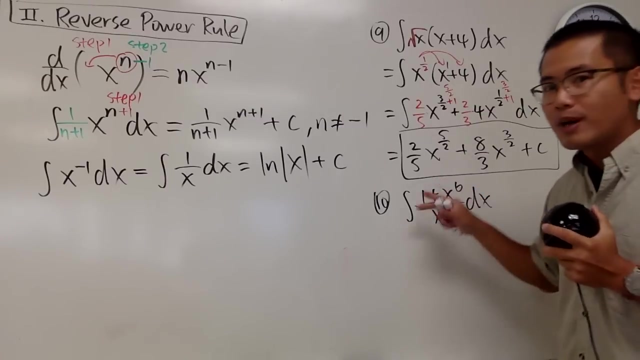 Let's look at the integral And we have one plus x to the six power over x squared dx like this. Well, notice that again, we cannot just add one to the power, add one to the power. We cannot do that yet because we have to do the algebra. 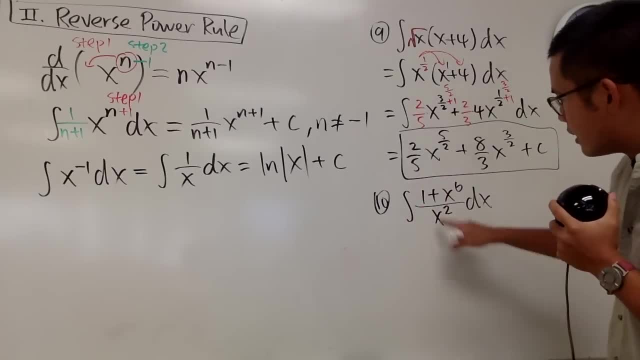 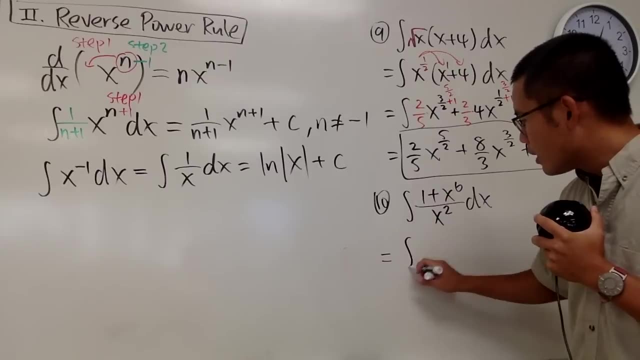 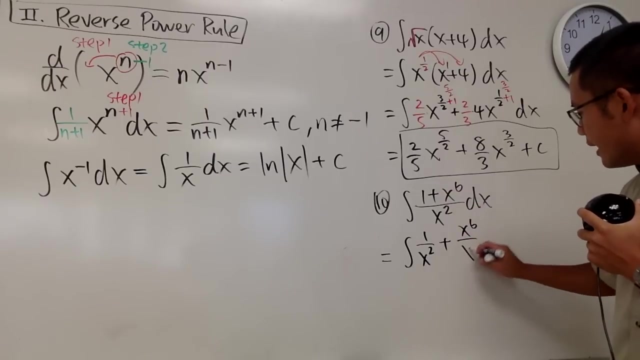 to make sure that no power is affecting each other. In this case, notice- we just have x squared on the bottom, So we can just split the fraction And we get the integral of one over x squared. And then we add x to the six power over x squared, like this: 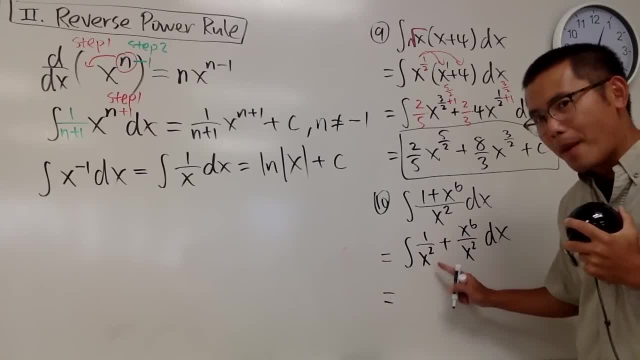 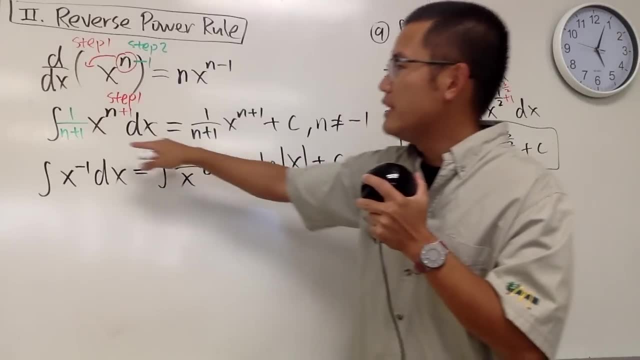 Now again, we have one over x squared, But we actually have to look at this as x to the negative two power, because in order for us to use this, it has to be x to some number for the power right here. So we look at this as the integral. 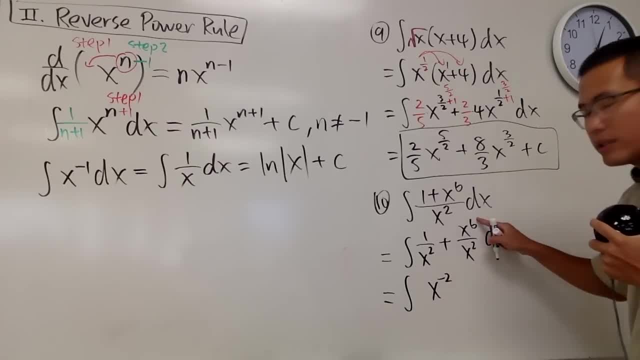 And this is x to the negative two. And of course, for this part we can just simplify by subtracting the powers. So we add this minus that We get x to the fourth power and of course dx. And now reverse power rule. 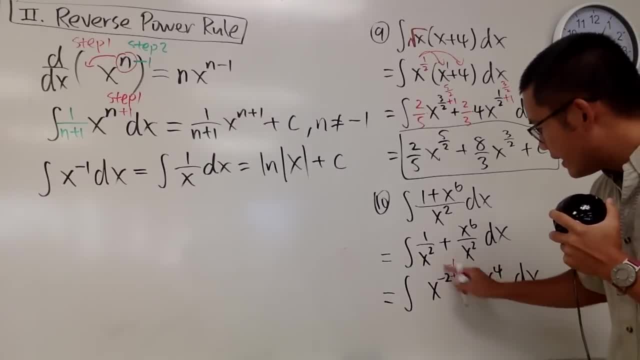 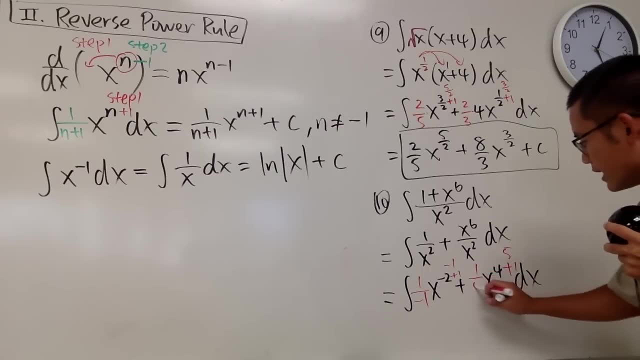 Add one to the power. Negative two plus one is negative one Divided by the new power. So I have one over negative one And for the second part we add one, which is going to be five And divided by that. 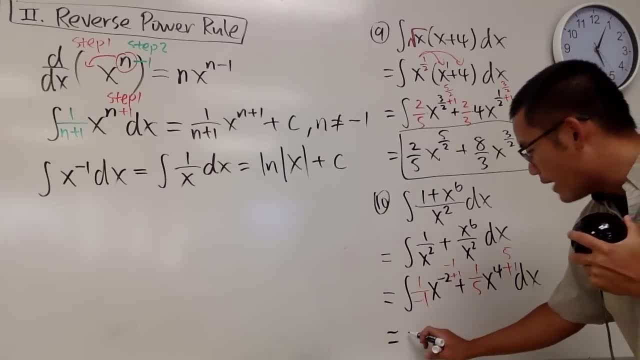 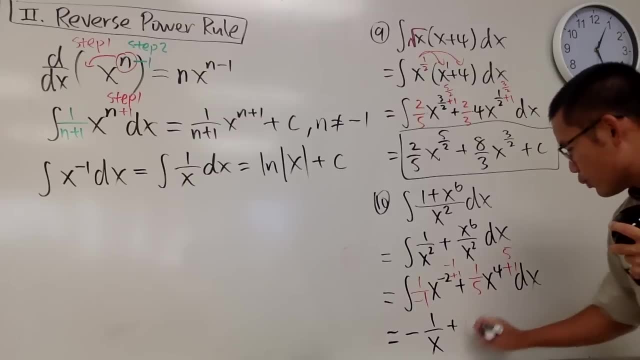 In the end we have one over negative one, That's negative x to the negative one. power is one over x, And then this is plus one over five And we have x to the fifth power And in the end we are done. 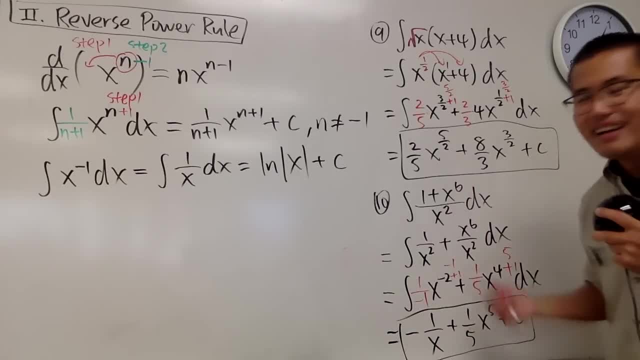 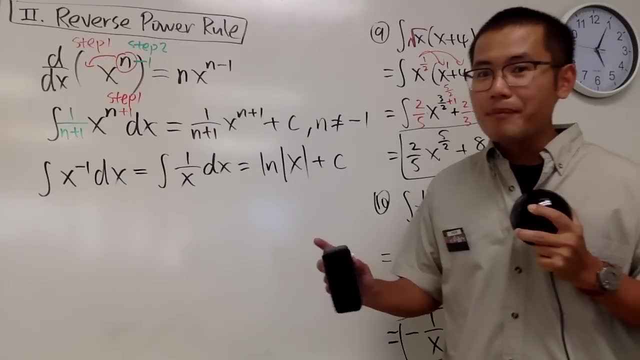 So put a plus c like this, And that's it. Okay, So I have these two examples for you guys for the reverse power rule, And don't worry, because later on you will see, we actually have to go back to first category or second category. 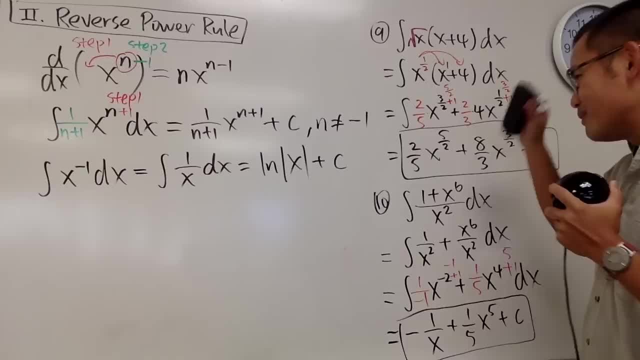 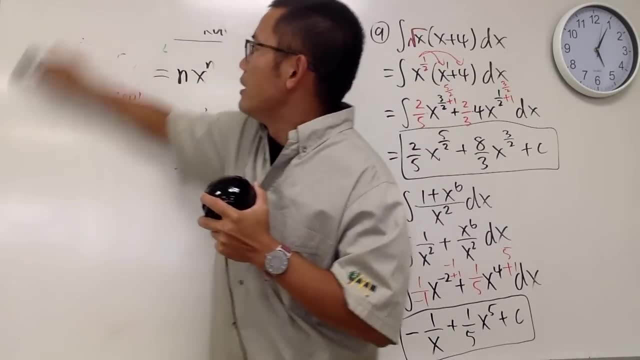 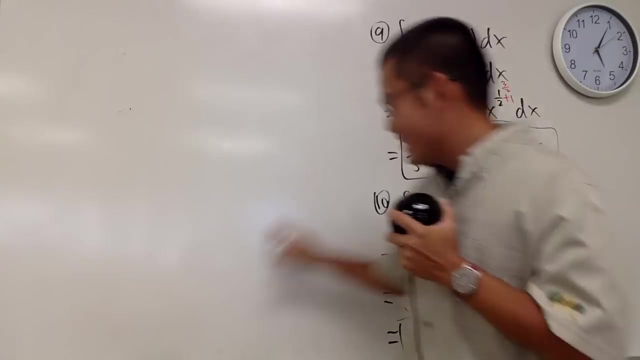 and third category, et cetera, to do the harder ones. So let me just demonstrate two examples for the reverse power rule for you guys. Now here is another technique that you guys might have learned back in Calc 1.. You definitely should have done this in Calc 1.. 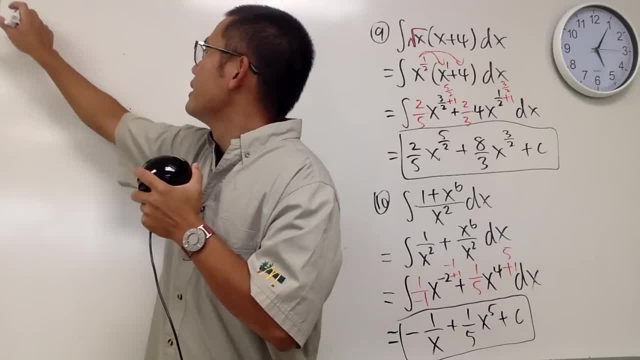 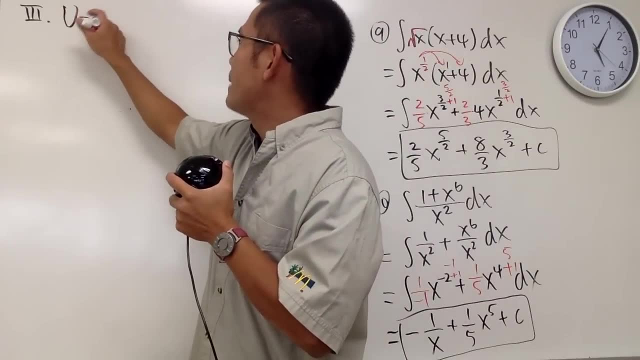 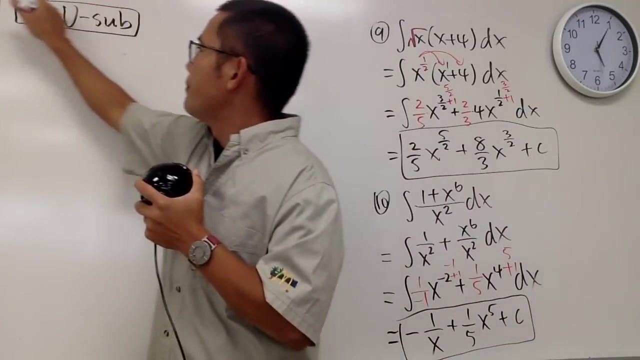 Now let's look at category number three, And for this one, this is the famous one, Of course: u-substitution. So of course, let me just put it as u-sub And let's talk about what u-sub is first. 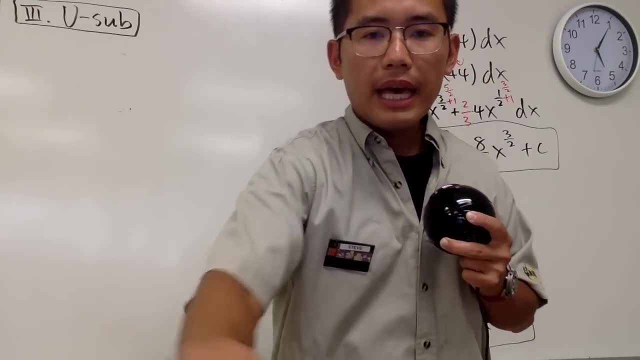 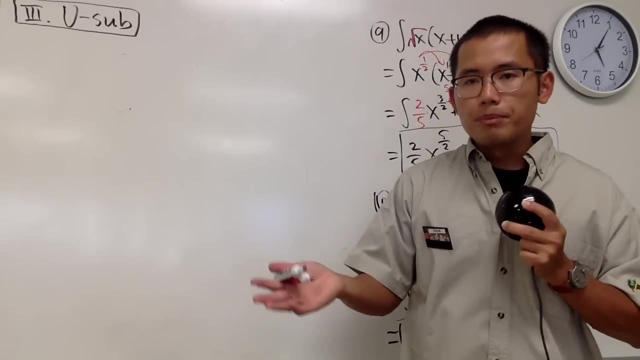 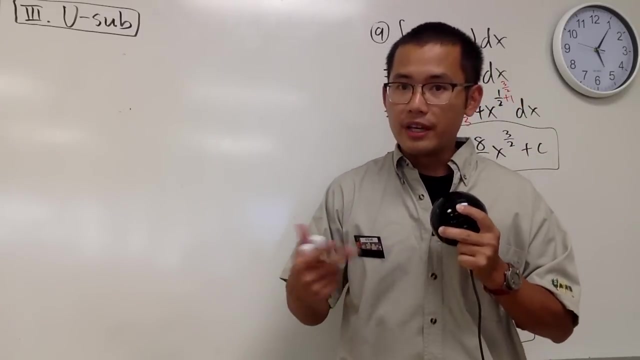 Remember earlier, we have the reverse power rule And we have to think about: okay, that's just reverse power rule, Because we have the original power rule to do the derivative. Now think about what other techniques do we have for taking the derivatives? 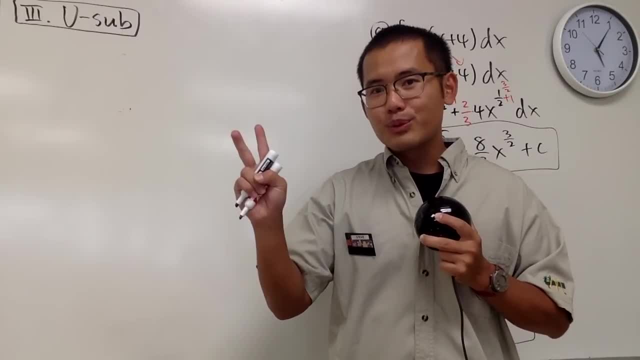 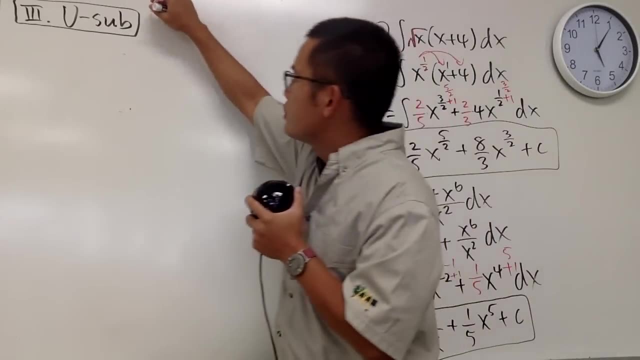 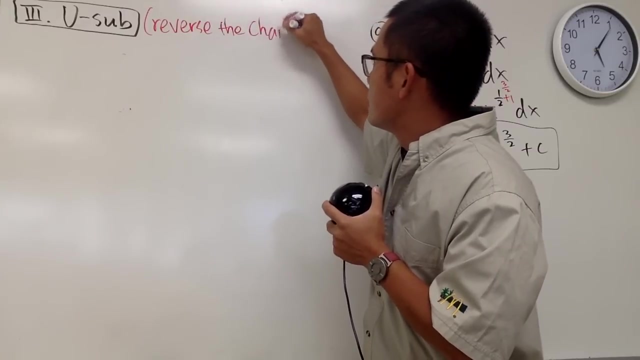 We have the power rule, We have the product rule, quotient rule and also the chain rule, right. The purpose of the u-sub right here is- you can just think about it as that we are going to reverse the chain rule And that's going to work out really nicely. 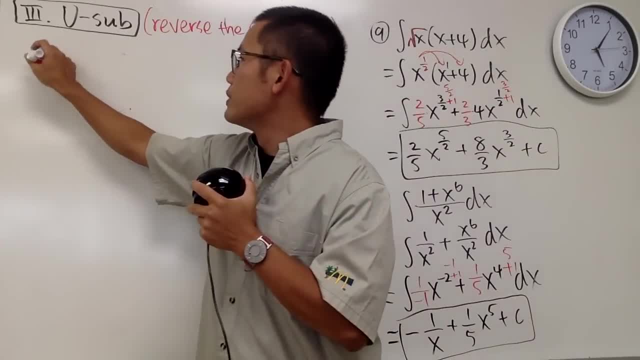 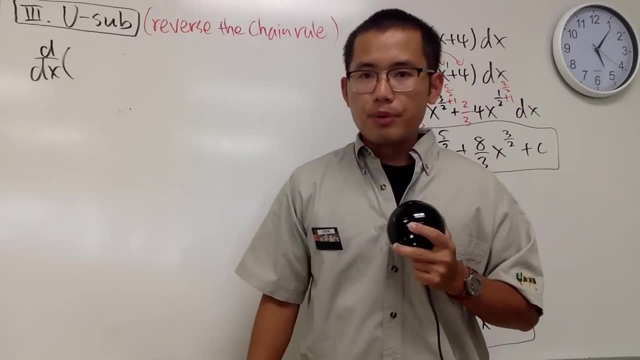 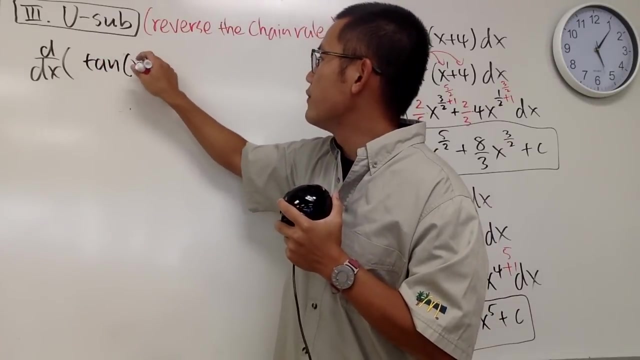 And let me show you First of all, again, we are going to see how to do the derivative first, And I'll formulate this nicely for you guys. Let me give you guys an example here, though Let me just give you guys: okay, let's say, we have to differentiate tangent of x to the worst power. 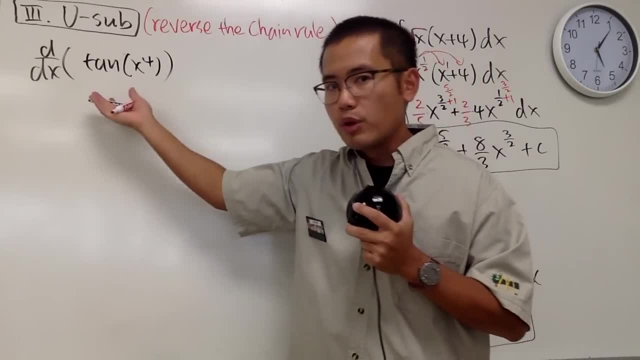 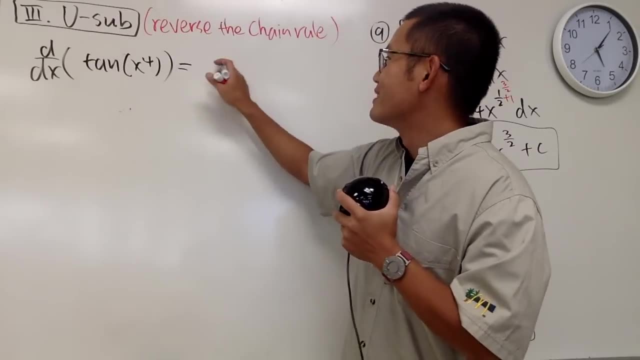 Like this. Well, to do the derivative right here. what we do is we ask ourselves: the derivative tangent is what? Namely secant squared? So we have secant squared And the input is x to the fourth power. 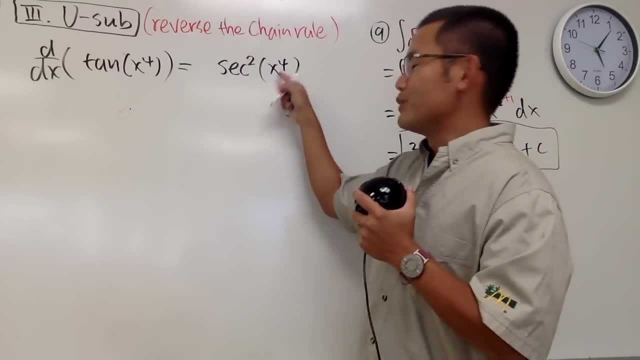 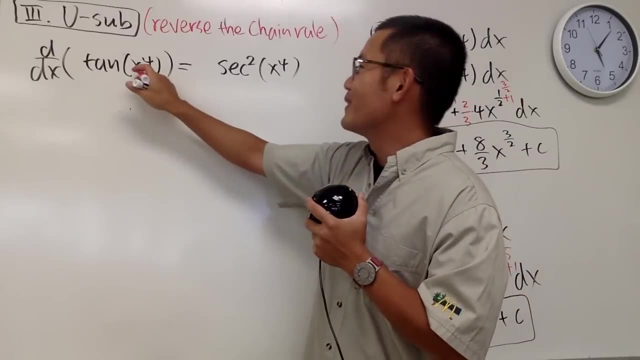 We just keep it as how it is for now. And then we actually just keep it as how it is for now. forever. Inside doesn't change. And then we are going to look at the inside and multiply by the derivative of the inside. 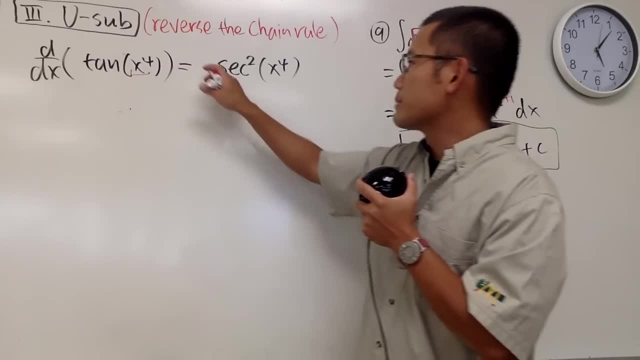 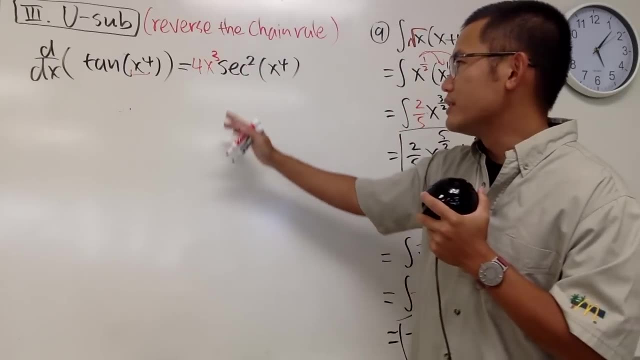 And that's because of the chain rule, And the derivative of x to the fourth power is 4x to the third power. So let me just put that down right here And, as you can see, this is how we take the derivative. 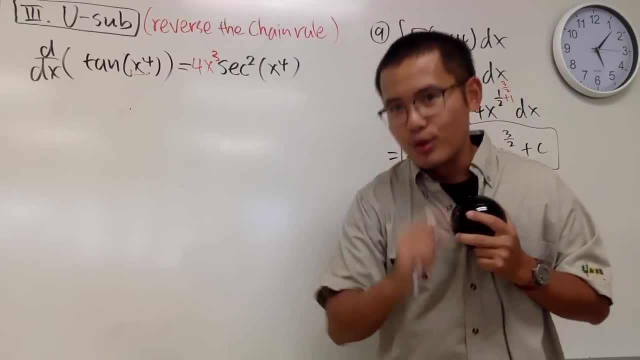 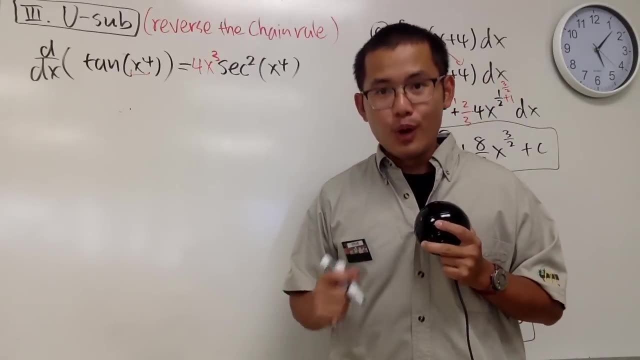 And now let me ask you: do I need to put down a plus here, right here? No, we don't. This is just the derivative. alright, Okay, When we know this derivative, in fact, we can know an integral right away. 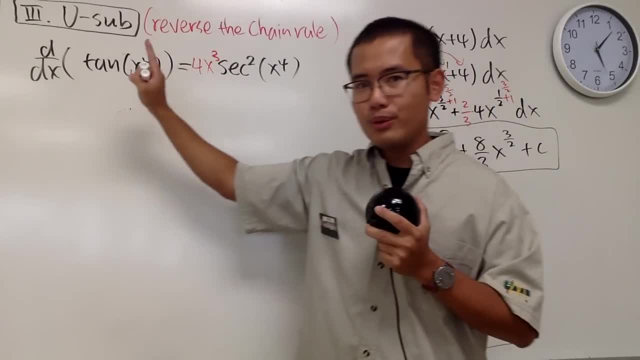 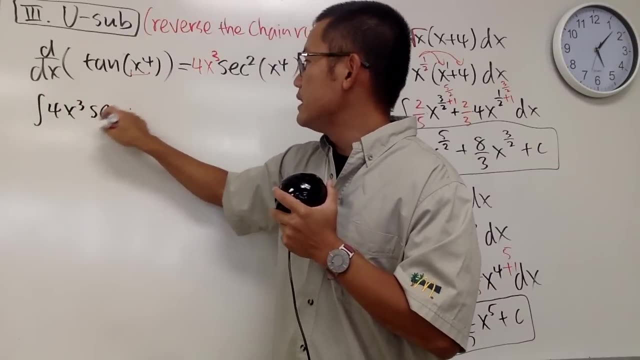 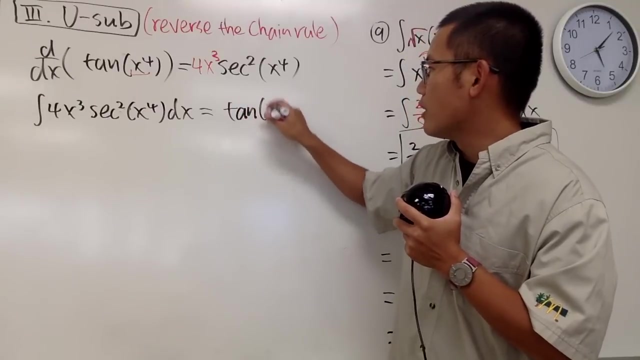 Namely, the integral of this is equal to that. So let me just write it down. If we have the integral of 4x to the third power and square of x to the fourth power, dx, well, it's just going to be tangent of x to the fourth power. 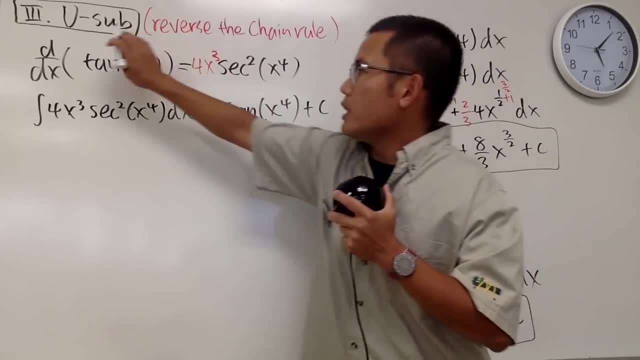 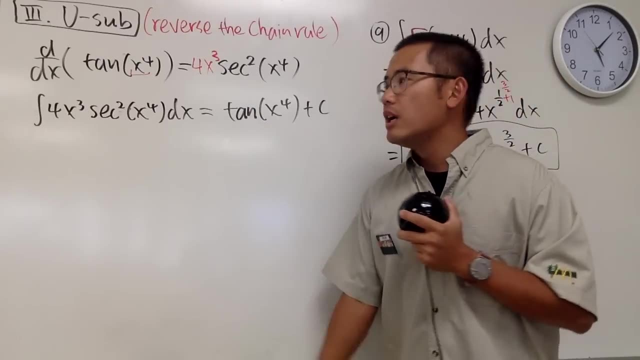 and in this case put down a plus c. So this is the chain rule. and then we can of course go backwards when we are doing the inside derivative. But now the question is, what if we didn't do this in the first place? 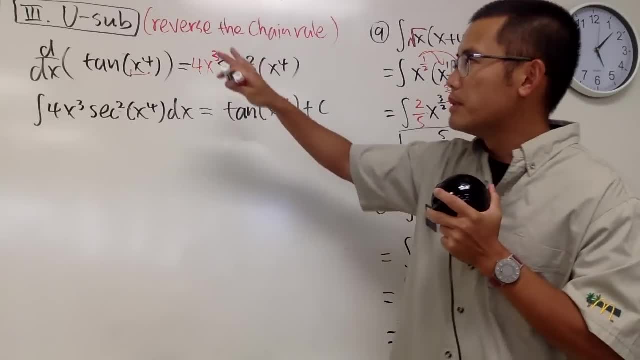 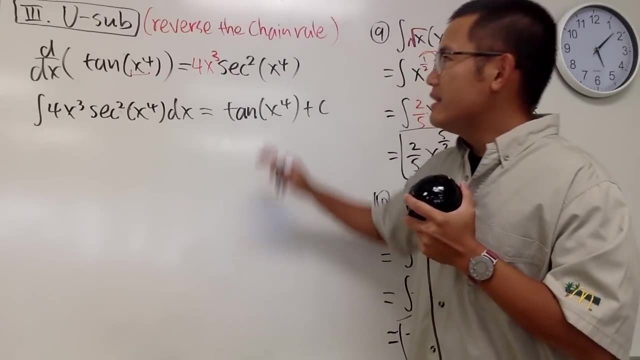 Well, this is how we are going to carry out the u-substitution: to help us clean up the, the usual things like this to undo the chain rule. You will see, And this is not the only purpose- You guys will see the following later on, right. 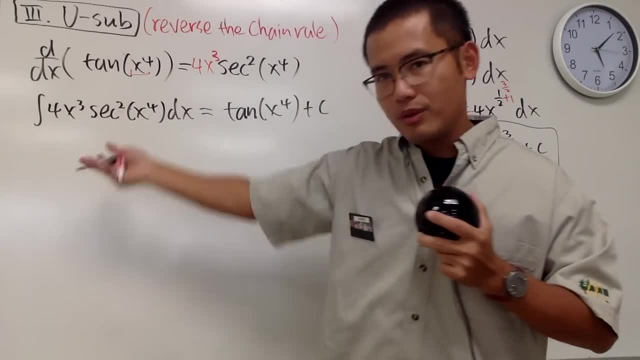 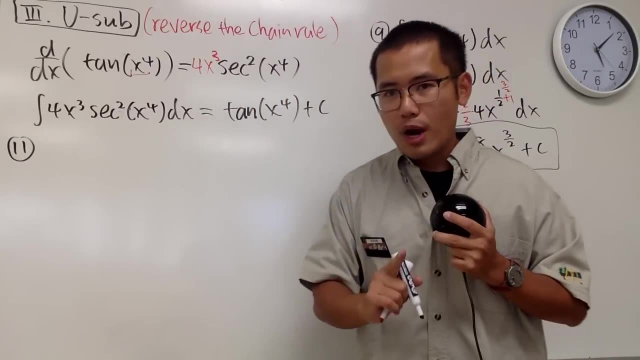 But let me just demonstrate how we clean up the chain rule and do the reverse chain rule. first, Namely, we have the number 11.. Let me just do this one for you guys from scratch, meaning that I'm not going to just relate on this part, right. 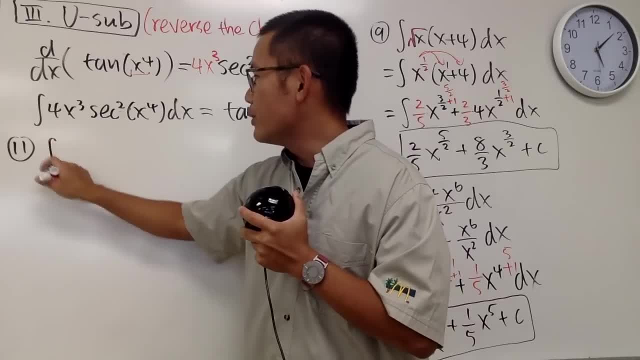 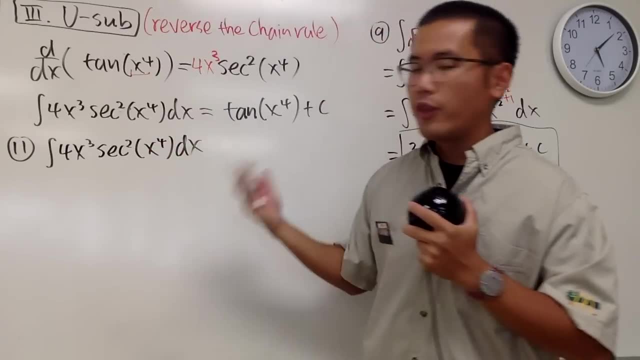 I don't know the answer. Anyway, let me just show you guys how to integrate 4x to the third power times secant squared of x to the fourth power, dx from scratch. Now here is the deal: Recall the chain rule. 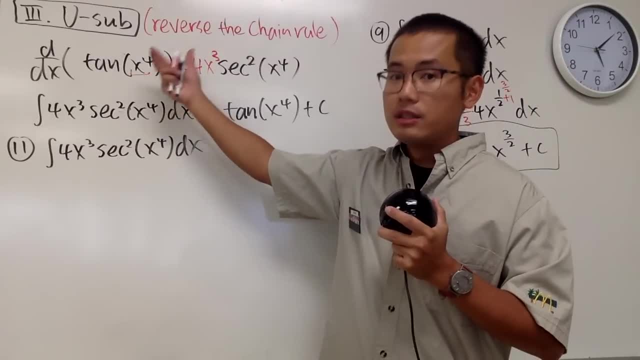 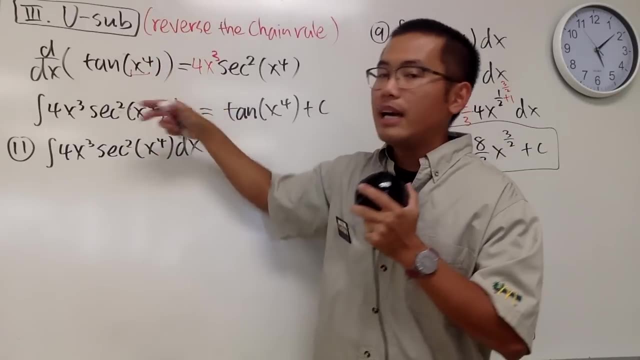 We usually just look at the inside and just ask ourselves derivative of what will give us. Sorry, We just look at the inside and ask ourselves what's the derivative inside and we multiply it right And when we are doing the u-sub, we just go ahead and look at the inside. 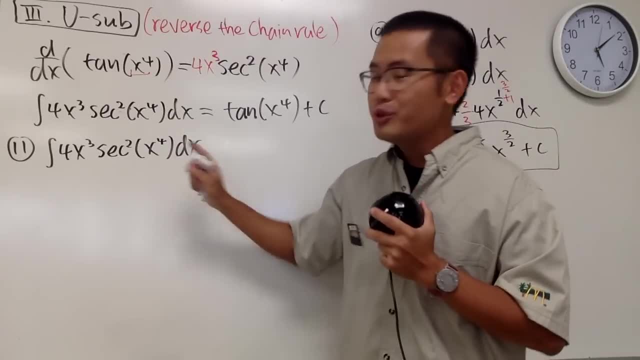 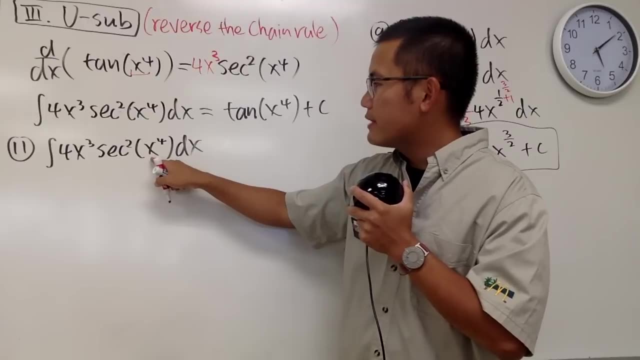 Usually- this is what I mean by usually okay. Usually this works out pretty nicely In this case. this is how we are going to do it. Notice we have x to the fourth power as the input function right here. Let's just go ahead and try it. 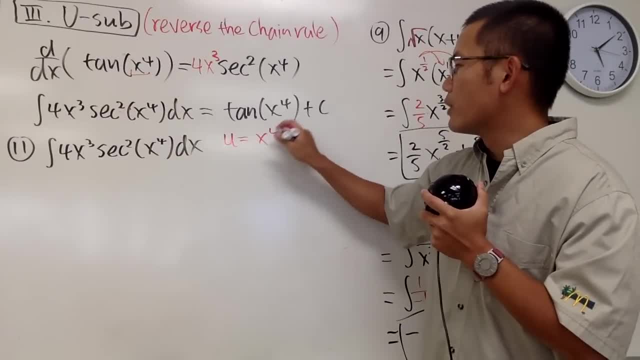 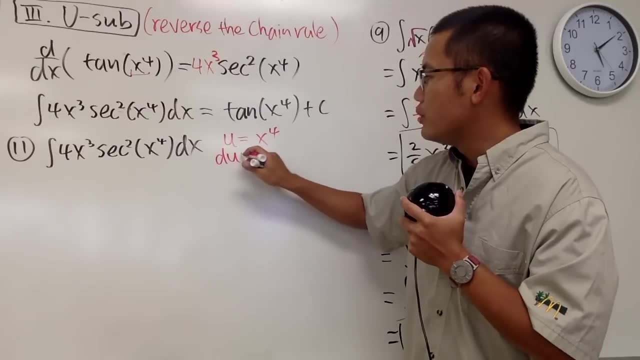 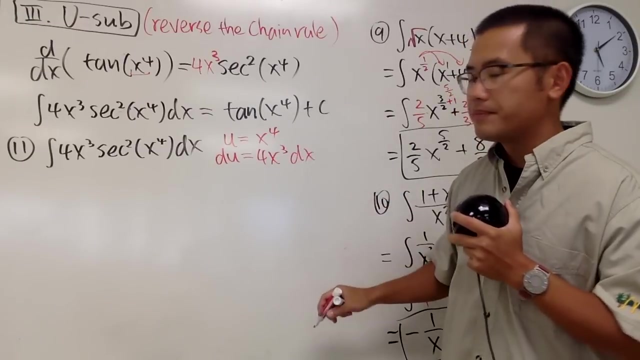 Let u equals 2x to the fourth power and let's just write it down. And then here is the usual deal. We have to differentiate both sides, so we have du equals. The derivative of this is 4x to the third power, dx. 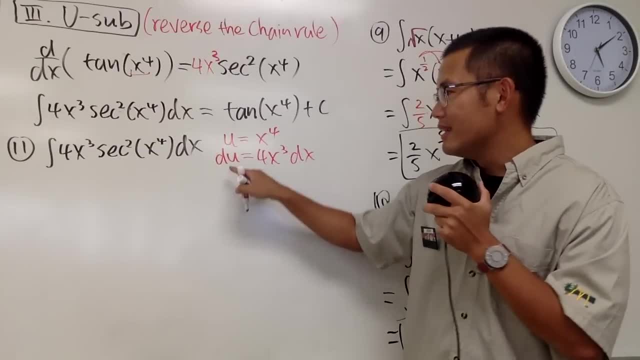 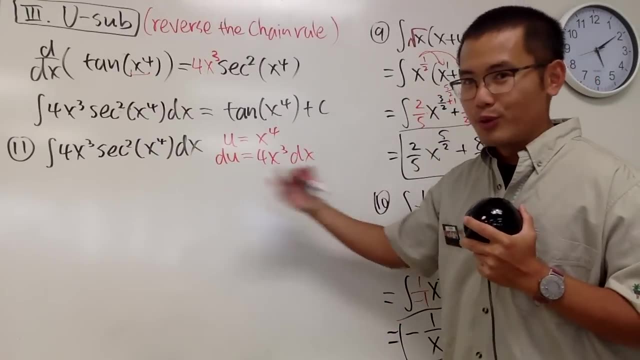 Notice, usually we put down du, dx, but you see we have, du is equal to this times dx, and this is what we call the differential. And just do it like this for you who are doing the u-sub right here: okay, And the next step is let's isolate the dx. 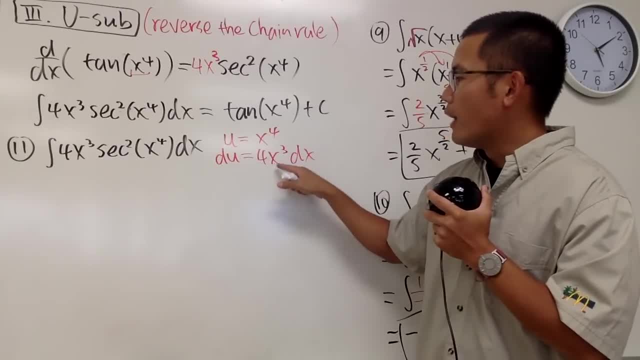 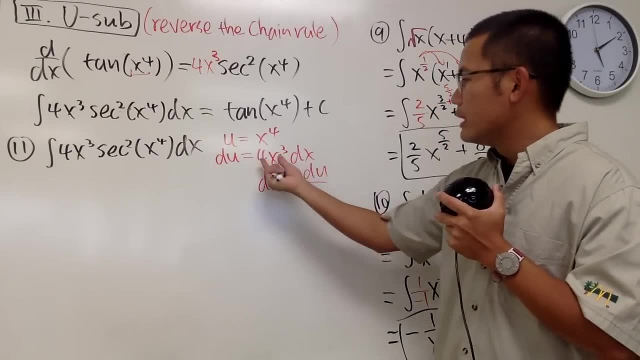 and we can do so by dividing both sides by 4x to the third power and you see, we will just get dx being equal to du over this. So we have the 4x to the third power like this. And now here is the story time. 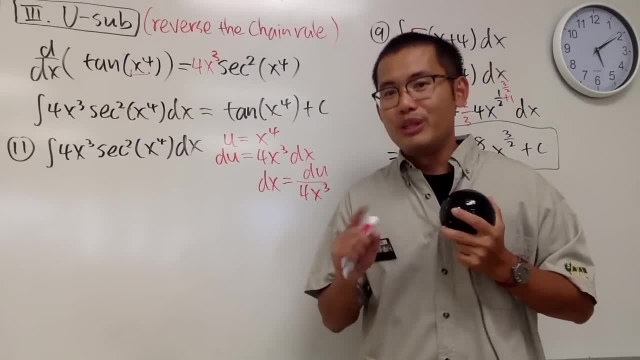 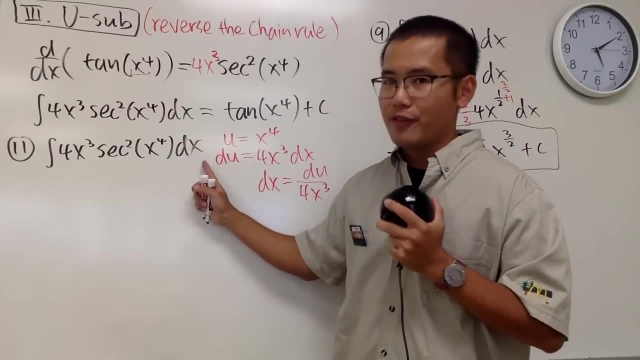 Remember my story. Usually it will be really, really helpful. Here is the idea: You have this integral and when you are doing integrals, always pay attention to d, whatever. In this case, we have dx and I call this the x-world. 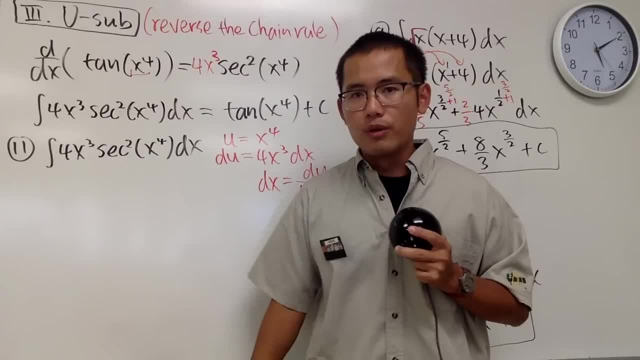 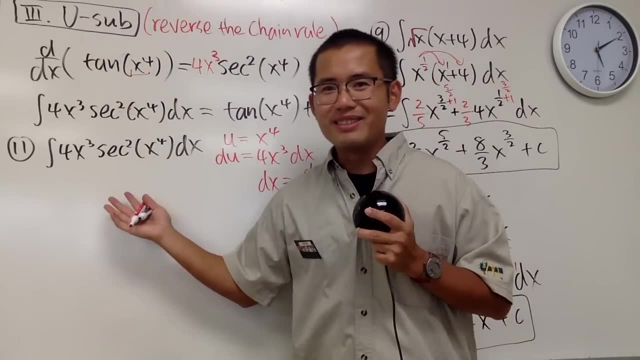 because we have the dx. This integral is in the x-world, But unfortunately, if you just look at this without knowing that, we wouldn't know what the answer to this is right. Well, here is the idea: We will take this integral from the x-world to the u-world. 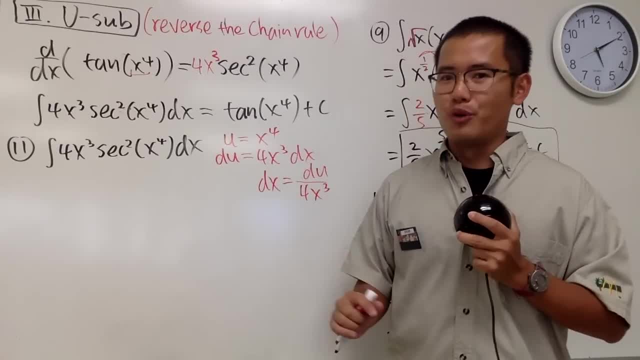 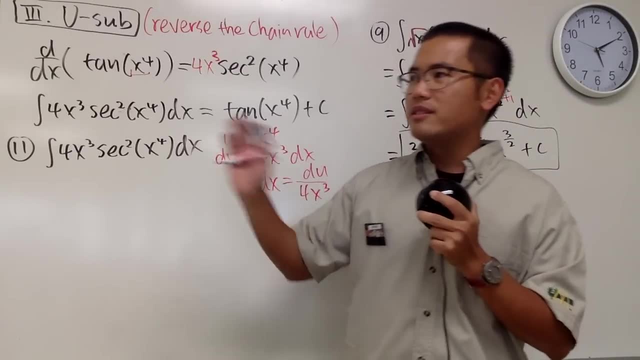 and once we get to the u-world, you will see it's much better over there, right? And let me just tell you guys, this summer vacation I didn't go anywhere. I didn't go to Disneyland, I didn't go to Disney World. 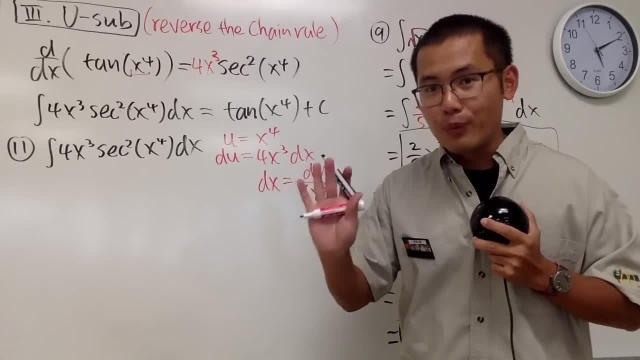 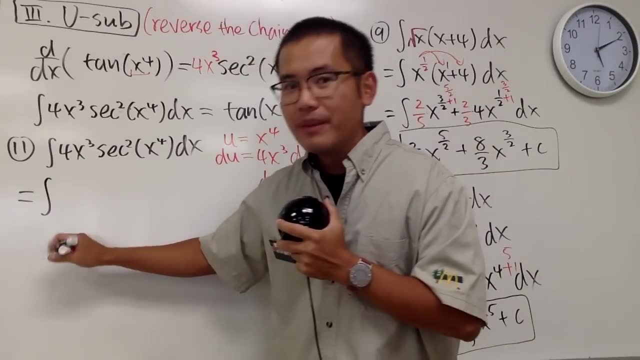 No, I went to the u-world for five weeks and it was a lot more fun. Anyway, here we go. We have this integral and let's just put down the 4x to the third power, and then, of course, here is the function secant squared. 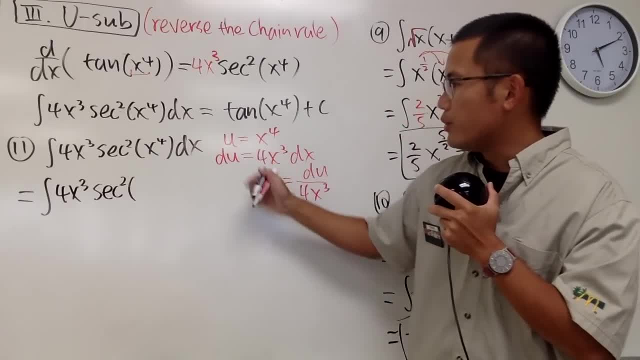 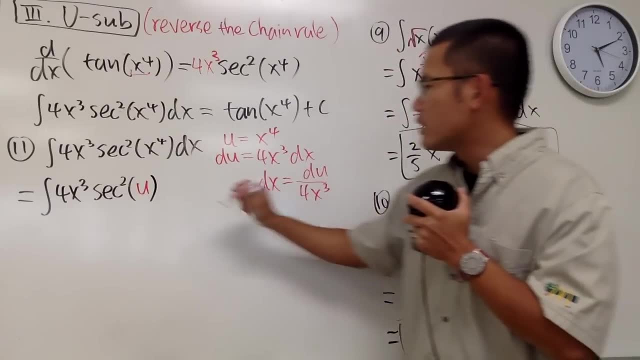 and we have the x to the fourth power and notice that's our choice for the u and let me just put that down. And in the meantime we also figure out: the dx is du over 4x to the third power, like this: 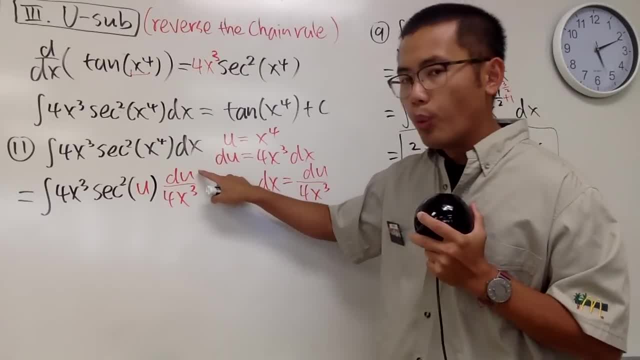 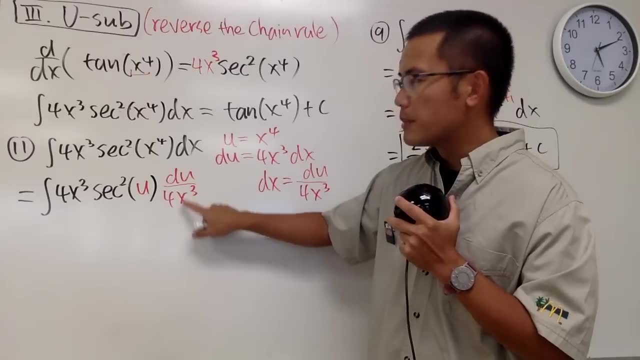 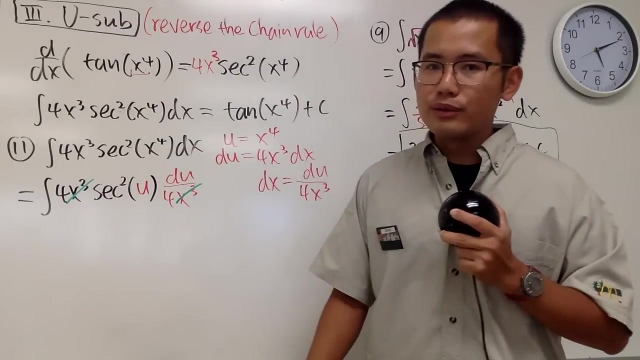 And now you have to remember one thing: In the u-world, x is not invited, and in this case it's really nice, because we have the over x to the third power here and here we also have x to the third power, So they nicely cancel each other out. 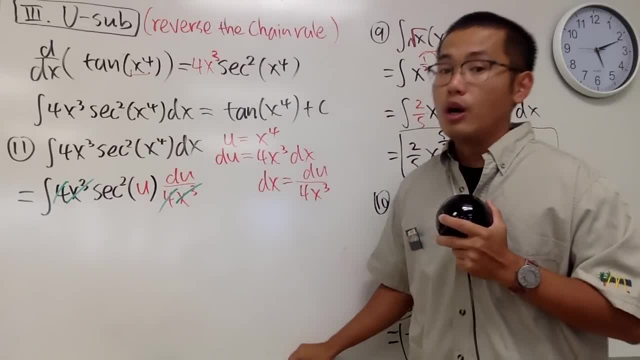 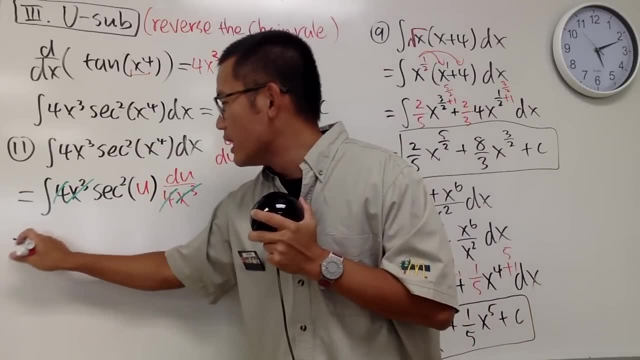 And, of course, this 4 and that 4, they also cancel each other out as well, right? So this is great. This integral is in the u-world now and we see that this is just the integral of secant squared of u du. 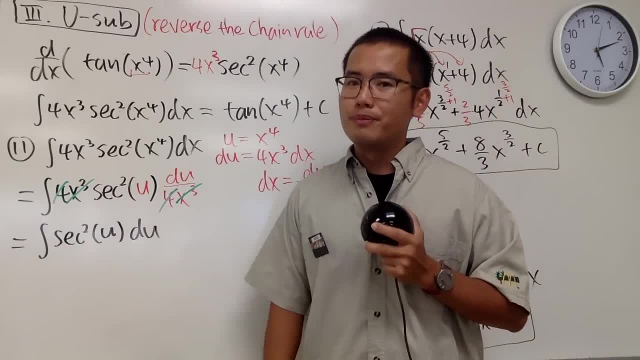 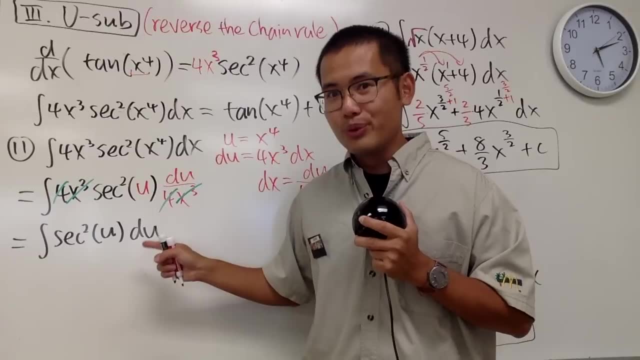 And now, what's the integral of secant squared u du? What's the integral of secant squared Tangent? and in this case it will be u, because we are in the u-world. So this, right here, the answer to this. 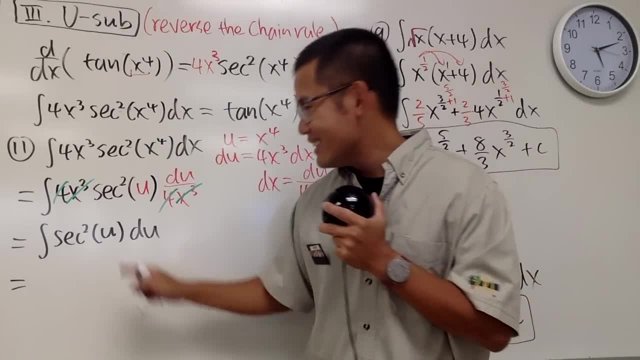 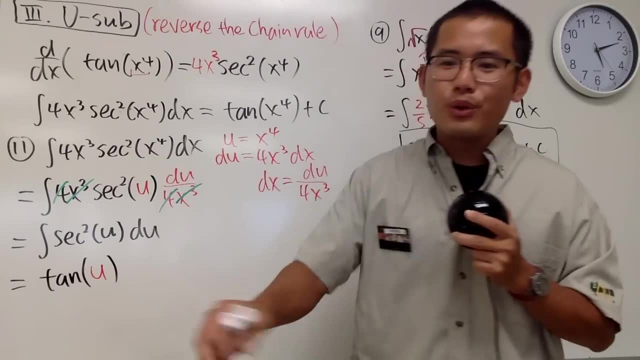 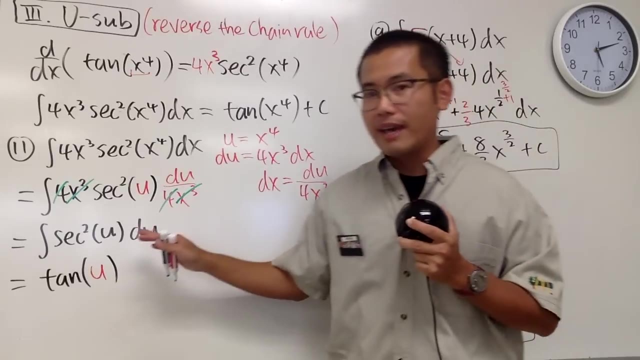 is actually just from question number one. Know our derivative right, So this right here will give us tangent of u like this: just like question number one, right? Just like question number one. However, we're not done yet because, don't forget, we were in the x-world. 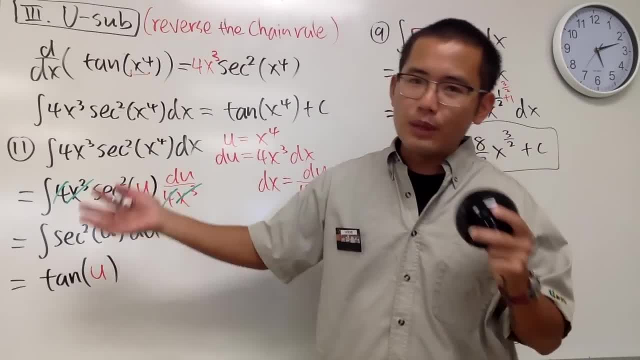 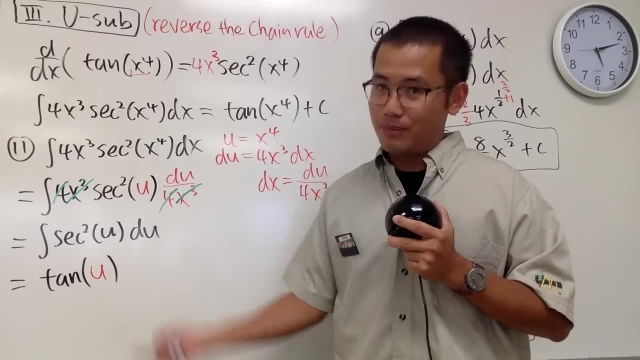 Even though we finished our integral in the u-world, it's just like we finished our vacation in the u-world. When the vacation is over, we have to get back to the reality, namely the x-world. So let's go ahead and look at: u is equal to x to the fourth power. 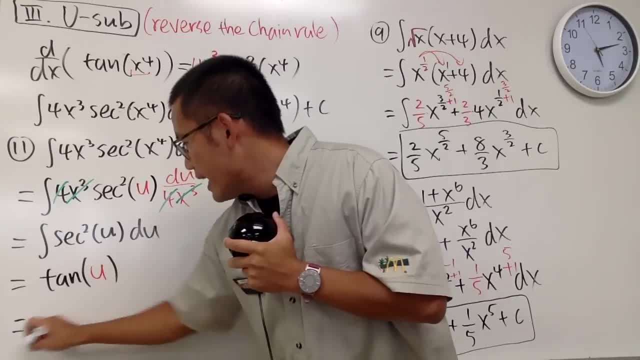 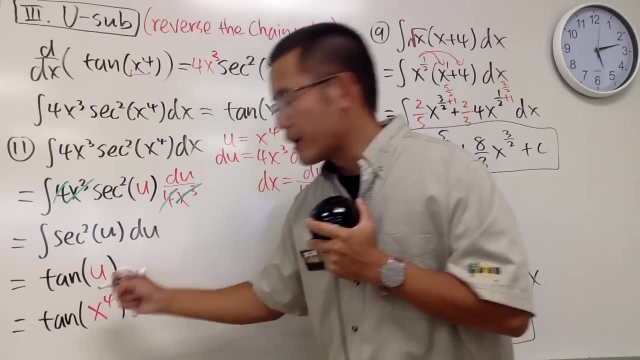 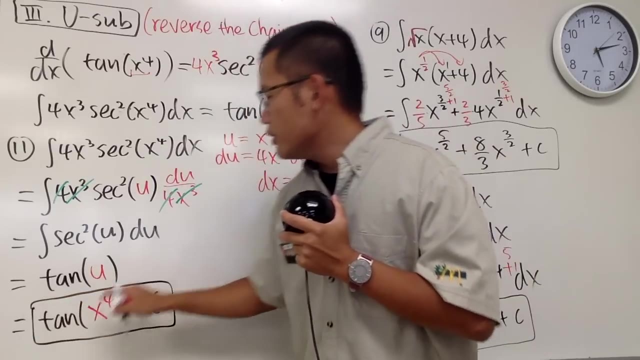 and put it right here. So in the end we just get tangent of x to the fourth power And this right, here is it, and I will just put down a plus c at the very end. Some people might say, hey, you should be putting down a plus c every single time after you integrate it. 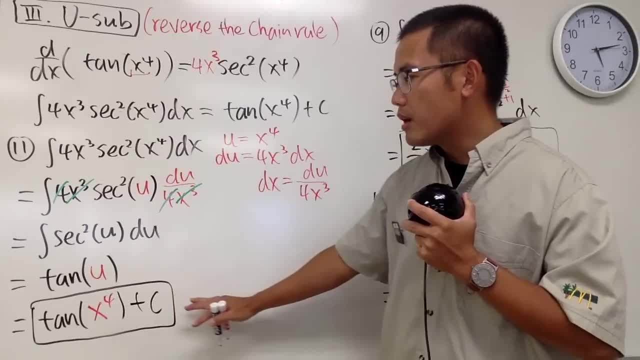 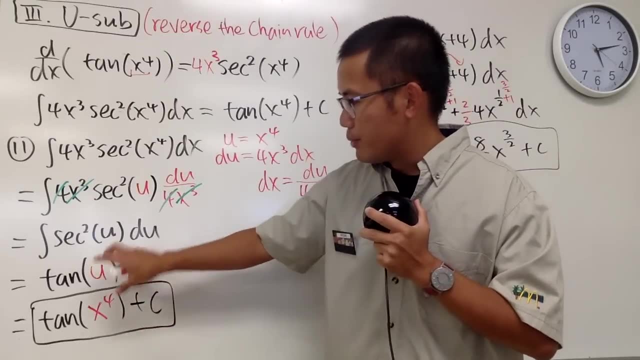 but we're just doing definite integrals right here, indefinite integrals. So we'll just put down a plus c at the very end, after I put this back to the x-world right And also later on we'll be skipping this step. 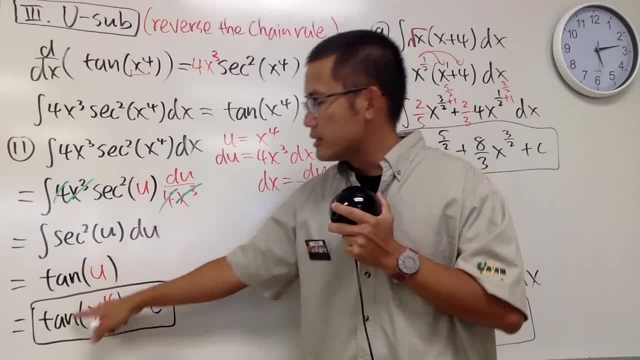 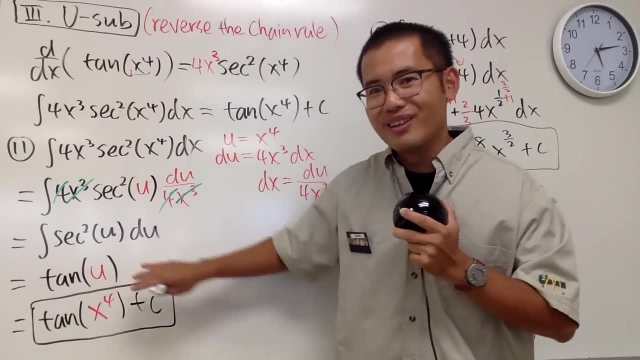 because you see, the integral of secant squared u is just tangent u, and of course we can just plug in the x to the fourth power in here right away. we can skip this step as well. right, And don't forget the plus c at the end. 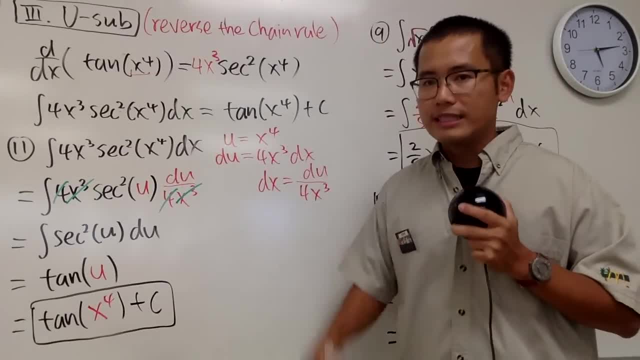 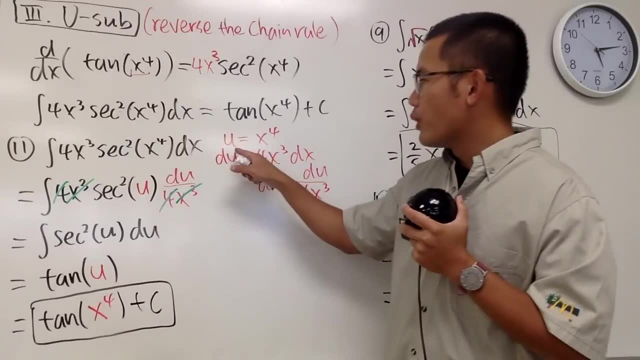 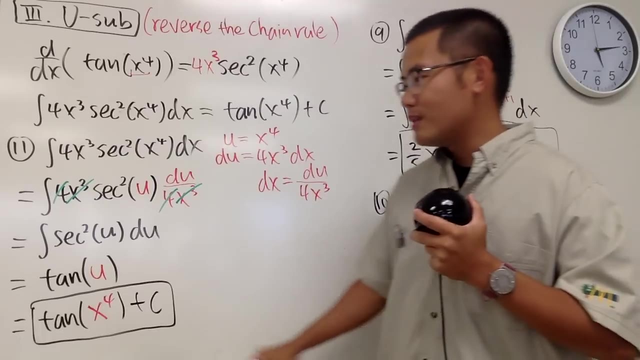 at the very end. So this is how you carry out the u-substitution right, And the hardest part of doing the? u-substitution is that you have to find out what choice for the? u will work out the best. Sometimes you may just have to give it a try a few more times. 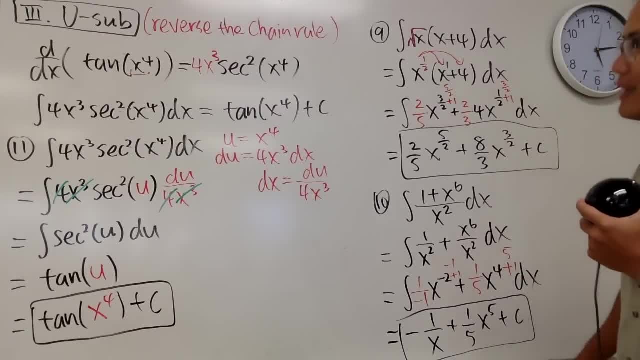 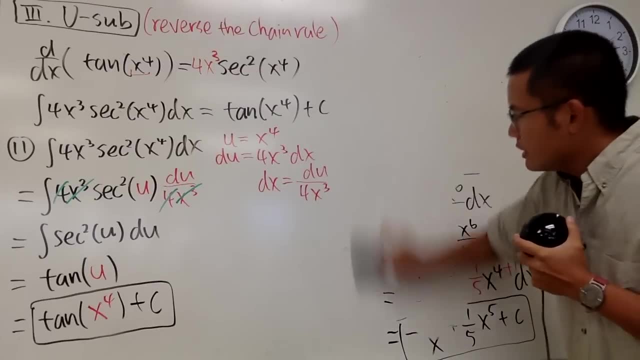 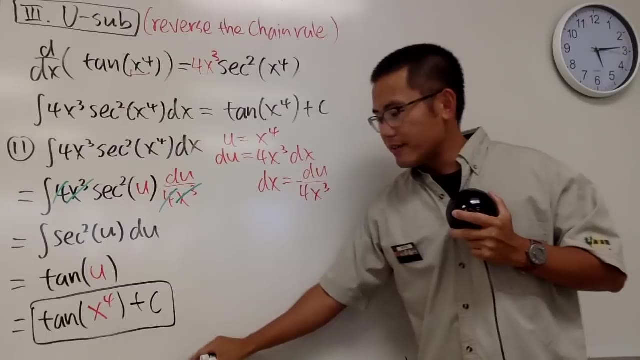 and the truth is sometimes u-sub doesn't even work. That's why we have other techniques as well. But anyway, let's look at the next example in this category and if you guys want to have more practice after this video, be sure you guys watch my 100 integral video. 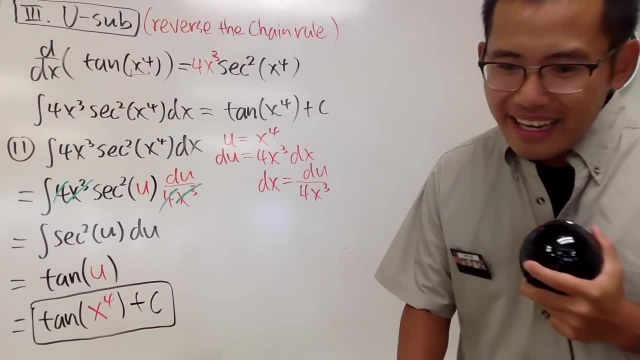 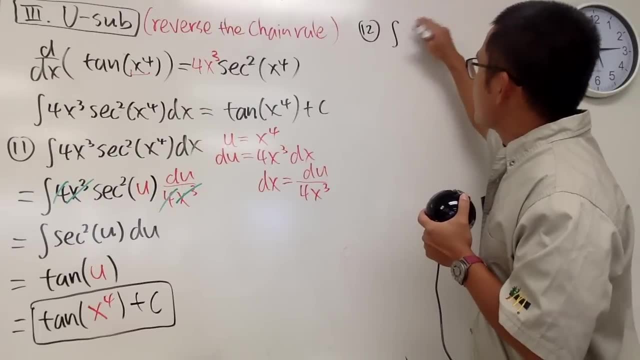 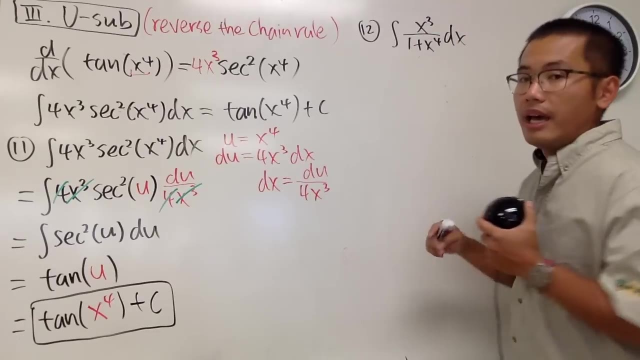 because I have 100 integrals in that video, right? Anyway, here we have this question number 12. right, here We have the integral and we have x to the third power over 1 plus x to the fourth power dx. 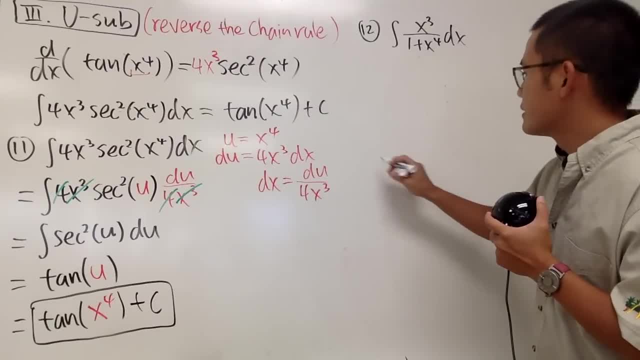 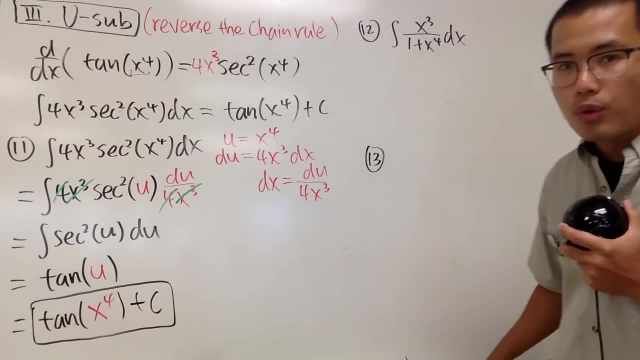 And in fact I would like to put down two questions right here at the same time. So we have the 12, and let me also put down number 13. Because for number 13, we will have the integral of, and I don't know what this is popping up for. 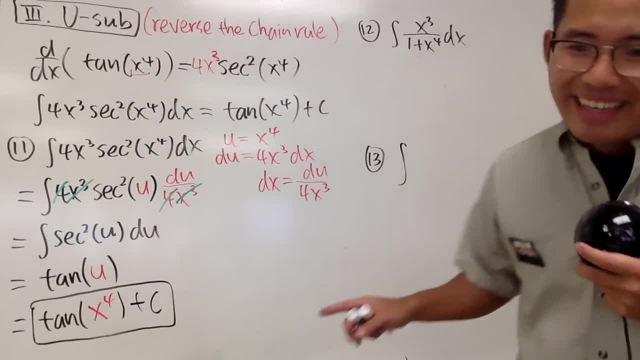 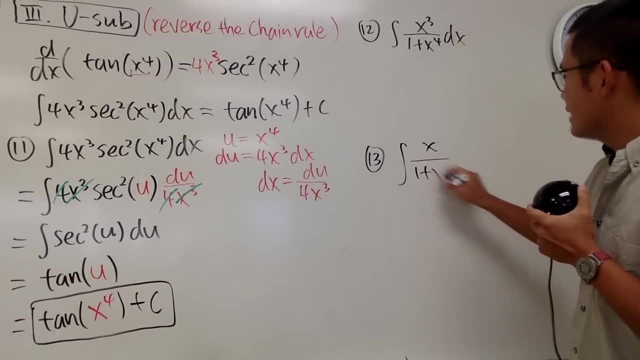 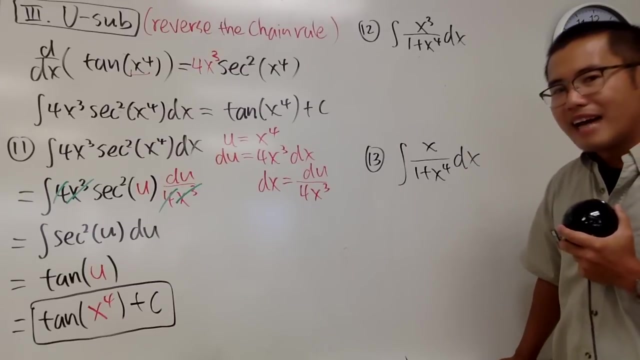 so let me just click that and it's still recording. so that's good, Alright. so for number 13,, we have the integral of x over 1 plus x to the fourth power, dx. As you can see, these two integrals, they look so alike. 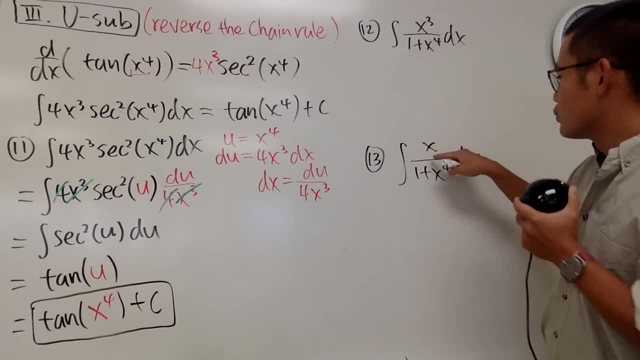 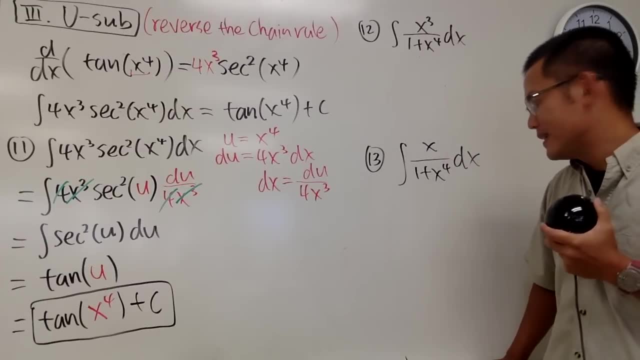 because for this one we have x to the third power and for this one it's just x to the first power, and they both have the same inside denominator. They look so alike, but sometimes it's tricky. This is the hardest part when you're doing integrals. 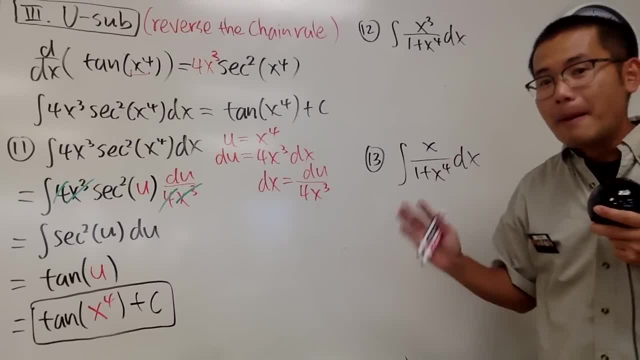 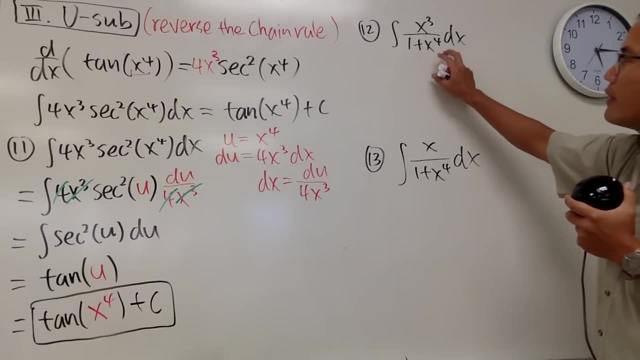 When you have two integrals, if they look so alike, maybe one integral is very different than the other, right? Anyway, let's see what should we do for number 12?? You should be what? Well, look at the top, we have x to the third power. 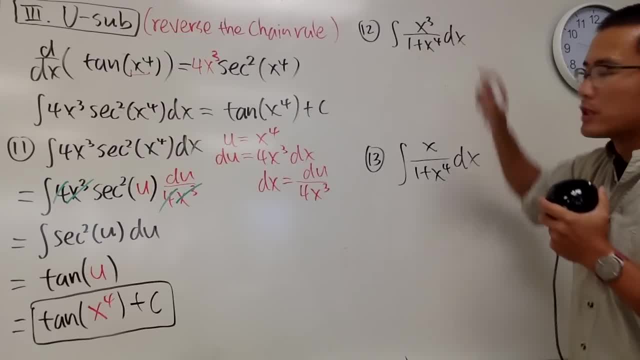 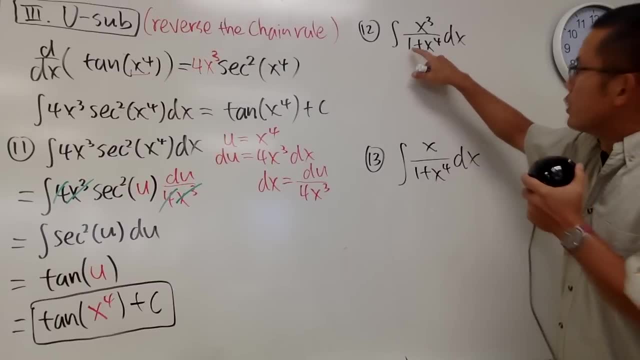 and look at the bottom, we have 1 plus x to the fourth power And you have to think about the relative every single time. If you look at the bottom, differentiate this: The relative of 1 plus x to the fourth power is: 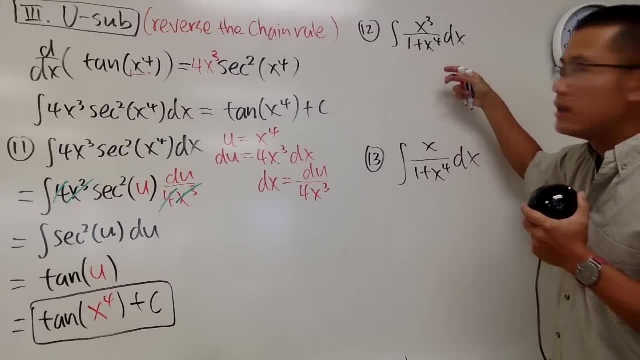 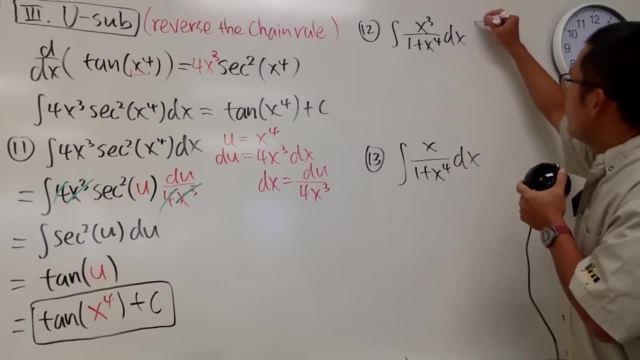 4x to the third power right, And we happen to have x to the third power on the top. That's very nice. That would be a good choice for you. So let me put that down. We are going to let u equal to 1 plus x to the fourth power. 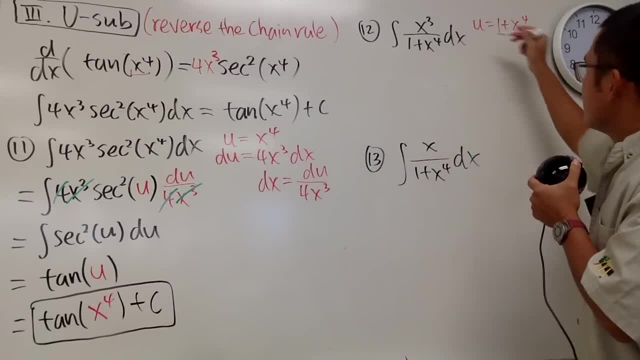 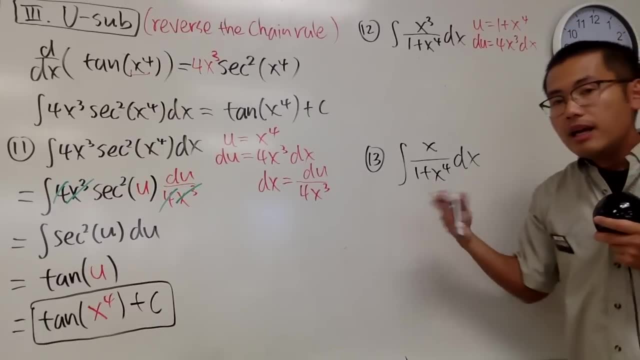 and then we'll do what we did over here. du will be the relative of 1 and 0, so we get 4x to the third power, dx, And let me just recommend you guys to isolate the dx, And we can do so by dividing this on both sides. 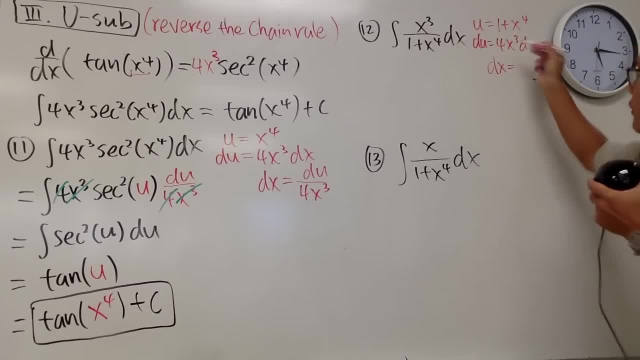 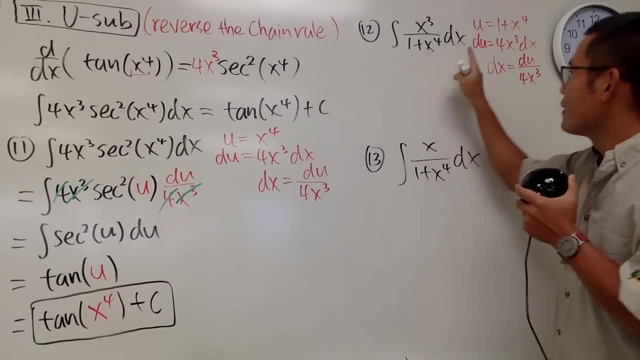 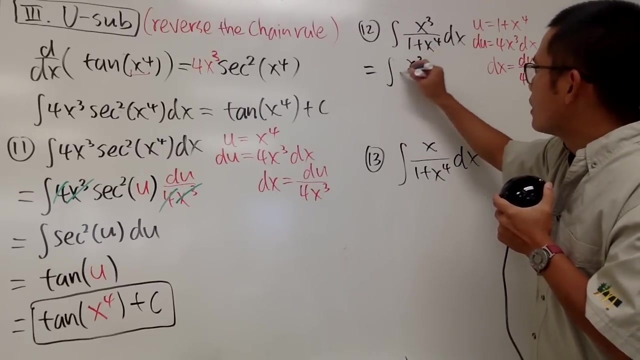 So we get: dx is equal to du over 4x to the third power, like this. And now again we'll take this integral from the x-world to the u-world And, as we can see, this will be the integral on the top- is x to the third power over. 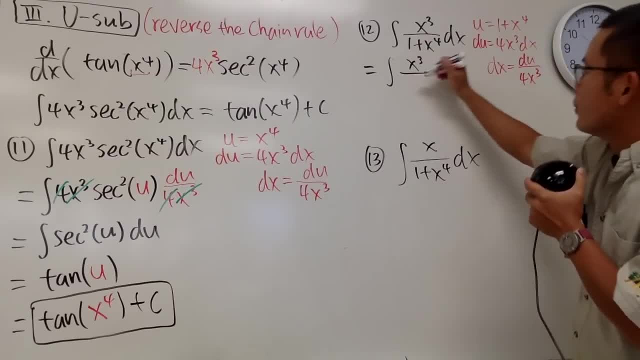 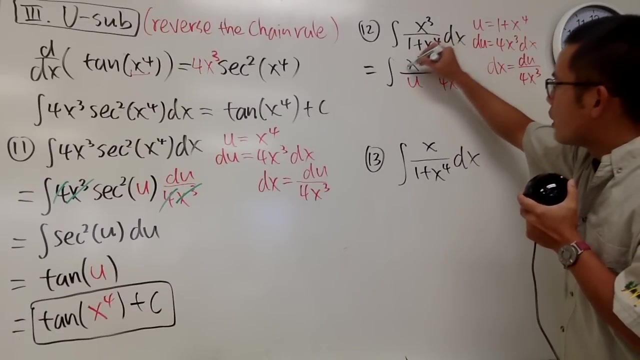 on the bottom, 1 plus x to the fourth power is the u right here And dx is du over 4x to the third power And this is very nice. We are in the u-world And notice that the x to the third power and the x to the third power. 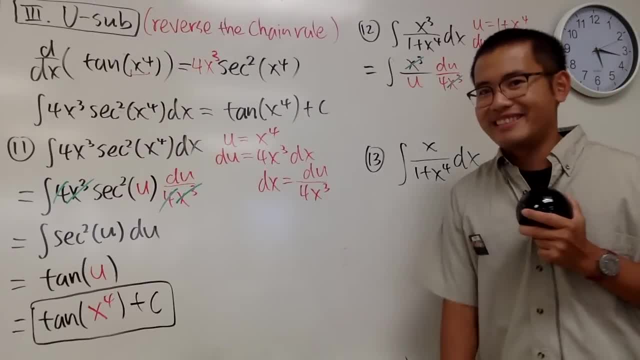 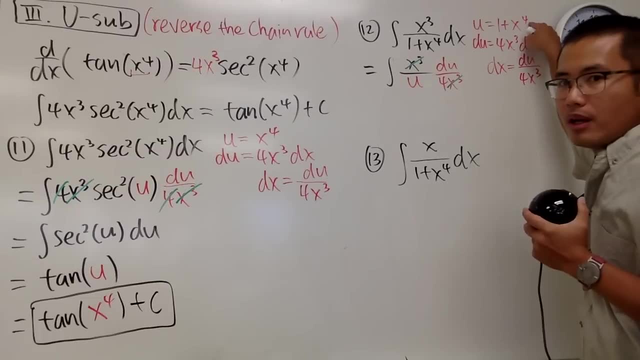 they cancel each other out, And this is so, so, so nice. One thing to notice, though: Notice how I let u equal to 1 plus x to the fourth power. I took the 1 with us Because when we differentiate 1,. 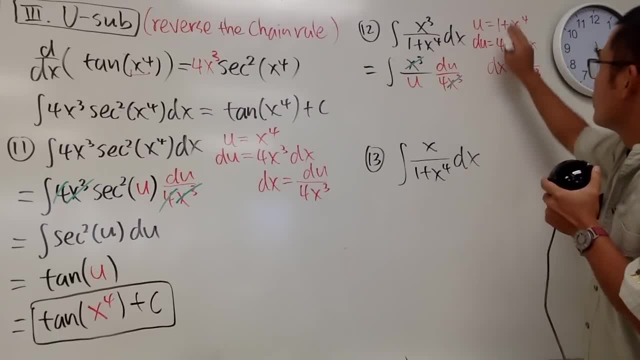 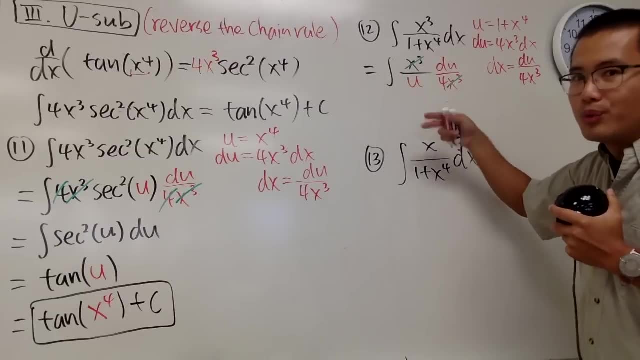 it's just 0. So that would be convenient. If you let u equal to just x, to the fourth power, you will just see the cancellation. But maybe you have a constant like 1 plus u, etc. Keep this in mind. 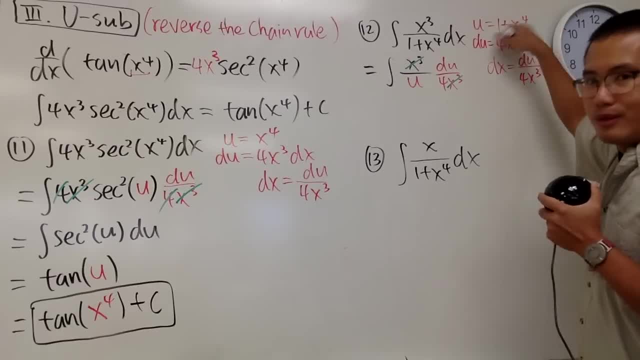 If you have a 1 plus whatever, take that with you. Maybe it works out pretty nicely. just like this, right here Now. this is what we have And notice. this is what we can do. Here we have du over 4.. 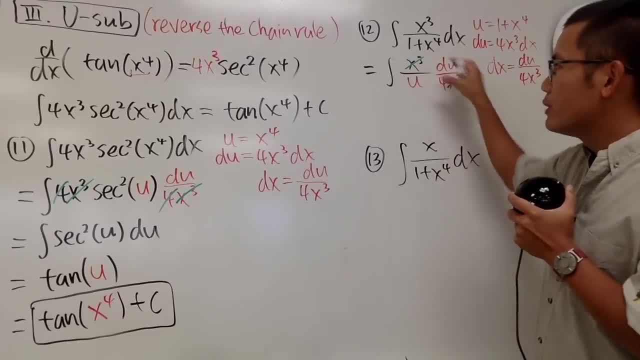 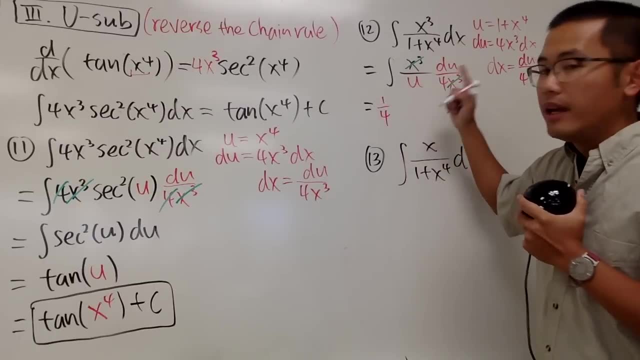 And the 1 over 4 is just a constant multiple. We can put that all the way in the front of the integral, So this looks like 1 over 4 all the way in the front, And this only works when we have a constant multiple. 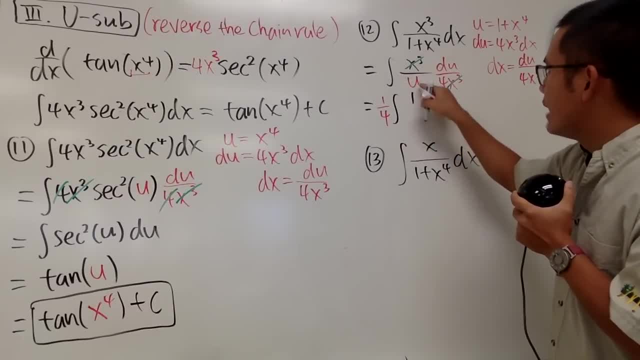 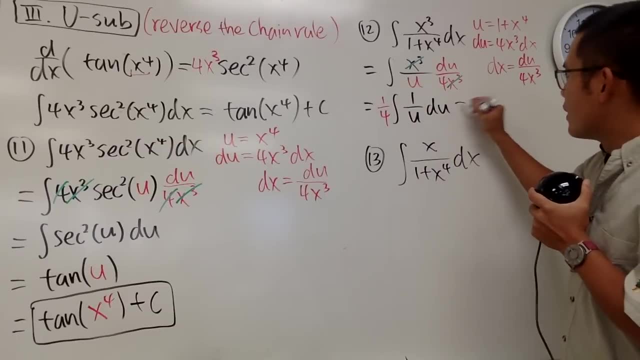 And then here we just have the integral And we have the 1. And this is the over u du And, as you can see, this 1 over 4 stays. This is still 1 over 4, of course. And what's the integral of 1 over u in the u-world? 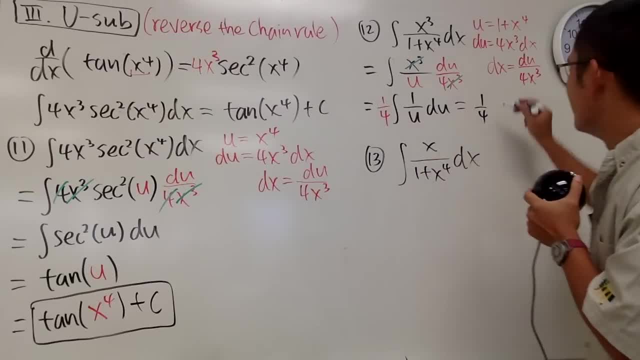 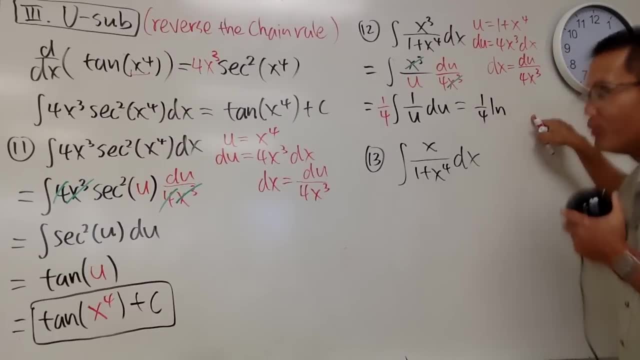 Well, it's just natural log absolute value of u, So let me just put that down. We have the natural log absolute value of the u- u right here. Now we know u is equal to this, So let's just put that down already. 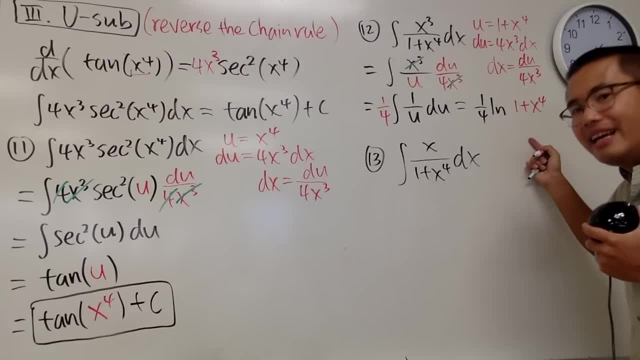 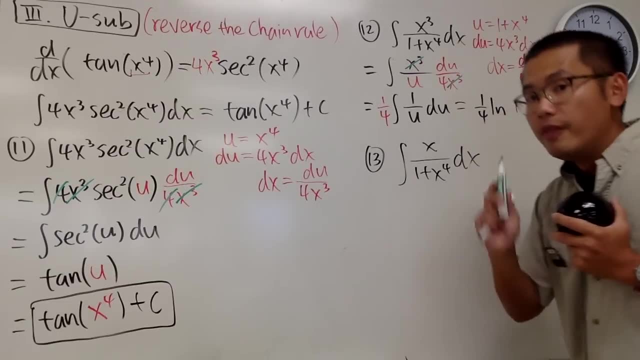 So this will skip. you know, we can skip one step, And I actually mentioned it: the absolute value. But in this particular case, focus on this. Notice that x to the fourth power, this right here- is always positive, And then we are always adding 1 to it. 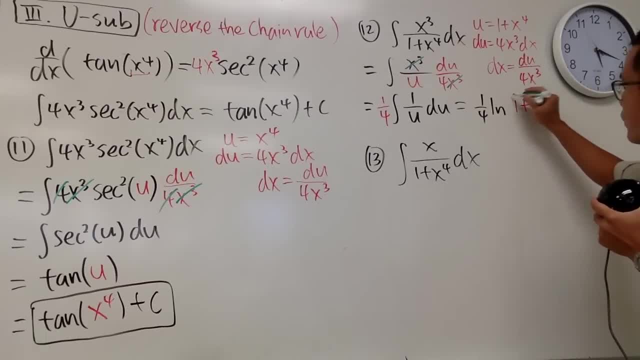 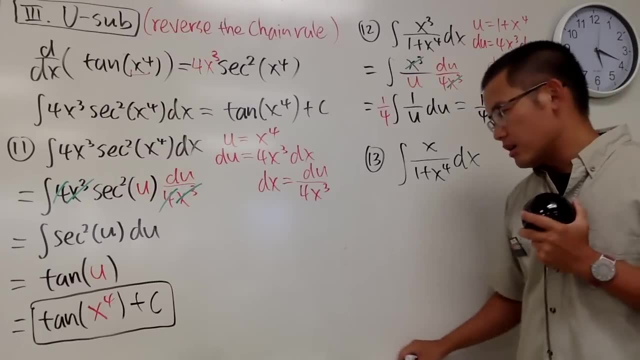 This is always positive as well. So in fact, we don't need the absolute value in this case. We can just put down a parenthesis And if you are using like Wolfram Alpha- or maybe you are checking the answer in the back of your book- 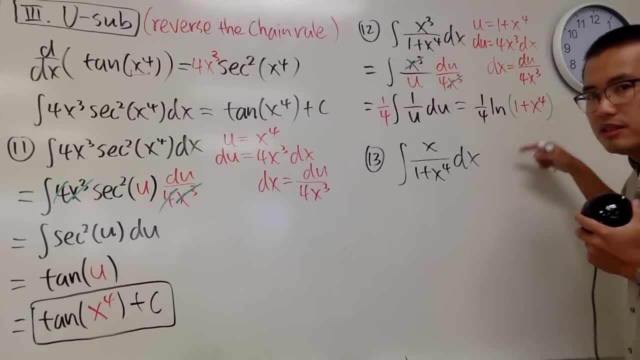 sometimes they don't have the absolute value, but rather they have the parenthesis. because of that reason, Because if the answer is always positive, you can just do this right here. So this right here is it the answer for that, And we are all done. 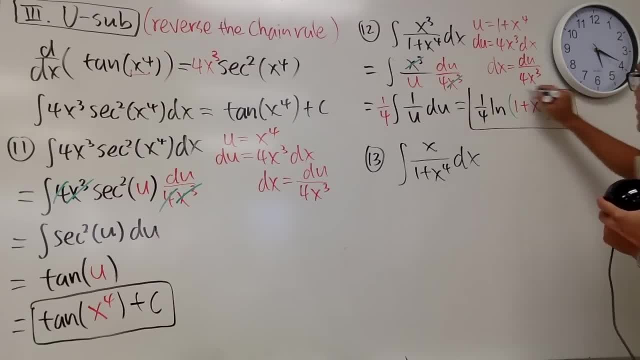 So we'll just put down a plus z, And this is it. Now, here is the trouble For number 13,. we only have x to the first power. If we put down this- well, you see we have that du is equal to 4x to the third power. 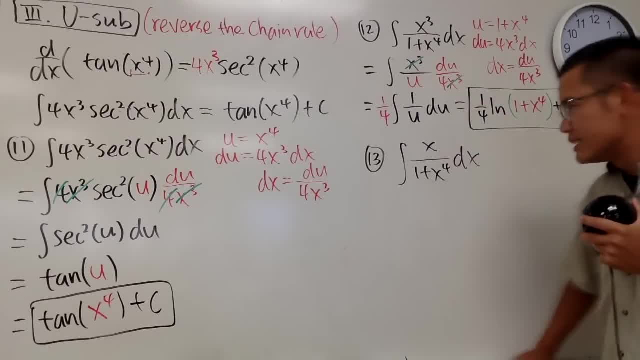 This is only x to the first power. That's no good, Hmm. So what can we do? I don't think this is going to be working out again. We will have to have a different choice, And now we have to think carefully. 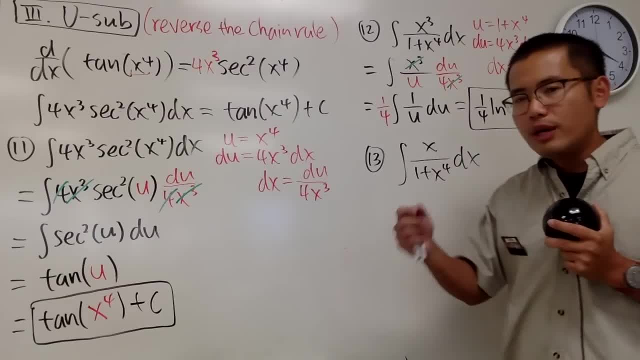 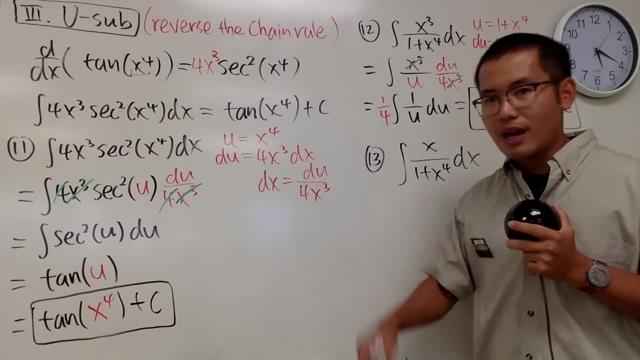 This is x to the first power. The derivative of what will give you x to the first power? Well, the derivative of x to the second power will give you something with x to the first power. right, And do we see any x to the second power here? 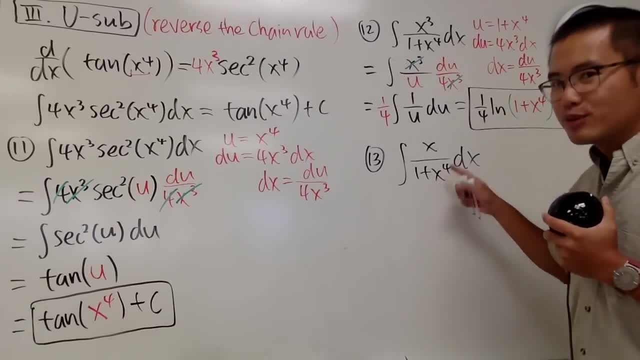 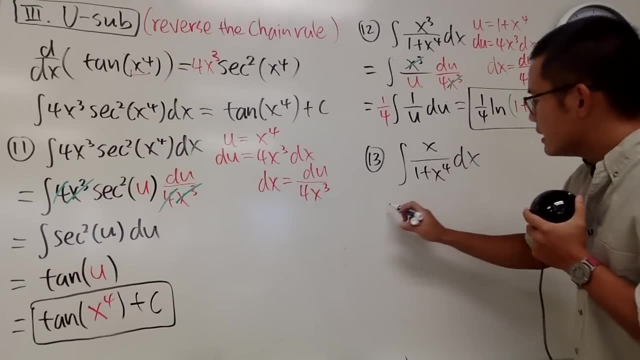 Not yet, but we can make it happen, Because if you look at x to the fourth power, we can look at this as what x squared, squared, And that's the key. If we look at this, this is the same as saying: 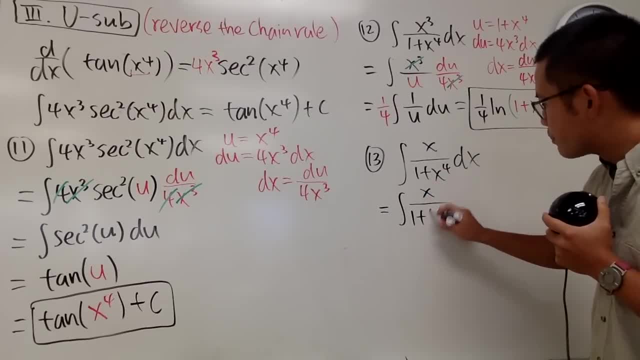 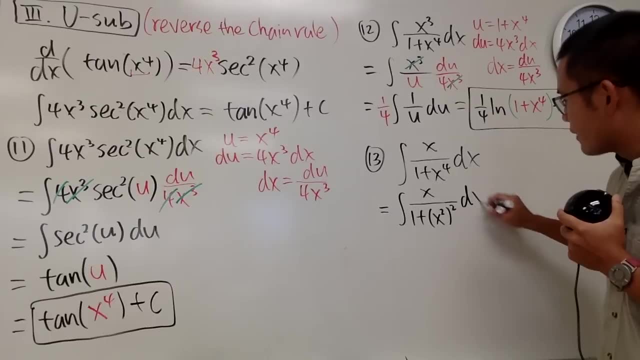 the integral of x over 1 plus parentheses, and we look at x to the fourth power as x squared to the second power And of course we have the dx right here And again. the reason we are doing this is because, if we now 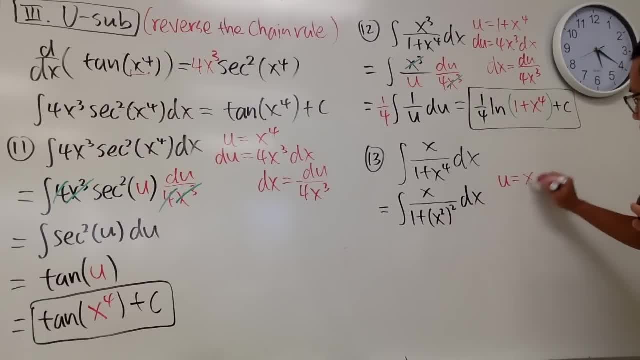 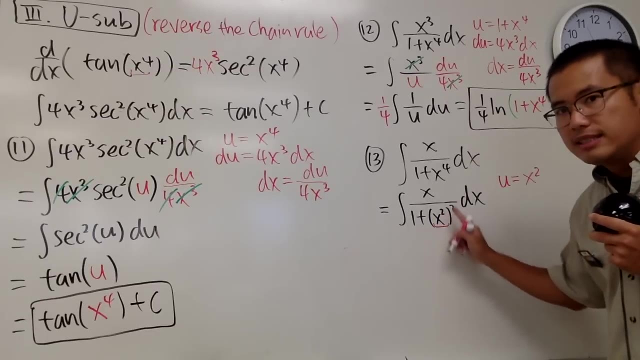 we let u equal to x to the second power. Notice I am not letting u equal to the whole denominator And I'm also not letting u equal to 1 plus x squared, Because the x squared is just the inside. It's just this little input, right here. 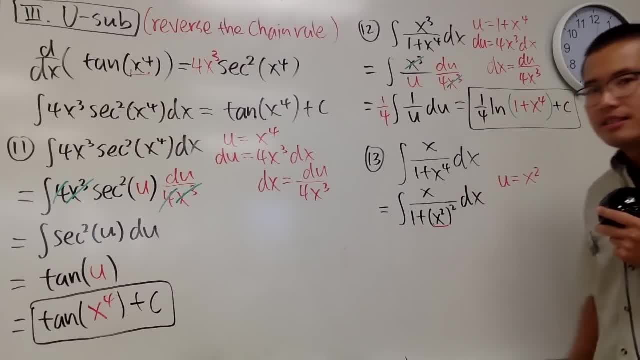 u is equal to x squared. That's my choice of u in this particular situation. And then do the usual business: Differentiate both sides. We get du equals 2x dx, And again, let's just isolate the dx. 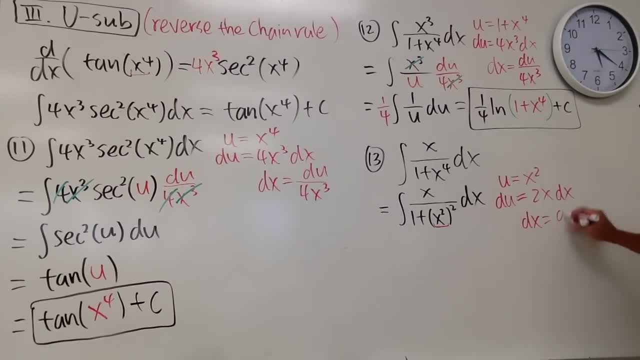 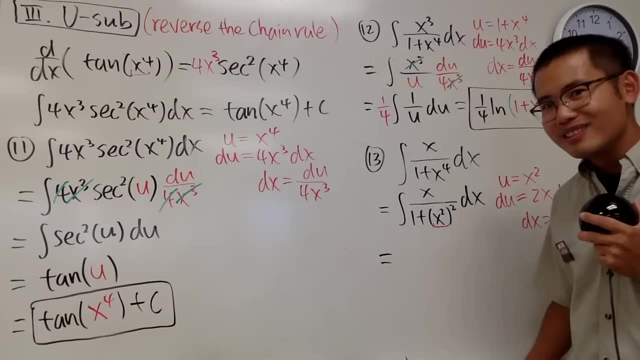 So we divide the 2x on both sides, We get dx equals du over 2x. Like this, We're going to take this integral to the? u world And, as you can see, we have the integral x over the 1 states. 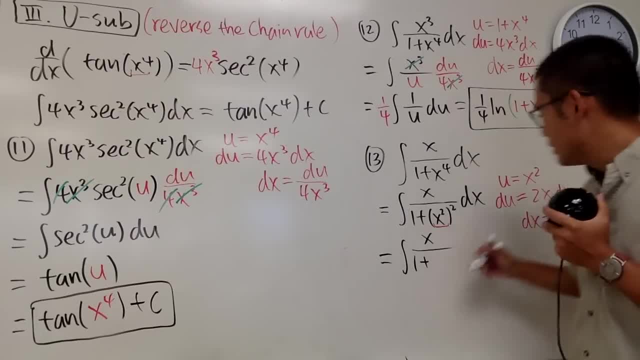 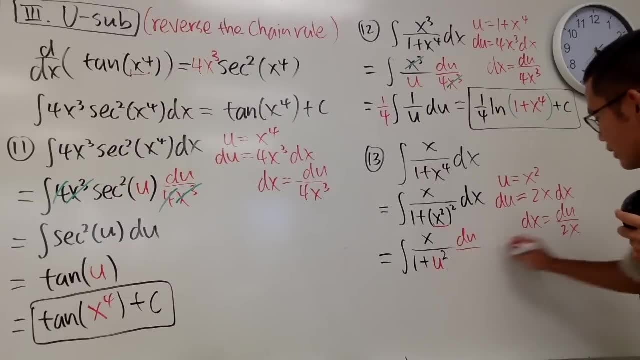 the plus states. This time it's just the input is our u. So we have u squared like this: And the dx is du over 2x And we are in the? u world. We still have x, But no more. 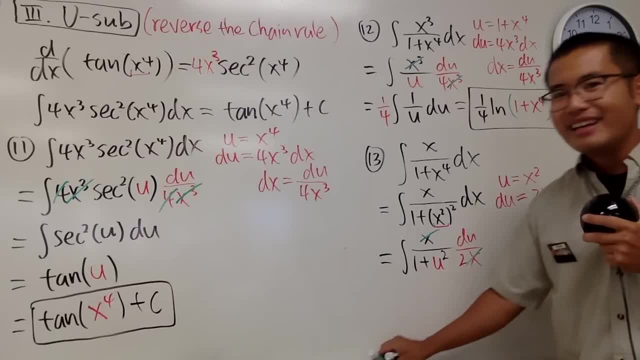 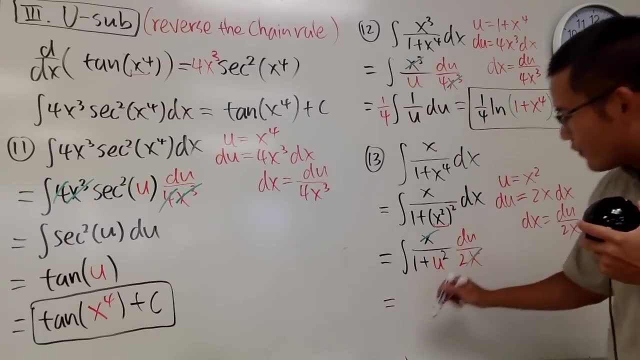 because they happen to cancel each other very nicely. However, we have a 1 over 2 as a constant multiple. It's okay. We can do what we did over here. We can put the 1 over 2 all the way in the front. 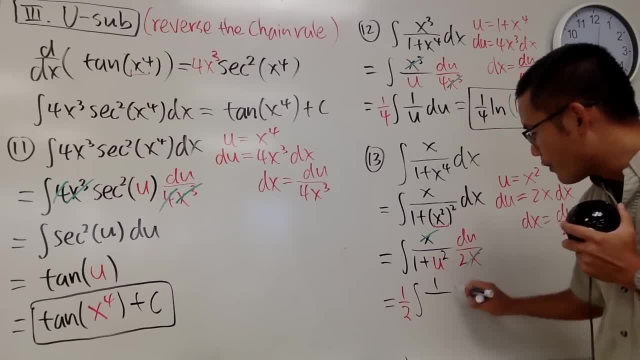 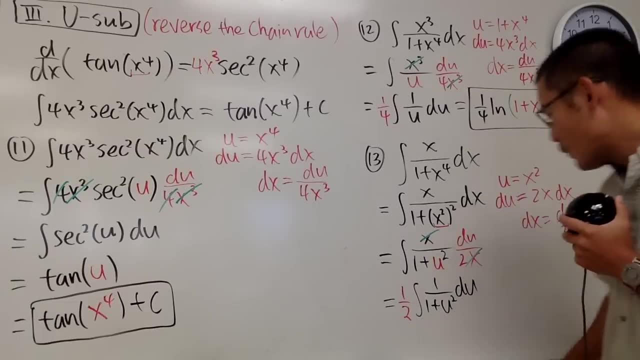 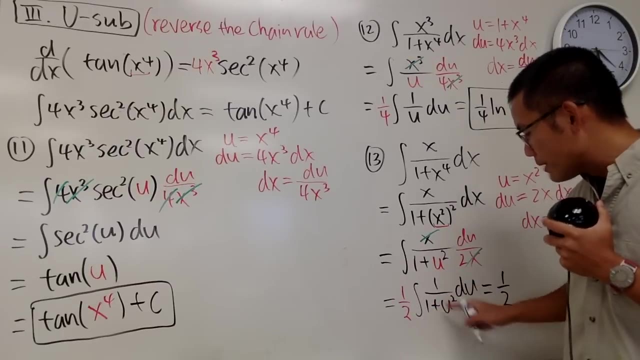 And then looking at the integral of 1 over 1 plus u squared in the? u world like this: Well, well, In this case, of course, let's just write down the 1 half first. But when we have the integral of 1 over 1 plus u squared, 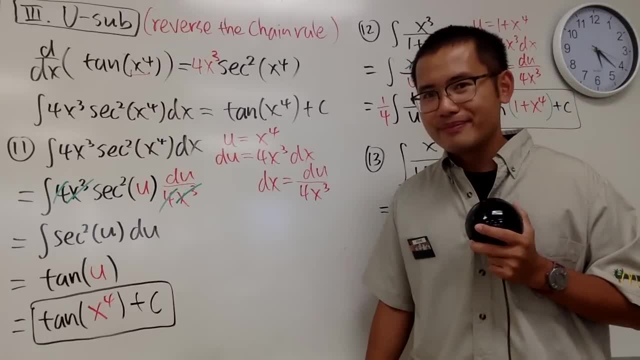 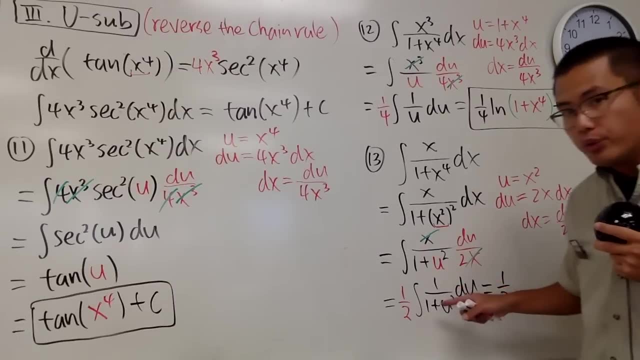 in the? u world. what is the answer for that? Well, the answer is inverse tangent. Again, know our derivatives. The derivative of inverse tangent of? u will give us this, So we will have the inverse tangent in this situation. I will put down: u. 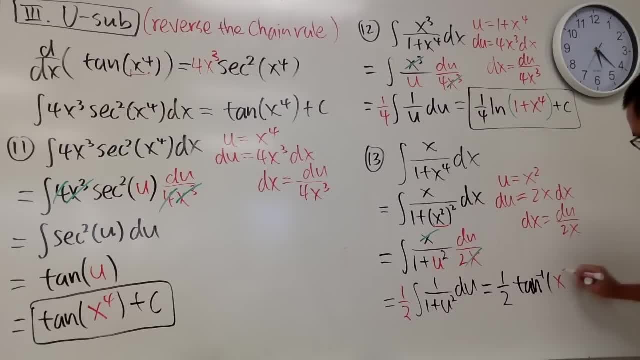 but we know u is x squared, So let's just put down x squared right here already. So that's it in this particular situation. As you can see, number 12 and number 13, they look so similar, but they are very, very similar. 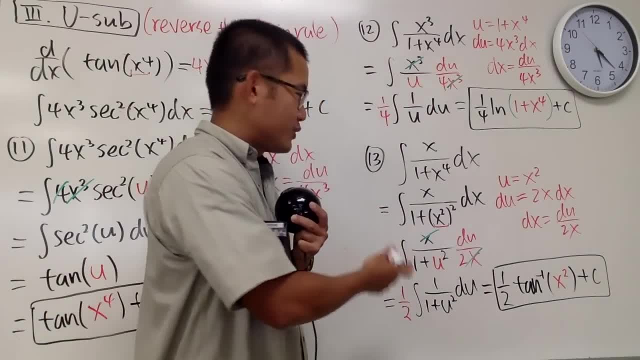 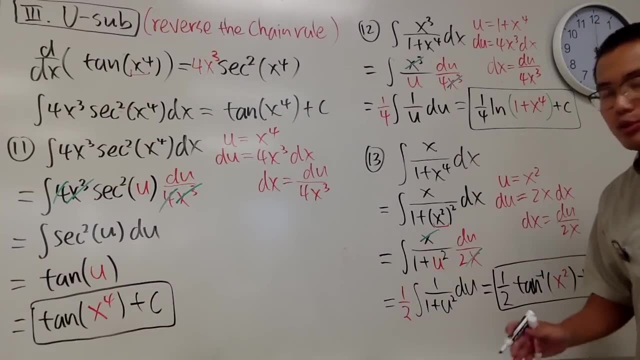 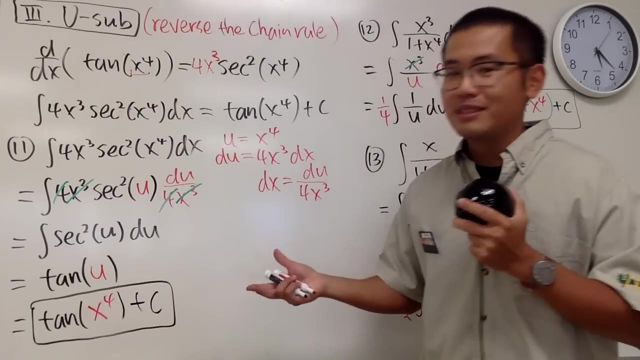 Of course I will say: number 13 is much harder, I will say: But once you practice it, you can do it too. So this is how u substitution works. And again, I'm only showing you guys these few examples, because we'll be using these techniques later on again. 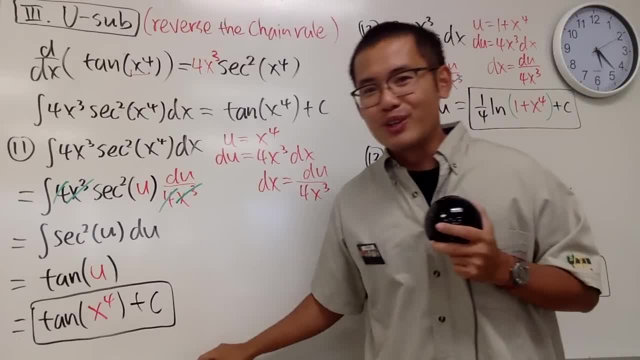 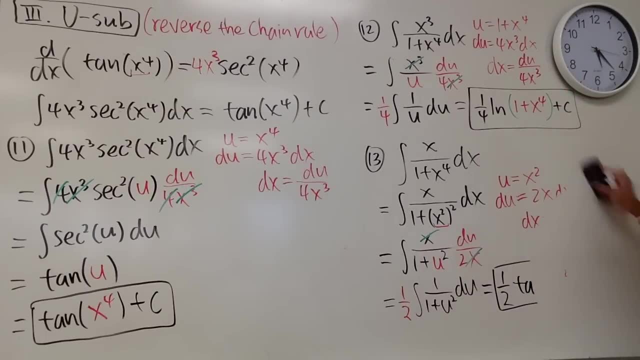 like over and over. So this right here will be just a good warm-up, so we can see how this works. That's all Okay. So now I'm going to erase all this right here. In fact, I don't know how long this will take me. 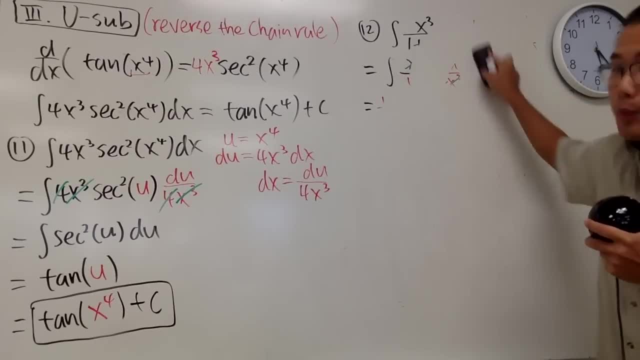 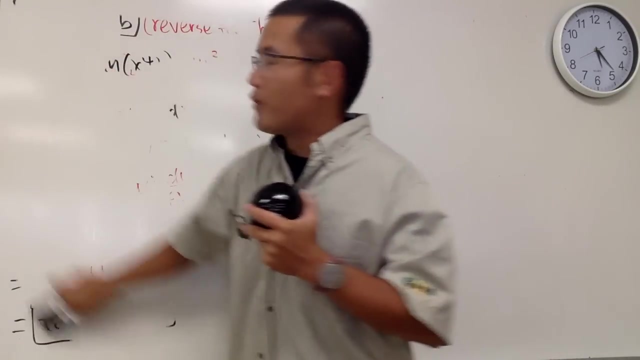 even though I know this is only 50 integrals that we are doing. but I am explaining how come the method works right, Why the method works and how the method works, And I'm trying to go over all this from scratch, So I really don't know how long this will take me. 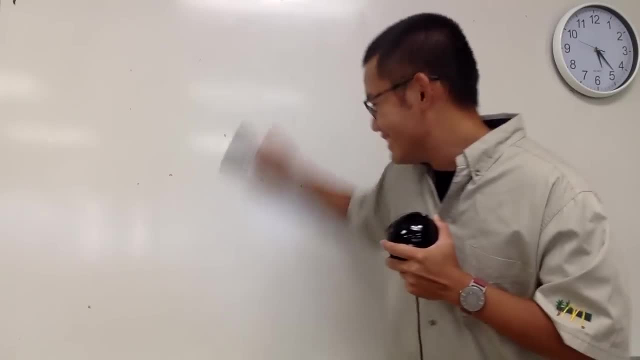 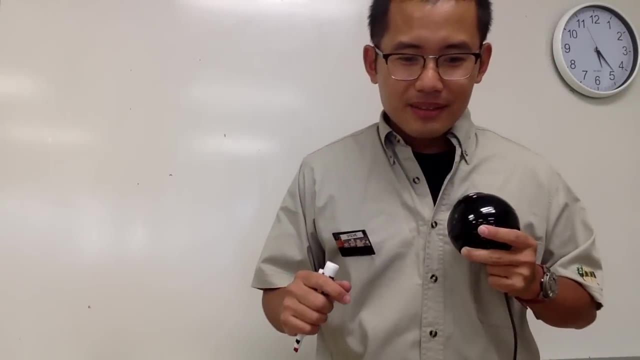 That's why I'm only doing 50 of them. All right, So that was category number 3.. I actually have one more for you guys, question number 14.. So let's do one more. This is still used up, okay. 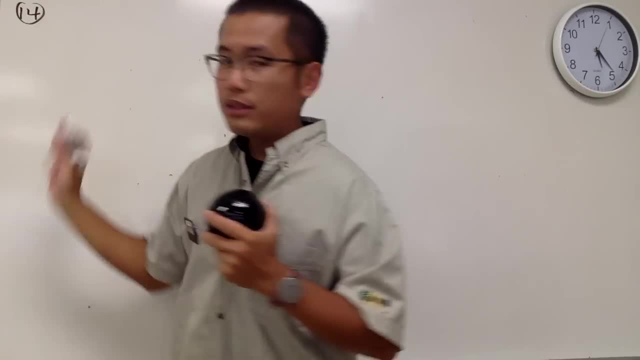 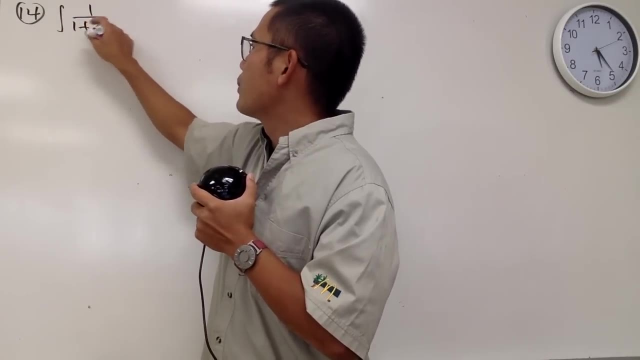 So I am not at the next category yet. So let's look at question number 14.. This right here is also slightly trickier. So let's look at the integral 1 over 1 plus square root of x, dx. The answer to this is non-natural. log of. 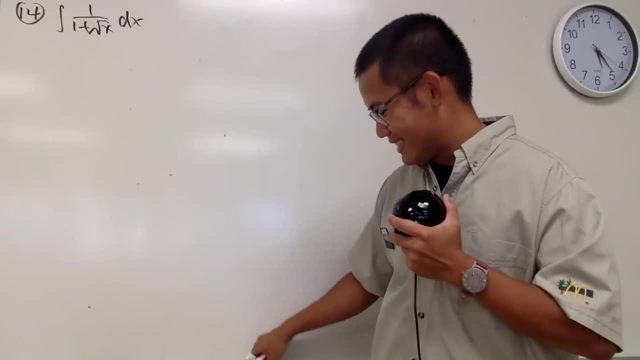 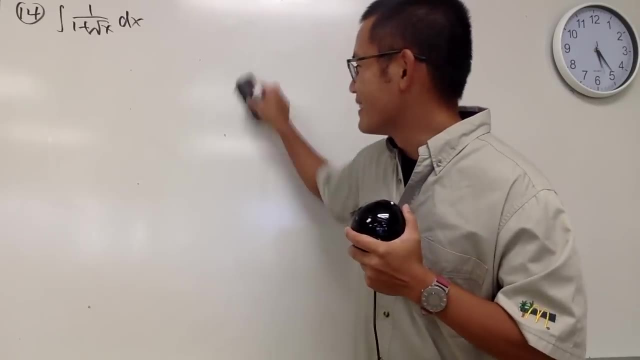 1 plus square root of x. It's not like that. So this is how I'll show you, And I'll tell you guys what I mean by what I said earlier. Okay, here's the deal. Unlike question number 13 and question number 12,. 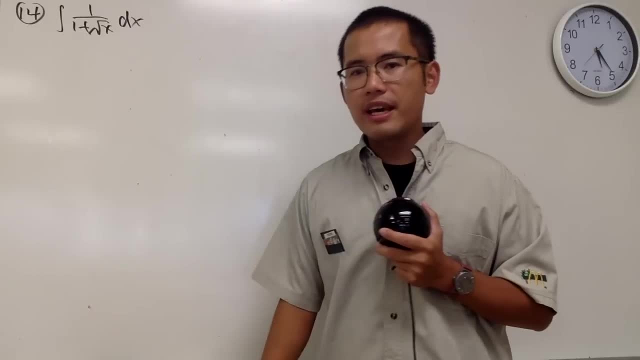 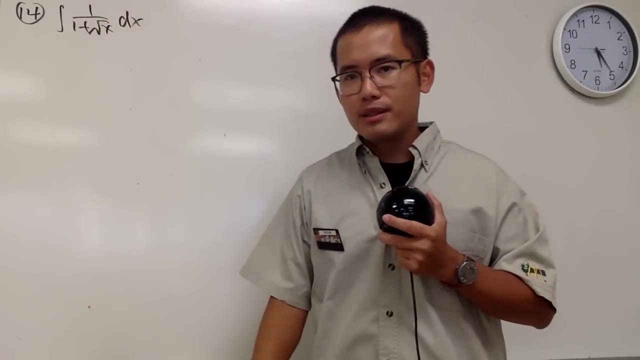 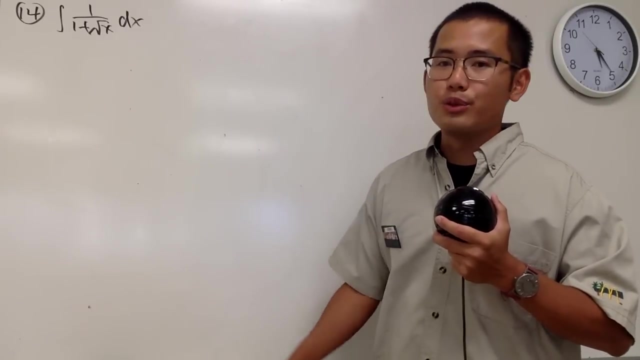 it seems that we don't have a lot to work with in this case. And can you think about the derivative of what will give us 1 over 1 plus square root of x? It's non-natural log of the denominator. Well, let's just carry out the u sub and see what happens, right? 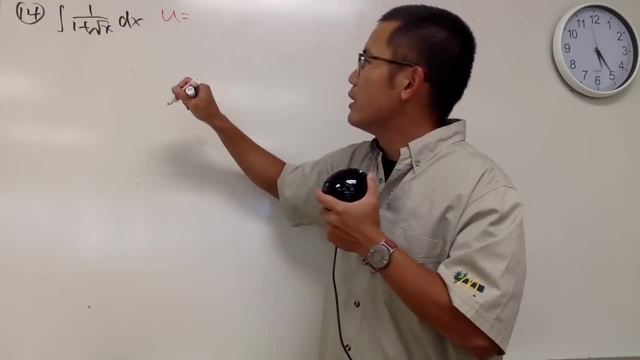 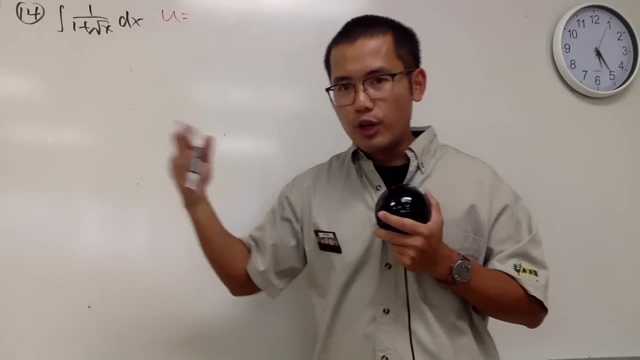 So I will put down u equal to well. here is the function part that we have the 1 plus square root of x, And I will take the 1 plus with us because if we differentiate the 1, it's just going to be 0.. 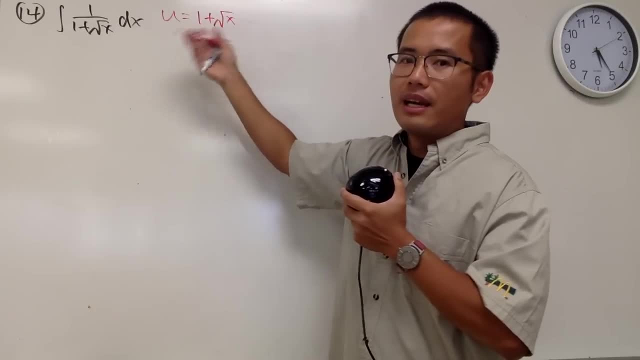 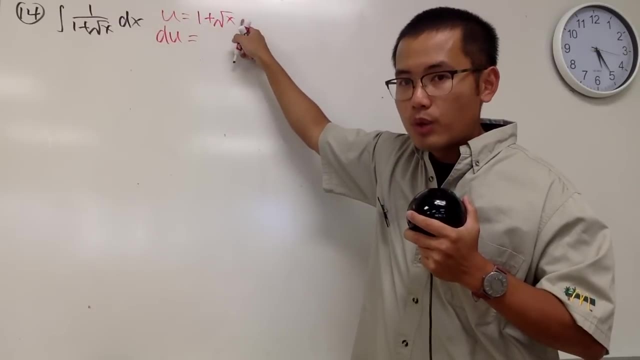 So let's write down 1 plus square root of x like this, And then, as usual, differentiate both sides. du will be: derivative of 1 is 0 and derivative of square root of x is 1 over 2. square root of x- dx, like this: 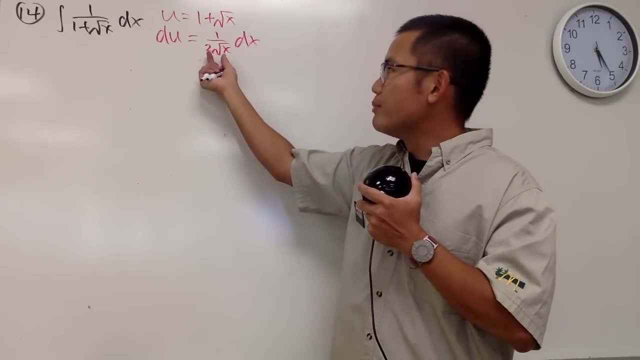 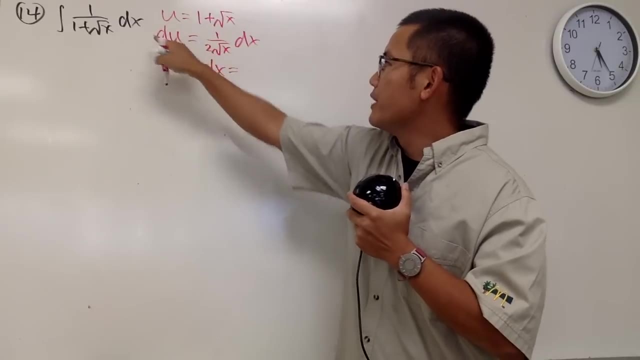 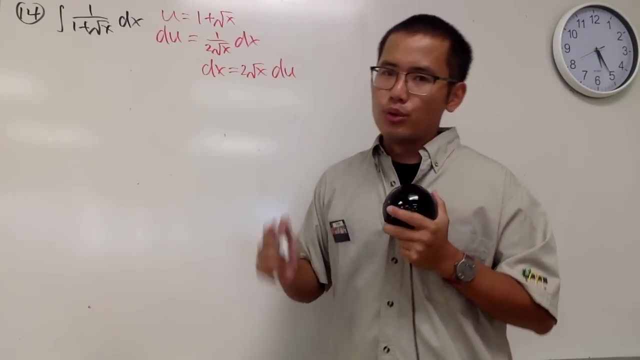 This time, to isolate the dx, we will have to multiply 2 square root of x on both sides. So we see that dx is equal to this over there: 2 square root of x times du. This is what we have Now. let's go to the u-world to see what happens. 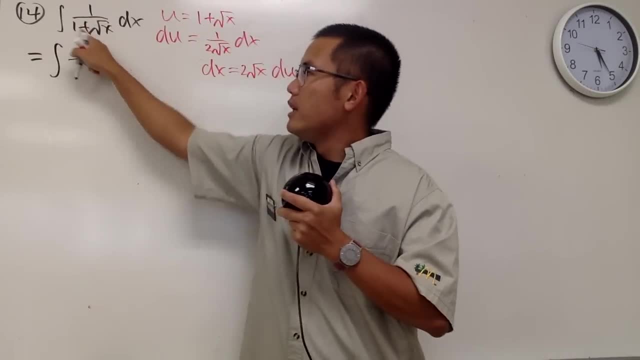 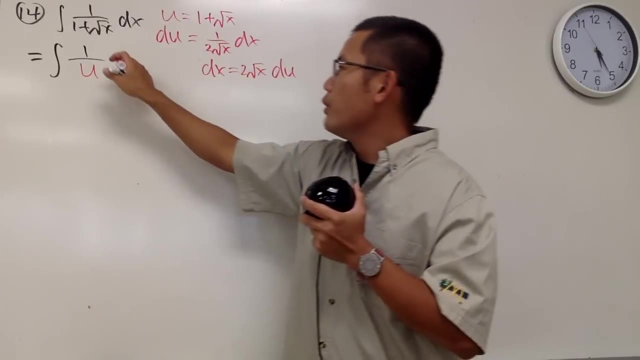 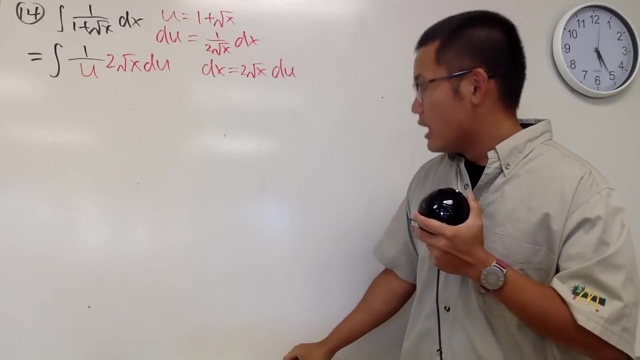 Here we have the integral and we have 1 over the whole denominator is the u, okay, And then dx is equal to this. Notice we have 2 square root of x, du, like that. So this is what we have, And here's the trouble. 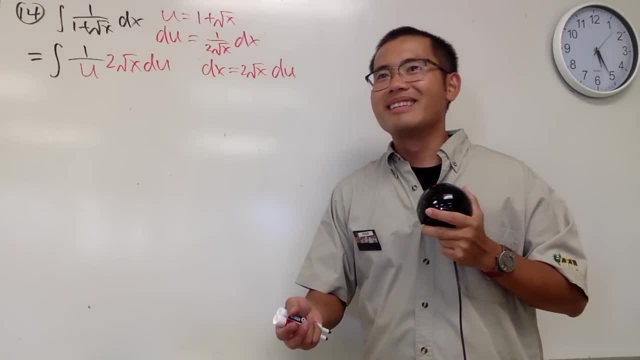 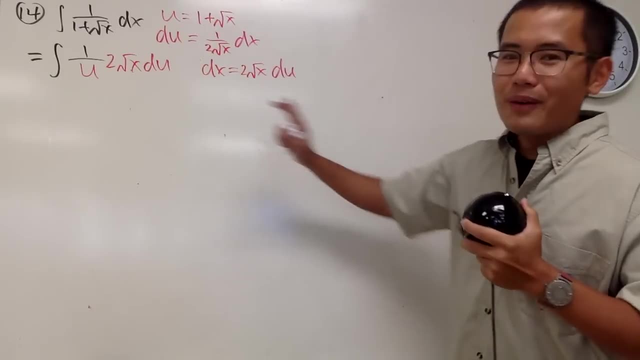 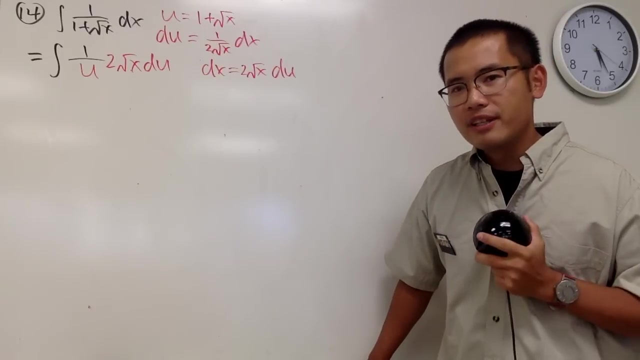 I'm recording. so, Oh, okay, Yeah, I think we're good, right, Thanks. So this right here is what we have. We have a trouble right here because in this particular case- notice- we are in the? u-world and we have the? u. 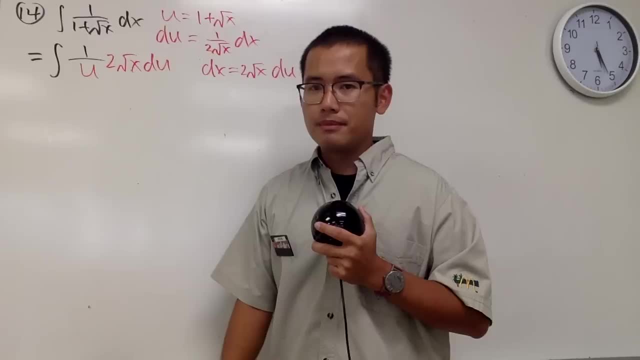 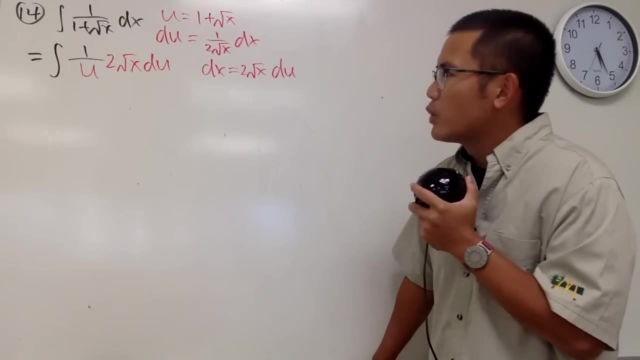 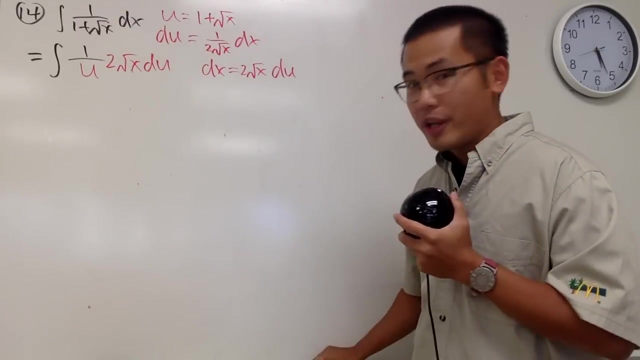 but we also have the square root of x. Keep this in mind. x is not allowed in the u-world, So it seems like we are stuck, but not quite, because. notice that we have the square root of x right here. Well, if you refer back to our choice for u, 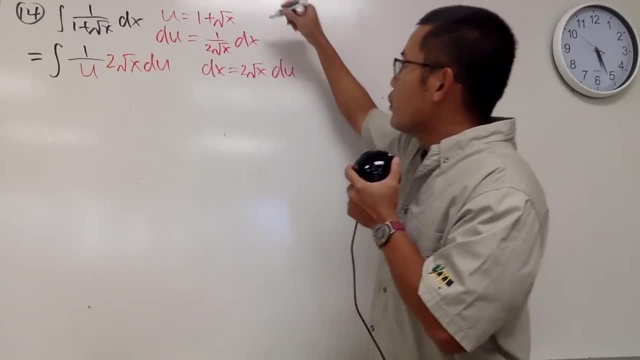 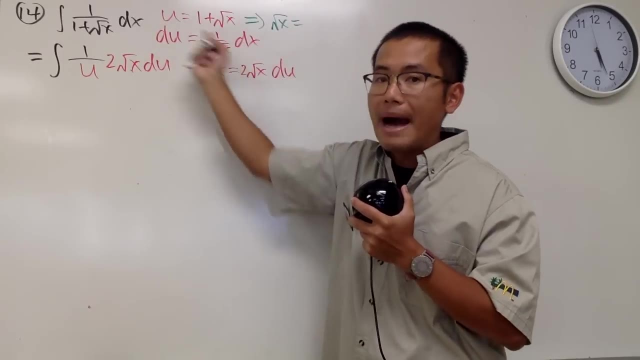 u is equal to 1 plus square root of x. In another word, we can just go ahead and subtract 1 on both sides and we can say square root of x is equal to u minus 1, right here, And that's very nice. 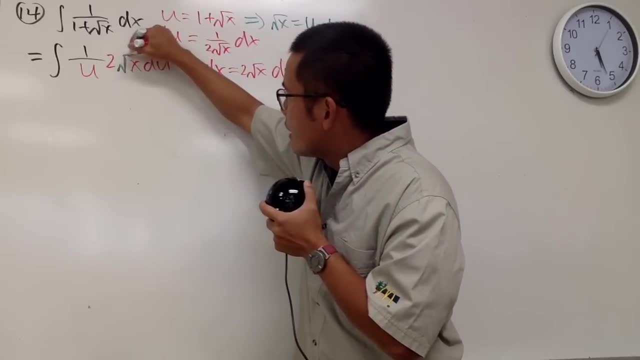 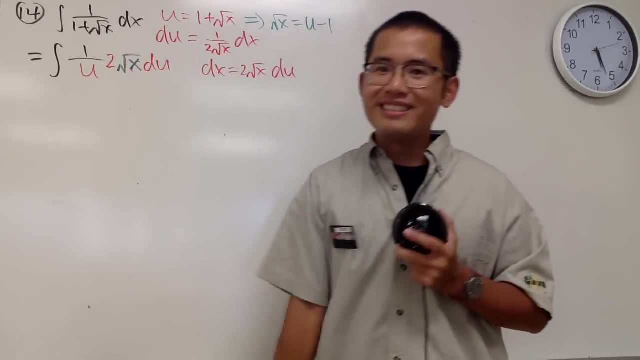 So if we look at the square root of x right here, we can actually just replace the u minus 1 to here and everything will be in the u-world. That's it. So that's actually really, really nice. Now let's do the following. 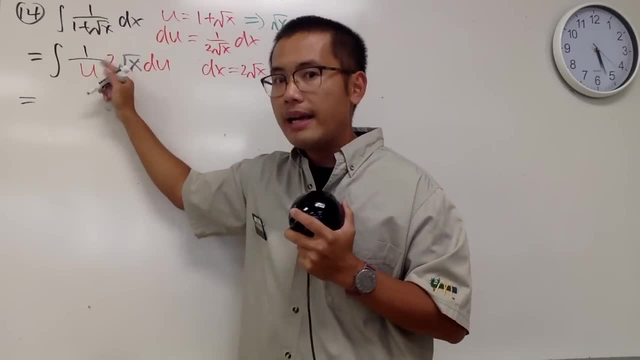 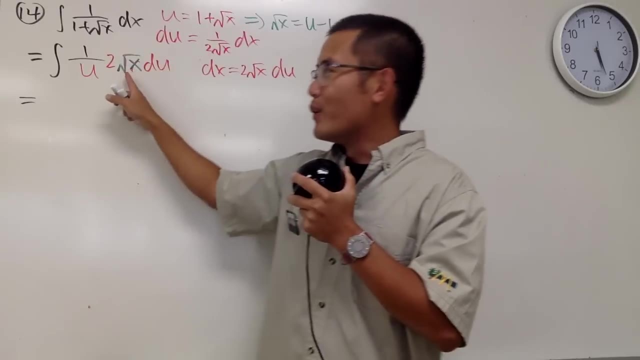 Here we go. This is 2, and it's just a constant multiple. I know why I said this is a 2.. Of course it's a 2.. This 2 is just a constant multiple, So we can put the 2 all the way in the front. 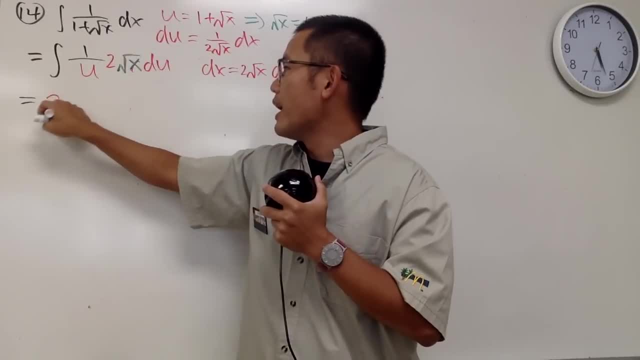 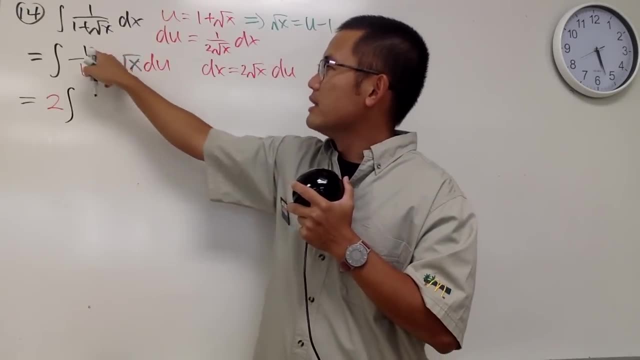 And let me just write that down already. And then we have the integral right here And notice that we have the square root of x. You cannot put the square root of x to the front. The function part has to stay in the integral. 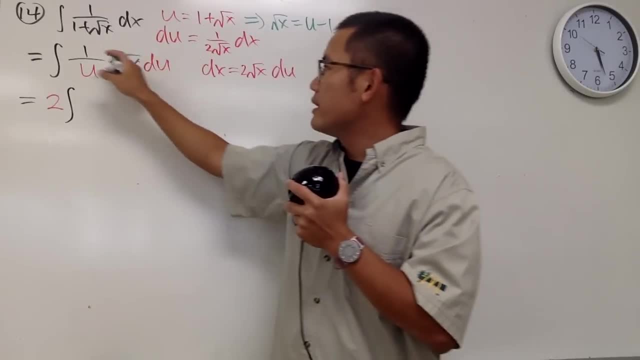 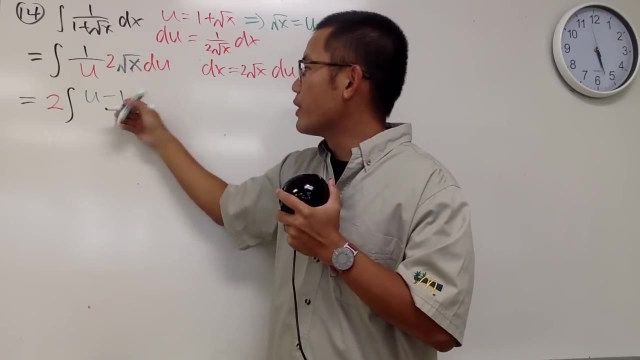 This right here is u minus 1.. So I will write it as this times that and that's the u minus 1 right here, And we still have the over u, and then we have the du, like this, And that's very nice. 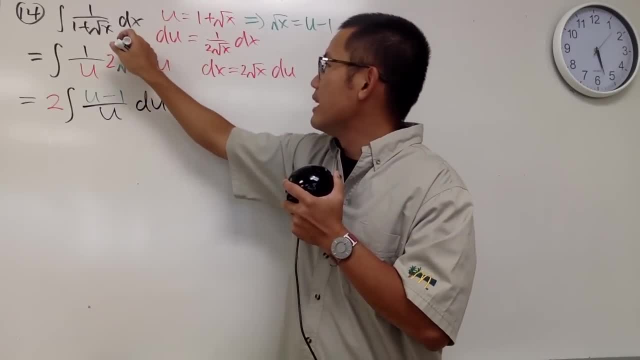 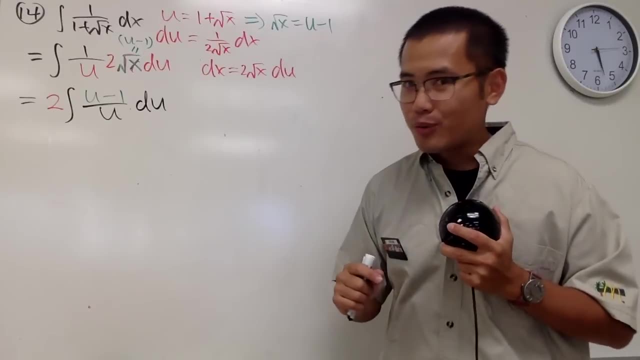 Again, all we are doing is just replace the square root of x as u minus 1, and then I'll put this on the top, and that's what we have. Now we are referring back to the second category, the first power rule. 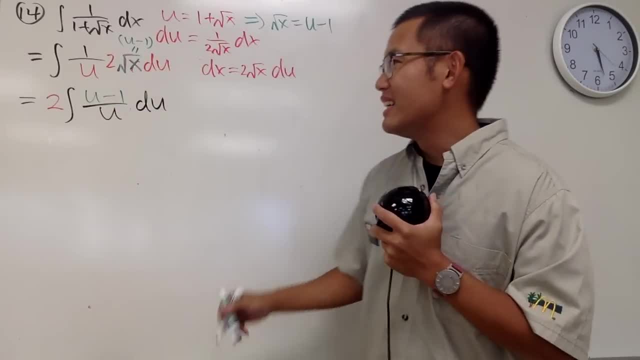 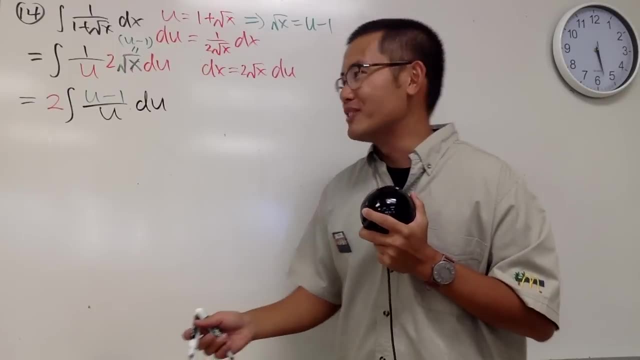 And to do that we actually have to split the fraction right. So you always refer back to the first couple categories of the integration techniques that we have mentioned so far. Anyway, here we have the following, The two states, and let's break down this as: 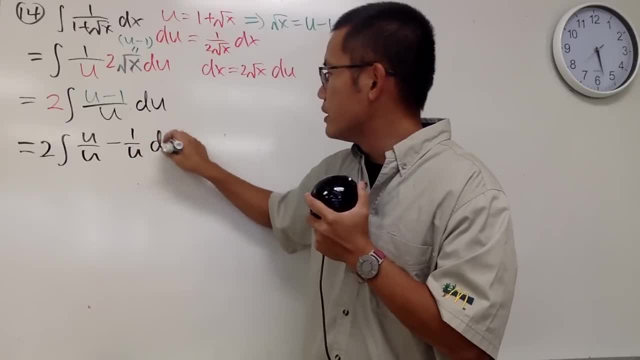 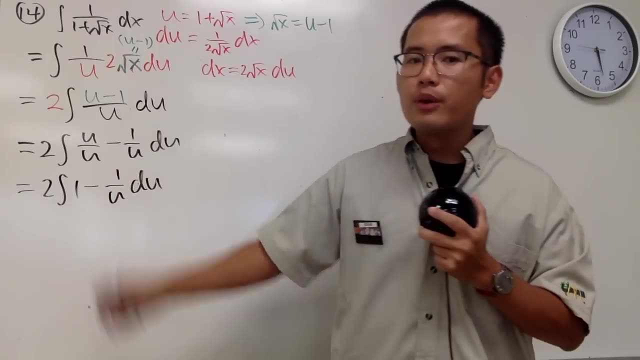 u over u minus 1 over u du, And, of course, this is just to integral. u over u is 1 minus 1 over u du, And we can finally integrate. Keep in mind, though, we are in the? u world, So this is going to be the following. 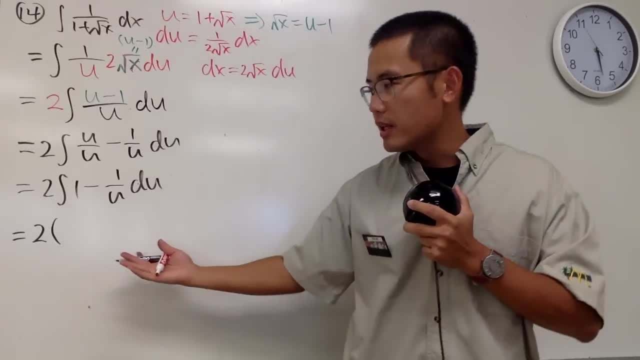 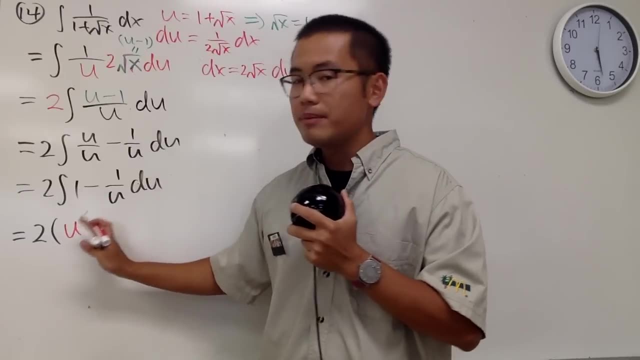 I will put down two parentheses, because I want to put down the result of the integration right here. Integrating 1 in the? u world, we get u. Let me just write it down right here. And then we have the minus and integrating 1 over u. 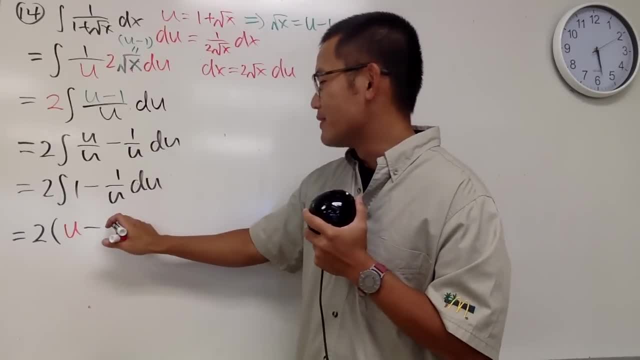 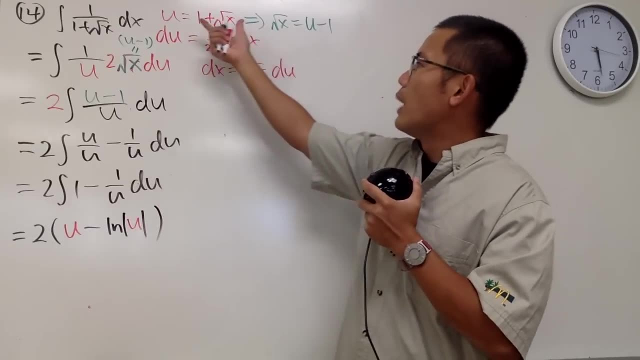 we get natural log of u with the absolute value, Like this Right, And in the end, of course, we can just put our choice for the u back here so we can get back to the x world. In the meantime, perhaps let's also distribute the two. 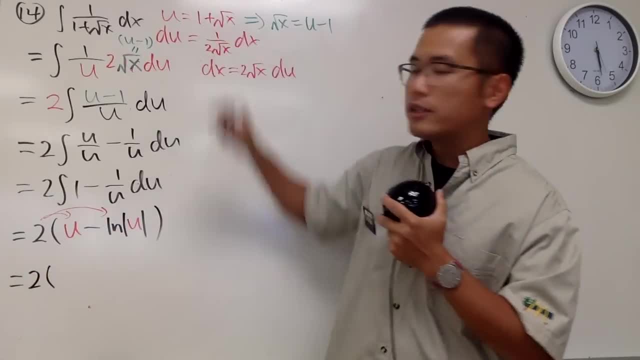 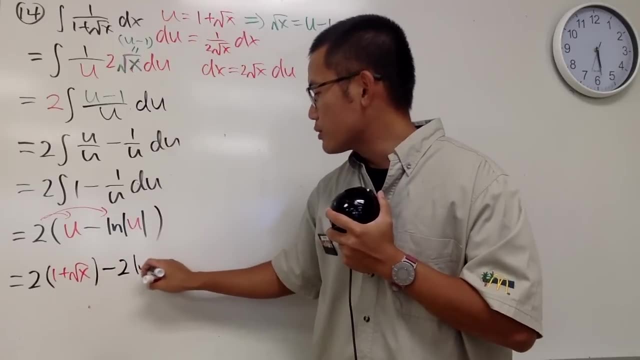 So finally we see we have 2 times: u is 1 plus square root of x, So we have this right here, And then 2 times that, So it's minus 2, natural log: u is 1 plus square root of x. 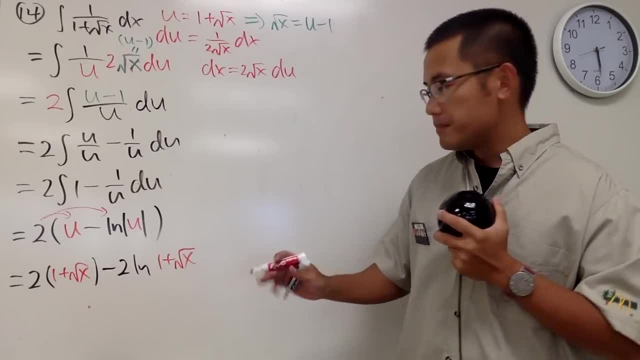 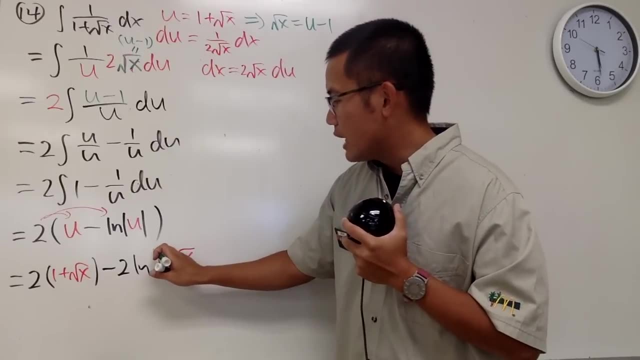 But notice square root of x, the output is not negative And in fact when you plus 1, this is actually always positive. So we don't need the absolute value. Parentheses is just okay, And in the end perhaps you can just distribute the two. 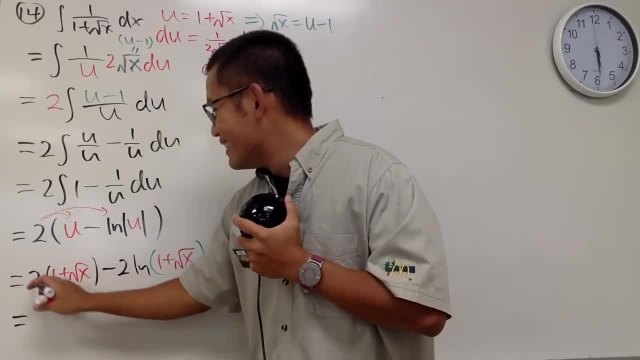 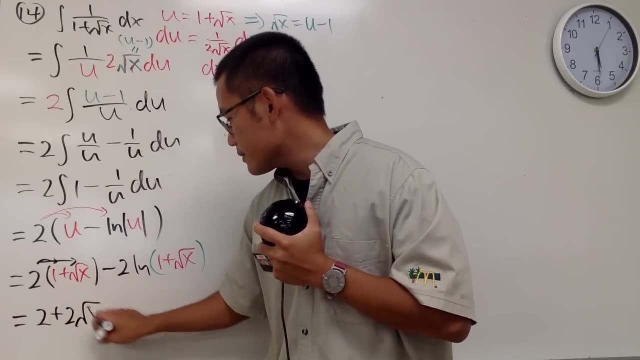 It's up to you, And if you don't, it's probably okay. Anyway, I'll just distribute real quick like this: So 2 times and 2 times square root of x And minus 2, natural log parentheses, 1 plus square root of x. 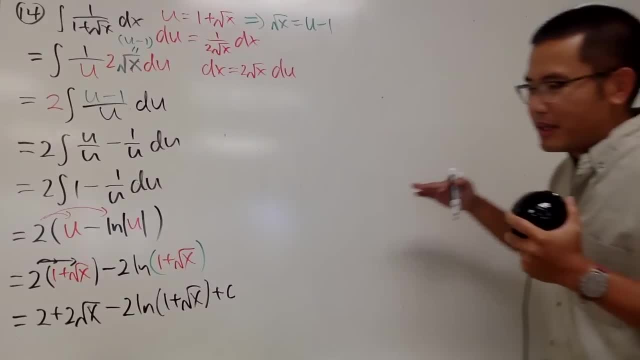 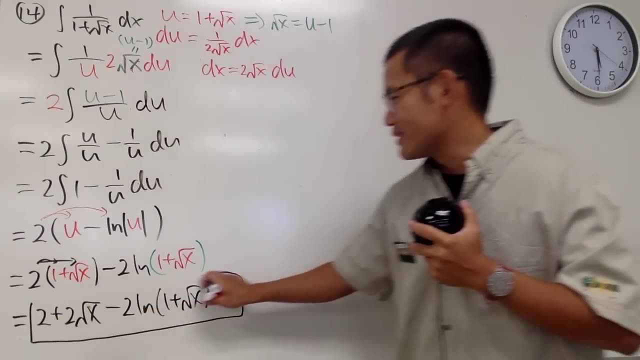 By the way, I should have said that x to the fourth power is always non-negative. It's never negative because it can be 0. I forgot to say that, but it doesn't really matter, Just the parentheses versus the absolute value. 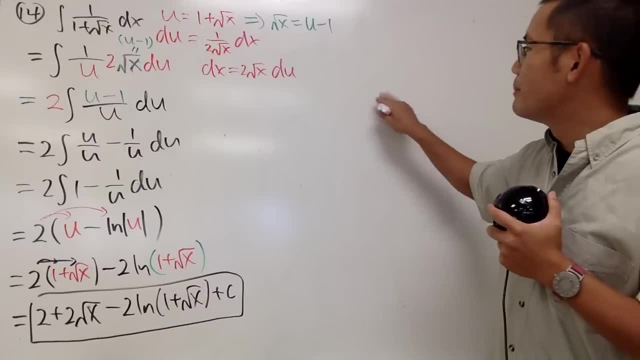 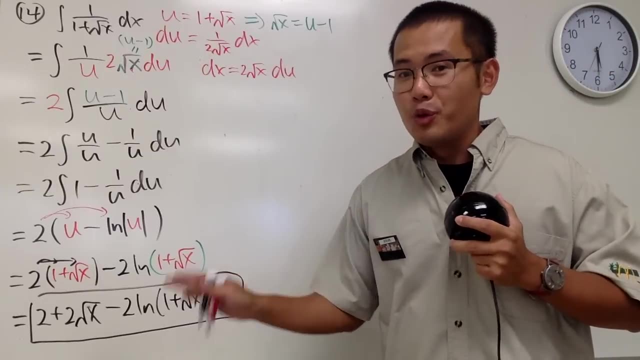 Anyway, in this case, this is it. So that's question number 14 for this. Okay, so seriously, we're done with the USAP. And now, actually, we're not done with the USAP. USAP will be going with us forever. 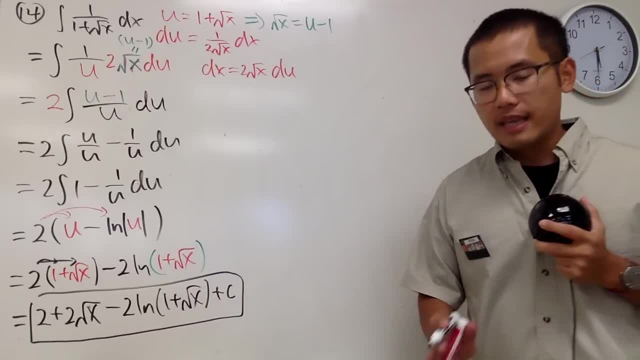 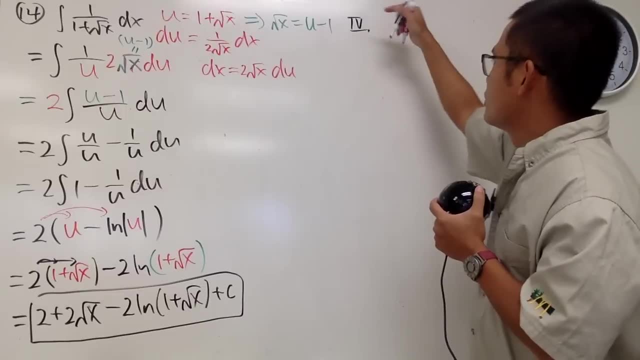 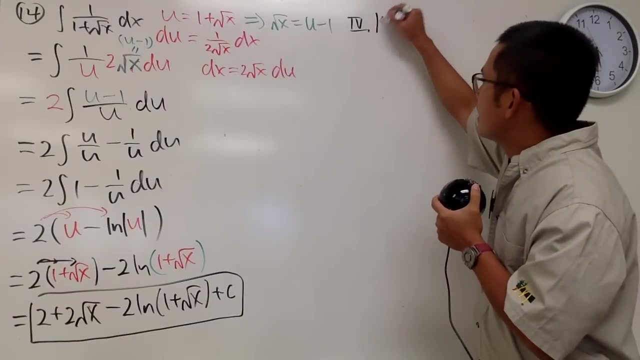 You'll see why. Now let's go to the next category. Here is category number 4.. I almost wanted to say number 5, but like this is my number 4, right? Well, for this particular one, I will title this as: 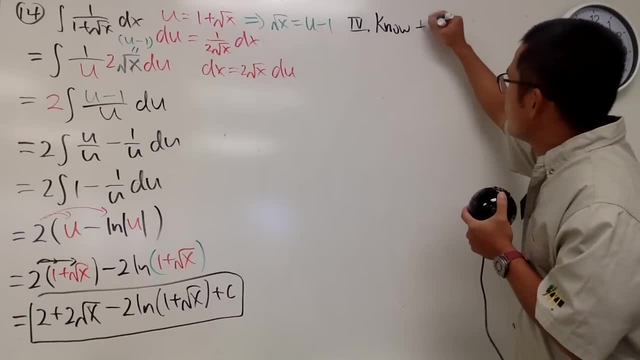 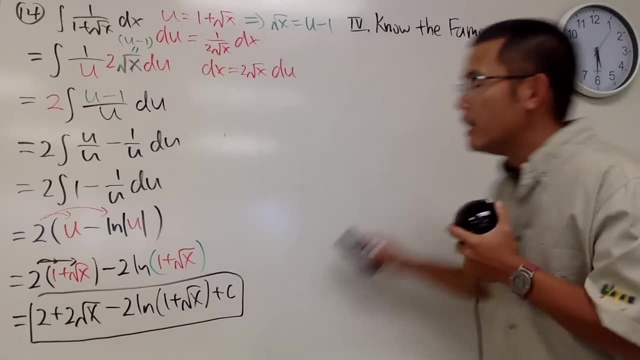 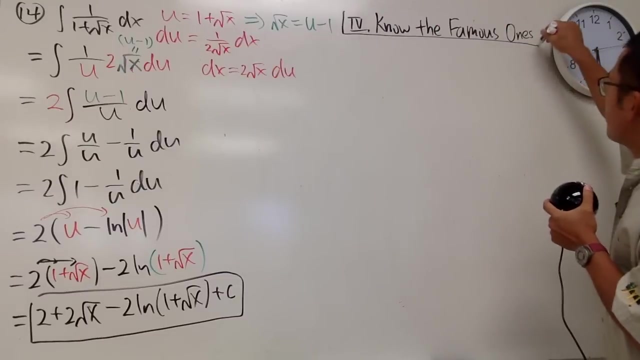 you are going to know some famous one. I'll just say know the famous ones. And I will explain what I mean by know the famous ones right here. This right here is technically part 1.. Right, So here is just a part 1 situation, the first part. 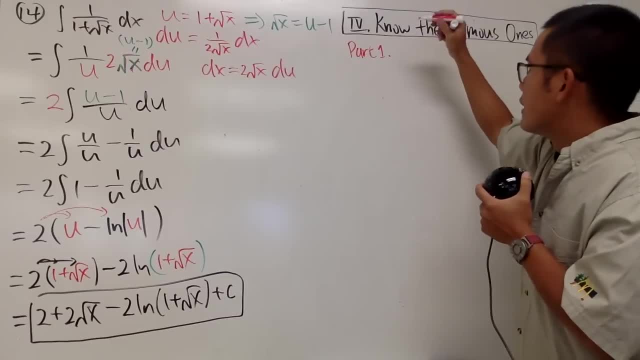 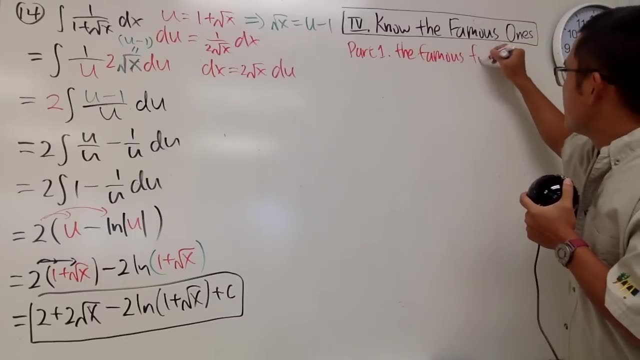 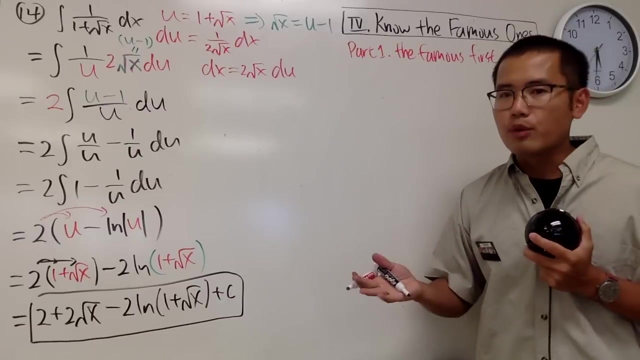 And this actually includes a lot, But part 1 just says that the famous. I'll just put down The famous first step. And this is extremely crucial because, of course, whenever we're solving a math question, usually the hardest step is the hardest part. 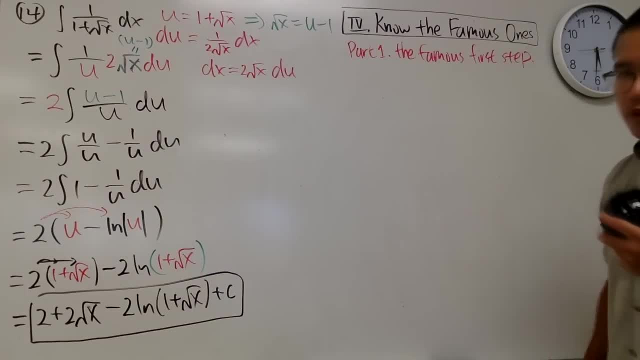 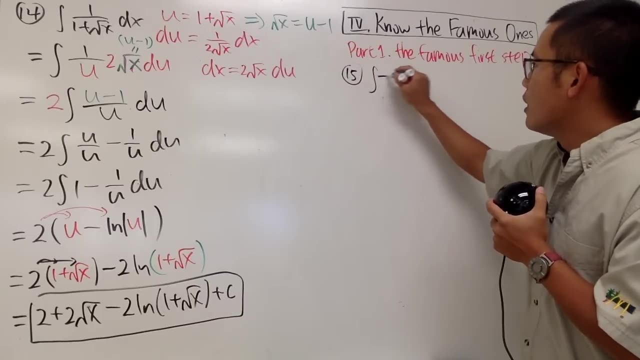 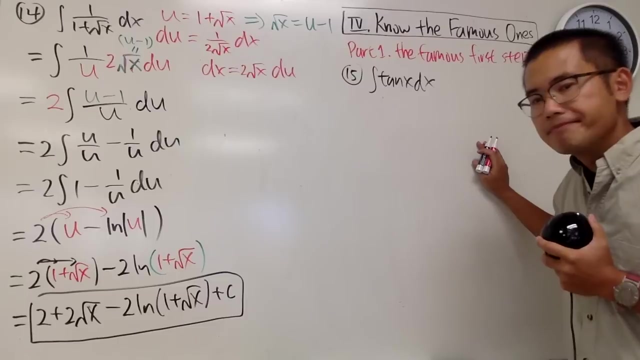 Yeah, so know, the famous first step, And I'm going to give you guys three examples right here. Let's look at next one, which is question number 15.. Let's look at the integral of tangent x, dx. Well, if you look at the integral of tangent x, we don't have a lot to work with. 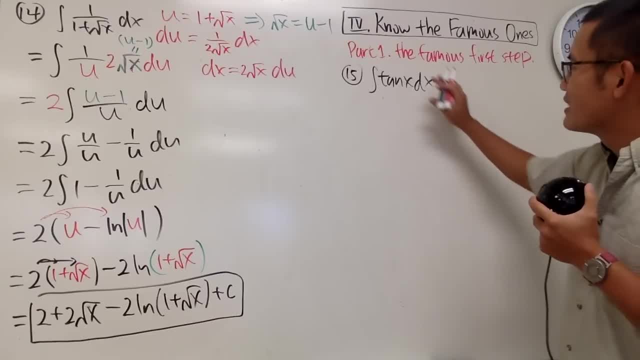 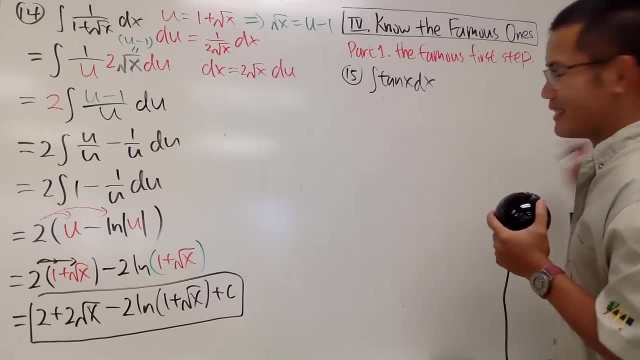 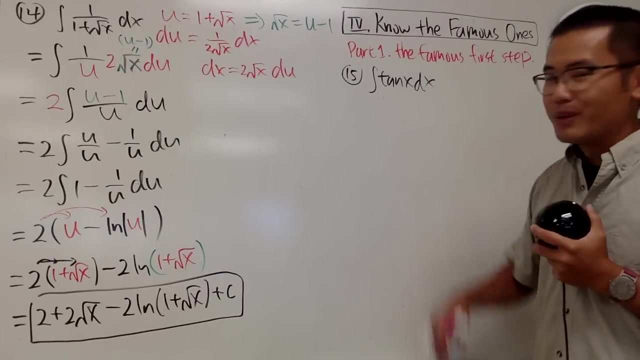 One way to do this is we can write it as sine x over cosine x, And then we can do some USAP Z? u equal to cosine. I'm going to work that out later, But if you just look at this right here, here is a way that we can finish this. 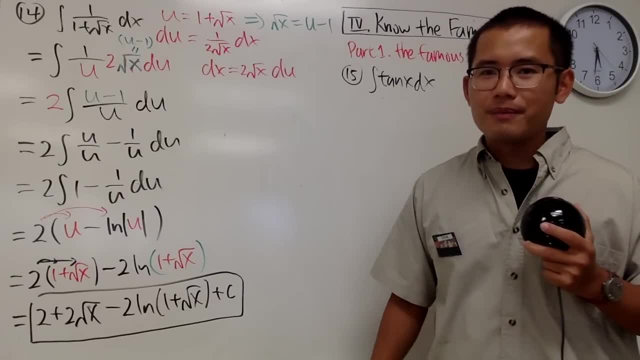 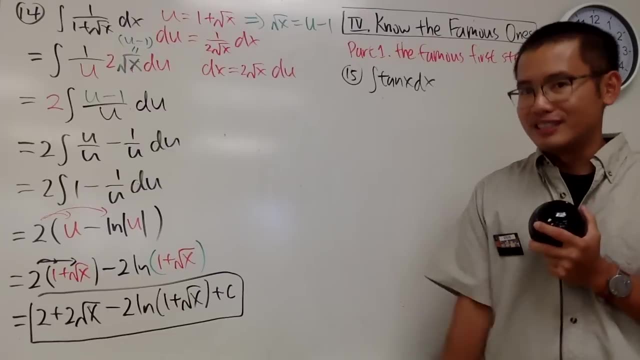 And this is another thing you have to keep in mind. Again, another storytelling: Whenever we're doing integrals, you have to keep in mind that tangent x and secant x, they are best friends. Again, keep in mind, as of integrals, tangent x and secant x, they are best friends. 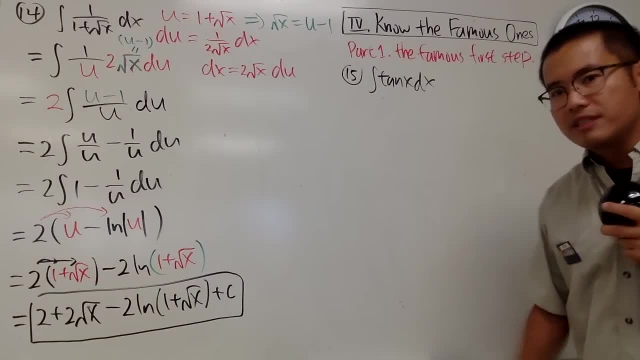 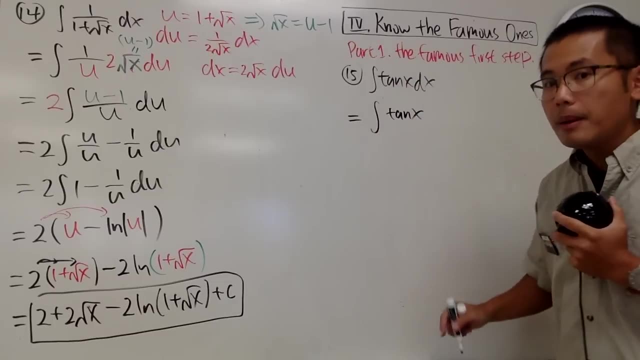 And in this case I only have tangent. Well, I want to have secant to help me out. And here is how you can do it. Let me just write down the integral and we have the tangent right here. But let me actually just multiply the top and bottom by secant x. 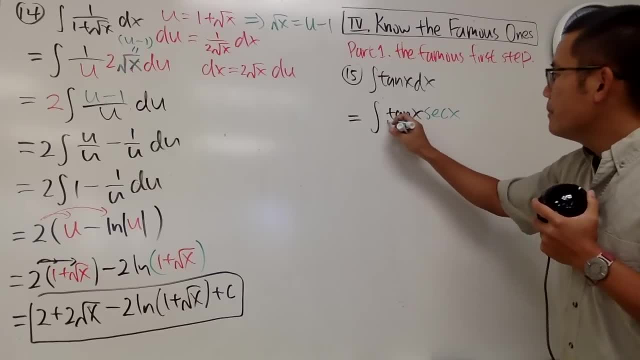 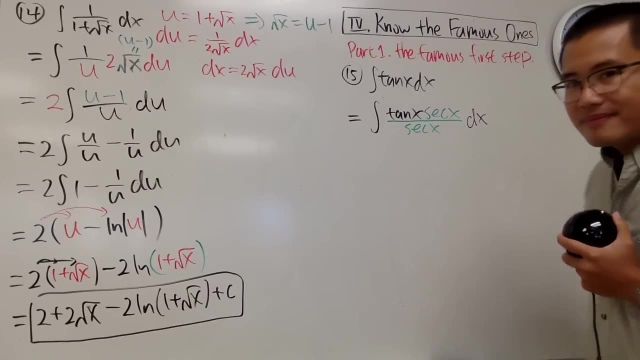 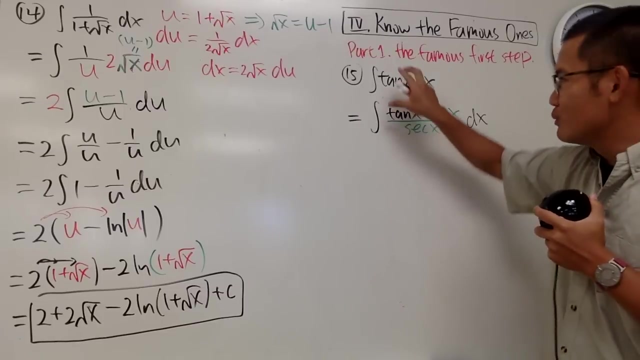 So let me just multiply secant x on the top. In the meantime let's also divide the secant x on the bottom And of course we still have the dx And notice this right here. didn't change anything because of course we're just multiplying by 1.. 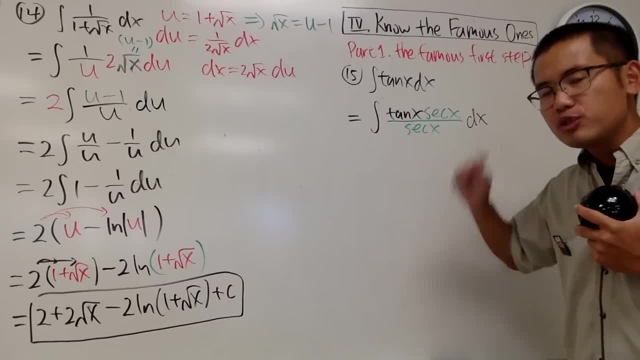 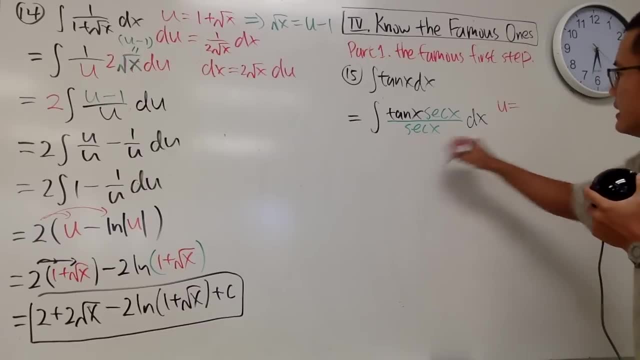 And this is still, of course, tangent x inside. But this is much more preferable because we can do a nice u-sub. now. In this case I will let u equal to secant x And differentiate both sides. we get du equals. the derivative of this is secant x, tangent x, dx, like that. 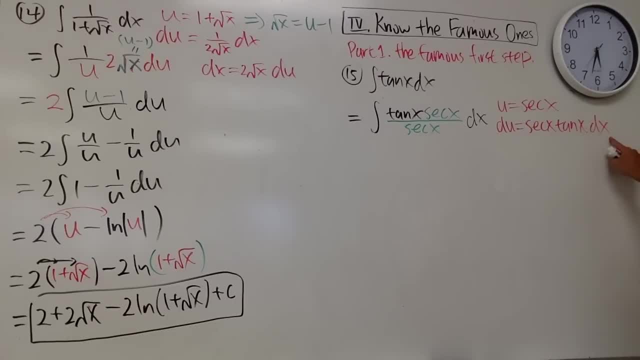 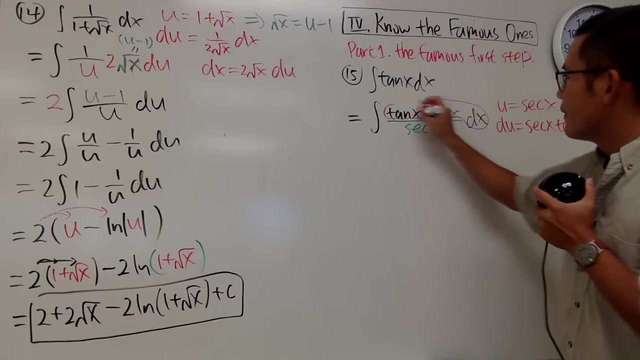 Notice the following: Secant x, tangent x, dx. That's exactly what we have right here. Of course, the order of multiplication doesn't matter. So you see that we have the tangent x times secant x times dx. All this right here is nicely equal to du. 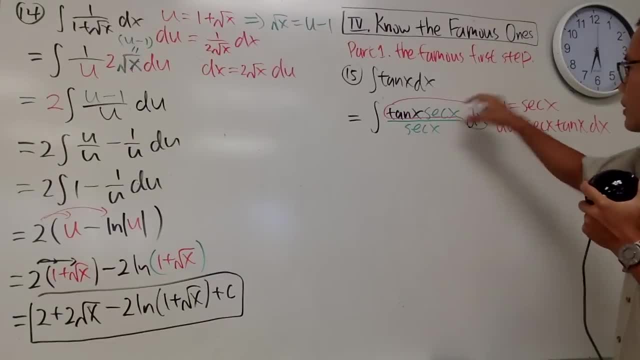 Whenever you can pair things up nicely, of course, you can just go ahead and replace that This right here is the du. I don't need to isolate the dx right. If you want to do that, of course you will just see this and that will cancel out. 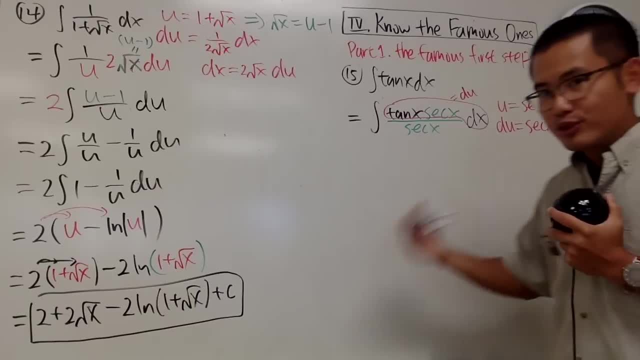 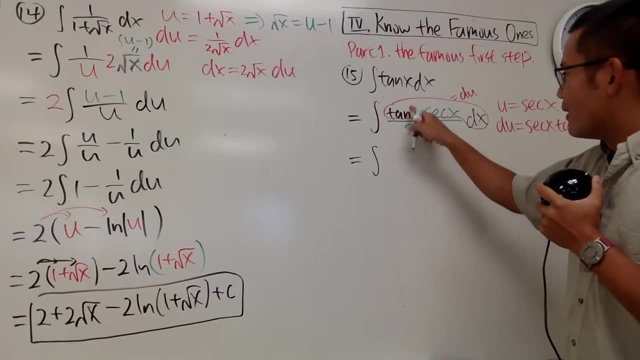 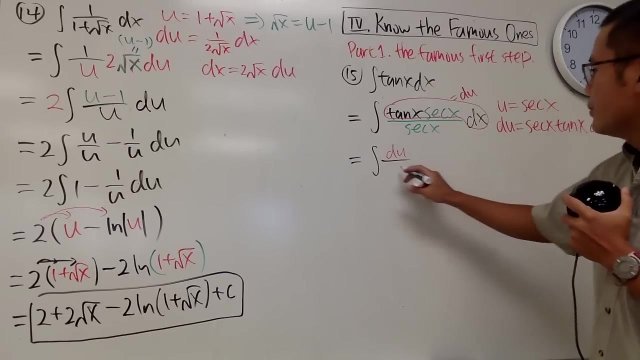 But whenever you have this being exactly the same, just go ahead and replace. That will be the ideal situation. Okay, here we have the integral. Now I will just put the du on the side, Because some people like to say du over secant x, which is our u. 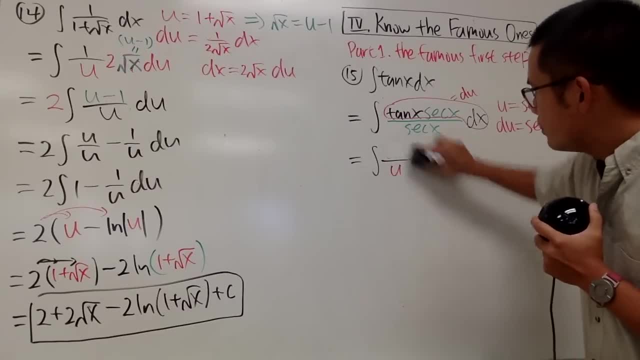 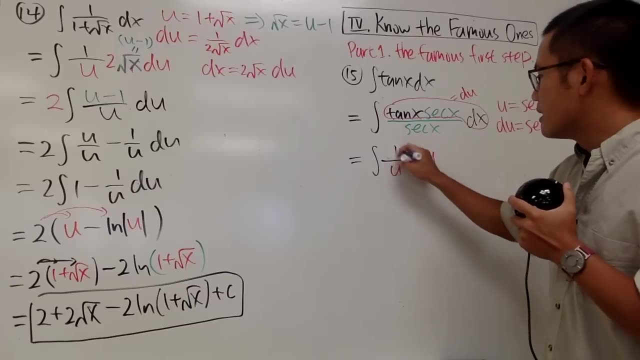 Some people like to write this, but I like to write it as du being on the side, Just for consistency purpose. du, whatever, always on the side. So, with that being said, the top is just a 1, right. 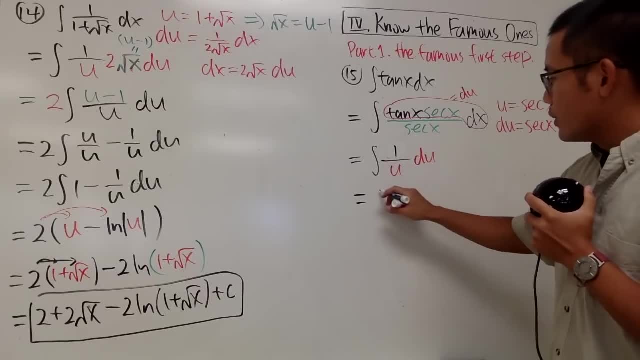 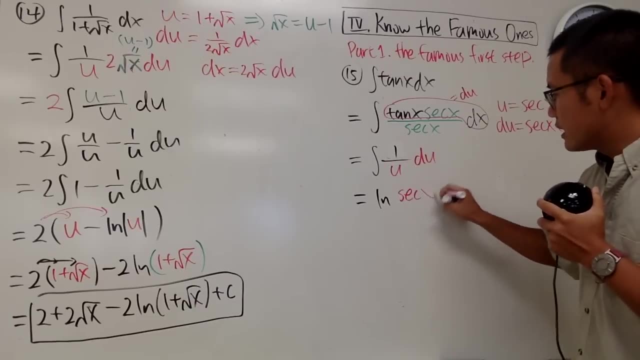 And of course in this case we can just integrate this In the? u world. we get natural log of u And u is secant x. So I will just put down the secant x right here. And secant x can be negative sometimes. 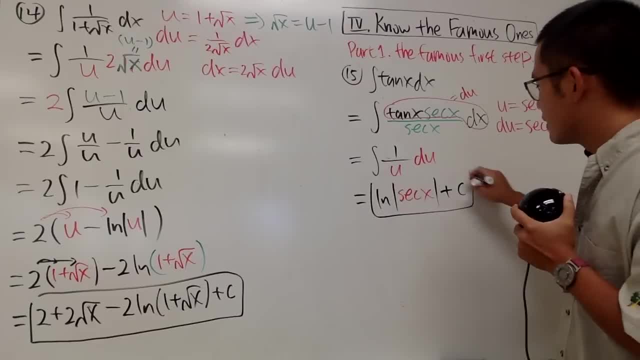 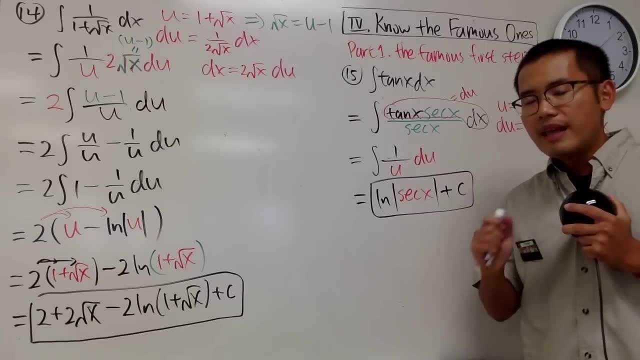 So we will have to have the absolute value, And we are done Right. So again, natural log of absolute value of u And u is secant x. This is it Now. this is what you have to remember. 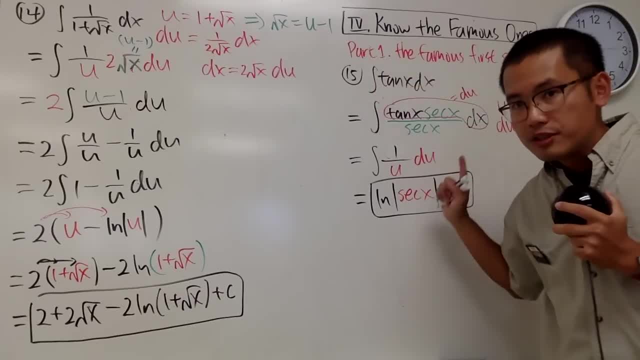 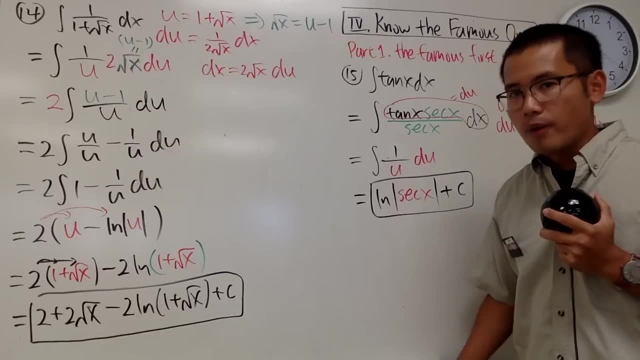 Later on, when we encounter the integral of tangent x, we are just going to write down natural log of absolute value of secant x, Because this right here is the standard result of this integral. So I am just going to have a notation right here. 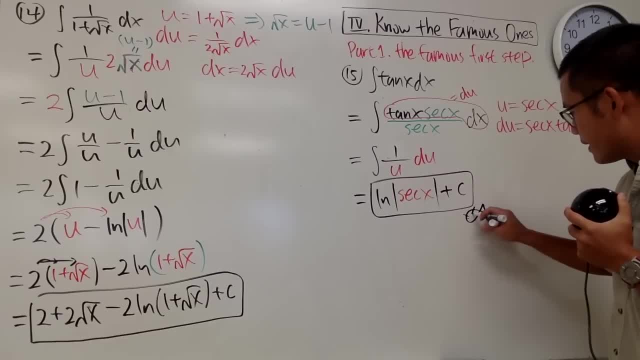 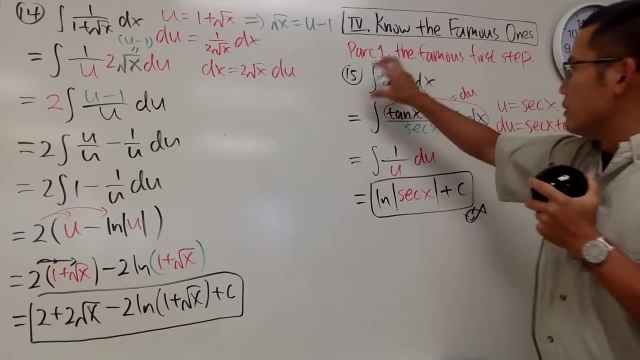 So perhaps I will just put down a little fish right here. You are going to remember this. Whenever I put down a fish, that means this is the standard result. You are just going to remember it So that you don't have to do this again. 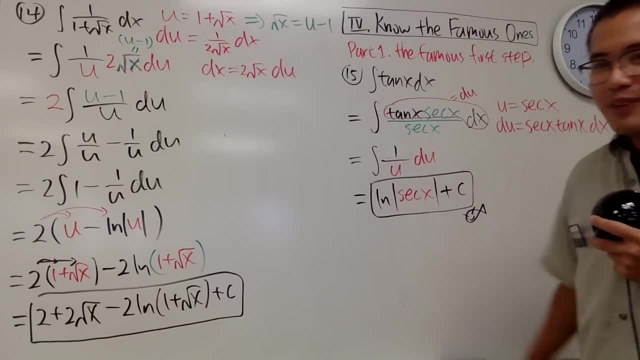 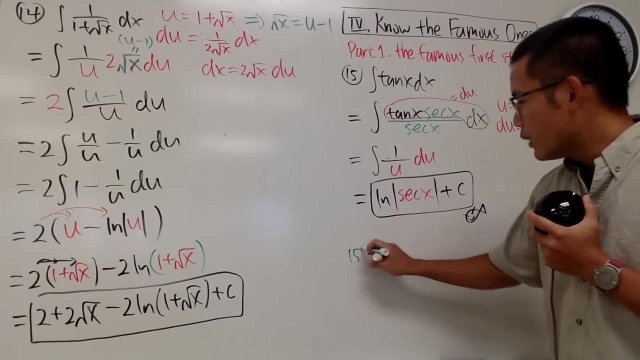 Unless the question is asking you: okay, please prove the formula right, Otherwise you can just go from here to here Because we encounter. so this is actually okay, So this is how we can do it. And again, if you want to look at how the other way is done, 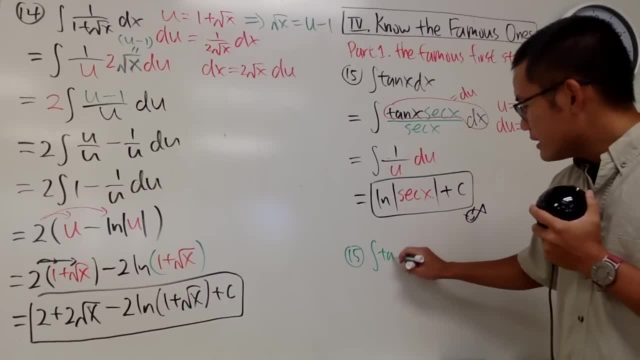 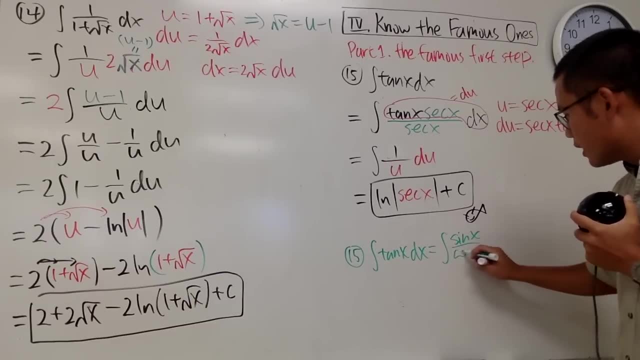 let's just put this down in green: Integral tangent x. Well, as we mentioned earlier, tangent is sine over cosine, So this is sine x over cosine x. In this case, we can also do a u sub, Let u equal to cosine x. 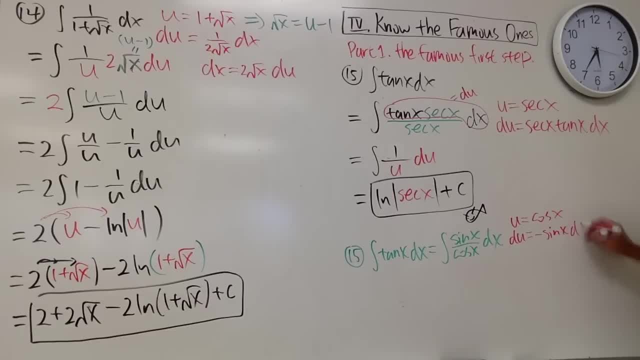 And du is negative sine dx. Well, in this case, let me isolate the dx, because I will show you guys, the sine of x will cancel out, but we have a negative sine right here, So dx equals this on the other side, 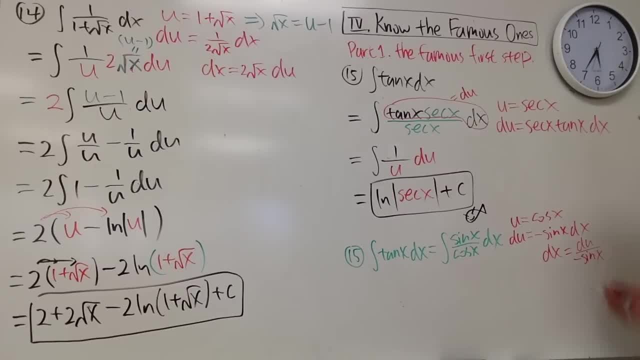 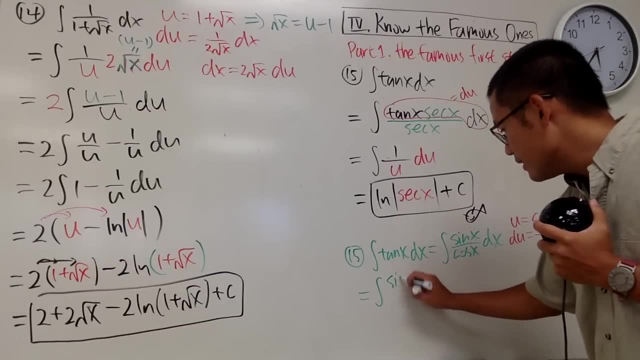 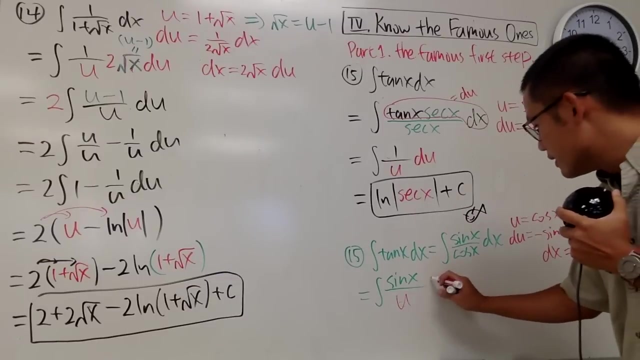 So we have du over negative sine x. Now take this integral to the u world. We get. the integral On the top is positive sine x, over the bottom is u And the dx is all this. So which is du over negative sine x? 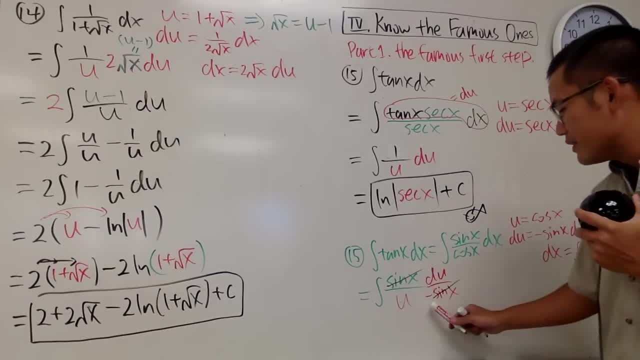 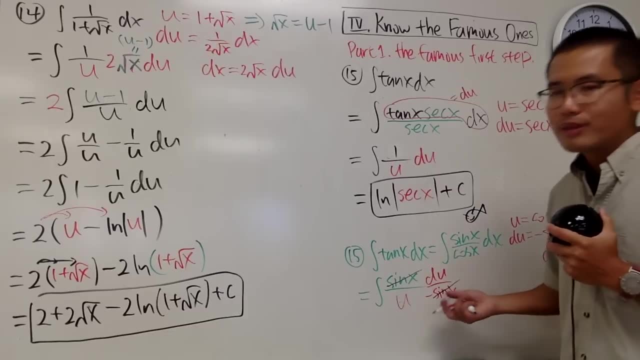 And now the sine x, sine x cancel. but we do have the extra negative sine. Earlier, you could have put down negative sine right here and then multiply by negative. Well, that's okay too, after you have wanted to do it. 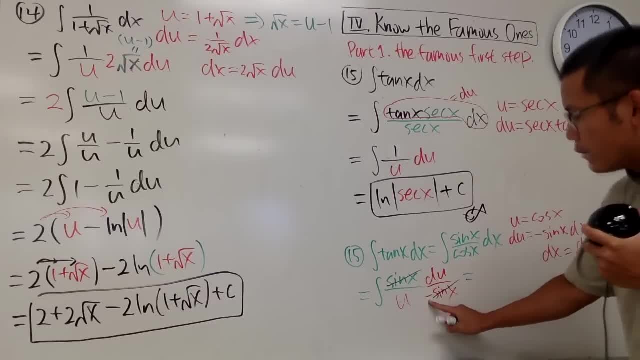 Anyway, in this case we have negative and we can put the negative in the front. So we have a negative integral and this is 1 over u. du Well notice, in this case, our choice for u is cosine x. Then do this one carefully. 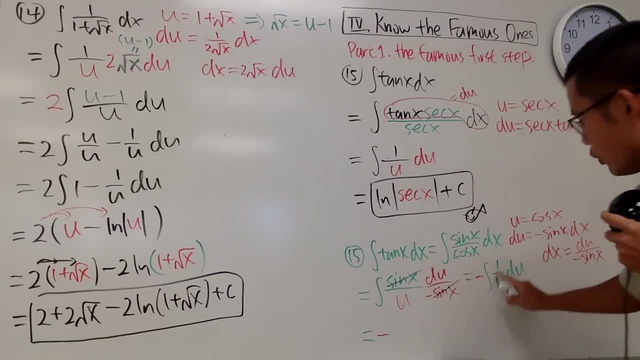 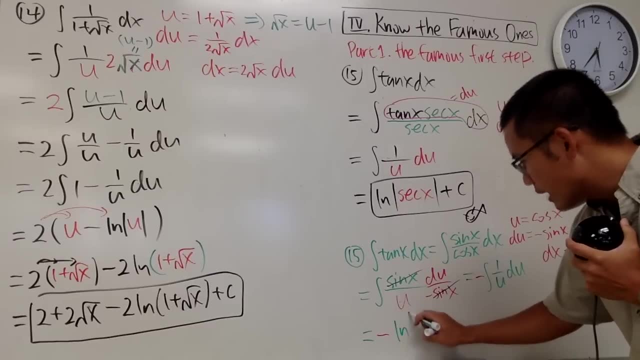 Here we have this negative right here. And then the integral of 1 over u is natural log absolute value of u, which is cosine x. So we have natural log absolute value of u for the cosine x, right here, Right. 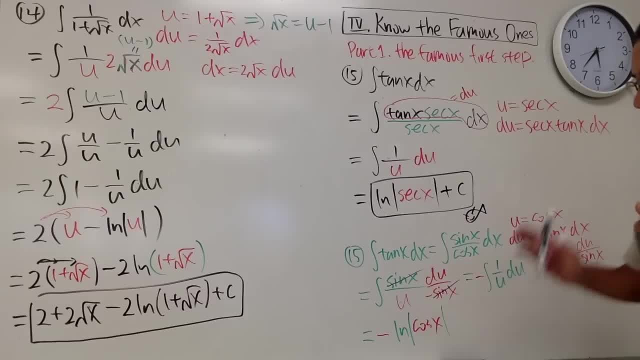 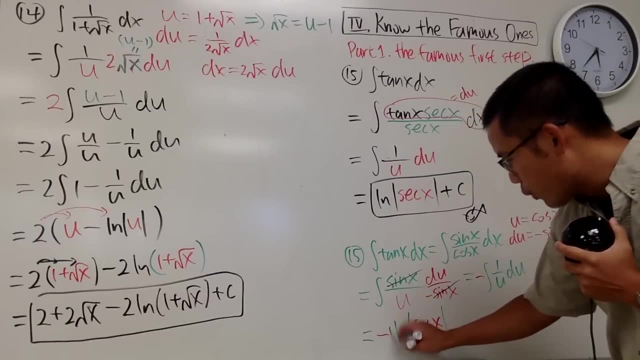 And of course you can put down a plus here, but not yet Notice this and that looks different, But in fact they are the same Because we happen to have a negative 1 in the front of a natural log. 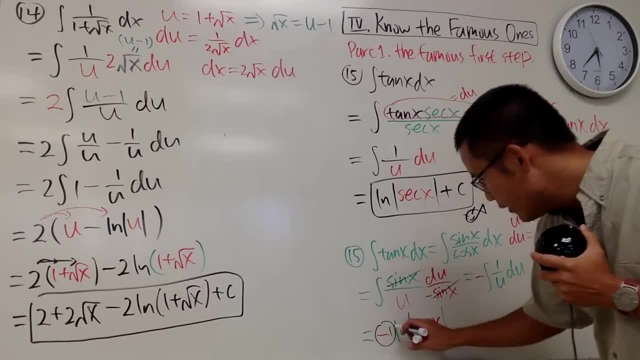 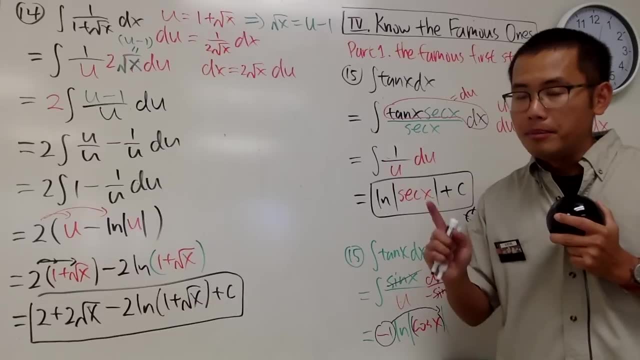 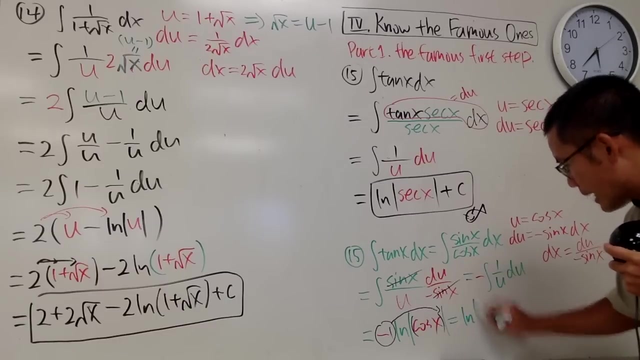 So we can use the log property. We can put the negative 1 to here And notice this is cosine x raised to a negative 1 power. It means 1 over cosine. So in this particular case we actually have natural log absolute value of cosine x to the negative 1.. 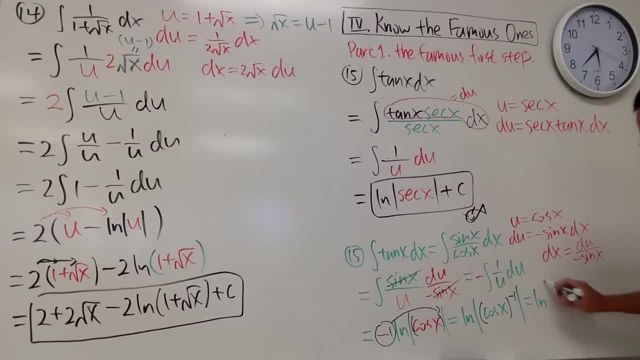 And this is equal to- Let me see if I have enough space- This is equal to 1 over cosine x, which is secant x inside. So we have natural log absolute value of secant x inside. So of course this is the same as that. now, 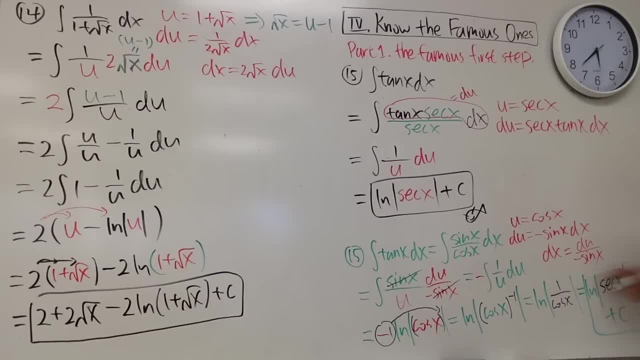 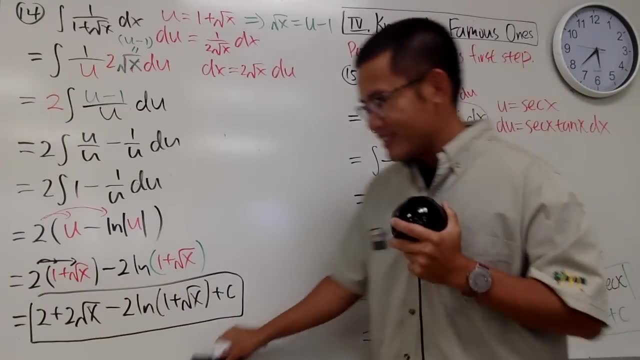 And I'll put down a plus here, right here. So, yeah, everything fit in that little place. Okay, we're done for that. So still pretty good, still pretty good, All right. so this is for the tangent x. 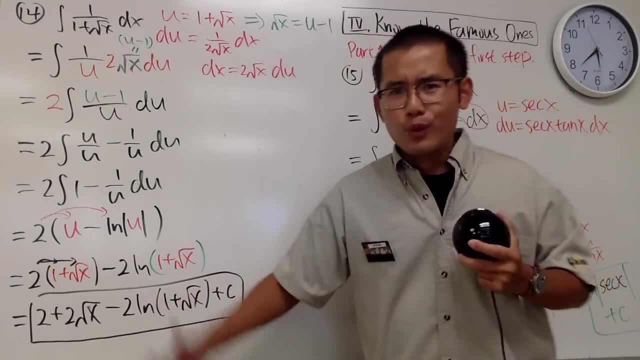 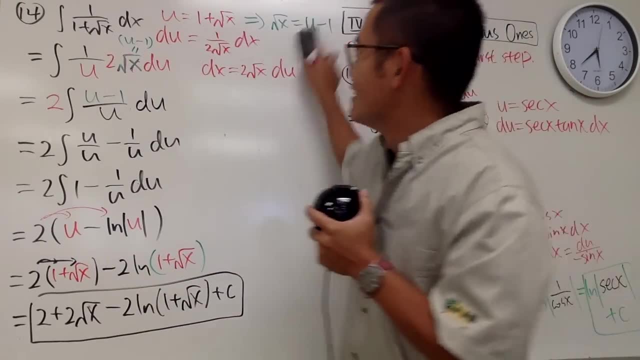 Now we integrate the tangent Man, who's the best friend of tangent Secant. right, Secant said: hey, integrate me, integrate me, We will integrate secant. So of course, that's what we'll do next. 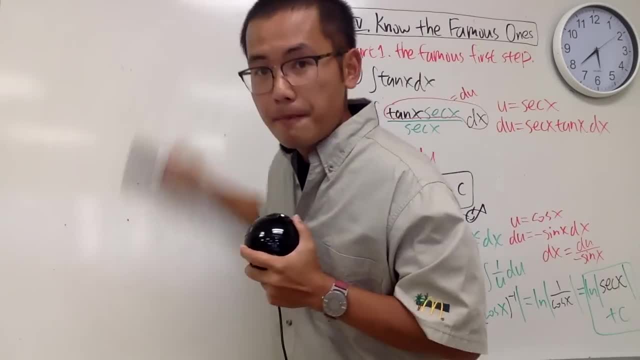 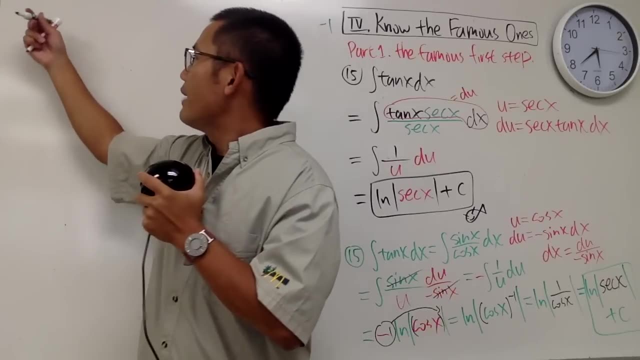 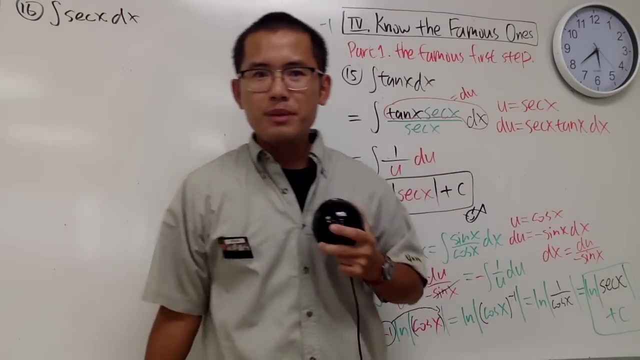 And I'm not going to erase this part yet, Let's just take a look right here. So here we have number 16.. Again, integral of secant x, dx: Integrate me, integrate me. Well, in this case, notice that secant x is just 1 over cosine. 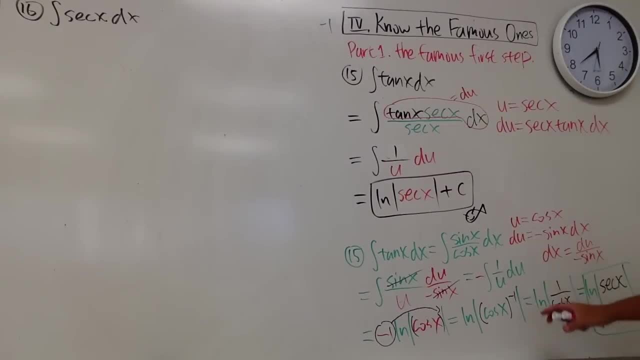 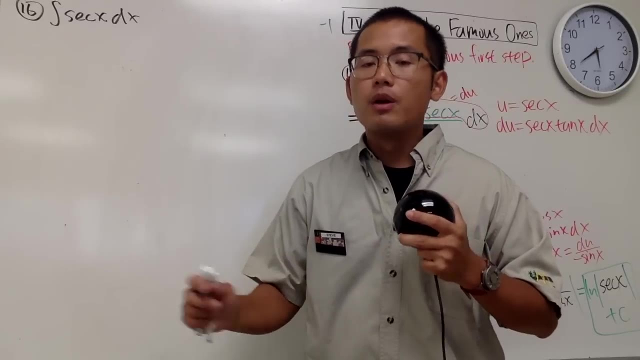 If you rewrite this as 1 over cosine, unfortunately we don't have the sign on the top. We don't have the sign on the top to help us out. In integrals, tangent and secant are best friends, Or sine and cosine are best friends, right. 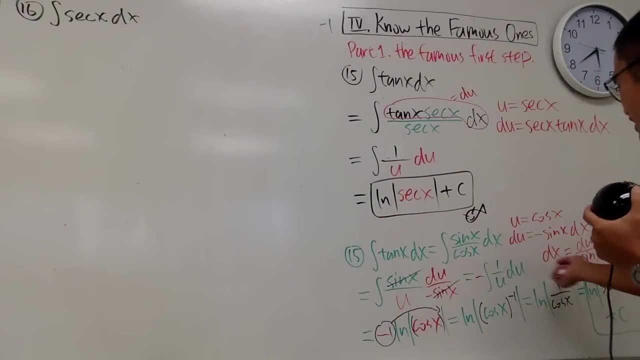 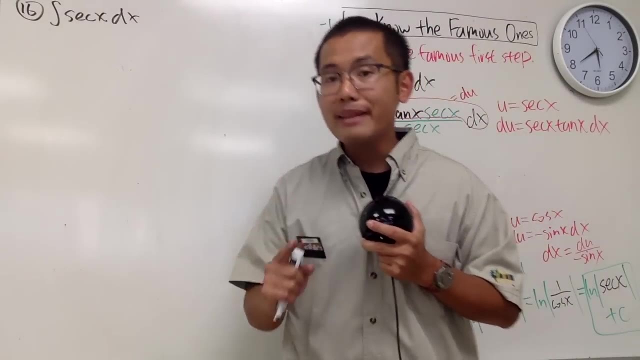 So, one way or the other, Tangent x works out really nicely for this, But secant x if you write it as 1 over cosine. not so much, Although it's still possible, But again in this category. 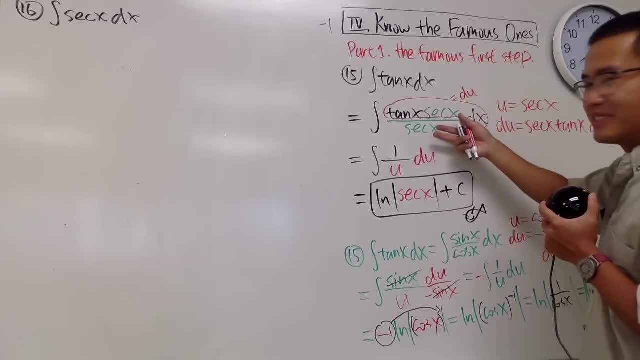 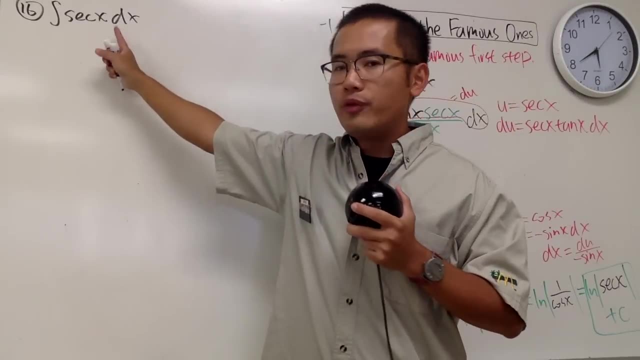 I'm going to show you guys the famous first step, Just like this, right here Now. it worked out really nicely if you write this right here slightly longer right Now. the secret for this question is that you have to. let me tell you what the secret is. 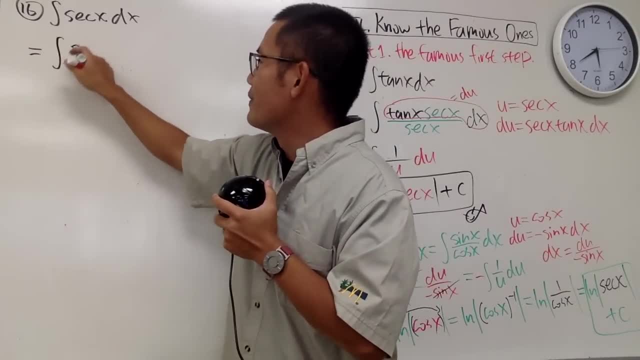 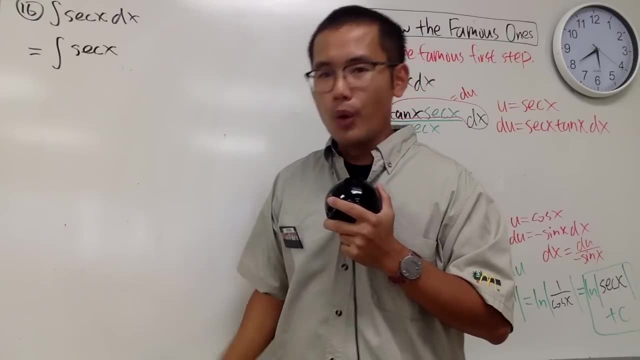 And this is the secret. Here is the deal. Let's look at the integral of secant x. And you might be wondering: do I just multiply the top and bottom by tangent x? Well, no, Because the derivative of tangent x is secant squared x. 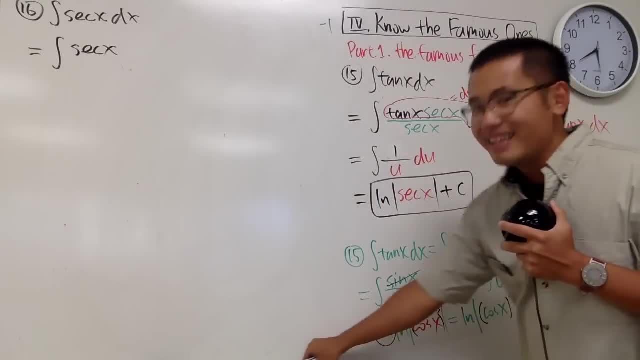 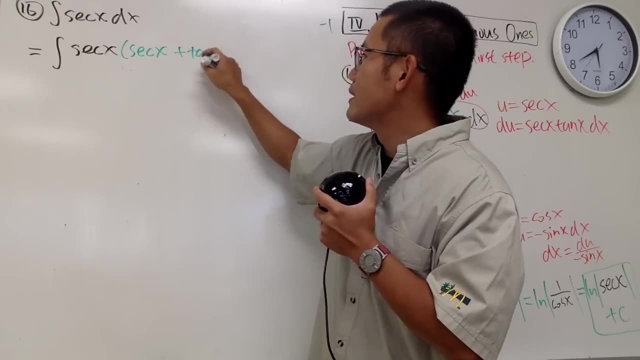 Here is the secret: We are actually going to multiply the top and bottom by secant x plus tangent x, And then, of course- don't forget- on the bottom as well. So let me write it down right here for you guys. 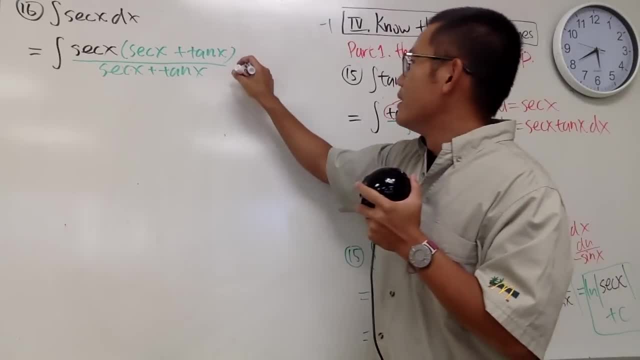 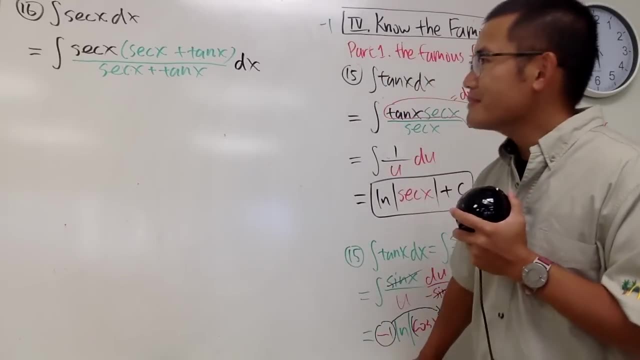 And I know what you guys are thinking. okay, Just hold up your questions. okay, Let me put down the dx. Let me just show you this actually works first And I will address your issue. Well, let's see if this works out nicely or not. 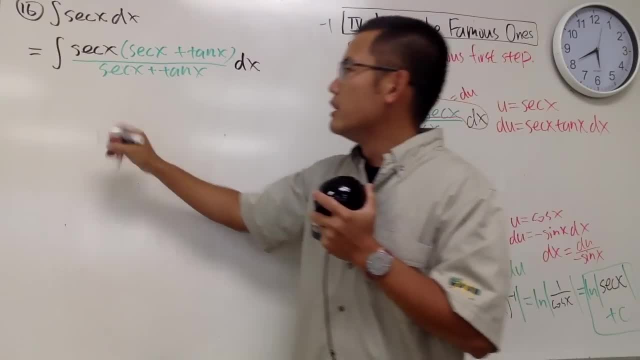 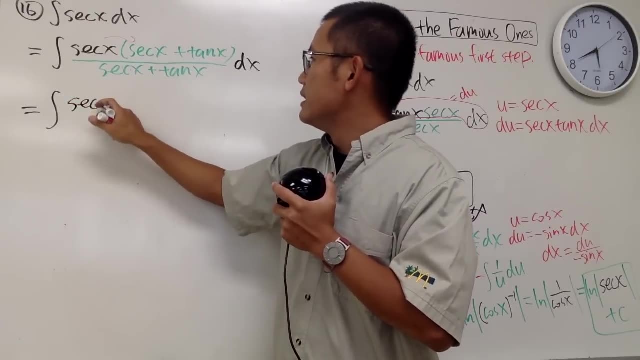 First of all, of course, on the top we can just multiply this out. So on the top we get the integral here, And this times that is just secant squared x, And then plus, and this times that is of course. 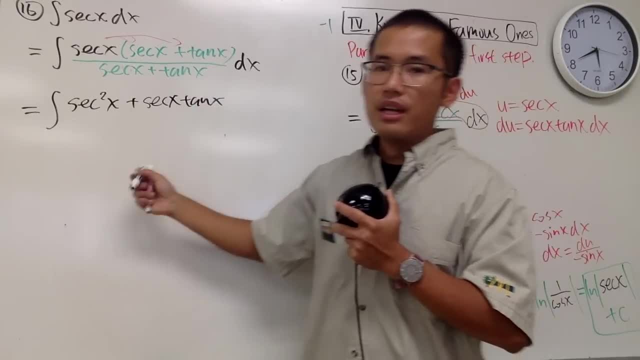 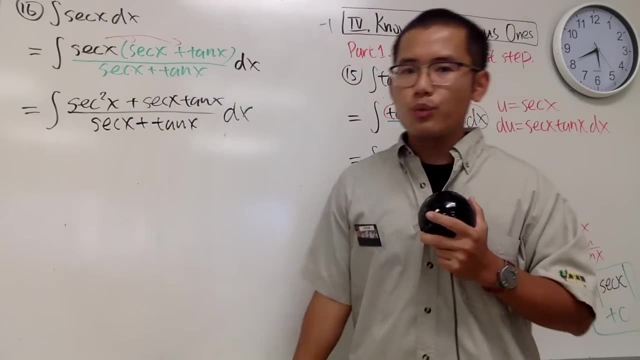 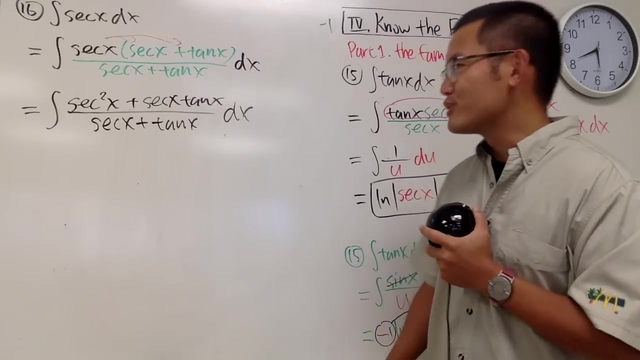 secant x times tangent x, That's good, And then over the denominator, which is secant x plus tangent x, dx, And that works out really wonderfully, of course. Now, why is this so much better? Yes, because we can do a u-sub. 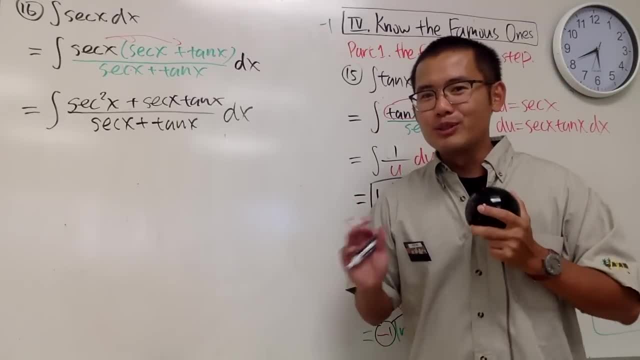 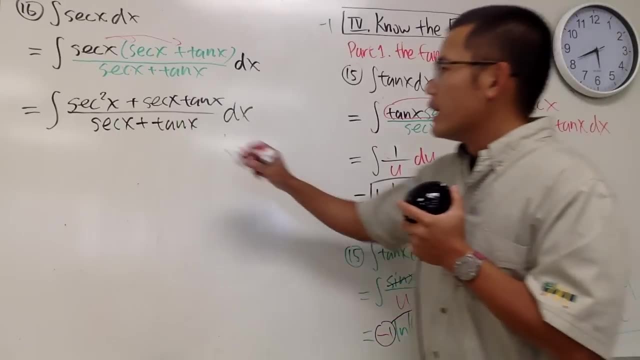 You see, u-sub is perhaps the most used technique in integrations, So get used to the u-sub. And of course, you have to know your derivatives really, really well. Well, here we are going to let u equal to the denominator. 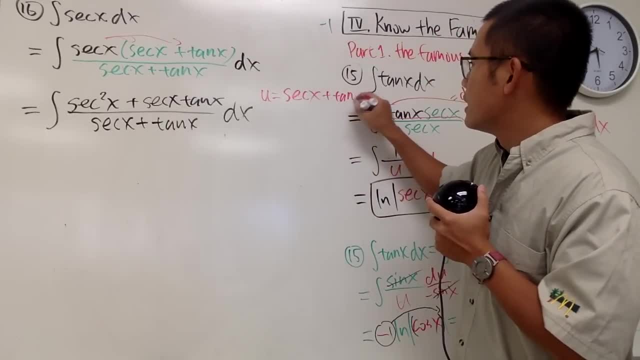 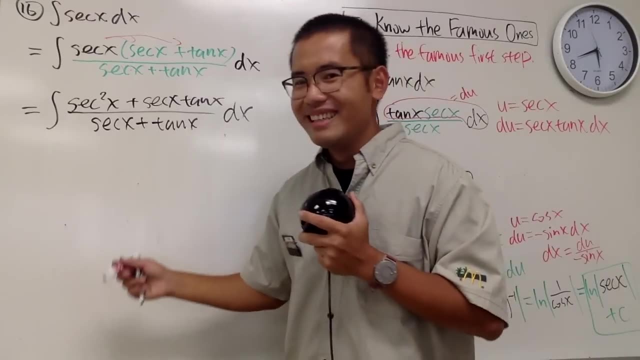 So let me just write this down: We have secant x plus tangent x, right? And let me actually just put it down here, because I know I don't have enough steps. Anyway, let u equal to secant x plus tangent x. 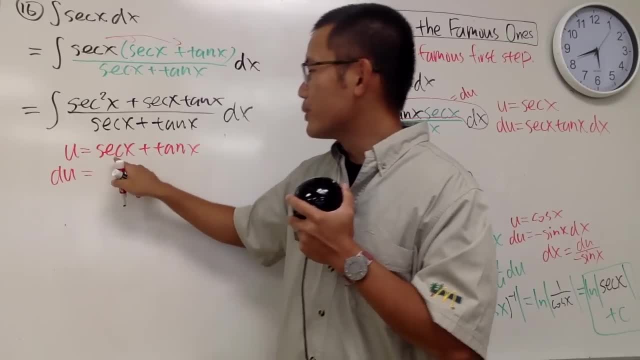 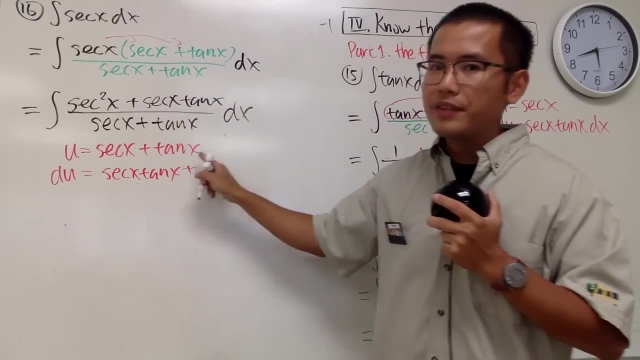 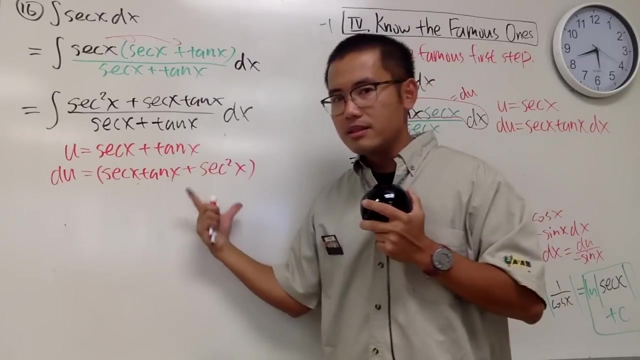 And we will differentiate both sides. du is equal to the derivative of secant, which is secant x times tangent x plus the derivative of tangent is secant squared x Parentheses. the whole thing right, Because this is the derivative from here. 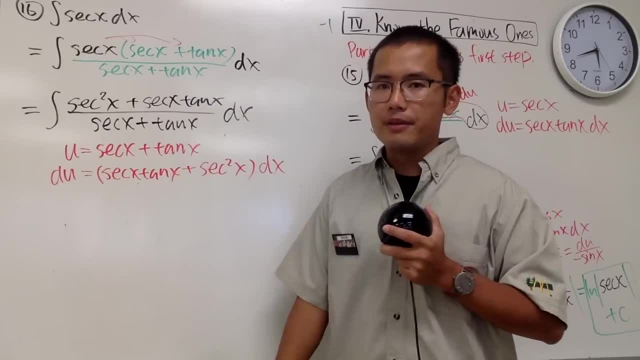 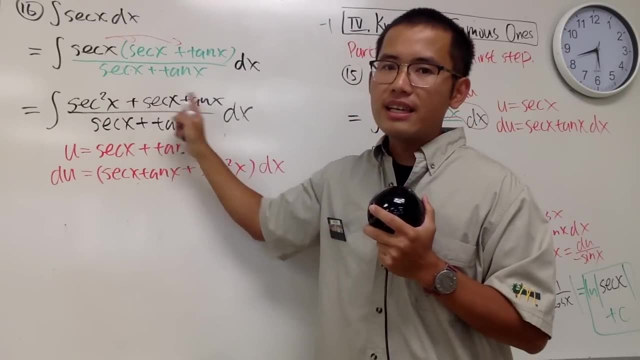 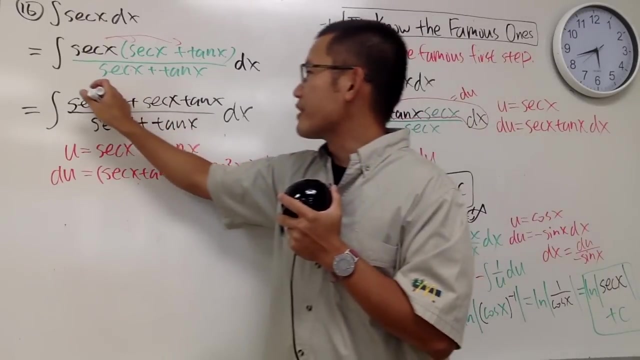 and then we have the dx. And now does this look familiar? We have the dx and we have the secant squared x plus secant x times tangent x. Again, of course, the order of addition doesn't matter, So in other words, the top right here. 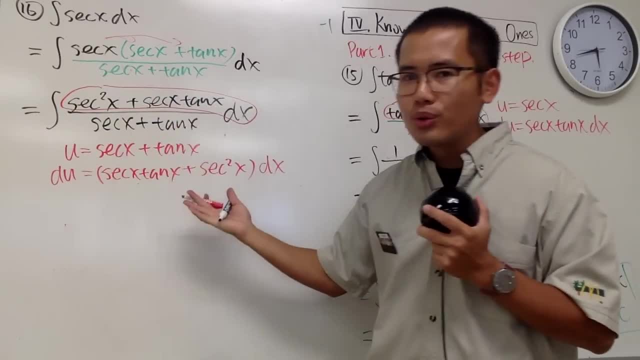 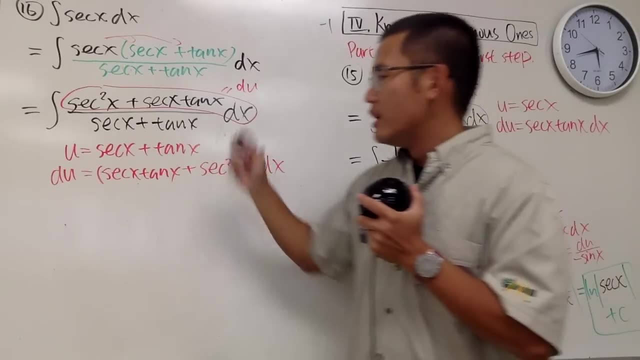 the whole thing. this is nicely equal to just the du And of course the bottom is the u, so we can actually go to the u-world. So we see that this is the integral. I will put down the du on the side. 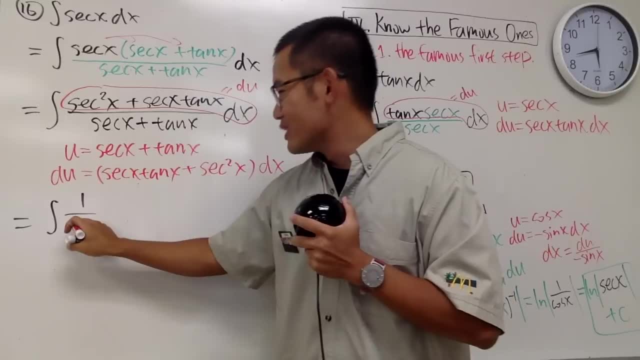 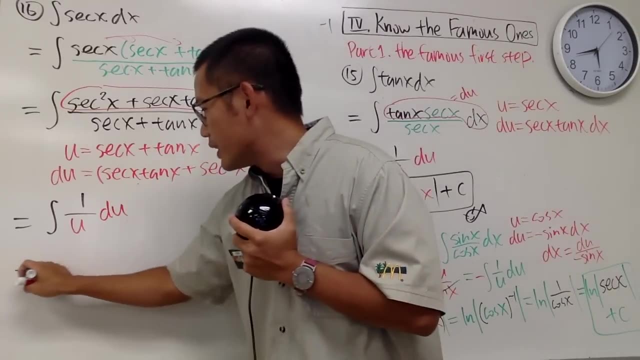 and we have 1 over. this is the u, so 1 over u, and then the whole thing here is just the du. So in the end you see that we get the integral of 1 over u, which is natural log. absolute value of u. 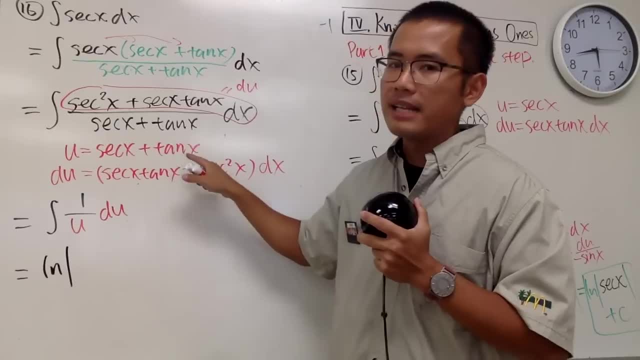 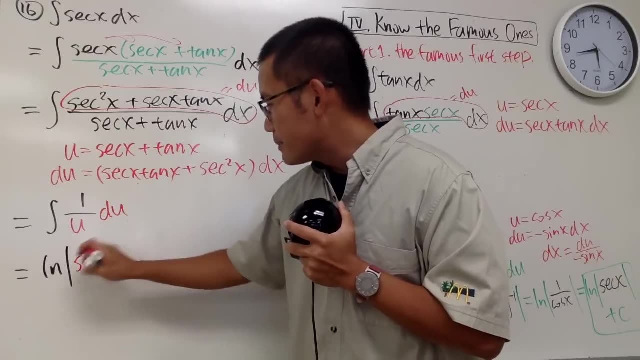 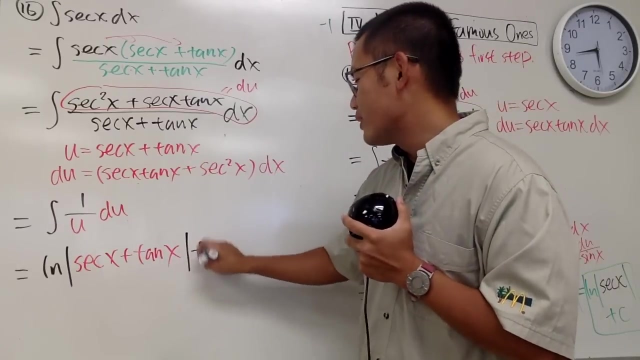 natural log absolute value. The u is this plus that, and this might end up to be negative. so we just write it down in the absolute value. So we have the absolute value of secant x plus tangent x, like this, And then in the end we put down the plus c. 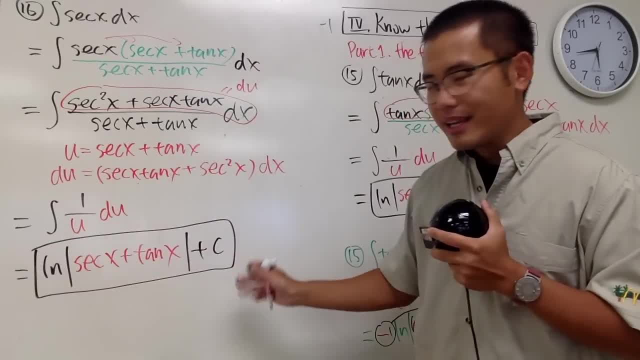 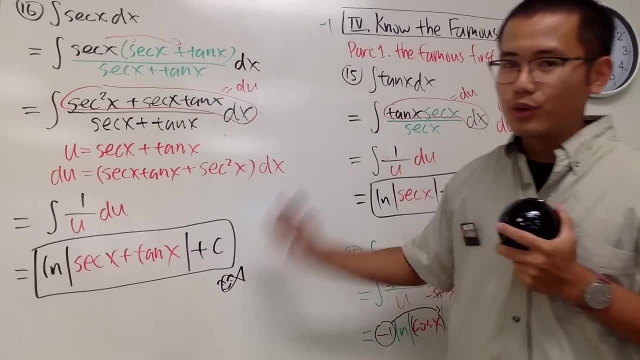 This is it. And again, this is actually a standard result, so you are going to remember this. so I will just put down a fish right here for you guys. So remember this result, right? Okay, I know you guys really wanted to ask me. 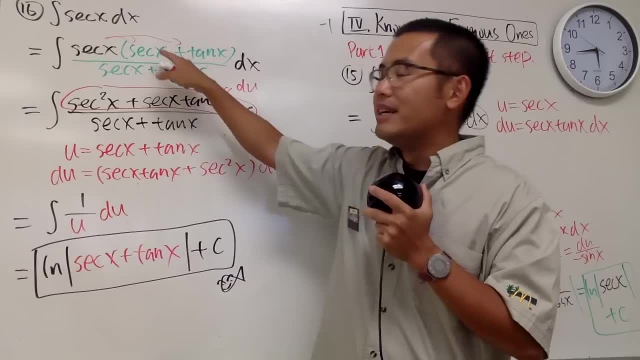 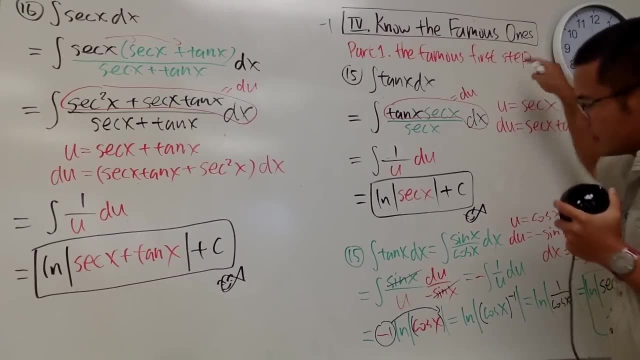 how in the world do I know to multiply the top and bottom by secant x plus tangent x. Well again, what's this category? The famous first step. This, right here, is a famous step that I will tell you, so you will know it. 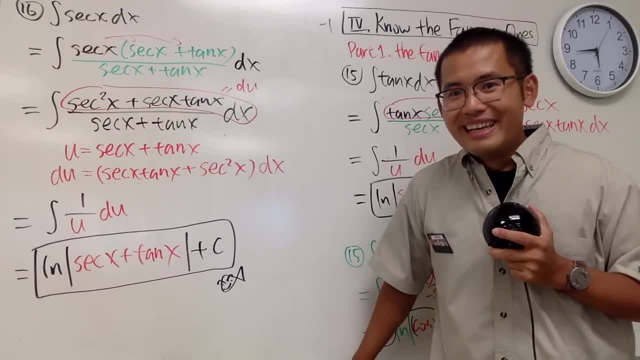 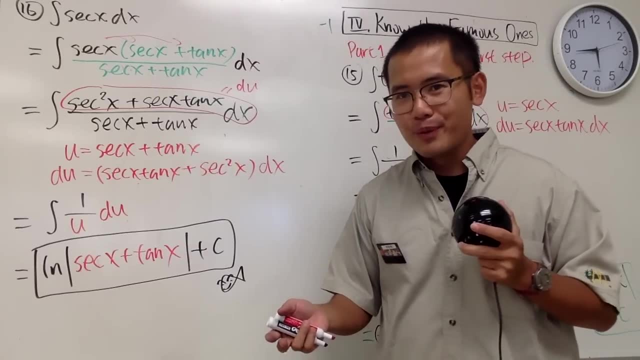 That's the idea. That's pretty much it. It's pretty much like asking you this: I can ask you who was the first president of the United States? Well, either you know it or you don't. right, Because that's a fact, right? 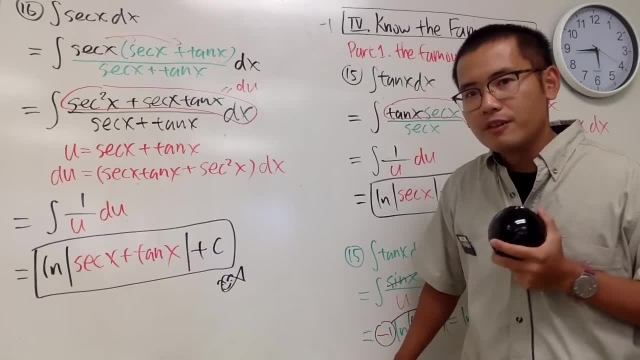 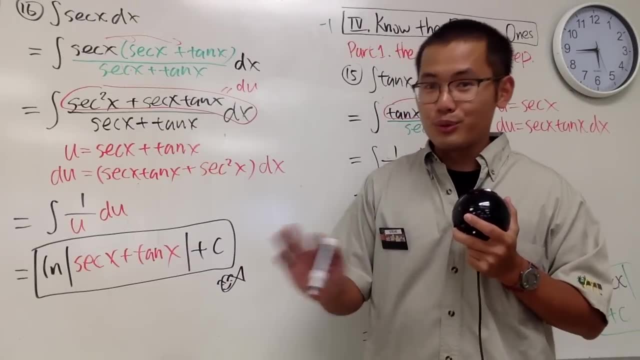 It's a famous fact right Comment down below, who the first president of the United States is. Don't look it up, alright, And you see that's something that you can not figure out. You cannot use Google to search it. 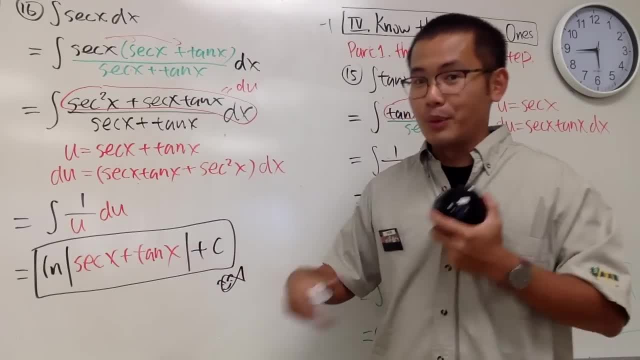 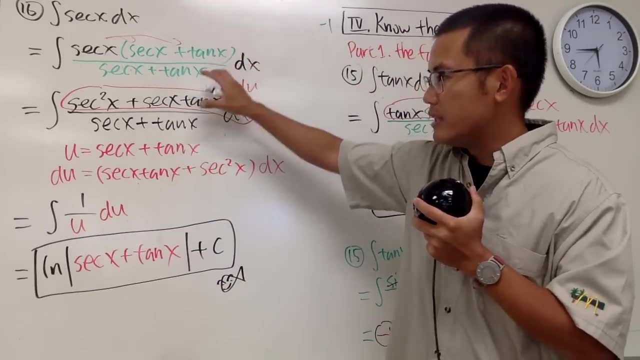 That's not thinking. to figure it out, You have to actually know it. so you know it. So here's the idea. This is the step that I will tell you, And once we see it, we are going to remember it And maybe later on we can use similar steps to solve. 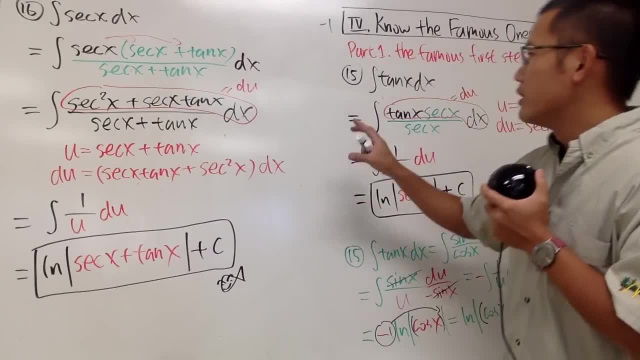 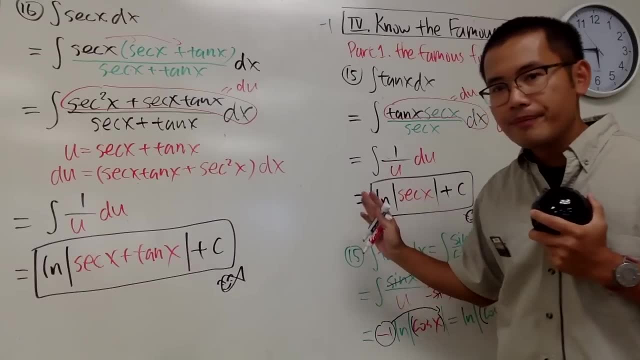 different questions or similar questions, right? So that's what I mean by this right here as the first, as the famous first step in this category, right, And this right here actually includes a lot of things, But I will give you guys another example. 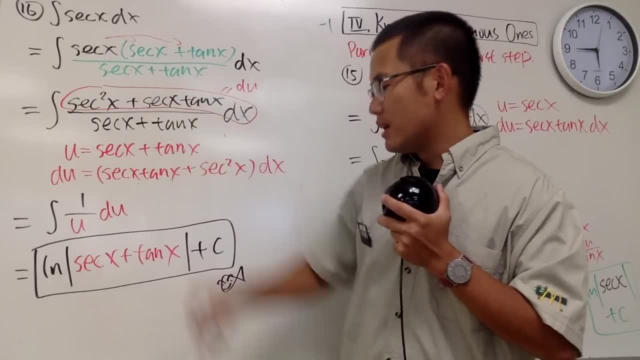 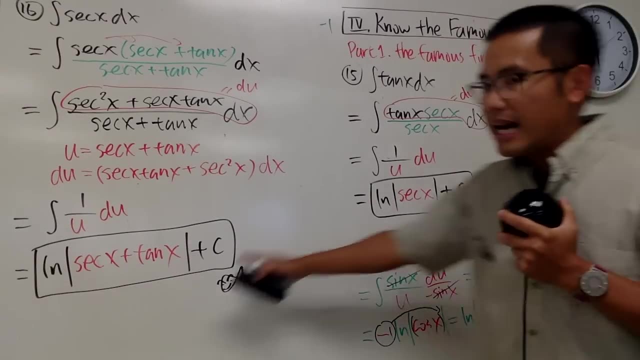 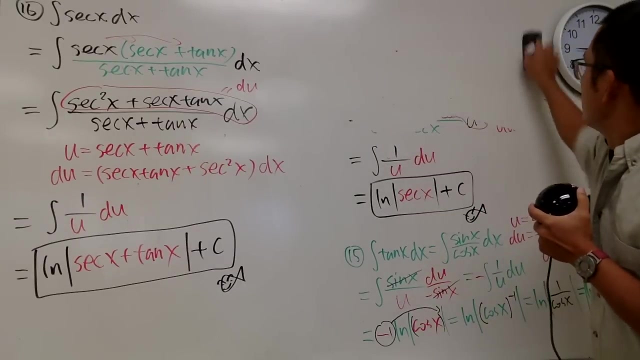 This is perhaps the most common one that you will encounter in Cal2.. And I will also give you guys another example, which is this one, But again this and that, remember the answers, right, Okay, so remember some of the famous steps. 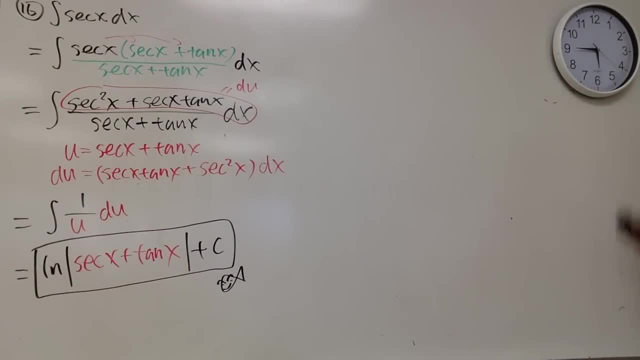 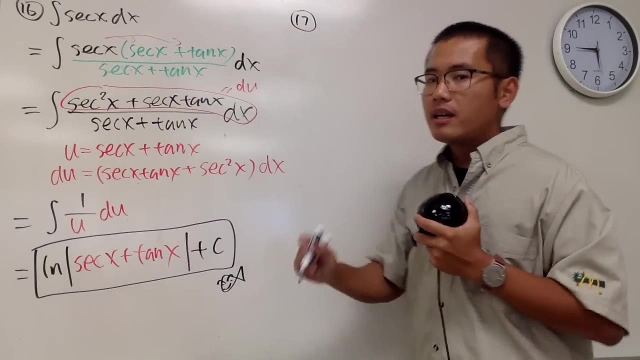 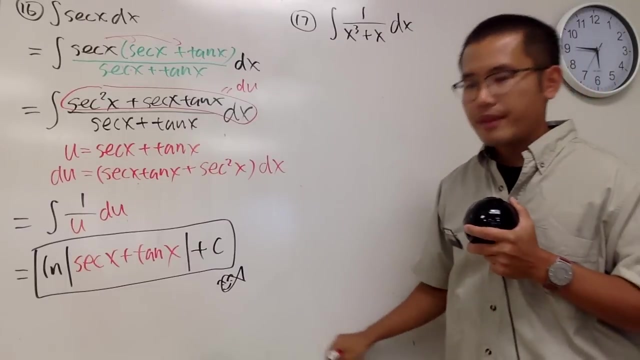 That's the idea And that's. I know it's so broad, but I think that's the best way I can put it. Anyway, number 17: right here. Here let's look at the integral of 1 over x to the third power, plus x, dx, right. 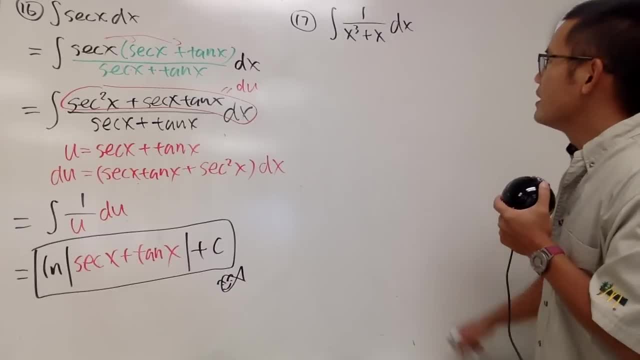 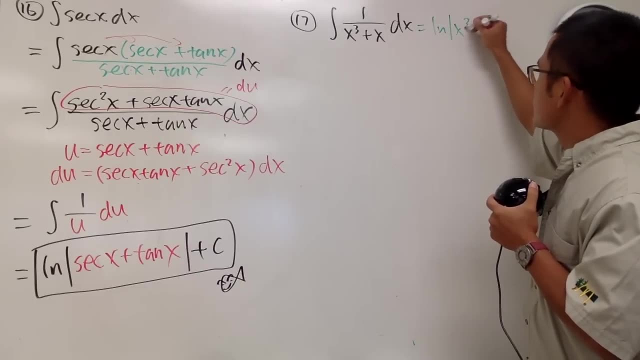 Man, you'll be thinking: hey, this is so easy, isn't it? Because we have the 1 over x. Isn't this just going to be the natural log and absolute value: x to the third power plus x? Let's see. 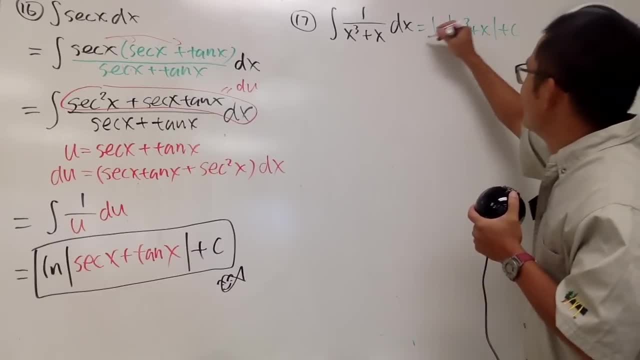 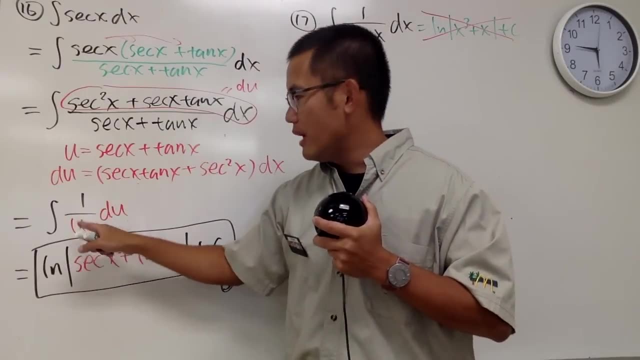 So easy, So wrong. No, This is not correct. To get natural log, you have to keep in mind, it has to be 1 over x to the first power, u to the first power whatsoever, But in this case we have x to the third power. 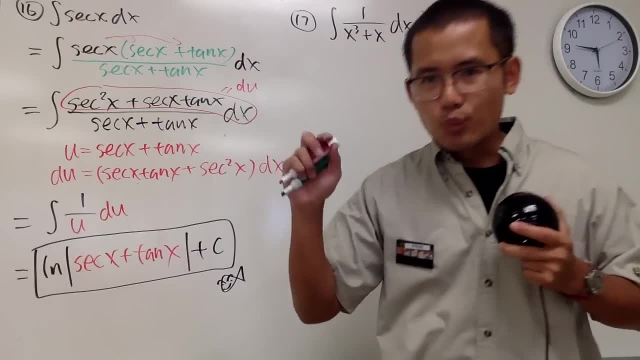 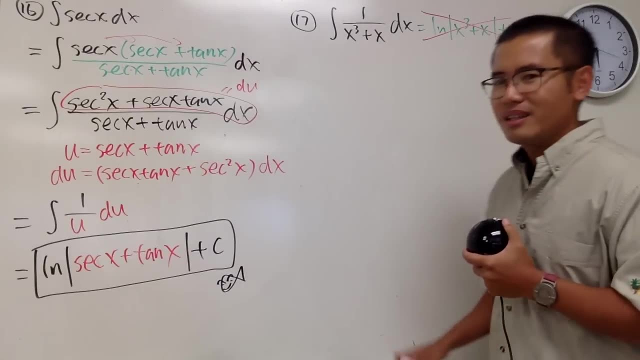 Remember the square root example earlier that we did 1 over 1 plus square root of x. That's not a natural log right away. You have to do a lot more work, right? Anyway, don't do that and we'll address this issue later on. 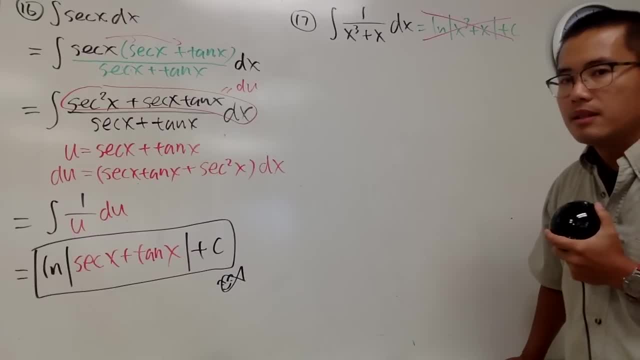 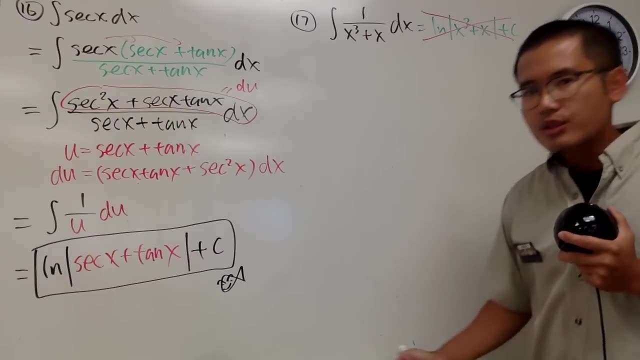 Hmm, How can we do this? Well, just kind of think back to the algebra x to the third power plus x. just like the good old days, we can factor out x to the third power plus x, factor an x from there, right. 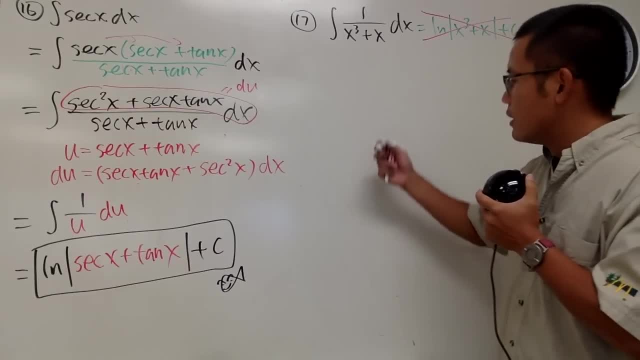 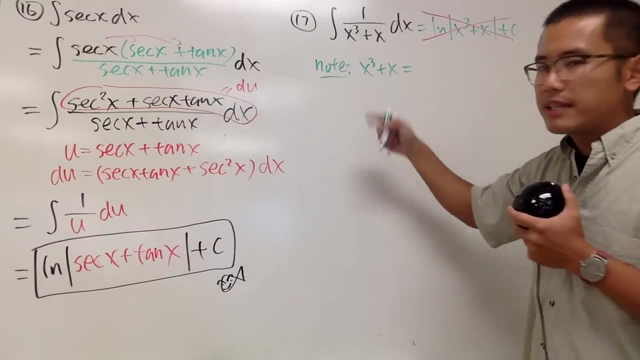 And when we do that? let me just put this down right here for you guys Note. all right, Let me just put down a notice right here. If I say x to the third power plus x, if I just factor out the x, 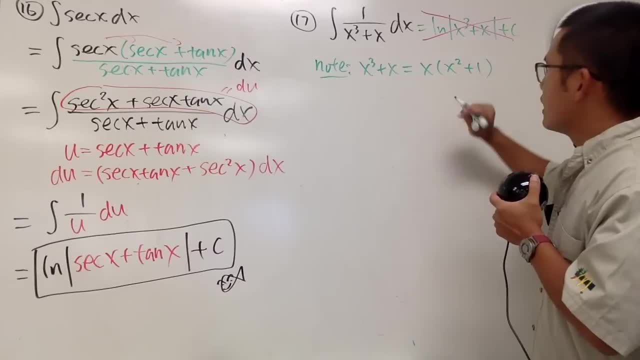 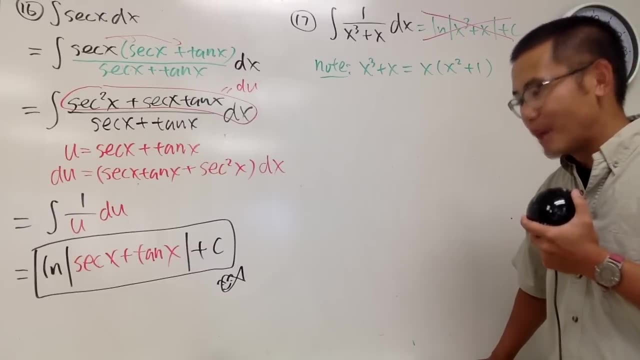 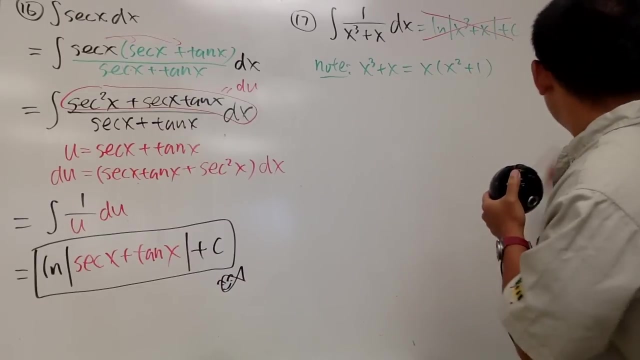 I get x times it's going to be x squared plus 1, like this, But it actually doesn't do us any good right away. This is still useful. That's the 10th category, But that's not after, like you know. 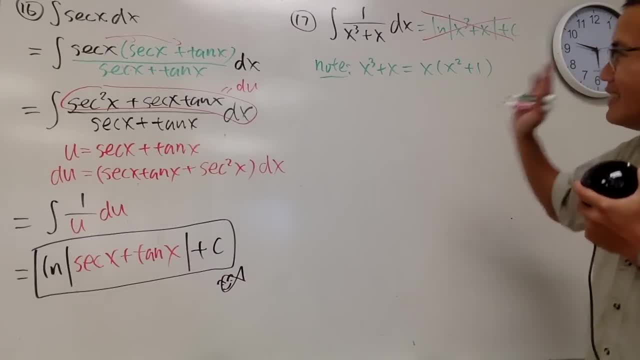 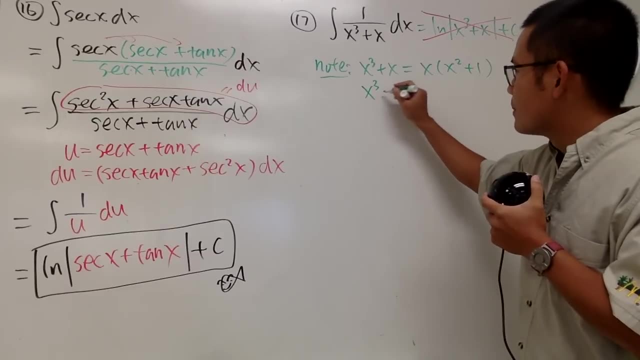 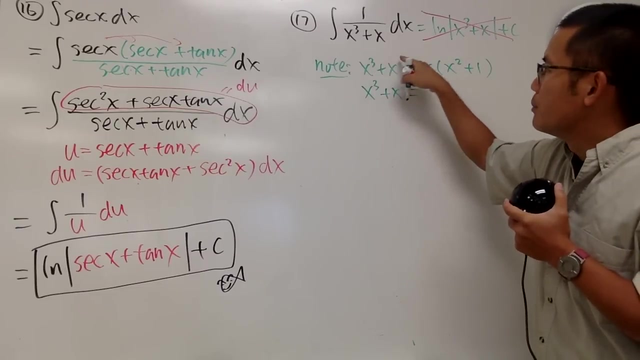 four hours or so, I don't know For this one. well, let's do the factoring with another way: x to the third power plus x Earlier when we factor. we just took out x to the first power because that's a small exponent. 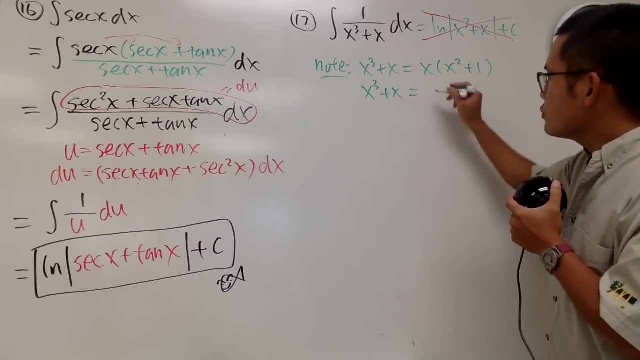 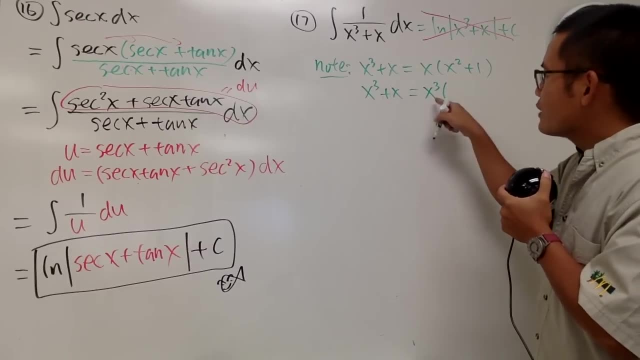 between the third power and also the first power. But can we also factor out x to the third power right here instead? Yes, This is how it will be If we factor out x to the third power here. originally you have x to the third power. 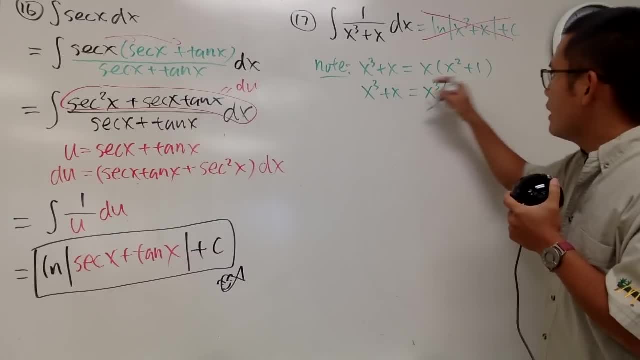 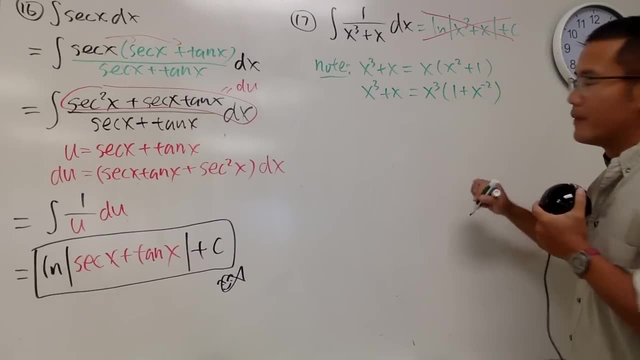 now we just have 1.. Originally we had x to the first power and now we will have plus x to the negative 2, because you needed 2 more, right? So we have negative 2.. If you don't trust me, just multiply. 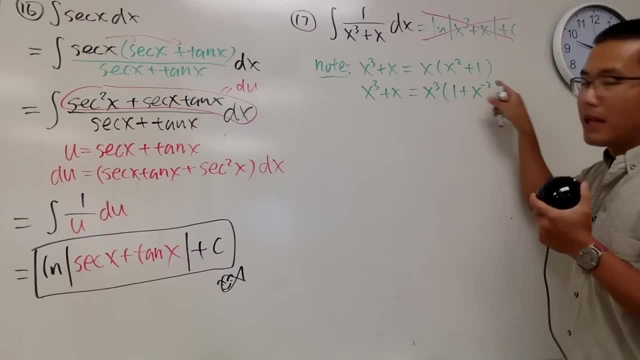 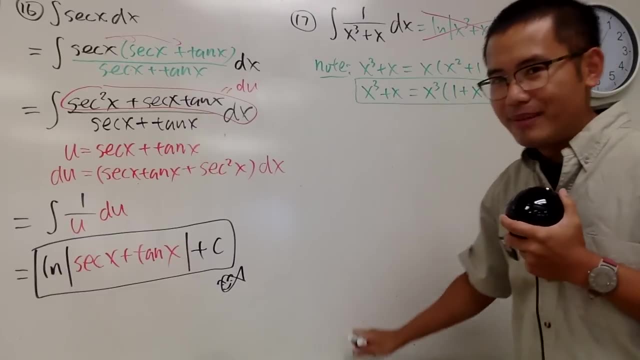 This times this is x to the third power. This times that you add the powers 3 plus negative 2, we get x to the first power. In fact, this is how we are going to use it. Now let me continue. 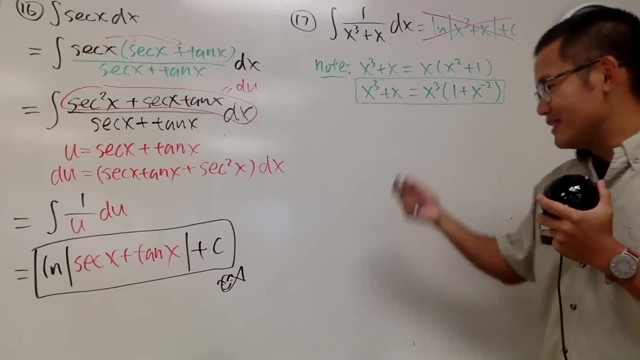 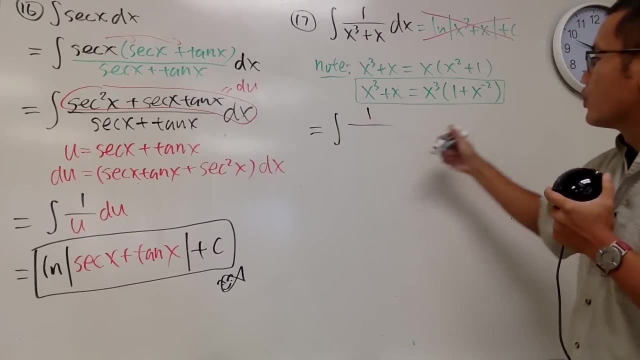 Again, that's what I mean by. I know the famous steps in this kind of particle situation. Alright, let's look at the integral 1 over this right here I will use this: x to the third power times 1 plus x to the negative 2 power. 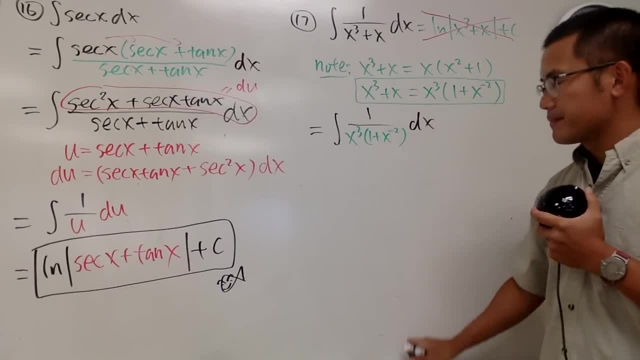 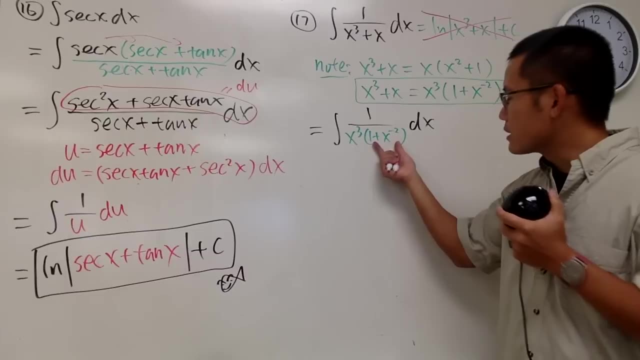 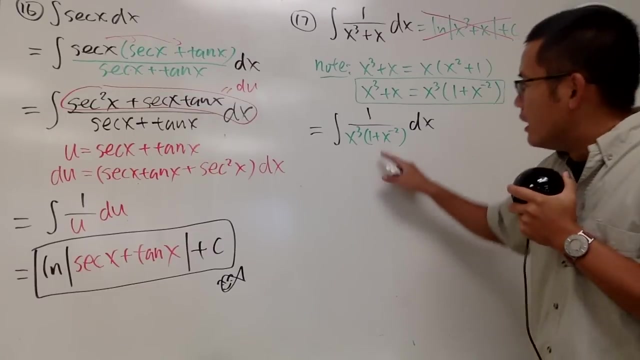 like this. And of course, we still have the dx. And you might be wondering: how can this be helpful? Well, notice this part Again. think derivatives. You have to just be aware of derivatives every single time. Derivative 1 plus x to the negative 2 power. 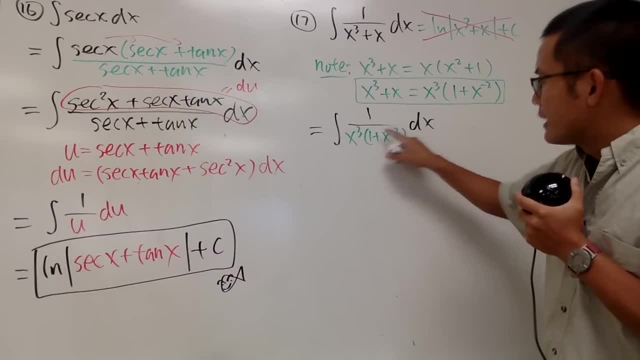 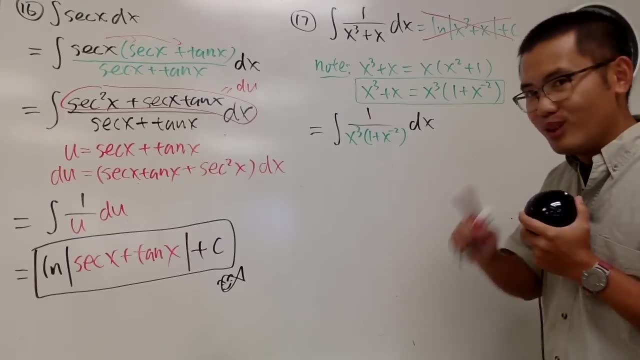 that will be 0 first, And then you bring the negative 2 to the front and we will have x to the negative 2 minus 1, which is negative 3.. Notice, here we have x to the third power, Isn't that? 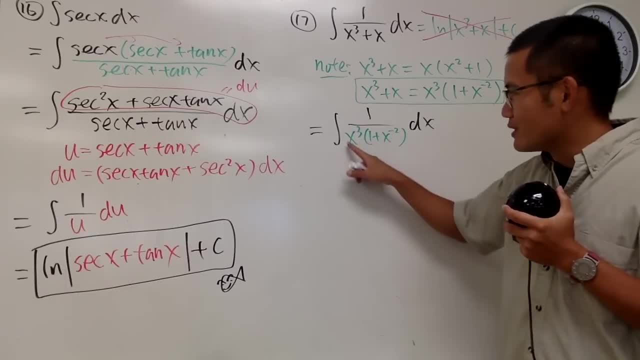 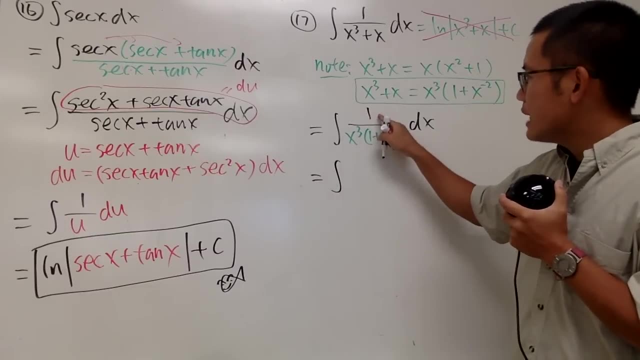 x to the negative 3 power, Because, of course, this is on the bottom. So here's the idea. Let's look at this right here as the integral, Bring this up and when we do that, when we do that. 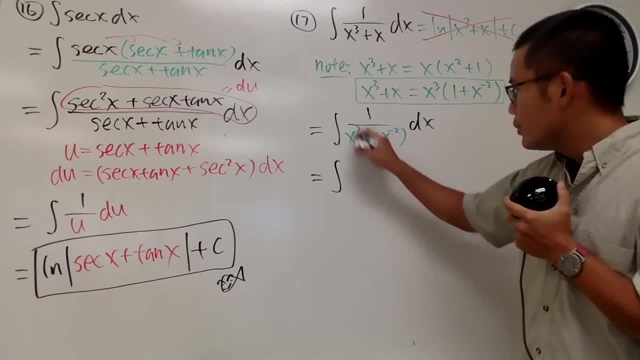 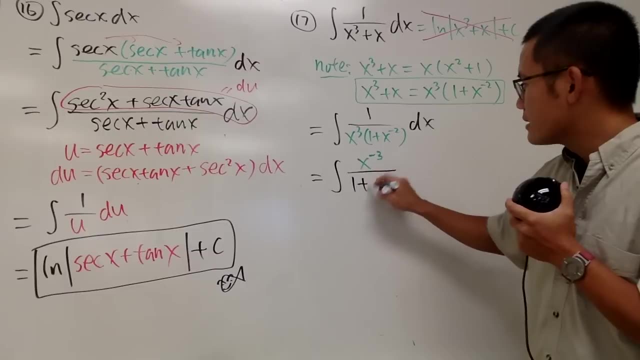 let me just put this down in green, Why not? When we do this part, we get x to the negative 3. And we have this over the bottom: 1 plus x to the negative 2. The x like this: 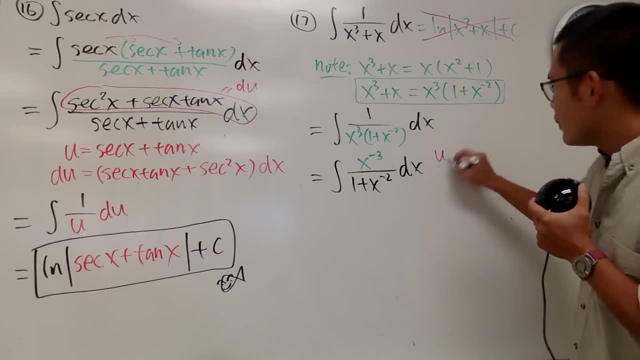 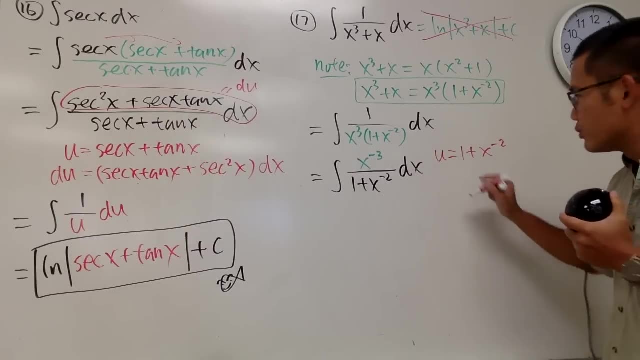 It is so much prettier because that u equals the bottom, that u equals the denominator 1 plus x to the negative 2. Differentiate this real quick. We get du equals, that will give us 0. And the derivative of this is: 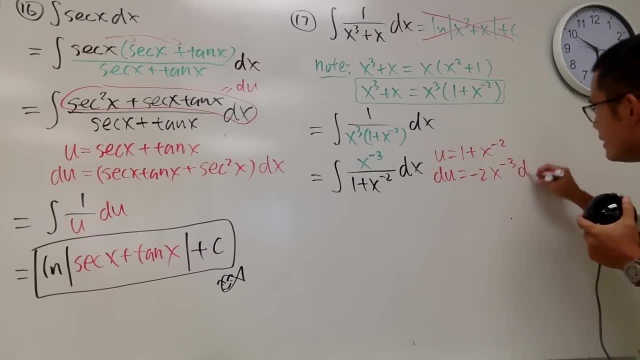 negative 2. x to the negative 3. power dx: Ha, We have x to the negative 3 right here. Very nice, And you see this case. let me just isolate the dx. Another way to do it is some people will say multiply. 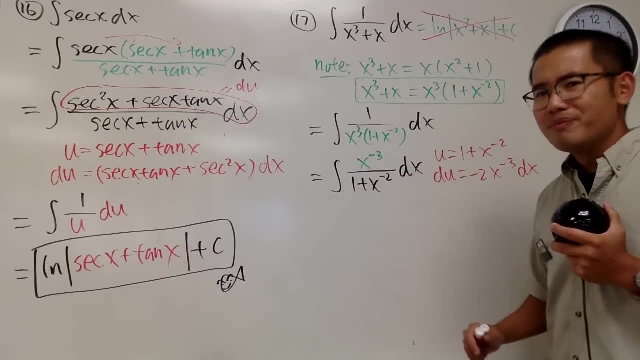 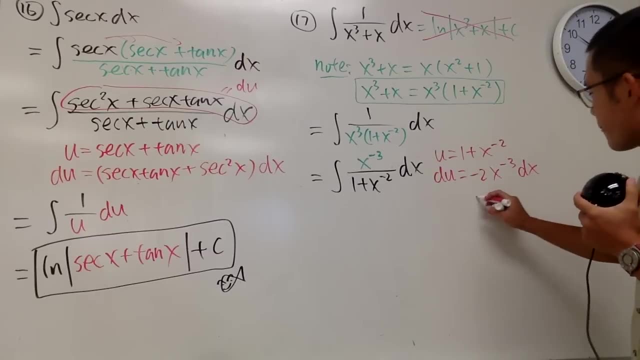 this by negative 2 and divide it by negative 2, up to you. But if I cannot see the whole thing right on the top, I would like to show you guys a cancellation. So let me just put on: dx equals to: 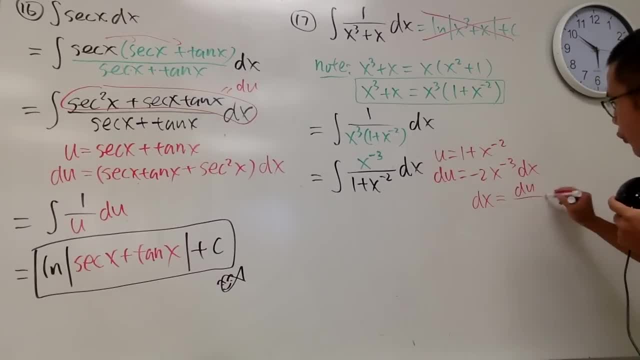 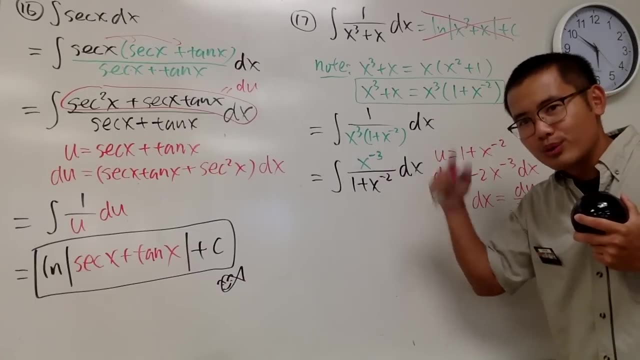 this divided to the other side. So we get du over this on the bottom, Negative 2, x to the negative 3.. And take this integral to the u-world, we get the integral and this is x to the negative 3 over. 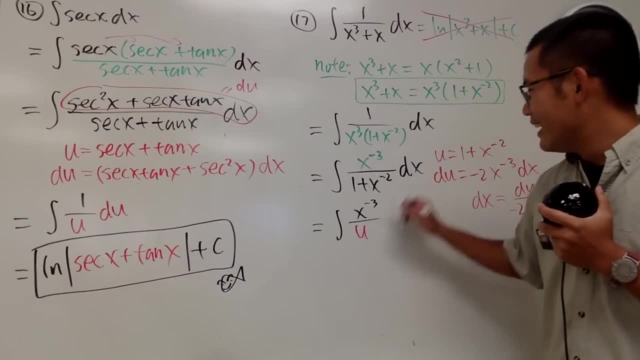 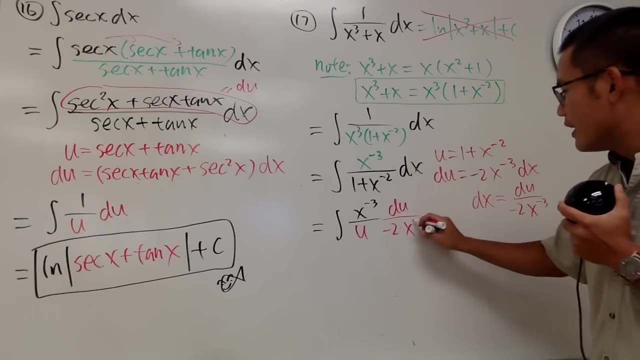 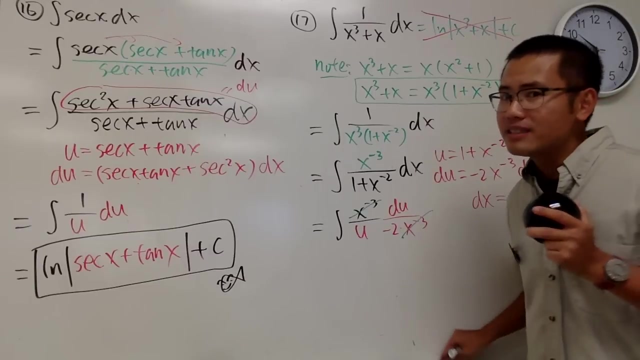 this guy is just the u dx is all this. so we have du over negative 2 times x to the negative 3.. And now this and that, cancel out. This is the u-world. No x in the u-world. We don't have x in the u-world. 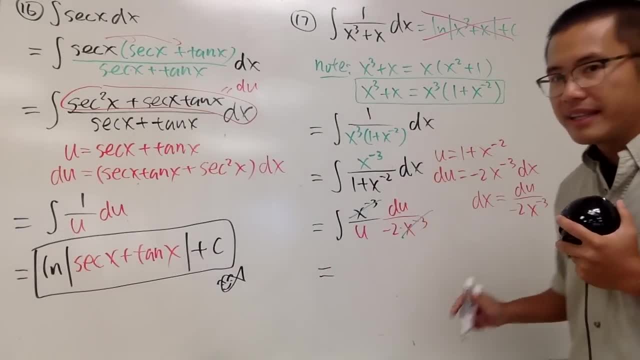 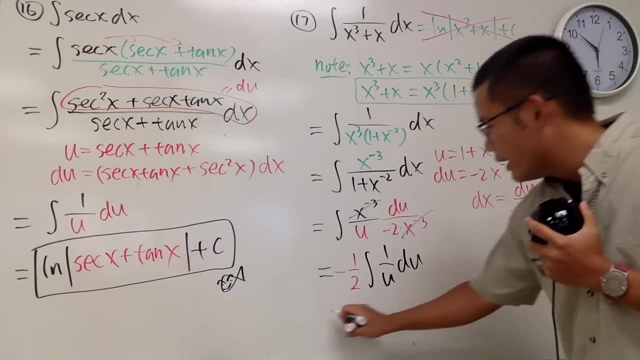 That's so nice. Now here we have 1 over negative 2.. So let's just take that all the way out and we have the integral 1 over u du, And this right here is going to be negative 1 half. 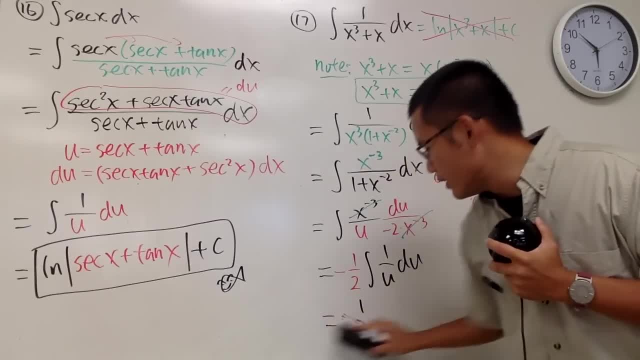 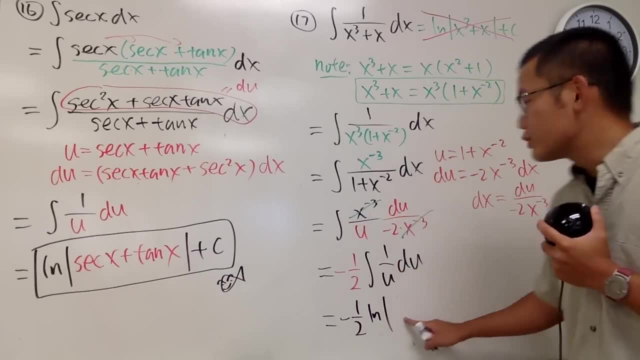 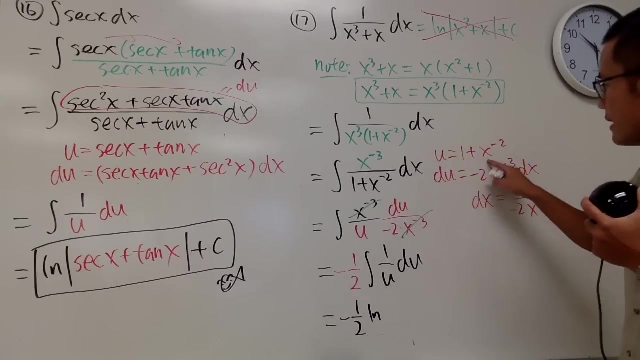 This is just a constant multiple Negative 1 half, And this is natural log absolute value of u. But u is what U is this. So we have 1 plus x squared. We have this 1 plus x to the. 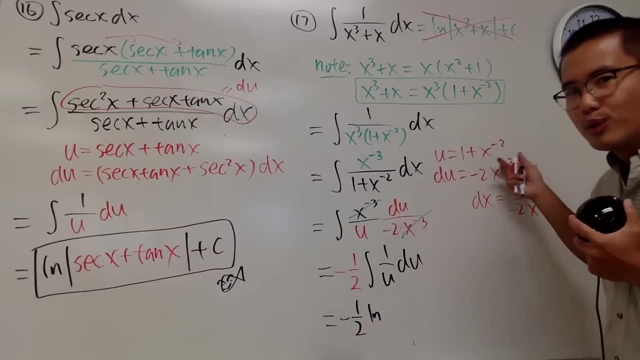 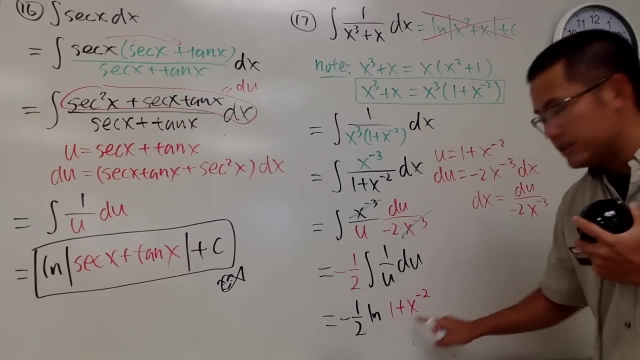 negative 2.. But this right here is 1 over x squared, which is never negative, So I will write it down as 1 plus x to the negative 2.. Since this is never negative, I don't need to worry about the absolute value. 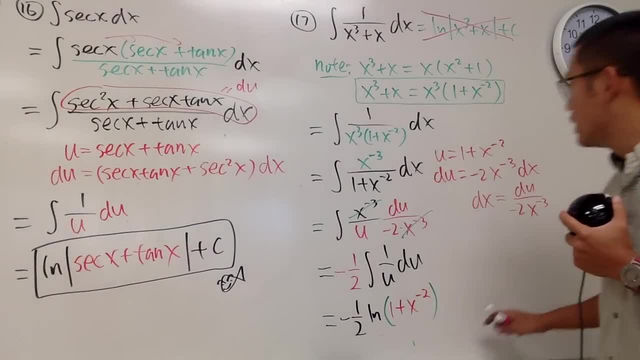 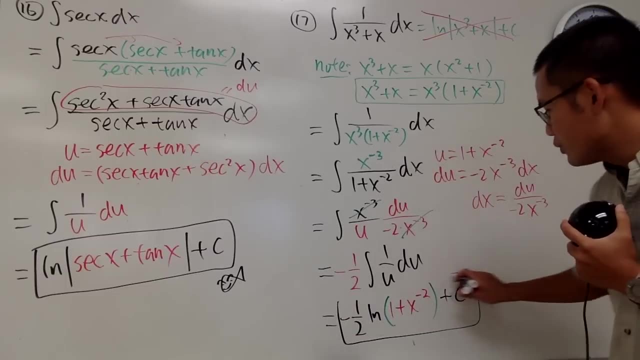 Parentheses will work out okay. So this right, here is it, and then we are done. So put down the plus c, And if you really want, you can of course change that to 1 over x squared, but I will leave that to you. 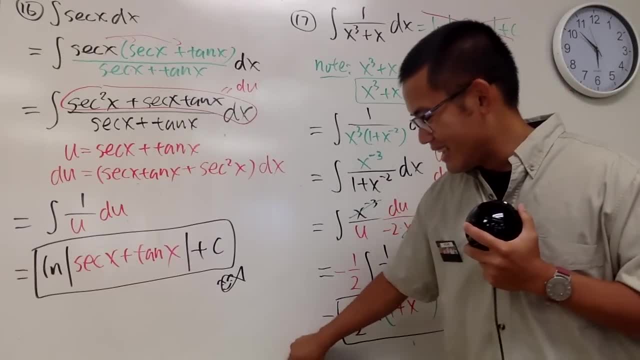 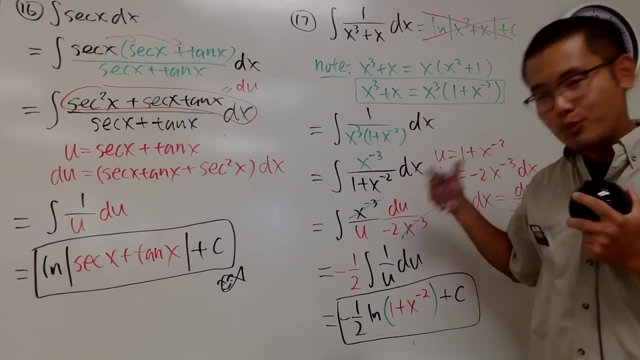 This right here is perfectly okay in calculus, Yeah, So this right here is it. You have to rethink factoring. And how do we know this? Well, again, I'm showing you guys this now, so later on you will be. 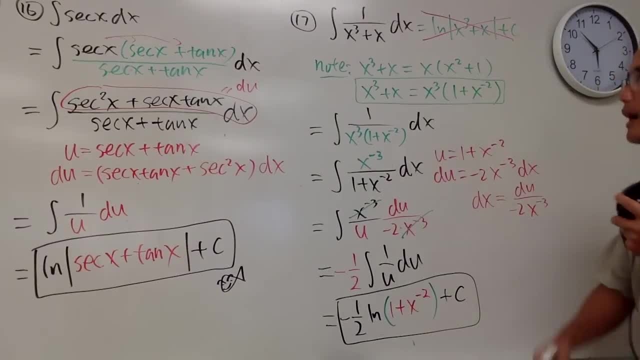 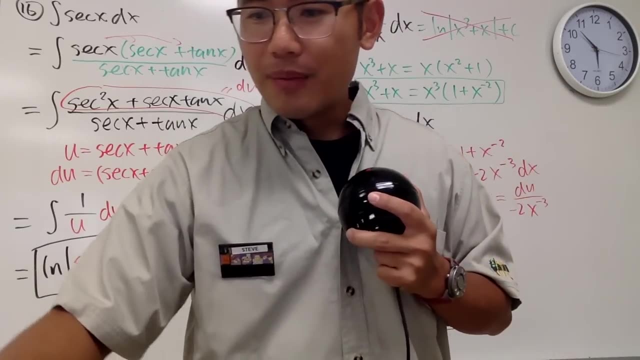 aware of this kind of first step, Right, Okay, So that was the fourth category and we are done with the first page. Pretty amazing. And of course we have more Again. you guys can go download the file I. 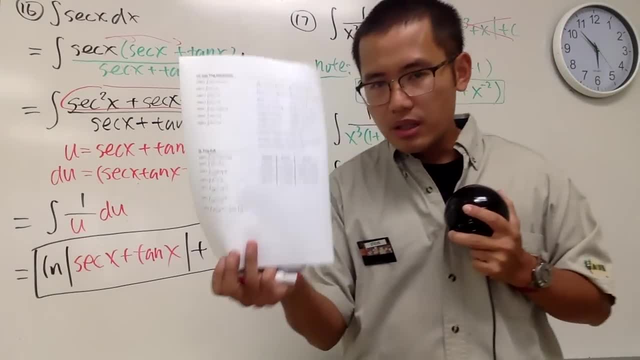 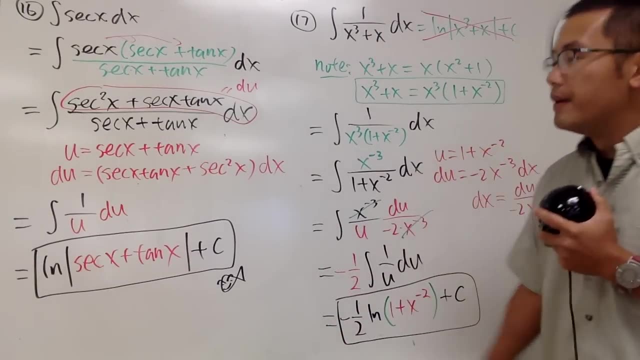 typed out the notes and also the identities that you need along the way. Okay, So be sure you guys make good use of it. And yeah, Now if you look at number 17,. this is a mistake. I just wanted to purposely. 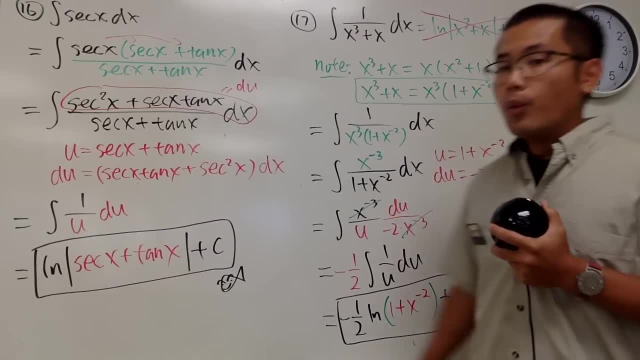 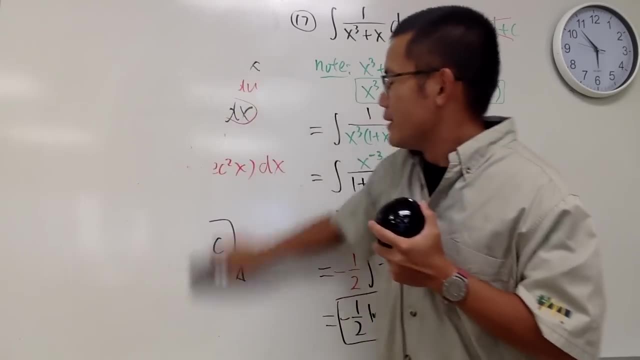 you know, illustrate it. Let's talk about the following, And before I do that, of course I have to erase the board And I will try to just record everything in one go, of course, as I said it, And I'm not going to. 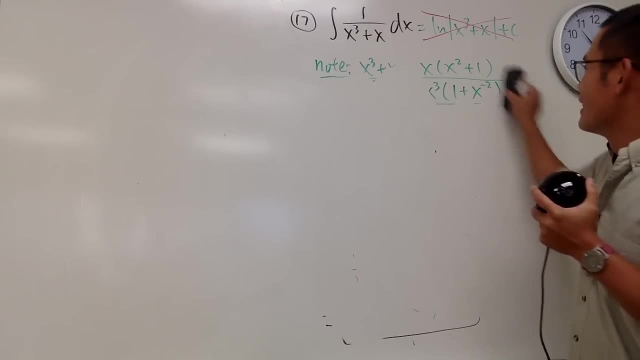 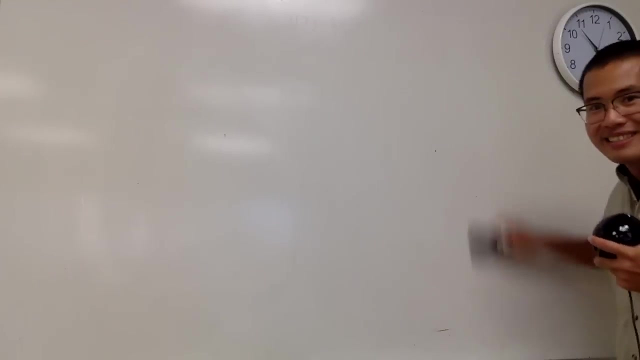 edit the video. And you guys noticed earlier, like the IT people, they came in to try to just like work on the computer over there, but they were so nice that I think they will just come back, maybe later or maybe. 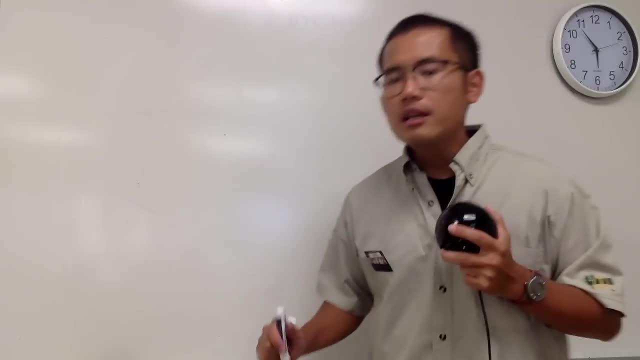 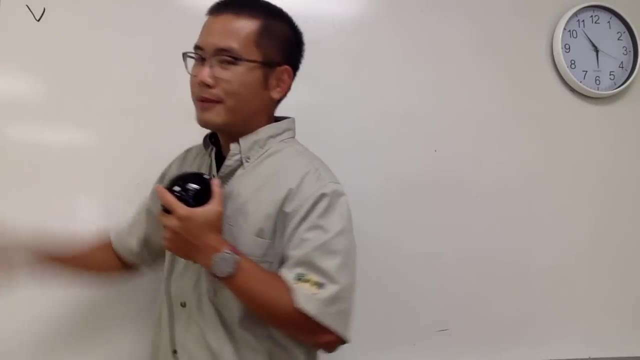 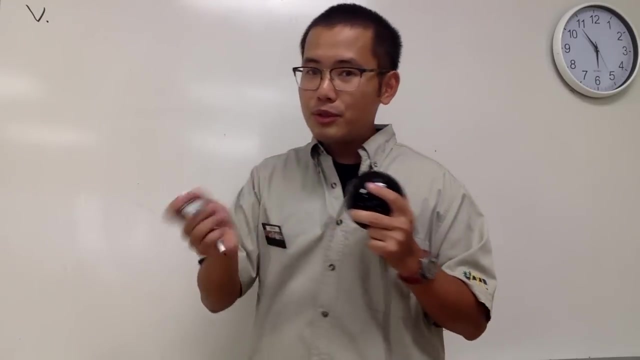 tomorrow or something. All right, Here is category number five. Let me write this down right here for you guys. And to write five, you write it as this V is five. Yeah, Here is the deal. I will call the following. Let me just 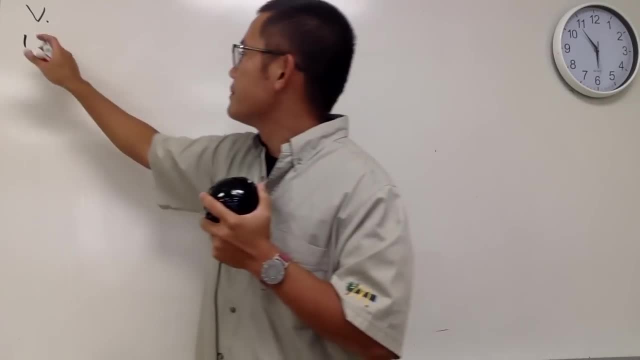 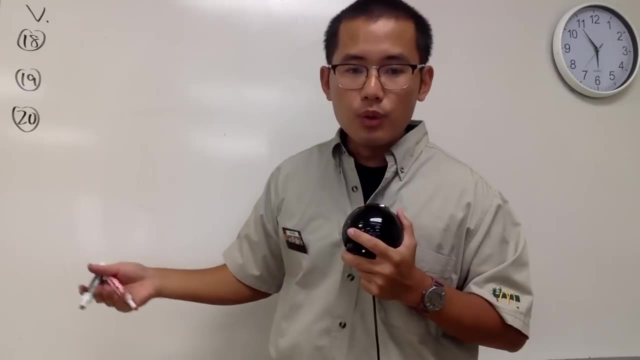 put this down right here for you guys. So this is number 18.. And again, I'm just going to write down the questions and the things that I want to talk about with you guys right now, And then I will tell you guys what this category. 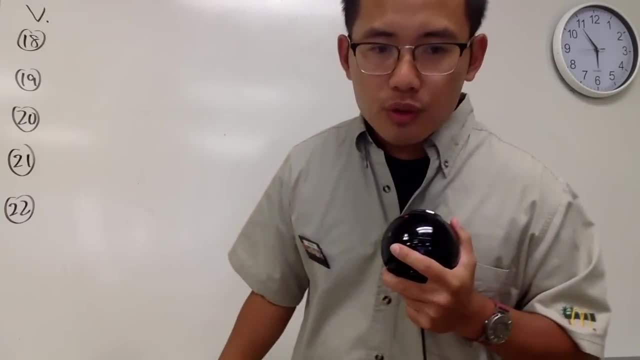 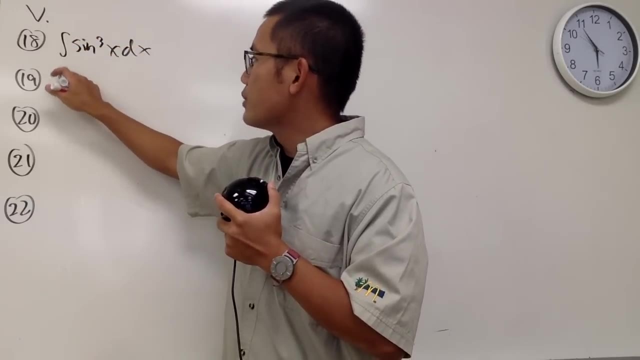 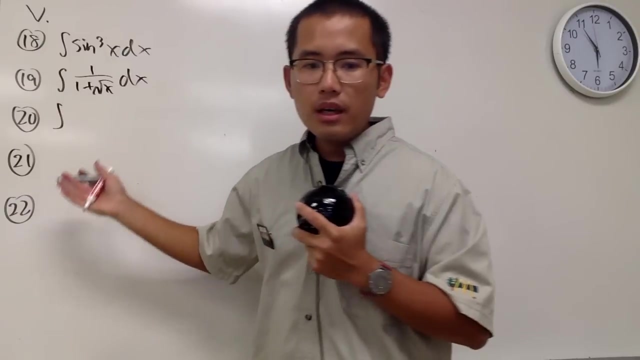 is all about. So five questions at the same time. The first question is the integral of sine to the third power, x- dx, And the next question is the integral of 1 over 1 plus square root of x- dx, And then number 20, the. 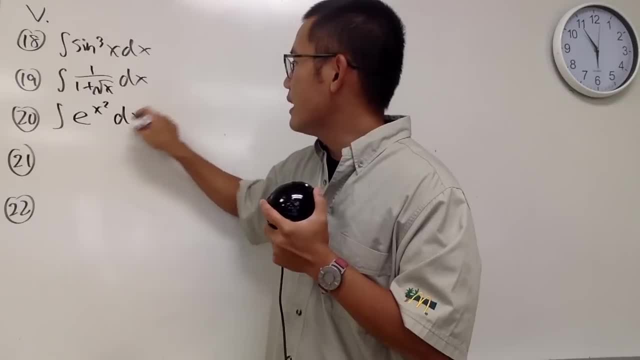 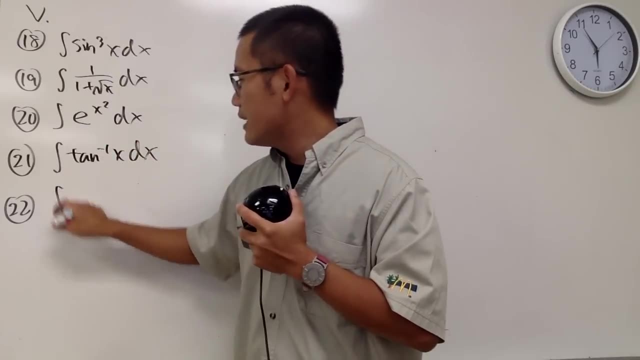 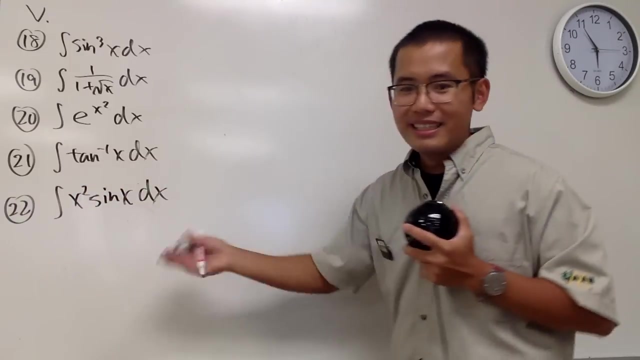 integral of e to the x square dx, And then integral of inverse tangent of x- dx And lastly, we have the integral of x square sine x dx, Like this. Alright, Now we are going to finish this real, real fast. 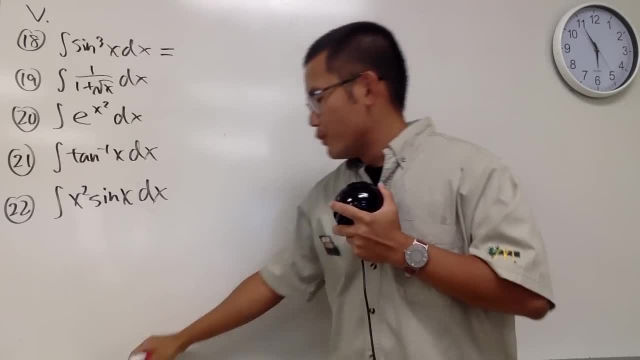 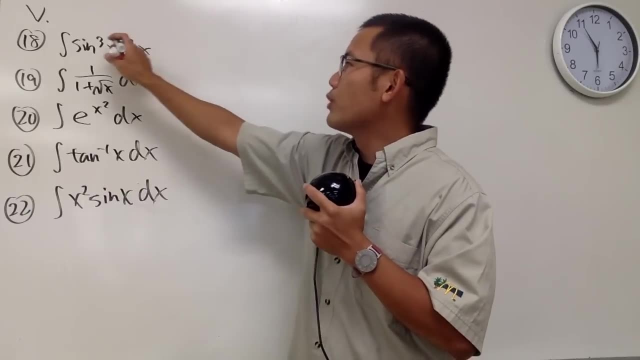 For the first one, notice that, hey, we have the integral of sine to the third power, Sine to the third power. Why don't we just go ahead and add 1 to the power, which is 4, divided by the new power, which is? 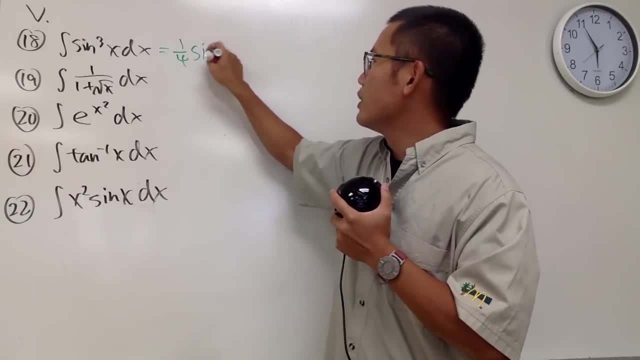 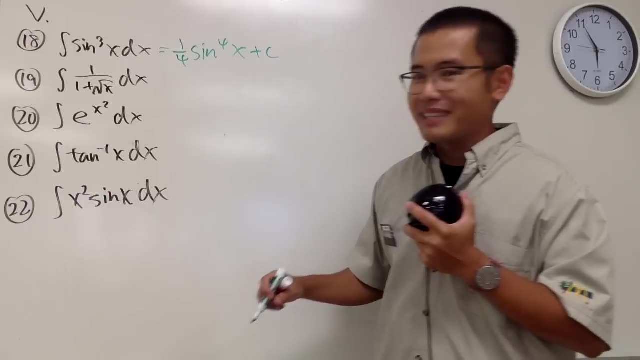 1 over 4, right here in the front. And then we have sine to the fourth power, x, like this, And again put on the plus sign. Good, I remember my plus sign. Next, we have 1 over 1 plus square root of x. 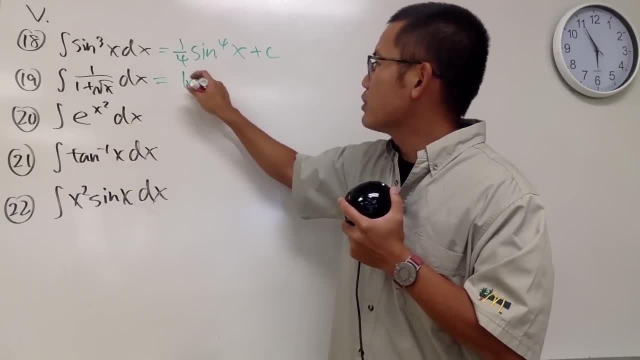 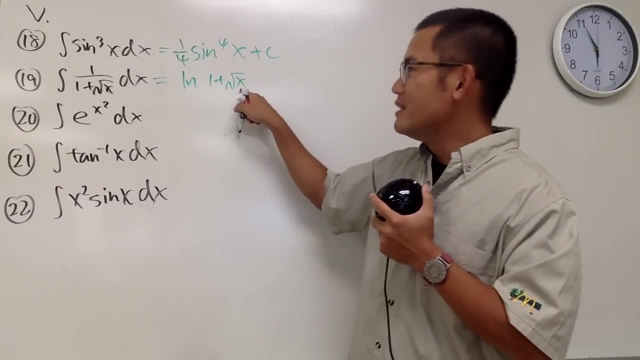 I see the 1 over. Huh, Easy Natural log And we have 1 plus square root of x. But remember, Black Pan told me that this is never negative. In fact, 1 plus that this is always positive, so I don't need. 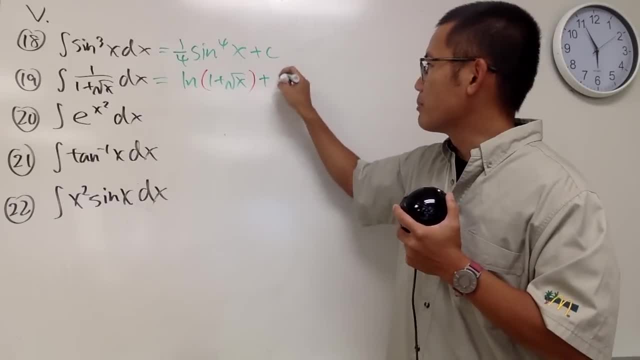 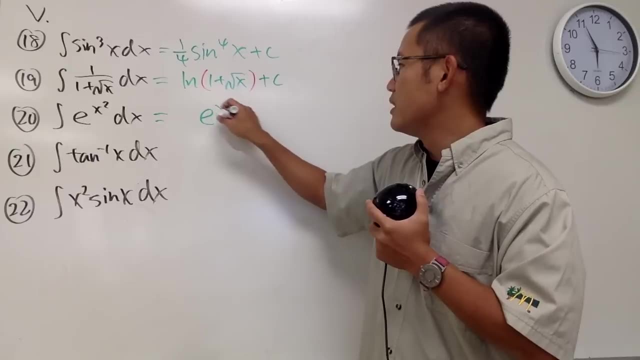 the absolute value I can just put on parentheses, And don't forget the plus sign. Next, Okay, The integral of e to the something. Huh, It seems like just e to the same thing. And think about what's the derivative of x. 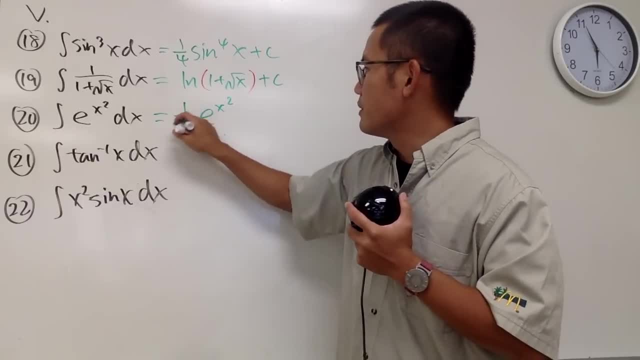 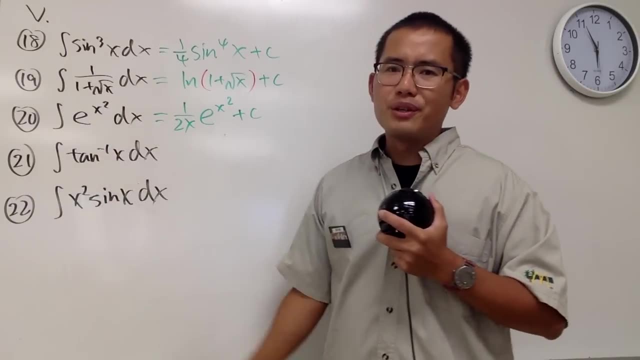 square 2x. Let's just divide it by the derivative. So 1 over 2x, this Done Plus c. Next Inverse tangent: Well, this right here: 1 over 1 plus x- square, Done Easy. 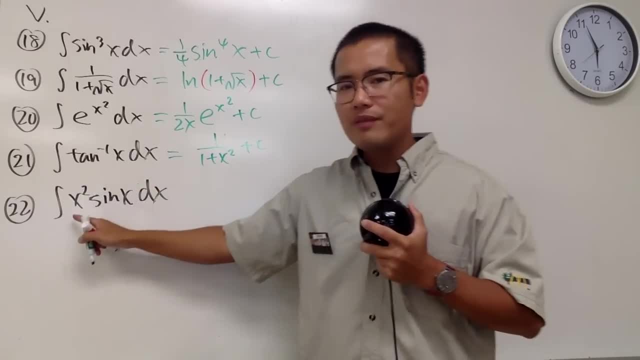 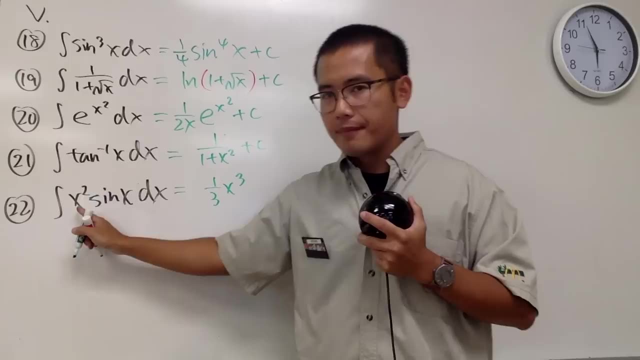 Number 22.. Hey, we see that we have x square. Let's do the reverse pole rule first. So that will give us 1 third x to the third power. And what's the integral of sine? Well, that should be. 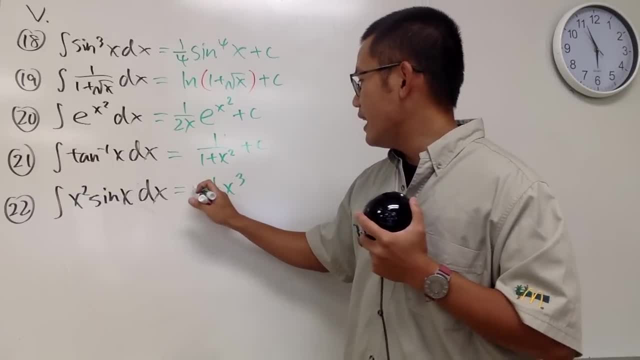 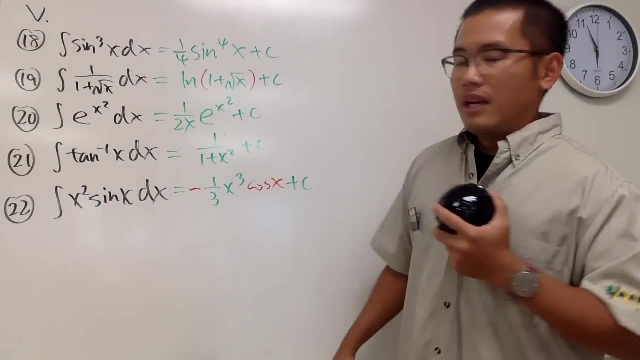 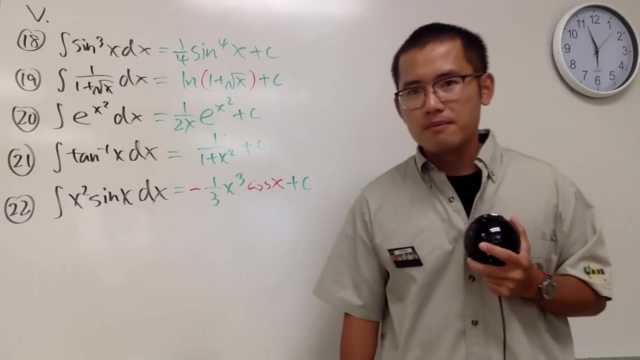 a negative cosine. So I have a negative cosine. So integral of sine is negative cosine. Yeah, we got it. And then plus c: Huh Man. Five examples. So easy, So easy, So wrong. Here is my fifth category. 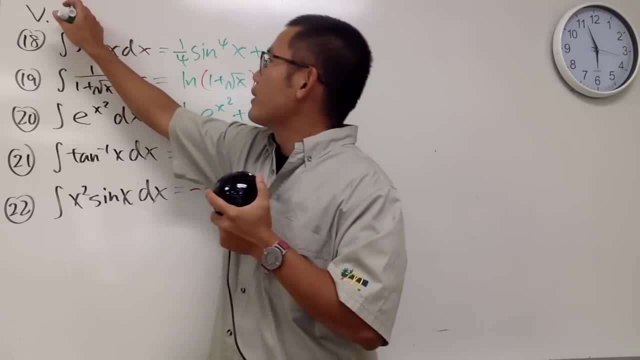 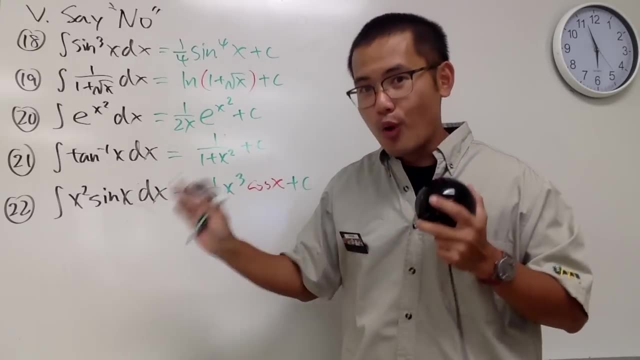 I call this right here, the integral addictions. So you are going to say no, Right, Right, You are going to say no And you have to be aware of. don't ever make this kind of mistakes, Say no to these. 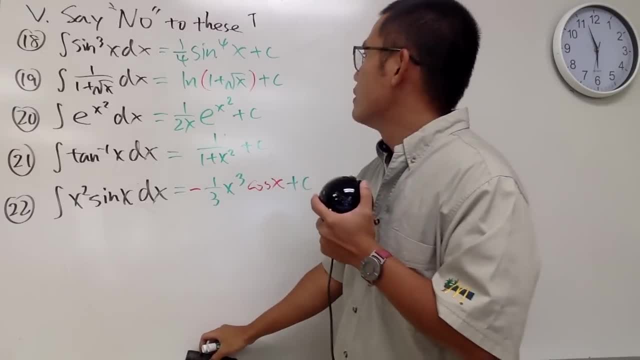 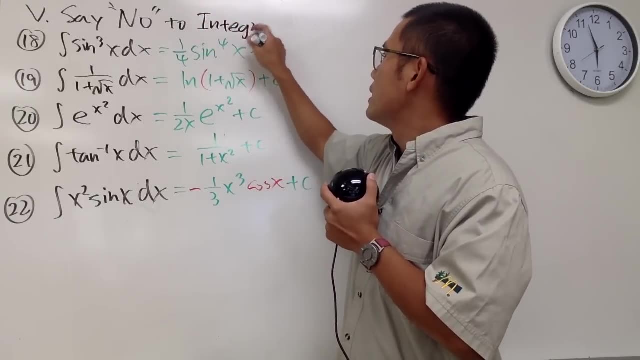 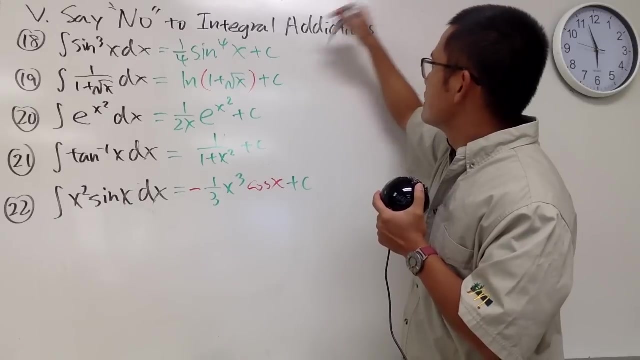 Oh, I just How do I say it? Oh okay, Oh no, I'll just say: Say no to integral addictions, Addictions, Addictions, Addictions, Like that. So this is my fifth category, And 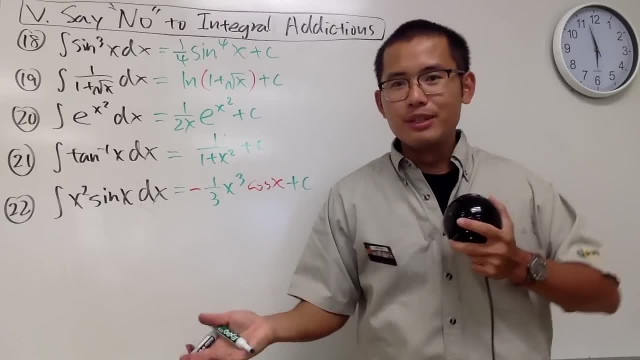 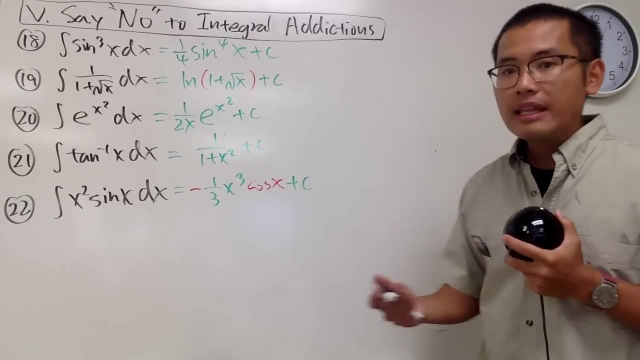 yeah, it's just pretty much the common mistakes that students will make, or the people would like to just do with integrals. I know this would be so easy and they are just so wrong. And now let's talk about why they are just so wrong. First, 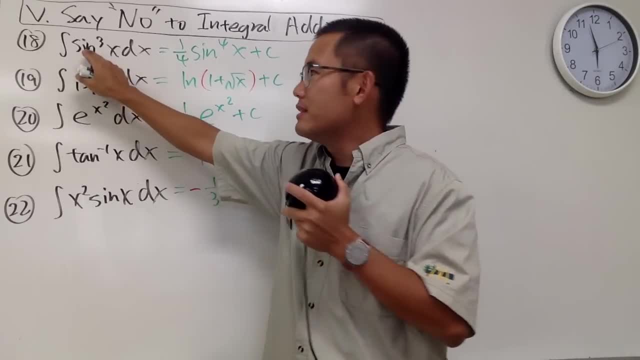 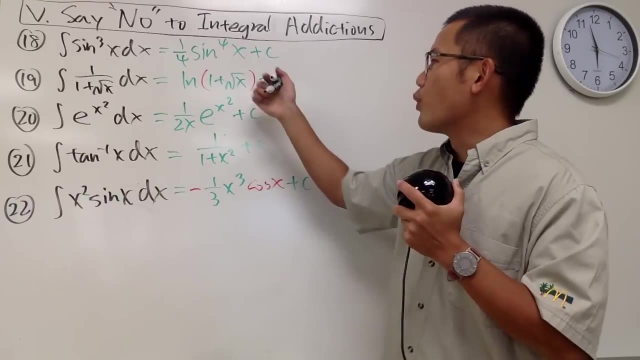 of all. this is the integral of x. This is the integral of sine to the third power. We cannot just do the reverse power rule when we have a function to a power. This is of course not correct. This is of course not. 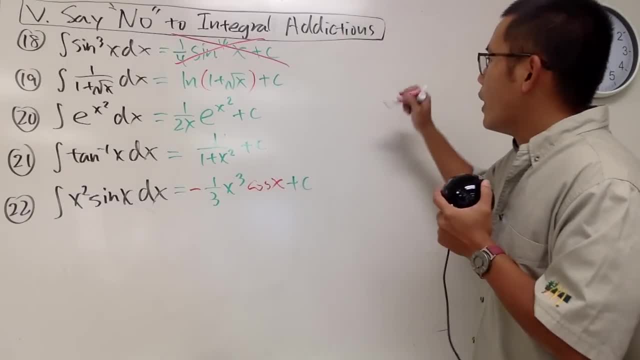 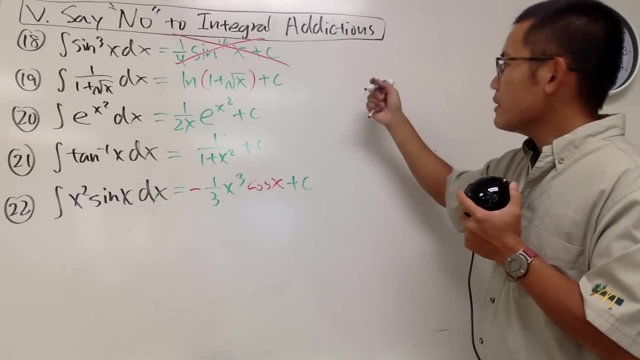 correct. Right, This is not correct. Well, it would have been much easier if- let me just say if- the question was: let's see, I don't have any other color, So this right here is the easier version, Okay. 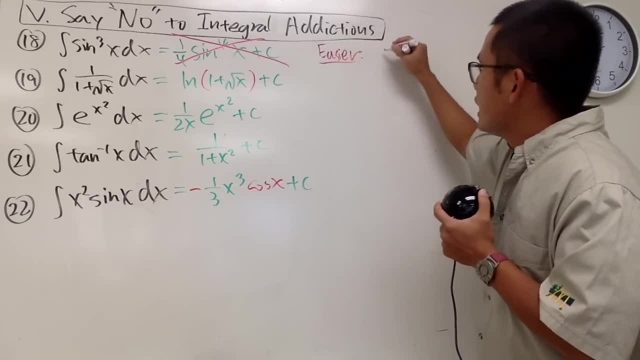 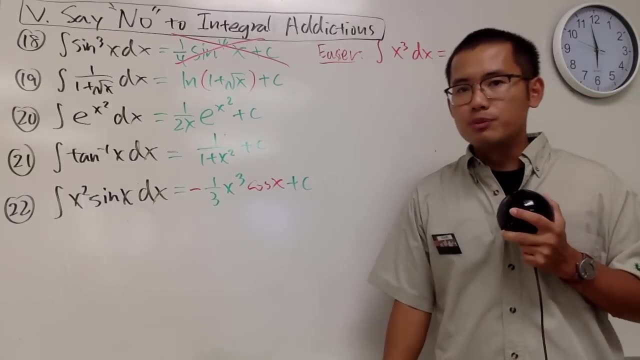 I'll just tell you, guys, It would be easier if we would dealing with the integral of x to the third power, dx. This, right here, would be, of course, much, much easier, Because x to the third power, of course, you add. 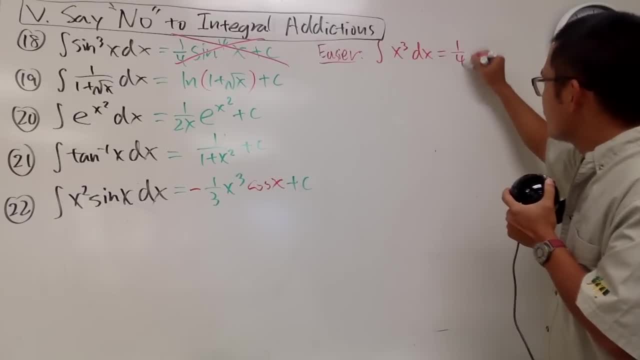 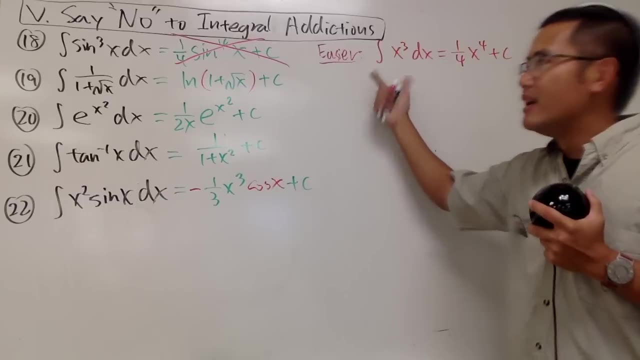 1 to the power and divide it by the new power, we end up with 1 over 4.. x to the fourth power, and then we're done Plus c. That's so much easier, If this was the question Right, And in fact I will also. 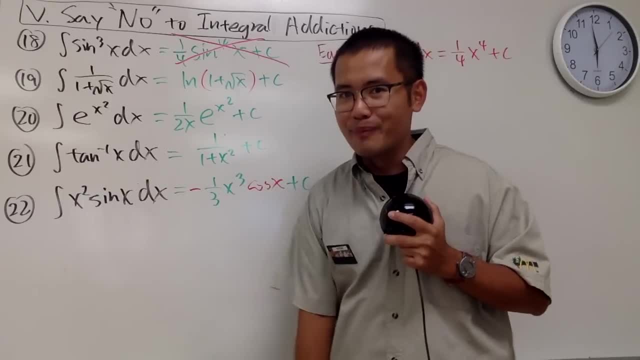 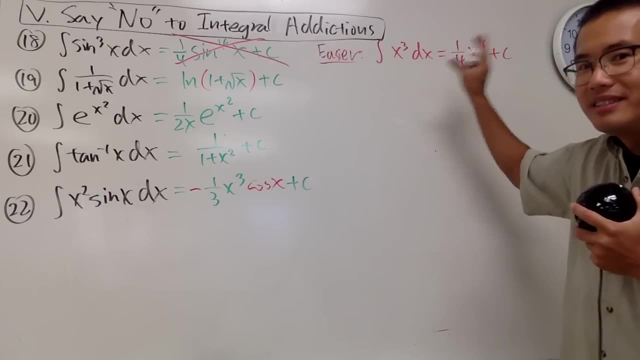 show you guys how to do this legitimately later on. So this would be the correction for number 8.. This is another correction. This is just an easier version. This is the the actual one. you can do the reverse power rule with, Alright. 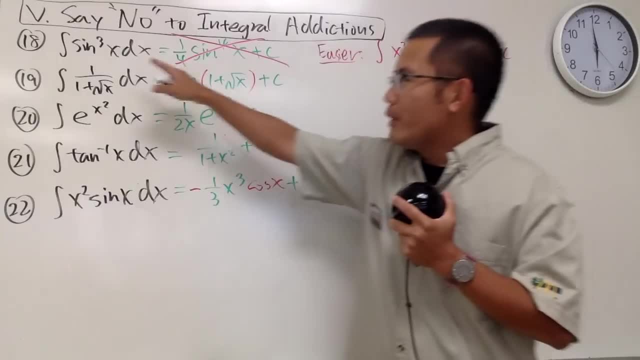 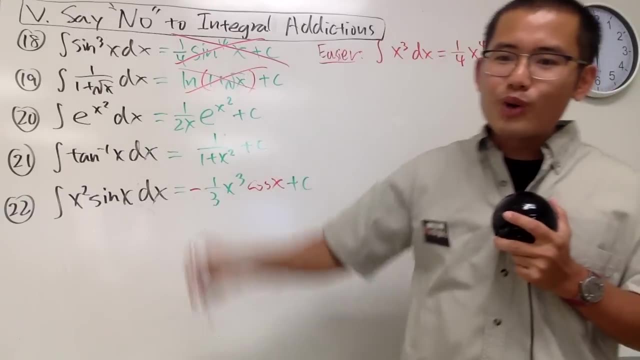 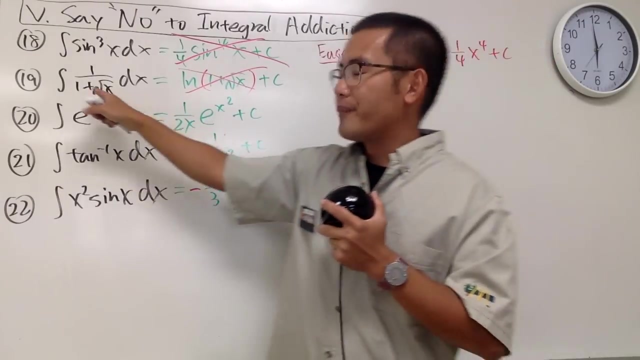 Number 19.. 1 over something. No, You cannot just do the natural log right here. This is so wrong. And I know this is so wrong because we did a question earlier already. That was question number 14.. This right here. 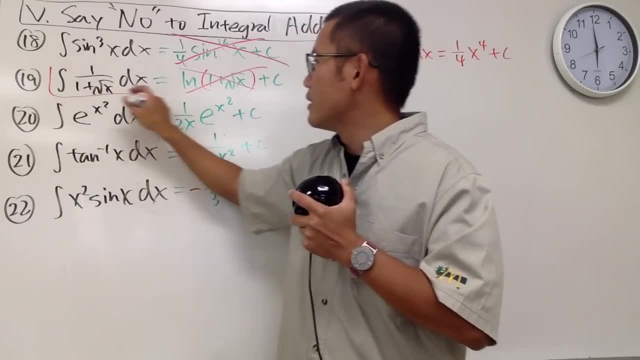 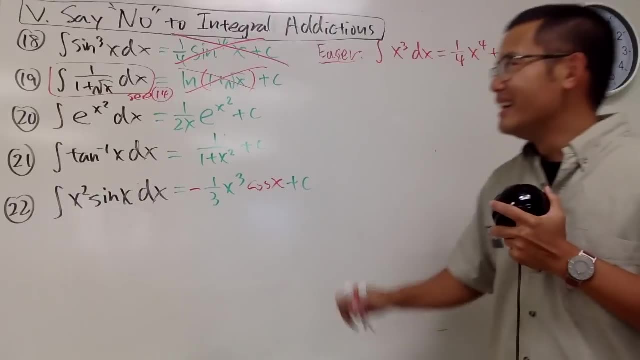 See question number 14.. Okay, So I'll just tell you This right here: See question number 14.. Which we did earlier. Just refer back. You cannot do this, And again I'll show you guys the easier version. 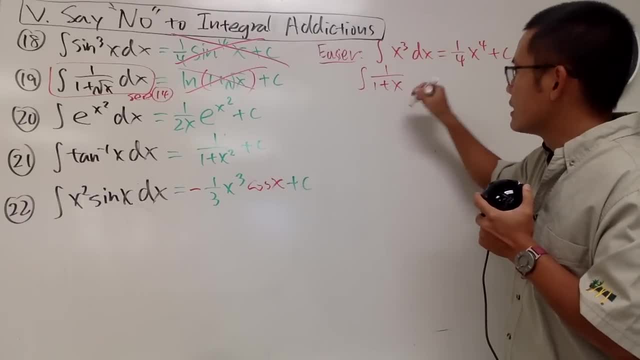 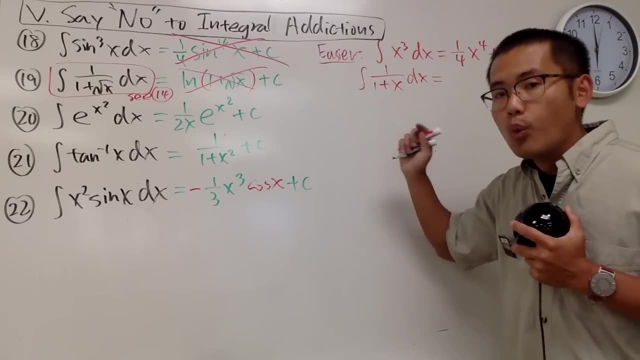 Suppose you're just integrating 1 over 1 plus x to the first power And you have the dx right here. Yes, This right here will give you the natural log. Why? Because you can do u sub, let u equal to the denominator. 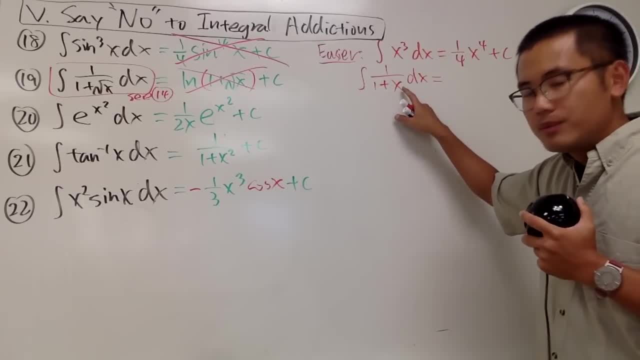 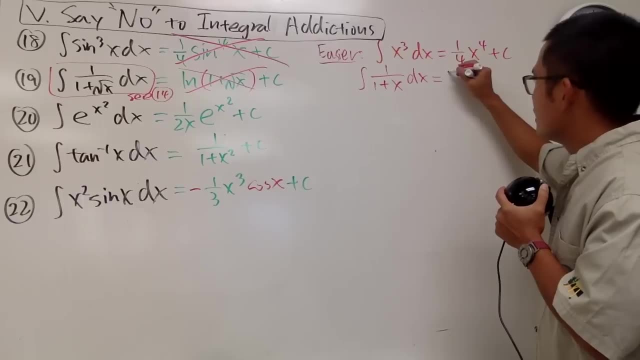 If u is equal to 1 plus x, the du will be dx. So you just integrate 1 over u in the? u world And that's going to give you the natural log, Natural log of the denominator, which is 1 plus x. 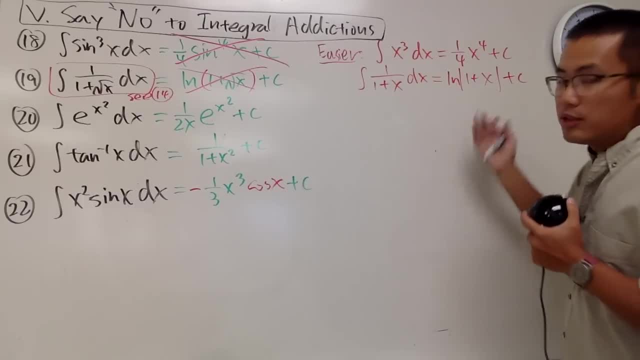 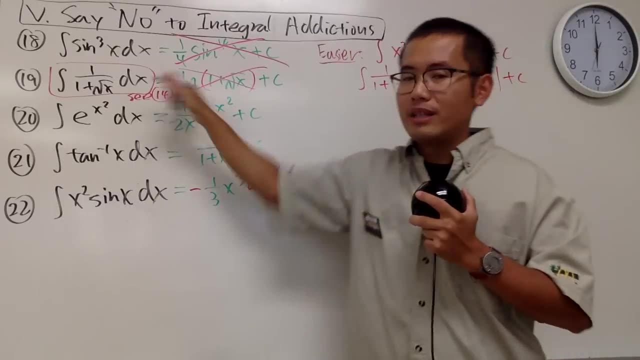 And we do need an absolute value right here And plus c. This right here is the easier version that people had in mind, But you cannot do the natural log right away like this. This is a really common one. I created this so many times on the exam, So don't make. 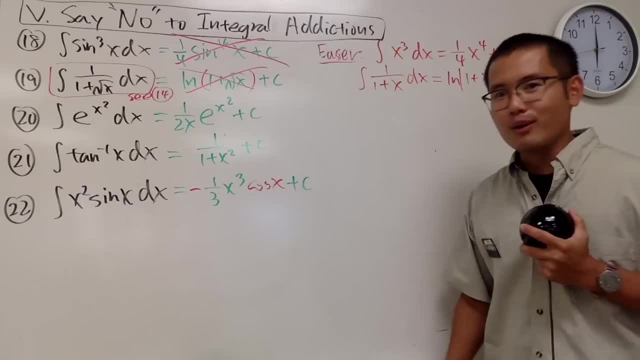 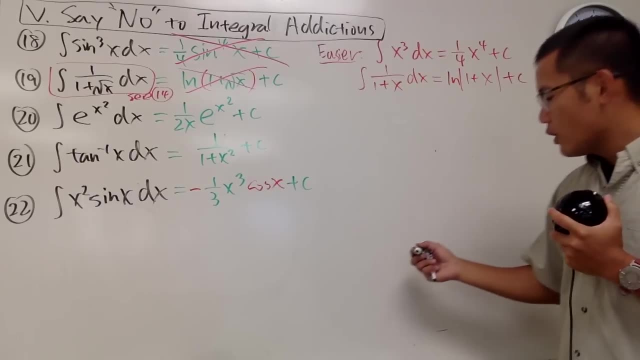 that mistake Right? This is so easy, but it's so wrong, I know. So this is the idea, And in fact, I will also give you guys some bonus on the side. So here are just some notes for you guys, okay, So some. 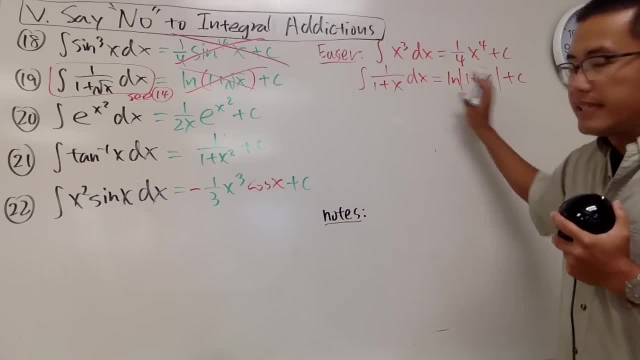 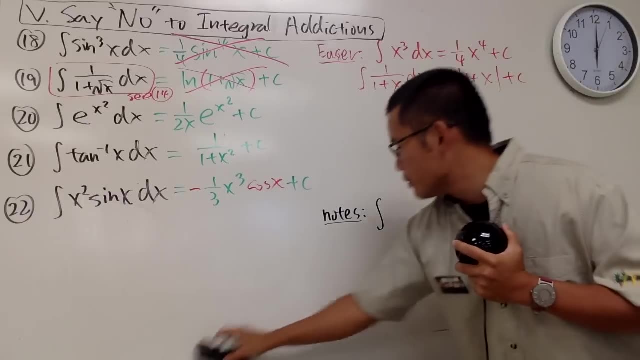 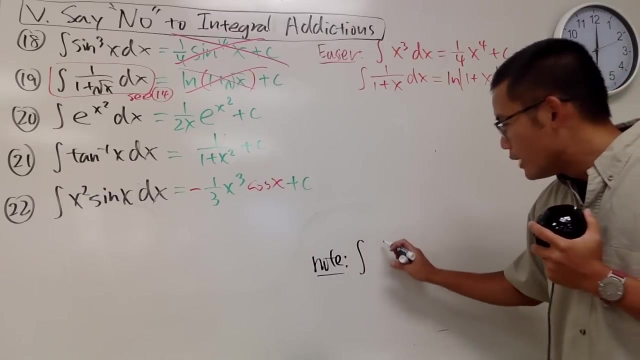 formulas for you guys To extend this idea, here is the formula we can use If we have the integral of 1 over. let me actually put it down right here. So notes: If we have the integral and if we happen to. 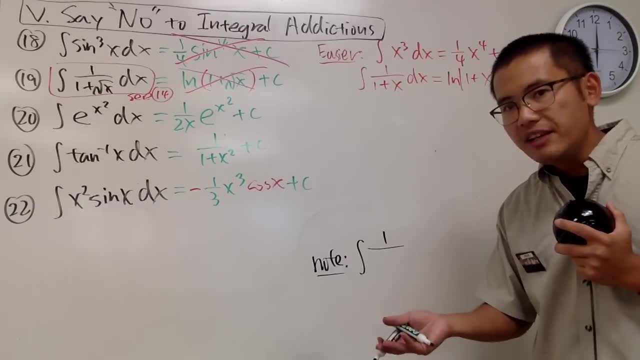 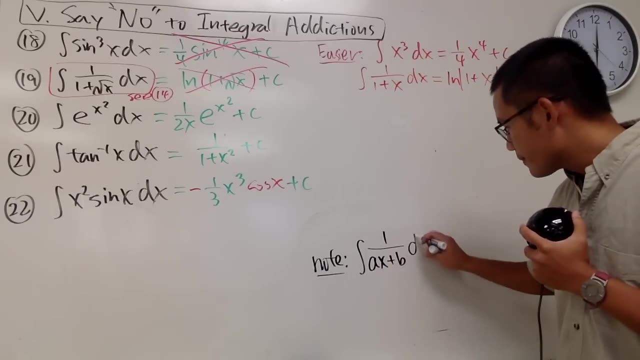 have 1 over if the bottom is just a linear function, namely ax to the first power plus b, and of course a cannot be 0, right This, right here. yes, we get a natural log and we can just have. 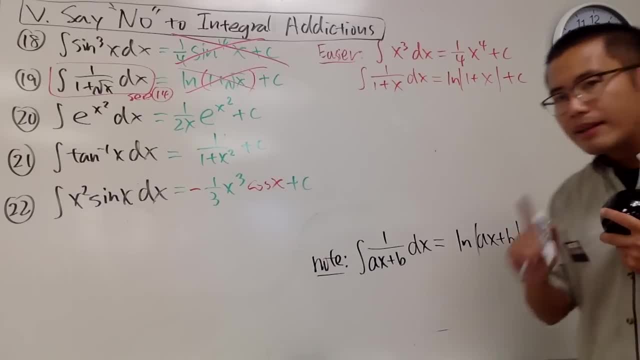 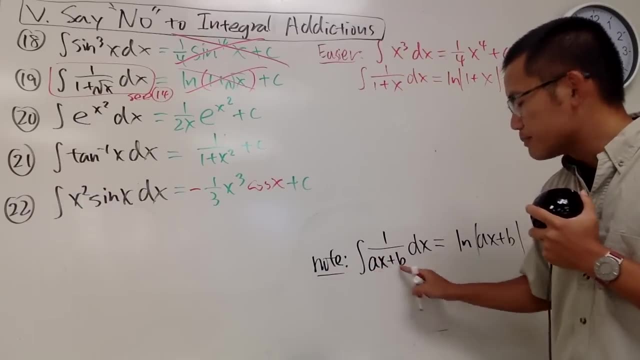 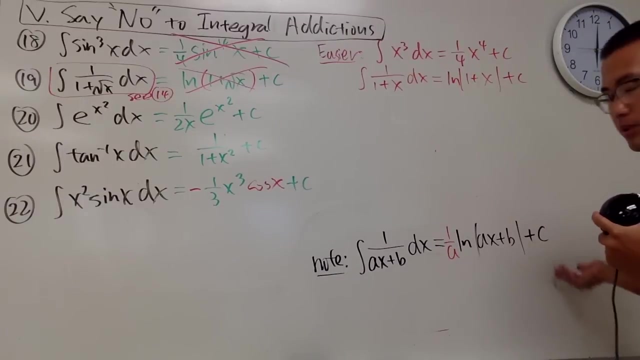 the ax plus b in the absolute value, like this, But don't forget to divide it by the derivative of the bottom. The derivative of ax plus b is a, and we have to divide it by that. So this right here will be a nice formula, of course, in the 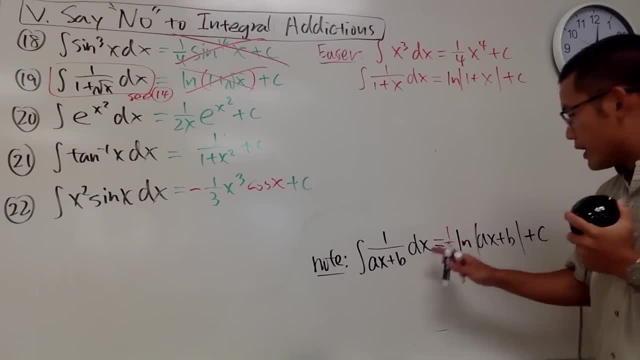 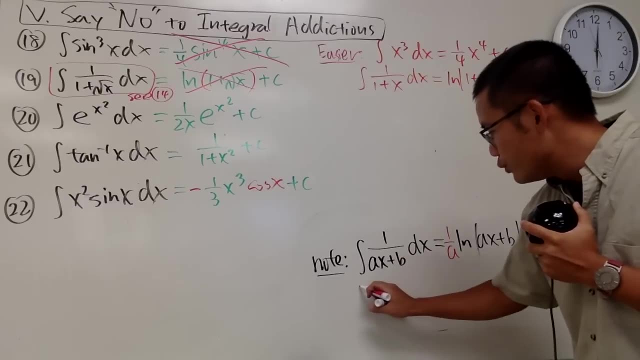 plus c, right, So you get this when you have 1 over and we'll be using this a lot. right Again, the reason we divide it by a is because if you do u sub u equals ax plus b. 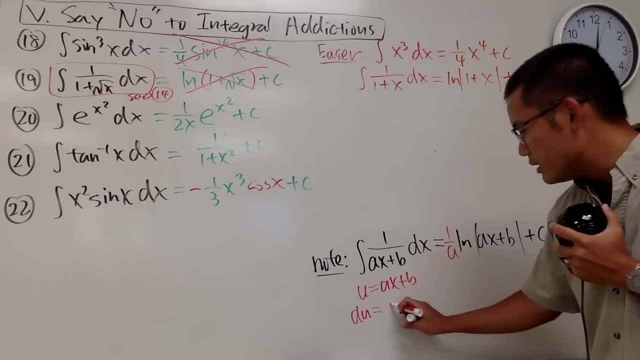 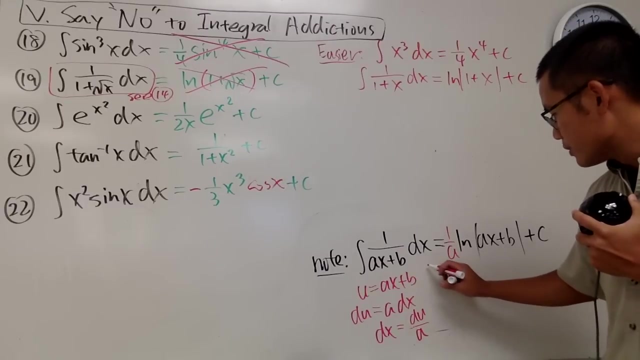 you get du equals. the derivative of ax plus b is a times dx. and you see that we have the dx equals du over a. And you see that this right here will just give you- let me just put this down right here- the integral of 1 over the. 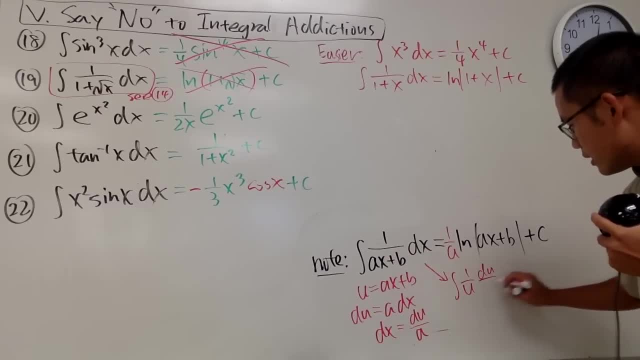 bottom is u and dx is du over a and notice we have the a right here. we can put that in the front and that's 1 over. so this is actually 1 over a, integrating 1 over u, du, 1 over a. 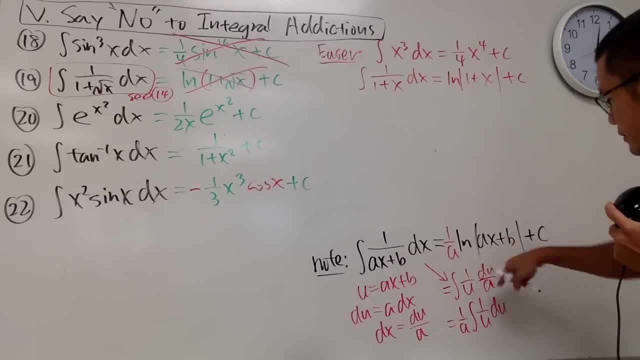 is right here, and then this will give us natural log after: the value of u and u is this: so just put it down like that. This right here is another formula that you should just remember, right, So you don't have to go through a u sub every single time. 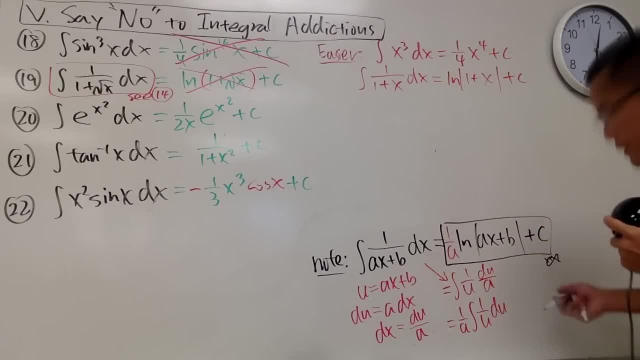 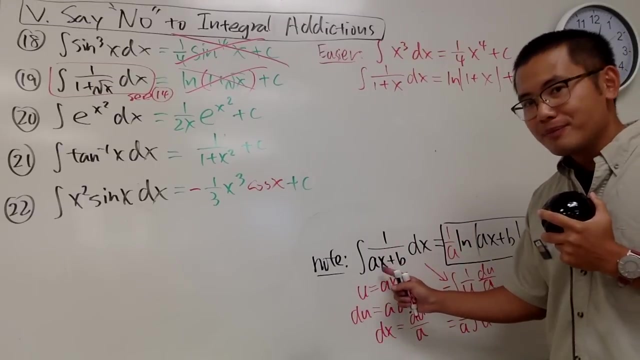 So this right here, is another fish right here. okay, Yeah, So again linear function. put it as natural log. after the value of that linear function right here, the top is 1, and ask yourself: the derivative of the bottom is what Which is. 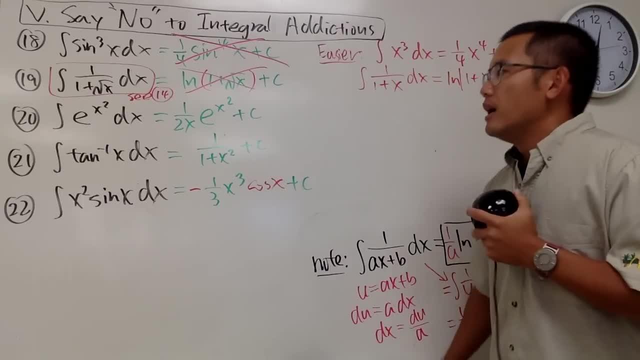 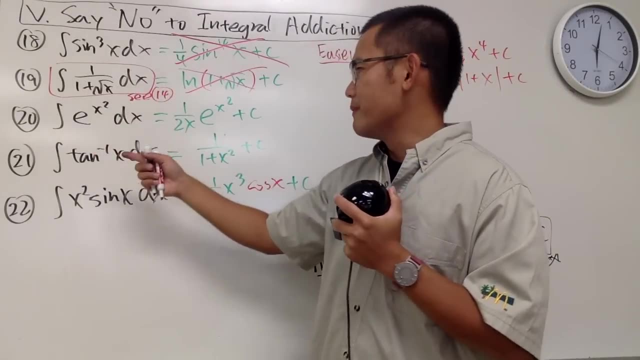 just a and then you just divide it by that. Alright, can we do the same thing for other functions, such as this one? Because that's if we start with it, okay, we have the derivative of x squared as 2x. 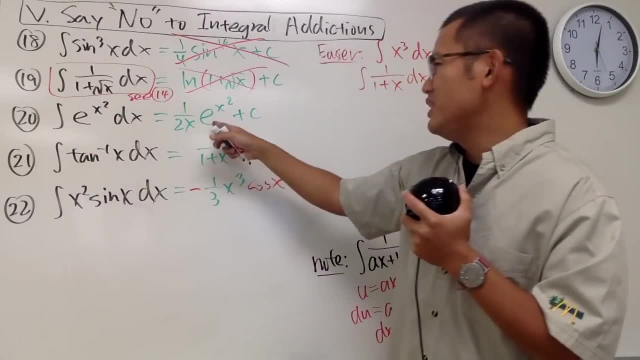 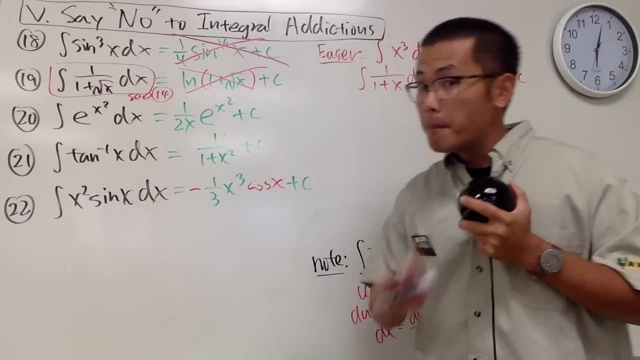 and the integral of e to the something should not just be e to the same thing and we divide it by the derivative of this right here because we're trying to reverse the chain rule. No, cannot do that. This right here is not correct. 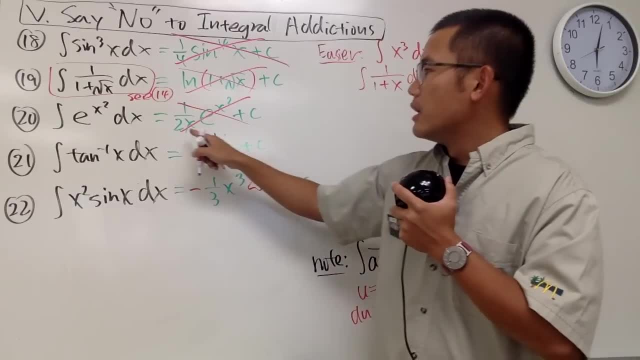 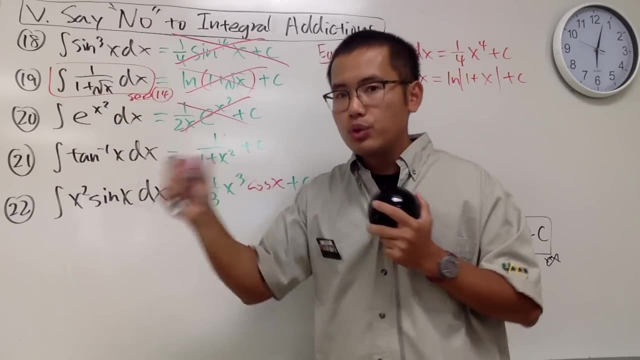 And the reason that this is not correct is because the derivative of 2, the derivative of x squared, is not a constant. The derivative of x squared is 2x and if you just divide it by 2x and you have this as the answer. 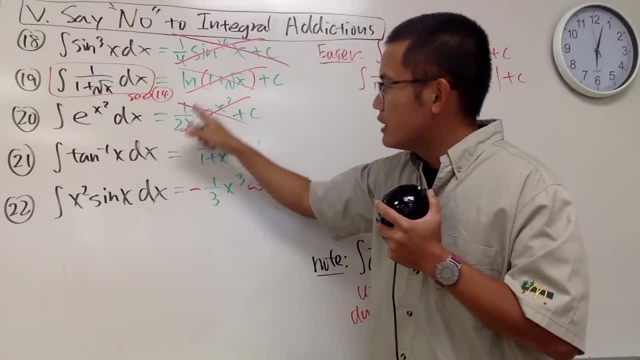 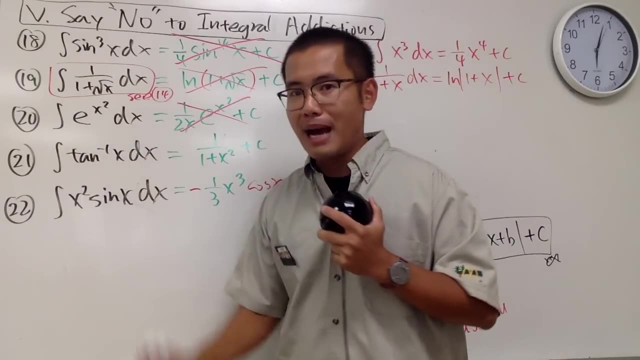 guess what, If you want to differentiate this, to check answer, you will have to use either the product rule or the quotient rule, and you will never get this back actually. So that's actually not correct. Here's the idea, though. 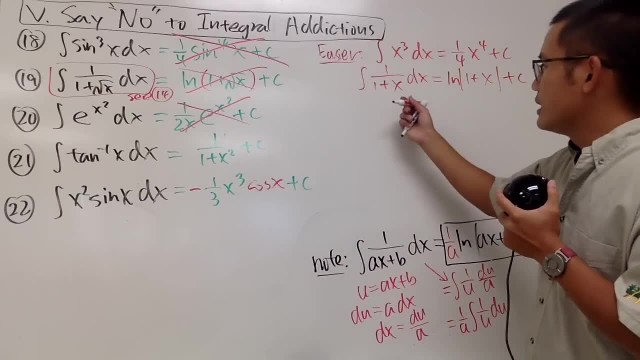 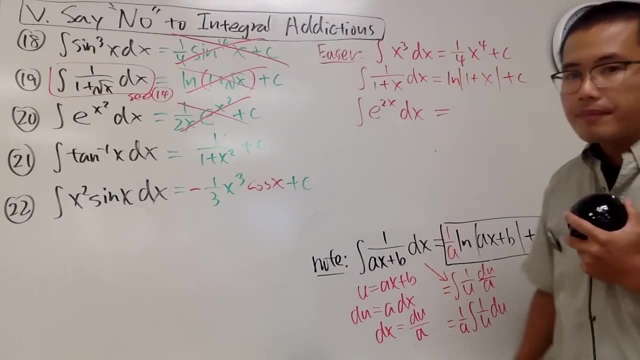 This question will be so much easier. so again, these are just the easier version. If you have the integral of e to the 2x, dx, right. If you have the integral of e to the 2x, this will be so much easier because you can just do. 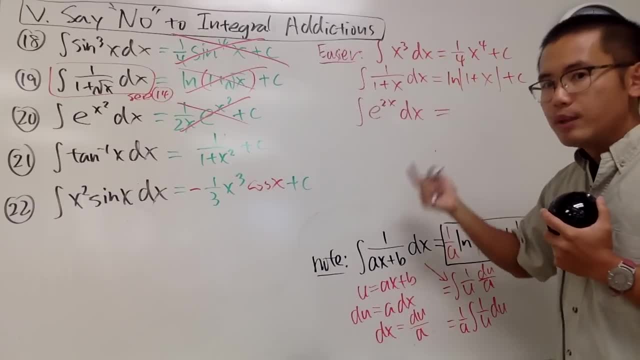 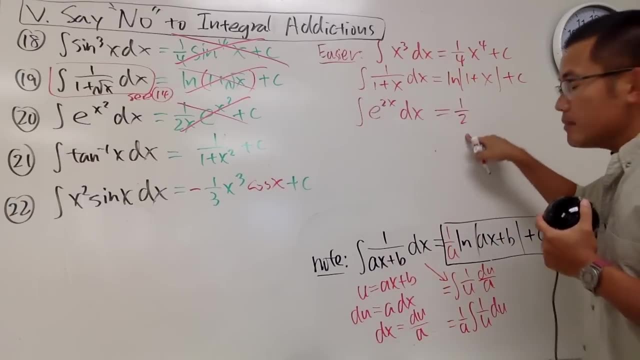 u sub, you can let u equal to 2x and the derivative of 2x is just a 2, right? In this case, you can't just divide it by the 2.. This is okay, You can just divide it by the 2.. And then: 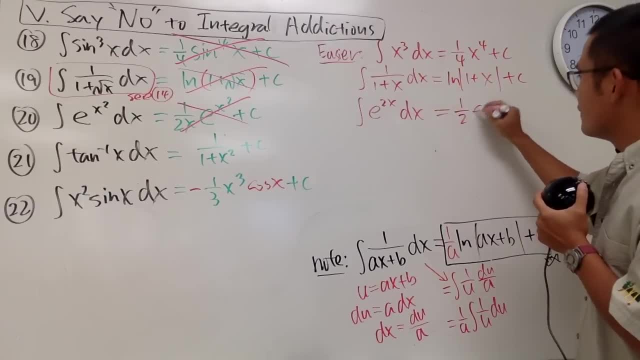 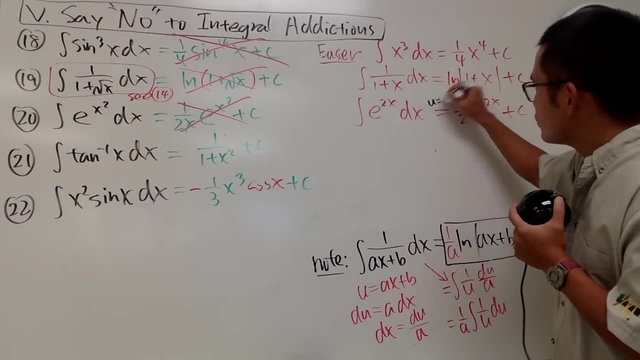 e to the 2x will just look at this as u. so you have e to the 2x like this, And you're done. This is okay Again. you just do u sub. let u equal to 2x, like this: 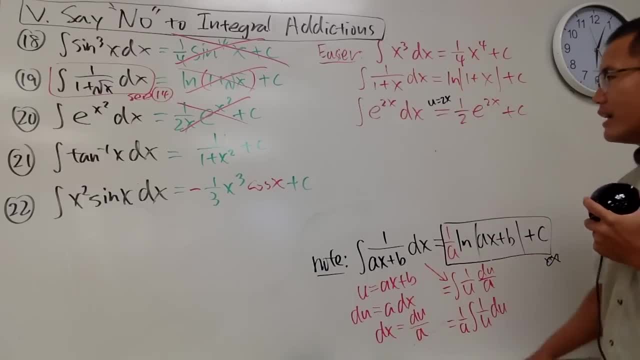 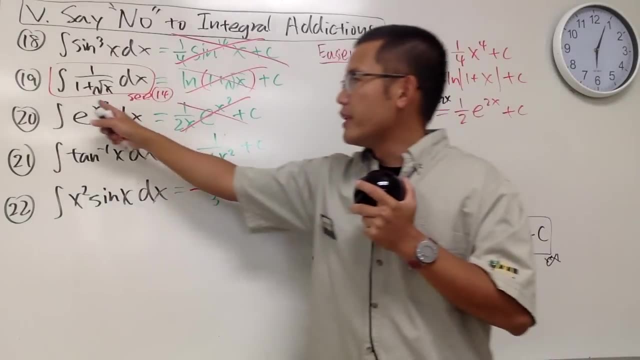 And, um, you might be wondering: okay, um, what's the difference between this and that? Again, the derivative of the input. if it's a constant, then you can just divide it by it, that's okay. but if it's? 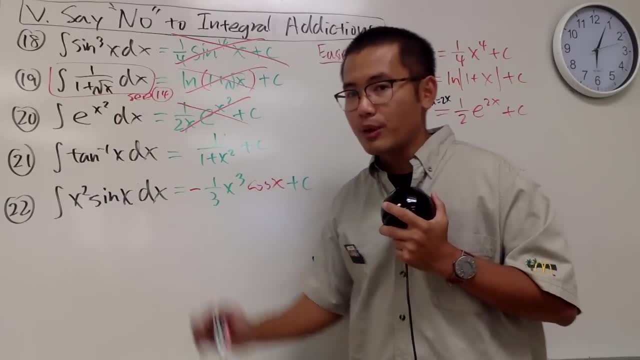 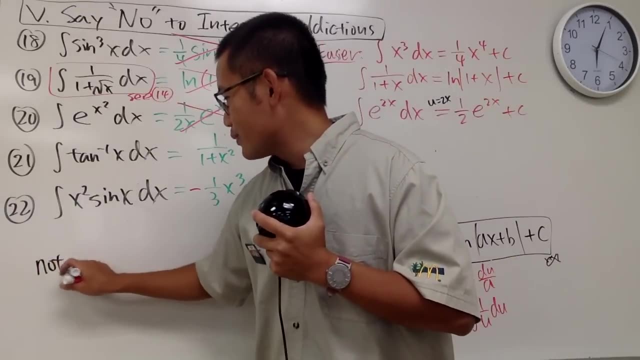 has a variable, you cannot just divide it by that variable. That's not okay. Again, I will give you guys another note so we can just write down a good formula. I think I'll just put it down right here. Why didn't I write down the formula? 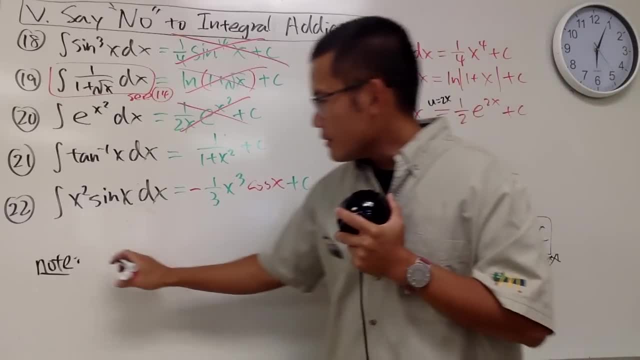 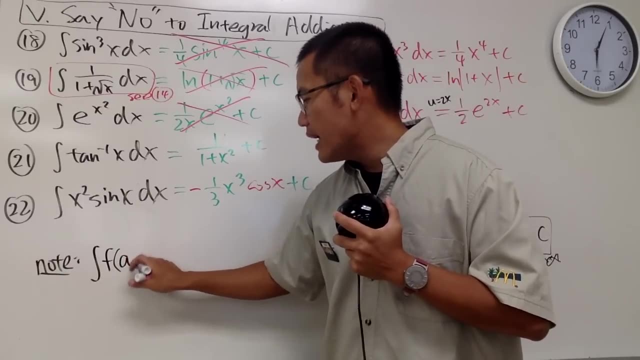 right here first. Anyway, here's the deal: When you have the integral, if you have a function, right, if you have a function, and if the input is ax plus b, like this, well, don't forget the dx, This right. 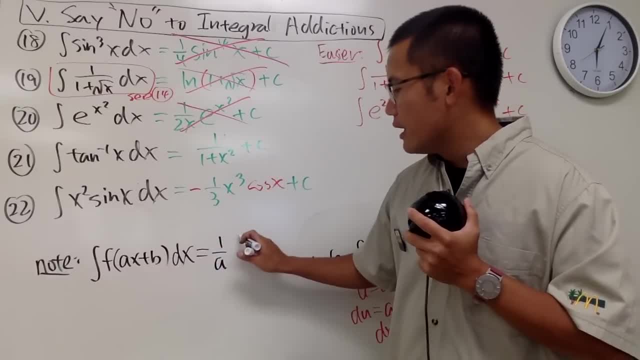 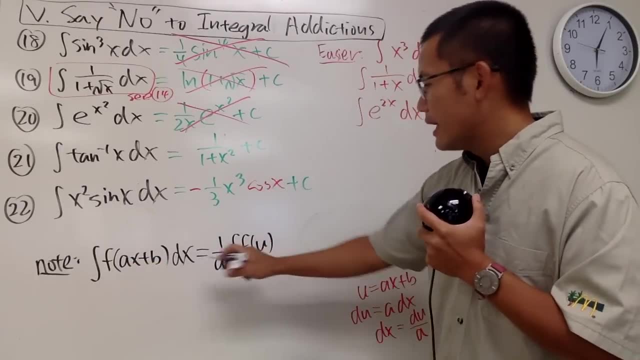 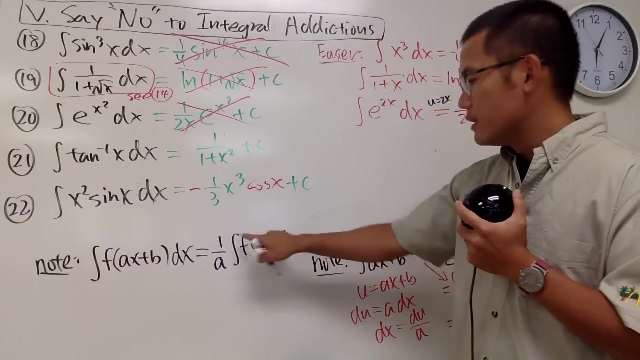 here is actually nicely equal to 1 over a integral of f of you. just look at the input as the u. so I have f of u and then du like this, And of course you just have to work out this formula. This is: 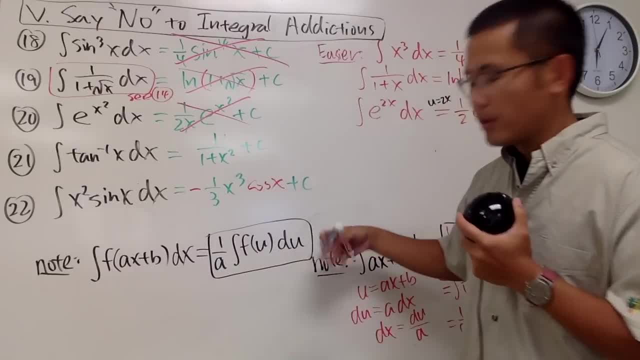 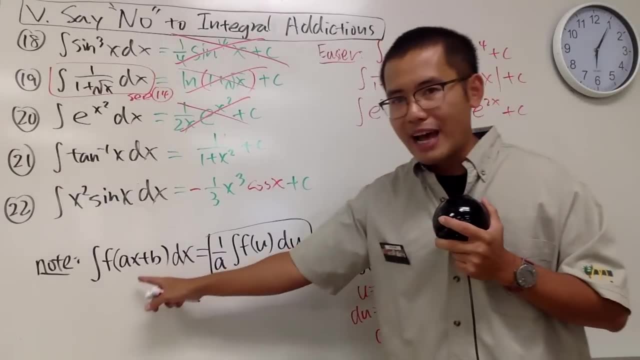 still an integral and in the end you're just going to, you know, work that out and then put it on plus c. In fact, this right here is just a specific example of that. So I guess this is a nice order. Now let me give you guys. 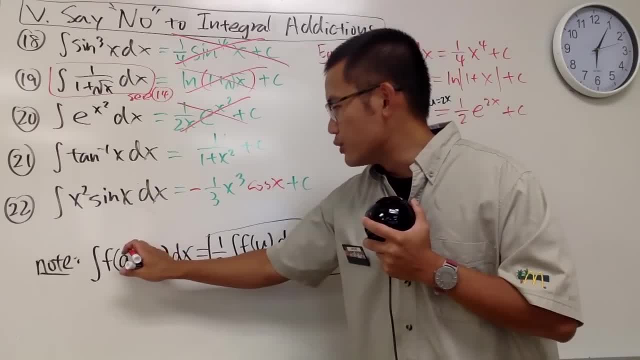 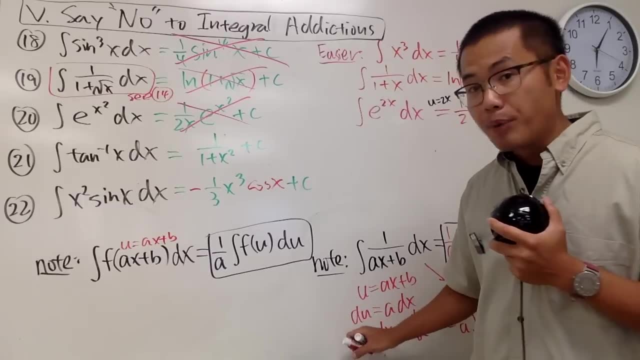 an idea. The proof of this is just that u equal to ax plus b, right, so you can just work that out. I'm going to leave that to you, but I'll show you, guys, some examples of how to use this formula. 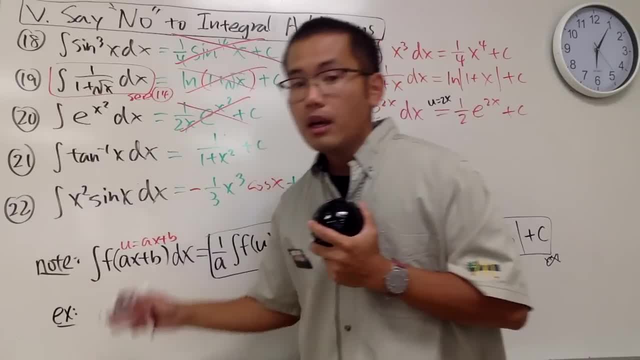 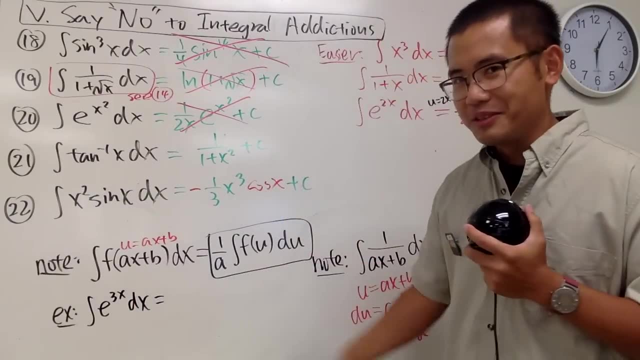 So here's the example: If we have to integrate e to the 3x dx- I know I did 2x and this is 3x. here's the idea. I look at this right here: 3x, and I ask. 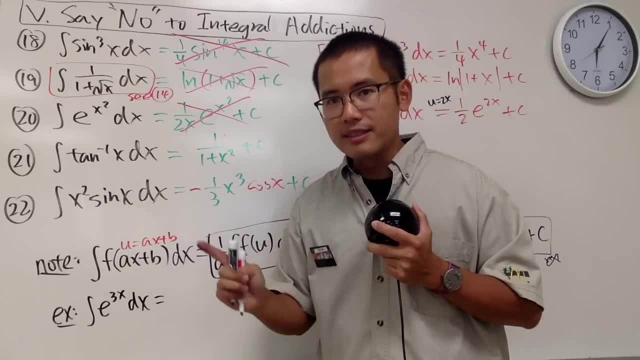 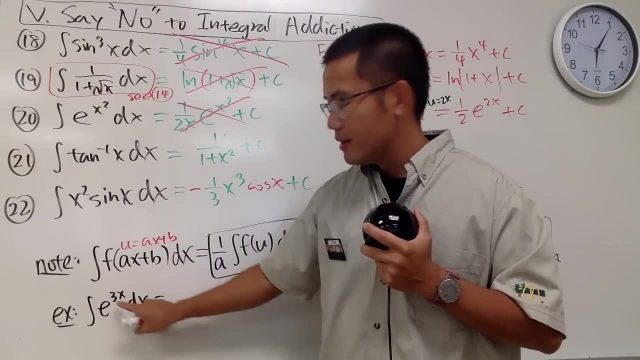 myself what's the derivative of 3x? It's just a 3,, which is just a constant multiple right. So what I do is I will just integrate e to the? u. it's like a block right here, which will give us 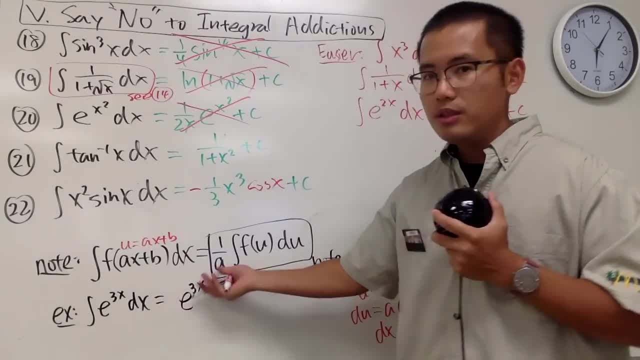 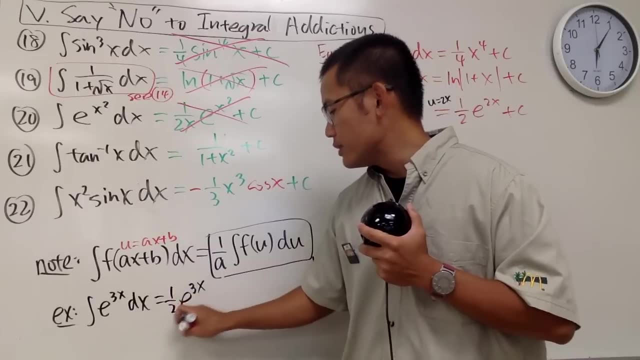 e to the same thing, right, e to the u like this, e to the block, e to the 3x. but I will have to divide it by the derivative right here, which is the 3, so divide it by 3.. So I get a 1 over. 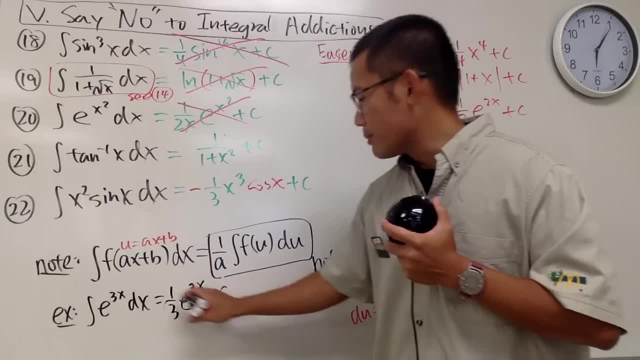 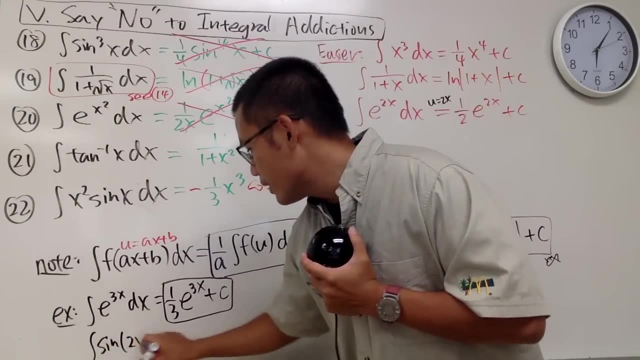 3,, e to the x, e to the 3x, and we're done plus plus c, Just like that. Another example: Suppose we have the integral of sine of 2x plus 5.. Well, this is how we do it. 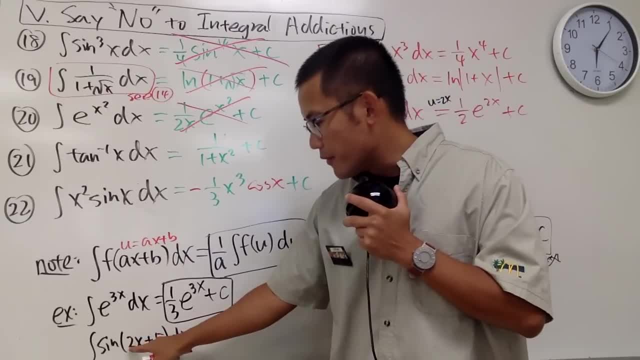 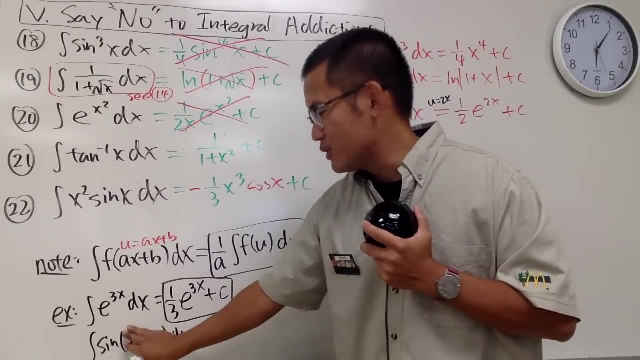 Notice that the input is just a linear function. the derivative of 2x plus 5 is just a 2, so we can do the following: Just don't look at it inside. just look at it inside. just look at it as a block. 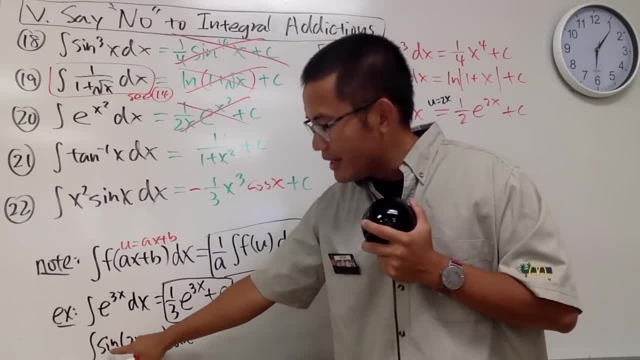 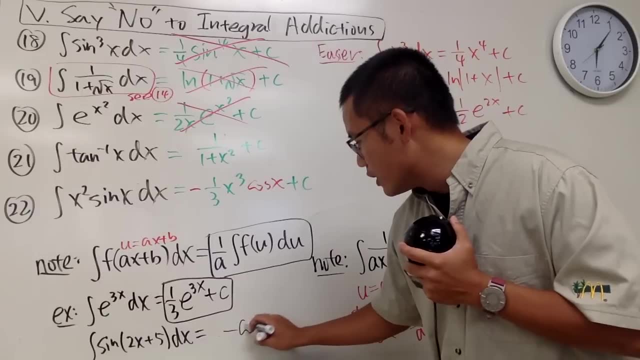 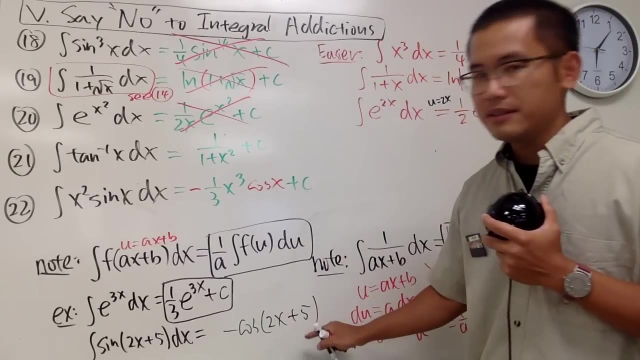 Ask yourself: what's the integral of sine, namely negative cosine, right? So when we go from here, we have negative cosine and you keep the input the same, which is 2x plus 5, like this. But you have to ask yourself: 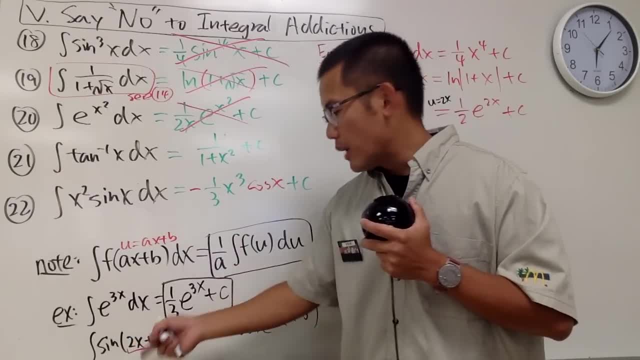 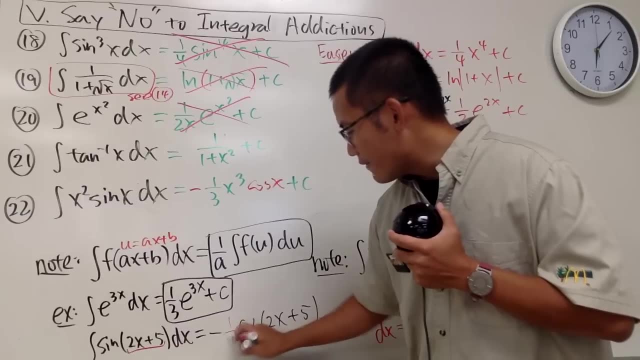 the derivative of the inside is what? It's just a 2.. And when you do it this way, because you are doing the anti-derivative, you have to divide it by 2.. So I will put down the 1 half right here. 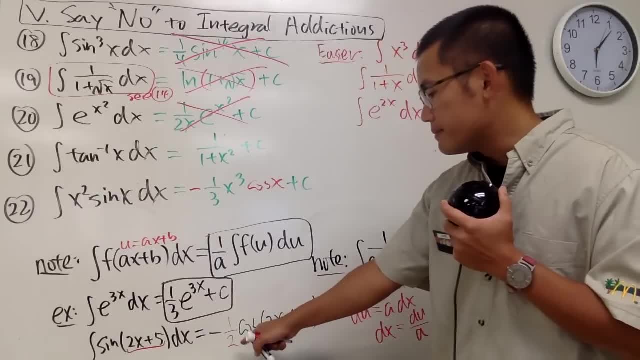 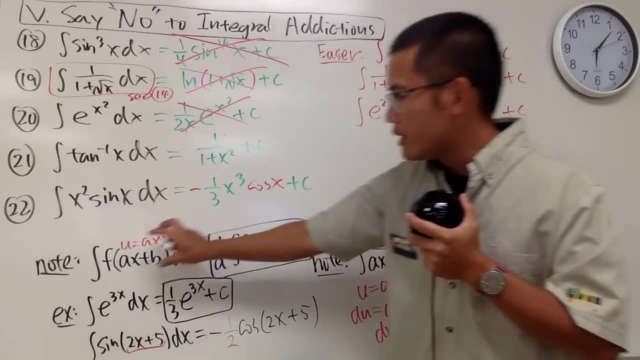 And of course that was still negative. but we just divide it by the derivative. right here, We can divide it by the derivative if the derivative is just a constant. That's what this formula is all about. Alright, So I put down the plus. 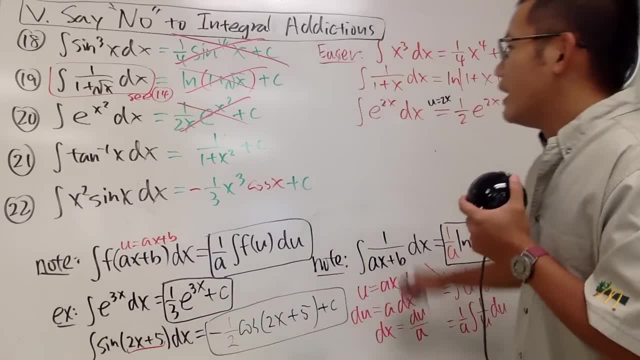 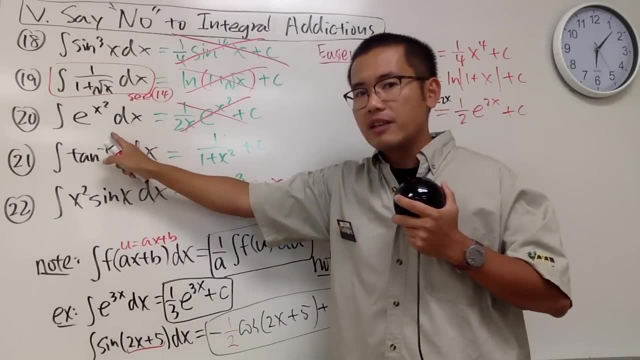 c: this right here is it for that, So that's why this right here was not okay. This right here is okay And I will tell you guys more about this kind of function coming up next for the category number 6.. Okay. 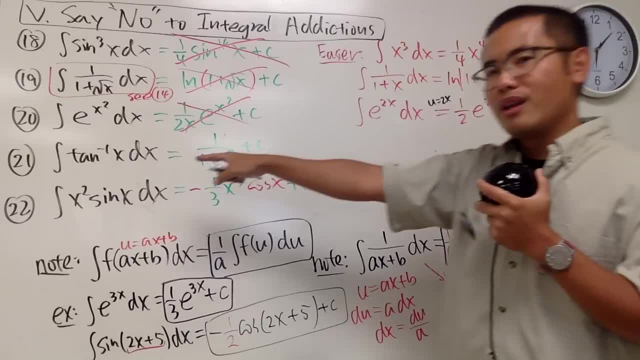 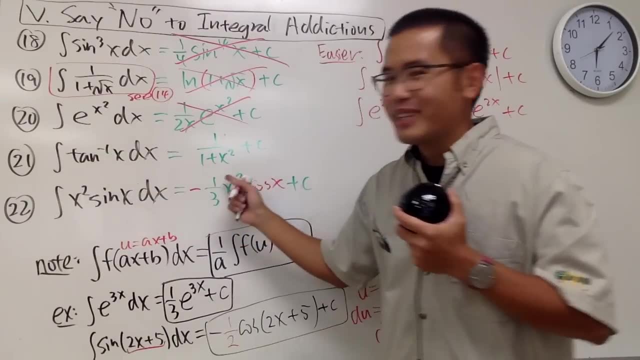 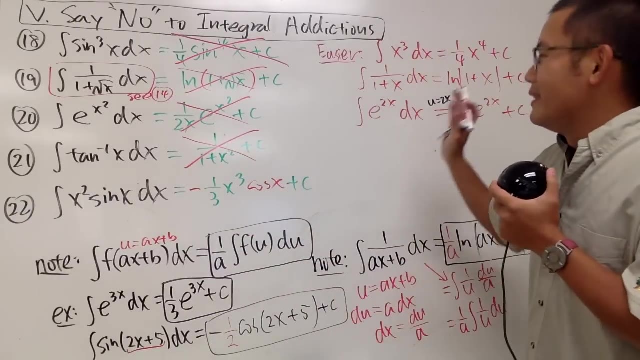 Number 21.. What's so wrong about number 21?? Yes, We are not facing the reality of doing integrals. This is just the derivative of inverse tangent. We are not doing integrals right here, So this is, of course, wrong. It would. 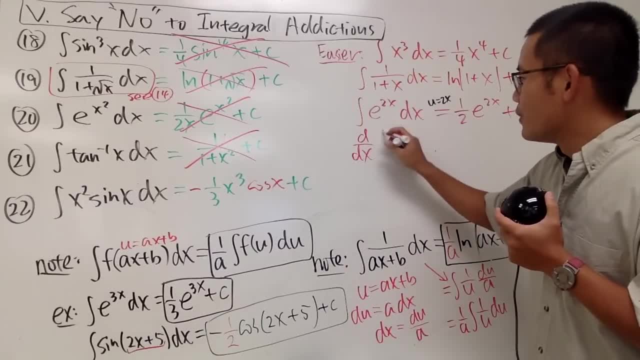 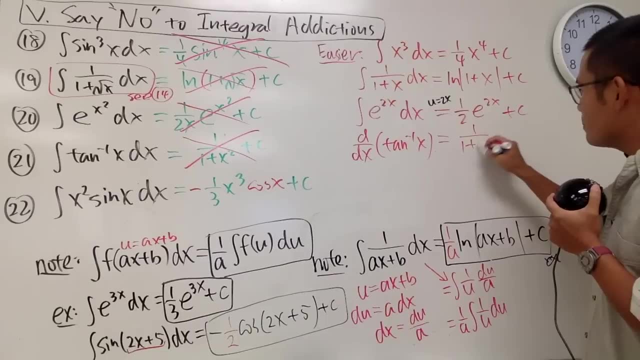 be much easier if the question is just asking us: hey, what's the derivative of inverse tangent of x? And if this is the question, then of course that's 1 over 1 plus x squared. I would totally agree with that. Do I need to? 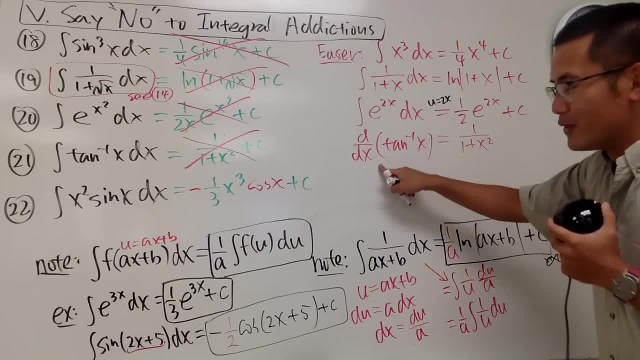 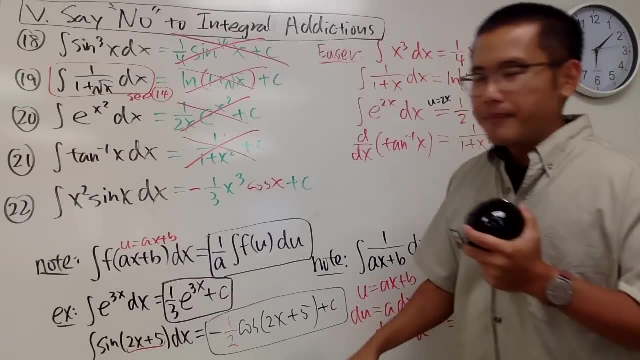 put down the plus c. No, Don't put down the plus c for derivatives. If you do put down the plus c, then we really have some integral addictions. Don't do that. Alright For number 22,. notice why this is wrong. 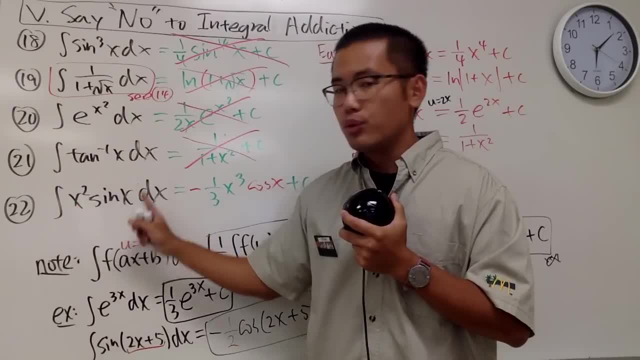 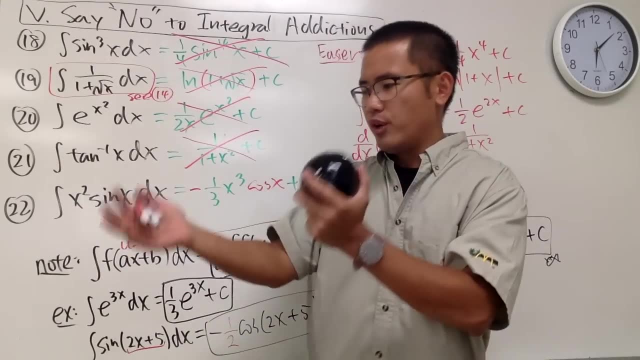 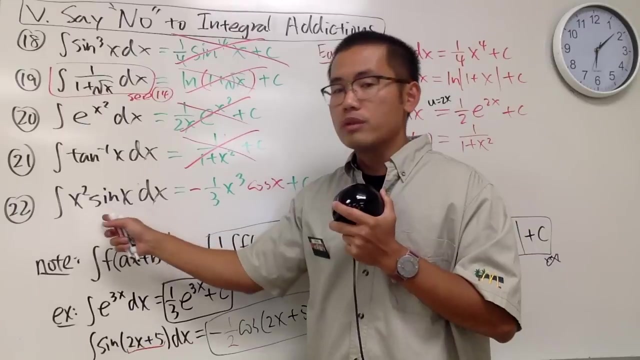 You see that we have a product of two things. Well, when we are doing the derivatives of a product of two functions, can we just differentiate the first and then times the derivative of the second? No, we cannot. Similarly, when we are doing integrals, we cannot. 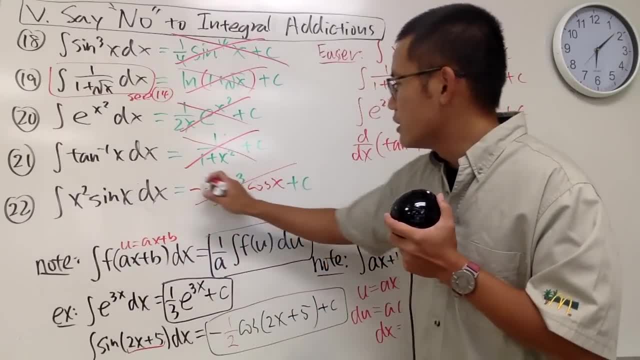 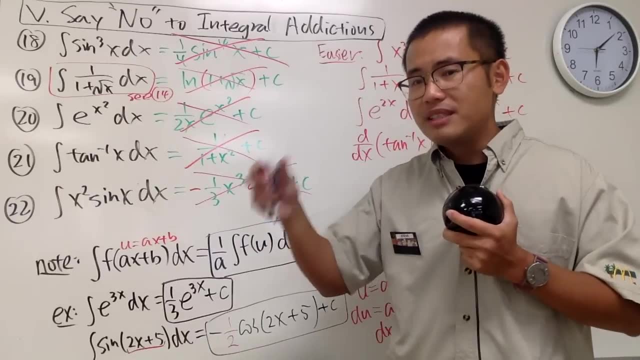 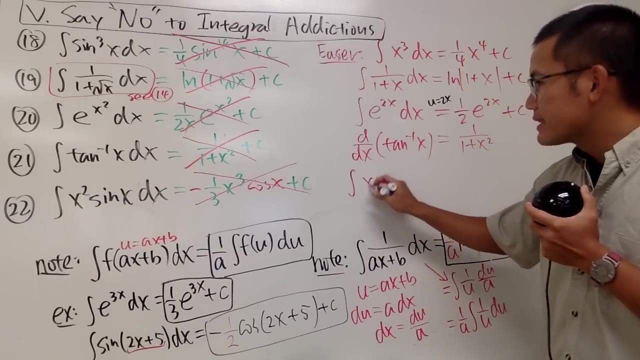 do so neither. So unfortunately this is not correct. We can only do like the, part by part or turn by turn if it's adding or subtracting in between. So if the question was the following: if the question was the integral of x squared, 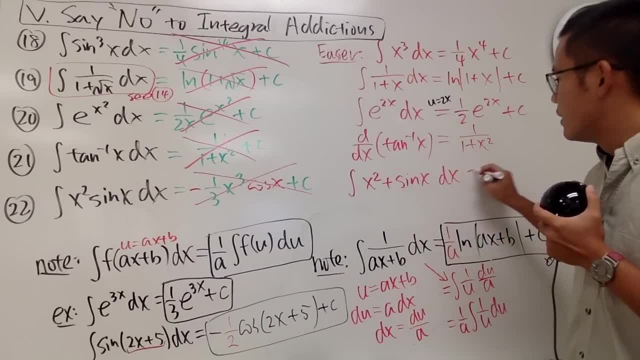 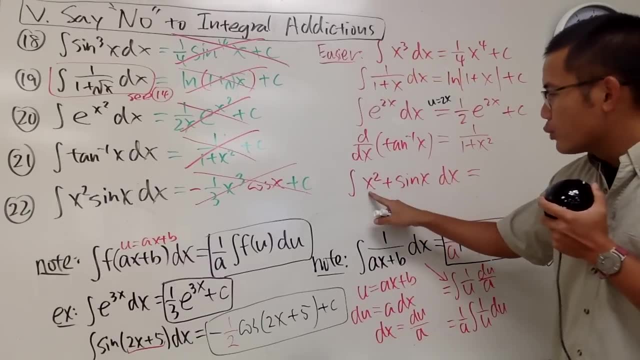 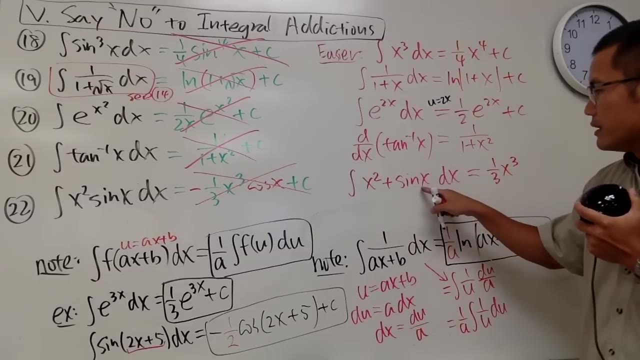 plus sin x, dx. if this is a plus or minus in between, then this would be so much easier because we can just integrate the first, which will give us one-third x to the third power, and then we combine with the answer from this part. 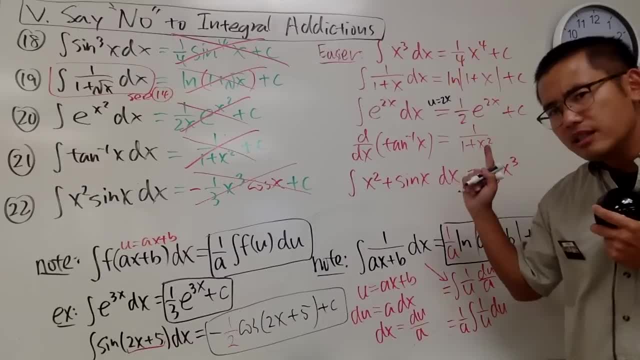 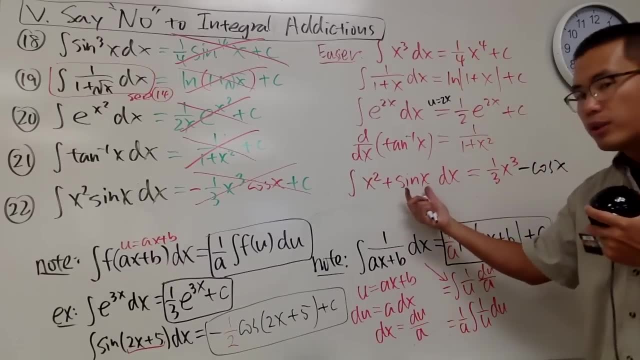 the answer of sin x is negative cosine. So we have the minus cosine x. Just integrate the first and integrate the second and put the results together, and for this don't forget the plus c. This, right here, would have been so much easier. 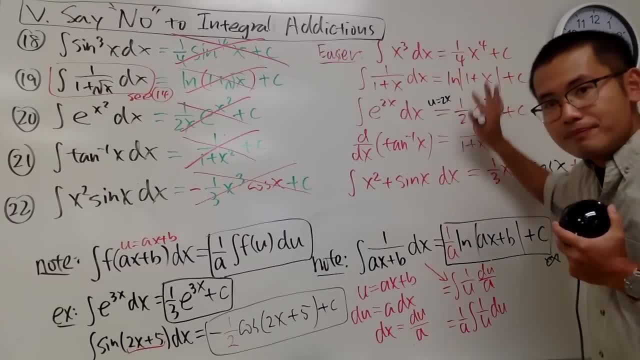 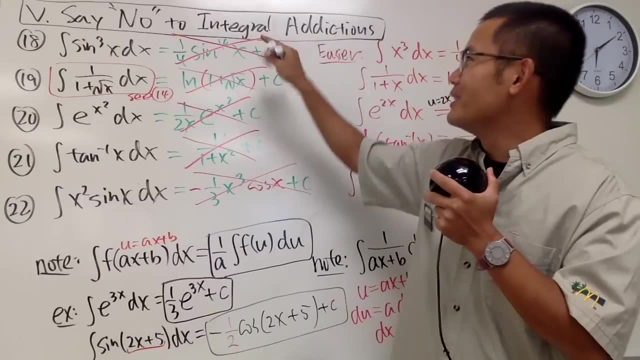 So these are the things that we like to do, But we cannot just do these kind of things for everything. No, That's why I call this the integral addictions. Right, Don't let this get you If you do this. 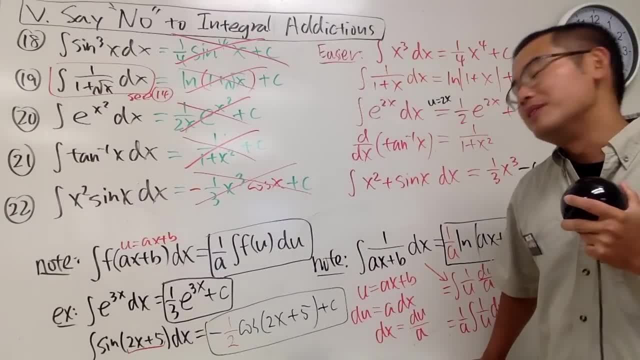 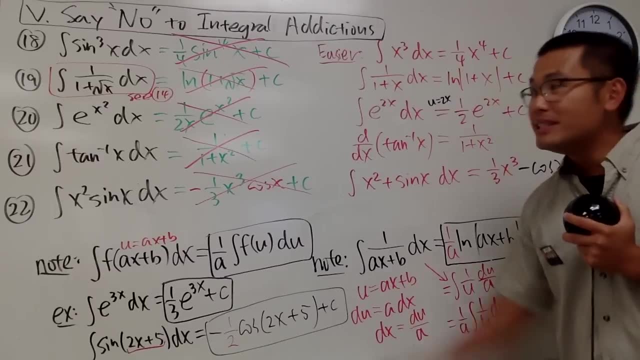 it would seem so nice, I know, but you would be so wrong. They are just so wrong, Right. So seriously, take a look of this board right here. This would really save your grade if you don't do that. So 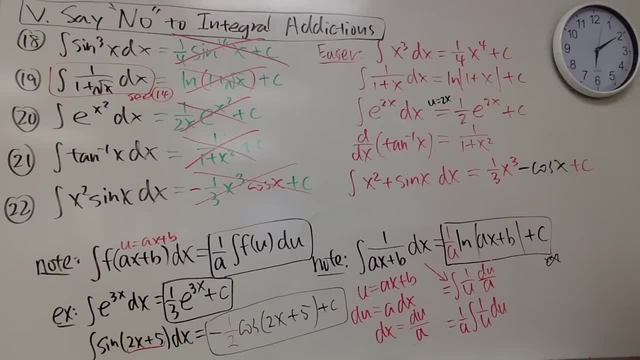 again, say no to the integral addictions. Alright. So how long has this been? I don't know, Let's see. Okay, one hour and twenty something minutes, Not so bad. Yes, we are done with the twenty two questions. but 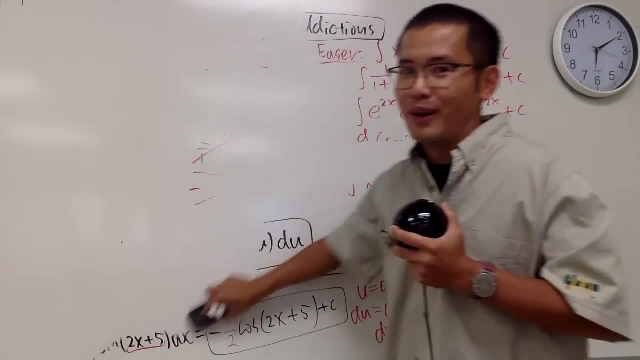 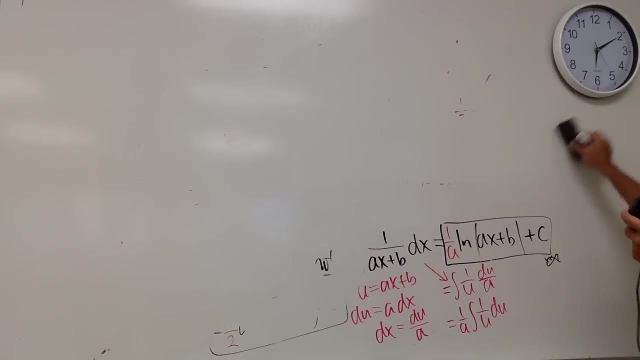 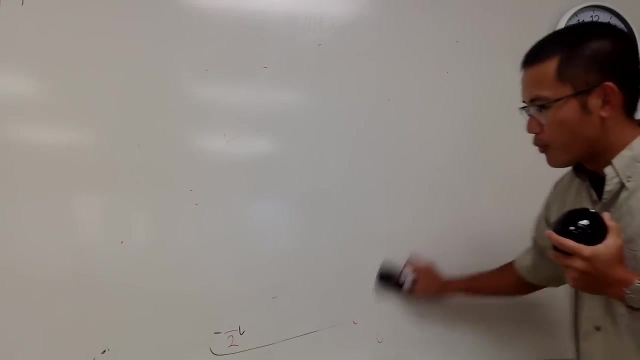 the new techniques and the longer techniques are coming, so I'm not extremely happy because the later ones are actually the harder ones. But hopefully you can see that everything that we are talking about is all built up from the previous knowledge, So in 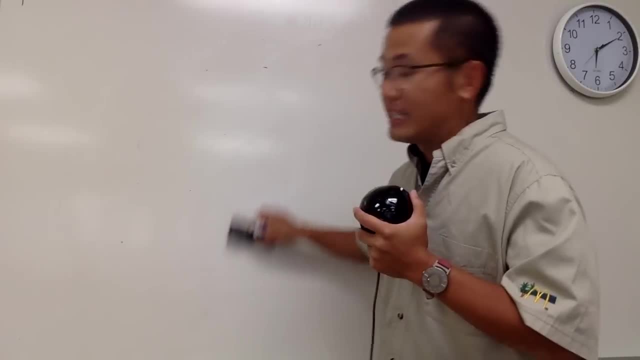 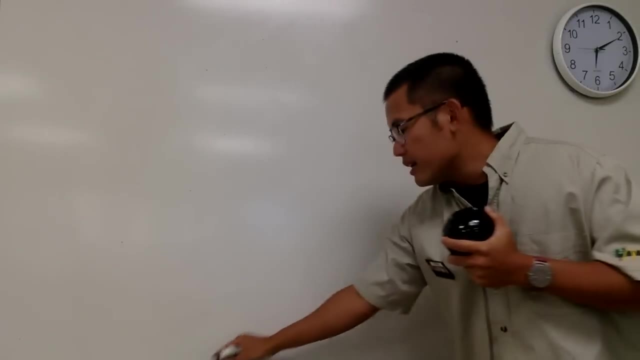 order for you to do category number seven. we better know category number one, two, three, etcetera, etcetera. Okay, So that was the integral addictions. I have a separate video on that if you guys want to check that out. 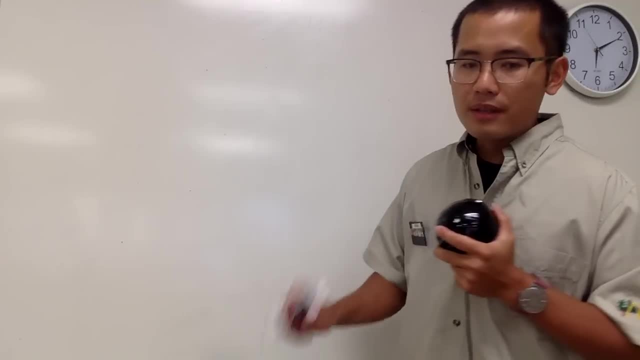 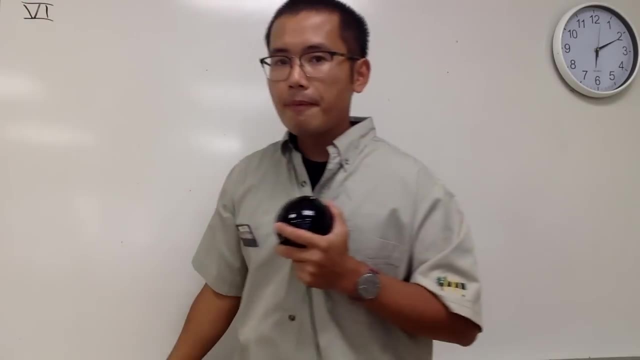 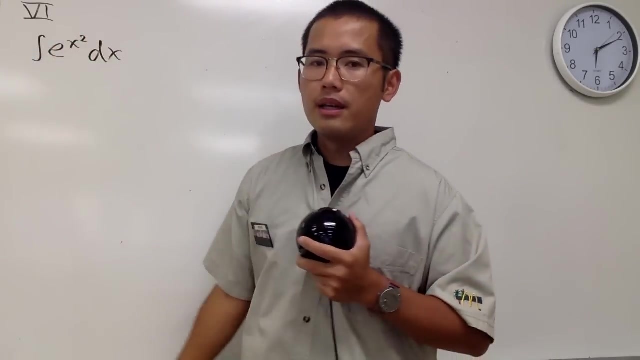 Now let's talk about the following. This is number six, Category number six, So it looks like this. Right Here is the deal. Earlier we saw that we have the integral of e to the x square dx And, as I told you, 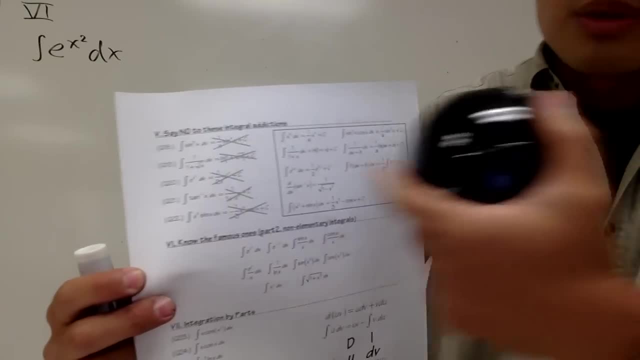 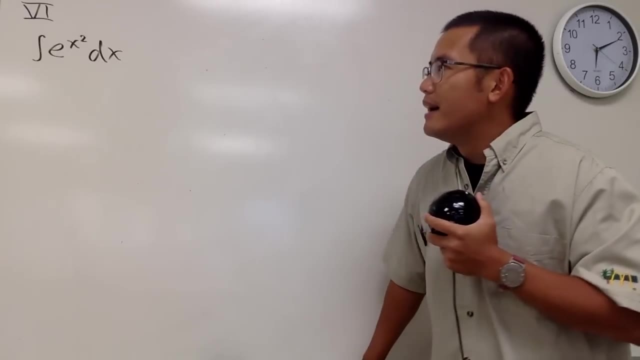 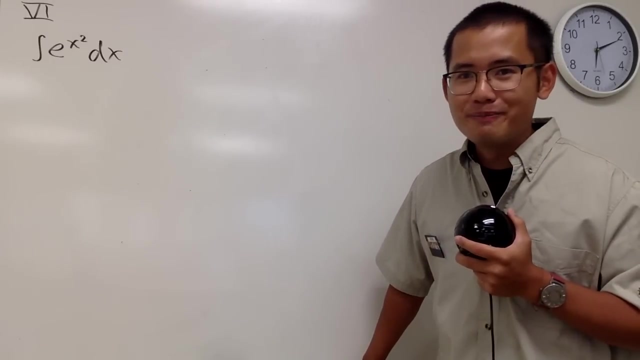 I'm going to show you guys the correction of how to do all these integrals. okay, But for this particular one, in fact, no matter what we do, we cannot find out the answer for this because it has no answer. That's all. 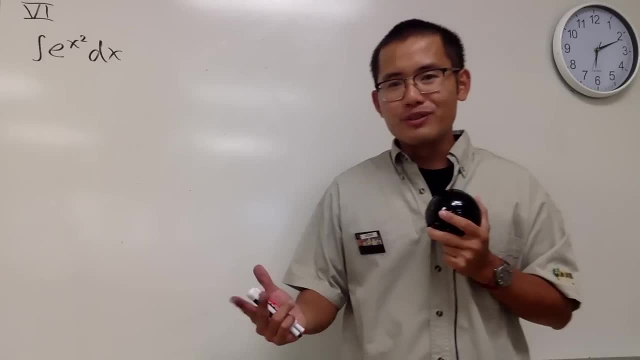 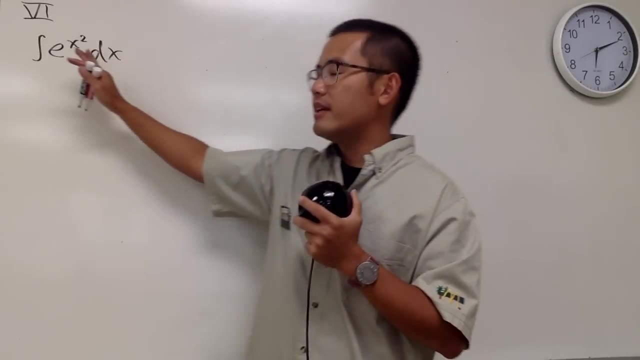 I'm sorry I had to break this news to you guys, but sometimes when we are doing integrals, unfortunately no matter which technique, which method we use, but we just cannot find an answer for this Right. So for this category. 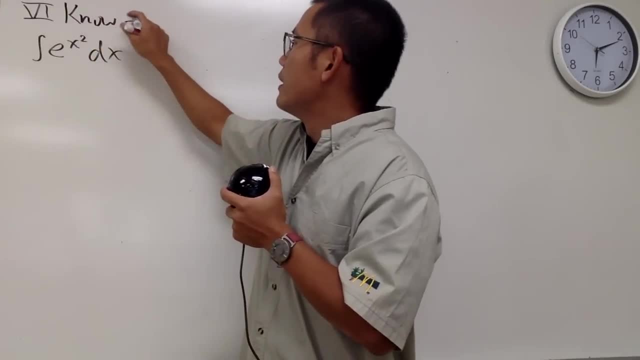 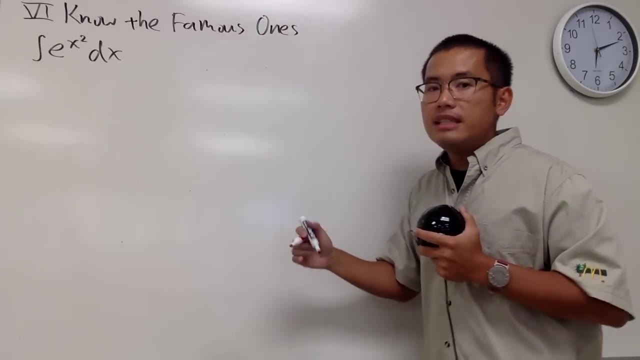 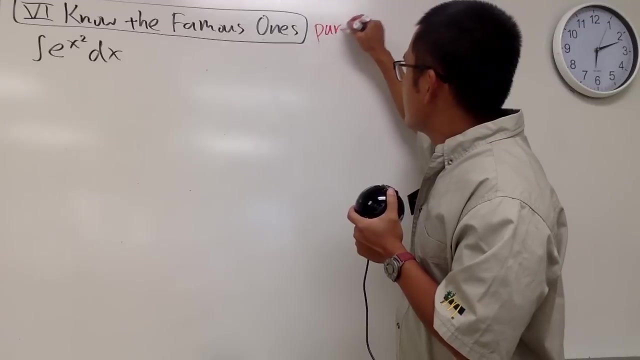 this is the second part of know the famous ones, And this is the part two. So let me actually just put this down right here. Right, So here is part two. And for the part two is that I would like to tell you guys. 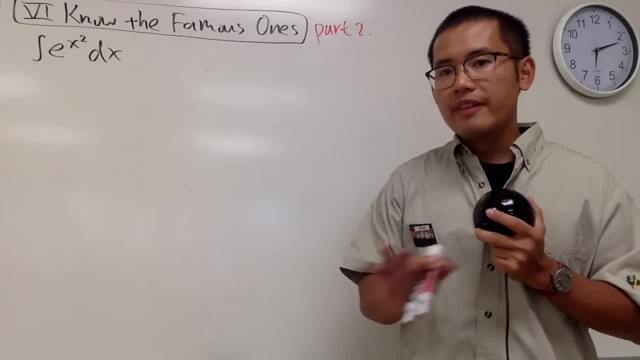 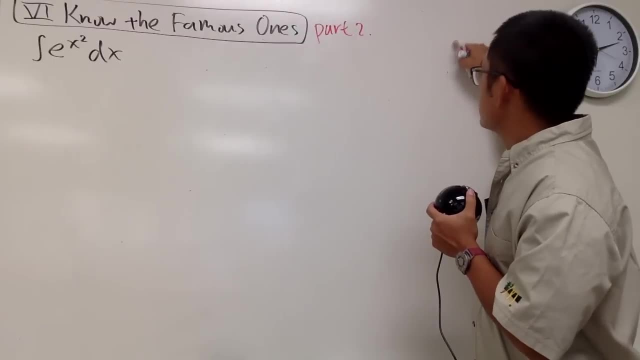 some of the famous integrals that they don't have an answer to And technically I should say the following integrals: they are what we call the non-elementary ones. So I will just tell you guys know the non-elementary. 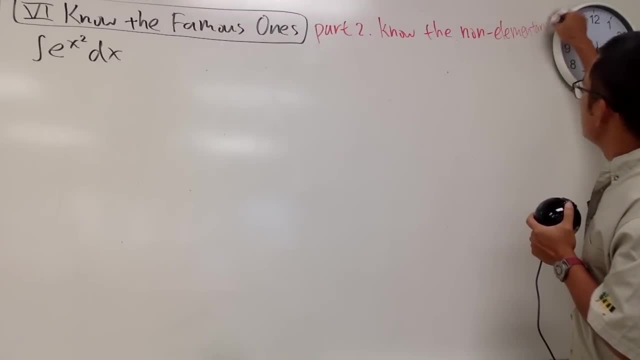 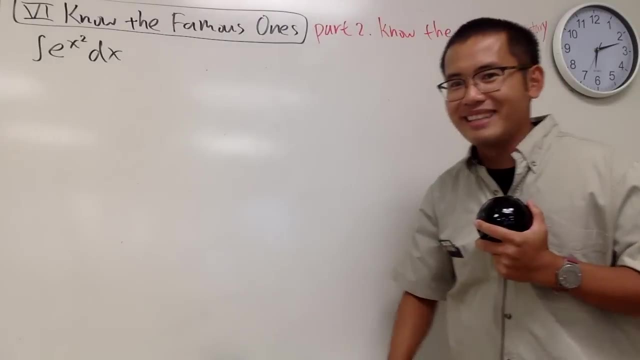 ones, Right? Hopefully you guys can see this. okay, Sorry about my handwriting, But it's on the PDF, so just go to download that and see that It will be much better, Alright, So first of all, let me explain the term. 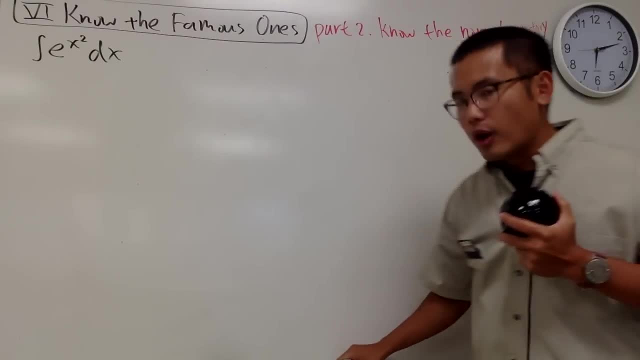 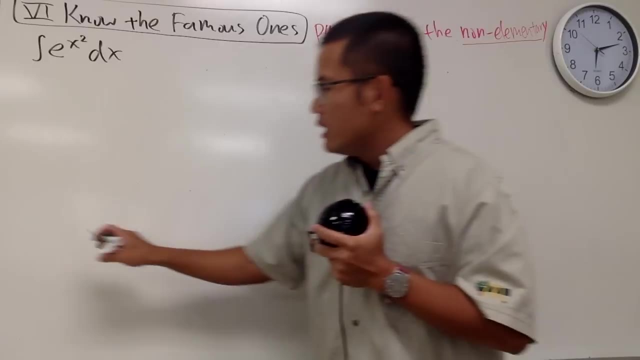 non-elementary. And to do so, let me just kind of use an example that we have talked, that we did like in the algebra class or so, If you look at square root of nine, for example, from the Google days, of course, 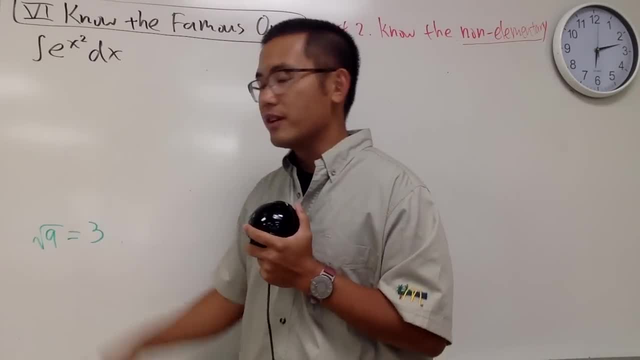 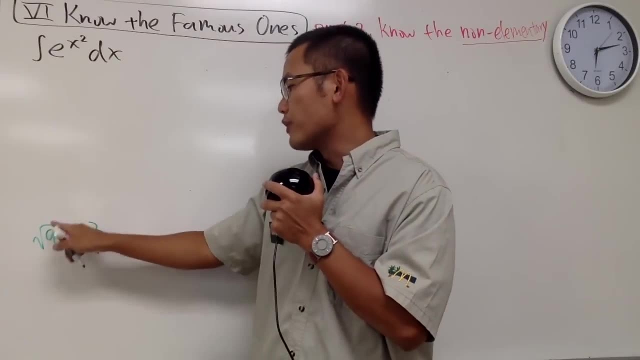 this right here is just equal to three, because positive three times positive three will give us nine. The answer is not negative three, even though negative three times negative three will also give us positive nine, but we define the square root of nine to be positive three. 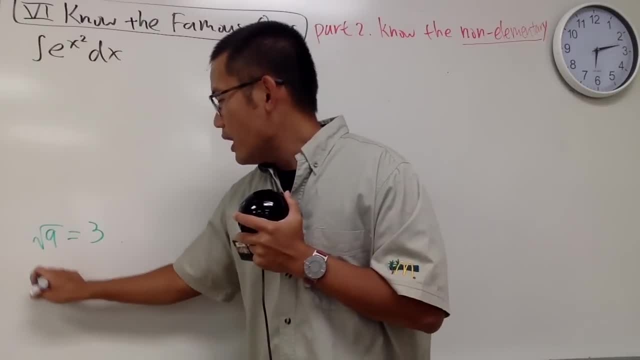 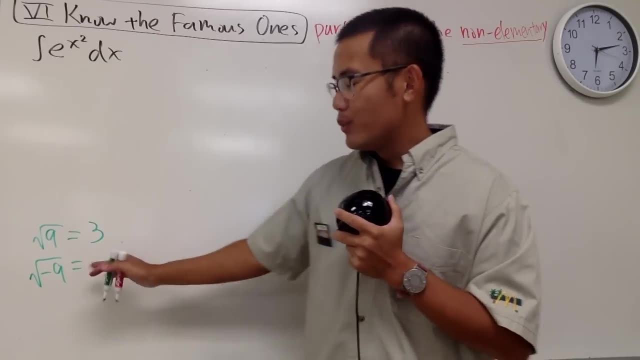 So that's it. But square root of negative nine. this right here is equal to what? Well, I know some of you guys want to say we have three i, But if you think about it before, complex numbers. 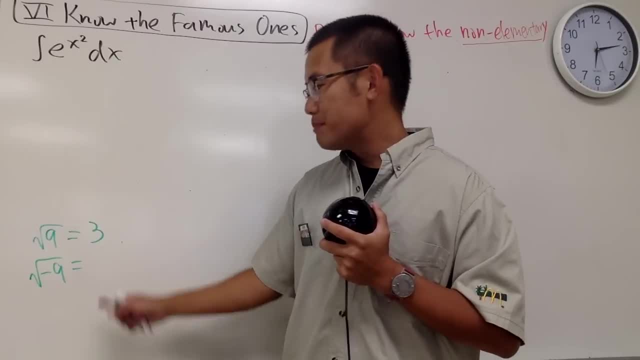 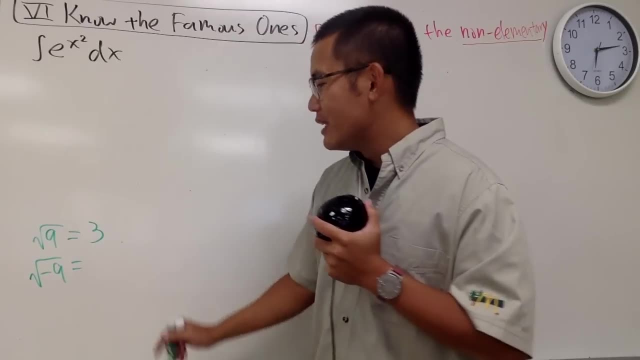 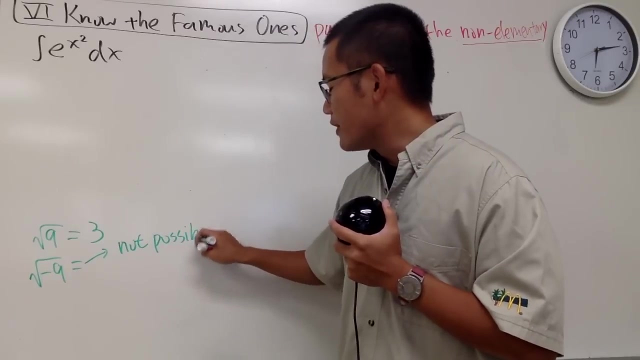 how would you answer this? Is it possible for us to find a number multiply itself, to get negative nine, In fact? it's not possible. So the first way that we can answer this is that it's just not possible. We cannot have a negative. 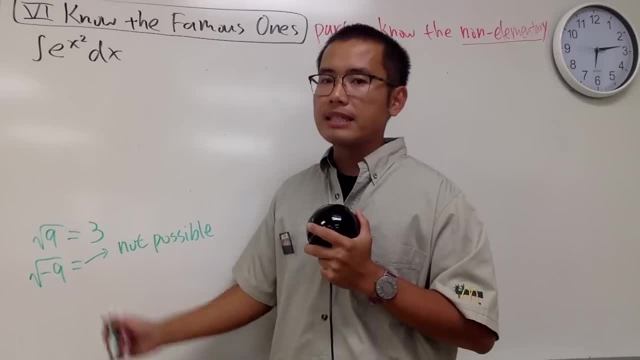 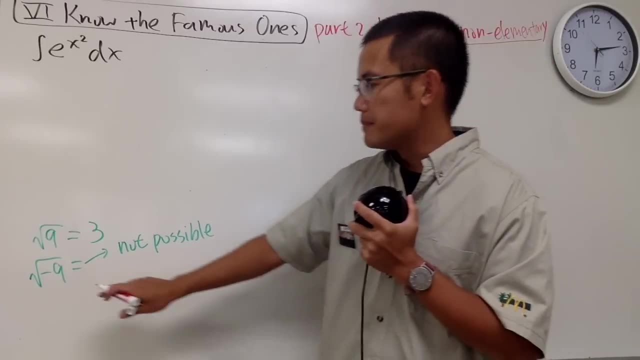 number inside of the square root. This is not possible, But the truth is, in fact we can use what we call the complex numbers, and that's how we kind of extend the idea of the square root numbers right here. so we can continue. 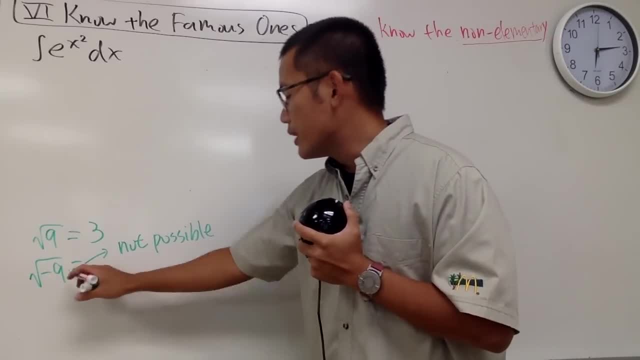 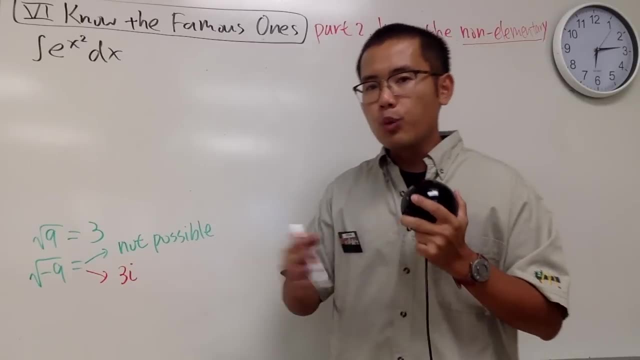 with our studies. So another way to answer it is we can say: this is equal to three i And this is not really not possible. It's just depending on which stage of the study that we are in Before the complex numbers. 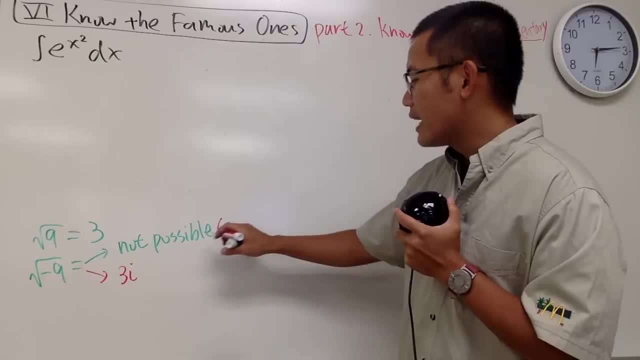 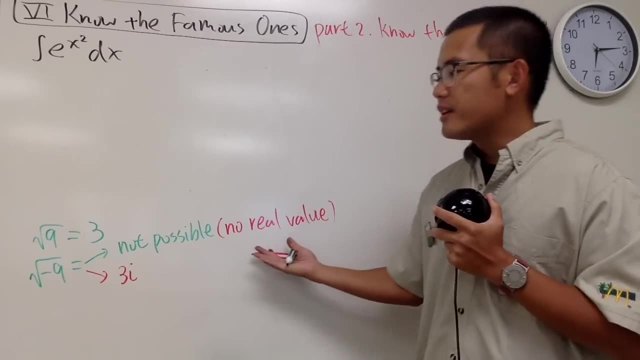 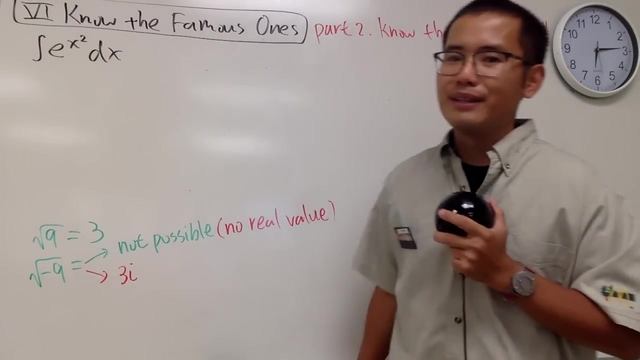 we would say this is not possible. but technically we should have said that this, right here, is what we call the non-real value. This would be a technical way to answer that, Because it does have a non-real value, namely three i. 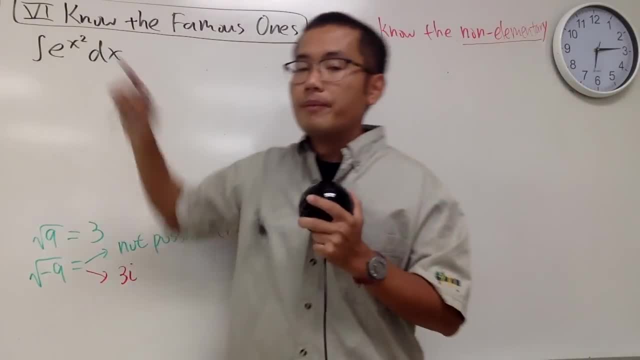 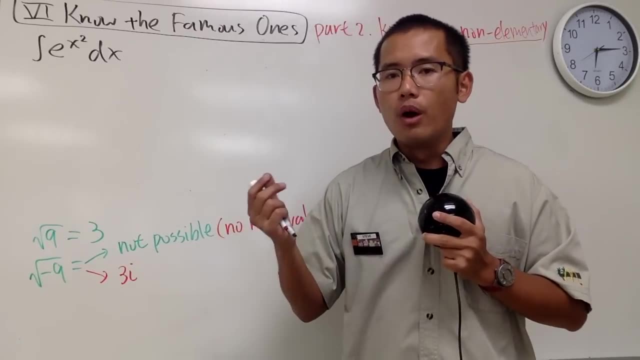 Now, here is the idea, This integral. no matter what we do, we just don't have our answers in the sense of by using our usual technique or our usual functions, such as e to the x sine cosine logarithms powers. 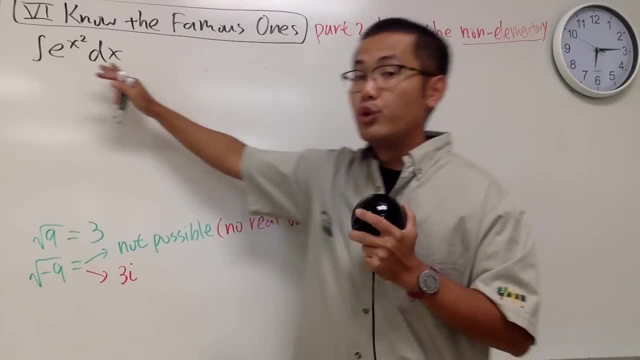 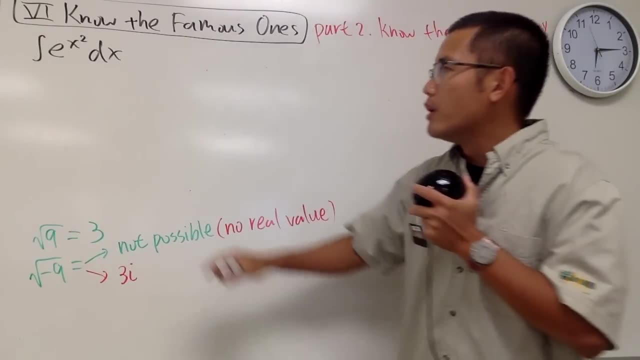 and whatever you can think of. But we do have special functions for this answer right here, But we are in Cal 2.. So here's the deal For Cal 2, when you see this kind of integral, no answer, That's all And the technical way. 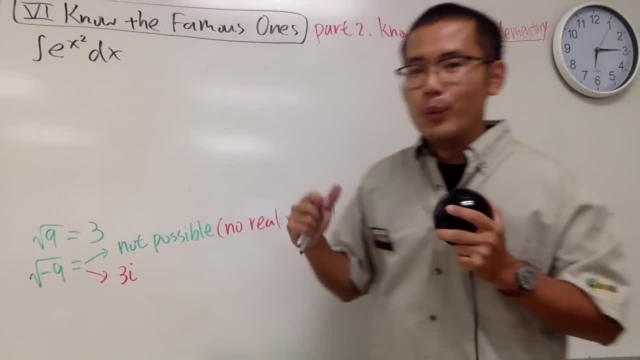 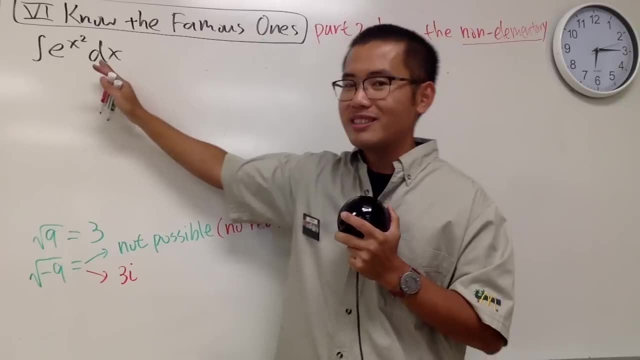 to answer that is non-elementary Because, again, we can use special functions to answer this right here. And if you guys are interested, you guys can watch my other video for the special functions right here And let me actually give you guys. 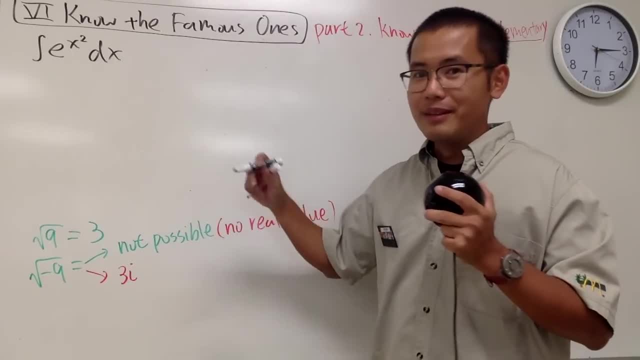 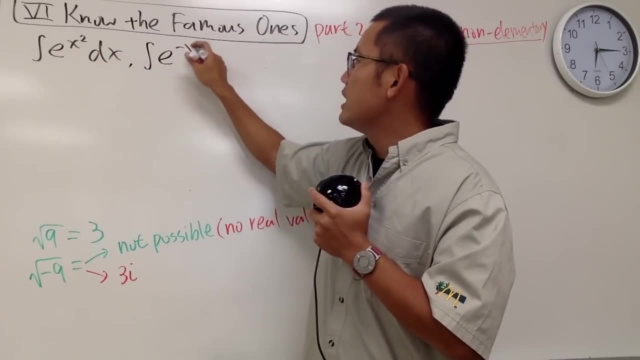 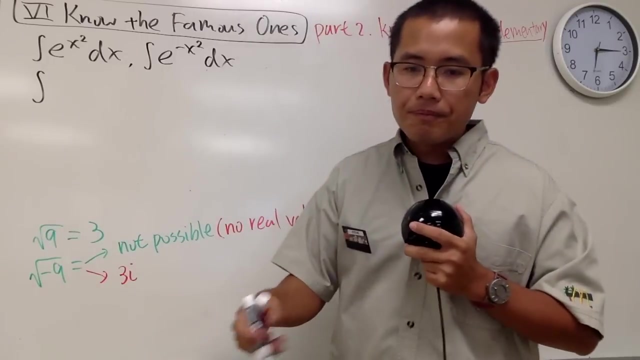 a couple more so that we can see the famous ones. Okay, So we can also look at the integral of e to the negative x squared dx. This one doesn't have an answer either, And let me just give you guys a couple more. 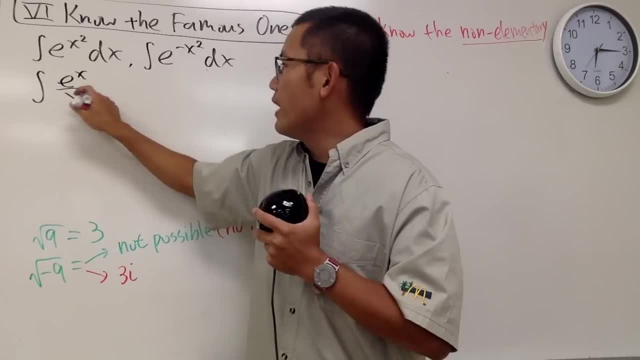 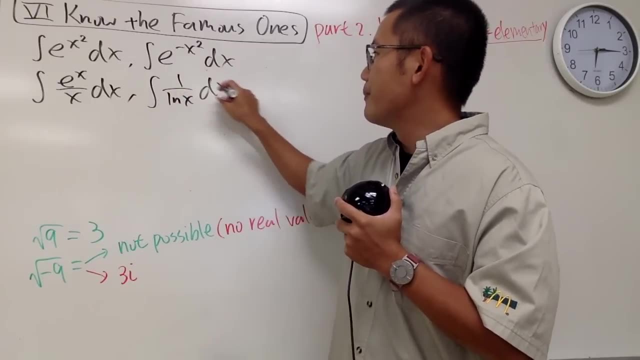 So we will also have the following: Let's say we have e to the x over x, dx. No matter what you do, we cannot get the answer Integral of 1 over natural log of x. No matter what you do, we cannot. 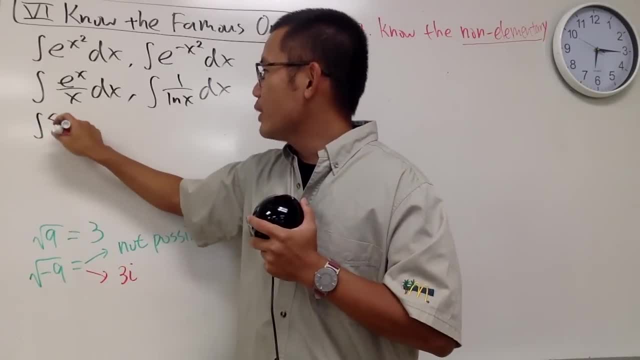 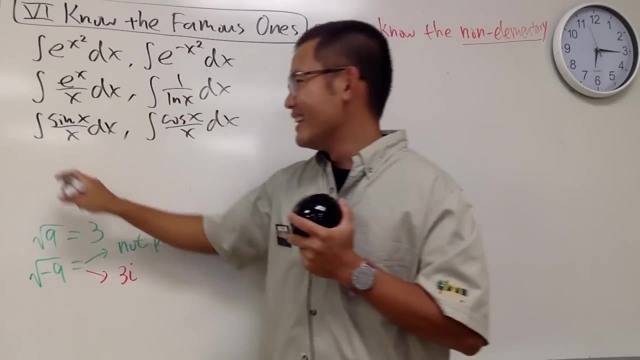 get the answer with regular functions and all that. Okay, Integral of sine x over x dx. Integral of cosine x over x dx. And then I'll just put down a couple more for you guys. okay, Integral of sine of x squared. 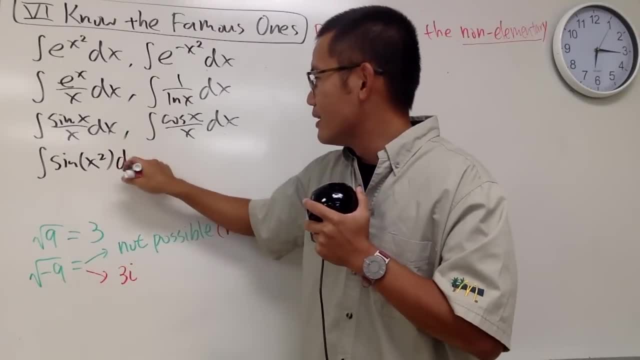 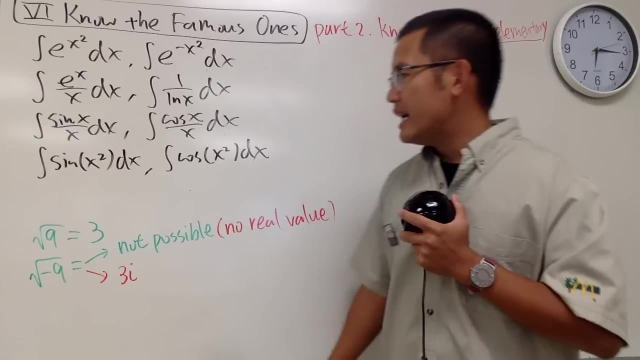 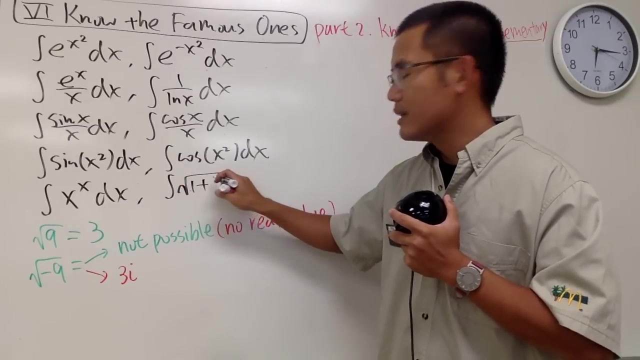 I know this looks pretty innocent, but it doesn't have an answer. dx Likewise. the cosine version also has no answer either. And integral of x to the x power. Integral of square root of 1 plus. Now, let's do this for fun. 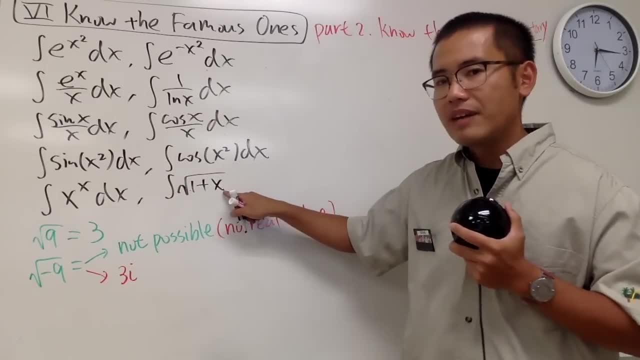 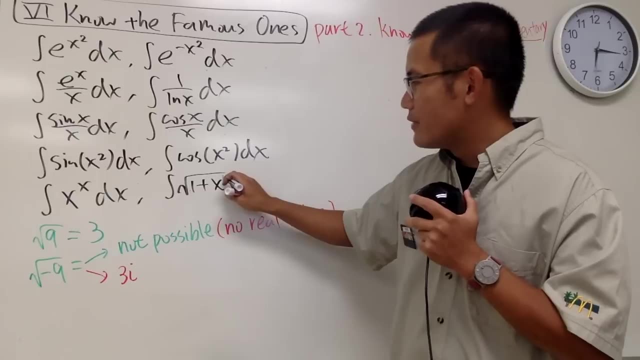 If you have the integral of square root of 1 plus x. does this have an answer? Yes, it does. You can do a u sub and then do reverse power rule. Good, How about if I have x squared right? here We still. 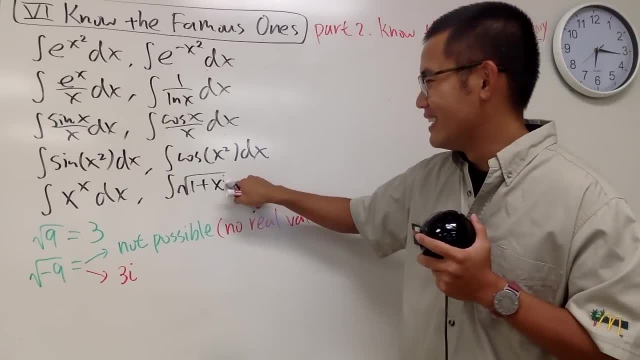 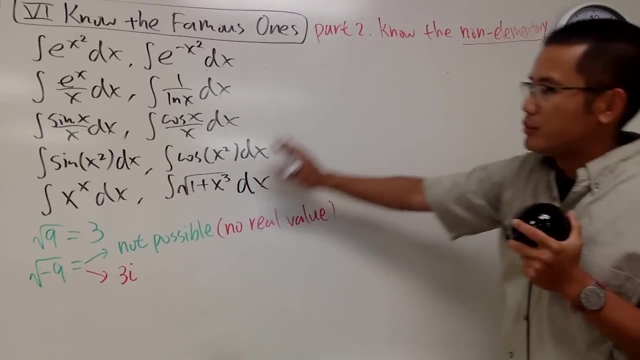 have an answer for this. We still have an answer for this, But the moment that we change this to a 3, this, right here, Non-elementary, neither Non-elementary, neither Non-elementary neither. So here are just some. 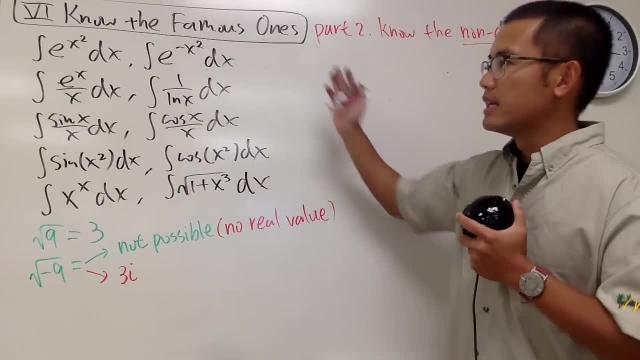 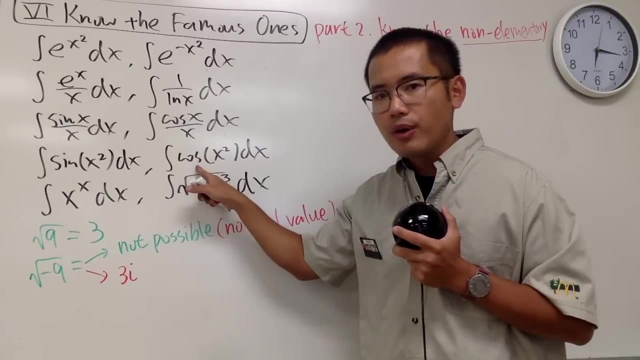 of the famous ones. and here's the idea why I want to tell you guys this right here. The idea is: okay, if you're encountering this integral, you try so hard with all the techniques that you have learned from this video or from your teacher and all that. but 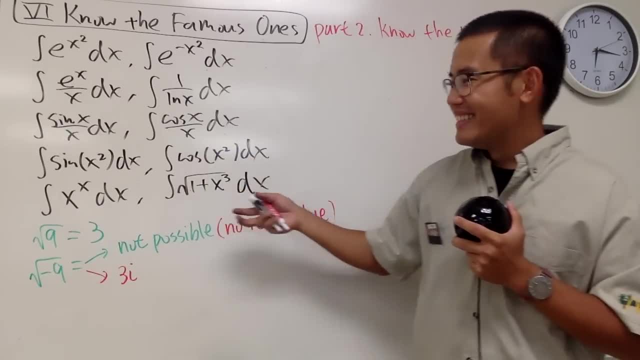 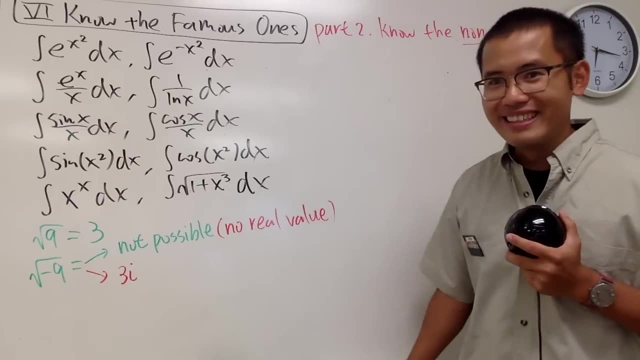 you spend like two, three days and in the end you find out: hey, we don't have an answer for this with the elementary functions. How would you feel Not good, isn't it? So here's the idea. You should definitely know some. 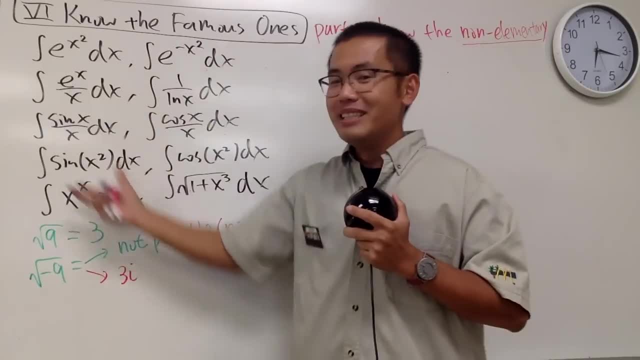 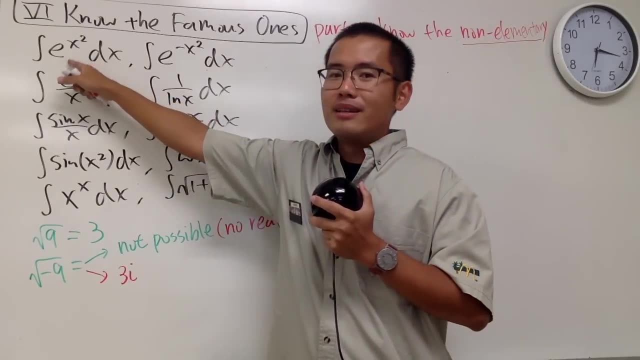 of this right here, so that if you happen to encounter this kind of functions, don't try to integrate it. So let's say a few times: right, I wouldn't integrate this by hand. The integral of e to the x squared: I wouldn't integrate this by hand. 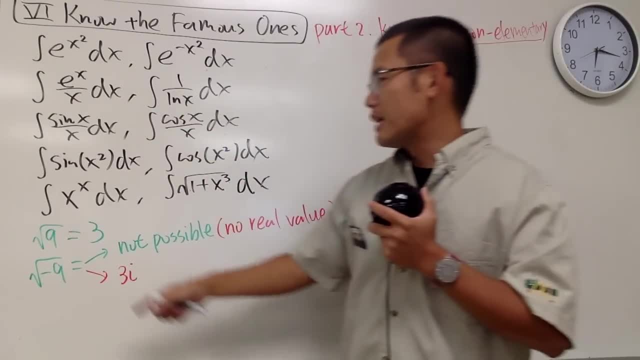 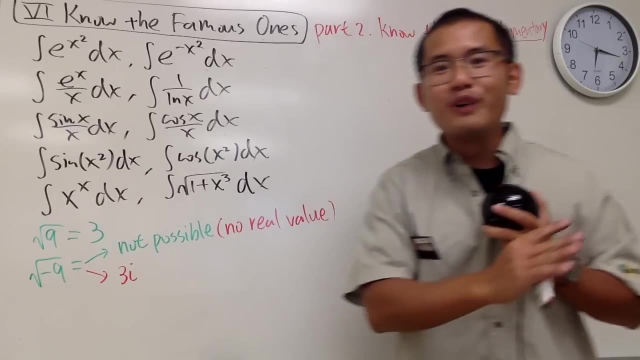 with regular functions that I have. If my students come ask me to integrate x to the x power, I would just tell them: hey, you know what? We don't have an answer for this. We'll just move on. That's all right. 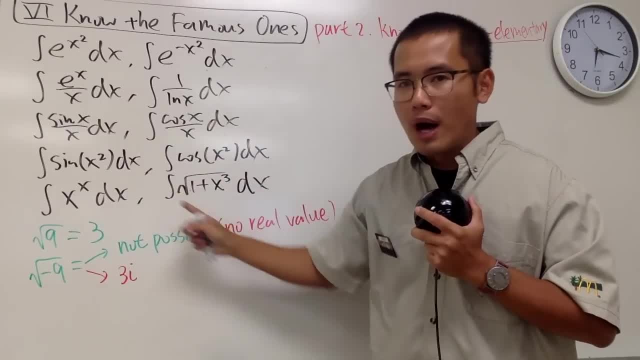 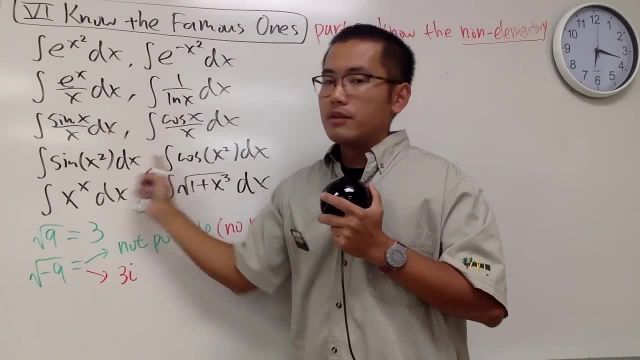 So know the famous non-elementary ones, so that we don't waste our time to actually integrate them Again for this right here. for this right here. they do have special functions for the answers, but that will be for later on, especially. 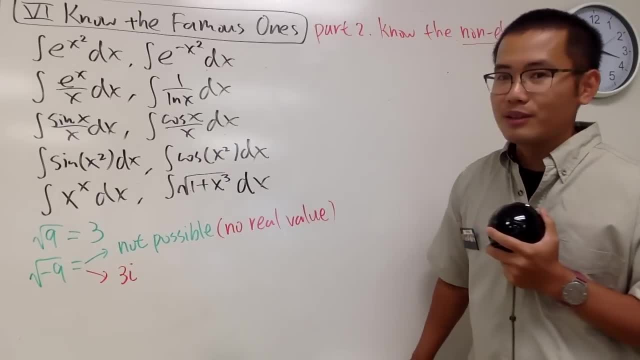 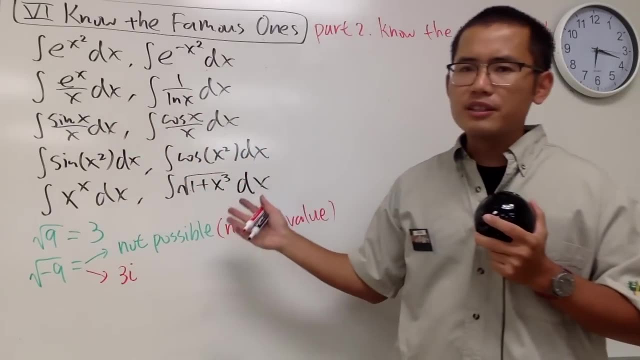 if you study some physics and you may encounter some of them, And I know some of you guys might be wondering if this integrals. if they don't have answers, why bother with them? Well, the truth is, although some of this they 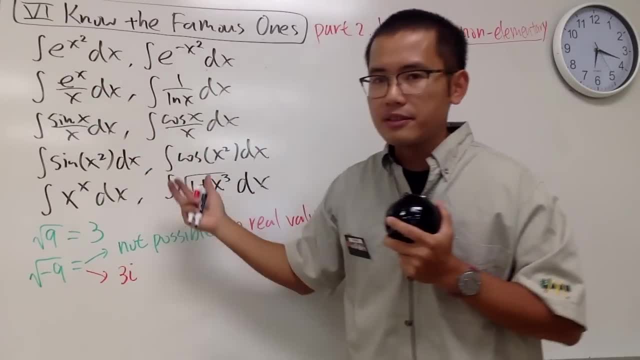 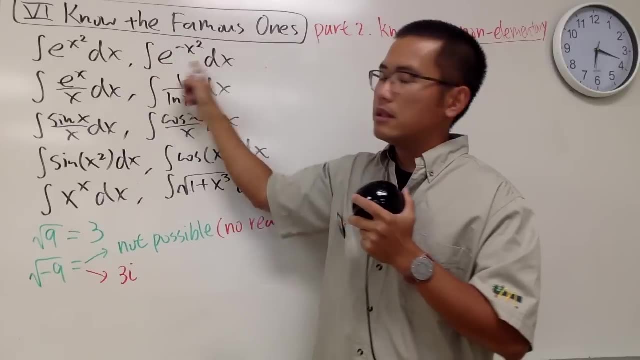 don't have answers, although this right here don't have answers, but some of them, they do have good applications. So, for example, this is my favorite one: The integral of e to the negative x squared, Because you'll be using 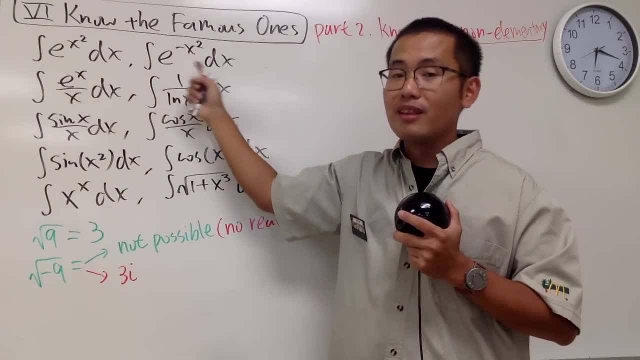 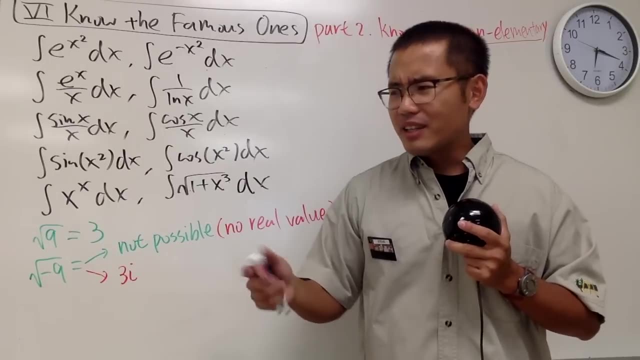 this in stats and probability a lot. if you guys ever wonder when you go out when a professor curves the class, like, if you wonder, like, what does it mean by curve the class? Well, we're talking about this kind of curve. 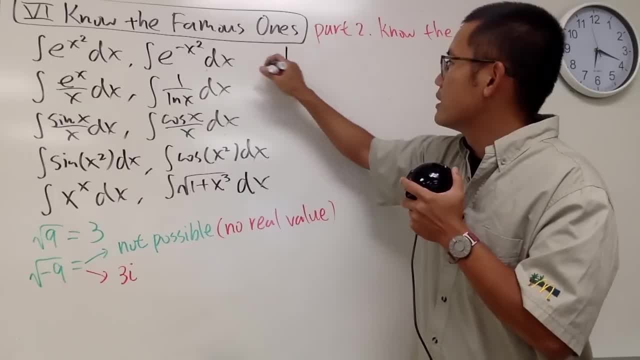 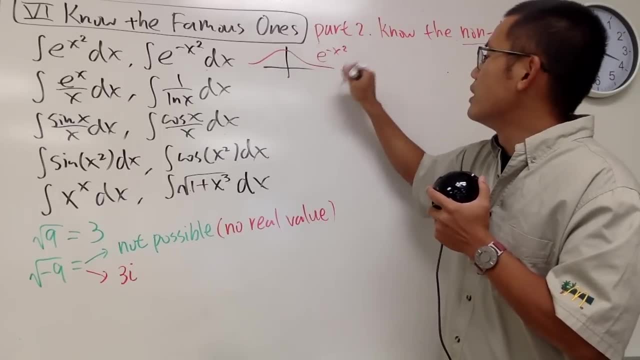 If you grab e to the negative x squared- let me just put that down for you guys- you will get the so-called the bell-shaped curve. This is e to the negative x squared And of course you have some constants. but this is the function part. 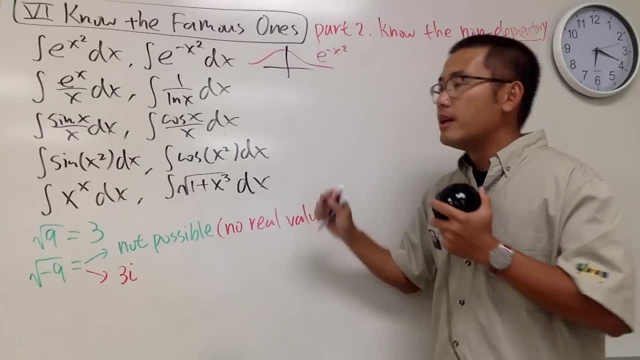 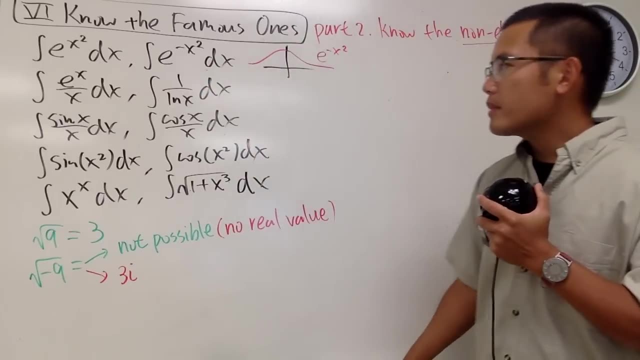 You have some constant multiple, but I'll leave that to you guys. But this is the kind of curve that we'll be studying in probability and also statistics, so it's very important, And I'm actually not sure about this, but in fact, 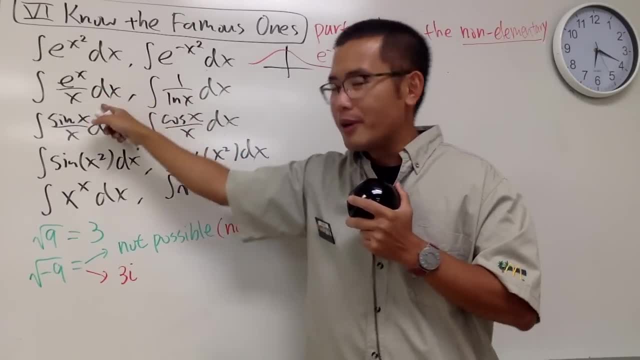 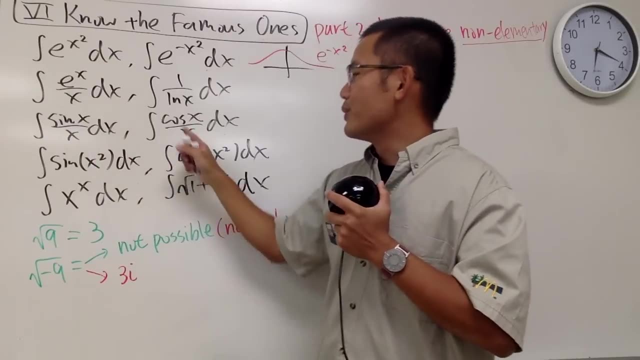 this and that are related. You can just do a substitution, You can go from here to here. You can do this in number theory and prime numbers. And these two signals, they are in signal studies, sine x over x, and this is just its cousin. 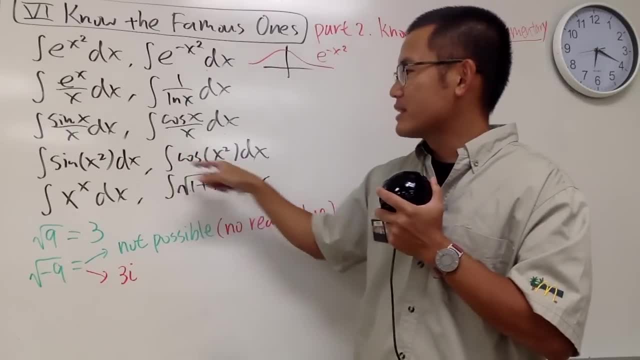 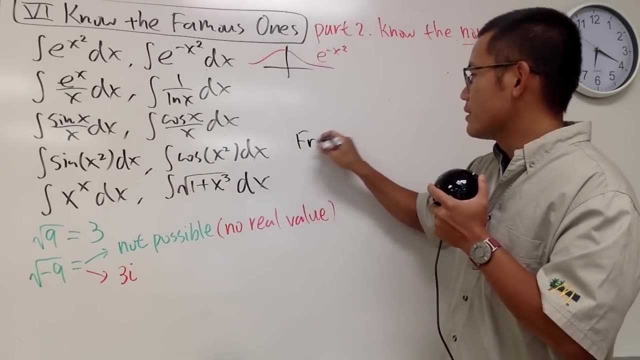 And then sine of x squared and the integral of cosine of x squared. these two are the Fresnel's integrals. So you guys will see this and I'll just write this down, just to be respectful. These are called the Fresnel's integrals. 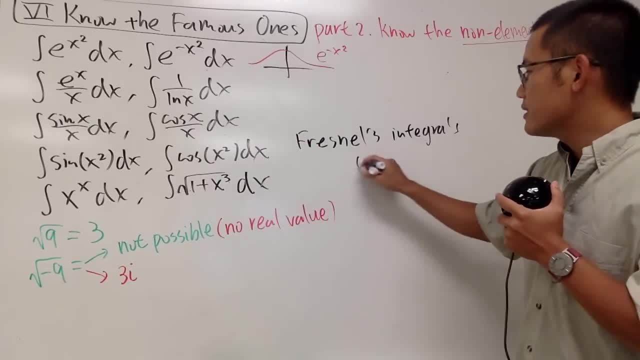 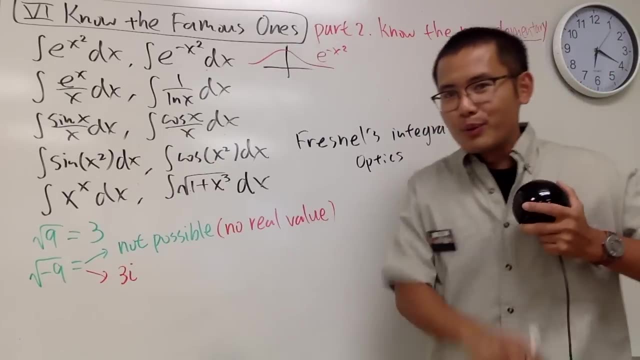 And you will study this in physics, especially in optics. Optics- Yeah, I think I spelled this right. I kind of feel tired already, but don't worry, I can continue with others. I didn't number any of this as integral. 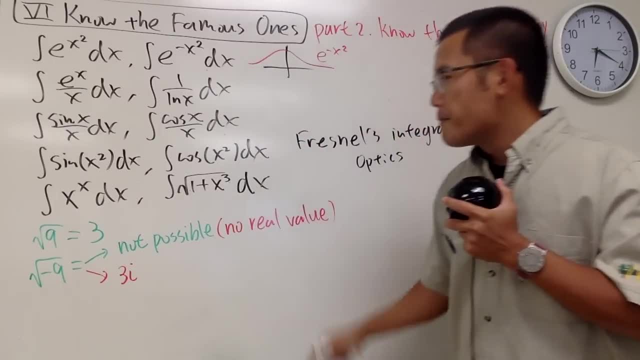 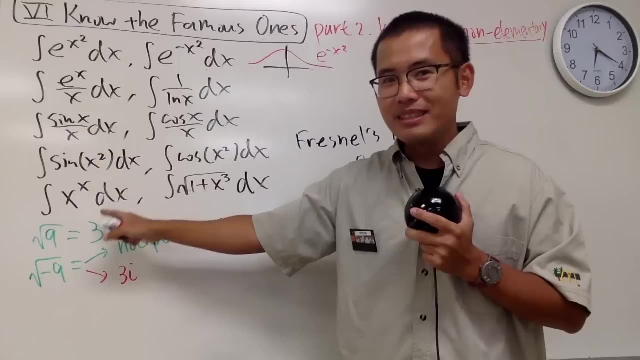 This is just a category. I'm not working on anything right here. okay, This one. I actually don't know any application for this, but a lot of my viewers, they have been asking me this, so I'll just put it down. 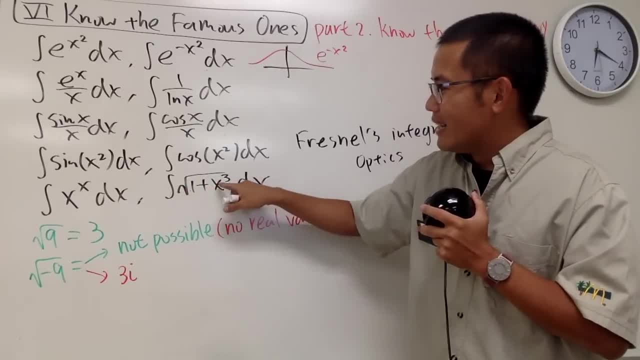 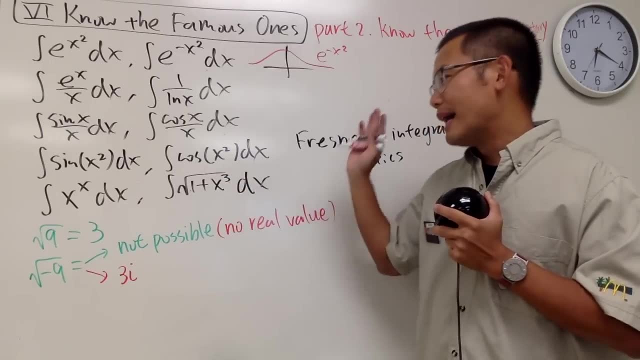 Again, when you have- if this was x over first power, you have the answer. x over second power, you have the answer. but when you have x over third power here you don't have the answer. I don't know the actual. 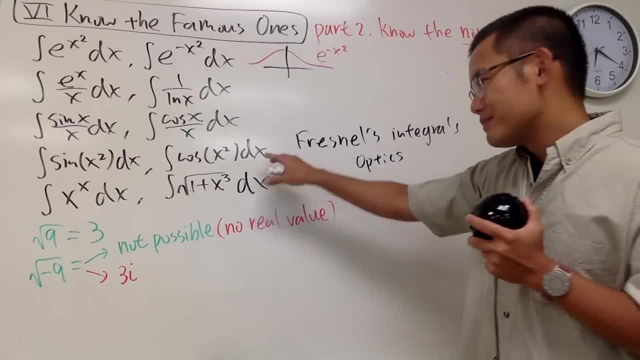 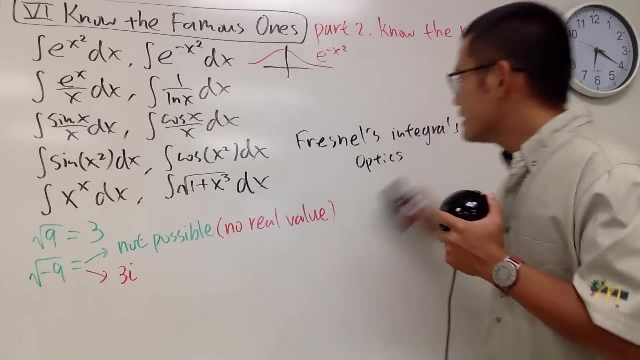 I think it's elliptic integrals. but again, if you see this, no answers for now, Just move on. That's all All right. So that's the idea. This is category number six. Know the famous ones? 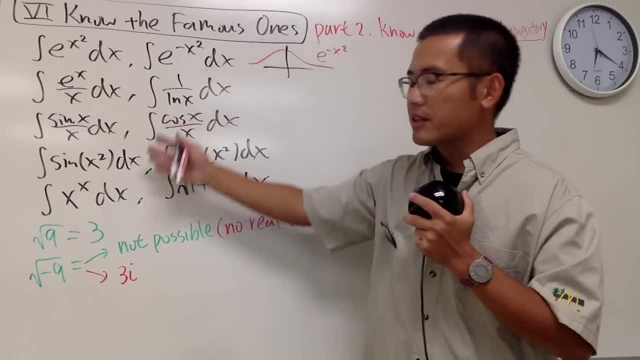 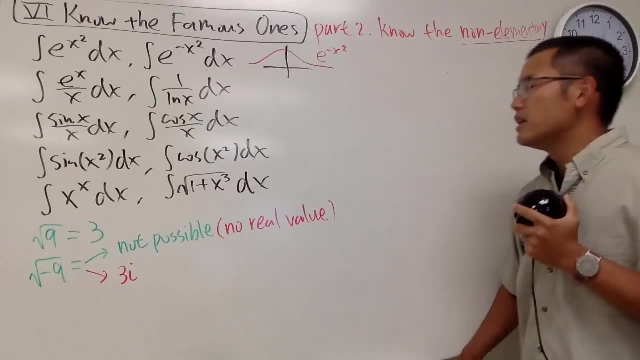 Know the famous non-elementary ones, So that if you ever encounter this, don't spend the time to integrate it by hand. You can use special functions, but that will be for later on, right, And before we continue, you might be wondering. 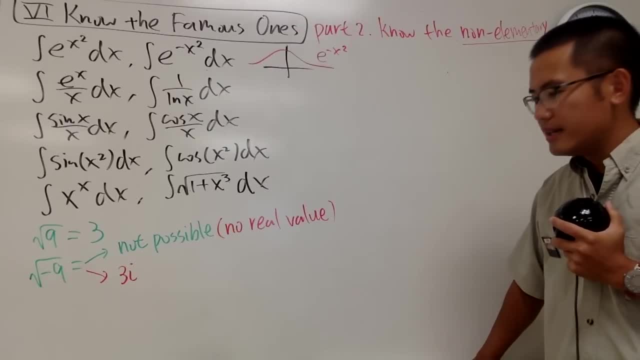 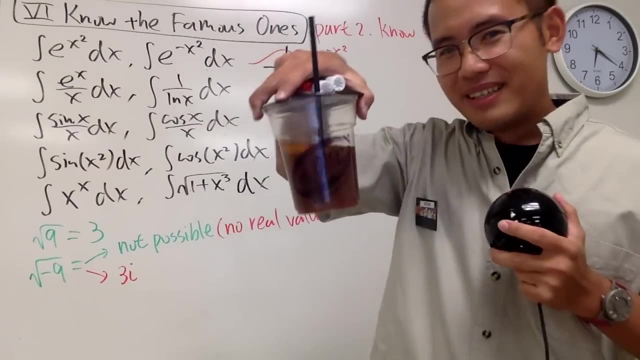 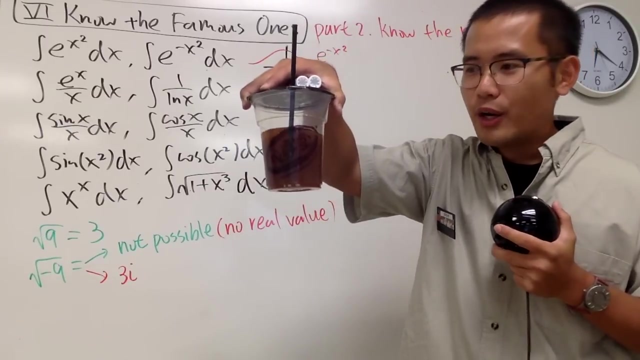 okay, we do have applications for this, and I should have said this. Actually, let me just drink something first. This is again, this is from half and half. It's a store, right, It's a tea house, And this is the Kuhn Quark black tea. 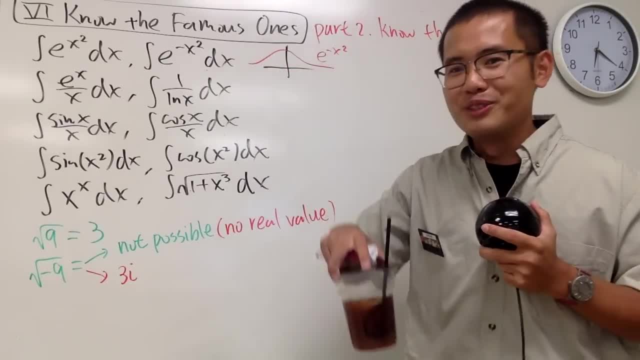 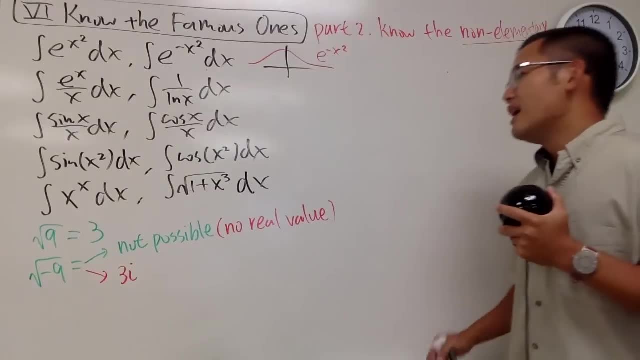 This is the same exact one that I got when I was doing the 100 integral video about half a year ago. right, All right. So we did talk about some of this. They do have nice applications, so that's why we care about them. 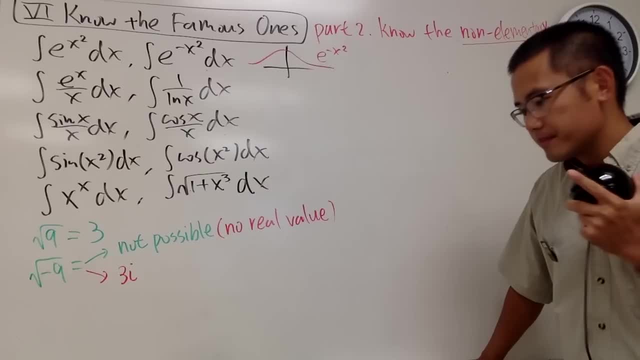 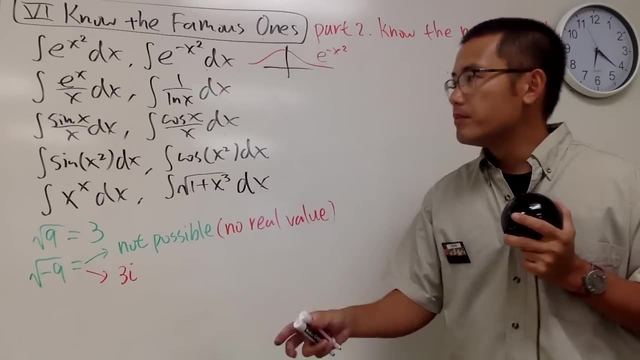 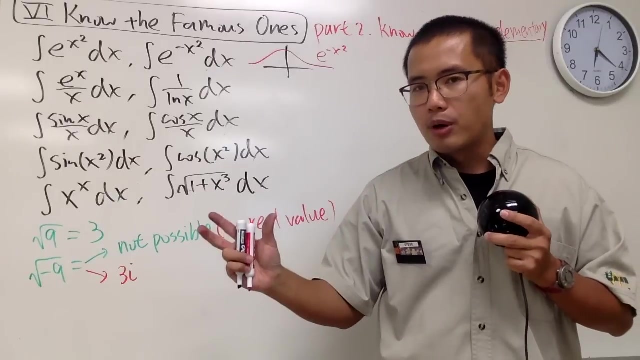 And let's talk about this right here. You have to really kind of pay attention to the difference between impossible, which are like this. right here, These integrals are impossible. right, You have to know the difference between impossible and hard. So let me just write this down right here: 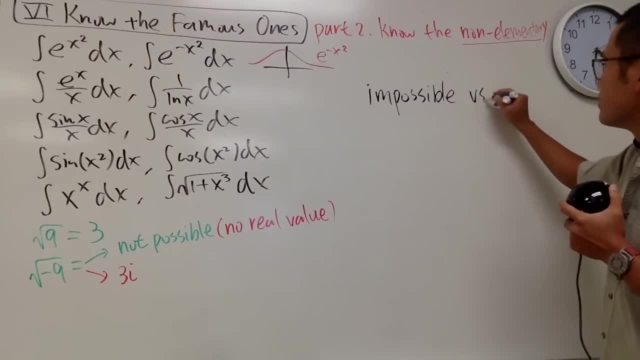 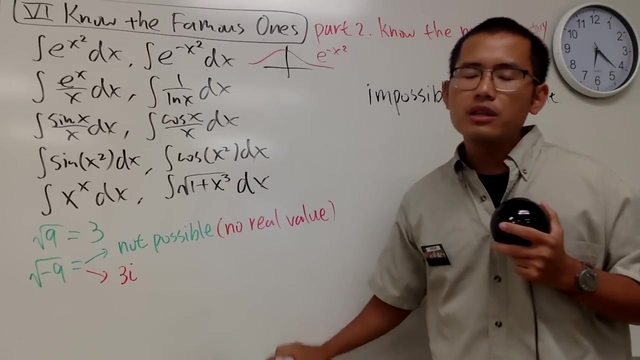 And of course we are talking about, like solving integrals, Impossible versus, perhaps let me just say, difficult. Yeah, All right, So you have to know the difference between impossible versus difficult. And perhaps, if you guys are still watching, 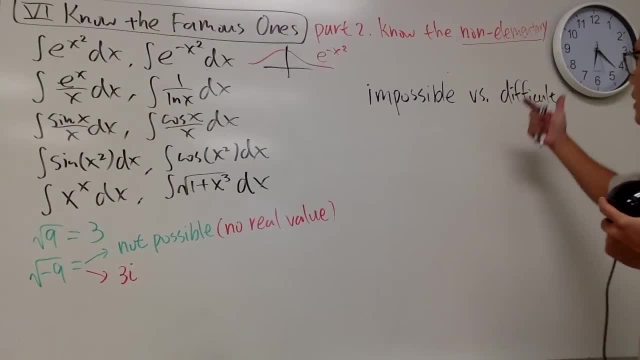 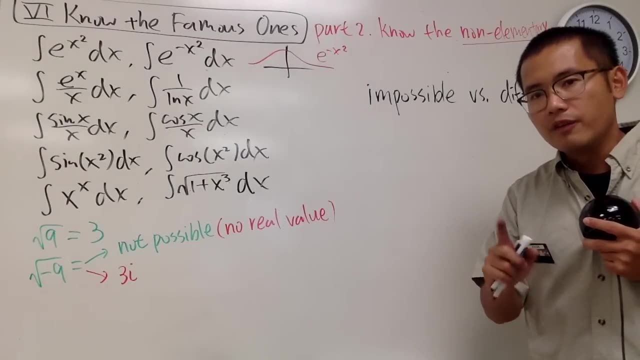 leave a comment down below and let me know what is your definition of the word difficult And in the meantime, you can also leave a comment and let me know your definition of the word Easy. right? I would like to read your comments first. 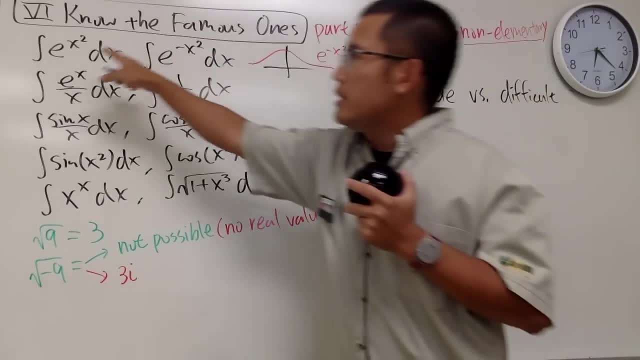 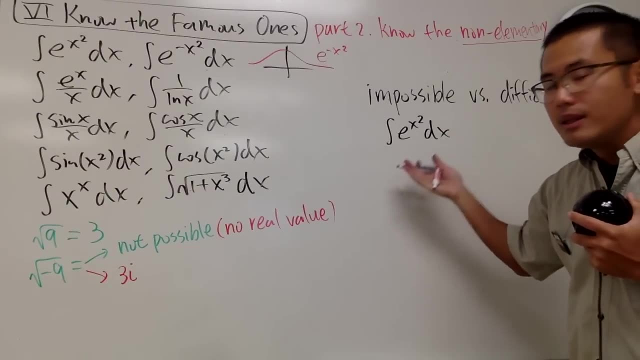 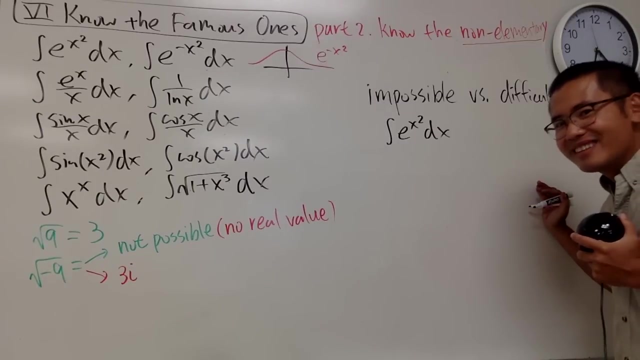 All right, Here's the idea. This integral is impossible. e to the x squared dx. And if you know this is impossible, just don't do it. Yeah Well, later on we'll be encountering some other integrals, such as the integral if we have x squared e to the x dx. 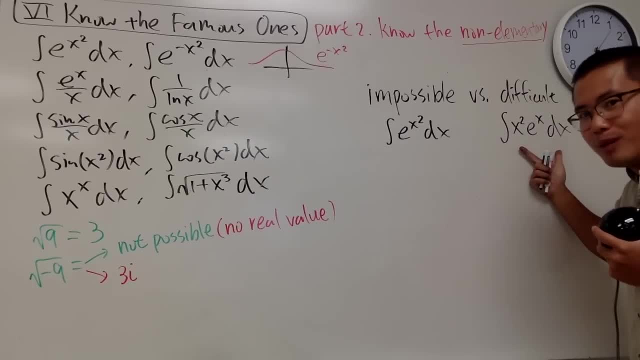 This integral might be difficult at the moment because we don't know how to do it yet. Unfortunately, we cannot do USAP to take up this integral at the moment. We just cannot do USAP for this one actually. Yeah, So here is my definition of the word difficult. 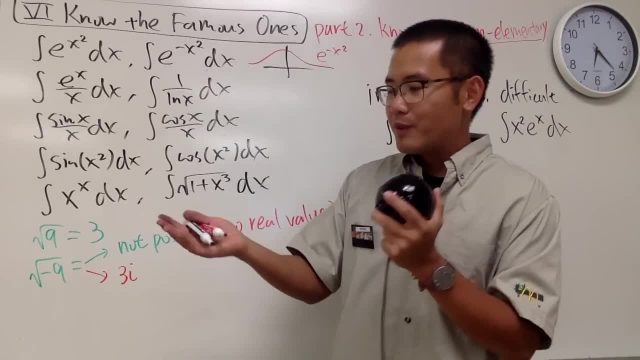 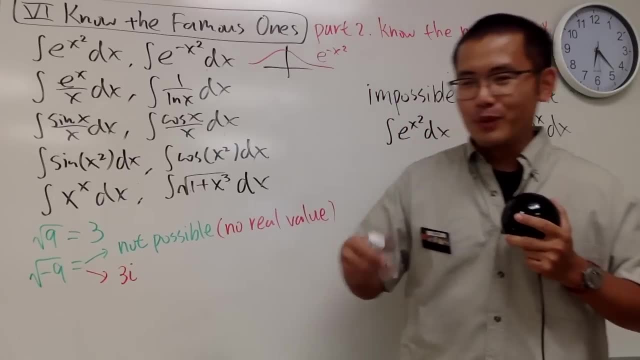 It seems that people will just tell you that whatever we cannot do is difficult. If we cannot do this, it's difficult. Similarly well, I should say. on the contrary, the definition of easy, in my opinion, is just anything that I can do. it's easy. 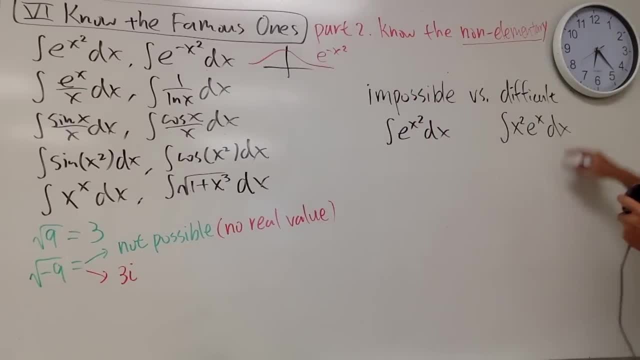 Anything we can do is just easy. Yeah, But anyway, here is the point I want to make. Don't look at this as difficult in the sense that it might be difficult at the moment, but once you learn the method, when you see how to do it. 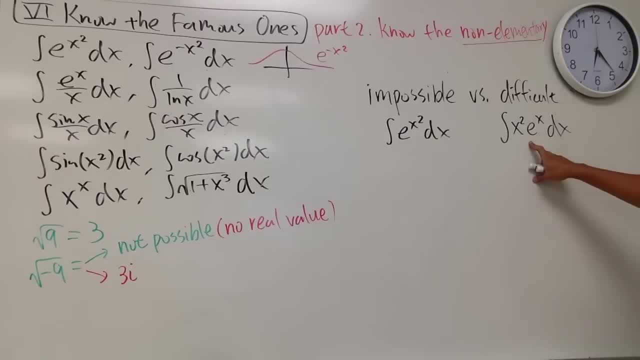 you should look at this as easy, right. This requires another technique, but you have to know that it's doable. It might be difficult at the moment, but it's doable, right? So later on, once you see this, 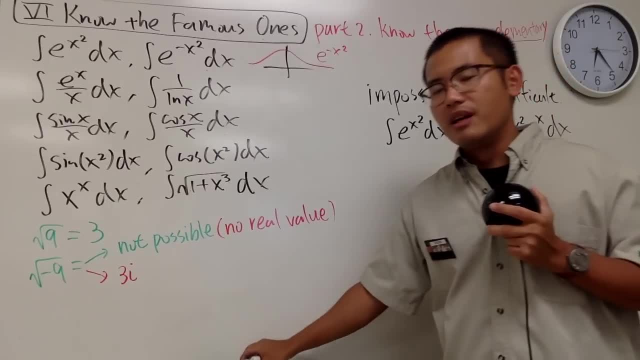 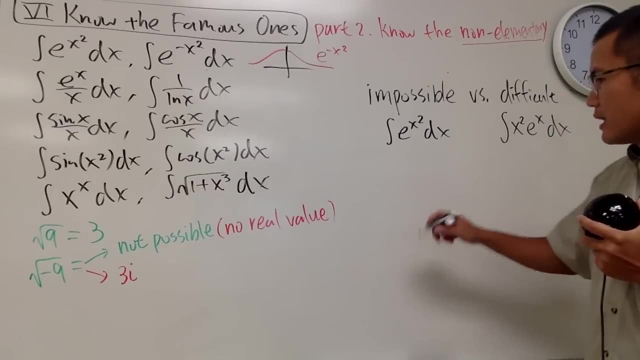 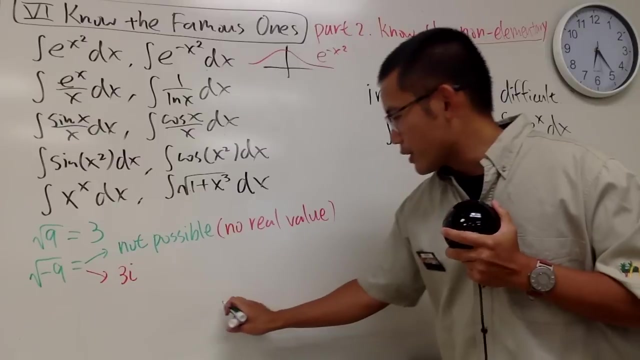 you just have to really practice the technique so that it will actually be easy. That's what I wanted to say. Let me give you guys another question from the Algebra class, so that you can see the difference between impossible versus difficult, right? So I'll just put this down right here. 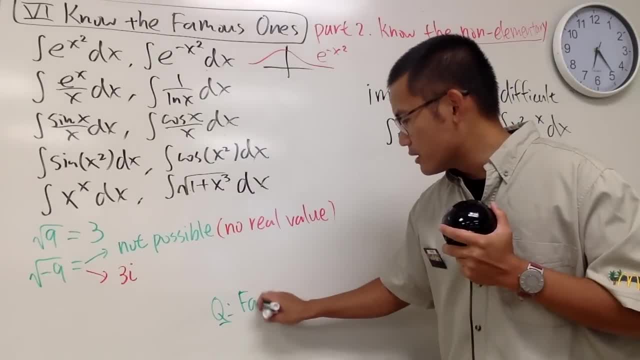 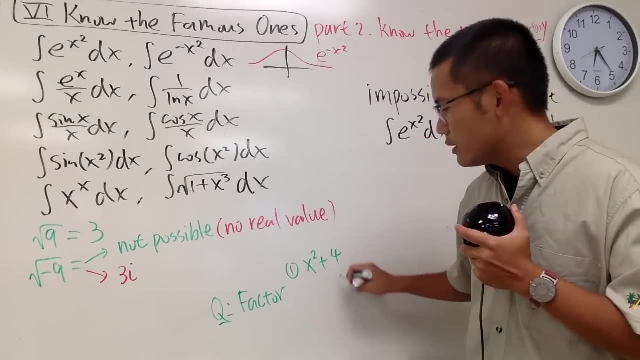 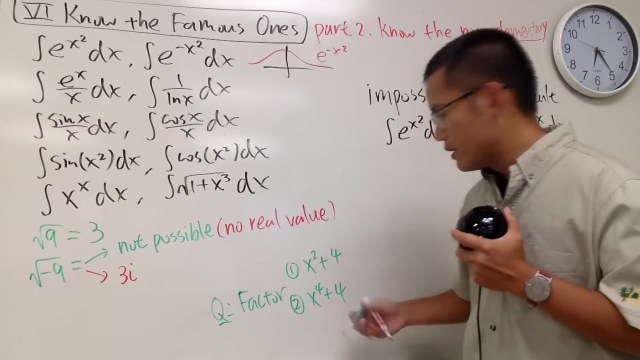 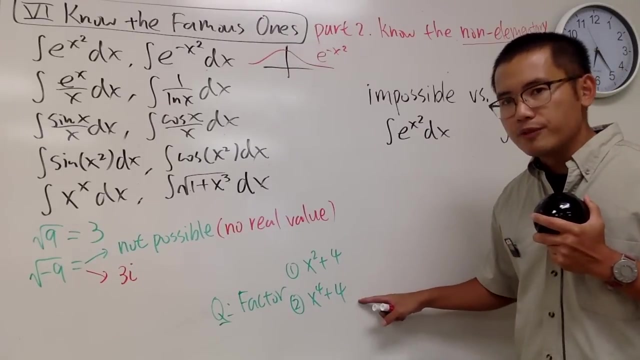 Alright, two questions. Let's talk about how to factor. Alright, I would like to ask you guys how to factor x squared plus 4, right here, versus x to the fourth power plus 4, like this: Okay, Which one is impossible to factor? 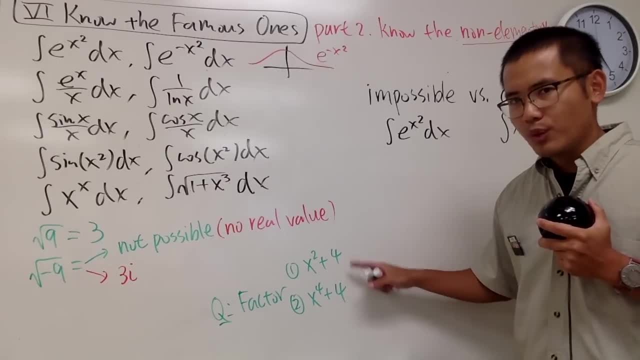 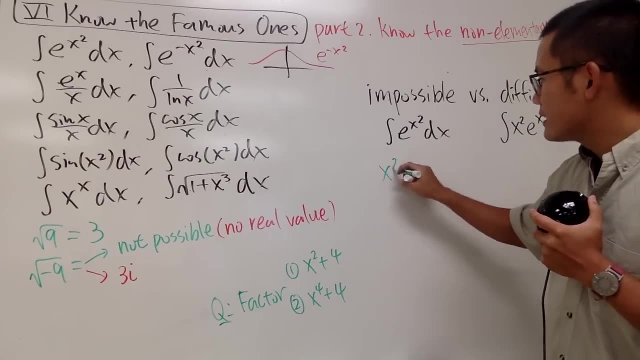 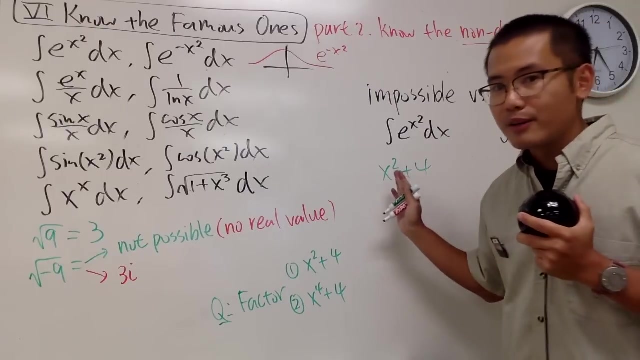 with real numbers, And which one is just difficult. Well, the answer is that this right here is impossible to factor x squared plus 4.. It's impossible to factor with real numbers because we know the sum of two squares. we cannot factor it x to the second power. 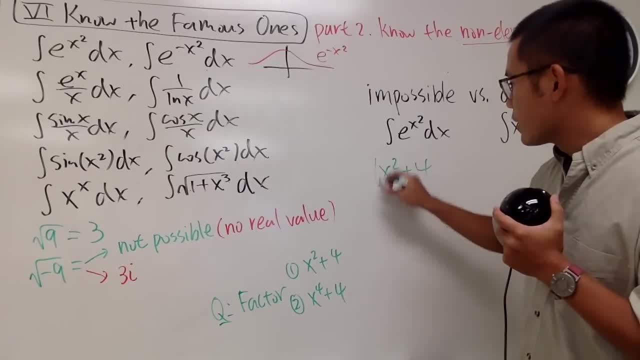 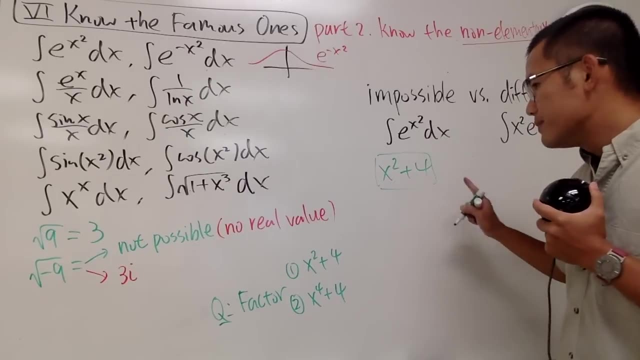 This is an irreducible quadratic. So this right here is impossible, And of course, I wouldn't bother to factor, because I know it's impossible already And again. we will be talking about this expression later on. That's why I want to bring this up, okay. 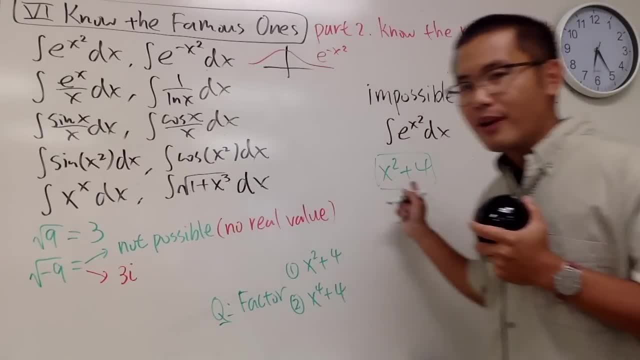 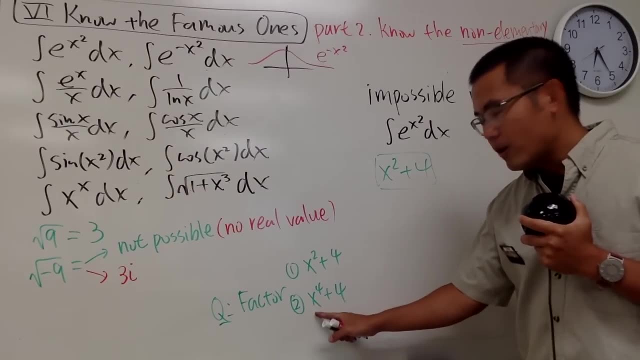 Again, we can use complex number for this right here. but that's not the deal, That's not the rule of the game. No complex number is allowed to factor this Well. with that being said, x to the fourth power is possible. 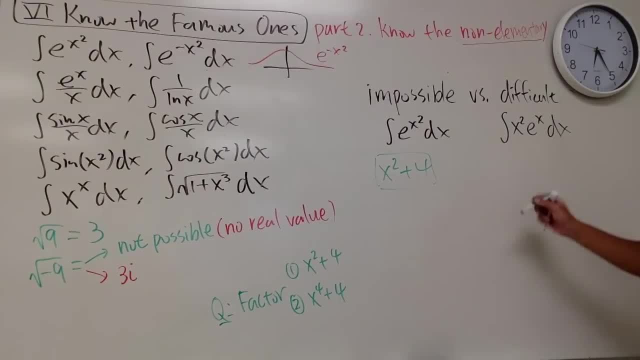 but it's just difficult at the moment. I will show you guys how to factor that. Have a look here. Suppose we want to factor x to the fourth power plus 4.. This right here is actually possible, although it's also the sum of two squares. 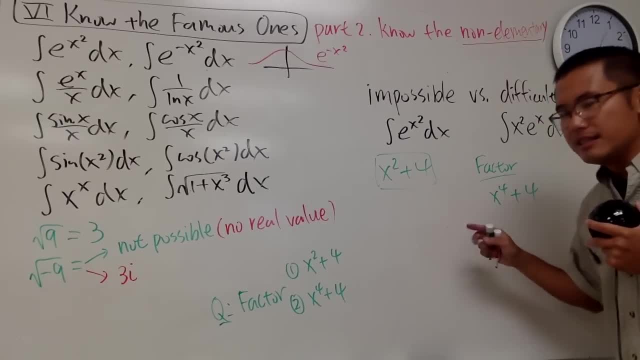 but this is x to the fourth power, So it's not like the quadratic. Here is the idea, Well. well, let's see, I have x to the fourth power plus 4.. It's really difficult for me, but I know this is doable. 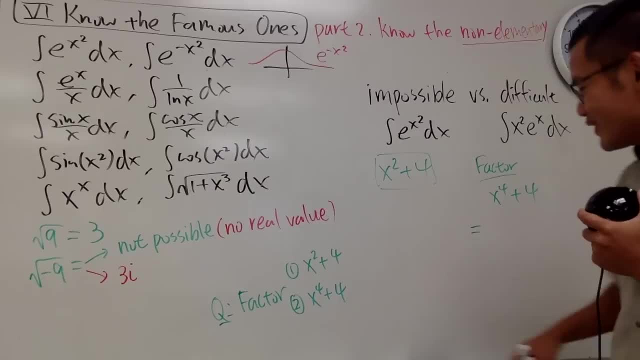 because, as I said, one of them is just difficult for the moment. Okay, so this is how we are going to do it. Think about the situation. How we would like to factor is that we will have a trinomial that we would like to factor, that. 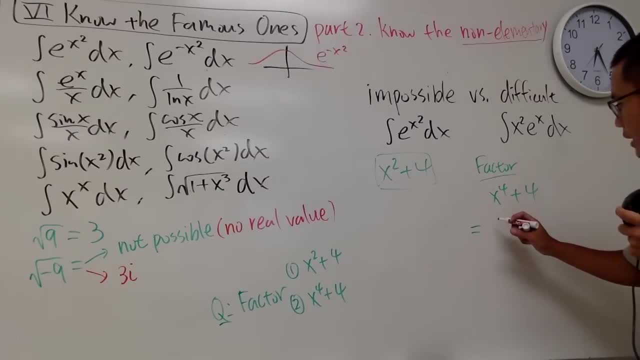 so we have a perfect square. Well, the form that we like is a parenthesis square and plus 2 times parenthesis, parenthesis, parenthesis, plus parenthesis square. This is the form that we like to factor, isn't it? Now can we just fill in the blanks. 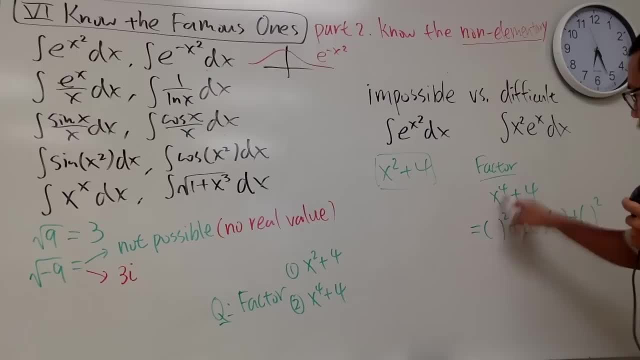 fill in the parenthesis. Originally we had the x to the fourth power. Okay, I can enter that which is x squared. x squared squared is going to be x to the fourth power. That's good. Originally I had a 4.. 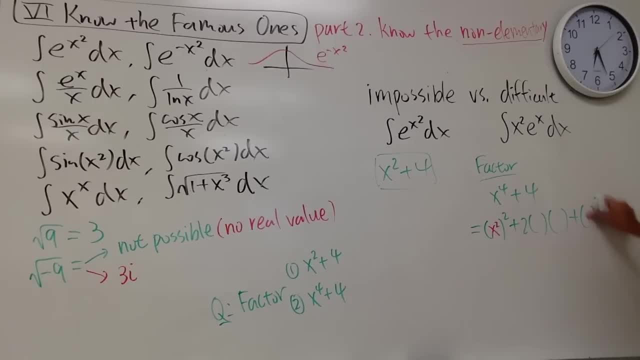 Let's put down 2 right here. 2 squared, of course, is a 4, so that's also good. Now I'm just going to put this parenthesis here. likewise, enter this right here. so that's great. 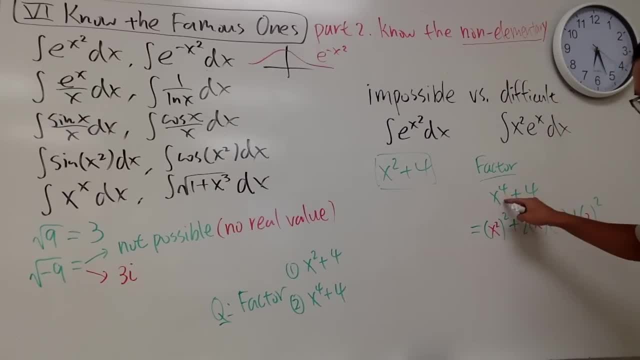 Notice, though, this right here: this is equal to that. this is equal to that, but this is the extra term. Well, I don't like the extra term because I'm changing the whole thing. That's no good. So let me just minus 2 times 2,. 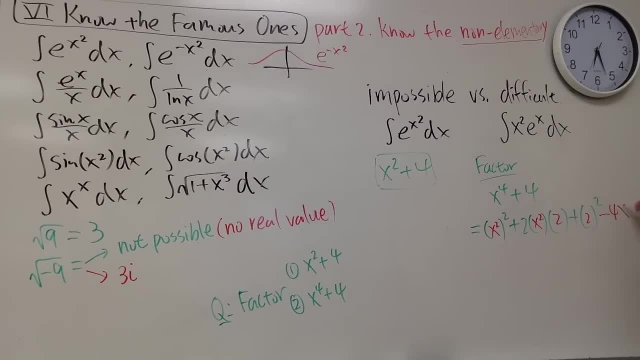 which is 4, and then we have the x squared term right here. Let me just minus the 4x squared after that, so that this and that can cancel out. We're still talking about the original expression. Now have a look. 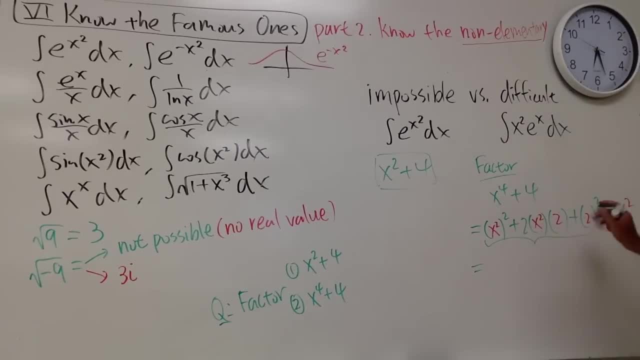 All this right here. this is the perfect square, and we can nicely factor this as a plus b squared and the a is x squared, and then we just need to add it with the b, which is the 2, and then square that. 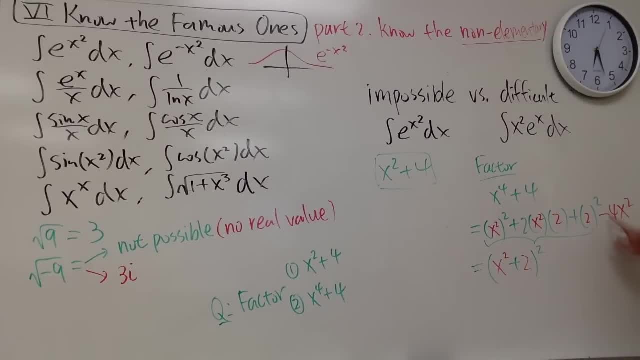 So this is the perfect square and the beauty is that this part is minus 4x squared. We can put this down as a parenthesis something to the second power. I can enter this as 2 inside and x inside, Because 2x squared will also give me 4x squared, like this: 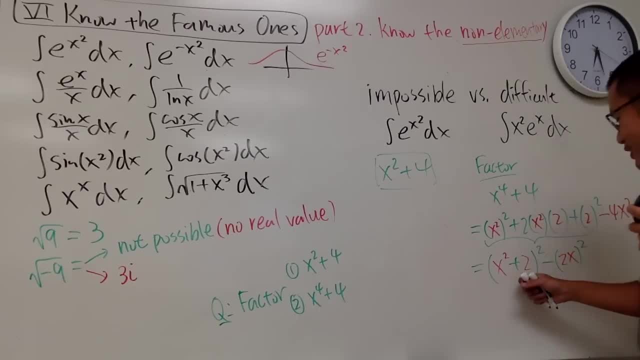 And now what can we do? Yes, this right here is a squared minus b squared, so we can factor this as the difference of two squares. So this right here is going to give us- let me just put this down- as x squared plus 2,. 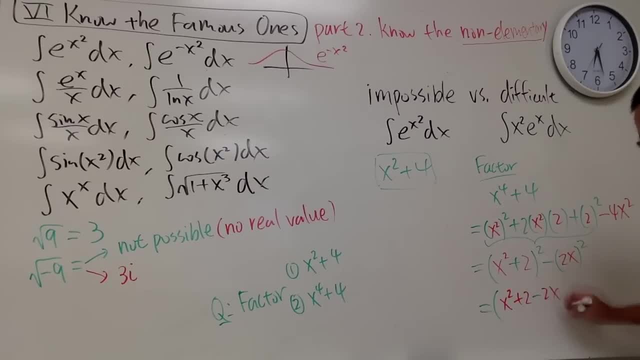 and then I will just say minus 2x, right, a minus b, like this times: a plus b, which is x squared plus 2, and then plus this, right here, 2x. As you can see, we just factored the heck out of this thing. 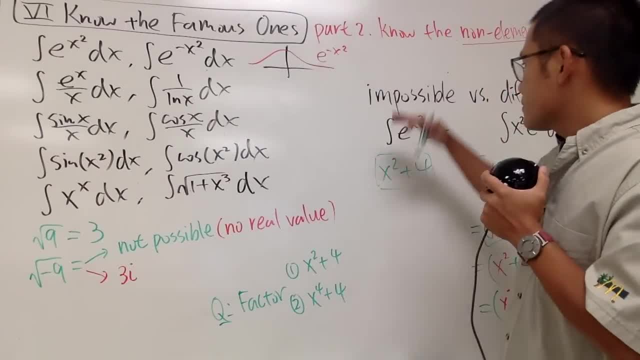 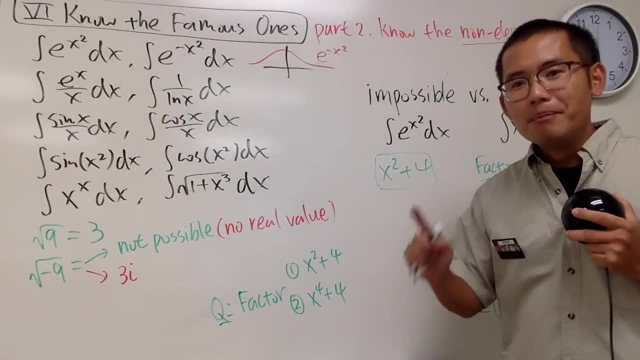 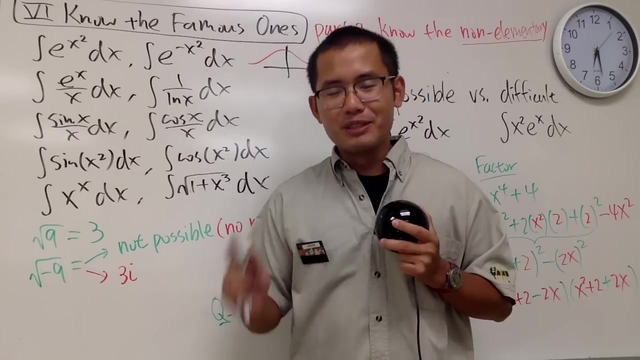 So, as you can see, this is what I mean by impossible versus difficult. Later on a lot of integrals, they will look impossible, but the questions that I'm going to give you, they will always be doable. You just have to learn a technique to do that. 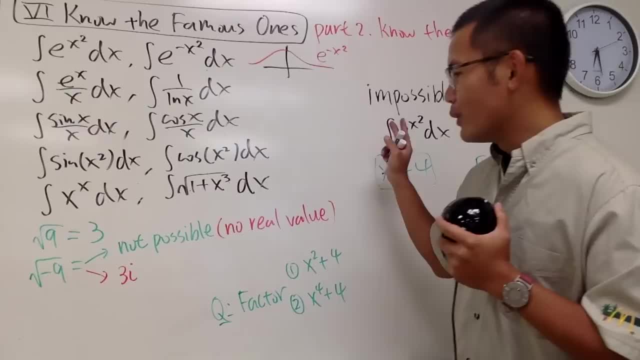 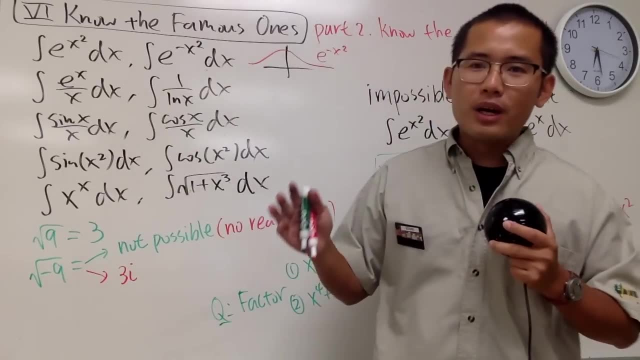 So keep that in mind On my exams, if you put down impossible or non-elementary, it's for sure wrong, because I will not ask you guys any of those questions. This is just like imagine if you're walking back to your car. 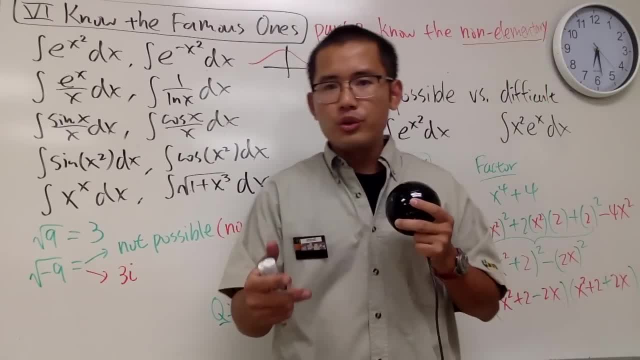 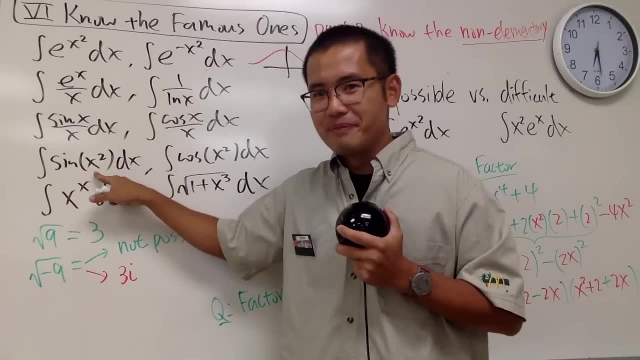 9 pm at night and somebody is approaching you. They want you to integrate sine of x squared in the parking lot, otherwise they are not letting you go home. You can take a look at the question and think about: hey, black pen, red pen told me that. 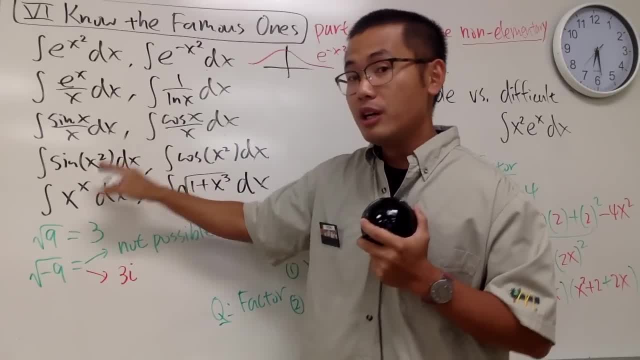 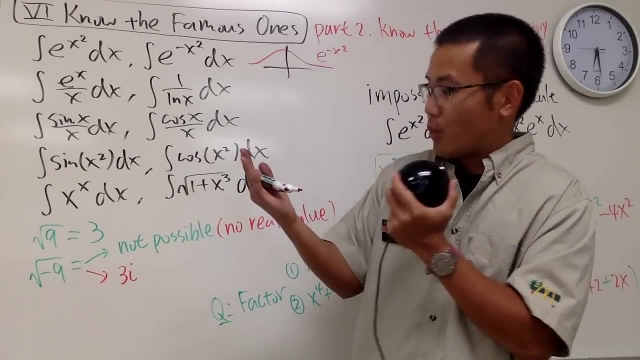 this right here is impossible. it's non-elementary. Just tell the person that this integral is non-elementary, Walk away, And then the person should be like: whoa, how do you know? That's the idea, right. 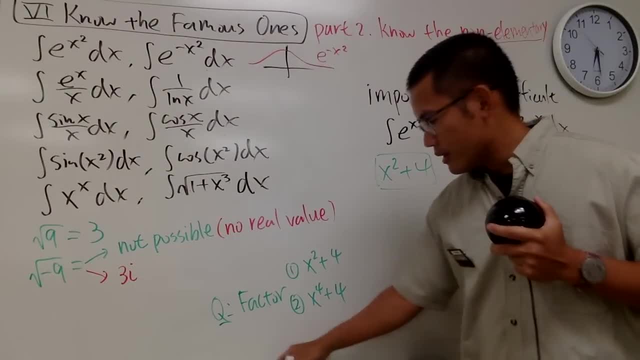 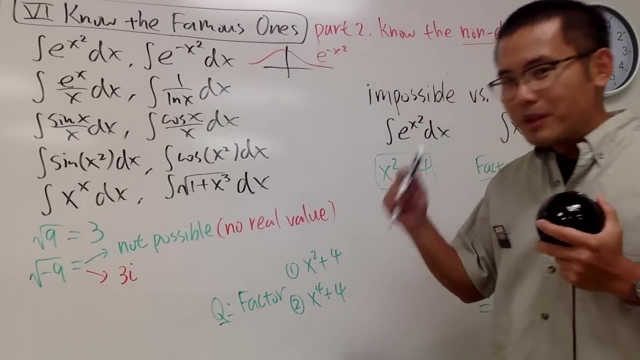 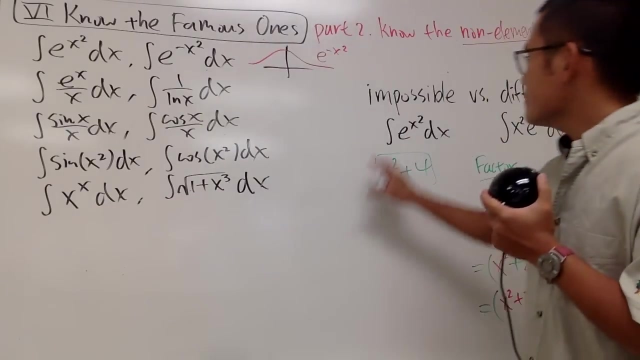 So that's the discussion that I wanted to have right here, And perhaps let me have one more little part with the discussion with you guys, One more discussion before we go right. Earlier that was a discussion between impossible versus difficult. 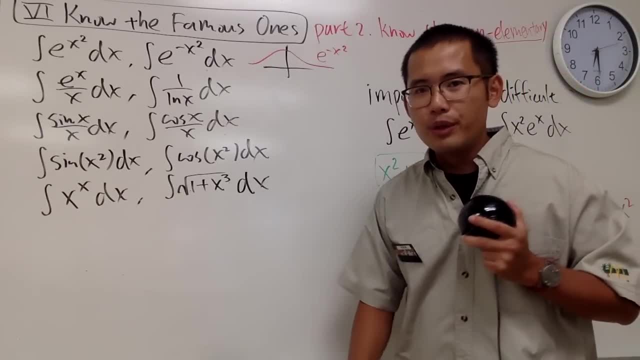 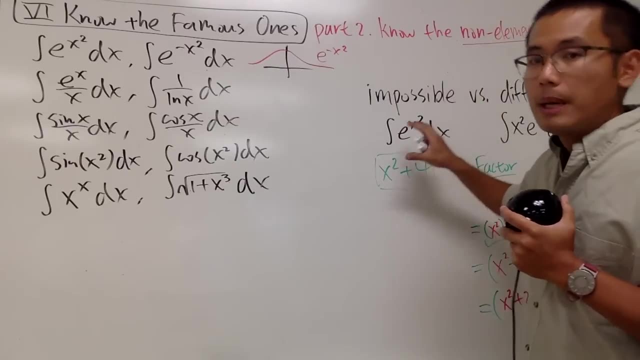 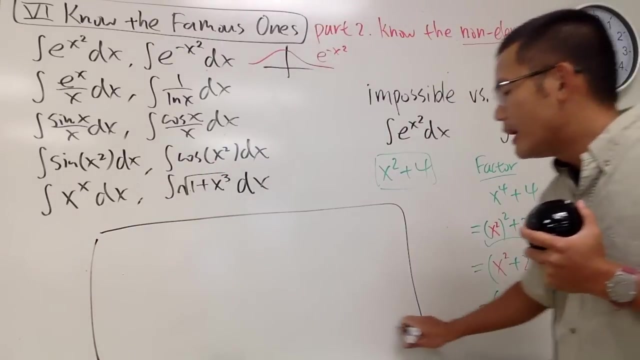 Now you also have to know the difference between impossible integrals, right, Non-elementary integrals. I should say non-elementary integrals, but they have application. However, sometimes you may have a situation that people just walk to you. 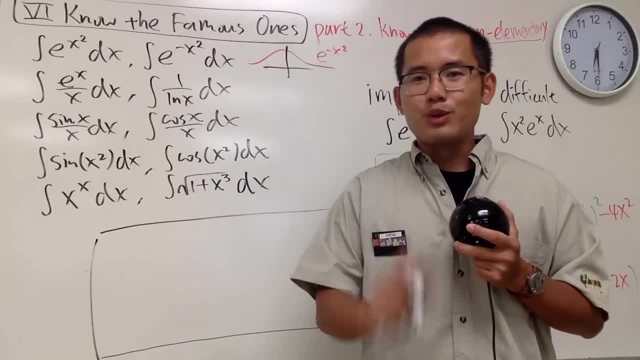 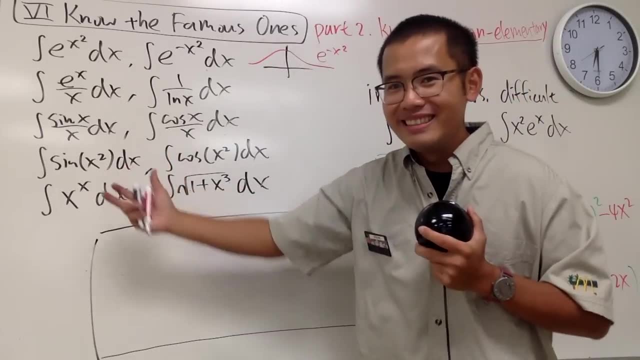 and give you a random thing, random integral- because they just want to mess around with you. That's all You have to know the difference between non-elementary but useful and for the time that someone is just trying to mess around with you. So let me give you an example. 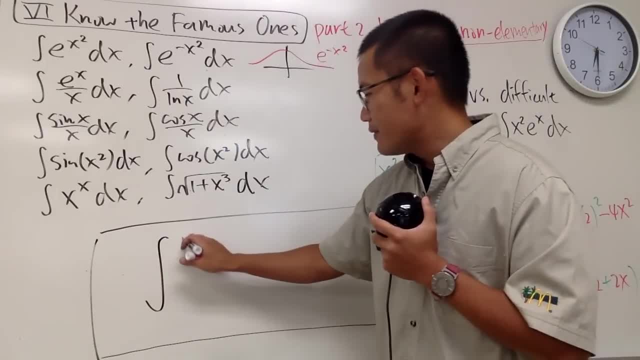 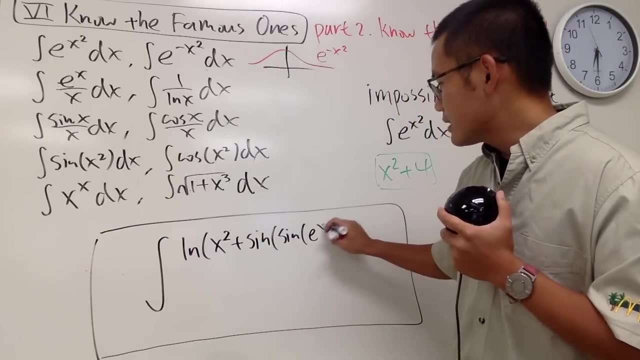 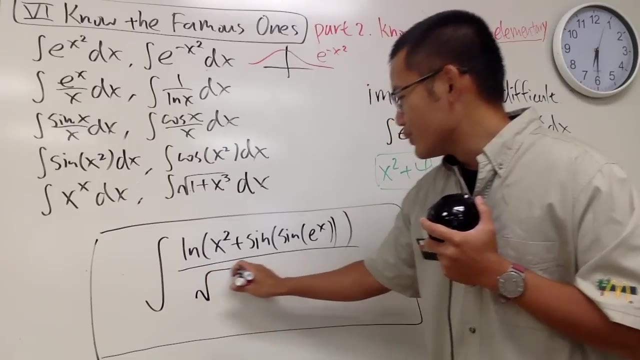 Suppose I give you the integral right. Let's say I have natural log of x to the second power, plus sine of sine of e to the x, like this parenthesis, parenthesis, parenthesis. and then, over square root of x, plus tangent of, 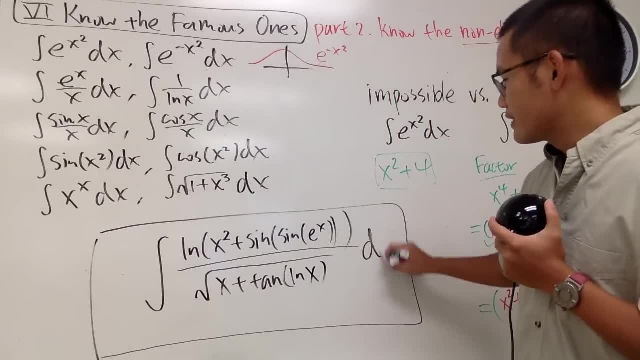 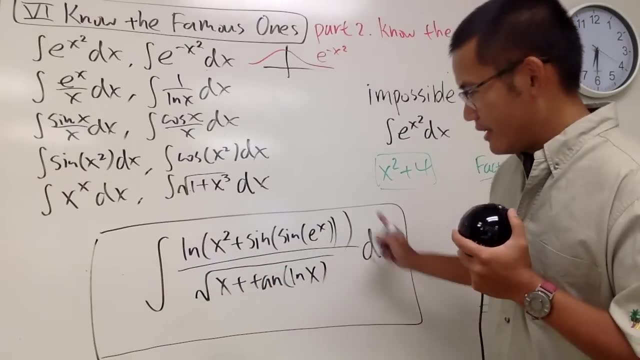 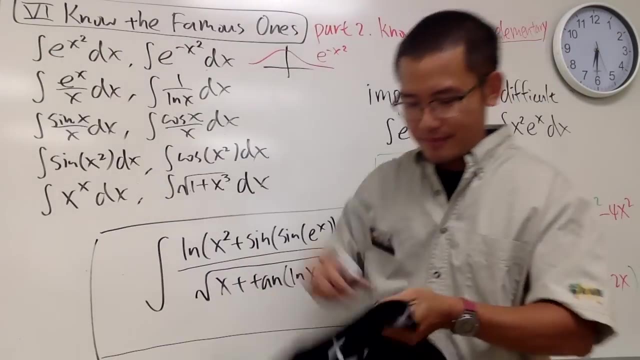 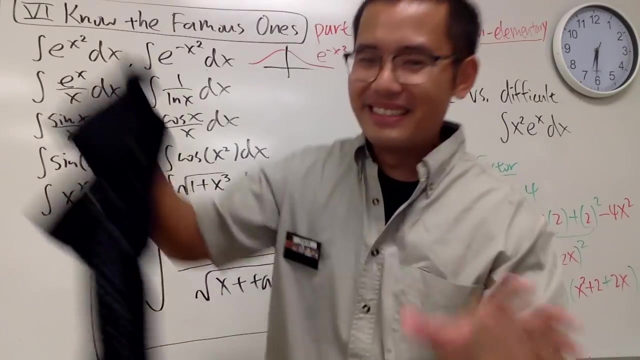 natural log of x like this dx right. So let me just make a proposal. If anyone can integrate this, I'm going to give you a t-shirt. If anyone can integrate this, I will give you guys a t-shirt. 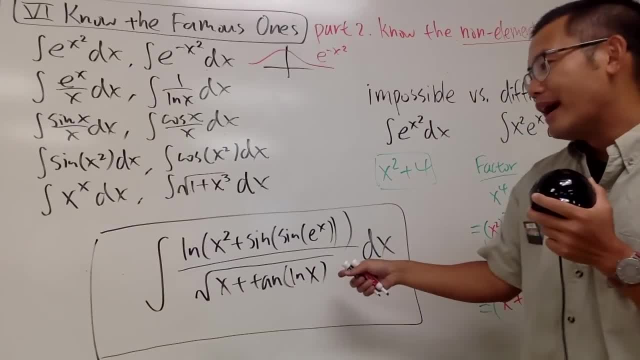 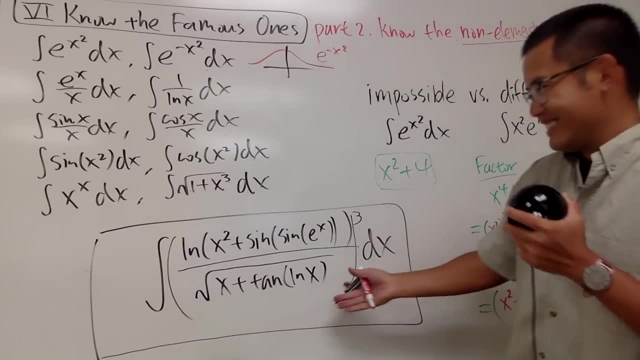 but you know what, Don't even try, because I hope you guys can see that. Actually, no, Let me just put this to the second power. That's the third power. Let me just say that. So, if you can integrate this now, 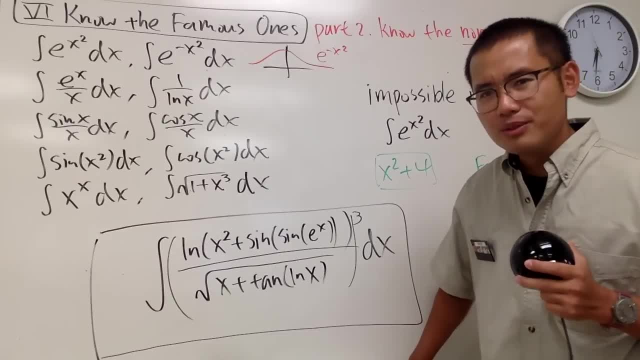 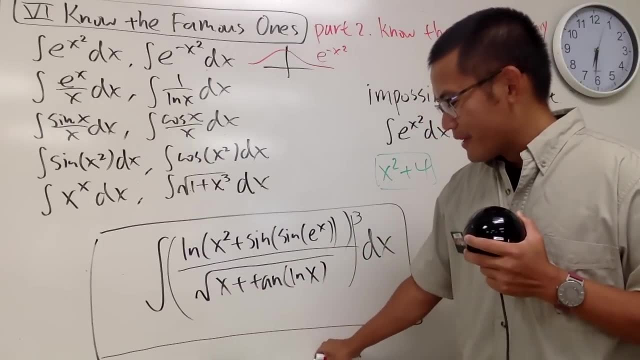 you will get a t-shirt, But don't even try, because you know this is the situation: that someone is just trying to mess around with you, So don't even bother with this, right? So this is actually a really good discussion because 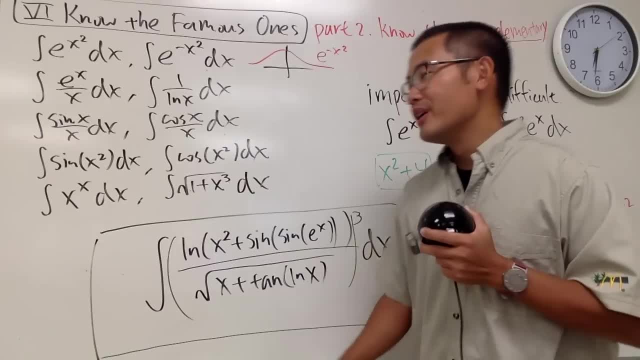 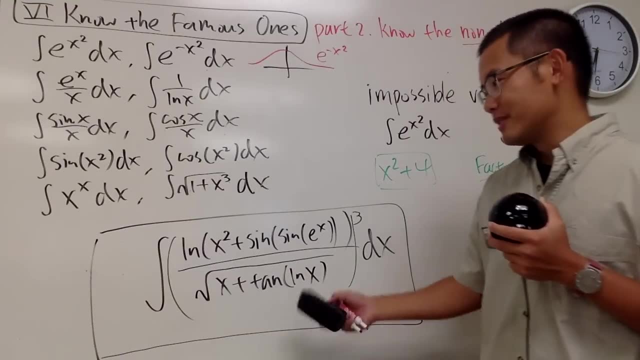 the more math that you study, the more integrals that you do. you may end up with like some non-limit integrals, and then in your class, some of your classmates will just try to mess around with you, Sometimes even teachers too, I know. 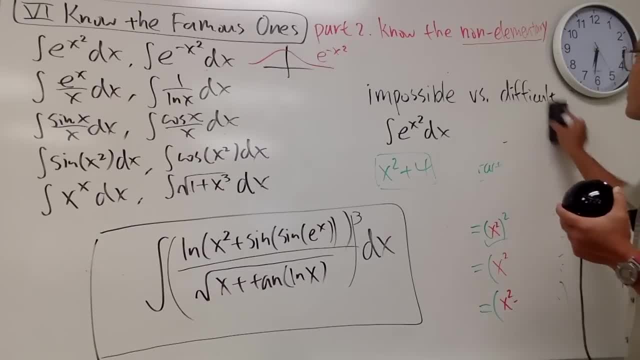 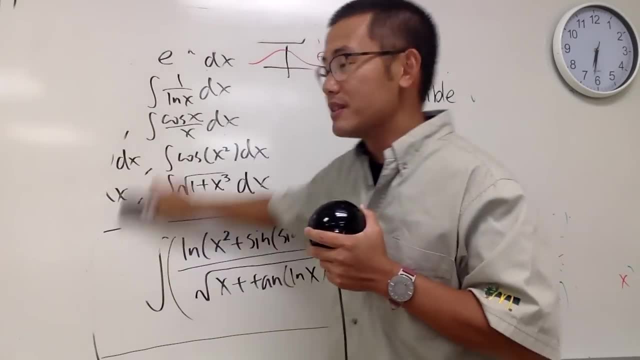 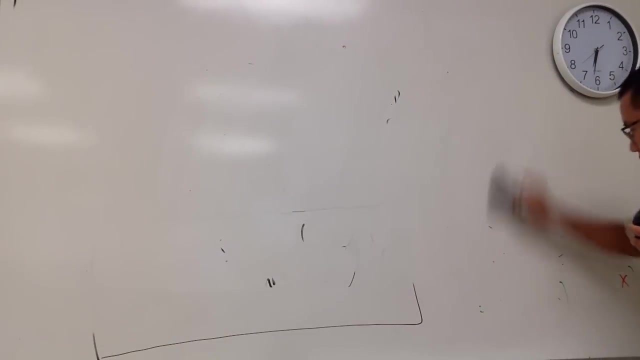 But like, yeah, Okay, So that was category number six, And now we have the hardcore techniques in calculus too. now, right, So for the other ones, for the rest of the video, it is actually going to take me the most of time. 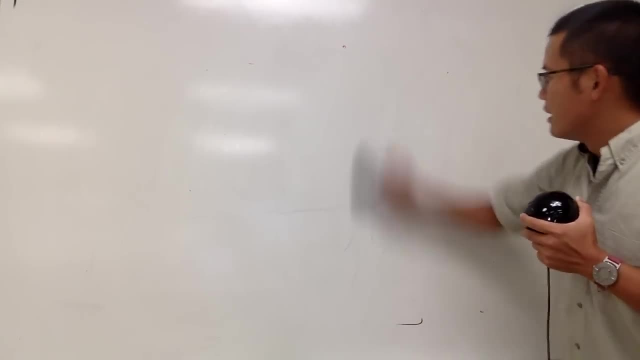 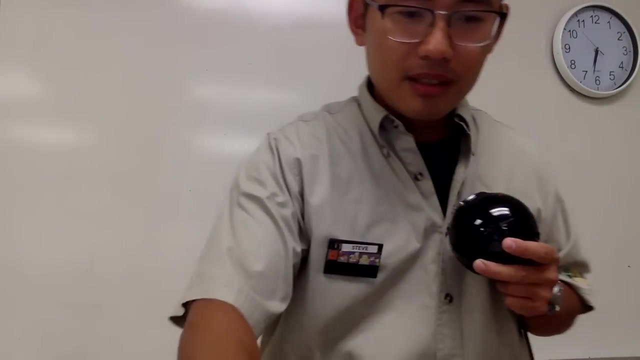 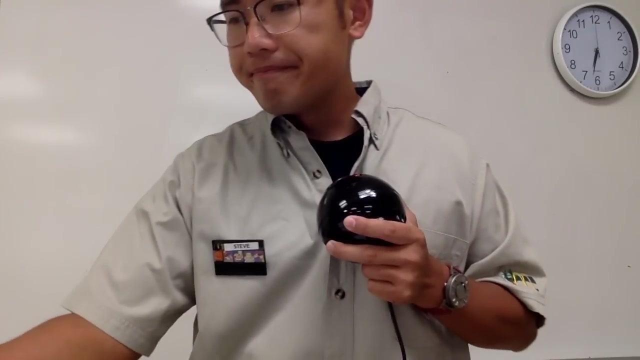 to do the rest of the questions, because here are the new techniques that you guys will have to know. Okay, So we have, let's see, Yeah, One hour 46 minutes, And then we have three pages to go. All right, 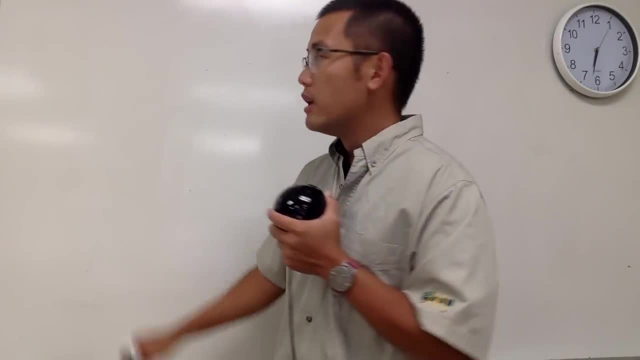 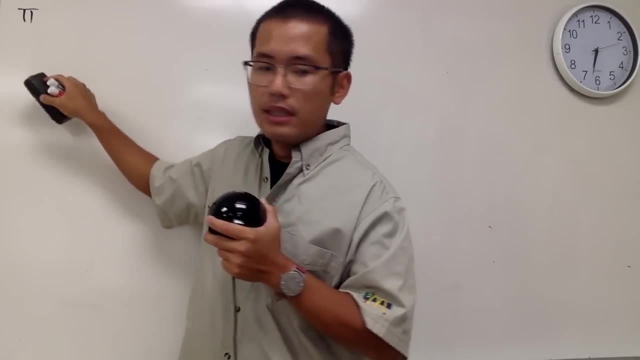 So for each new technique I will have to prove that to you guys, Why The method works. Well, how did we come up with the formula? So pay close attention. Here is category number seven. So this is how we write seven. 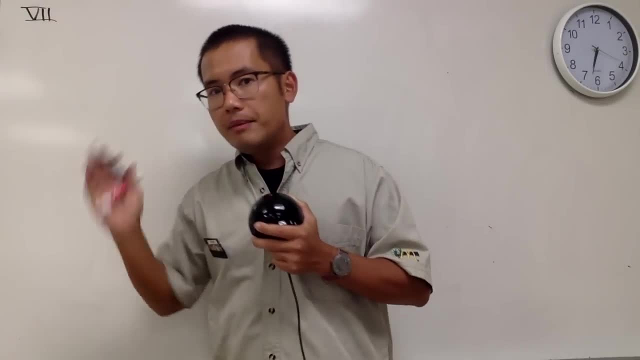 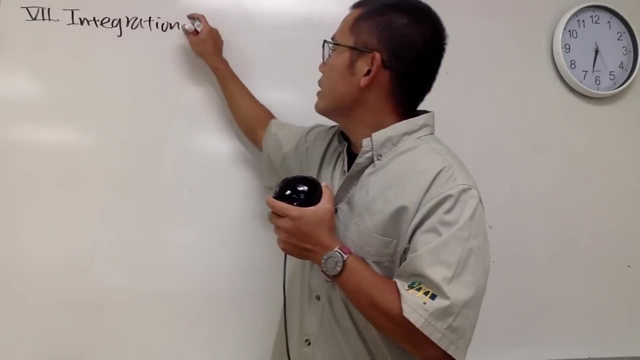 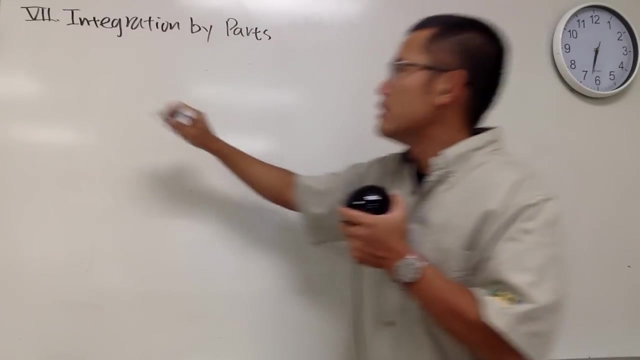 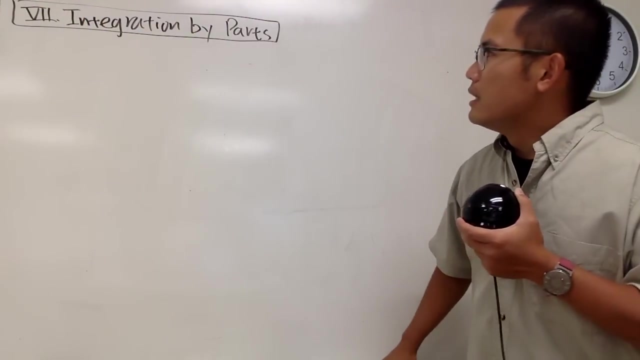 Like this: yeah, So let me just tell you guys what the technique name is. This is called the integration by parts, Integration by parts, Abbreviated as IBP, right? So let's just talk about this first. Okay, 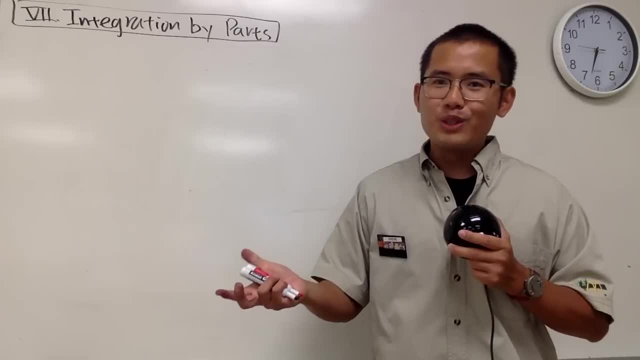 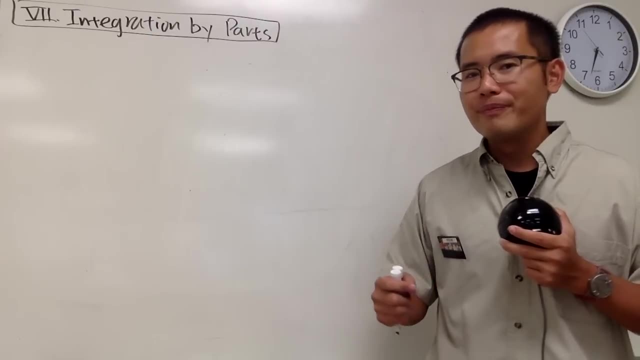 Earlier we had a reverse power rule. Of course we're just reversing the usual power rule, right, And we also had the use-up, And use-up is just like a way to reverse the chain rule. Now, when we have integration by parts, 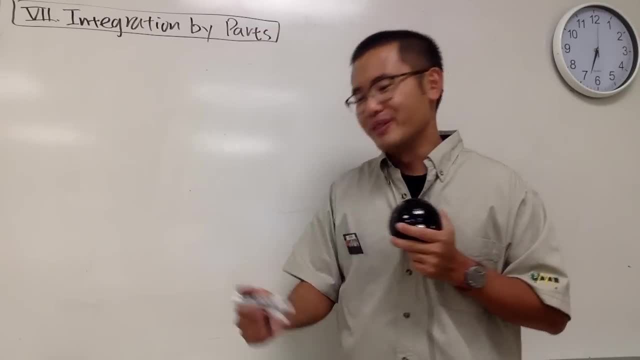 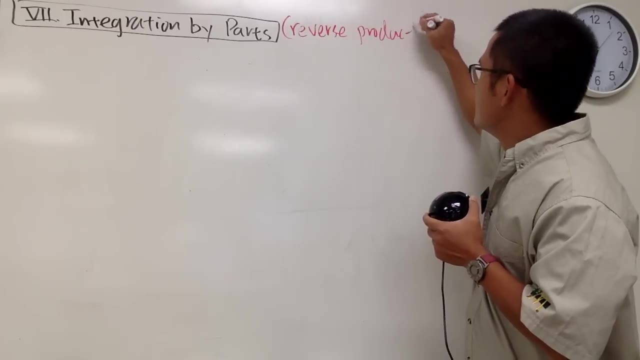 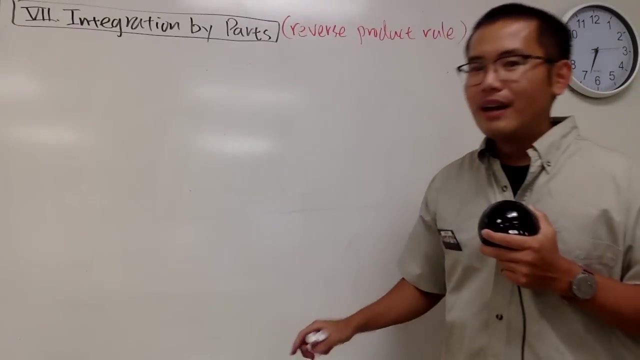 this is the time that we are going to reverse the product rule. So I will just tell you we are going to reverse the product rule, right? So this is the idea And, just like how we did it before, I will have to tell you guys the Google product rule first. 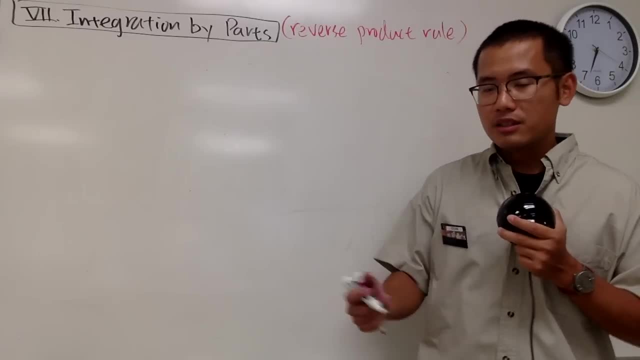 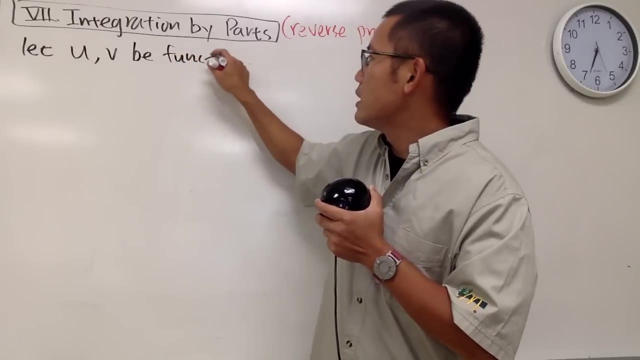 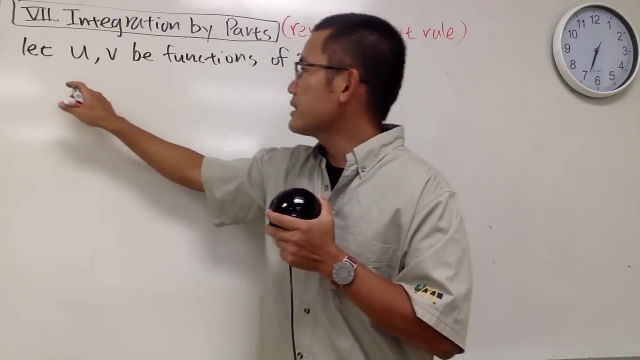 and then I will derive the formula that we need for the integration by parts. So here we go. First of all, let me just tell you guys that let u and v be functions of x, right, And of course we are talking about product. 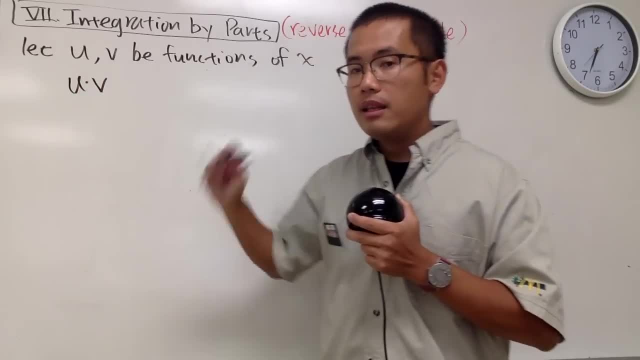 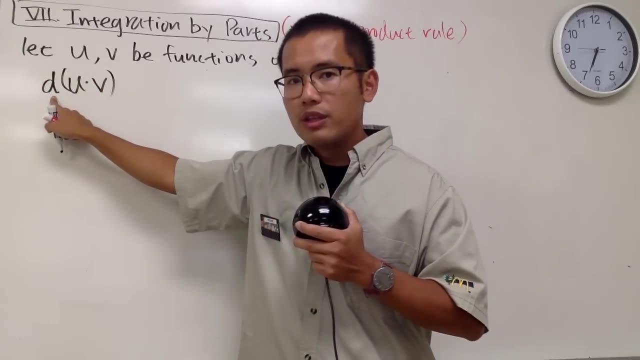 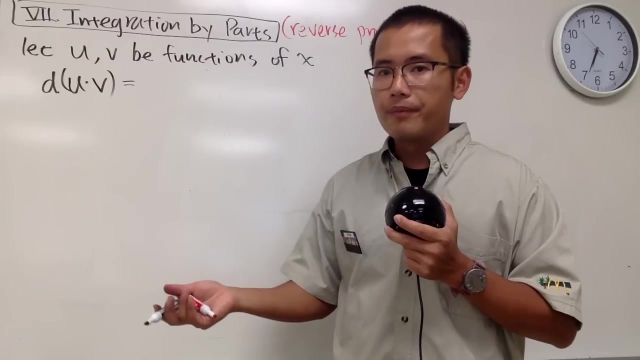 So let's look at u times v, And we are going to differentiate this. And let me just put down d of this to mean that we are going to differentiate the product of u and v, And here is the usual formula for the product rule. 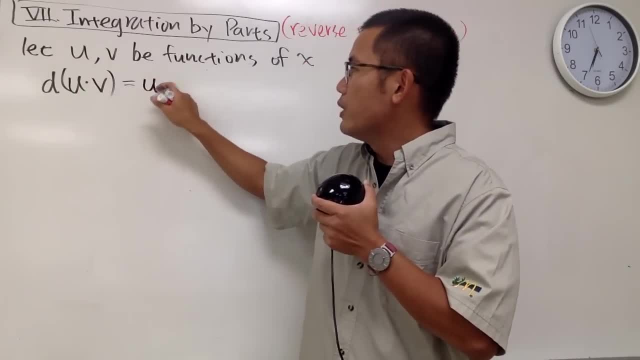 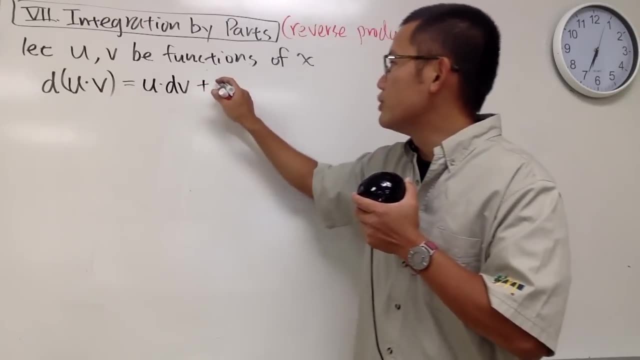 What we are going to do is we are going to keep the first function, which is u, and we multiply by the derivative of the second, and that will be dv, And then we are going to add the second function, which is v. 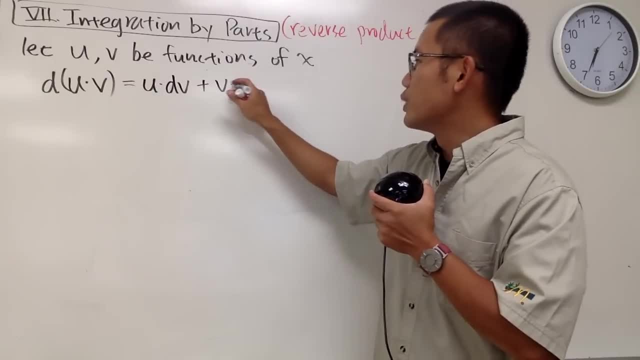 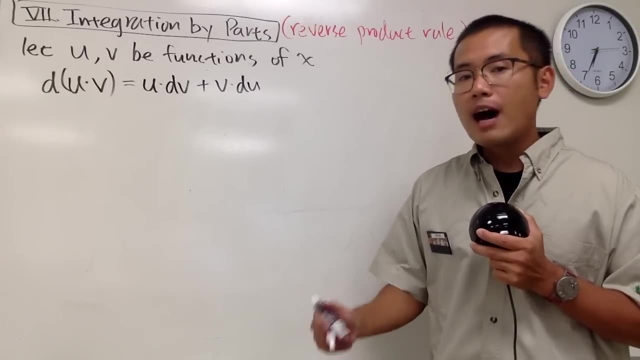 and multiply by the derivative of the first, which is the derivative of u, and we will just write it as du, the derivative of u, like this. So this is the product rule. Now we are going to reverse it. Well, to do that, we will be integrating, of course, 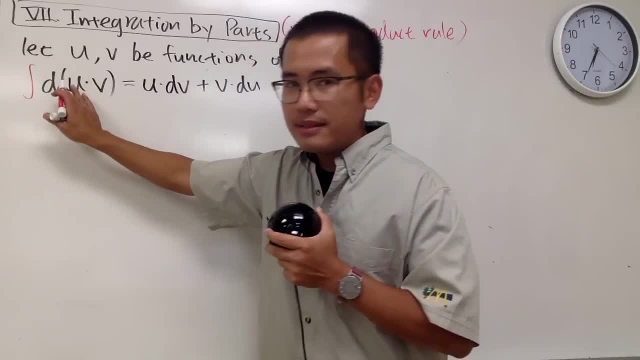 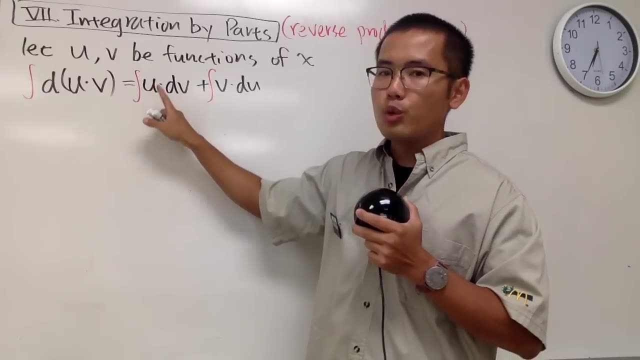 And the beauty is that we can just integrate this and integrate everybody, Because, remember, if you want to integrate the right-hand side, this is the sum. so we can integrate the first and integrate the second. So that's it, And the beauty of all this is that. 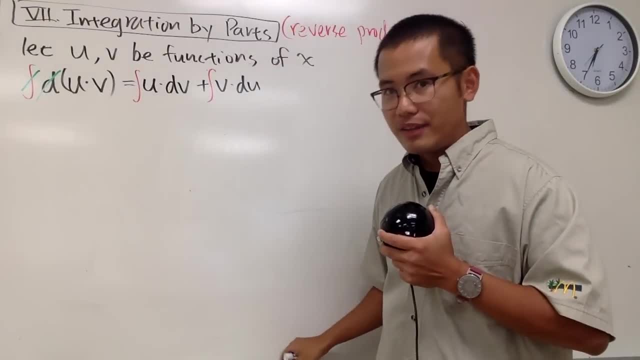 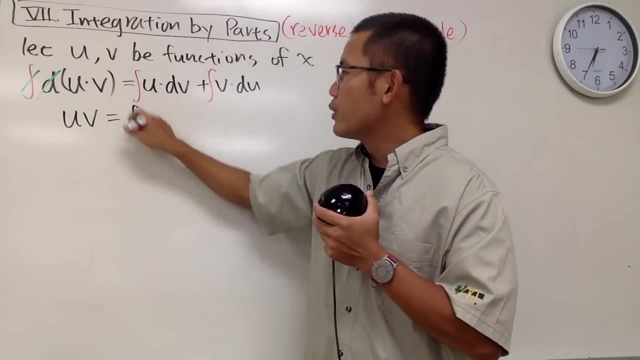 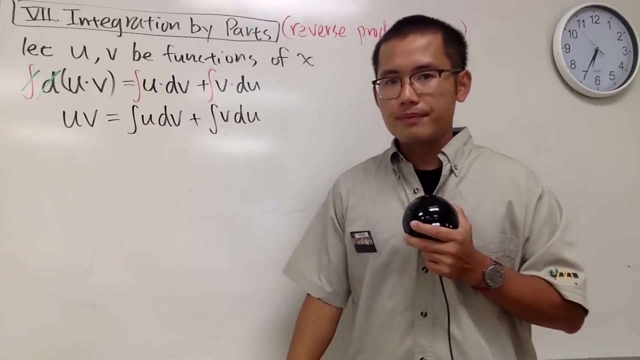 the integral and the derivative. they will cancel on the left-hand side. And now we have uv, meaning u times v, right here. This is the integral of u dv plus the integral of v, du like that And notice how we have two integrals on the right-hand side. 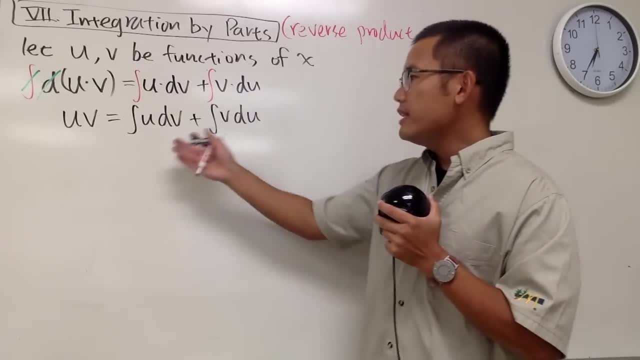 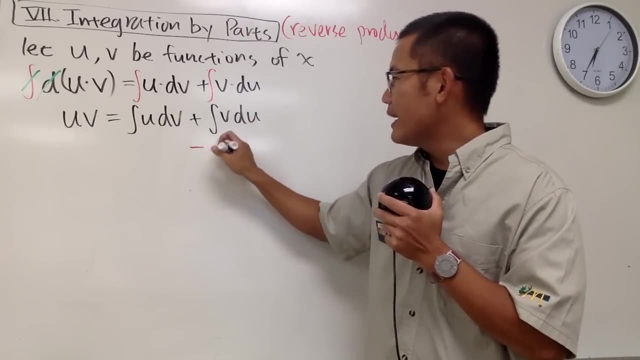 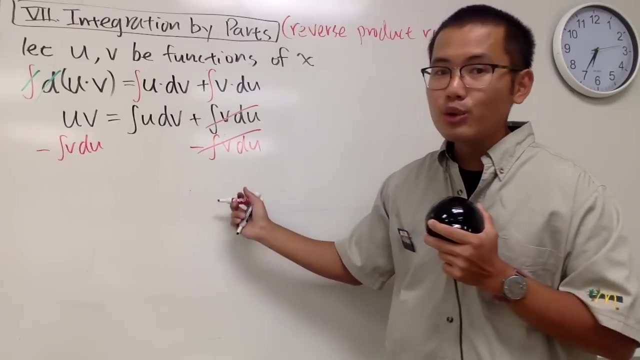 We don't like that And we will just subtract one integral to the other side, And traditionally we subtract this one on both sides. So we are going to minus the integral of v du on both sides And, as you can see, this and that will be cancelled. 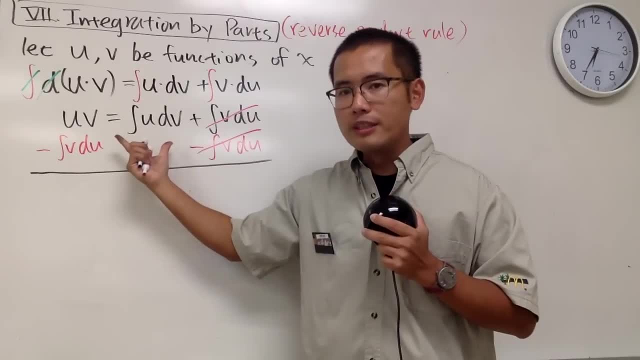 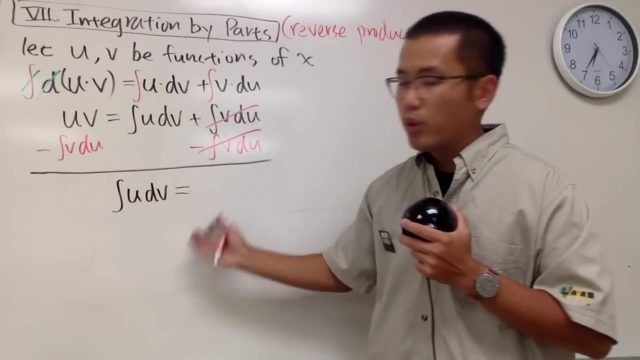 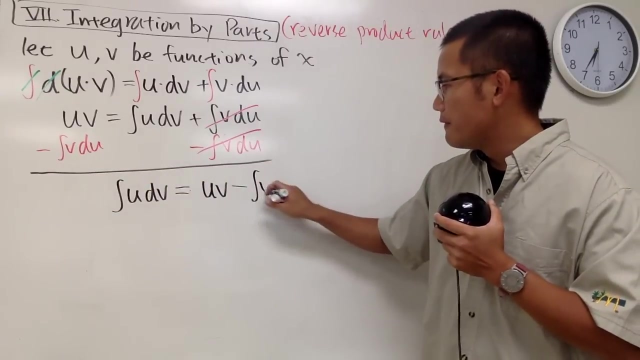 And we have this integral on one side. Let me write this down first, though. So we have the integral of u- dv. That's equal to the left-hand side, is uv minus the integral of v du. This right here is the formula. 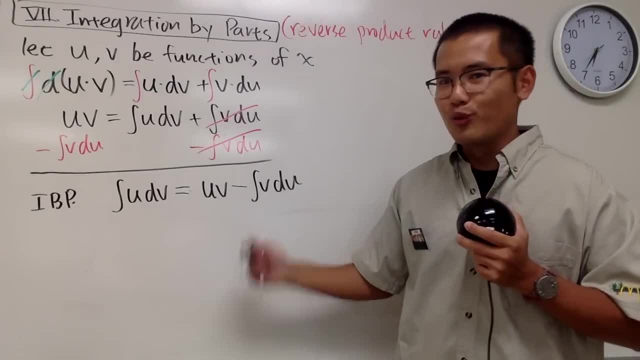 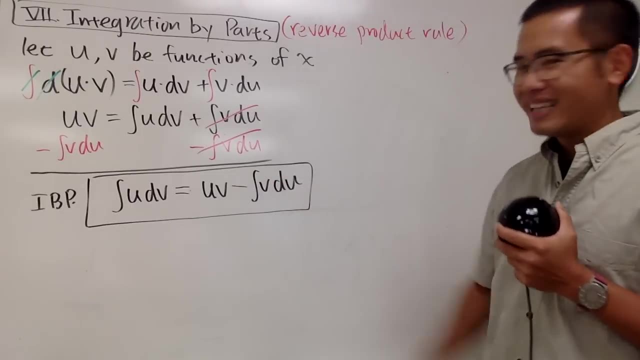 for the integration by part, And this is what I call the traditional format. So this is the traditional format for the integration by part, the u dv format. Now let me give you guys an example And let's do two questions side by side. 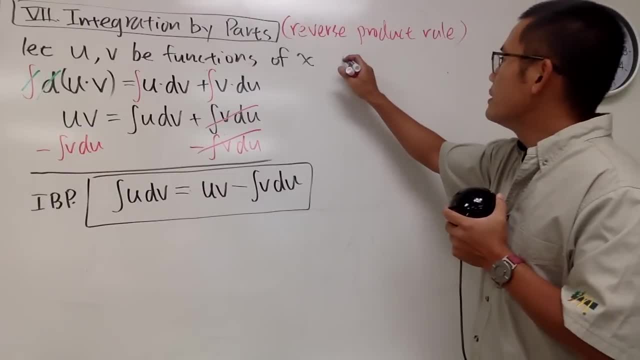 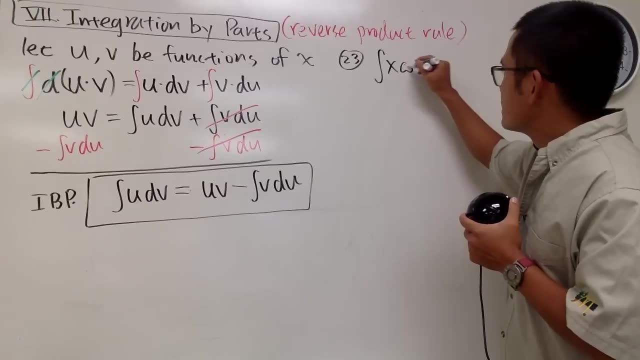 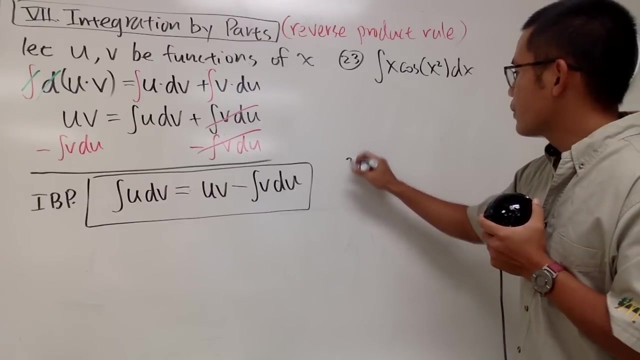 on top of each other again. So here is the deal I'm going to give you guys, question number 23.. And we have the integral of x times cosine of x squared dx. And right here we also have question number 24,. 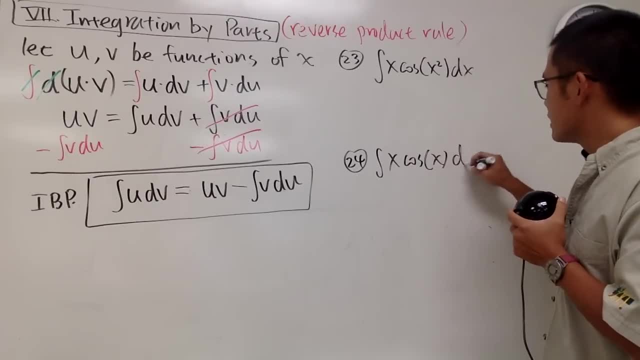 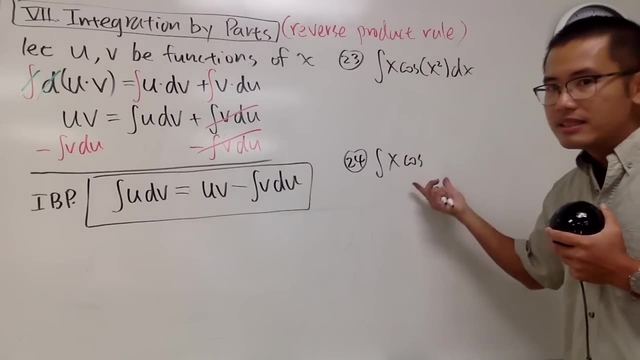 the integral of x times cosine of just x, dx, Like that, Okay, And in fact if you just have one x inside of the cosine, you don't need the parentheses. So let me just put this down right here: If you have x squared, 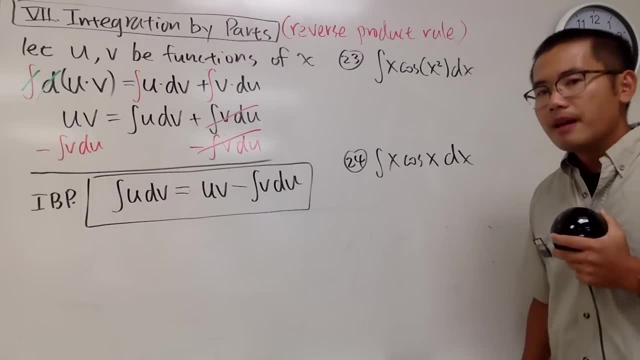 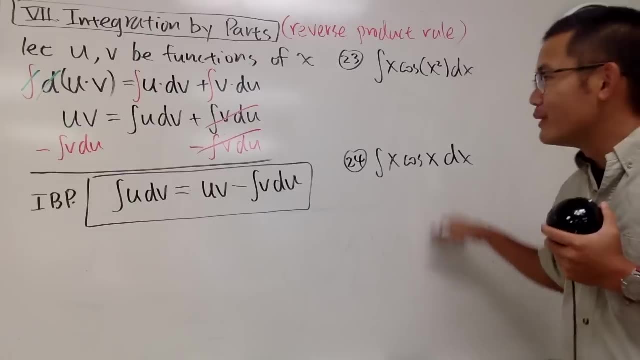 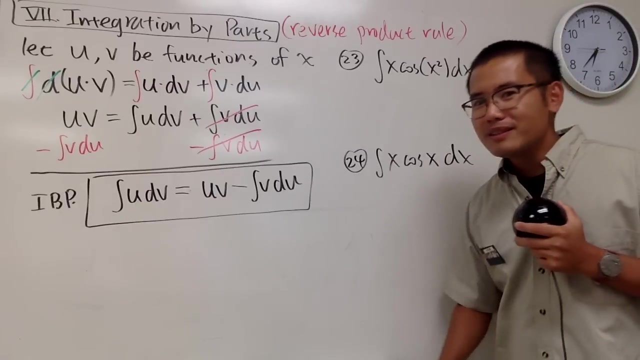 be sure to use the parentheses. okay, Now, if you have a choice to have just one of this integral on the test, which one would you rather have? 23 or 24? Michael Jordan or Kobe Bryant? Of course, 23,, right. 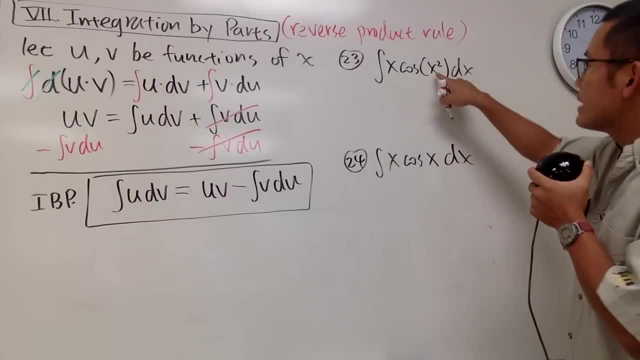 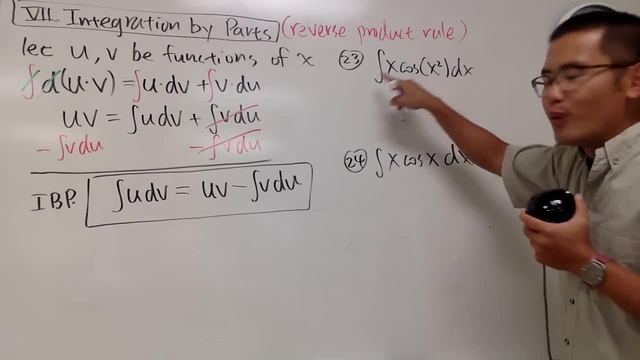 Well, the reason for this is that notice how we have x squared inside. The derivative of x squared is 2x and we have the x on the outside, So we can do this with u sub real quick. Let's just make that happen. 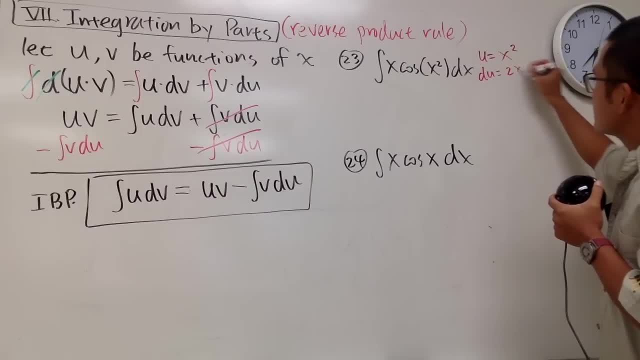 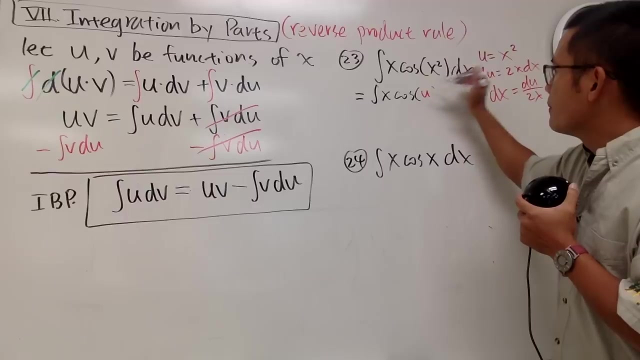 Let u equal to x. squared, du is equal to 2x dx And divide the 2x on both sides, dx is equal to du over 2x. Take this integral to the? u world, We get the integral of x cosine of u. 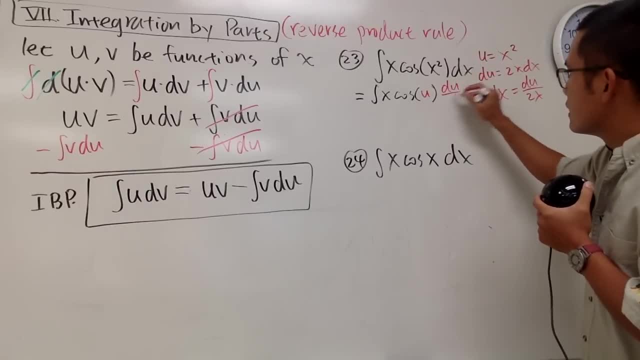 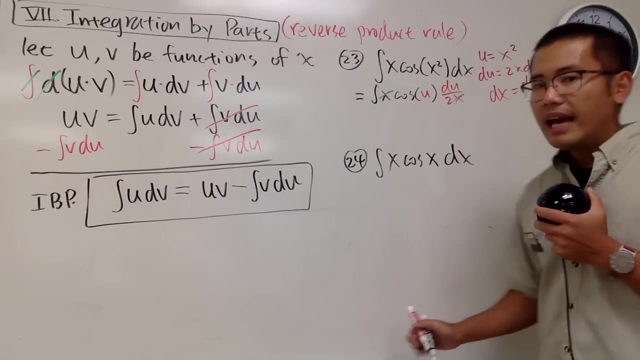 And this right here is du over 2x, And this is so wonderful Because the x cancel each other very, very nicely, And of course we have the 1 over 2, and that's the constant multiple. It doesn't hurt us at all. 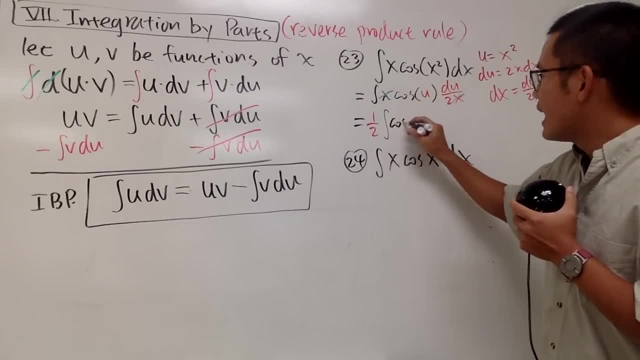 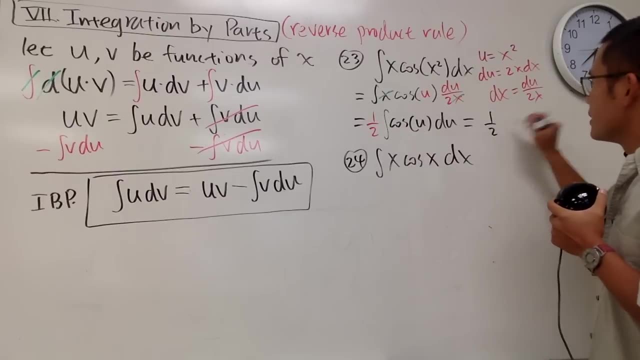 And then we have the integral of cosine of u du like this: Well, 1 half is just 1 half, No big deal. And then the integral of cosine is positive sine. So we get positive sine right here And we will have the? u right here. 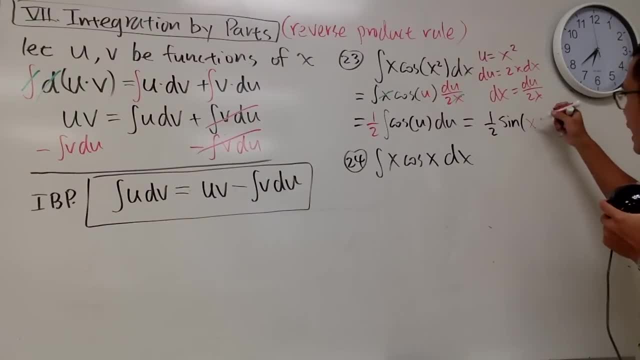 But u is x squared, So I just put down x squared right here, And the answer to this integral is just 1 half sine of x squared, And we're all done. So put a plus c. This is it, However, for question number 24,. 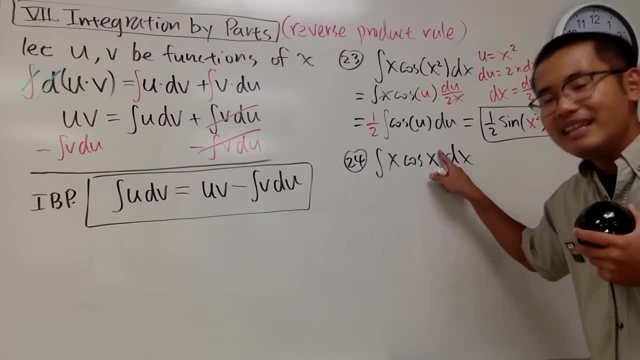 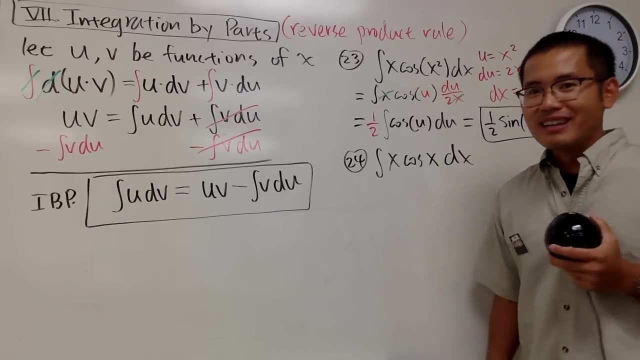 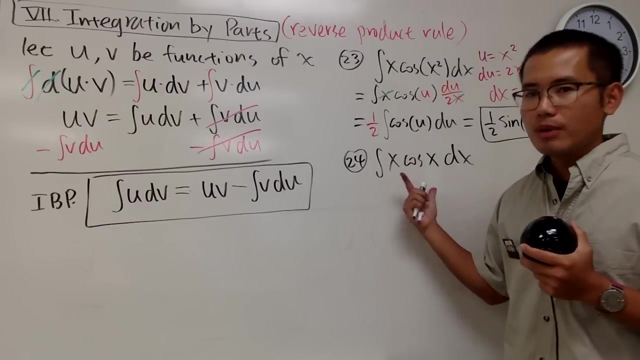 we don't have the x squared right here anymore And in fact u sub won't work. You can try, But u sub just won't work. I'm sorry, And now you see this right here might look impossible before. integration by parts. 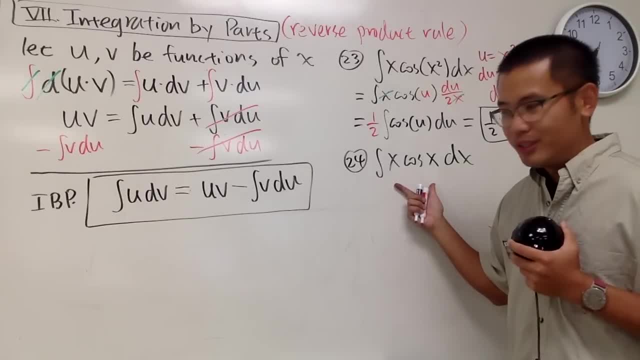 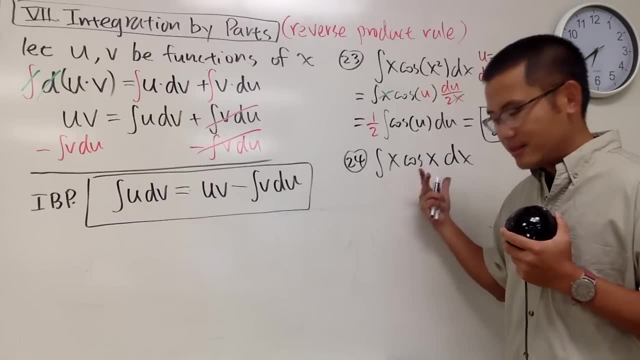 But with this method it's actually really possible. It might be just difficult at the moment, but once you practice a little bit, once you are able to do it, try to say that hey, this is pretty easy and that's how you can get the confidence right. 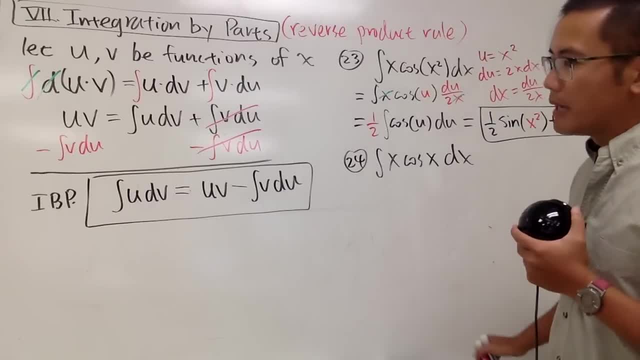 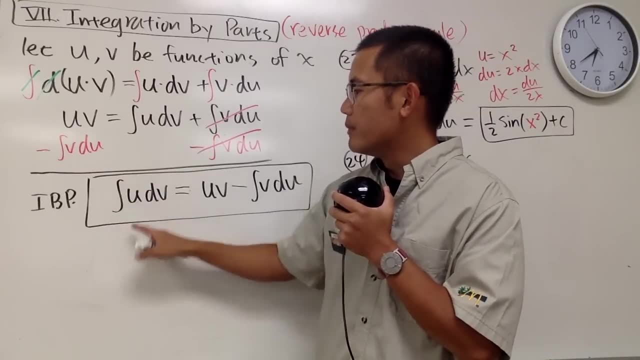 Okay, This is how you are going to work out the UDV format. Have a look right here. The idea of the integration by part is that notice how we have the integral of UDV And we end up with this formula and we have another integral. right here. 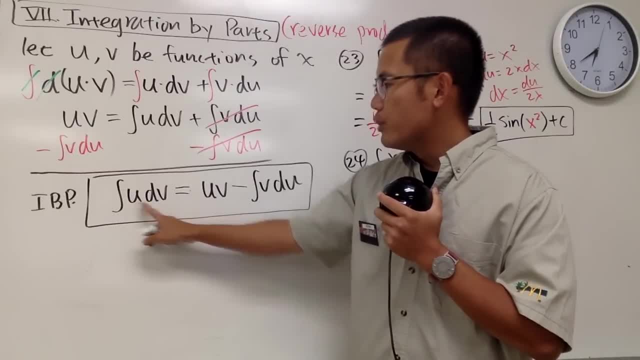 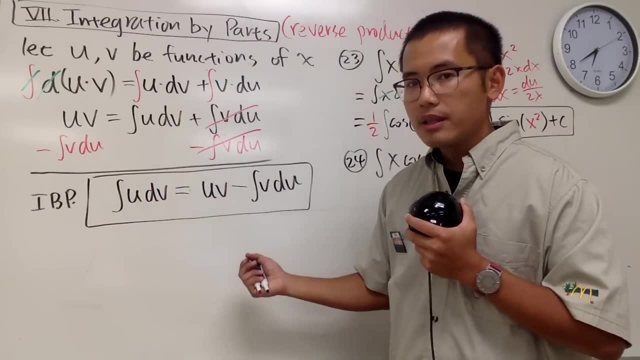 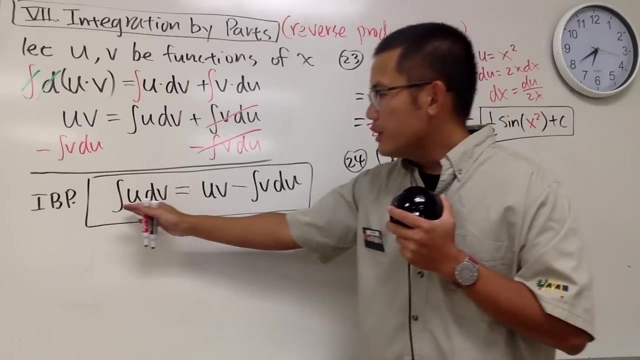 Notice: here we have U, here we have DV, And you see how we have the V right here. From DV to V we have to integrate And from U to DU we have to differentiate. The idea is that look at the integral right here. 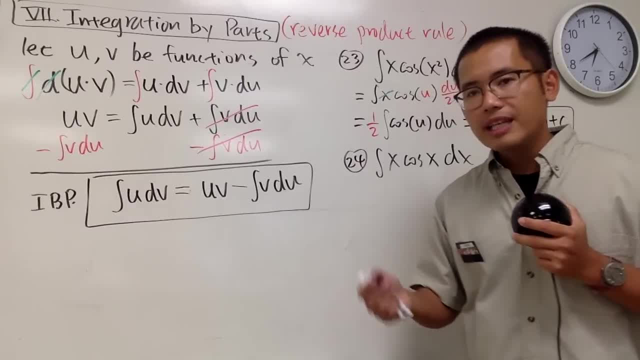 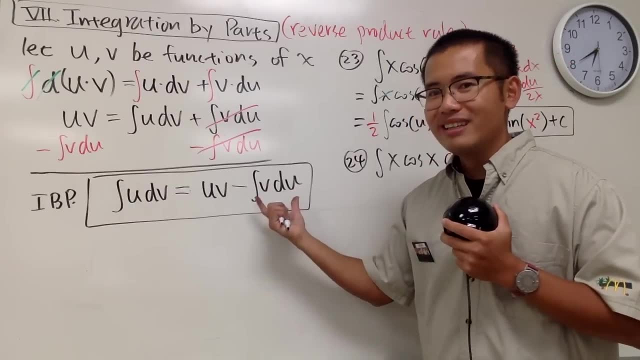 We are going to pick one part to be differentiated and the other part to be integrated and use this formula right here to construct our answer, And hopefully this right here is an easier integral than the original. That's the idea Now. this is the setup. 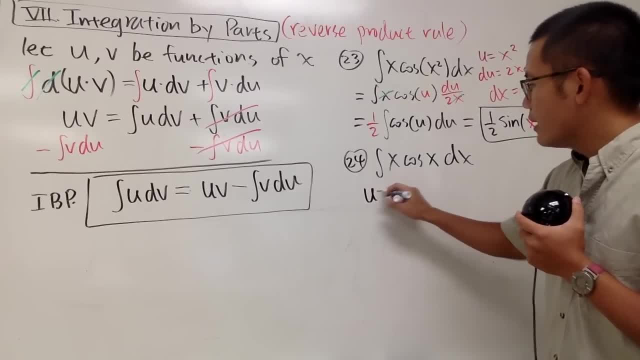 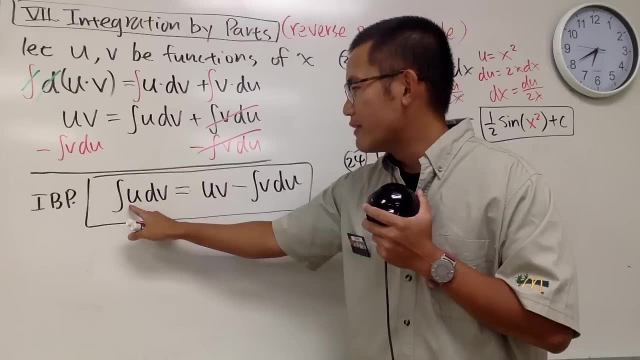 I will tell you: First of all, let's put on U right here and we are going to make our selection, and then I'm going to put on the DV right here, right, Notice that we have the UDV, UDV. 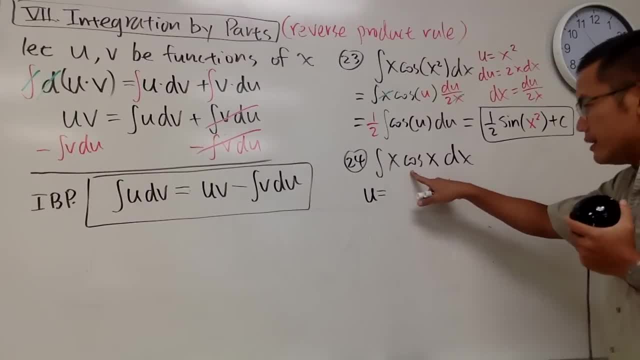 We are going to make our selection And in this case let me just tell you guys this: first, We are going to be putting down cosine X DX to be our DV. Let me just write that down: Cosine X DX to be our DV. 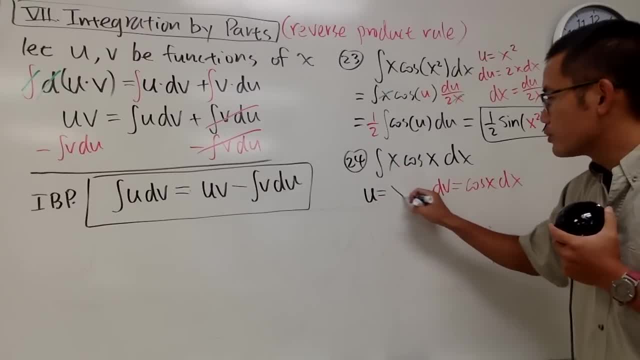 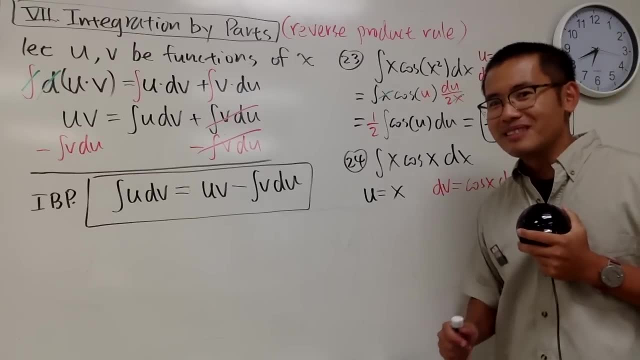 And then we will be putting down the X for the U. So let me just write that down. And you might be wondering why I make this selection. Well, again, perhaps just like this is the famous step, But no, We will talk about that later on. 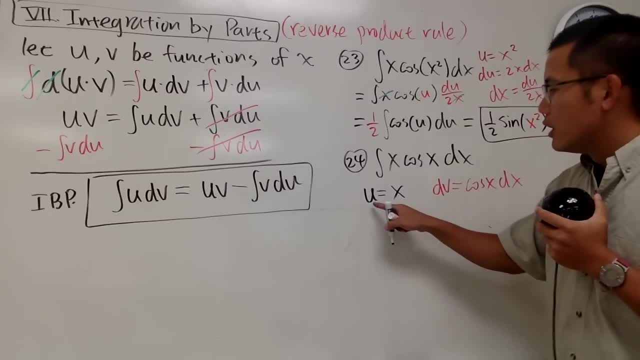 Anyway, this is how we make the selection, and then we will just proceed To go from U to DU. of course, we just differentiate. Differentiating X, we get 1, and don't forget the DX. So in this case it's just: DU is equal to DX. 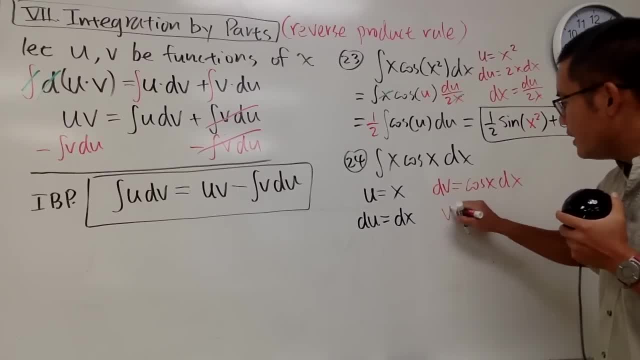 However, for this, though, we have to go from DV to V, and that's integrating both sides here, And here is the idea. When you make your selection for DV, you always have to ask yourself: can you integrate this part nicely? 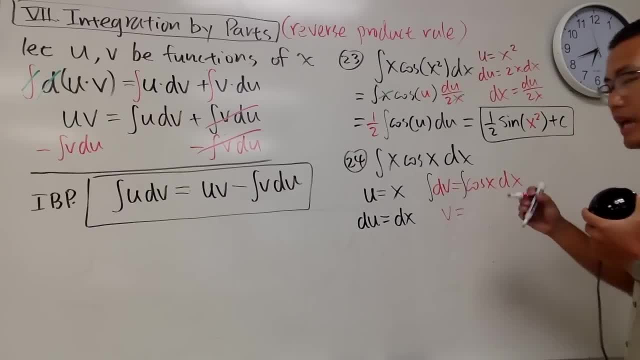 In this case, yes, we can right. So, integrating cosine, we get positive sine. So when you go here, we get positive sine X. And in this situation, even though I integrated, but do not put down plus C, because this is not the whole integral, 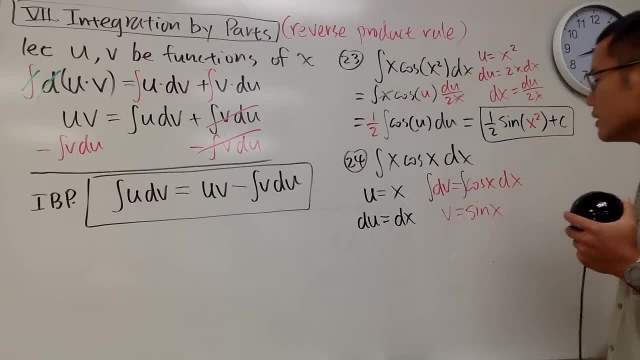 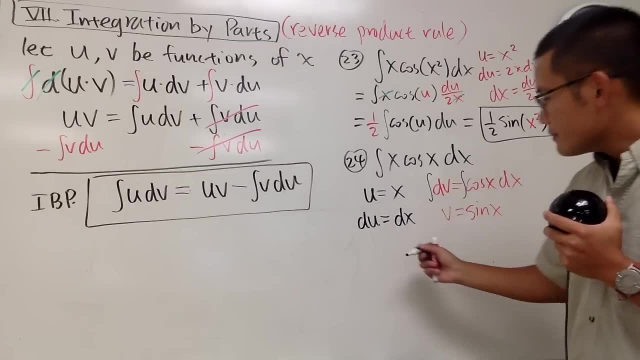 I will just put down the plus C at the very end, right? So this, right here, it's pretty much the same thing, right? I just break it apart and then this is the setup. Now, this is how you are going to construct the answer. 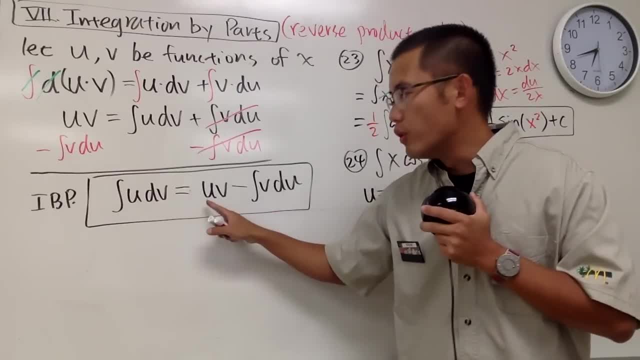 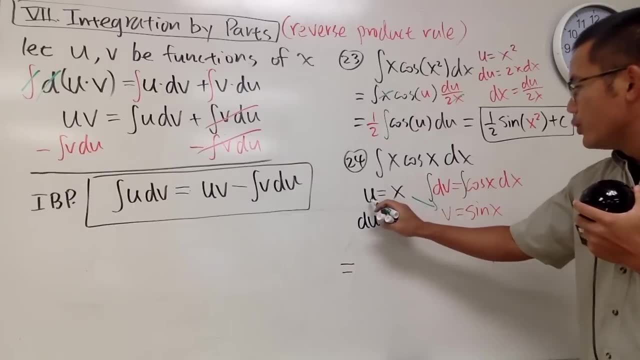 Here we are going to do. you see, integral U DV is equal to U V and U V happens to be right here This times that U times V, and we're just going to put down the X and this together. 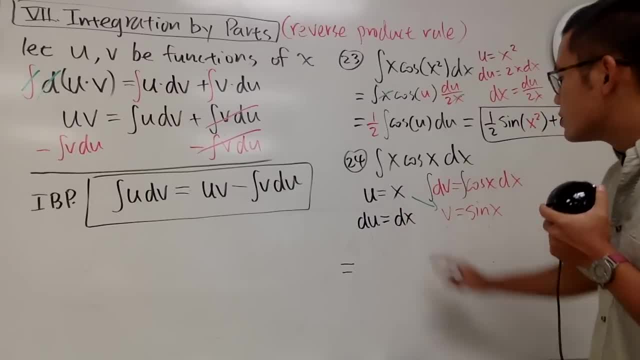 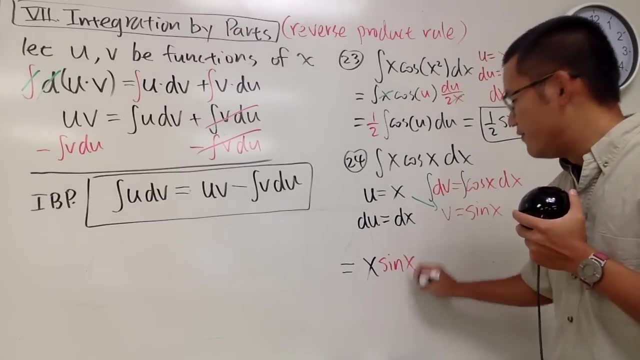 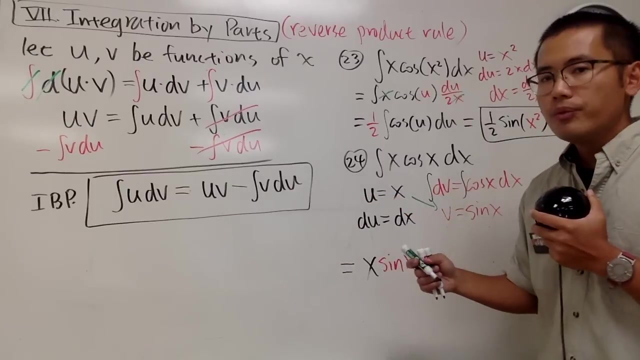 Of course, this right here is just a name. These are the actual ingredients that we want. So U times V is just X times sine X, X times sine X, and that's very nice, And then we have to minus the integral of V DU. 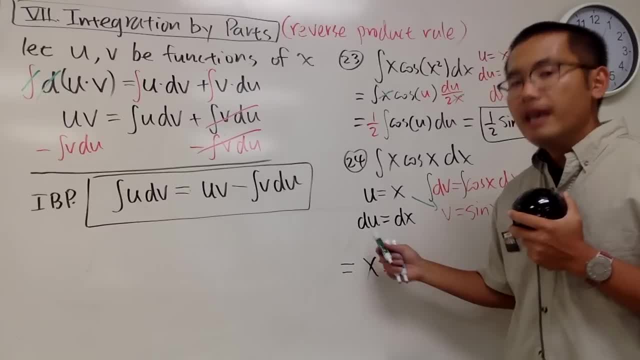 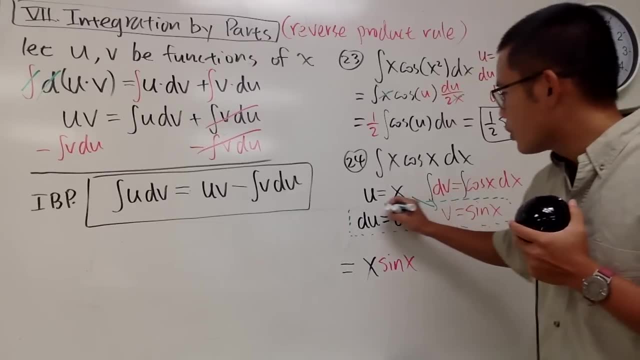 Notice, the V is right here and the DU is right here. In another word, we are going to just multiply this row. We are going to multiply this row And we have to put that in the integral, and this is the minus integral. 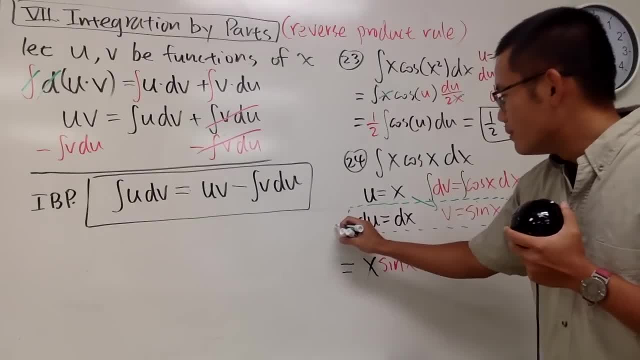 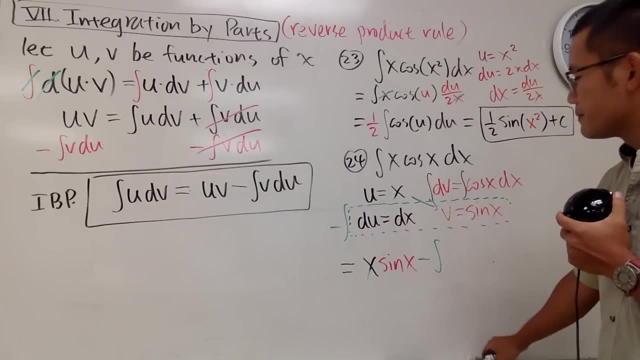 This is the minus because of what we did. So remember, we have to minus the integral of this times that. So let me just put it down right here: Minus the integral Again. we just have to put this and that down. 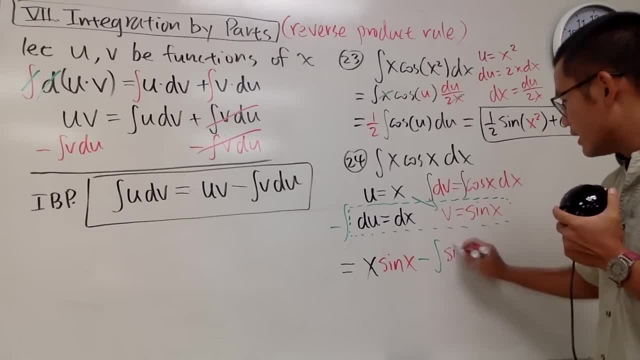 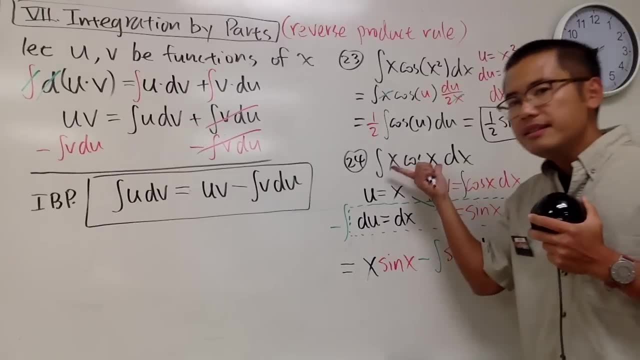 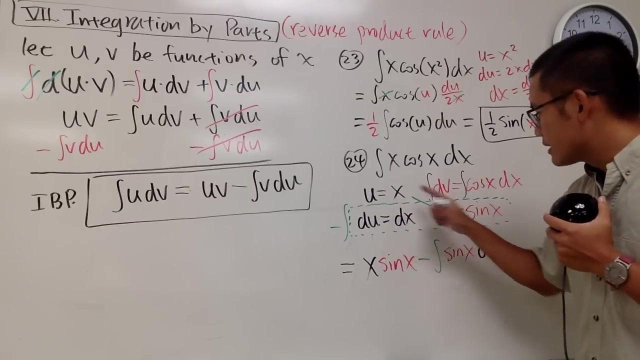 Let's write down the sine X first. So we have the sine X and then the DX right here, and that's the DU part. So this is originally what we have, and now this is the first part of the answer. When we did this diagonal right this times that 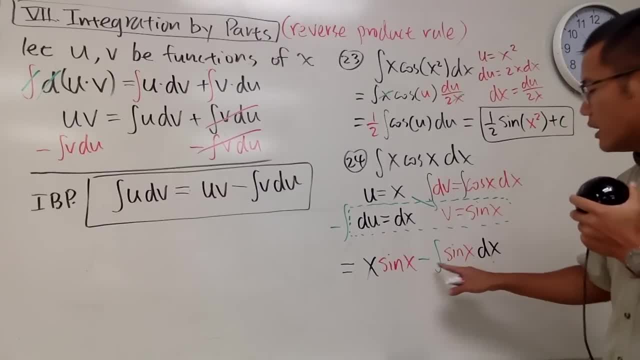 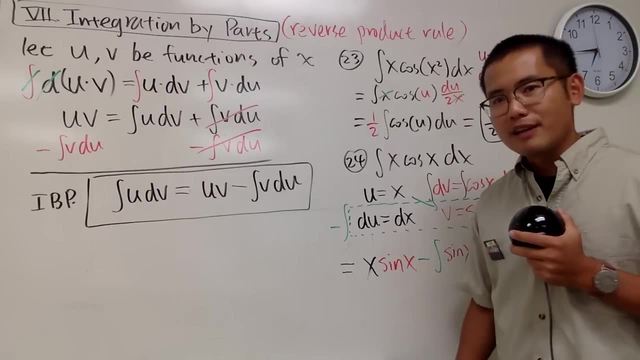 And then we still have another integral to work out, the integral of negative, the negative integral of sine X. And what's the integral of sine X? Negative cosine X, And that's pretty much it, because this right here we can totally do it. 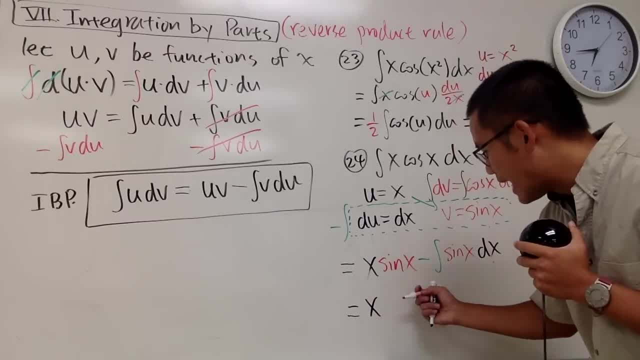 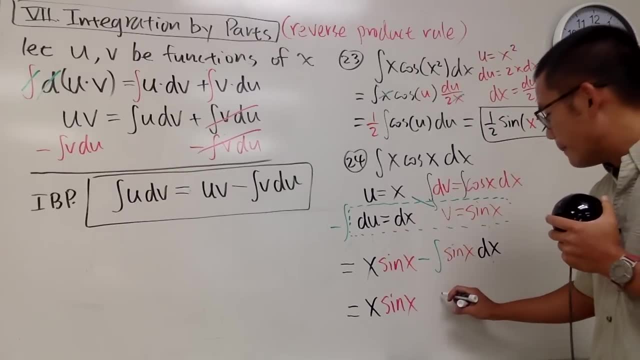 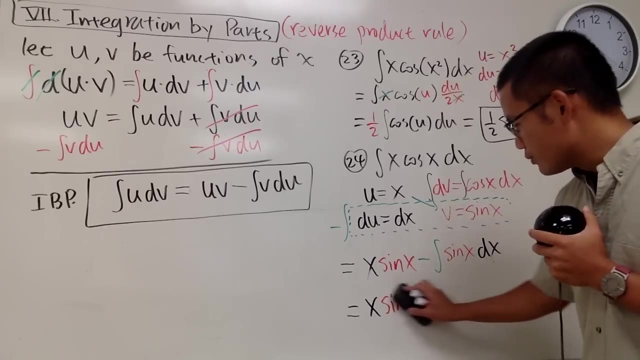 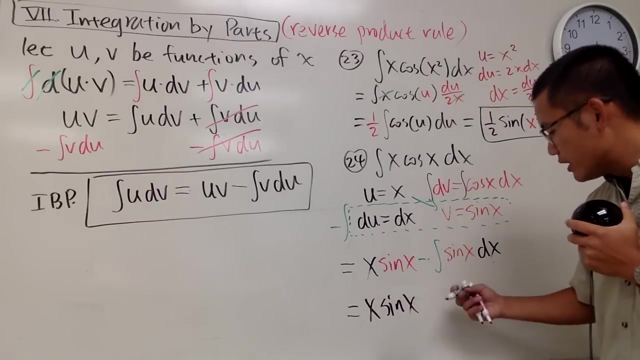 So we get this. We have X times sine X, but the integral of sine X is negative cosine X. So notice how originally we have this negative already. Let's actually just write everything right here back: X sine X. Notice how originally here we have this minus already. 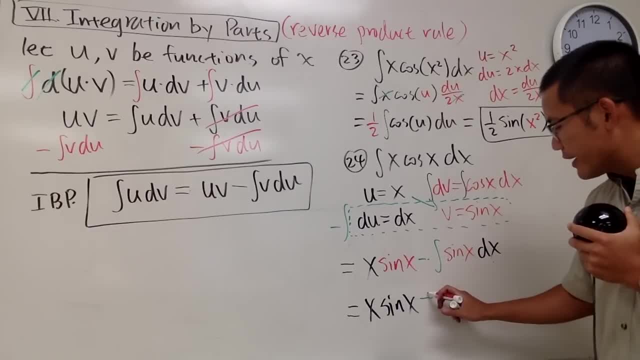 but the integral of sine is negative, cosine negative times. negative is positive, and then we have the cosine right here. That's it And we're all done. So put a plus C right here. This is the answer for that right. 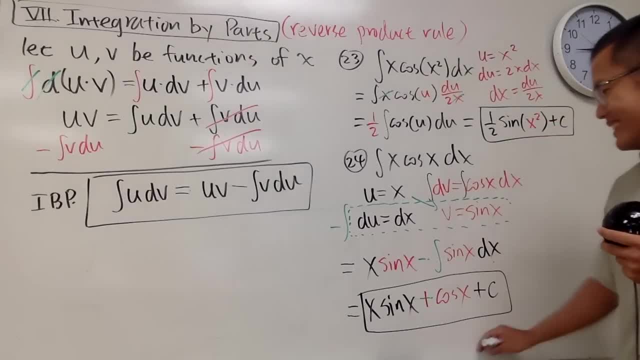 So, integration by parts, integration by parts: Take one part to be differentiated, the other part to be integrated. That's the whole thing, right? So take a look, take a look, take a look Again. this might seem impossible. 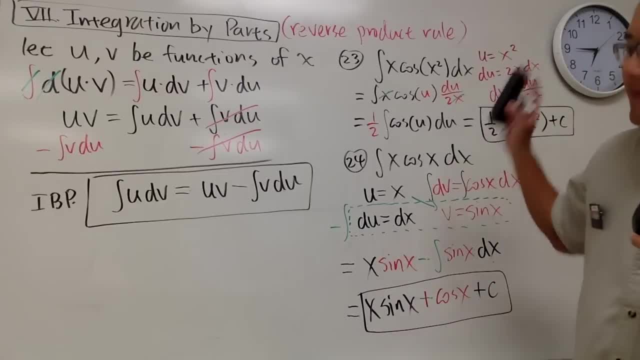 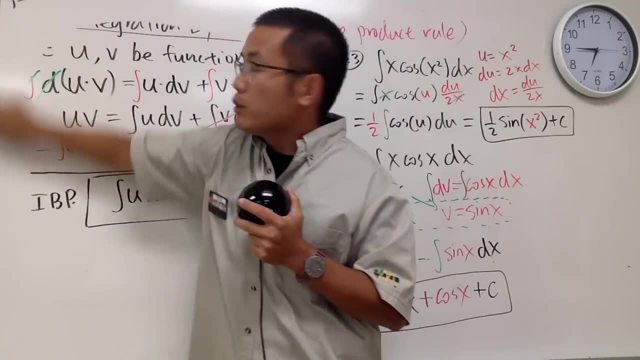 but sometimes it's just that we don't have the tools yet. right Now I will show you guys a couple more examples for integration by parts, and I will also show you guys a much better setup than the ones that we just did. 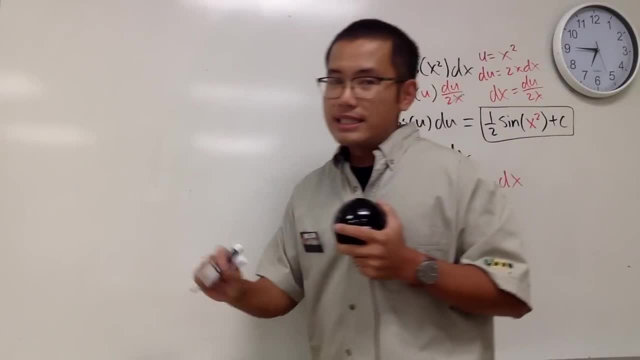 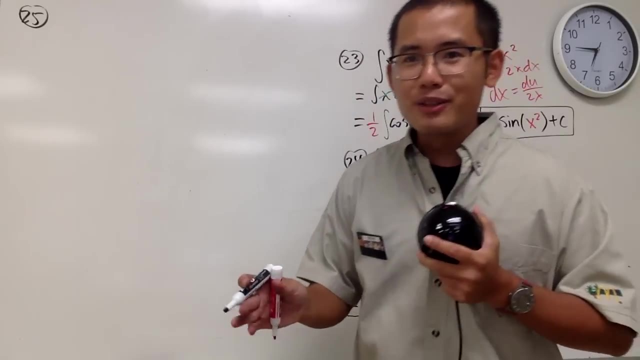 So number 25, oh man, it's not 50% done, even though, yes, this is 25, but again, the methods will take the most amount of time because I have to go over all the new methods. I'm trying to do all this from scratch, right. 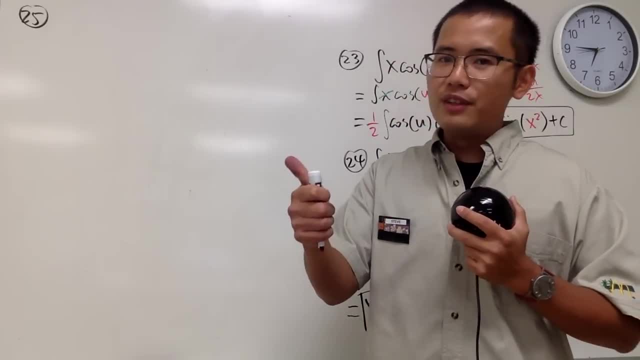 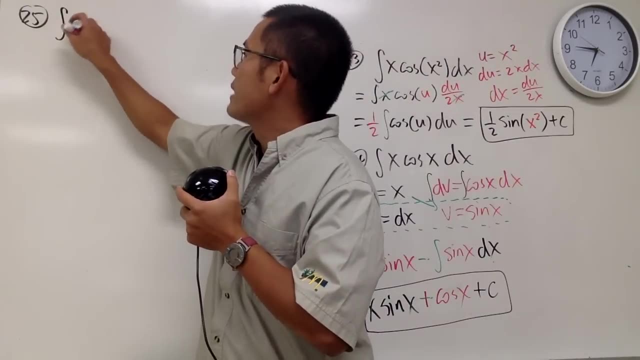 And if you guys find this video to be helpful, just give this video a like. Thank you guys so much. I really appreciate that. Okay, number 25.. Let's look at the integral of x to the third power. natural log of x- dx. 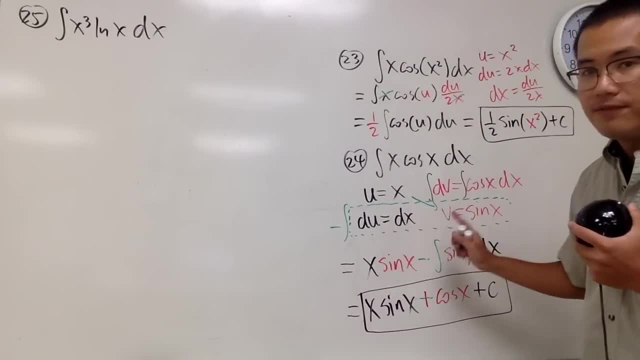 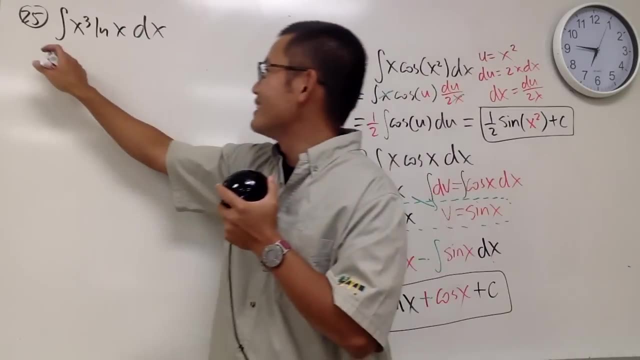 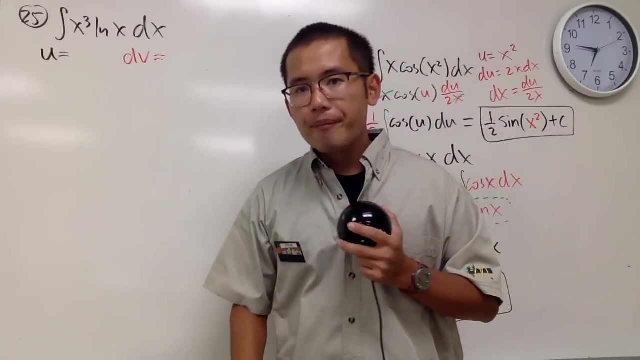 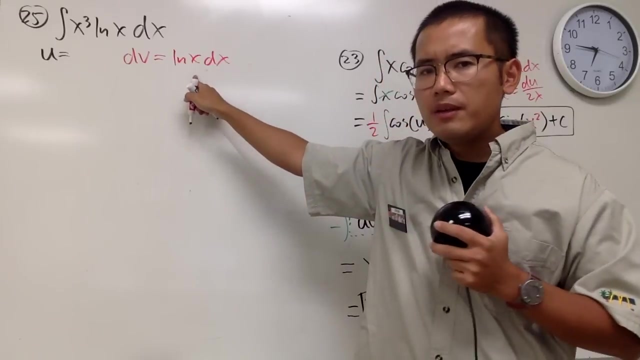 Well, we are going to set this up first. Again, we are in the integration by parts section, so you know you can expect that we use integration by parts. Let's put on u and dv. Okay, now, this time let me put down ln dx. first for dv. 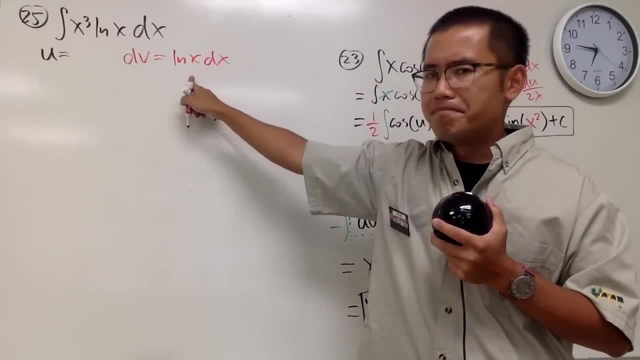 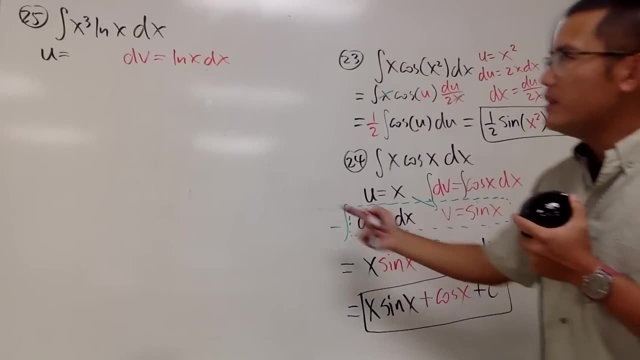 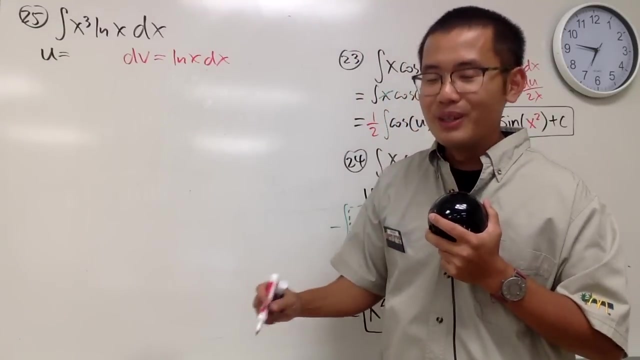 Is this a good choice? No, because, remember, if you have dv right here, you actually have to integrate the dv in order to get the phi And what's the integral of natural log of x? Well, to do that, you actually have to use integration by parts. again. 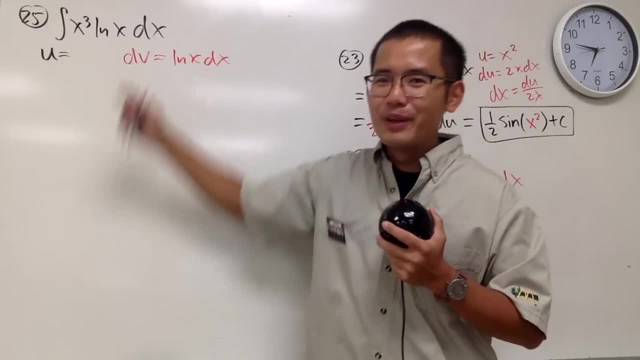 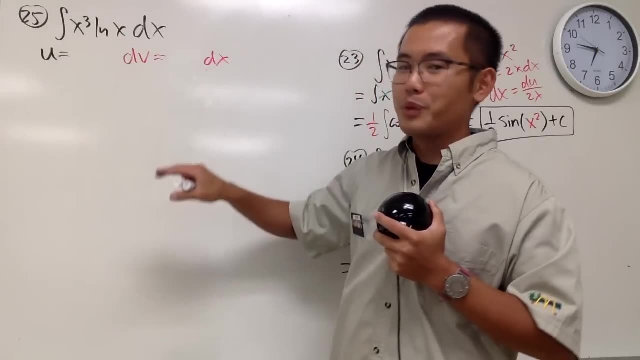 And I don't think you want to integrate by part instead of the integration by part question, right? So we are not going to do this Again. natural log of x. we don't want to integrate that. Well, in this case let's just switch it. 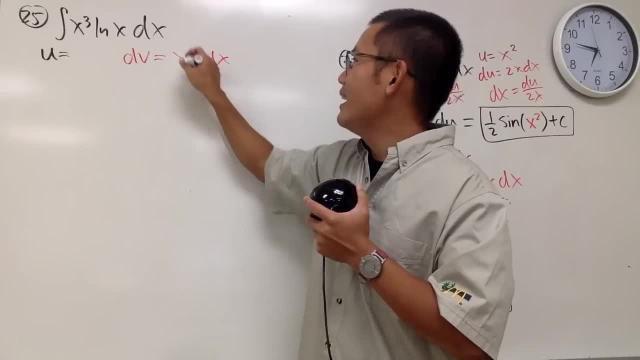 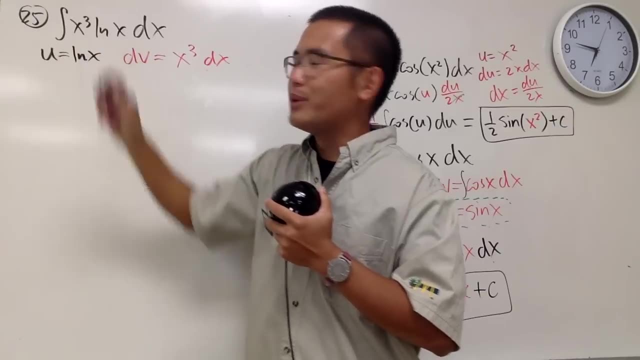 So let's go ahead and integrate the x to the third power. So I'll put the x to the third power for the dv and I will put natural log of x to be the u, And this is going to work out so much better. 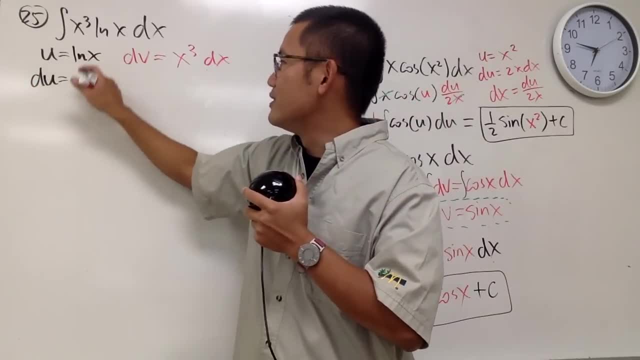 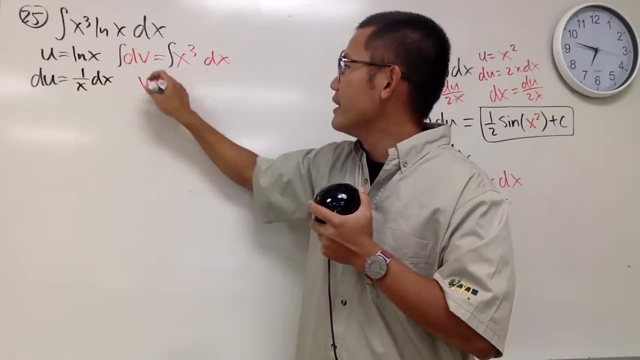 because you'll see that if I differentiate this, this is just 1 over x, dx, And if I integrate this, this is not that bad at all. We get phi equals 1 over 4 x to the fourth power, just like that. 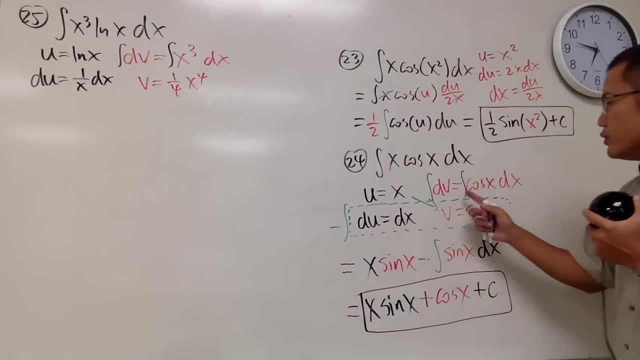 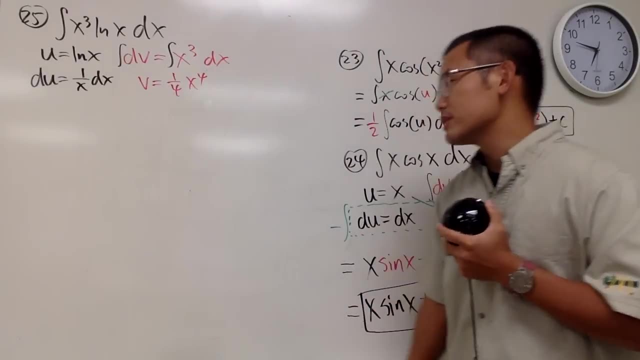 It's very easy to achieve right. So, again, you should always consider what you are going to pick for the dv, And when you do that in this case, it works out much better. of course. Now we're just going to construct our answer. 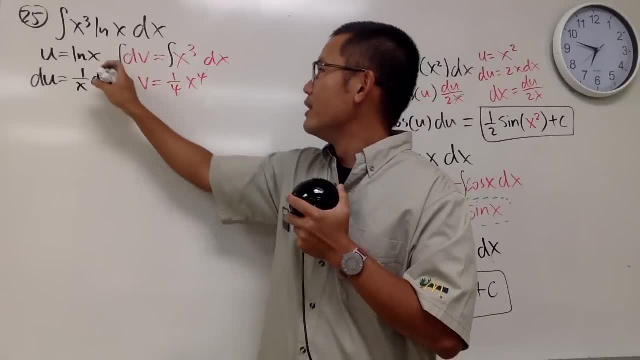 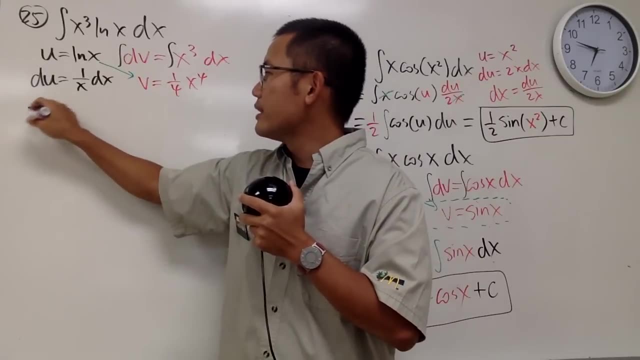 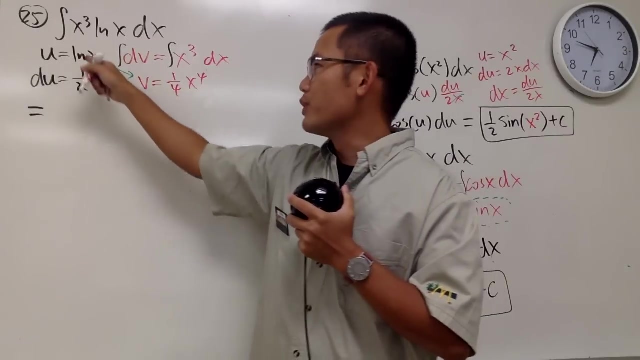 Of course here is our favorite diagonal: u times phi. So that's the first part of the answer and I'm just going to write it down right here for you guys. We have this times that and we write down the polynomial first, before the natural log. 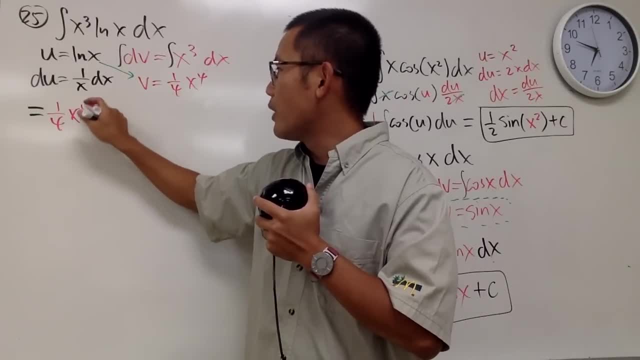 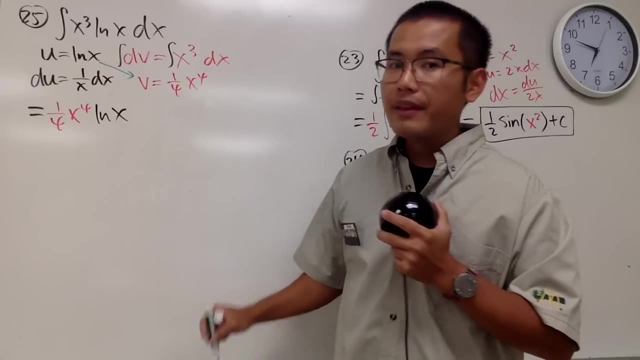 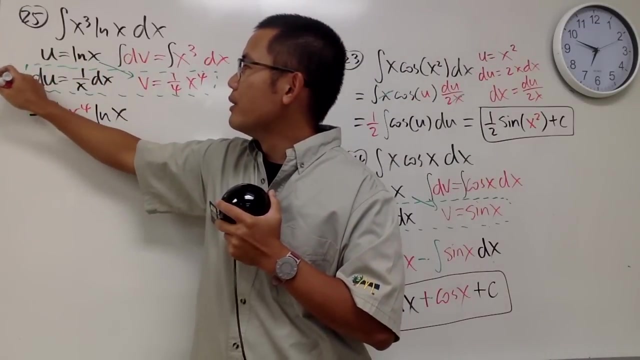 so this power 1 over 4 x to the fourth power times. natural log of x like this. That's the first part of the answer. Then we are going to multiply by this row And don't forget, we have to put them in the integral right. 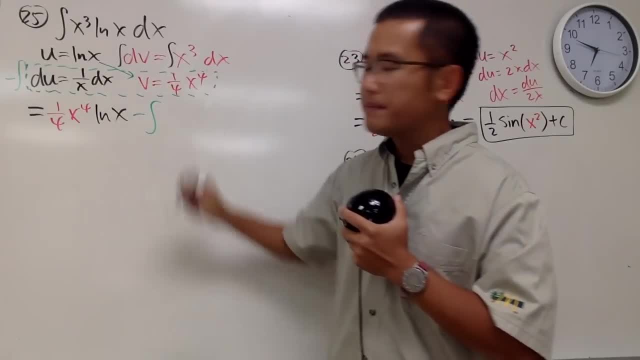 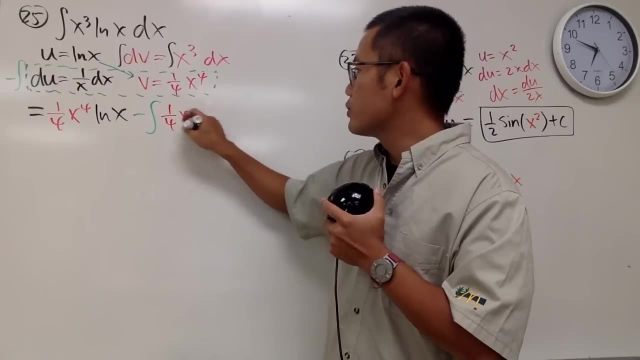 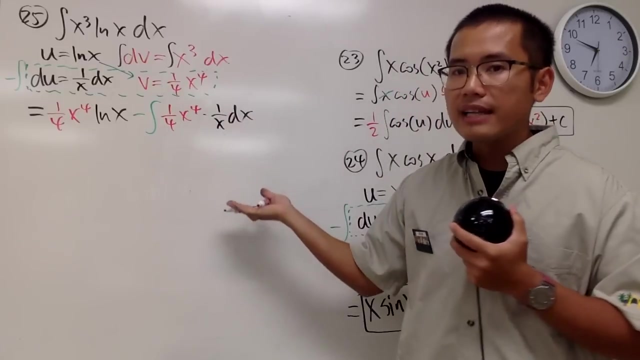 It's the minus integral of this data, so minus integral, right? Okay, Let me put down this right here, which is 1 over 4, x to the fourth power, and we also have this part which is 1 over x, dx, like that. 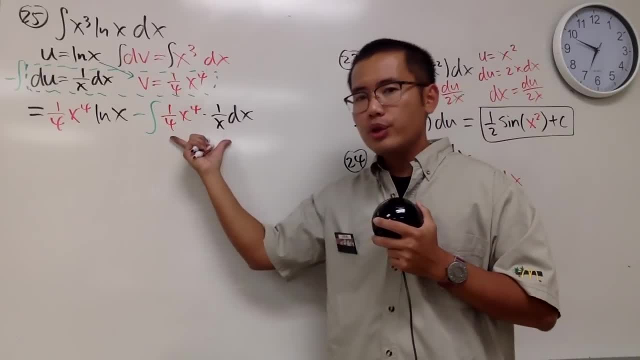 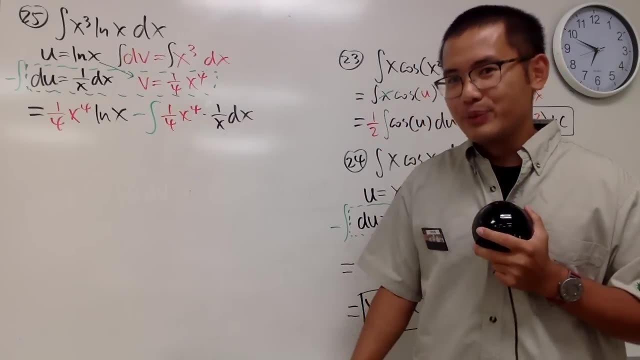 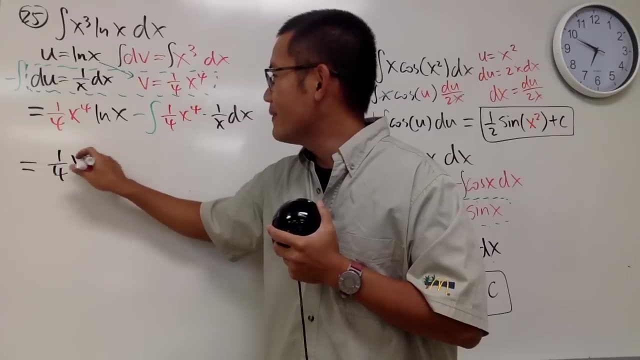 And whenever we're doing integration by parts, pay attention to this integral that we just produced. Can we easily integrate this? In this case? yes, we can, because it's easy. Anyway, this is 1 over 4 x to the fourth power. natural log of x. 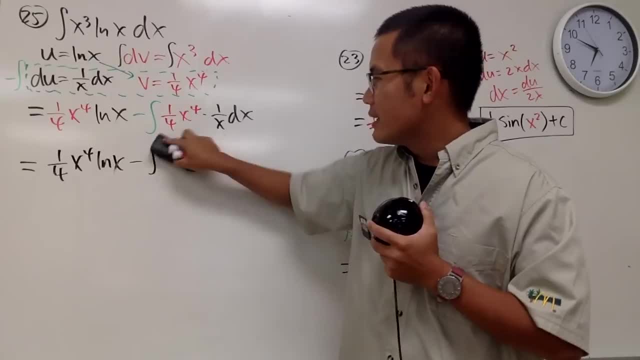 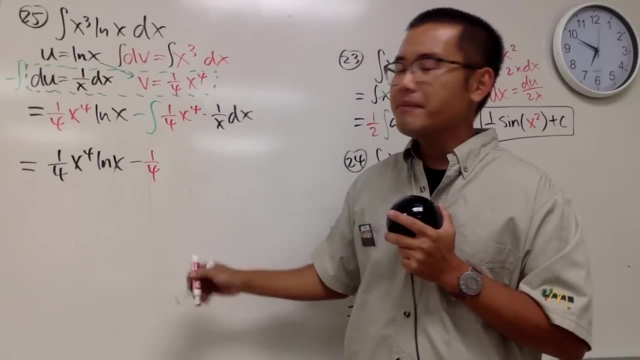 And again, this is still minus integral. but I will do the following for you guys. You see that We have the 1 over 4. Let me take that out to the front of the integration sign, and then the integral, And of course this right here is easy to integrate. 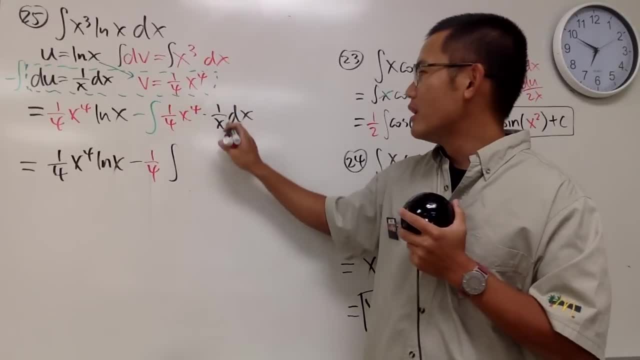 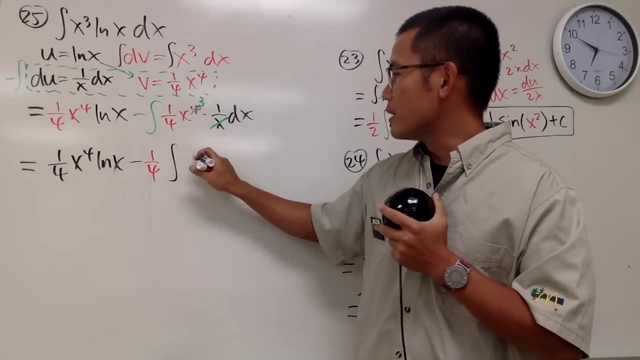 because 1 over x times x, plus fourth power. Of course we can reduce this and this becomes the third power. So here we just have x to the third power, isn't it Like this? And to integrate this we have to use the second category. 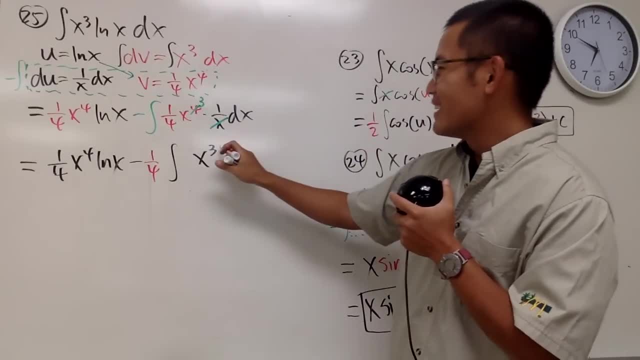 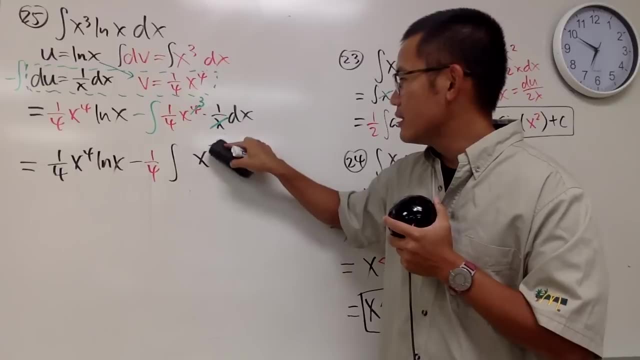 namely the reverse power rule. All right, We are going to add 1 to the power, which is 4, and then divide it by the new power. Actually, let me just do this in green so that it stands out better than that. 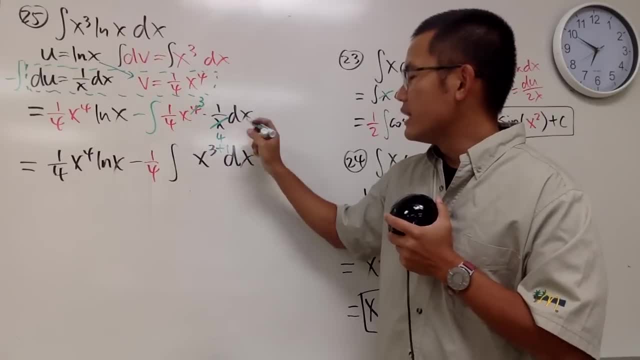 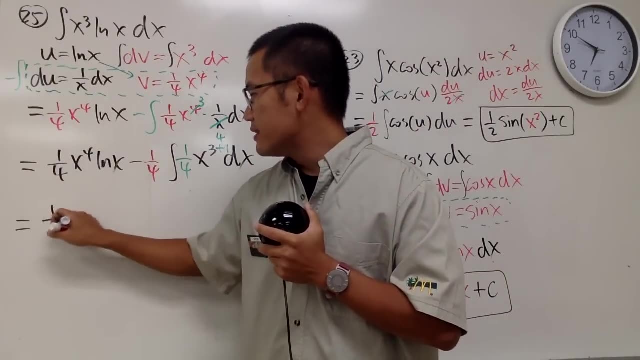 We add 1 to the power, which is 4, and then divide it by the new power, which is 1 over 4. right here Now, all in all, the first part of the answer: 1 over 4. x to the fourth power. natural log of x. 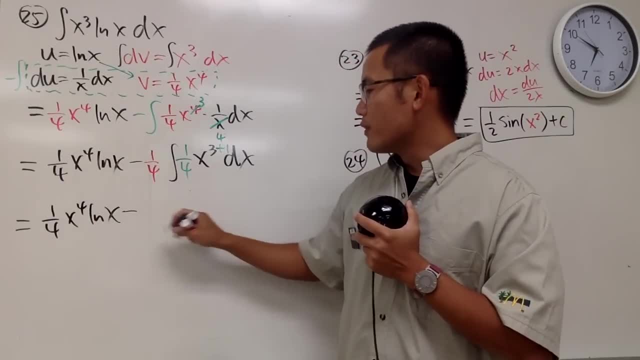 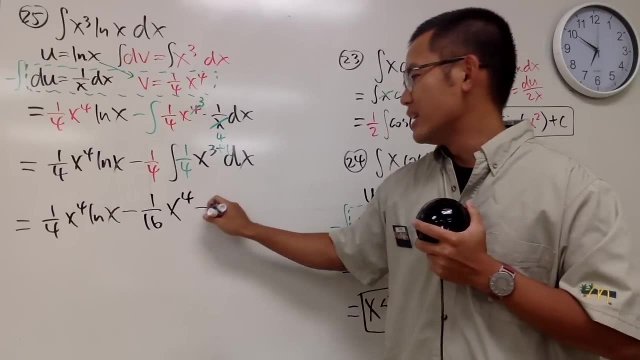 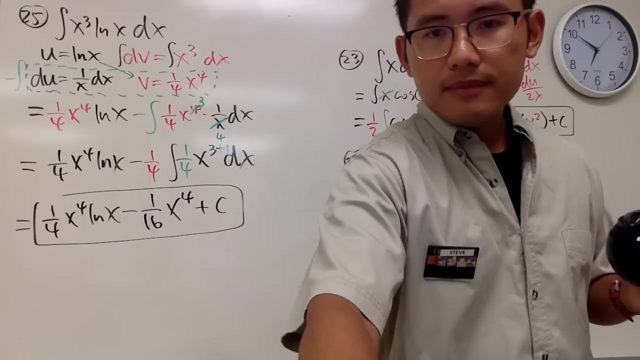 And then minus 1 over 4 times 1 over 4, that's 1 over 16,. x to the fourth power. And yes, this is it Plus C, And we are all done. All right, We are doing well. 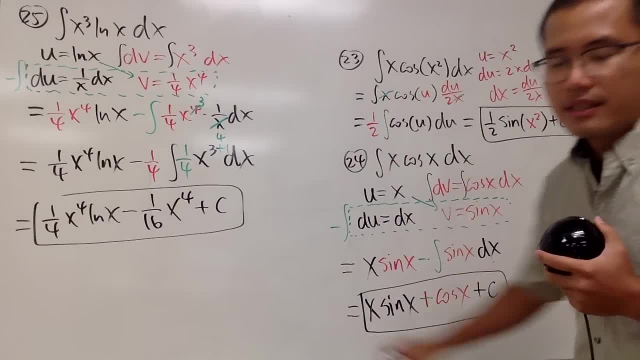 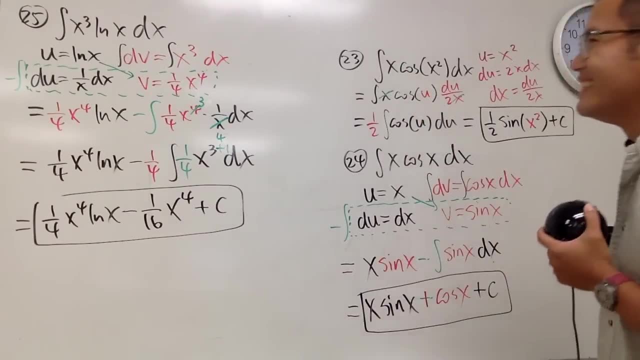 And yeah, So that is it. And let me see how many gigs does this take? 10 gig, OK, So that's the idea. All right, So it's actually not that bad. Again, this might be difficult at the moment. 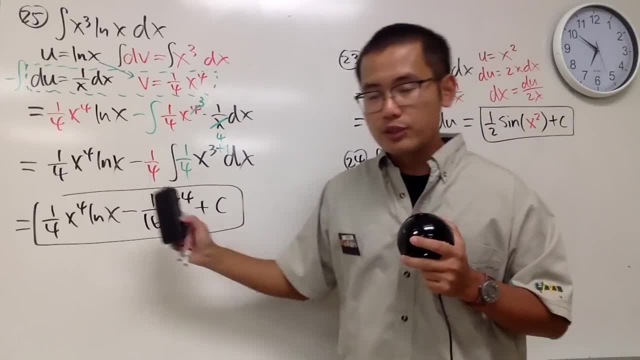 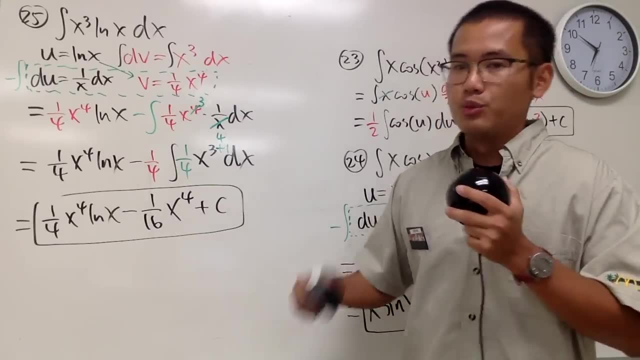 but you just have to practice and try to do this from scratch on your own. If you can do this from scratch, 100% on your own, then you can really feel like you are getting this material All right. Now let's do question number 22.. 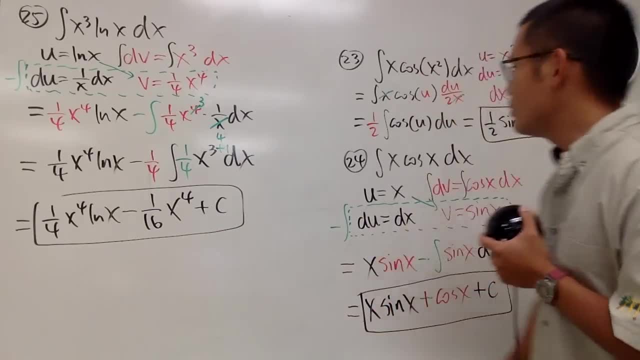 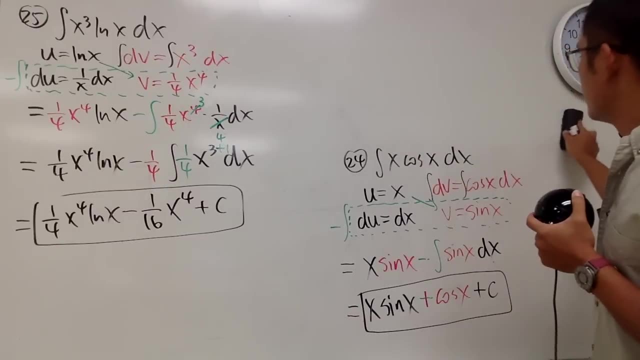 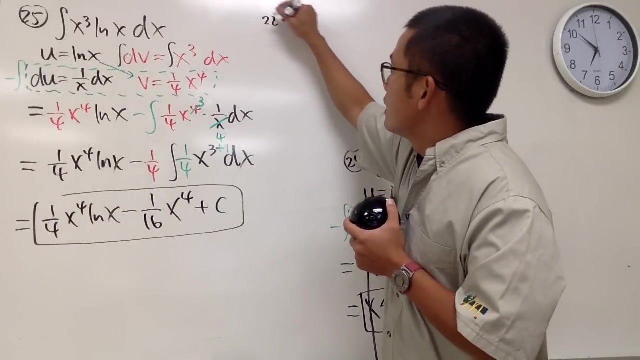 Man, this is 25.. But we are going to go back to 22.. I will tell you just why I'm going to keep this right here. I will put down question number 22 right here, Yeah, And I'll put down star next to it. 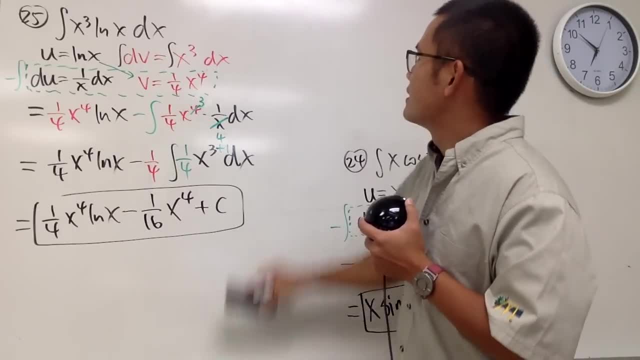 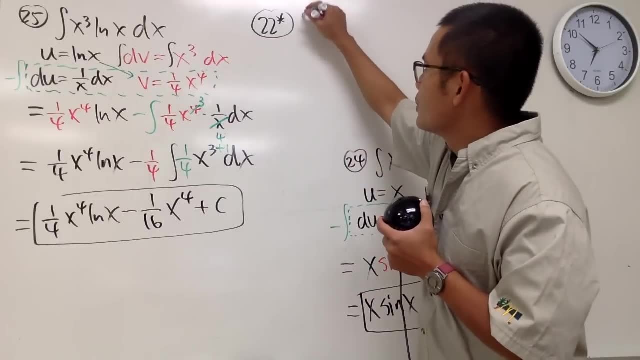 Yeah, This is 22 star. Doesn't look nice, Let me do it again, 22.. 22 with a star next to it, Like that. And if you guys look back to question number 22,, it's the integral of x squared times sin, x, dx. 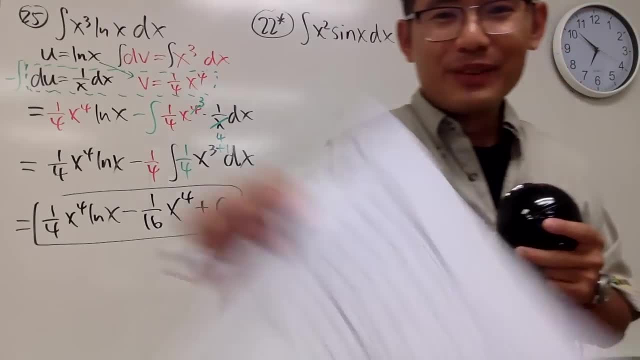 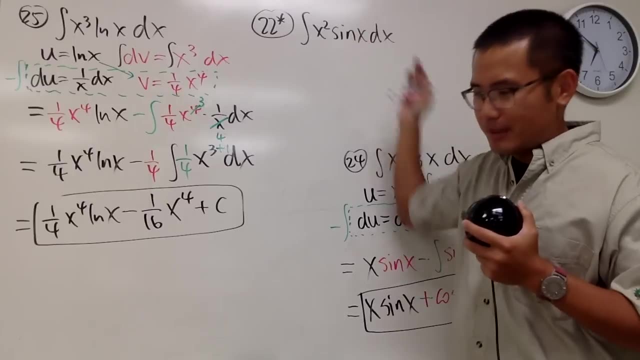 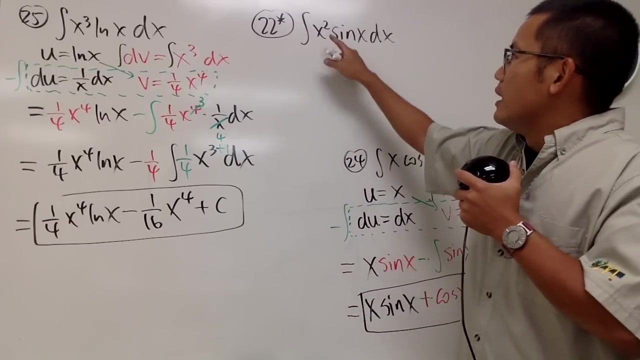 Yep, This question that we had right here earlier, right? So I'm not just going to integrate the first and then integrate the second and put them together, No, But in this case we can actually integrate this by parts. It would be much easier. 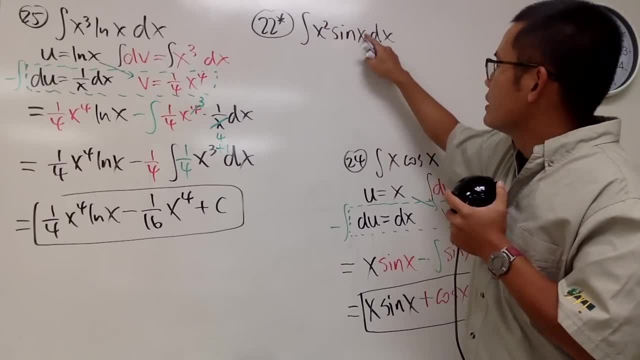 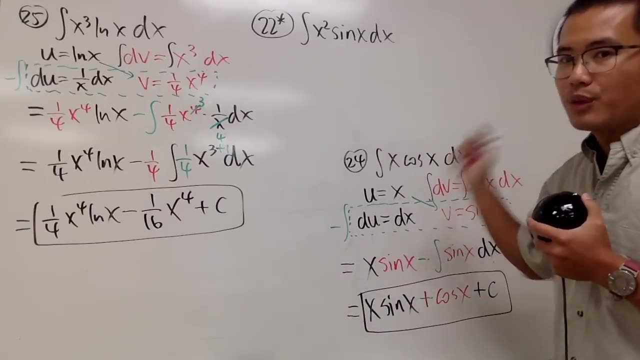 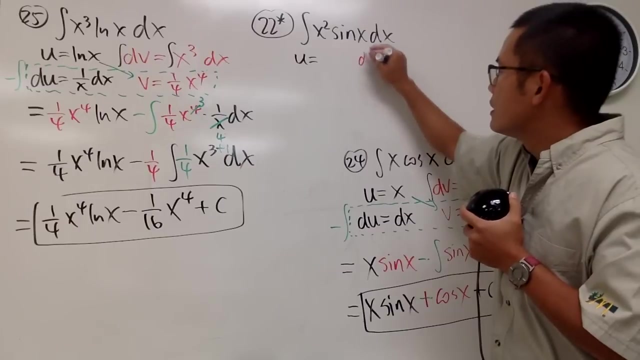 if we don't have the square here, But if the square is inside sin square, That would be question number 23.. Idea, But here we have this, So just deal with it. Okay, So let's make our selection: u and dv. 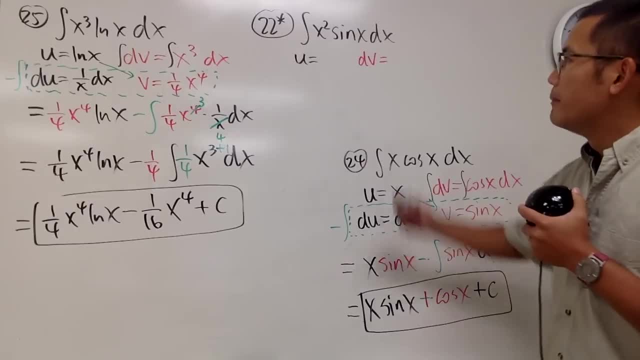 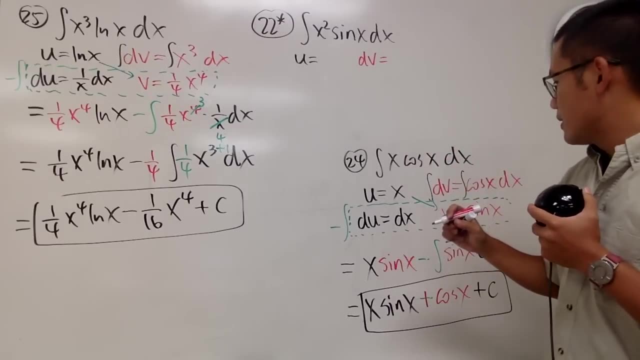 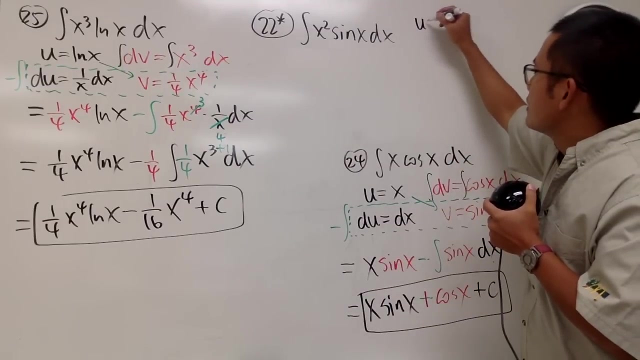 u and dv. Well, I'm going to differentiate the x squared and I'll integrate this, because we can totally do that And actually to save space, I have to put this on the side, Sorry. All right, I'm going to put down u and dv right here. 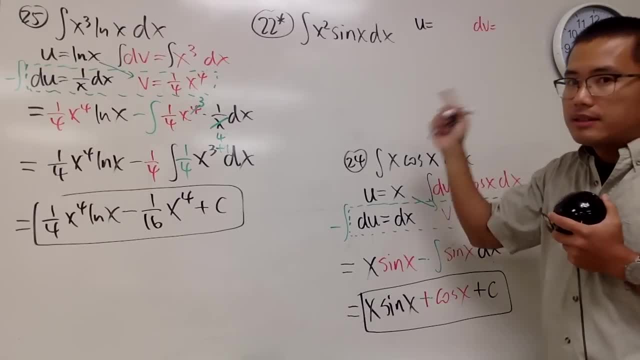 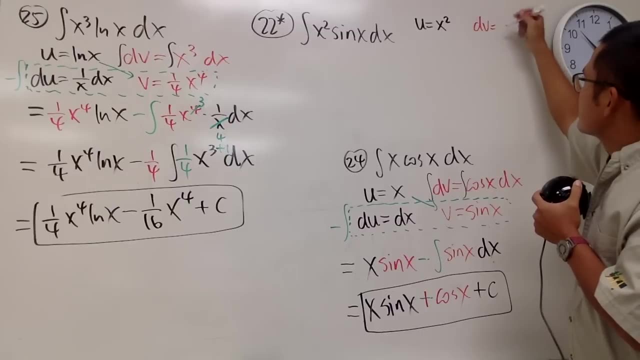 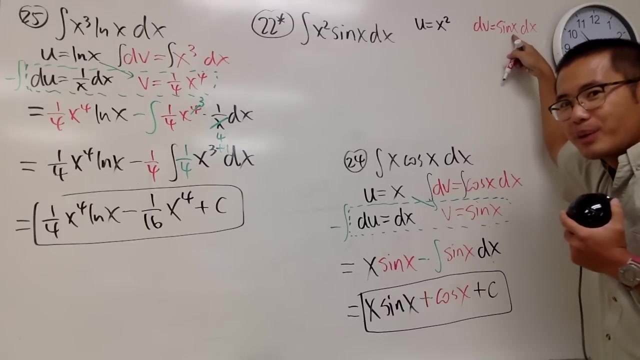 u and dv. This time we are going to make our u to be x squared and the dv to be sin x dx. And again, the reason I'm choosing this is because we can totally integrate this without trouble And of course, we can also differentiate this. 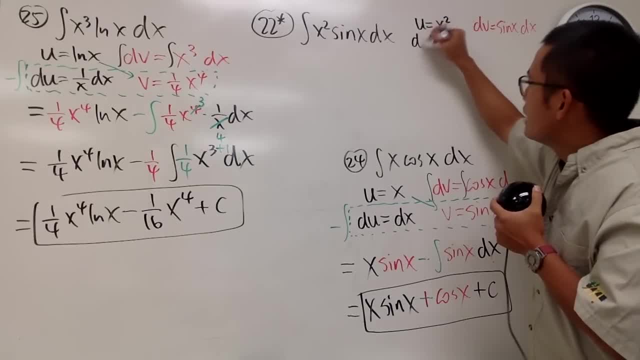 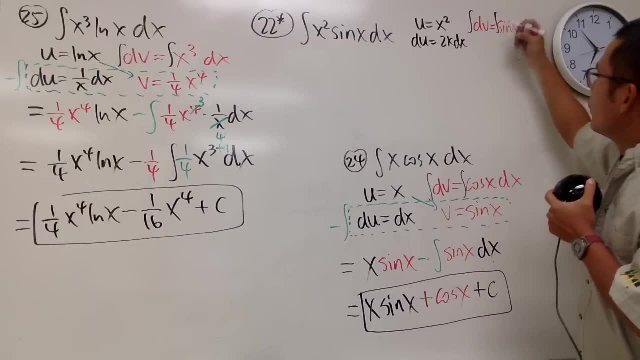 Right, So let's go ahead and make that happen. You see that we have du, which is going to be 2x dx, And integrate both sides right here we can get the v And the derivative. sorry, the integral of sin x is negative cos x. 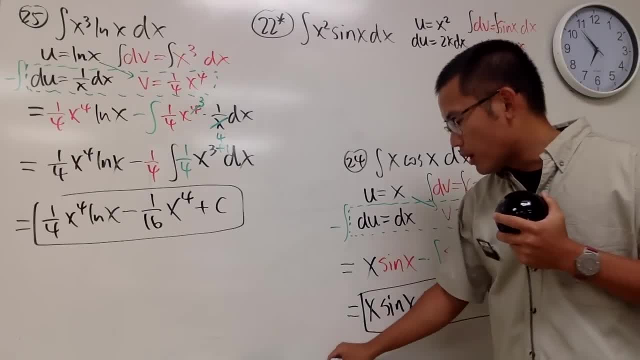 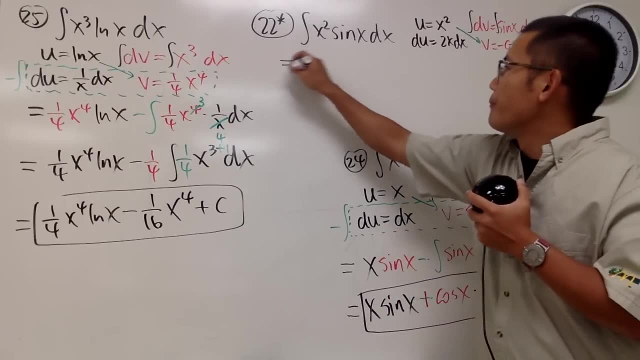 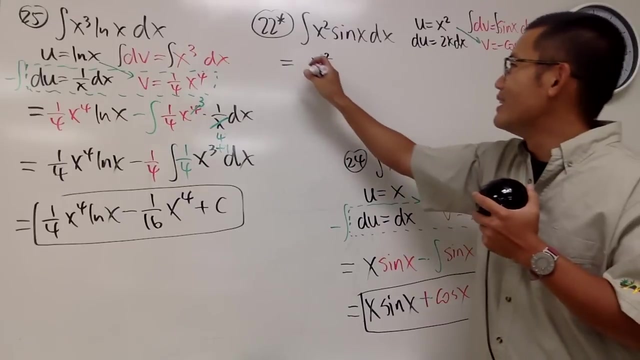 Like that. And now let's put down the first part of the answer. We do this times that And we have the following Here. we go This times that we have x squared times, negative cos. So I will just put down negative cos, x right here. 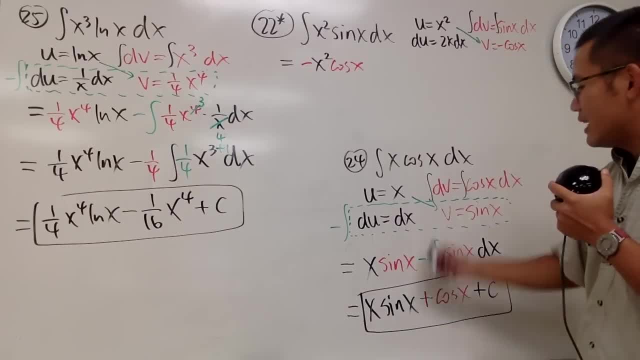 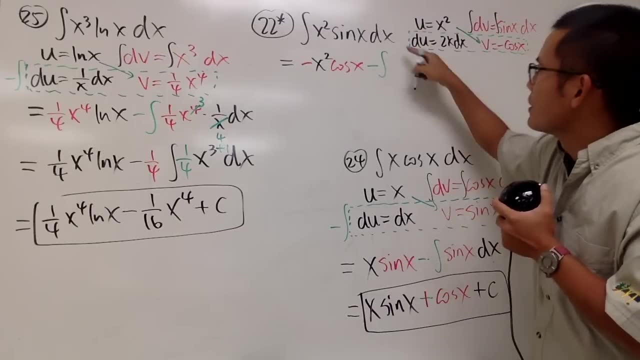 Yeah, And then I'm going to have to multiply this row And keep in mind we still have to have the minus integral, Right? So minus integral this times, that, And for the inside, here we have the 2x. 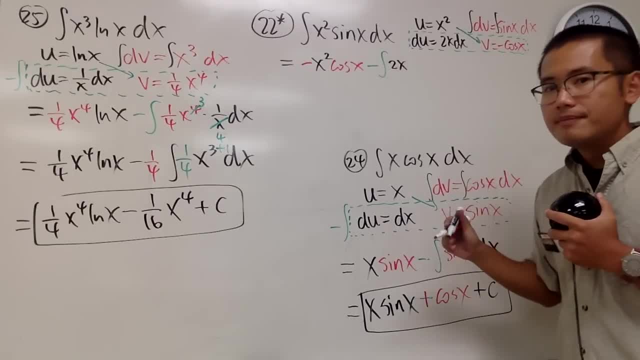 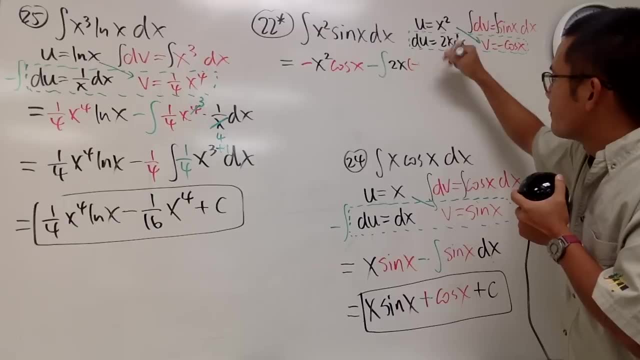 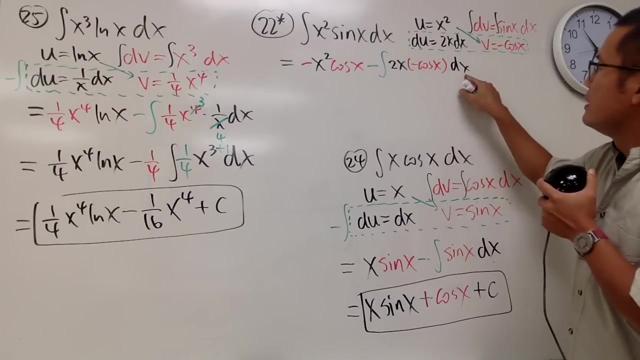 Let me just put it inside right here: 2x And we have the negative cos. so I will put down negative cos right here And of course we still have the dx. So notice, this is the du part. This part in black is the du part. 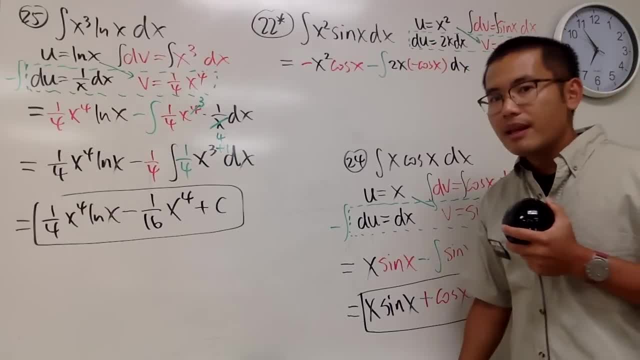 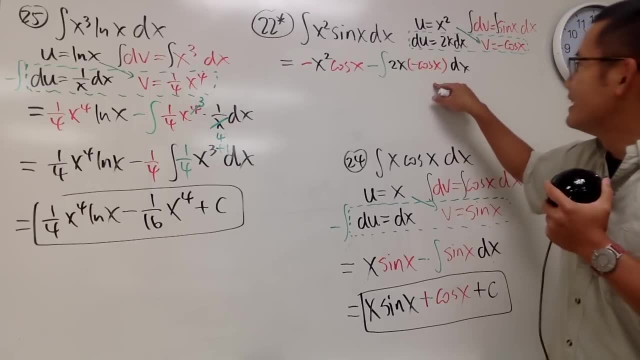 And this right here is the phi part. Okay, Just like that. Now, this is pretty much it, But notice we still have the integral And if you clean things up, this is going to be the following: This is equal to negative x squared. 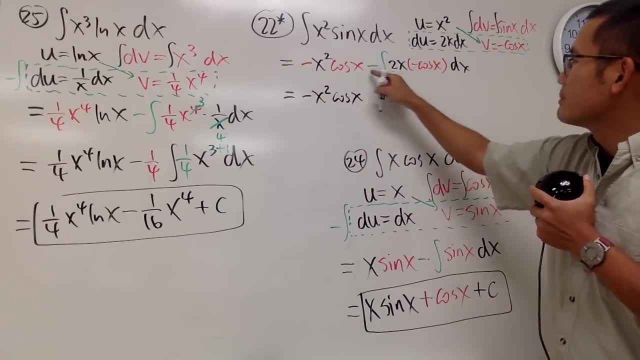 cos x. And then, okay, minus, minus becomes plus, and put the 2 in the front. We have the 2 in the front, And here we have the integral right here, and this is just x. now and then. 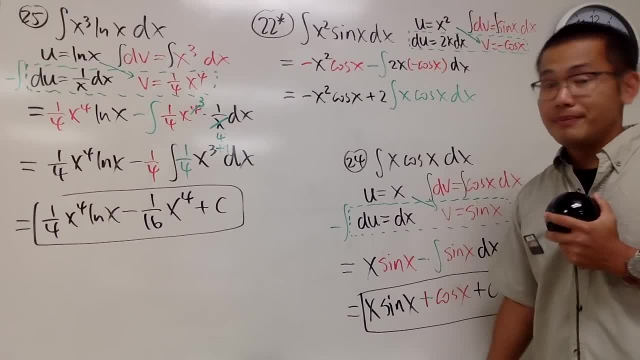 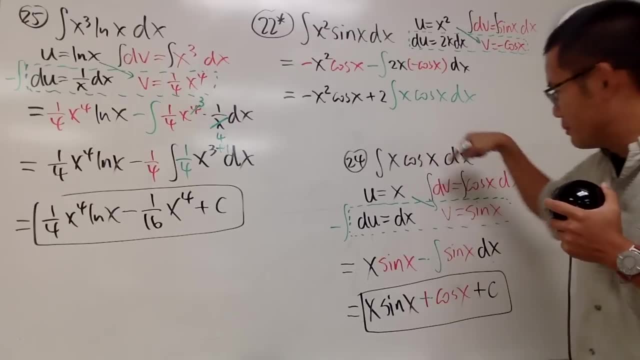 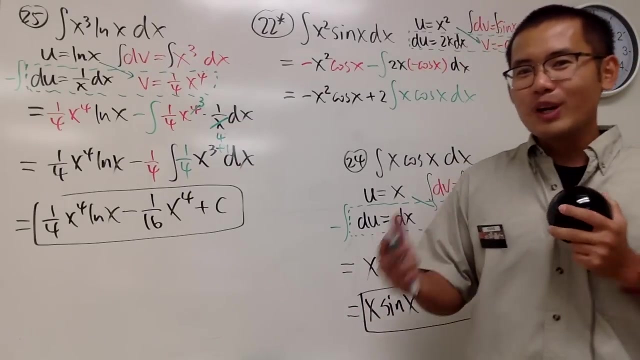 cos, x, dx, Isn't it? Yeah, How would you integrate this Integration by parts again? Yeah, So the problem is that sometimes we have to do integration by parts more than one time, And of course we can just enter this right here, because 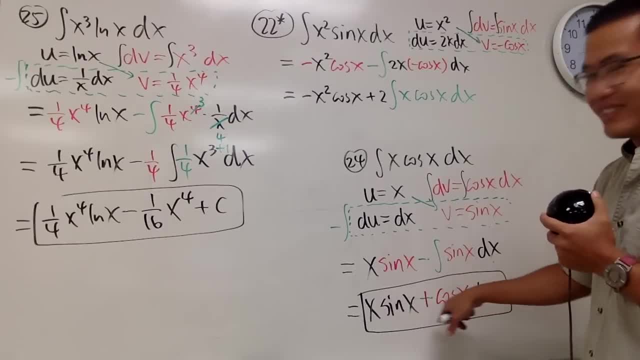 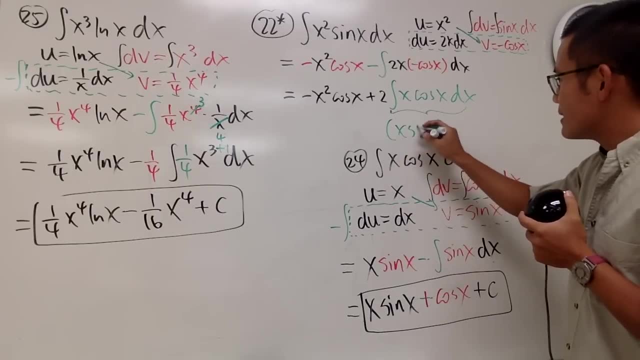 you see, that's what I do, that's what I did, right? I set up all this so that I can just use the answer from here. The answer to this is, of course, that I'll just tell you guys: All this is x times sin, x plus cos x. 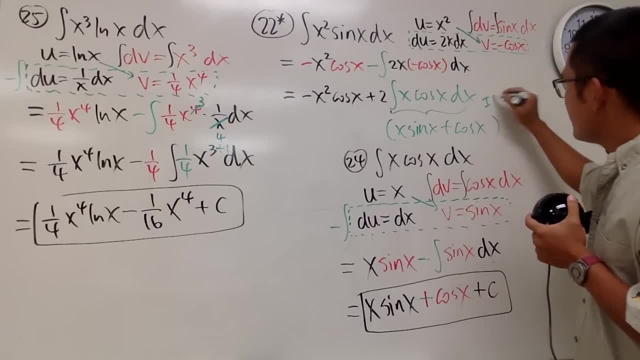 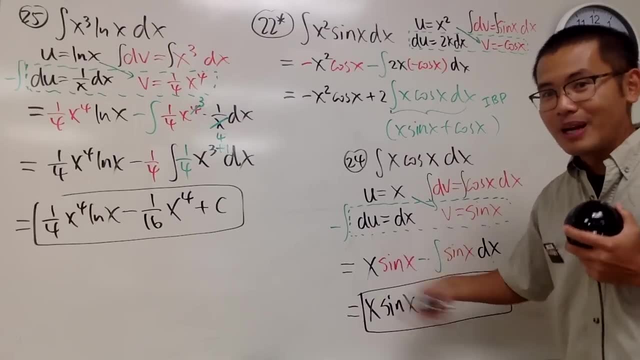 Yeah, And again this right here: we need another integration by parts, And we, if we didn't do this earlier, we would just have to do this on the side right, Just so that we can get the answer for that part. 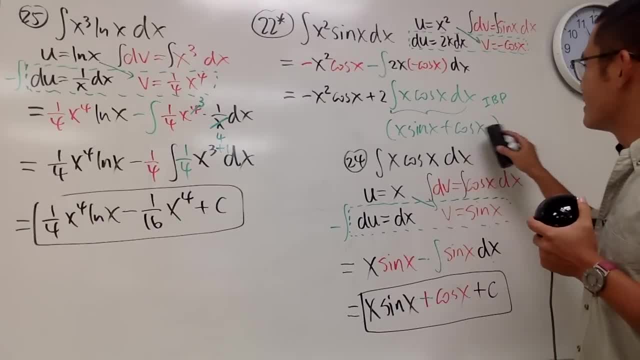 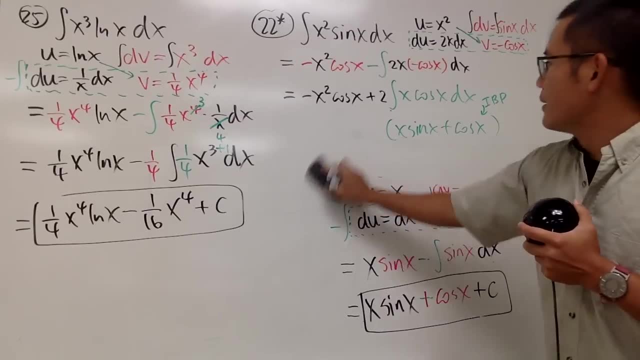 So that's pretty much the idea. Now I can erase this, because I put down the answer already, And let me just put this down: Integration. we'll probably get that, Yeah, Okay, And then we are just going to put down the other parts. 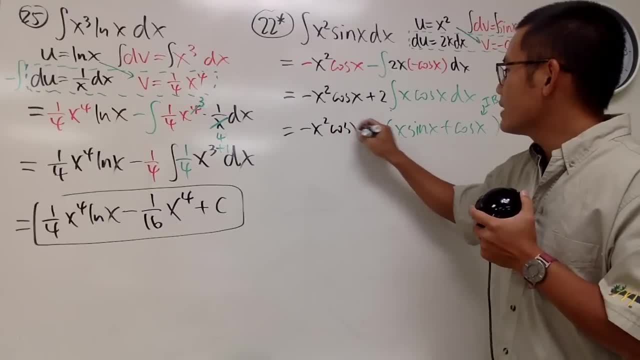 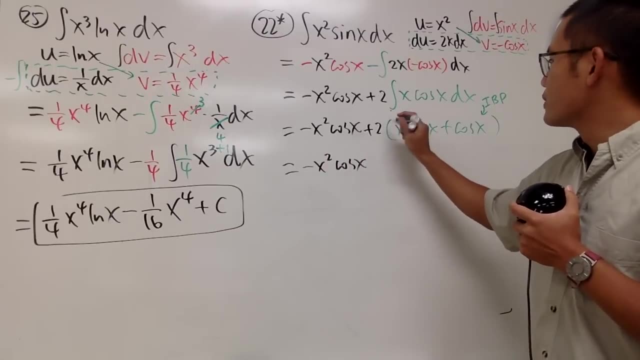 So this is equal to negative x squared cos x plus 2 times all that And in the end, of course, this is negative x squared cos x. And of course we can distribute, distribute, And this is plus 2x sin x. 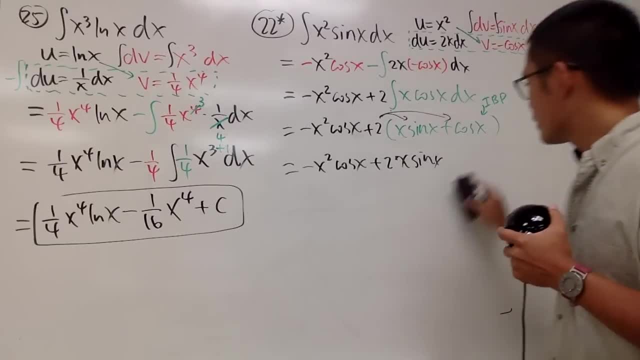 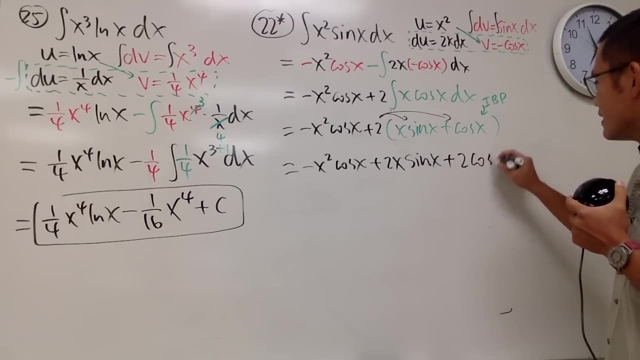 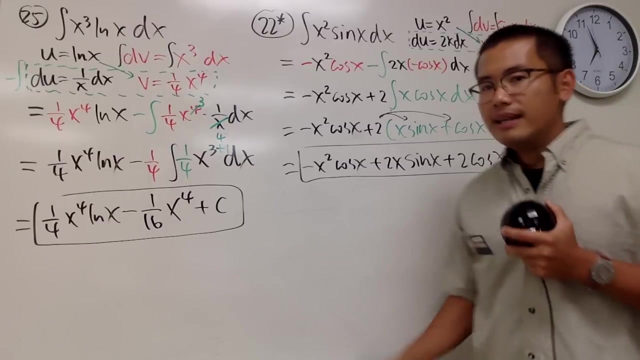 And then plus 2, cos x, All that good stuff. So that's pretty much the idea. And again, the annoying part is sometimes we may have to do integration by parts more than one time. So that's it. 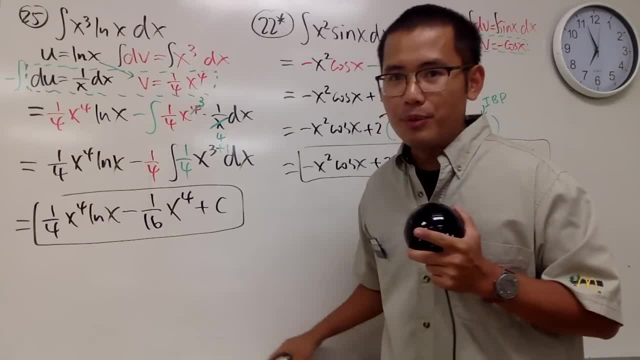 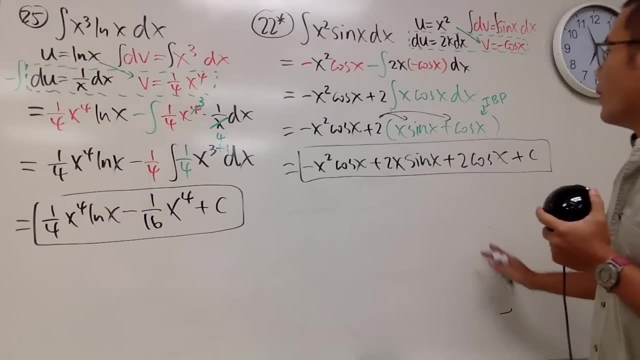 Just like this, But I know some of you guys might have watched my video before already. Yes, I'm about to show you guys that, And I'm also going to show you guys why that method work. Well, here is the deal. 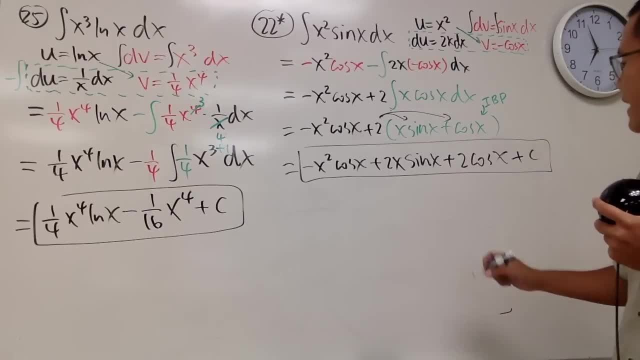 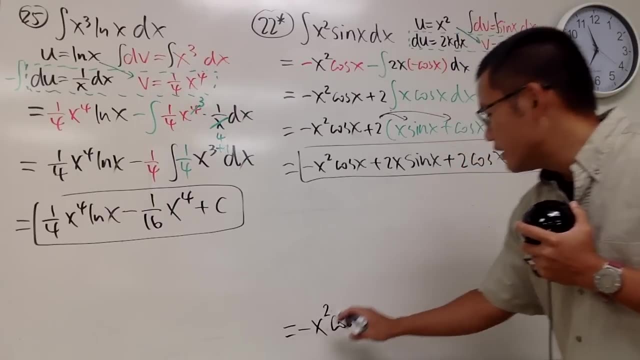 Hopefully we can all agree that this is the answer And, in fact, let me actually just write down the final answer right here so that I will prove to you guys this is actually correct. right, So we have negative x squared. 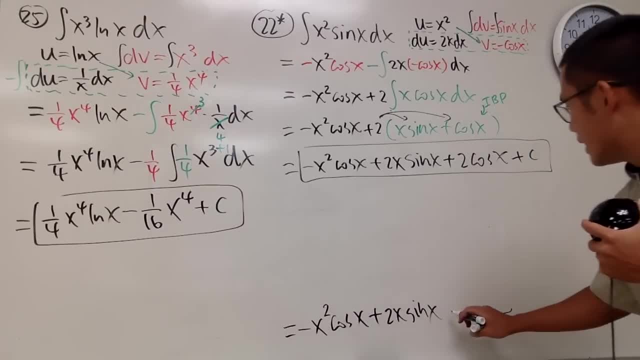 cos x plus 2x, sin x plus 2. cos x Plus c. So this right here is the final answer that I think we can all agree on. Now I'm actually going to go back here and then I'm going to do some. 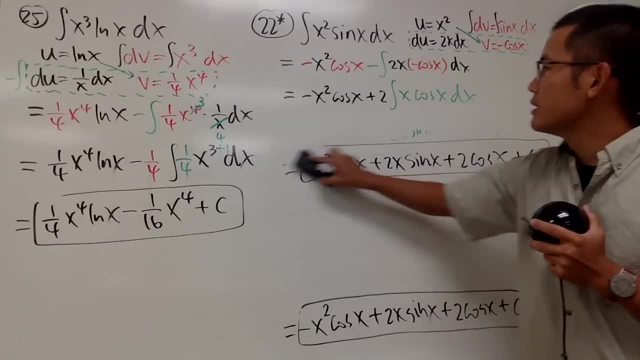 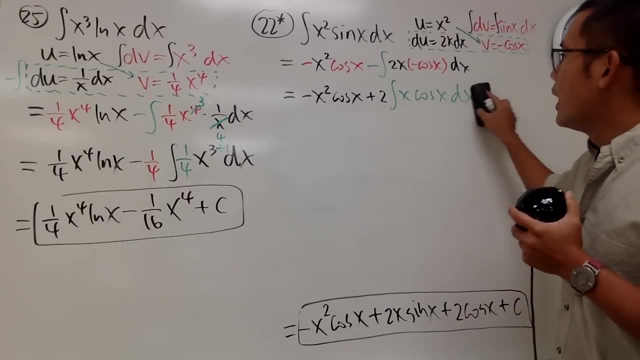 like maybe extra work for a good purpose. You will see, Earlier, that's the point that I want to just do that for you. But now I want to actually erase this part as well. I'm going to redo this from a different approach. 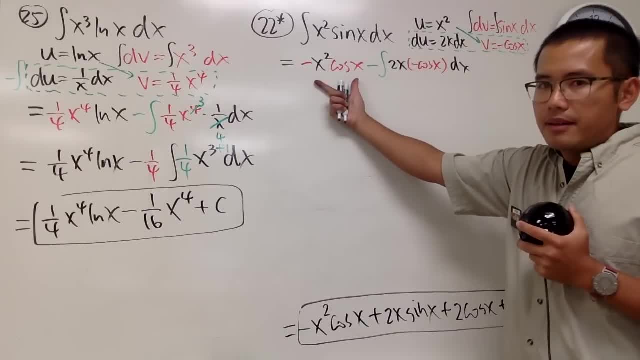 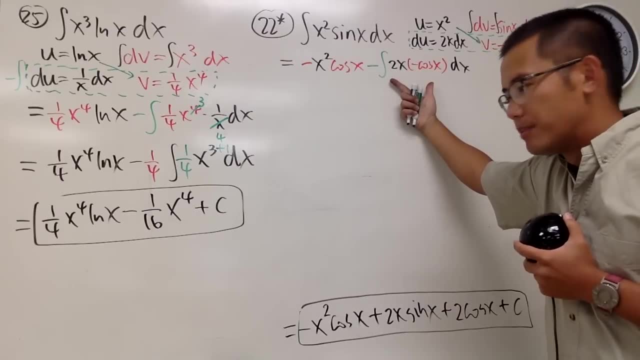 Okay, here we go. This is done. That's the first part of the answer. This part I still have to integrate by part, because I showed you guys that earlier And suppose we don't have that Now. we just have to do the following. 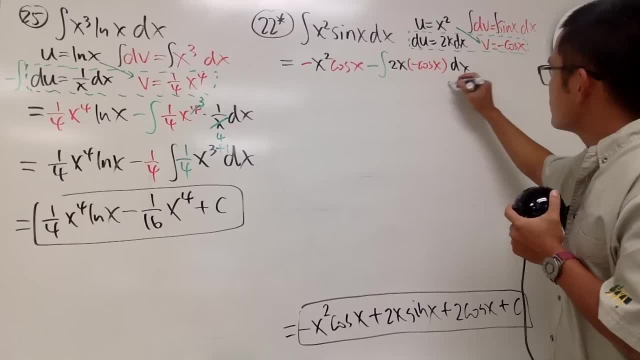 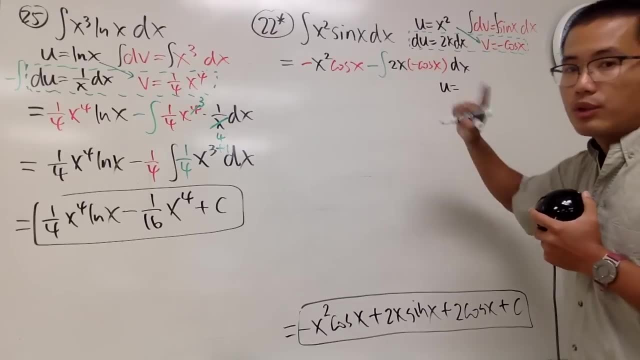 Right here I will just put down u and dv again. So I will just put this down. Let me just put down: okay, here we have the u, which is I'm going to select 2x to be the u. 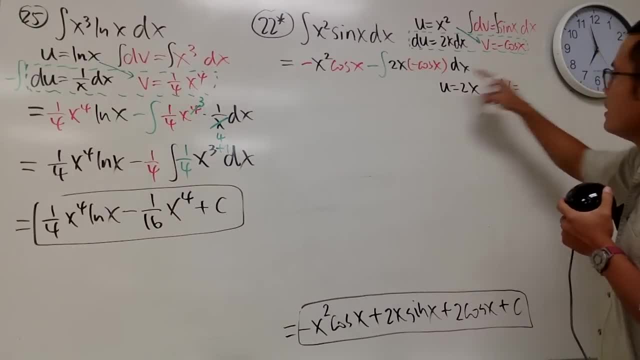 And I will put down dv to be negative. cos, x, dx. I know you guys are wondering why I want to do, why I'm doing this, but I will explain Again. go through the usual thing. du is equal to just a 2 now. 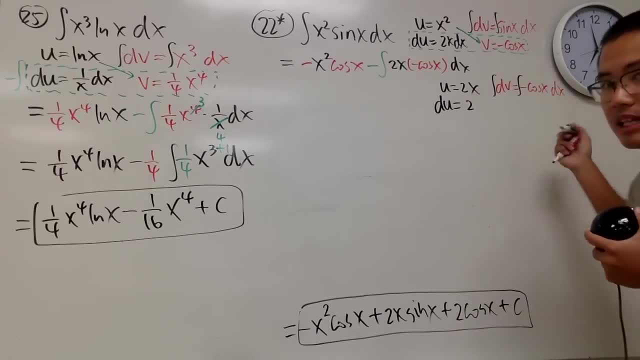 And then integrate. integrate and integral of negative cosine will give us negative sine. So this is v equals negative sine x. And yeah, this times this and then multiply this row so we can get another integral, Alright. 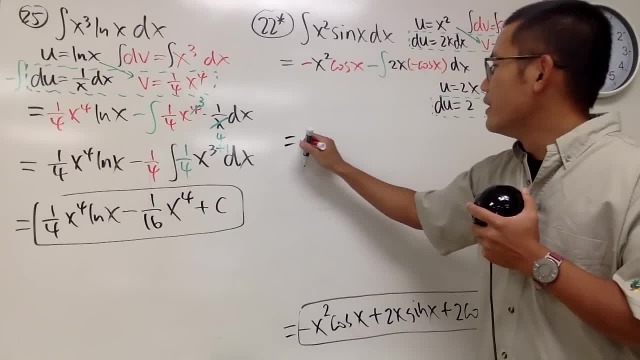 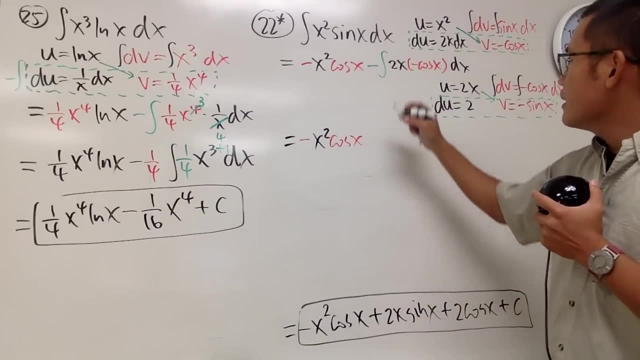 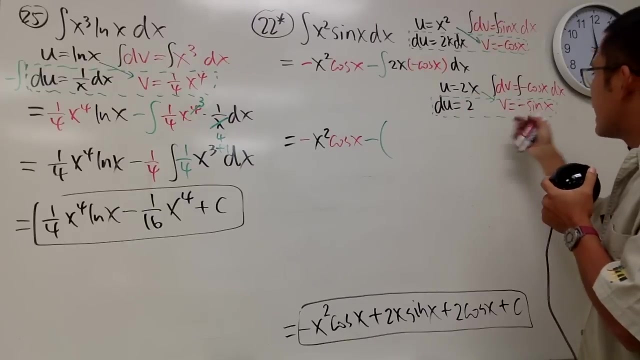 let's see Here we have all the way in the front negative x squared cosine x minus, and I'm just going to open the parentheses Because when we do this we can produce the answer right- And 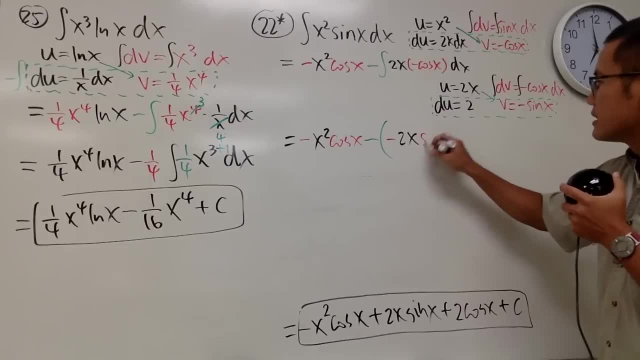 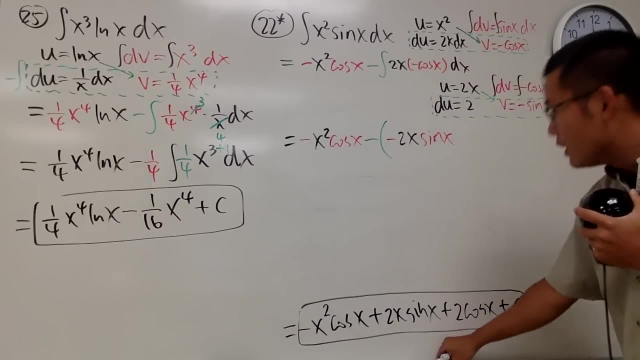 the first part is 2x times that. So we have the 2x right here And then the negative sine x Right 2x negative sine x. That's the first part of the answer for this integral And. 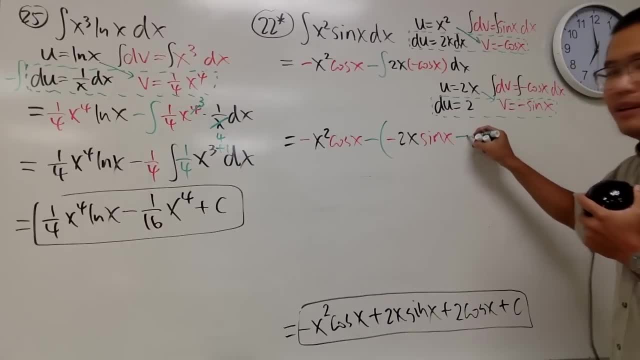 remember, when we multiply this we have another minus integral, So minus integral, And inside here we have 2 times that. So let me just put down 2 times negative sine x Like this: dx- Oops, I forgot the little dx. 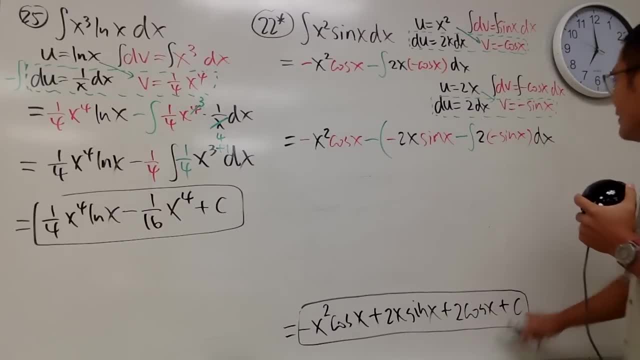 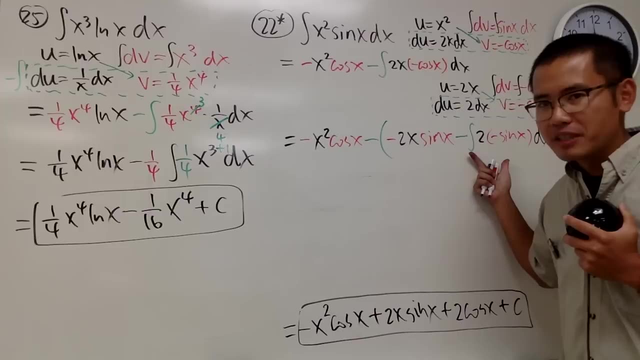 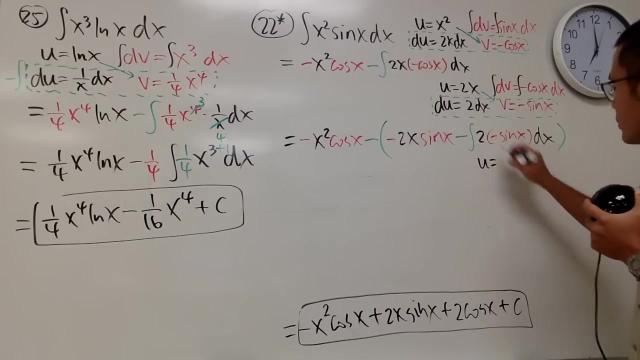 So 2 dx Like that. Well, this is the integral that we can actually just integrate, But I would like to do the integration of parts again, So just be a little bit patient. okay, Right here let me just put down: u equals 2.. 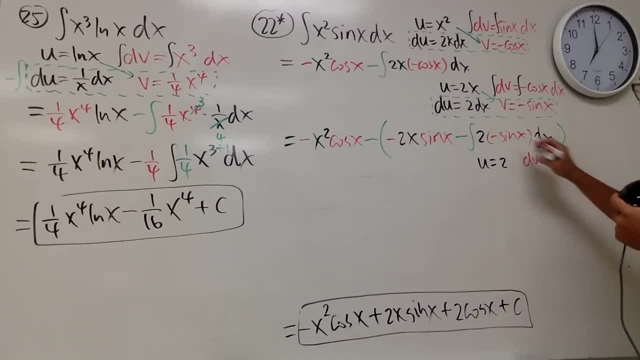 And I will pick. dv equals negative sine x. And whenever you have dv, don't forget the dx. Now I can differentiate this: du is equal to 0. v. right here, the derivative of cosine will give us negative sine. 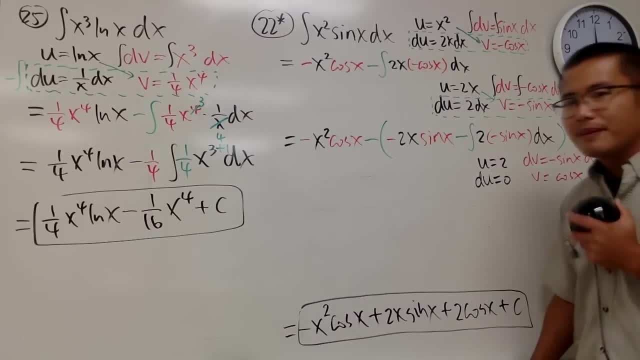 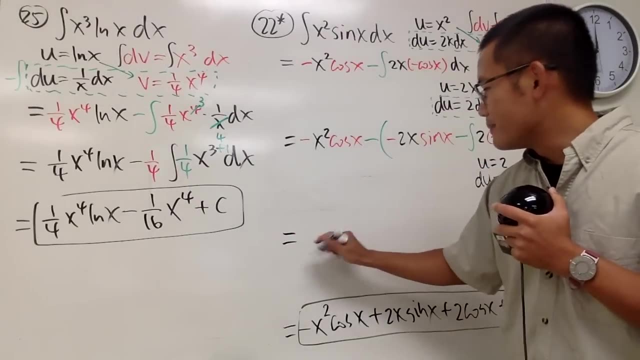 So this is it Right. So v is positive cosine From here. this is the answer, But let me put this down, okay. So, all in all, let me write it down: Negative x, squared, We have cosine x. 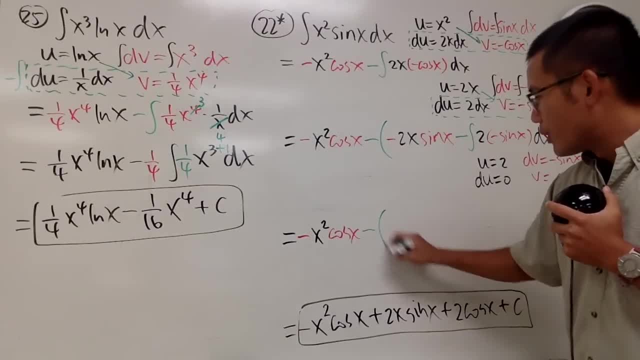 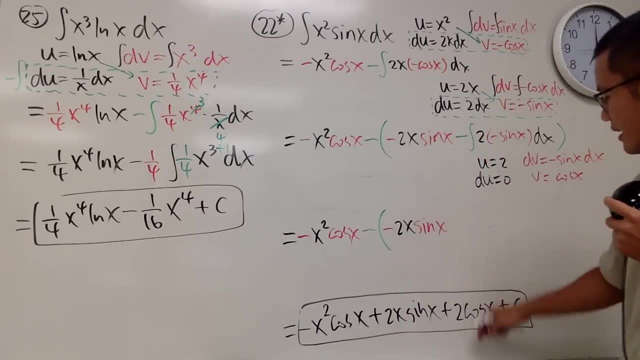 And then this is minus parentheses. And then we have over this part And this is still the same thing from earlier. And then here we have this minus And notice that integral will just open the parentheses And 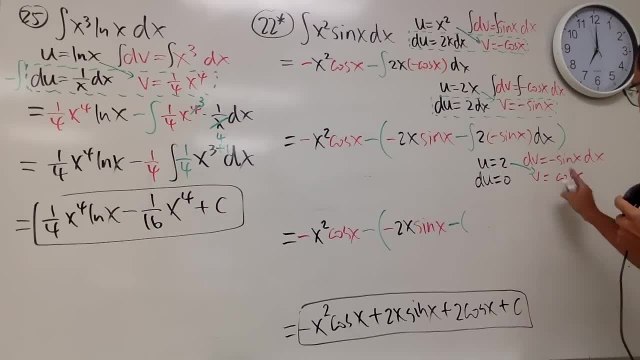 we do this times that, Namely 2 times cosine x, And that's the first part of the answer for this integral. So 2 times cosine x here And in the end, this times that is just 0.. 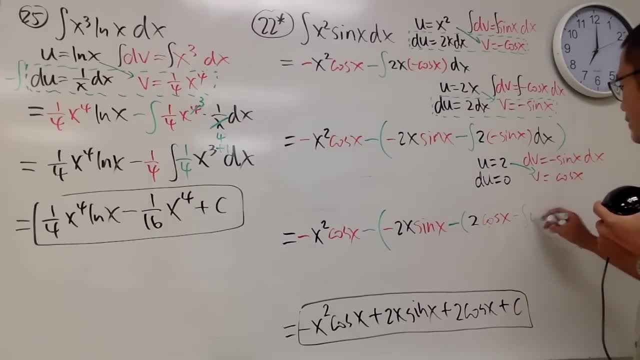 So you just pretty much. if you want, it's a minus integral of 0. But it doesn't really matter anymore. This part doesn't matter anymore. Integral 0 just gives you a constant. So it doesn't matter anymore. 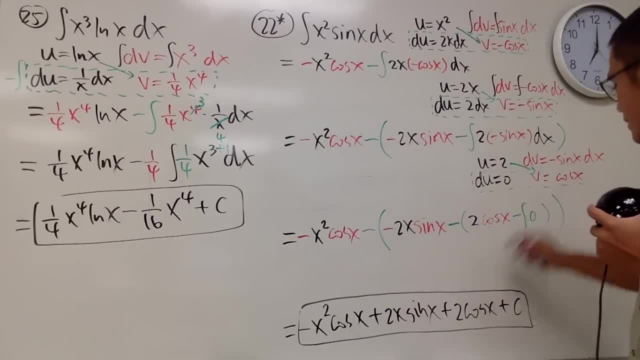 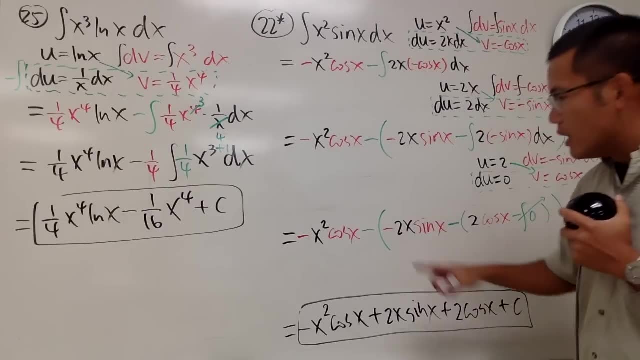 Right In the end. this right here. just don't worry about it. This is going to give you the constant Right. Integral 0 is a constant, So again, don't worry about it. Focus on the function part. 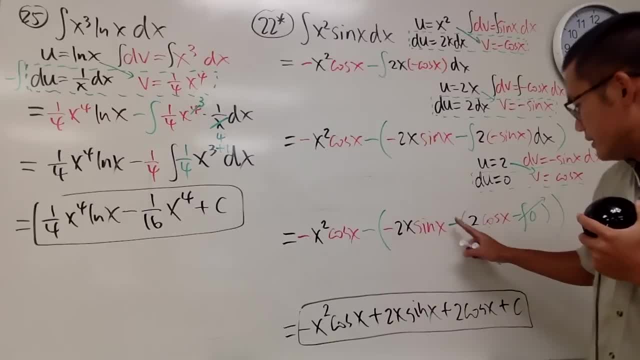 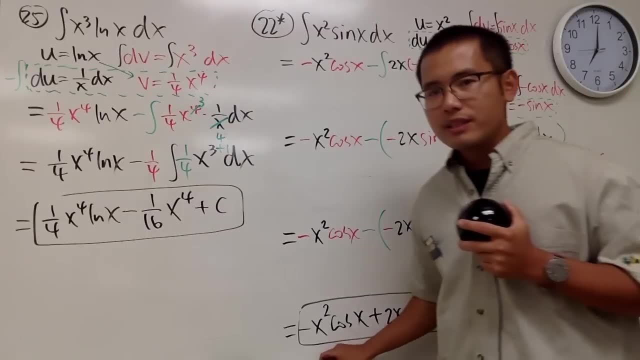 This is the same as that Negative negative. is this Negative negative? I still get that. Hold on. So this is how it works, But now, of course, it's taking a while. It's 7 pm already. 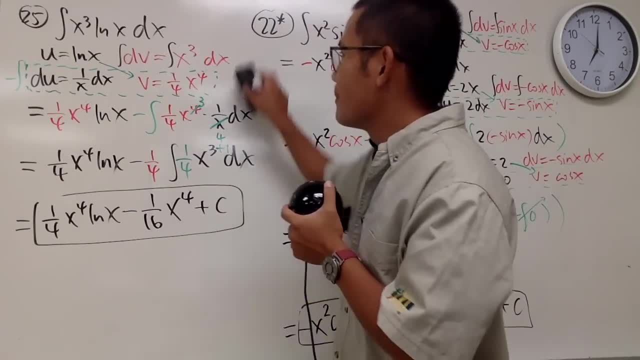 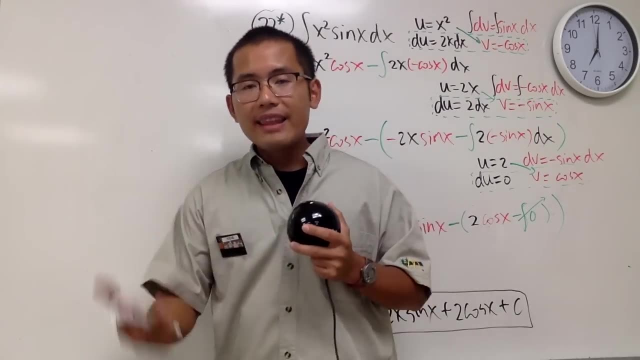 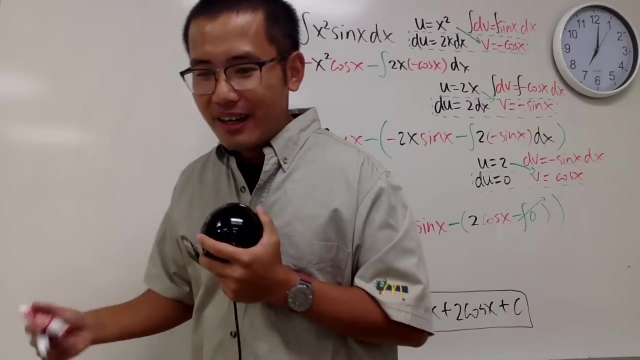 Man, if I do this like 10 more times, that's no good. So I would like to show you guys another way to formulate the, the, the, the integration by parts, Right? So again, number 22,. 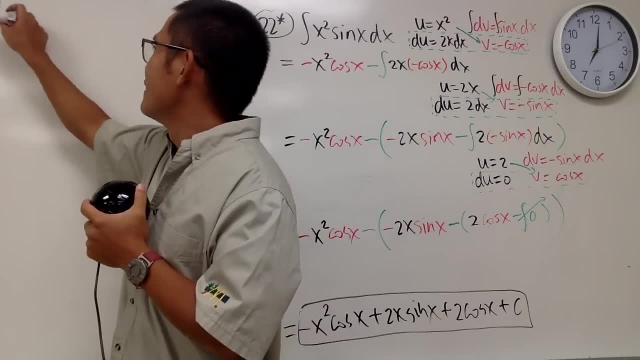 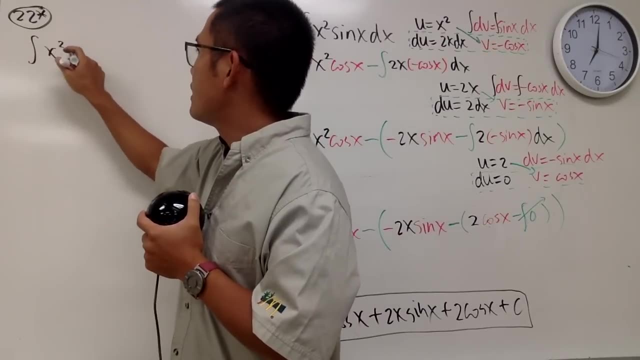 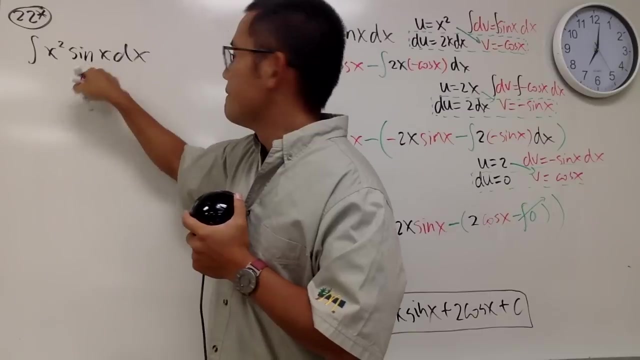 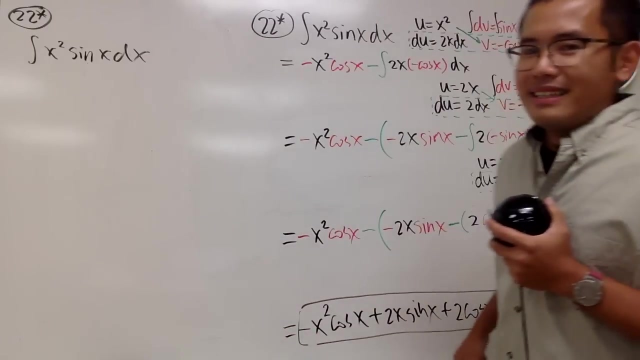 one more time. This is how I explain the following method. Okay, Here is the DO. If I'm integrating x squared sine, x dx. Okay, This is the most exciting part for now. Right, So far up to now. 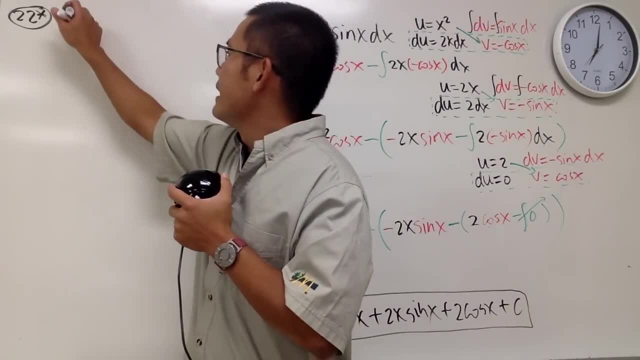 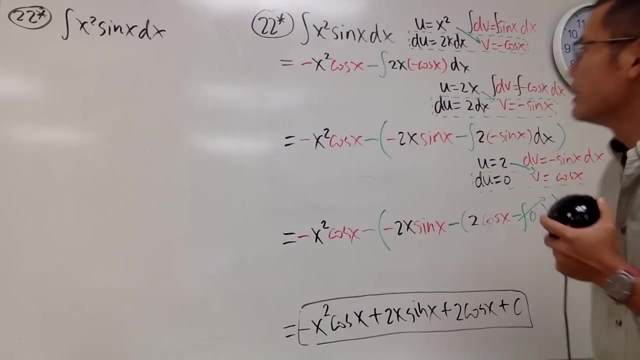 I will put this down right here. Yeah, Integral x squared sine x dx. All right, This is the most exciting part up to this point. Focus on the following: Look, Earlier u is 2x And then you see that du is equal to 2,. 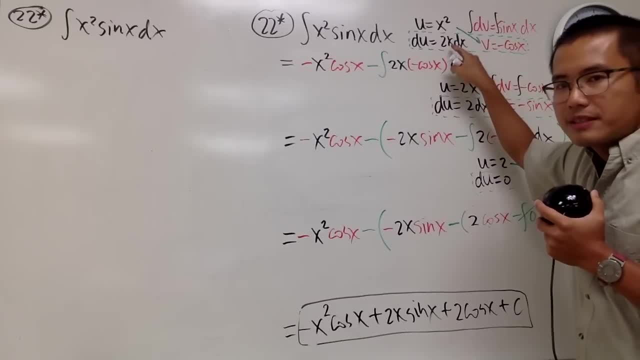 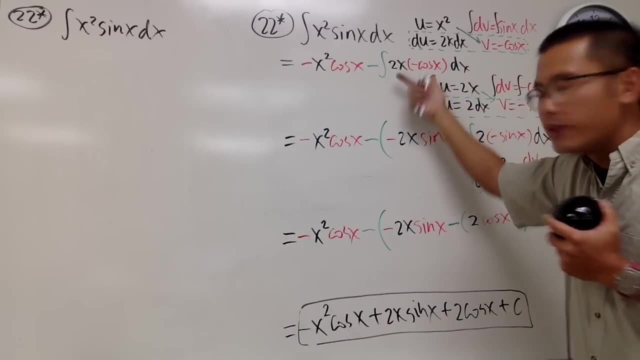 sorry, u is x squared, And then du is equal to 2x, And then I just put another u to be 2x because I have to do the integration by parts again Here. right, u is equal to 2x. 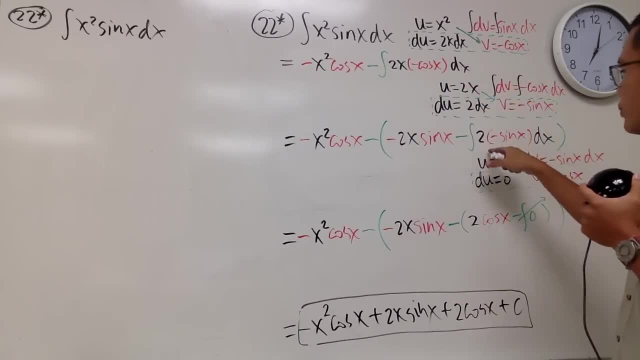 And then I differentiate it, And then I differentiate the 2 again. Notice, this format is just not ideal because we wrote down this twice. Likewise, we wrote down this twice. Why don't we just like continue? Why don't we just continue? 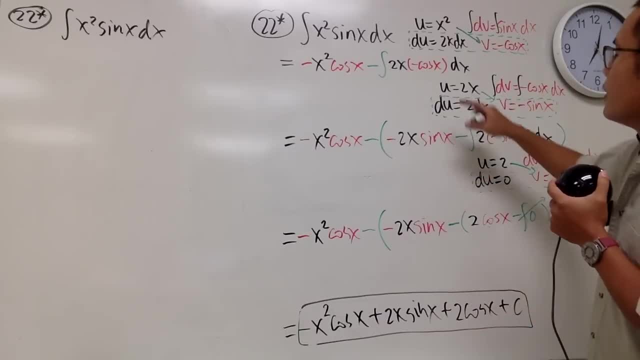 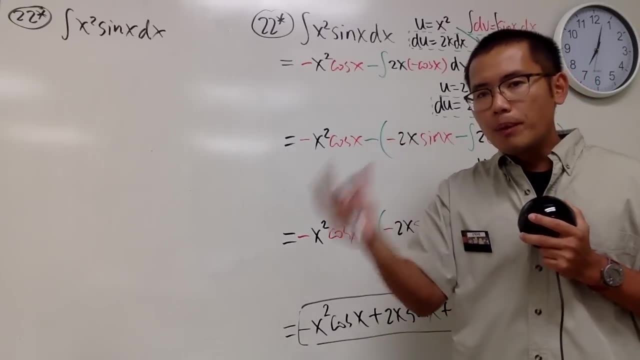 with the same fashion. right, And here's the deal. Whenever you are doing an integral, as long as it needs integration by parts, the idea is that you are going to pick one part to be differentiated and the other part to be integrated. 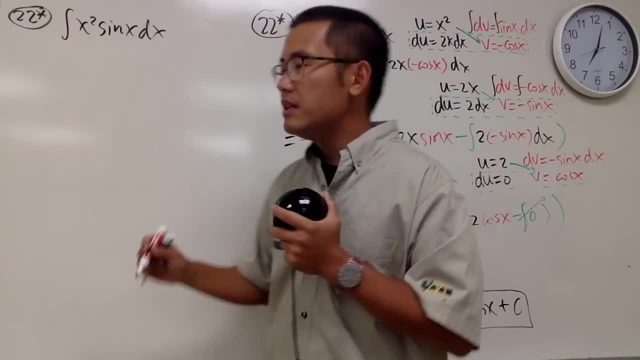 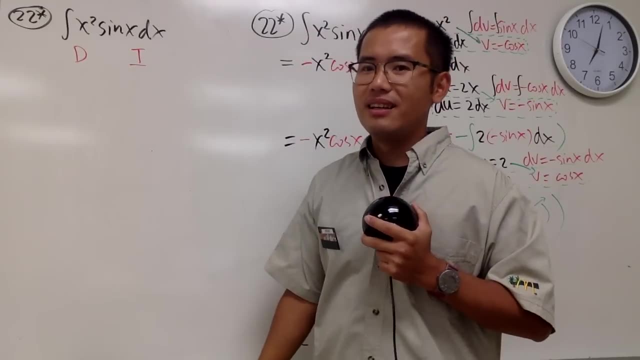 That's the idea. Keep that in mind. All we need is one part to be differentiated and the other part to be integrated. That's the idea. So let me put this down for you guys. Earlier, our choice was: x squared to be differentiated. 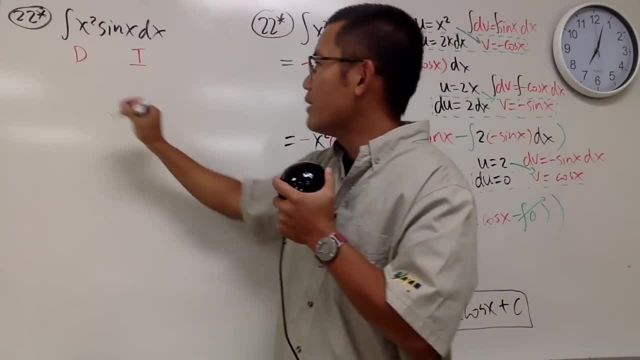 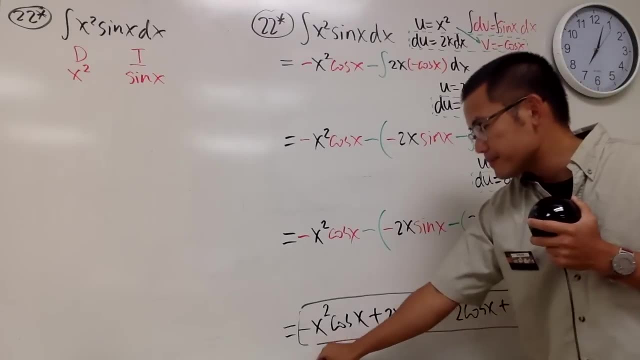 and sine x to be integrated. So I'll put this down: We are going to differentiate x squared and we are going to integrate sine x. And don't forget that originally we have this times that as the original integral, And then 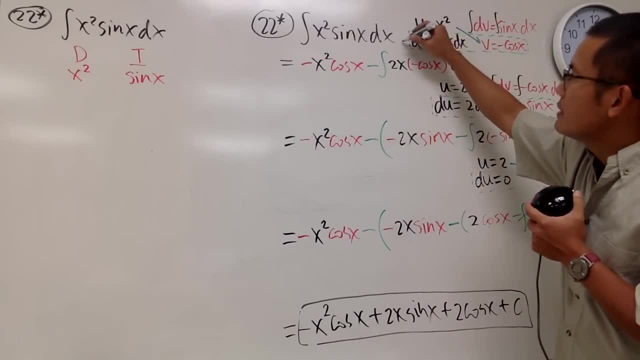 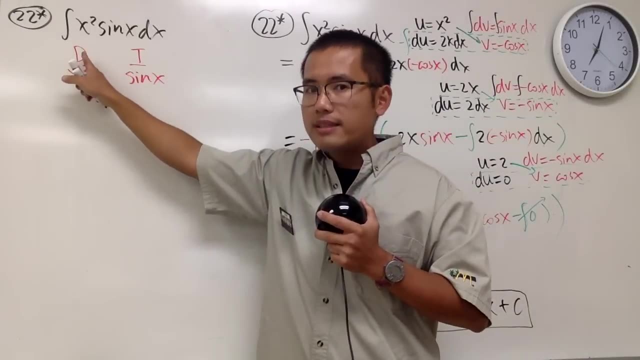 when we do this times that we have a minus integral Right. This is a minus integral. That's why I put it on right here Now. this is what we are going to do: Always set up d and an i and, on the side, 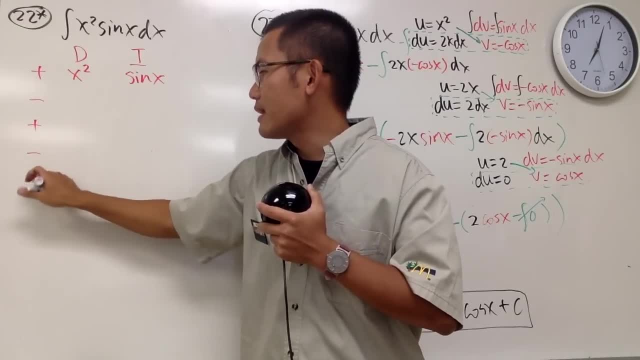 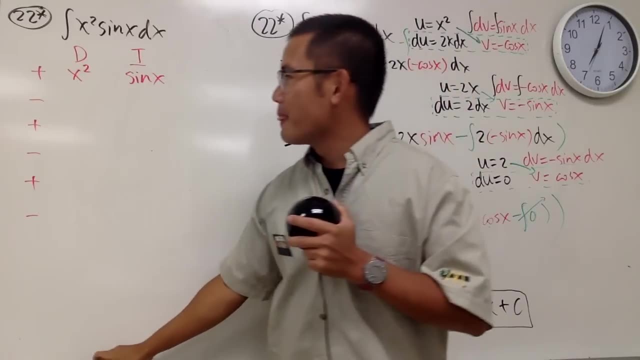 put down: plus, minus, plus, minus, plus minus. I don't know how many I need. I do, but like usually I don't. Let me just put down a few Again. originally: x. squared times sine x. 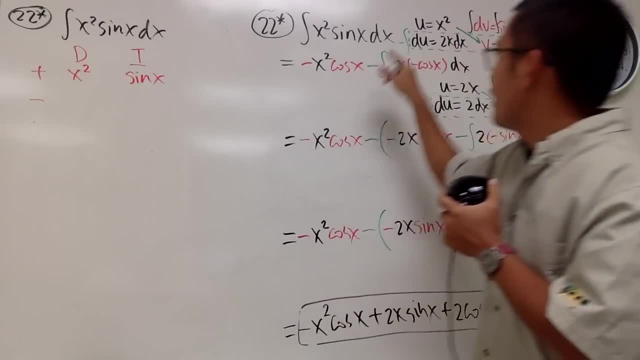 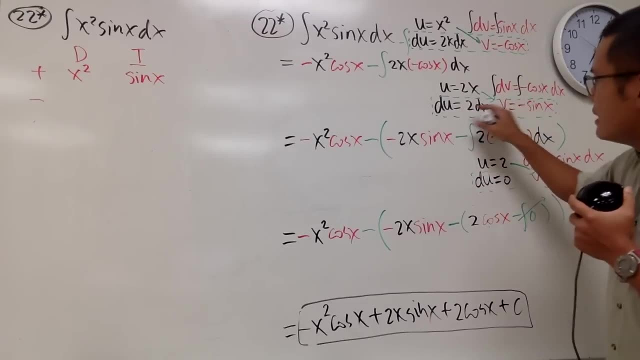 that was a positive integral, But in the next one you are going to have the minus integral, So minus. But you know, later on you are going to do this again And this is going to be another minus integral. 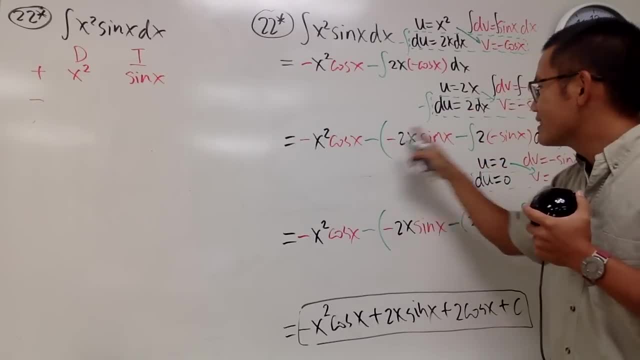 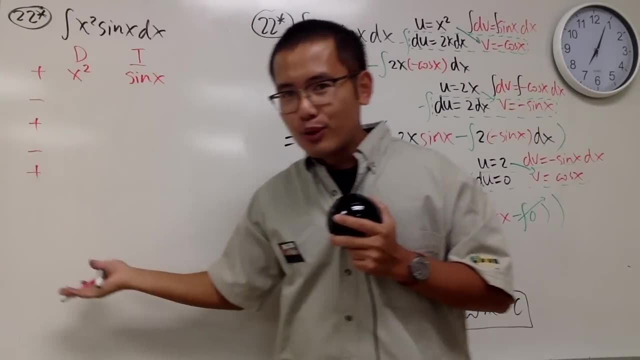 Which is this one right here. And then minus times, minus is a plus. That's why you set up plus minus, plus, minus, plus. I don't know how many I need, Just put down a few of them to get ready. 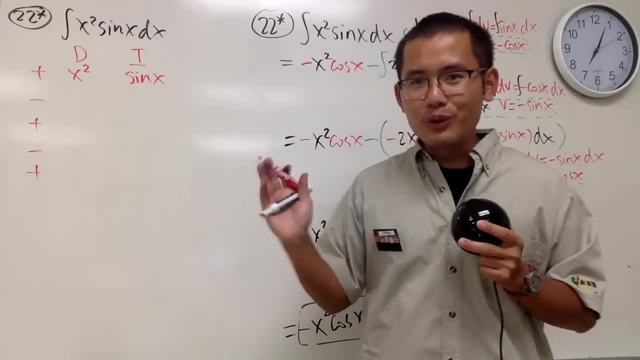 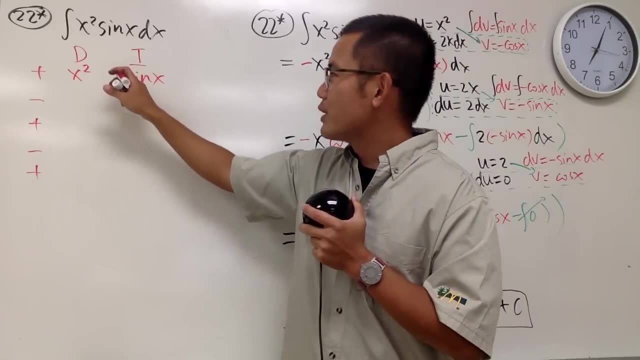 Alright, So that's the format, And this is the so-called d i method, The d i format, The d i setup. Alright, And now just do what I'm going to do. Let's go ahead and integrate sine x. 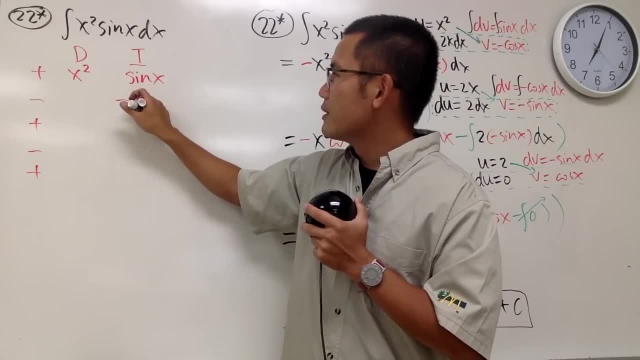 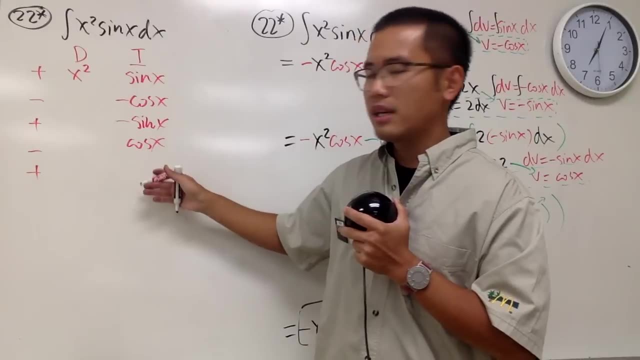 The first integral is going to be negative cosine x, Next we are going to get negative sine x, And then next it's going to be positive cosine x. And can we keep on going? Sure, Integrating cosine, we get positive sine. 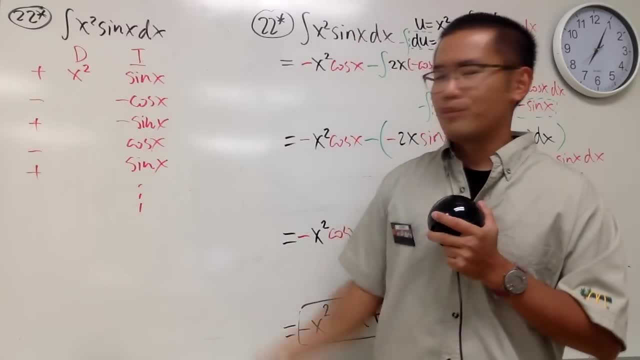 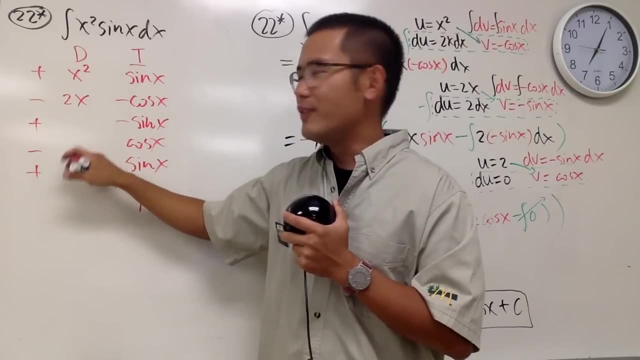 And then, of course, you can keep on going forever. In the meantime, why don't we just look at the d column and just differentiate this guy? Differentiating x, squared, we get 2x. Do it again, Differentiating 2x. 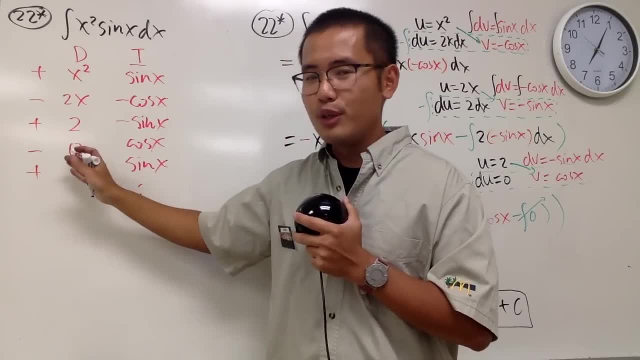 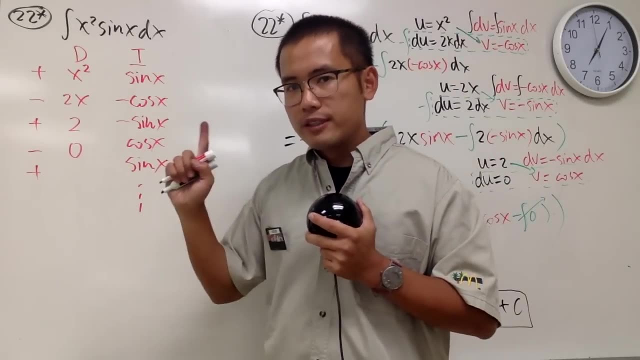 we get 2.. Differentiating 2,, we get 0.. Differentiating 0,, we get 0.. Doesn't matter anymore. Here's the idea. This is what I call the first stop When you see 0, in the d column. 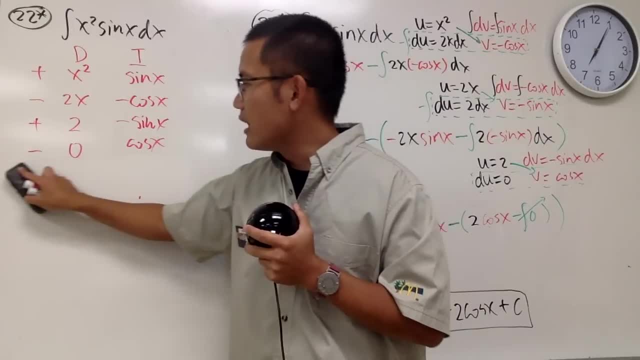 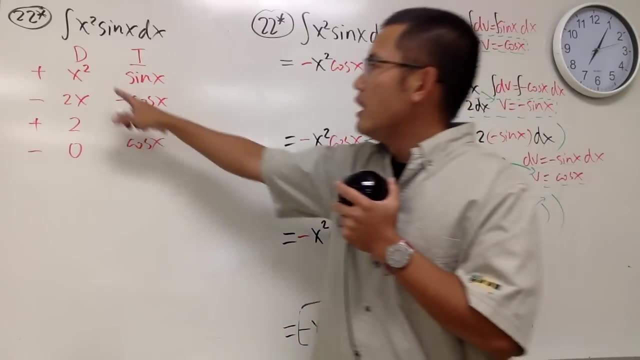 you're just going to stop. So in fact we didn't need the last row right here. So that's pretty much the setup with all the things that we did. And notice x squared 2x, 2 and 0,. 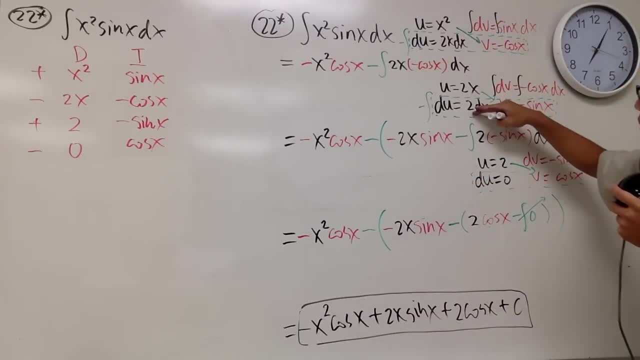 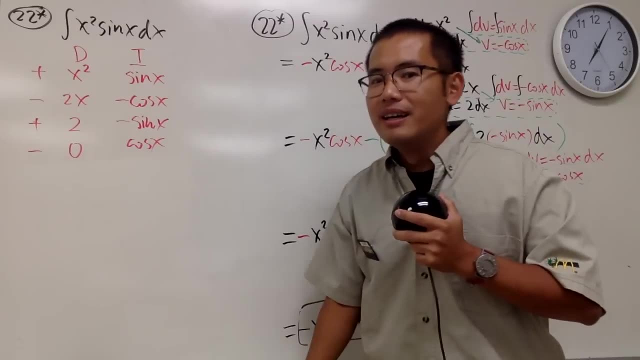 it's right here: x squared, 2x, 2 and 0. And that's just the part that will keep differentiating and we were able to get to 0.. Similarly, we integrated the sine and then we get. 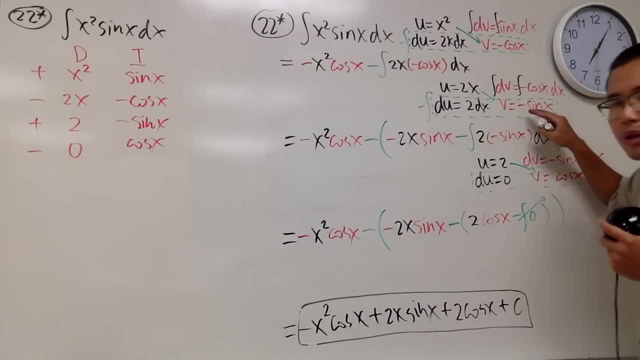 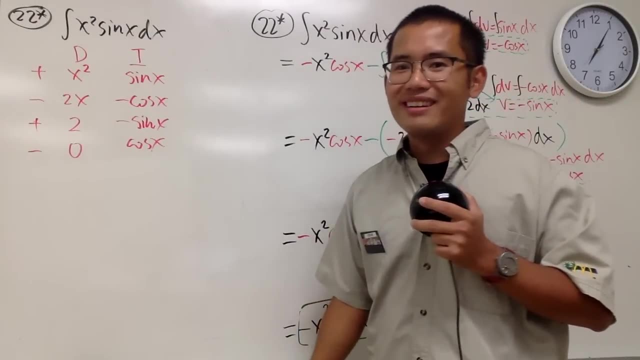 negative cosine and then we integrate negative cosine. we got negative sine and then we integrated negative sine and we end up with positive cosine. That's exactly what we did right here. Now, here is the best part When we are doing this. 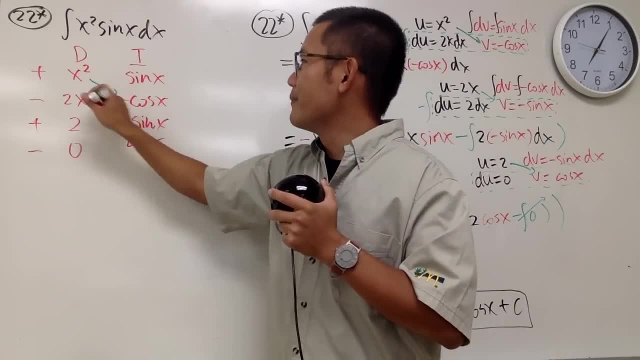 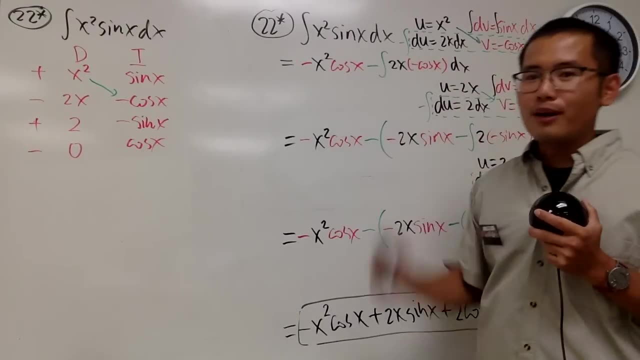 we are just going to multiply it diagonally this times, that, and that's going to be the first part of the answer. And that's exactly what we did. That will be the first part of the answer, right here. And the truth is: 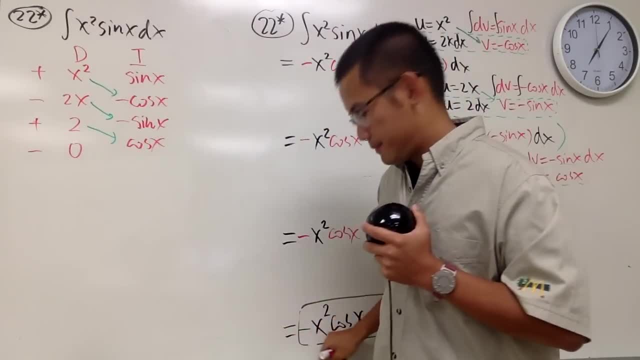 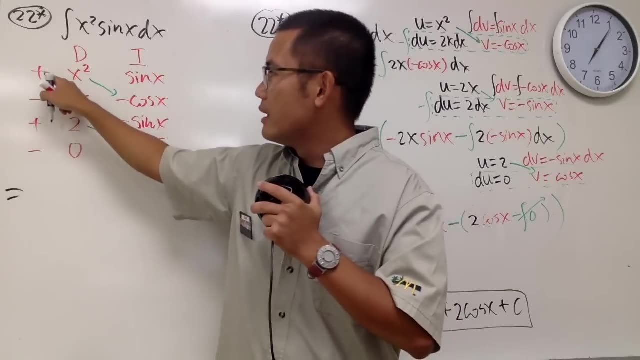 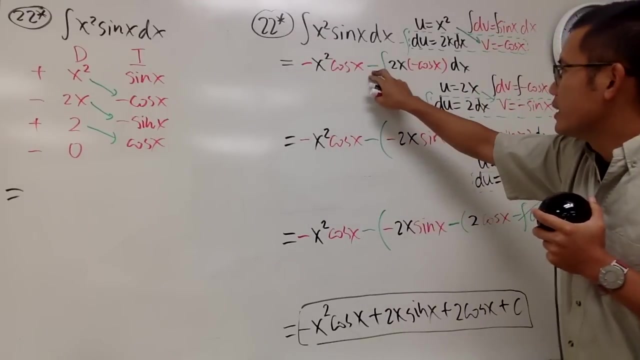 we just multiply all the diagonals and when we do the diagonals don't forget to account for the sign right here And the plus minus alternates, because again you have the positive integral already in the beginning. negative integral, Negative integral. 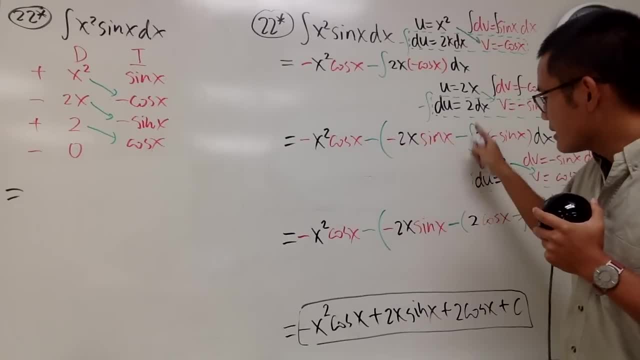 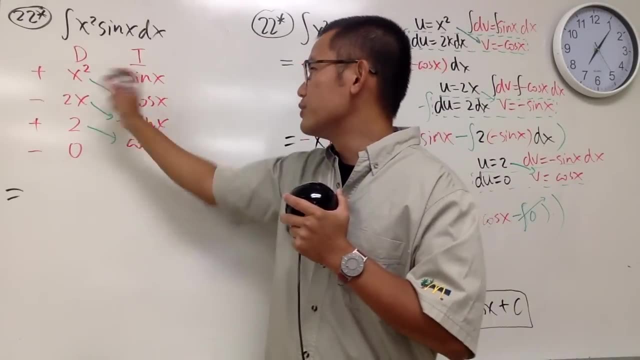 But another negative inside of the negative. So this is actually a positive integral and that's what we did right here. So that's why you have the sign alternating on the side. Now just make it happen. Here we have x squared times. this. 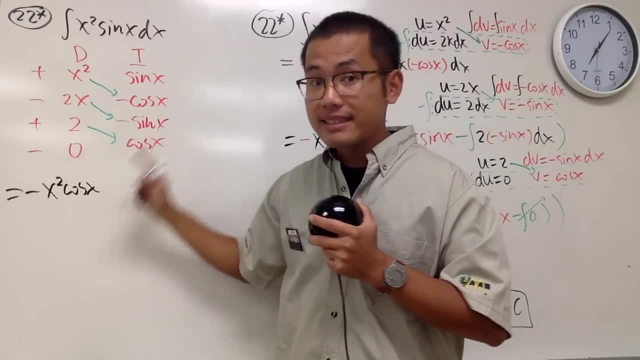 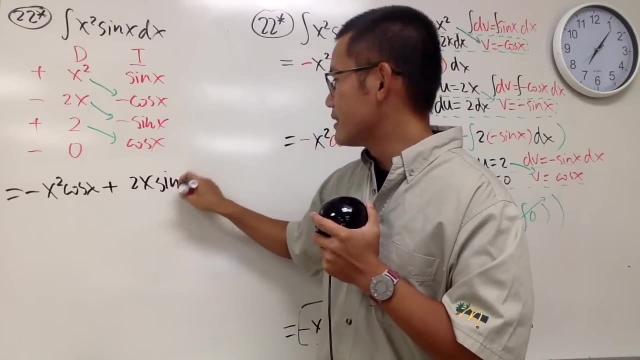 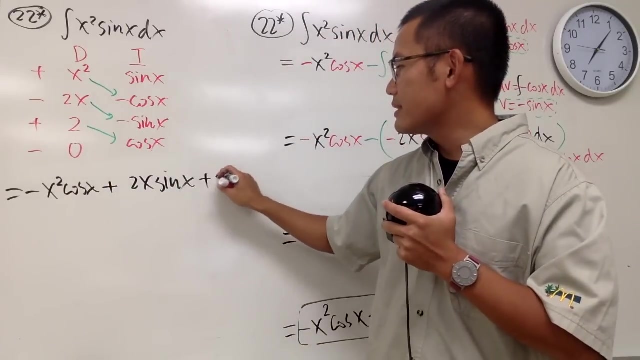 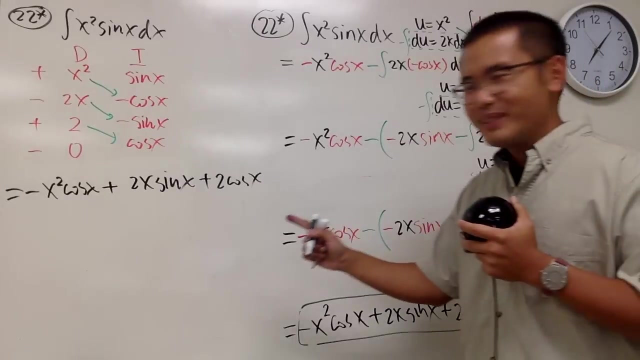 namely negative x squared times cosine x. Next negative 2x times negative sine, That is plus 2x sine x. Again negative times negative. Next positive: 2 times cosine plus 2 cosine x. Ah, we are done. 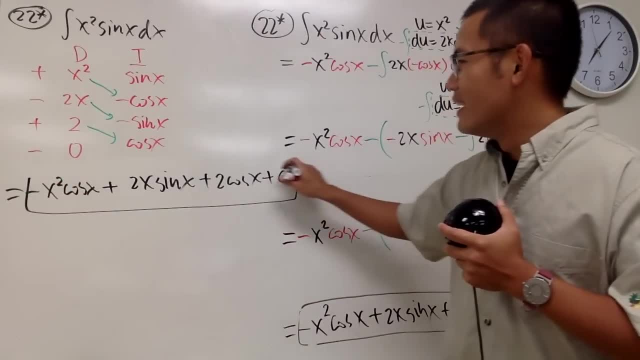 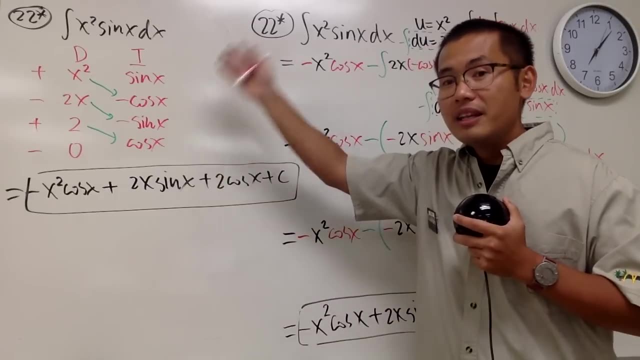 Look at that Plus c. This is it Right? This right here is it? You are using the di setup. This is not magic. This is just a nicer way to set up the integration of the parts, because you see that this is kind of redundant. 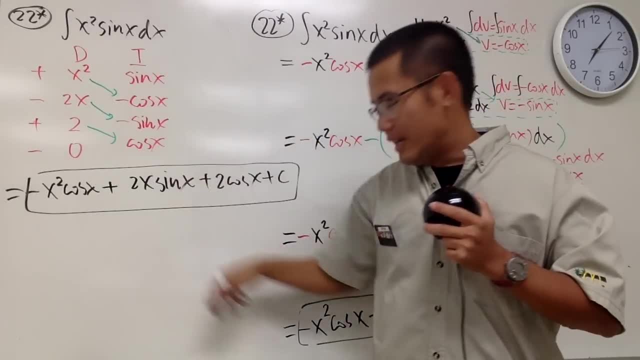 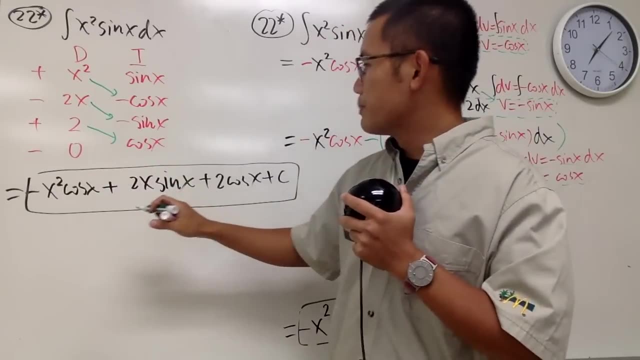 Right, This is just much more efficient. And let me tell you, we have three stops to go over, and this is the first stop. This is the first stop. Let me just put this down right here for you guys. Right, This is. 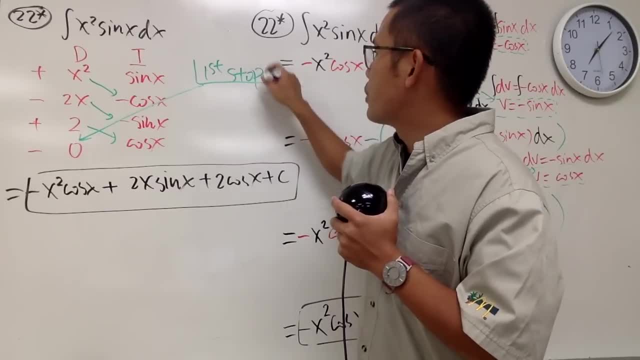 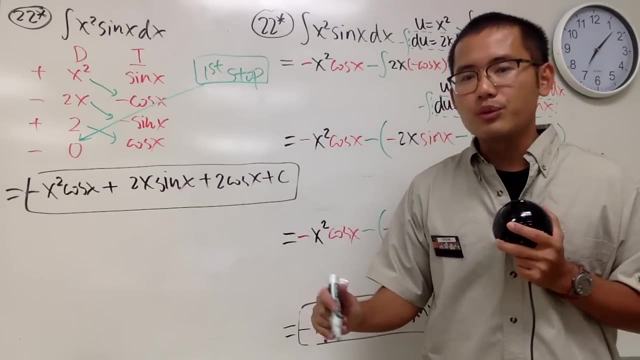 the first stop. I do have a separate video on, you know, the di method, but this is going to be the video that you need to know all the integration techniques that you need for calculus 2.. So here we have it. 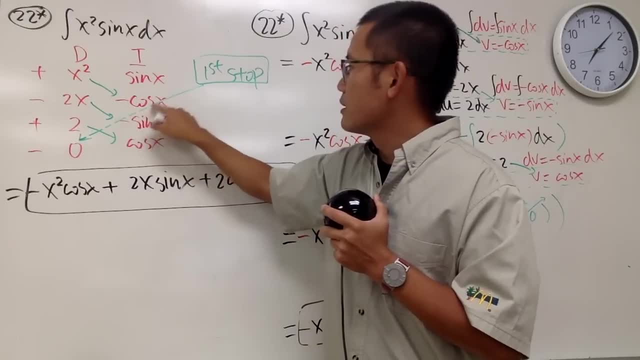 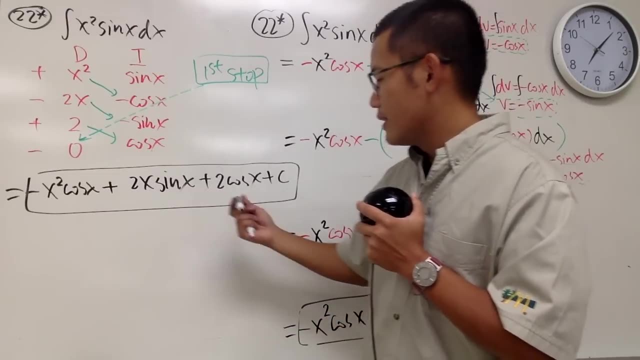 For the. let me just do it like a dash line, For the first stop right here is when you see the zero in the di column. Let me, man, I just want to make this. this is the first stop. Yeah, Hopefully this works out better. 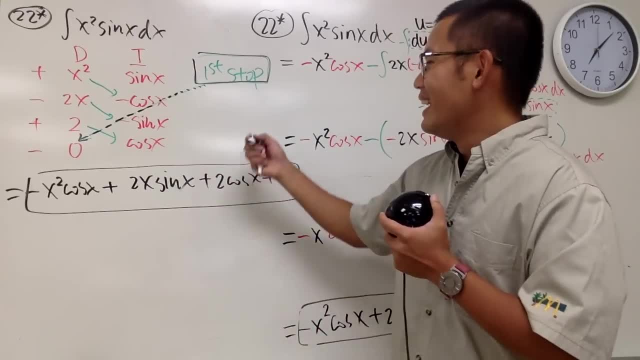 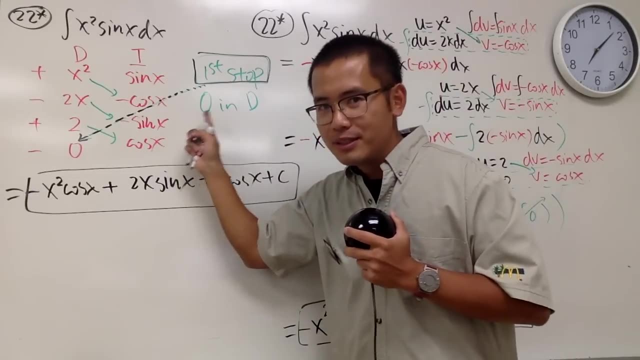 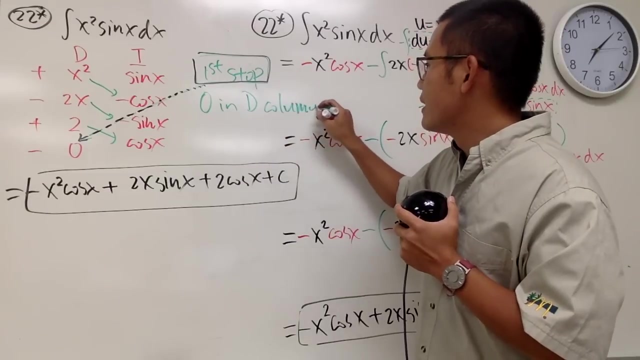 Anyway, first stop. we will see the zero in the di column. This is this is my zero, All right Zero in the di column. This is my zero, All right Zero. in the di column Column. When you see the zero. 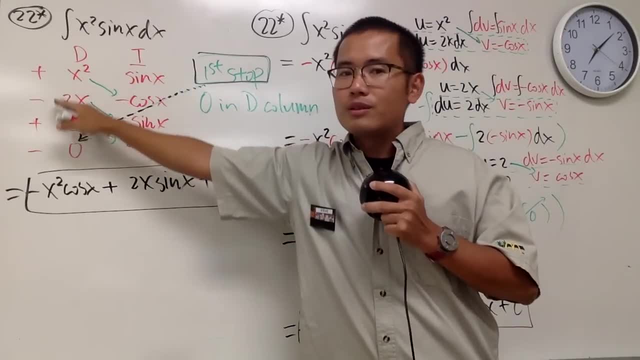 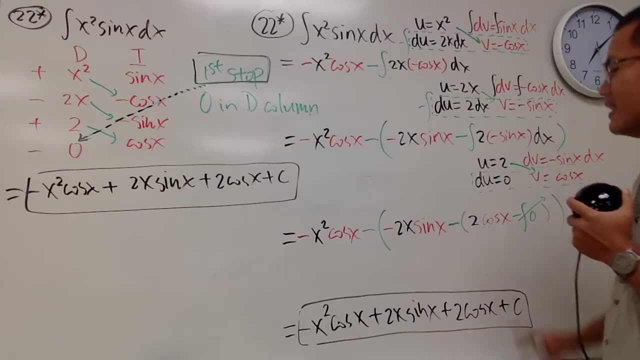 in the di column, you stop and then just multiply the diagonals along with the sign on the side, and that's how you get the answer for that. That's it Right? So that's the idea. And again, if you still are not convinced, 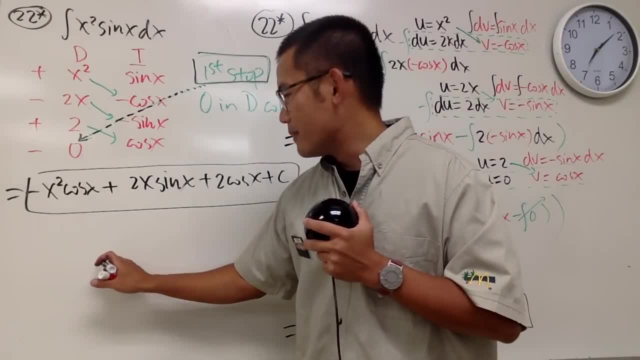 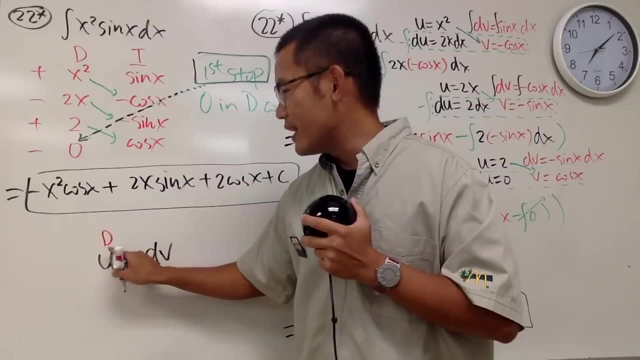 that why this method work. let me just show you. Check this out Earlier. you have the u and dv, Yeah, And we are just going to differentiate the u and we are going to integrate the dv When we differentiate the u. 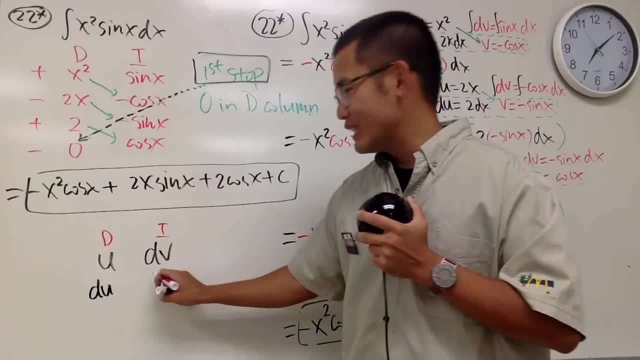 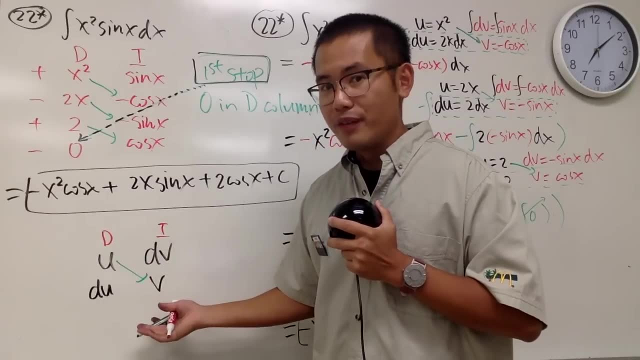 we get du, and when we integrate the v, we get v. And you see, when we multiply this and that, that's the first part of the answer, namely uv, And then, don't forget, you are going to minus the integral. 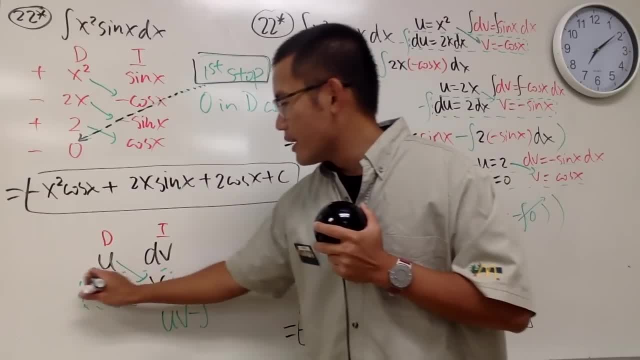 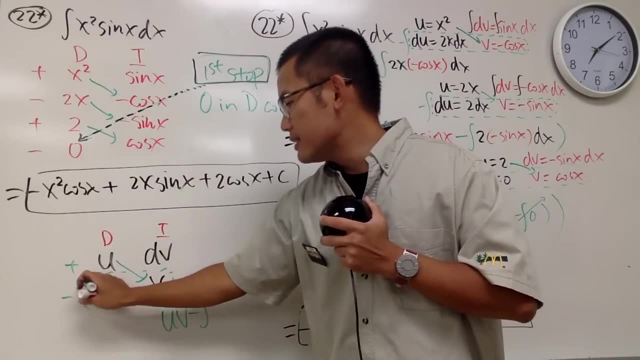 And that's when you multiply this right here And it's a minus because, as I told you, we have the plus minus on the side Plus minus, and then we have the minus and this is still an integral when you multiply this and that. 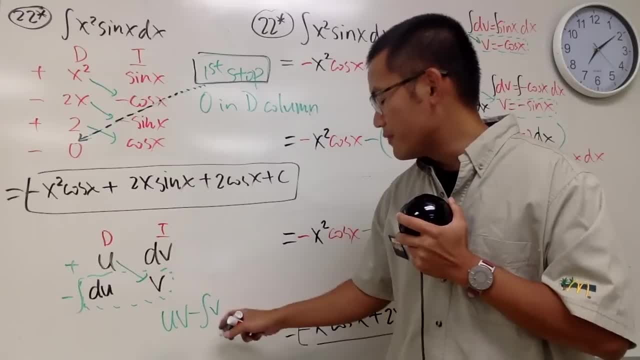 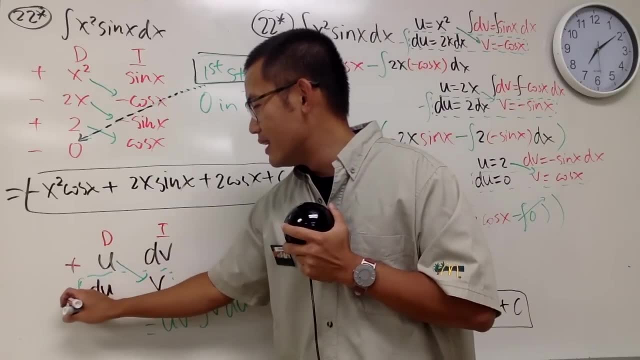 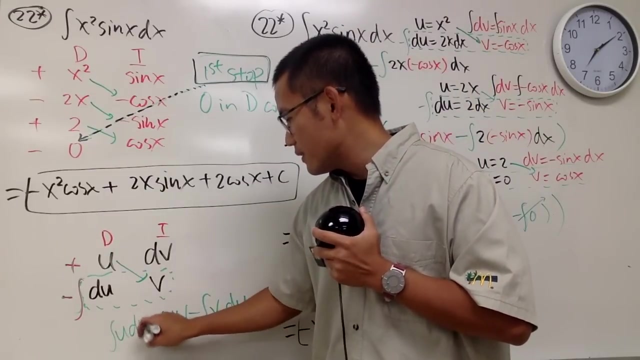 which is the integral of vdu. You put down v first and then du. Isn't this the same as the formula that I presented to you guys earlier? Yes, it is Right. So this is the integral of u dv. 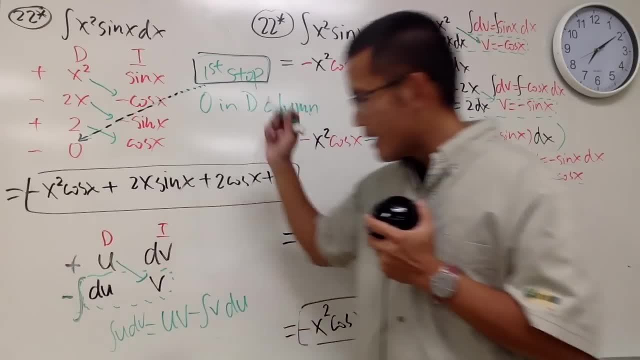 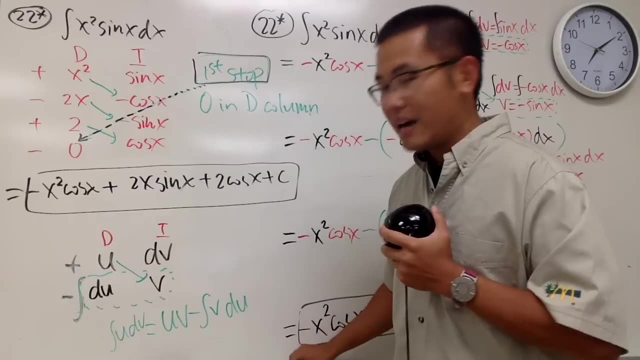 Yeah, So it goes like this. Yeah, So again, just a different way to set up the integration part. This is the first step And now we have a couple more to go. Yeah, Hopefully you guys are finding this helpful. 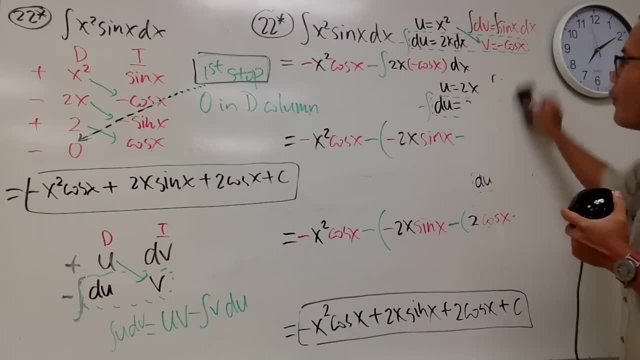 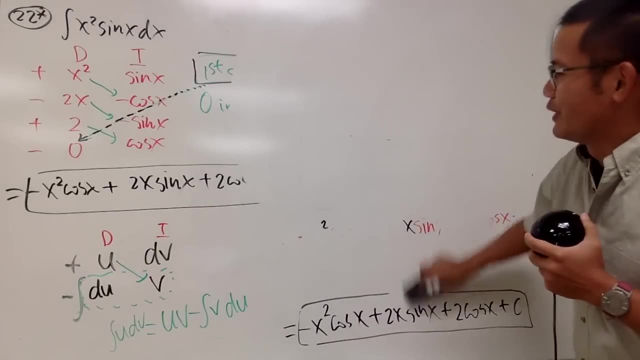 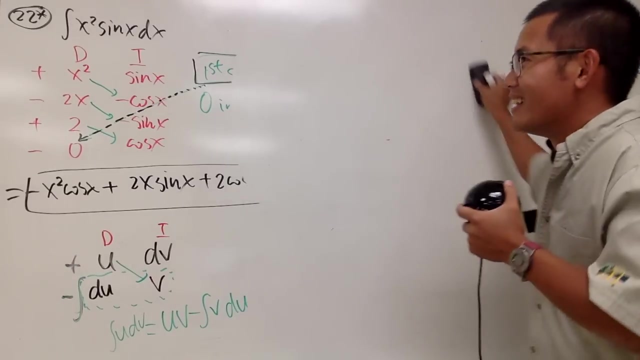 because this is taking a lot of time to go over. It's not. I'm not just trying to work out the question, I'm trying to teach all the details. So I expect to spend a lot of time for this video, Maybe longer than the 100 integrals. 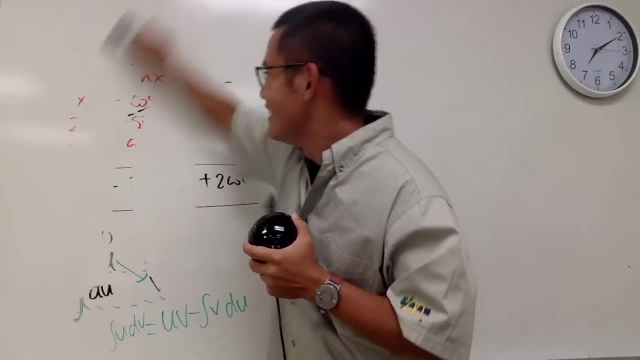 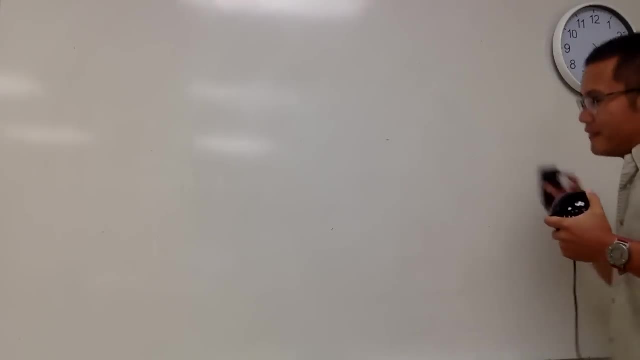 That's why I can only do 50.. So hopefully you guys don't mind If, if you guys want, I can come up with like another 50 questions, just randomized and Cal2Level only, and then just all these techniques. 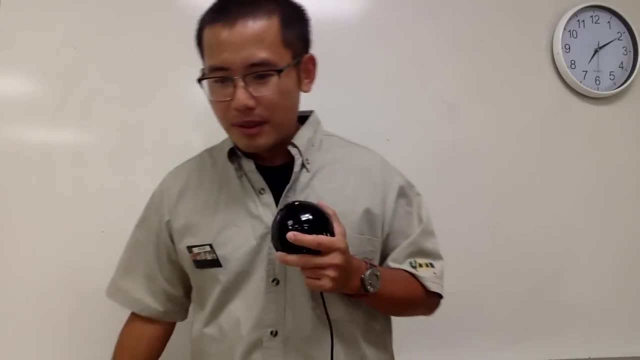 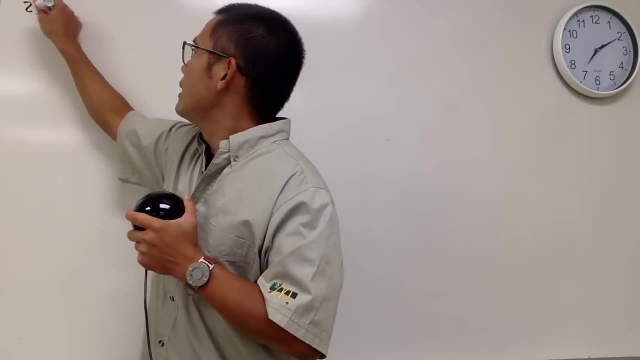 And if you guys want to maybe leave a comment down below and let me know, All right. In fact, let's take a look at question number 25.. Again, And let's look back to the integral of x, to the third power. 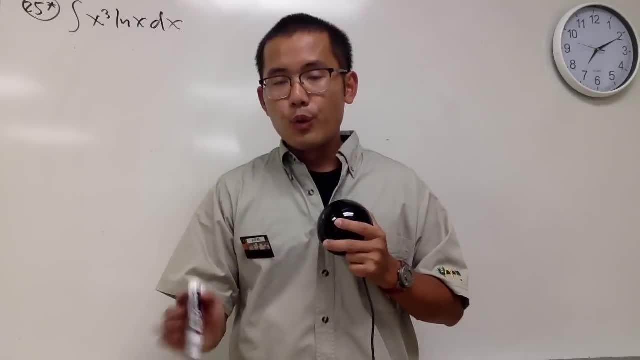 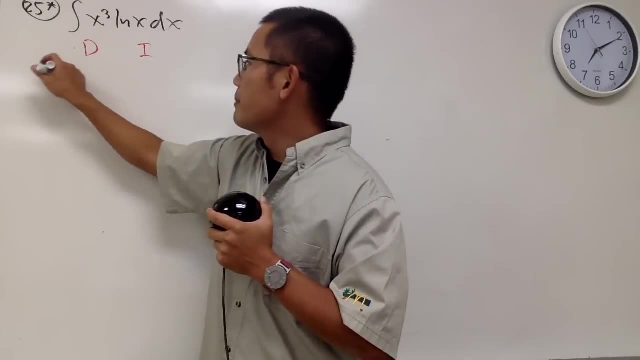 natural log of x dx. This time we are going to do it with the di set up And this is how we do it Right here. I will put on the d and also the i plus minus plus on the side, just to get ready. 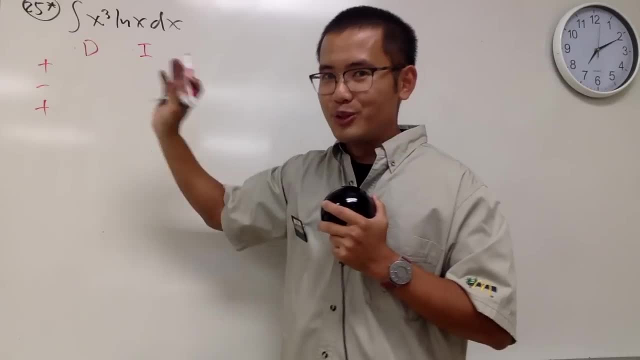 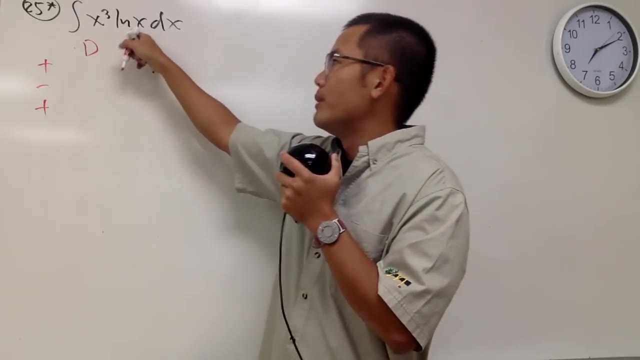 Okay, We did this earlier, So you should be familiar with this, right? Well, I'm going to pick one part to be integrated and I'm not going to choose ln of x. I will integrate x to the third power and I will be differentiating. 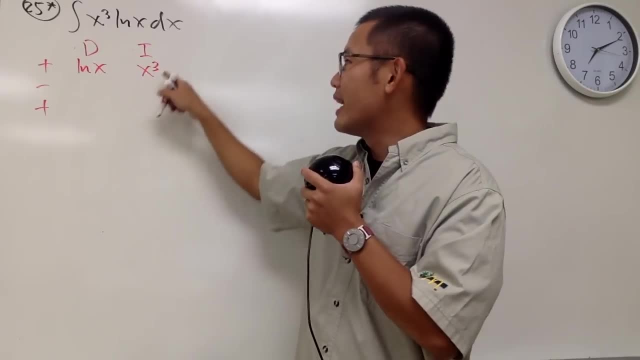 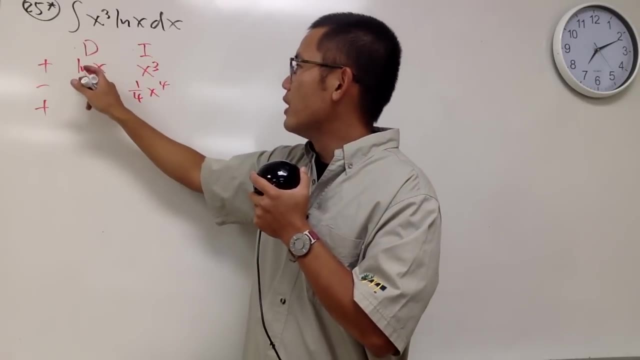 natural log of x, because when I integrate x to the third power, this is doable, I get this. And when we differentiate ln, x is 1 of x, this is also doable. Now, here we have a small trouble. 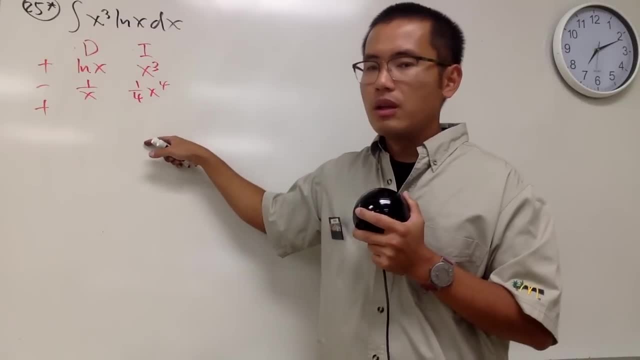 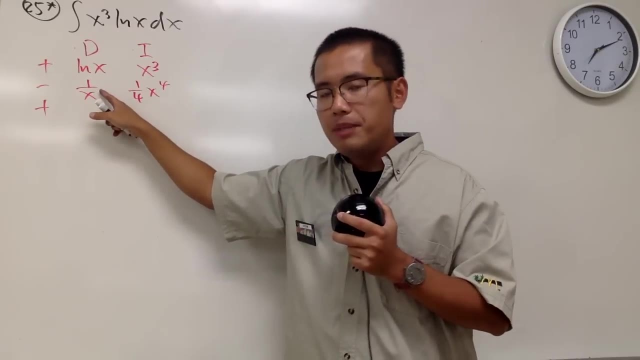 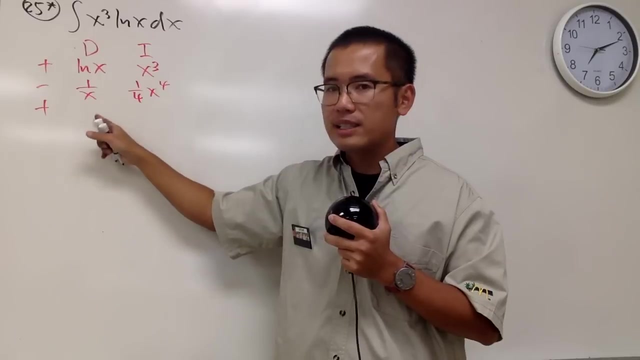 So we keep going. In this case, here we can. we can keep integrating this Good, But what if we keep differentiating? 1 of x, The next one is going to be negative. 1 over x squared, and the next one: 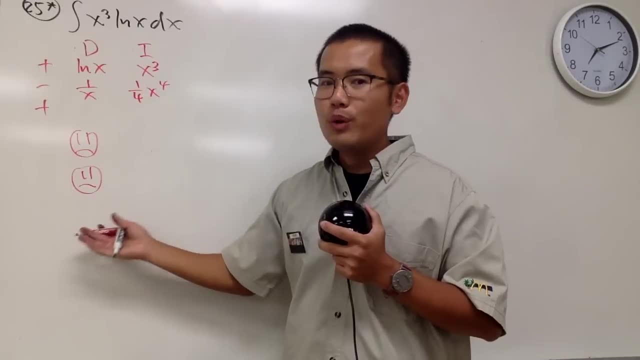 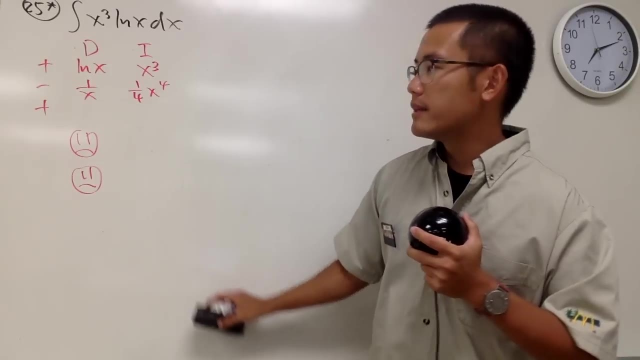 is going to be not good, Not good, And we will never get to 0. Right. So this is very different than the first stop situation. That's why I want to go over this with you guys. In fact, we are going to stop. 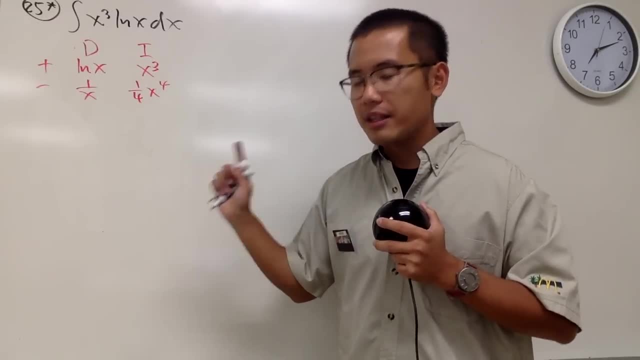 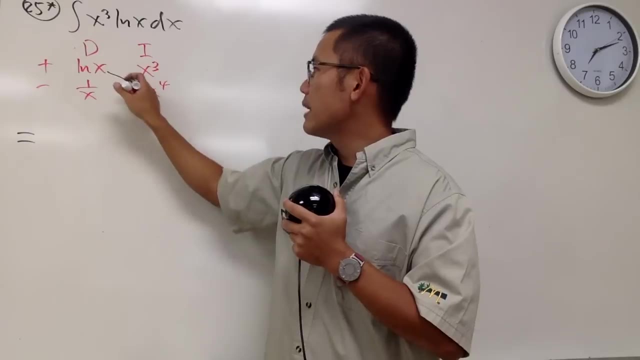 right here. In fact, we are going to stop right here Because this is just like the traditional format. What we do is go ahead, just do this times, that which is 1 over 4. x to the 4th power times: ln x. 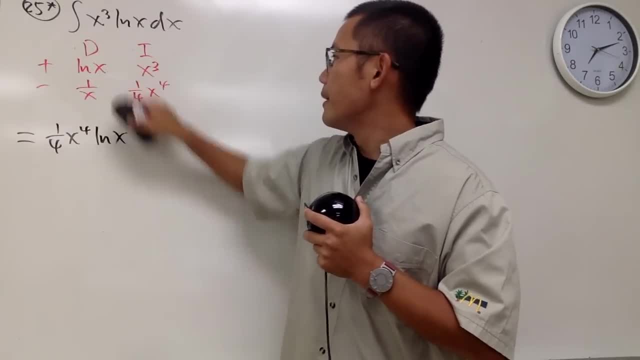 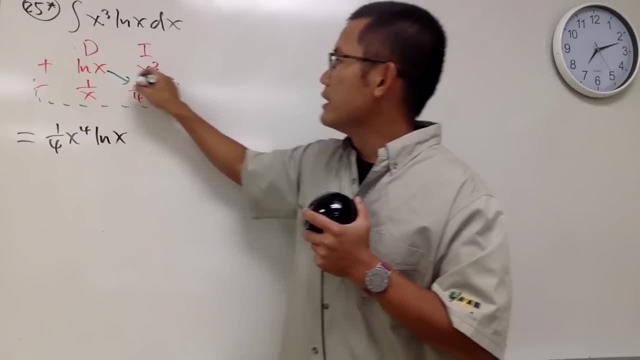 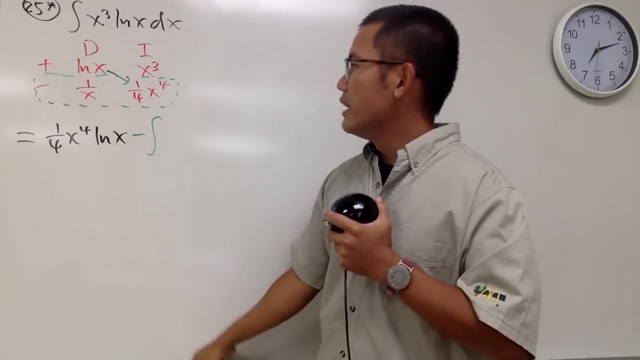 And then we are going to multiply the second row and that will be still inside of an integral and this is a minus Notice: we have a minus times positive, times positive, So it's a minus as a minus integral. And then 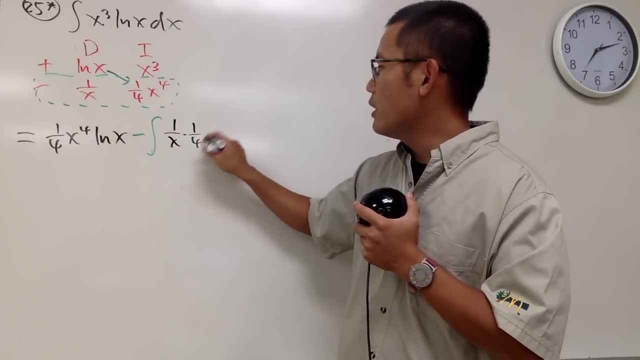 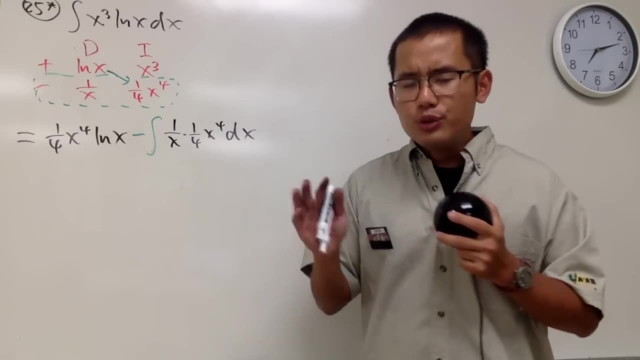 we just put this and that together inside, So we have 1 over x times 1 over 4, x to the 4th power, dx. And the reason that we stop right here is because you should have a sense of danger. 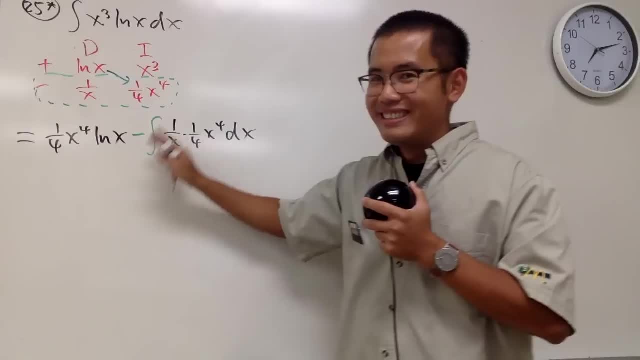 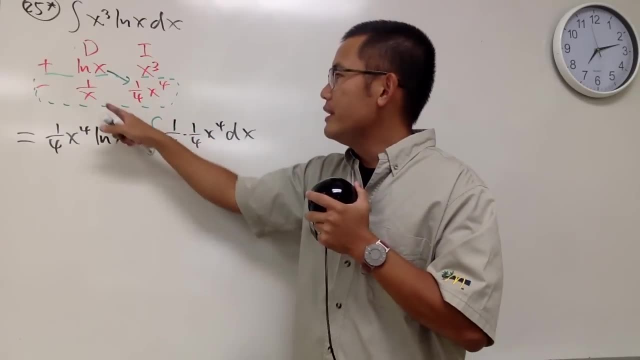 If you keep on going seriously, we can never get to 0 in the d column. So that's the first thing. But the idea here is that in fact, we can actually integrate the product of this and that, Because 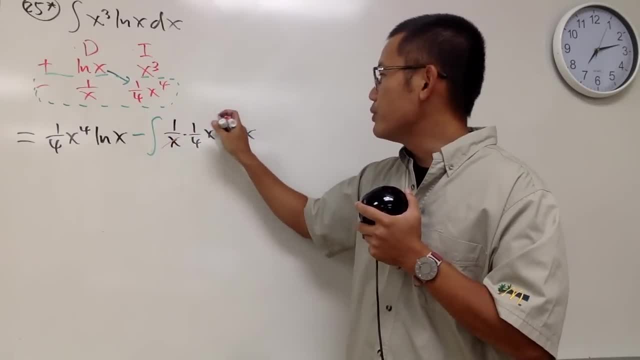 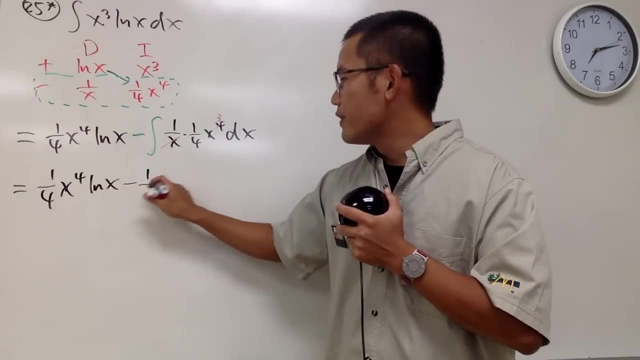 when you have the product right here. of course, this and that can be reduced, And we are just looking at 1 over 4, x to the 4th power natural log of x And then minus 1 over 4. 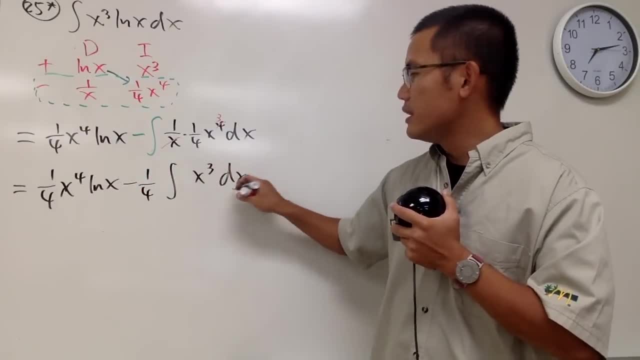 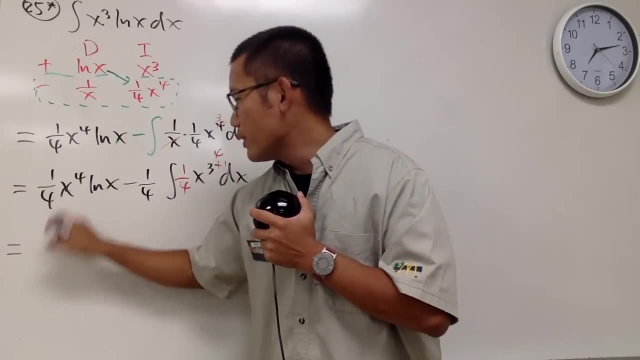 integral: x to the 3rd power, dx. Of course we can integrate this, Add 1 and divide it by that, and we are done. So finally, 1 over 4. x to the 4th power. natural log of x. 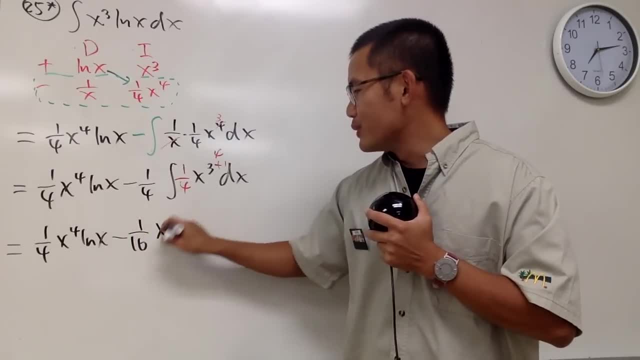 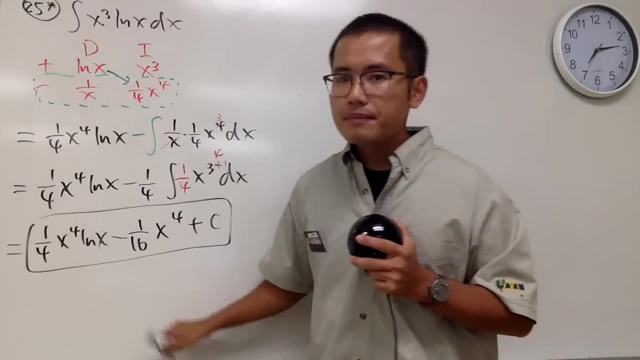 this times that minus 1, over 16, x to the 4th power plus c, Just like that. Here it's the second stop. This is just like a traditional, traditional UDP format. The second stop is that. Let me just put it down. 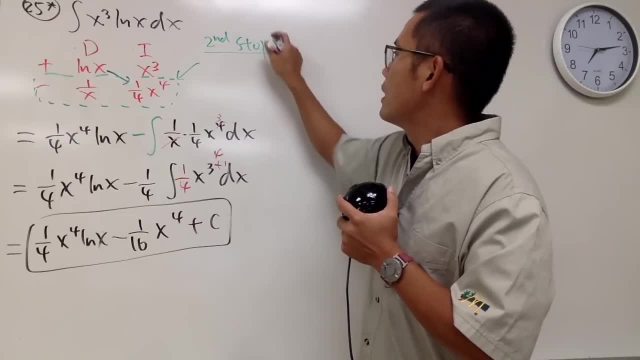 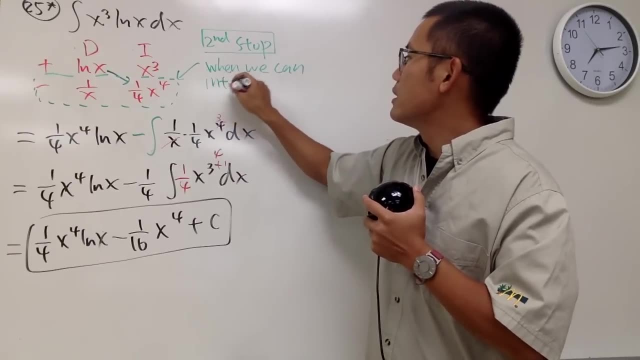 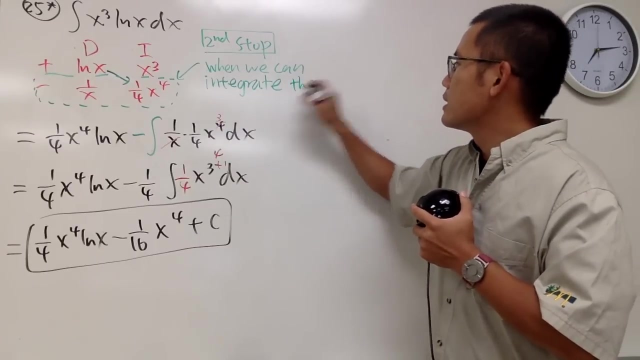 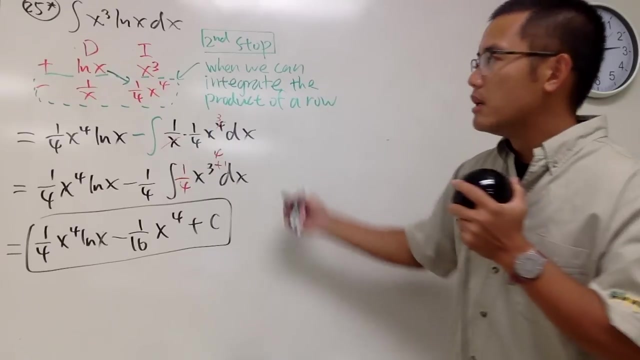 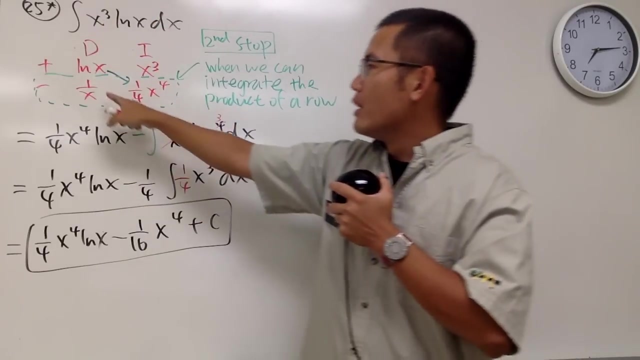 Second: stop. Yeah, When we can integrate, whenever we can integrate- the product of a row, of a row, then we stop. Notice earlier this times that that's the original question. We couldn't do that right. But when you do this, 1 over x. 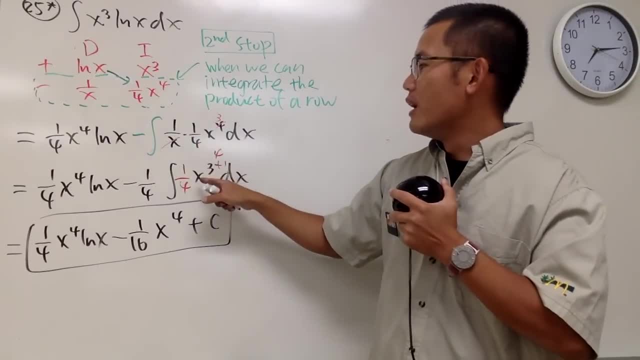 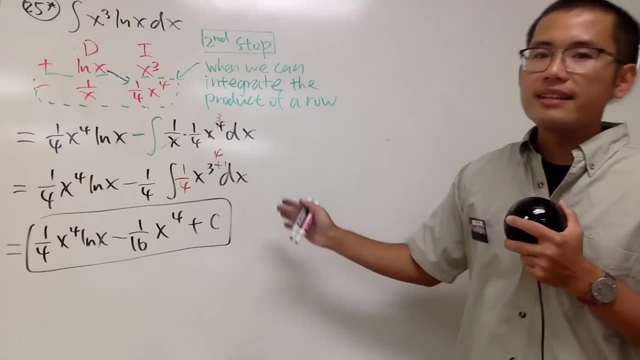 times 1 over 4 x to the 4th power. this is just 1 over 4 x to the 3rd power and of course we can integrate x to the 3rd power. We can integrate the product of a row. 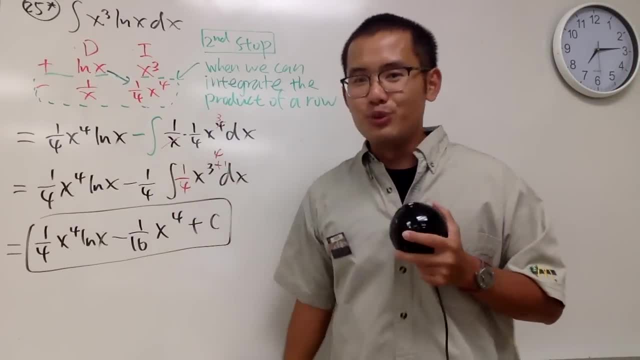 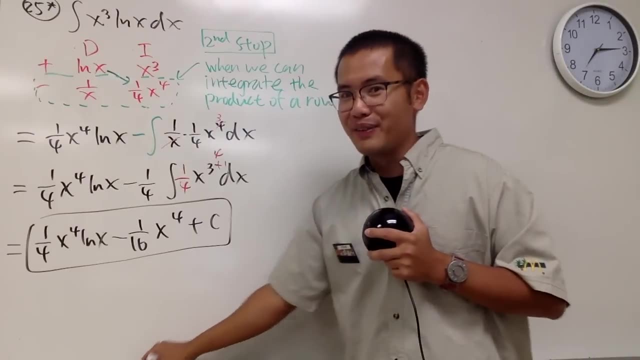 then in that case we just construct it and do the usual thing. This is the reverse power row situation. So that's pretty much it and that's the second stop, Right? So that's question number 25.. Notice, yeah, we are actually. 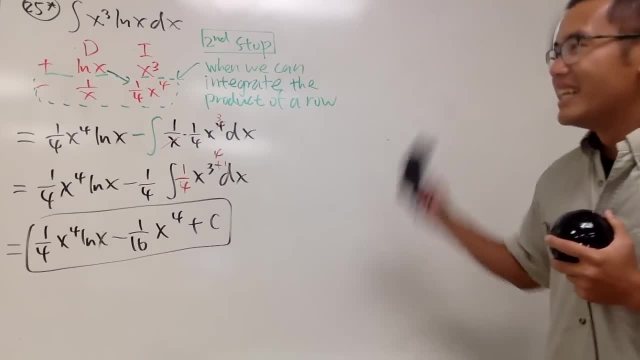 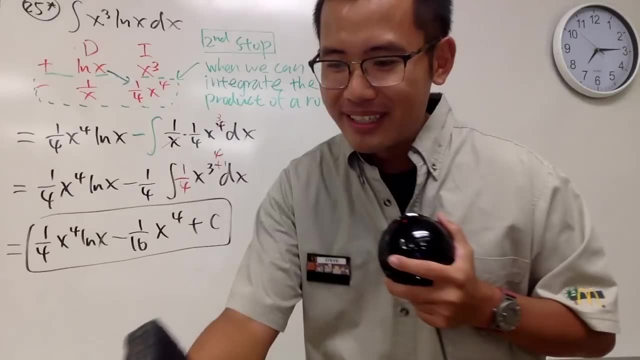 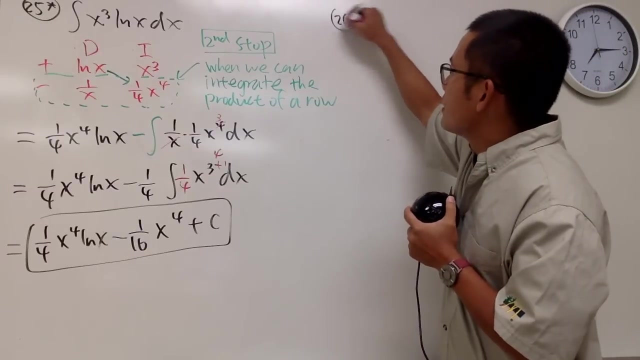 doing more than 50 integrals, because we do some integrals more than one time. So this is question number 25, star meaning question number 25, another look Right, So let me also put down this one. So we have. 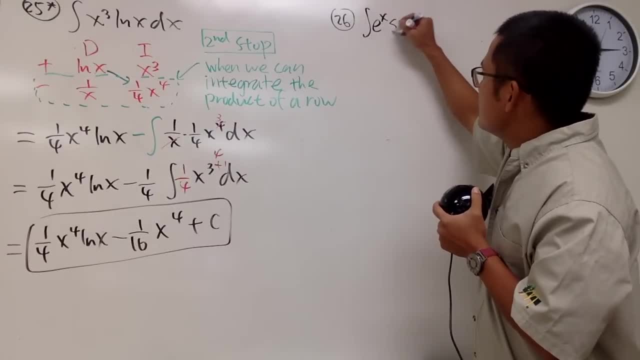 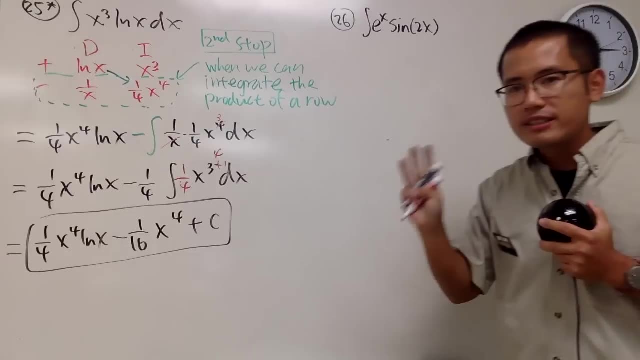 x to the 6th right here, and we have the integral of e to the x times sin of 2x. This is going to be a very special one, you'll see. This is also going to explain the third stop and you guys will see this. 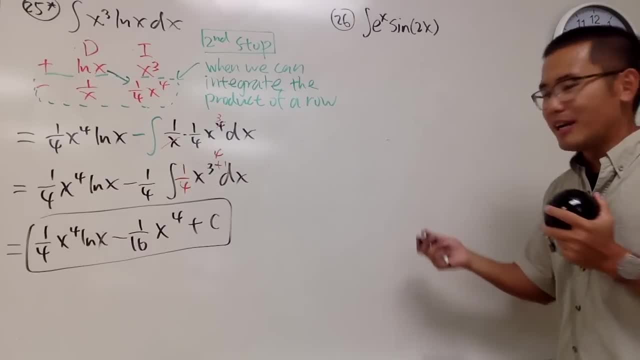 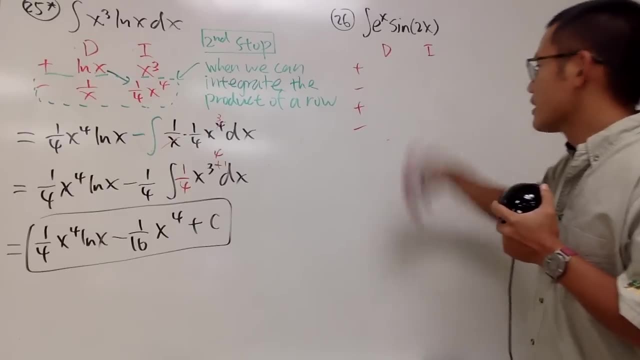 in differential equation later on as well. So be sure you know how to integrate this kind of things. Okay, here we go. Well, again, you can imagine that we have this integral minus on the side to get ready. Well, in this case, 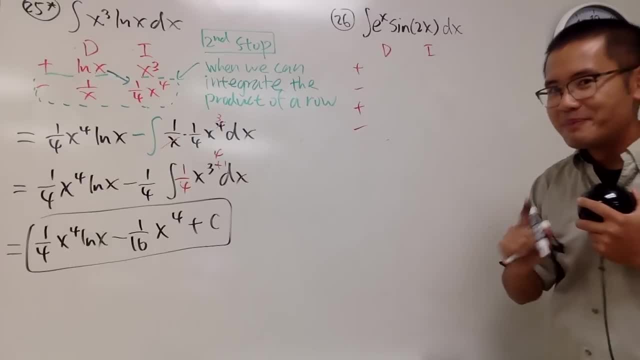 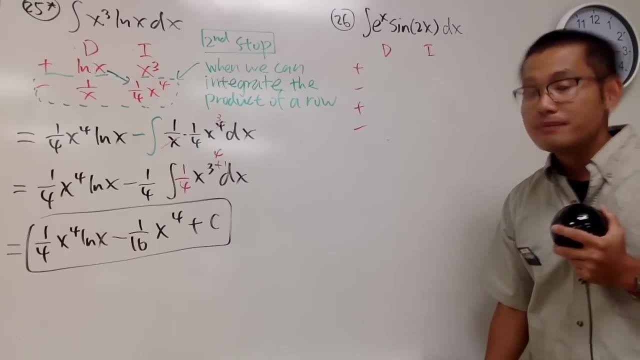 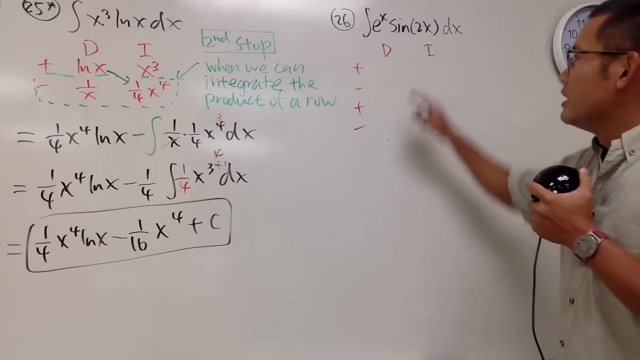 again, let's choose what we should be integrating. Should we integrate? should we be integrating, sin of 2x? Well, I should ask: can we integrate sin of 2x? Yes, And in the meantime, can we also integrate e to the x. 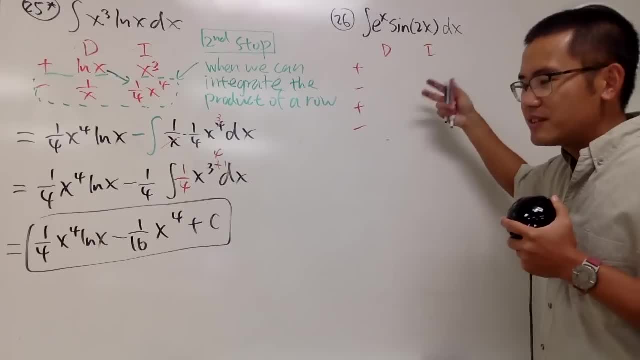 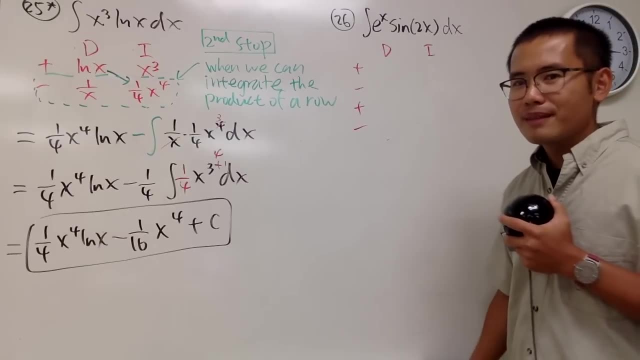 Yes, And imagine that we have a negative sign and all that stuff. they will just keep repeating. Likewise, if you integrate e to the x, it's just already e to the x, right? The truth is, it doesn't matter which one you integrate. 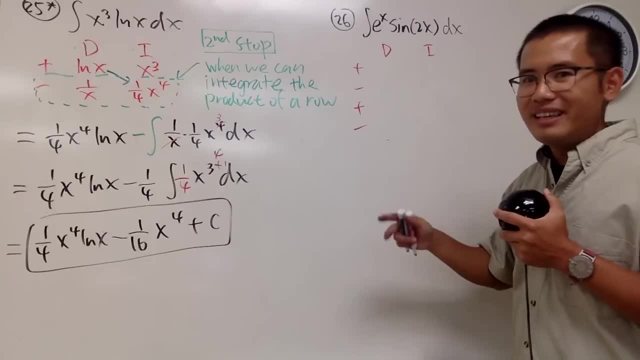 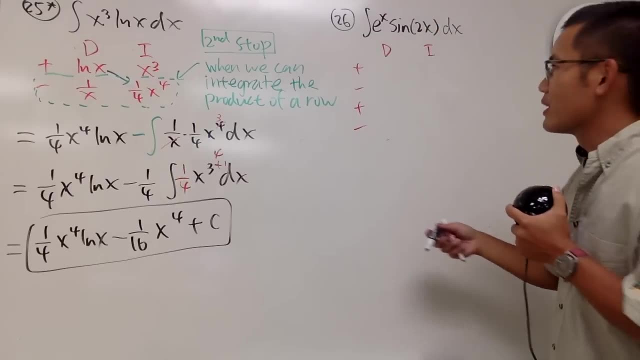 or which one you differentiate in this situation, because in the end you will see that it's just going to be repeating anyway because of the property of the sign and also an e to the x and all that stuff. So in this case, let me just 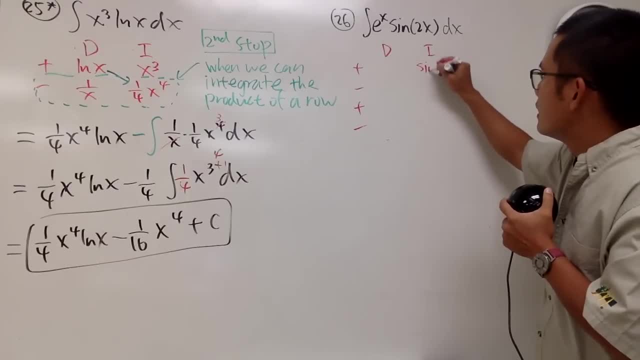 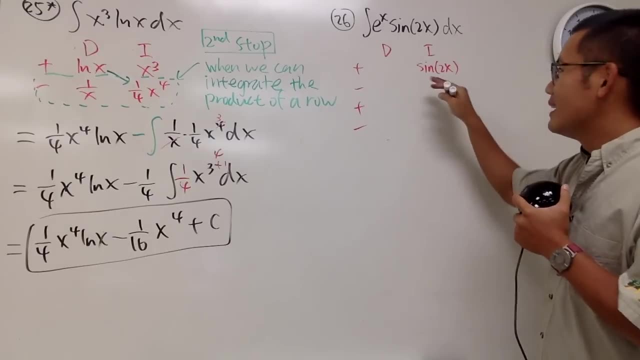 integrate e to the x, just for practice purpose. I know it would be easier to integrate e to the x and if you want to do that, yes, you can just try that on your own. but again, I just want to show you guys, let's differentiate. 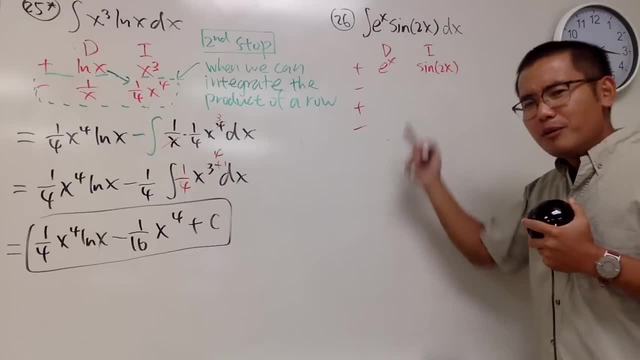 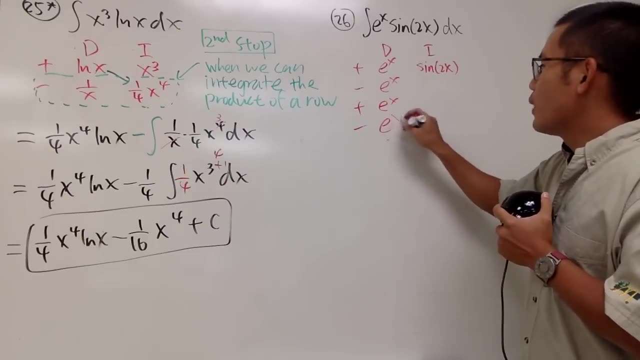 let's integrate this and then differentiate e to the x. How many times can you differentiate e to the x all day long? right, I know, we can just integrate, differentiate this. we can do whatever we want with e to the x all day. we can just do it. 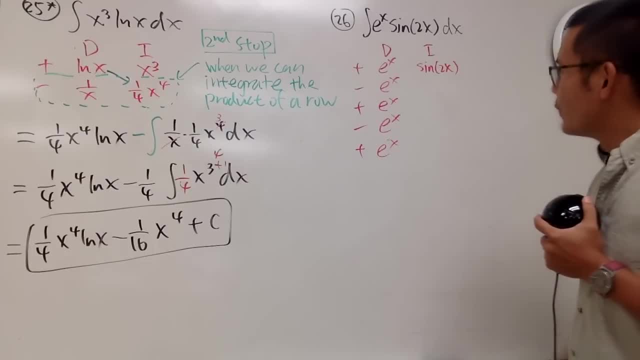 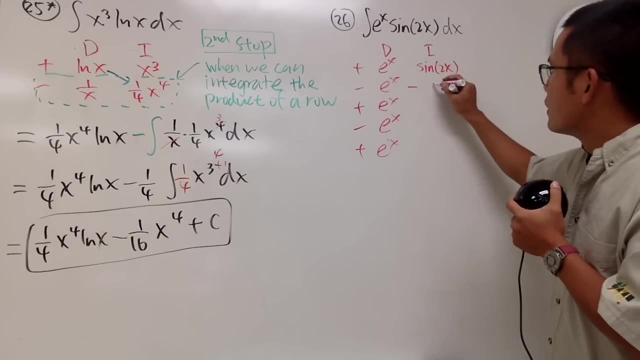 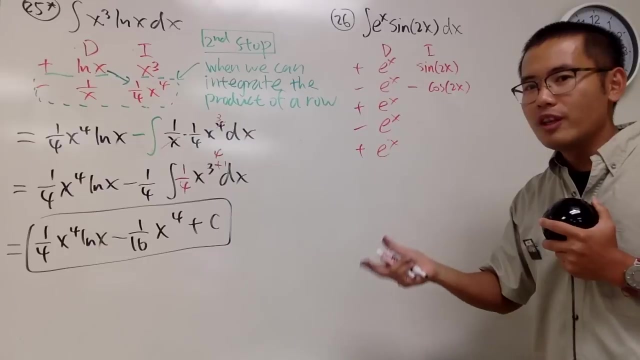 whatever It's not being tired. Well, face the reality. let's go ahead and integrate sine of 2x. when we do that first, we get negative cosine of 2x, and you see, this is why I want to integrate this, because we can practice. 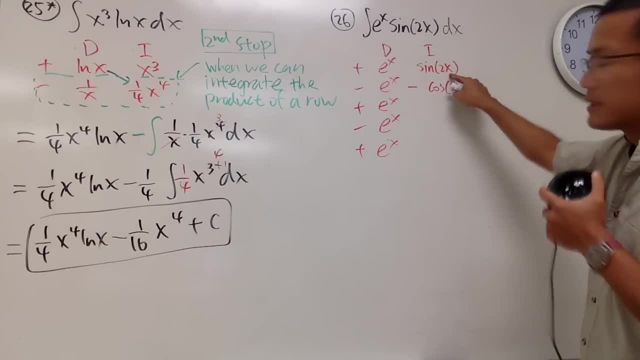 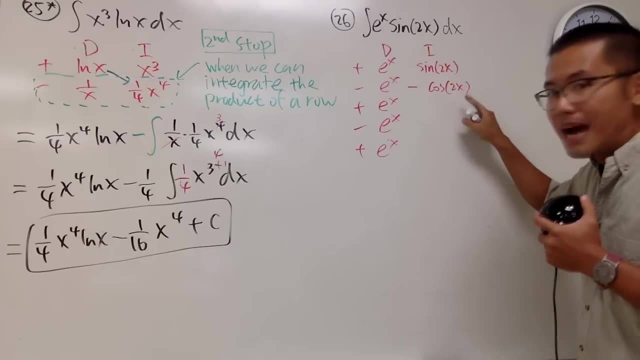 with one of the formulas I mentioned earlier. The derivative of 2x is just a 2, so integral of sine is negative cosine and we leave the 2x inside to be the same. but we have to. we have to divide it by the derivative of 2x. 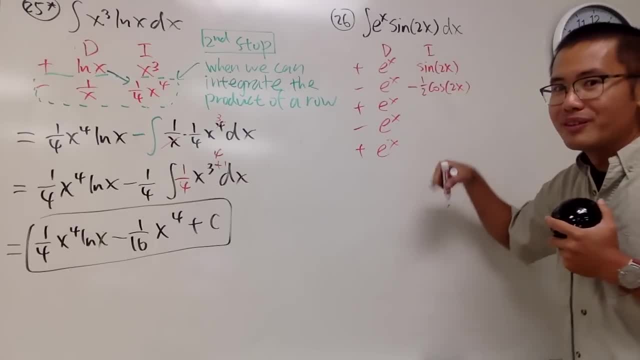 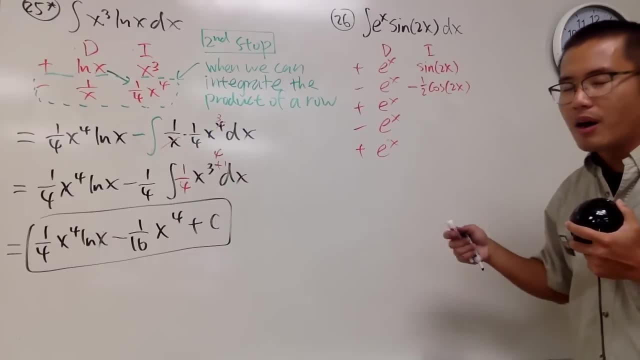 which is 2, because of the reverse chain rule. right the u sub if you want, but try to do this in your head, because if you write down all the u substitution part, it's just going to take way too long anyway. in fact, we need more. 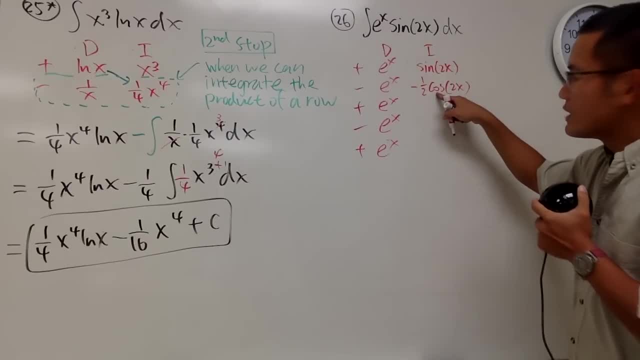 and let's just go ahead and do more. integral of cosine is positive sine, so we put down sine and the input stays the same and we have to divide it by 2 again, so it will be 1 over 4 and it's negative earlier, so we just maintain. 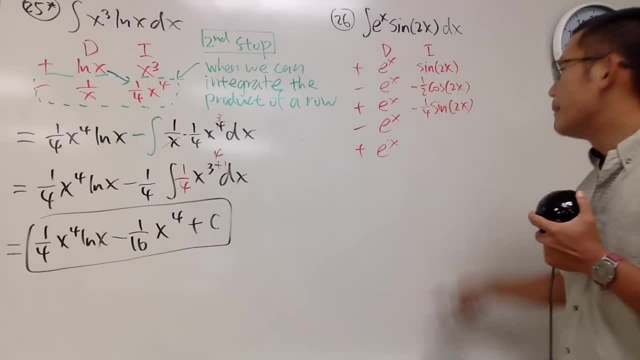 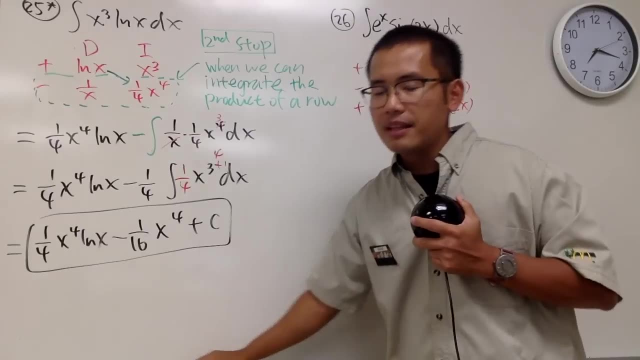 the negative, and so on, so on, so on. I'm not going to keep on going. in fact, this is all we need. we didn't need this 2 again. sometimes I don't know how many I need. I'll just put down plus minus, plus minus to get ready. 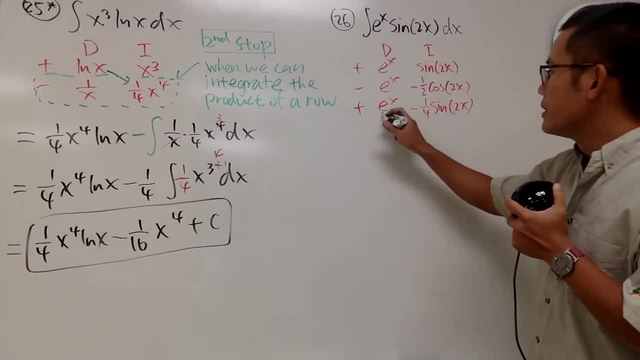 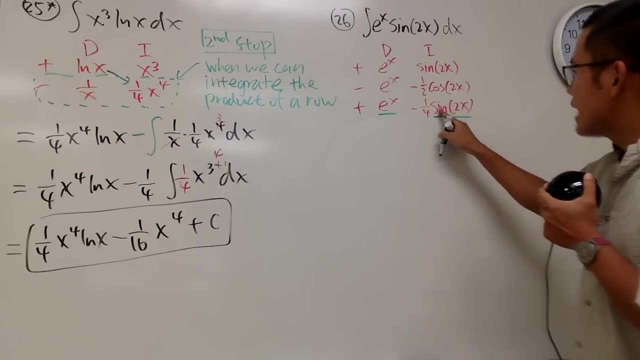 but this is what I need. here is the third stop, and the reason that I'm stopping right here is because you see that we have the e to the x and pay attention to the function part. this is sine of 2x. e to the x, sine of 2x. 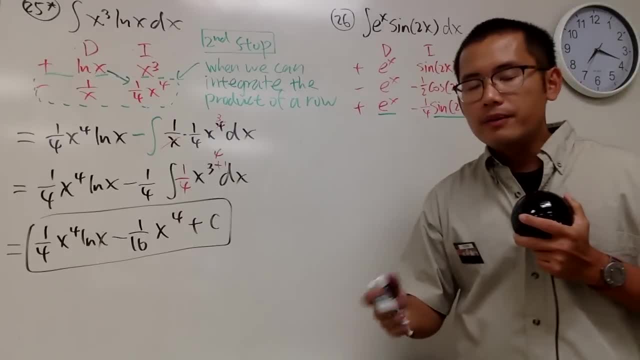 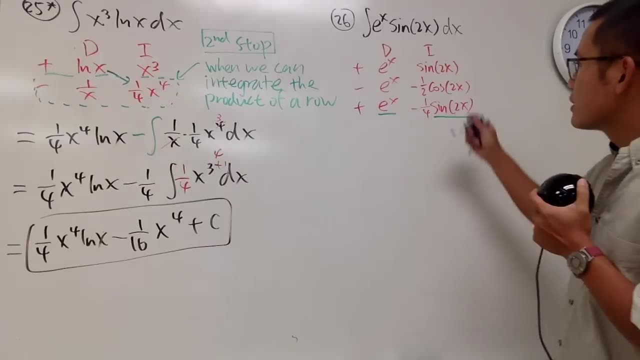 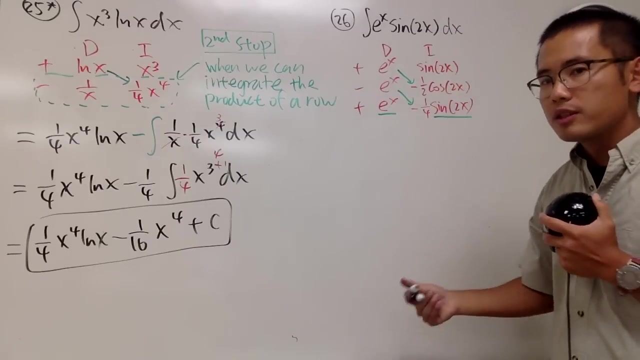 it repeats from the original. whenever the function part repeats, you stop right here, right now, just like what we did earlier, let's go ahead and put down this times this along the sine, right here, and this times that we have 2 diagonals, so we have 2 parts. 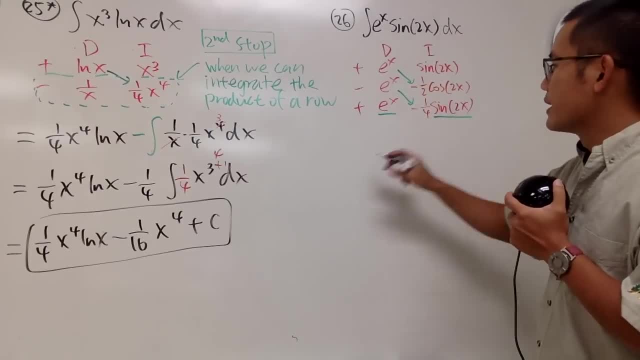 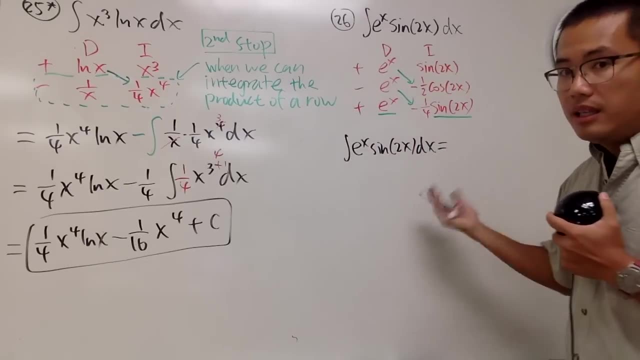 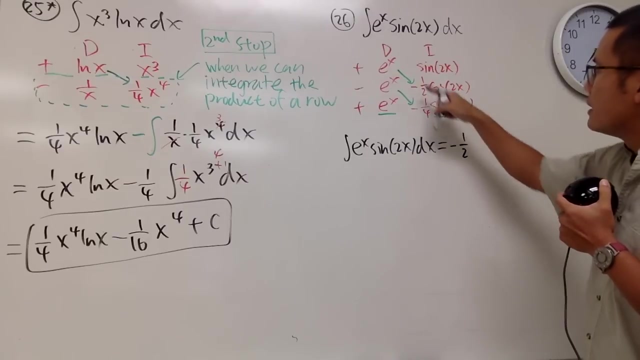 of the answer and for this particular one, we are going to write this down again. let's write down the integral e to the x sine of 2x dx. this is going to be e to the x times that. so I will write down minus one half. 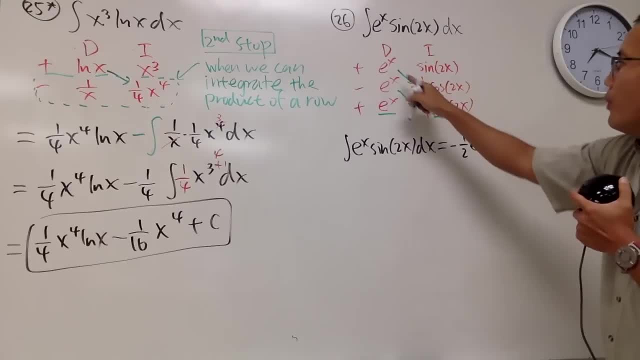 e to the x, yeah, and times cosine of 2x, like this: yeah. and next we are going to do negative times, negative, negative times, negative, which is positive, and 1 over 4 and e to the x and we have sine of 2x, like that: 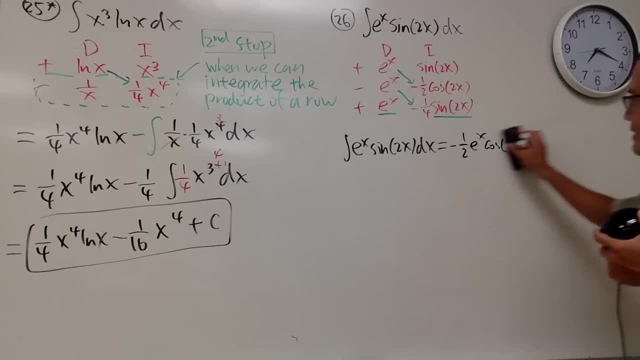 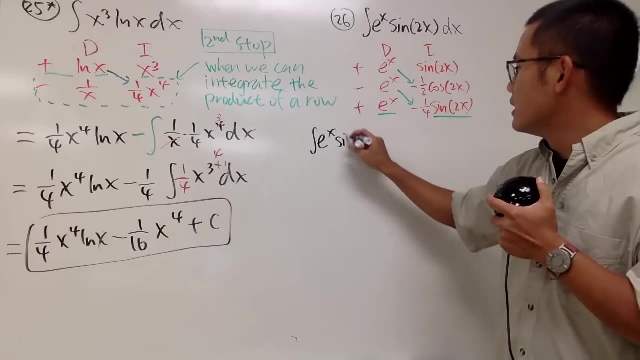 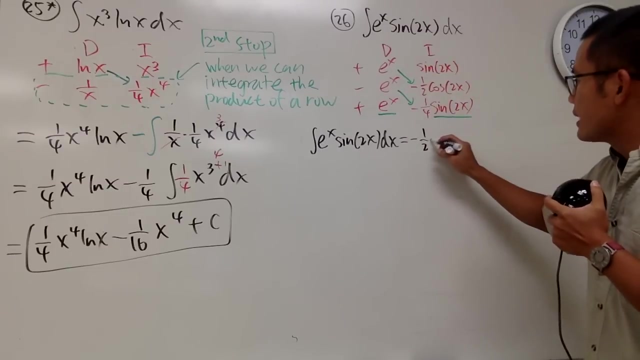 man, I don't have enough space. let me just try again. you guys will see why. anyway, let's do this times this, which is- I will write it down again- integral of e to the x. okay, okay, this times, this negative one half e to the x, cosine. 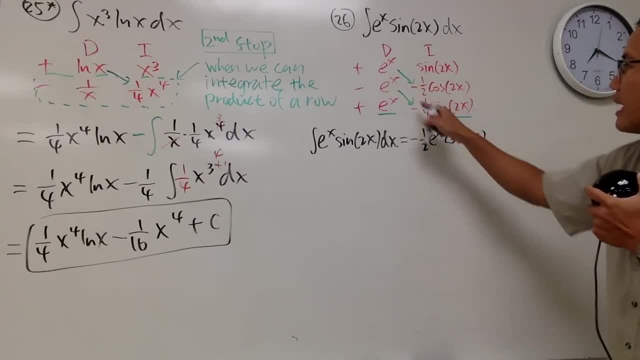 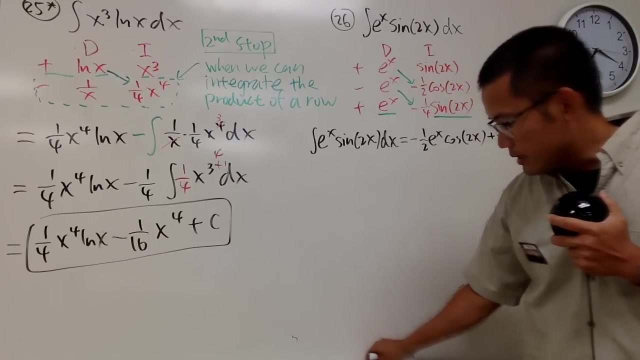 of 2x and then this times that negative times negative is plus 1 over 4 e to the x sine of 2x. lastly, well, we don't have a diagonal anymore and the thing is we have just put this down right. this is a. 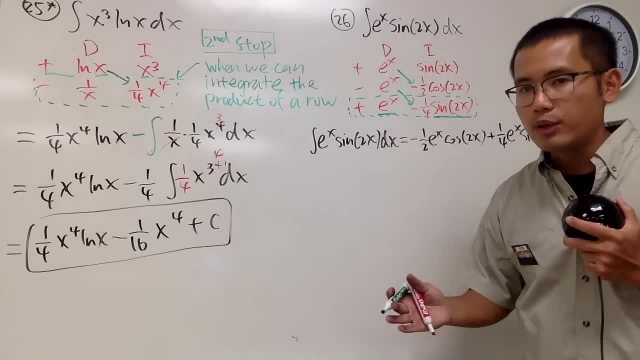 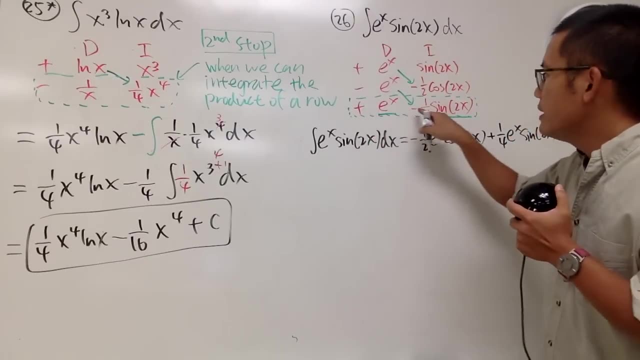 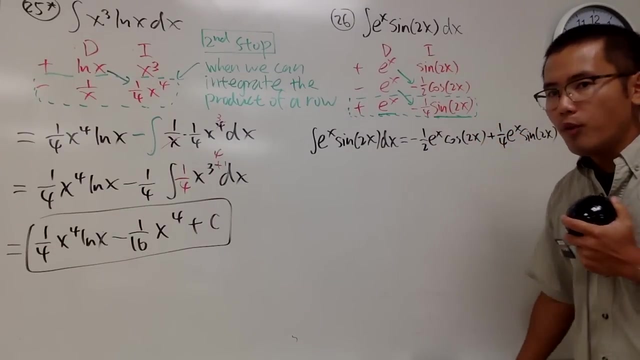 positive, this is a negative, this is a positive, this is a negative, and this is a positive and this is a negative. so we have a negative and we have a constant multiple, namely 1 over 4. so let's put down 1 over 4, right here. 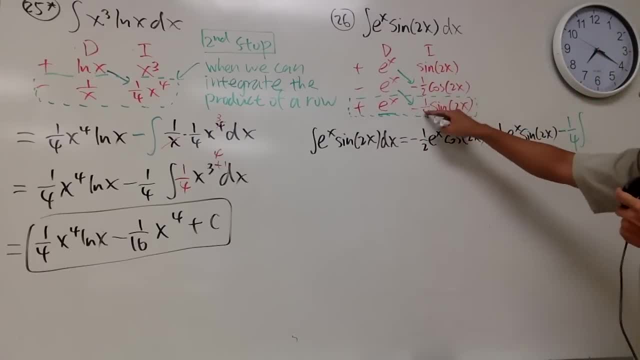 and don't forget, we still have an integral right. so again, the constant multiple is just put in the front and of course inside, here we still have e to the x and also the sine of 2x. the functions stay inside and of course we still have the dx. 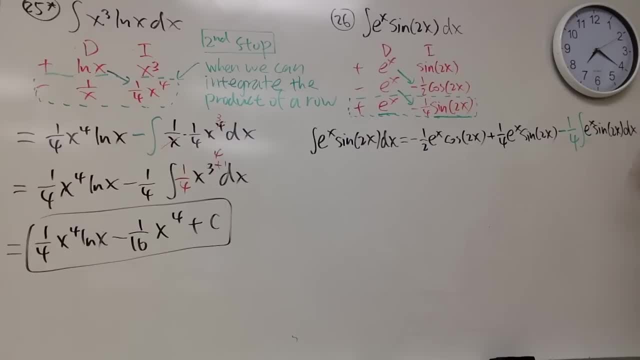 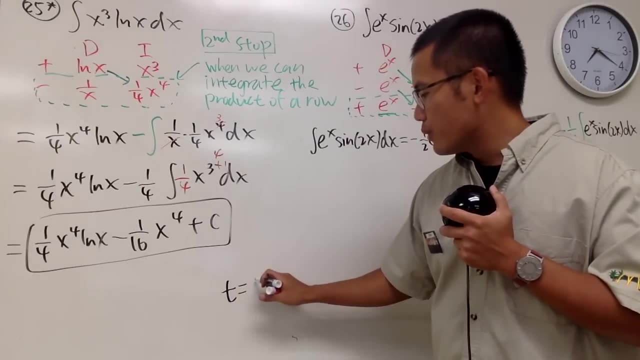 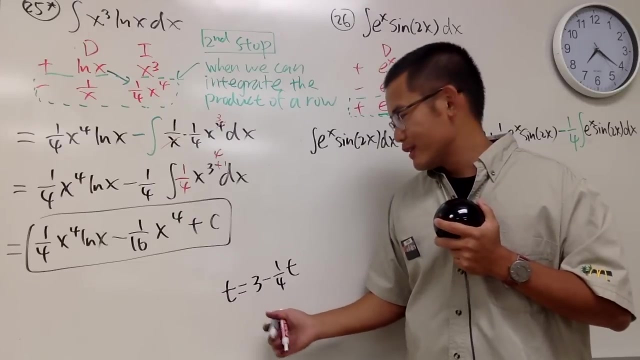 right here. so this is the idea. and now let me just ask you guys a question back in the day. suppose you have, let's say, t is equal to 3 over 4 t like this: how would you solve for t? well, first of all, you can just add: 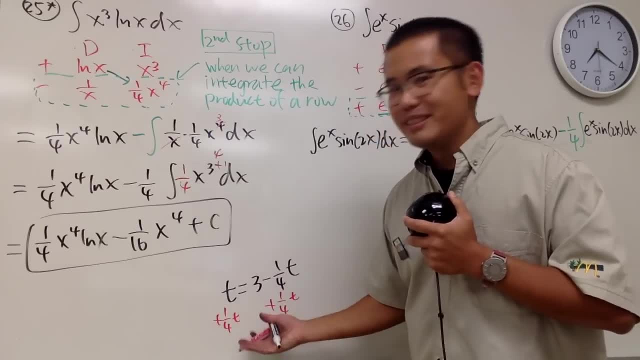 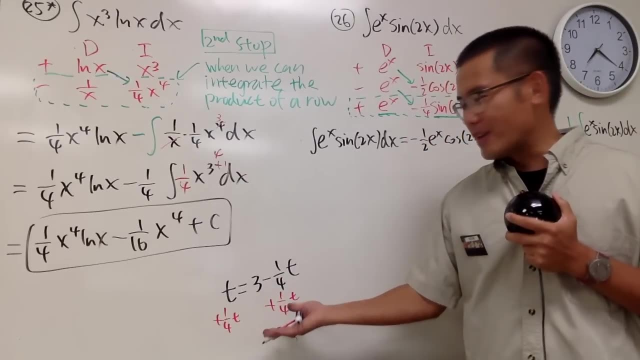 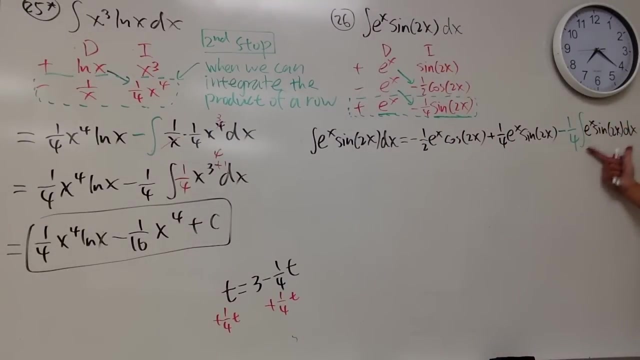 1 over 4. t on both sides, isn't it? well, don't you guys miss this day, because you can just do this and you can get like 5 points on the test already and now notice we have this integral right here and we have minus 1 over 4. 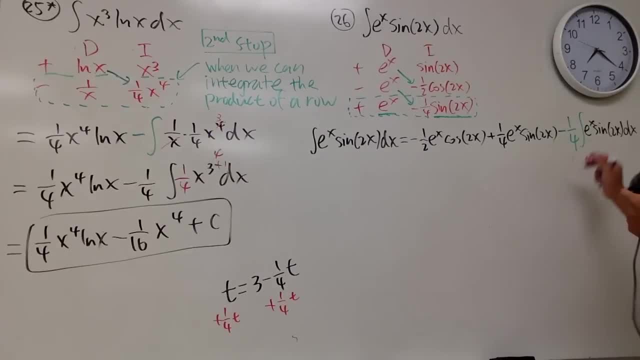 of the same integral. so this is the repeating situation and all we have to do is just go ahead and add 1 over 4 of the integral e to the x sine of 2x dx. on both sides. put 1 over 4 integral e to the x. 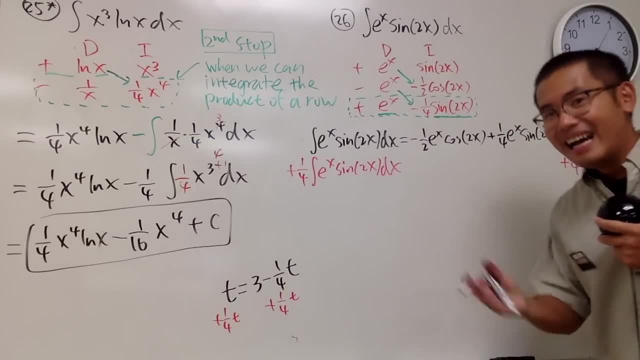 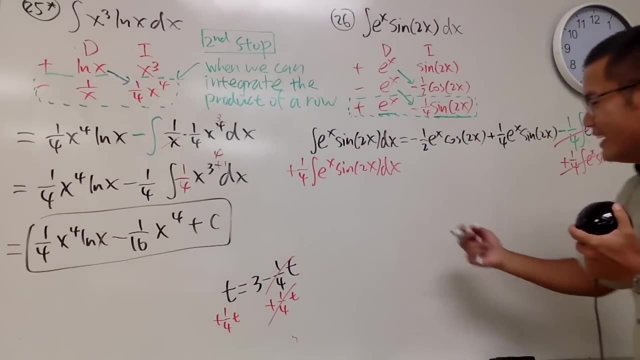 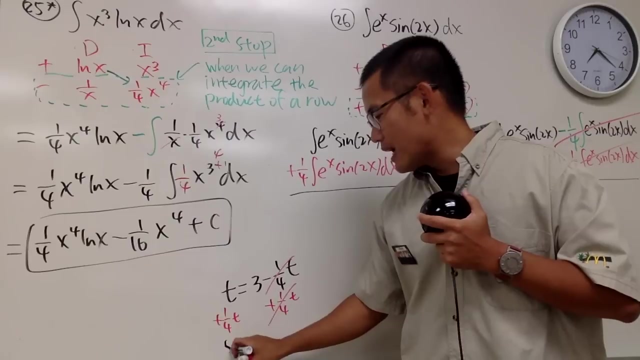 sine of 2x dx on both sides and notice this and that will cancel out, just like this right here. very nice, so we'll see that of course this is 1t plus 1 over 4t is just 5 over 4t. 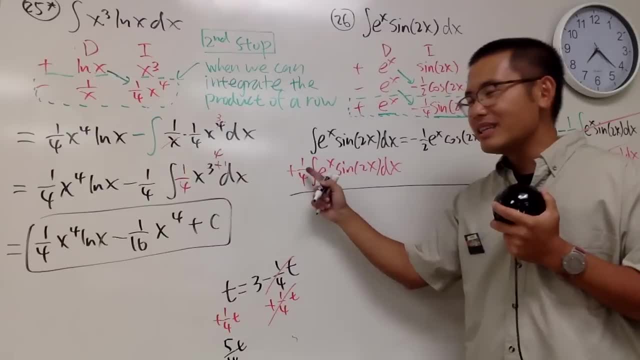 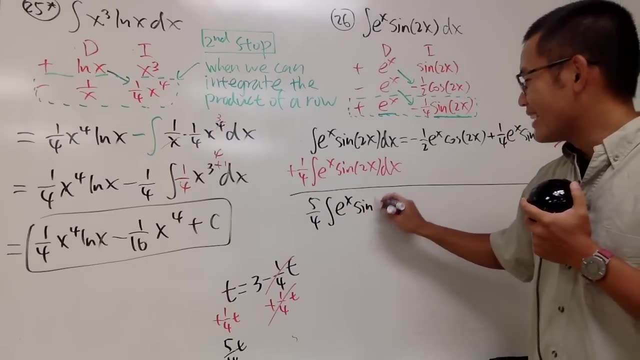 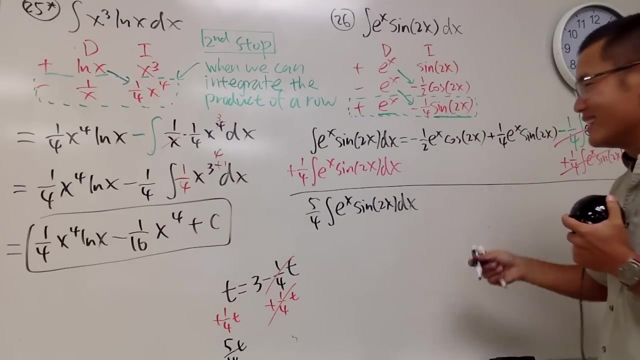 well, in this situation we have 1 integral plus a quarter more, namely we get 5 over 4 integral of this test, right e to the x sine of 2x, dx. yeah, and this two things. that's just the part of the answer, so let's just write that down. 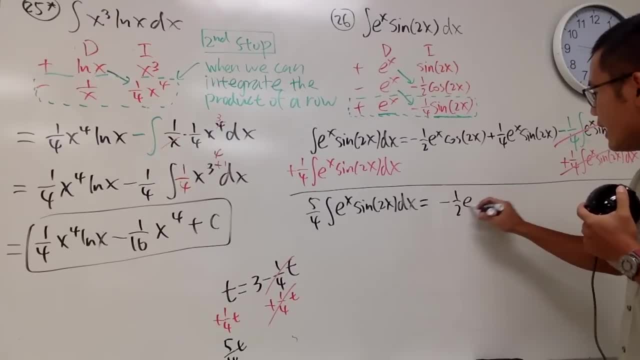 this is equal to negative, 1 over negative, 1 over 2, e to the x times 2x, and then we add it with 1 over 4 and we have e to the x and sine of 2x. yeah, and do I need to? 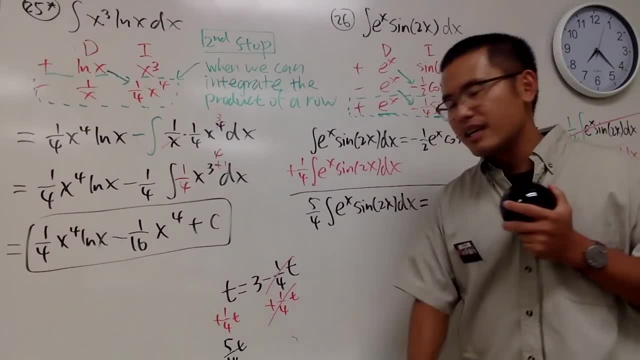 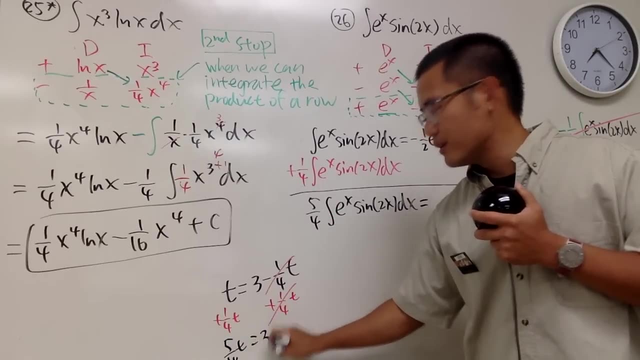 do I need to put down a plus e right here? no, not yet, because we're actually not done yet. we don't want the 5 over 4, just like when you have 5 over 4t is equal to 3. we don't want that. 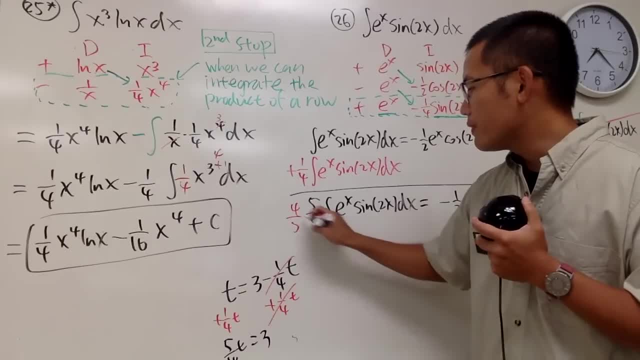 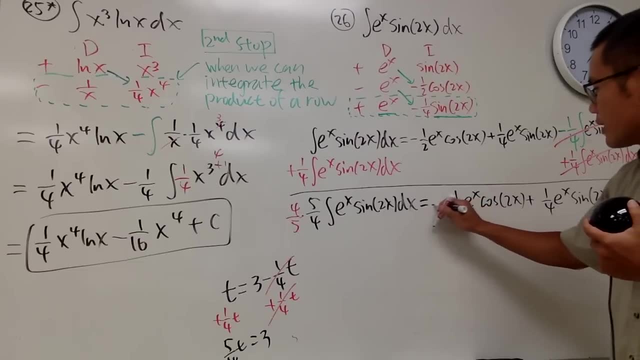 in this case, what do we do? just multiply everybody by 4 over 5. multiply this by. multiply this by 4 over 5. multiply this by 4 over 5. so let me just actually put it down like this: multiply this by 4 over 5. 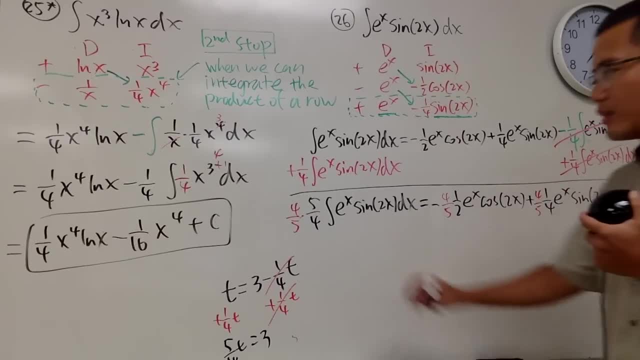 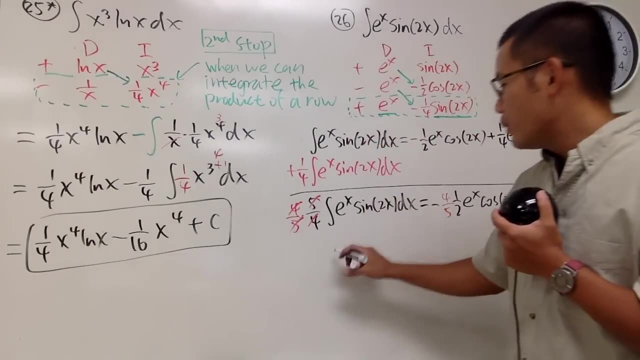 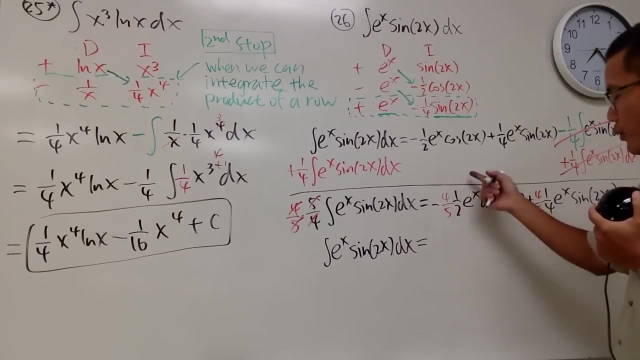 that's multiplying. multiply this by 4 over 5, so that this and that, this and that, this and that cancel. very nice in the end. ladies and gentlemen, here we have the integral e to the x sine of 2x, dx equals. work this out, of course, reduce the fraction. 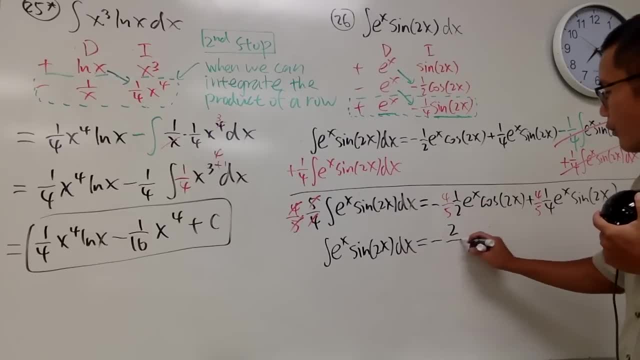 if this and that cancel, you get 2 on the top over 5 e to the x and cosine of 2x and 4 is cancelled. so we get plus 1 over 5 e to the x sine of 2x and we are all done. 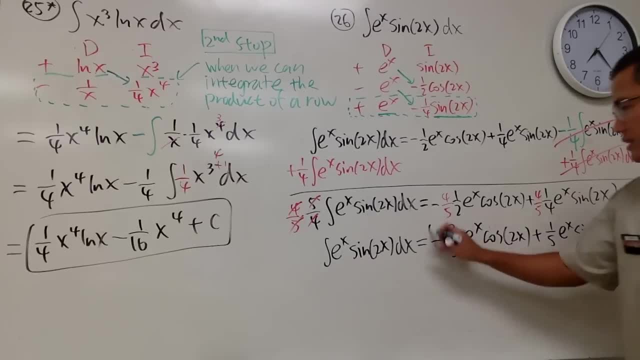 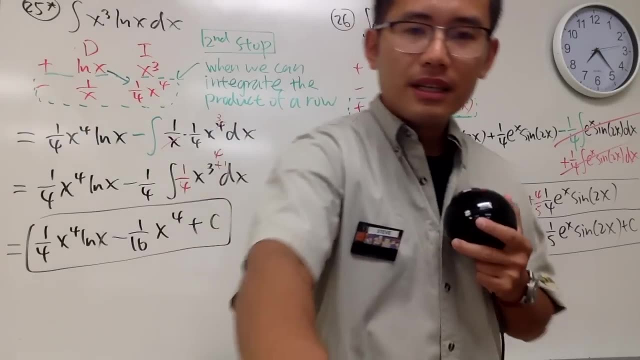 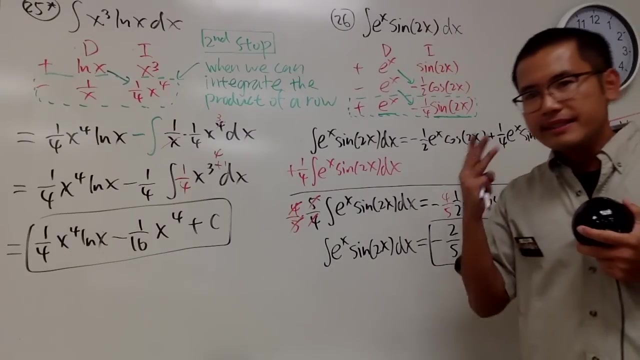 so plus c. this is it right? so that's it. and I do have the plus c, so that's legit. so this right here is the third stop, and let me write this down right here for you guys. for the third stop again, you are going to pay attention to the. 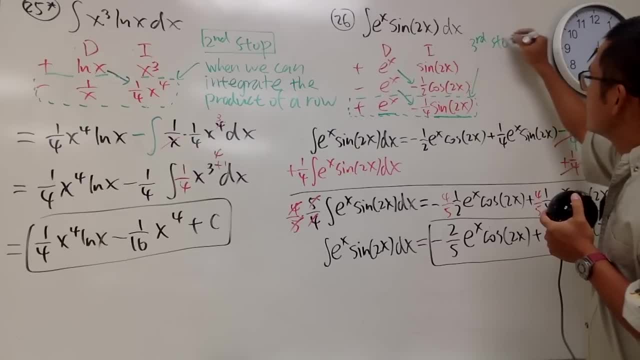 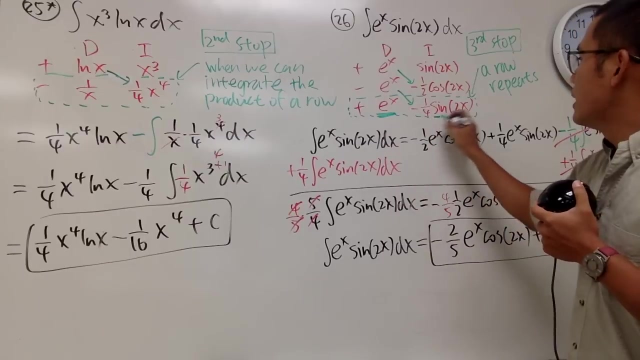 row third: stop, right, third, stop. and to keep this simple, I will just tell you guys, when the row repeat, repeat again. we are just focusing on the function part. right, the function part. the constant multiple is meant to be in the front of the integral. so this is what I mean by. 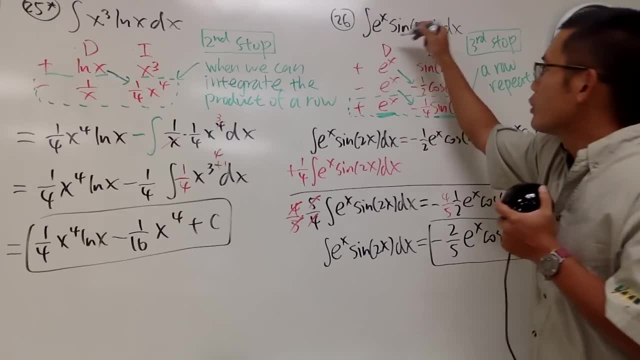 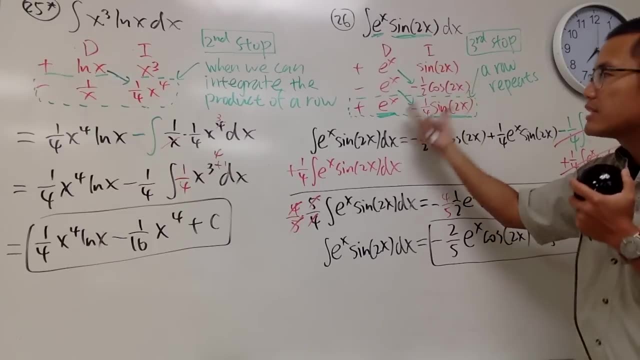 when you see a row repeats from the original, because originally we had the x, we had the e to the x and also sine of 2x: e to the x, sine of 2x. that's why we stopped it. right here, right and again anytime you want to. 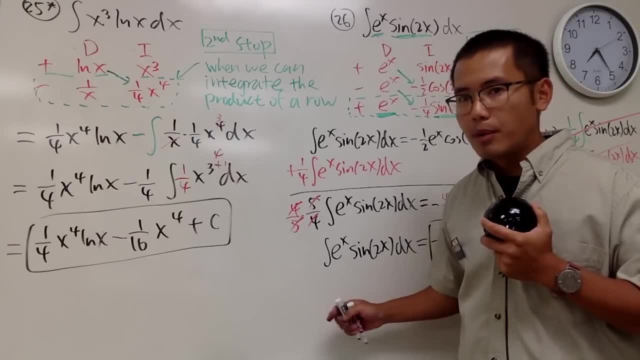 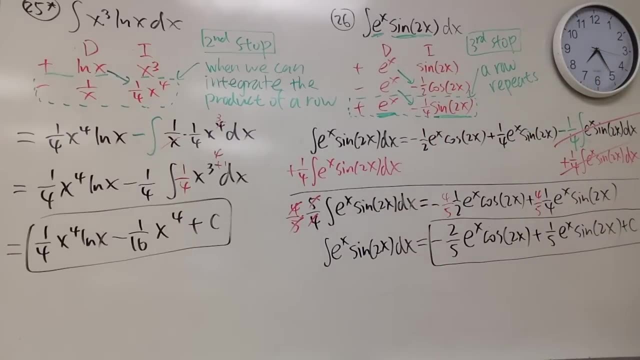 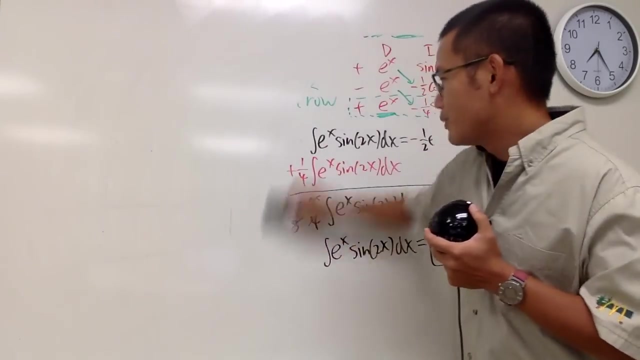 anytime, when the integral is meant to be done with integration by parts, you can use the di setup, because it's just the easier way to set up the udv. that's the idea, right? so take a look, take a look, take a look. yes, good, so now. 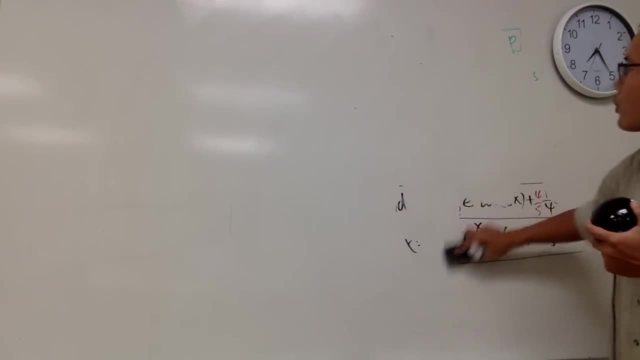 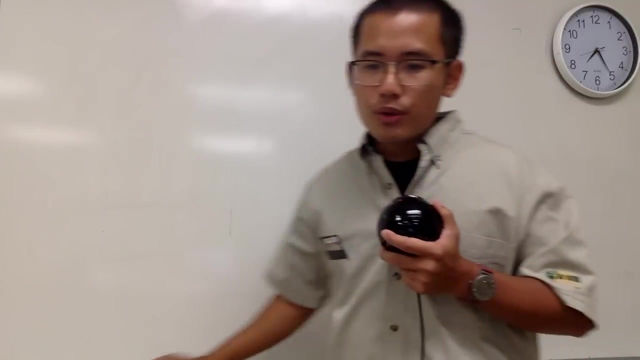 we're really talking about the calc 2 part, like the integration by parts is usually done in calc 2, unless your calc 1 teacher also mentions that. and now we're just going to do some more examples with the integration by parts. right, and let's do. 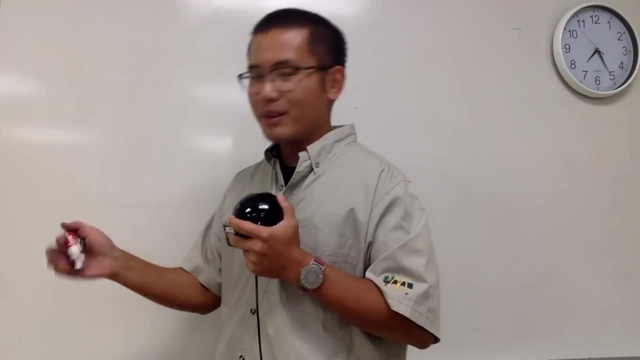 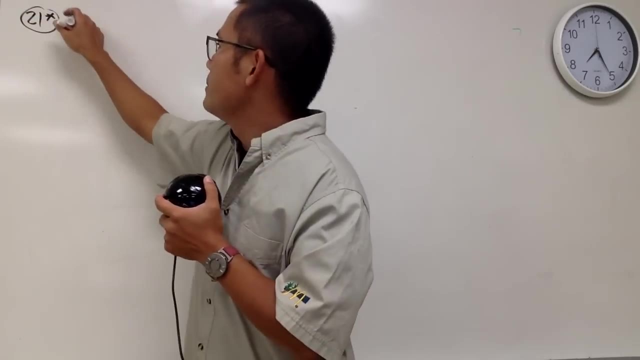 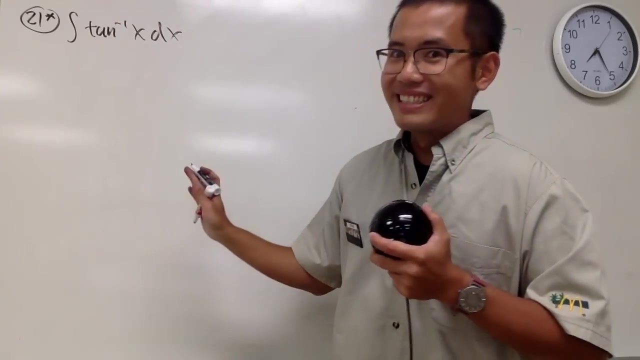 one of the questions that we saw earlier and we haven't talked about it yet, so this is question number 21. right, revisit it. name the integral of inverse tangent of x, dx like this: well, the answer is not: 1 over 1 plus x squared. that's not an answer. 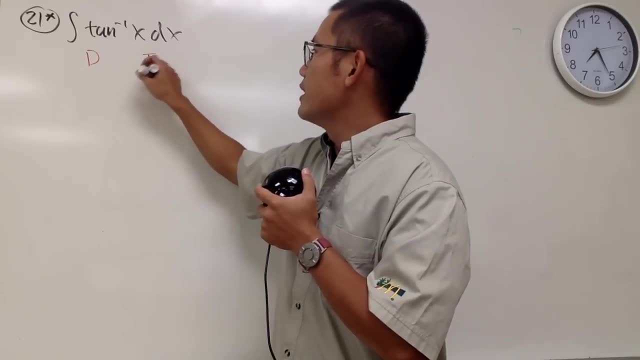 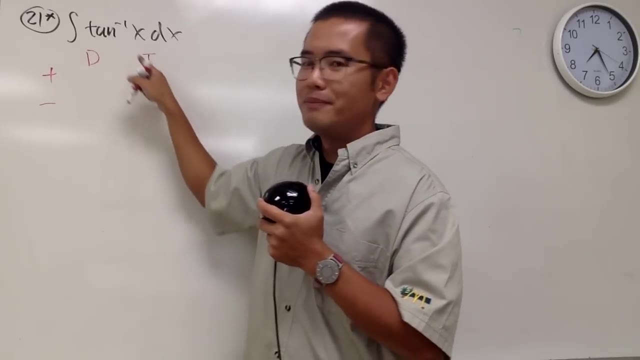 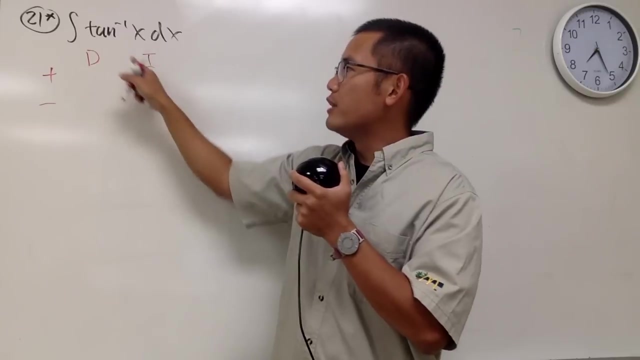 here's how you do it: differentiate, integrate right plus plus minus on the side, just to get ready. well, should I put down? I shouldn't, of course. we are not going to put down inverse tangent right here to be integrated, because that's the original question. so in this case, 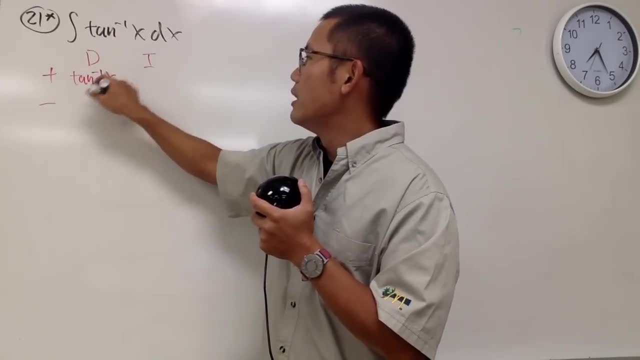 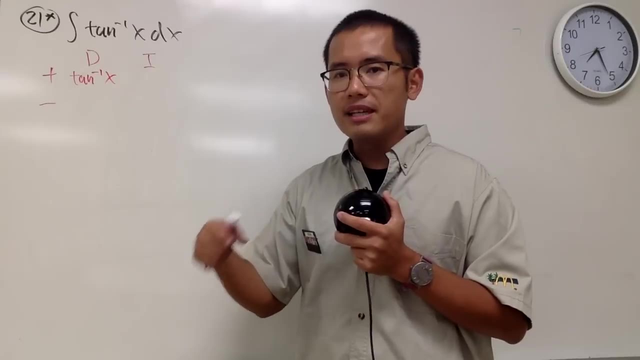 let's just go ahead and differentiate inverse tangent right here. and in that case, what can I integrate though? well, remember, we have the dx. it's kind of like 1 times dx or whatever. just put down 1. keep in mind we are in the x world. 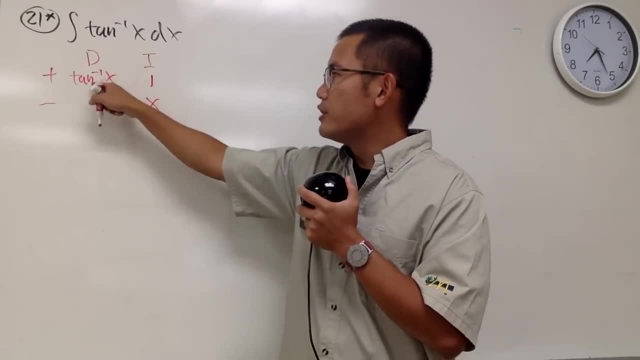 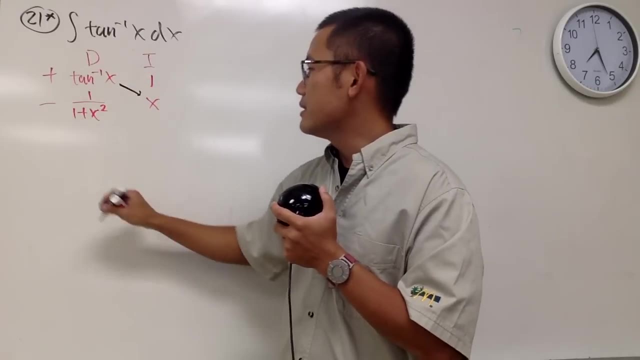 so let's integrate 1, which is x, and differentiate this, which is 1 over 1, plus x, squared, just like that. and now let's put down the answers together: this times this, which is going to be x, times that, and let me just draw my arrow in green. 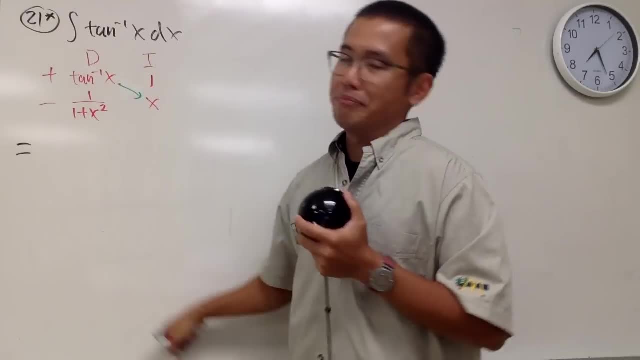 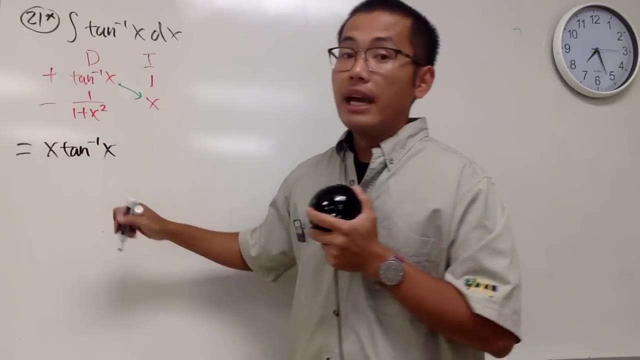 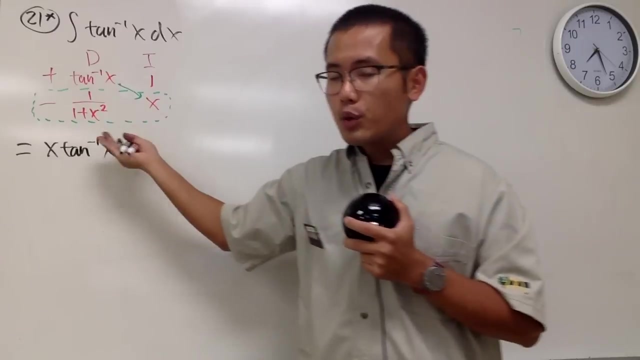 I know I don't have my blue marker. um yeah, so too bad, but anyway, this times this inverse tangent of x, and then we are going to multiply by this row and in fact we can actually integrate the part of this row. that's why we stopped it right here. 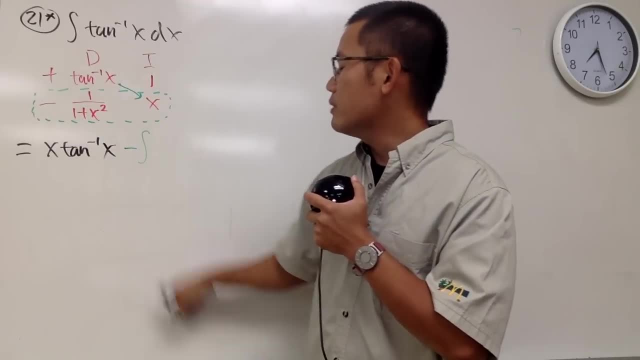 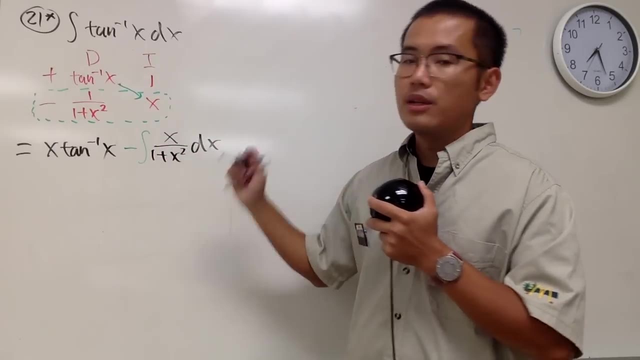 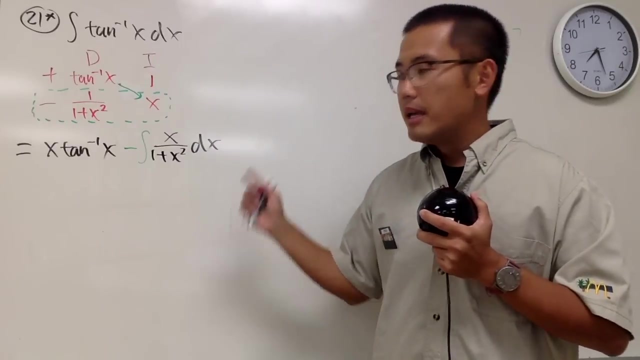 minus times positive, so it's a negative integral and we have x times that, so we have x over 1 plus x squared dx. right here? right, can we integrate this? yes, to do so. we can just do u sub, and by now you should be comfortable of doing u sub. 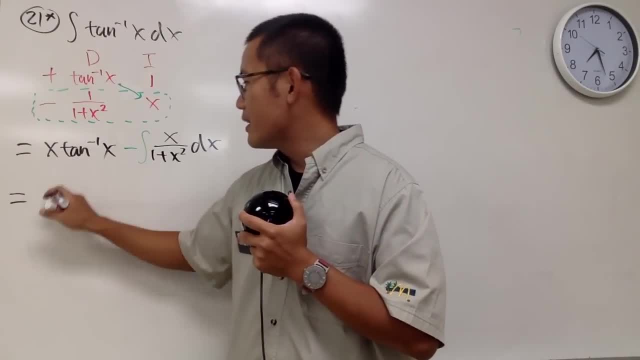 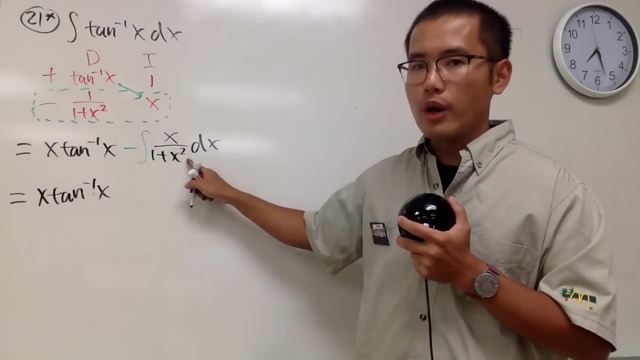 on your own. so I will leave that to you guys. alright, I will tell you guys that this right here is x times inverse tangent of x and you let u equal to 1 plus x squared, differentiate that you have 2x. but you don't see. 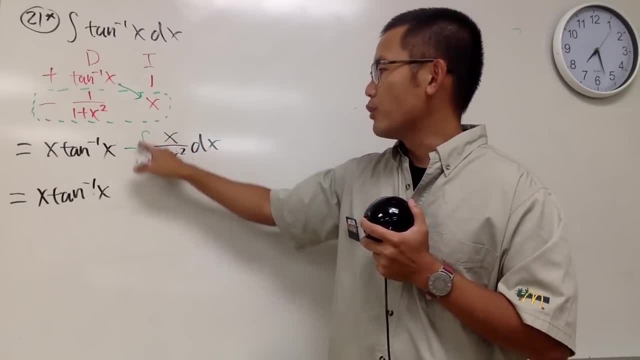 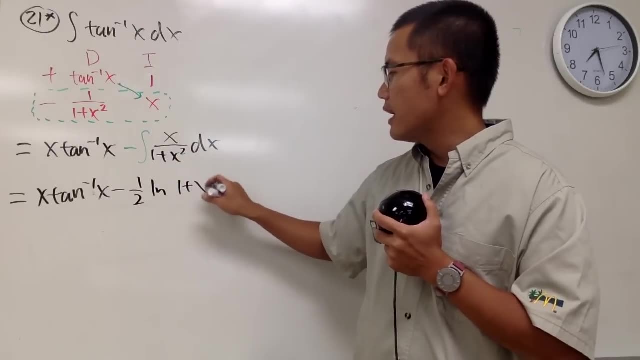 the 2, so you have to divide it by the 2, right? that's the idea. you can put down 2 and then work for 2. up to you to get the bottom, which is 1 plus x squared. but this is always positive, so parentheses. 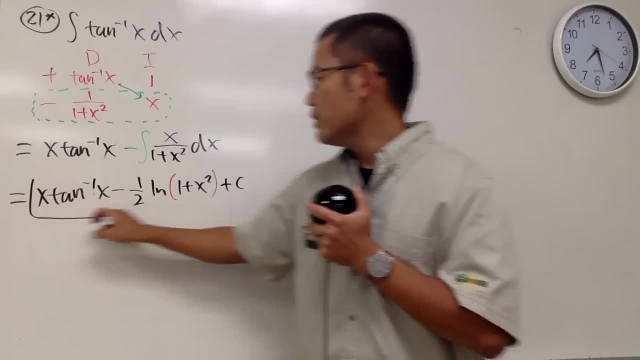 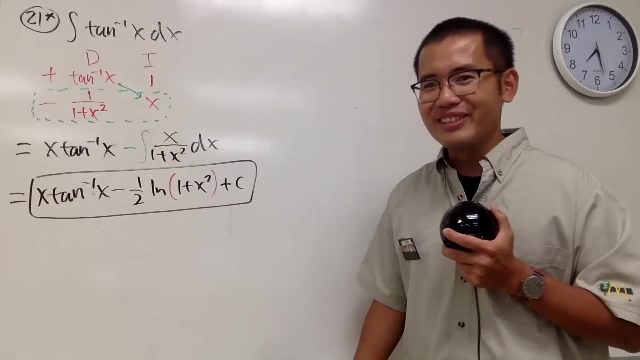 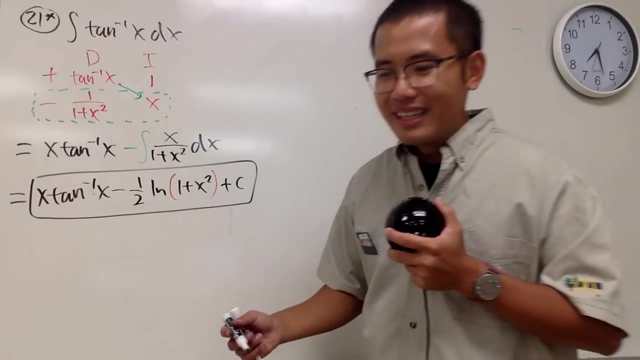 is enough, plus c. again, work out the u sub on your own, then u equal to the bottom. you should get that right. so that's how you get the answer for the inverse tangent, integral of the inverse tangent. ok, now, finally, I'm moving forward. let's look at: 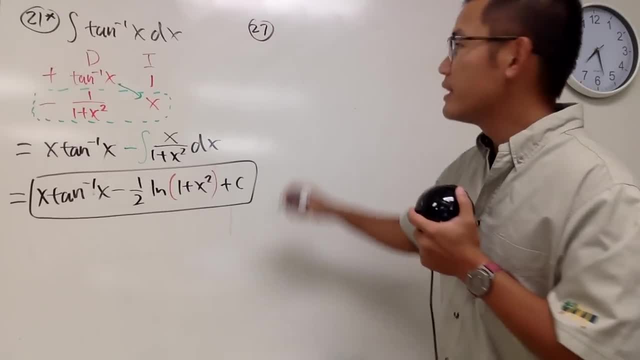 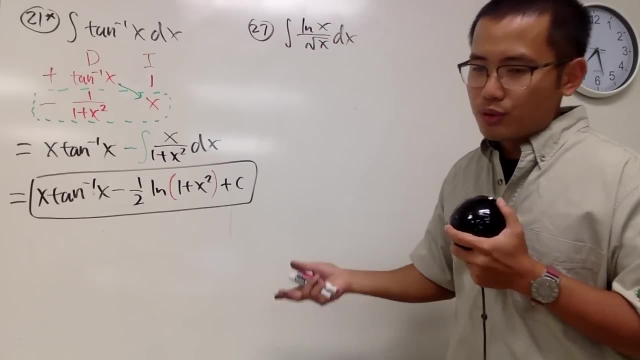 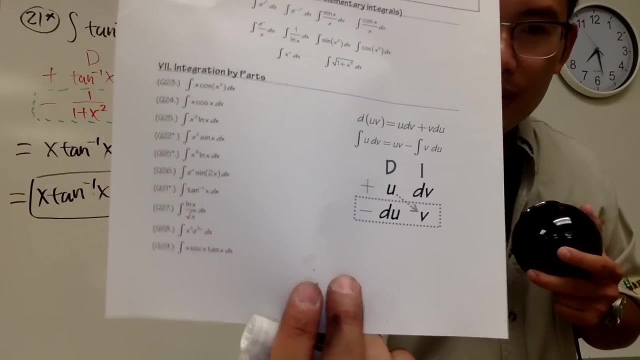 question number 27. alright, question number 27. let's look at the integral of natural log of x over square root of x, dx, and you actually should try this question on your own before you continue watching. you have the few more questions right here. alright, so 27,, 28,, 29. 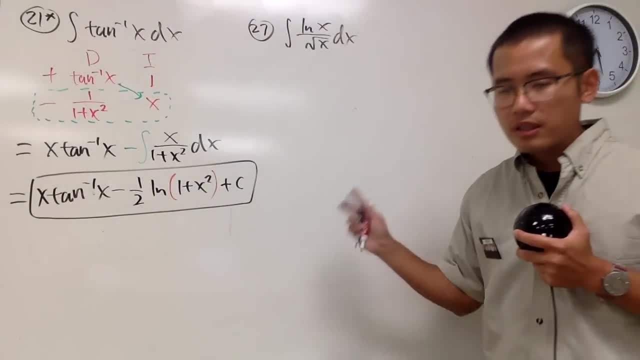 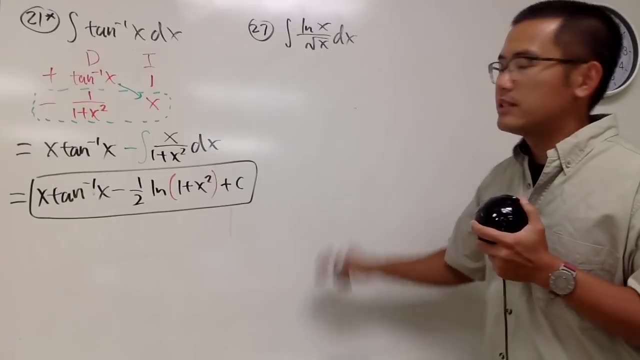 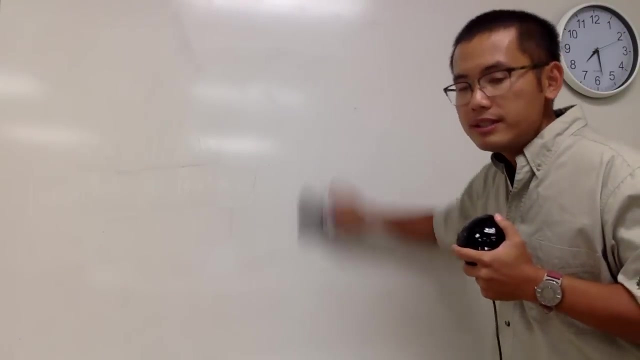 pause the video and just work out this on your own first and then continue watching. yeah, but anyway, let me just write this down. let's look at. actually, let's do this. you guys do the question now. alright, I'm going to erase the board right here and I'm going to write down: 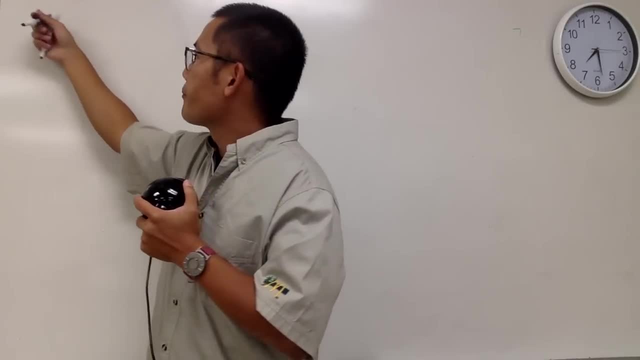 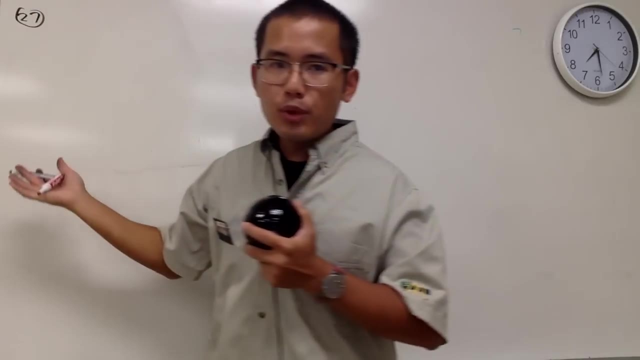 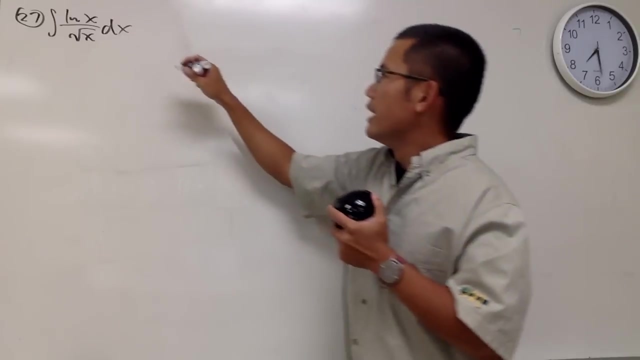 28 and 29 right here, right? so question number 27, 27. question number 27: we have the integral of natural log of x over square root of x dx, and then we have 28, which is x square e to the 3x dx. 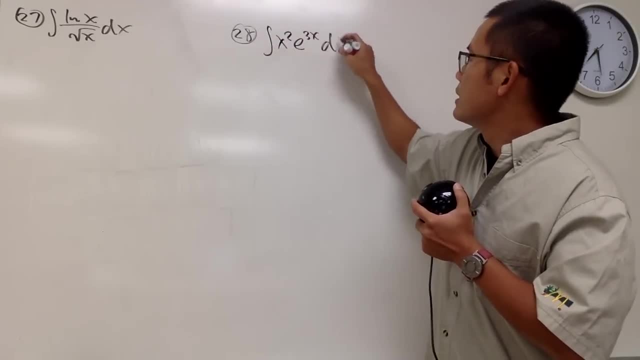 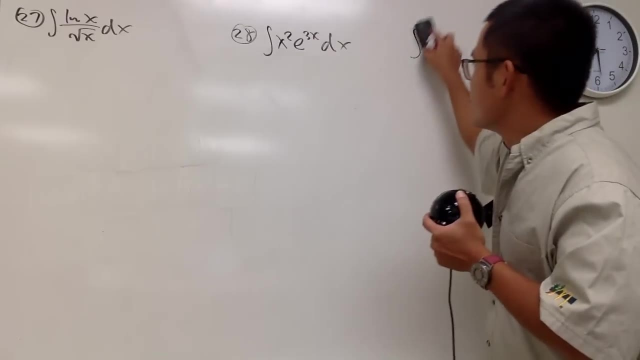 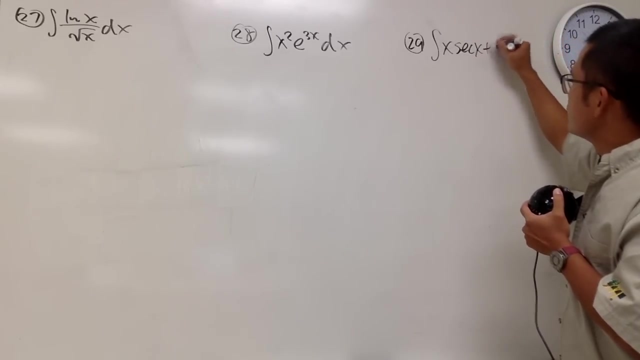 and lastly, we have 28, which is x, and we have- I mean I think some of you guys relate to do- the integral of three functions. let's look at 29: integral of x, secant x, tangent x, dx, like that, alright, so again try the questions. 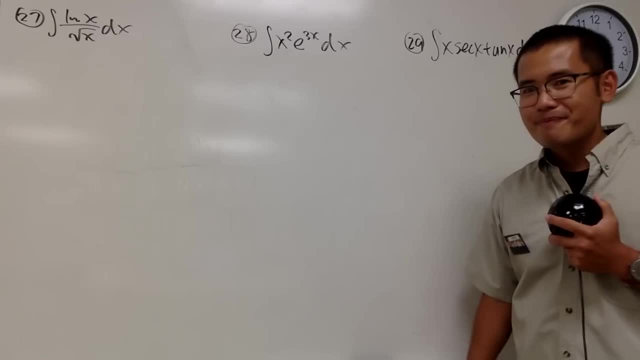 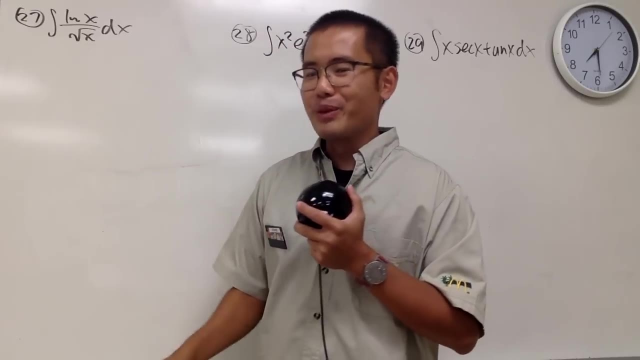 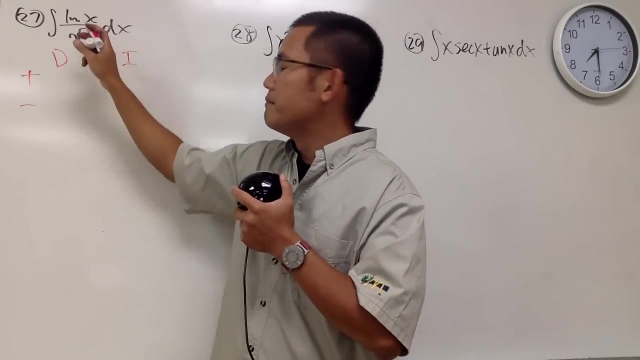 I'm going first before you watch the other solutions. okay, trust you guys. now let's do this one together for the first one. again, you know this category: just integration by parts d and i and a plus minus. we are going to be differentiating. natural log of x. 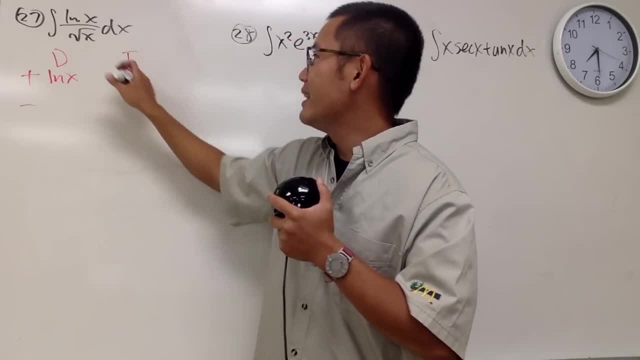 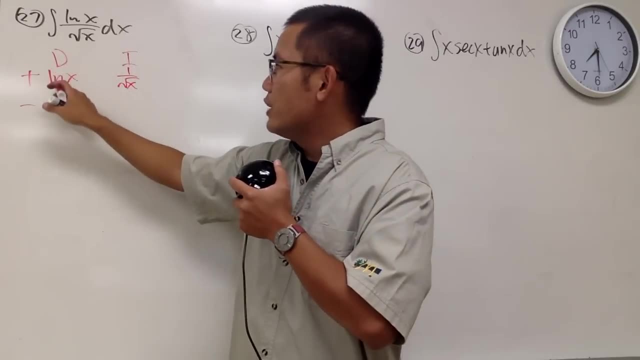 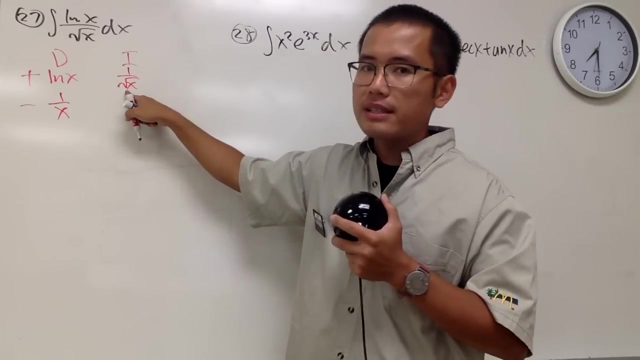 again: yes, because I can. we can integrate one over square root of x. everybody can do this. reverse power root: okay. differentiating natural log of x. we get one over x, integrating one over square root of x. this is that: saying x to the negative one, half power. 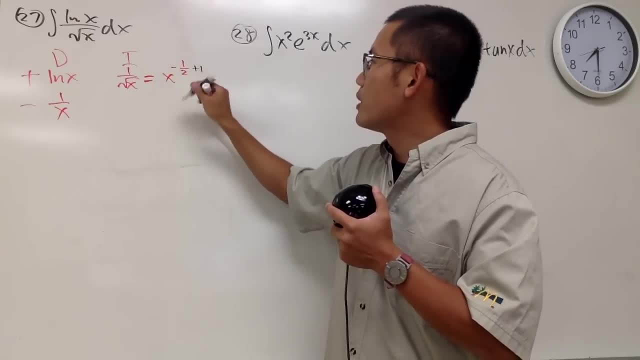 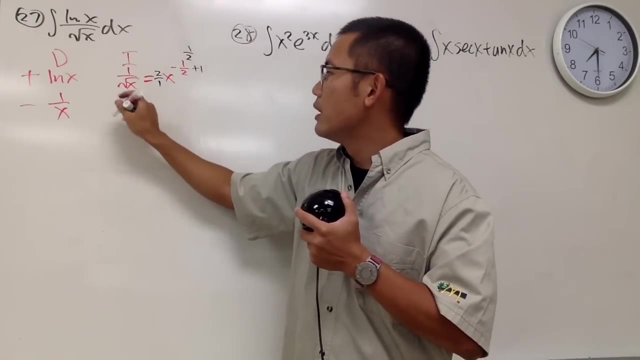 and of course do the reverse power rule. we are going to add one to the power and that will give us positive one half divided by the new power which is two over one. so we get two and we have x to the one half power right here. so let me just 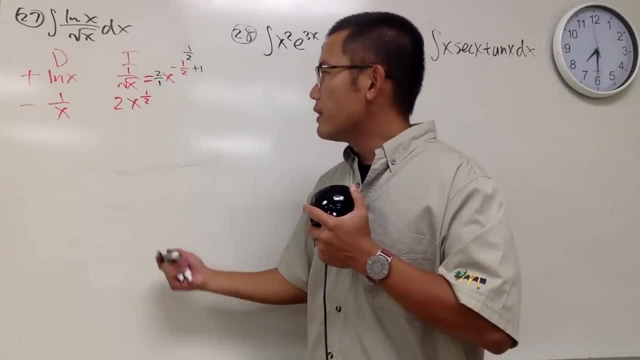 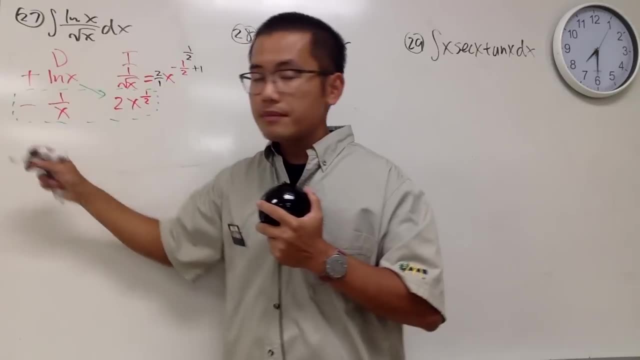 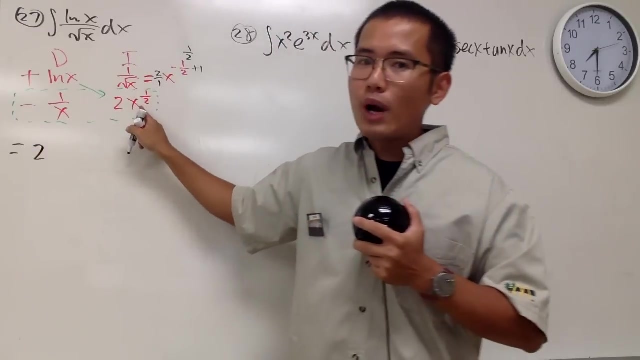 put this down. yeah, now we can just construct the answer. first of all, we are going to do this times that which is, and then we can actually get the integral of the part. so for the first part we get two, and let me just write the x to the one half power. 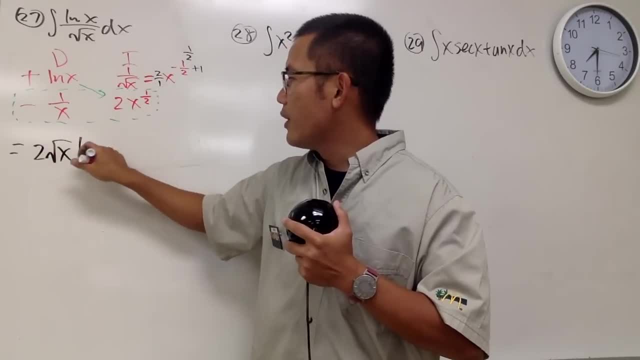 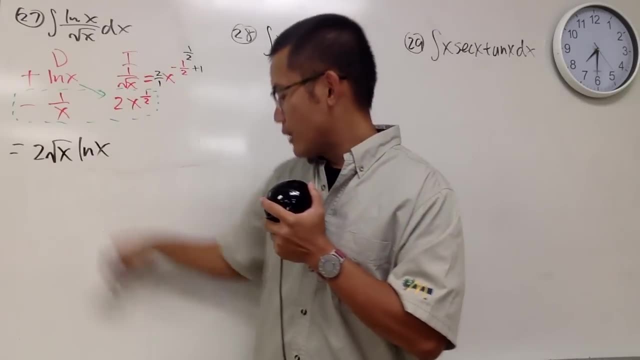 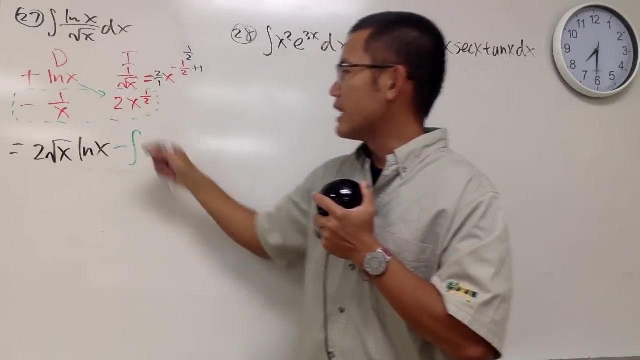 as square root of x right here, and then the ln of x. usually the ln of x is at the end. we have this and then we are going to have minus integral of this times that. so minus integral, and we will just do this times, that this time. 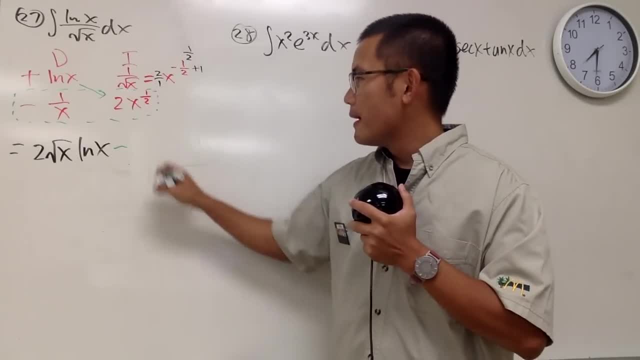 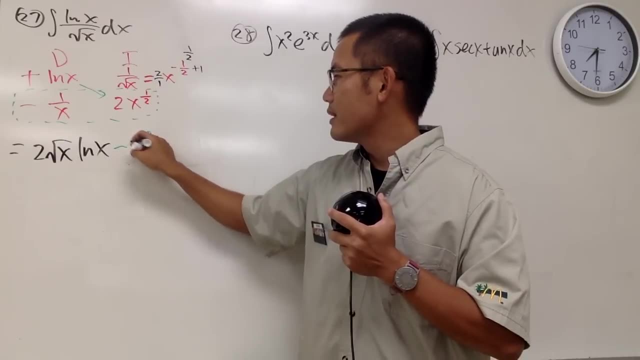 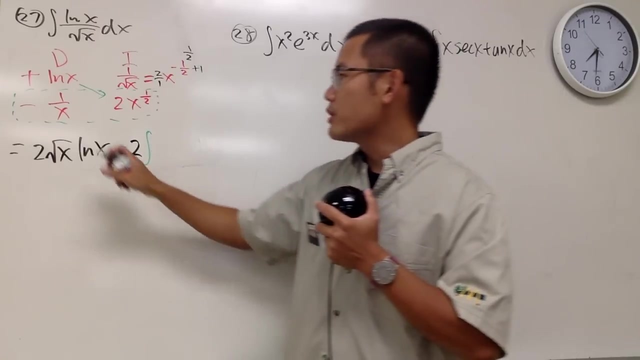 let's practice. let's just write down the integral like this: minus the integral, we have the two. let's put that down right here. let's put that down right here. and then we have one over x times x to the one half power. well, in this case, 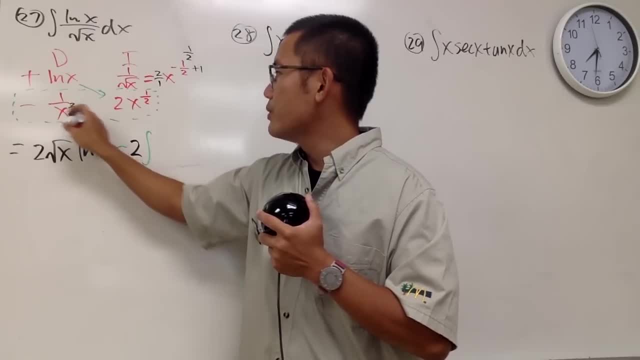 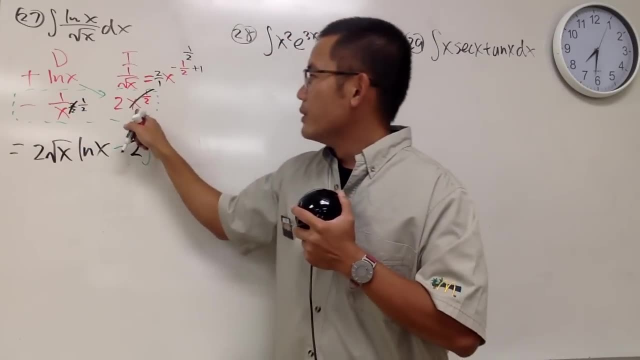 when we multiply, this can be cancelled. this is like two over two. so we can cancel this out and this becomes one over two on the bottom. so in another word, this times that will give us one over x to the one half power, and that's going to be. 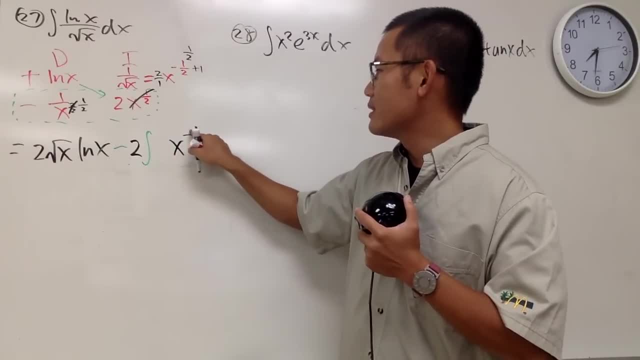 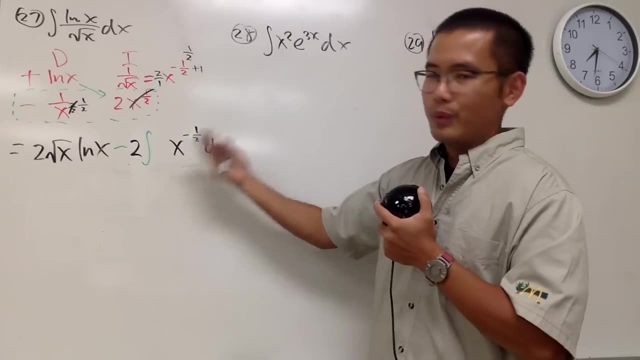 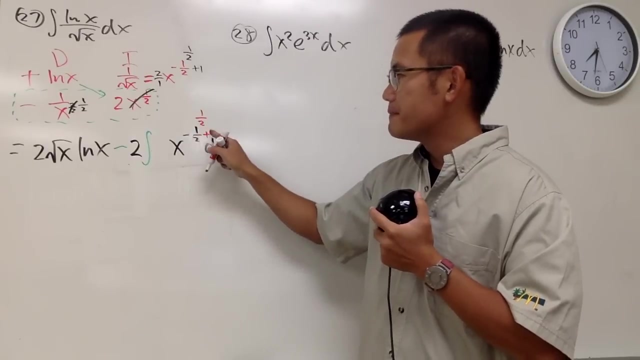 x to the negative one half power, like this, if you would like just do one half minus one, it's easier perhaps. so that's the idea and this one we can integrate, because we did that already. so we just add one which is going to give us positive one half. 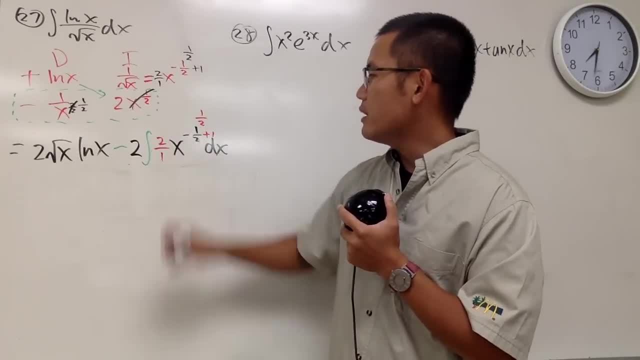 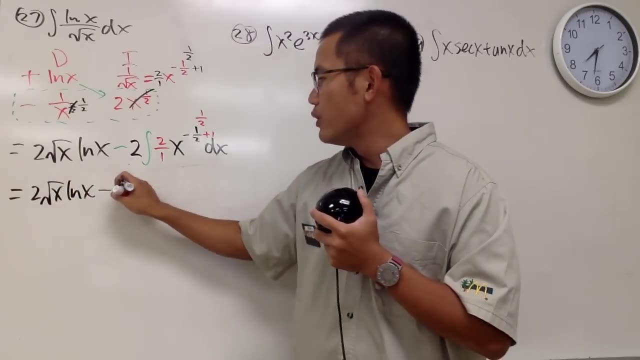 divided by positive one half is the same as multiplied by two over one. so multiplied by two over one, right here we get two, square root of x, natural log of x minus four. and then this is square root of x and we are all done so plus z. 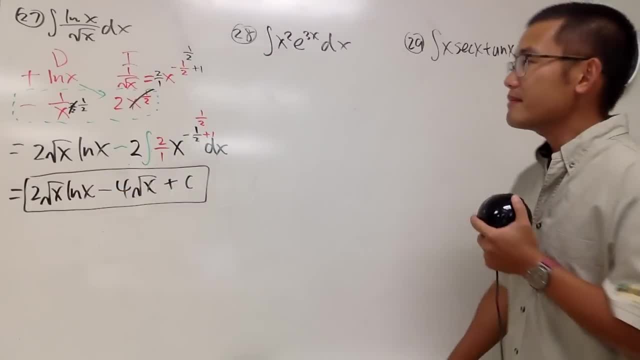 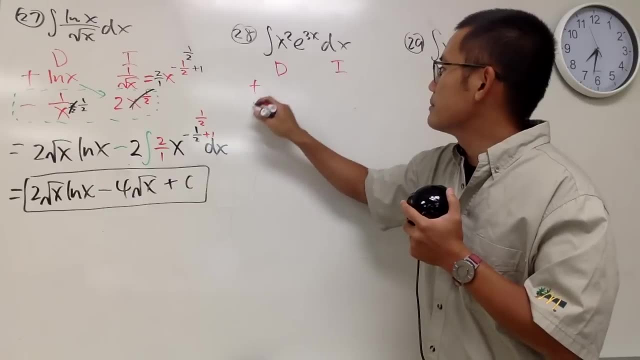 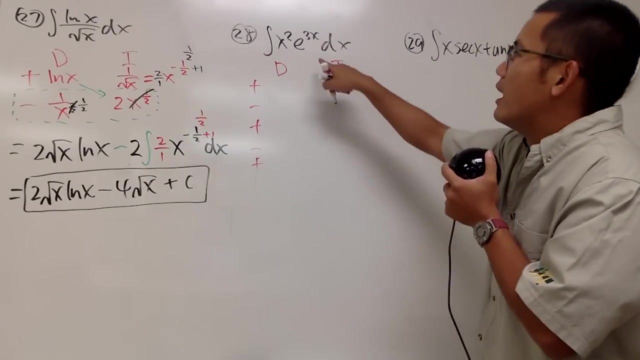 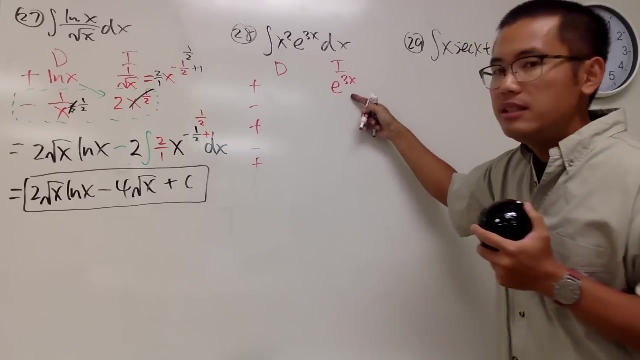 this, is it right? okay, question number twenty eight, of course, differentiating and integrating plus minus, plus minus. I don't know how many I cannot do, but like I don't know, anyway, I'm going to integrate e to the three x, because this is easily achievable and, in the meantime, 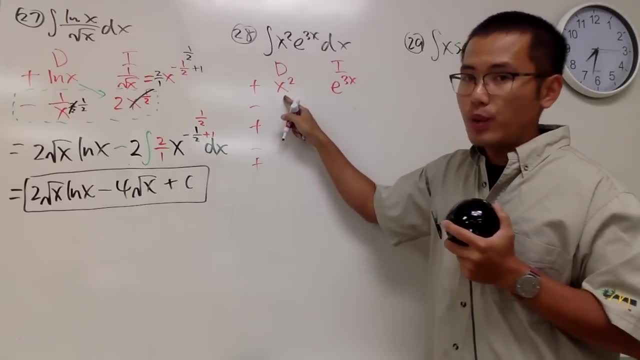 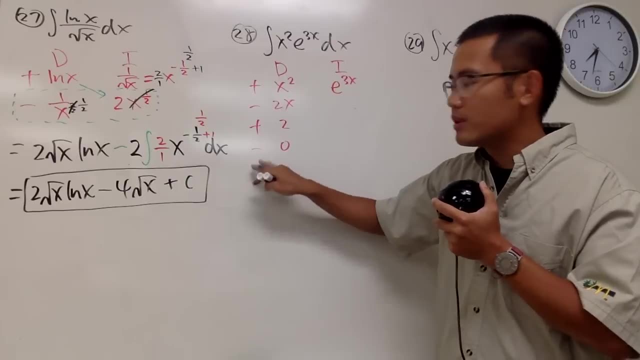 we can also differentiate x square, and this is great because we can actually make this equal to zero. differentiating x square, we get two x and then two and then zero, so we don't need the last row now integrating e to the something. this is going to be what. 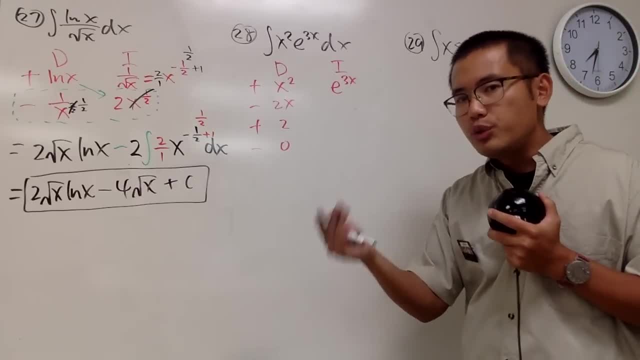 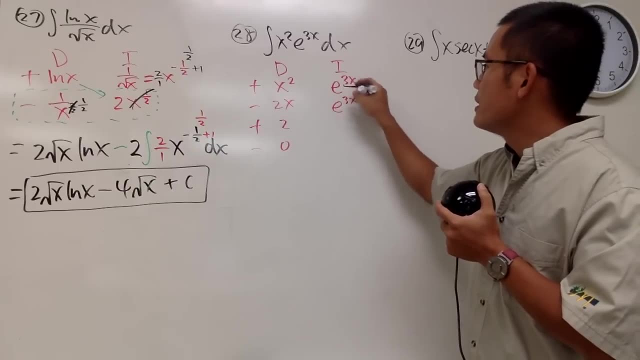 notice, we have three x. the derivative of three x is just a three. so, integrating this, we get e to the three x and we have to divide it by the derivative of this, which is three. so we have the one third here and then do it again: we have e to the three x. 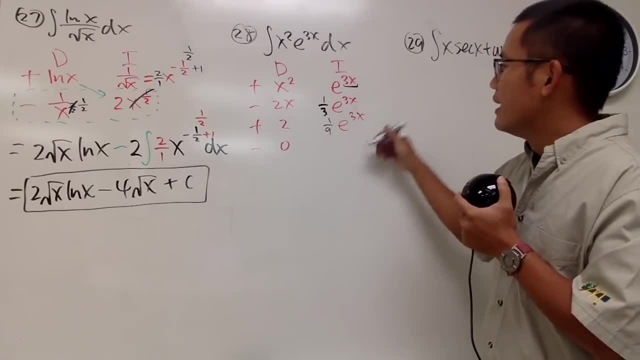 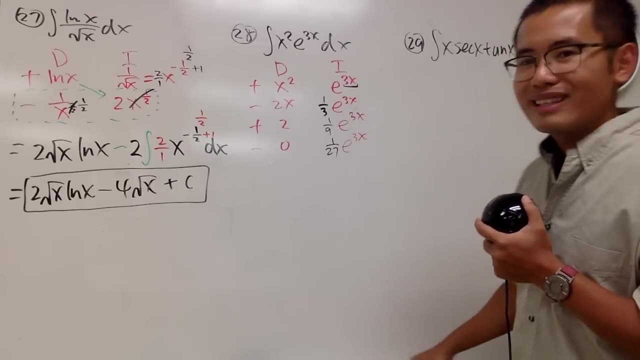 divided by three, again, so we get one over nine. do it again, so it's e to the three, x divided by three, so it's one over twenty seven, just like that. this is great, because for this one we're just going to multiply the diagonals and we have. 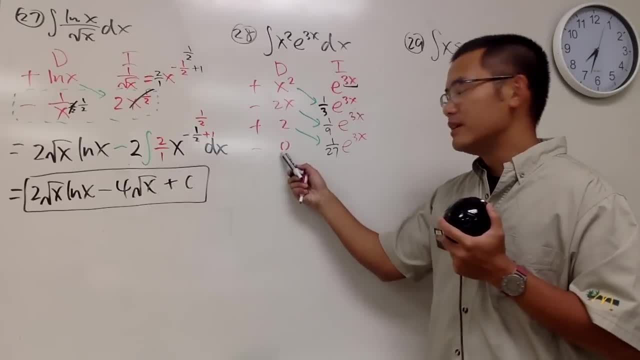 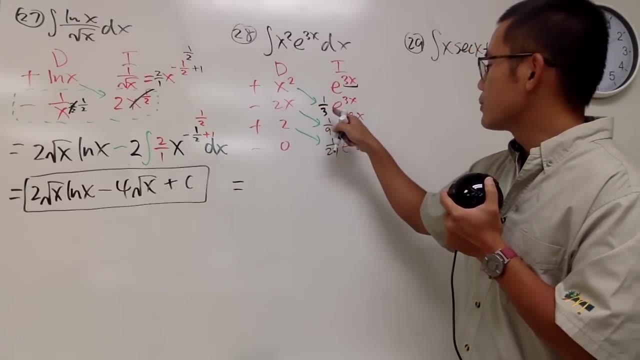 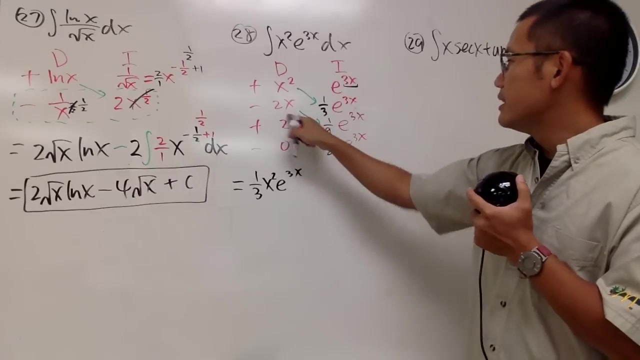 one, two, three, three parts for the answer. that's all zero times five, doesn't matter, right, alright? so finally, we see that the answer is x squared times that. so let's put down one third x squared e to the three x, and then this times that is minus two. 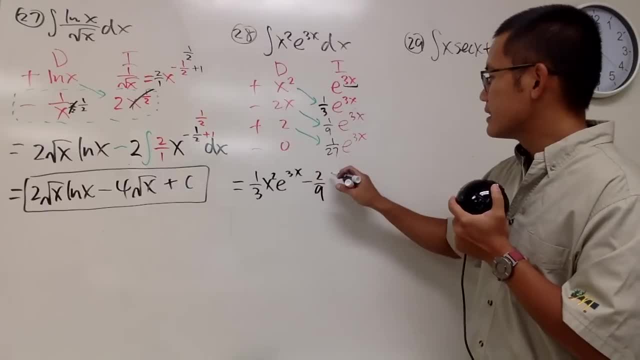 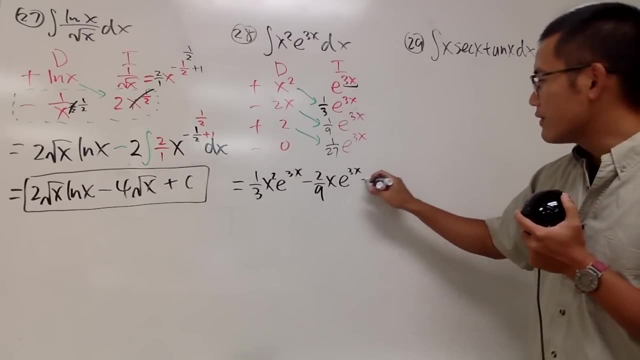 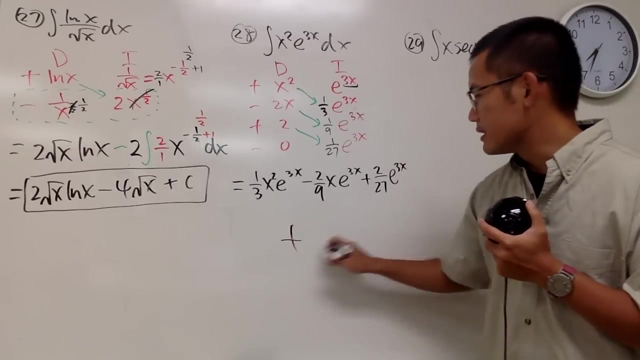 over nine, x times e to the three x and lastly, we have this times that which is plus two over twenty seven, and e to the three x, like this, and in the end let's just put down plus c, like this: yeah, and you might be wondering, 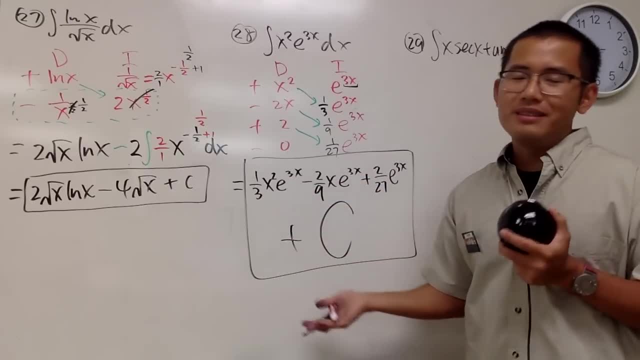 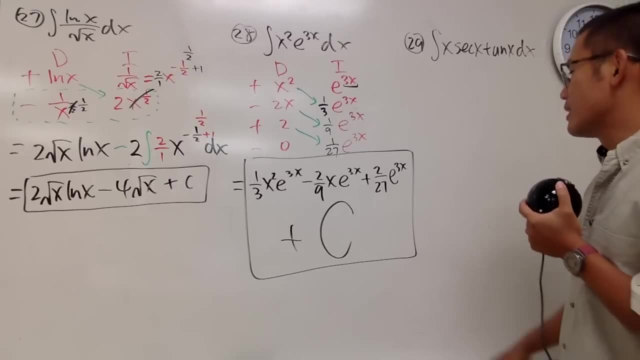 like: should I be factoring out the e to the three x? well, the answer to that is: it doesn't really matter, because if you factor it out, people will say: why don't you multiply it out? right, so it doesn't really matter that much. alright, for this one. 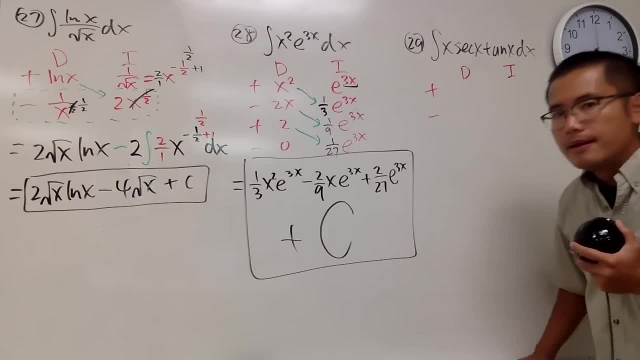 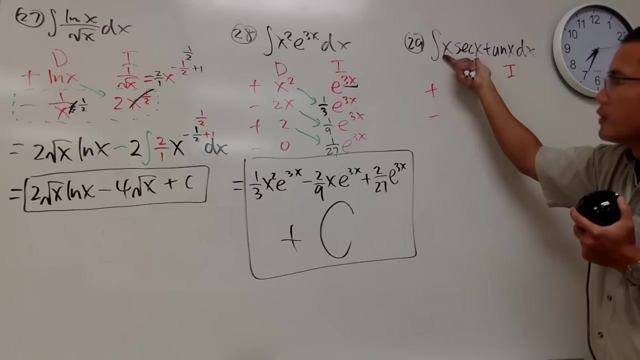 alright, d, and then i plus minus. well, so, um, i can integrate tangent x, but in the meantime that will make me differentiate both of this. that will just i will have to use the product rule that's not preferred. i can integrate secant x, but i will have to be. 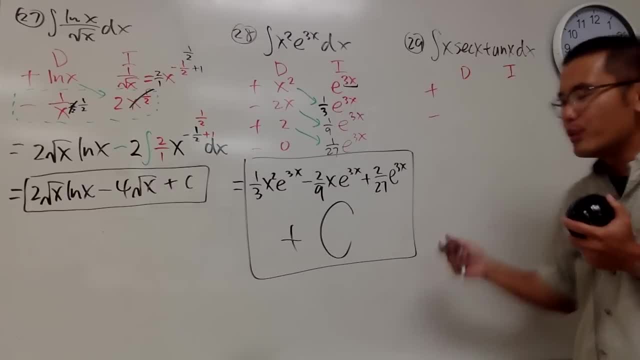 differentiate x and tangent x. that's not preferred. why don't we try to integrate this guy and that guy? because that's just as easy- integrating secant x times tangent x- and we can just differentiate x. How's that? This is still okay. this is the breakdown. 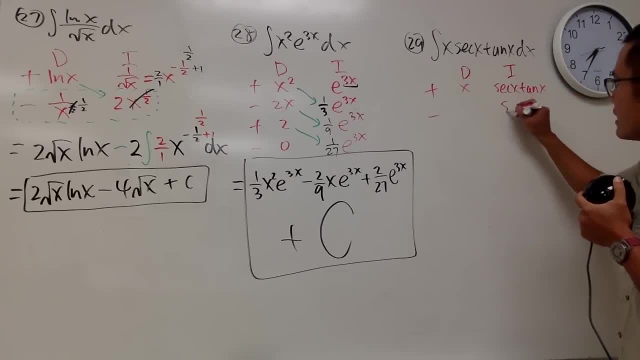 Okay, in this case, integrating this, we get secant x. that's good. Differentiating x, we get 1, that's great. Yes, You can just do the diagonal and then put this in the integral, but we can take advantage of that. just say: integral: differentiating 1 is 0,. 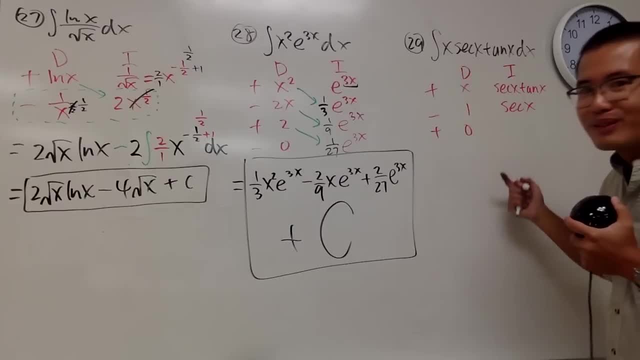 just do this integral right here so you can just do a diagonal. that's easier. Integrating secant, we get natural log absolute value of secant x plus tangent x. How do we know? Because we did that question already. Anyway, in the end, of course, we're just going to be doing this times this, this times that. 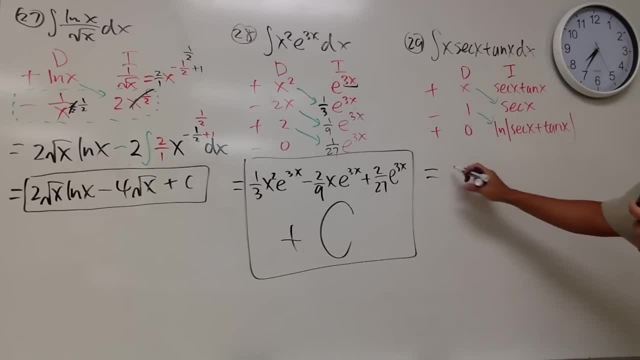 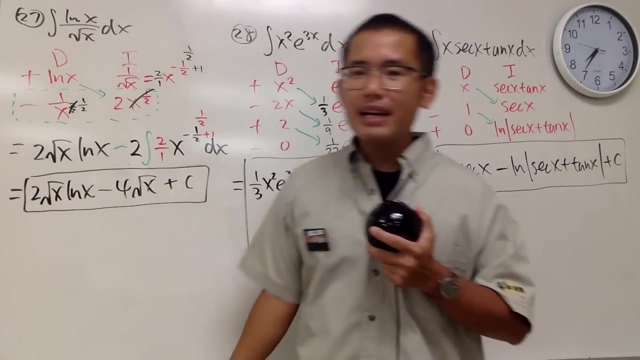 Alright. so here is the idea: We have x times secant x and then minus 1 times this, which is just natural log, absolute value of secant x plus tangent x, like this, And plus c, like that. And if you want to do minus c well, technically that's fine too. it's up to you. 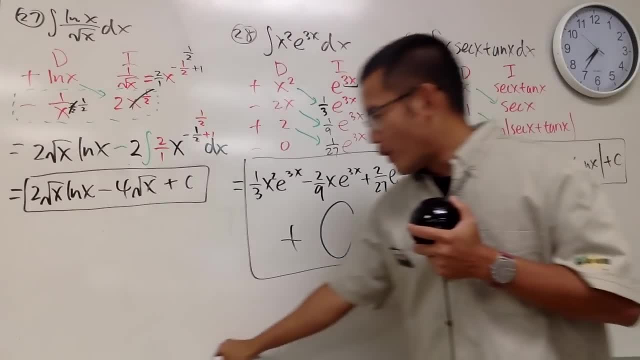 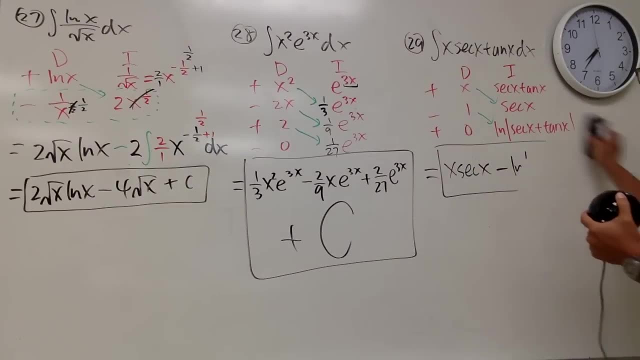 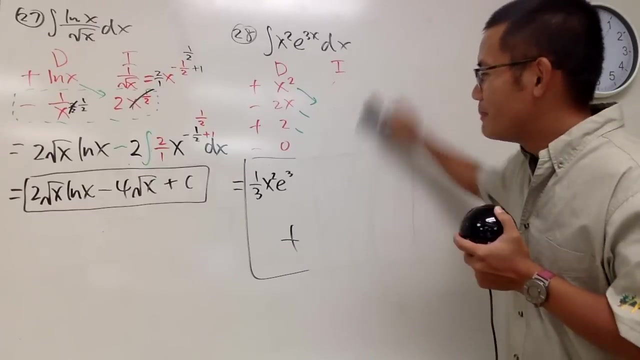 So this is taking quite a lot of time. this is, let's see, almost 3 hours, 2 hours and 15 minutes. Alright, let's see. That's why I wasn't so happy in the beginning, even though we did like 8 questions in like 10 minutes. 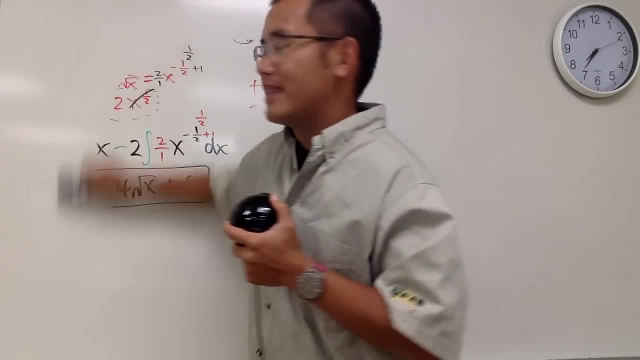 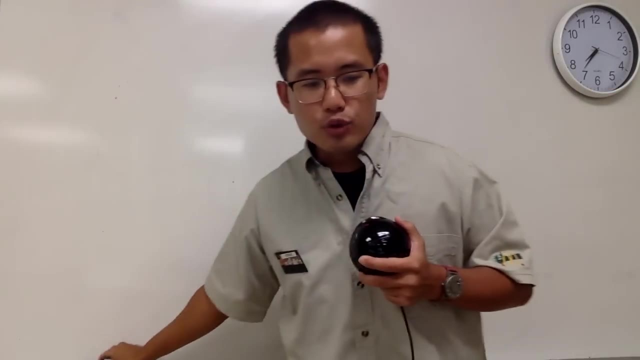 but I know I actually I knew like the longer part, the harder part, is this. But anyway, with that being said right here, that kind of concludes the integration by parts section. right Now we have a few more things to do. 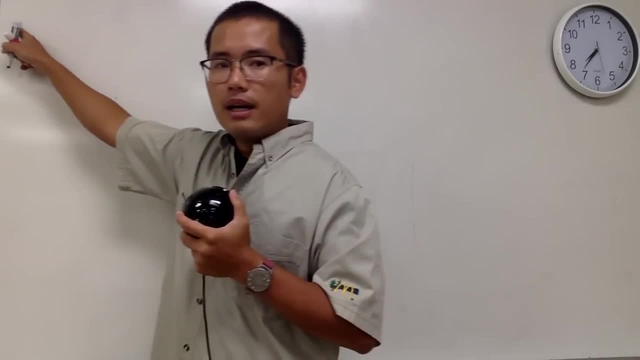 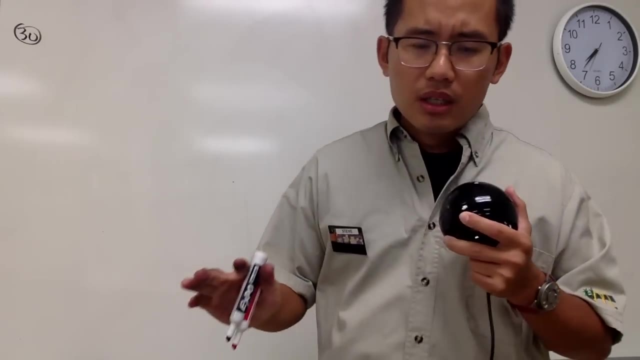 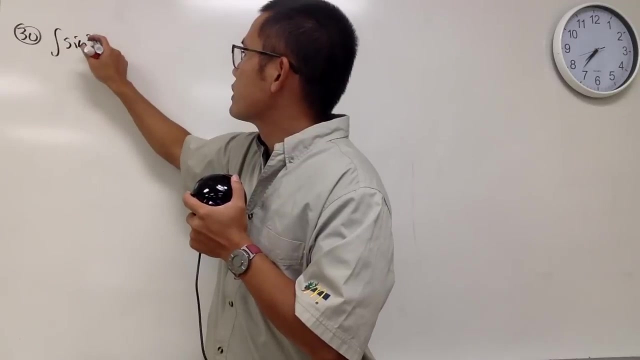 Let's look at question number 30.. And for this one, I'm just going to write it down for you guys, and then we'll discuss what we should be doing. okay, Let's look at the integral of sine squared x, cosine x, dx. 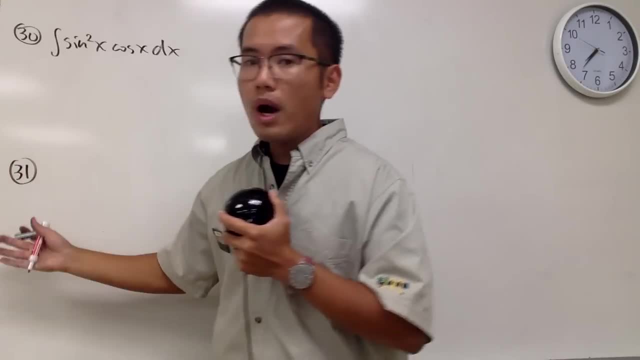 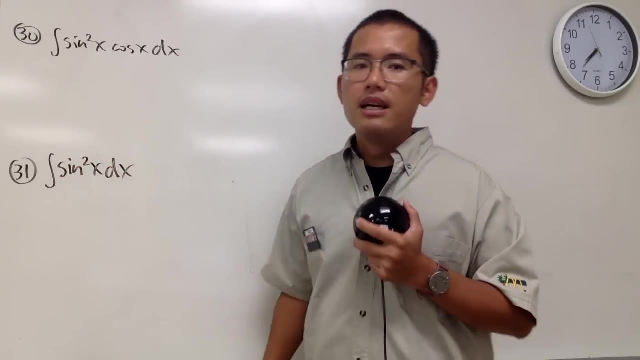 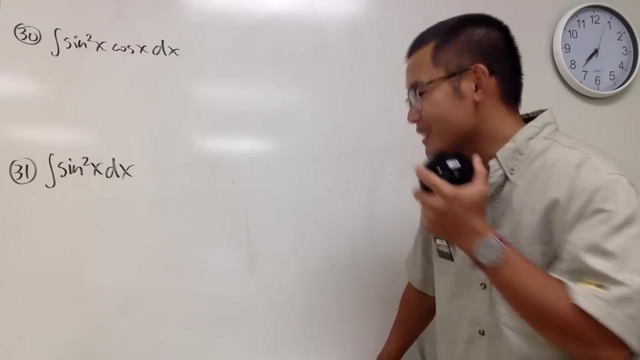 And in the meantime, let's also be looking at question number 31,, which is the integral of sine squared x, dx, like this: Okay, If you have a choice to put 1 on the test, which one would you choose? Hopefully by now your guess will tell me you would like to have question number 30 to be on the test. 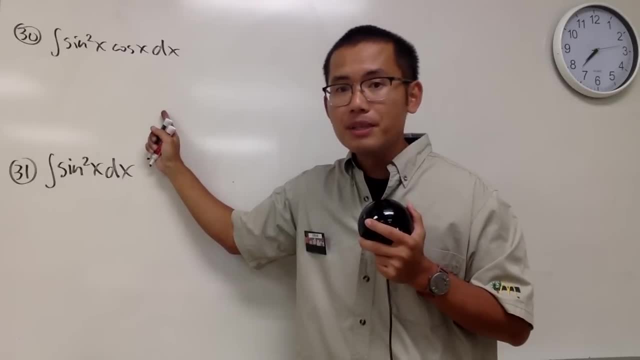 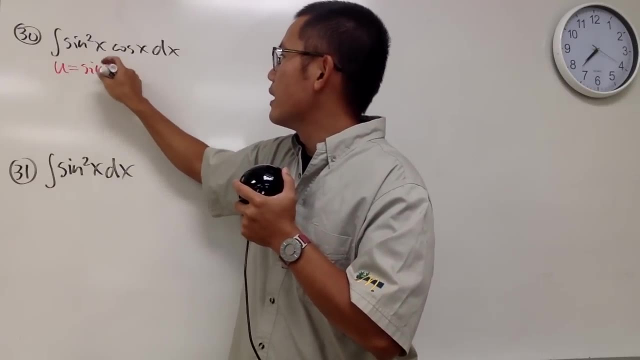 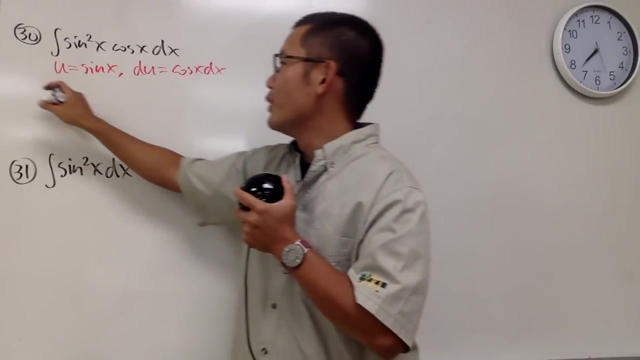 because it's easier. And the reason it's easier is because we can just do u-sub for this. Let u equal to sine x And you notice du will be cosine x dx right away. And you see, we can finish this really quick, really quickly. 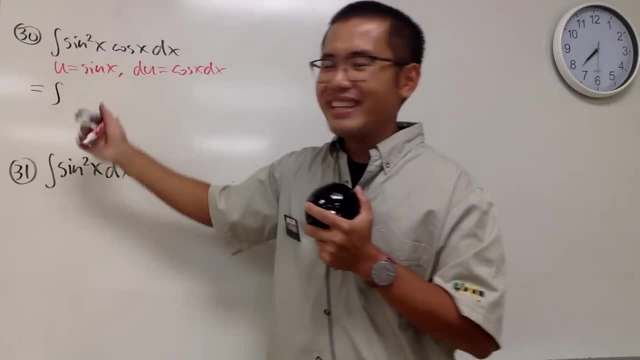 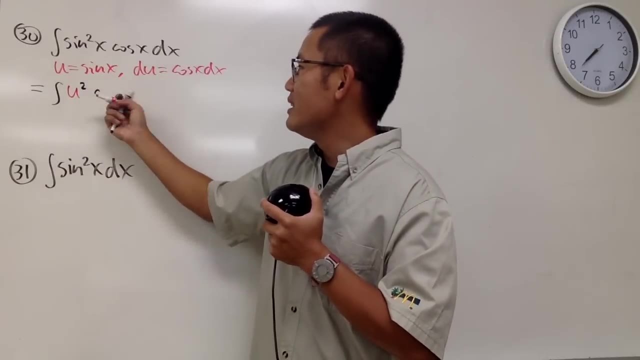 And you see, we can finish this really quick, really quickly, And you see we can finish this really quick, really quickly. This is just the integral of u squared, And this whole thing is just the du. So we have u squared, du. 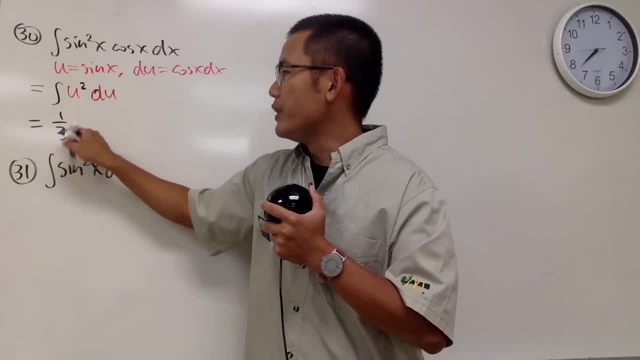 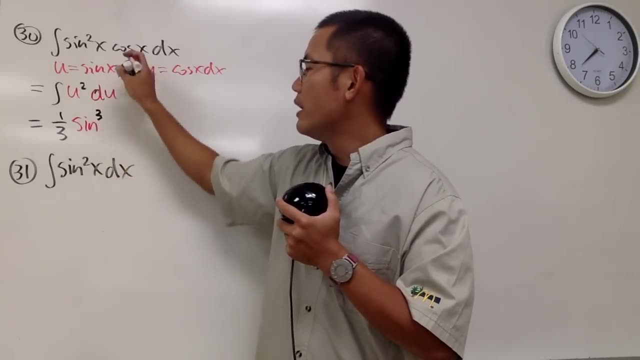 And of course this is just 1 over 3, right. And then u to the third power, but u is the sine, so let's just put down sine and then to the third power, and the input is x And put down plus c, right here. 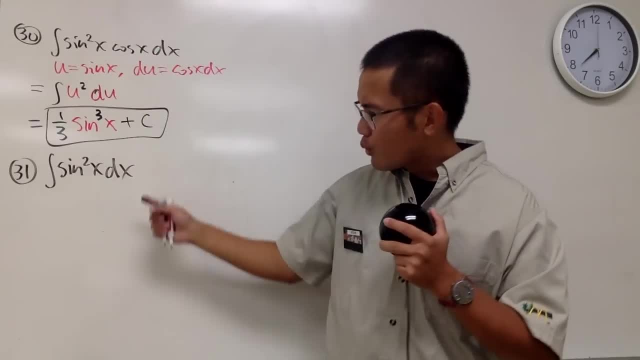 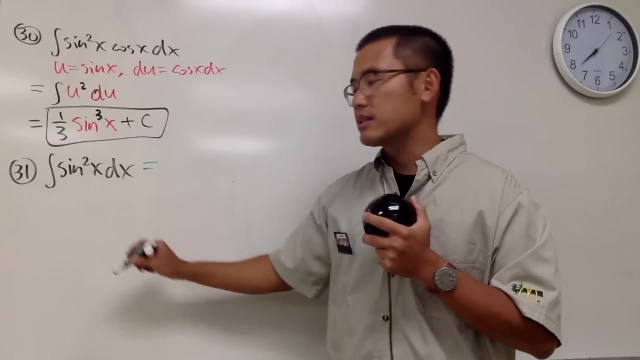 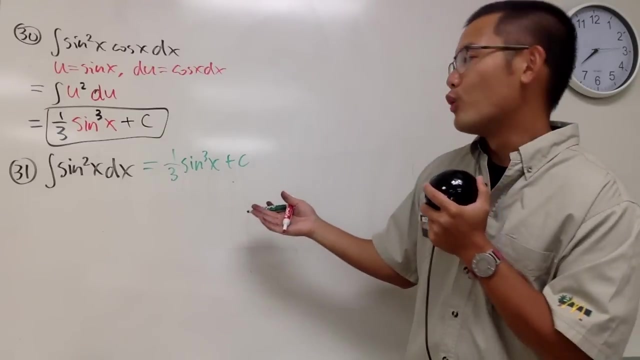 Right Now for question number 31,. is the answer to this question? because we have sine squared x. is this equal to 1 third sine, to the third power, x plus c? No, it's not, And the reason is because this one is not the same as that. 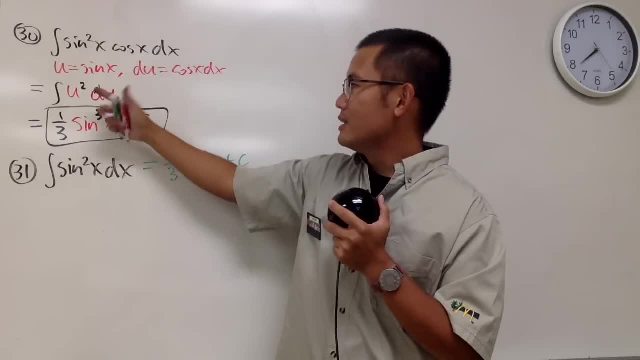 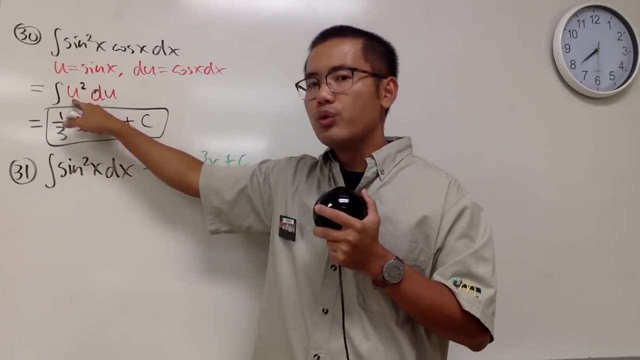 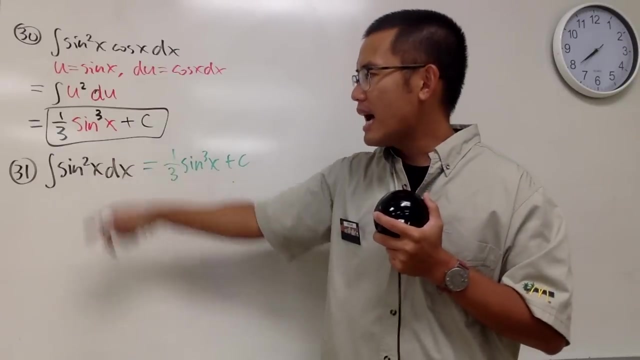 Earlier it was easier because we have the cosine x to help us out. So we can just take this to u-world. We can only do the reverse power rule when we have x or u to a number right, Like this, But when we have sine cosine tangent to a power like that, 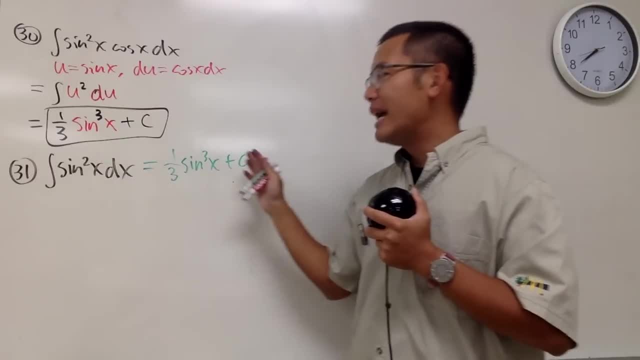 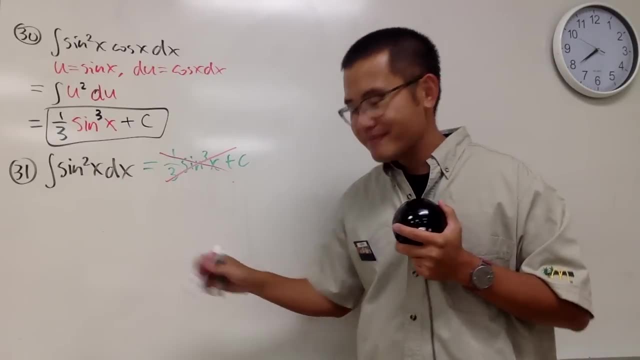 unfortunately, we cannot just add 1 to the power and then divide it by the power. No, this is not correct. This is one of the integral addictions earlier, right? So unfortunately, Huh, man, I told you guys. 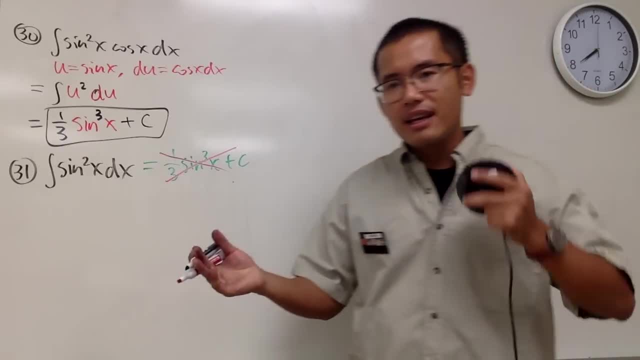 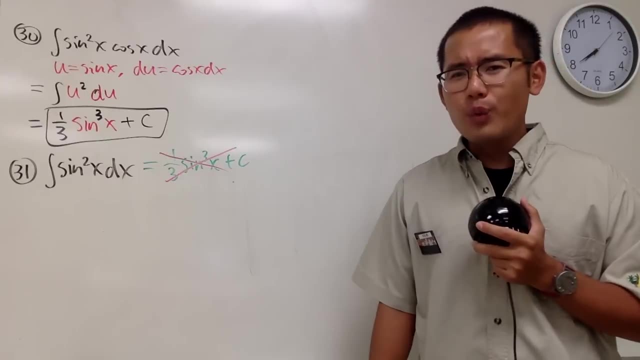 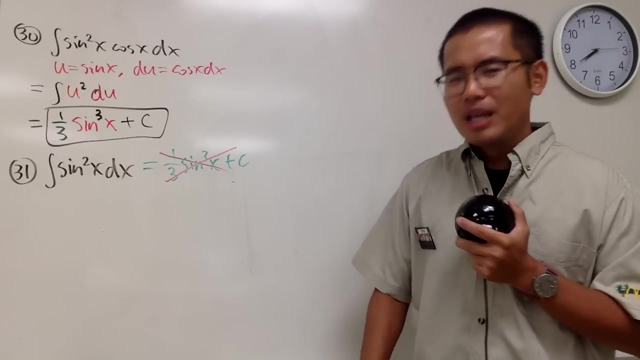 When we're doing integrals, sine and cosine are best friends. But for question number 31,, sine x, I mean the cosine x ran away, Cosine stitches. That's no good. What a bad friend. But it's okay. 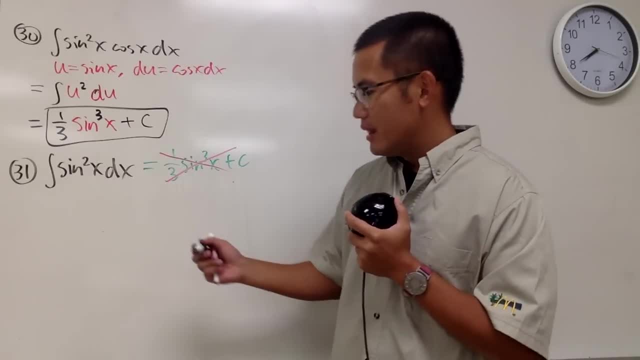 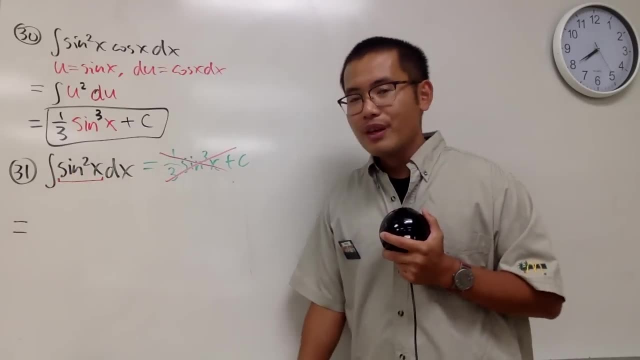 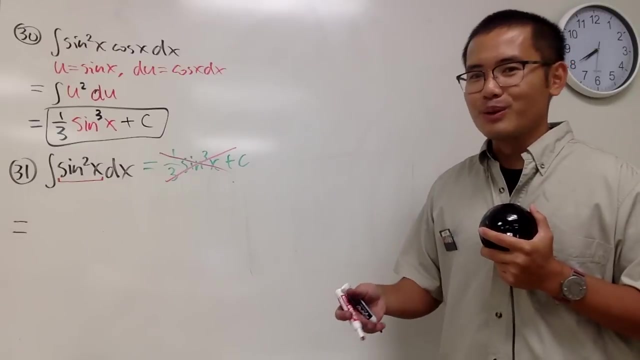 We can still survive. Here is the deal. Let's look at the following Today. let me tell you guys, Sine squared x. Well, if you refer back to the things that we did in the past, namely I was going to say MF240,, 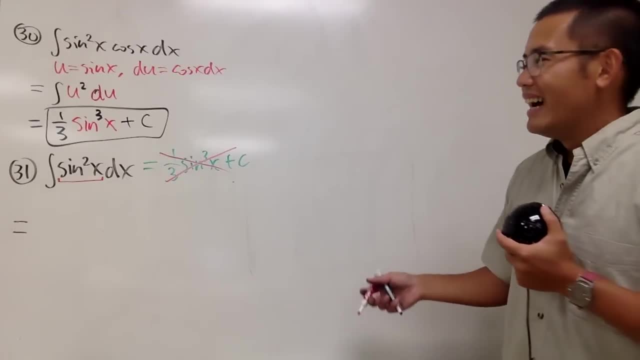 but I guess don't know what. MF240 is Bad trick, And we actually have a lot of identities that we've seen before, So let me just write down these two for you guys. We know that when we have sine squared theta. 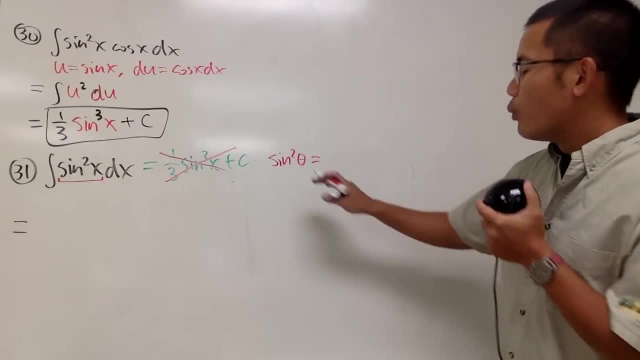 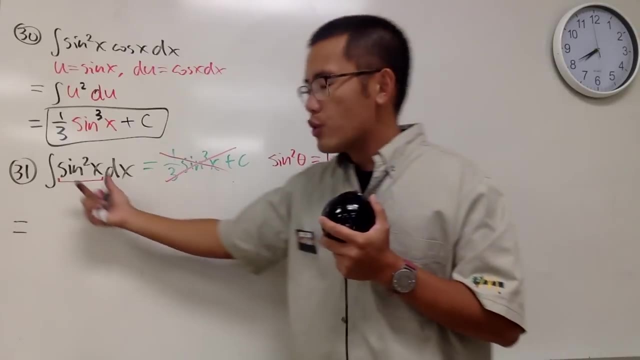 well, we have two versions of this identity. One way to break this apart is, of course, 1 minus cosine squared theta. But if I put this right here, can we integrate 1? Yes, But can we integrate cosine squared? 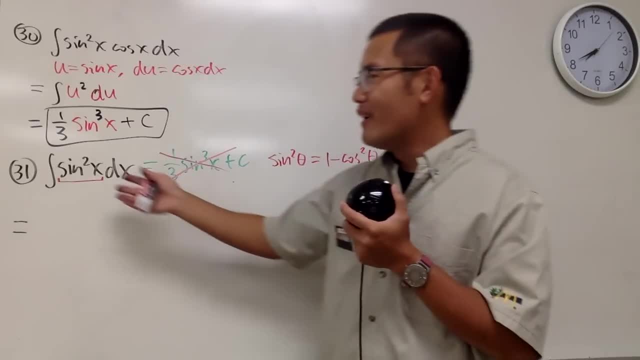 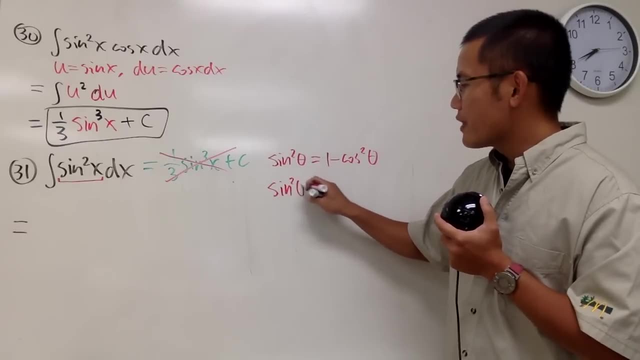 Not so much, Because that would be just as difficult as the original question, So that's not preferred. However, we do have another identity when we have sine squared theta And when I'm writing down the identity, let me put down the theta to be the angle. 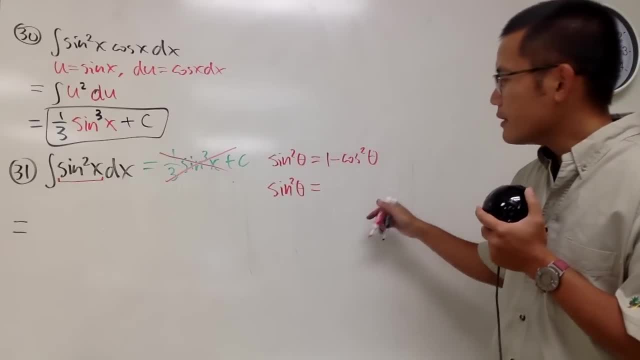 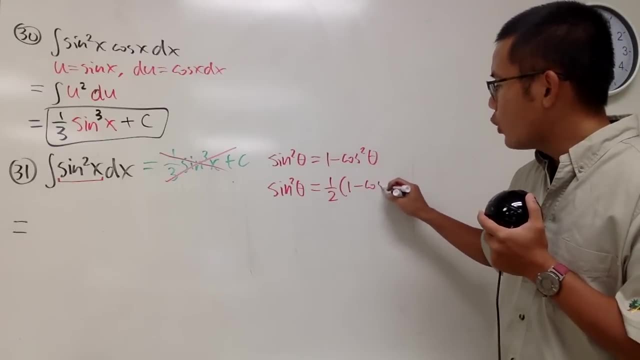 for the variable. I know I'm using x over there, right, But for this one we can actually write down 1, we can actually get 1 over 2 times 1 minus cosine of 2, theta like this: 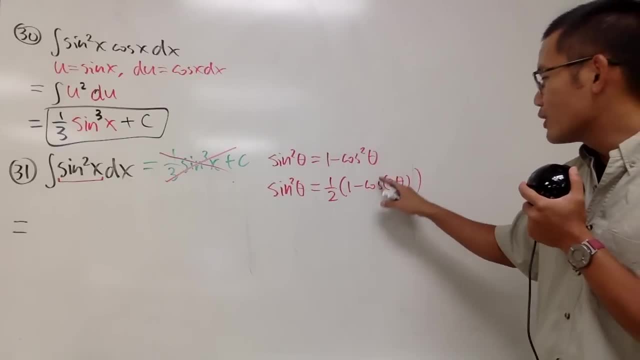 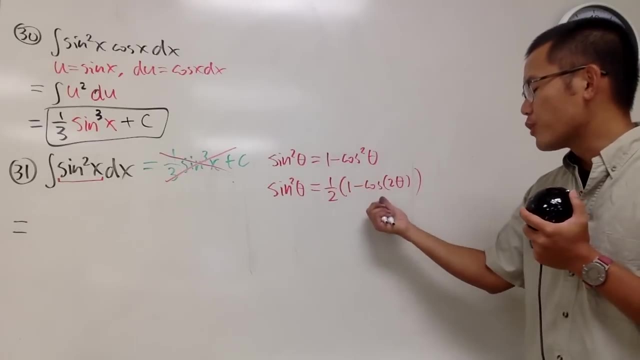 And if you look at this, notice that we have just cosine to the first power And the input here is just 2 times theta. I call this the power reduction formula And of course you can also say this is the half angle or the double angle formula. 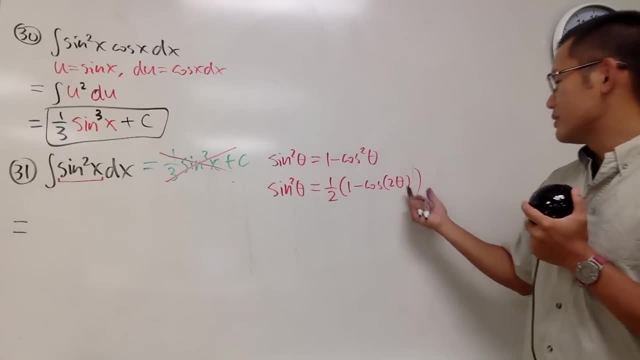 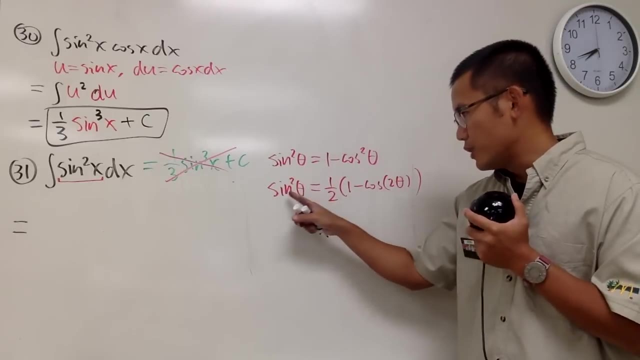 Depends on how you want to look at If you go from here to here, or maybe go from here to here half angle, double angle, right All that stuff. But I will say this is the power reduction when we have sine squared. 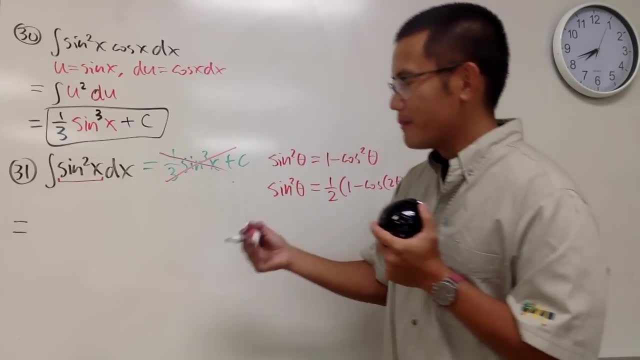 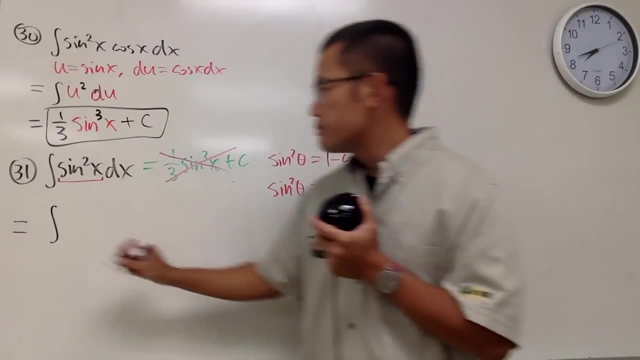 This right here will help us out tremendously. Let's put it down right here. Here we are going to integrate: This is the same as that: 1 half is the constant multiple. Let's just put that in the front And then we have this. 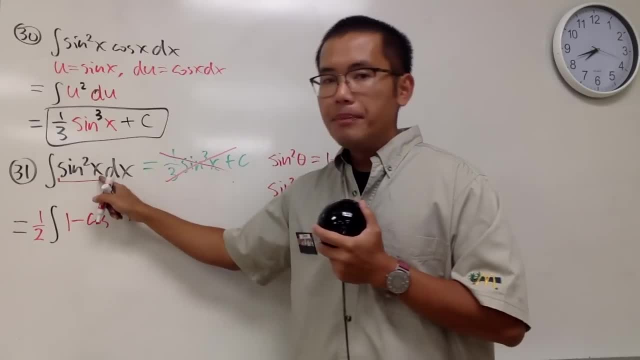 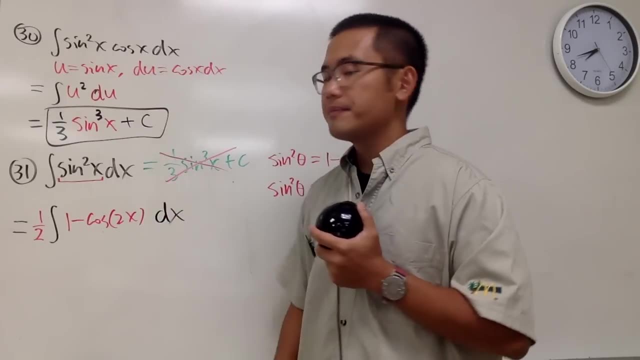 which is 1 minus cosine, And because here we are using x, so we will have cosine of 2x, like this, And of course we still have the dx on the very outside. Now 1 half is just a constant multiple. 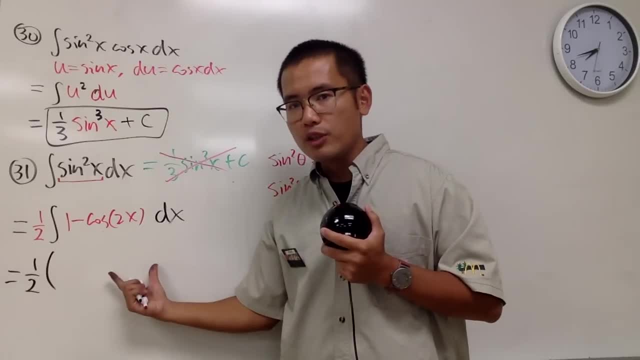 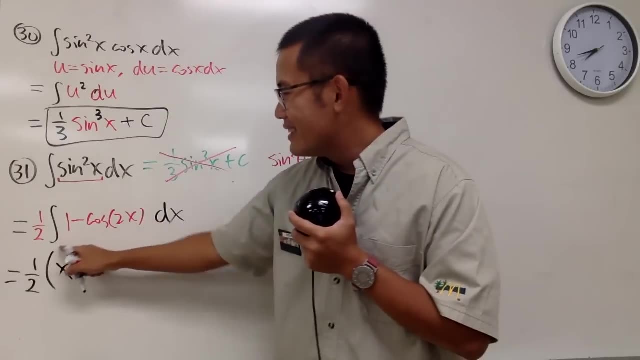 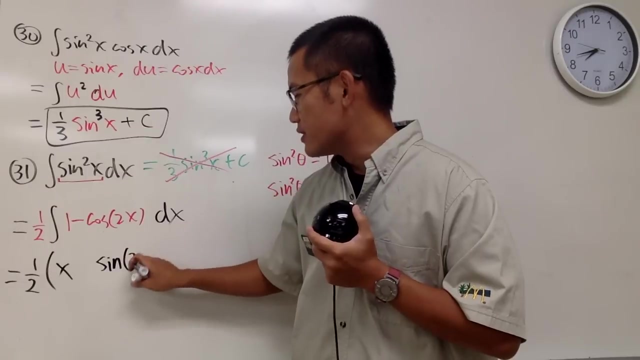 Let's put that down and open the parentheses for the result of integration. Integrating 1 in the x-world, we get x- Good. Then integrating cosine, we get positive sine- Good. And the input stays the same because the input is just a linear function. 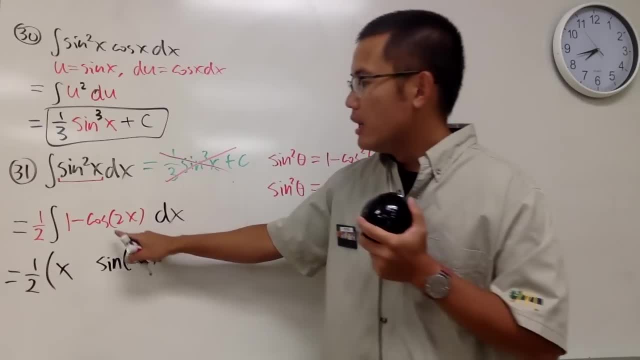 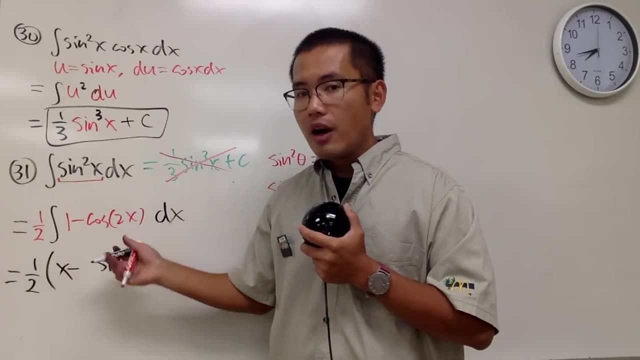 namely 2x. in this case, And because when we are integrating cosine we get positive sine, so the sine right here stays to be negative. However, when we go this way, we have to look at the derivative of the inside. The derivative of 2x is 2.. 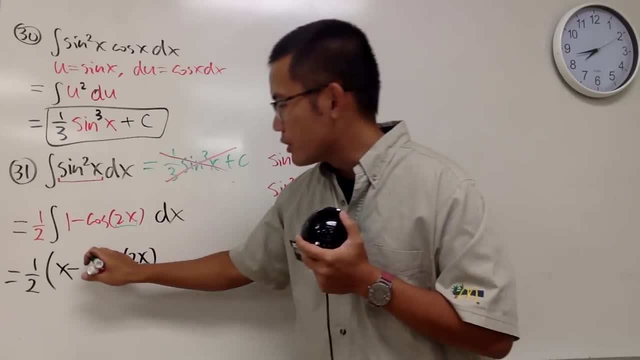 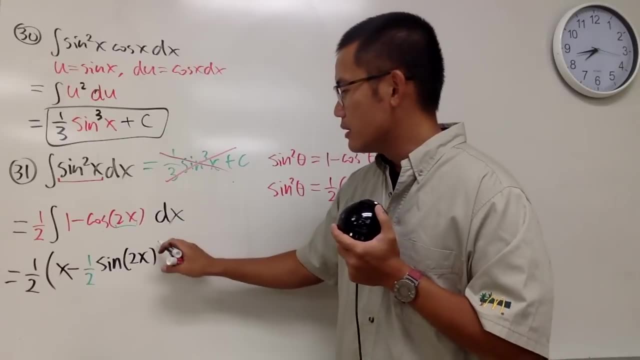 It's a constant. only We have to divide it by 2, so we have to have the 1 half right here, And that's why I told you guys about the formula earlier. That's pretty much it In the end, of course. let's just distribute this little 1 half. 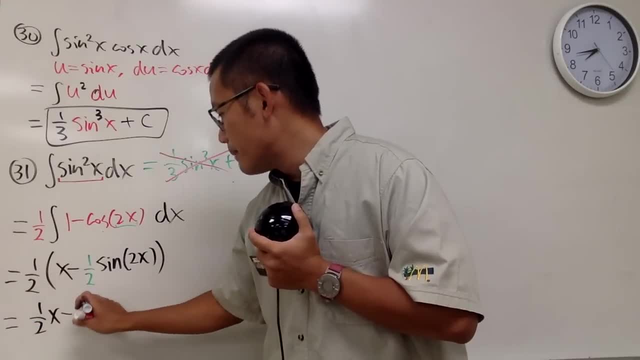 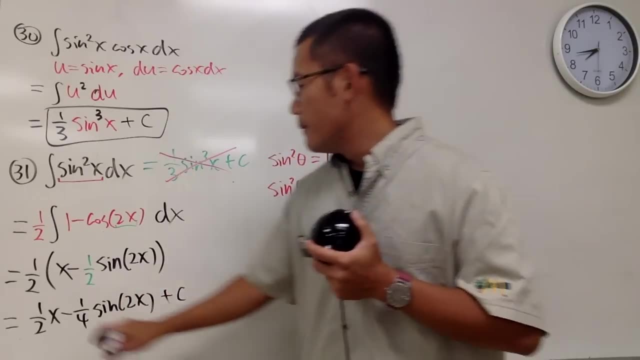 So when we do that, that's 1 half x and then minus 1 over 4, sine of 2x like this And we're done Plus C. If you want to use the double angle identity to break this apart, it's up to you. 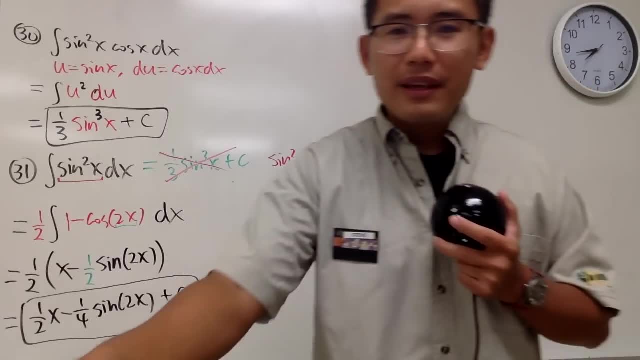 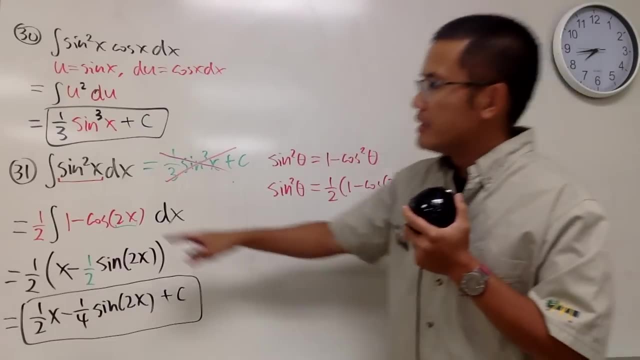 but this is totally okay. So here is the idea. Okay, my laptop is still recording, so this is good. Here's the idea. You see how we just conveniently use the trig identity to help us out. Maybe you can do it. 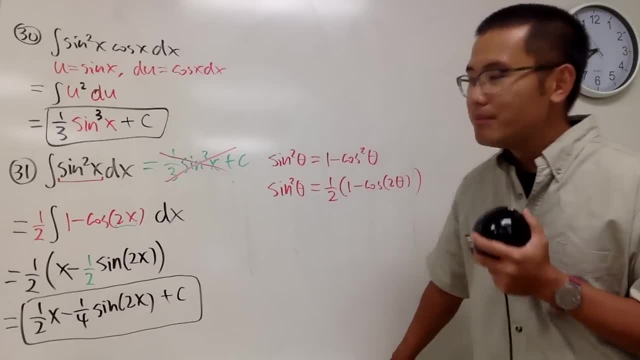 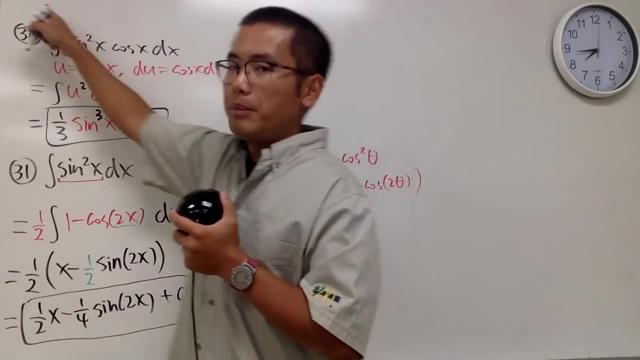 by some other way- integration by parts or whatsoever- but identity, it was the way to go. So for this category, which is category number 8, let me put it down right here For you guys. this is how I write the 8, yeah. 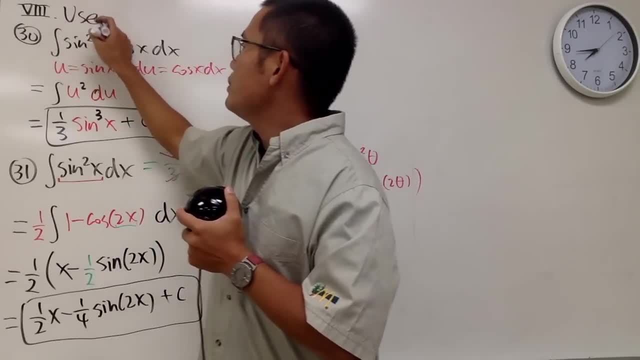 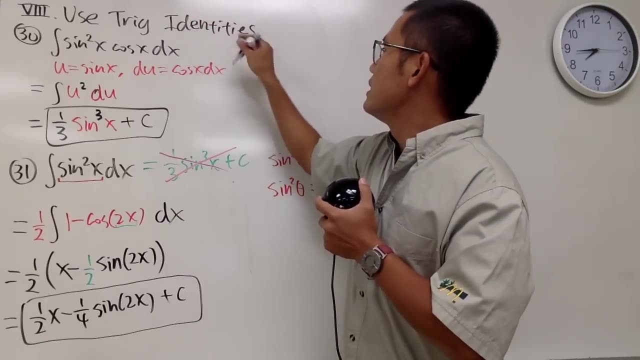 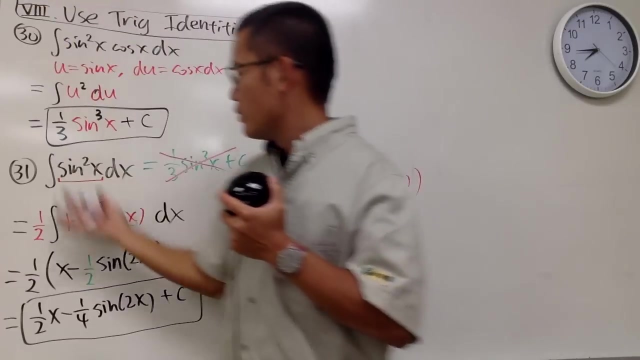 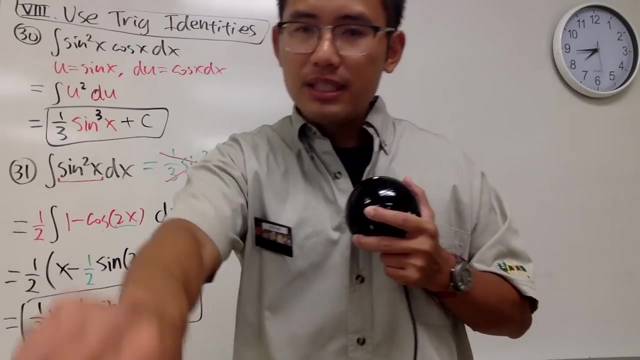 Like this. I'll just tell you, guys, we are going to be using trig identities like this. All we are doing is just use trig identities like this: Very, very nice, Very, very nice, right, And I'm debating to see if I want to write down. 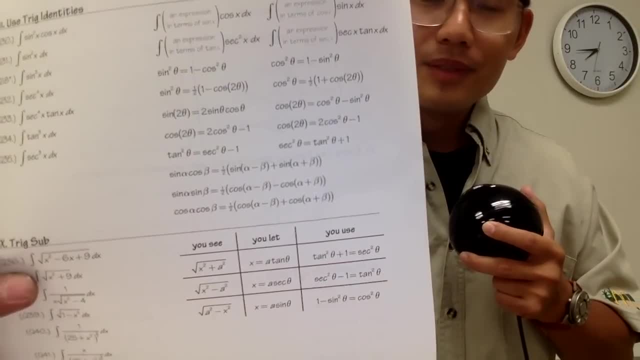 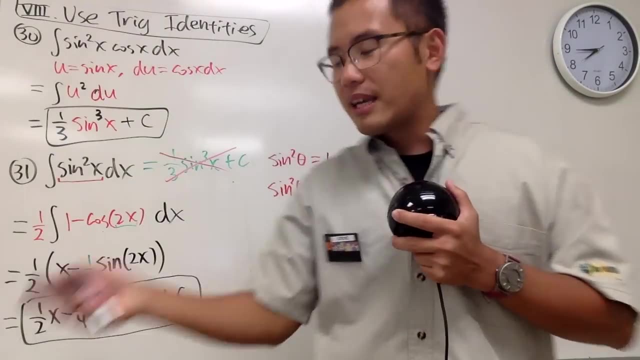 the identity right here for you guys. Just take a screenshot or maybe just go download the PDF. So these are the identities that we'll be using, right? So we have the sine cosine, etc. etc. and also secant tangent. 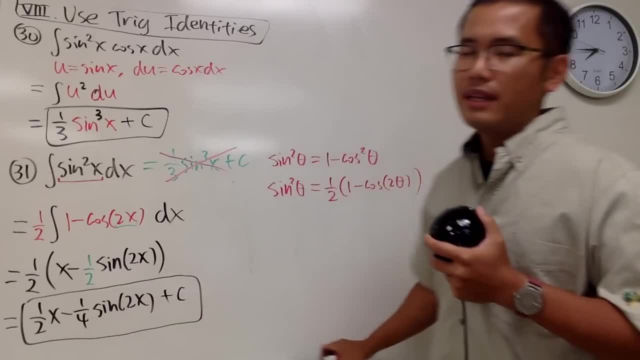 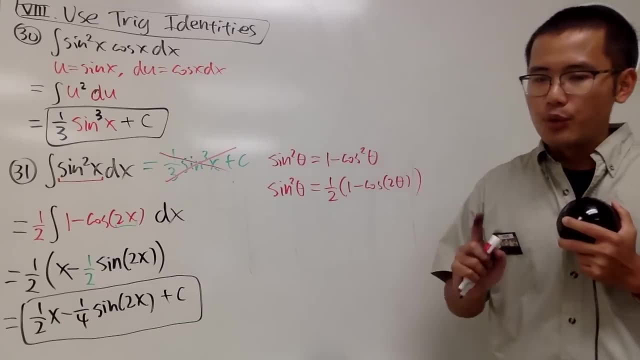 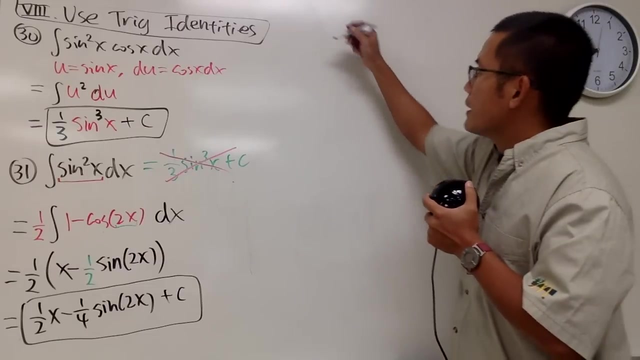 However, knowing the identity is not enough. We also have to have strategies. I will be writing down the strategies right here for you guys. So let me actually put down the strategy. I will explain what I mean by all this. Here are the strategies. 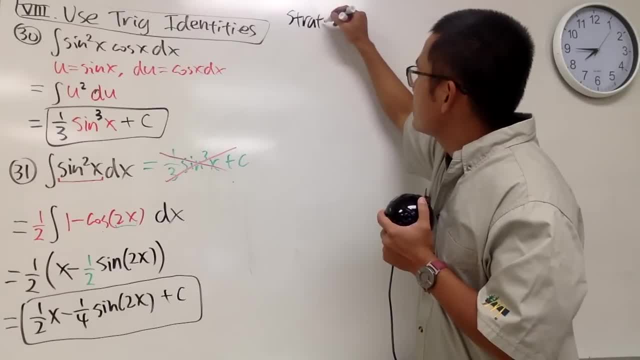 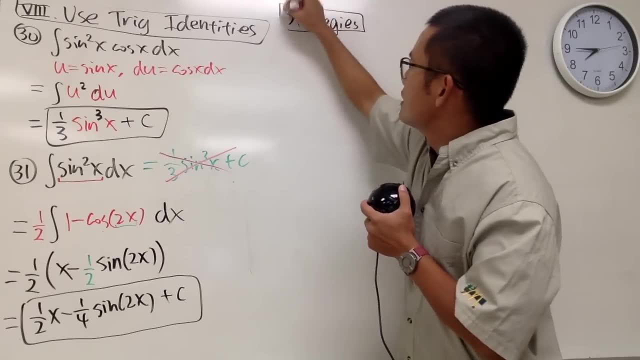 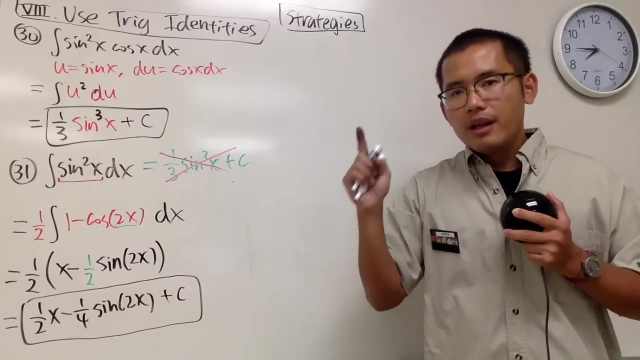 Let me just put it down: Strategies. I guess it's like this, right? I also have this on the PDF, right, So you can go download it if you would like. We have two cases to consider. The first case is when we have an integral with sine cosine. 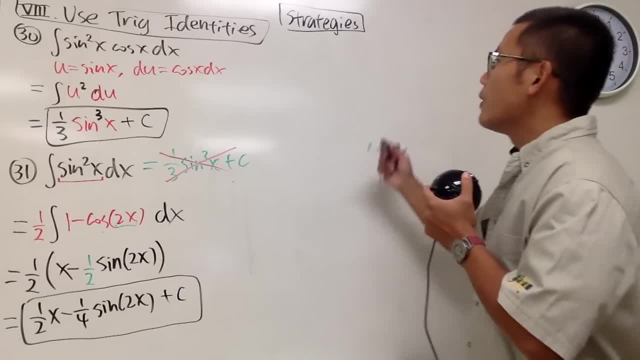 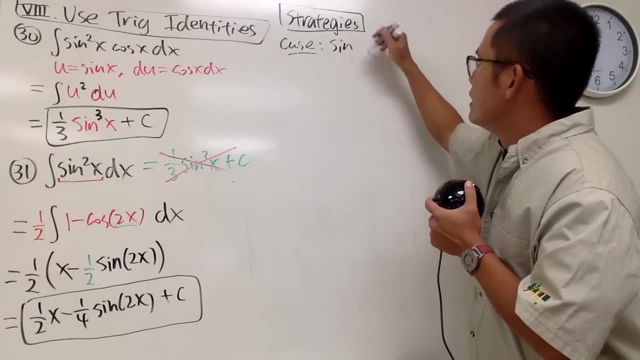 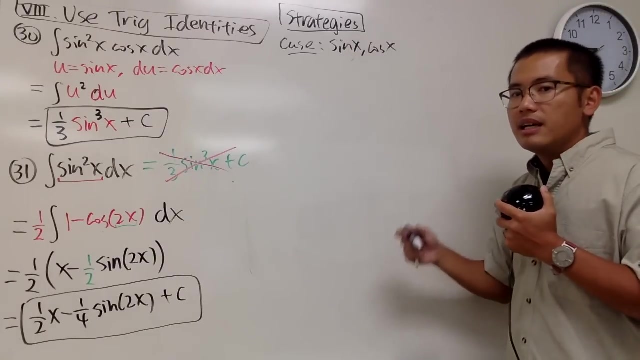 And keep in mind they are best friends, right? So strategy: This is the case when we have sine and cosine, Sine x and cosine x And notice they have to have the same angle, Maybe just x and x. Here is the first situation. 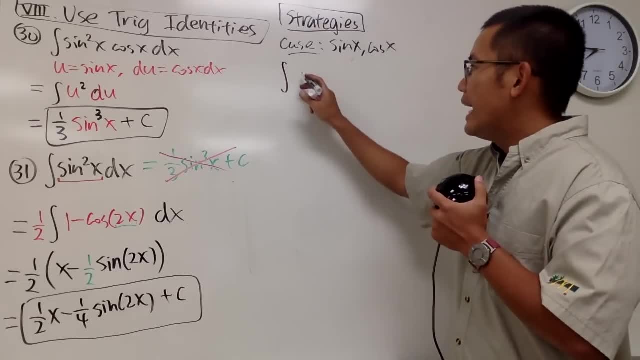 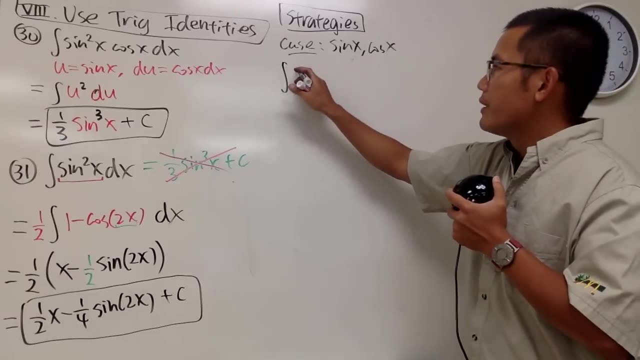 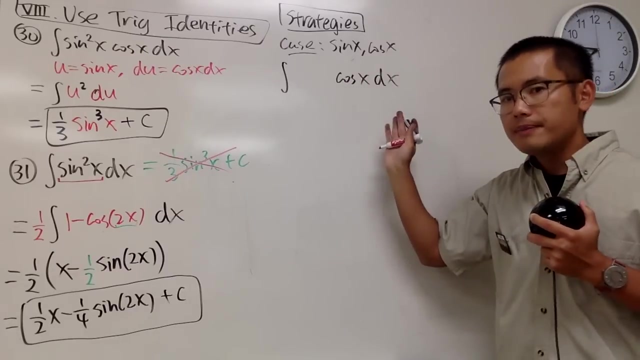 Suppose we have the integral like this, And if you happen to have, Let me actually No, I'll just put it down- Suppose you have the integral right here, And suppose you happen to have cosine x dx somewhere like this. Well, what you wish to happen is: 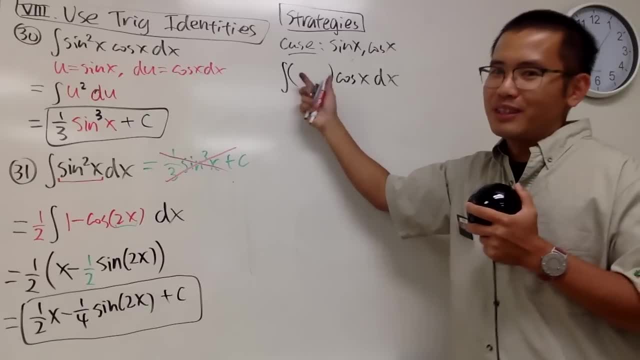 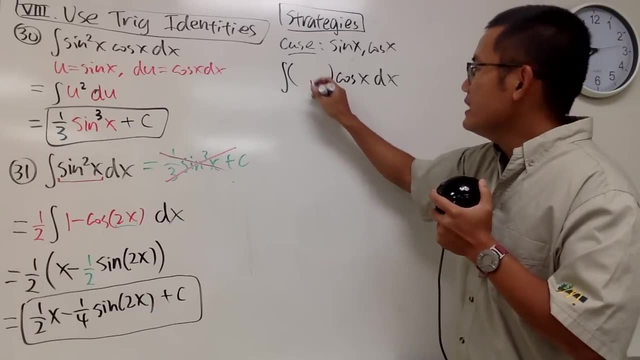 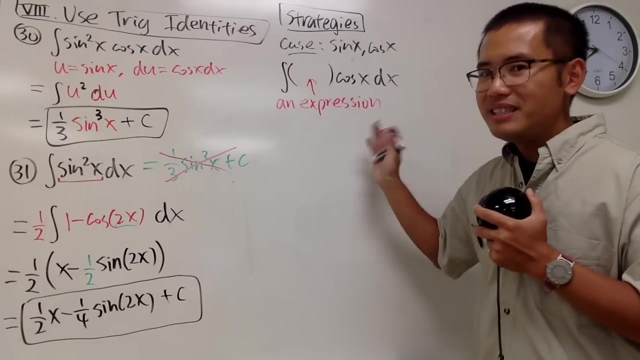 maybe the expression in the front. I know, if you have nothing right here that's actually better, But if you have cosine x, dx right here, what you wish to have is this part is an expression: Hopefully easy enough, Hopefully, easy enough. 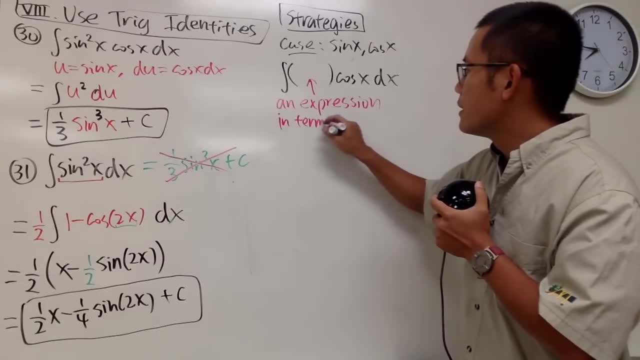 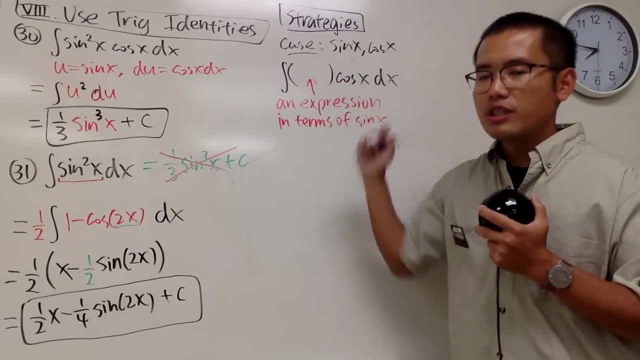 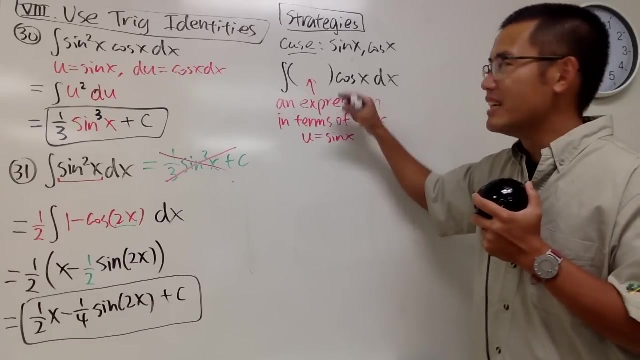 An expression in terms of sine x, And the reason for that is because if this is an expression in terms of sine x, we can just go ahead and let u equal to sine x And du is equal to cosine x- dx, And we'll be able to take this integral to the? u-world nicely. 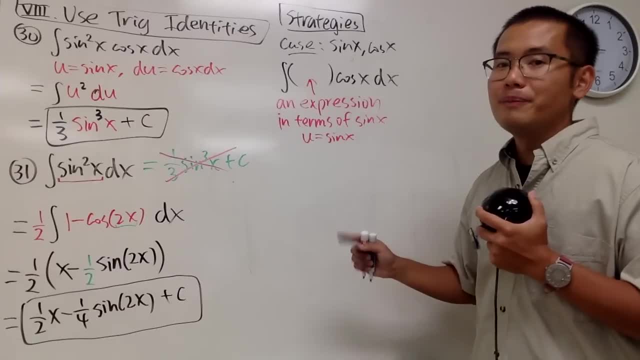 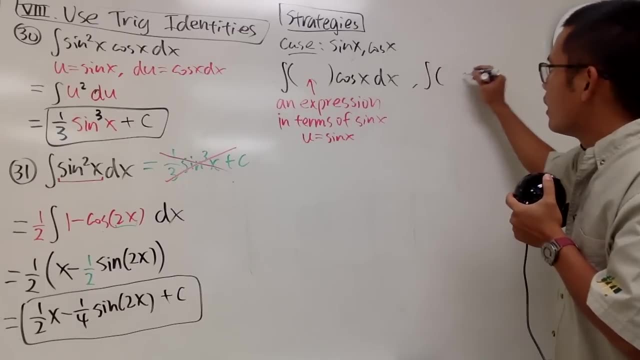 And again, hopefully this expression is nice enough. If it's crazy, then unfortunately we cannot do it so much right. Well, similarly, if we have the integral of something in the front and we happen to have sine x right here, dx. 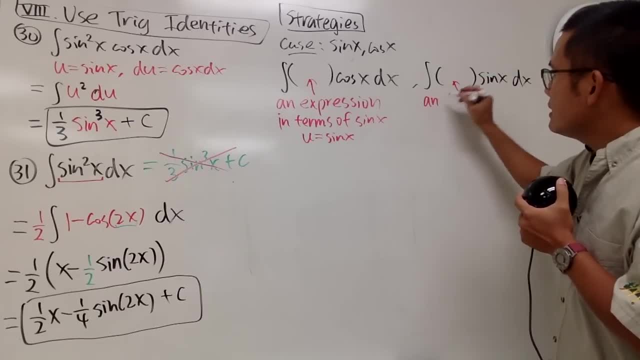 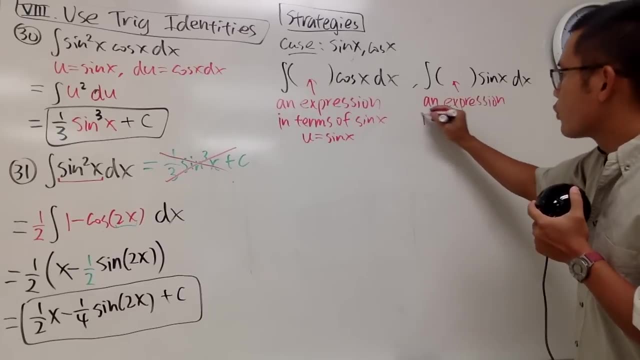 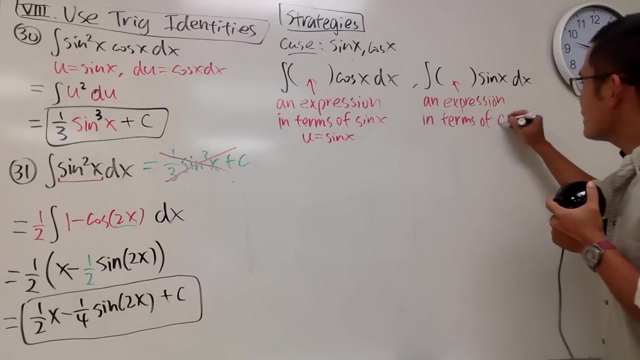 In that case, we hope that this is containing an expression- Hopefully easy enough, of course, And we just want in terms of What, Yes, Cosine x. We don't want tangent, We don't want anything else, Just trying to convert them into cosine x. 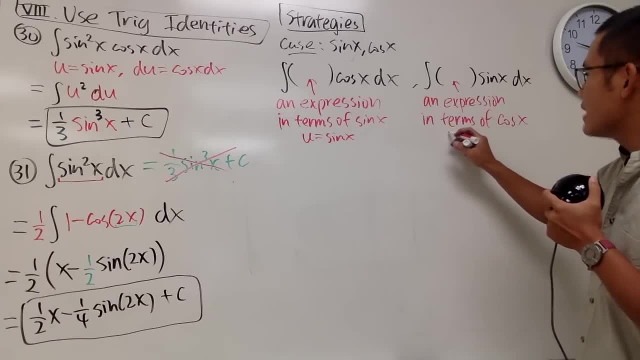 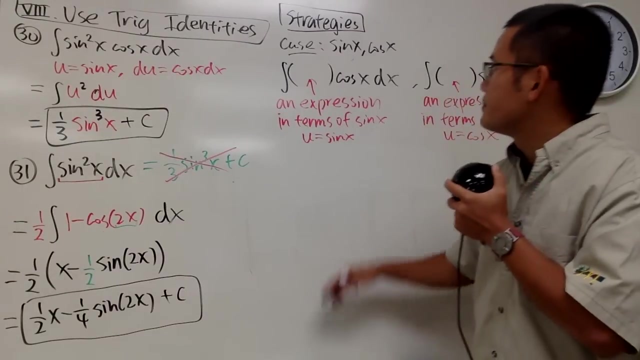 That would be the ideal situation, because once we have this in terms of cosine x, we can take a u-sub that u equal to cosine x, And then du will be negative sine x, And then you can just go from there, right. So this is the strategy for the sine-cosine situation. 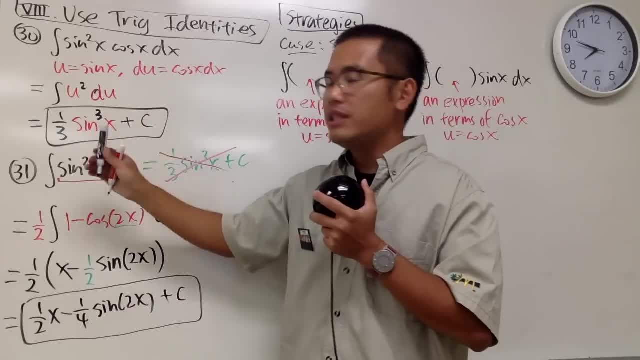 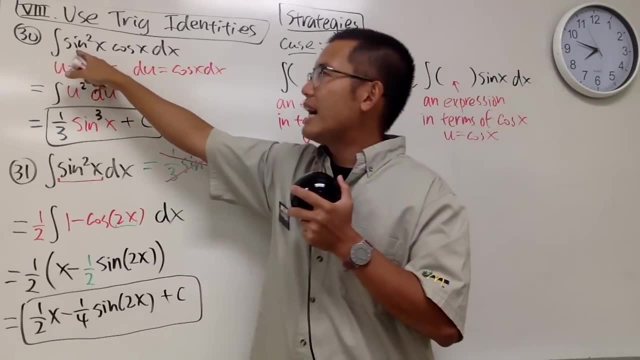 And that's exactly what we did right here for question number 30. You see, we had a cosine x dx right here And in the front we nicely had an expression in terms of sine x. This was sine x in the parentheses. 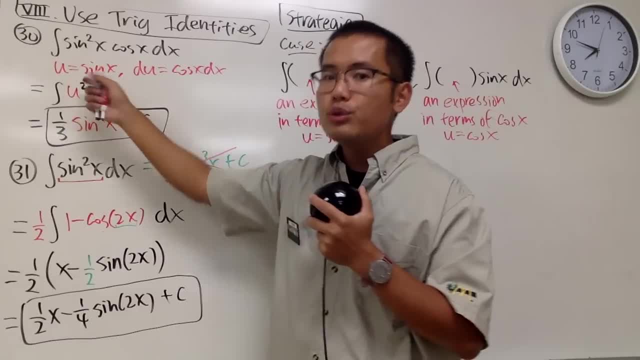 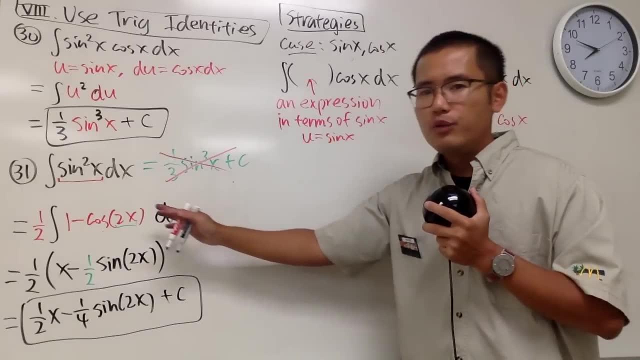 and then square that. So sine x times sine x, So we were able to say that's u squared, So that's very nice, So that was good. But sometimes, if you cannot make that happen, if you have an even power like this, 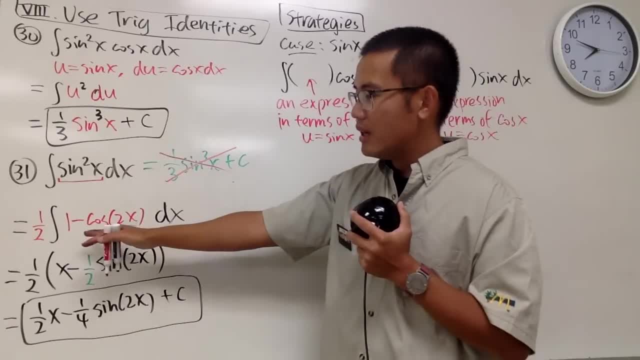 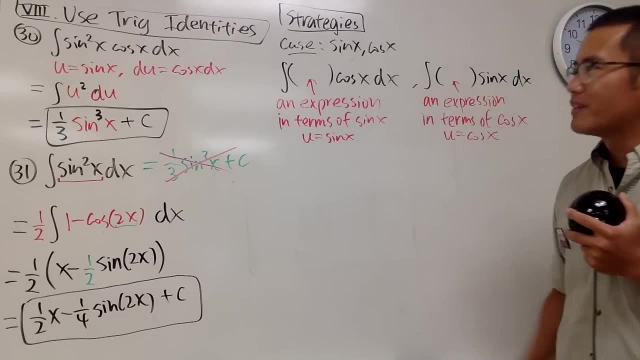 maybe we'll just have to use the double, Maybe we'll just have to use the power reduction formula, like this right. So this right here will be the easy situation, I would say, and we'll have the strategies for that. Now let's look at another example. 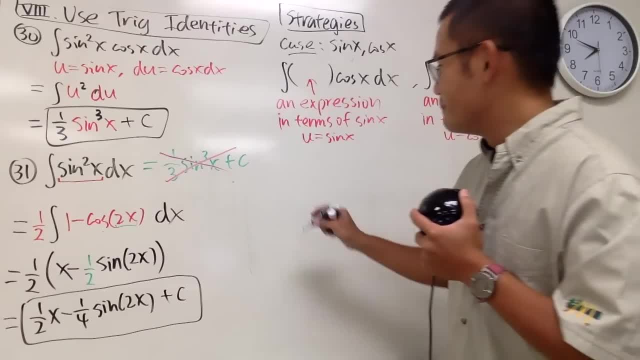 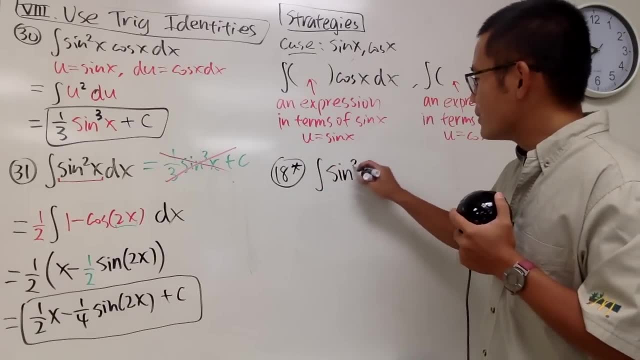 And this is question number 18, the one that we did earlier, but we didn't really do it, So let's look at question number 18.. Name the integral of sine to the third power: x, dx. So it's very different than that. 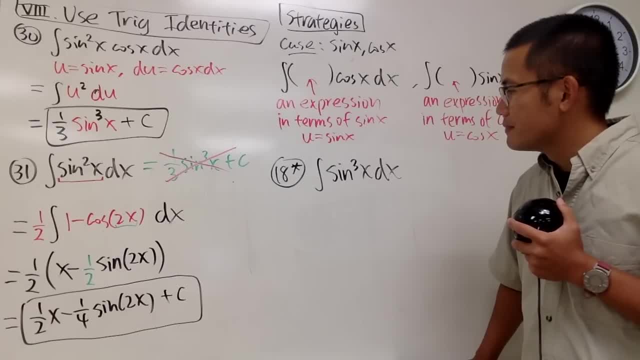 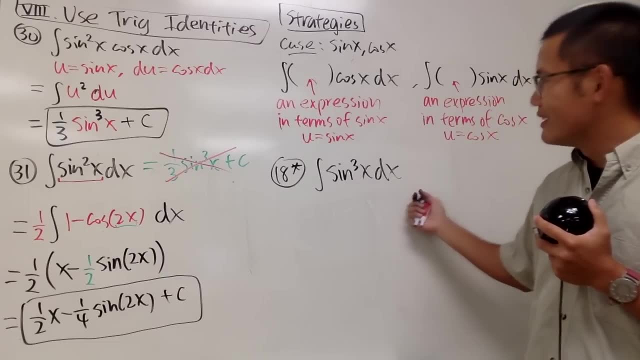 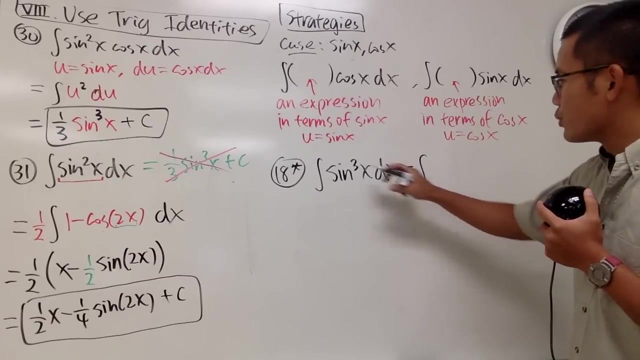 Hmm, Well, this is an odd power situation. Can we take one of the sine out And then we'll be talking about this expression? huh, Very nice. So now have a look here. This is equal to the integral and we have sine squared x times sine x dx. 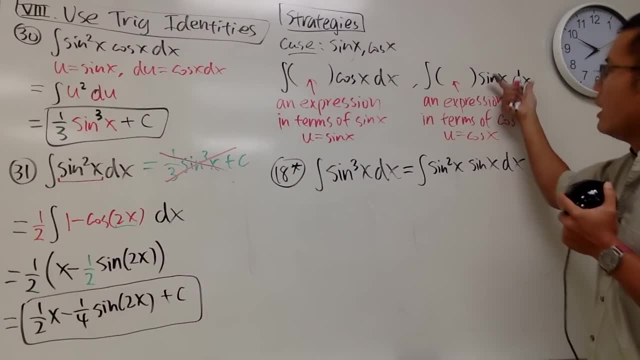 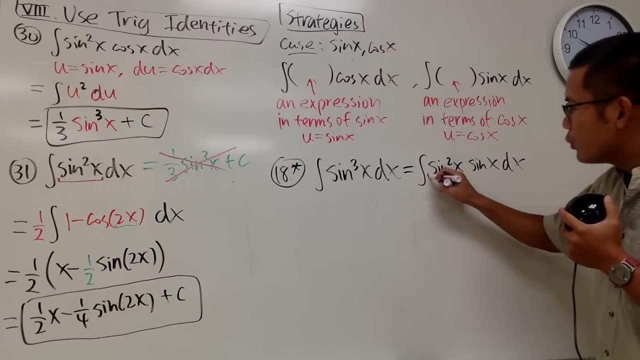 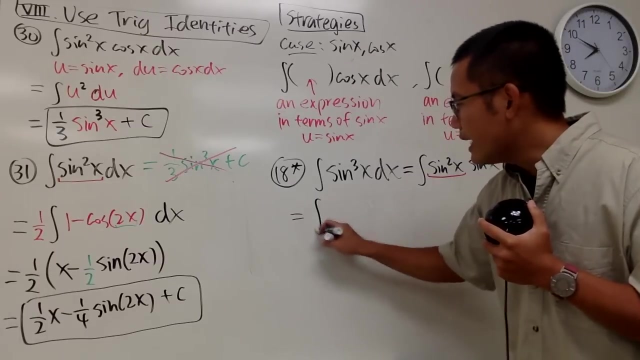 And in this case we have the sine x right here and we hope that the front right here is an expression in terms of code, cosine x, and at the moment we have sine squared x. In this particular case, we are actually going to rewrite this as: 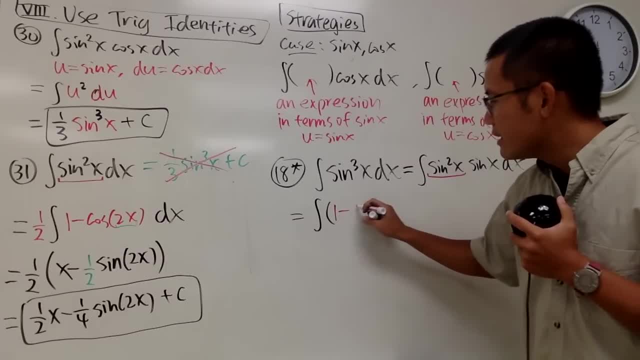 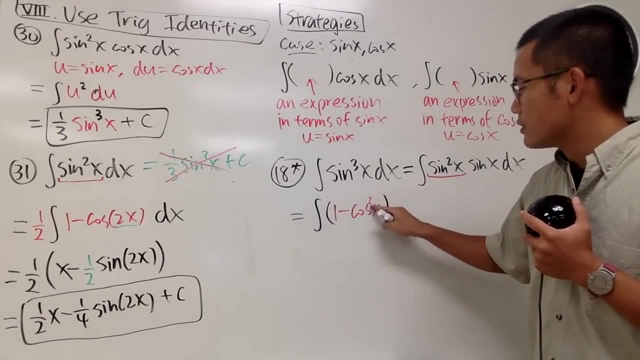 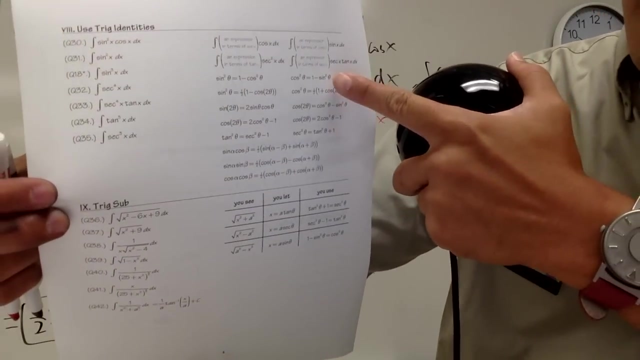 parentheses, with 1 minus cosine x to the second power. So I'll put it down like this. So remember the identity I gave you. You have two of them, So using this one now. Again the reason that we're using this one now. 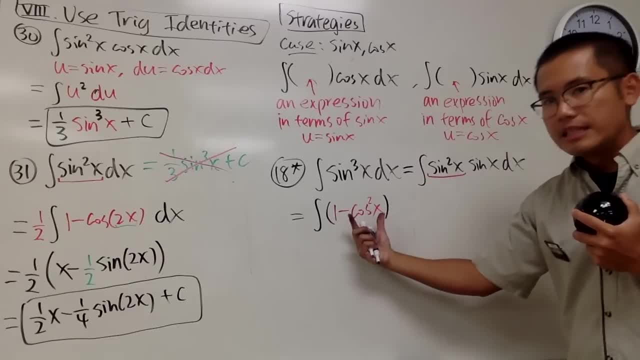 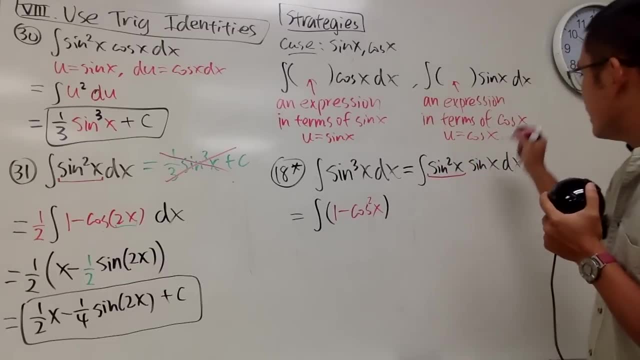 is because we want this right here to be an expression in terms of cosine x, and this means 1, and then minus cosine x to the second power, like this, And then of course, we still have the sine x. We have to face that. 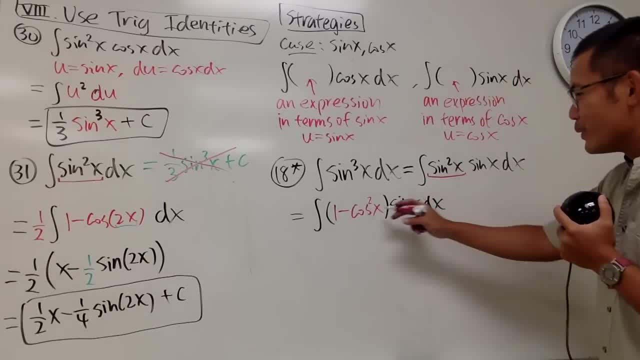 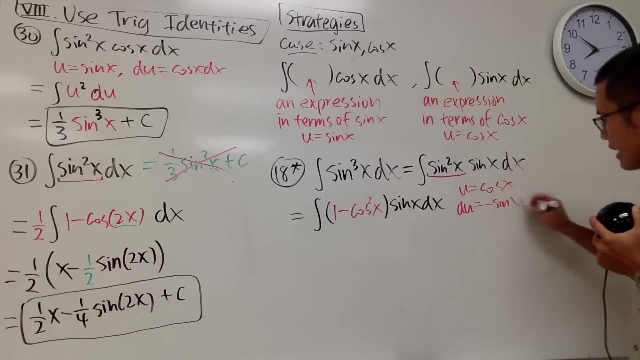 And this is not that bad at all, because we can just do a use-up that u equals to cosine x, just like the discussion here, and then du is equal to negative sine x dx. I will show you guys the cancellation: You end up with a negative. 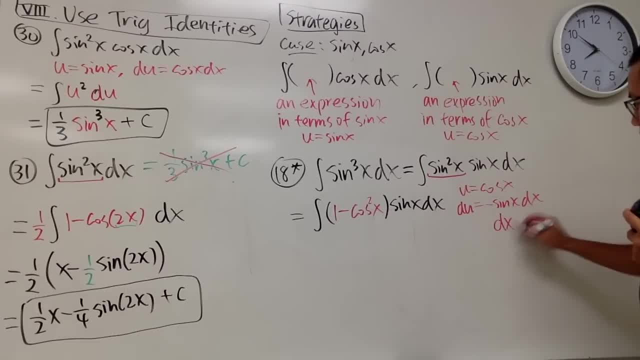 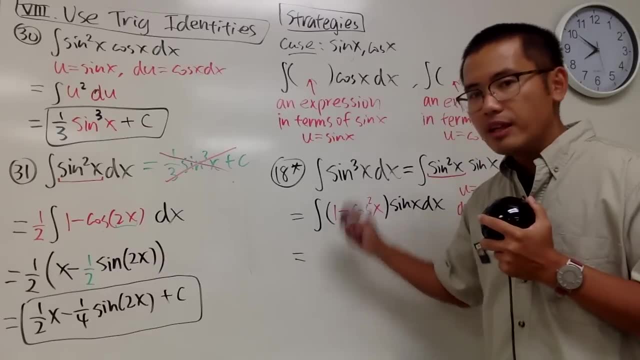 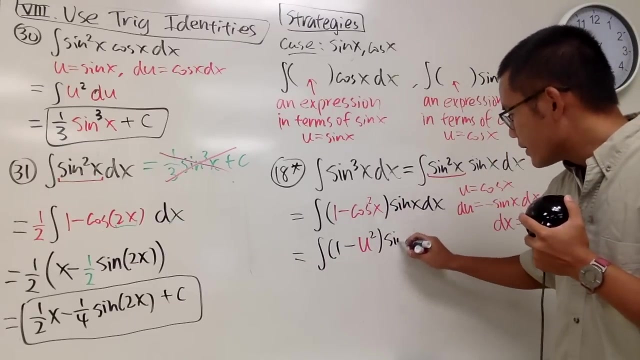 Let's divide this on both sides. dx equals du over negative sine x. Now here we have the integral. This is 1 minus this is u and we have the square Sine. x stays for now, because dx is this, namely du over negative sine x. 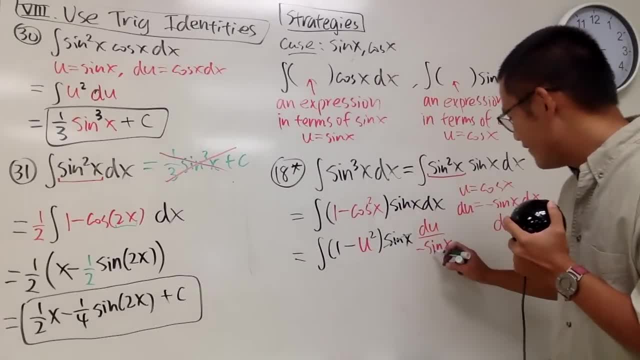 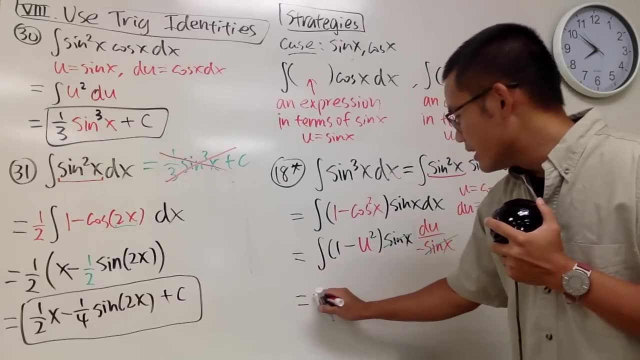 and we are going to cancel the sine x. Very, very nice. No x in the u-world. Put the negative all the way in the front. So we are looking at the negative integral of 1 minus u-square in the u-world of course. 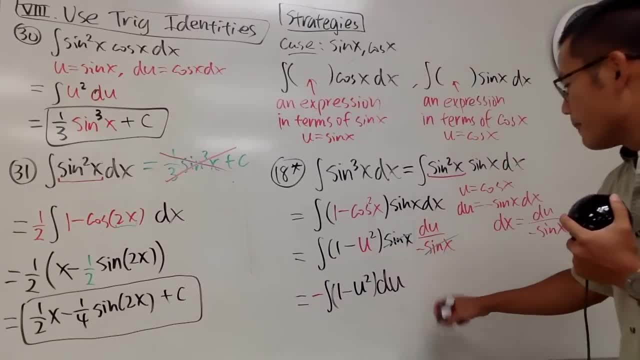 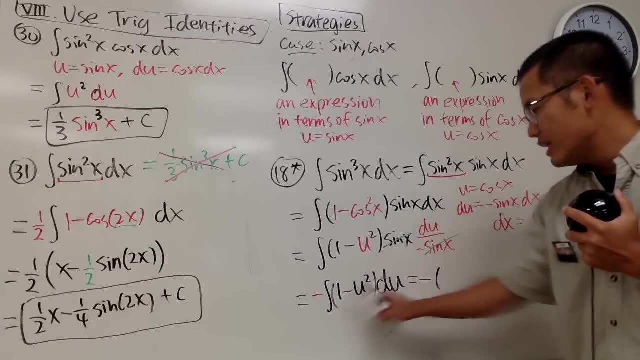 Parentheses were not up to you, I would say: Now we are just going to say this: Negative parentheses: integrating 1. Integrating 1, all right In the u-world, we get u. And then minus, Because I have the minus on the outside. 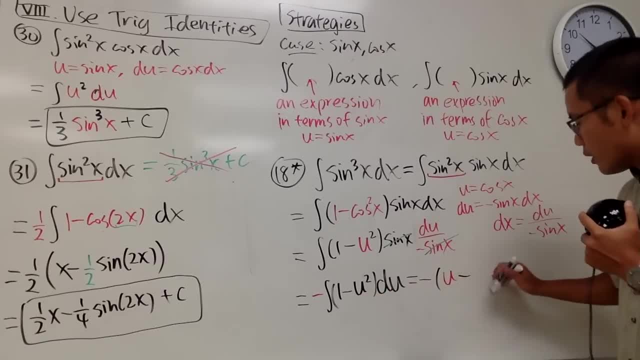 I haven't distributed it yet. Minus Integrating this in the u-world, we get 1 third u to the third power like this: In the end, put this back to the x-world so we get Distribute this. 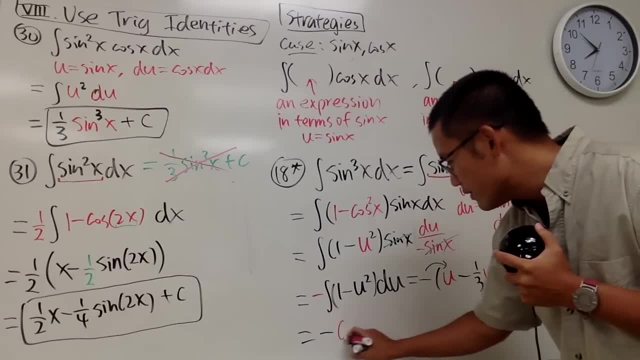 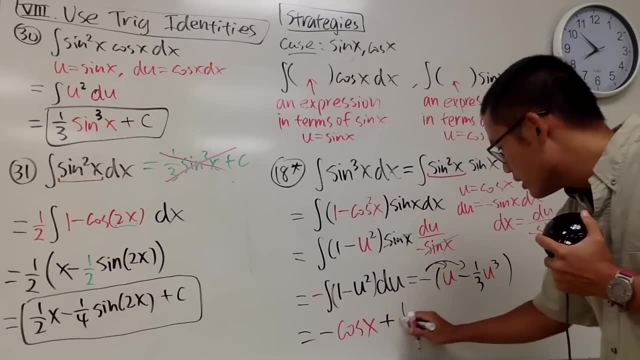 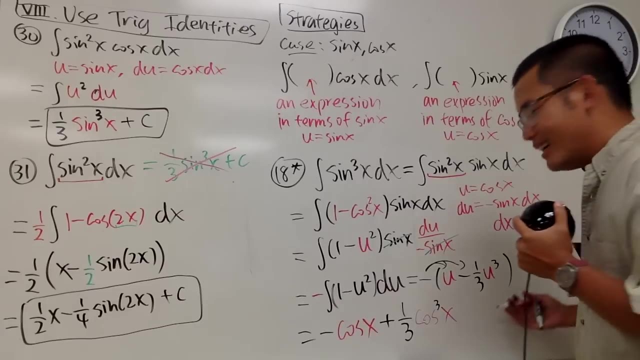 We get negative, u is cosine, so we have negative, cosine x. And then negative times negative, we get positive: 1, third u is cosine, so we have cosine third power, x. like this Are we done? Sure, we are. So this right, here is how you take care of sine to third power. 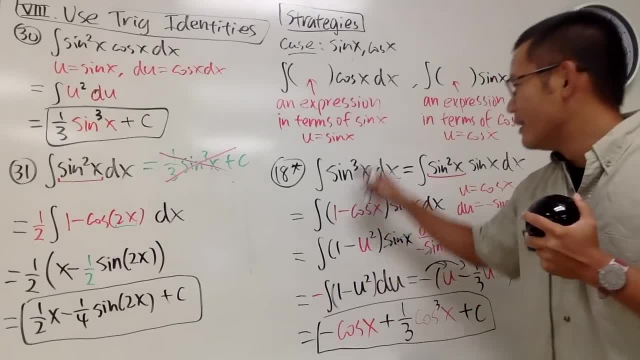 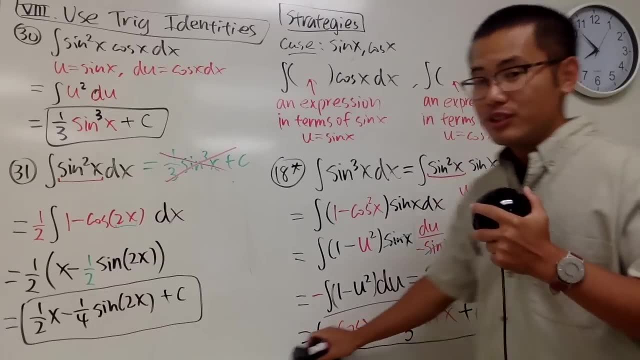 You don't just add a power and then divide it by the new power. No, it's not like that. This is how we do it. Follow the strategy. Follow the strategy, just like that. All right, So that's pretty much the idea. 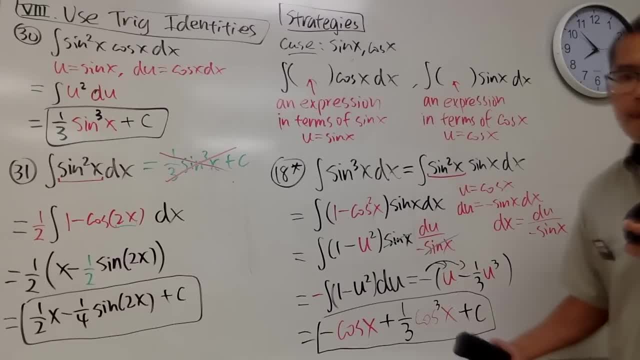 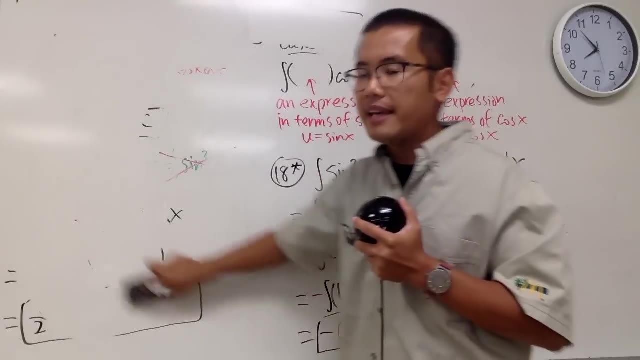 So have a look right here And we are going to do more, of course. So here we go. Let me just erase this And we are going to do the next case And remember when we're doing: integrals sine cosines are best friends. 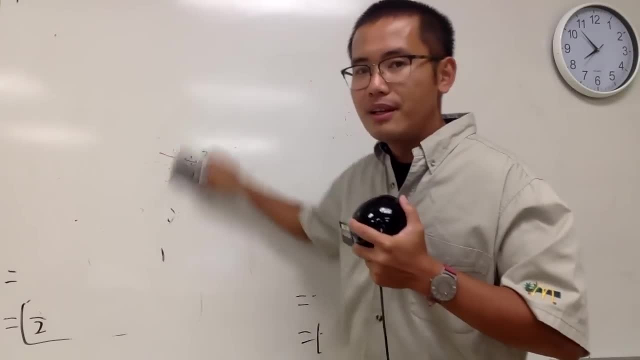 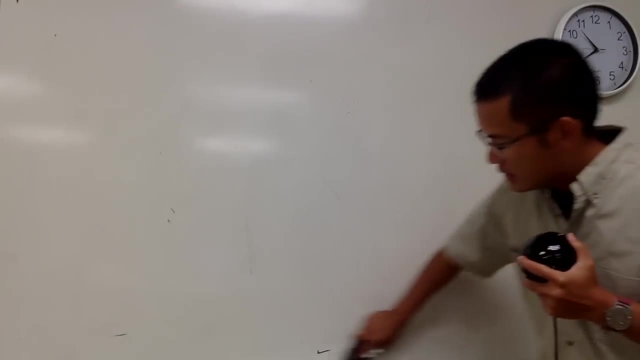 Tangent and secant. they are best friends And of course cotangent and cosecant are best friends. but usually I don't know and I don't really like to ask those questions on my exams because I think that's slightly overkill. 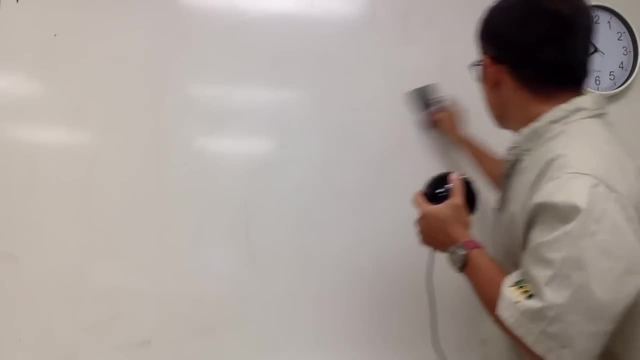 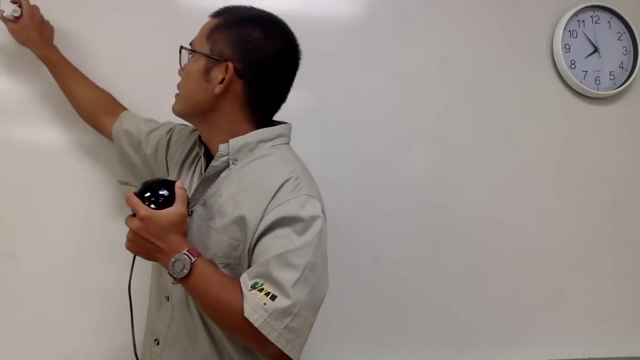 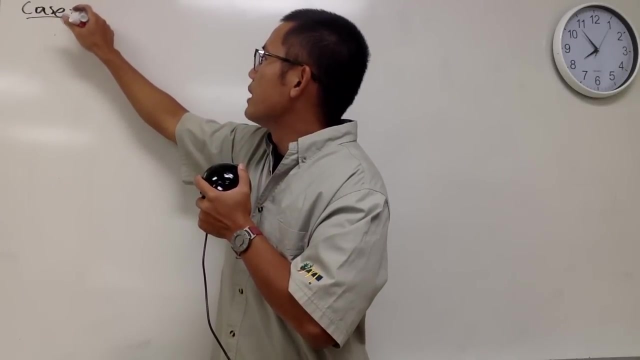 because that's just kind of repetitive compared to the other ones. So I will leave that third case for you guys. But for the other case right here, this is the other case When we have tangent and secant. so let me just put down tangent x and secant x. 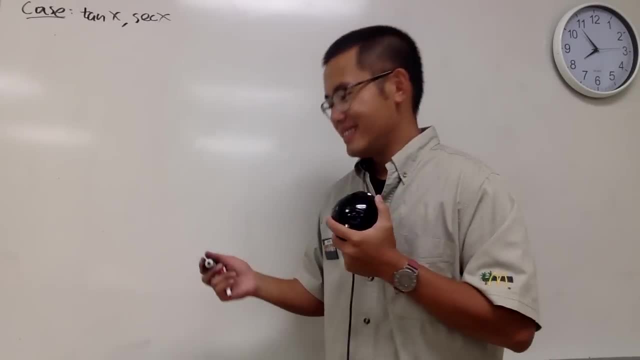 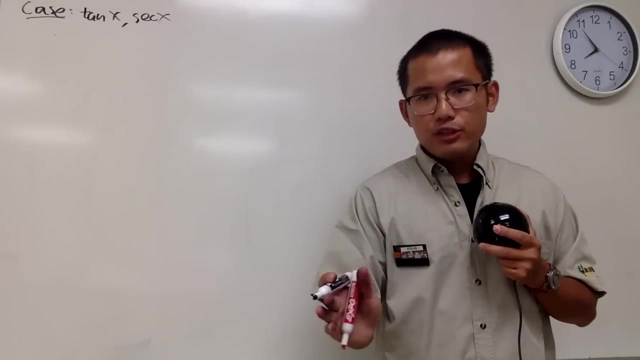 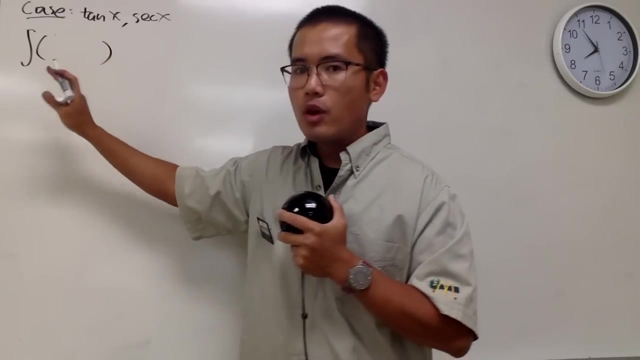 Okay, Oh man. Yeah, I know It's tiring, It's okay, We can do this. Okay, Tangent secant, Let me ask you if you have an integral, if this right here, you are able to write it. 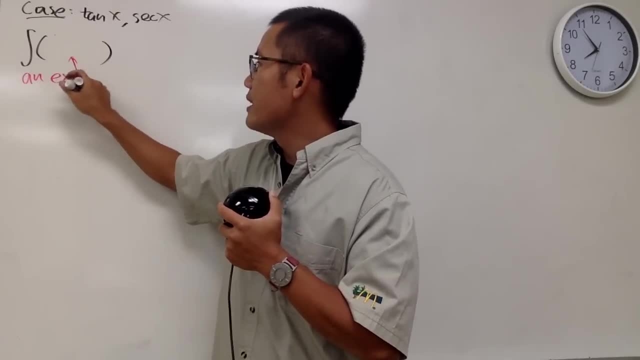 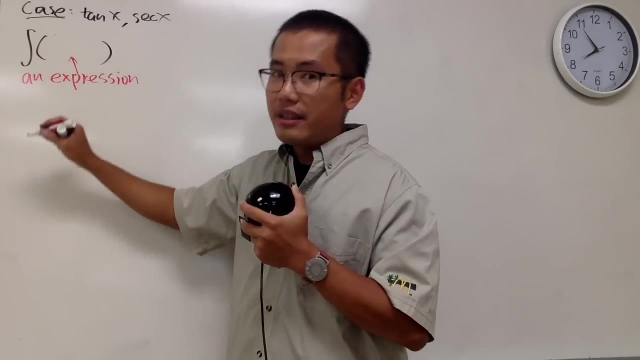 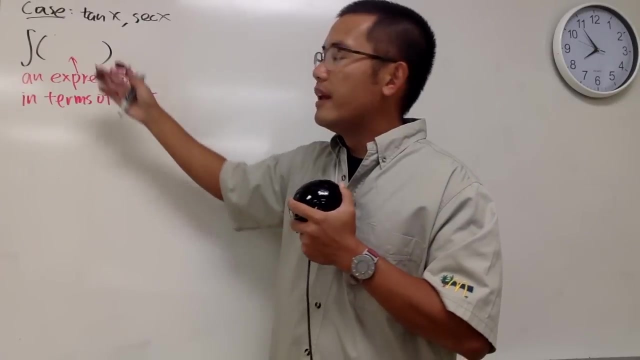 in terms of an expression. Again, let me just put this down to be slightly formal or rigorous. If this is an expression in terms of tangent x, then in that case, what do you wish to have on our side? Yes, Hopefully you guys all said it. 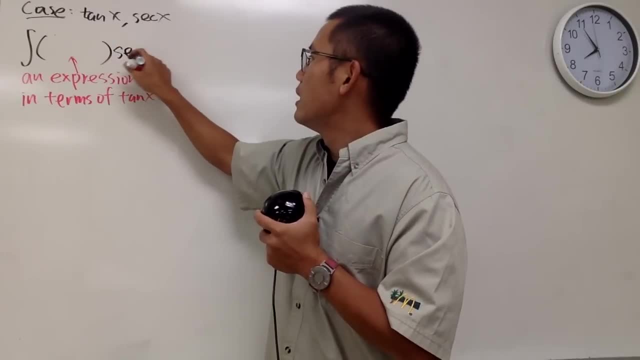 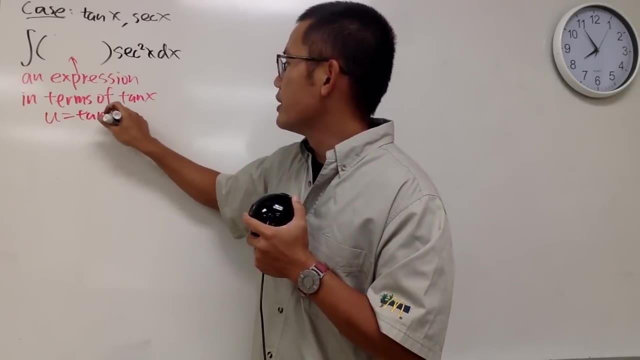 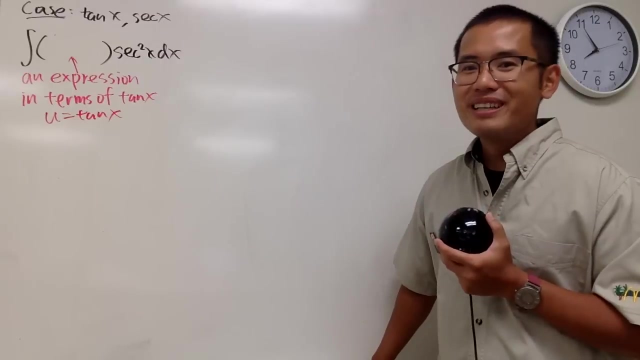 Secant squared x, dx, And the reason for this is because, well, we can let u equal to tangent x. And I know you guys are thinking, yeah, it's pretty much all about your substitution. Pretty much Because I like to say that. 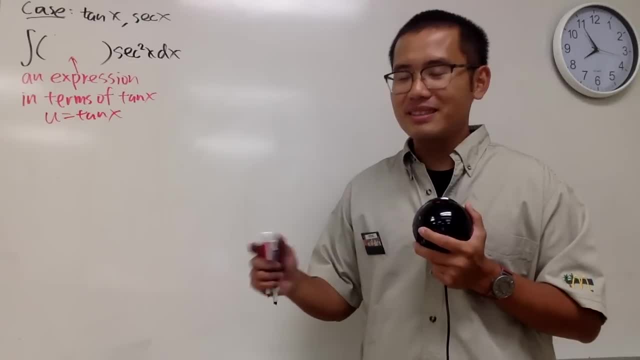 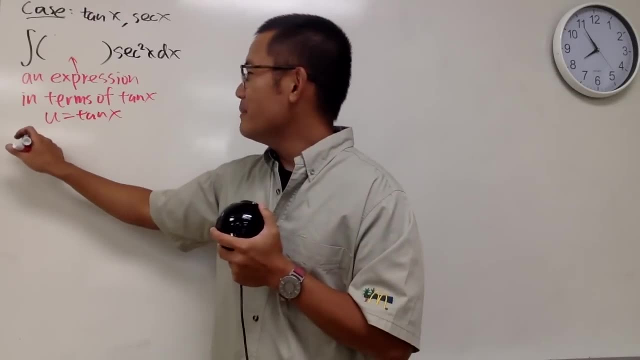 u, substitution is perhaps one of the most used technique. Right, The most used technique. It's like the backbone of integration. That's just how it is All right. Similarly, if we have a parentheses like this integral of something, and in this case, 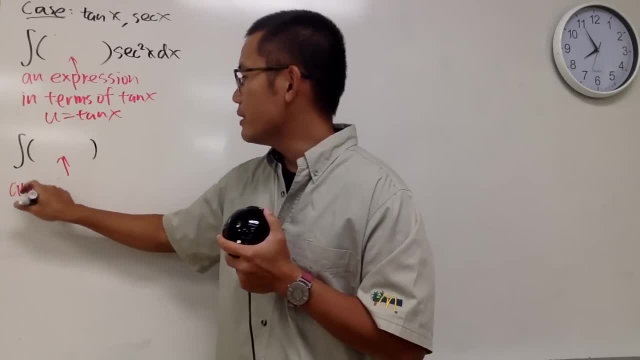 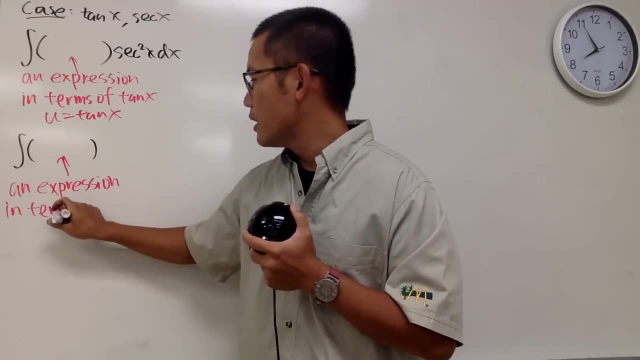 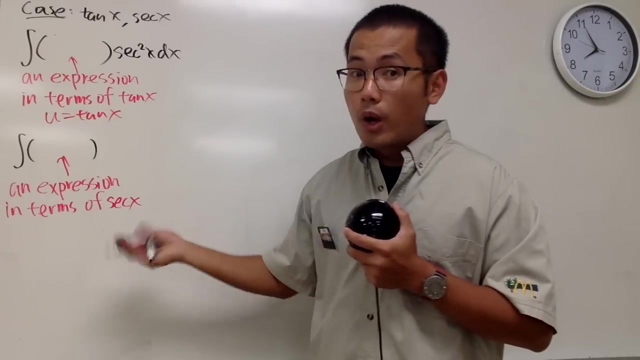 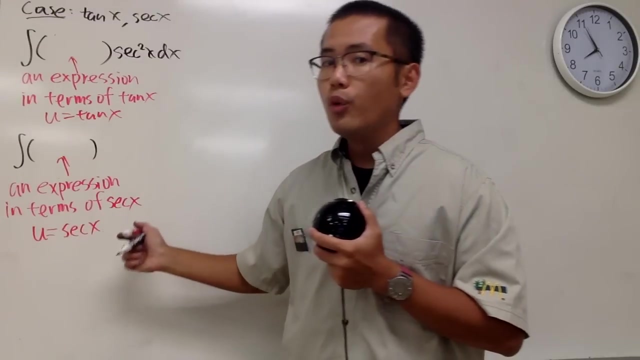 if we happen to have an expression- let me just say an expression in terms of what? Of course, Secant x. Well, in this case, you know the deal: If you want to use u equal to secant x, then we hope to have. 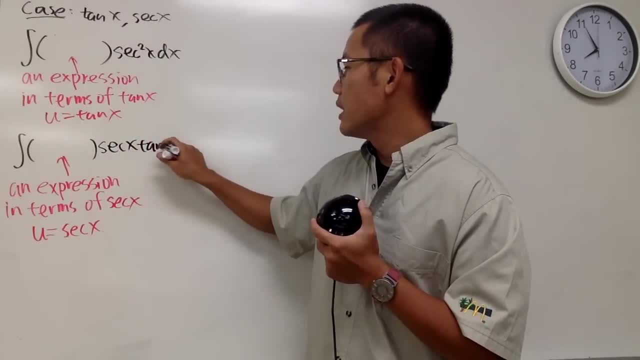 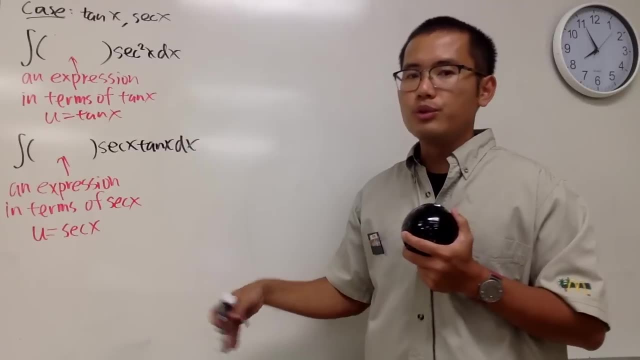 secant x, tangent x on our side to help us out. So that's another situation, The tangent-secant situation, And these are the strategies And we'll just have to use the identities to make things happen for us. And let me just put down: 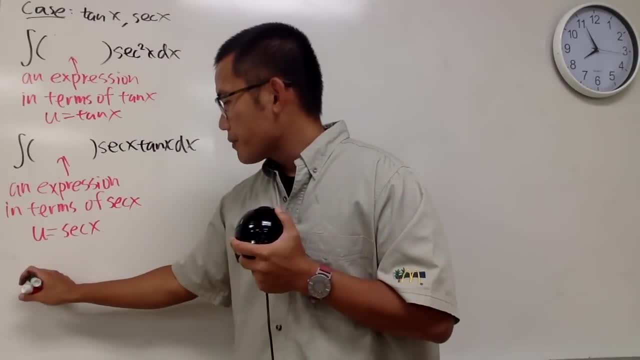 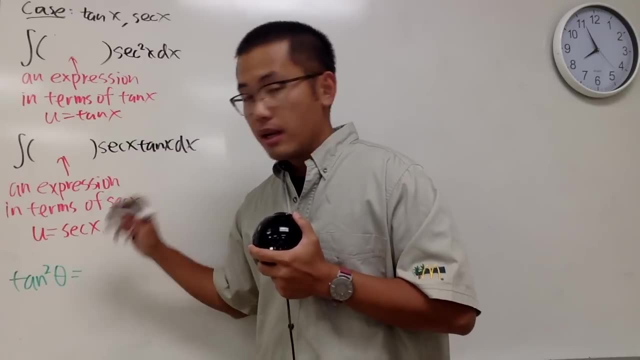 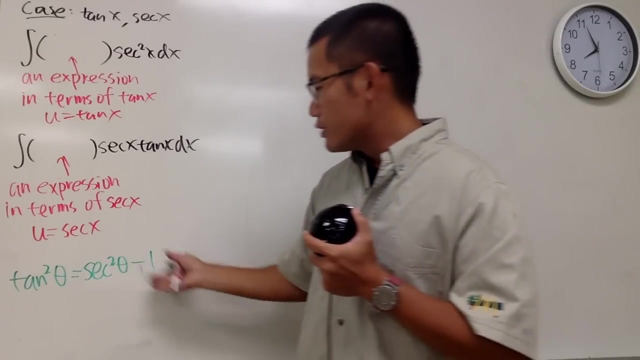 the identities right here for you guys. Well, for the identities, I'll put down theta and all that. okay, So when we have tangent squared theta, this right here is equal to secant squared theta minus one. Similarly, I can just add one on both sides. 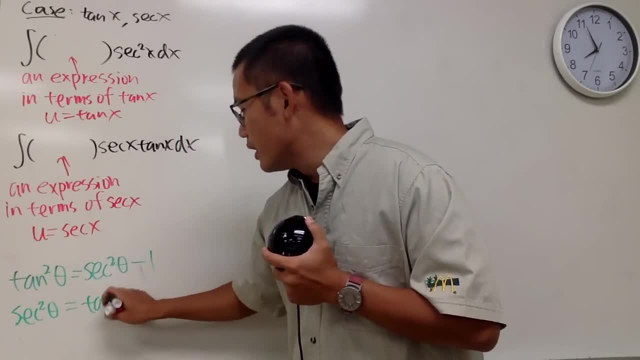 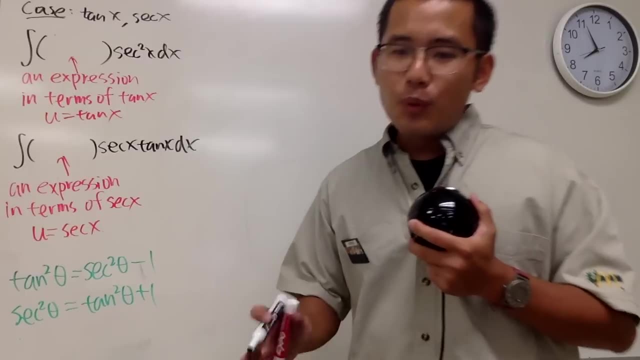 If you have secant squared theta, this is equal to tangent squared theta plus one Like that. So that's the idea. Now, again, I want you guys to try these following questions And we'll have- I'll put down three questions. 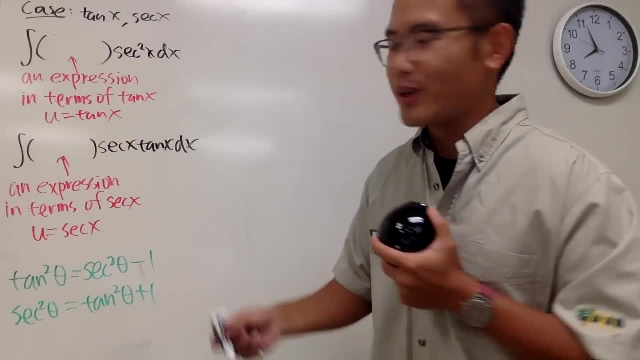 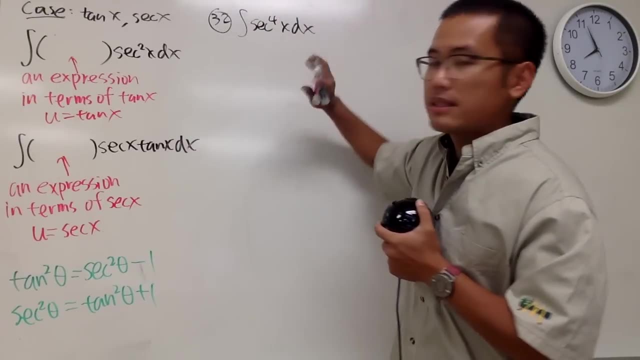 for you guys to try. Well, I just you should have been trying these questions along the way, Anyway, 32. Let's look at the integral of secant to the fourth power- x, dx, Right- And let's see how much space I need. 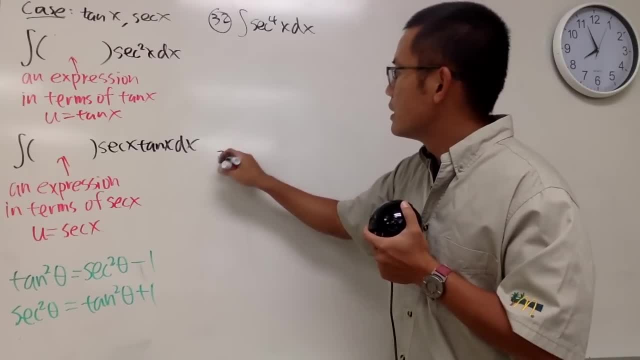 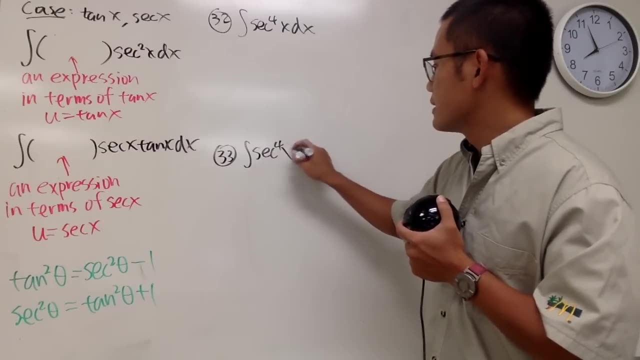 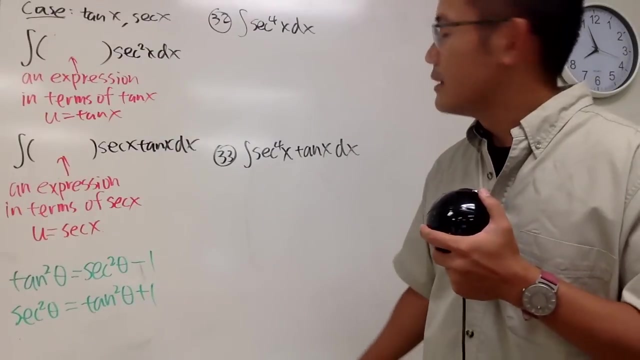 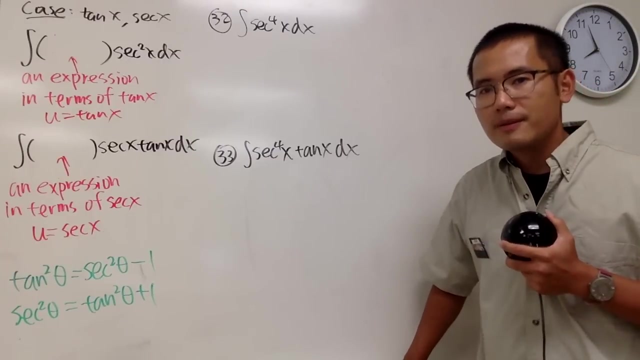 Probably I will do 33.. Integral of secant to the fourth power: x, tangent x. All right, So two questions, 32 and yeah. So pause the video and try these two questions first. I'm still here. 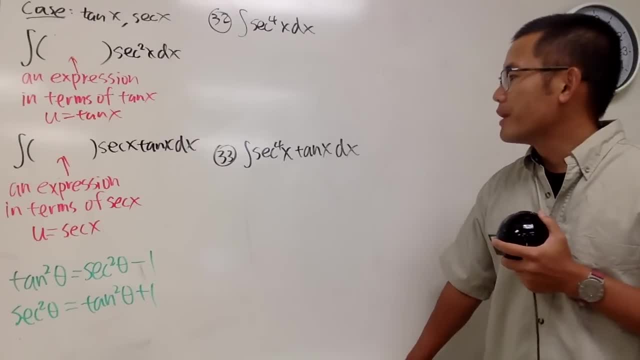 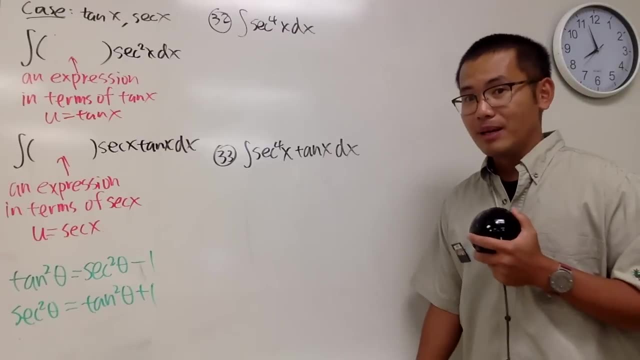 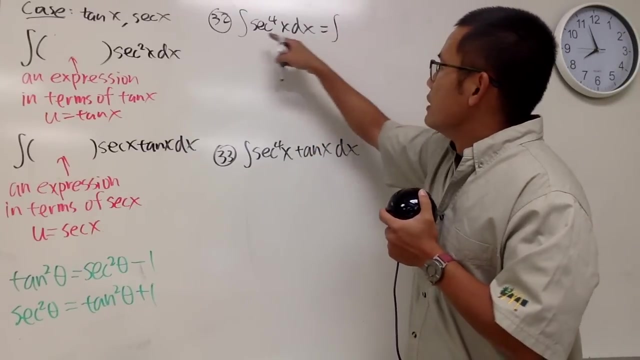 I know, Okay, So let's just do number 32 first. They look similar. just kind of have to think about how to do this too. okay For number 32.. Well, for this one. secant to the fourth power. 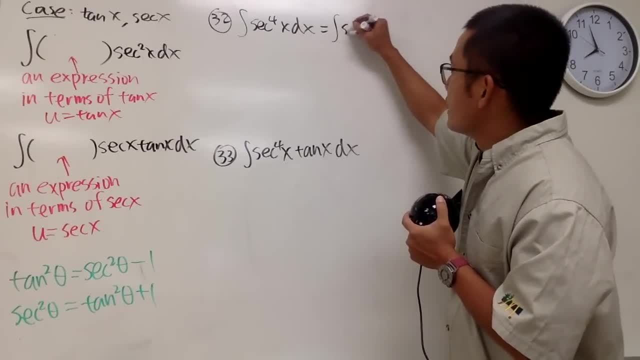 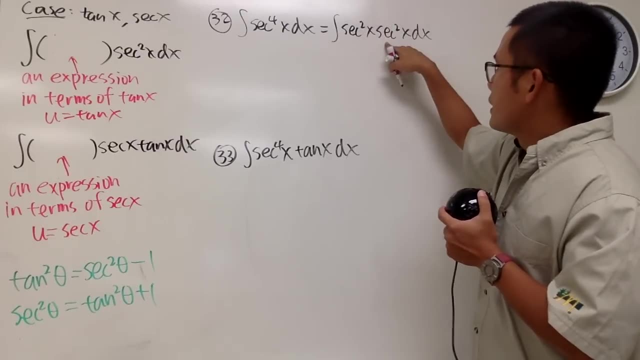 okay, we can just split it into secant squared and secant squared. That's very nice. So secant squared x times secant squared x dx. Very nice. Now this right here is secant squared x already. Can we make? 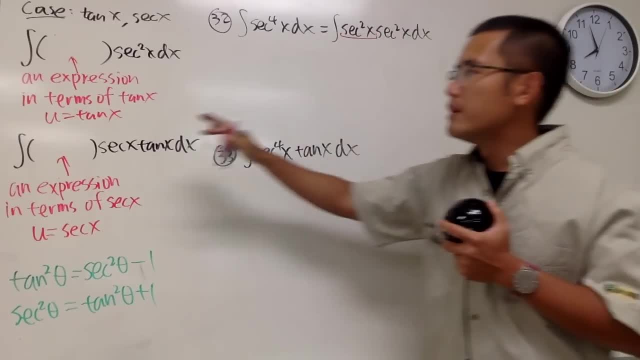 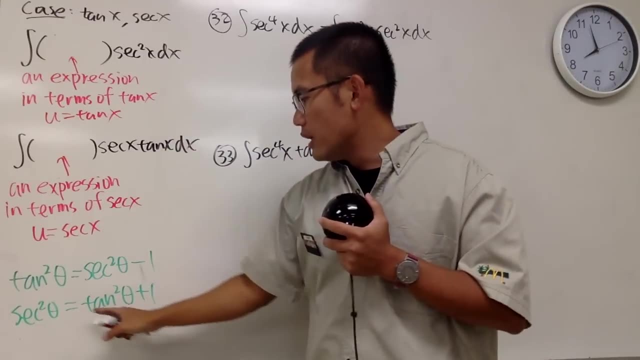 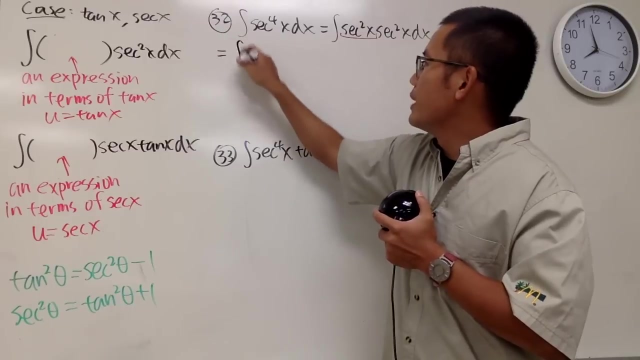 the first part, an expression in terms of tangent x. Sure, we can, Because here is just secant squared x, which is equal to tangent squared x plus 1, isn't it? Yeah, So this right here is equal to the integral. 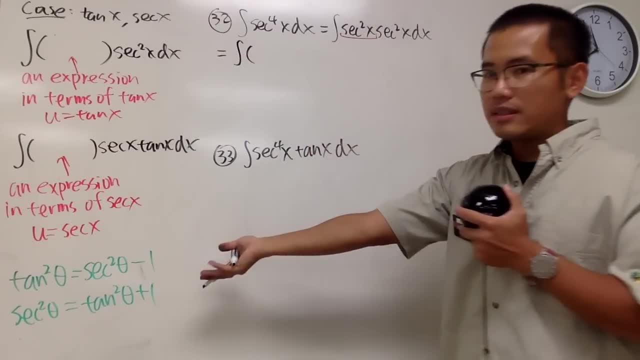 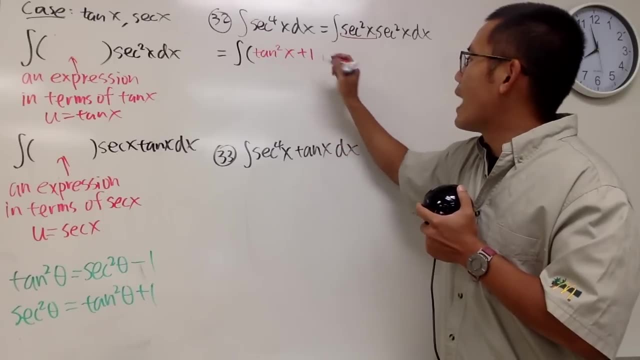 parentheses. this part is again. I'm using x. That's just the identity, so I use the theta. Here we will have tangent squared x plus 1, and then we have the secant squared x dx, like this: 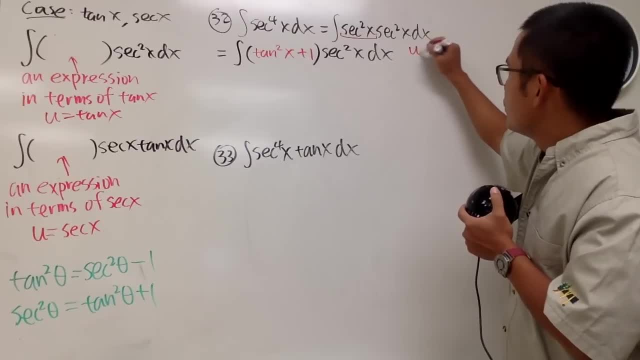 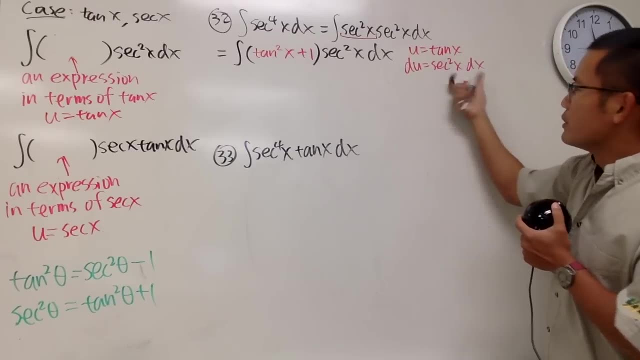 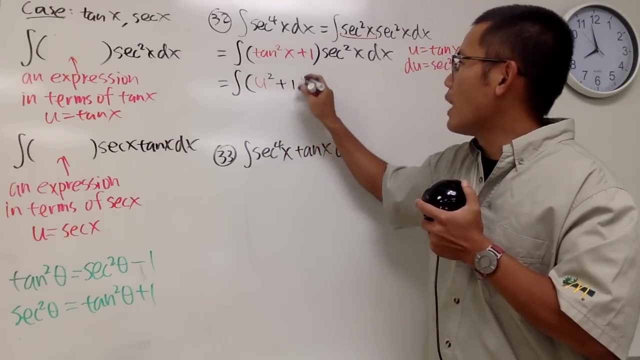 From here let's do a u-sub real quick. Let u equal to tangent x. du is secant, squared x dx, And you see, that's nicely equal to our du. In another word, we get the integral of u squared plus 1,. 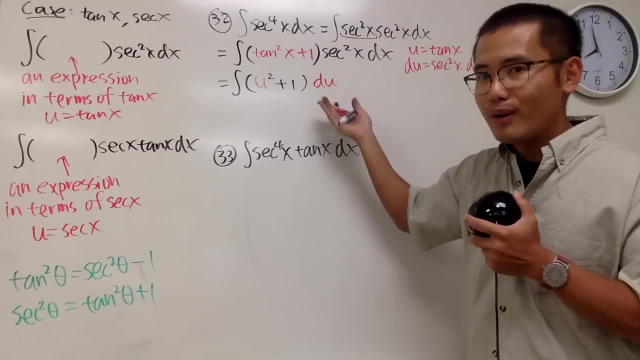 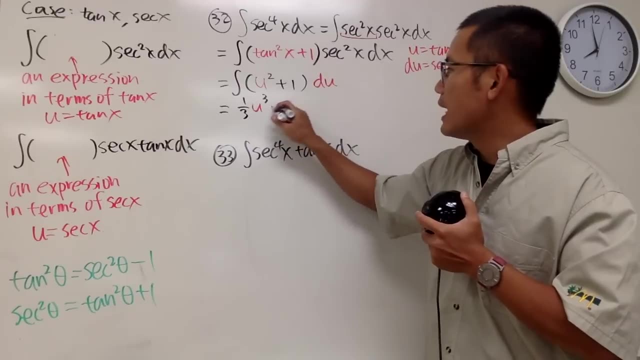 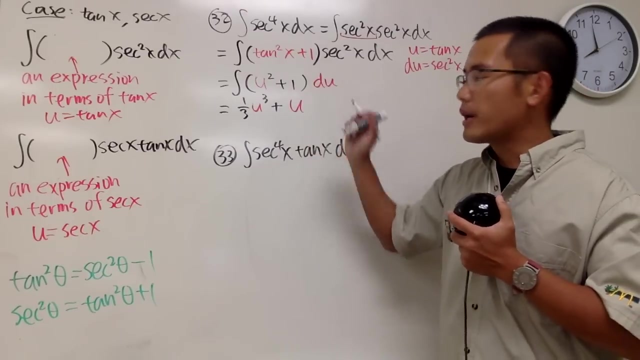 and this right here is d? du Now. integrate this in the? u world, we get 1? third? u to the third power plus. I really want to emphasize that. this one 1, integrate that in the? u world, we get u. 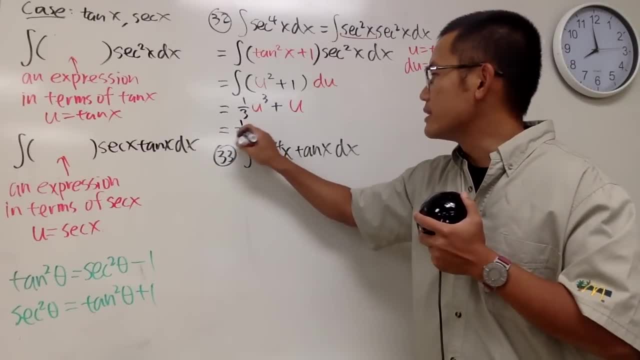 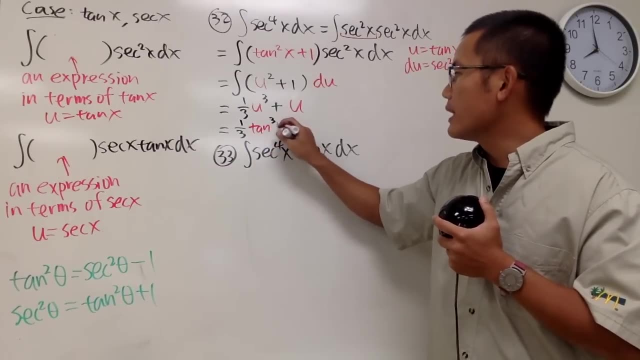 okay, And in the end, of course, go back to the x world. This is 1 third. In this case the u is tangent, so we have 1 third tangent to the third power, x, plus tangent of x, like this: 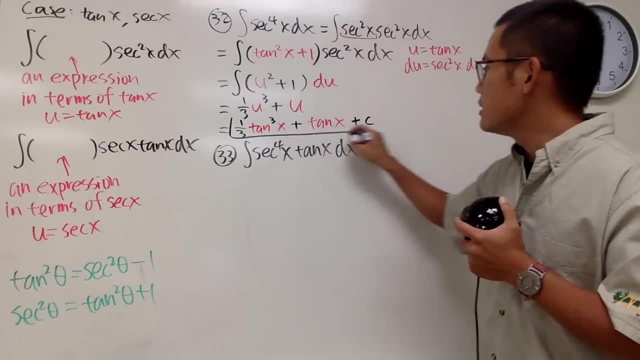 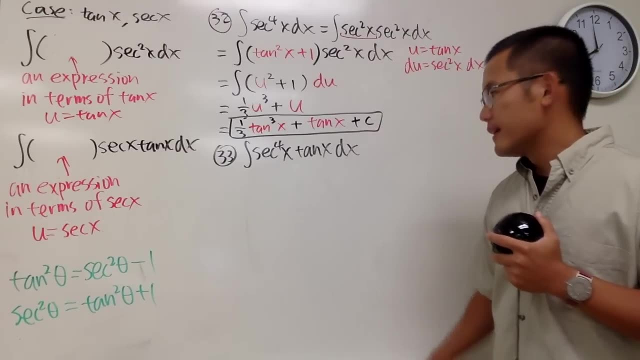 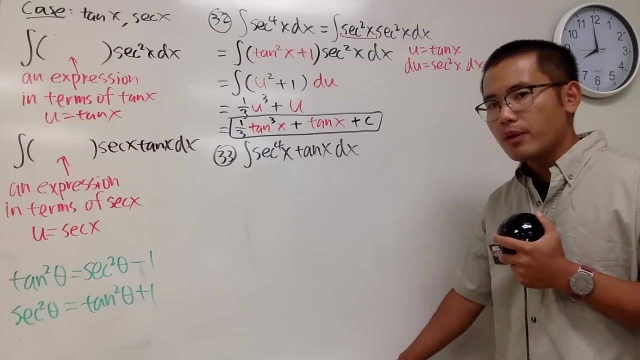 And we are all done. therefore, of course, put on a plus c, and that is it All right. Now for number 33, and let's see how can we do this. I have a tangent factor. I have secant to the fourth power. 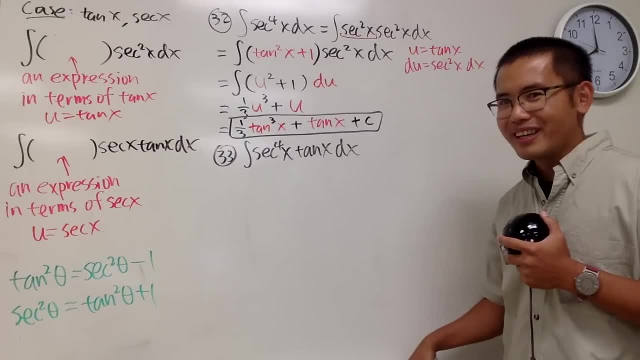 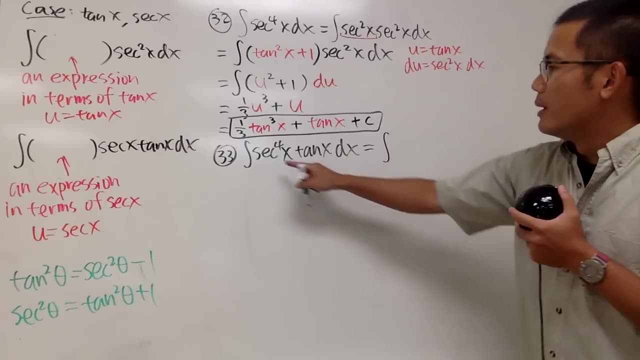 I think that's too much. that's too many secant. Why don't we just take one out? So have a look here. Let me do it this way. Well, can we look at this as the integral? put one of this right here. 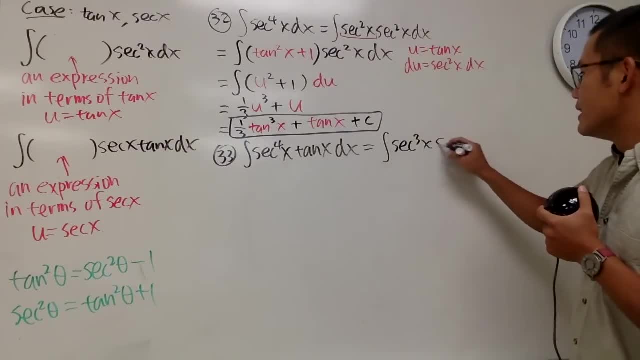 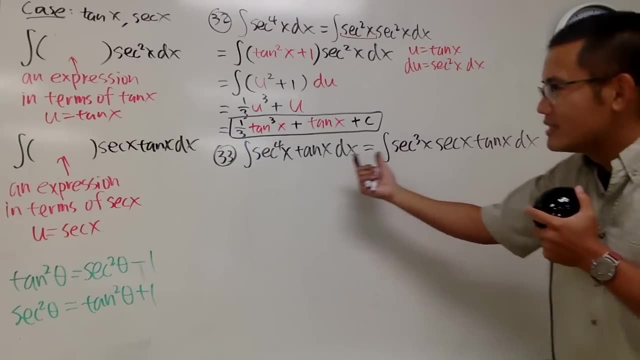 so we are looking at secant to the third power, x, and then we have secant x times tangent x, dx This times. that, of course, still gives us secant to the fourth power, and that's very nice. Now, 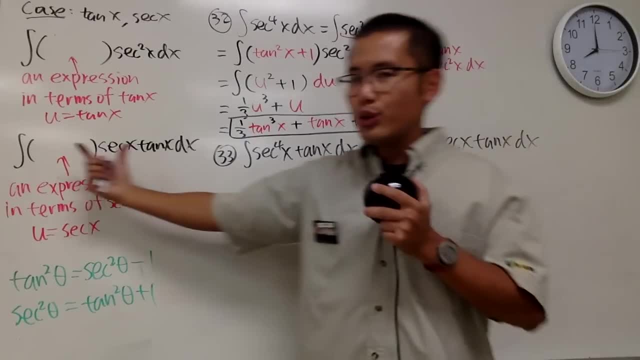 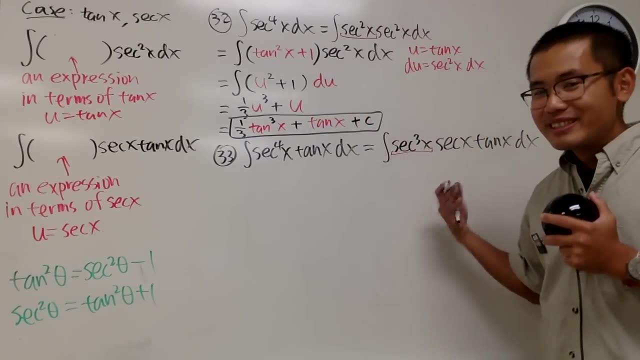 we have all this secant x times tangent x. Do we have an expression in terms of secant x? Yes, we do. That is right here. That's very nice. So this is actually very easy to do because we can just. 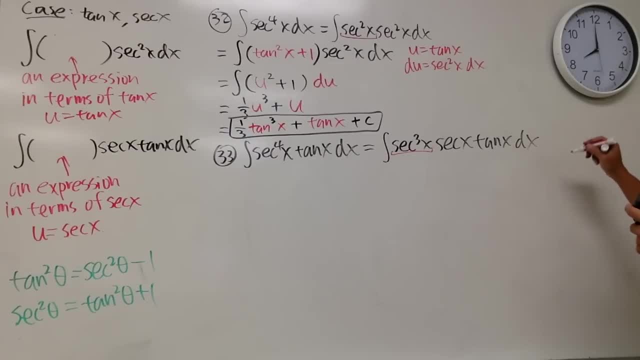 take a u sub. we can let u equal to that and I'll actually put this down here. I will let u equal to secant x and we can see that du is equal to secant x, tangent x, dx. So. 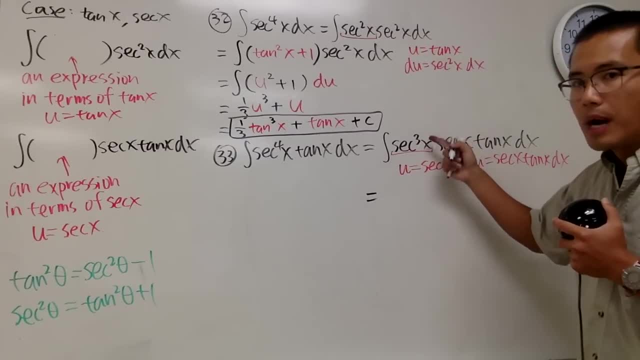 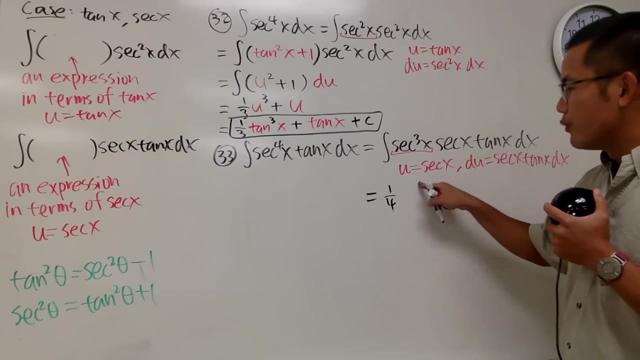 in the end, you will see that we just have to integrate? u to the third power in the? u world, and I will leave the detail to you guys. You end up with 1 over 4? u to the fourth power, which is: 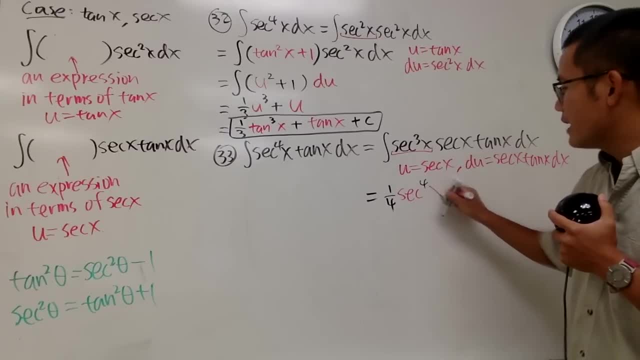 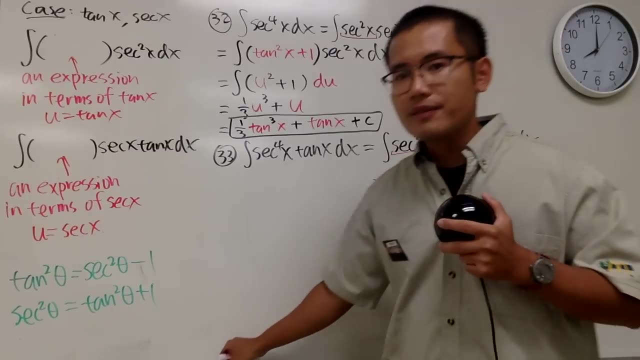 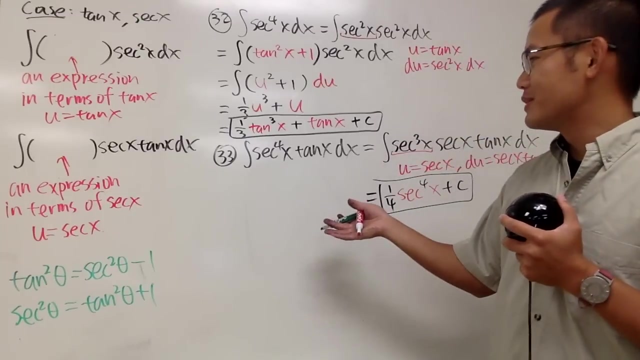 secant to the fourth power and we have the x plus c Like this Right. So this is good, This is great, This is wonderful. But what if you didn't do it this way? What if you really want to just 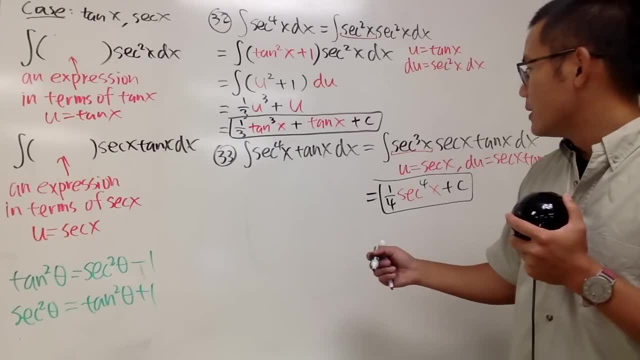 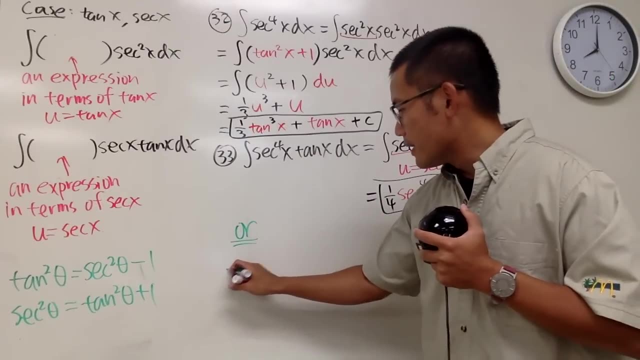 have the secant squared to look at. Well, let's have a look. So this is nice, Or I will just put down, or right, If you look at this as follows. as follows: if you put down, if you put out. 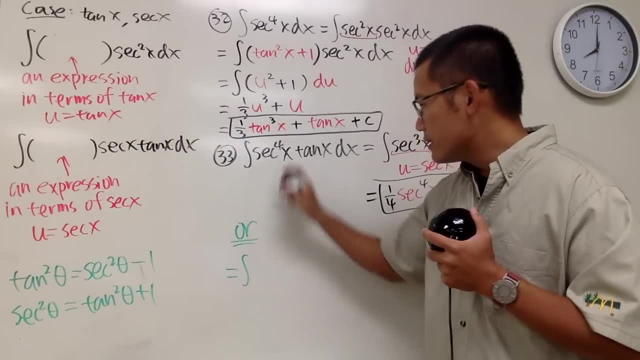 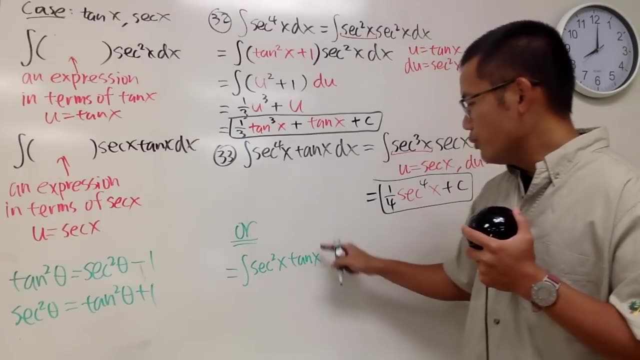 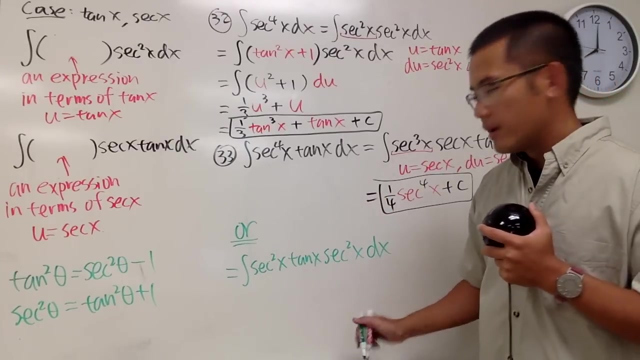 two of the secant squared. so if you're looking at this as secant squared x times tangent, x times two more right here, because all in all you must have four right. If you look at it this way, here you have. 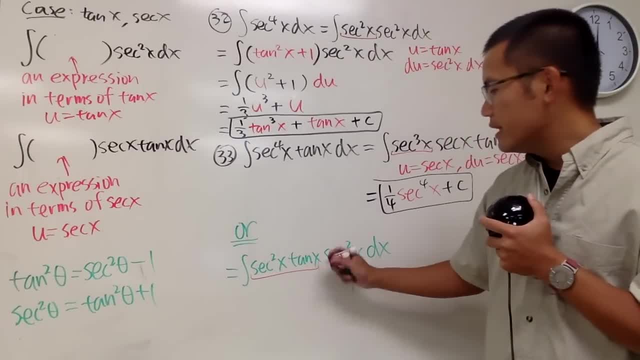 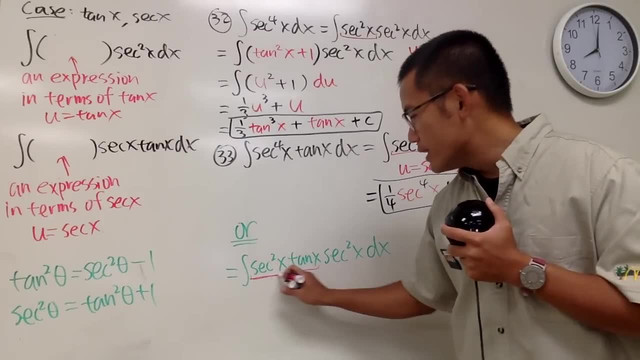 secant squared x. Well, in that case, can we make this part an expression in terms of tangent x? Yes, Because notice how this part is just equal to that which is x, of course. So of course, I can put this down as: 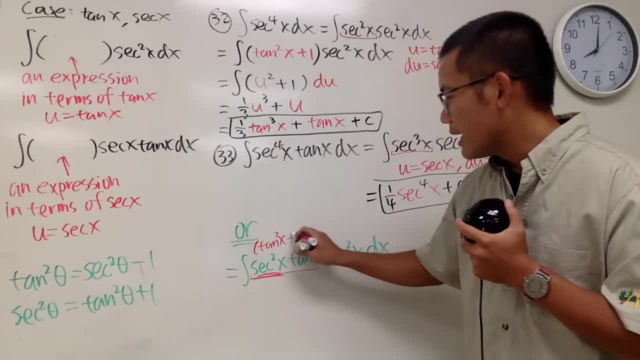 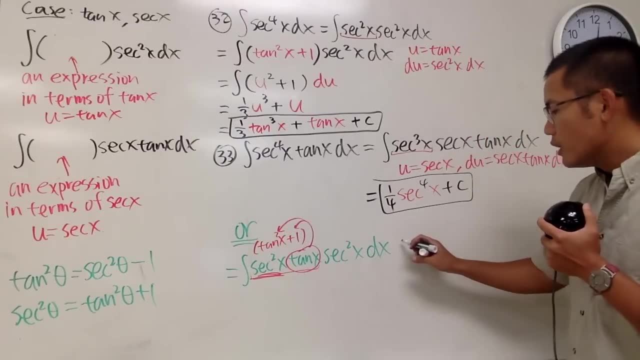 tangent x or tangent squared x plus one. And don't forget, we still have the tangent x right here, So we can distribute, distribute. So you notice we actually have the integral and this whole thing together is. 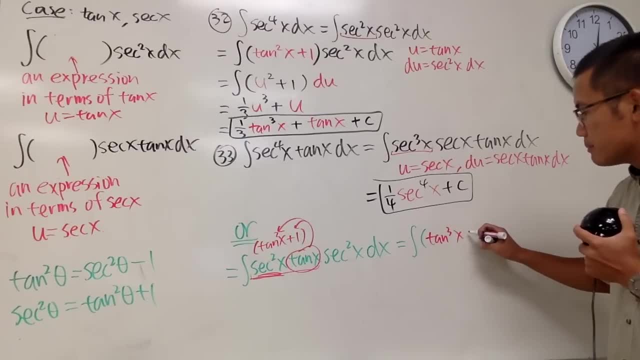 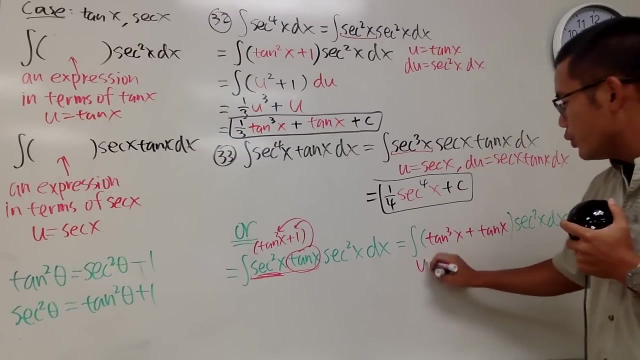 parentheses: tangent. third power x plus tangent x. Yeah, And then we have the secant squared x, dx, right here. If we do it this way, well, well, u will be tangent x, du will be secant squared x. 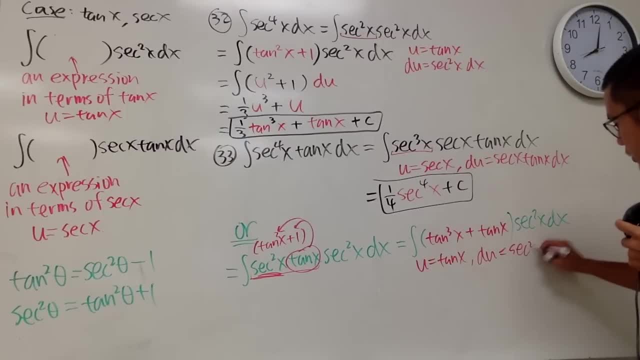 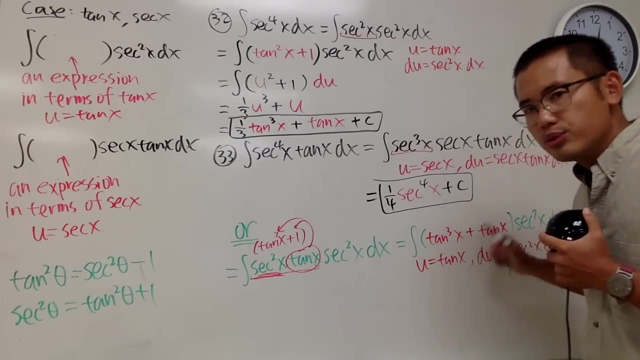 dx. This is the du And you have u to the third power plus u to the first power. Well, in this case- again, I will leave the details for you guys to work out- u to the third power, integrate that. 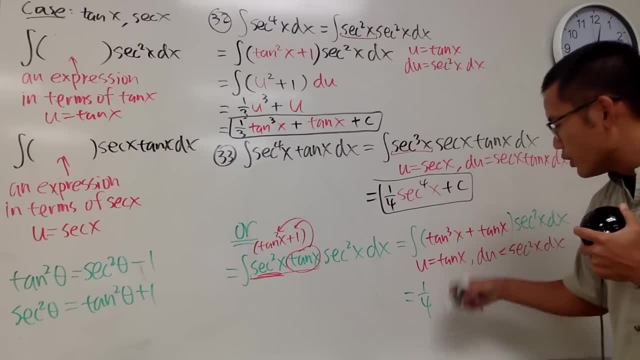 we get one over four: u to the third power plus u to the fourth power, So that's, in this case, tangent to the fourth power, x. Then integrating this. well, it's u right, So we actually end up with: 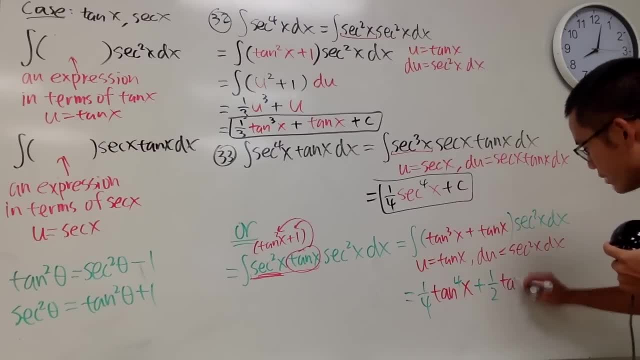 plus one half u squared, and that's one half u is the tangent, So it's tangent squared x, like this, And when we're done we put down the plus c. Hey, this looks legit too. Look at that. I don't think. 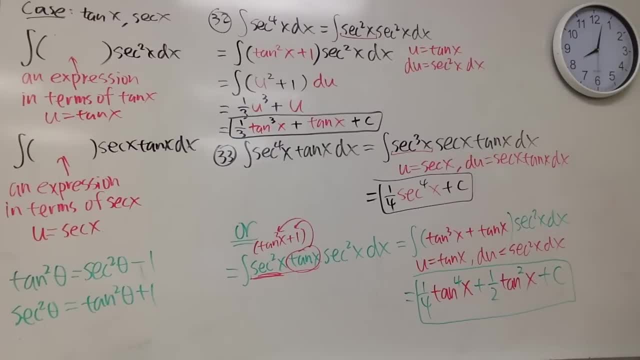 I make any mistake? Huh, Oh, sorry, blocking you guys. So take a look. Ah man, I seriously don't think I make any mistakes. Did I or did I not? I don't think so, But 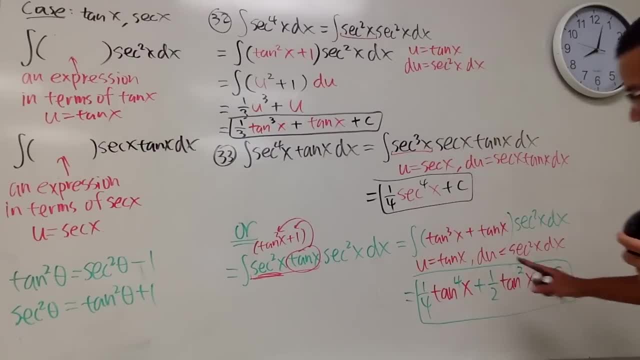 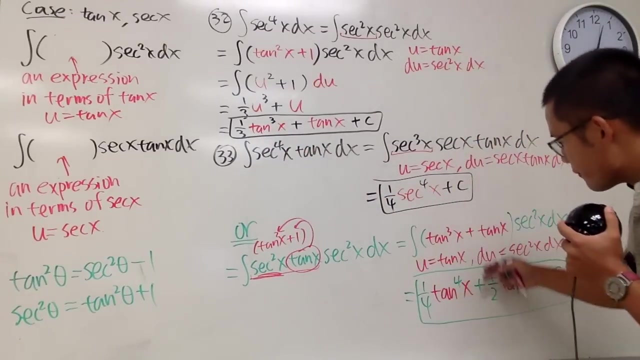 this and that they look so different. What's the deal? Well, here's the idea. The truth is, if you differentiate this function and you also differentiate this function, you will actually end up with both of them. will give you this for the derivative. 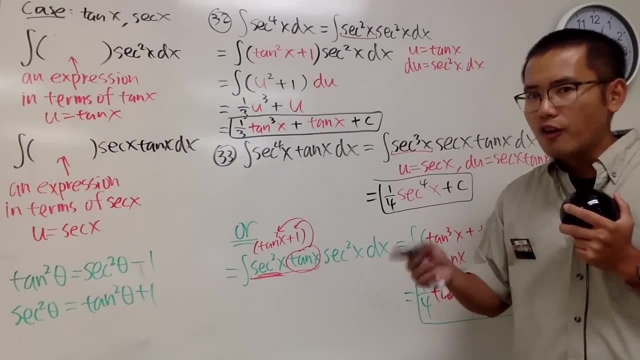 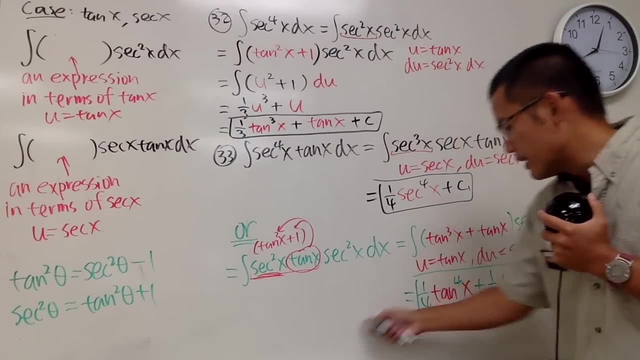 However, the constant here and the constant here, they are very different. They are just off by a constant. So technically, I will just tell you guys, maybe this is a c1. In that case, I will label this as c2.. 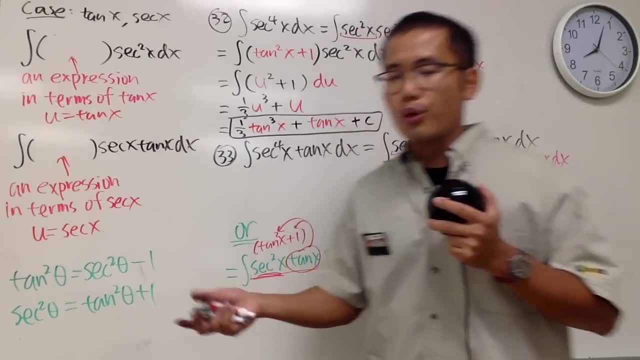 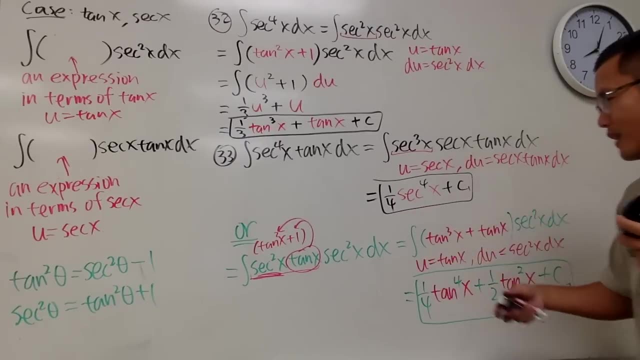 It's just off by a constant, And usually I will just show you guys a computer program and you can get on your GeoGebra- which is the program I like the most besides the Wolfram Alpha- and you grab this. 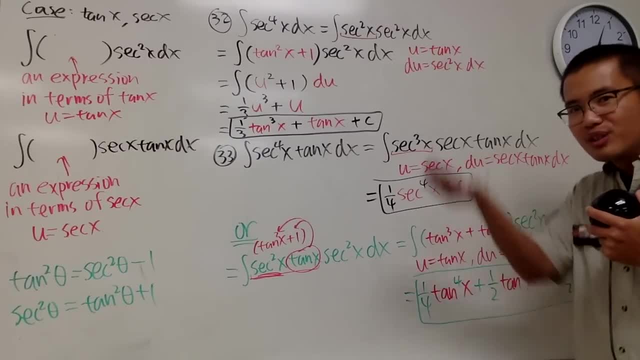 you will see that they have the same shape by just off, by 1 over 4.. So I'm going to leave that to you guys because I want to show you guys the computational technique for all the integration. But if you guys would like, 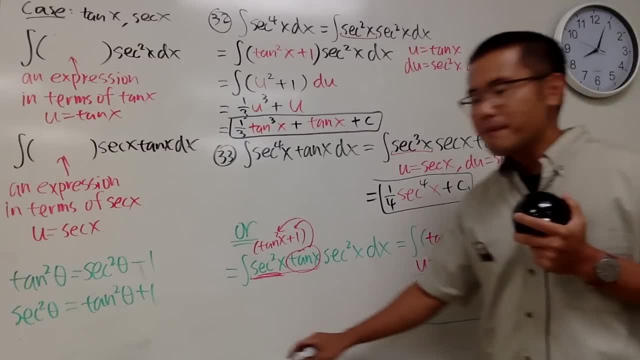 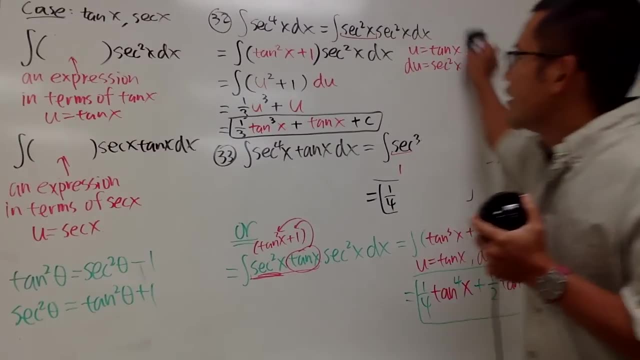 you guys can leave a comment down below. I will do a video for you guys with the software. Yeah, So this is the idea. This is question number 33.. Okay, Pretty good, pretty good, And now let's compare two more questions. 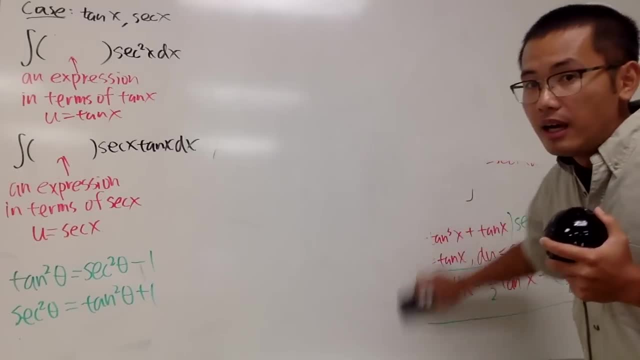 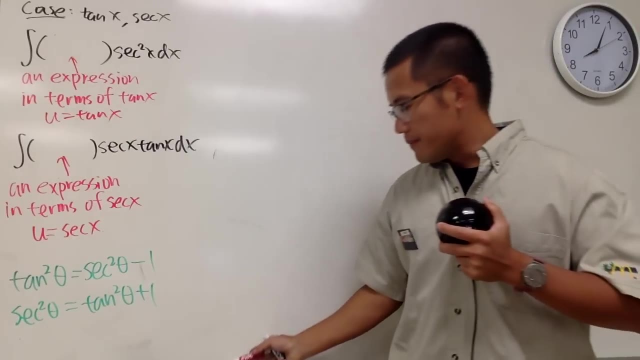 Still tangent and secant. And keep in mind, this video is just like introduction to the integration techniques, So it's like an integration technique for beginners And if you want to be good at it, you really have to do a lot more practice. 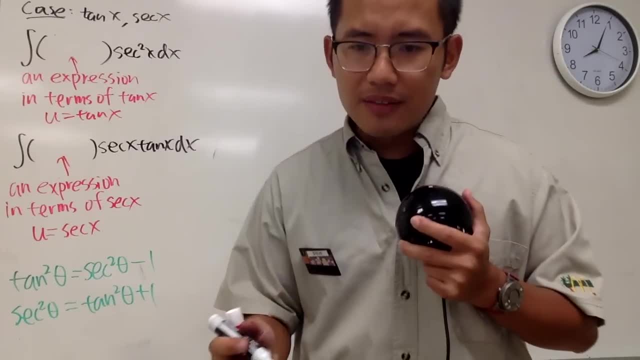 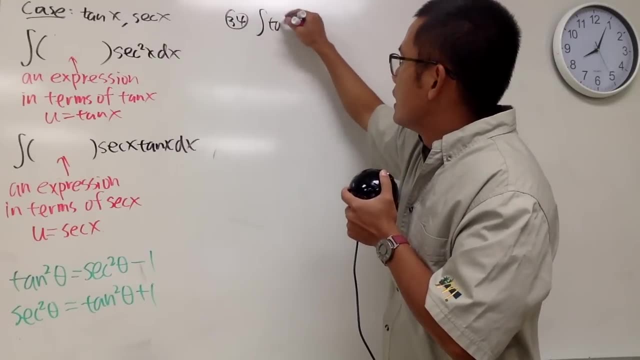 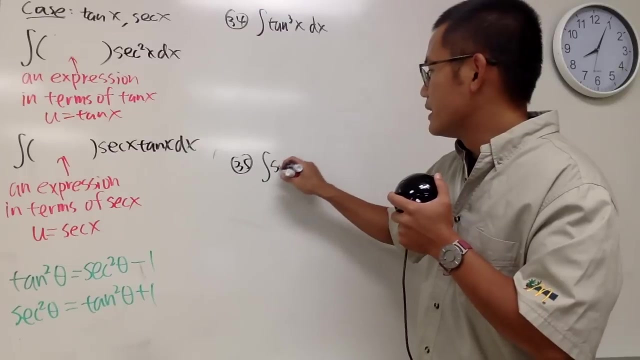 than just 50, right. Anyway, we have two more in this category. I want to put it down: number 34. Okay. Integral of tangent third power x, dx. And number 35. Integral of secant to the third power x. 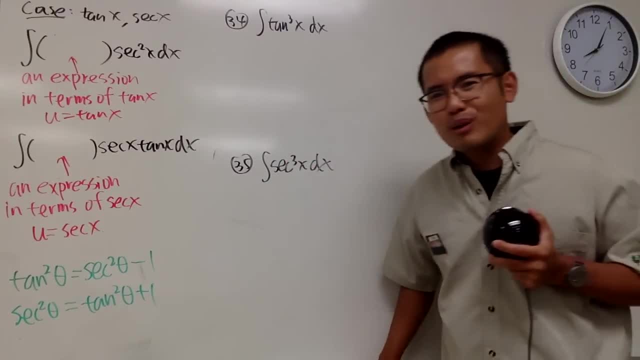 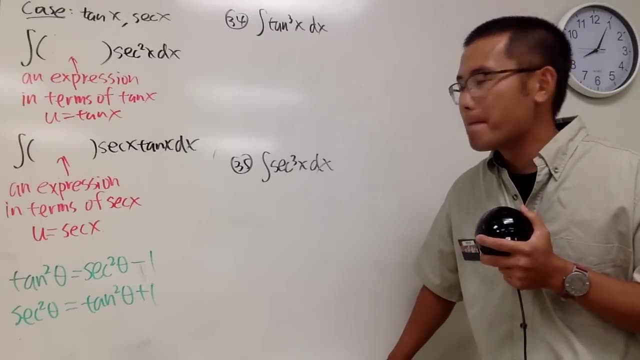 dx. I know I did a fourth power earlier and now I'm talking about third power. In fact, the third power for secant is harder. Yeah, I know We only have 15 questions. Well, actually we have a lot more questions. 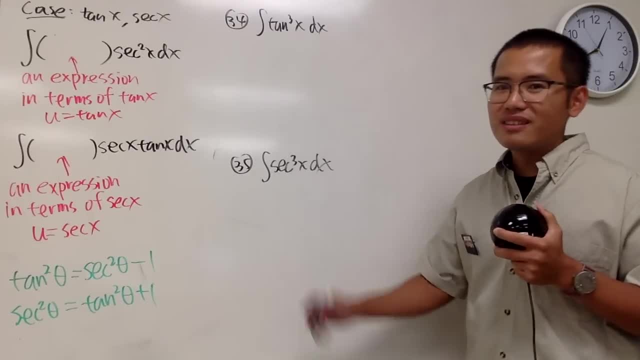 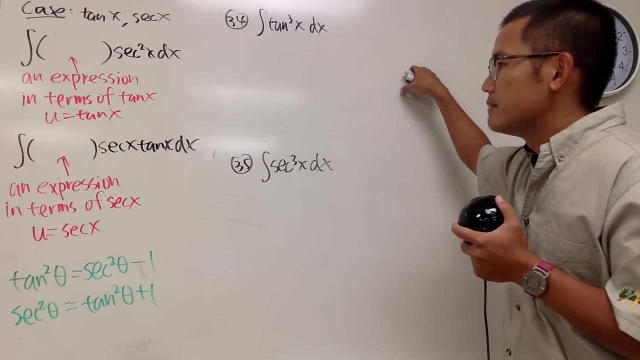 to go over. Anyway, stop complaining Which one's easier, This one's easier, Let's do this one first. Okay, Let's see, Let's see, Let's see. Hmm, We have tangent to the third power. Well, 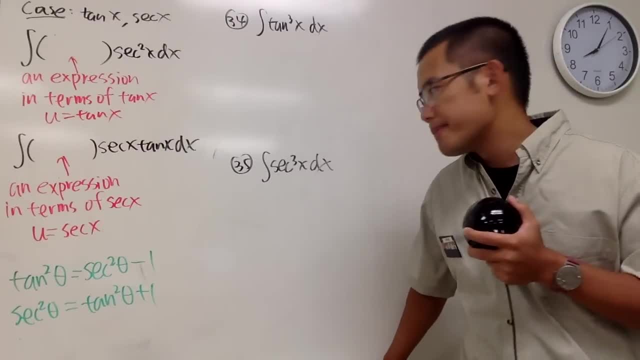 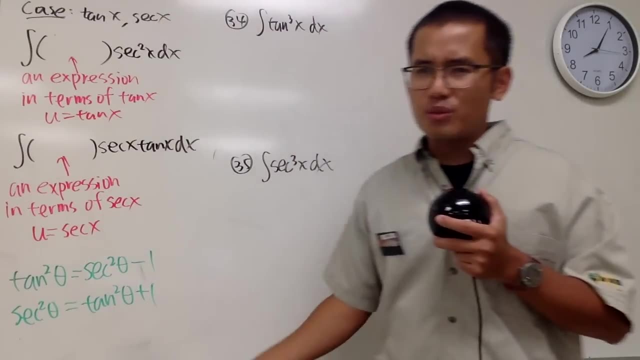 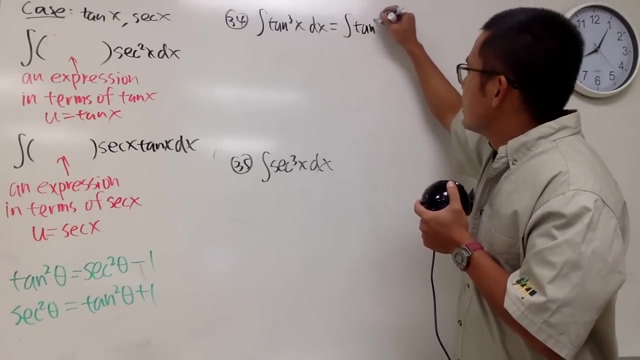 we can draw, we can make some change if we see tangent square. So maybe that's breaking apart anyway. So if we look at this, let's look at this as integral and let's look at this as tangent square x times tangent x. Okay, 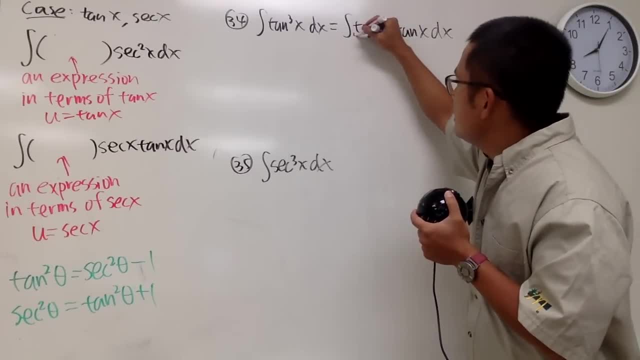 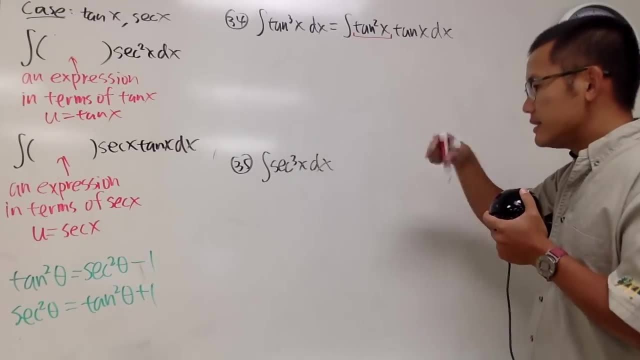 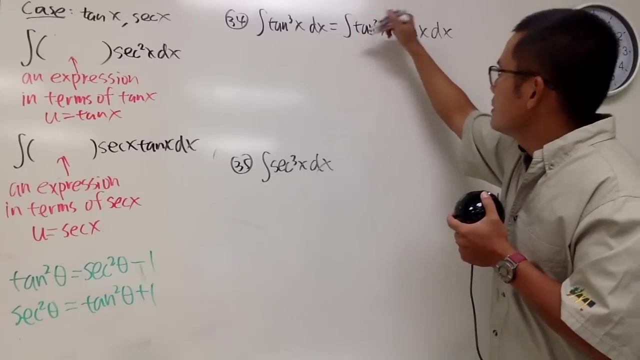 Pretty good. Well, in this case, here we have that, Right, So we can look at that as secant square theta And let me just write. let me just let's put this on like this: I'll put our parentheses on the top. 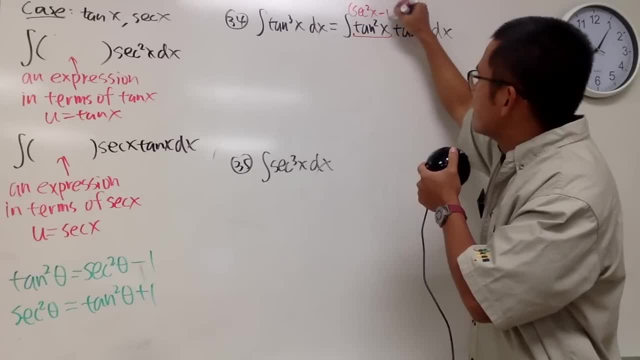 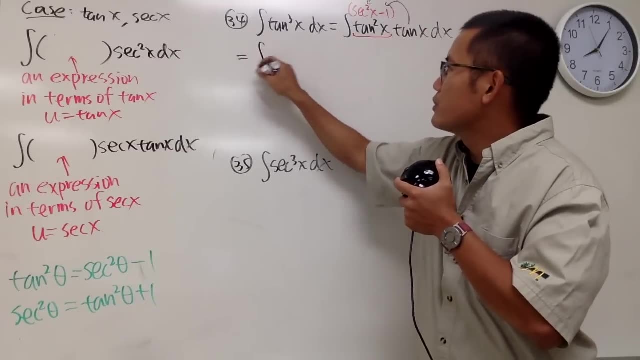 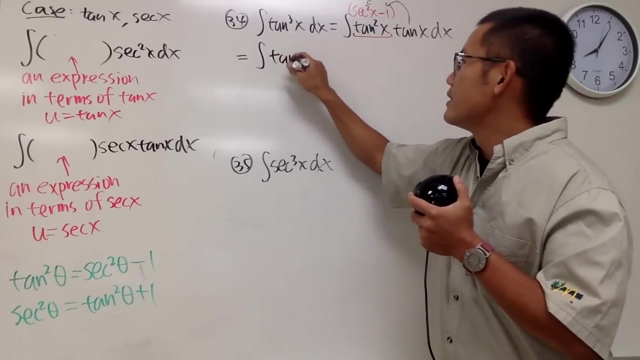 which is secant square x minus 1, like that, And of course we have the integral. So we see that this is actually the integral and we have the secant square times tangent x. Let me put down the tangent x first. 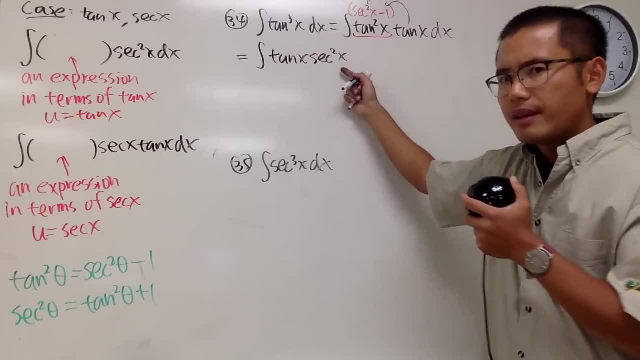 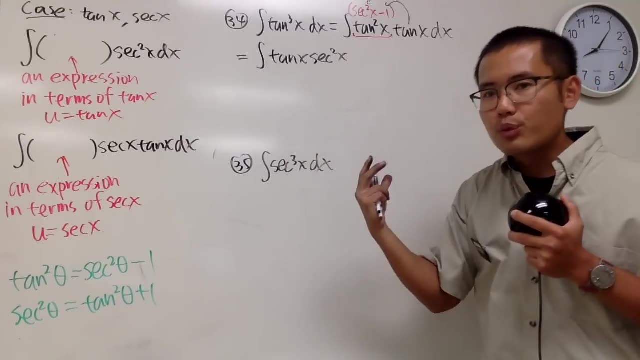 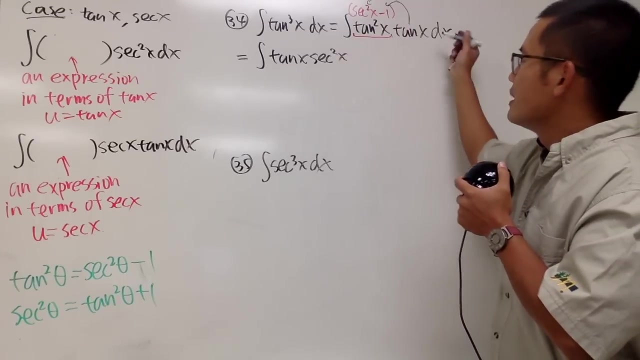 Tangent x: Yeah Times secant square x. Can we integrate this? Yes, And remember, you see we have a subtraction in between, So we actually have two integrals. We can just split it because we have two integrals. 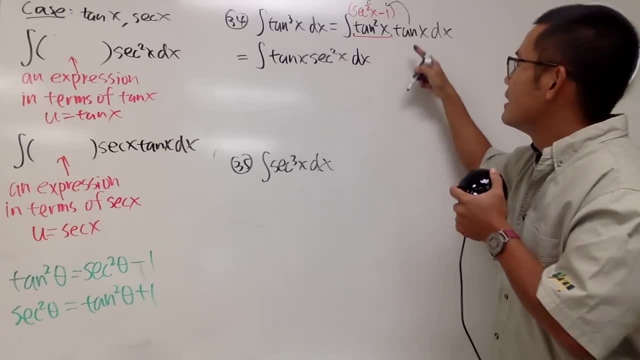 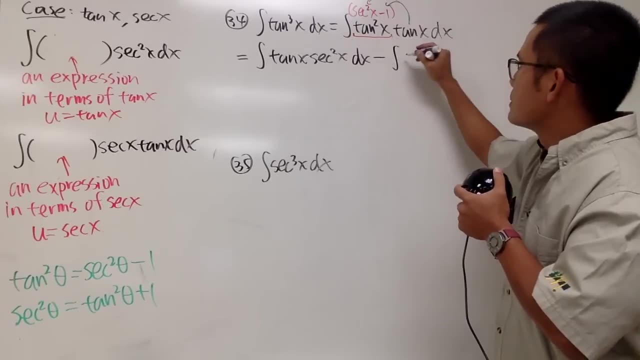 So let me close this integral by putting down the dx Next, Right here. I'll do this: times that, and this is still an integral, So it's minus integral. and then we have tangent times 1, which is just tangent x, like this: 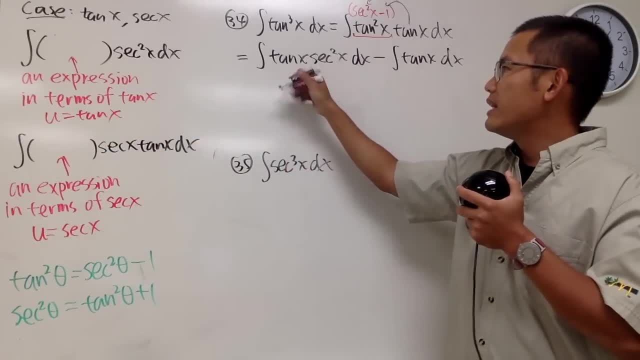 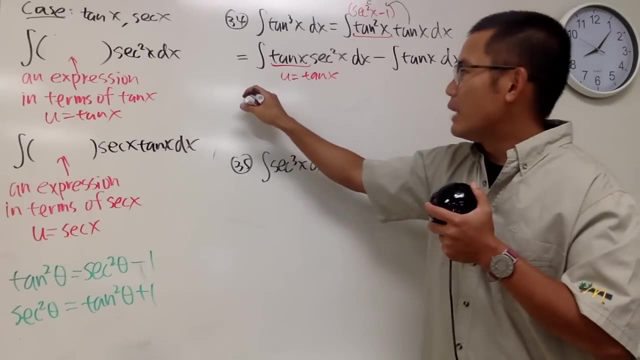 This one. hey, we can do this because we have tangent right here, and you can, of course, let u equal to tangent x, and that will pretty much do the work right On your own. For this part, you end up with integrating u. 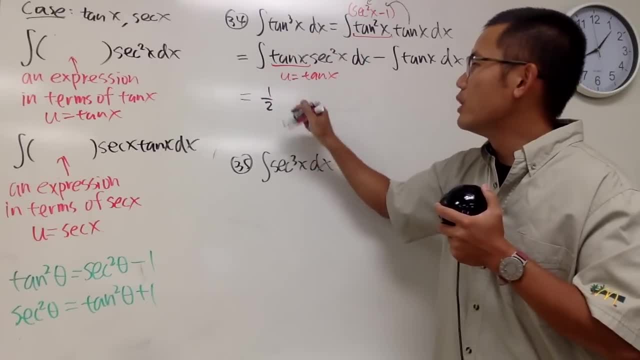 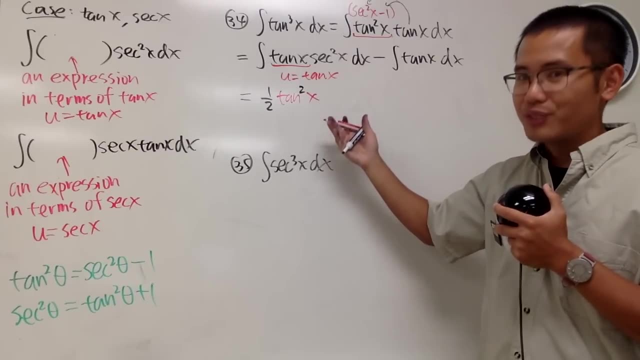 in the? u world which you'll get 1 over 2, u squared, and that's just tangent squared x like this. That's it for the first part. For the second part you have to remember the answer right Minus the integral. 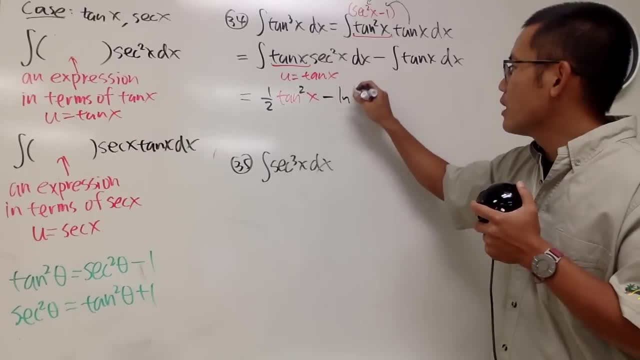 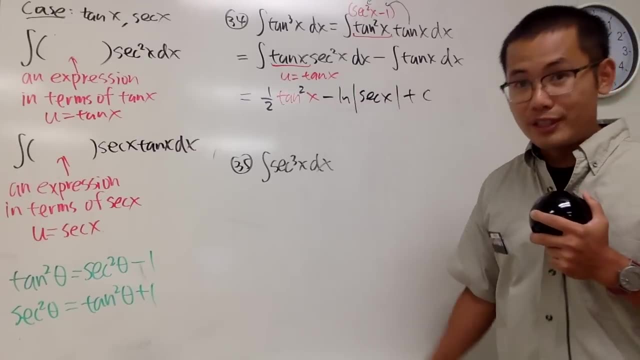 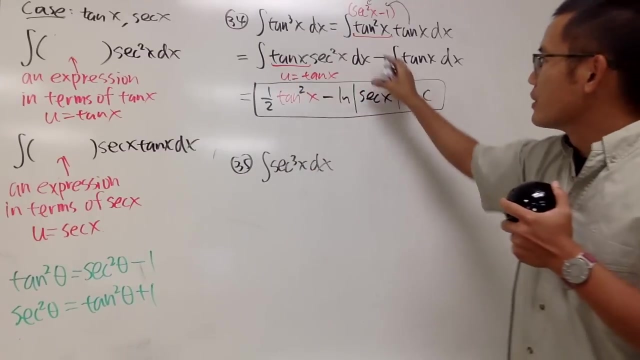 of tangent x is natural log absolute value of secant x. How do we know? Because we did it already. So a lot of these questions, they are all set up, it's all based on the things we did before. So again, 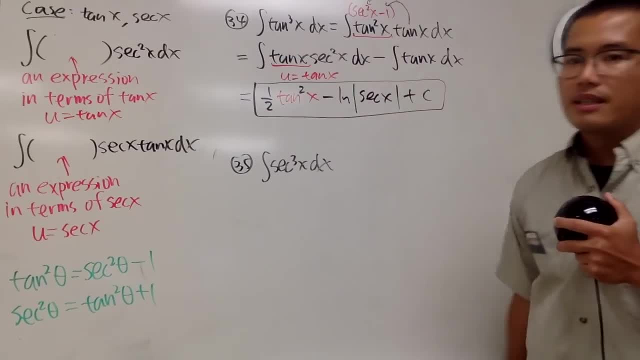 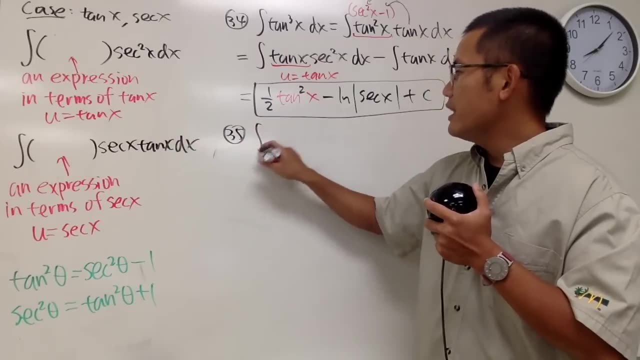 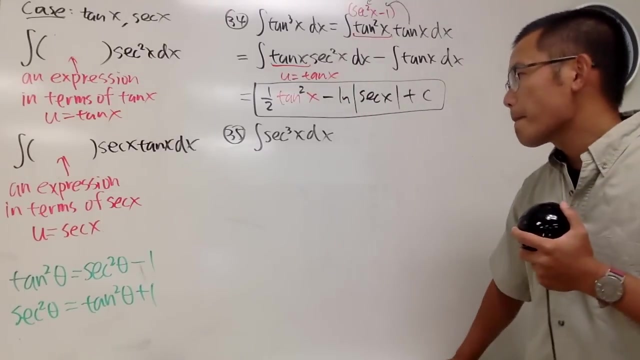 this right here is for that, and this is this, okay. Okay, and then for question number 35, I just want to have more space, so let me rewrite it here: Integral of secant to the third power of x, dx. All right. 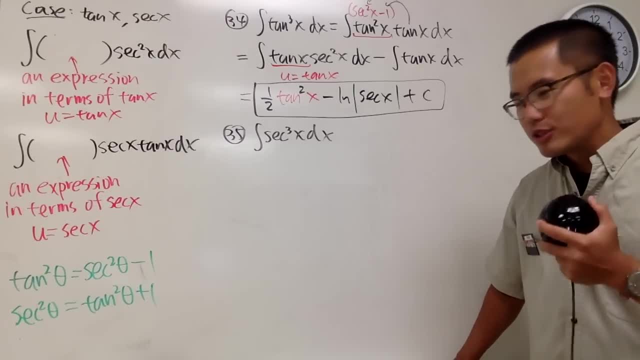 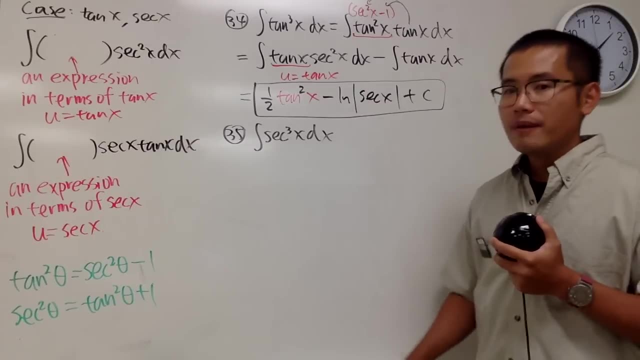 This is not easy. this is not easy, okay, But you should just practice a few more times. you should get comfortable with it so that you will think that this is actually easy, And once you feel like, hey, this question I can do it. 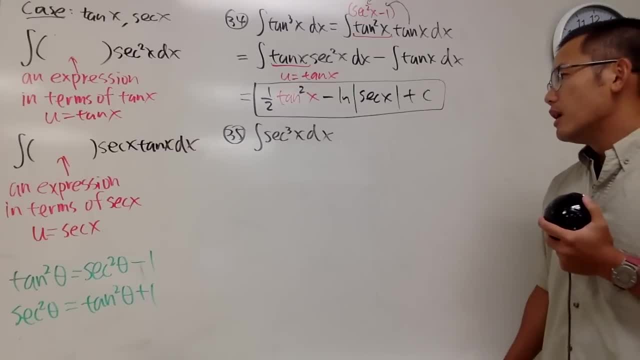 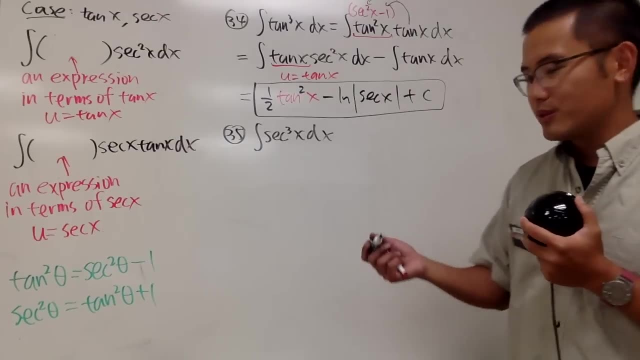 and you can say that, hey, it's actually pretty easy. Okay, Can we do our way over there? Let's just give it a try. This time, though, I will just do it in green to see what happens. Integral split it. 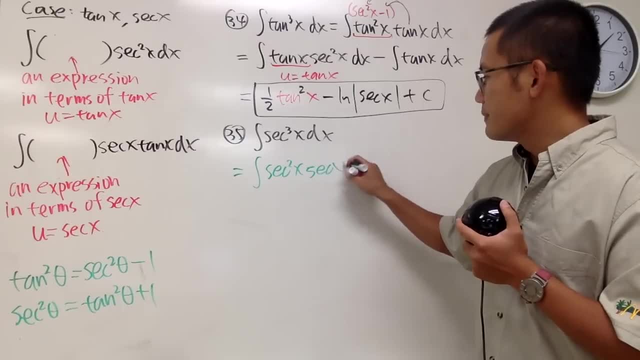 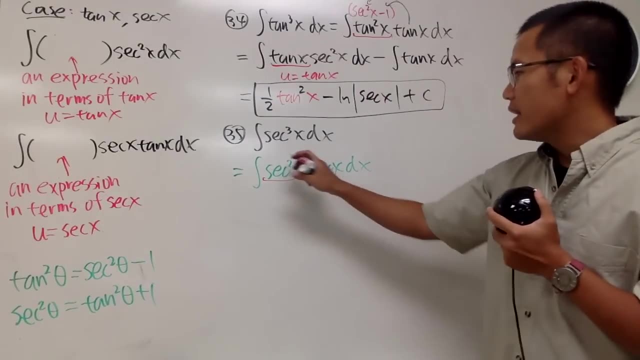 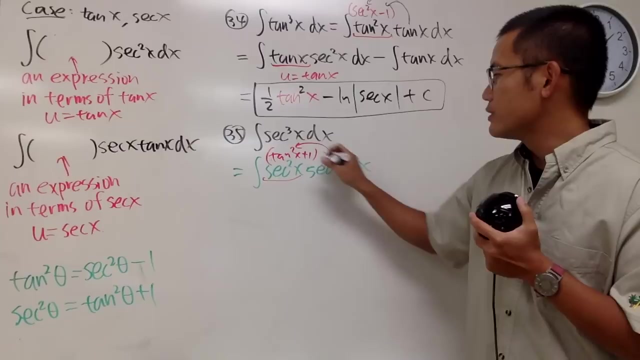 we get secant squared x, secant x, dx. Good, This we can change. which is that? Okay, This is tangent squared plus one. Tangent squared x plus one- Good, And then, of course, distribute. 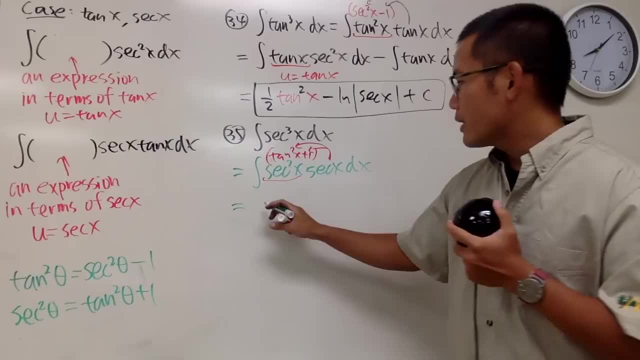 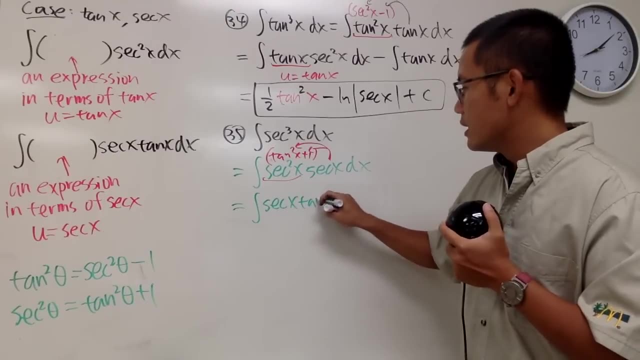 distribute. that's exactly what we did over there. Good, Perhaps I can write it as integral: secant x times tangent squared. so I just have secant x times tangent squared, x. yeah, this times that. Close that and then plus integral. 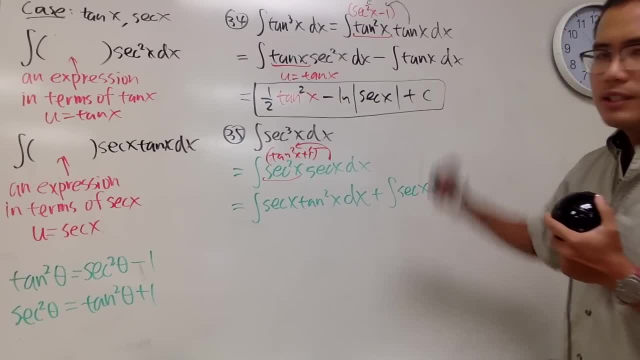 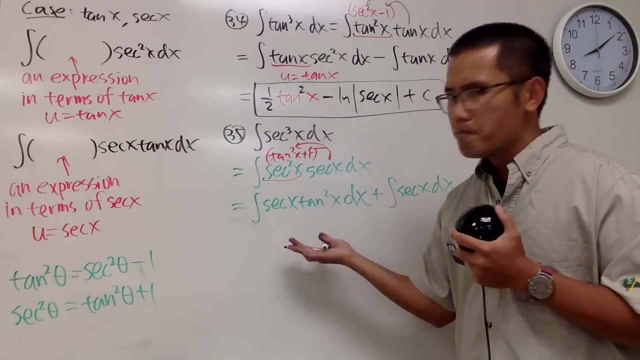 of x times one. Ah, very similar. That was so difficult for this. Hey, we see the tangent, squared and secant. Can we do u sub? No, If you let u equal to secant x. well, if u is. 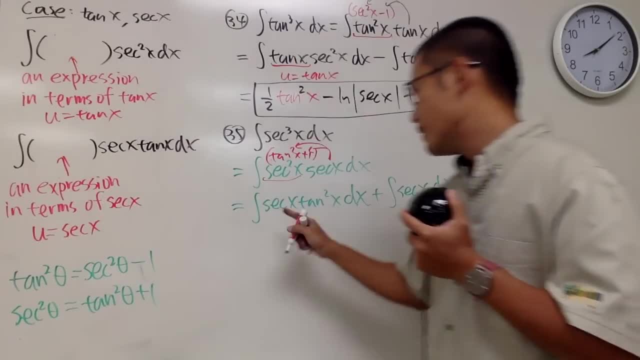 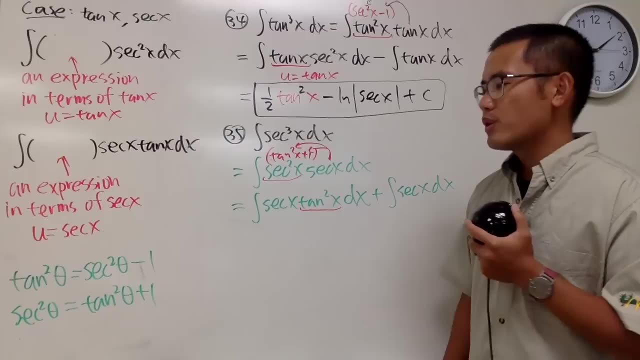 secant x. you actually have to have secant x, tangent x, But you don't have one secant x here. Okay, Hmm, maybe we have the tangent squared x. I have the identity, So let me just put it down as. 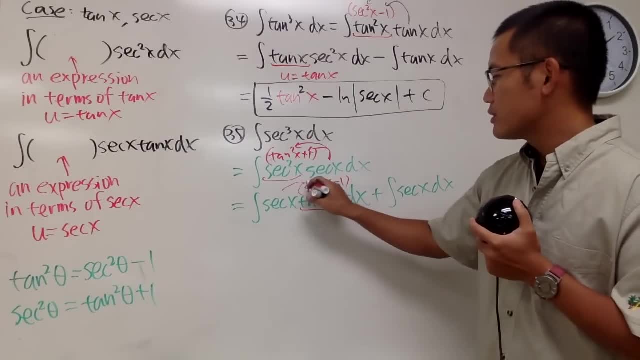 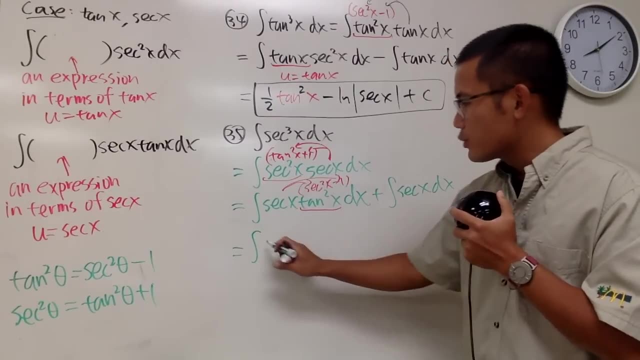 secant squared x minus one. and let's just distribute, distribute. Well, first part, we get again. this is still integral. Integral of secant x times secant squared. this is secant to the third power, x. Let's close that. 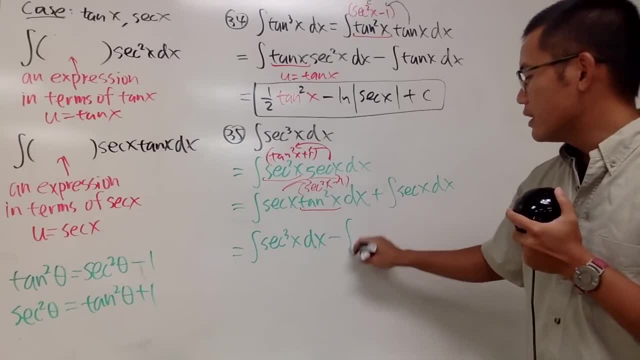 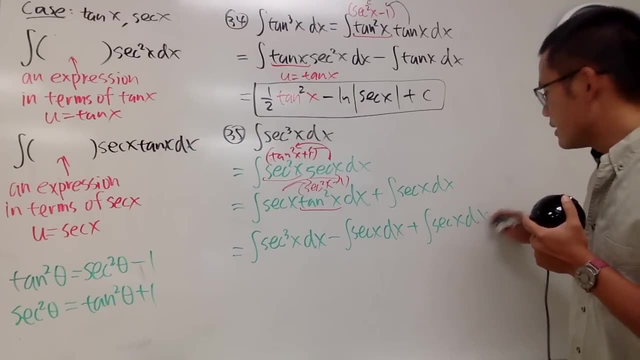 Minus integral secant x times, that is integral of secant x times one. just this. And don't forget, we still have plus integral of secant x dx. And notice on the right hand side. of course they are the same thing. 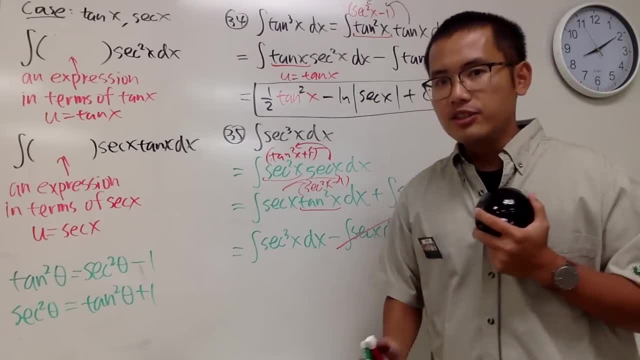 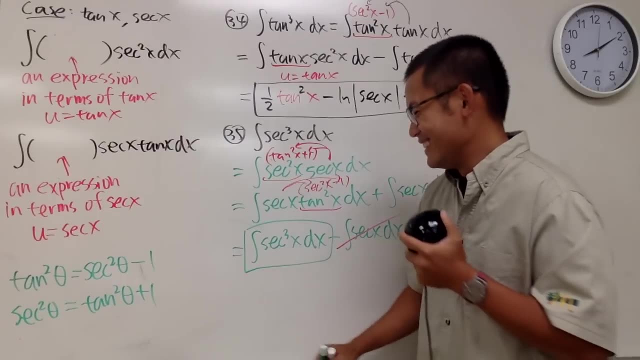 And up is the sign right. So we can of course cancel And, as you can see, ladies and gentlemen, the integral of secant to the third power x, dx, is just equal to the integral of secant x to the third power x. 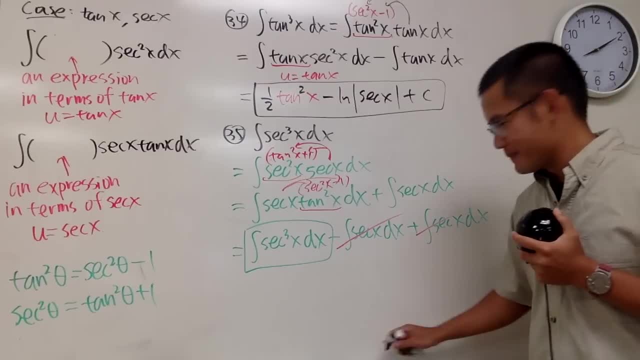 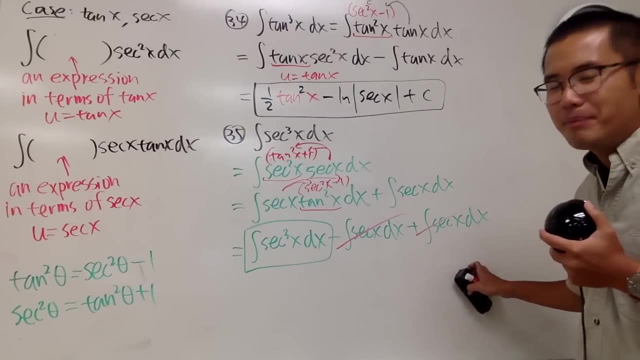 This is just so awesome, isn't it? But no, We're going around in a circle. I know, Unfortunately, this right here. we didn't have the answer at all. We're just like going around in a circle. This is not. 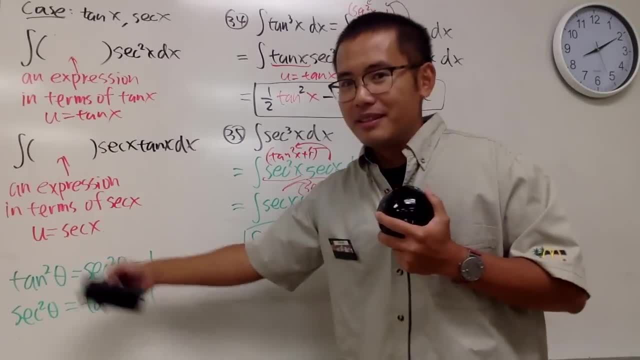 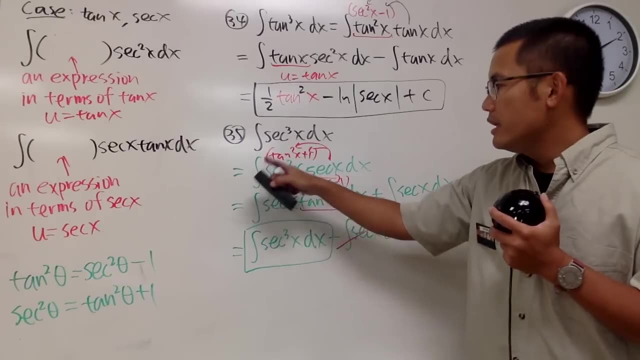 what we want at all. And the problem is this: We're just using the identities and again just going around a circle. Now, well, if you look back here, in fact, integral of secant squared x times secant x. 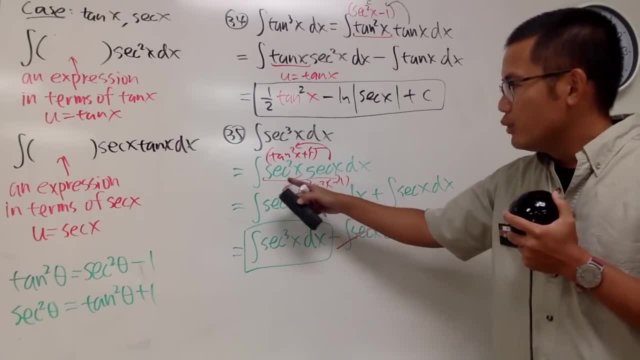 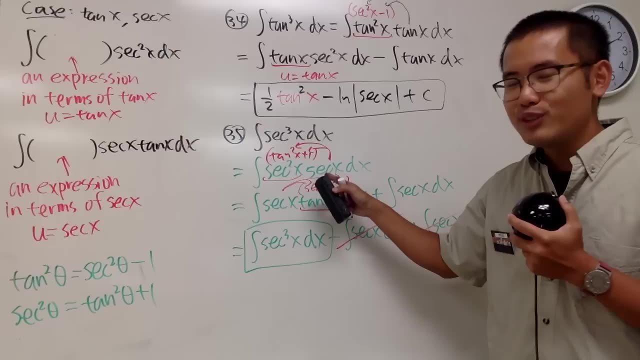 Don't use identity, because if we did, we will be going around a circle. Look at this, Look at that. Can we integrate secant squared? Yes. In the meantime, can we also differentiate secant? Yes. When you can integrate. 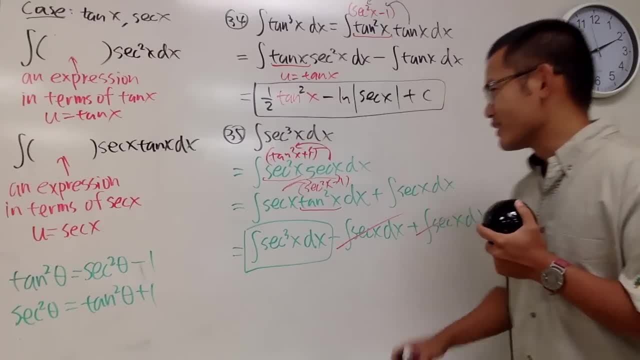 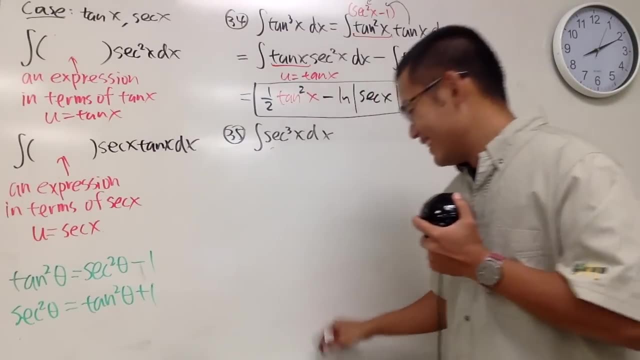 something and differentiate something else. why don't we try integration by parts? So that's the idea And that's exactly how we do this one right here. So let me just erase this. That's why I said this is much harder, right. 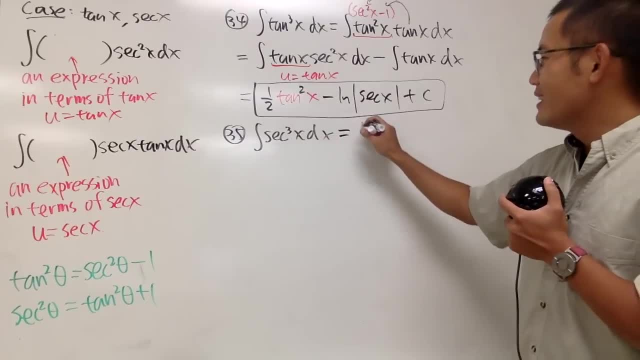 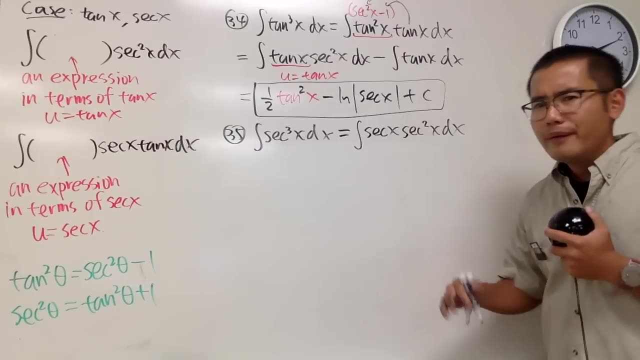 Anyway, here is the DO. We are still going to look at this as integral and let me put it down as secant x times secant squared x. and you might be wondering how come I don't want to change this to tangent. Here's the idea. 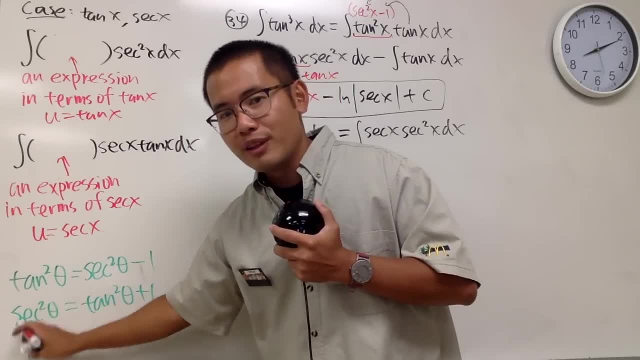 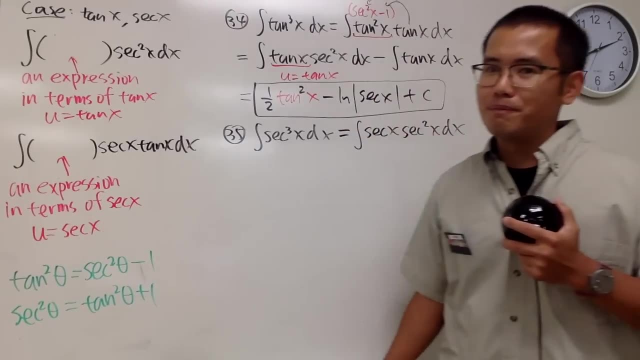 Imagine: if you want to get secant to the first power, you have to take square root. You have to take square root. This is the square root of tangent squared x plus 1.. I don't think you want to see the square root. 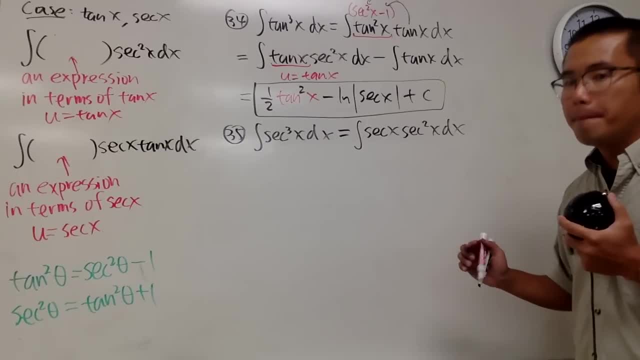 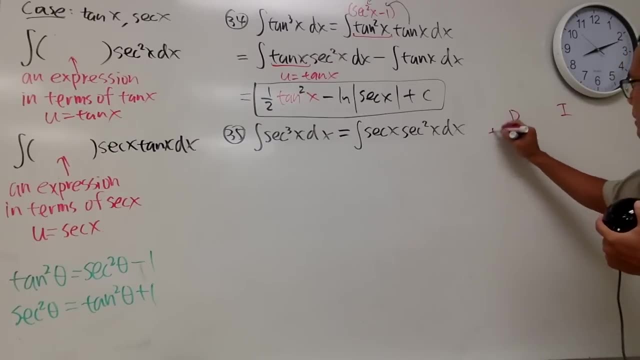 That's the next category. Anyway, right here we'll be doing integration with the DO. I will put it down right here for you guys. Here is the D and here is the I. Let's put down plus minus to get ready. We can integrate. 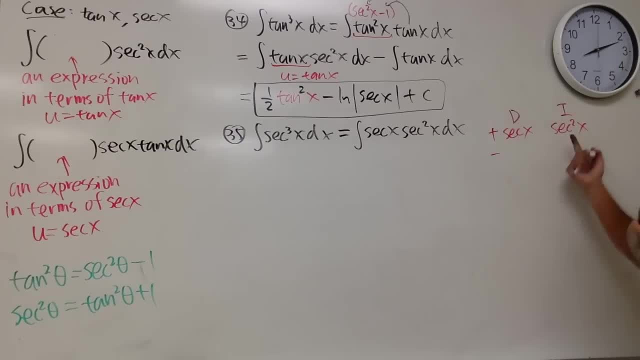 secant squared nicely, and we can differentiate secant x. So let's do that. Integrating secant squared is tangent x. How do we know? Because we talked about it. That's actually the first question in this video: Differentiating secant x. 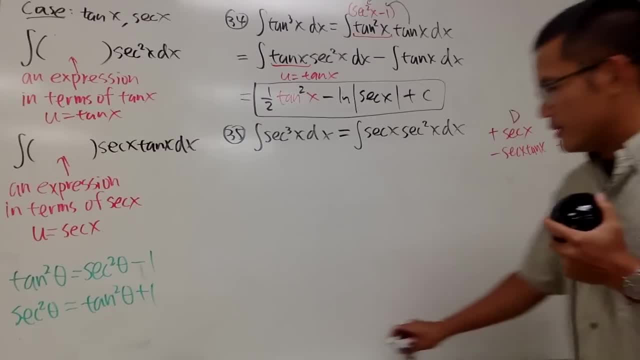 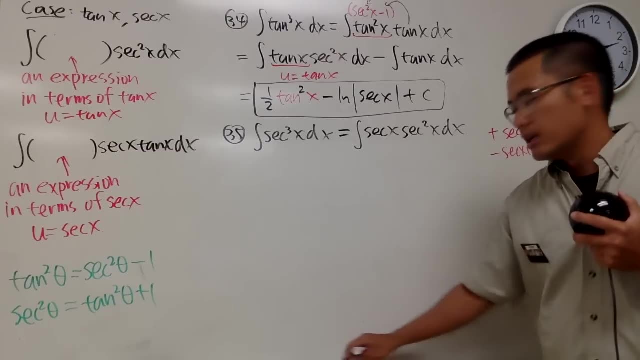 is secant x, tangent x, right. So let's see how should I write it out? Of course, this times, that is the first part of the answer and we still have to do this times that That's the second part of the integral. 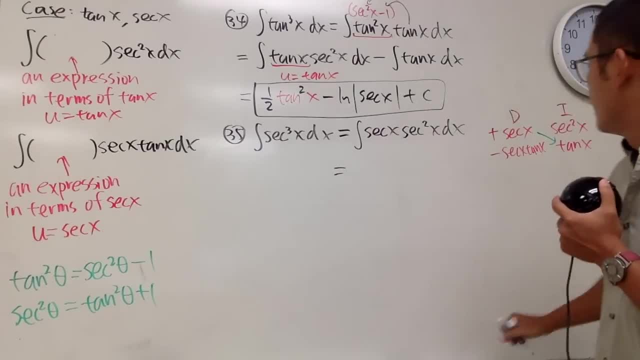 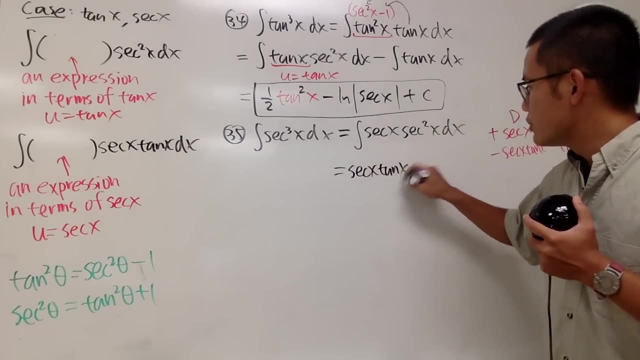 right. So let's see This part. we will have this times. that That's the first part of the answer. So we have secant x times tangent x, and that's awesome. Now for the second part. we are going to. 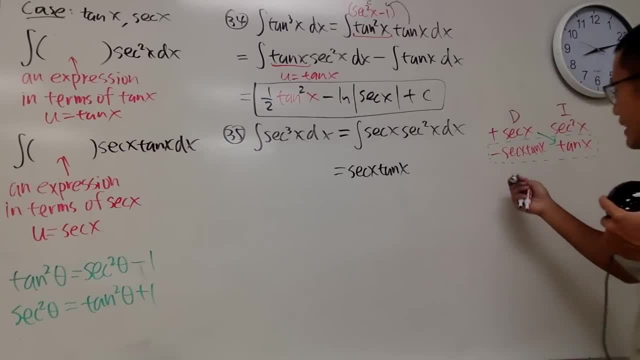 multiply by that, That's a minus. so we should put down a minus and you have the integral. Check this out: Here we have secant x, Here we have tangent x times tangent x, so that's tangent squared x- dx like this: 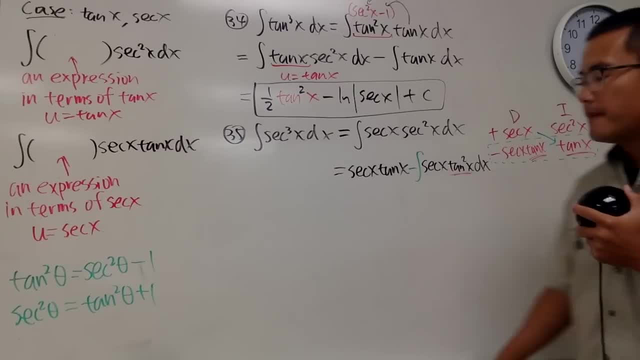 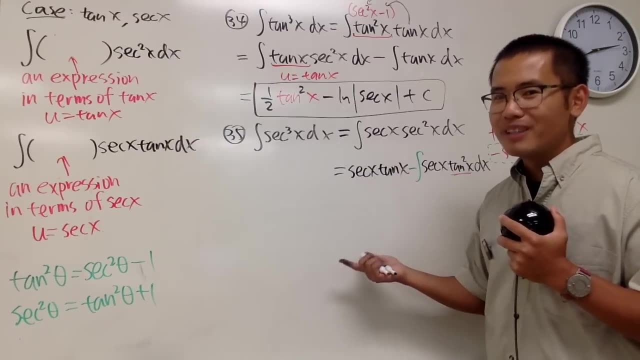 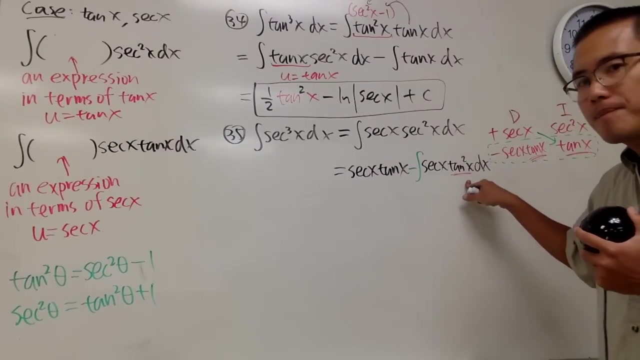 Right Again, tangent squared, And so, as you can see, when we do this, we actually squeeze out the first part of the answer than earlier. right Now, can we integrate this? Well, let's try to use identity, because u-sub is. 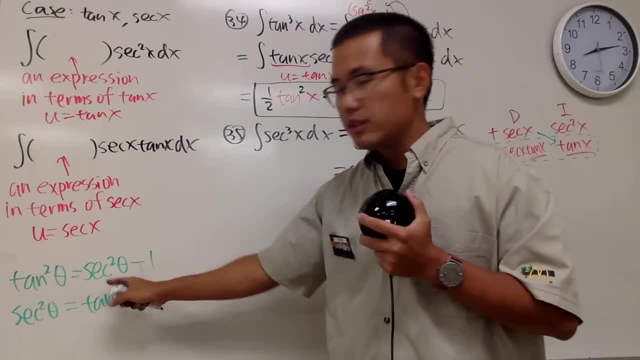 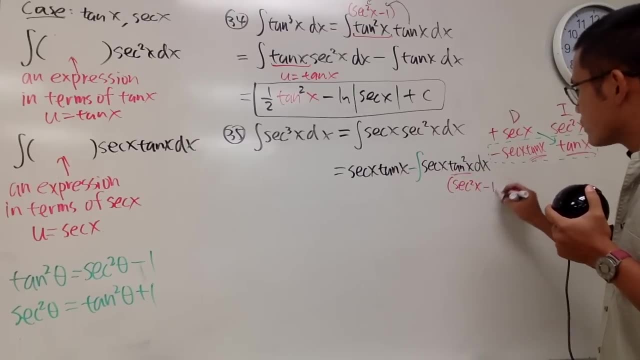 not going to help us out, So I'm going to use identity right here. which is this? right here? right? So, as you can see, tangent squared x is equal to secant squared x minus 1, yeah, And of course we can do what we did earlier. This is still in the integral, though, So we actually end. 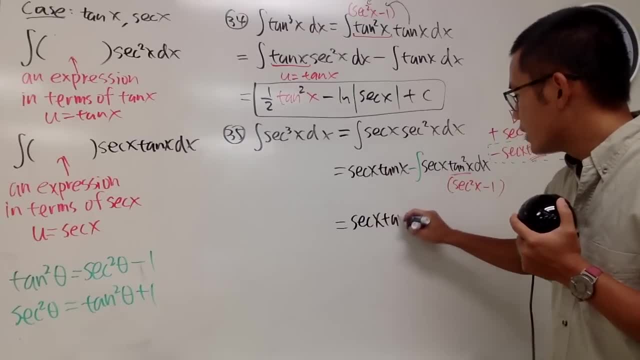 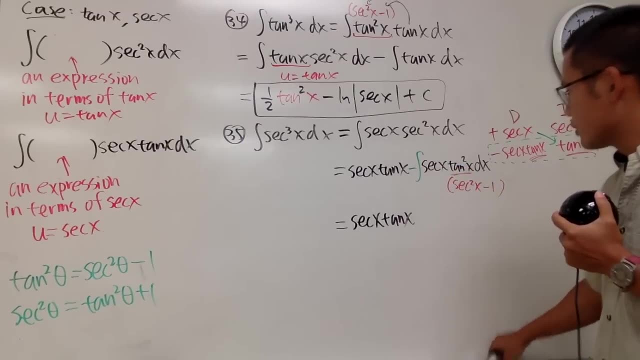 up with secant x, tangent x. That's the first part of the answer. Then we have to minus. let me just put this down to make it clear: minus the integral, secant x times this, This is the second power, That's the first power. So we get secant to the third power, x, And let me just close this integral. 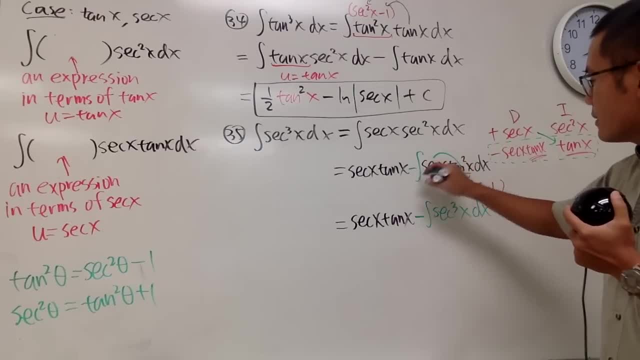 right here, And next I will take the minus right here, the minus secant x times the minus 1.. Minus times minus, we still have to distribute and that will give us a plus right Minus minus, it will give us a plus Secant x times 1, don't forget that's still inside of the integral. 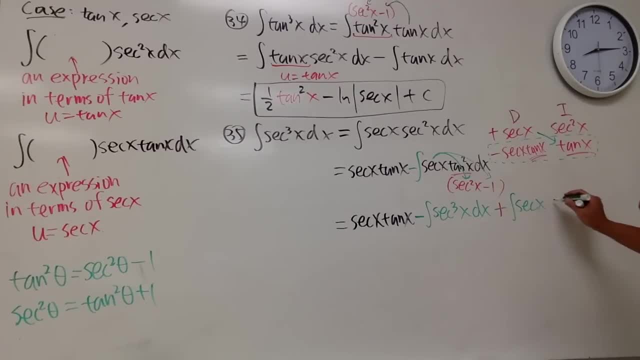 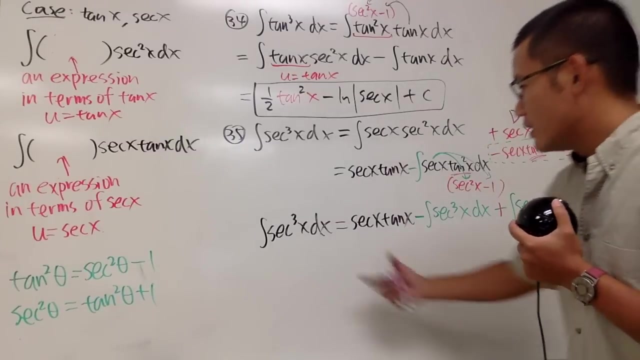 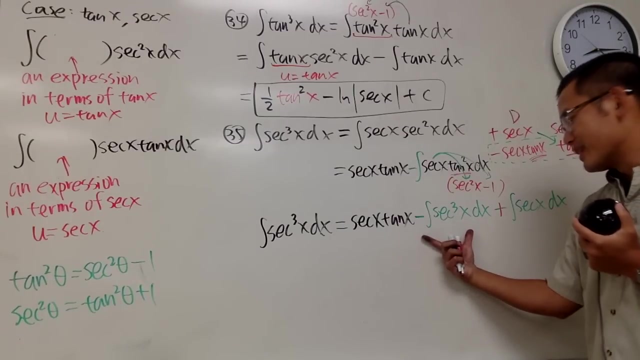 and that's still secant- x- dx right here. Now let me put down the left-hand side. Keep in mind: we still have the integral of secant to the third power: x- dx. As we can see this equation here, this is equal to: hey, we have a minus integral right here. It's the same. 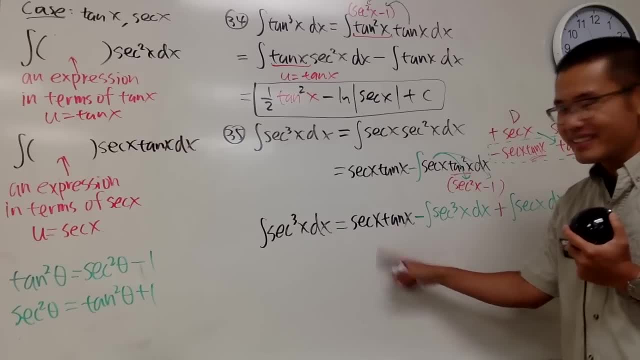 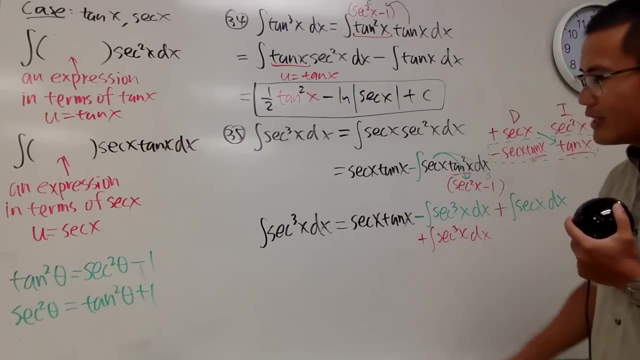 thing, And this guy is the first part of the answer. That's great. Well for this. why don't we just add integral secant to the third power x dx on both sides? Yes, this is another repeating situation. They definitely should know for your Cal 2 class, eh? They cancel out Now have a look. 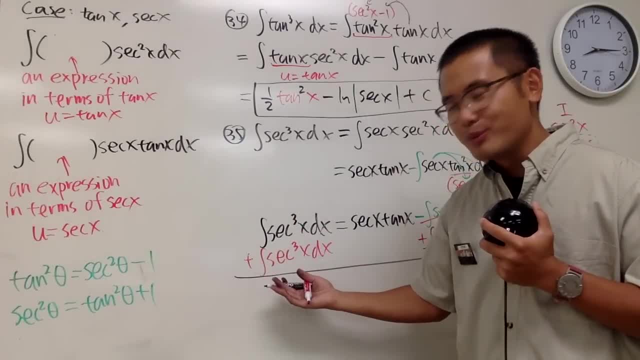 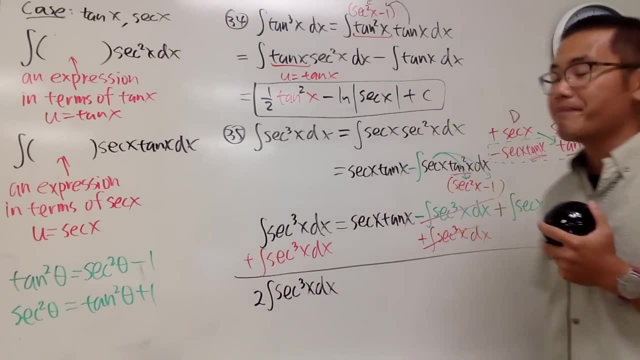 This right here: one integral in black plus another integral in red. All in all, we have two integral of secant to the third power, x, dx. like this. Great, Then we have. this is the first part of the answer. 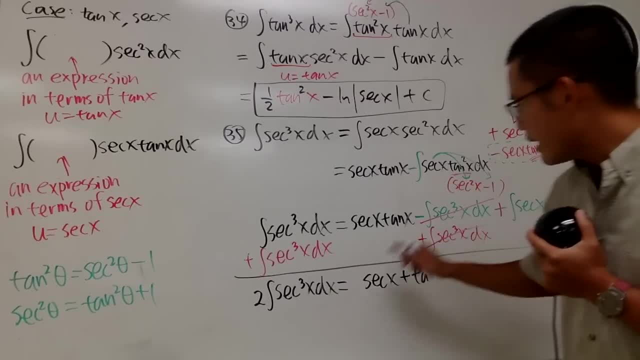 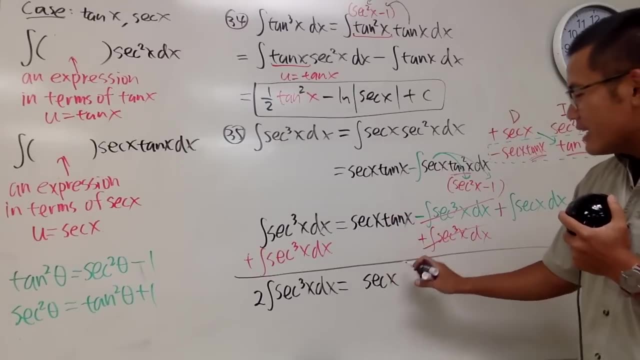 namely secant x plus sorry tangent. this is multiply. Man, I have to work on my t, but this is time. this is: this is t: Secant x times tangent x. yeah, Then, for this part, we already done in. 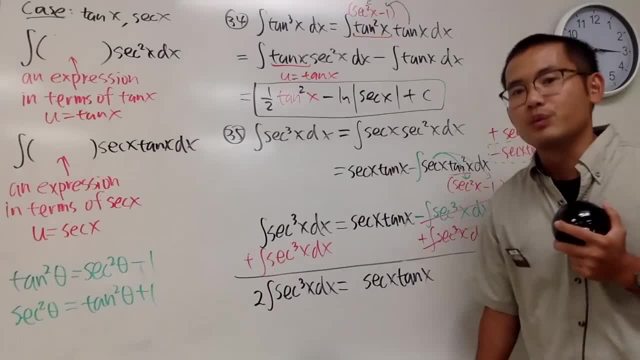 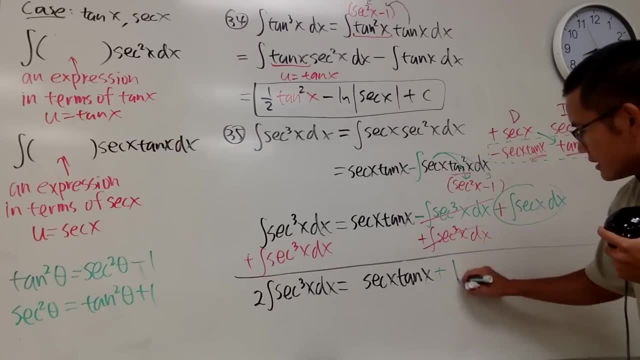 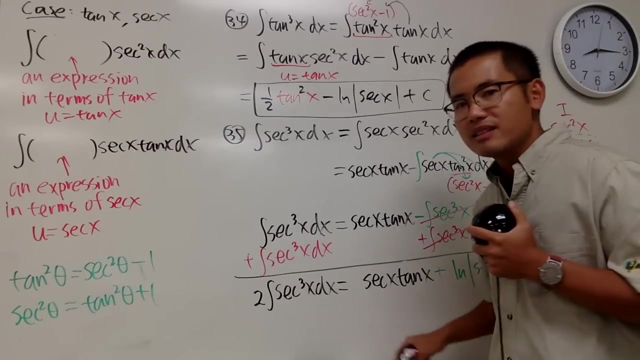 fact don't we know the answer for this? Yes, we do, because we did it already. This right here is plus, because that's plus, and the answer for the integral of secant x is natural log after the value of secant x plus tangent x, like this: But are we done yet? No, because we have the two right. 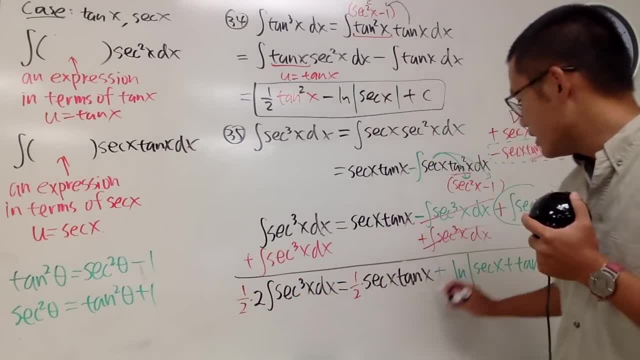 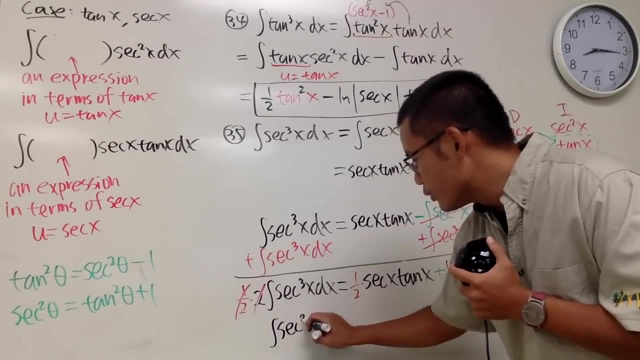 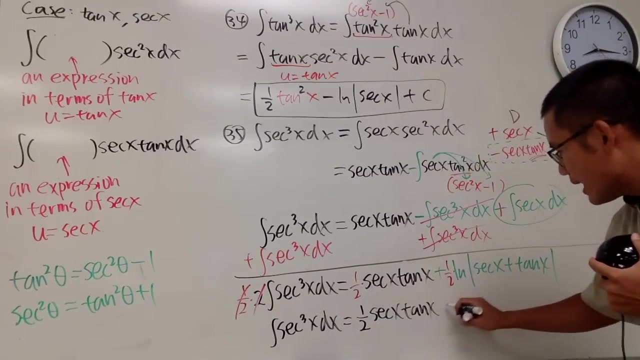 here. It's okay. Small fix: Multiply everybody by one half so that they will cancel. Finally, integral of secant to the third power x dx is nicely equal to one half secant x- tangent x plus one half natural log. absolute value of secant x plus tangent x. This is a multiplication, this is an addition. 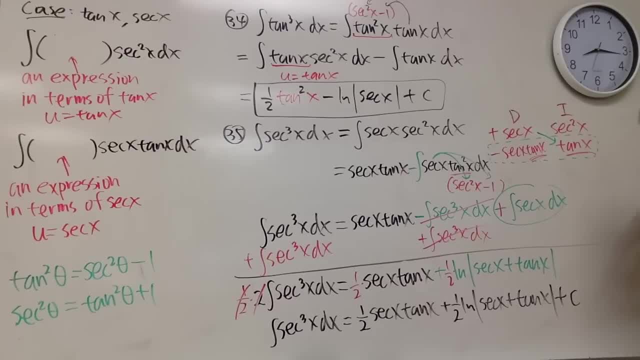 between okay, And then in the end we're all done. Put plus c, This is it Right. So that's it. Sometimes not only you have to use trig identities, but also, again, you have to use the categories that. 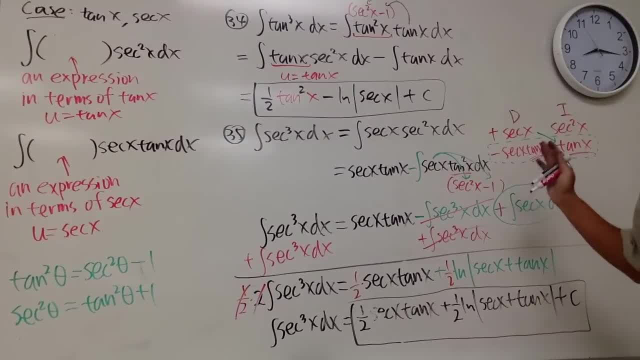 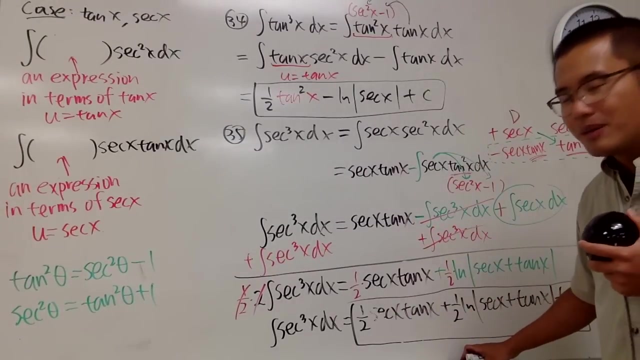 we have mentioned previously, We used integration by parts for this one, So that's so wonderful, isn't it? Yeah, Practice this one a few times, though I make my students practice this 100 times. No, just kidding, But I did make them practice on their own from scratch right after they see this. 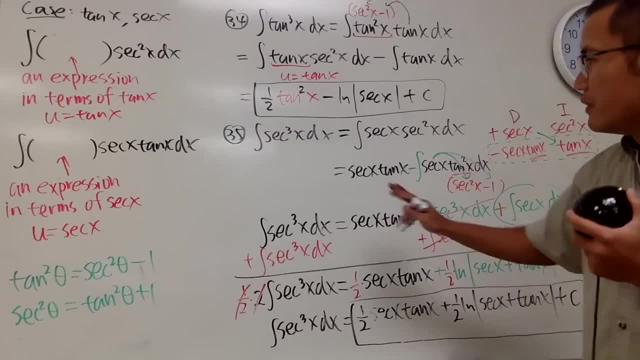 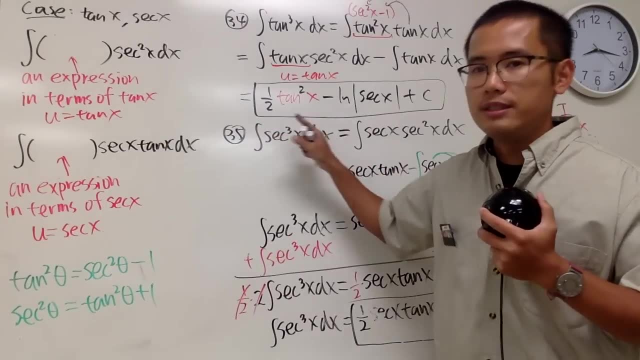 So this is how they can build up their confidence. You guys should be doing it too. If you think this question is like kind of hard at the moment, then get out a sheet of paper. try to reproduce this 100% on your own, without looking at the notes, without watching my video. 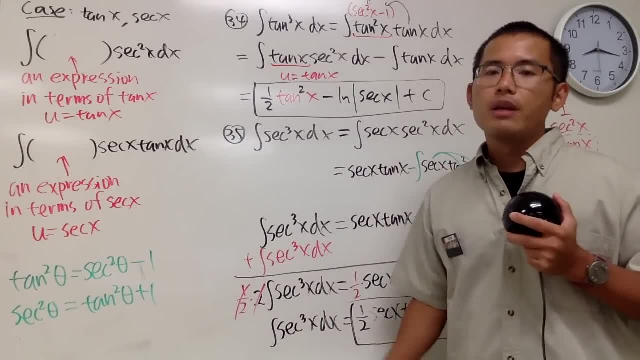 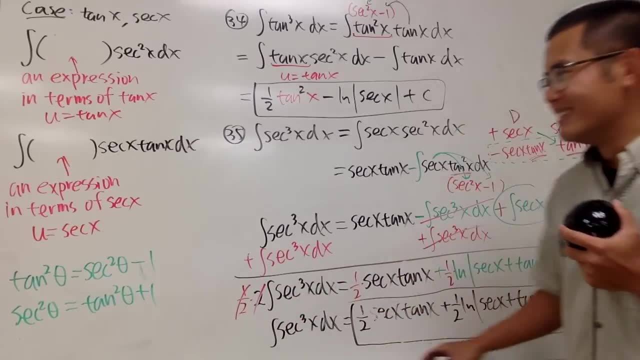 Try to see if you can redo the whole thing again or not. If you can, that means you are really getting it Better. yet, do it again the next day so that you can really remember how to do all these questions. Okay, So this is wonderful. 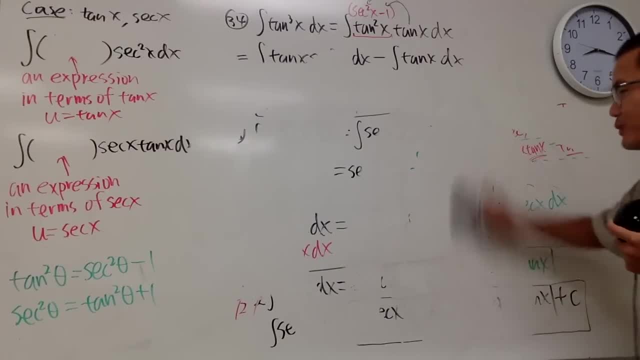 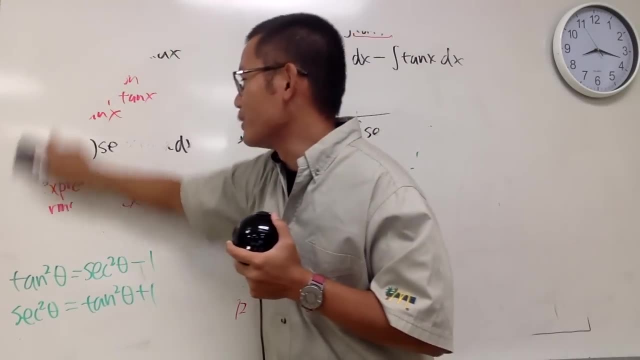 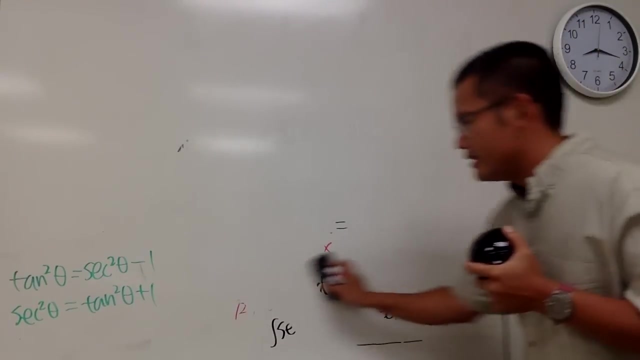 Subtitles by the Amaraorg community. Now, not only no, we don't have just, it's not just 15 more questions. We have about like 20 more questions And we have two more categories. so that's the big part. I'm not worried about the questions, I'm worried about the categories. 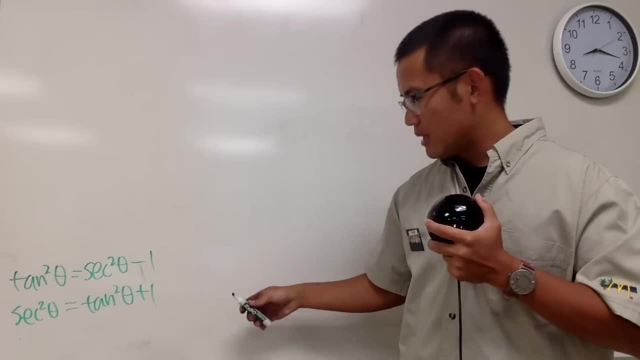 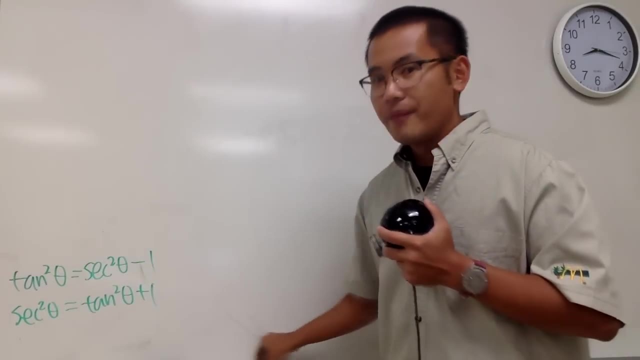 Notice I have this right here on the board. I still have it. huh, Perhaps I'll put on one more right here. Let's put this down right here. Uhhh, Actually, let's just, let's. that's just to write it down here. 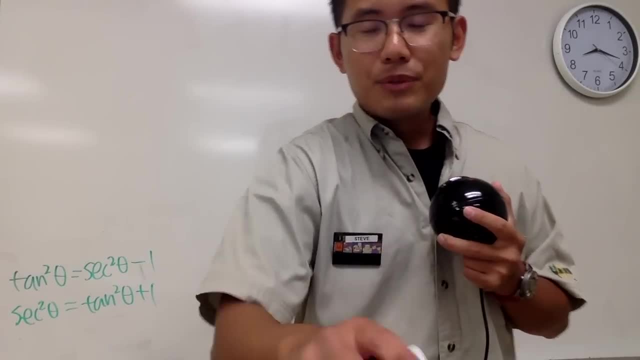 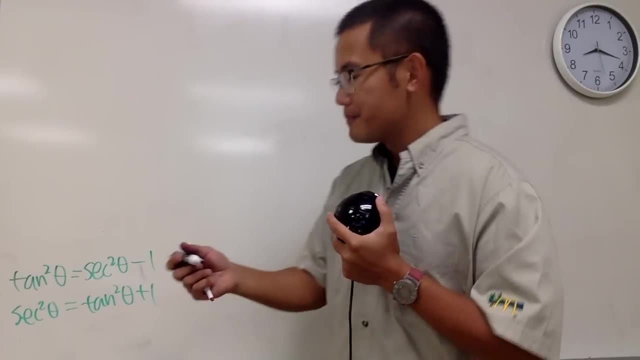 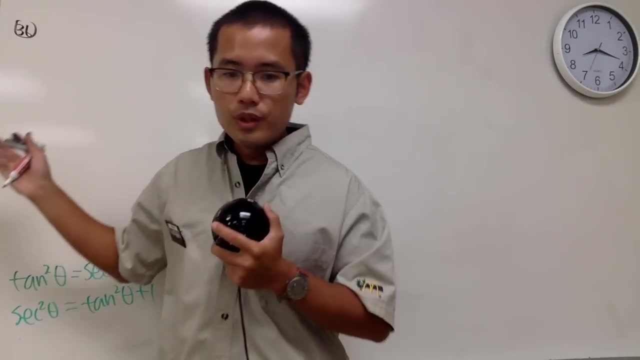 Let me know how you guys are doing, If you guys are watching this so you can prepare for your cal2 test. leave a comment down below and let me know, And I wish you the best luck as well. Okay, So here is the next category, but I will show you guys number 36,, which is: 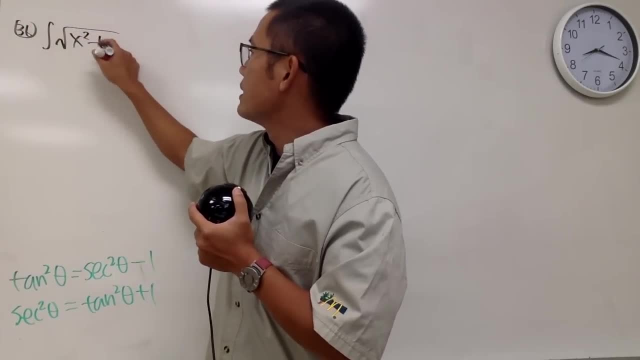 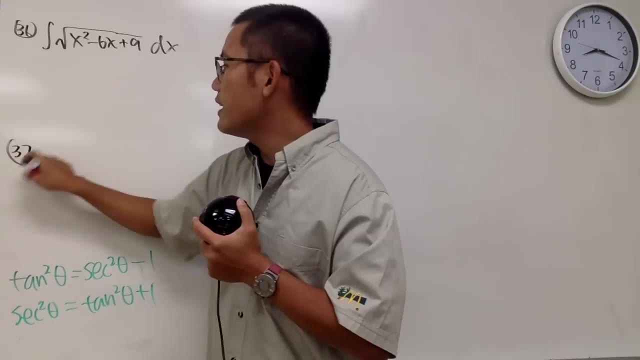 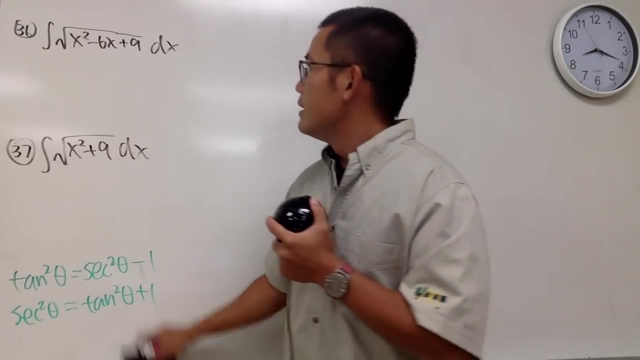 The integral of square root of x, square minus 6x plus 9.. dx. and let's see question number 37, integral of square root of x squared plus 9. dx. like this- I don't know why my word state is like really bad. 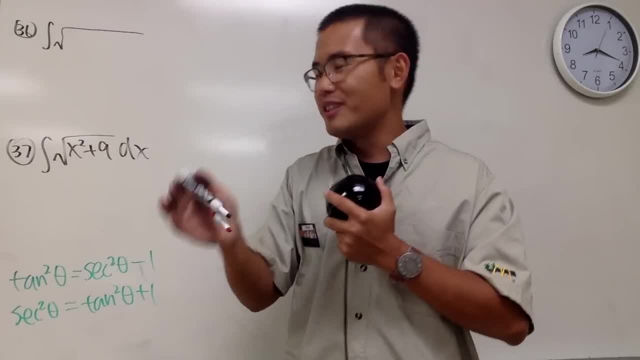 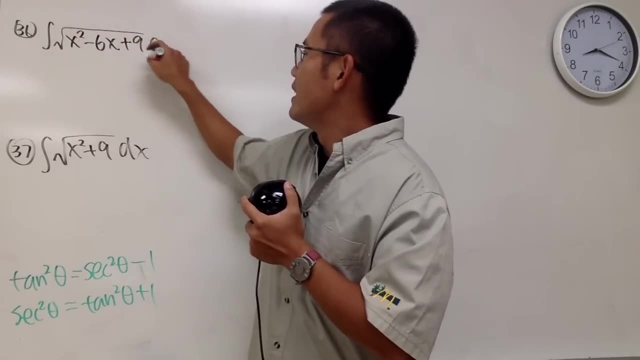 My secret of filming my video. my camera is always tilted a little bit. If you guys notice it. if you do, just let me know too. That's kind of cool, Yeah, But anyway, hopefully you guys can see this okay. 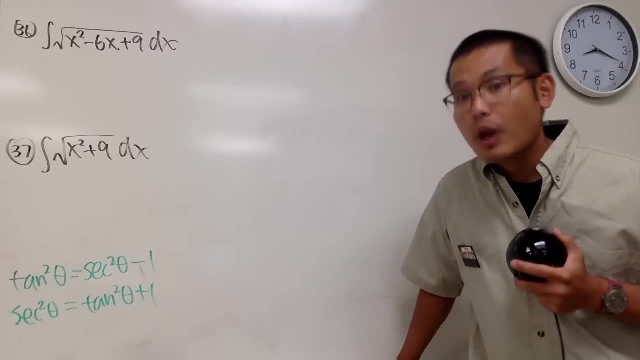 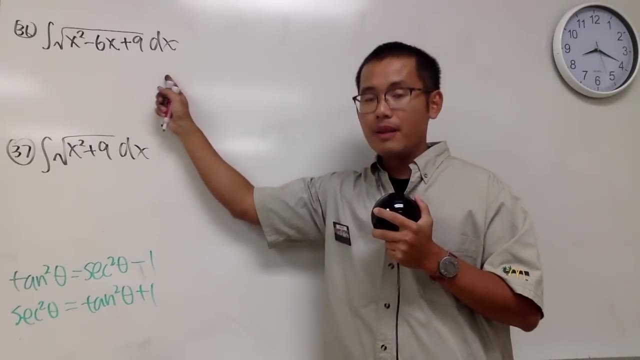 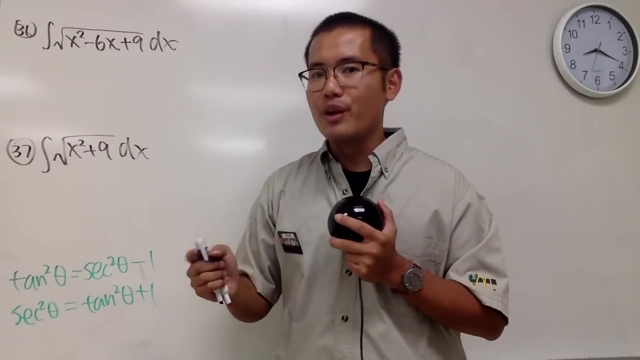 Anyway, we have two integrals on the spot. Which one would you like to do on the test? Hopefully you guys will tell me this one, because it's so much easier, because this trinomial inside it happens to be a perfect square. 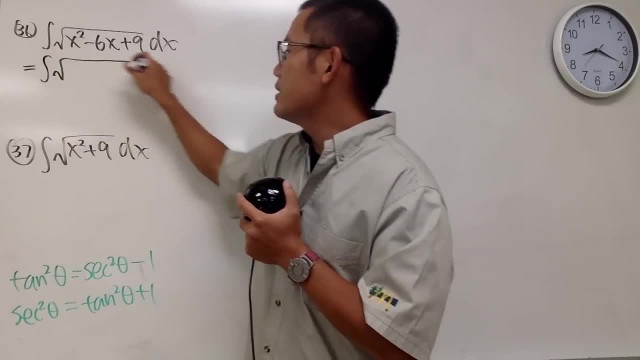 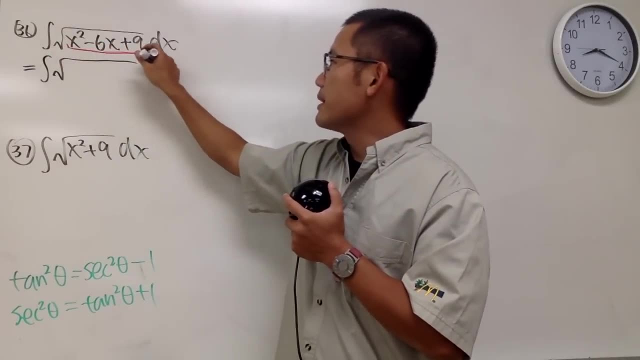 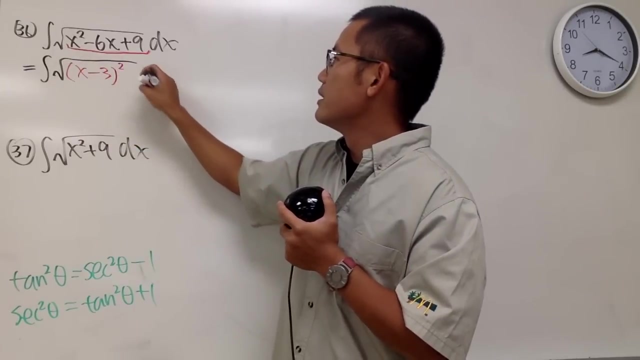 So check this out. This is just the integral of square root, The whole thing inside. we can factor it and we get x minus 3 times x minus 3, and that's going to give us x minus 3, parentheses squared dx. 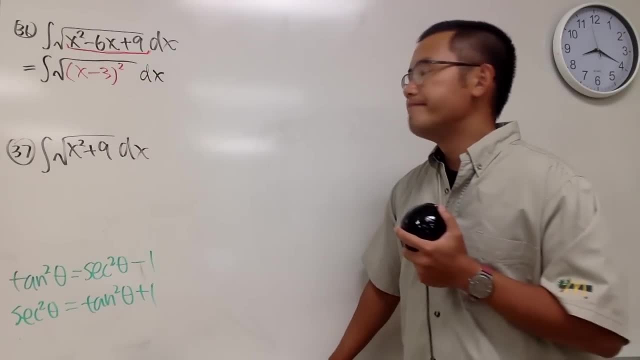 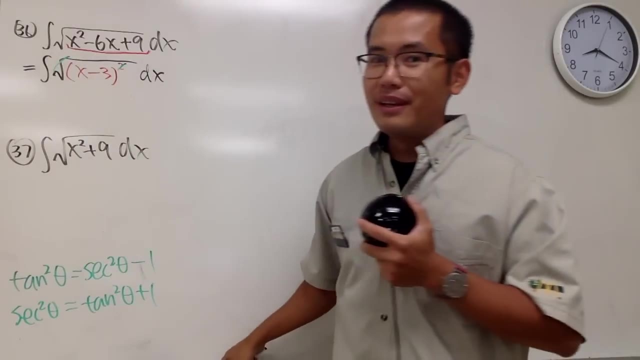 And that's so nice, isn't it? Well, what's next? Of course, just cancel the square and the square root already, man And this and that, just cancel the out, And in the end we're just integrating one half. 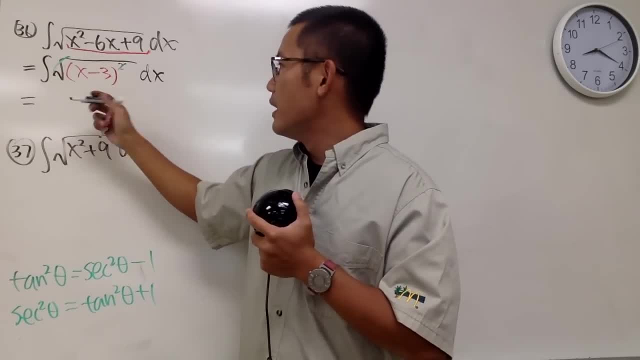 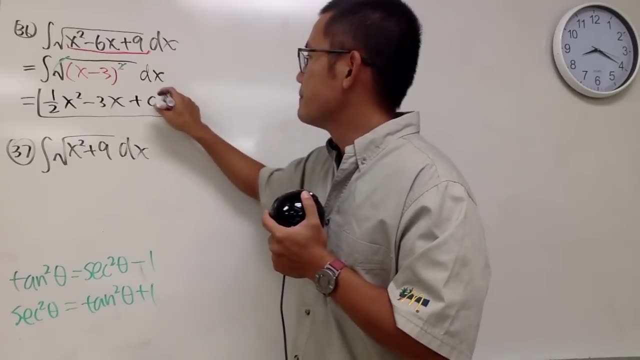 well, we're just integrating x minus 3, right? Okay, And let me just put on the answer: one half x squared minus 3x, and we're done plus c like this, Right? I know some of you guys will be wondering. 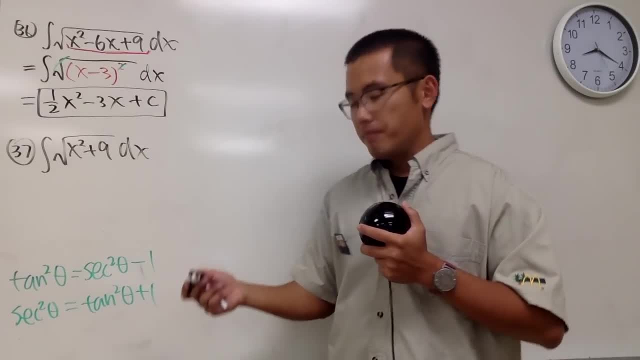 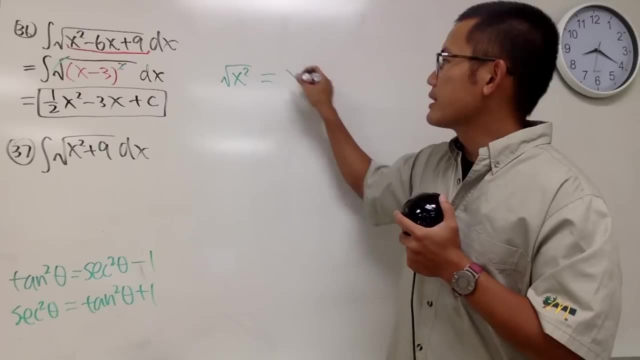 hey, shouldn't we be putting down absolute value? Can you tell me? yes? Here's the idea. If you have the square root of x squared and you say this is equal to x because you just want to cancel this out, this is not entirely correct. 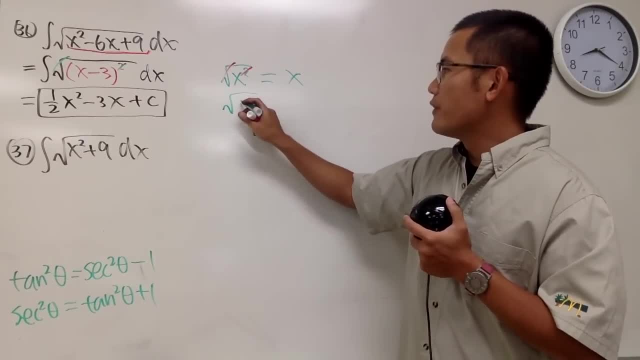 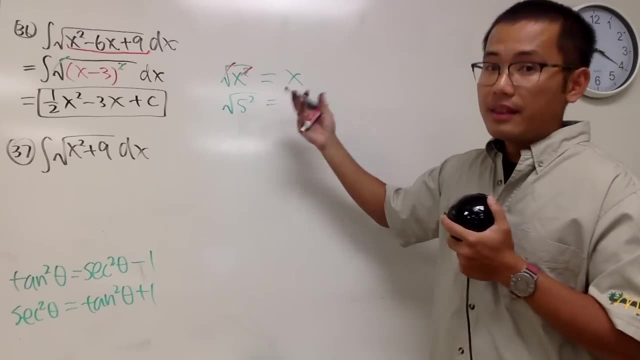 Here is an example: Yes, If you have square root of, let's say, nine, that's down to nine square root of five. squared This right here, you get five, because you can cancel this out. that's very nice. 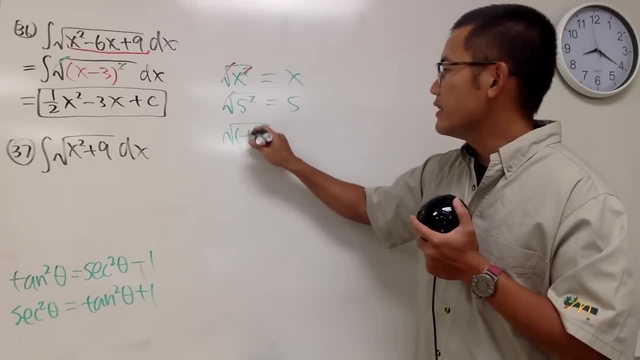 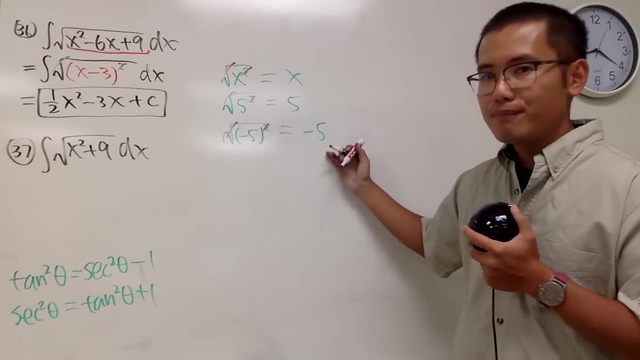 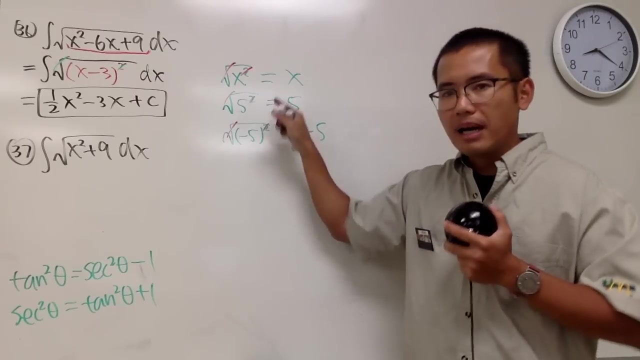 However, if you have the square root of parentheses with negative five squared, can we just cancel this out and say the answer is negative five? No, we cannot, because the output of square root, this is the principle, this is the positive square root. 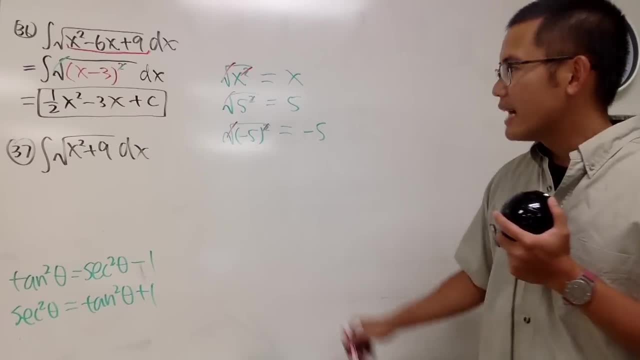 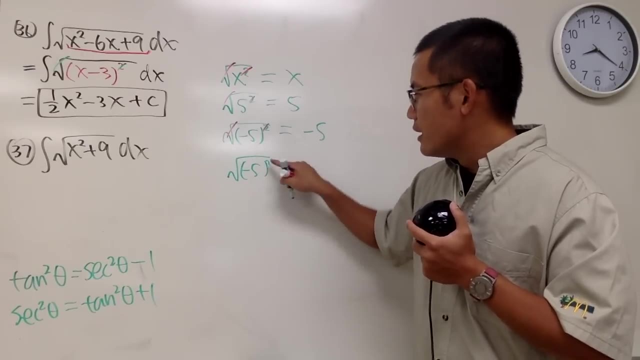 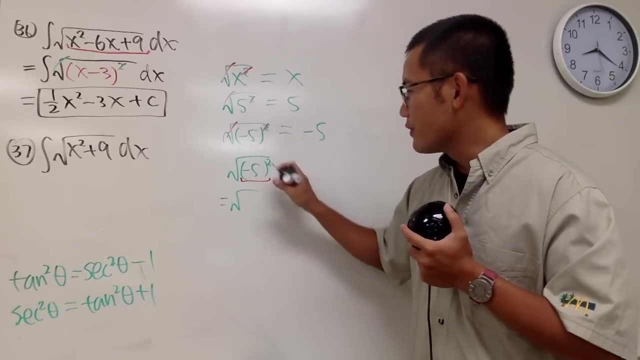 the square root should always be positive. and another thing is that when you have this expression, this right here, square root of negative 5 square, this right here should be done inside out because of the word of operation, and you end up with square root of negative 5 times negative 5, which 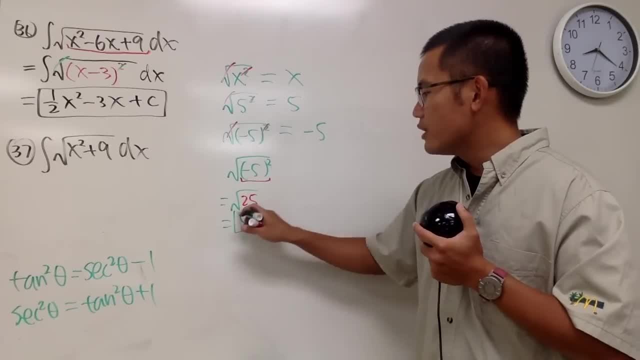 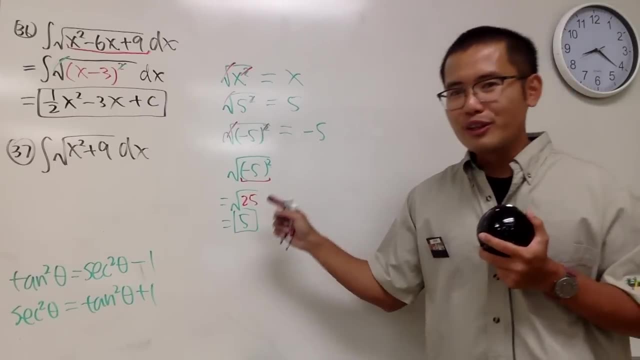 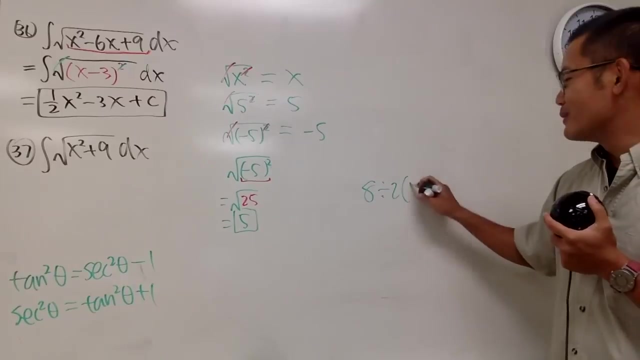 is positive 25 and you end up with 5.. this, right here, should be the current answer. this is not. i know this is the word of operation, but unfortunately this kind of question never goes on. never go viral. yeah, it's just that i don't know. 8 divided by 2 times 2 plus 2.. this order of 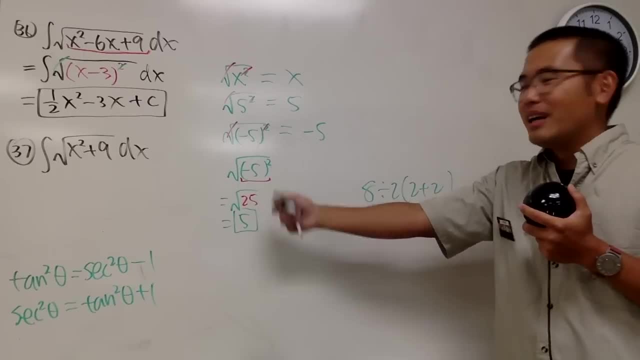 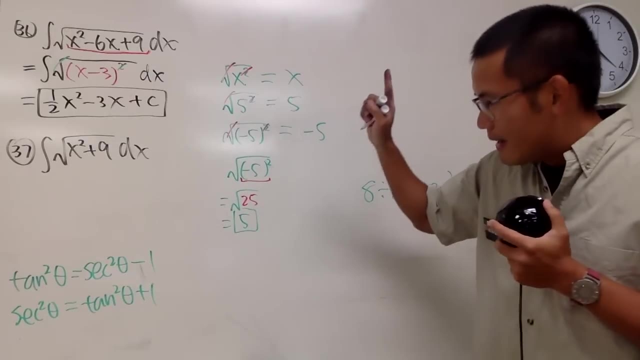 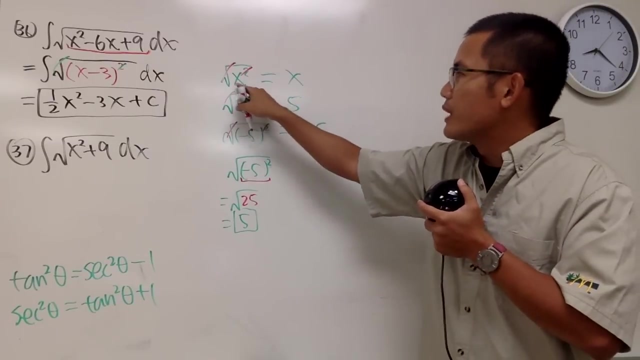 operation question goes on viral. this never. i don't know why. i tried it, yeah, but i don't know, man, and, by the way, i don't know anyway, this answer is 5, but you cannot just cancel it out. one way to fix it is the following: when you cancel the square and the square root, you're just going to attach the 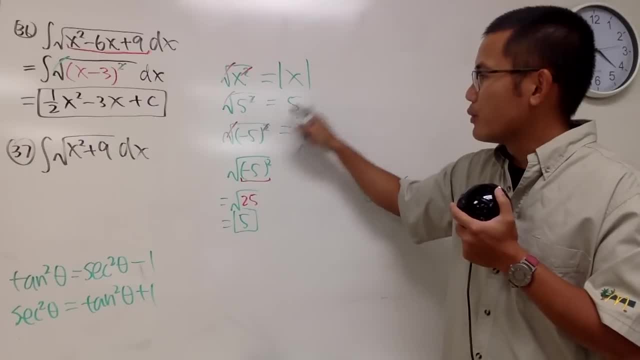 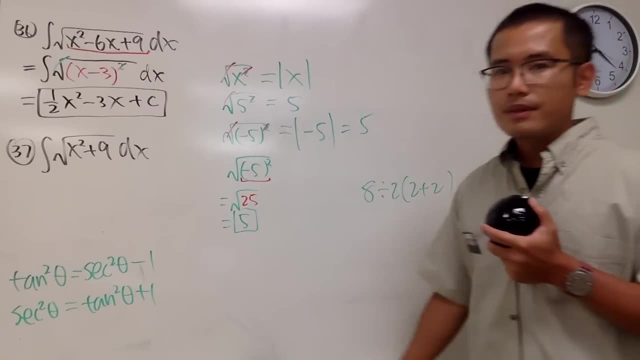 absolute value. that's the idea. you see, if you have the absolute value, when you cancel this out, just attach the absolute value. absolute value of negative 5 is still 5.. this is good. so this is pretty much how you do it. and now you might be wondering: why did i put on the absolute value then? 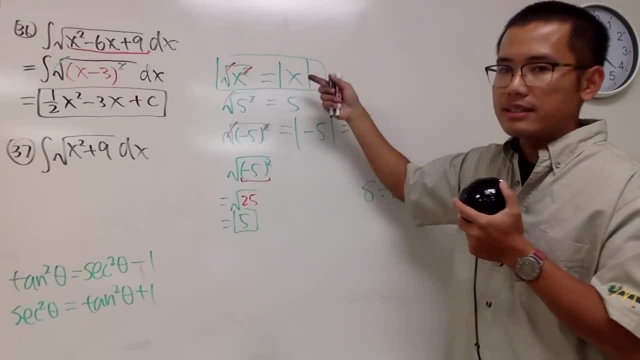 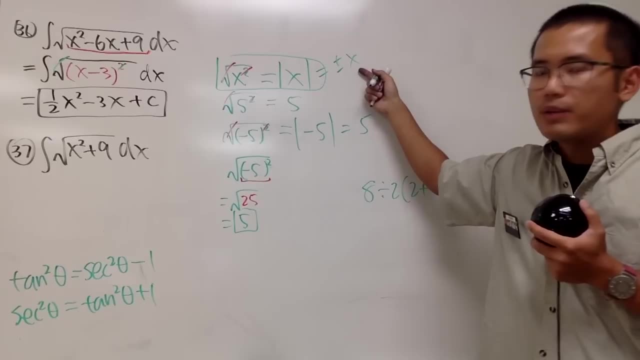 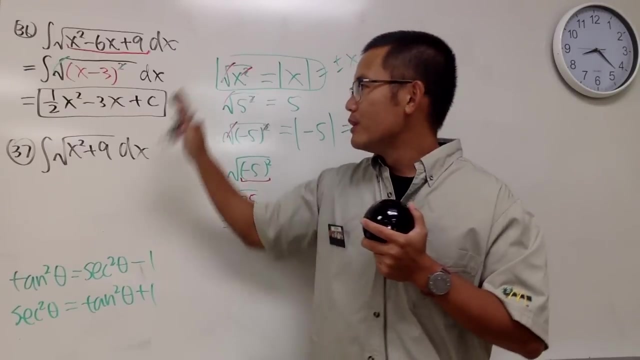 well, because the idea is that if you have the absolute value of x, you will just be looking at plus or minus x, either positive value or negative value at the end. right? well, the idea is we are just trying to focus on the integration technique, so i don't really need to worry about the 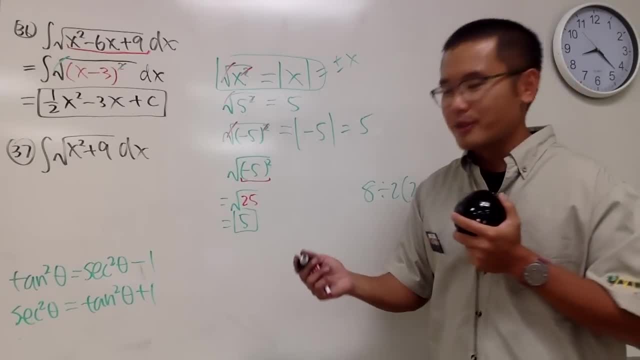 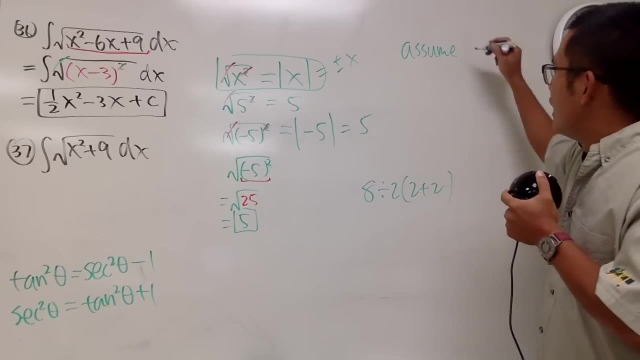 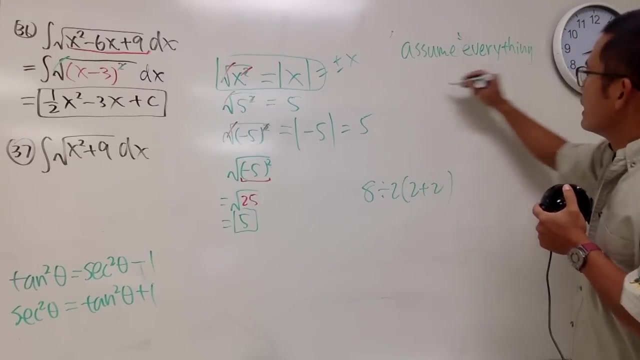 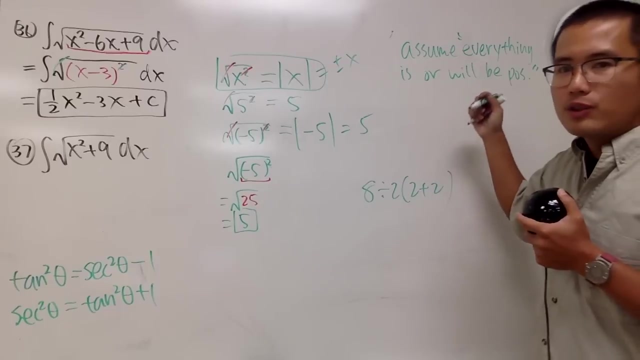 absolute value. what we'll do is, let me just make an assumption right here. okay, i'll just write it down. we are going to assume for the rest of the handout here i will just assume i put on a quotation mark right here- everything is or will be positive. right, i'll just assume everything is or will be positive. so when i have 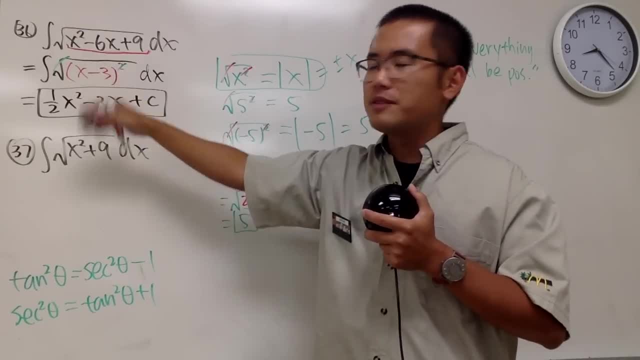 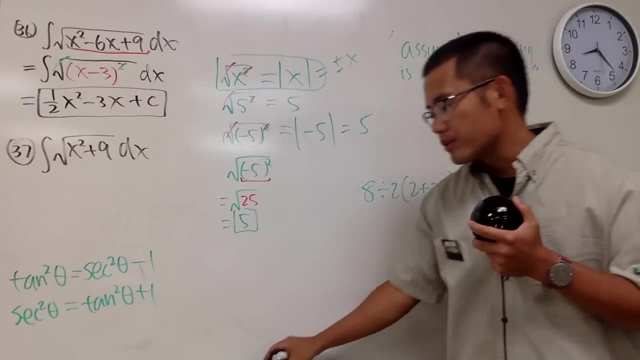 x minus 3. right here i'll just assume this is positive. so when you cancel the square, square root, just deal with positive anyway. well then they will be positive in all that stuff. so i'm not going to worry about the plus, minus nor the absolute value, just focus on the integration technique. 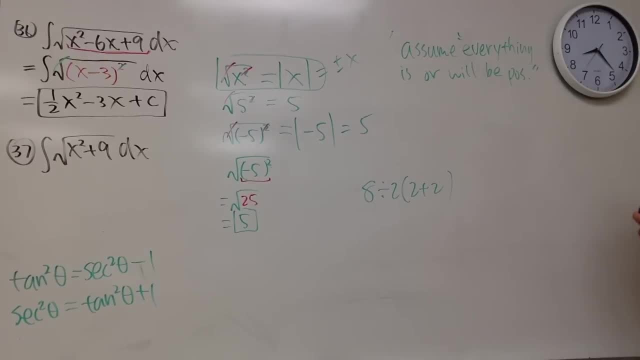 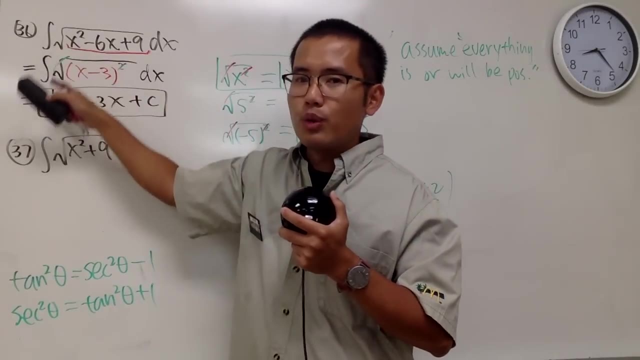 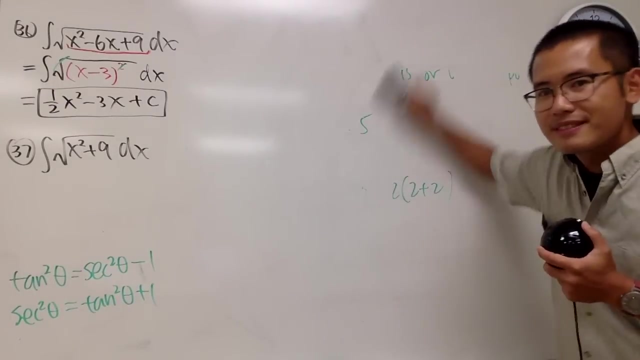 that's the idea, right? so keep that in mind. yeah, and the truth is, absolute value only matters if you have a definite integral going from one number to one number. that's the time it matters, so that's why let's just not worry about that. yeah, so that's just a little discussion. 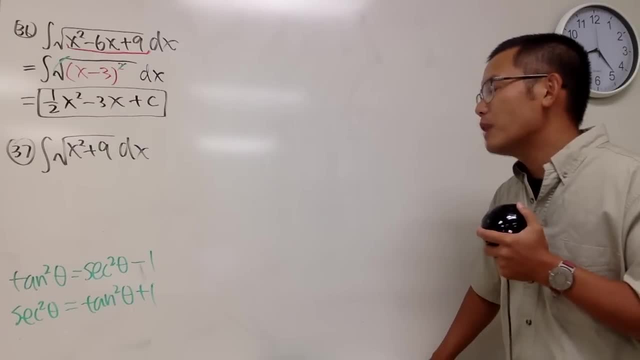 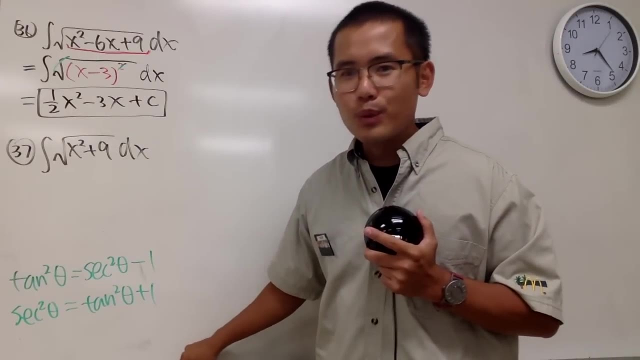 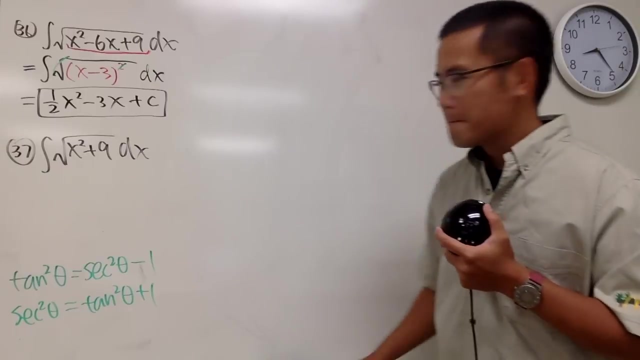 what's that man who took away the negative six x? that would have been so nice again. i'm stuck. hopefully by now you guys can see that Sometimes, when we are doing integrals, the more the better, such as this one When you take away the minus 6x. no, this is not what we want anymore. 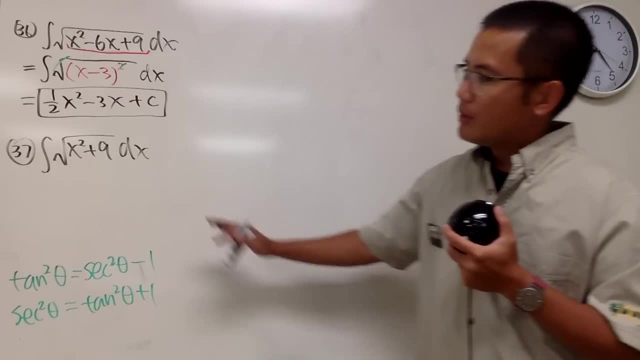 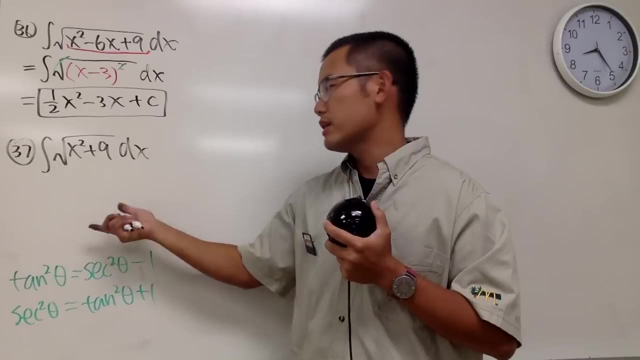 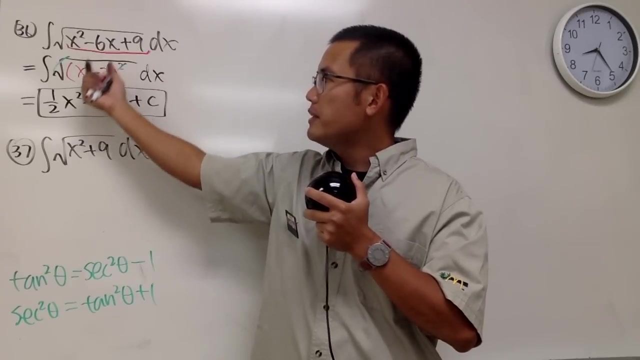 Hmm, Well, have a look here Inside. here we have the sum of 2 squared x squared plus 3 squared right. So two things and we're adding up. Notice how this equation was so much easier, because it was a perfect square inside. 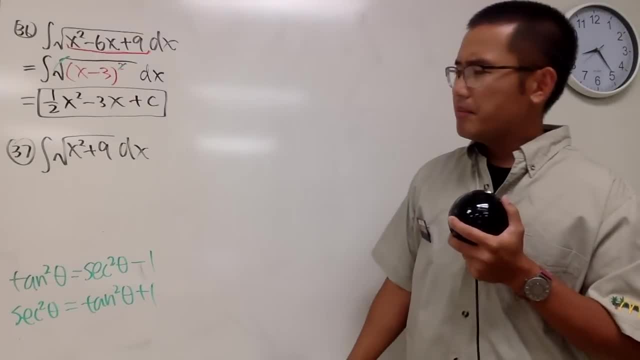 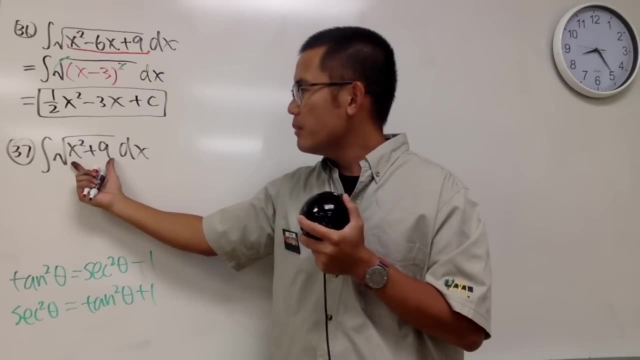 So that the square and the square root will cancel each other out. And perhaps the question is that: can we somehow make that happen with x squared plus 9? Can we somehow make this into a perfect square, so that the perfect square and the square root will cancel each other out? 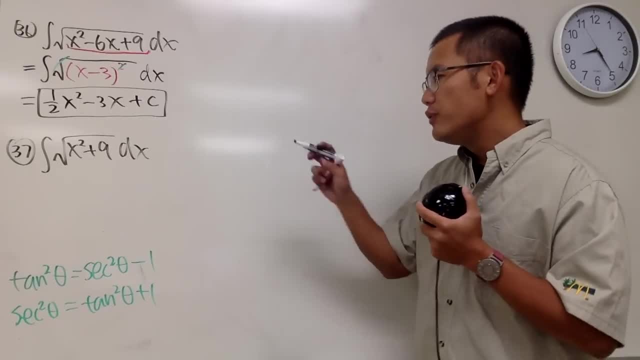 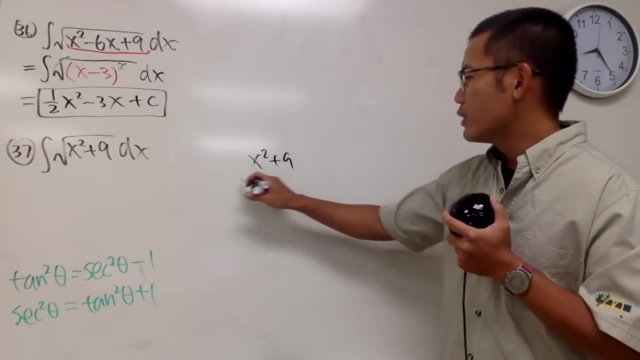 Like how we did it over here. Well, the truth is, if you want to do it with algebra, no, Because even though you can put down x squared plus 9, and you can write this as x squared minus 6x plus 9,. 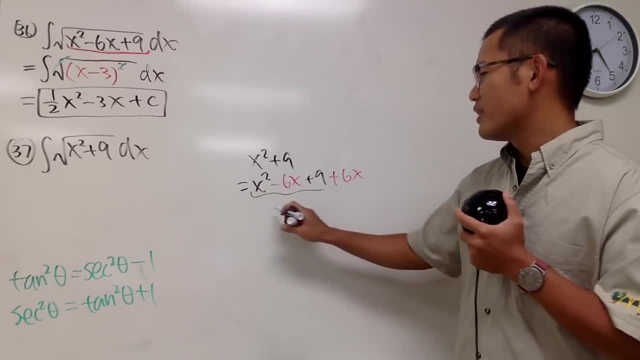 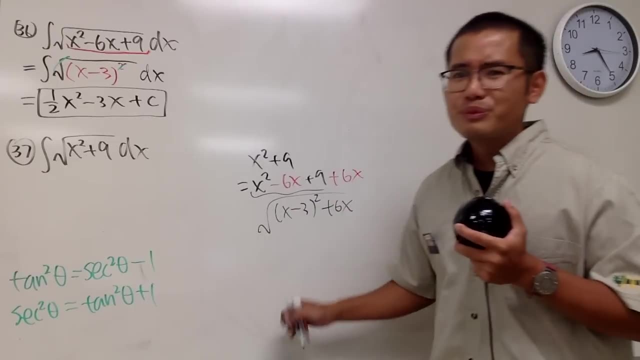 but don't forget, you still have to add the 6x. You can complete a square right here which is x minus 3 squared, but you still have to plus 6x afterward And take the square root. Still cannot do anything. 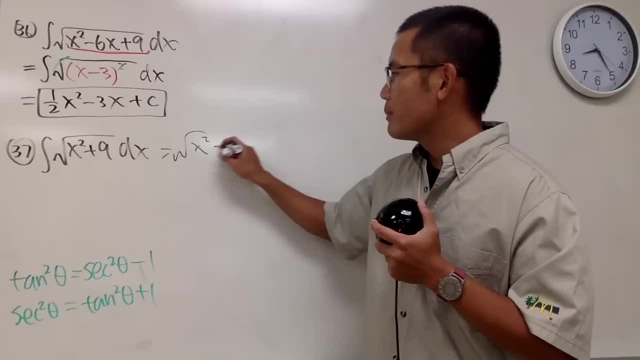 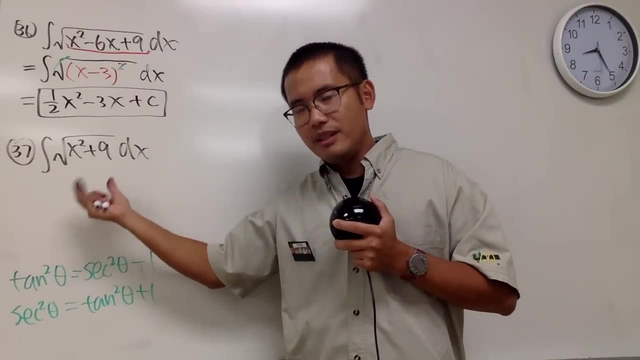 Oh, I know, Can I just do the square root of x squared plus square root of 9?? No, don't do that Order of operation inside out, so you cannot just take the square root of the first and square root of the second. 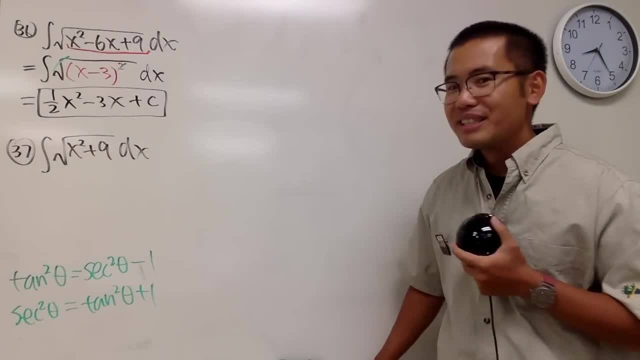 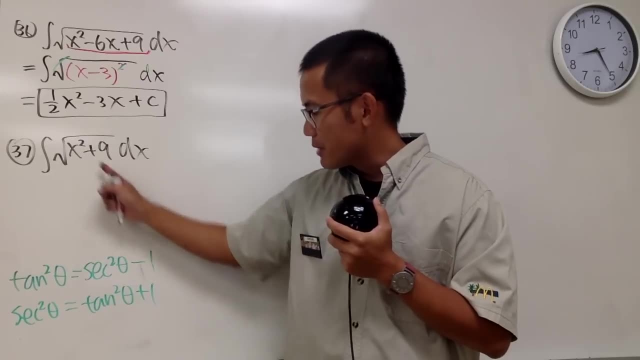 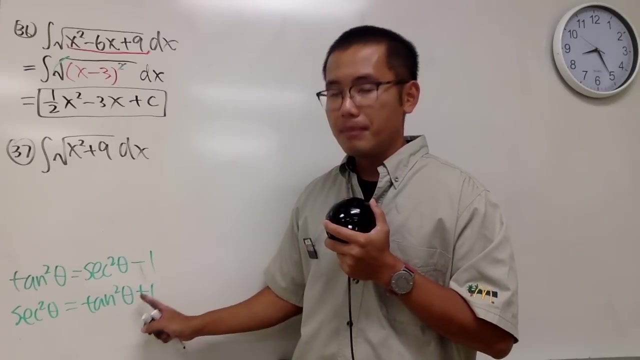 No, it's not like that. Take a look at the thing right here. Have a look, Especially this one, because I notice I have the plus that matches with the plus right here. Look at here we have tangent square theta plus 1.. 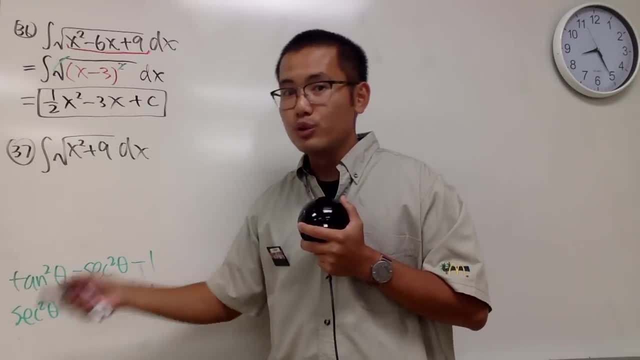 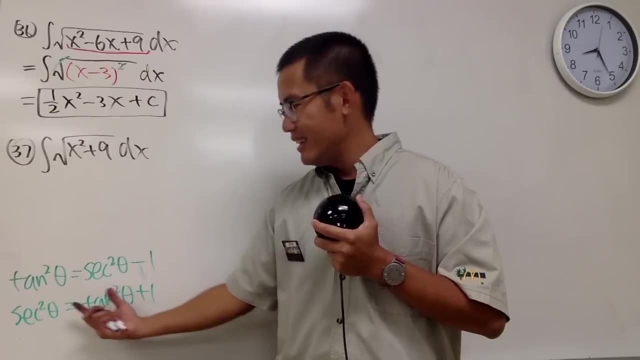 Two terms. On the left-hand side, we just have one term. Very nice, isn't it? Well, this is how we can complete a square in the theta world. Oh yes, I mentioned about the theta. Welcome to the theta world. 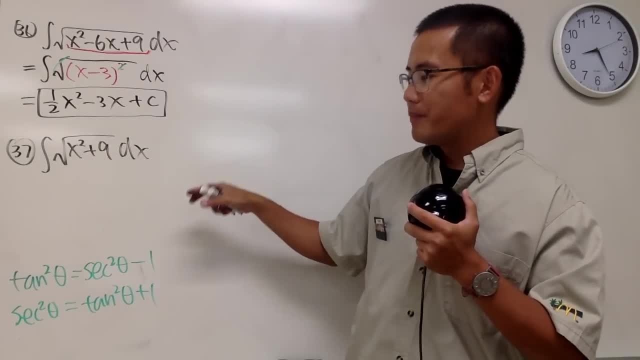 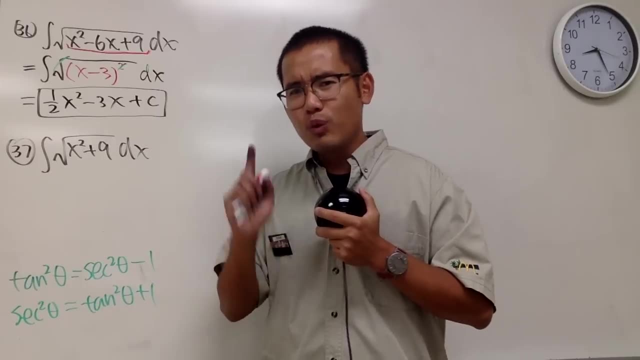 It's not possible for us to complete a square and just get one perfect square instead of the square root in the x world, but we can do so in the theta world, and that's what I want to show you. right, And let's see. 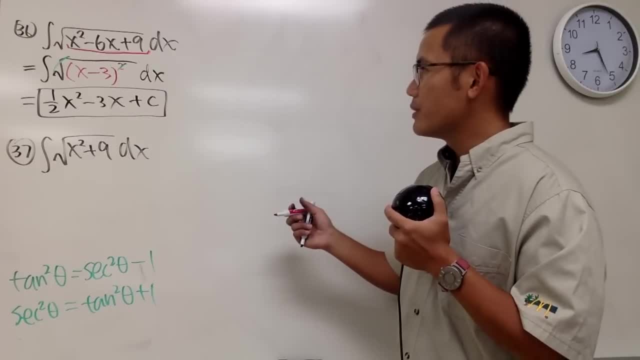 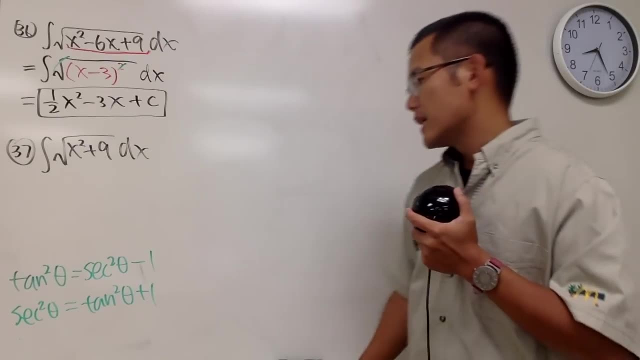 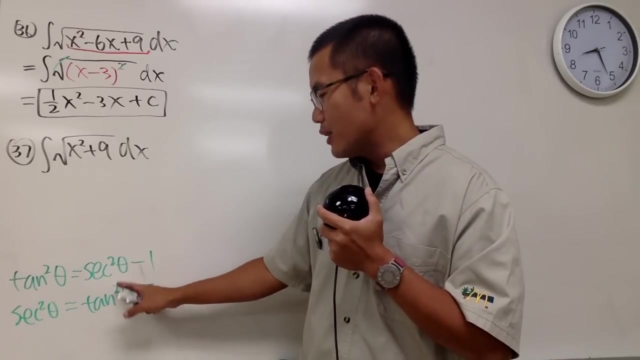 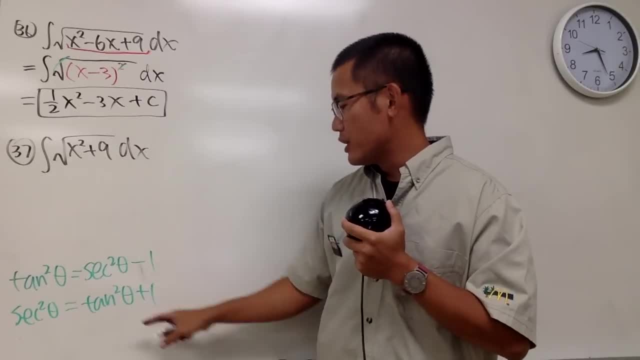 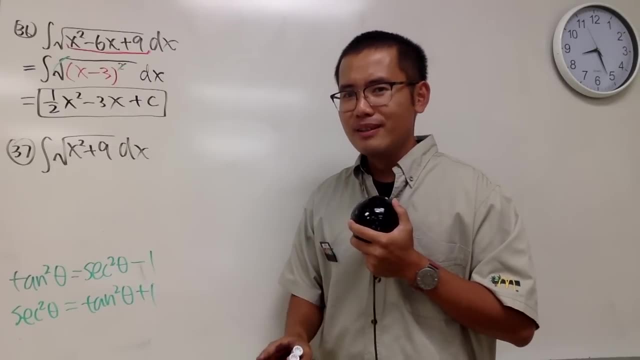 I have tangent squared theta plus 1.. The plus match, but this is 1, this is 9.. That's not good. How can I make the 1 equal to 9?? Don't say plus 8.. Okay, thank you. 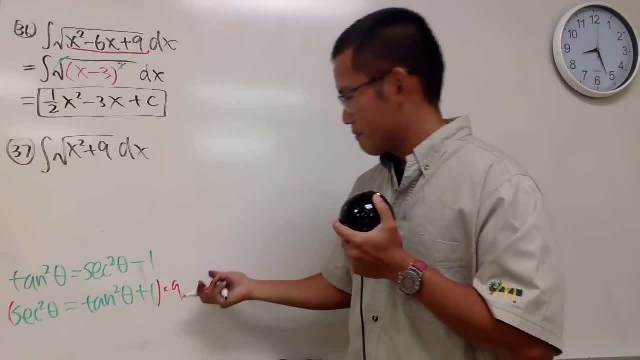 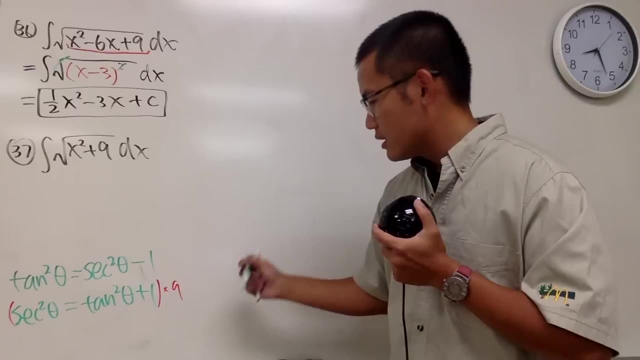 Yes, multiply this equation by 9.. That works, yeah. So let's just play around with these identities to see what we can get. Wow, Wow, Wow. do that. check this out Over there. we get- let's put on this first- 9 times this we. 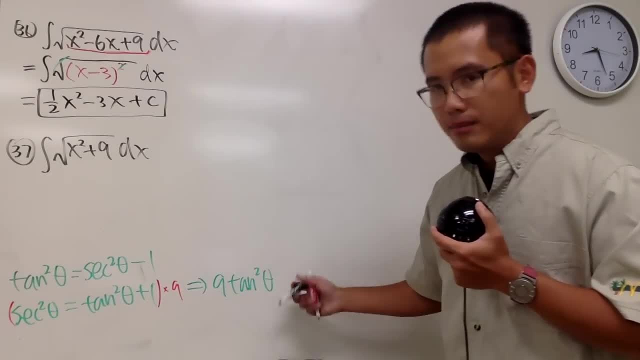 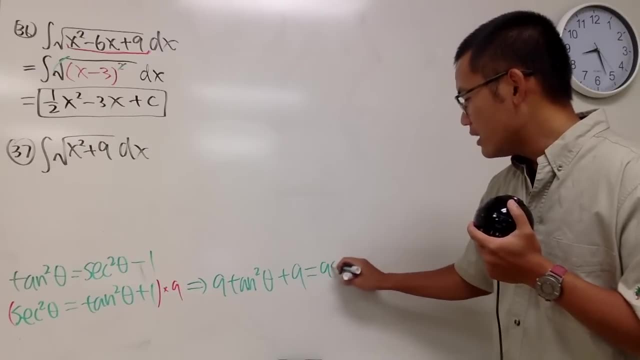 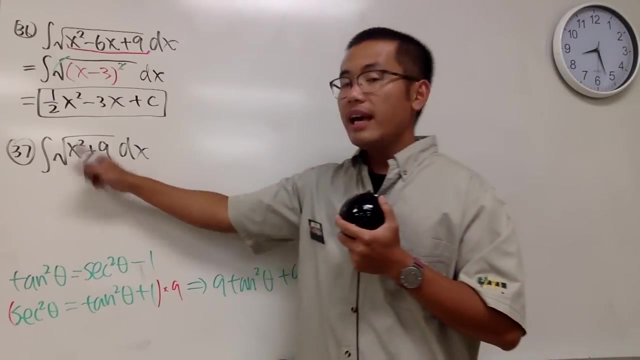 get 9 tangent square theta plus 9.. Good, And that's equal to 9 secant square theta. So that's equal to 9 secant square theta. Very, very nice. Well, notice that this right here is x to the second power. I want to have a quantity square. This is a 9 tangent square. 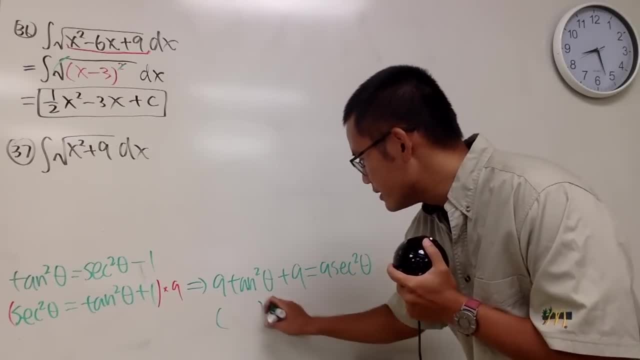 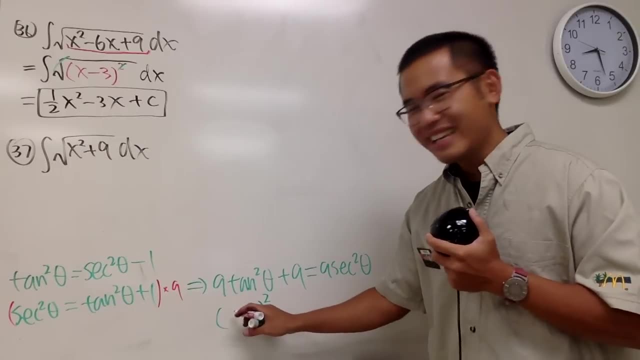 That's not good, but we can do the following: How about let's look at this as a parentheses square on the outside and let's play a game called filling the parentheses? You guys go Yes, inside. here we just enter the 3 and also tangent. theta 3 square is 9, tangent. 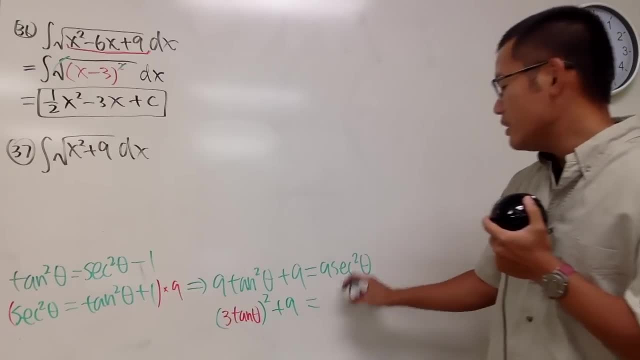 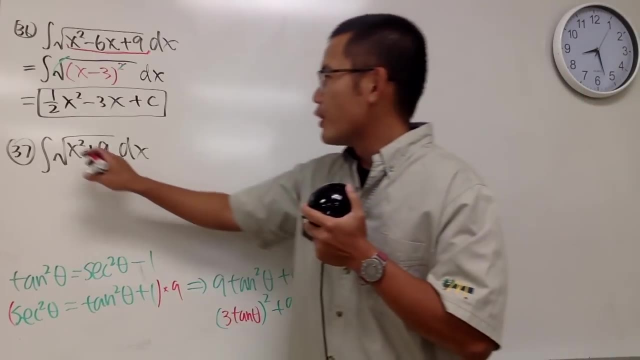 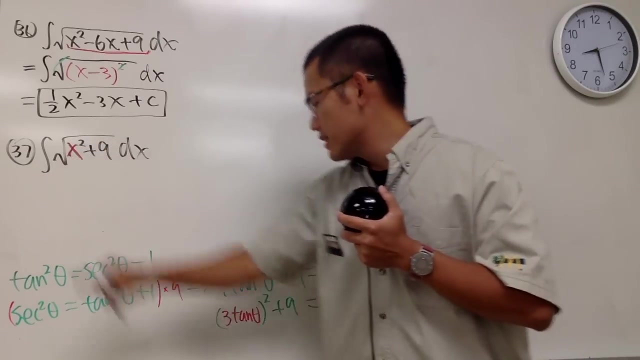 square is that, and put a plus 9, and this will be a nice, perfect square. 9 secant square theta like that. Now check this out Right here we have x. Wouldn't it be so good if we take x and make it equal to 3 tangent theta? That would be so wonderful. 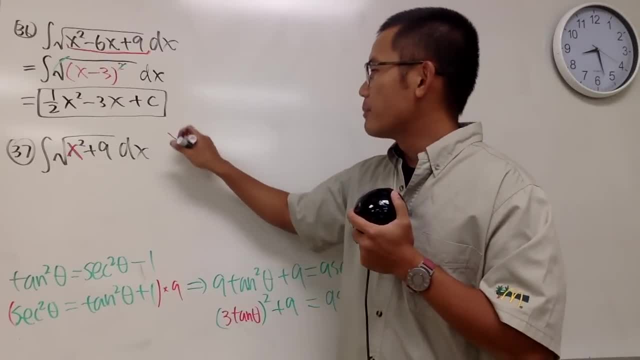 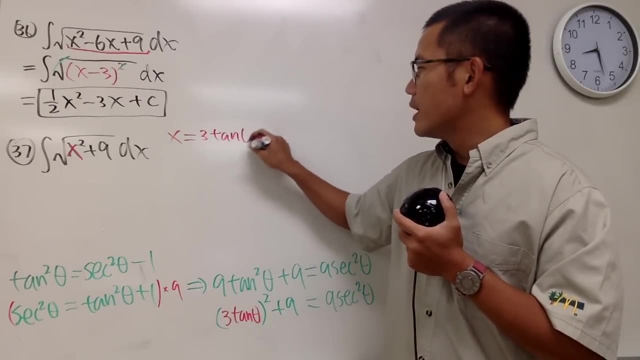 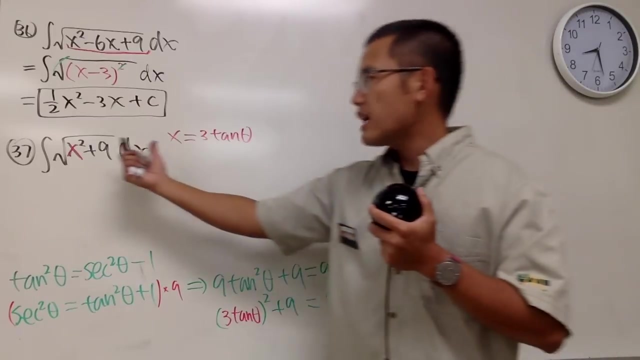 isn't it? That's exactly what we're going to do: Start by saying that x equals to 3 tangent theta, Because, again, if x is equal to 3 tangent theta, it will work the same thing. It will work out to be like this, and we can just put this inside of the square. 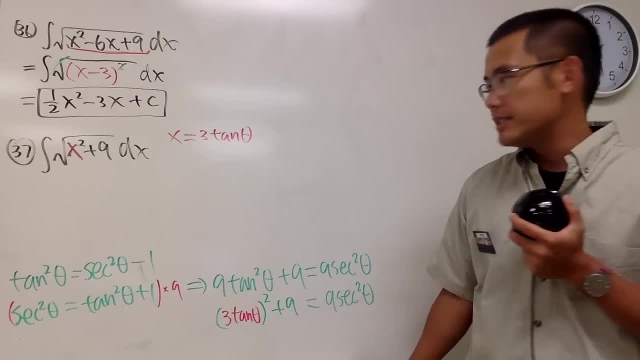 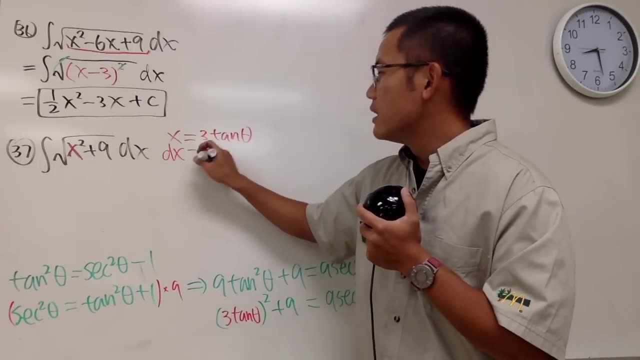 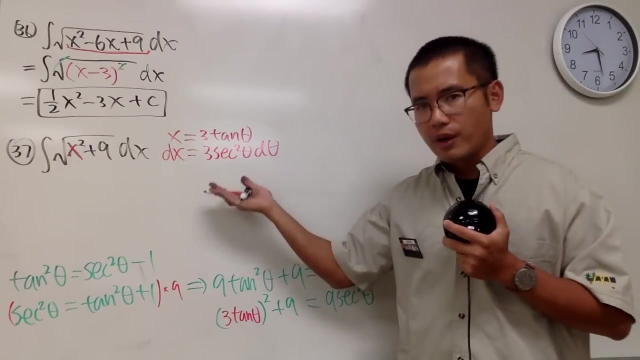 root and square root of this guy will cancel very, very nicely. So that's the idea, Okay, but don't forget the usual business. We still have to differentiate both sides. dx is equal to the derivative of this, which is 3 secant square, theta, d, theta. Don't forget about this. 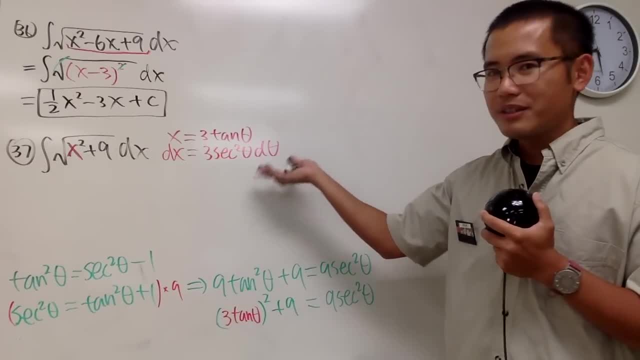 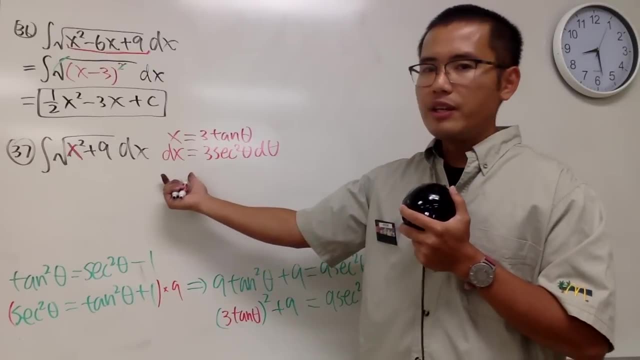 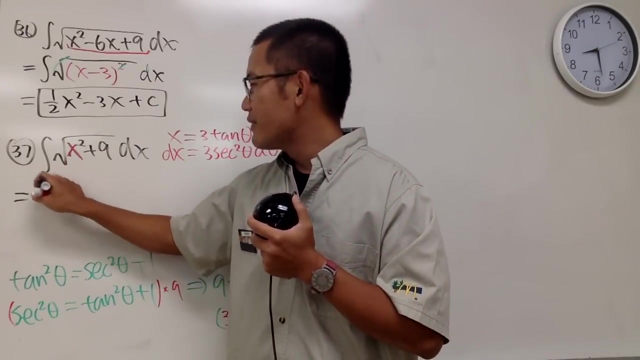 This is like a really crucial thing that people forget. all right, So don't forget about that. Keep this in mind. And when we do this kind of substitution, dx is right here already, so we can just put everything back, to take everything to the theta world. Let me show you. Here we have. 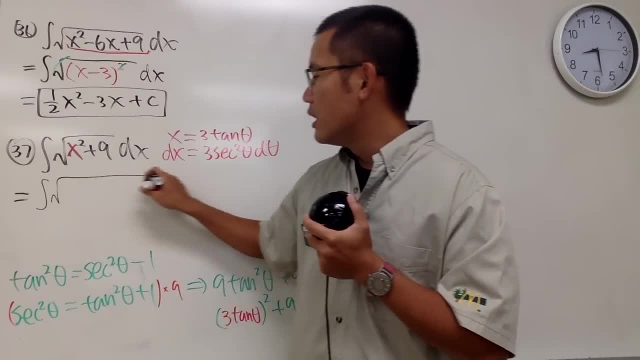 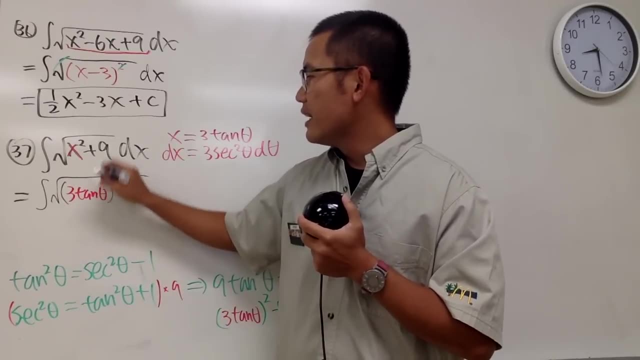 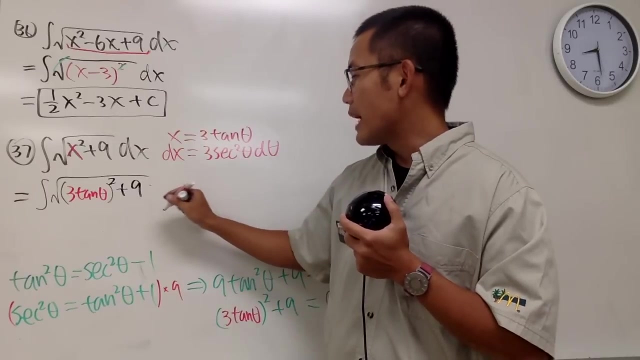 the integral and we have the square root. This x is just that. so I'll put down the parentheses with 3 tangent theta inside and then we'll square that, and then we have plus 9 after this and the dx is all that. so I'll multiply it by 3.. 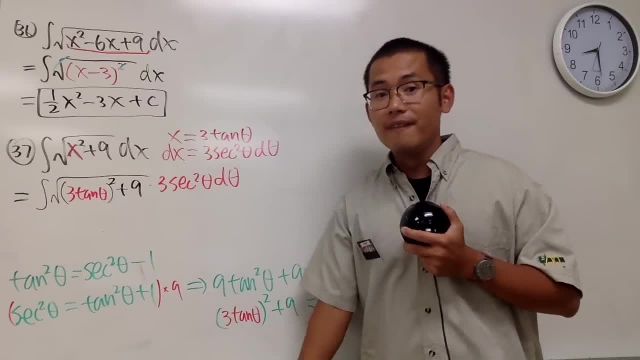 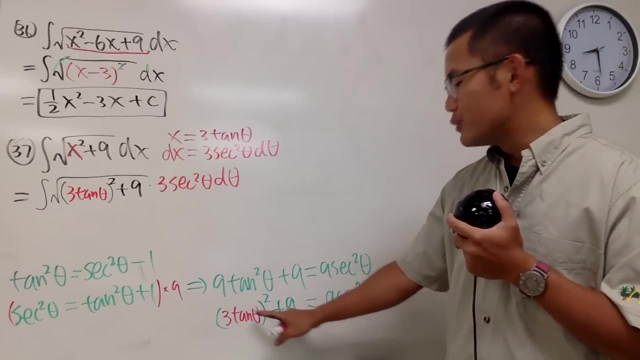 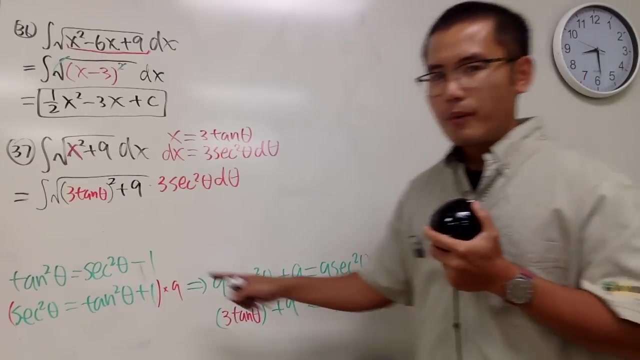 Secant square, theta d theta like this. Very nice, isn't it? Now check this out: 3 tangent square theta square. 3 tangent theta square plus 9.. This is just the same as that which is the same as that. So if you work this out, you end up with this. So of course, we can. 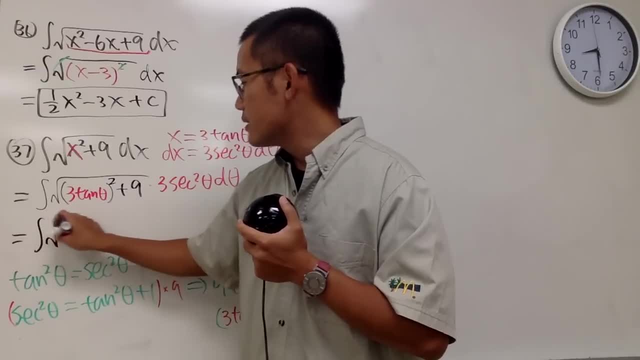 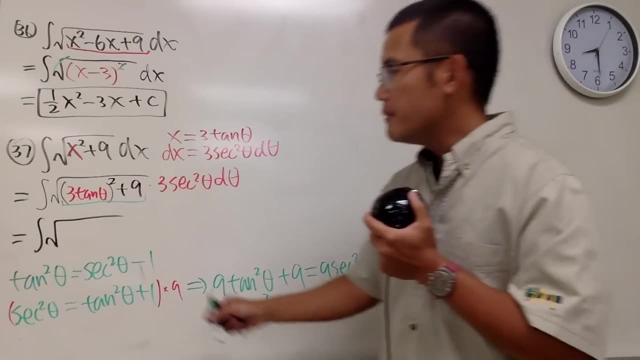 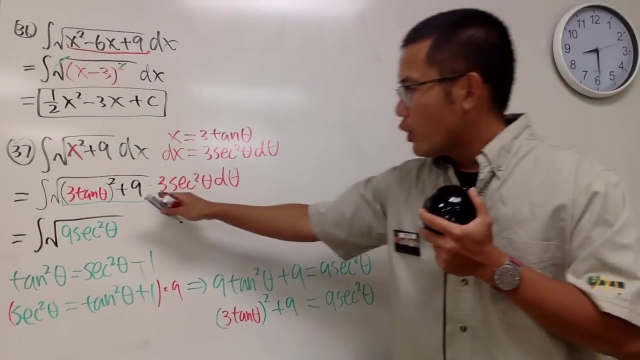 look at the next line as the integral, as the square root, This whole thing. here again, just work this out and use identity. We will just end up with 9 secant square theta, and that's very good. Don't forget we still have the red part. 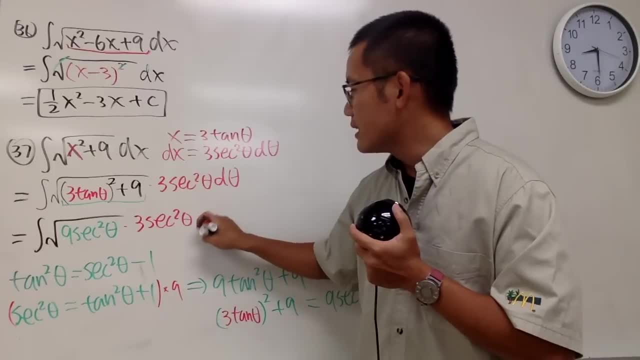 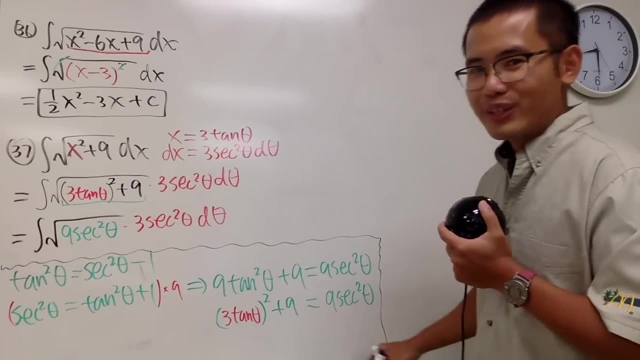 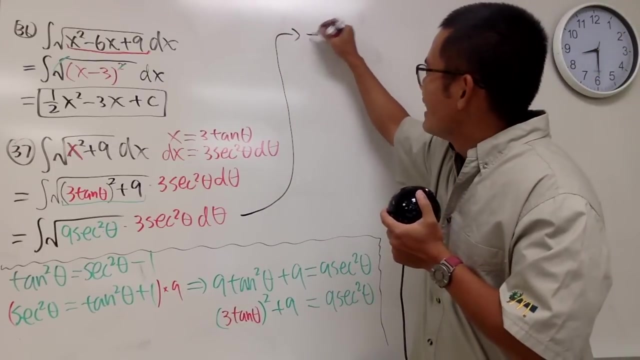 so let's multiply by 3 secant square: theta d theta. okay, So again, let me just kind of draw a little separator like this. That was my scratch work. Okay, We need more space. Big integral sign: All right, Integral, All right. Square root of 9.. This right here is a product of two. 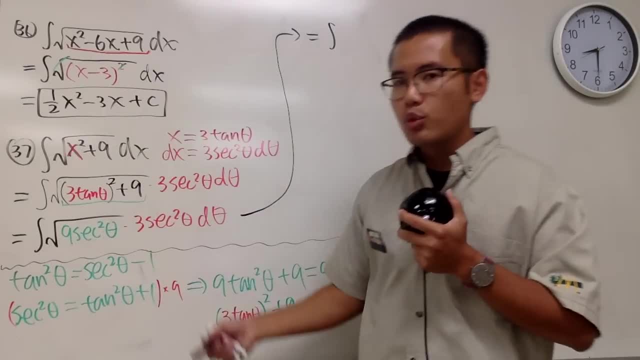 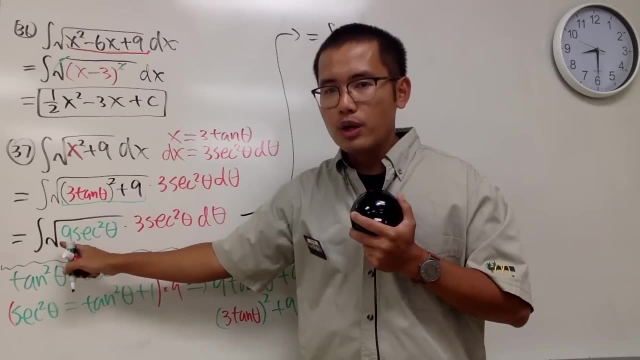 things and we can just take the square root of the first and then the square root of the second. That's nice. So here we have just the 3, and then secant square and then square root. This and that cancel. Don't need the absolute value, yeah, So I just put down. 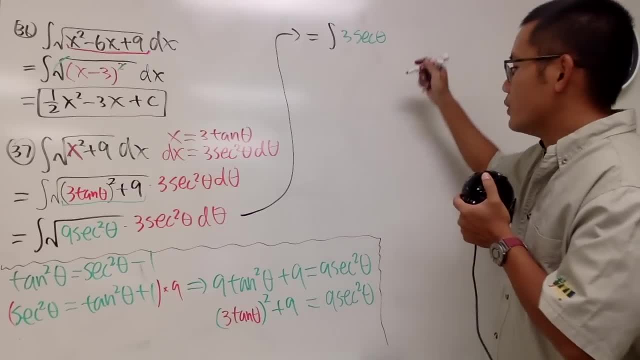 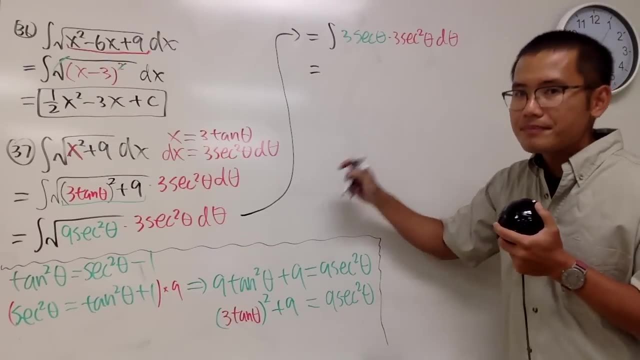 secant theta. and then- don't forget this- We still have 3 secant square theta d theta. Now, ladies and gentlemen, 3 times 3 is 9.. Let's put that all the way in the front: Integral. 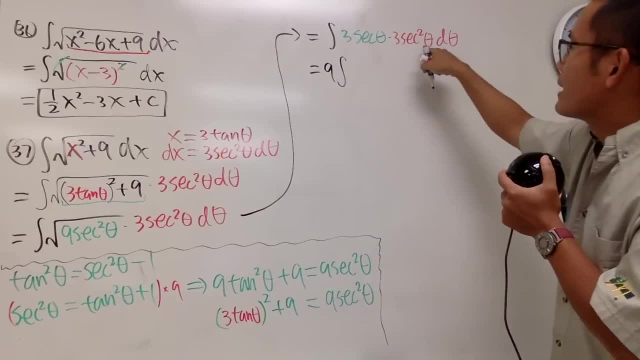 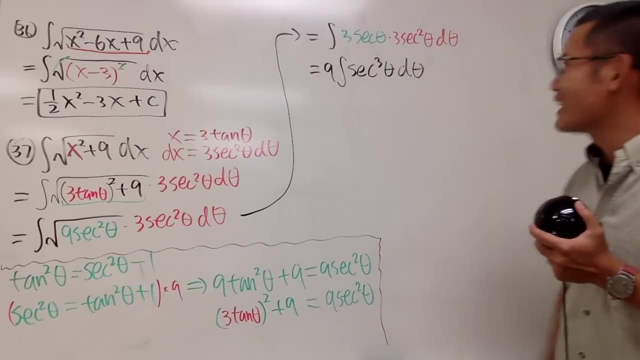 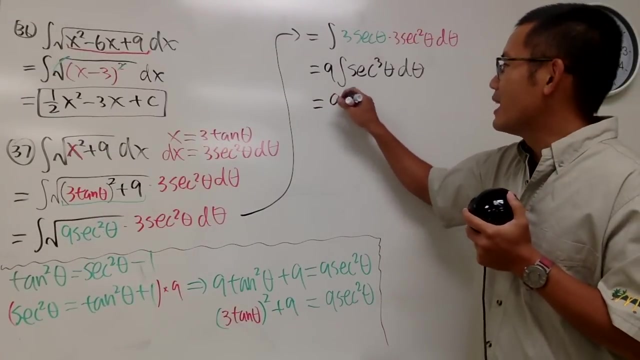 yes, yes, yes. Secant to the first power times. secant to the second power is secant to the third power. theta, I know You guys are like, oh my god, right, That's why we did a secant to the third power. Of course, we'll just use the result that we got earlier, so just, 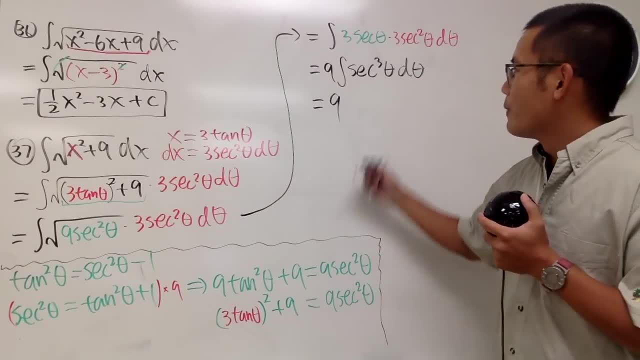 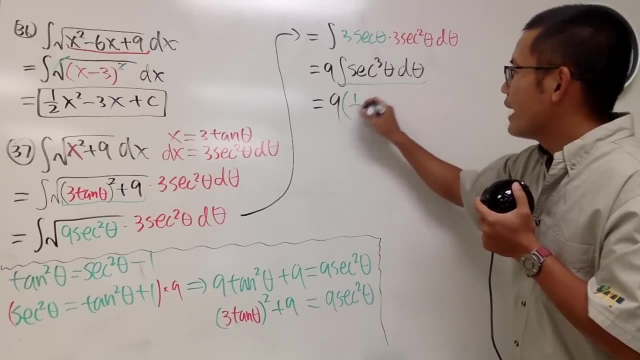 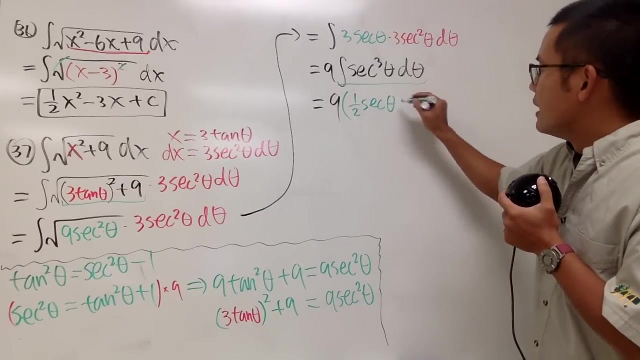 look back to the things that we did earlier And we'll just use the result that we got earlier And when we have that, I'll just put down parentheses for you guys. The answer to this part is 1 half secant x times well, we're using. we're in the theta world. This is secant. 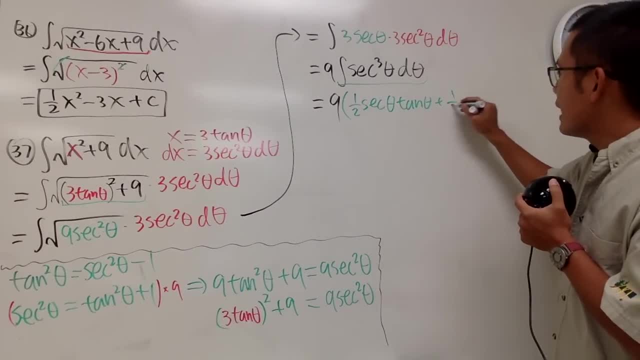 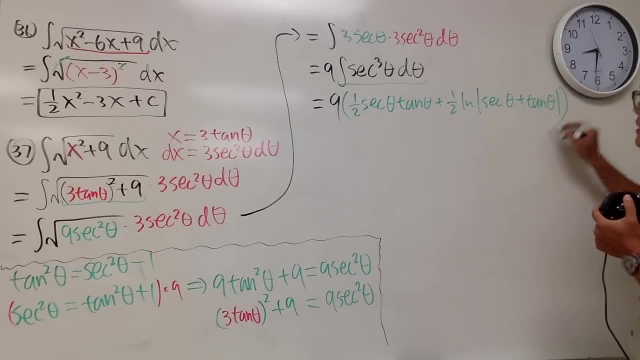 theta times tangent theta plus 1 half natural log absolute value of secant theta plus tangent theta like this. So again, that's why I set up this worksheet, So in this video, in this way, a lot of things we have just looked back to, the things that 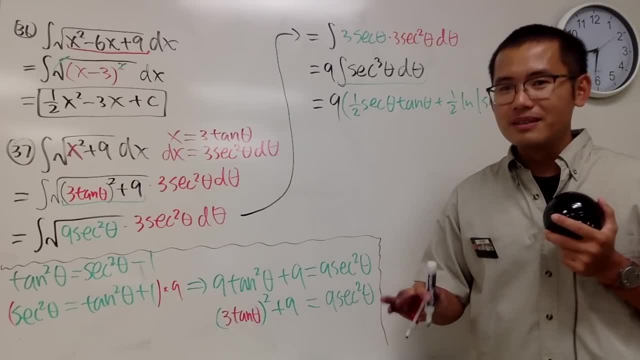 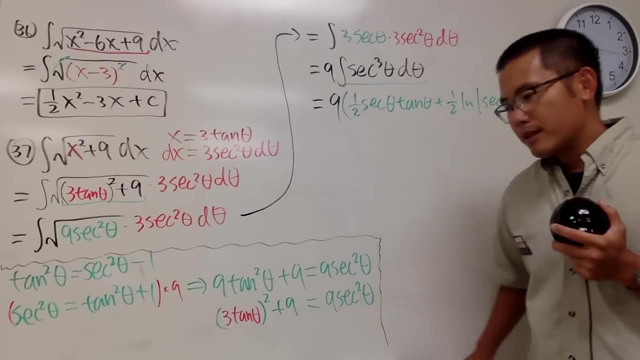 we did before. This is why it makes calculus hard. yeah, because you have to do a lot of things, that you have to remember a lot of things from the past. But practice is the key. and then, just putting it over, you can do it too. One day you'll be able to say: 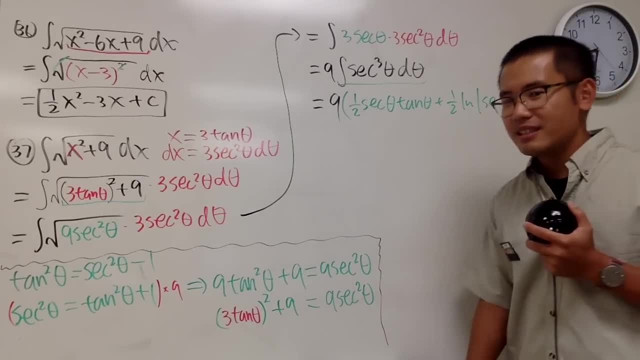 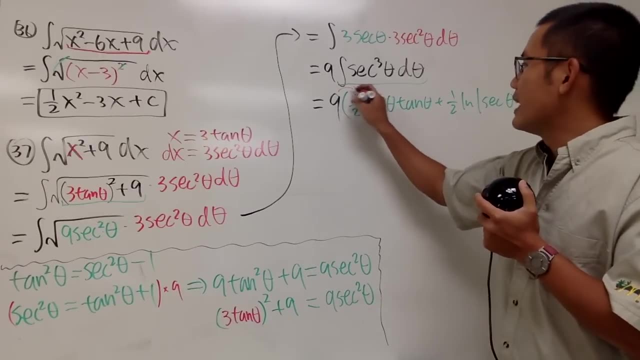 hey, this is actually pretty easy After you have to practice so many times. We are not done yet. I know I'm sorry. we have to distribute the 9 to the parentheses, but also, just like usual, right now we are in the 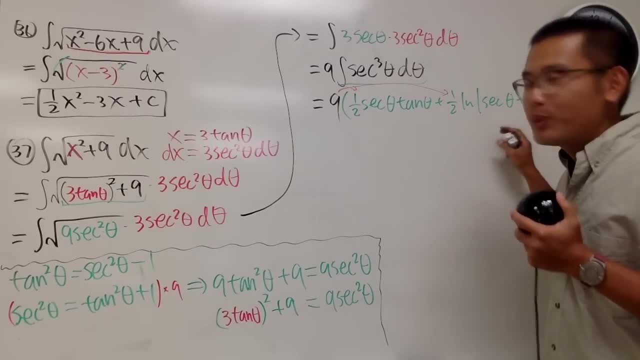 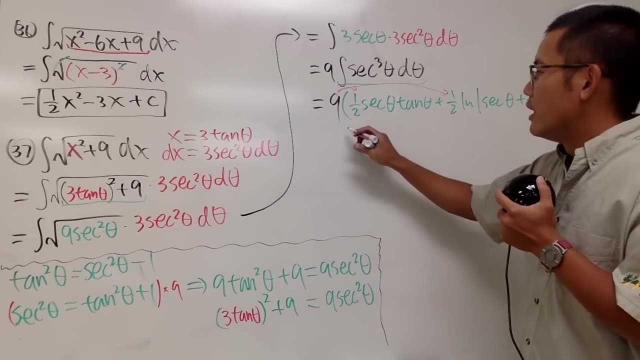 theta world. This is just as cool as the u-world, but we have to go back to the x-world. Well, how We are going to look back to this again? Have a look here. We know x is equal to 3 tangent theta. 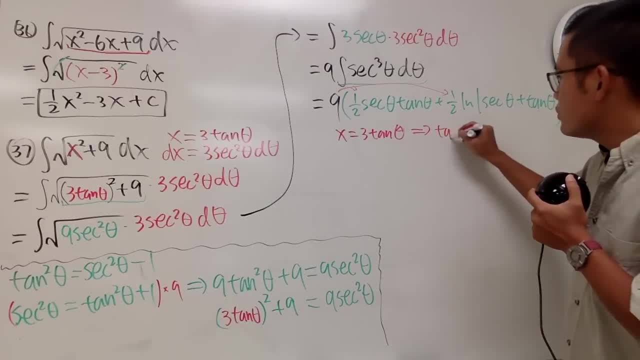 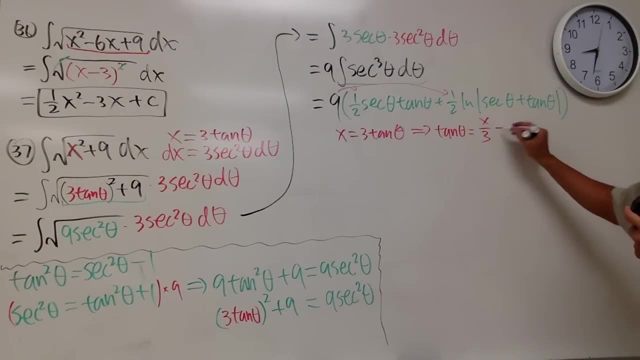 Well, from here we can devise u on both sides, so we get tangent theta equals x over 3, and from here we can draw a right triangle. and we like to use the right triangle because we'll be able to figure out sine cosine whatever from right triangle, That's. 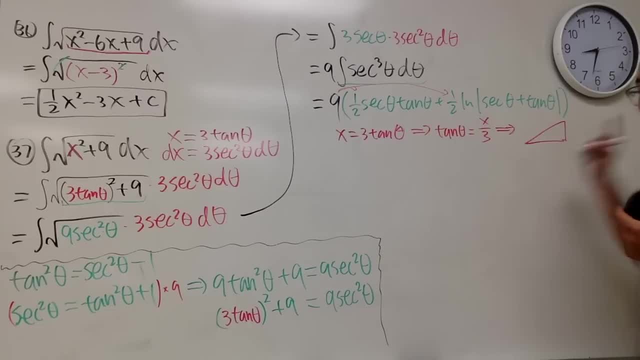 really easy. So here is the right triangle. I would recommend you guys always draw the right triangle this way, Put the right angle here and the angle theta here, just for consistency purpose. Now, tangent on the right triangle is opposite over adjacent, so the opposite. 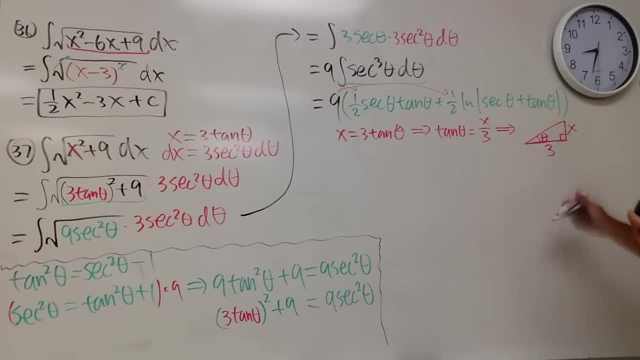 and the tangent in a upper right triangle is also the opposite, and the tangent in a lower right, right here is x and the adjacent here is 3. And you have to finish this triangle means that we will have to figure out the hypotenuse. And for the hypotenuse, 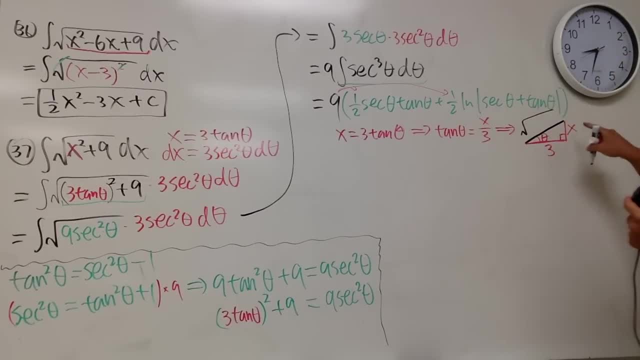 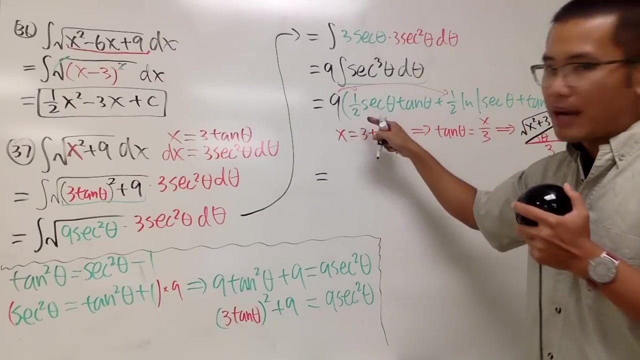 it's not that bad. You first open the square root and you do the sum of two squares. So you do x squared plus 3 squared and, yes, that's pretty much the original square root. All right. so let's see: 9 times 1 half, we get 9 over 2.. Good, Here we have secant theta. 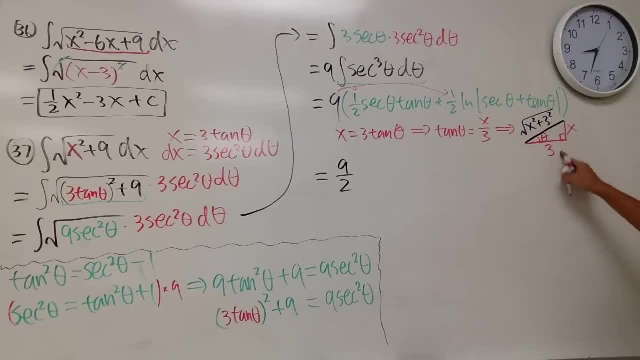 By looking at this picture here, secant is hypotenuse over adjacent, so we have this over that. So we have square root of x squared plus 9 over 3, because 3 squared is 9, so that's why I put it down. Then we have tangent. theta tangent is just x over 3, or it's right here. 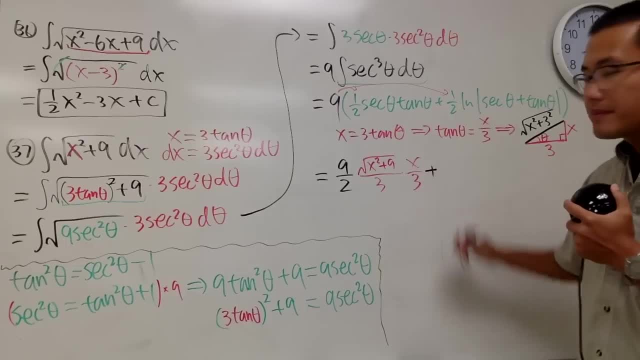 So we have x over 3.. And then we add 9 times 1 half, so again it's 9 over 2.. And then the rest is pretty much the same thing: Natural log, absolute value. And here we have the secant theta which is this over that. So square root of x squared plus 9. 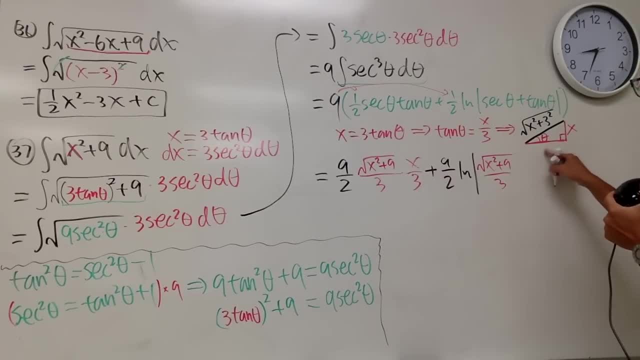 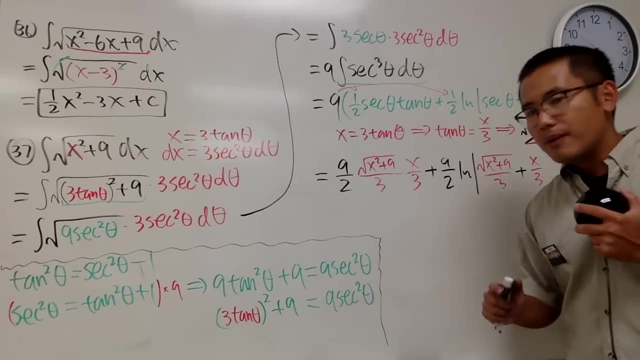 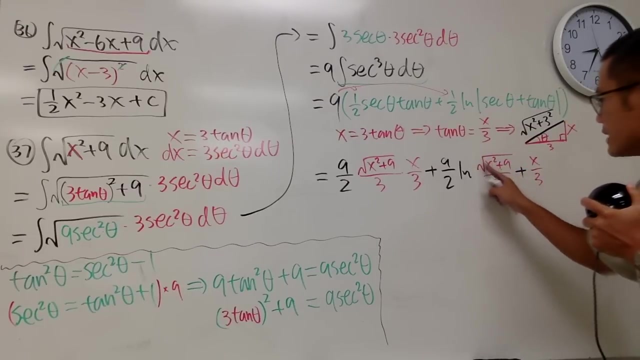 over 3.. And we have the tangent theta, so plus this over that, so x over 3, like this Now, in fact, once we get to this point, once we get to this point, notice how this is always bigger. 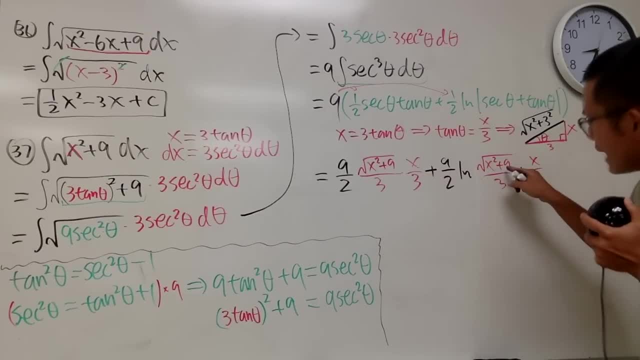 than x, because this is pretty much x. When you add 9 to it inside of the square root, this is always bigger than x. So, in other words, this is always going to be bigger than that, And this is always positive. Well, at least this is never negative. So in the end, 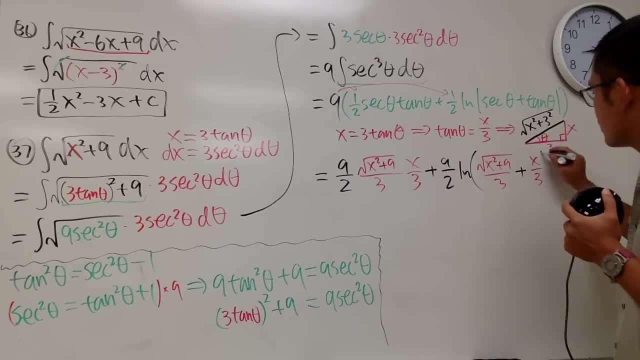 the inside here is never negative, So parentheses is actually okay. Yeah, You can try a number on your own. You can try: x is equal to negative 17. You will see, the result is always positive anyway. So that's pretty much the idea. However, we're not entirely done yet. 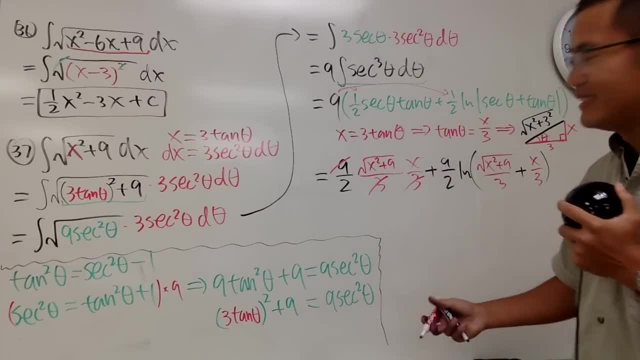 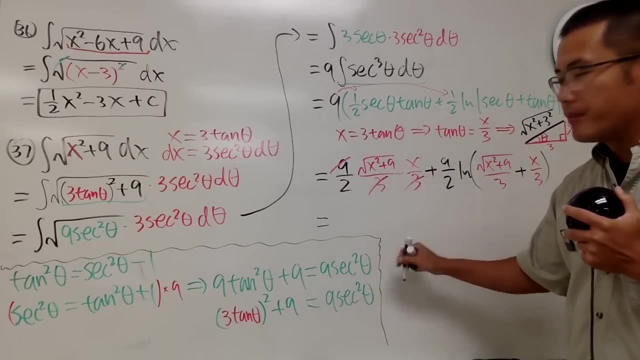 3 times 3 is 9.. Cancel, cancel, cancel, cancel. Yeah, I know, But not only that. I also have to discuss another thing for you guys. Let me write this down for you guys: 1 half. we have the x right here. 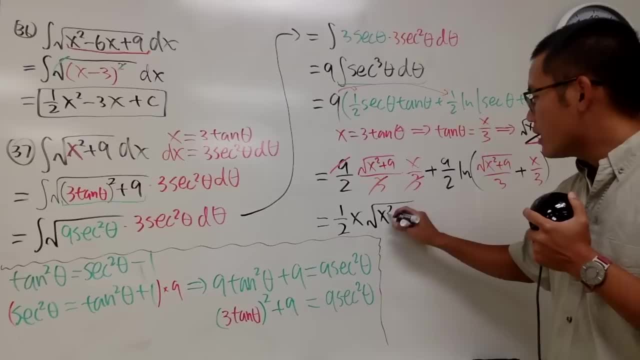 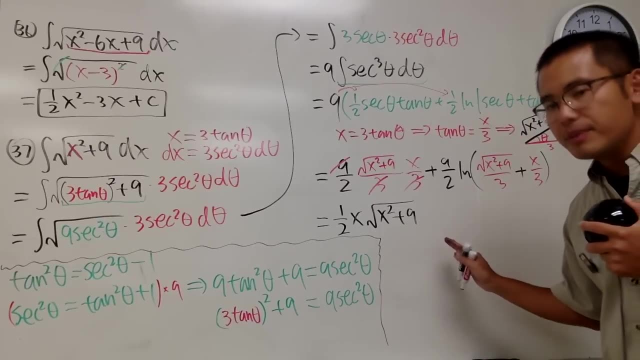 Let's put that down, And then the square root and then the x squared plus 9.. That's good, And if you just want to put this down as how it is on my exam, that's totally okay, because I know the trouble that we have to go through. I understand, You understand too. 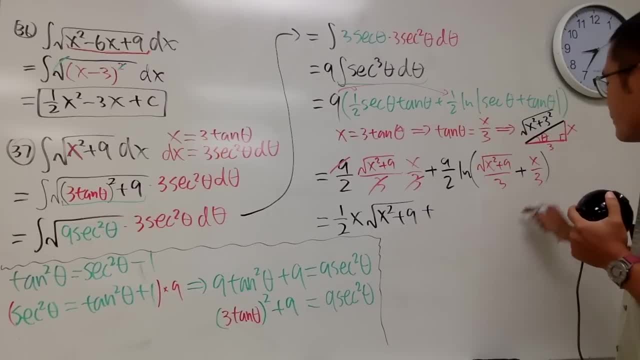 So if you want to just write that down, that's totally okay, But let me put this down for you guys. Let me write down 9 over 2, natural log Notice for this part. of course you can combine the fractions. 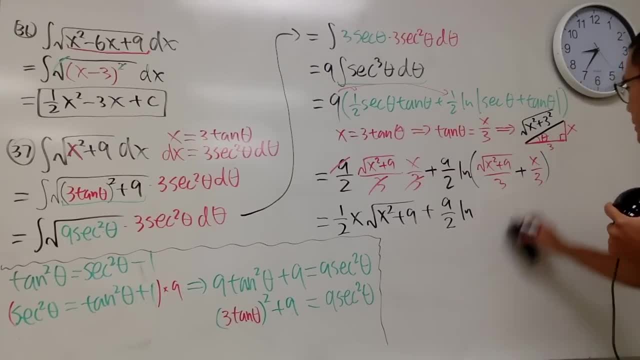 Of course, we can just write this over 3.. Yeah, So let me just do that for now, right here. So we have this plus x over 3, like this, And we are going to use the log property And the. 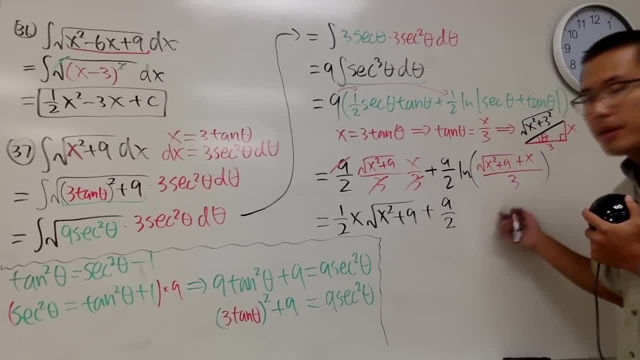 property is, of course, natural log of the top minus the natural log of the bottom. So technically I can look at this part as natural log of the top, which is square root of x squared plus 9, plus x, like this, and the minus natural log of 3,, like that. All right, And now I should be putting down. 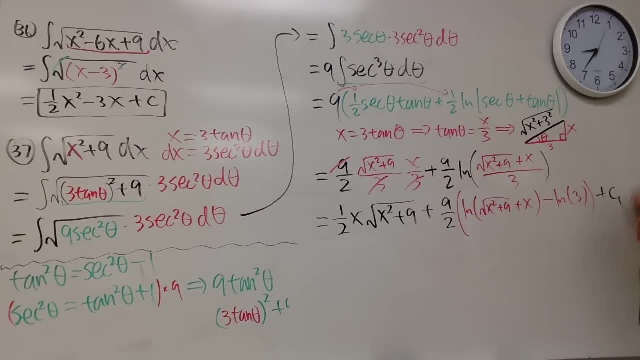 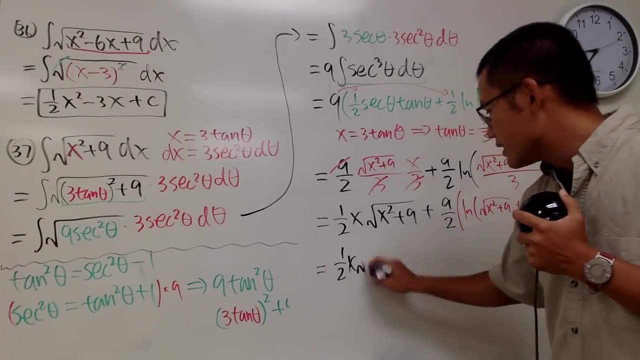 a plus c. I should put down plus c1, like this, for example. Here is the deal. This part I know states the same. So 1 half x square root of x squared plus 9.. Next, this times that. so it's. 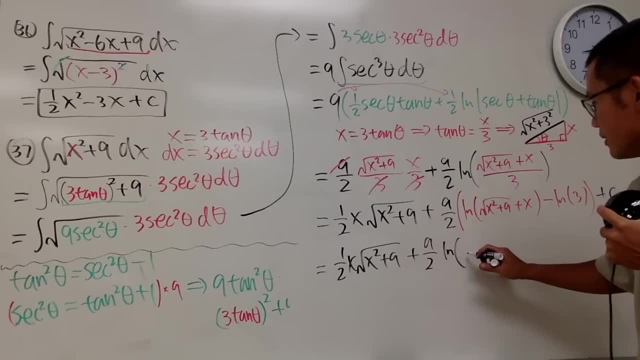 plus 9. half natural log of square root of x squared plus 9.. So that's good, And now I'm going to look at this part of x squared plus 9 plus x like this: Well, the next thing I will have to do is: 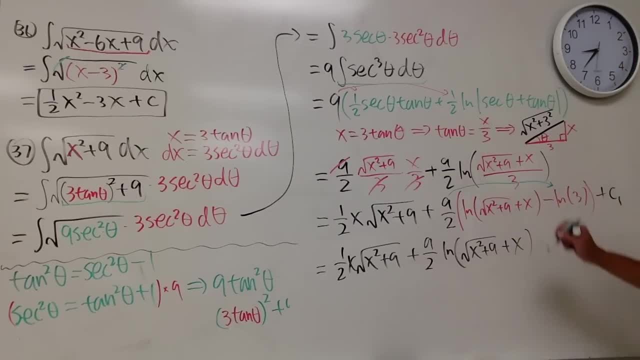 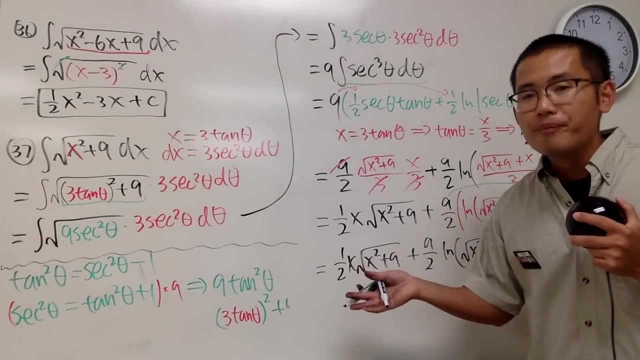 this times that. But you see, 9 half is just a number, It's just a constant. And negative natural log of 3 is also a constant. This times, that is just a constant plus another constant. It's just a constant. There's no variable. So in the end we can actually just combine all the. 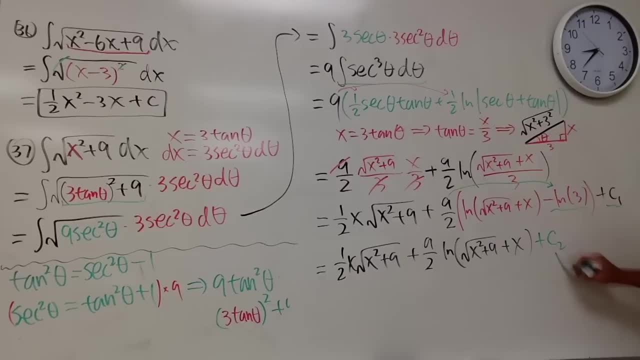 constants together, We can just say: oh, this is a constant, This is a constant, This is a constant. And again, this would be combined as this is: I say, negative: 9 over 2 ln, 3 plus c1.. That's the. 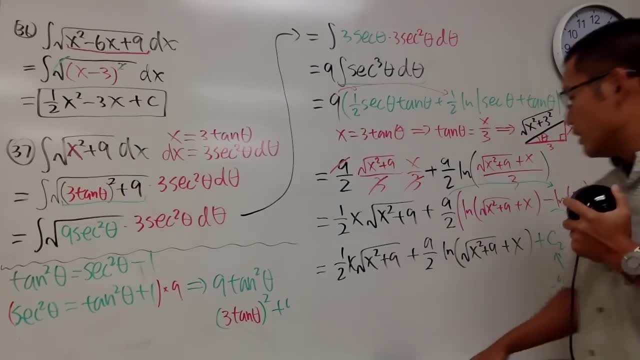 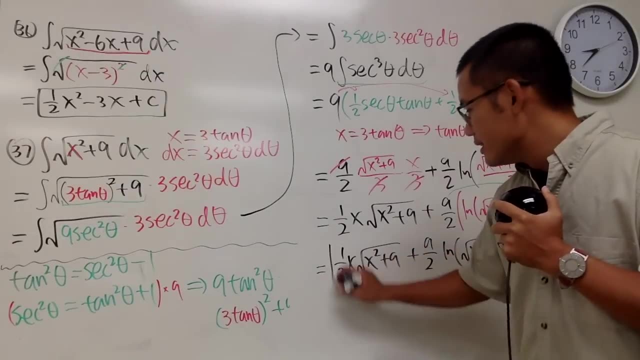 idea. They're just numbers, So we'll just put that as a number. This is the final answer. So if you would like, you can just say that's plus c, But I will just leave it like this And this whole thing. 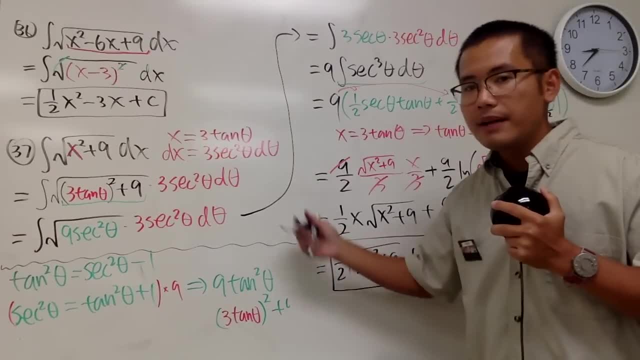 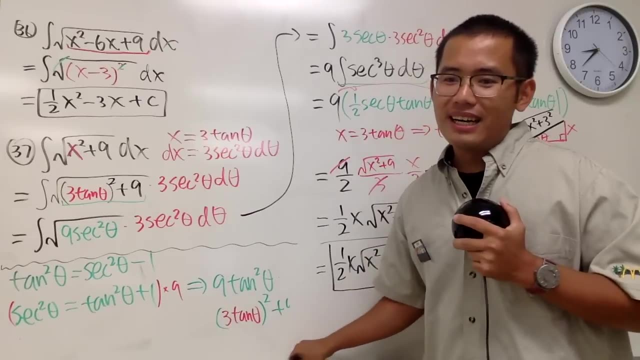 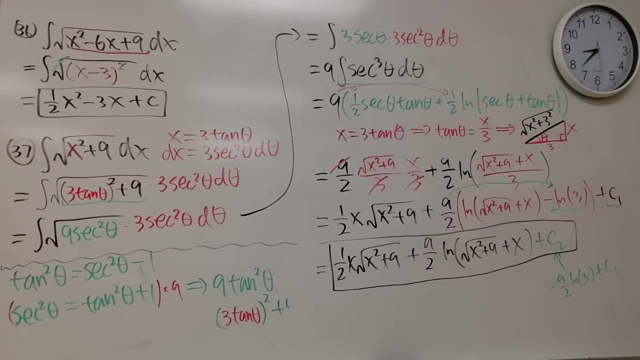 is the answer right? So that's this question, And I haven't told you guys the category for this one yet, huh, So just take a look again, Man. yo, this is. yeah. I hope I didn't make any mistake for this one, because if I did, 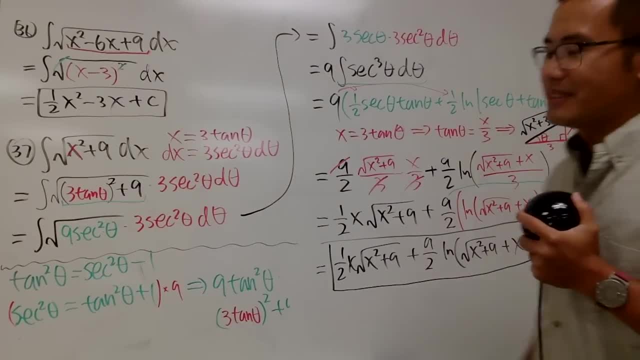 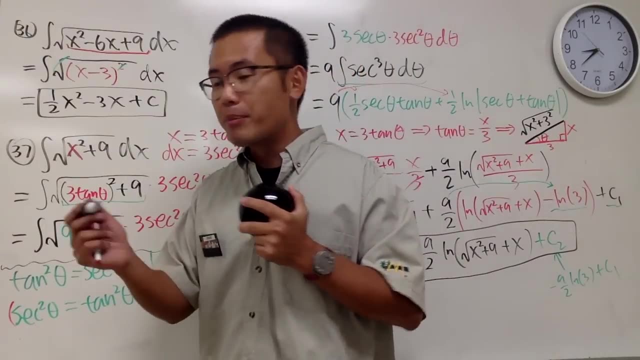 then it's not fun. Yeah, this is. you'll be crying, I don't know. Anyway, this is 37. And this is category number 9.. This is the part that you have to know. We are going to the theta. 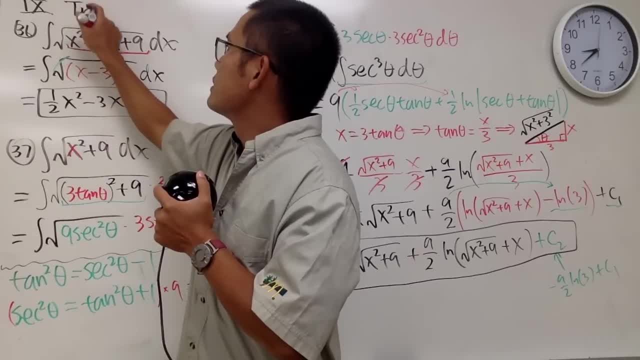 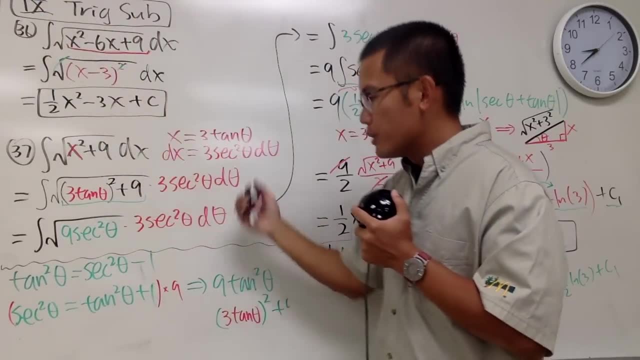 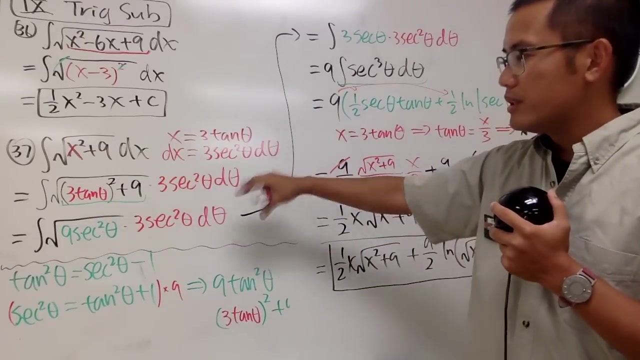 world. And, ladies and gentlemen, I will just tell you guys, this is called the trick sub, Because not only we're utilizing the identities, but again we actually have to use take x to the theta world first, and then do the derivative and then integrate it. 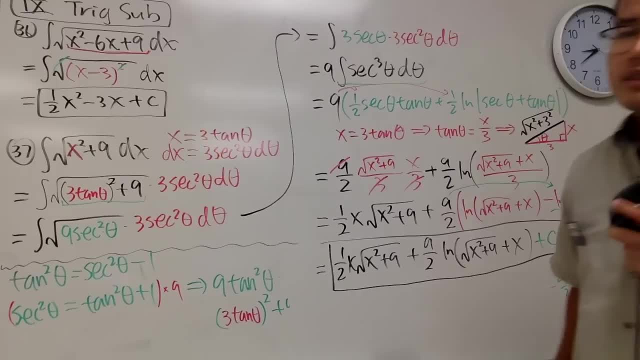 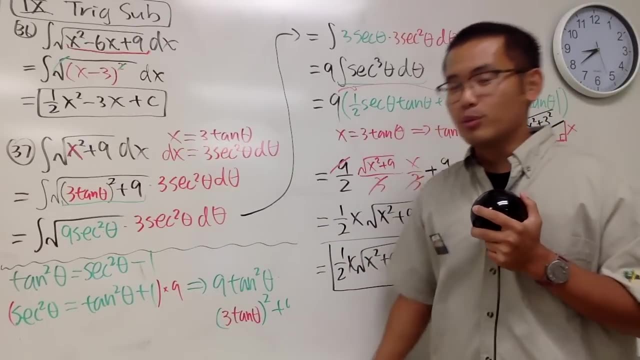 integrate in the theta world and then go back to the x world. So that's the trick Substitution, And sometimes it works out pretty nicely, just like this. Also, you can do that one with integration by parts, but you will have to have another function. but maybe that's later on. 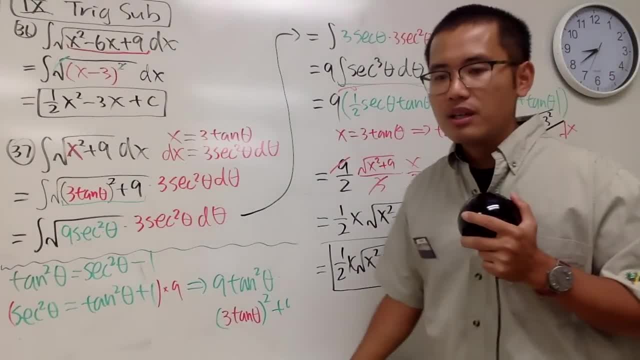 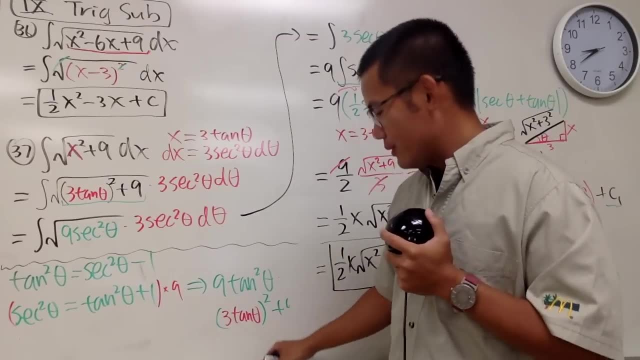 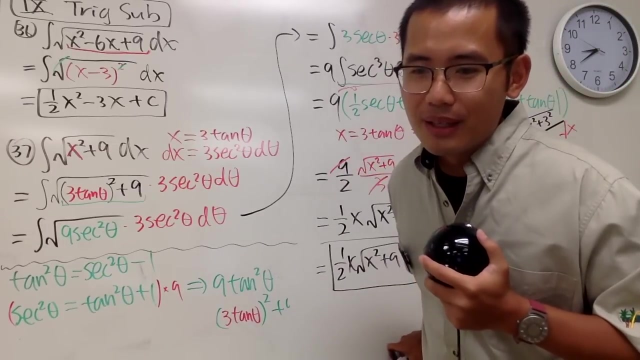 This is the standard way to do it for the trick substitution Right. So I'm going to erase the board and I will give you guys a couple questions for you guys to try out. yeah, Well, we have, I will give you guys. 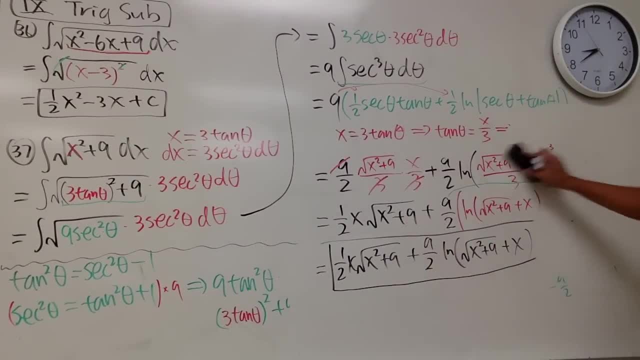 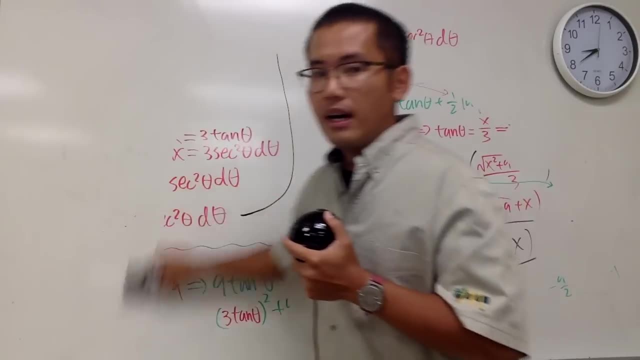 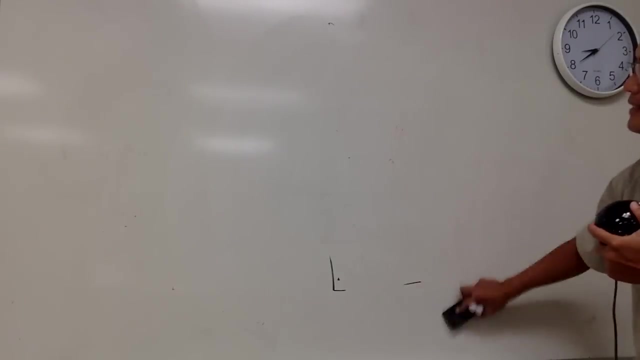 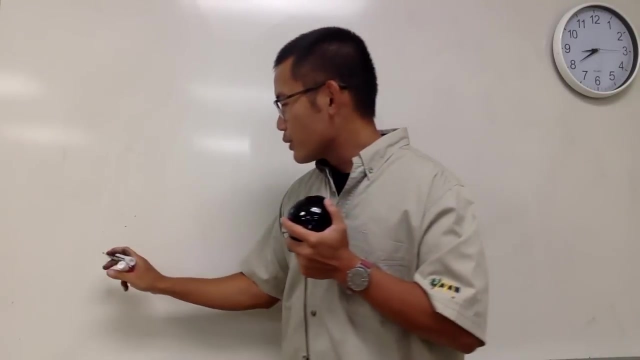 three questions for you guys to try. Of course, it's just the last. the next three questions, So again. oh, actually I will have to, man, let's see, let's see, let's see. I will actually draw this for you guys, So recall. 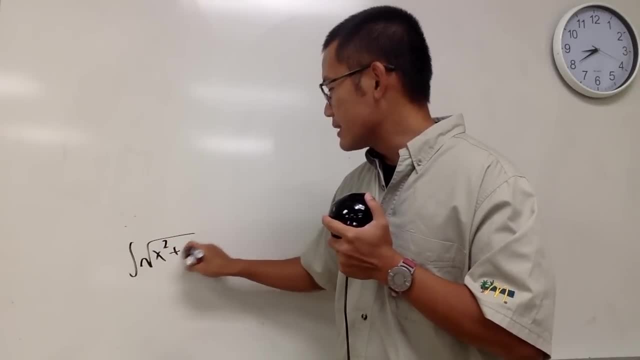 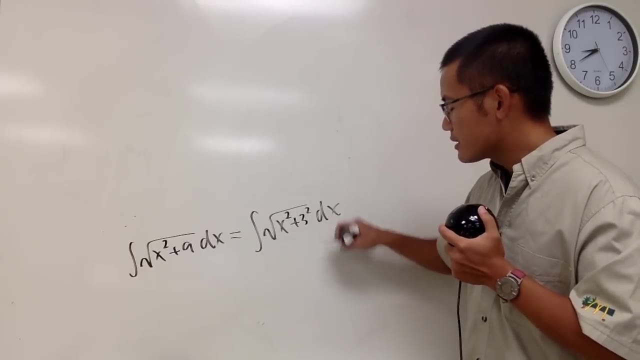 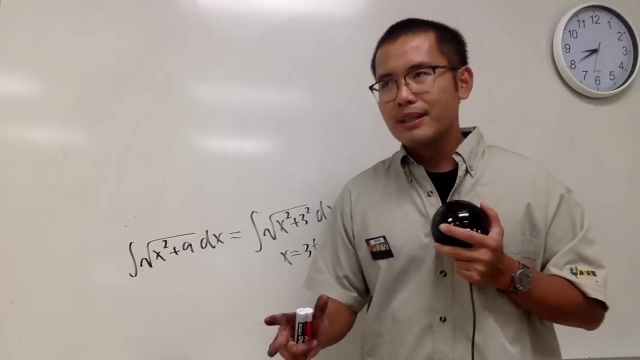 earlier, when I have the integral square root of x squared plus 9, dx, That's the integral of square root of x squared plus 3 squared dx. What we did was x is equal to 3 tangent theta. Now let me give you a nice chart, Chart, Chart, chart. Let me give you. 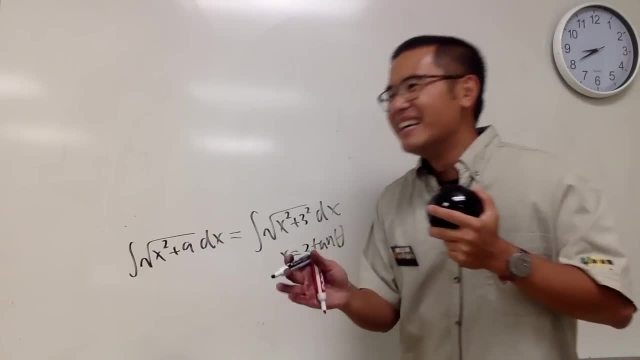 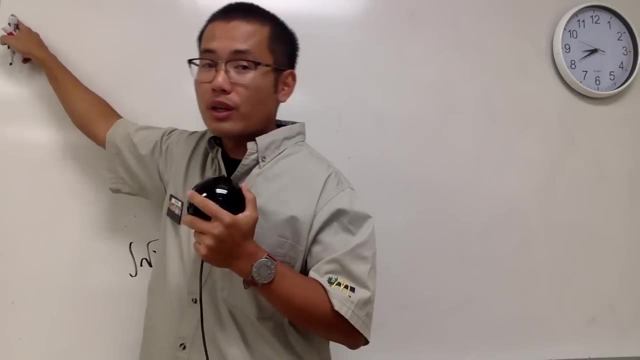 a nice table on what you see, what you do and what you use. okay, So this is the table and it's also on the PDF file. We'll just put it down right here for your convenience. So first of all, 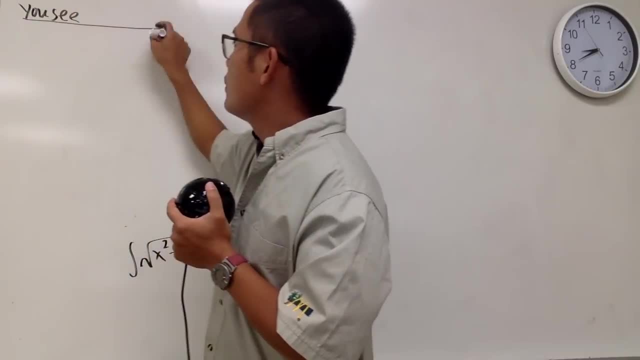 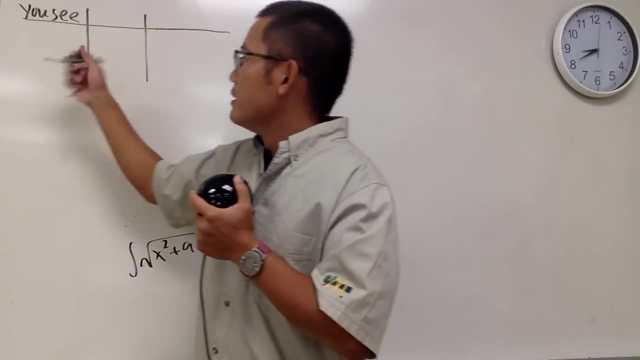 I'll just put it down. When you see the following, go ahead and try this right here. I'll try to keep it small so I can put all the things on the board as well. That was the first one. yeah, It works. 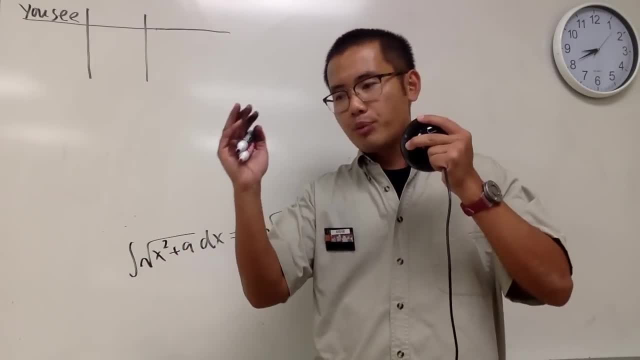 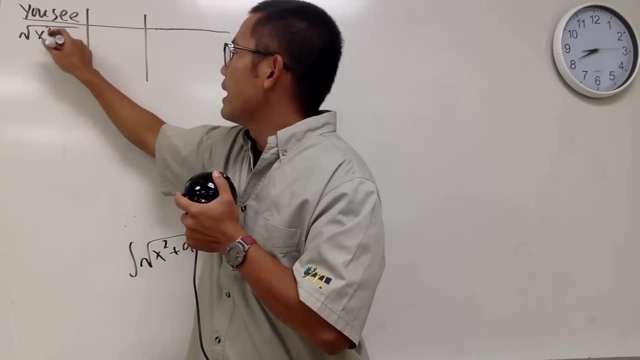 really well when you have square roots, but the truth is, when you have parentheses to some power, it might also work too. But anyway, first situation: square root of x squared plus the number a squared, Because remember earlier we only had the 9. If we look at this, this is x. 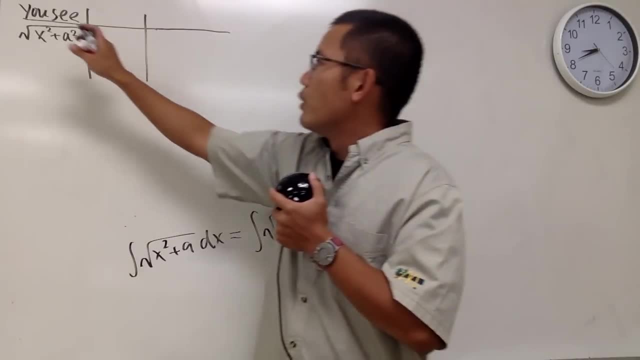 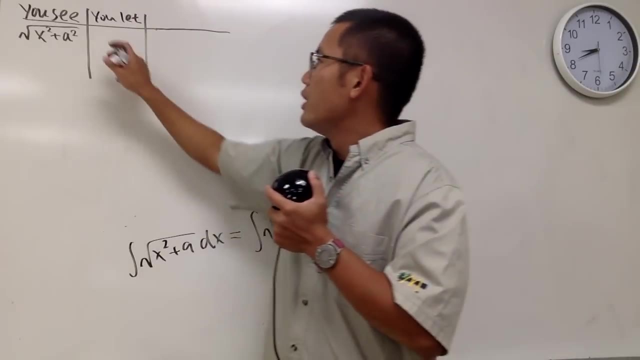 and this is 9.. These are two squared root of a squared. So if we put the square root of a squared equal to three tangent theta, So if you see this, then you are going to let- and when I say let, that means you are going to do the substitution- you are going to let x equal. 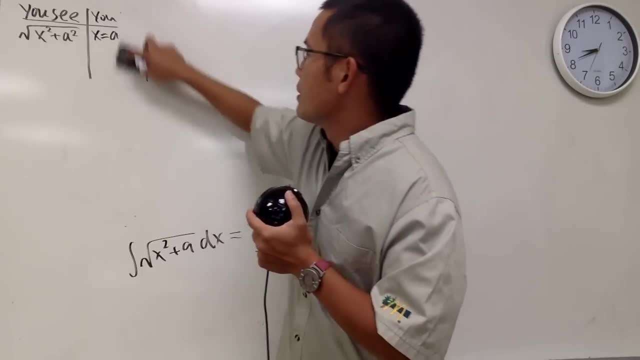 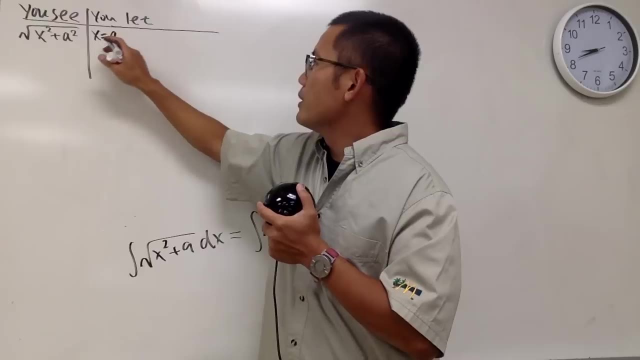 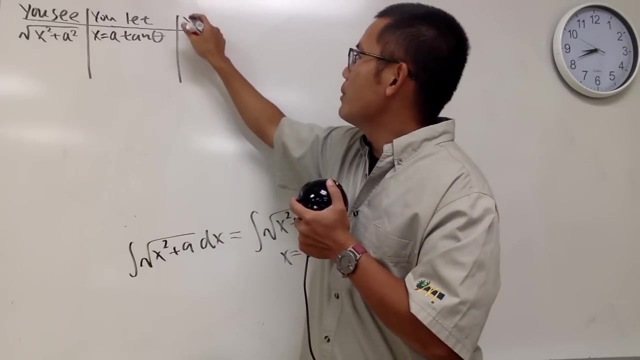 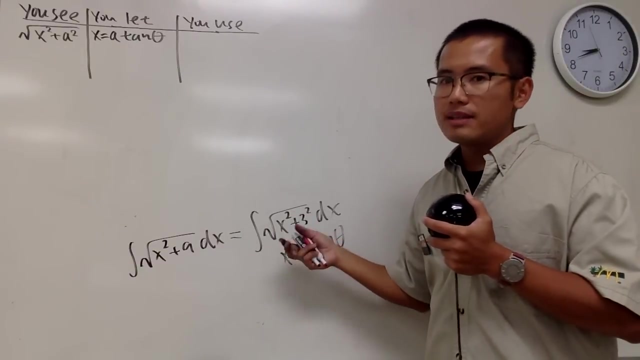 to a. I'll draw it bigger. I'll draw it bigger. okay, I'll draw it bigger. you are going to let x equal to a tangent theta like this right, And you are most likely going to be using the identity right here. You will be having tangent squared plus one after you. 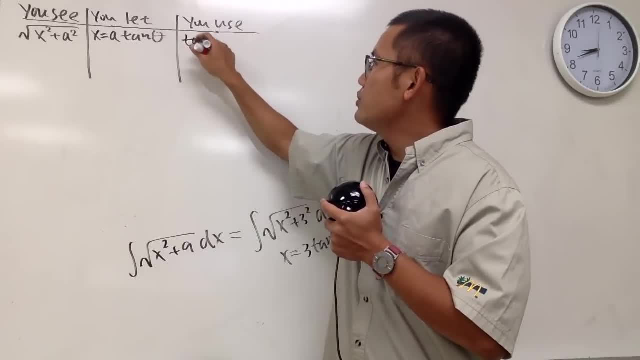 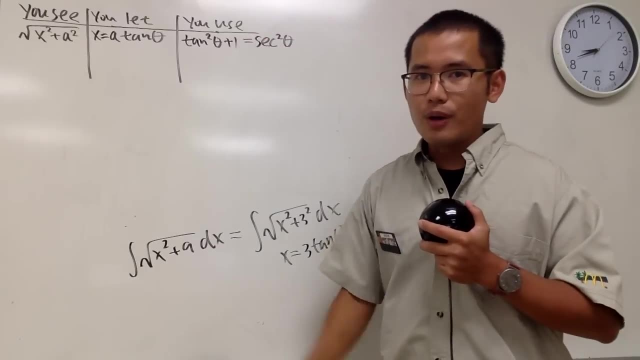 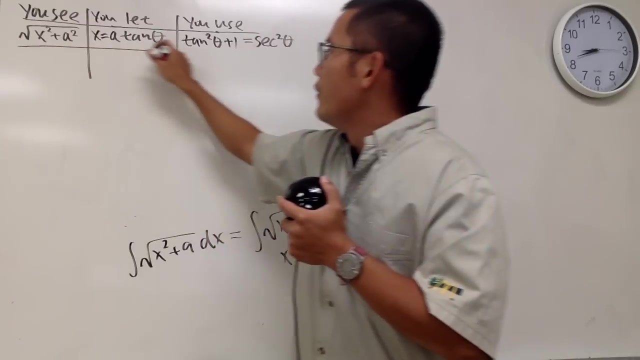 factor all that. so you will be looking at: tangent squared theta plus one equals secant squared theta, like this. So, what you see, what you let, what you use, Well, we have other choices as well, because, for example, if you have a subtraction in 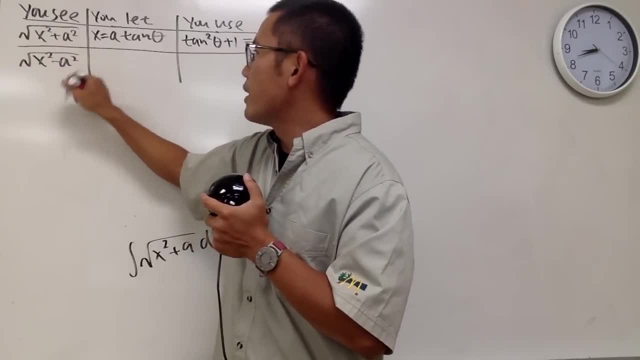 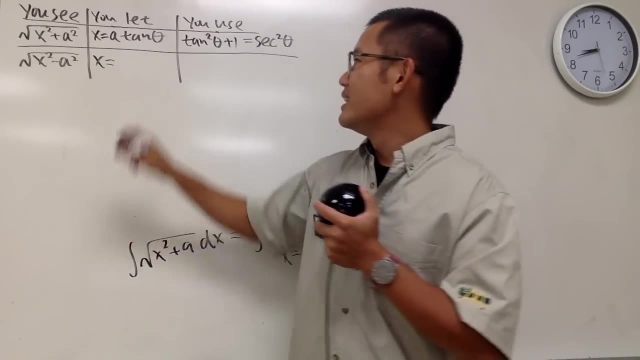 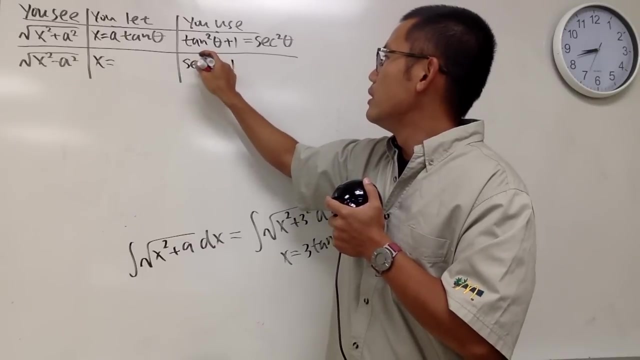 the middle square root of x squared minus a squared. well, in this case, we'll be using what Secant? because we will have. we will have the secant squared theta minus one right Secant squared theta minus one, and this is equal to tangent squared. 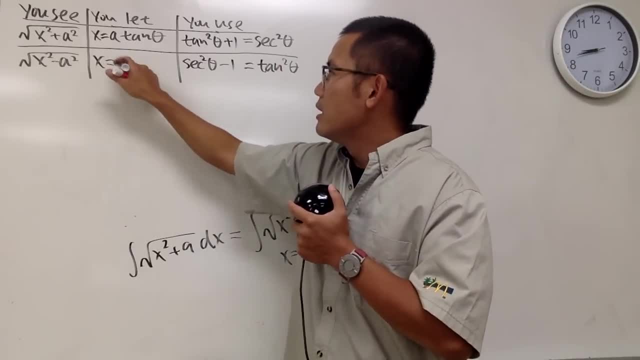 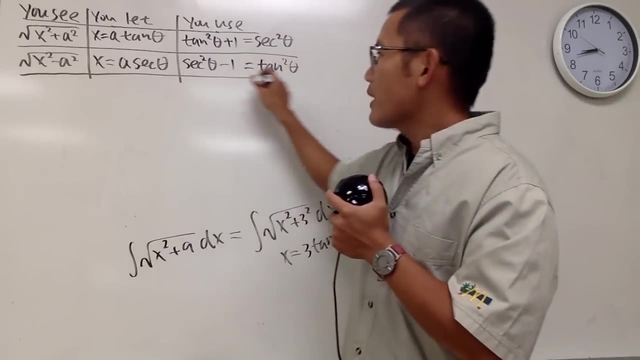 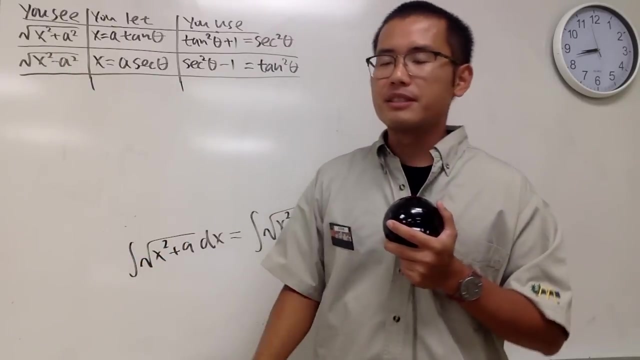 Like this: So x will be a times secant theta. okay. So we have these two situations and in fact we have one more, because what if we switch the order of subtraction? Of course that matters, If we switch the order of addition, it doesn't matter. but here, if we have the 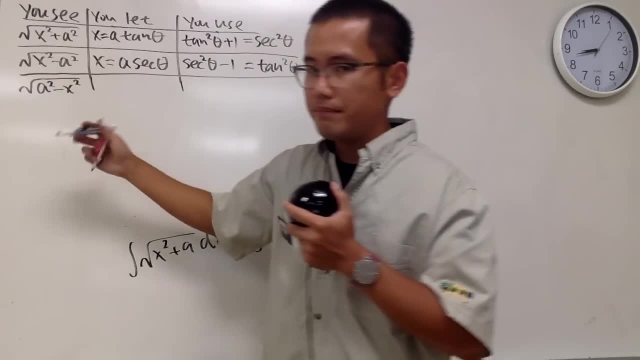 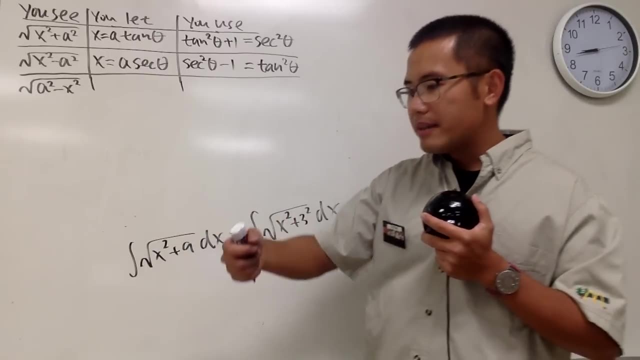 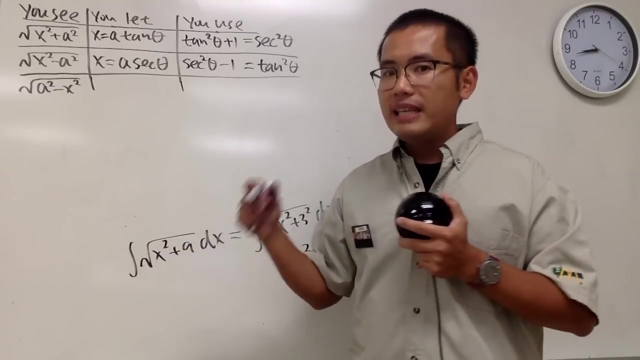 square root of a squared minus x squared. okay, it matters. now x should be what Then? well, one number minus a trig function squared would be another trig function. squared, Sine will cosine right In this case. in fact, we are going to be using, we are going to be 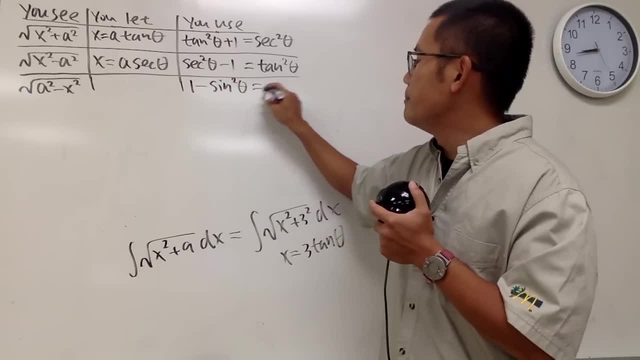 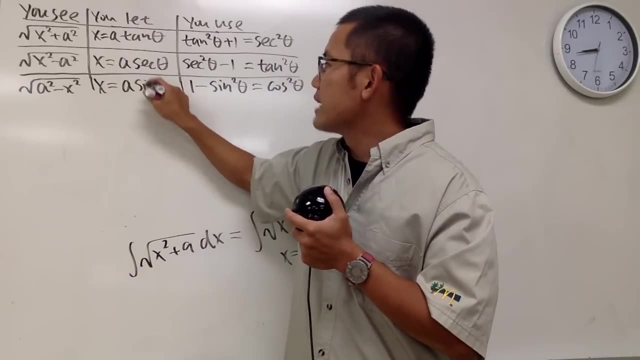 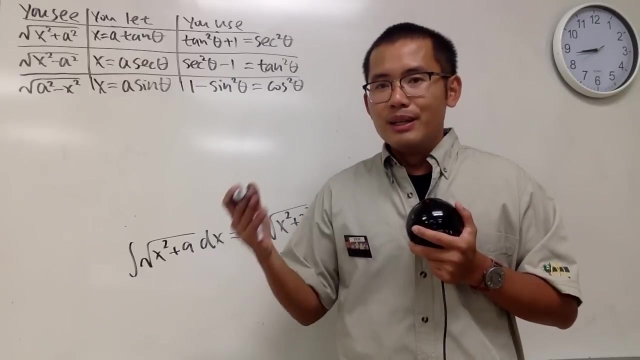 looking at one minus sine squared theta being equal to cosine squared theta, and we will take x equals to a sine theta, And if you wonder why we don't use cosine, it's just simply that roughly cosine is negative sign and nobody likes negative, So this right here works just fine. 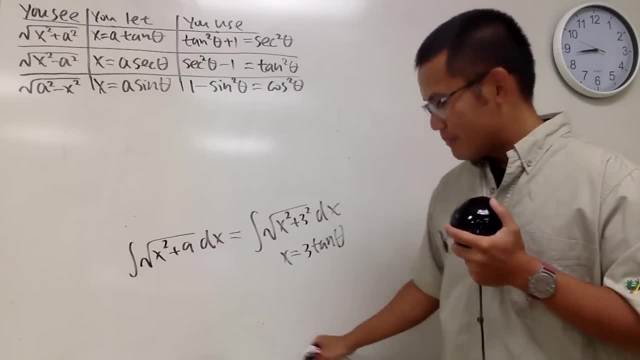 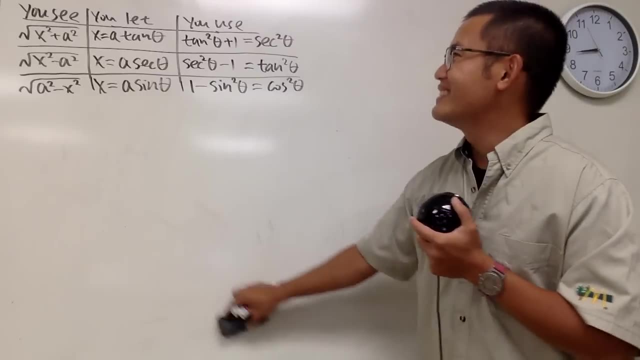 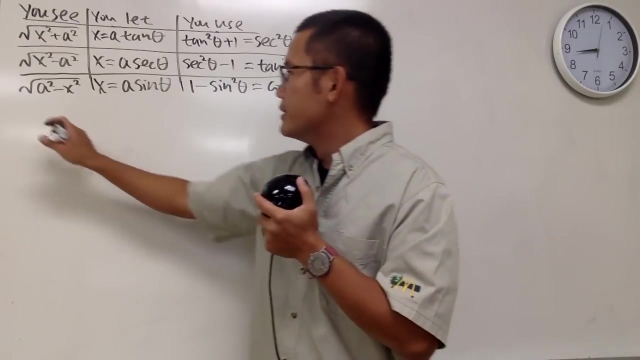 If you want to use the cosine substitution, go ahead. up to you, Yeah so, and just be careful with the negative sign, but we should stay positive. So this is the chart that will give you a pretty good guideline of the following equations: Okay, so 38, integral one over x. 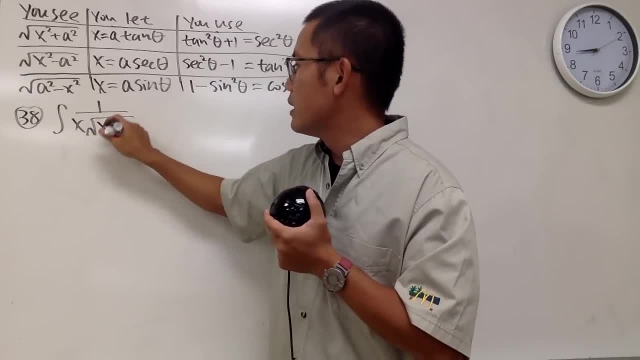 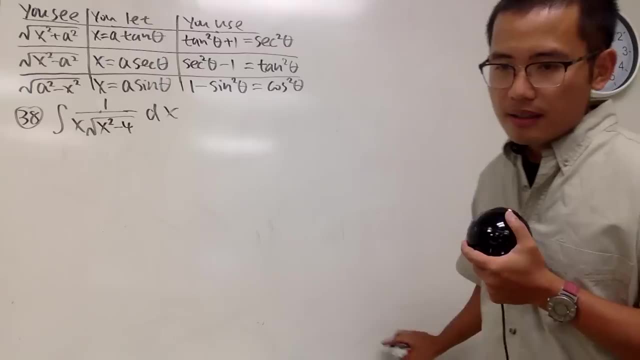 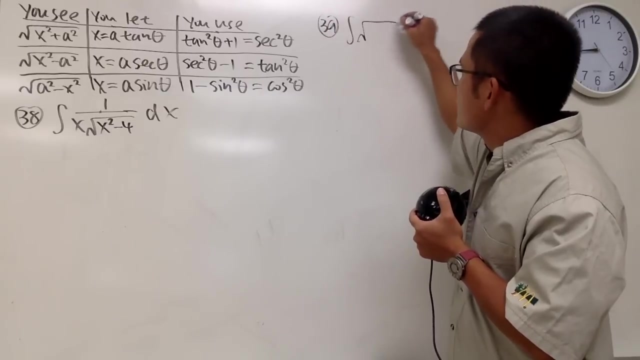 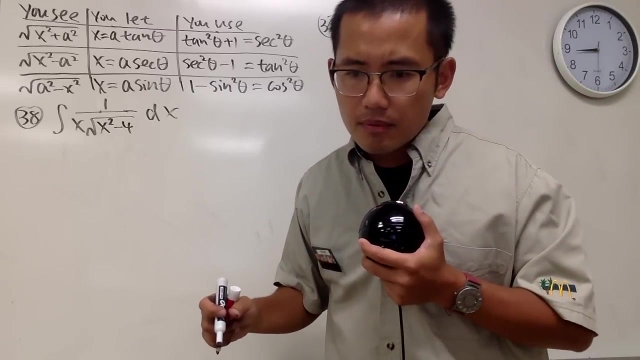 square root of x squared Minus 4 dx. Right, So the number 38.. And let's see I should have enough space to do number 39.. Integral of square root of 1 minus x squared dx. Yeah And okay, so just these. 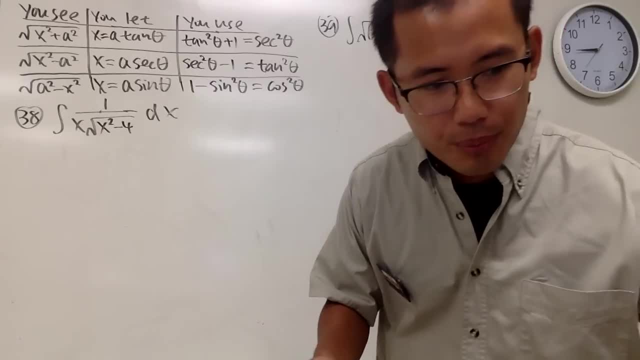 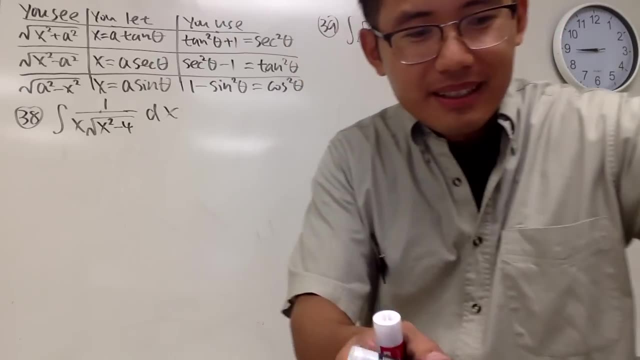 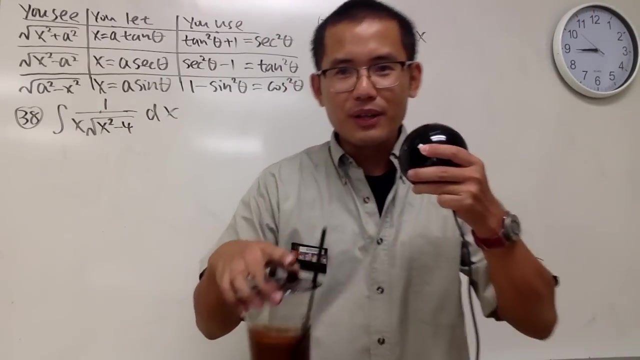 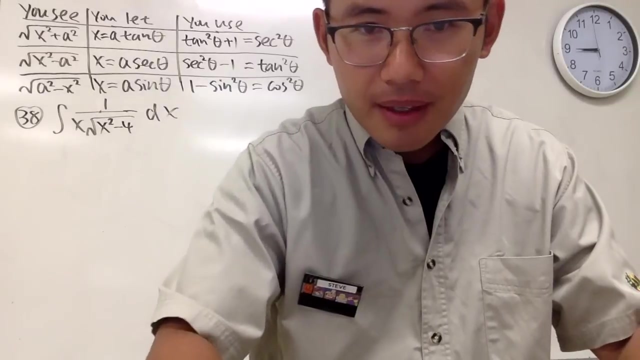 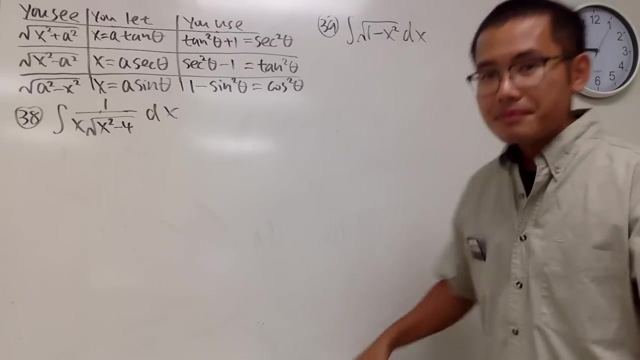 two questions on the board now And I'm going to take a restroom break. I don't. this is, yeah, Give me a light, because I have to hold this mic, but I don't know for how long. but Let's see, Four hours It's not so bad. I don't know if I can finish this in five, but who knows? Anyway, get to work on these two questions. I'll be back. 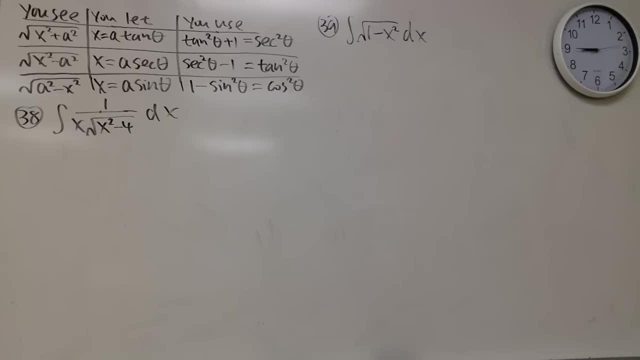 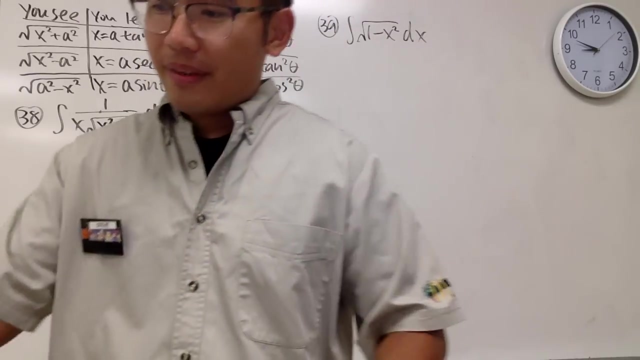 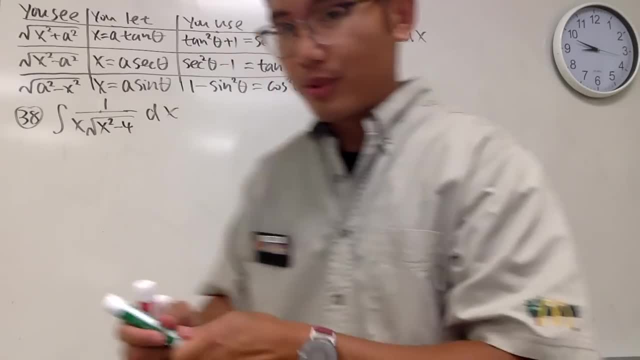 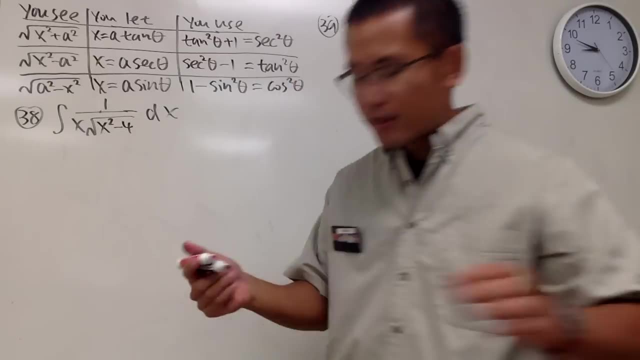 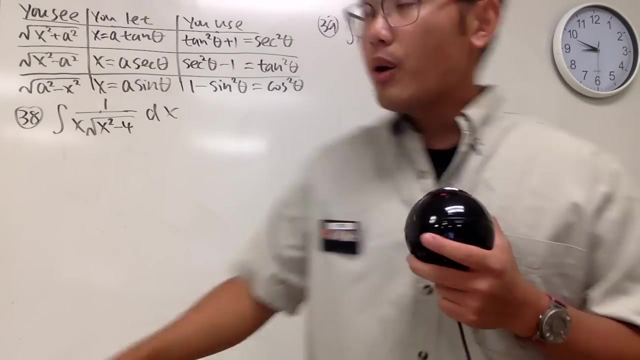 So I will. I have the green one too, so I just want to change it, Just want to have fresh markers for the video And then the other one. I'll just do it later, Okay, So let's take a look right here. 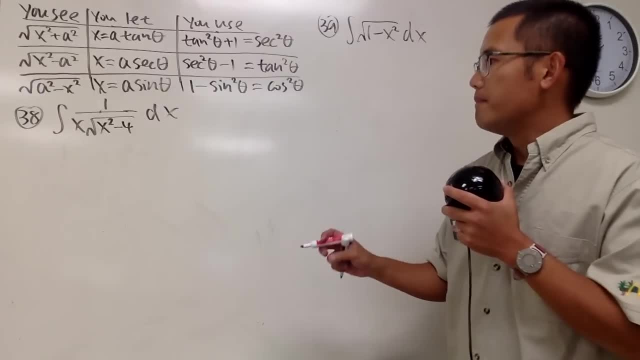 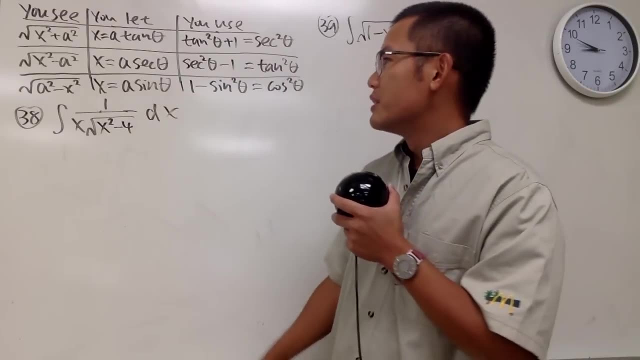 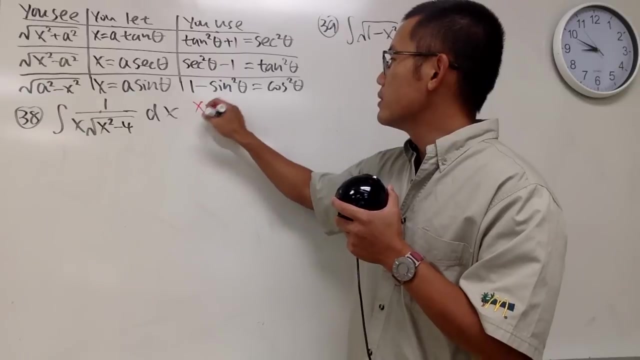 All right, good. So for this one, notice how we have the x squared minus 4, and 4 is like the same as 2 squared. So we are talking about this situation. Very good, Yes, we'll just take x equals 2.. 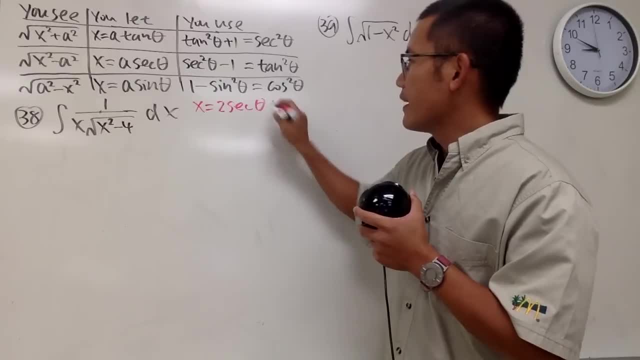 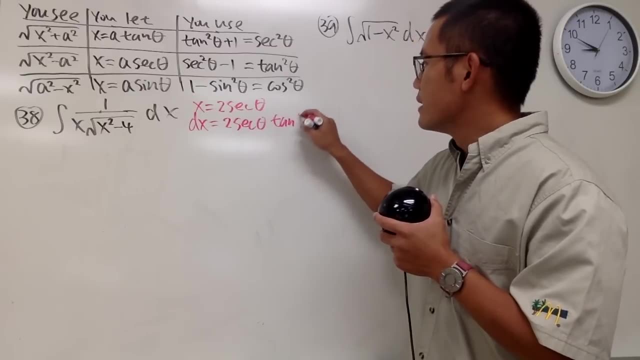 a is 2, so we have 2 secant theta like this And go ahead and differentiate it. So dx is equal to 2 secant theta times tangent theta d theta. So that's it. That's very nice. Now here is the video. 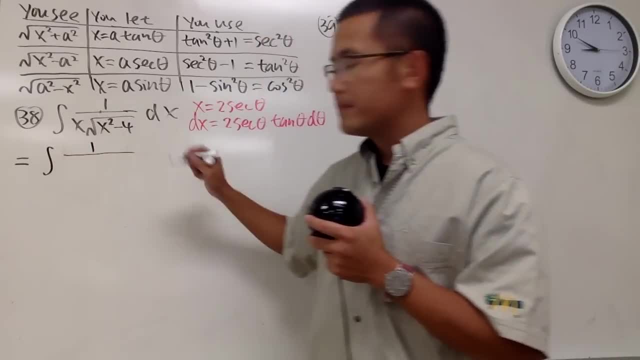 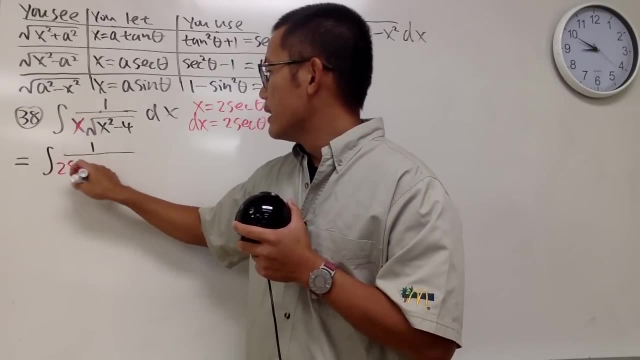 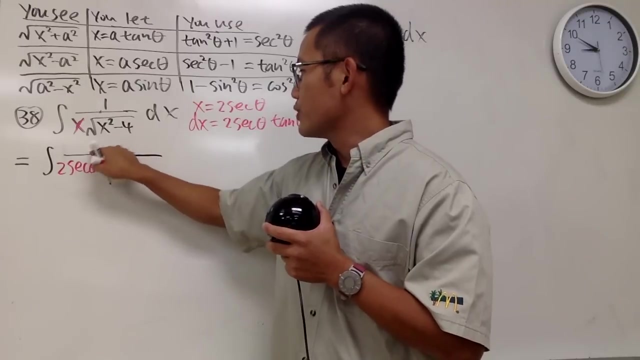 We have the integral and this is 1 over. well, for this part, this is an x, So we will just have 2 secant theta right here, of course. Then notice how we have the square root and I know the 1 should be right in the middle. 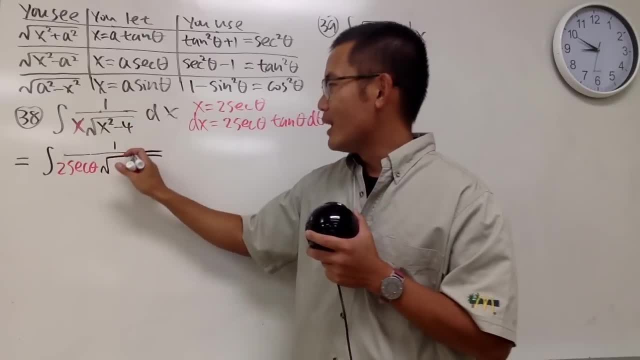 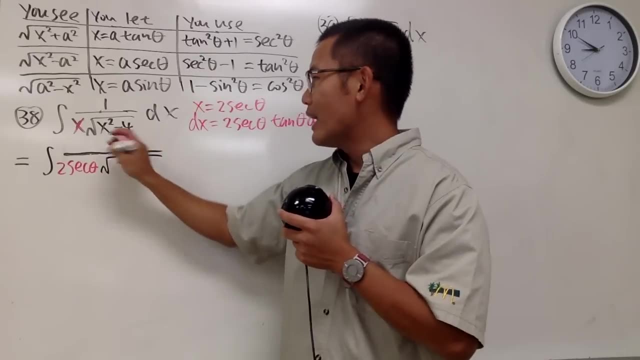 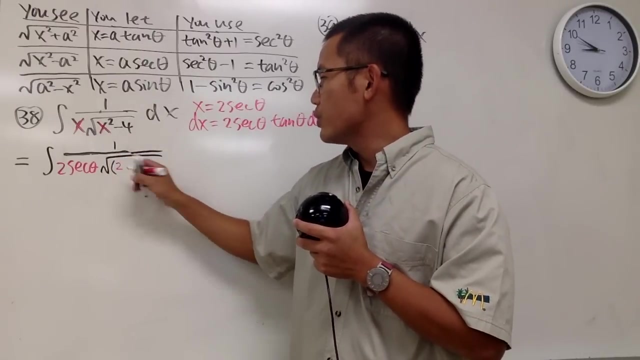 like this: We have the square better, We have the square root and inside here we have the x squared. So what we have to do is we will have to put down parentheses and then the 2 secant, theta and square dot guy. 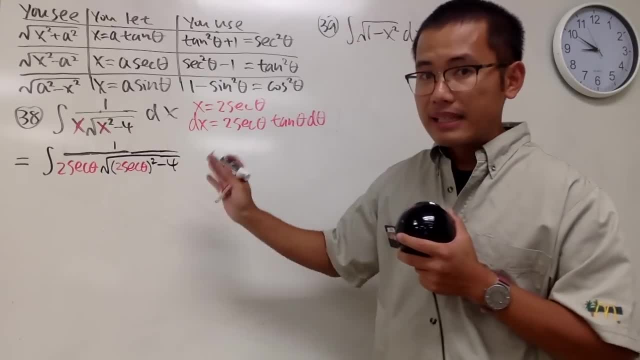 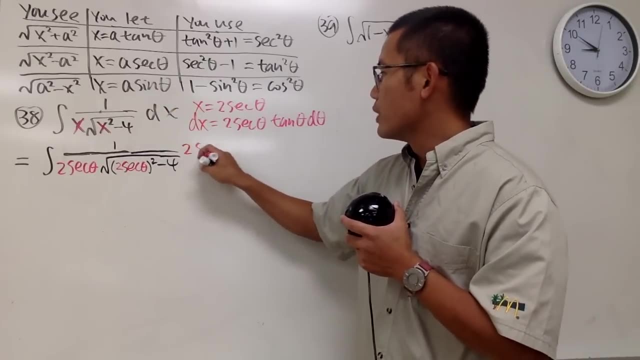 and then minus 4, right, But this is not it yet, because the dx is all this. You also have to put that down. So let's put down 2 secant theta times, tangent theta d theta. That's very nice. 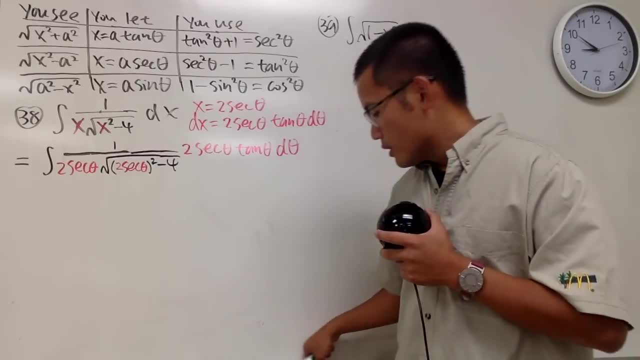 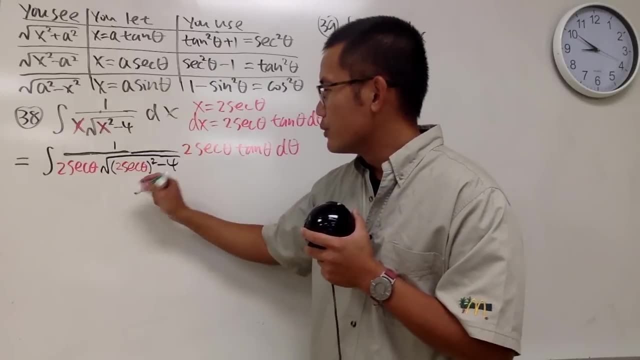 Now let's focus on simplifying this square root. Well, you can also do this in your head, but I will show you guys all the work for this one right, And this is how we do it from scratch. Of course, you can do this as square root. 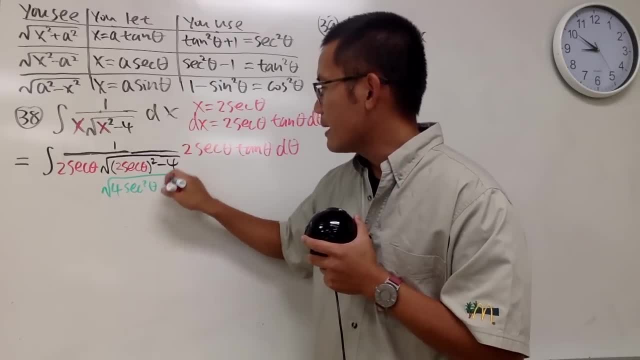 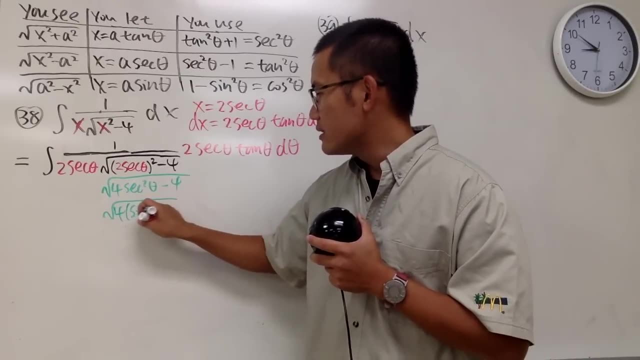 2 squared is just 4, and then we have secant squared theta minus 4.. And then, of course, this is a square root And we can factor out the 4, and then we can say this is secant squared theta minus 1.. 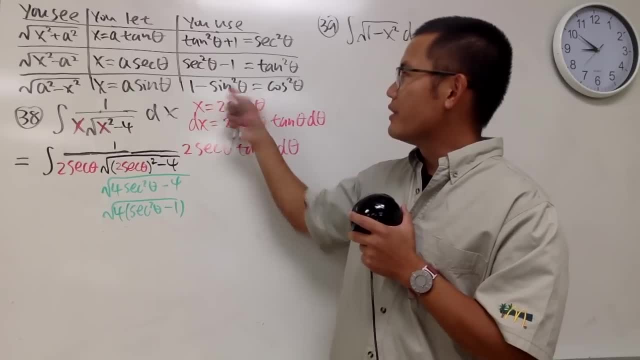 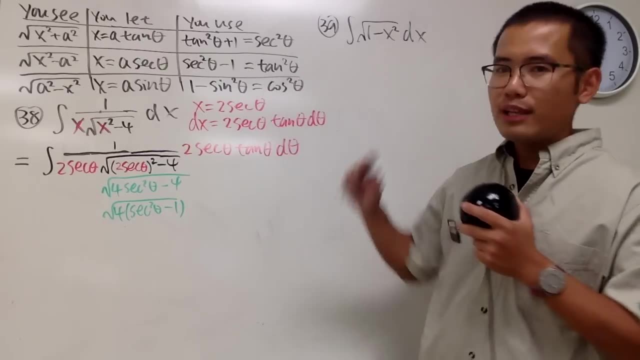 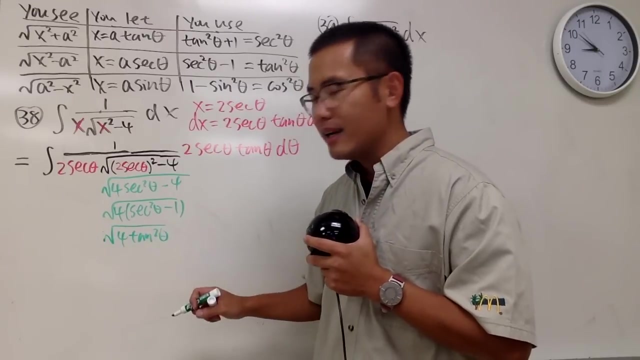 Now you see, If you do the substitution right here, you are going to use this identity. Look at it this way: Secant squared theta minus 1 is just nicely equal to tangent squared theta. So this is square root of 4 tangent squared theta. 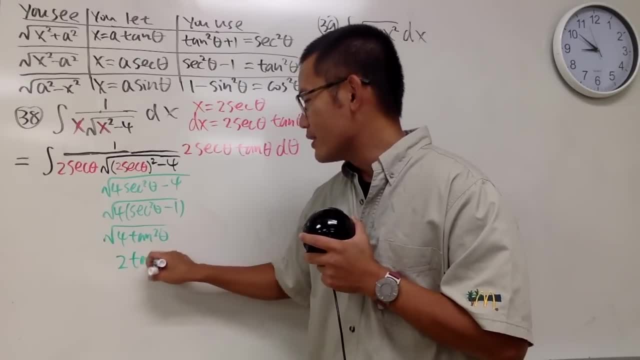 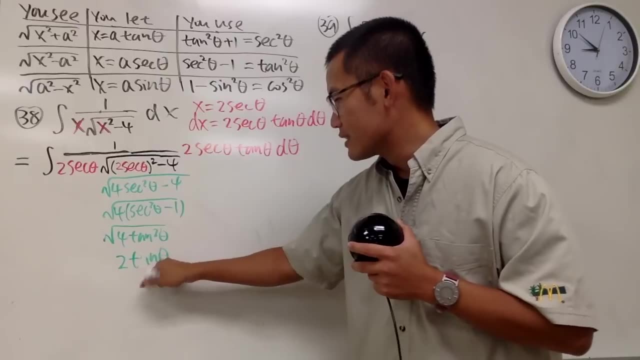 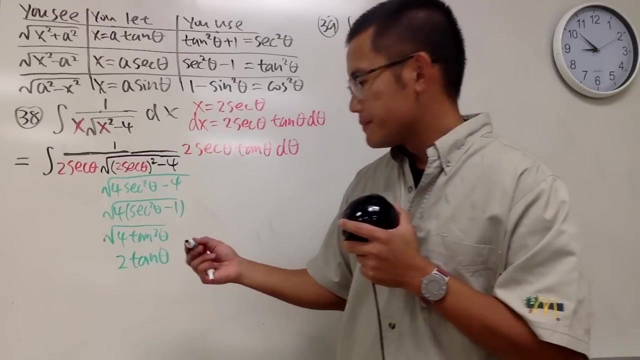 Then you get 2 tangent theta like this. Very nice. So just focus on the square root and just simplify that square root, Yep, Okay. So let's see what we have. In fact, we can cancel a lot of things. 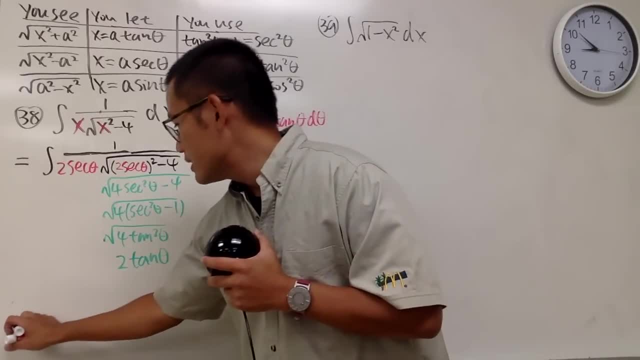 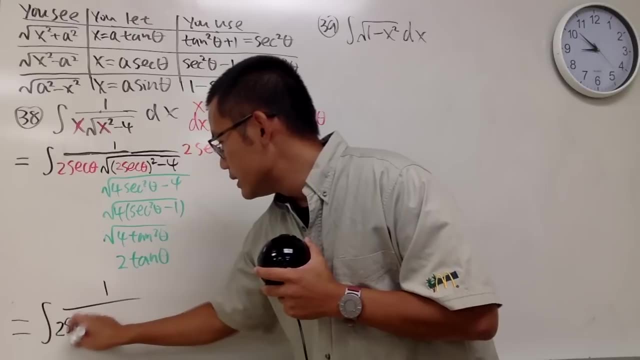 That's really crazy, But let me just put this down nicely for you guys. right? So we have the integral 1 over. Notice how we have the 2 secant theta here. And then this is the green 2 tangent theta. 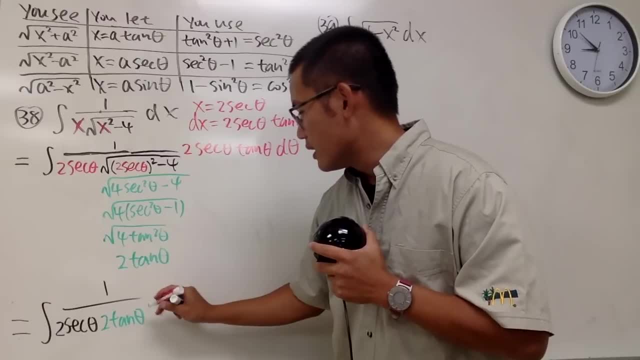 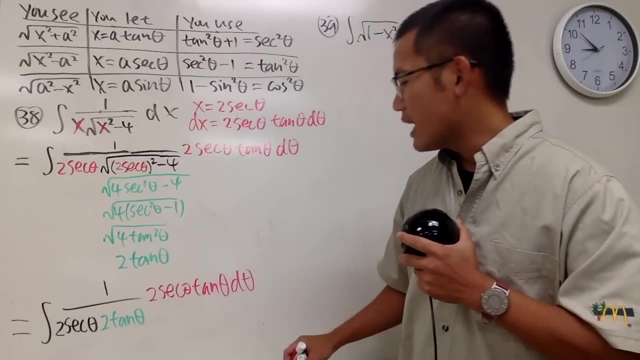 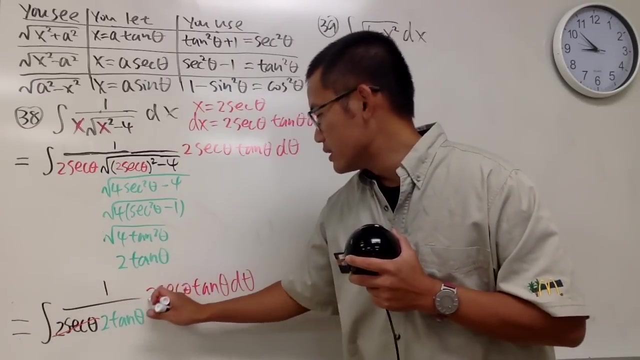 And how we have all this, which is the 2 secant theta, Tangent theta, the theta. And of course we can just cancel things out. See this, This cancel out. Better yet, tangent theta, tangent theta. also cancel out. 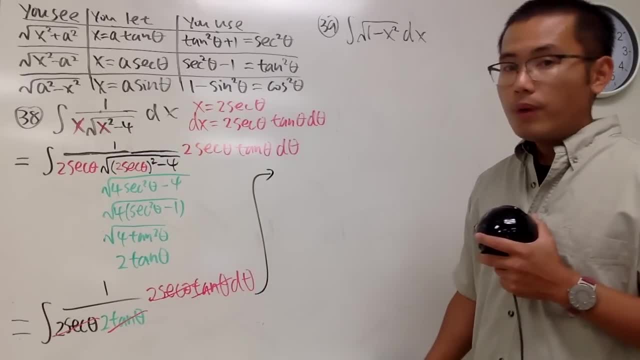 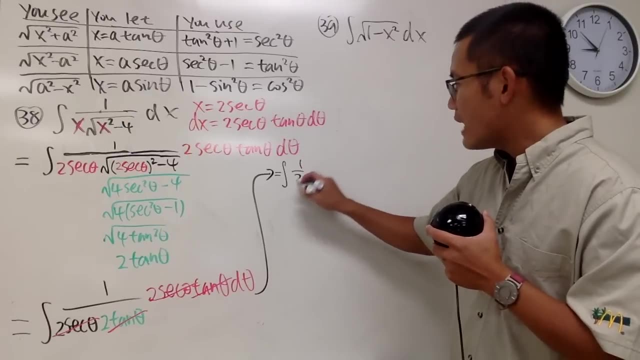 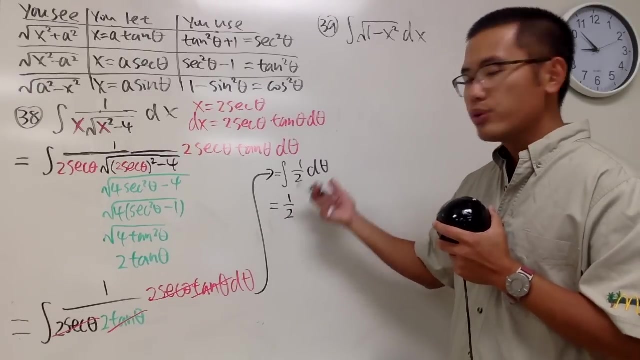 So now let's see: Well, here we just have the integral Notice that we actually have a 1 half. So we have the integral of 1 half And we are in the theta world. right, And integrating 1 half in the theta world is just nicely equal to 1 half theta. 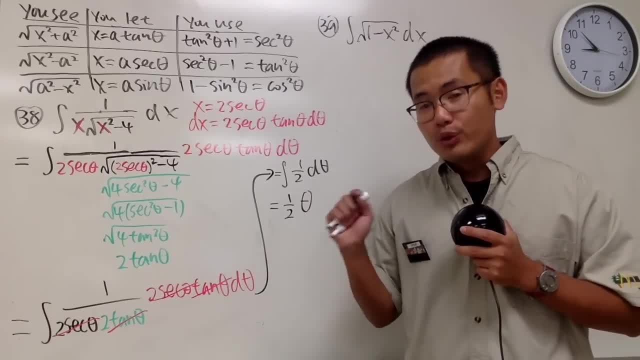 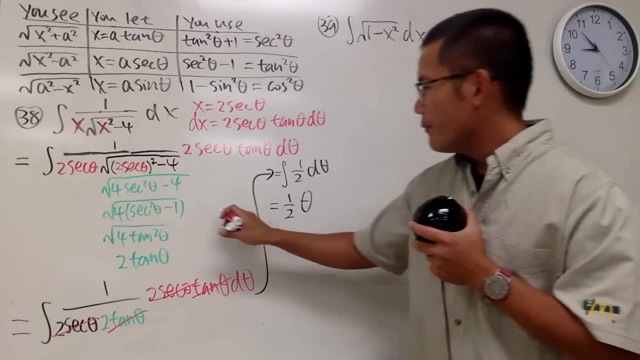 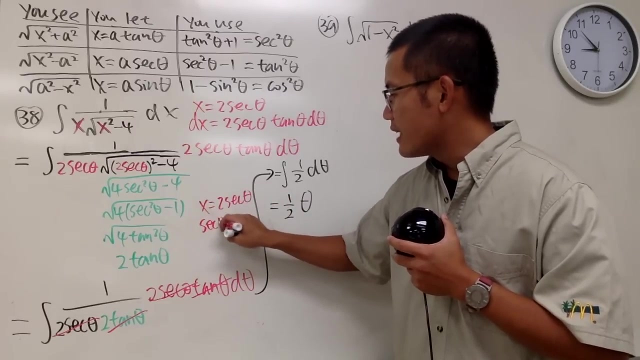 And here is the difference between the one I showed you. We don't have to draw triangles, because we are looking for what theta is Here. look, We know. x equals 2 secant theta. In other words, secant theta is equal to x over 2.. 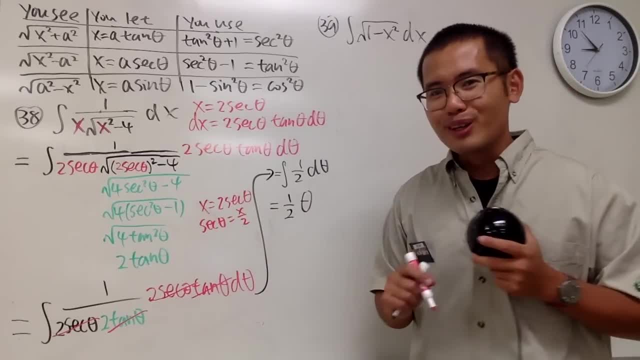 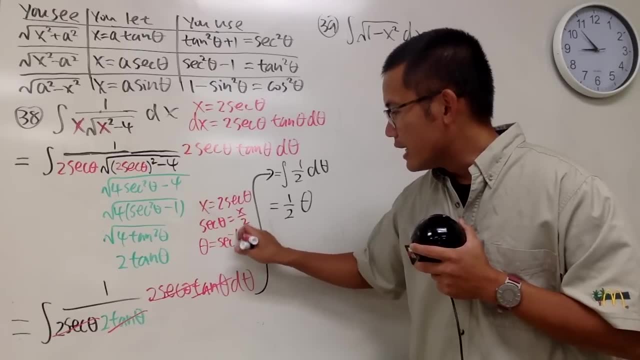 Well, we can take the inverse on both sides, And that's what I talked about in the beginning of the video. right, Right here. we can take the inverse on both sides, So we get theta equals inverse secant. You write it down like this way: 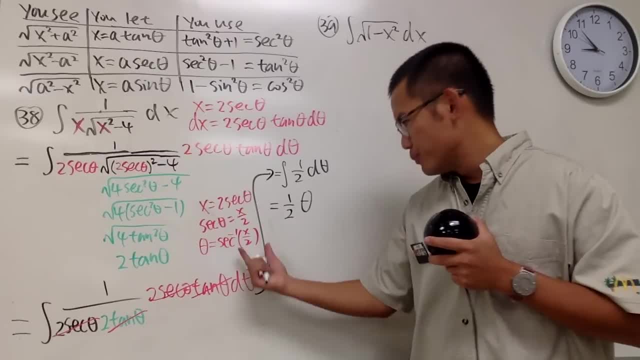 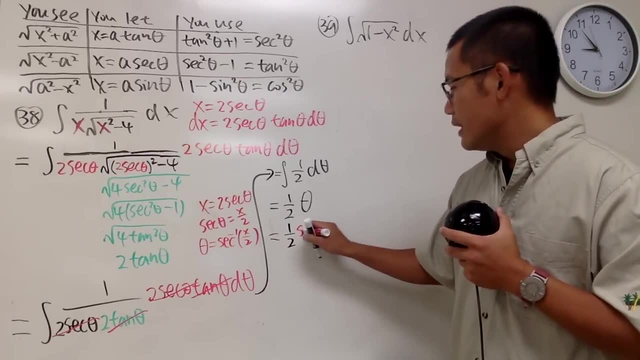 And then the input is x over 2. Put this right here for the theta. That's it right. And we have 1 half inverse secant of x over 2. And that's it So. put down plus c. 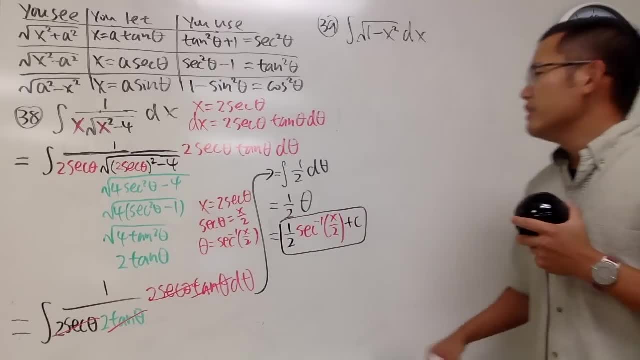 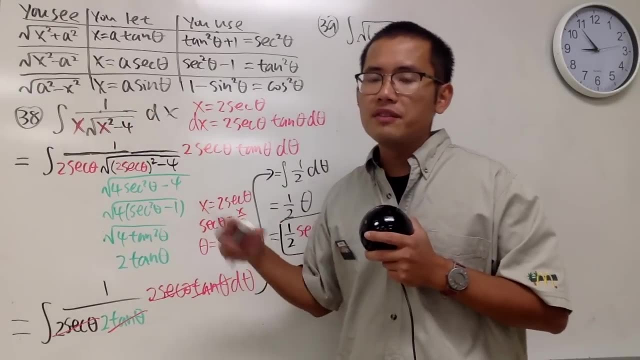 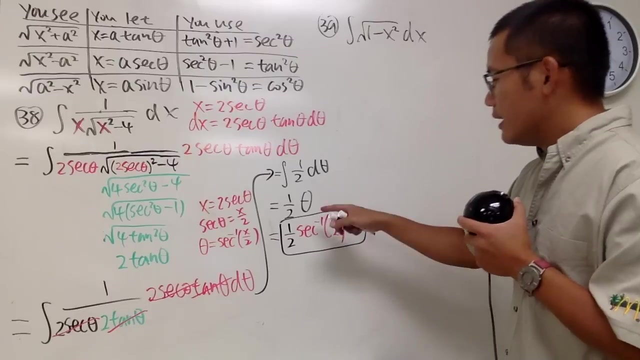 This right. here is the answer right, And you might be wondering: isn't there a derivative of this? Yeah, if you remember this right here by knowing the derivatives, that's actually okay too. 1 over x squared, root of x squared minus a squared is 1 over a inverse secant of x over a. 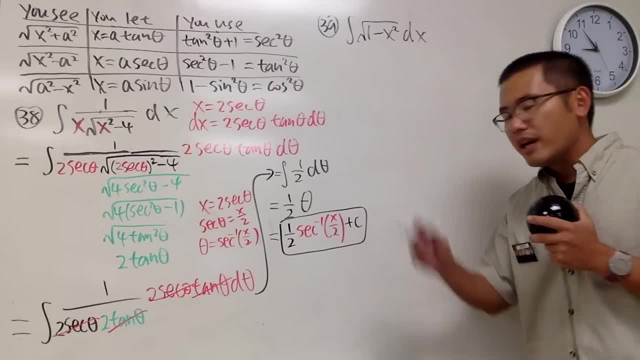 But this is how you prove it. I think it would be easier for me to show you guys this. Anyway, that's 38.. We have a couple more to go, That's all, And let's see if we can go home by 10 o'clock. 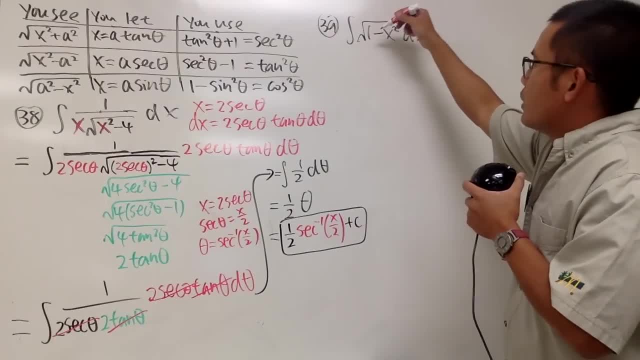 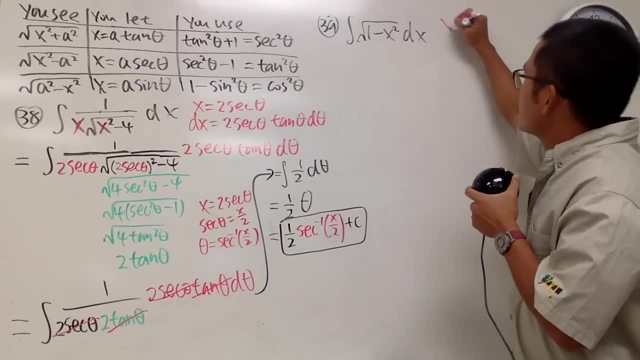 No promise, though. We'll see Integral of square root of 1 minus x squared. This right here is the sine situation, And a is just 1.. So that's pretty nice. So I will take x equals to sine theta. 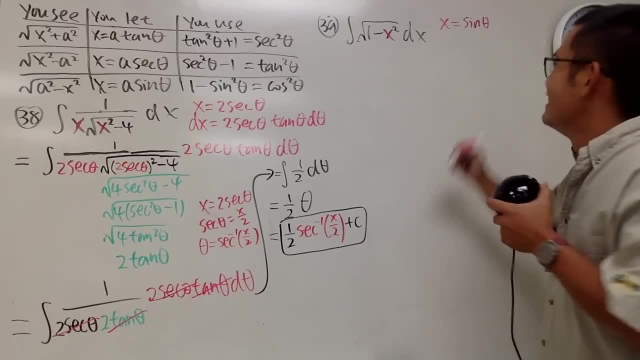 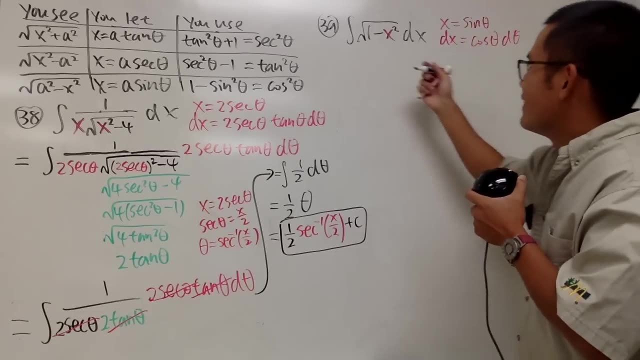 And if you want to leave dangerously, you can say: x is equal to cosine theta, And I'll leave that to you. Anyway, dx is equal to positive cosine theta, d, theta. How good is this? Now, this is the integral of square root. 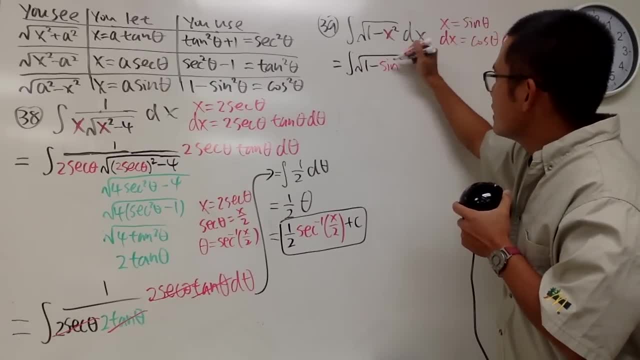 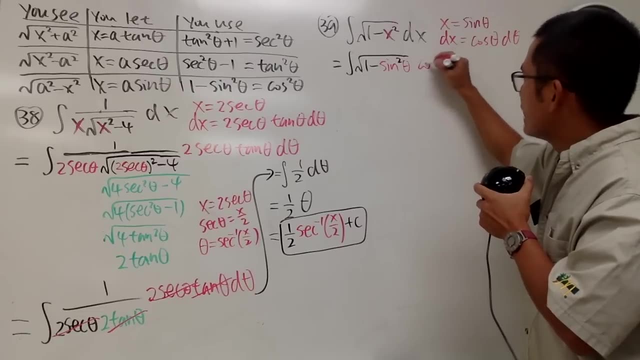 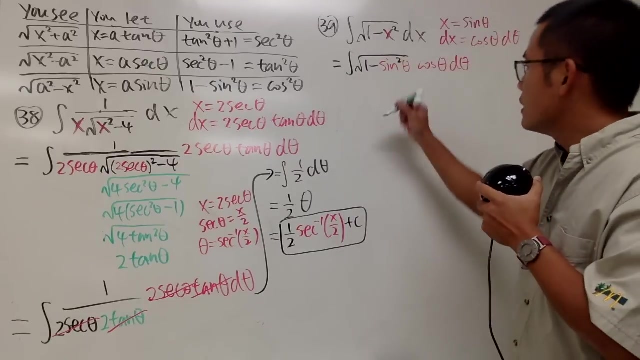 Here we have 1 minus. Here we have sine squared theta. And don't forget that dx is this, Which is cosine theta d theta. Then we see that here is the deal. This part is just the square root. Inside is cosine squared theta. 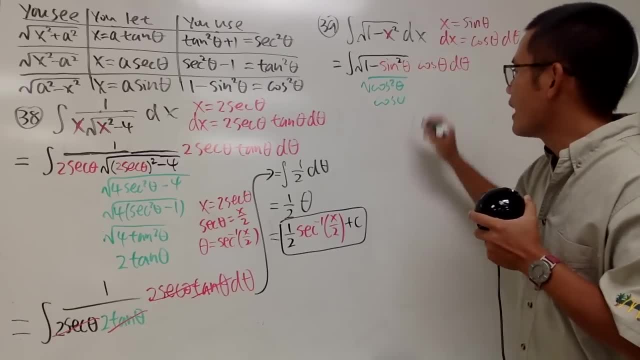 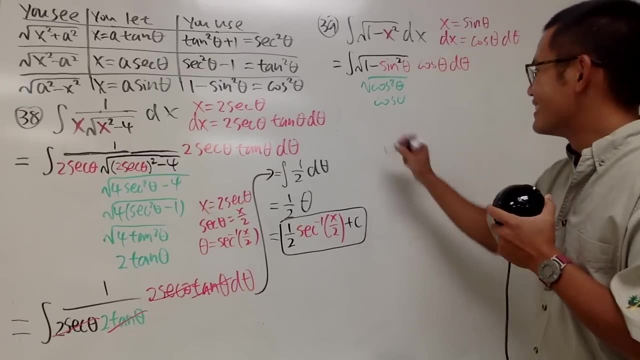 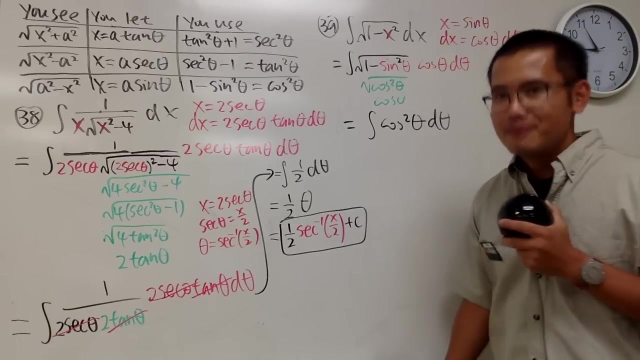 The square root and the square they cancel, So it's just cosine theta. Now you have cosine theta Times cosine theta, So both of them together gives you integral of cosine squared theta d theta. Yeah, this is why I didn't show you guys a lot of examples earlier for the trick identities. 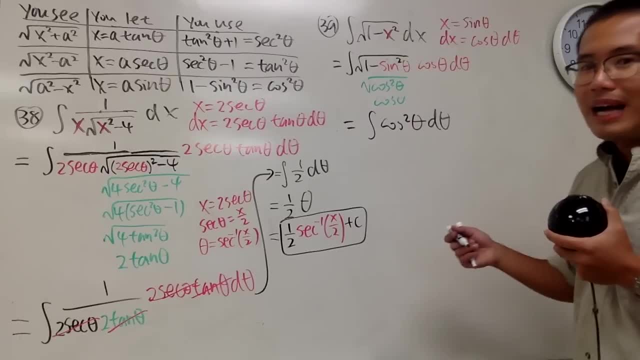 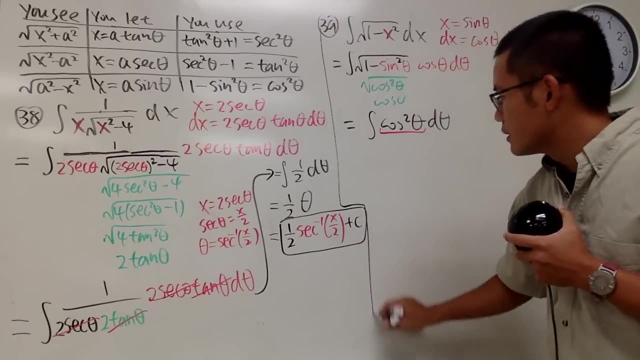 Because we'll be doing that right here anyway. Yes, for this one we will have to use the power reduction formula for cosine squared theta, And let me just put this down right here for you guys: Here we get 1 half integral. 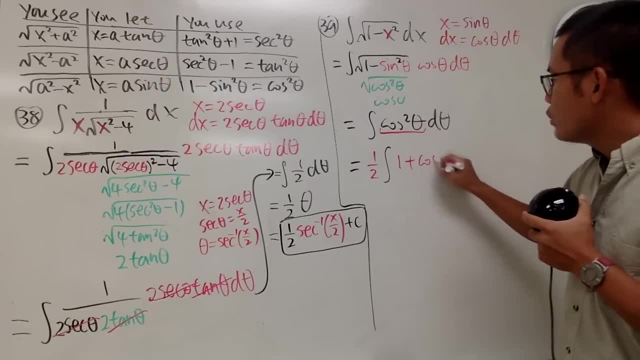 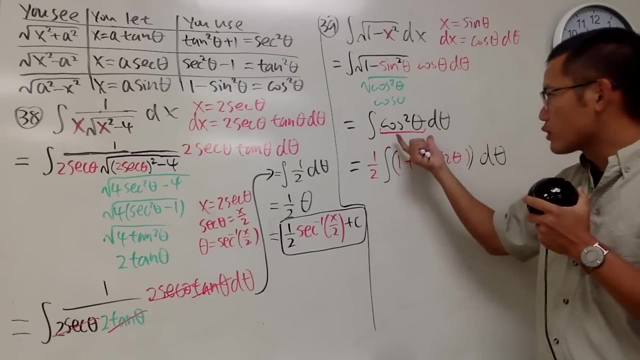 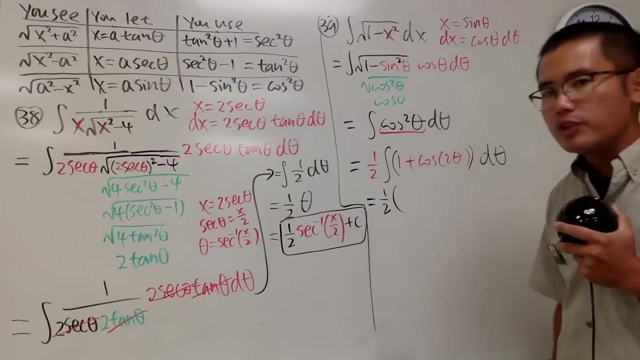 And this is 1 plus cosine of 2 theta, like this Right. So again, the red part is the power reduction formula for cosine squared theta. And now we can actually integrate this. Put the 1 half parentheses for the result of integration. 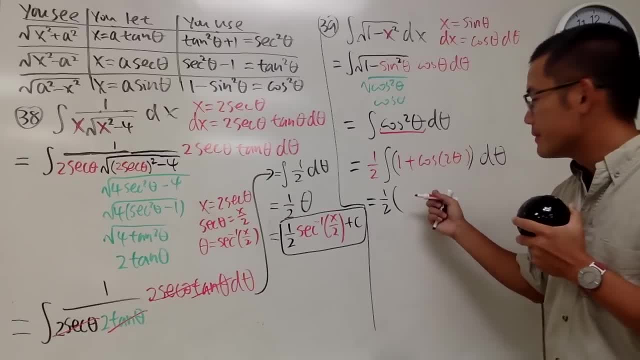 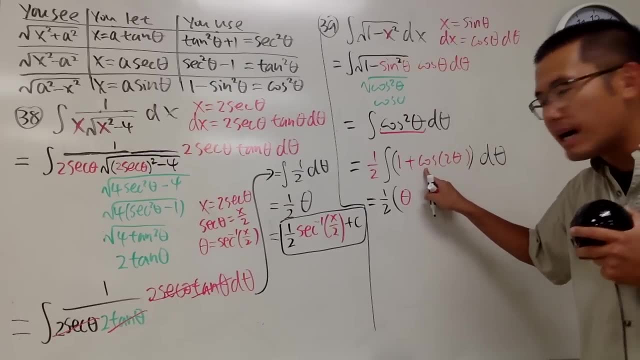 Integrating 1 in the theta world, we get theta Right. So let me just put this down in red. And then integrating cosine, we get positive sine. So we still have the sine right here. So I put down the sine right here. 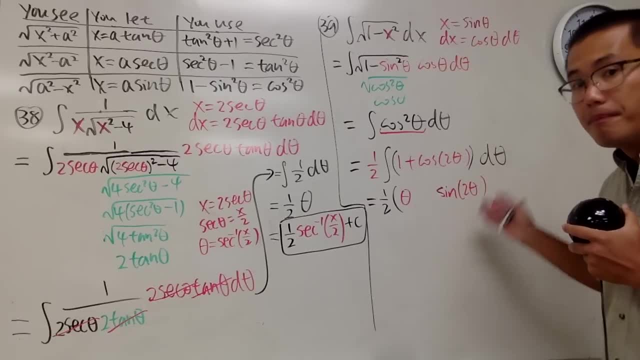 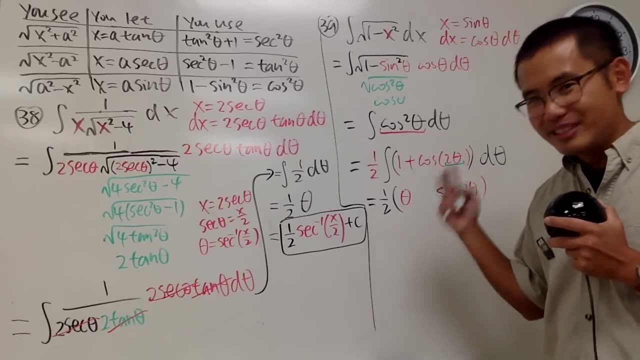 And the input is 2 theta. So it stays the same. But don't forget, we have to divide it by the derivative inside. The derivative of 2 theta is 2.. It's just a number, So we can divide it by that, right here. 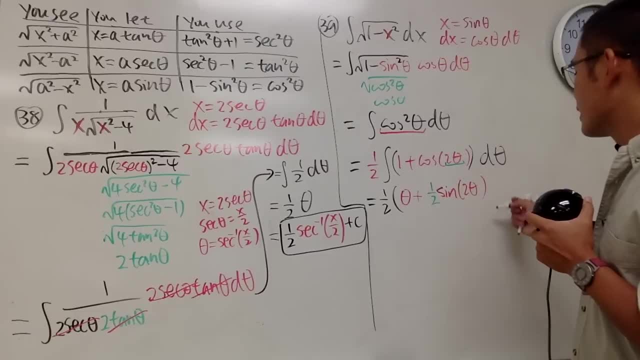 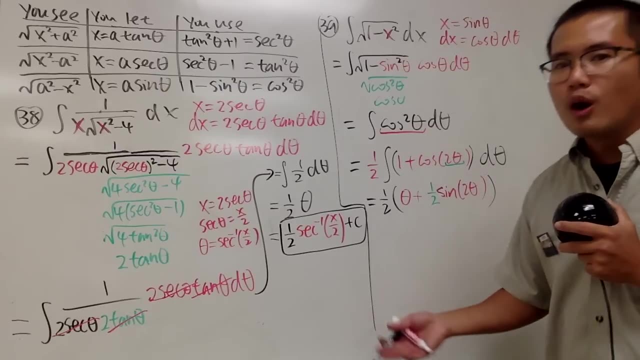 Again, it was positive, So we maintain that positive right here. So that's pretty much the integration, Like this. Now we have to go back to the x-world And this is how we can do it. We can draw the triangle. 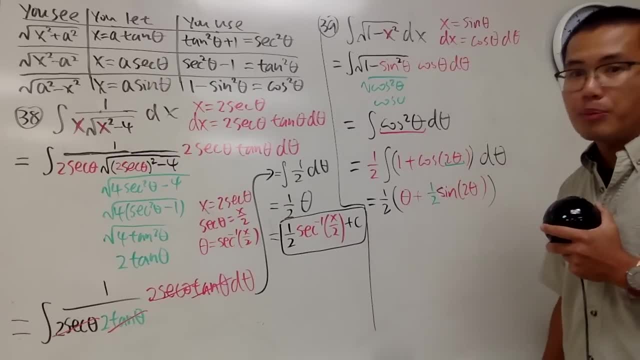 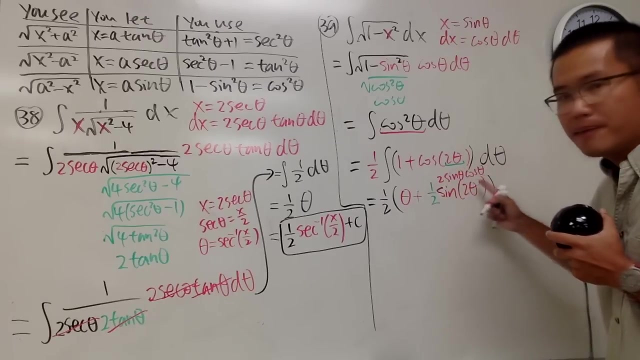 But the problem is that this is 2 theta. Not preferred it Because we only know sine of theta. That's much easier. So this is what we can do Again: identity Sine 2 theta is the same as 2 sine theta times cosine theta. 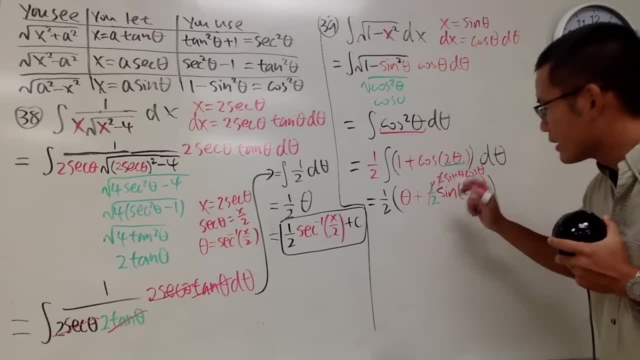 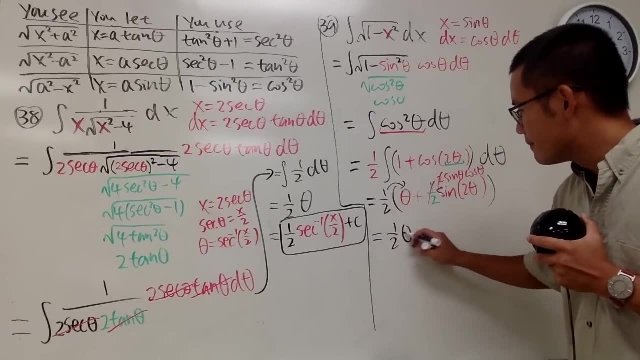 And you see, 1 half and 2 cancel each other out. Okay, Now let me write this down for you guys. Take 1 half multiplied by theta. That's what we have. Take 1 half multiplied by theta. Next we add: 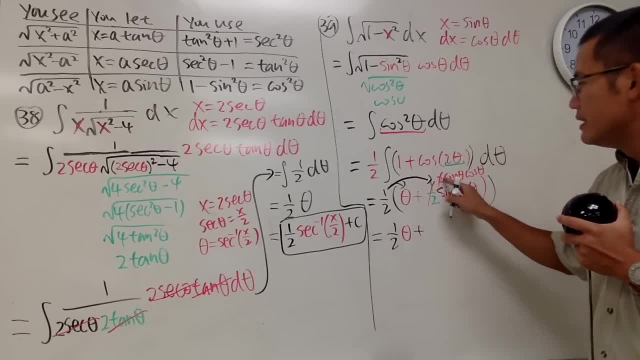 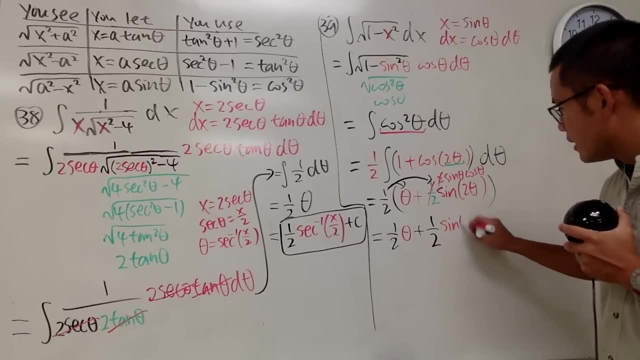 We take 1 half times this, This and that cancel the out, But we have this 1 half, So we have 1 half, And then we have sine theta, cosine theta, And this is just an angle Theta, It's not 2 theta anymore. 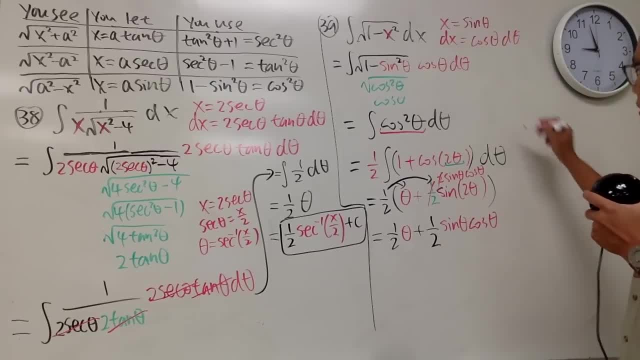 So this is what we have. Okay, We can look at this right here. Put it down right here for you guys. We know sine theta is equal to x, Which is x over 1.. Because of this, right here, From here, we can draw a right triangle real quick. 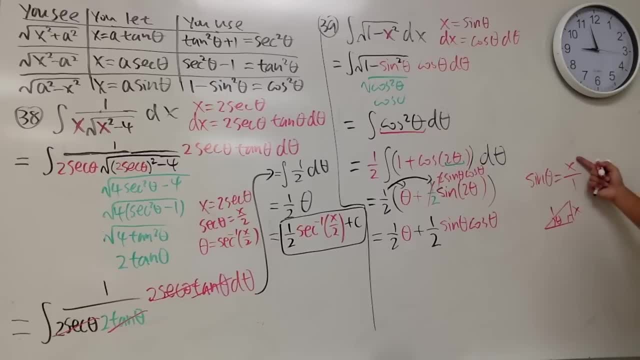 The angle, theta is right here, x is right here And 1 is right here Because it's opposite over hypotenuse Like this: And to figure out the adjacent You just open the square root Hypotenuse square, Which is 1 square. 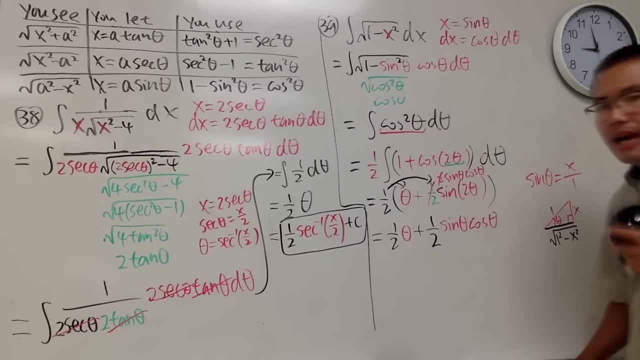 And minus the other side square, Which is x square, Like this. Yeah, And I think some of you guys might be thinking, Hey, Why don't I say theta equals inverse sine of x And just put this guy in here and here and here. 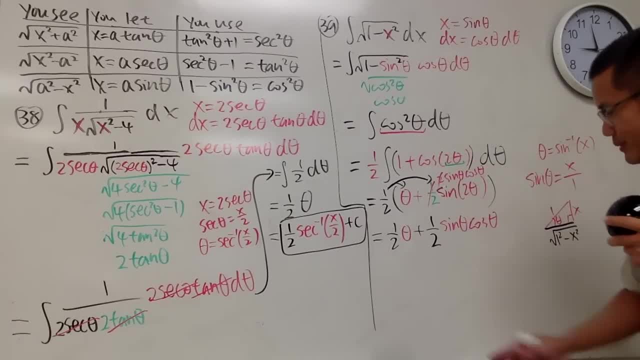 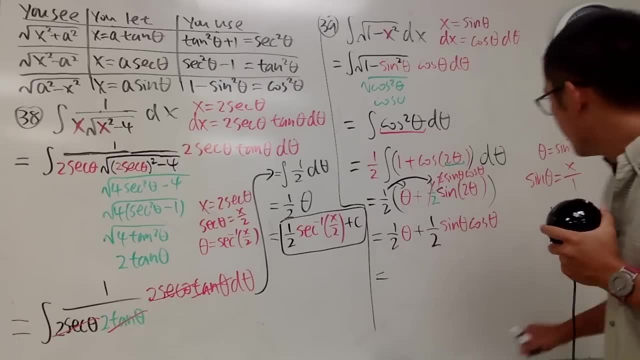 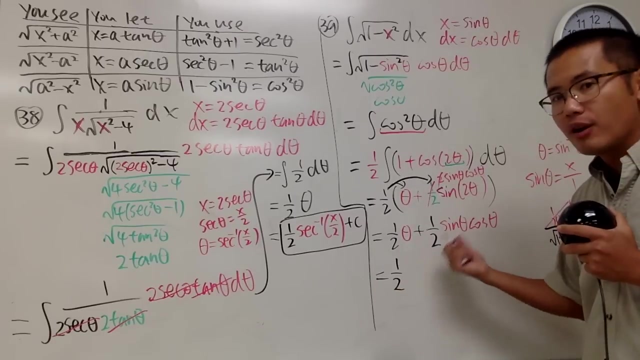 Well, Here is the deal: Draw the triangle, You earn your points on the test. No, Just kidding. Here's the reason why. Okay, Notice how, for this part, We have 1 half theta, Which is just the inverse sine of x. 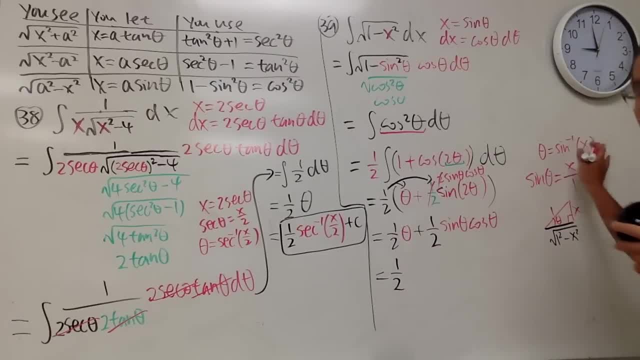 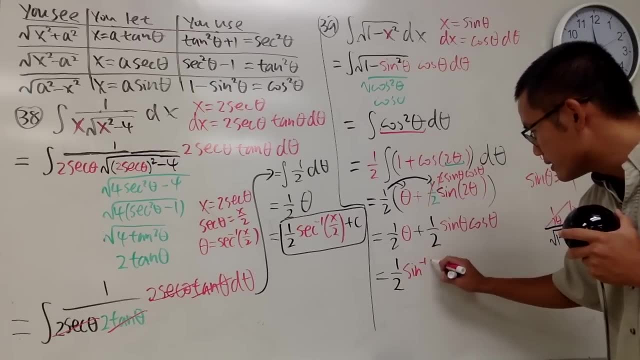 There's no trick function, It's just the angle theta. So it's the inverse right here, And that's what happened right here as well. So here we have the inverse sine of x. That's good, Well, Plus, Here is the problem. 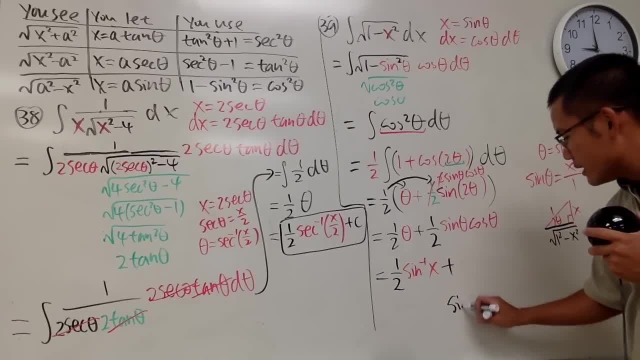 If you put this right here, You end up with the expression Sine of. Well, this is okay. If you put this right here in this expression, You end up with cosine of inverse sine of x. If you just enter this Right here for the theta, 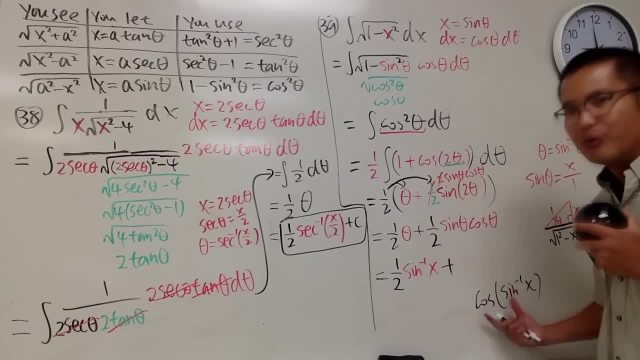 I will have to ask you How intimidating this is. Very much Right. So That's why I said: Please just draw a triangle If you have to figure out the sine and cosine Tangent, etc. Right, Anyway, Here is the 1 half. 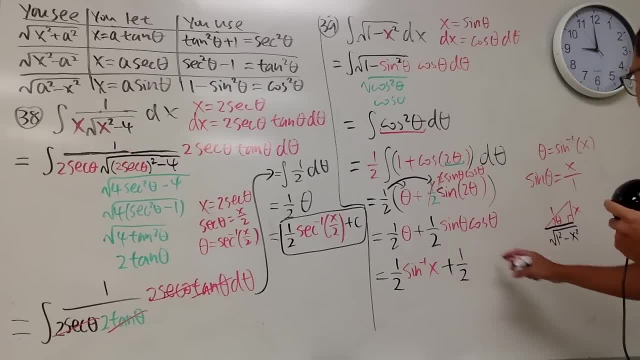 And then we have the Sine theta, Which is X, Why X? X, Yeah, X. And Finally You have the cosine theta, Which is this Over that Adjacent, over hypotenuse, Which is: 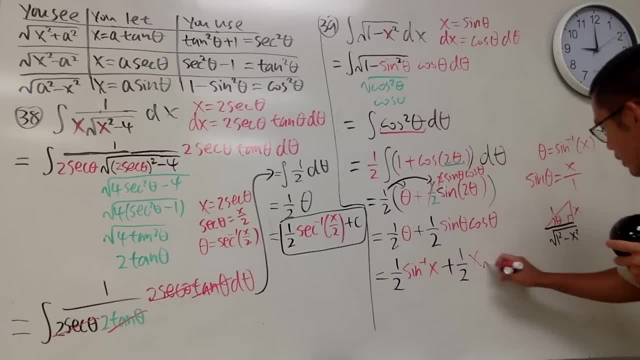 Square root of 1.. Minus x Square Over 1.. Which doesn't really matter, This is it. Yeah, This is it, And in the end We're all done, So We put down the Plus. 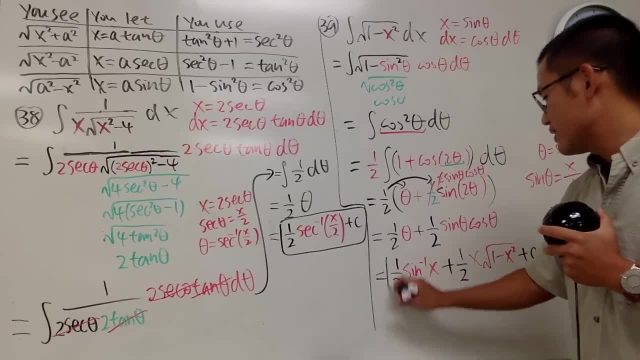 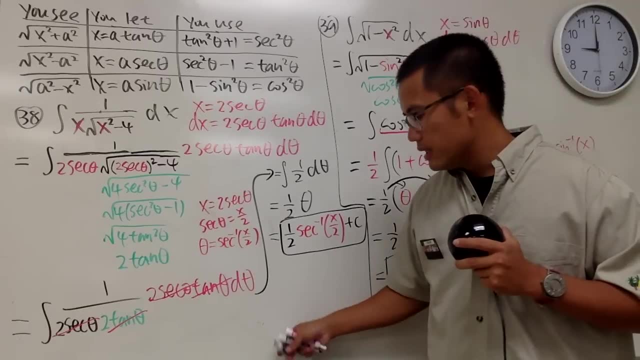 C For the answer. That's it Right. So This is it. The truth is, In fact, You could have done this With Integration By parts. Yeah, I will see If I can finish The whole video. 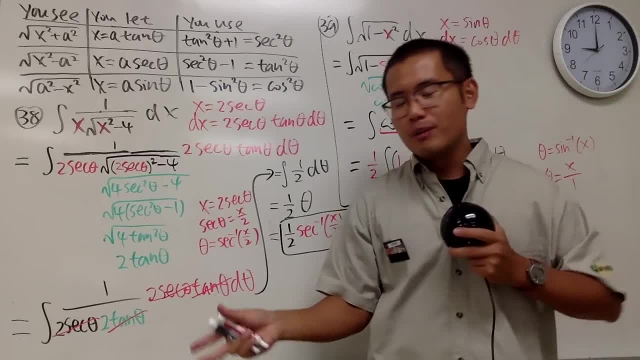 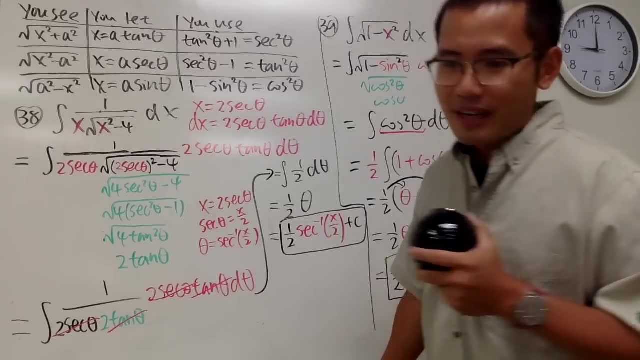 By 10 o'clock. I will do it, But Most likely I won't. I will see Maybe 10.. I don't know, We'll see. By the way, This is It, Number 39.. All right. 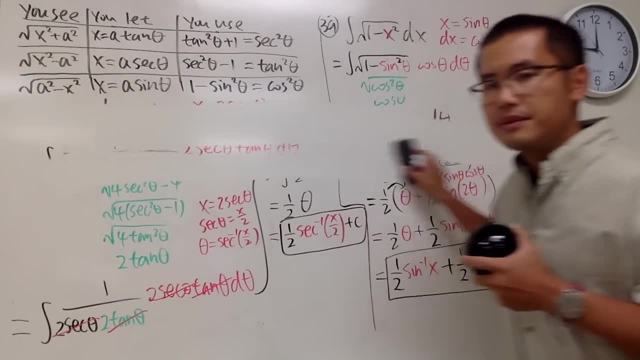 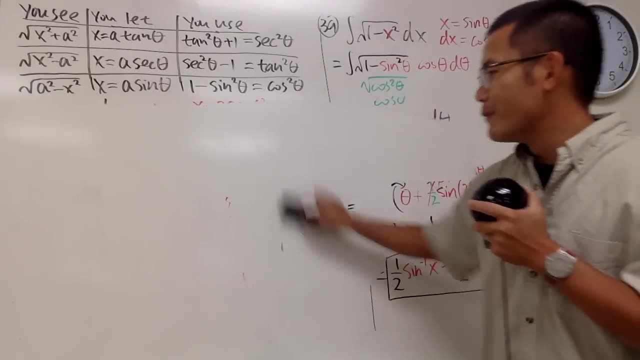 Next two questions Side by side. So Let me know How you guys Are doing, What class Are you guys Taking, Which university, Which college, Which high school Do you guys Go to? And Yeah, 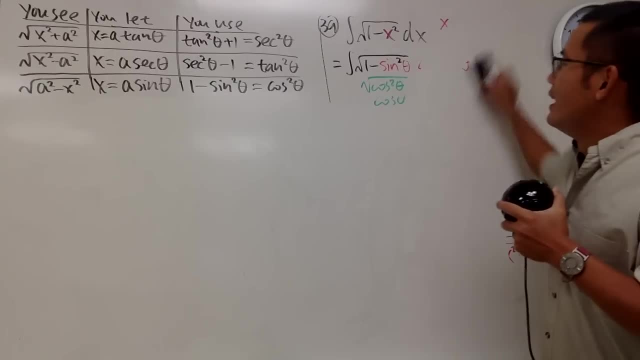 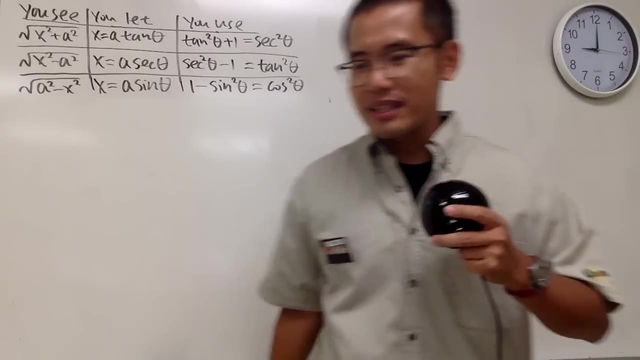 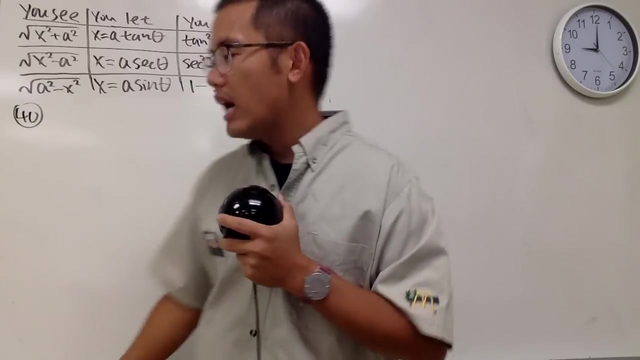 All the stuff And tell me Which Is, Tell me Which Category Is Your favorite. That too, All the stuff, Anyway. So Number 40. We have The integral Of 1.. 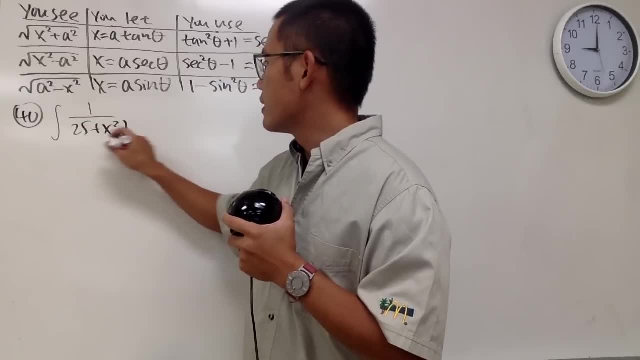 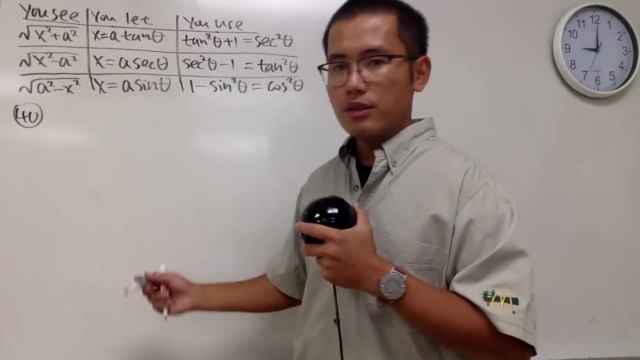 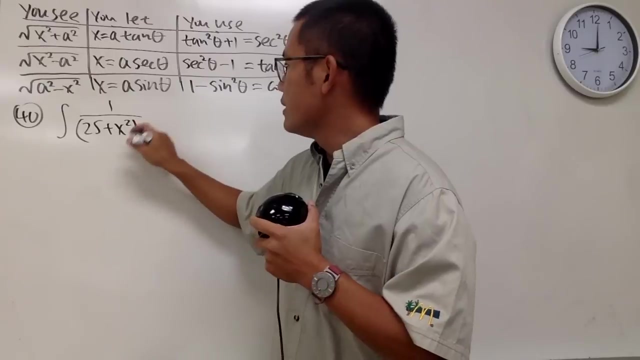 Over 25.. Plus X Square To The 3. Half Power. Oh Man, I have to write it down Bigger. So Let me see Integral 1. Over 25.. 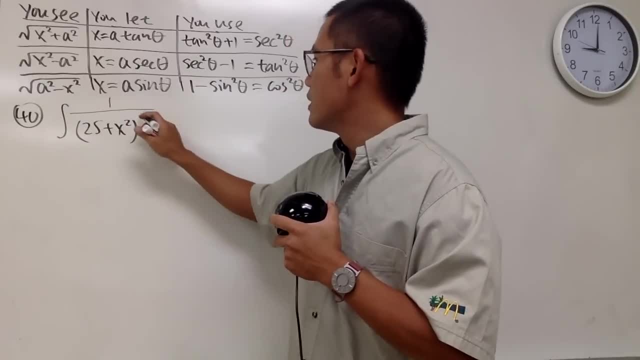 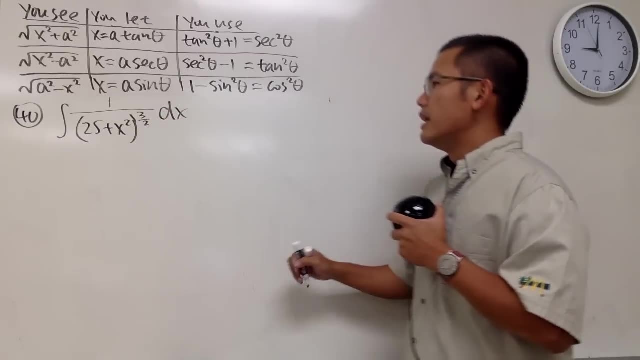 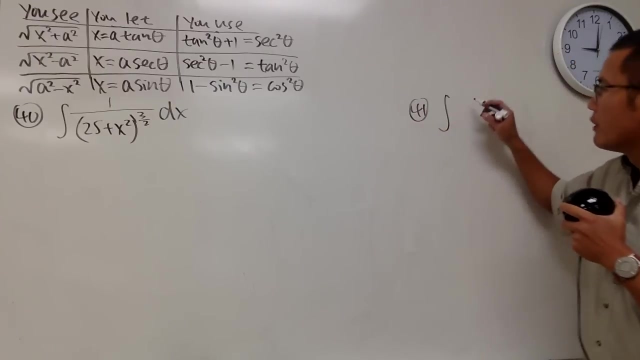 Plus X Square To The 3. Half Power, Like This. Okay, The X, Of Course. And How, Leave Some Space, I'll Come Here, I'll. 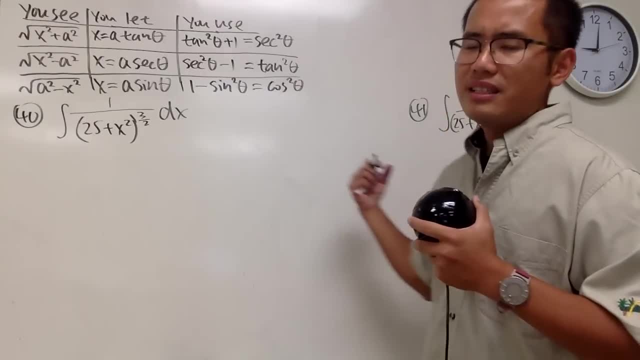 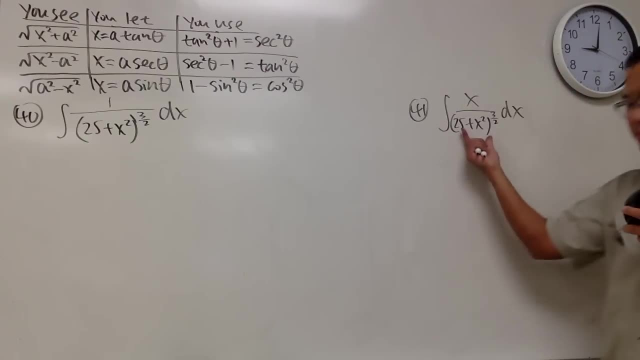 Say, Let's Say This Is Number 41. Let's See, Thanks To The X On The Top Especially, You Have This Right Here We Can. 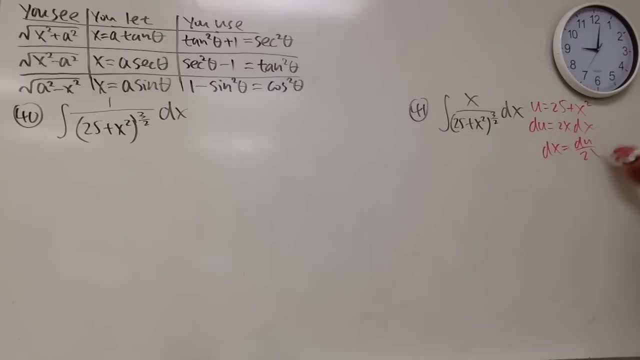 Just Do A Use Up That You Equal To To. I Mean 25.. X Over Inside, Here Is The U, So We Have U To. 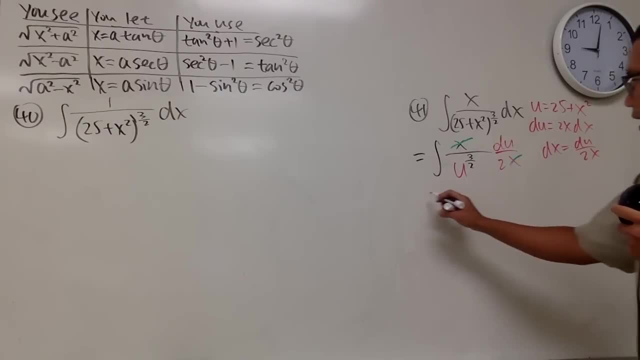 The 3. Half Power D X Is That Which Is D? U Over 2. X, And Of The Power D? U, Then We Are Going. 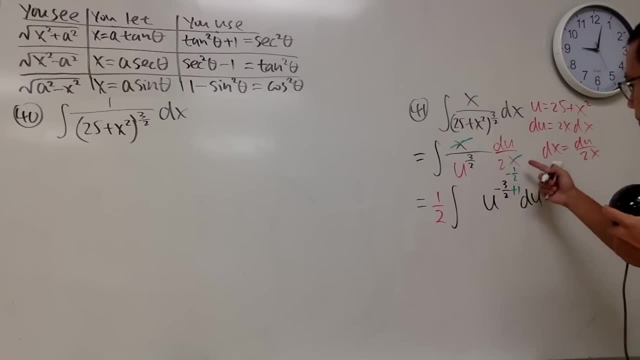 To Add One To The Power: Negative 3. Half Plus 2. Over 2. Which We Get Negative One Half. Yeah, Yeah, So We Have. 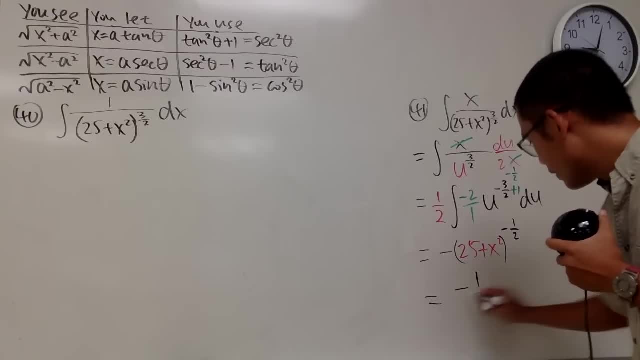 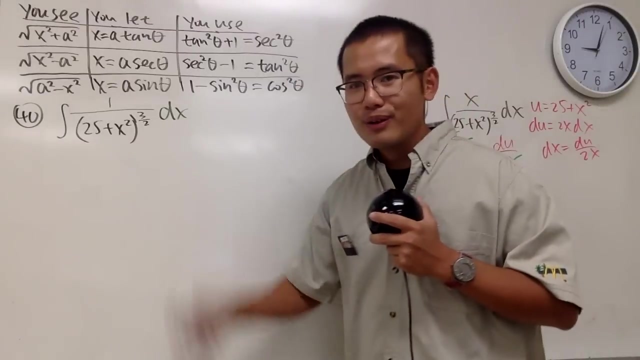 The Power, And Perhaps That's Just Right. Yes, Negative One Over. Bring This Down To The Nominator: Open The Square, Root 25.. Plus X. 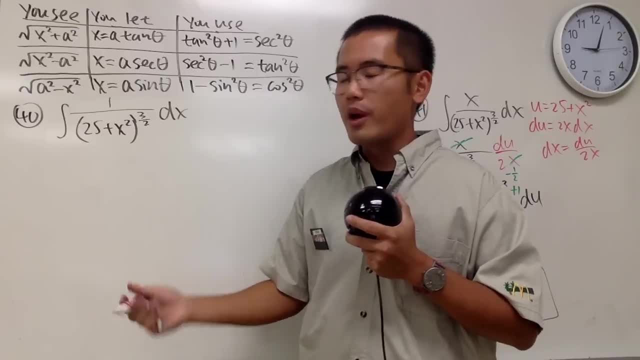 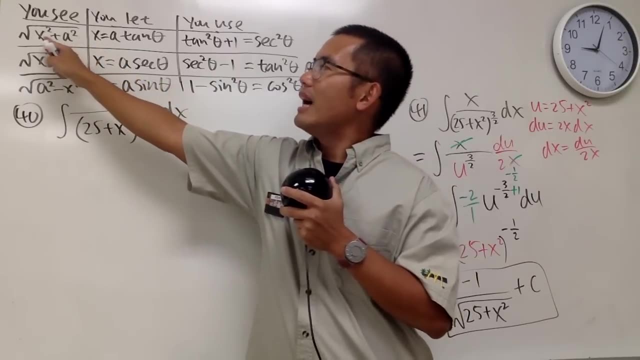 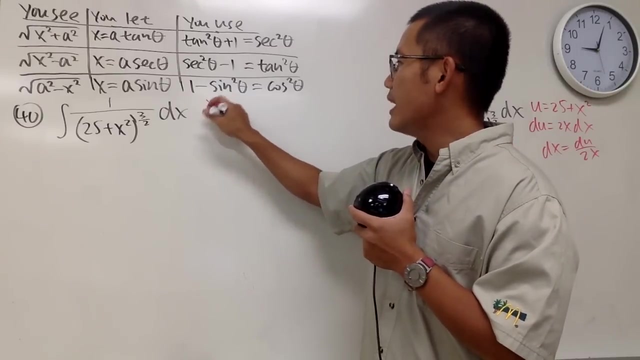 Square, Just 5.. Is The Same As 5. Square, So This Is 5.. Is The A Will Be This, Even Though I Have X. 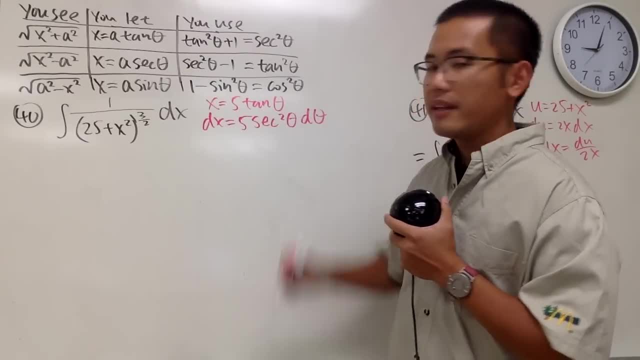 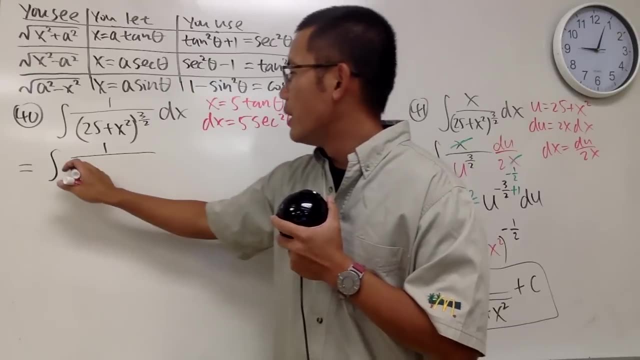 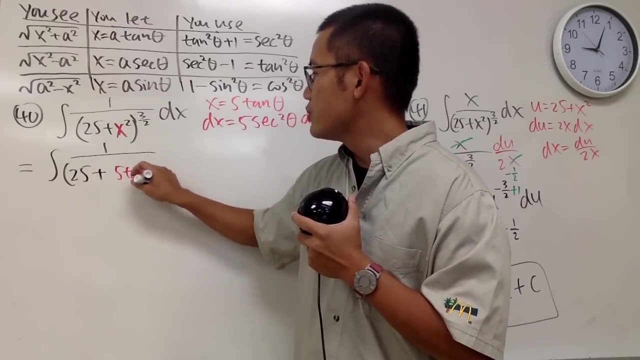 Square Plus A Square. But No, The Here Is The Integral One. Over Parentheses We Have The 25. Plus The X Is 5. Tangent. 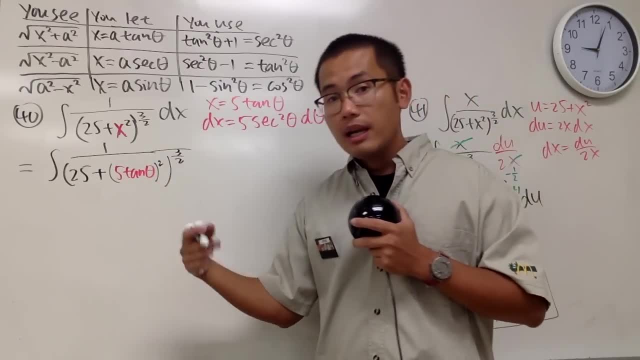 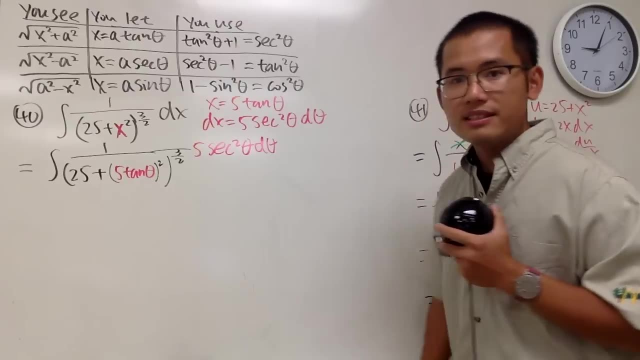 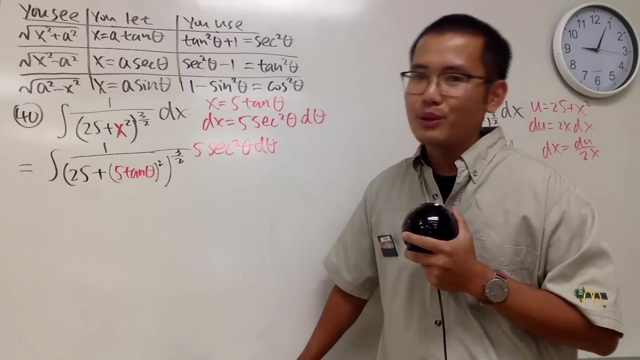 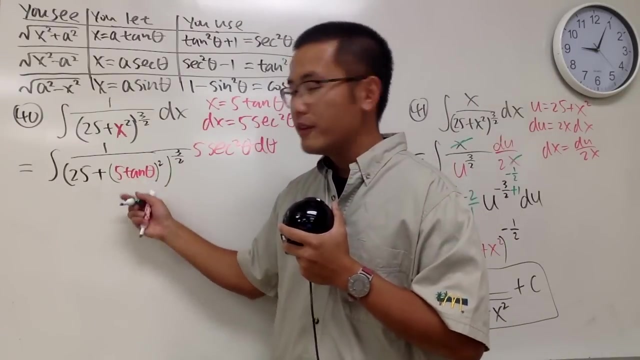 Data And We Are Going To Square That And Then On The Square Now Where To Work This Out. Man, It's Okay, It's Not So. 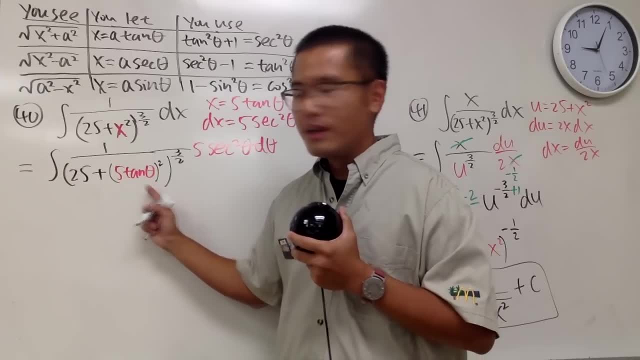 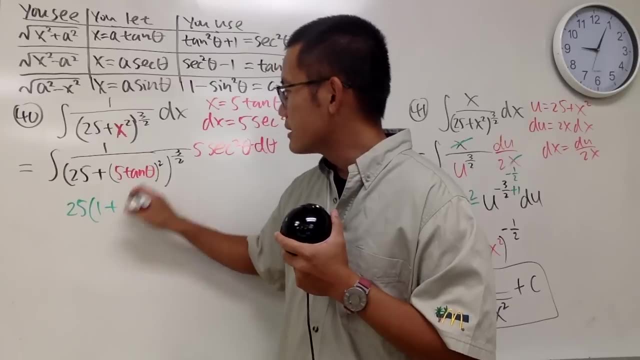 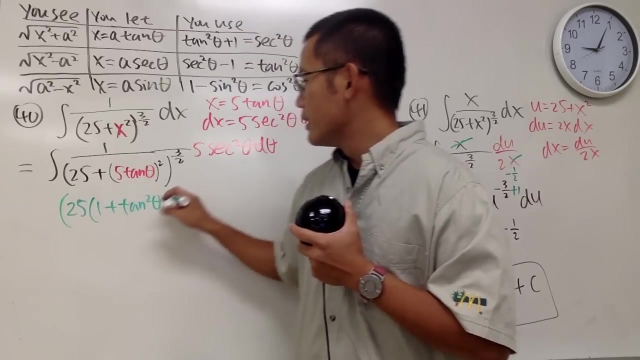 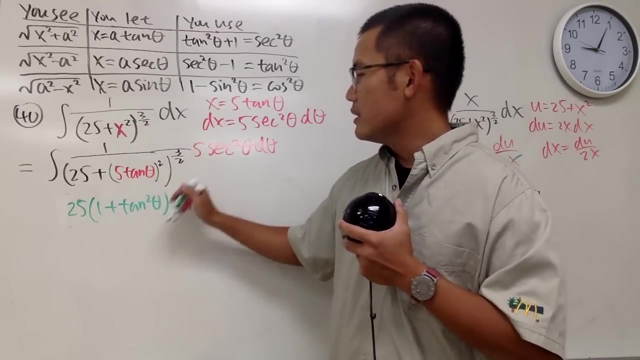 Bad, Check This Out. Okay, Just Do This In Green. Here Is The Inside, Which Is This Thing To The Three Half Power, But For The 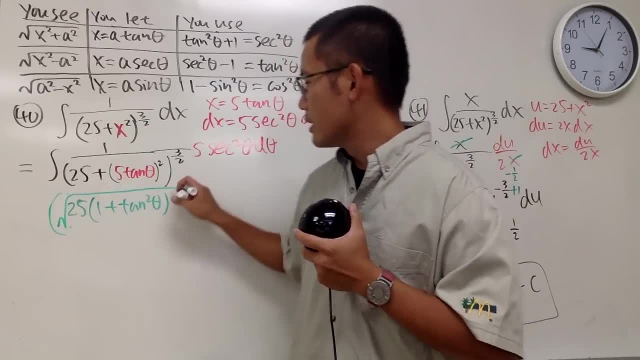 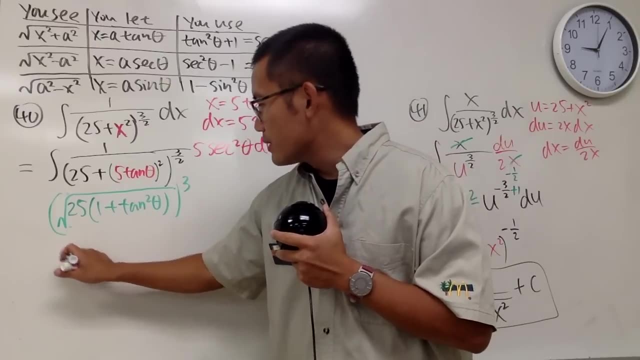 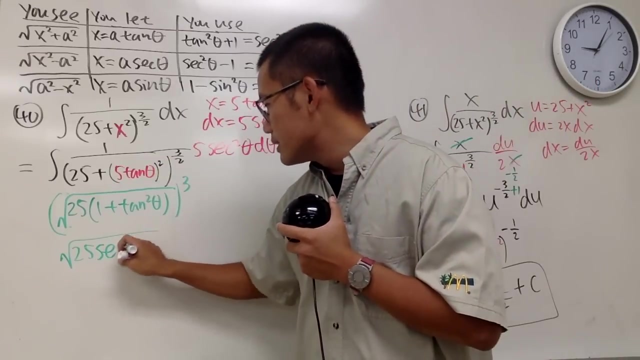 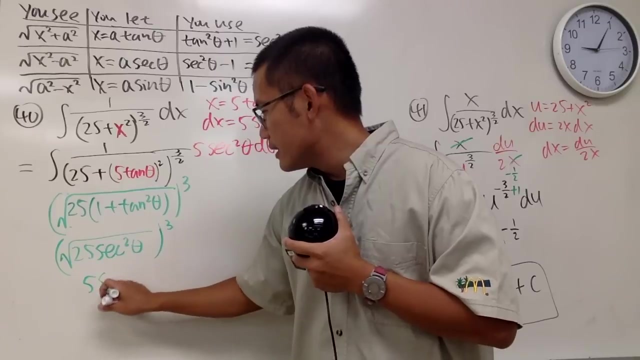 Three Half Power. The Truth Is, The Half Power Is The Square Root And Then The Third Power. Let's Just And Again Inside Out, We. 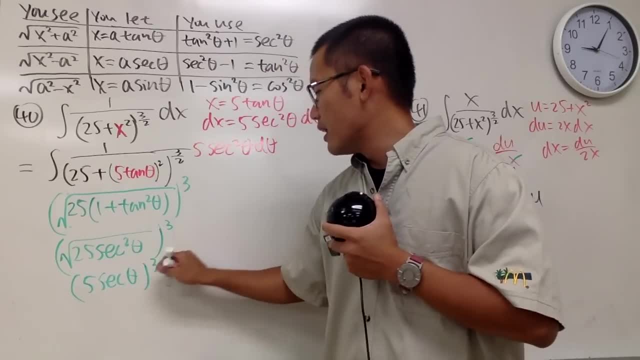 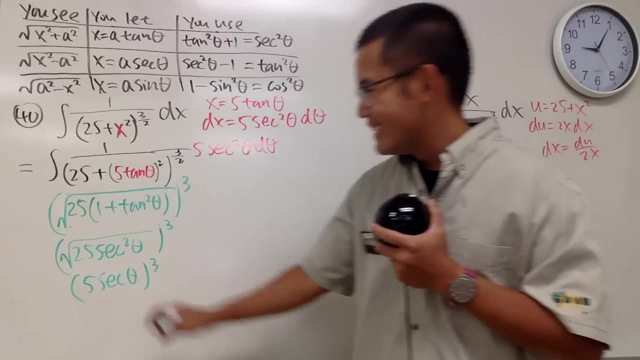 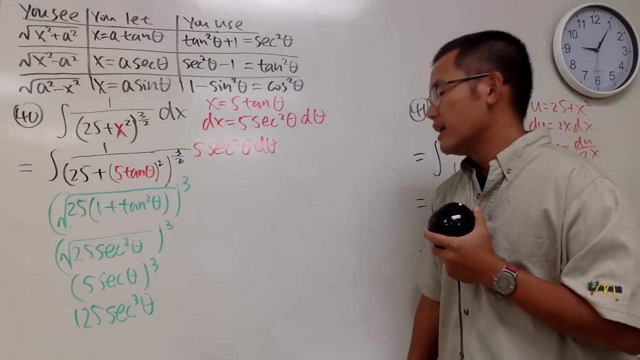 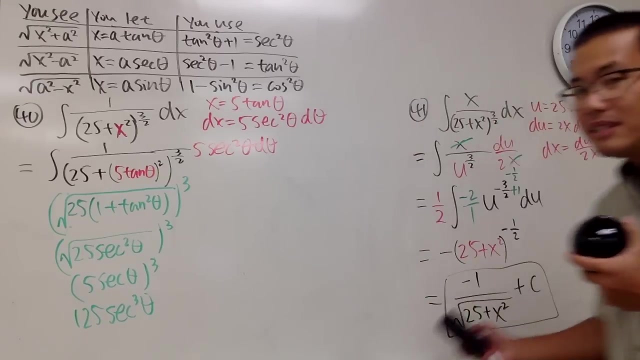 Get Five And Then Secant To The First Power, Theta, And Then The Third Power On Outside, Yeah, Because Again, This And That Can But. 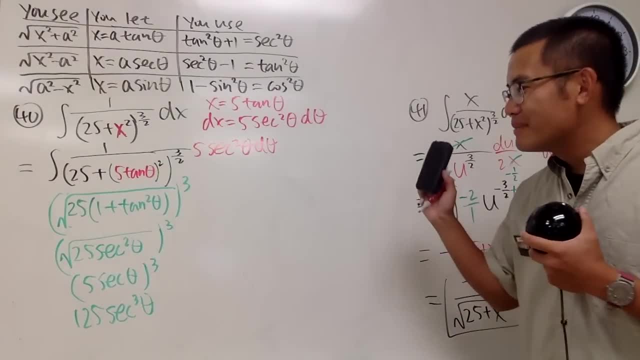 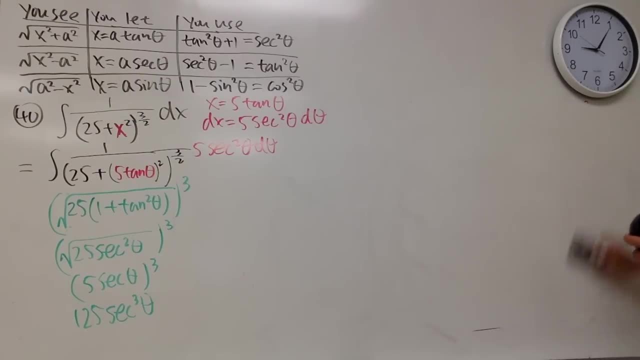 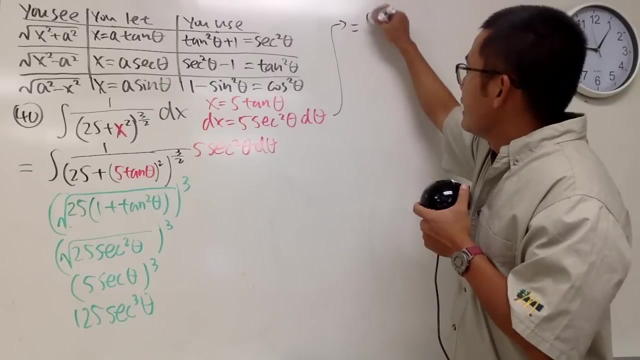 This Question Is Done. Your World Was Pretty Easy. I'm Going To Erase This One, Of Course, And I'll Just Put This Down Nicely. 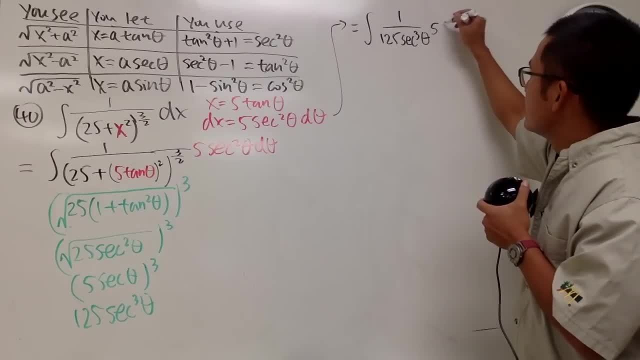 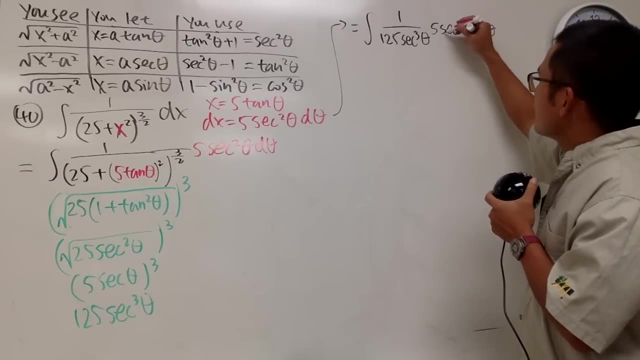 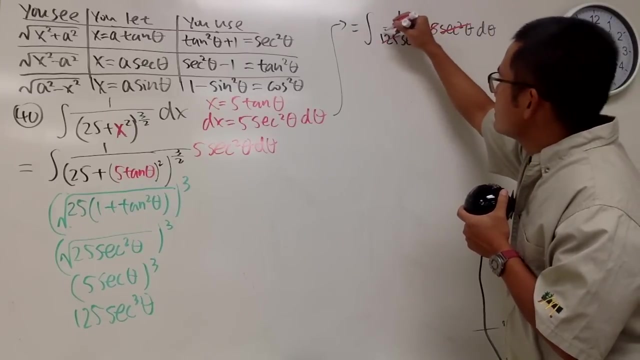 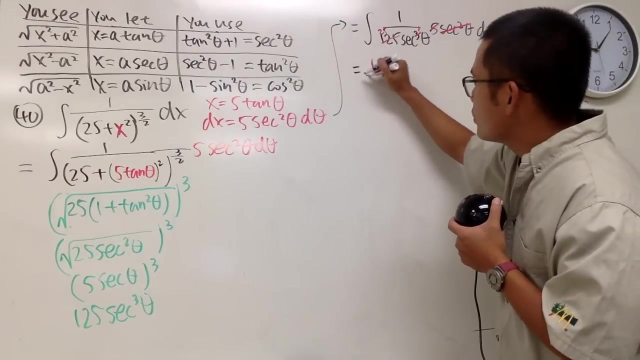 For You Guys. So Secant Square Theta, Theta, Right. So, After All The Simplification, This Is What We Have. Then We Can Can Sort This. 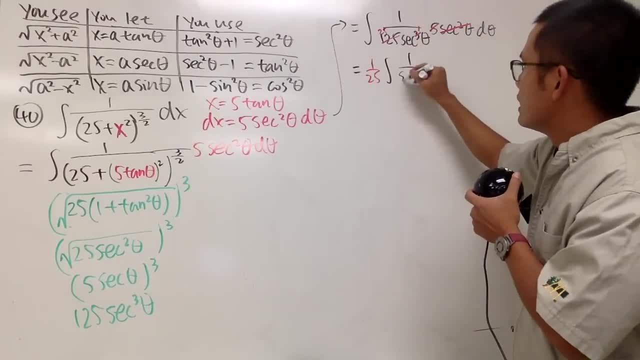 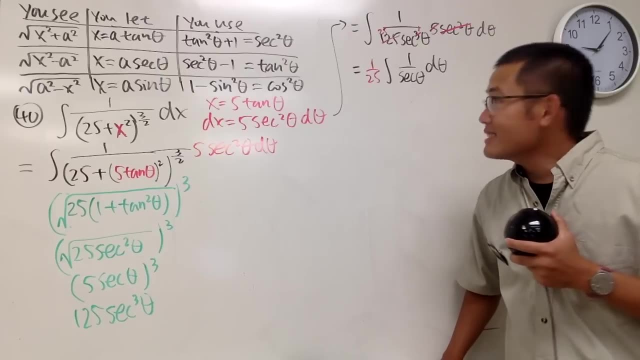 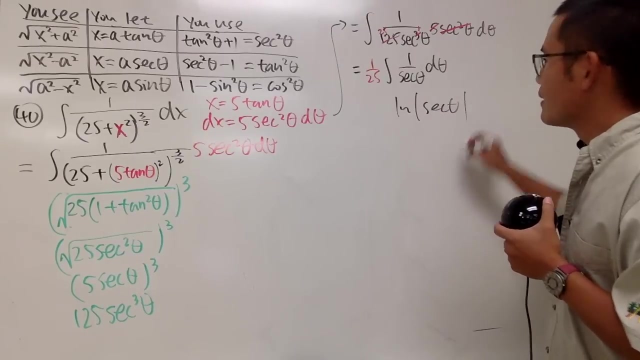 Secant Square And Now We Have Just One Theta. How Can We Integrate Secant Theta In The Denominator This Right Here, Easy, Natural Log. 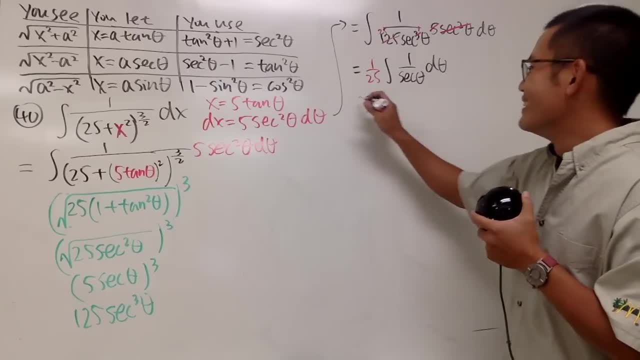 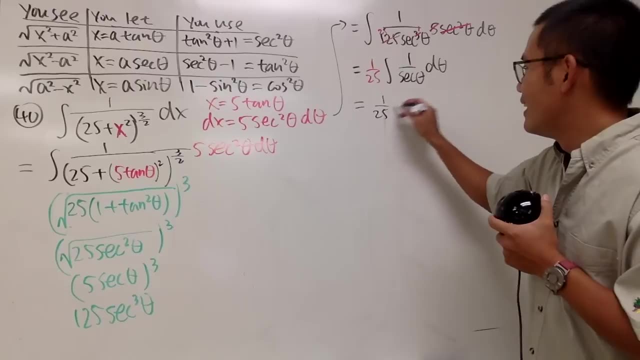 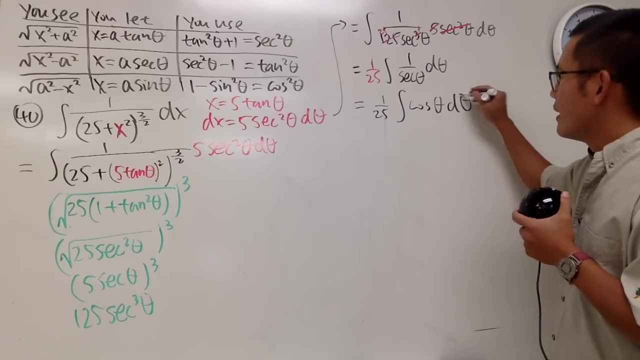 After The Value Of Secant Theta. No, Just Kidding, Don't Do This. Okay, So We Integrate Theta Right Cosine, Theta, D Theta And. 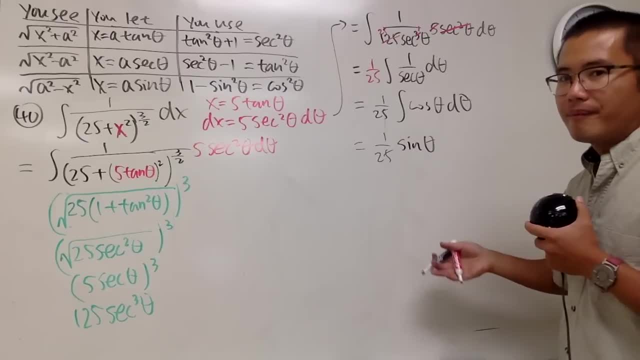 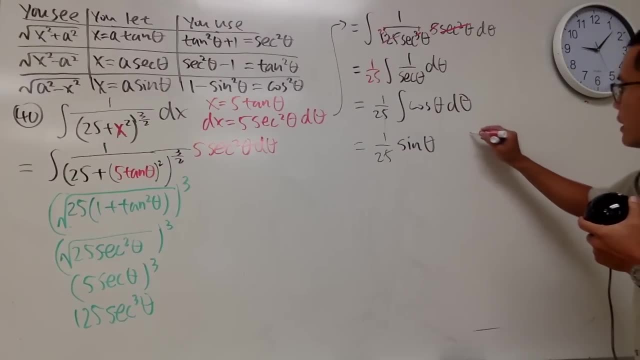 What's The Integral Of Cosine Positive Sign. So This Is One Over Twenty Five. Integrating This, We Get Positive At The Right Triangle X. 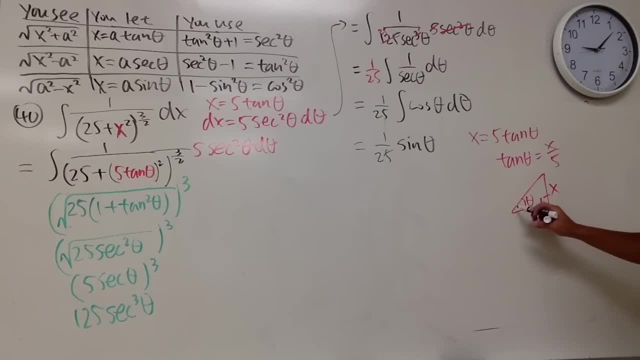 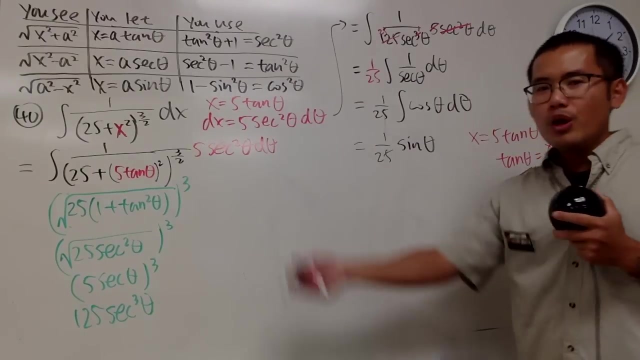 Over Phi Is Opposite Over Hypotenuse, And So Opposite Over Adjacent, And Then The Hypotenuse Is Right Here, Which Is The Square. 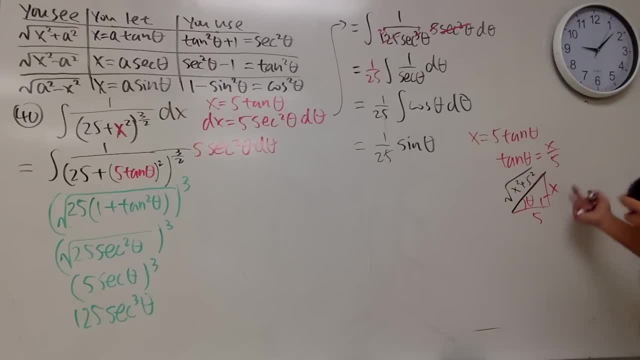 Root Of Sign Theta Is Namely Opposite Over Hypotenuse. Finally, We Have X On The Top Over This Twenty Five Right Here By The. 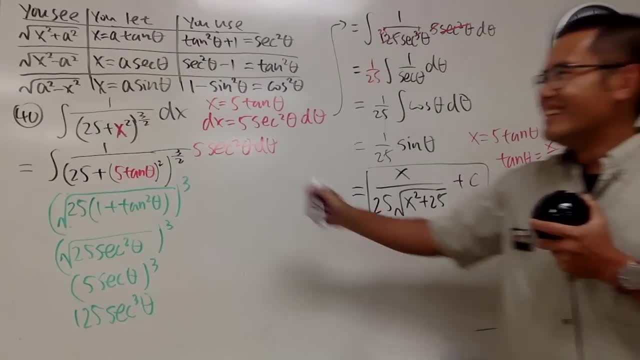 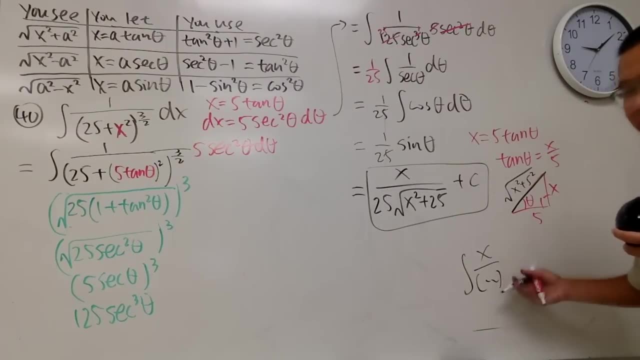 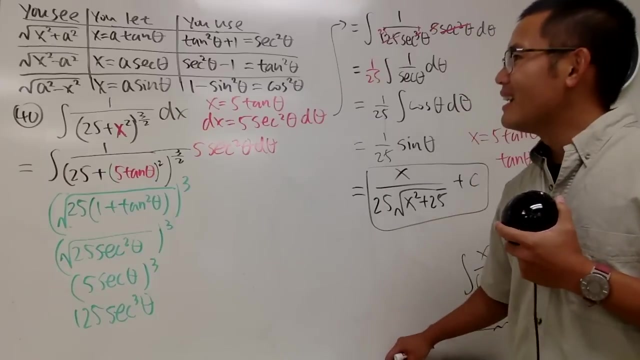 Hypotenuse. Hypotenuse Is Square Root Of X, Right And Earlier. When We Have The Integral Of X Over Blah, Blah, Blah And 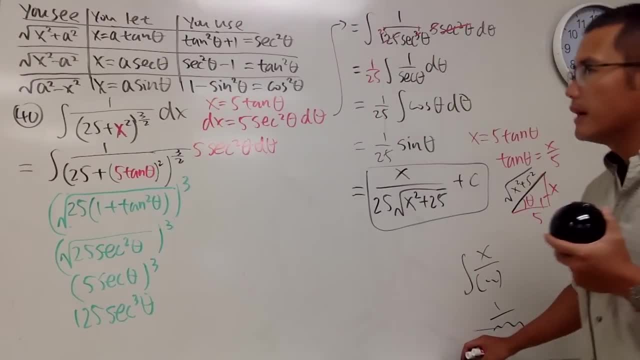 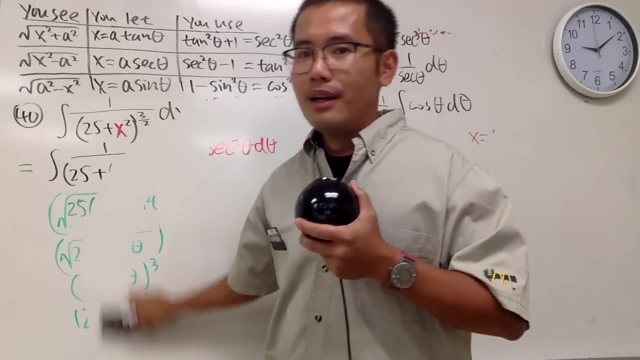 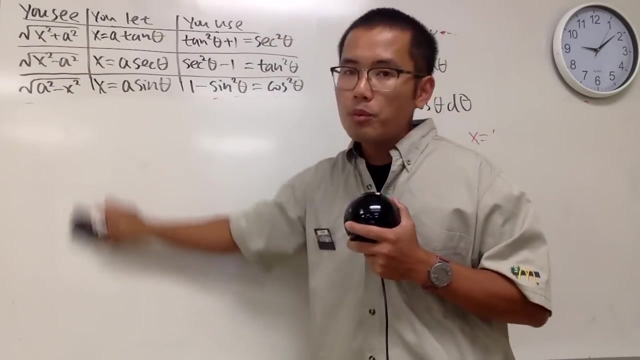 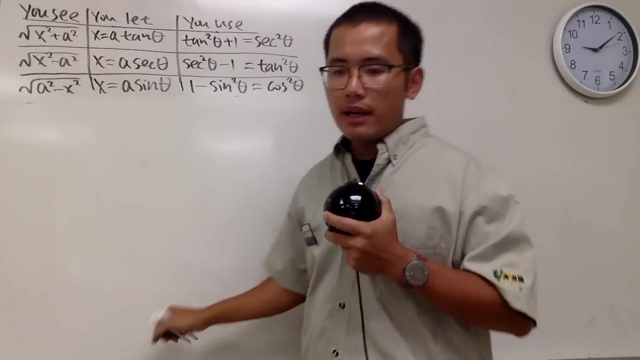 The X Ran Away The Answer One Over. That Was Pretty Cool. So This And The Following One Is Going To Be Crucial Because It's 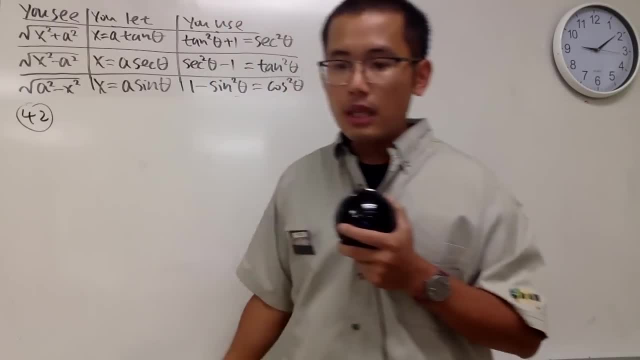 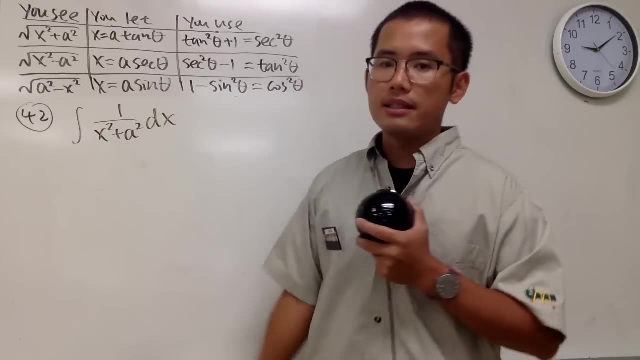 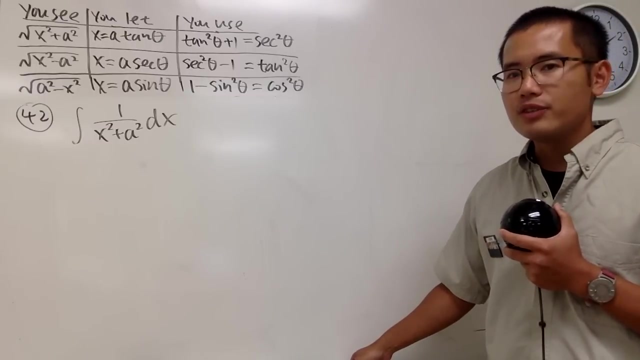 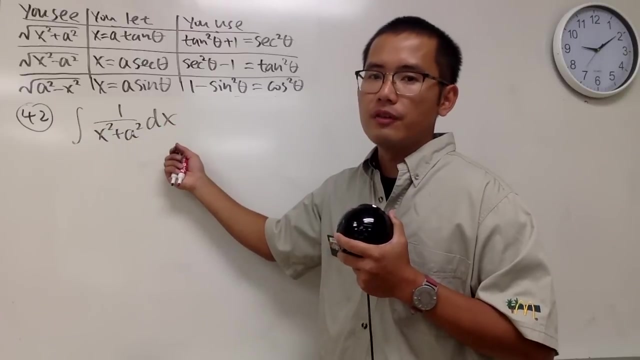 Going To Be A Formula That Will Be Using For The Last Category. Okay, So Here We Have. Imagine, If You Have Just A One Right. 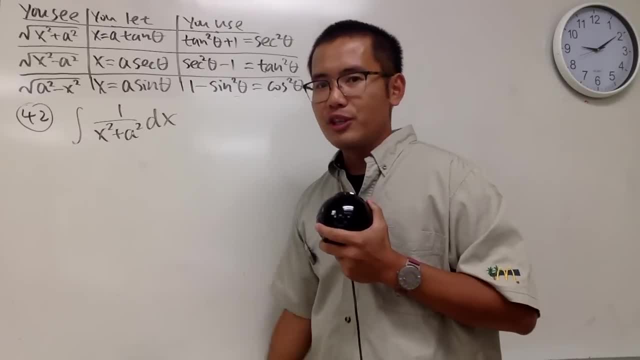 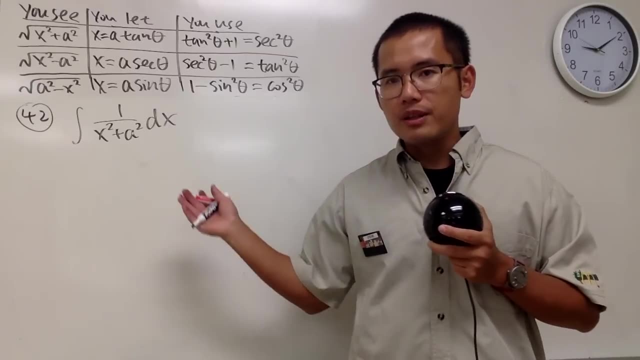 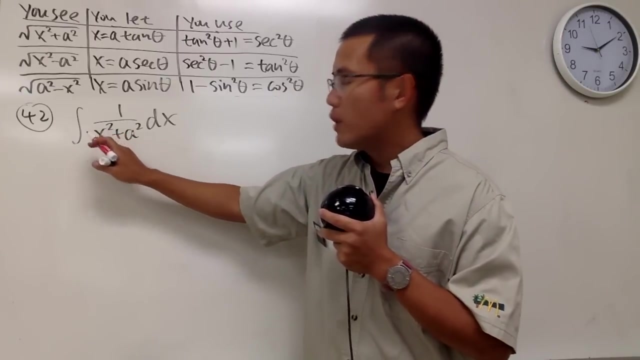 Here One Over X Square Plus One That's Inverse Tangent Of X. That's Okay, But If You Have A Square Right, We Can Still. 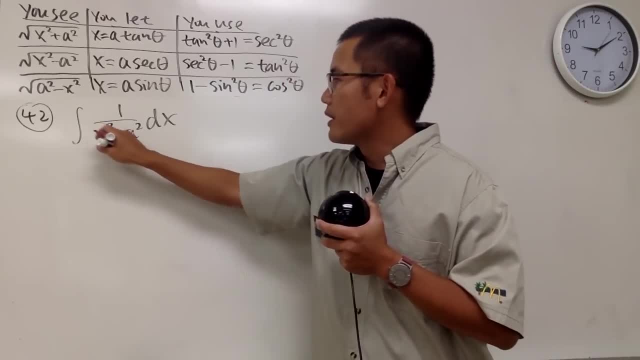 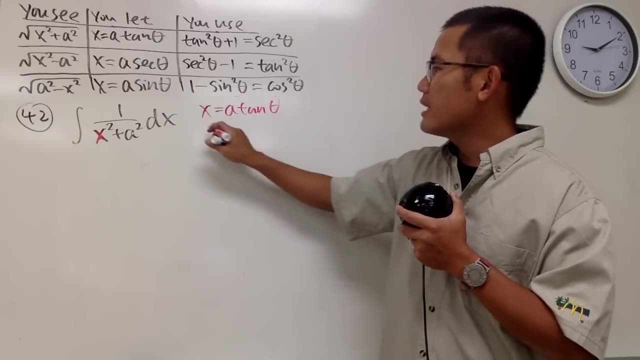 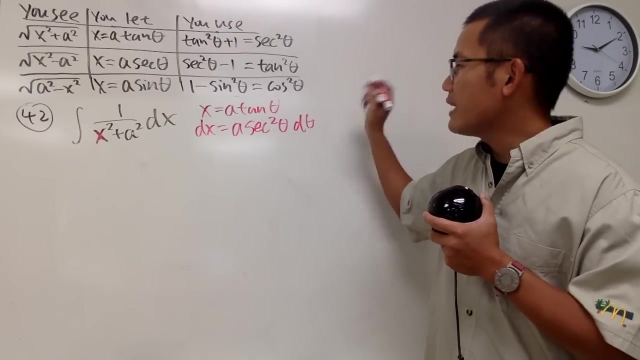 Take The Substitution And You Will See How It Works Out. Nicely. We Have X Right Here Plus, So It's A Tangent Situation. Take. 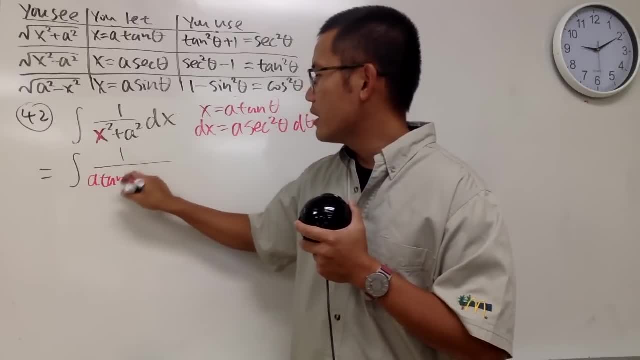 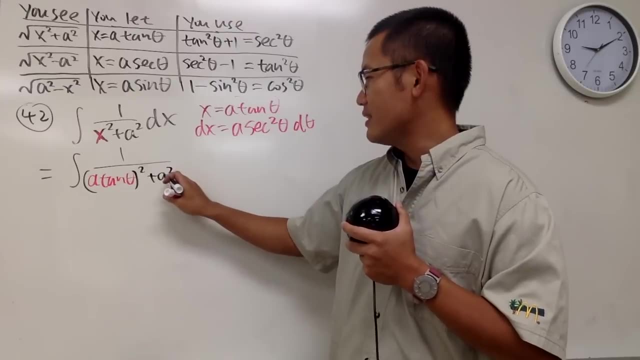 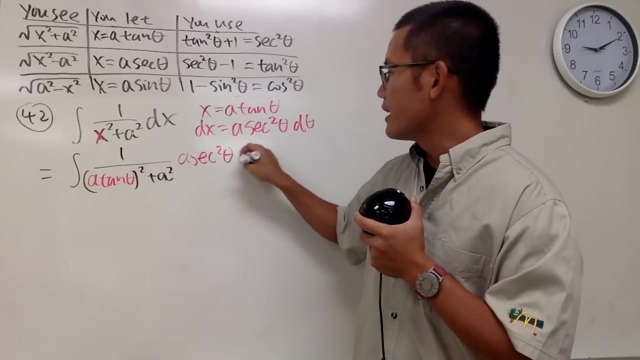 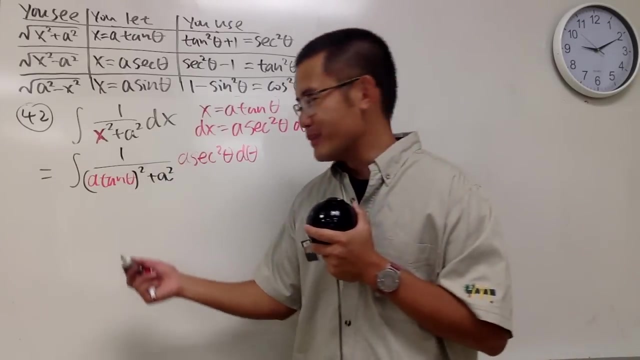 X Equals A Tangent Data Square Plus A Square. This Looks Like A D. X Is All That Which Is A Secant Square, Theta D. 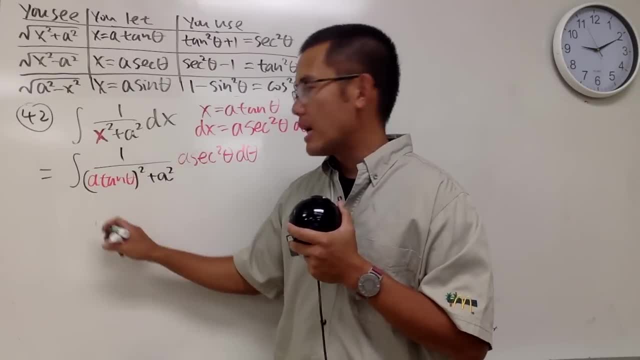 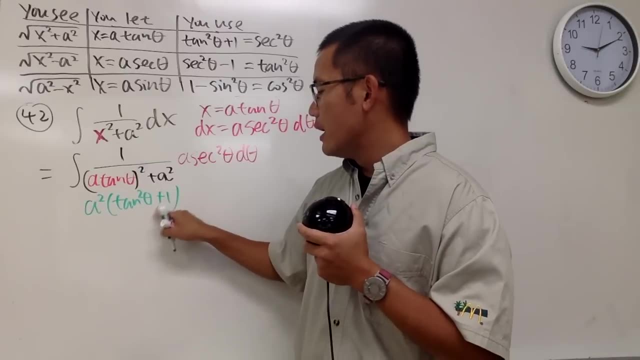 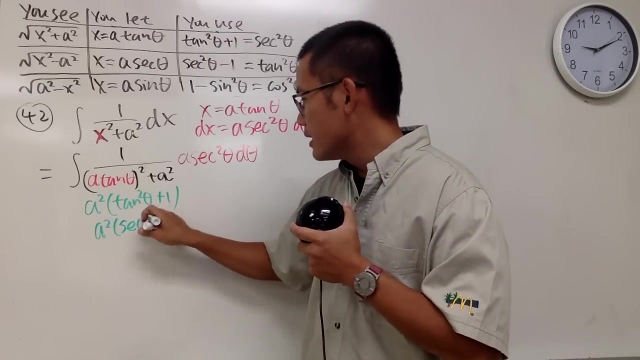 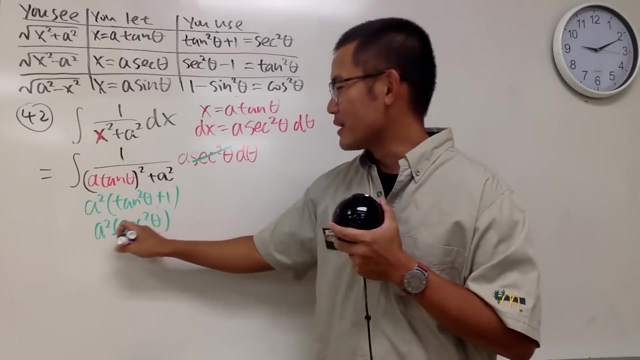 Theta. Now, Let's Do This Again. Then We Have Tangent Square, Theta Plus One, And This Is A Square, And This Right Here Is Secant. 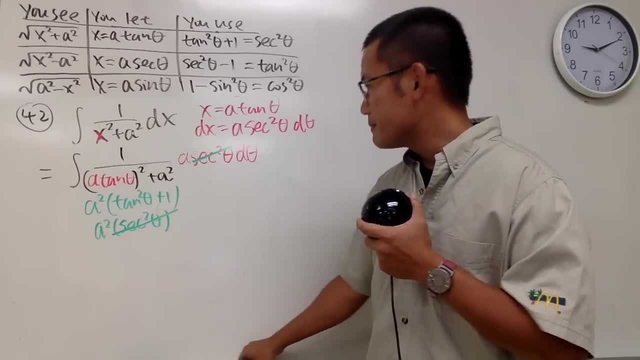 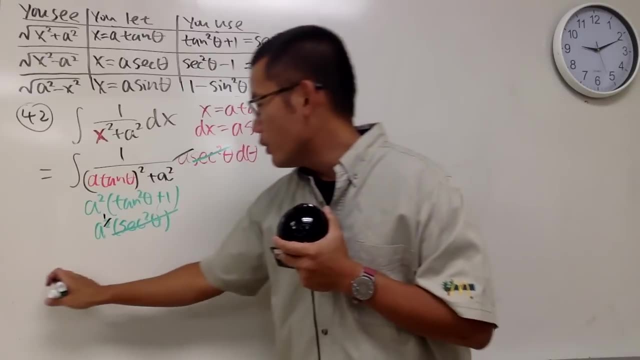 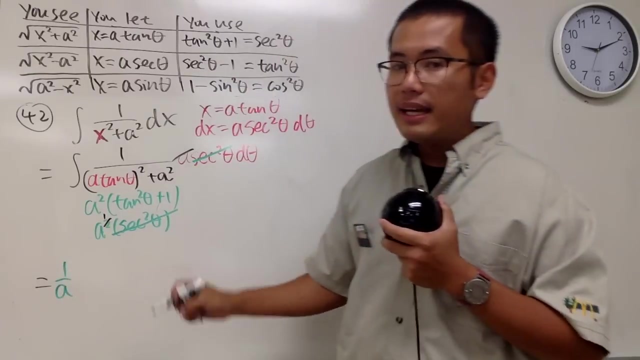 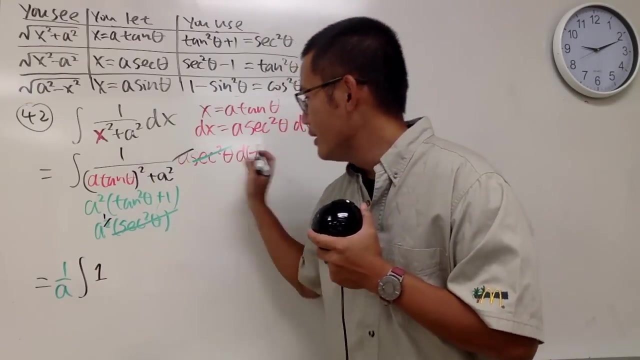 Square Theta. So This Is Secant Square Theta Like That. So All In All We End Out With One Over A All The Way In. 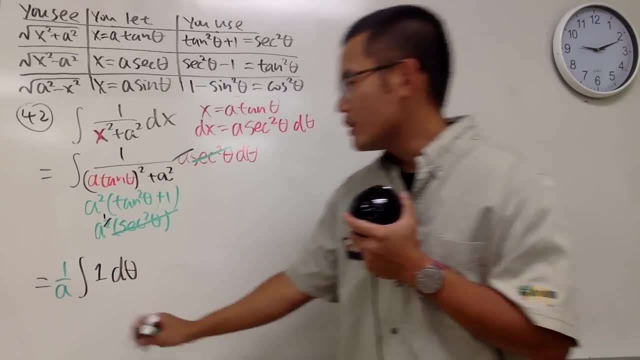 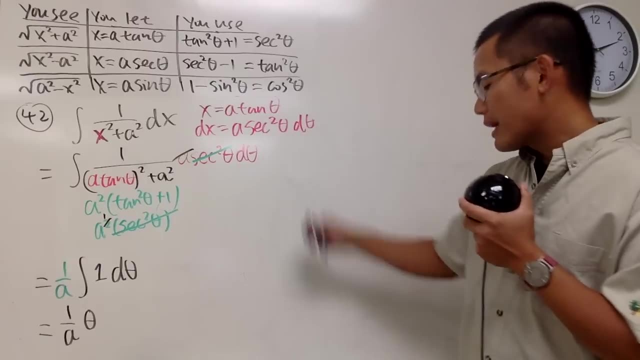 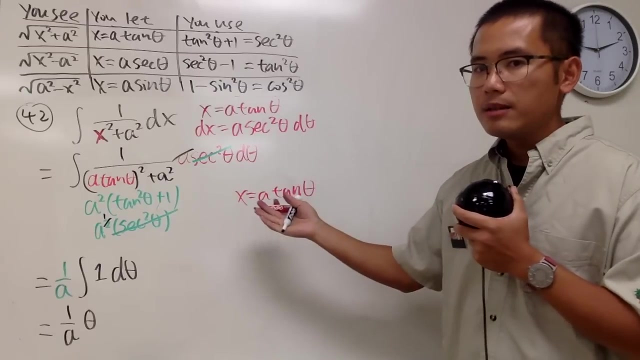 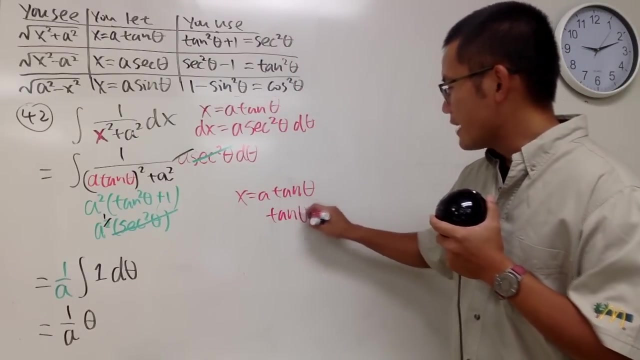 The Front. Let Me Put This Down In Green. And Then We Have The X Is Equal To A Times Tangent Theta Divide A On. 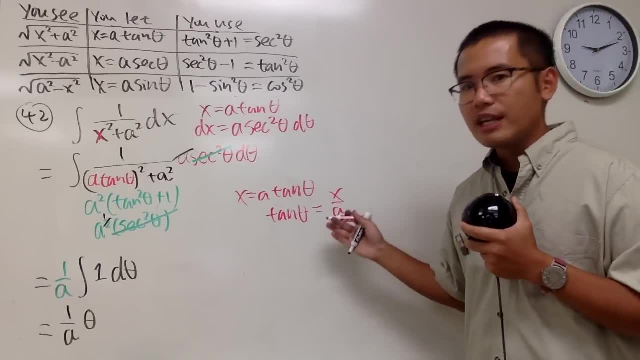 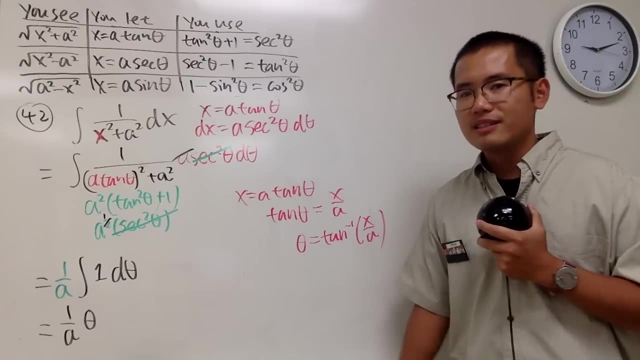 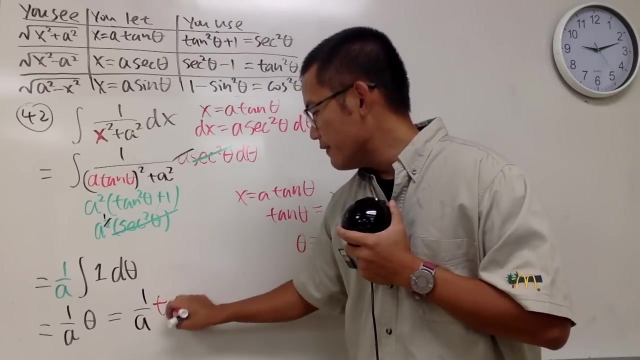 Both Sides And Of Course A Cannot Be Serial Solved. We Get Tangent Theta Equals X Over A, Tangent Of X Over A Like. 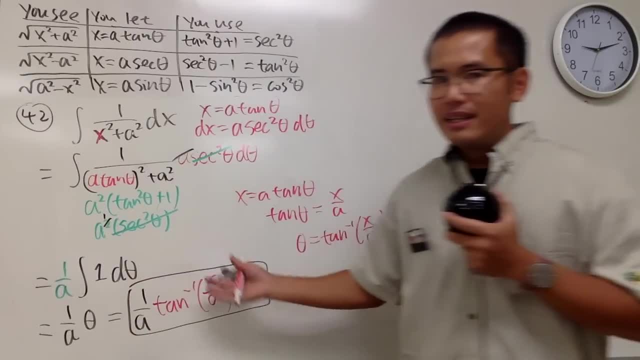 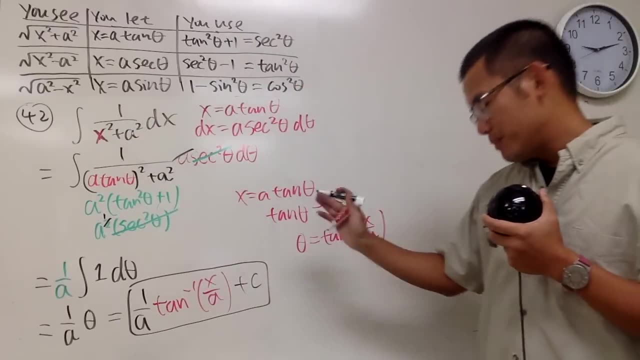 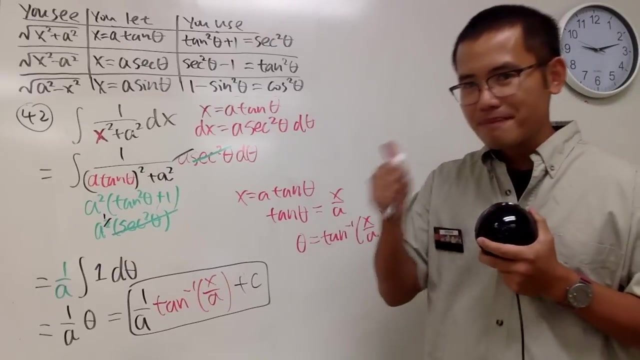 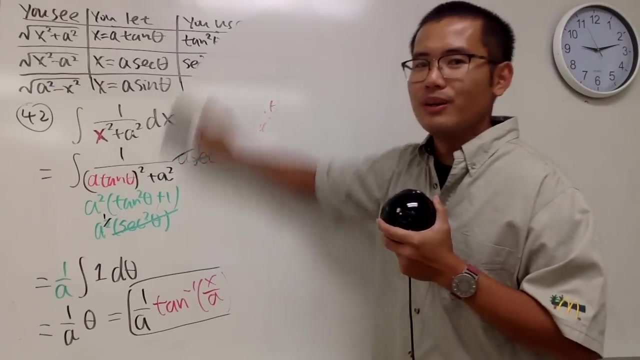 This, And With That We Are Done. Again, This Is The Formula That We Are Going To Use For The Later Part. Right, So We Have. 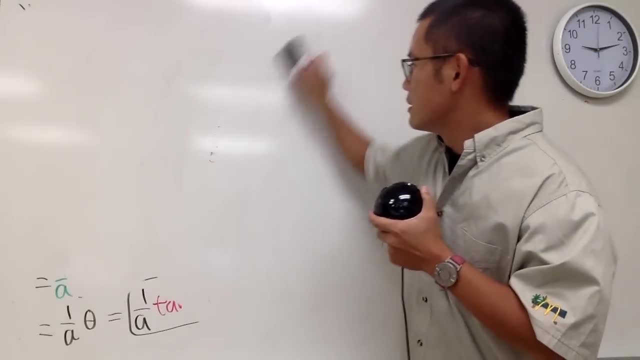 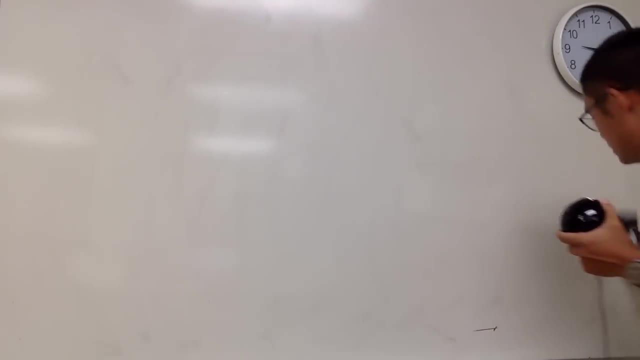 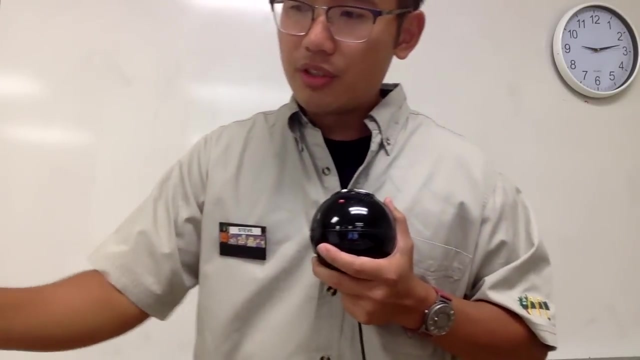 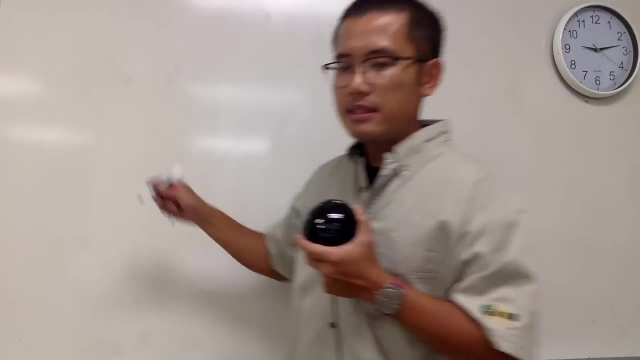 More To Go And We're Going To Say Bye, Bye To The Trick. Substitution For Now. Okay, Yes, Last Page, And Then Let Me Just 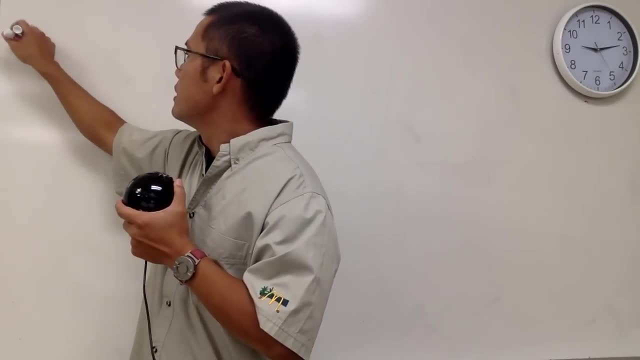 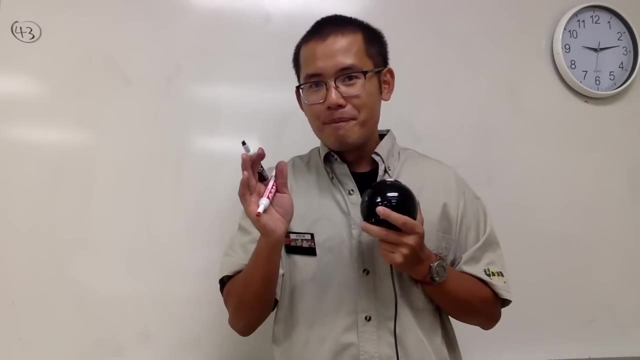 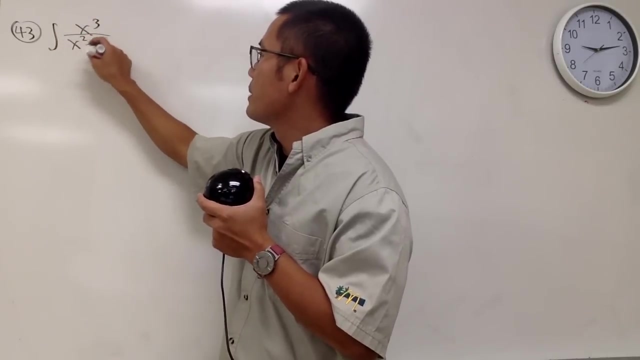 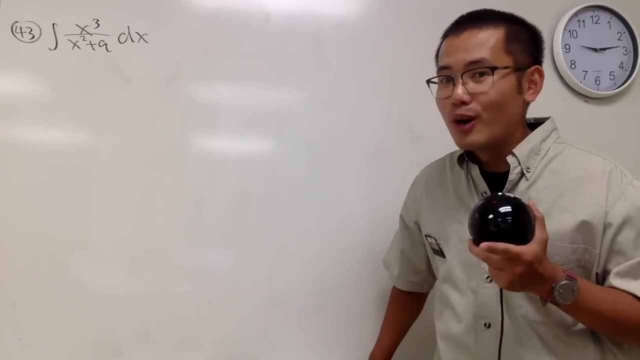 Check The Question. This Is The Last Category, But Again, I'll Just Do A Question As An Introduction. So Let Me Know How You Guys 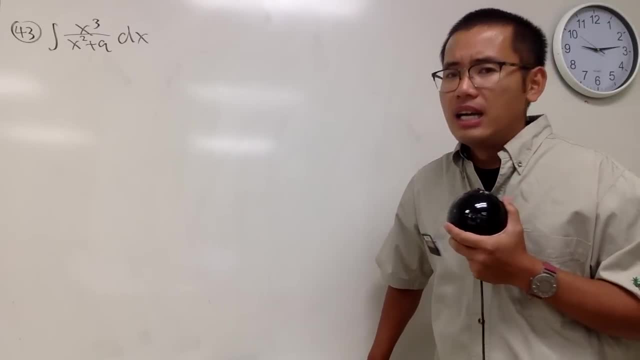 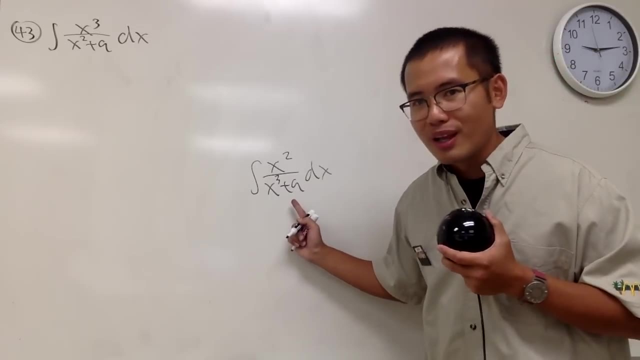 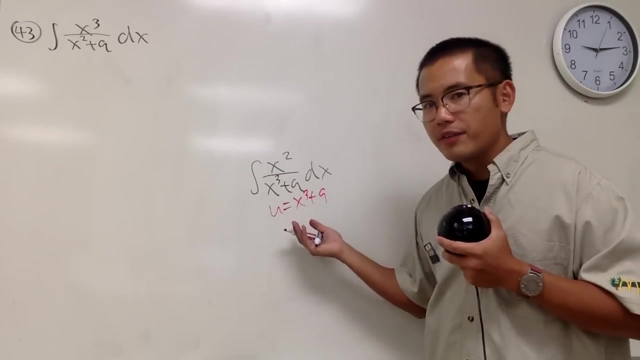 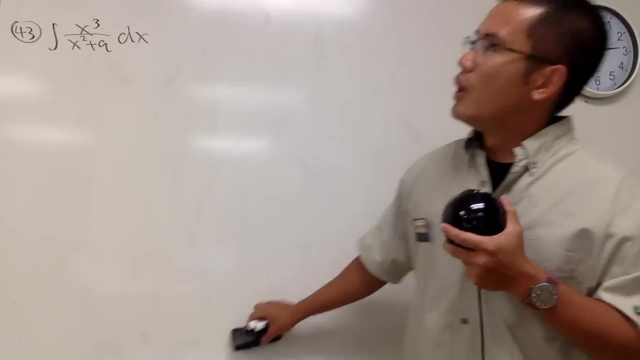 Are Doing All That Stuff Anyway, Over X Plus, Third Power Plus Nine Dx. How Do You Do This One? Just Use Up, You Can Let. 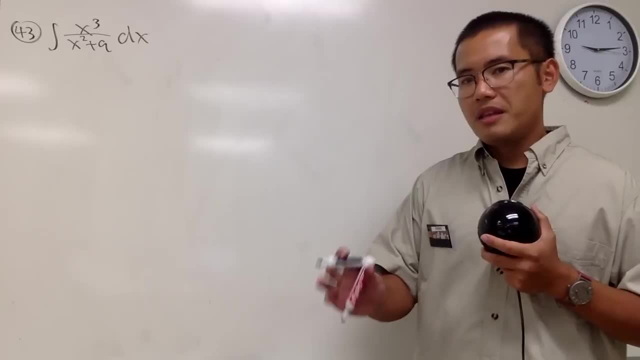 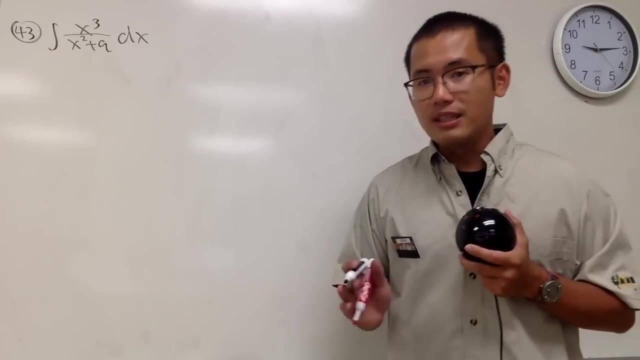 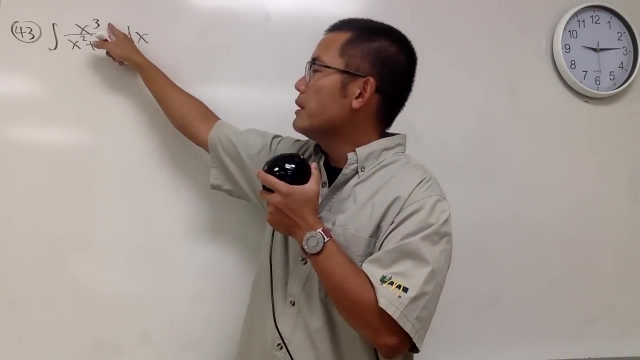 You Equal To The Bottom That You Could Do Whatsoever. It's Just A Lot Of Algebra And You Have To Remember The Setup. Here's: 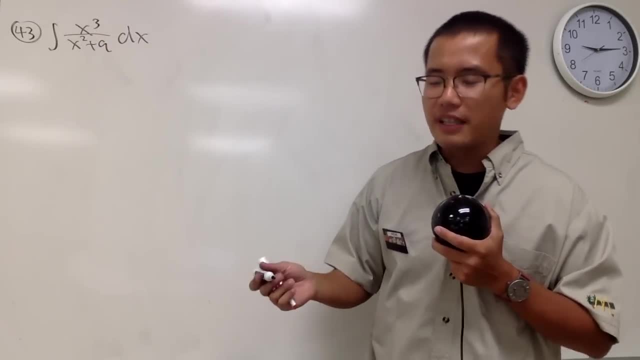 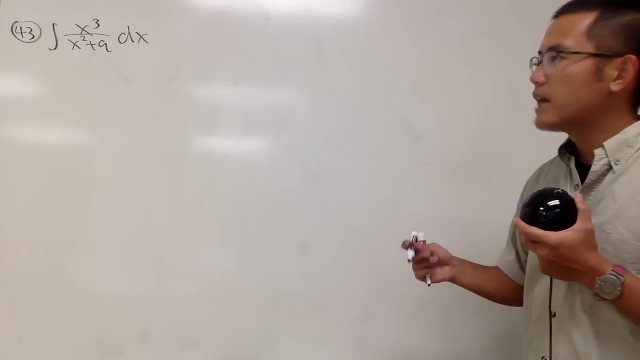 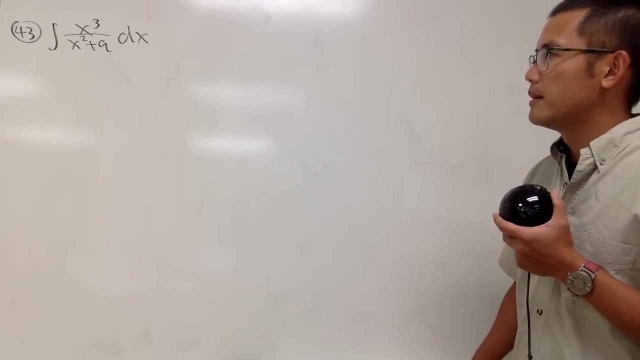 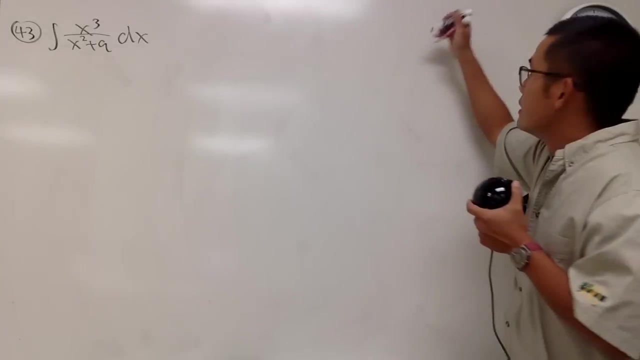 The Deal. This Is Not What We Preferred. It Because The Degree On The Of All People Let's Put It Down Right Here. Let Me 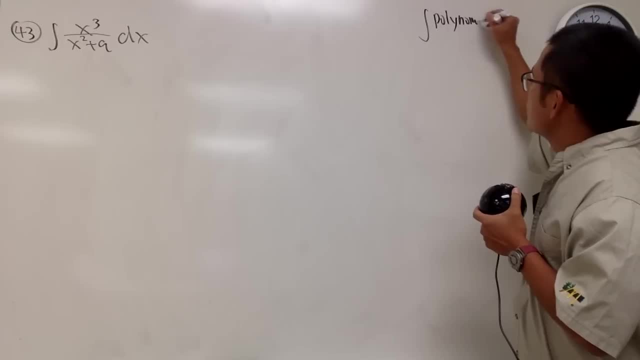 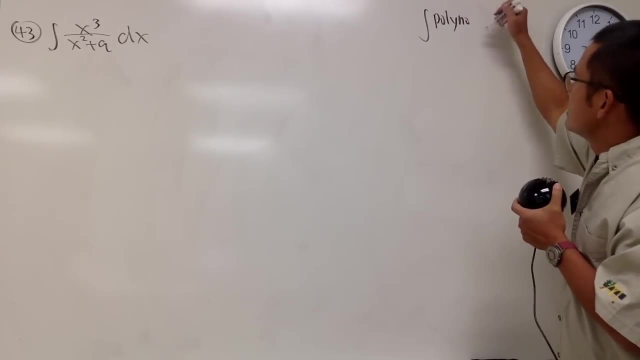 Just Put This Down Right Here. Let Me Just Put This Down Right Here. So The Last. And when we are talking about a polynomial, we have to pay attention to the exponent. 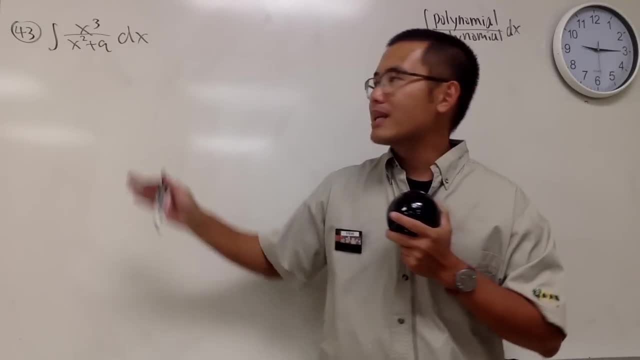 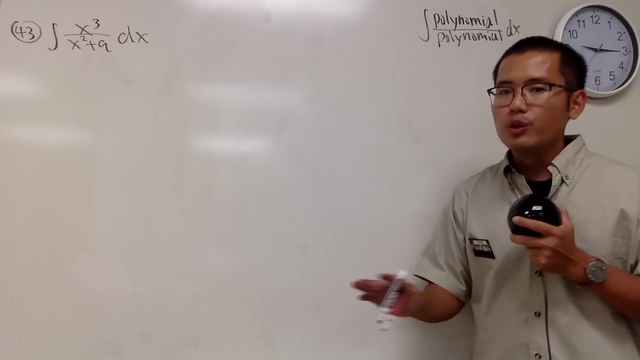 The exponent. they have to be positive whole numbers or sometimes just like zero, like you don't have the x. So that's what makes an expression polynomial. You don't want square root, you don't want negative exponent, you don't want e to the 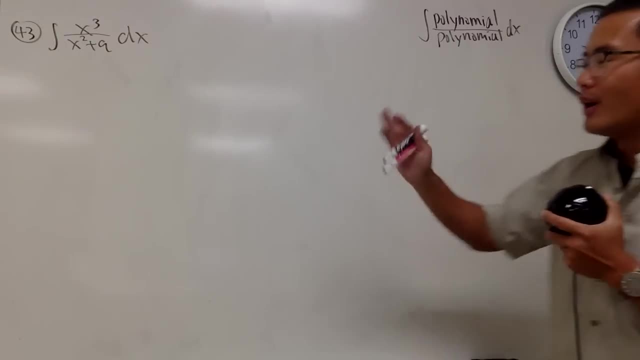 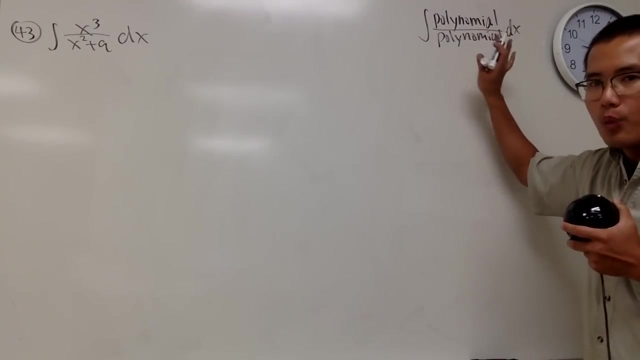 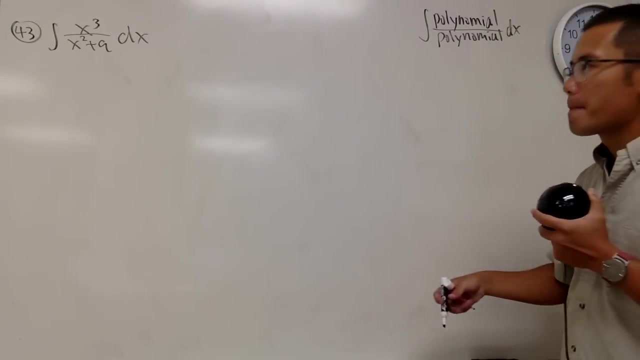 x. you don't want ln x, So it's just. you know we can deal with the usual factoring, etc. etc. back in algebra days. This is the form that we want. This is the form that we are dealing with for this last category. 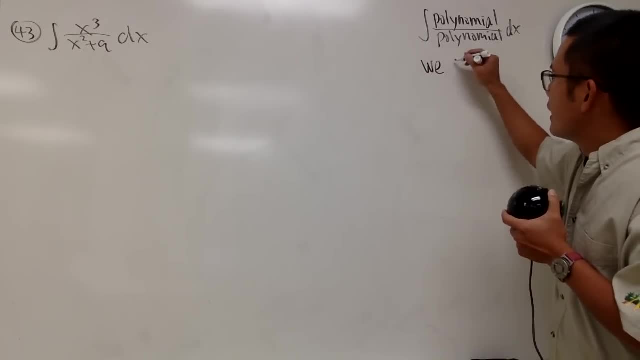 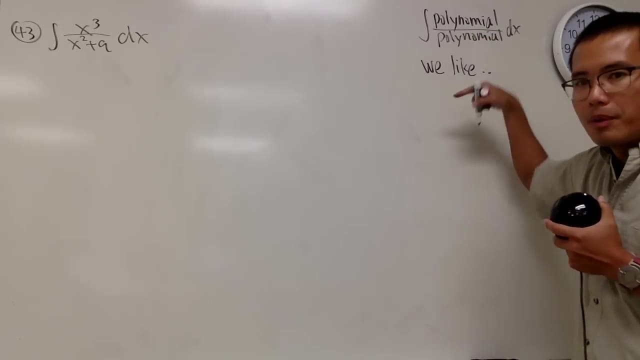 Well, let me just give you guys the following. Here are the integrals that we like whenever we are integrating a polynomial over a polynomial. The first case is that if you have the integral of 1 over and, of course, if you don't have, 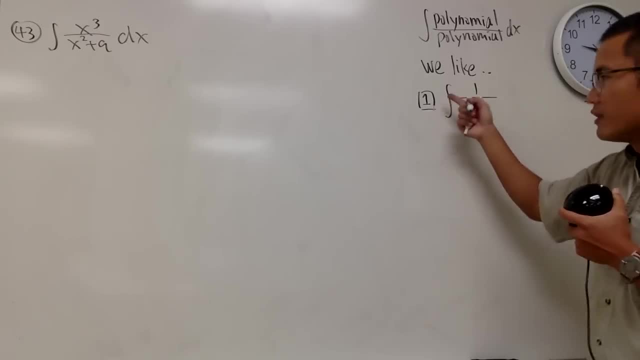 1, you don't have a polynomial. If you have, let's say, 17,, you can just put a 17 in the front. So I'll just put on 1 right here for simplicity's purpose. Anyway, if you have 1 over ax plus b, dx- well, I think we have discussed this earlier- like 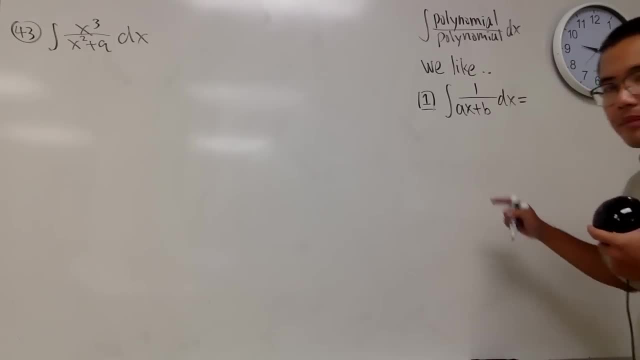 I don't know how many hours ago, But this right here is a linear function situation, So we can just do the u-sub and then you end up with a natural log situation. right, That's very nice. The answer for this is 1 over a natural log. 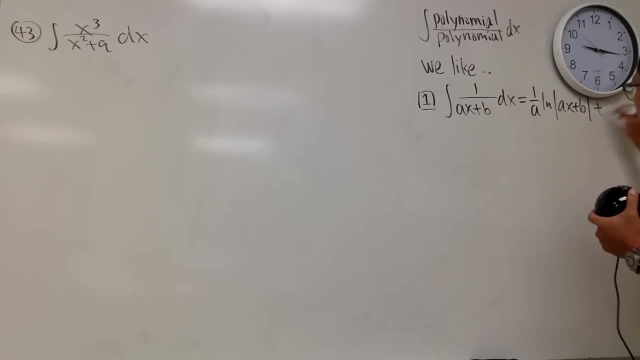 Natural log, absolute value of ax plus b and then plus c, of course. So this is definitely one of the rational functions that we like. OK, second one. Well, let's put down the one that we did earlier. When we have the integral of 1 over x squared plus a squared dx. 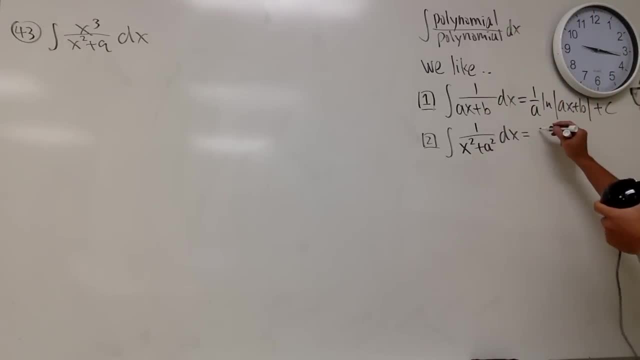 We did this earlier for question number 42. And the answer is 1 over a Inverse tangent of x over a and then plus c. of course We also like this because we just did that earlier. right Now let's look at some variations of this. 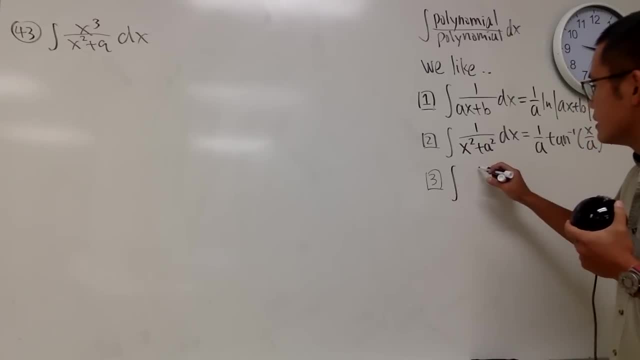 Suppose we have a quadratic on the bottom and we happen to have this x on the top. If we just have x on the top, we actually do hope to have a nice quadratic on the bottom. And the quadratic is: I just want to have ax squared plus a squared dx. 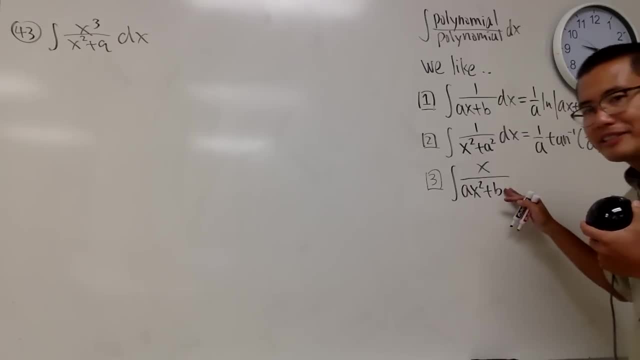 OK, Plus b. I don't want any more x, Because if I differentiate the bottom I get 2ax, That's all, And then that will cancel with the x on the top. So I can just do u sub for this. 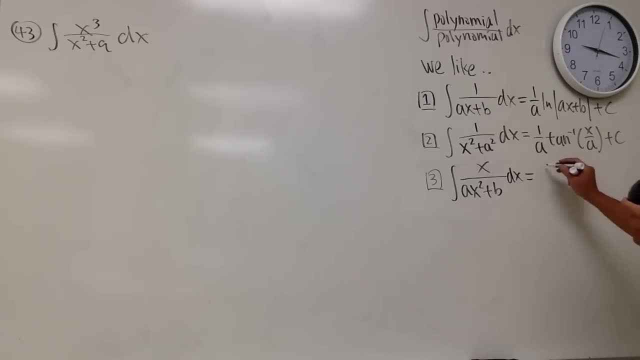 I'm going to leave the work for you guys And the answer. in the end you end up with 1 over 2a Because, again, if you differentiate this, you get a 2a and all that And you end up with natural log because the x will cancel out. And then on the bottom you'll just get a u if you do the u substitution, And then you end up with natural log because the x will cancel out, And then on the bottom you'll just get a u if you do the u substitution. 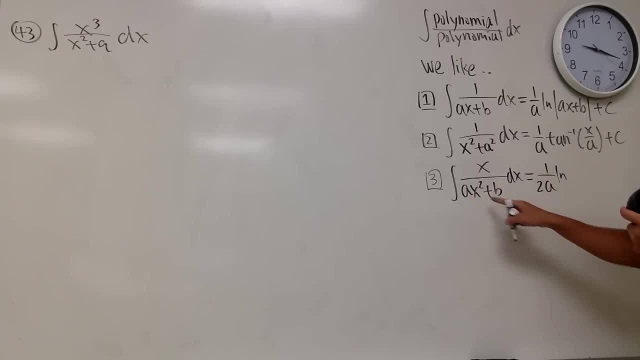 And then on the bottom you'll just get a? u substitution, And then on the bottom you'll just get a? u substitution, Because I don't know the a and b for now, a assuming, not 0, of course, otherwise it. 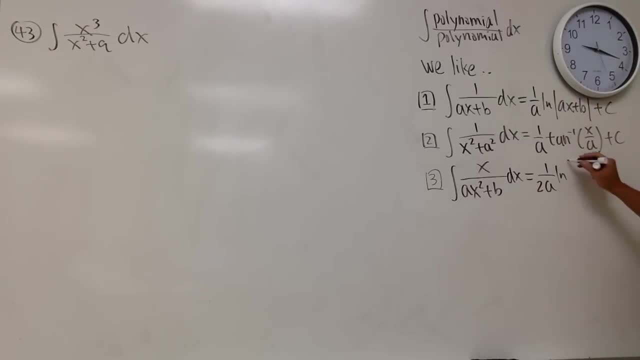 would be boring, So I will just write it down as the absolute value, ax squared plus b and then plus c, like this: Perhaps these three are the most common one that we have to remember and use This right here. you don't really need to memorize it. 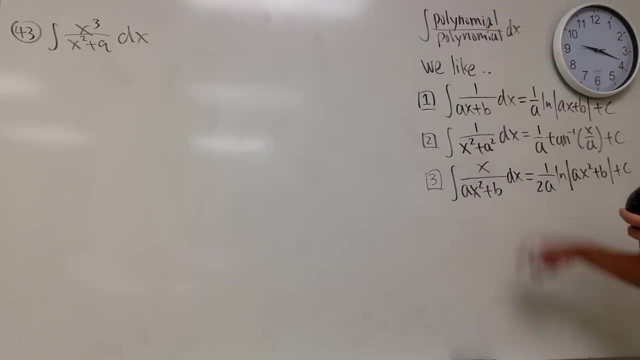 You can just do u sub real quick, But you can also eyeball this and then just do it in your head or something. That's also great. So let me just put down these three, and then I do have more on my handout. 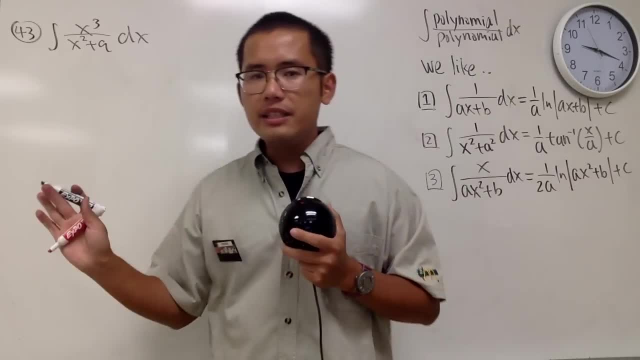 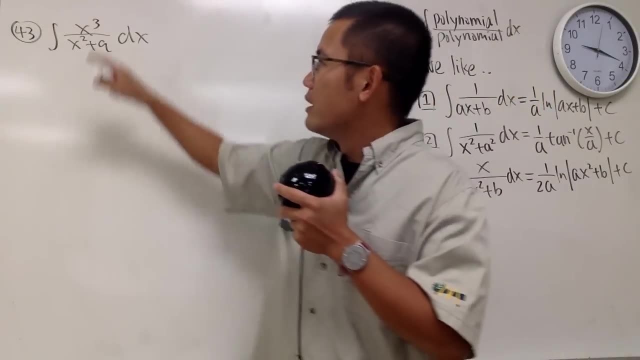 You guys can just refer to that. But anyway, let's see how can we make this into one of these. Yeah, let's see. Here is the DO First case, when the degree on the top is higher than the degree on the bottom and 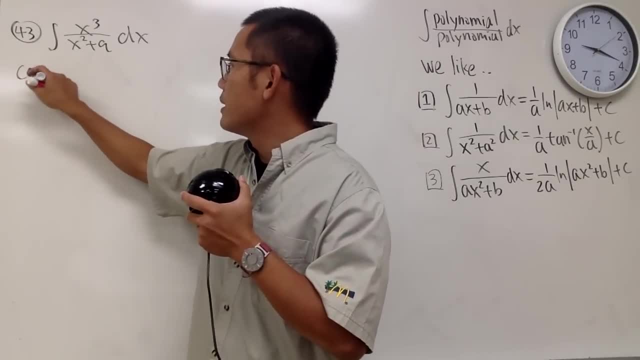 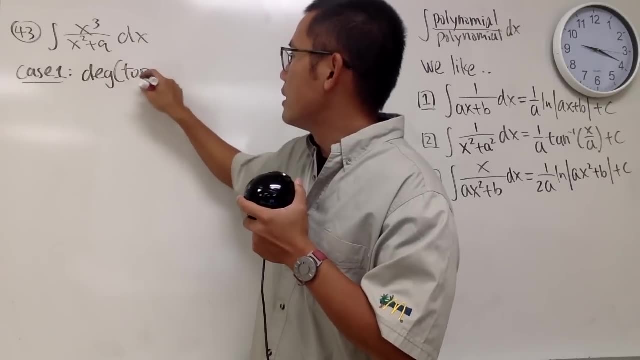 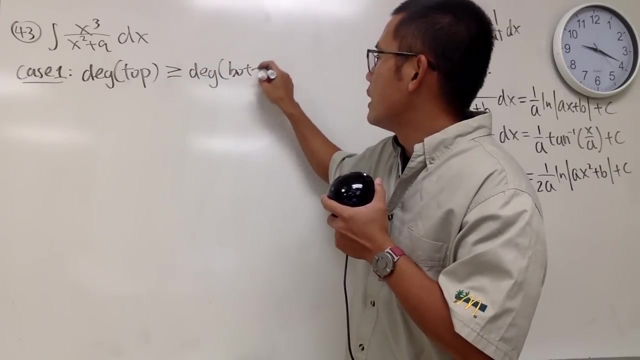 sometimes equal to you, also do the following. Case one, right Case one: The degree on the top, The top polynomial is bigger than or equal to the degree of the bottom. And again, DEG stands for the degree, namely the highest power of x in the polynomial. 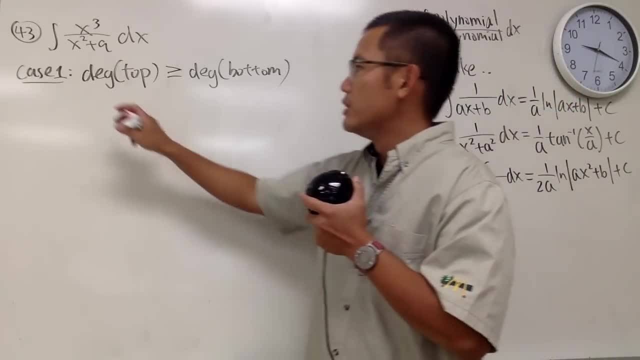 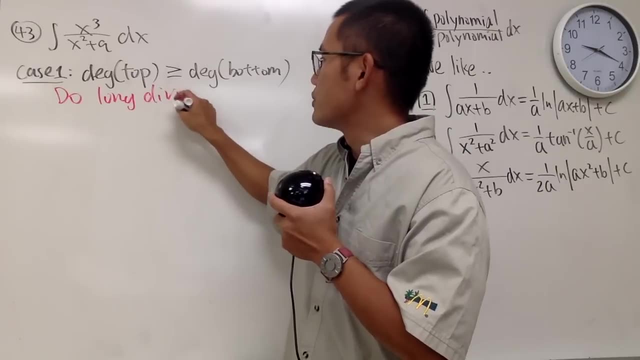 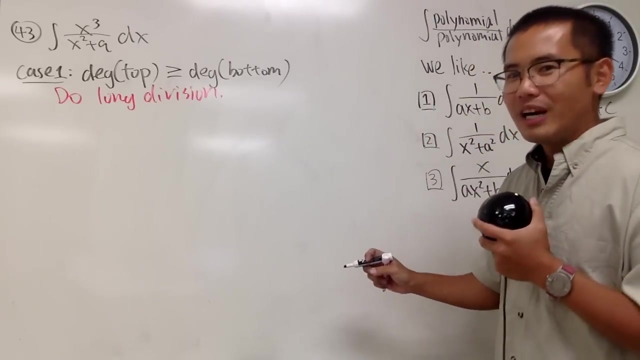 Right. In this case, what we are going to do is, I'll just say, put it down right here. We are going to do long division, Polynomial, long division, Right? Yes, In this case, when you have an improper fraction, such as 17 over 3, well, what do we do? 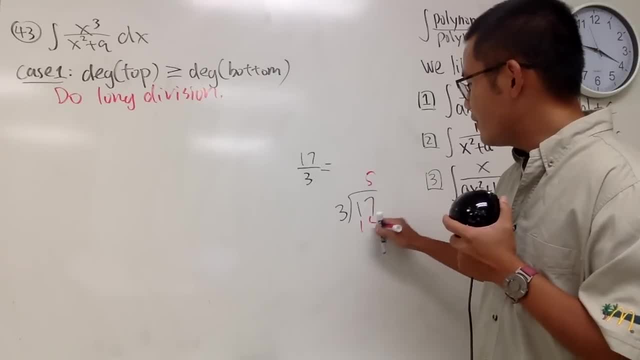 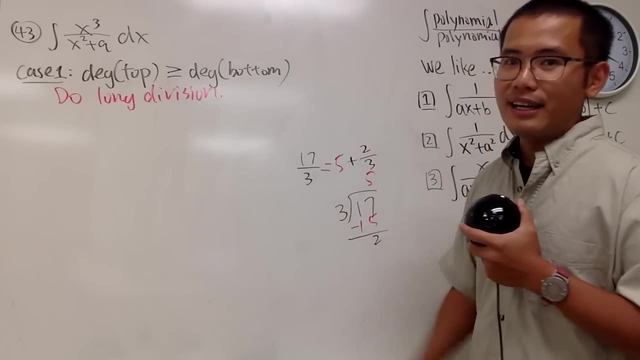 17. inside 3. on the outside, 5 times 3 is 15, minus that you get 2. And you can get 5, and you can get a proper fraction plus 2 over 3.. That's the idea. 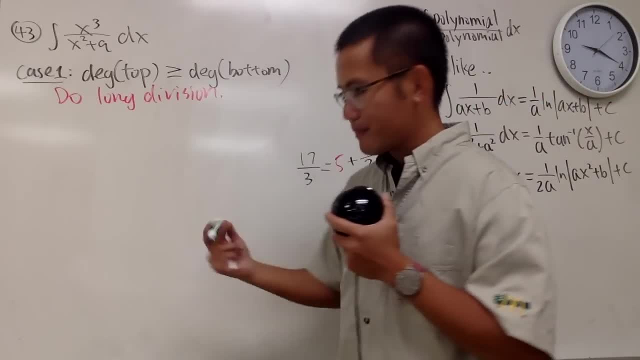 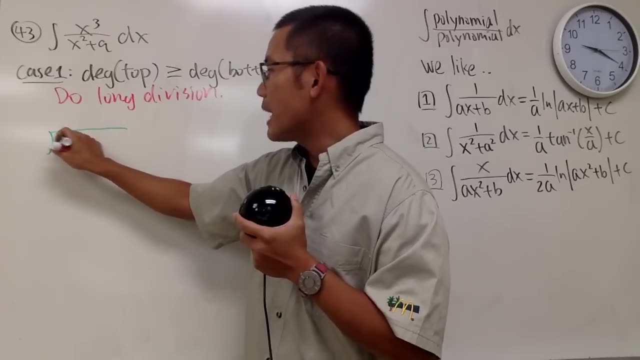 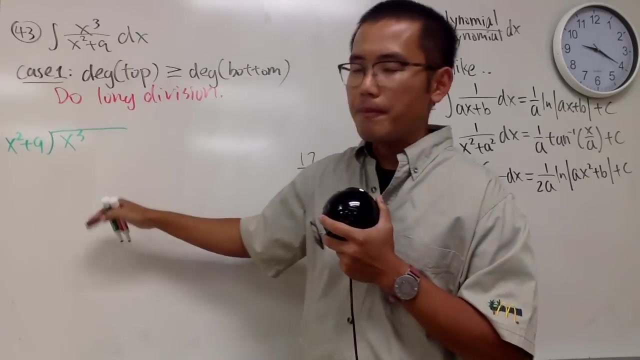 We do the same right here, right? So I'll do this in green and red Christmas color. Here we go. This is how you do it. Put the top inside, just like how we did it over there. You have x squared plus 9 on the outside. 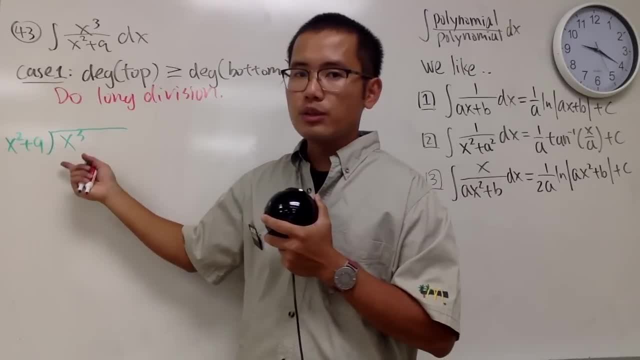 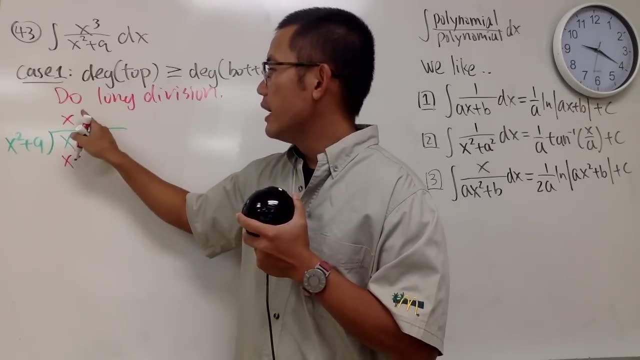 Now you have to ask yourself what times x squared will give us x to the third power, And the answer to that is just x. We need the x x times. this is x to the third power, and don't forget to do this. times that which. 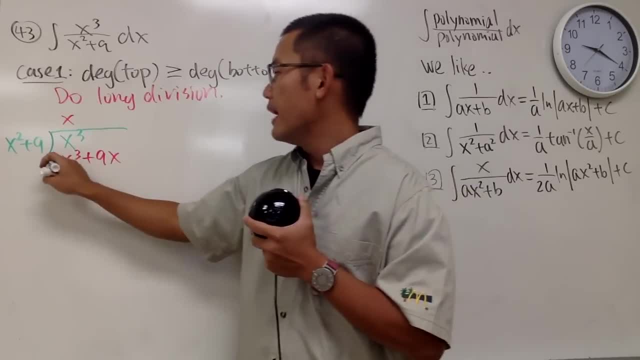 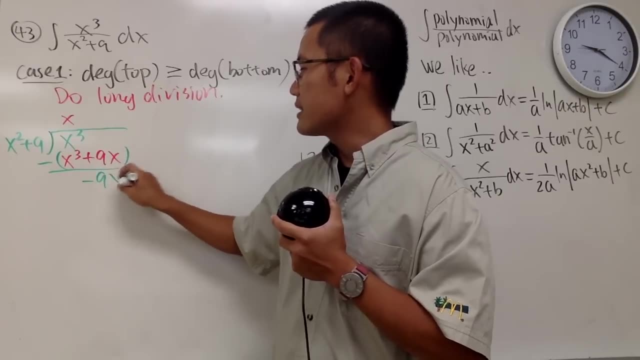 is plus 9x. Okay, And then we are going to subtract This minus that is 0. 0, minus that is negative 9x. That's it. When the degree right here is lower than the degree right here, we have to stop. 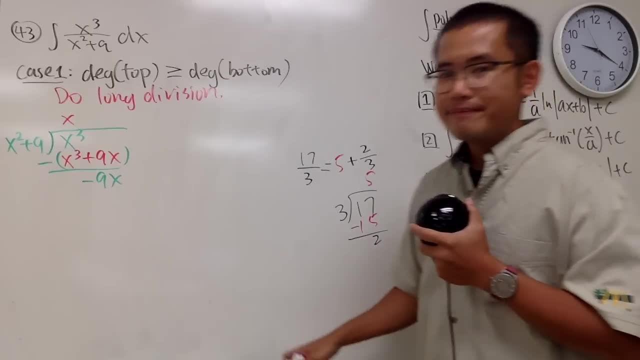 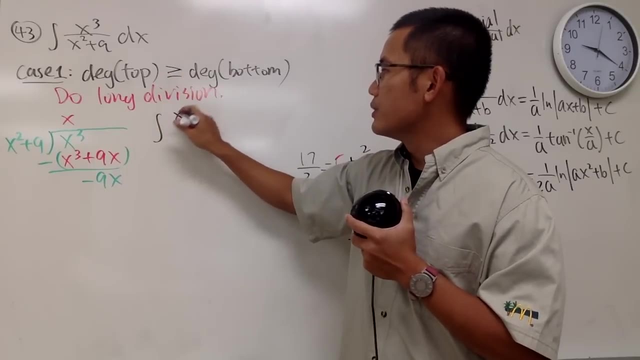 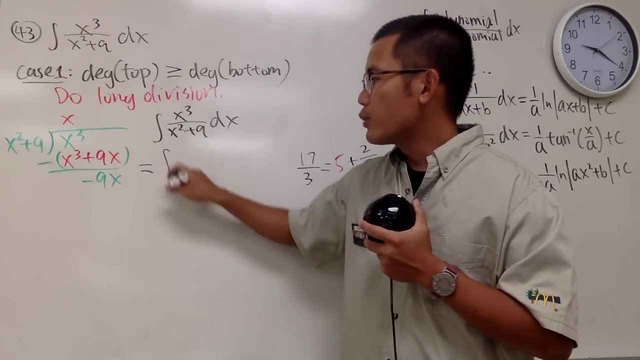 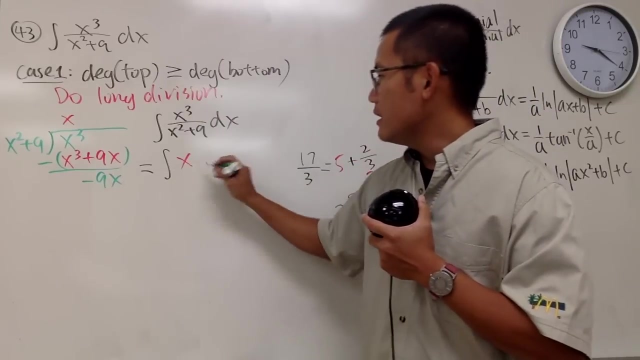 Just like the number right here is smaller than that, we stop. Okay. so here is the idea To integrate x to the third power over x, squared plus 9. now this is really the same as integrating x, And we are going to have the minus 9x. 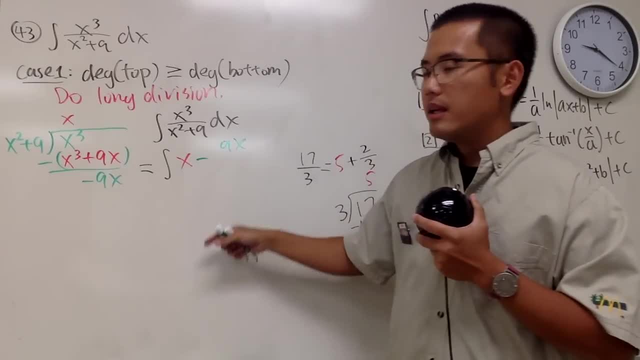 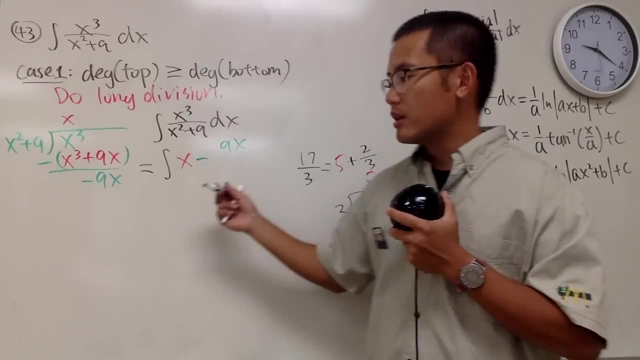 This is the remainder and you just put that on the top. Technically it's plus, but plus negative is negative right here, And we are going to divide it by the original denominator, which is the x squared plus 9, like this: dx. 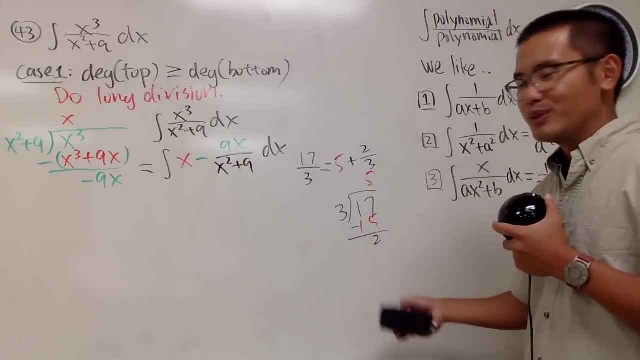 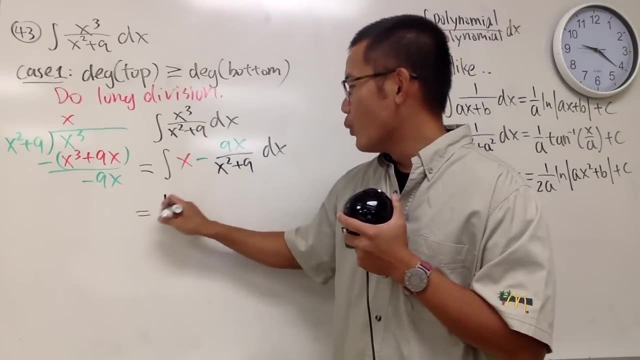 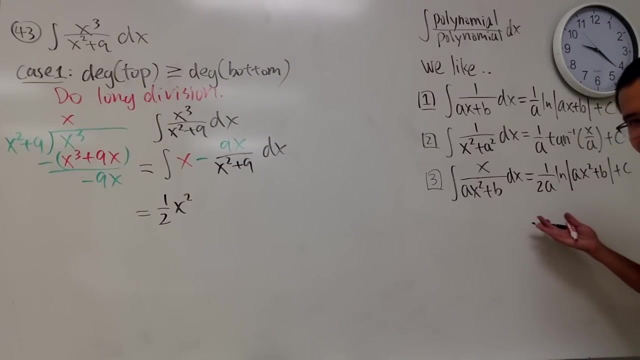 Let me just erase this right here already. When was the last time you guys did this by hand? Okay, We can totally integrate this, because when we integrate x, we just get 1 half x squared. And now to integrate this, perhaps let me just show you my fancy formula. 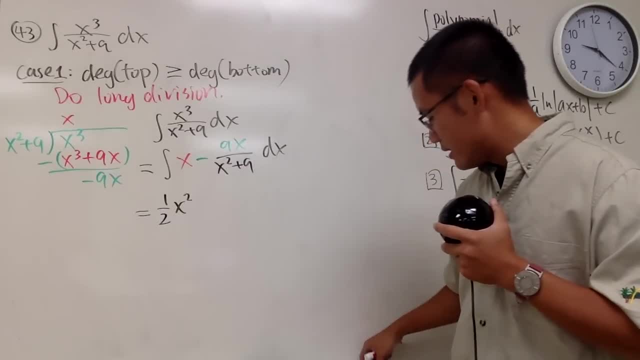 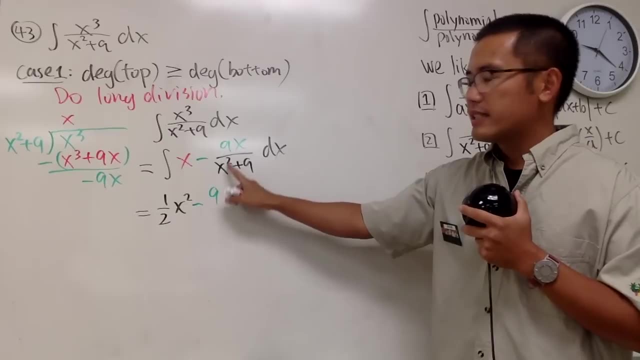 Minus is the minus, so let me just put down the minus 9 right here, Minus 9.. So we are looking at x over x squared plus 9, which is this formula: x over 8x squared plus b. 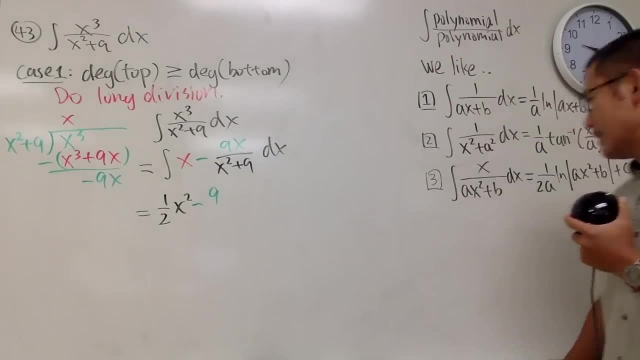 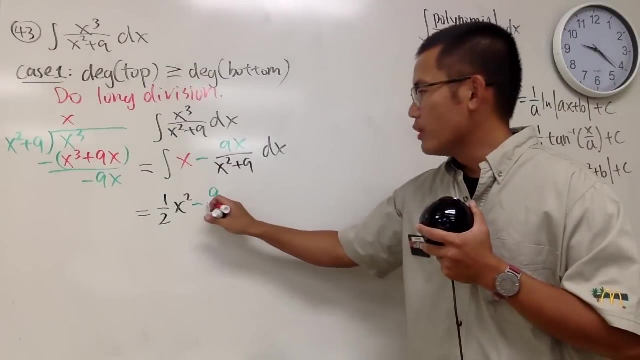 8.. In this case, it's just 1.. Yeah, So the answer for this part is 1 over 2a. Well, that will just give us 1 over 2 times 1, which is just 2.. 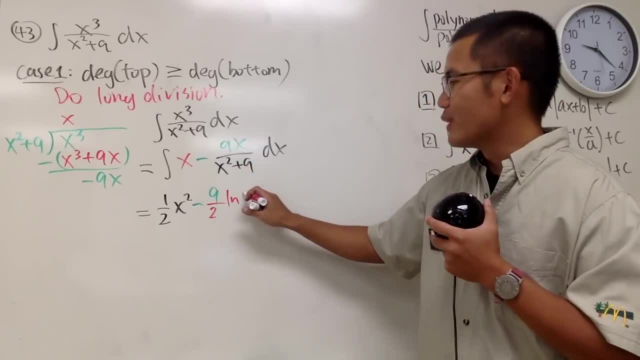 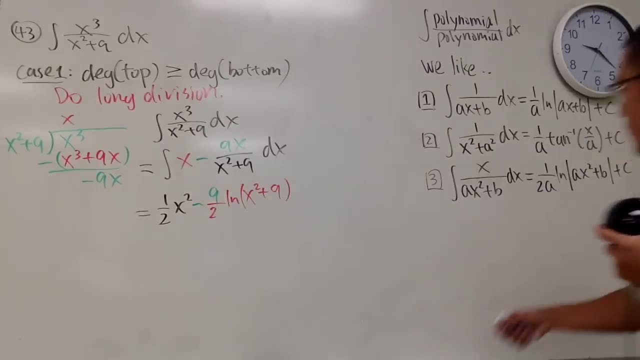 And then natural log, and this is actually always positive. so we have x squared plus 9.. Parenthesis is enough, because we know x squared plus 9 is always positive. This, right here, I put in the absolute value, because sometimes a and b may be negative. 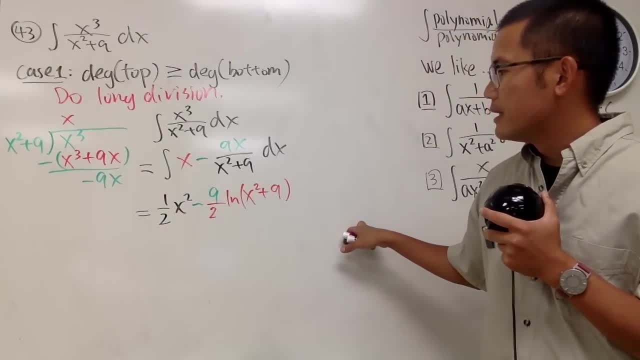 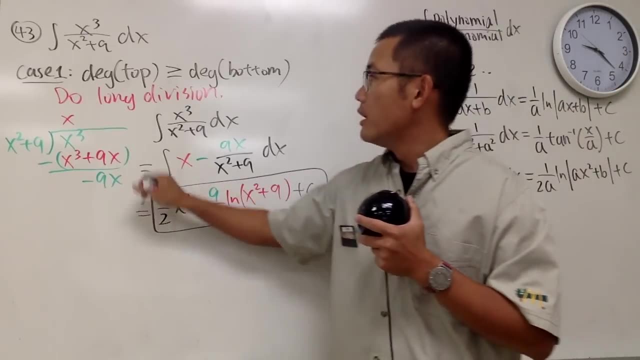 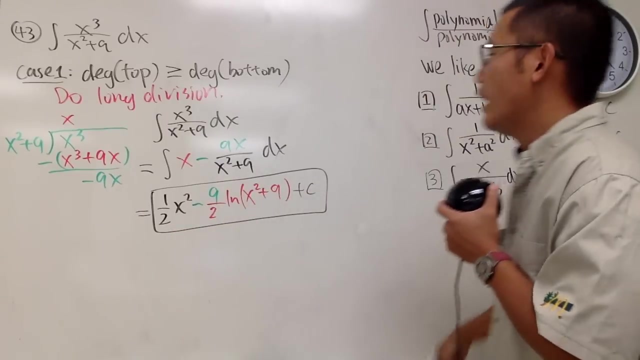 so we don't know. Yeah, That's it, So done. Case 1. If the degree on the top is bigger than or equal to the degree on the bottom, go ahead and do long division and you will be able to get to one of these. 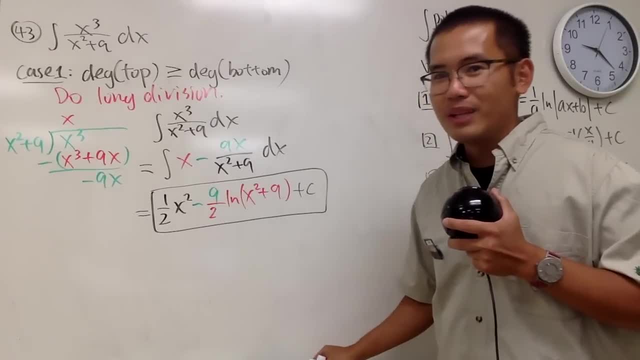 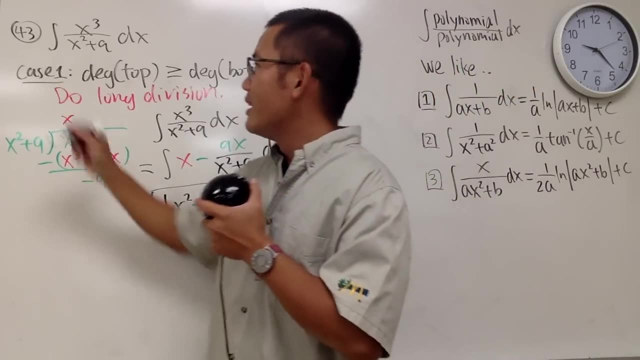 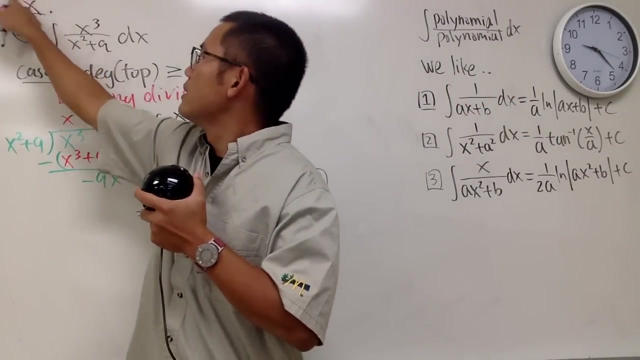 or maybe two of these, and also the regular powers that we like to integrate, etc. etc. etc. Okay, Okay, Here is the last category, The last category, As you can see, the things that we were doing, the things that we were doing. this is supposed to be number 10, Roman numeral right. 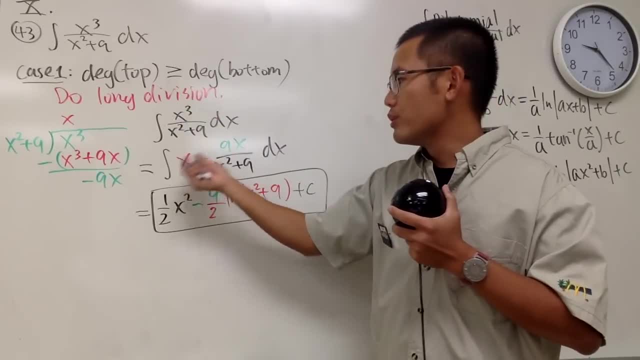 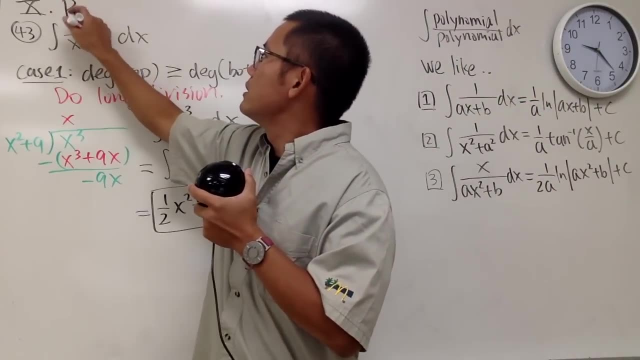 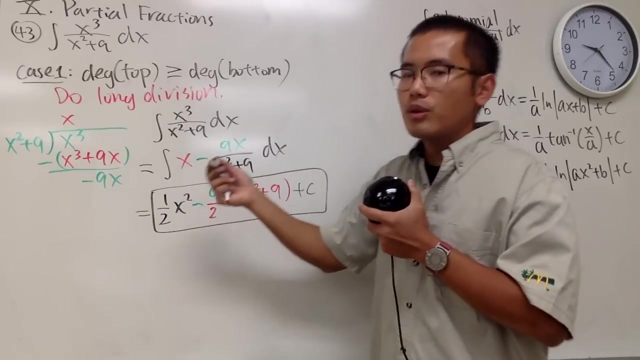 The thing that we did is we have a fraction and we broke it down into two fractions, a fraction in the algebraic sense. okay, This right here it's called the partial fractions, And sometimes this is also called the partial fractions- decomposition. 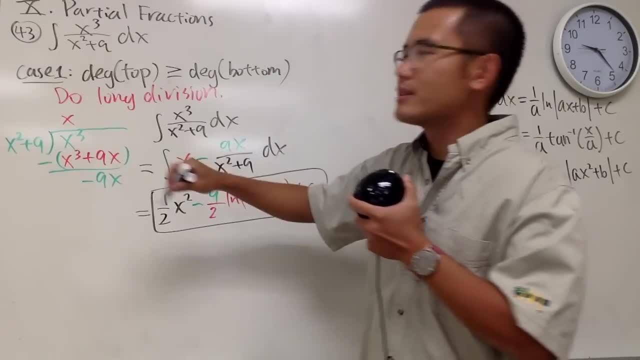 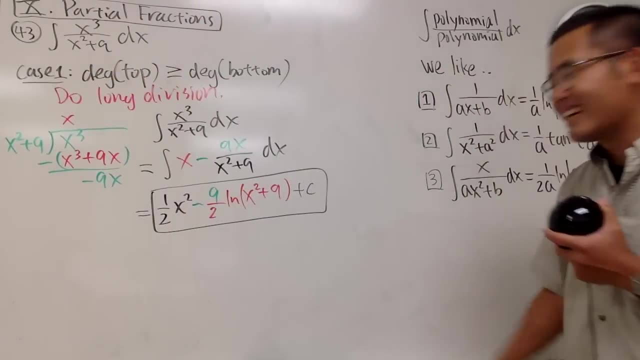 So let me just, let me just keep it like this: Partial fractions right here. Decomposition just means that you break it down, that's all, Yeah, So partial fractions like that. I'm going to leave this on the board, just for simplicity, just for benefit for us. 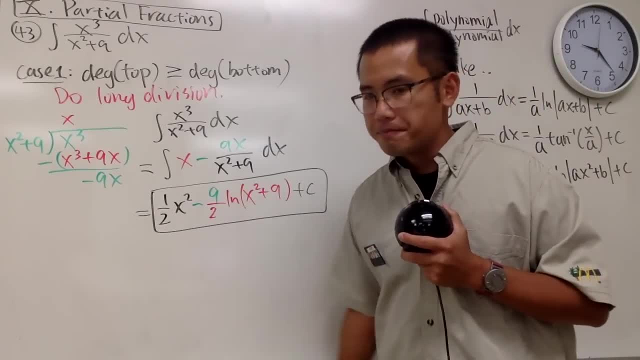 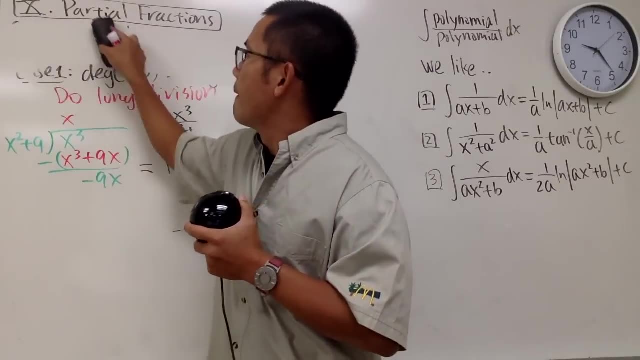 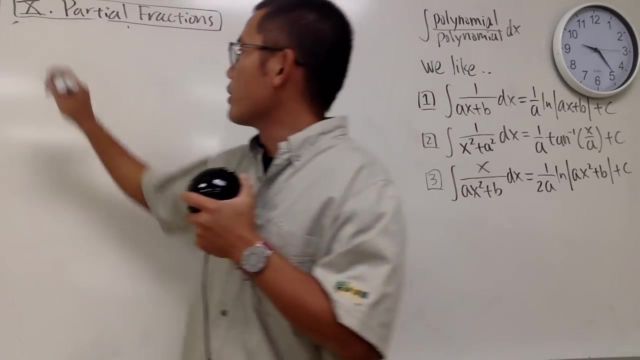 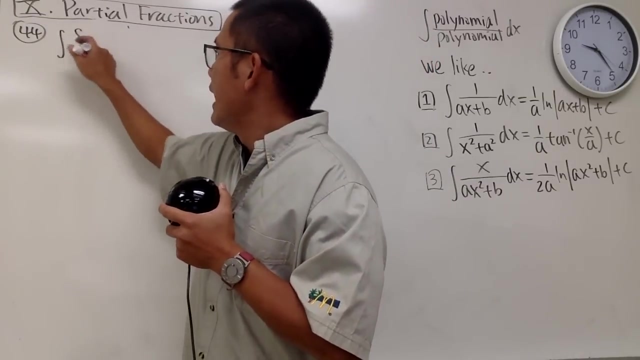 You know that. So case 1, right here Now I'm going to demonstrate case 2.. Huh, Case 2, name the equation number 44. And here we have integral of 8x minus 17 over. 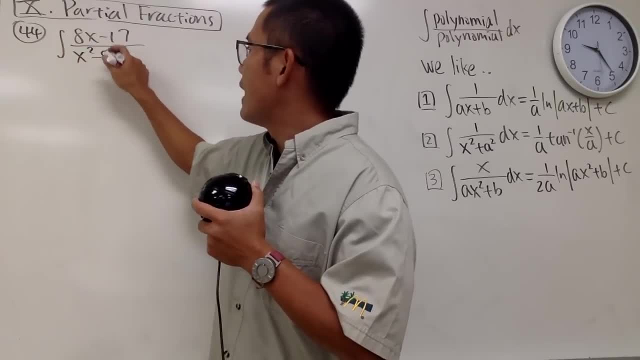 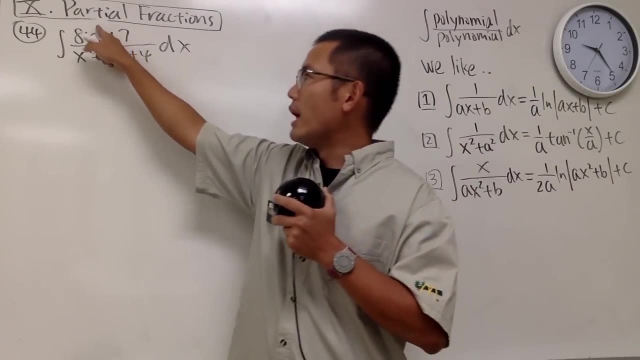 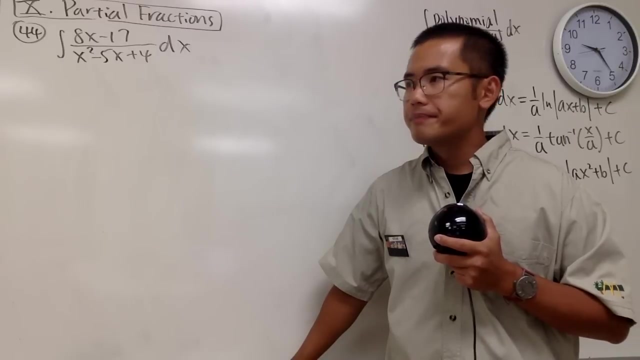 and we have x squared minus 5x plus 4 dx, like this. Now, degree on the top is 1.. Degree on the bottom is 2.. We don't need a long division. Well, what do we do in this case, though? 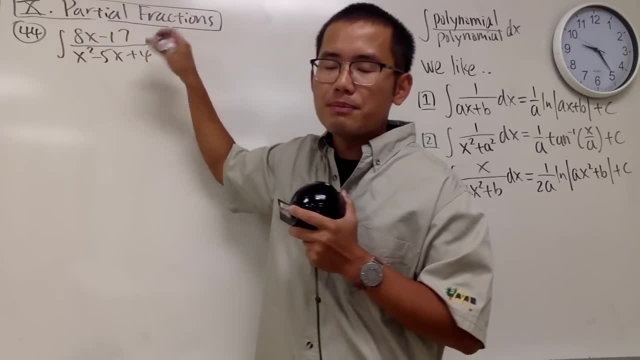 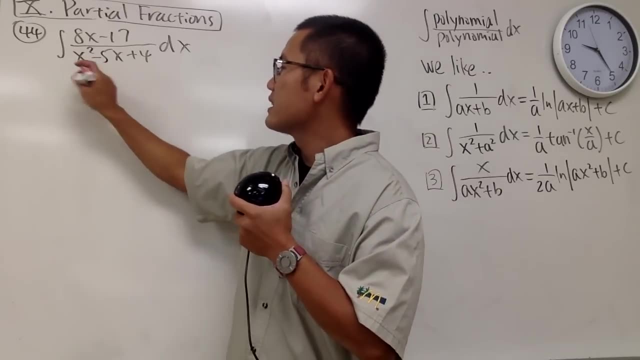 Okay, Focus on the bottom: x squared minus 5x plus 4.. Back in algebra. what did you guys used to do? Just factor it, yeah. And if we factor this, we get x minus 1 times x minus 4, isn't it? 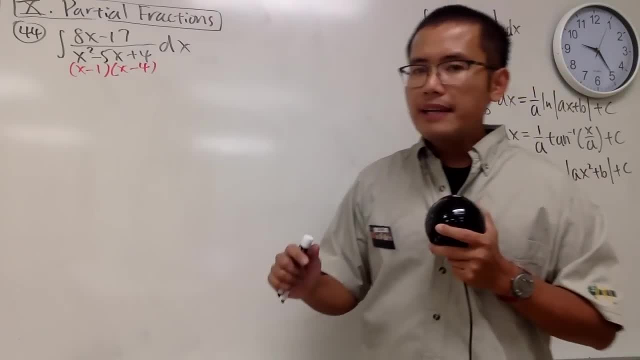 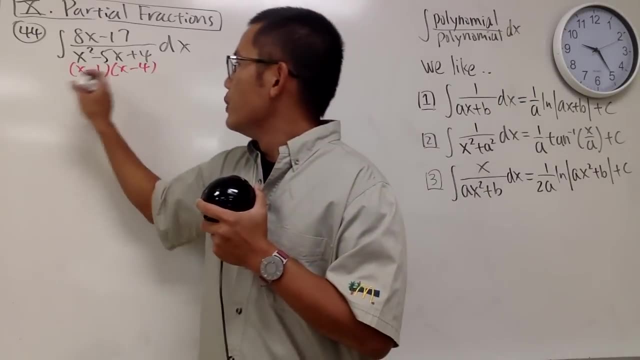 Yes, it is So, that's good. So case 2, we are going to categorize: What kind of factors do we get from the denominator? In this case, we see that we have two linear factors and they are different. 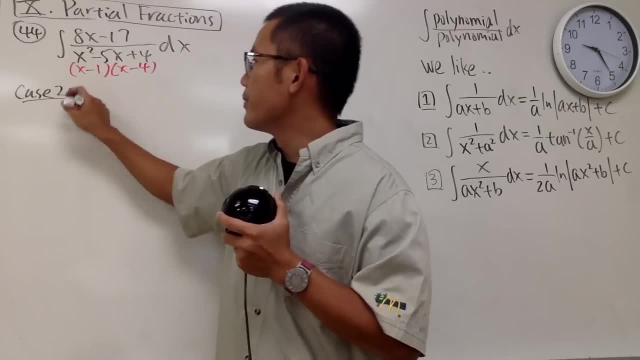 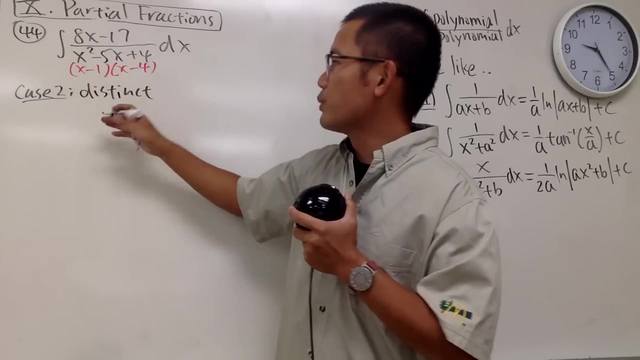 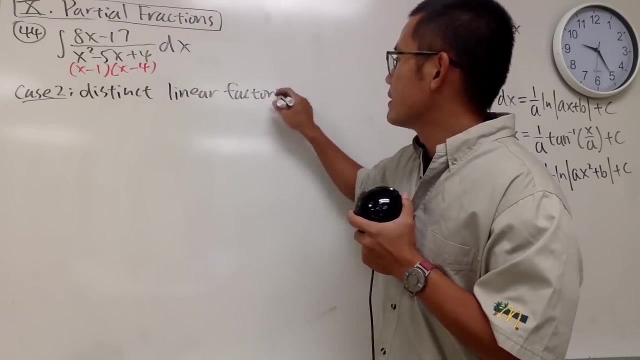 So that's the second case, Case 2.. We see right here this, right here is the, I'll just say distinct. I don't know why math people like to use the word distinct. It just means different, Distinct linear factors, right. 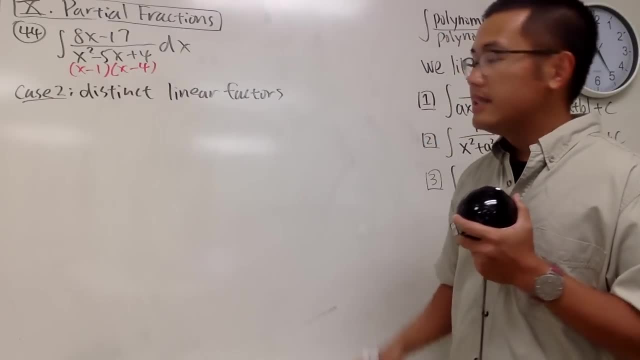 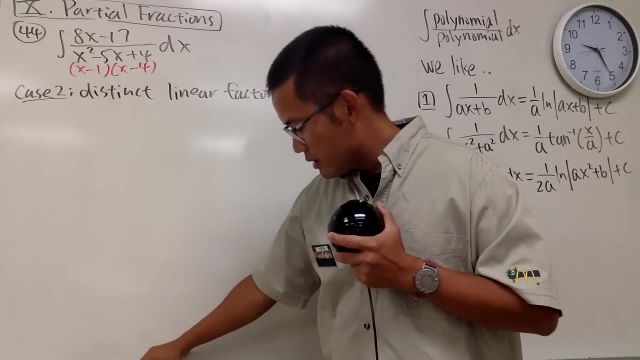 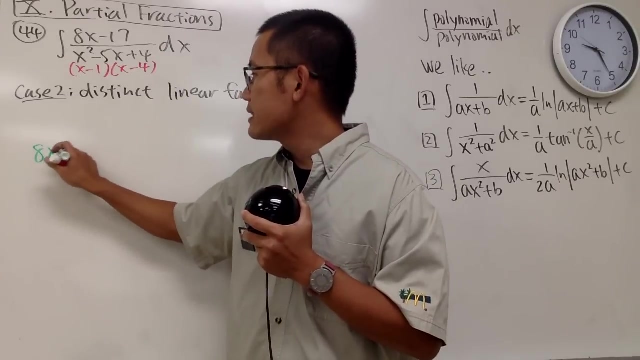 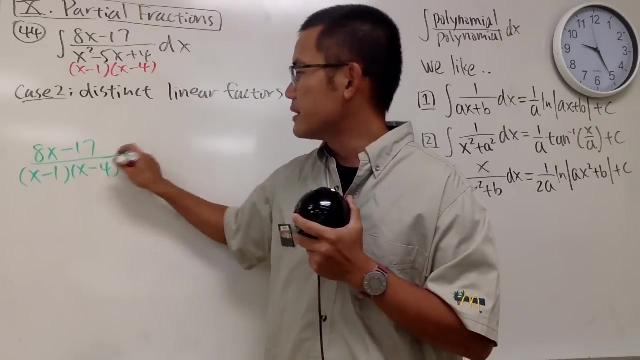 Distinct linear factors, And this is how we can break the fractions apart. Let me show you. Let me just do this in green again. So let me put this down, And this time I'll just write down 8x minus 17, over parentheses: x minus 1 times x minus 4, like this: 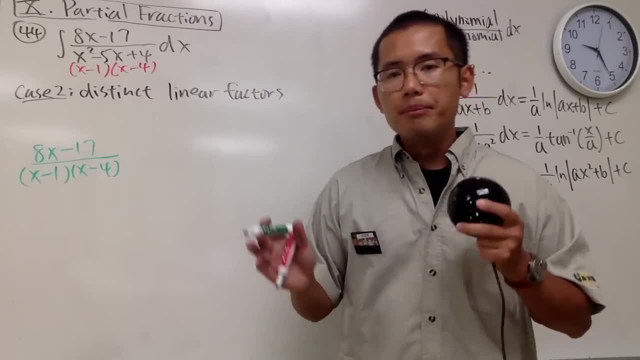 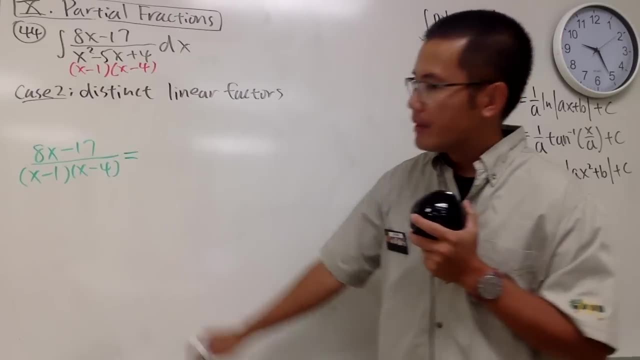 Keep in mind of the setup. The setup is the most important part, Because if you don't have the right setup, the whole thing would be messed up. So here is the idea. We have two different or distinct linear factors. 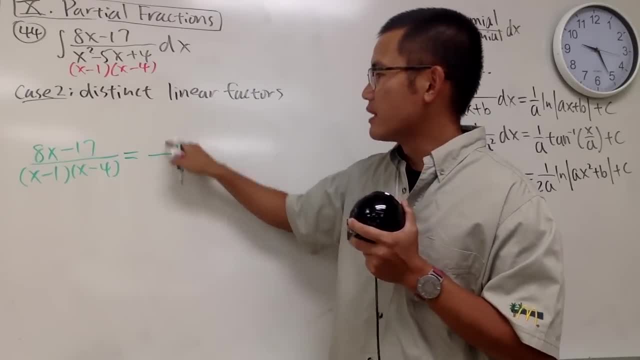 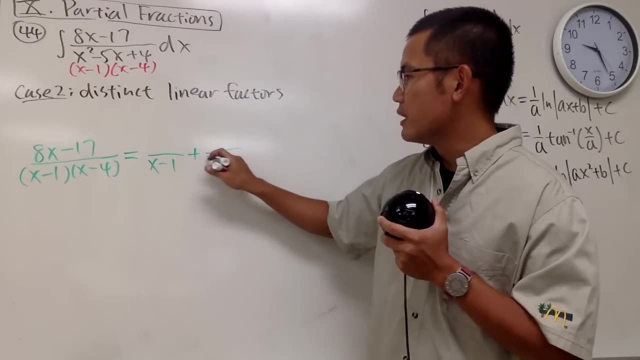 The first one, we are going to be able to write it as something over x minus 1.. And the second factor is going to be plus, combined with the second one, which is x minus 4.. Right, And you might think: what are we doing exactly? 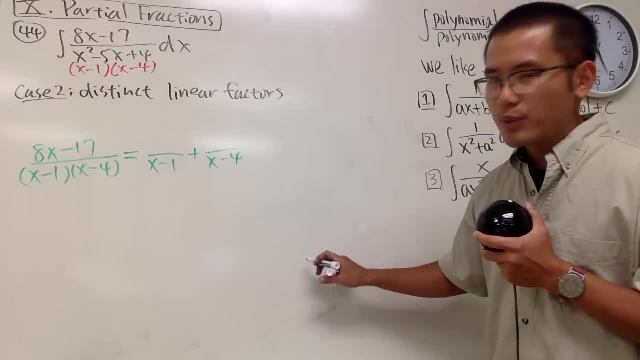 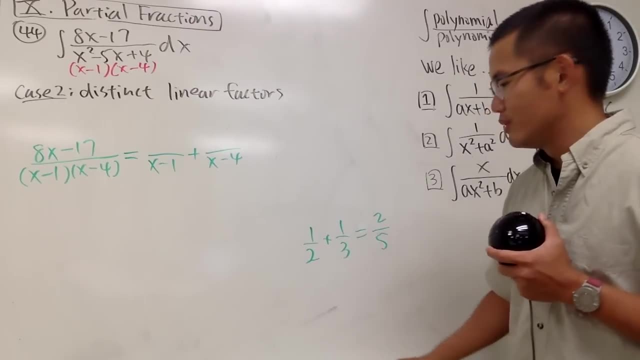 Let me give you an analogy. Imagine the good old days when you are doing 1 half plus 1 third, The answer is 2. fifth, Yeah, No, Just kidding. Haha, That's the most common mistake, right? If you first see fractions. 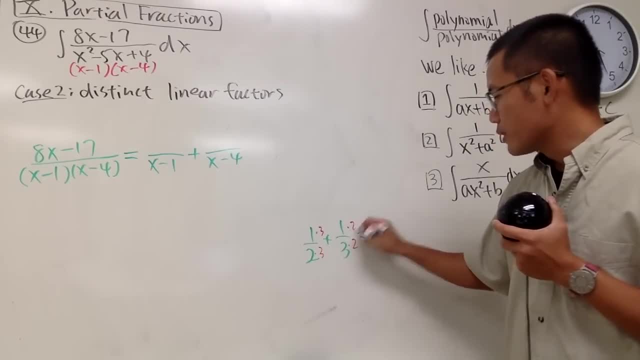 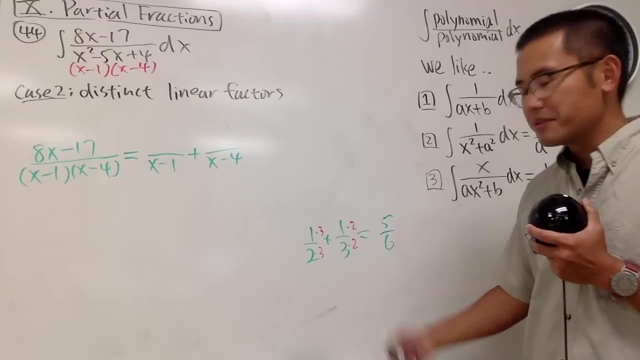 But anyway, you can get the common denominator multiplied by 3, multiplied by 3, multiplied by 2, multiplied by 2.. 5 over 6.. We can add fractions, of course. This is a legitimate way to do it. 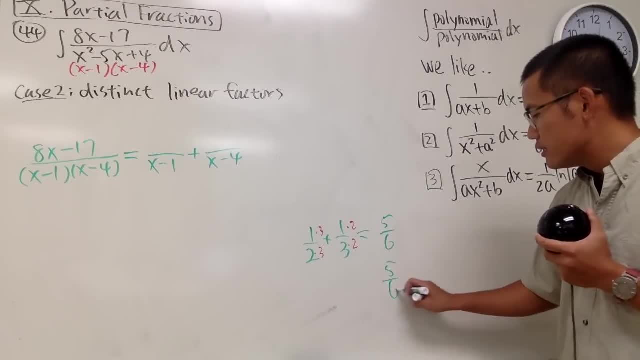 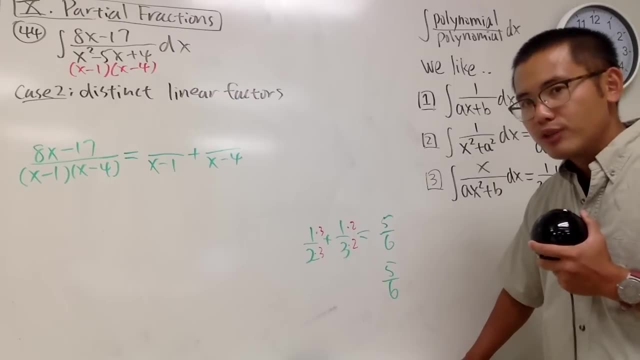 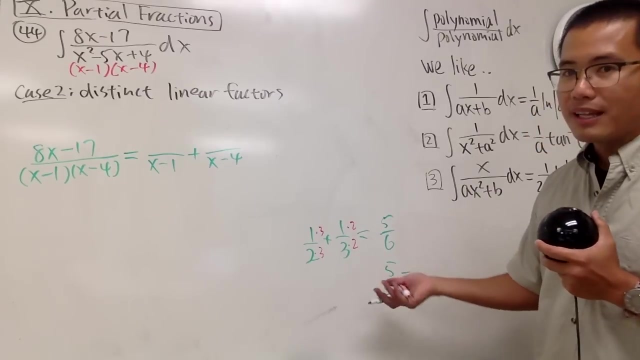 But if the question is: is the other way around: If I give you 5 over 6, can you give me 2 fractions that add up to 5 over 6?? Well, by knowing this, we know it's just going to be 1 half plus 1 over 3.. 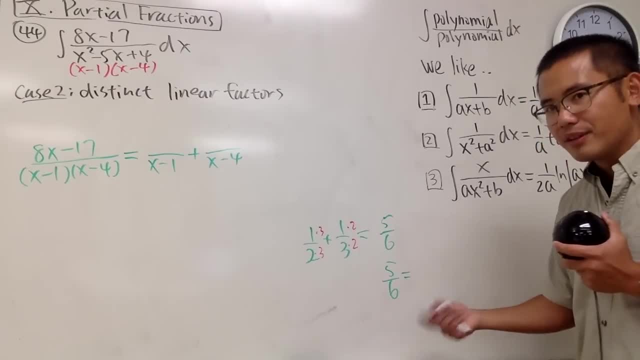 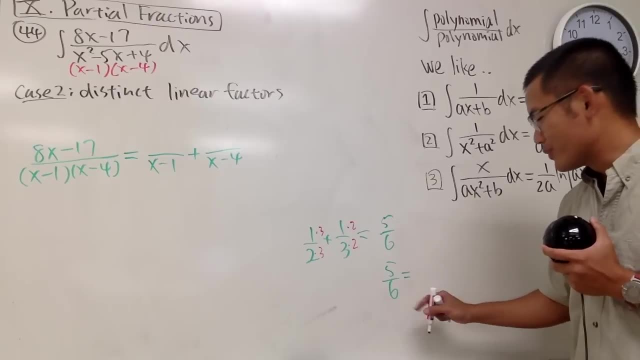 But another way to do it is, of course, let's have the different denominators. Otherwise you can look at this as 1 over 6 plus 4 over 6.. That's not fun. You can look at the 6 as 2 times 3.. 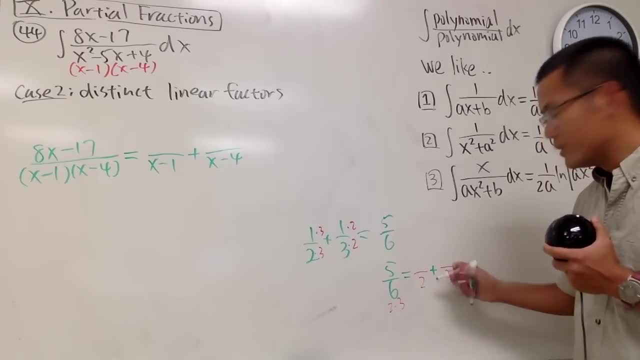 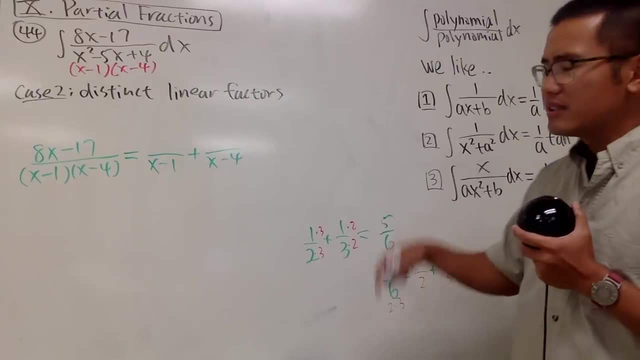 And you can look at this as something over 2 plus something over 3.. In this case, this is slightly more interesting, And Yeah Right. So that's exactly what we are doing. We can also break the fraction apart, And when you have this right here, 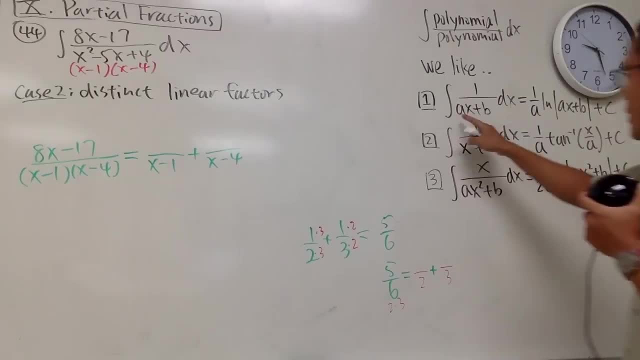 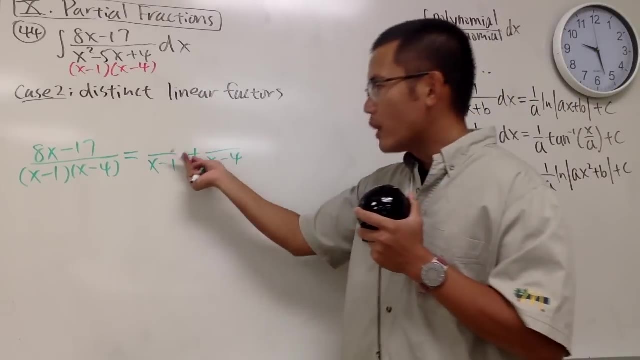 if you figure out what number this right here is. that's one case that we like. That's the idea of partial fraction. Anyway, I don't know what the number is on the top. Here is the idea. If the degree on the bottom is 1,. 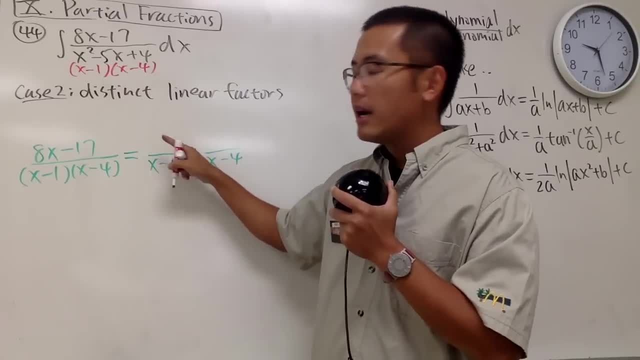 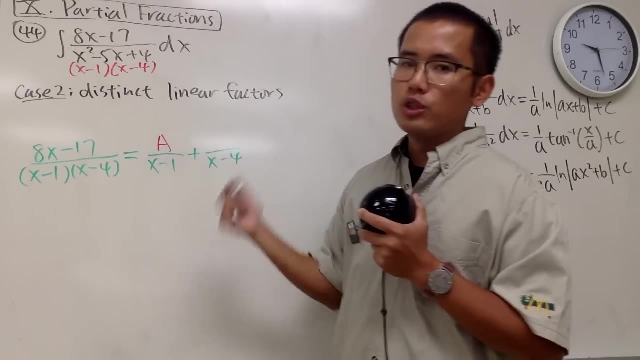 then the degree on the top has to be 0.. The degree on the top has to be 1 less than the degree on the bottom. So this is linear. On the top it's just a constant And traditionally we just put down A. 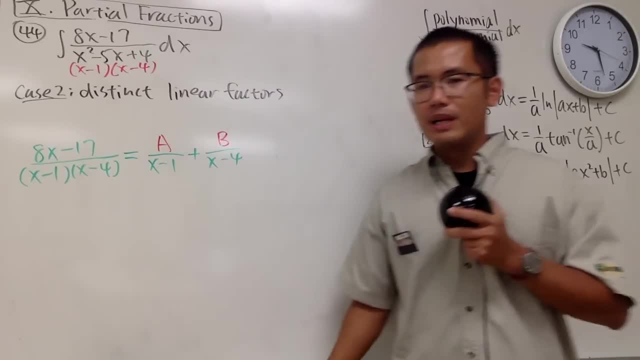 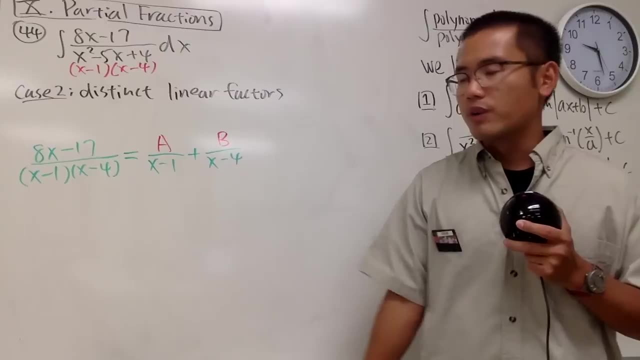 Right here. I don't know what this is. Put down B And then we'll find it out. Now let me show you guys the fastest way to do this, And we'll do all the work first. This is how you are going to do this. 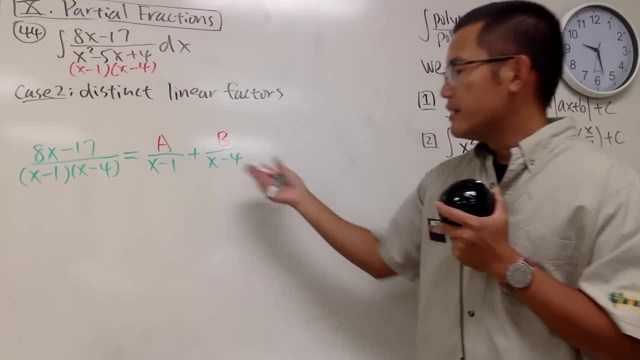 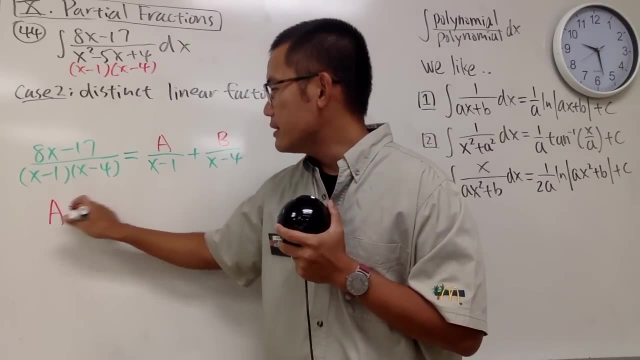 when you have distinct linear factors, Right, And you can extend this to 3 or 4 different factors- Same idea. Anyway, I will show you guys how to figure out what A is really. really quickly, Look at A If you want to look at A. 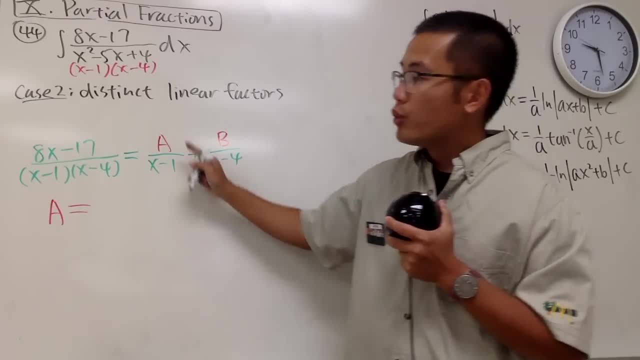 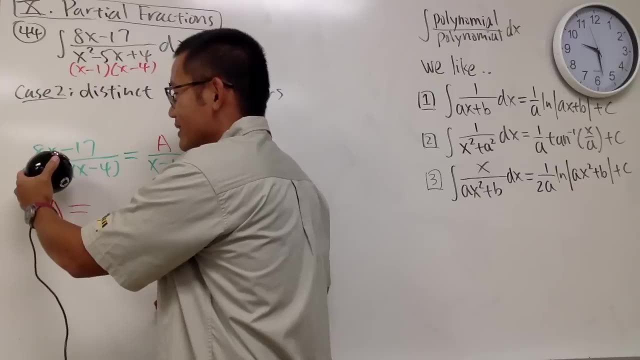 look at the denominator, which is x minus 1.. You go back to the original and you are going to use your both hands. You are going to cover up the x minus 1.. You are going to cover this up. You have to use two fingers. 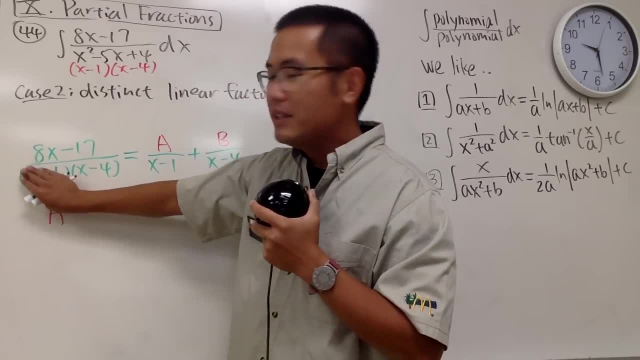 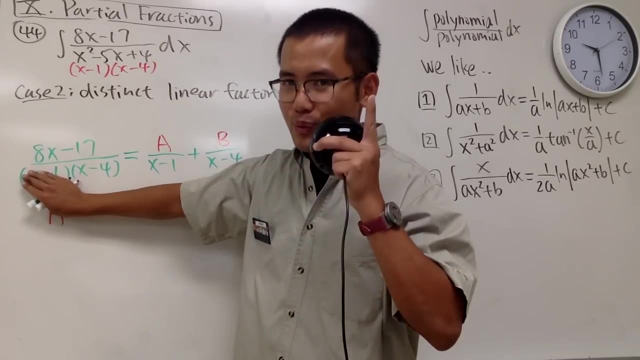 I have to use my two hands, alright. And when you cover this up, you have to ask yourself: how can you make x minus 1 equal to 0?? x has to be what x has to be 1.. So I will let x equal 1.. 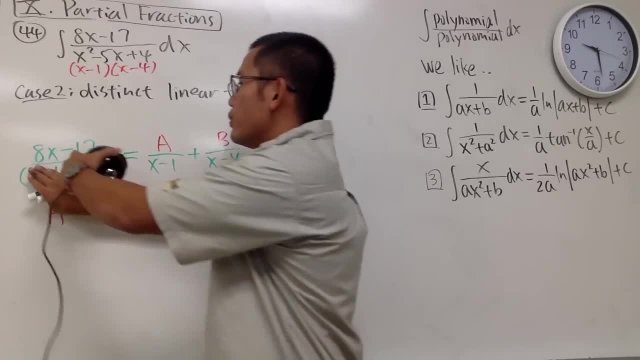 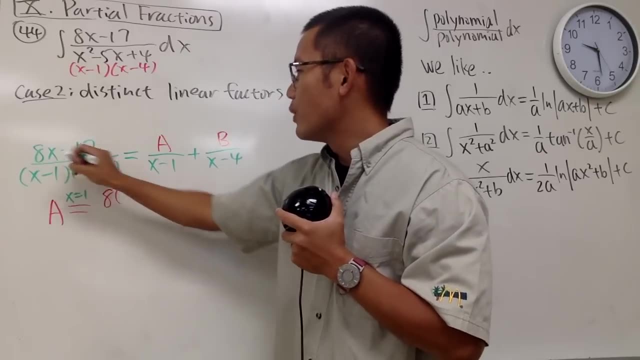 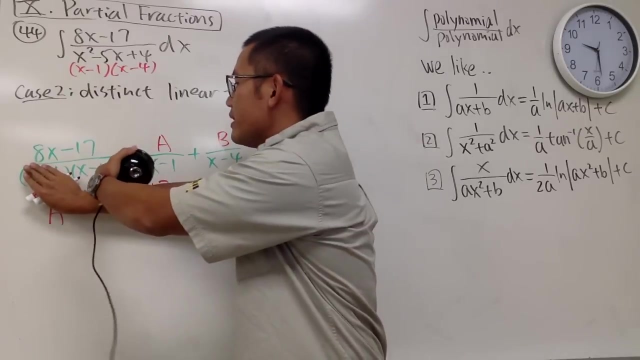 And I will be plugging x equal 1 into here and here, And then that will be the perfect way. Let me write it down: We have 8 times 1.. And then minus 17 over putting 1 in here. So we have 1 minus 4, like this: 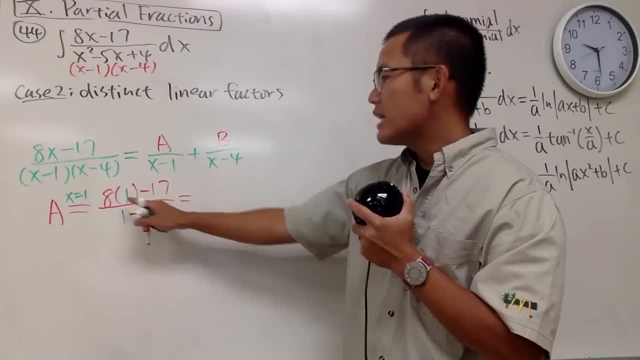 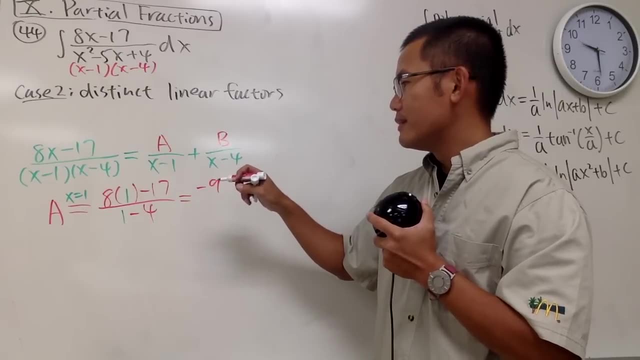 And of course now it's just a matter of computing it On the top, is 8 minus 17, is negative 9,, I believe. Yes, Over negative 3. And that should be equal to 3.. Yeah, That's it. 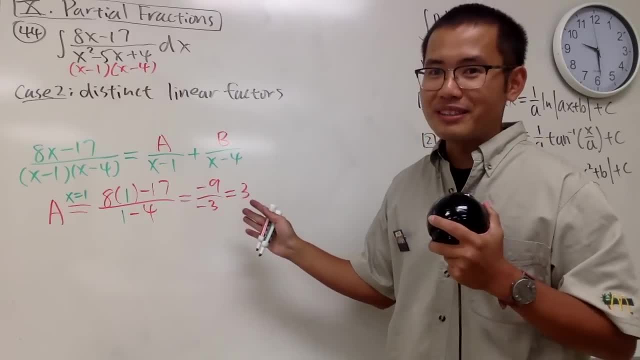 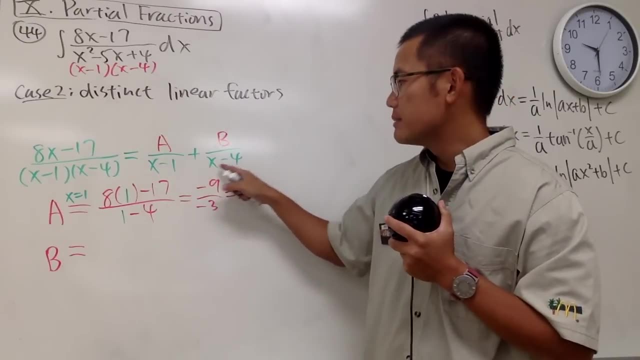 Now I know, Don't worry, We'll do another example, which is the b, To figure out what b is. well, the denominator for b has x minus 4.. We go back to the original. We cover up the same exact denominator. 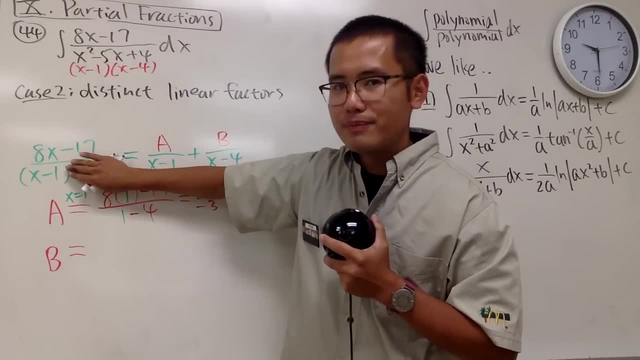 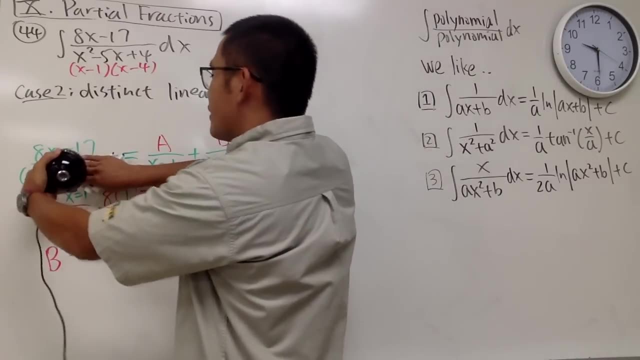 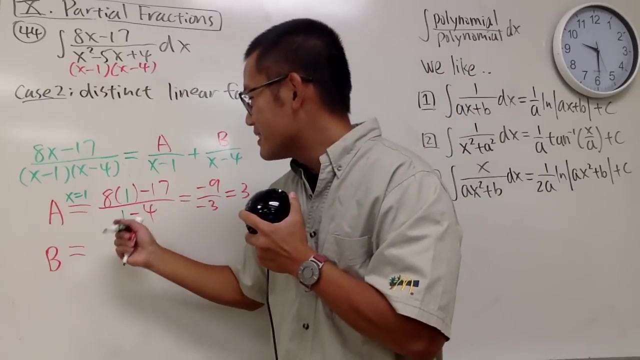 And how can we make x minus 4 equal 0? Well, x has to be positive 4.. Then we put in the 4. 4. Into here and here, And then just work it out. Yeah, So we will just say x is equal to 4.. 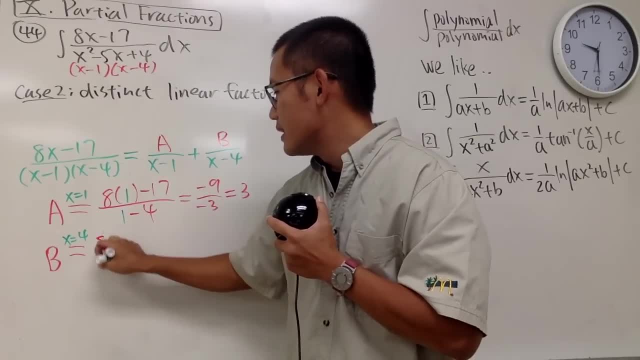 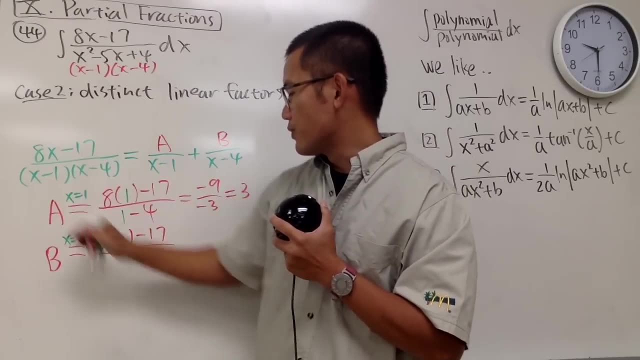 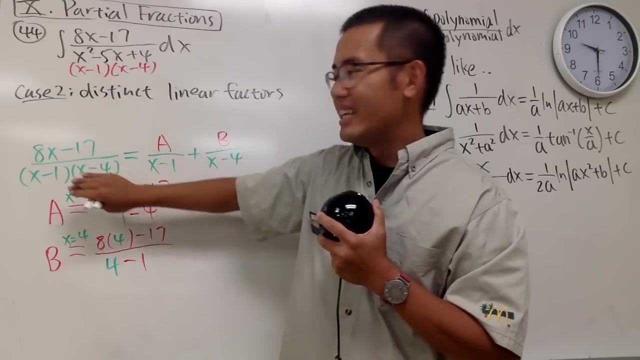 Put it here. Put it here, So we have 8 times 4 minus 17. all over, This is 4 now, because x is 4.. And then minus 1.. And do not plug in 4 into here, because you covered this up already. 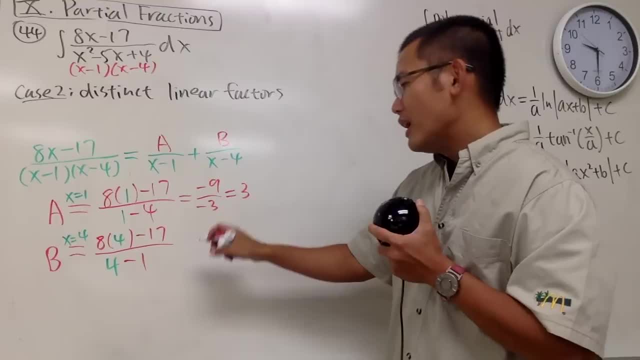 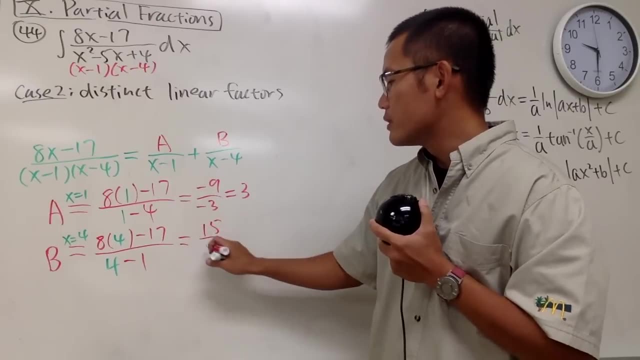 Right, This is called the cover-up method And we'll work this out. This is 32.. Minus 17 is positive 15 over 3,, which is 5.. And with that, a is 3, b is 5.. 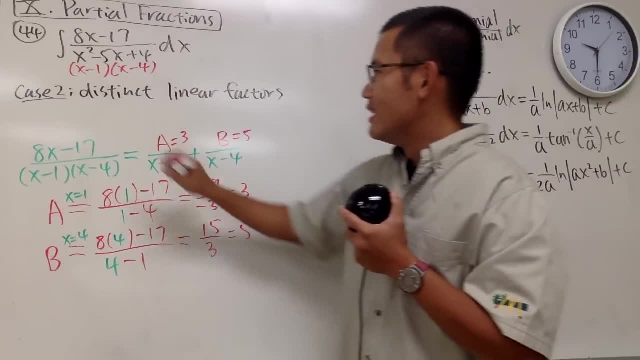 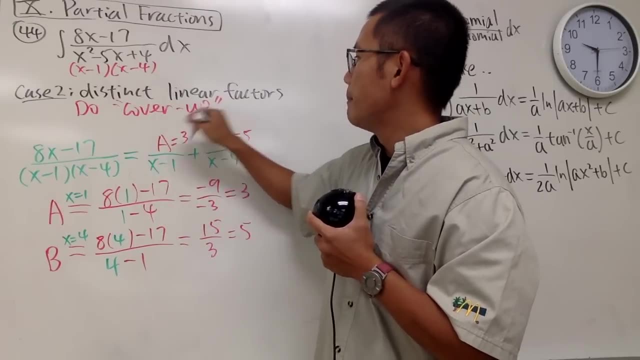 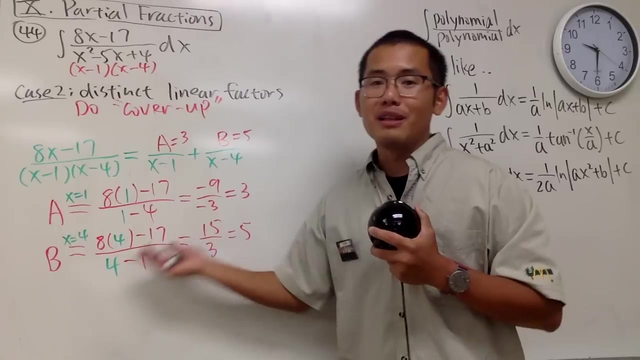 We are done Again. this is called the cover-up method. So I'll just tell you, guys, Do the cover-up method. This is the fastest way to do partial fraction And this is the amount of work that you have to show in my class. 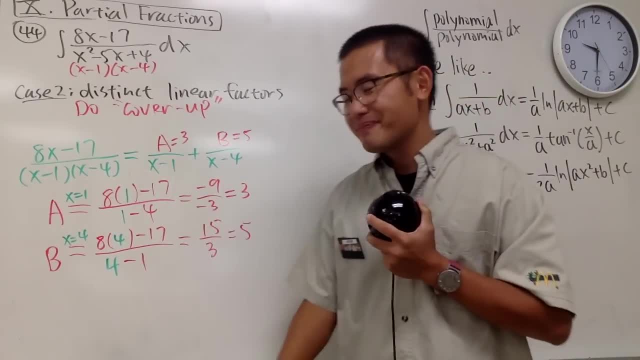 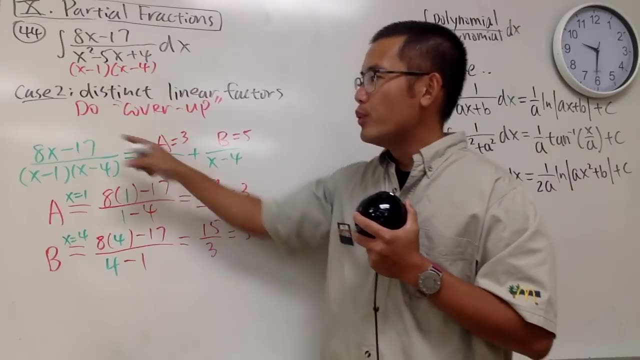 And if you are used to this, you can even do this in your head. Let me first convince you guys that these two are the correct numbers. If we add this up, we end up with this. Let me just convince you guys that real quick. 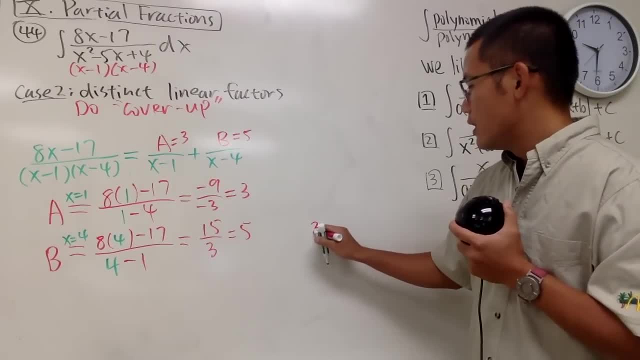 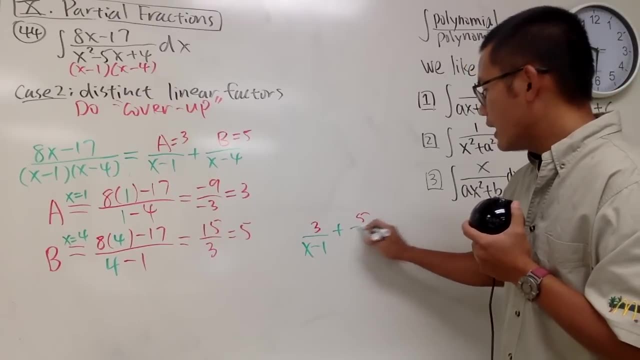 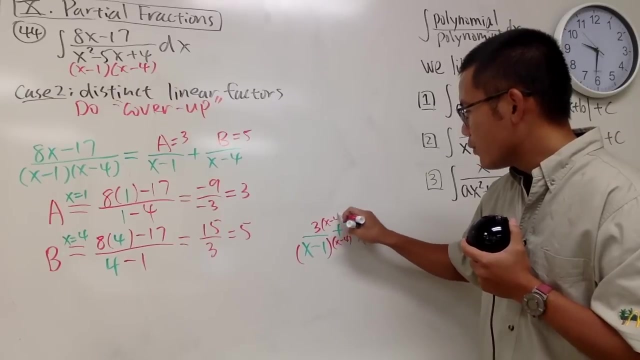 Yeah. So check this out: 3 over x minus 1.. Combine it with 5 over x minus 4.. Of course I have to get the common denominator, which is x minus 4, and then x minus 4.. And then for this one, 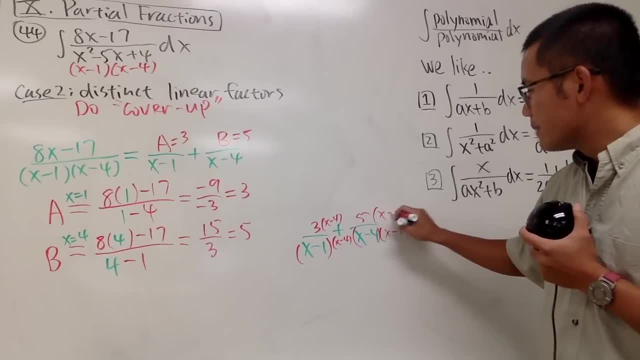 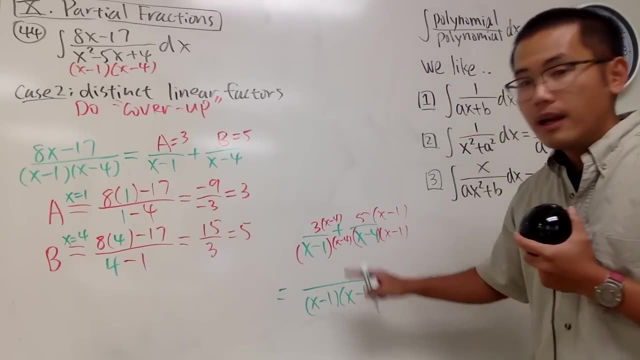 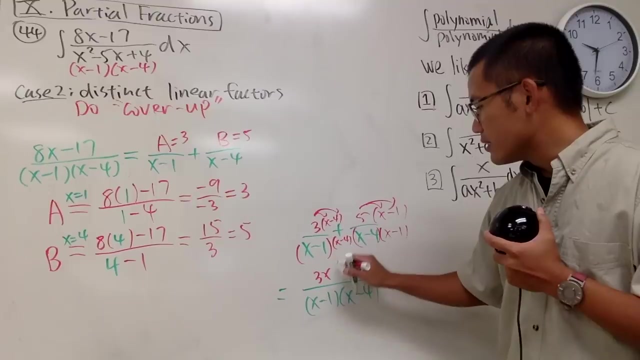 I need the x minus 1 and x minus 1.. And look, both of them will have the same denominator: x minus 1 times x minus 4.. On the top, distribute, distribute like this: This times this is 3x minus 12.. 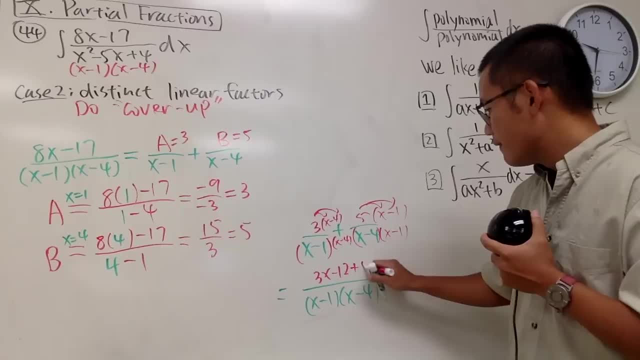 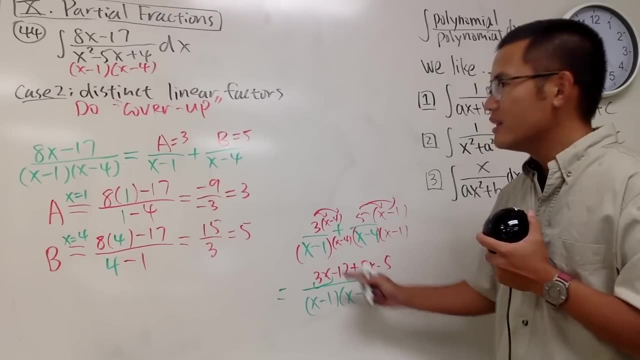 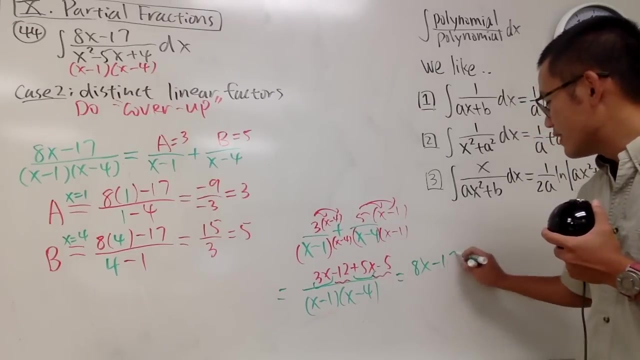 And this times this is positive: 5x minus 5.. This right here is 8x right, And then this right here and this right here is minus 17.. And you see that it works. We got the original fraction back. 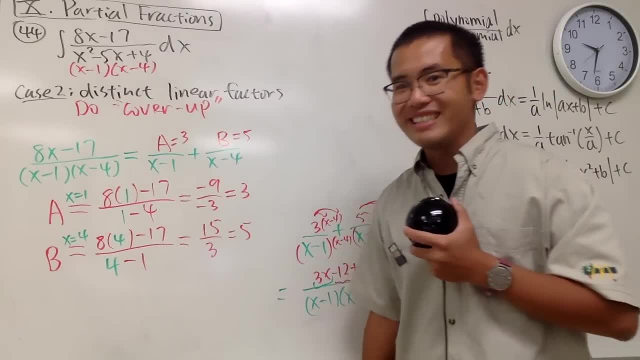 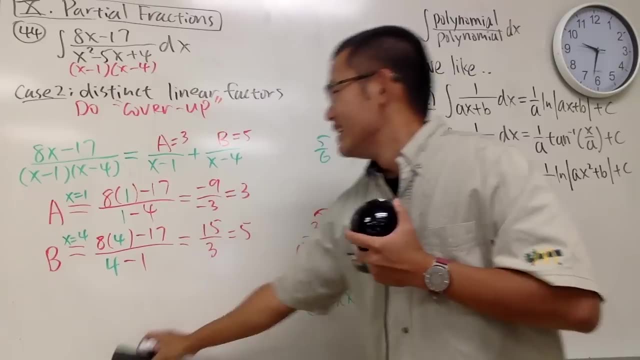 And in fact you have only one way to do it. when you are doing the algebra version of it For the number 5 over 6, you can find a lot of fractions. They add up to be 5 over 6.. But that was just an analogy. 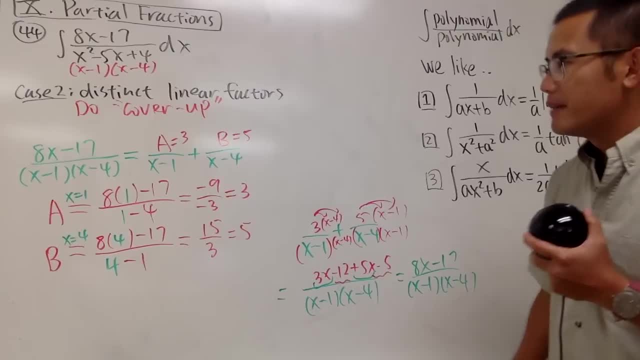 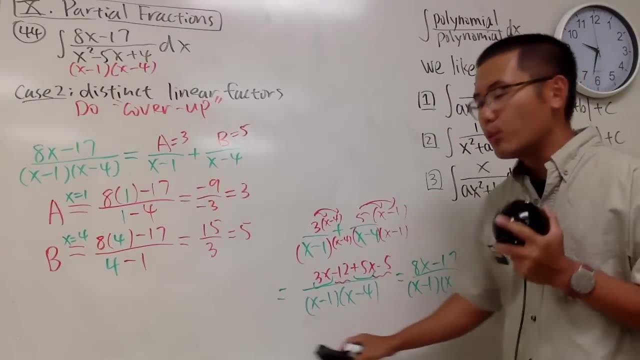 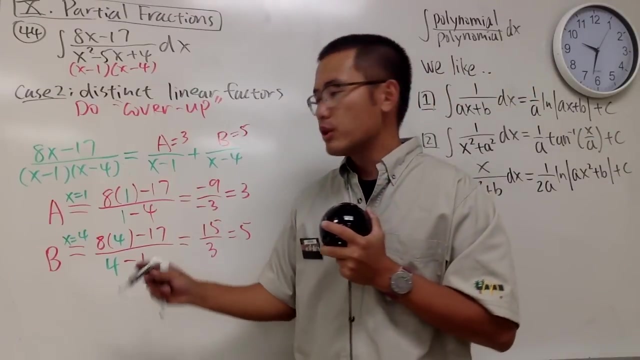 a quick analogy for it. Anyway, that's the idea, right, This is the Capra method and it works. Now let's talk about why it works. Here is the deal: Why we just multiply, sorry, why we just plug in: x is equal to 1. 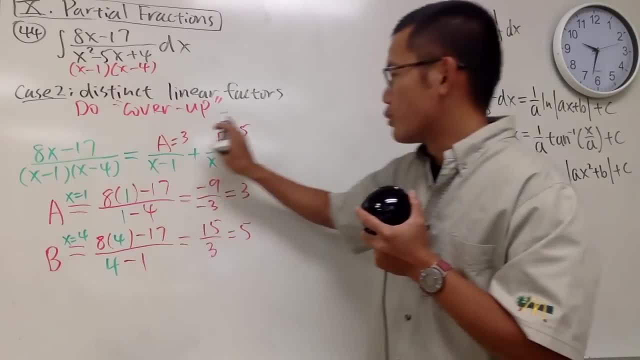 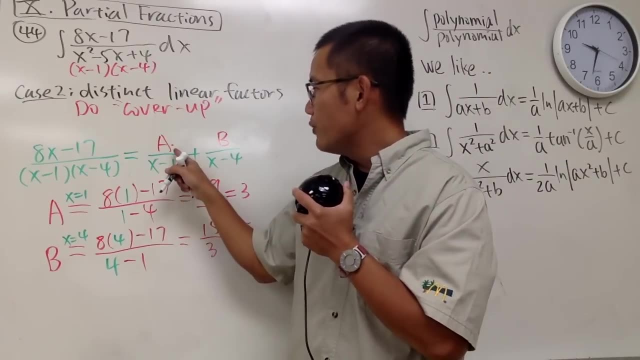 to solve for a. Look at this expression. Let me erase the a and b, because suppose I don't know? Well, if I want to figure out what a is, this is all I have to do. Let me work with this equation. 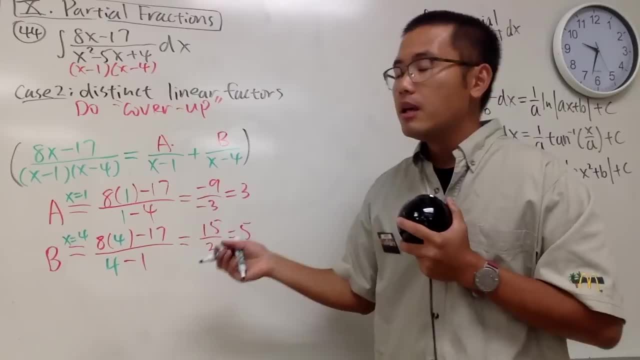 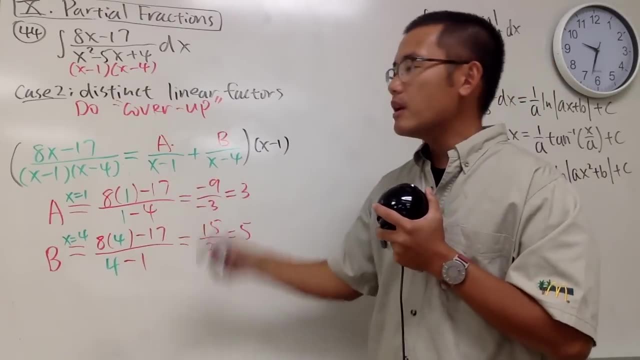 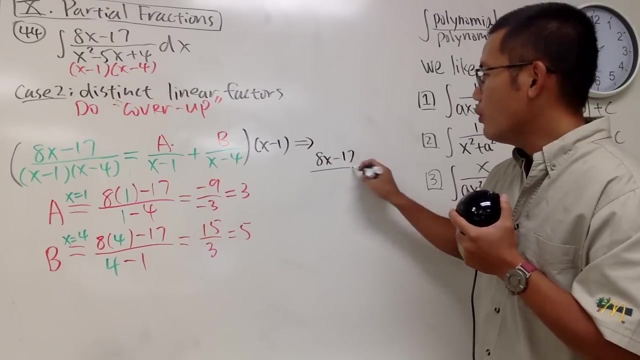 I will multiply everybody by the same thing, And let's just multiply everybody by x minus 1, so that I don't need to deal with that anymore. Okay, take this, multiply with this, We get 8x minus 17 over. 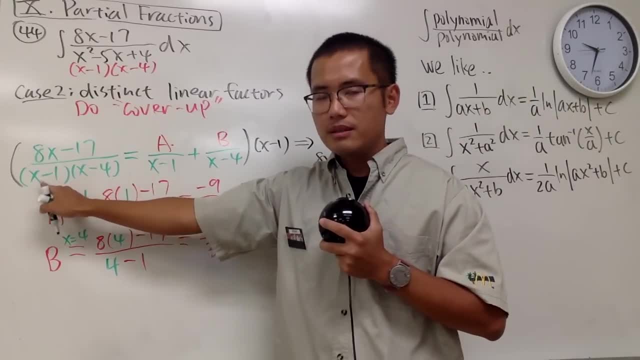 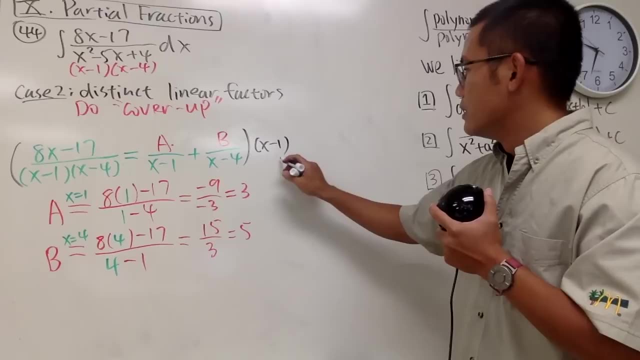 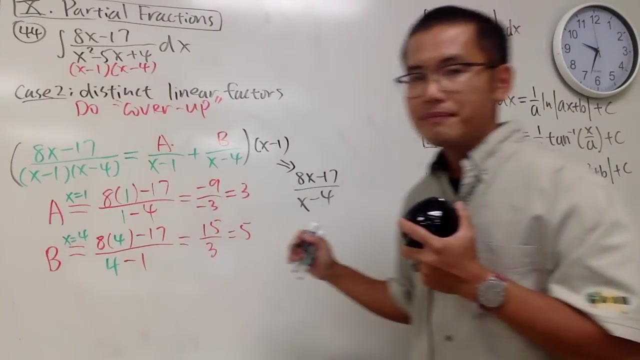 well, x times 1, and this can solve. so we just have x minus 4,. yeah, So let me write it down better: This right here will give us 8x minus 17 over x minus 4.. Cancel, so we have this. 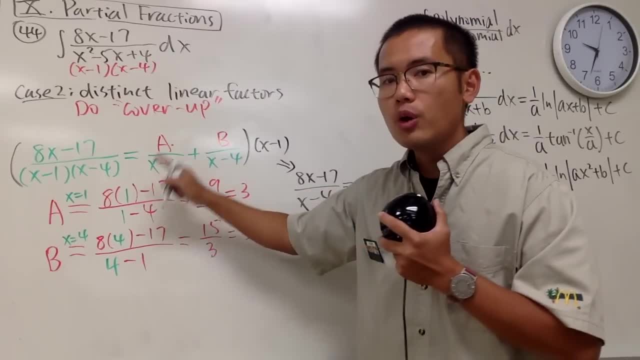 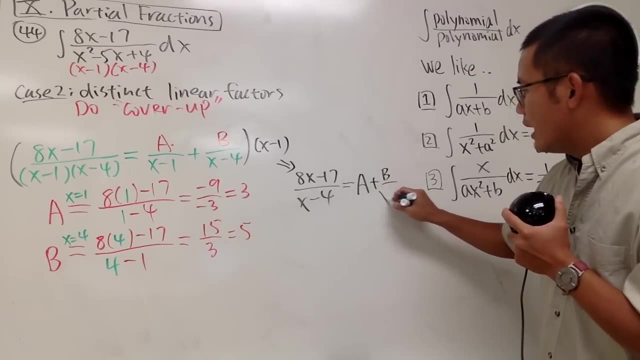 And that will be equal to this times that they cancel. we just have the a, Then we have this times, that which is plus b over x minus 4, times x minus 1, like this. Now let me ask you: 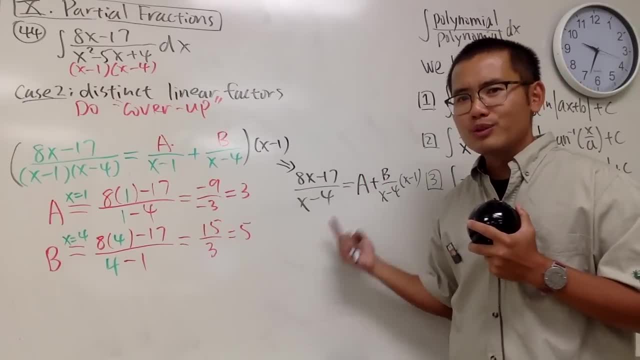 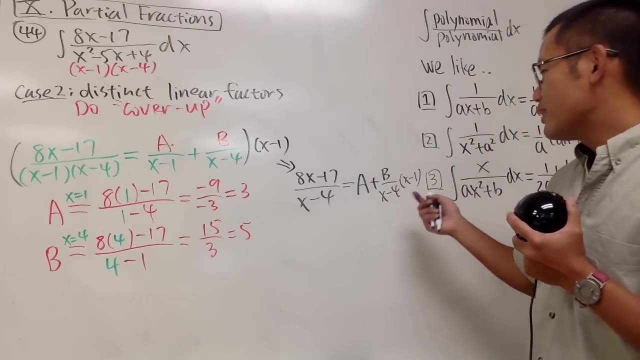 if you look at this expression, how many unknowns do we have? Three, Namely a, b and x. x can be anything that you want. a and b are the ones that we are trying to find out. They are the constants. 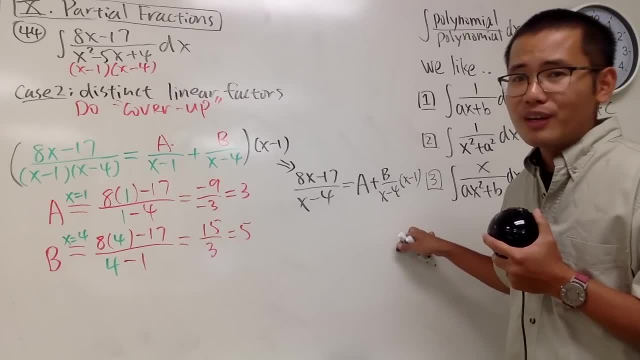 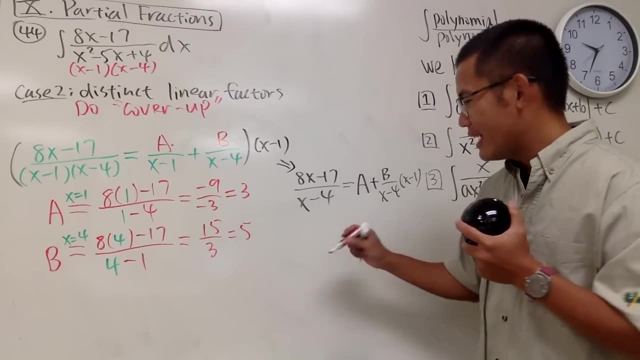 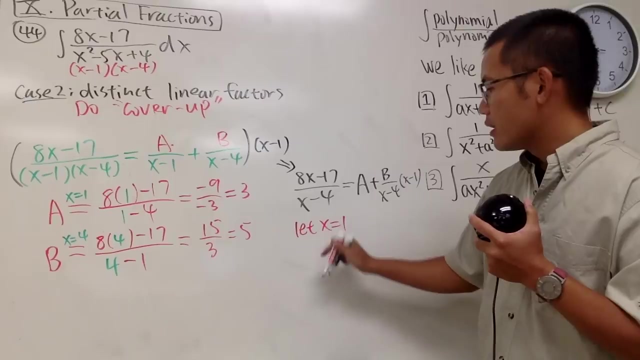 and we can plug in any number that we want for x. Well, wouldn't it be so nice if we choose a small number to plug in And that number is: let x equals 1.. When I'm putting 1 into x, right here and right here. 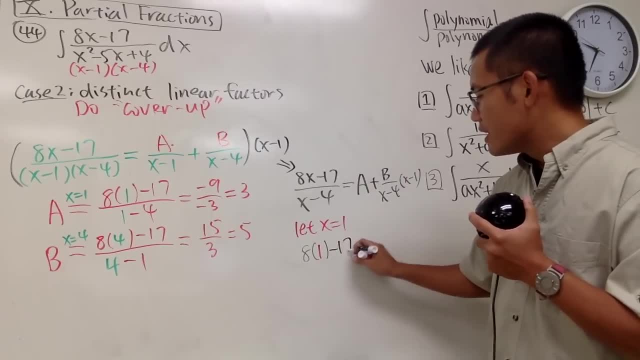 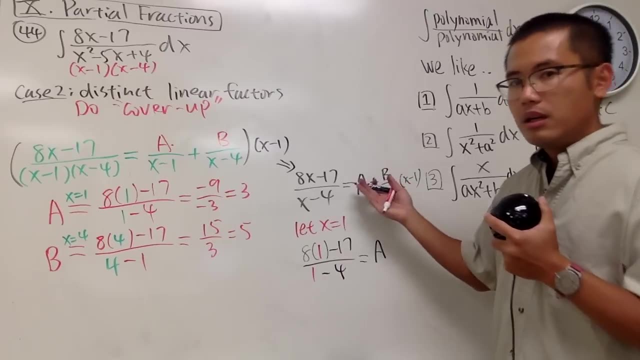 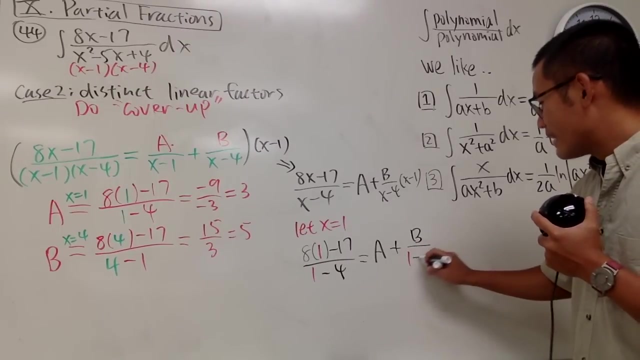 I get 8 times 1 minus 17, over 1 minus 4.. That will give me a and of course I have to plug in 1 right here and right here- and I know some of you guys see already- We have b over 1 minus 4.. 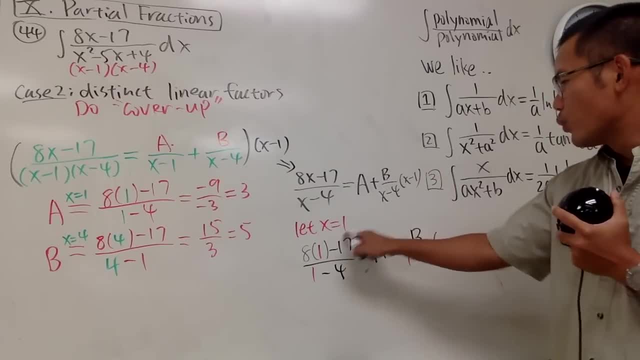 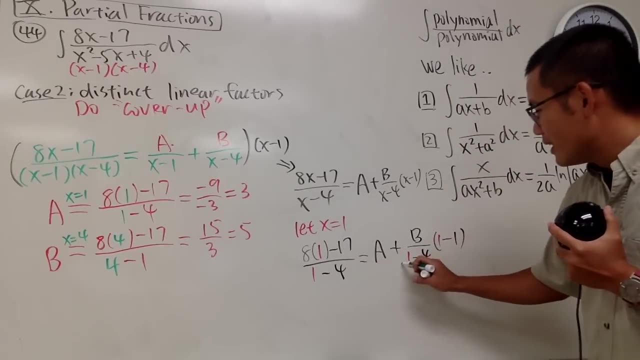 This looks not so surprising, but the moment we're putting 1 in here, we get 1 minus 1.. Of course that's 0.. This part times 0, hey, b doesn't matter anymore. In another word, x. 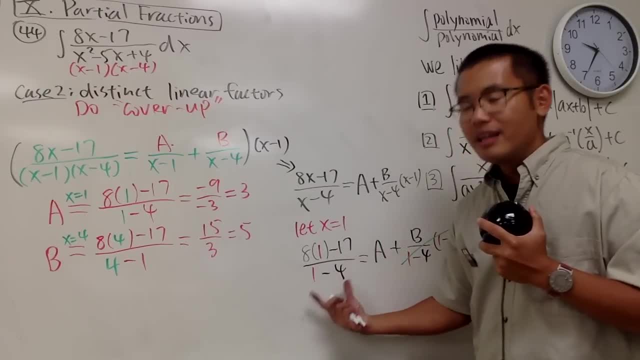 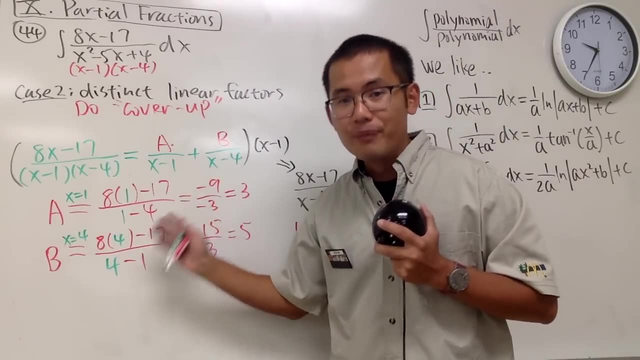 in another word, a is equal to this expression, and that's exactly how the COBRA works, And this is the fastest way to perform it, and this is the amount of work that you have to show. Just remember the correct setup and the correct number to plug in. 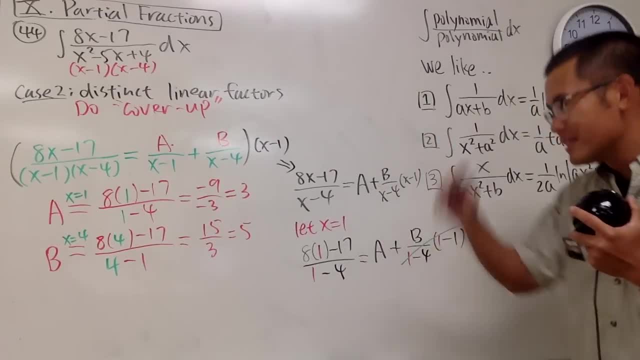 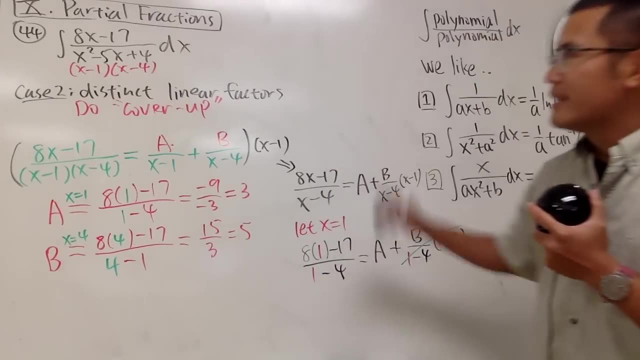 and the correct term to cover up, Right? So that's the idea. Same thing for b, but I'm not going to write it out. It's the same thing, All right. So this is very nice, but we're not done yet. 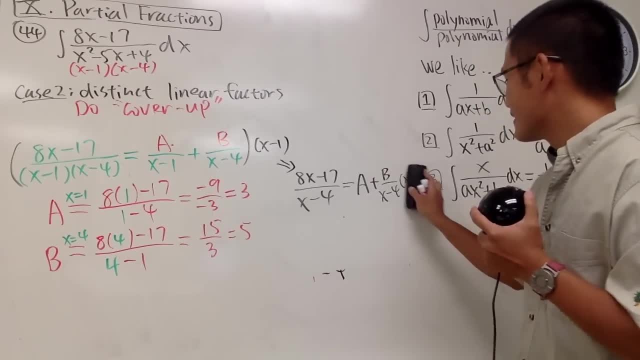 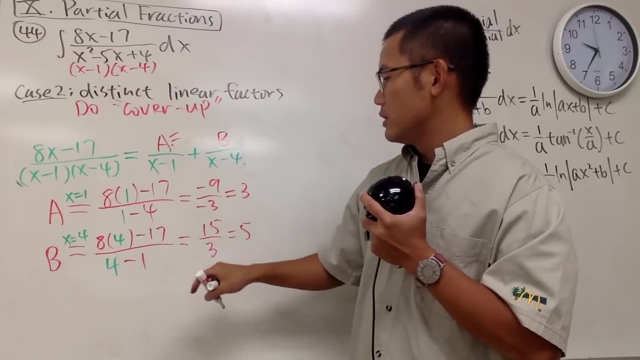 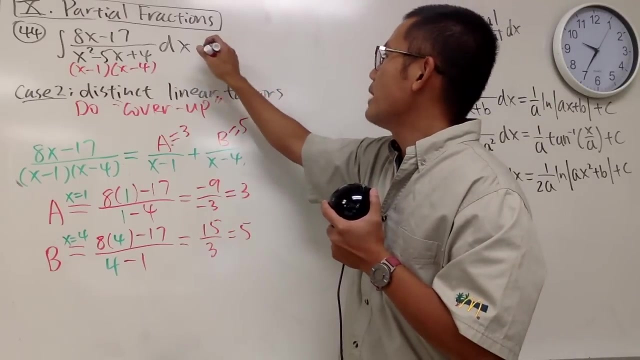 because we haven't integrated yet. This is just the algebra. Well, well, a is 3 and b is 5.. Let me just put on the integral right here, Hopefully you guys don't mind. Here is the integral And to integrate this: 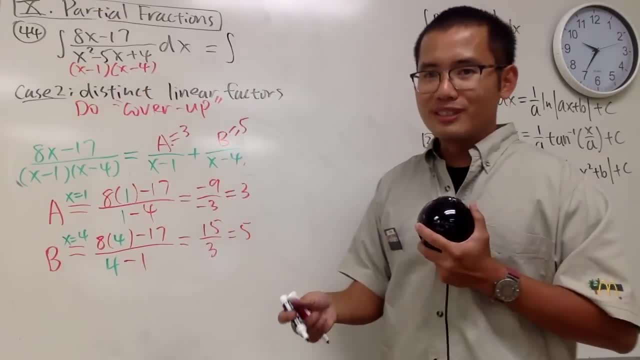 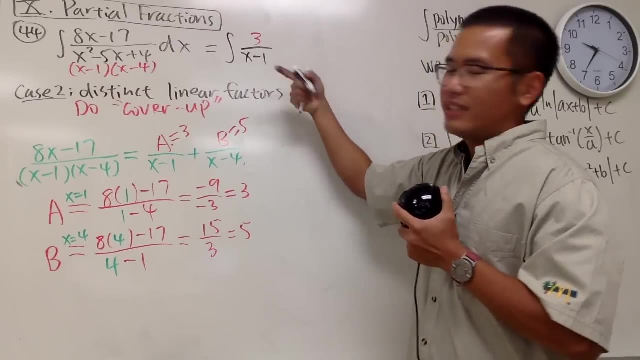 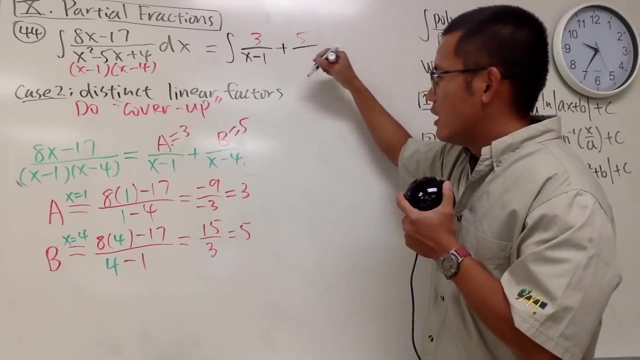 we'll just integrate this and that separately and then put the results together. Here we have 3 over x minus 1. And you can close it. but it doesn't really matter in my opinion. You can just put down plus 5 over x minus 4,. 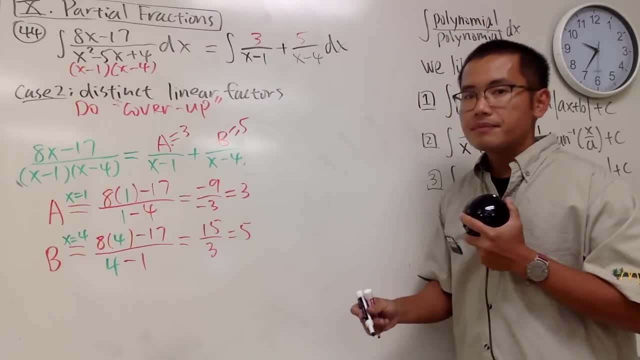 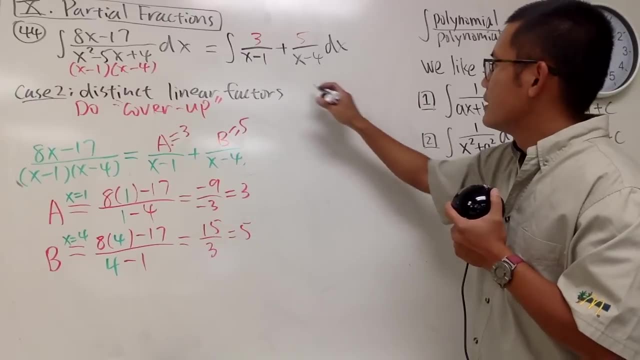 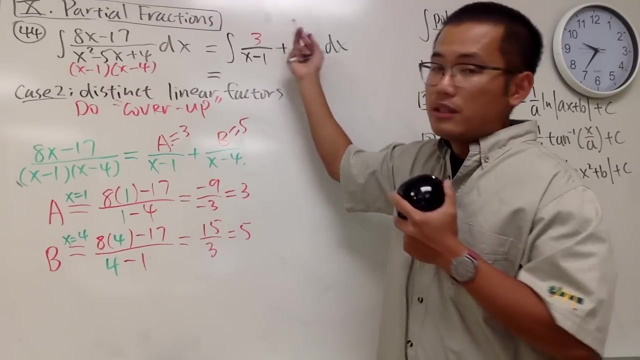 like this dx Right Now. do I have enough space Man? let's see. I'll put it down right here. Hopefully you guys don't mind that much. The integral of this 3 is a constant multiple. 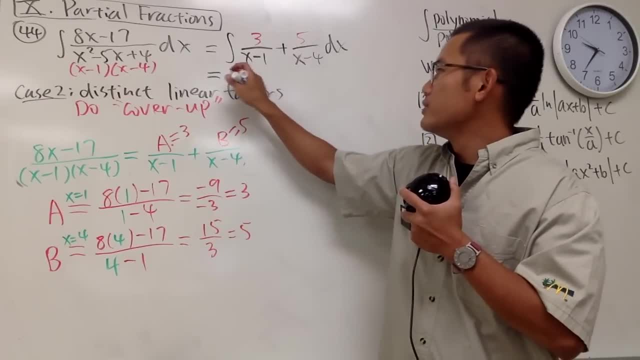 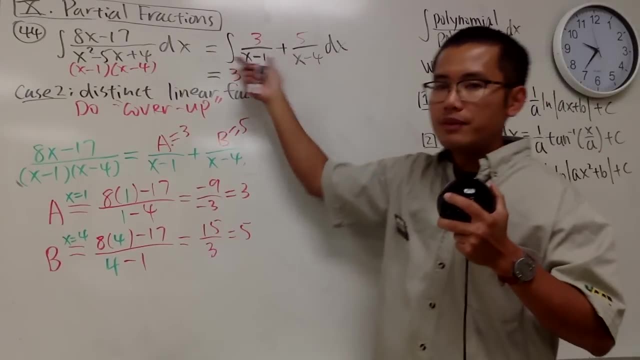 so you're just going to multiply 3, and then you have 1 over x minus 1, and that's the linear factor, which is this situation. The derivative of the bottom is just 1, because the a value is 1.. 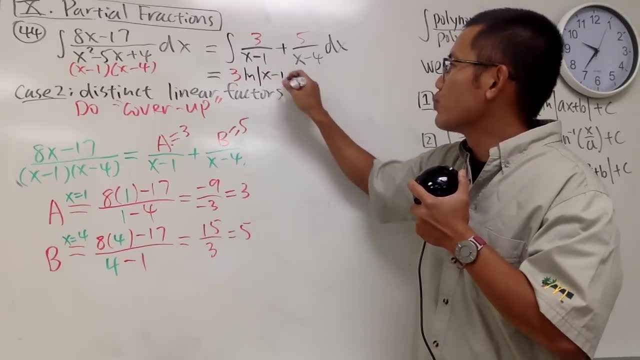 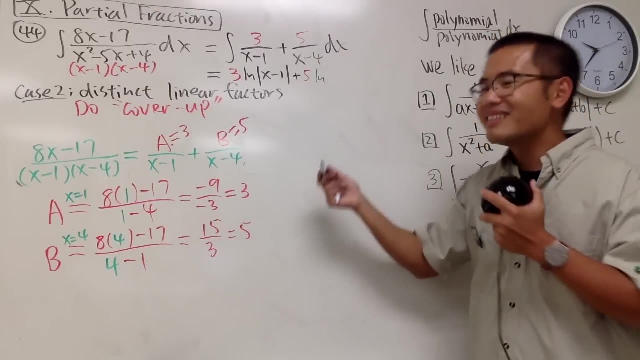 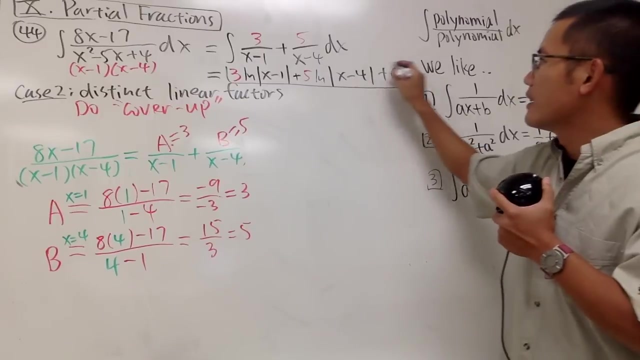 So you get natural log absolute value x minus 1.. Next you have the plus 5, and then natural log absolute value of x minus 4 plus c done Right. So this right here is the second case: Linear factors. 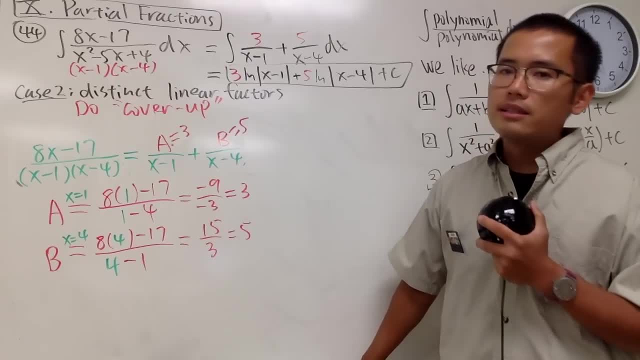 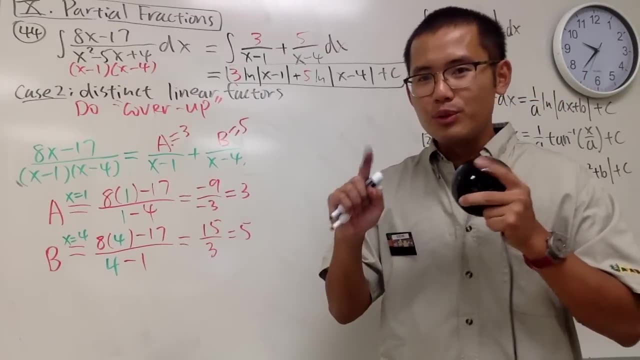 and they have to be all different. right. Distinct linear factors. In this case we just do cover up In class. I used both hands on the test. I know you guys will be using both fingers, but that's pretty much how you do it. 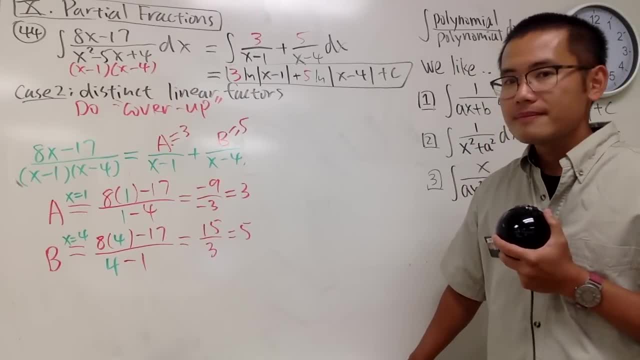 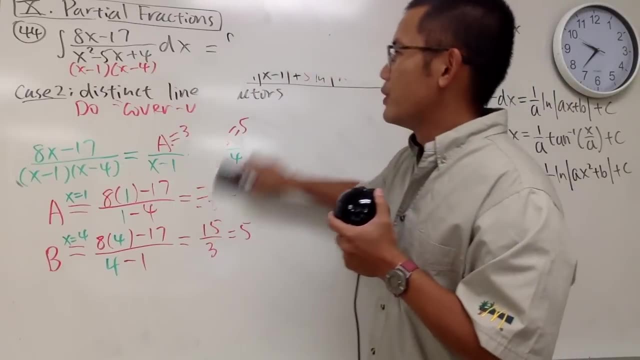 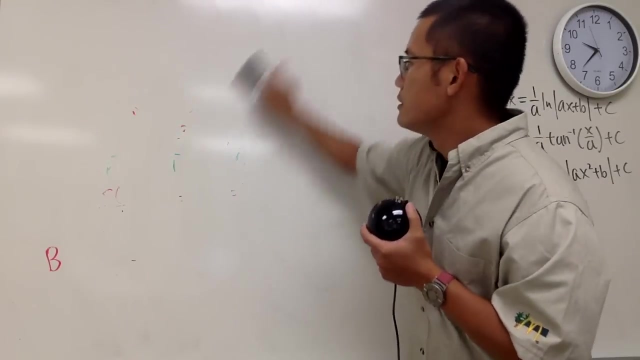 Right, So take a look, All right. So now let's move on to the third case, and I'm just going to erase this so I have more space. Erase the whole thing. So I will actually put down the case 3 right here. 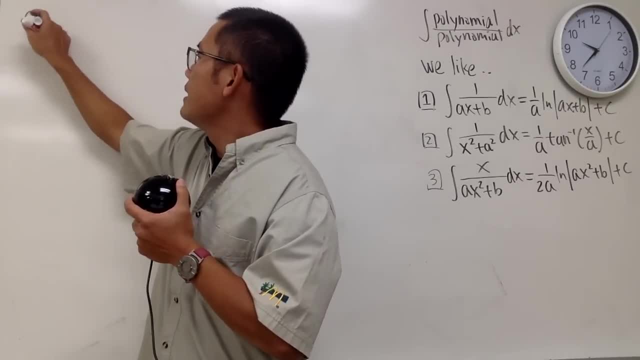 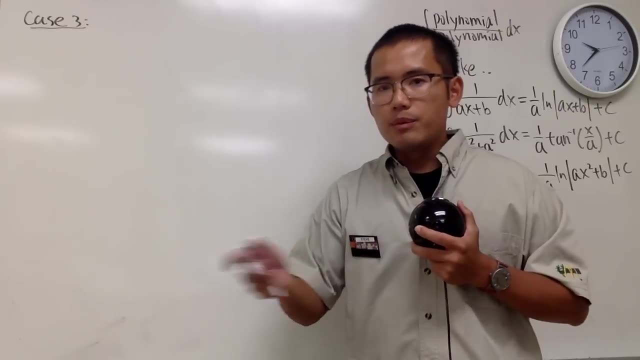 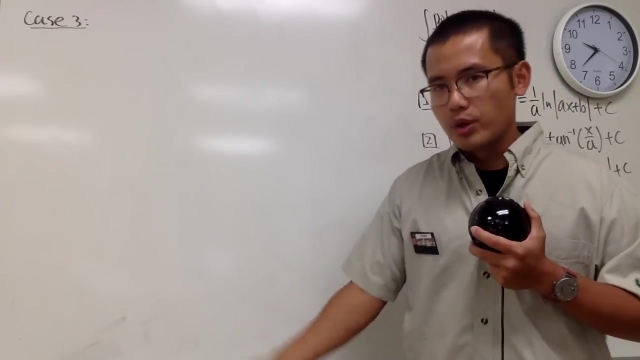 for you guys. first in this time, Here we have case 3.. Well, earlier we were talking about the distinct meaning, just different right Linear factors ax plus b. But sometimes you may have quadratic like x squared and all that. 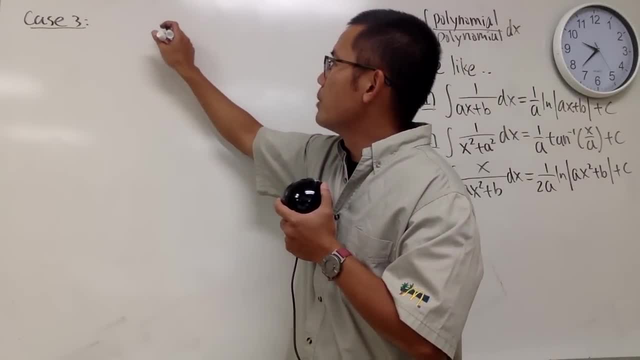 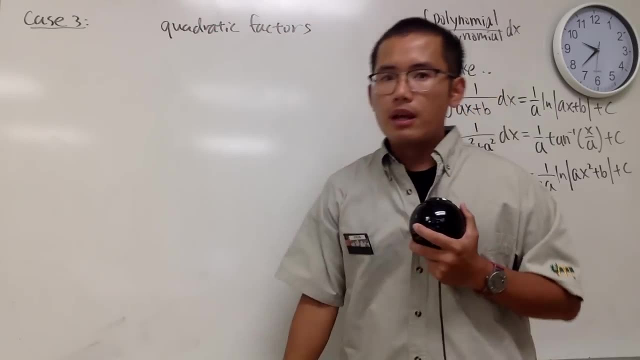 Well, let me just put this down first and I'll tell you guys what case 3 is all about. So let me just say, here we have quadratic factors. Well, let me just use this little board right here for you guys. 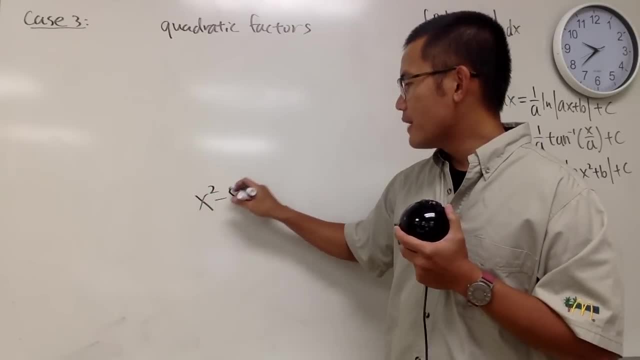 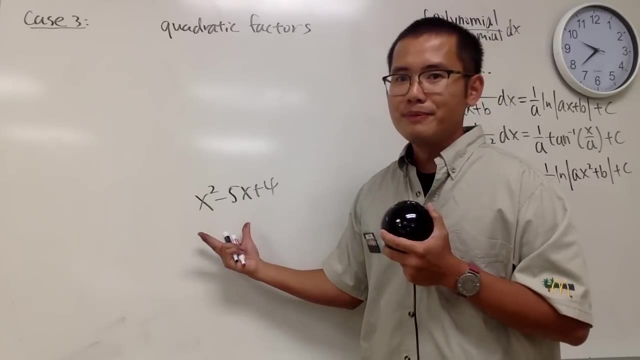 Okay, When you have x squared minus 5x plus 4, it is quadratic. Yes, it is because you have x squared. Good, But do you really have to deal with this quadratic? No, because you could factor it just how we did it. 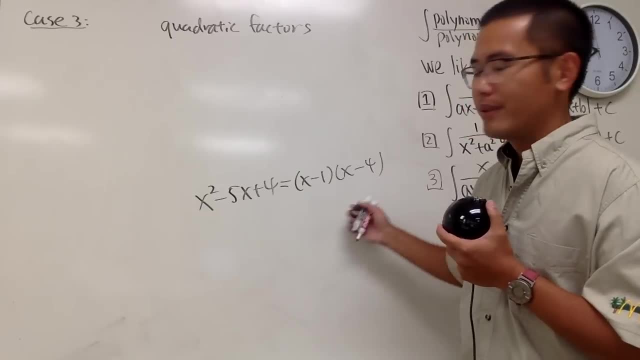 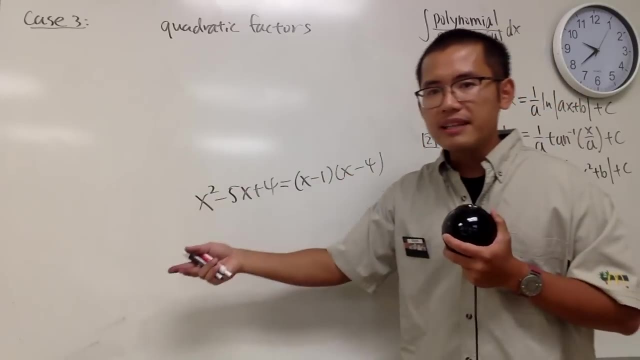 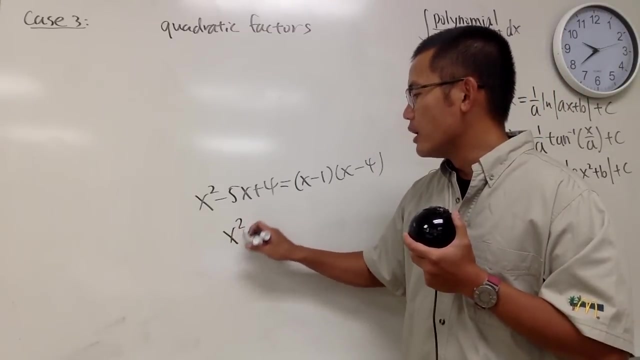 You have x minus 1 times x minus 4.. So if you see this in the denominator, go ahead and factor it. so you are actually, in the second case, Different linear factors, right. But if you have a factor such as x squared plus 4,. 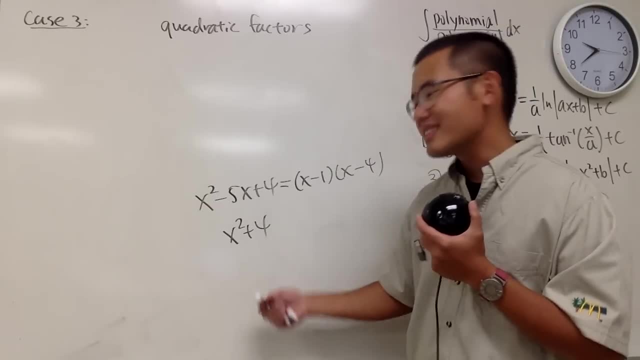 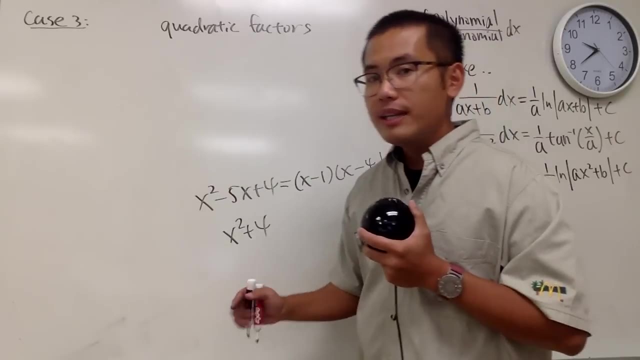 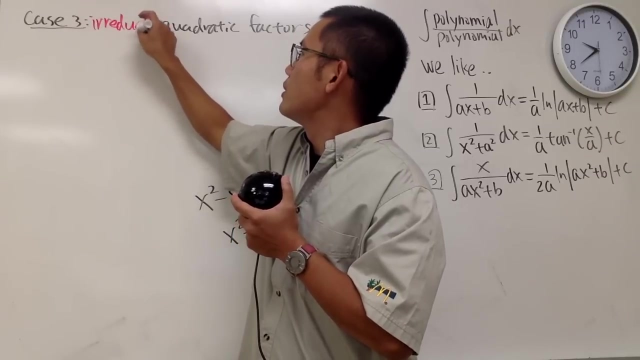 can we factor this? No, we cannot. We have been talking about this for a while already, right This, right here. we cannot factor it with real numbers. So for case 3, this is the case that when we have irreducible, 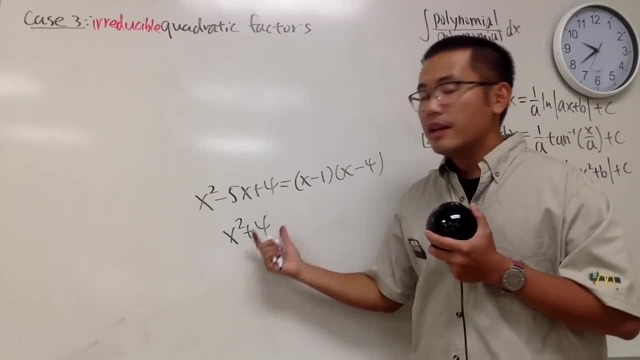 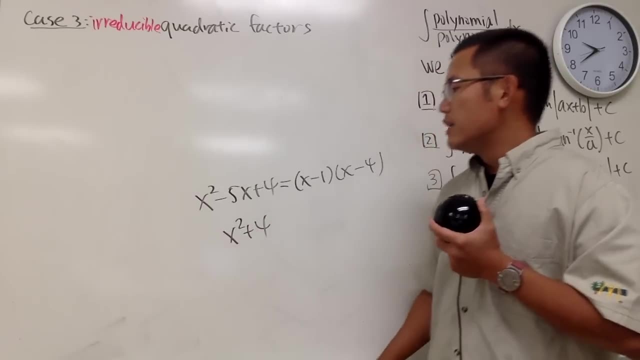 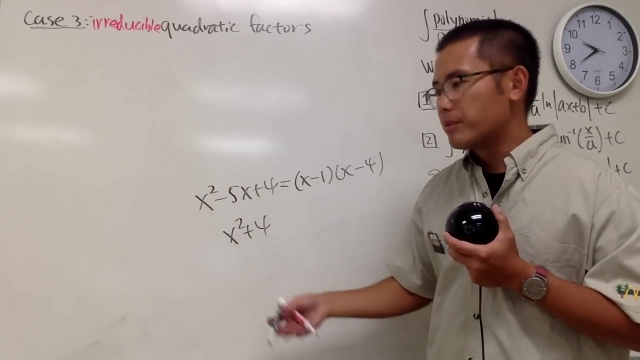 meaning that it's not because we cannot factor this. the worst thing is that it does not have any real number root. It does not have any real number root. Sometimes you may be able to solve the quadratic equation and you have real number solutions. 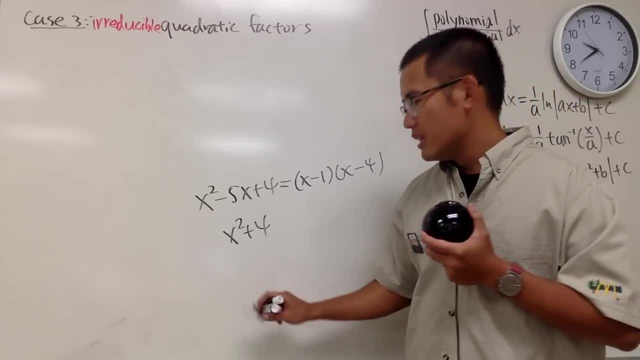 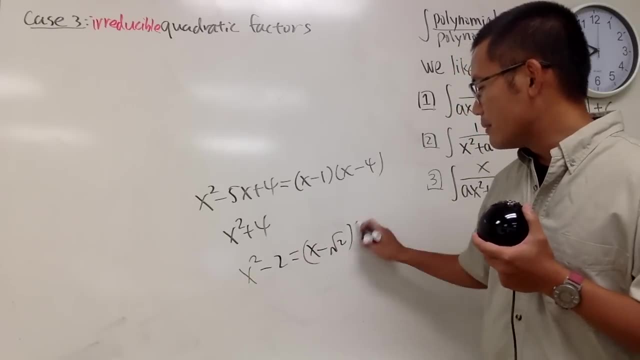 And in fact you can factor it. You may have like radical answers such as x squared minus 2.. You can factor this: This is x minus square root of 2 times x plus square root of 2.. But nobody likes to factor this. 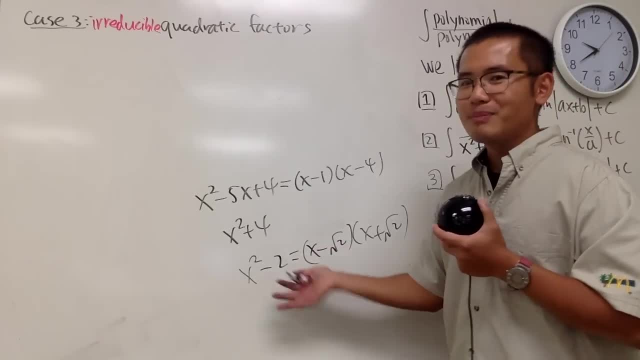 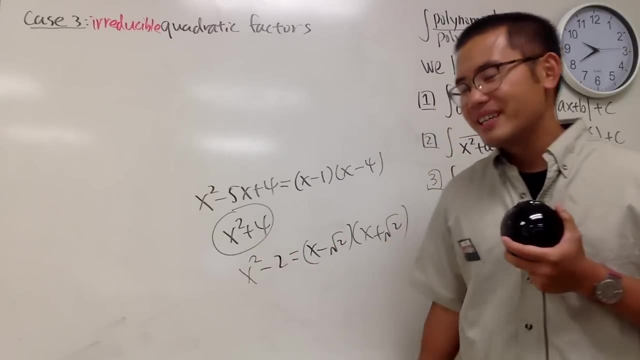 I know I'll try not to ask this kind of question on the test, but maybe once in a while you guys will have to handle that. But no matter what we do, we cannot use real numbers to factor this out, right. 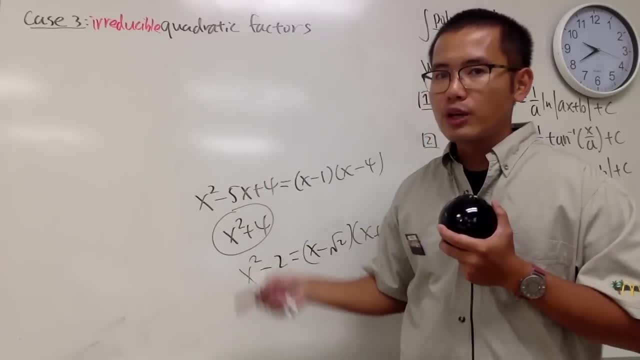 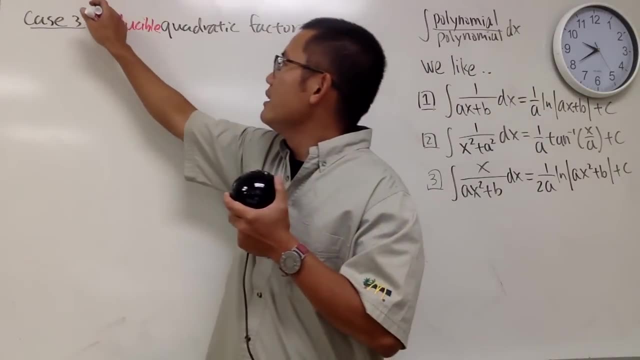 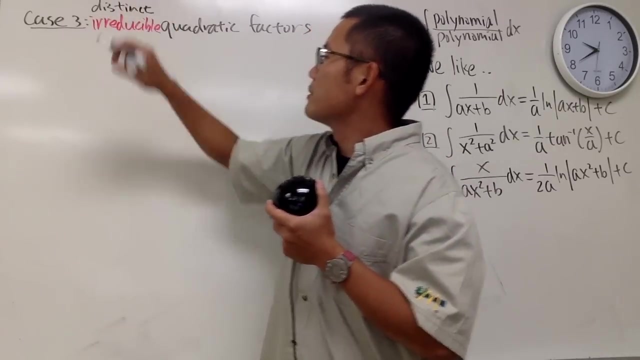 So this is what we mean by irreducible quadratic factors, And this will be case 3.. And of course, let's also mention that it has to be this thing, because for the third case and all that, this thing means just different. yeah. 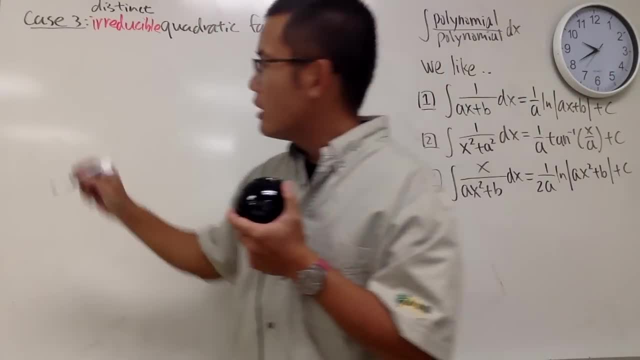 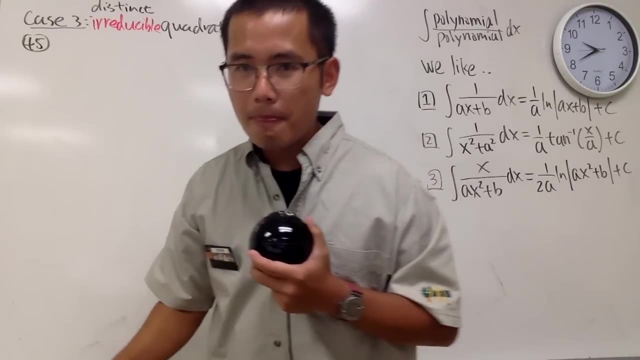 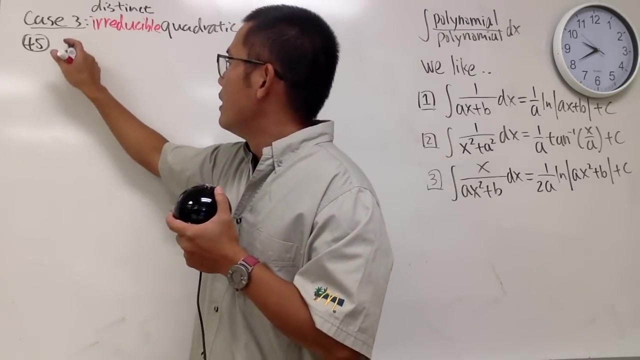 Okay, So I actually have the denominator factor d for you guys already. What am I saying? Five hours, Five hours, Okay, We can pretty. I cannot finish this by 10.. It's okay. 45. We have the integral. 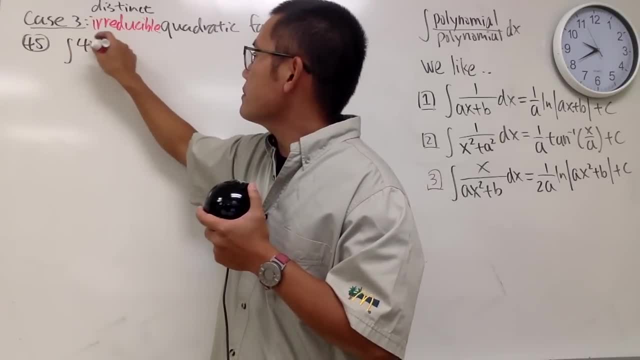 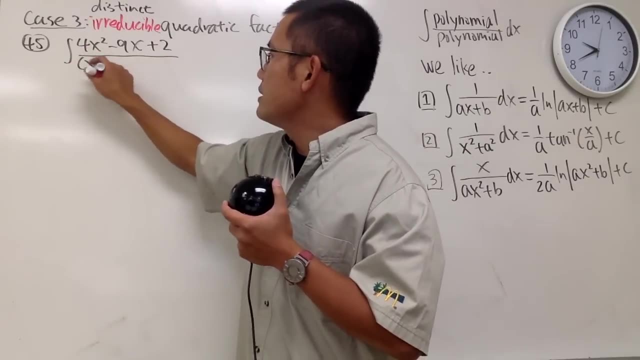 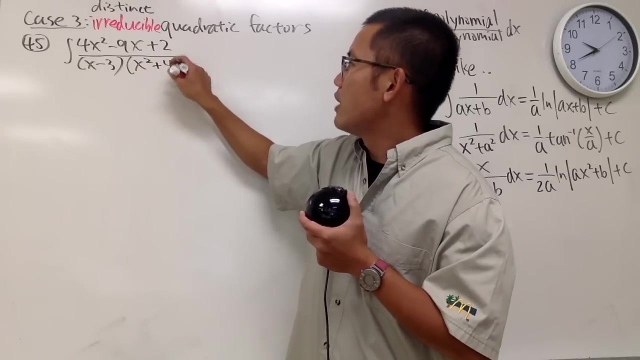 and here we have 4x squared minus 9x and plus 2 over parentheses, x minus 3 times x squared plus 4.. So I've found out the denominator for you guys already And right away. you see that we have. 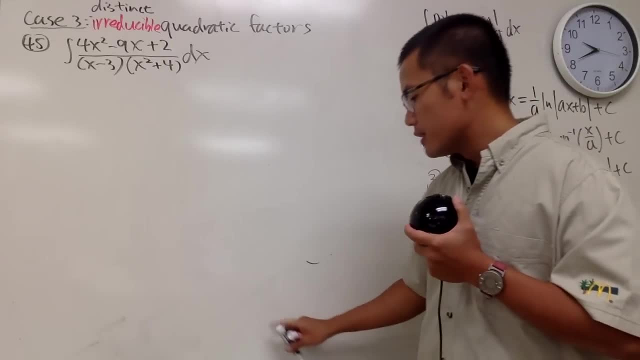 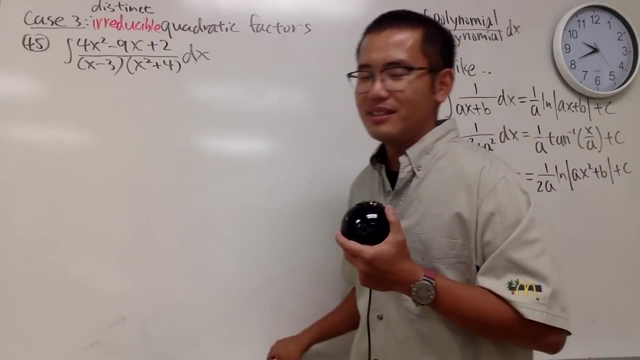 an irreducible quadratic factor. Now let's focus on the partial fraction first. This is all about the partial fraction. I know Just a lot of algebra. It's just how it is, Okay, So let me put this down right here for you guys. 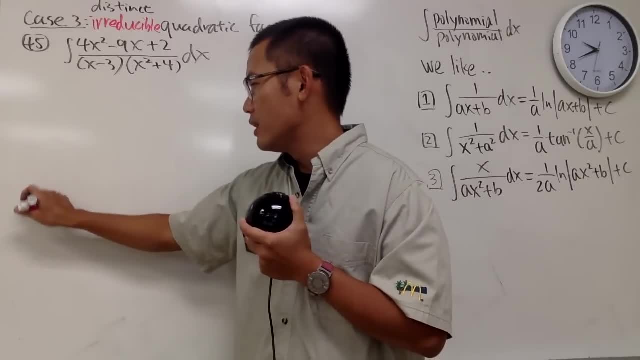 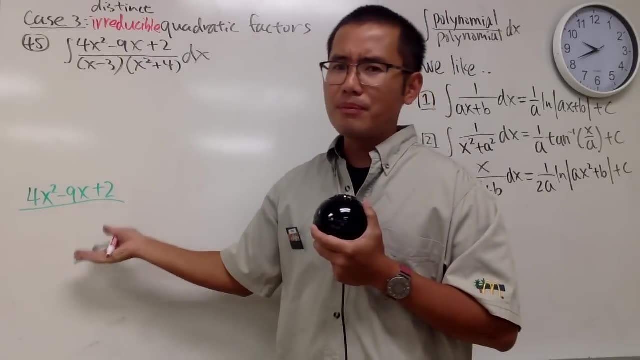 Let me write down this right here. I think this is the amount of space I need, hopefully 4x squared minus 9x plus 2.. You don't need to worry about finding the top Doesn't matter, Just the bottom, okay. 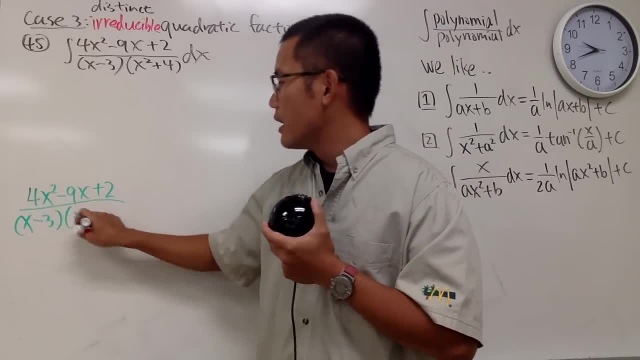 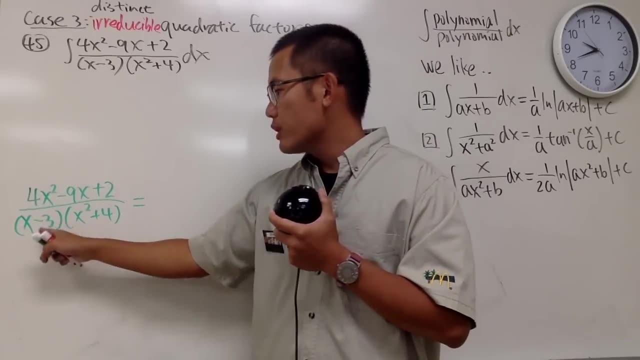 Over x minus 3 times x squared plus 4.. First thing, first degree on the top is 2.. Degree on the bottom is 3.. So we don't have to do long division If this is 4x to the third power. 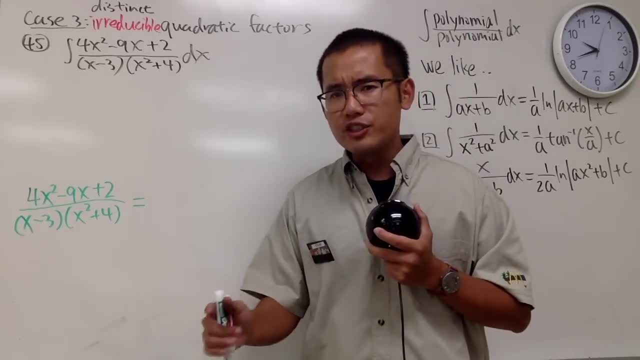 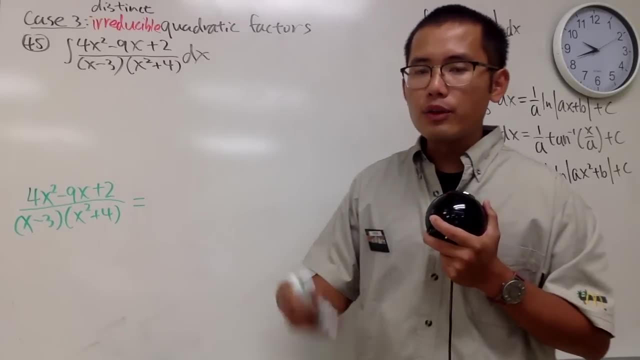 we have to do long division right. So always check the degrees, Always check the degrees. And here's the setup. This right here is x minus 1 to the first power. It's a linear factor, So we have something over x minus 3.. 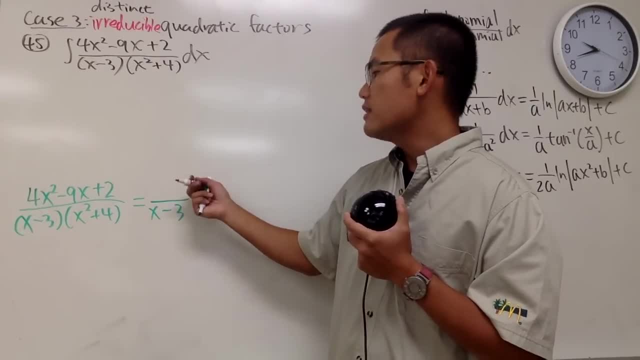 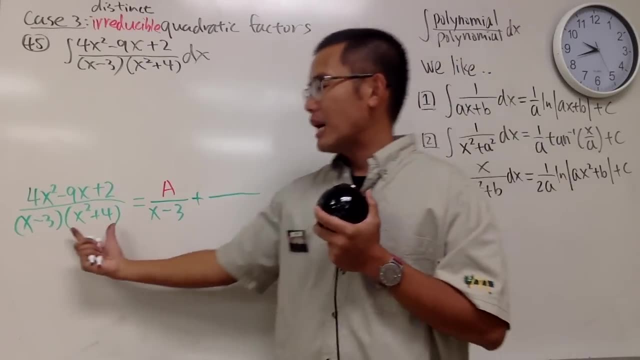 And I will tell you this right: here is just some constant which is: we don't know a for that right, And then we add the width. Next thing that we have is this, which is x squared plus 4,. 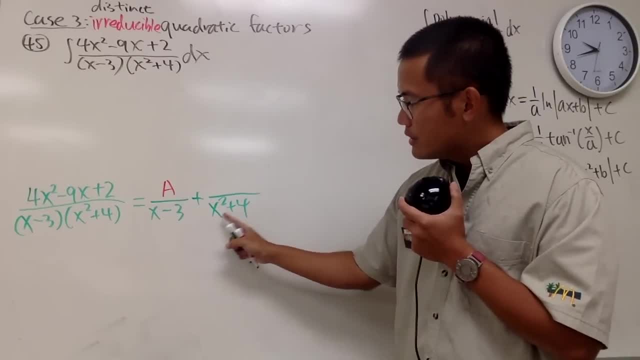 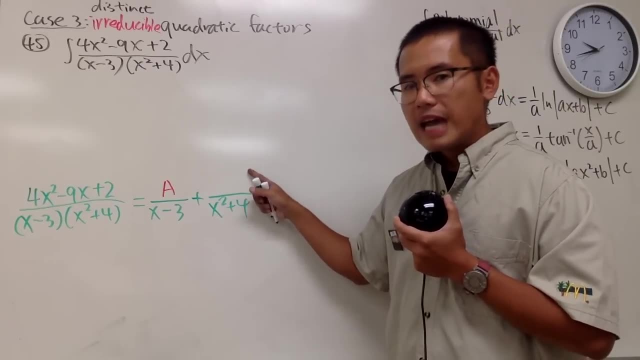 like that This time, though, notice that the bottom is quadratic, And remember what I said earlier. Well, if this is quadratic, when we set it up, the top will always have to be one degree less than the bottom, So we will have to have a linear term. 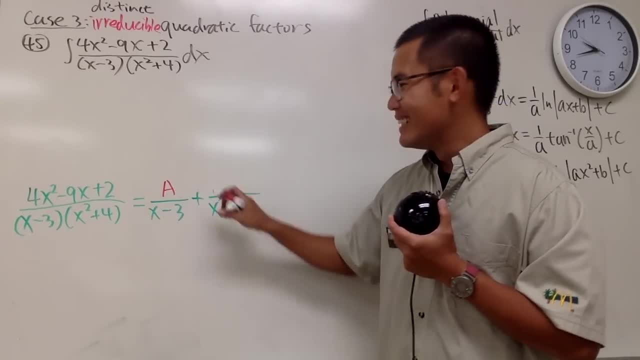 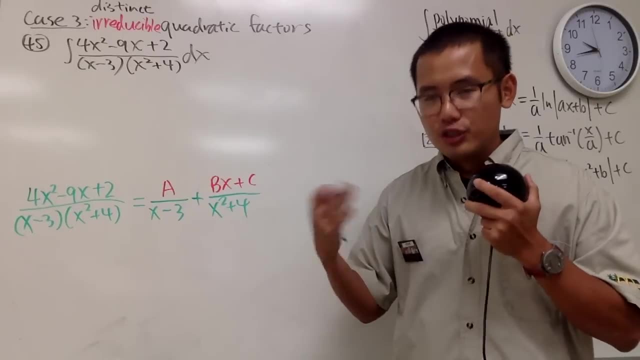 I used a already, So we'll just continue with our alphabets. We have bx to the first power and plus c. You have to make sure you have the complete, the general version of the linear form, like this right. 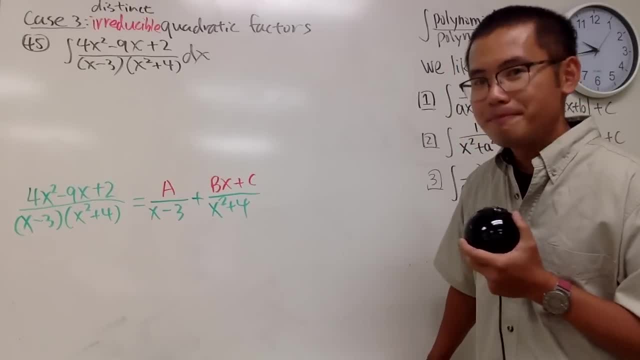 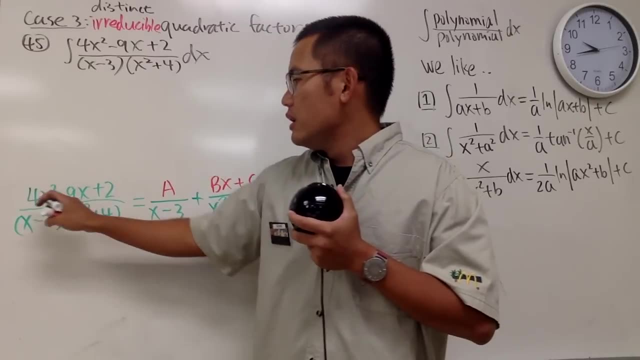 And, yes, we just have to figure out abc for this. Yeah, Okay, Notice again, we really didn't need to worry about the top, except for the degree. If you have this, that would be the setup. If you have this plus 21,. 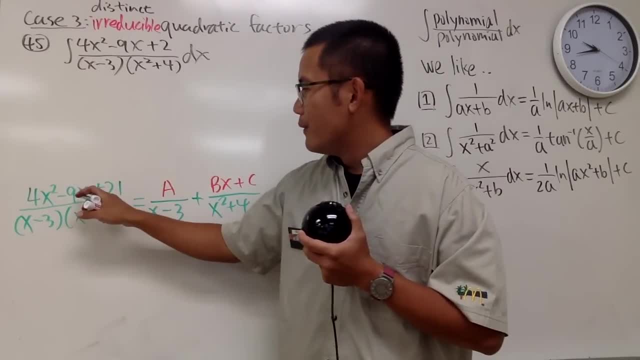 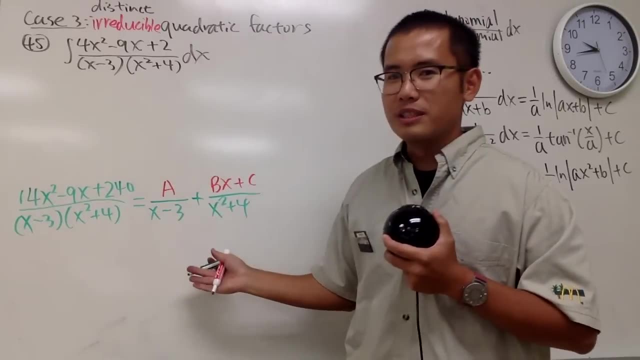 it's still the same setup. If you have this plus 240, it's still going to be the same setup, right? If you have 14x squared, it's still going to be the same setup. Okay, I know, I'm sorry. 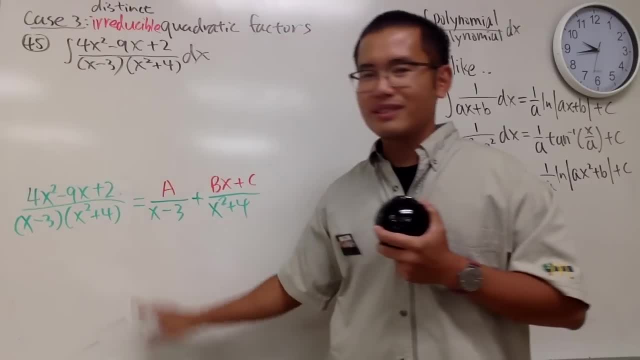 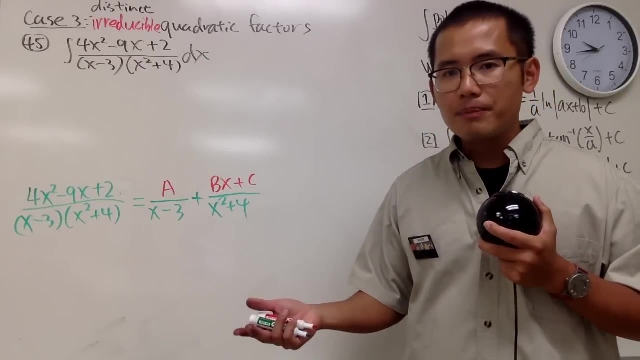 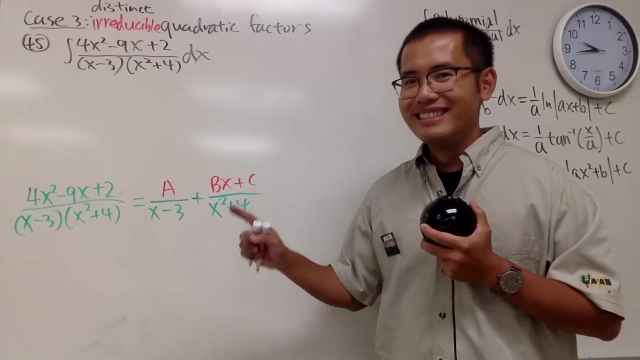 I had too much fun, So let me just erase that. That's just a point. yeah, All right. Our favorite way to do this is the cover-up. Good news for you, We can do cover-up with one letter. That is a. 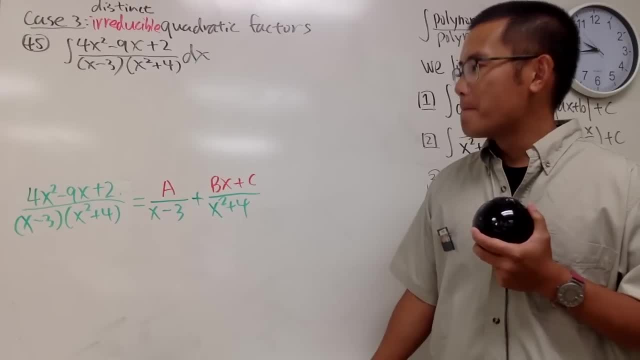 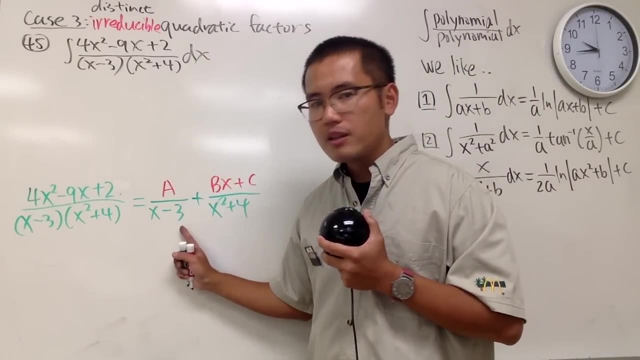 Yeah, We can do cover-up right here for the a. So pretty good. Pretty good Why? Because a has x minus 3 for the denominator. We can come here and cover this up And we can also make x minus 3 equal to 0.. 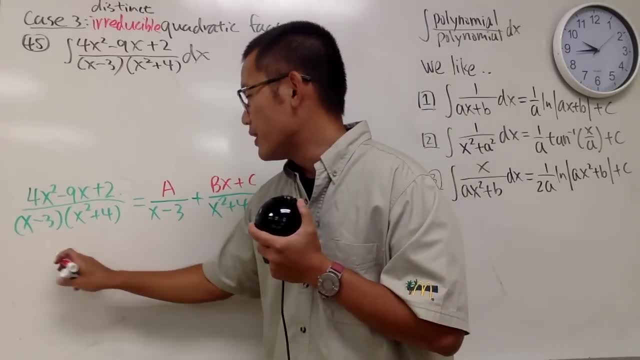 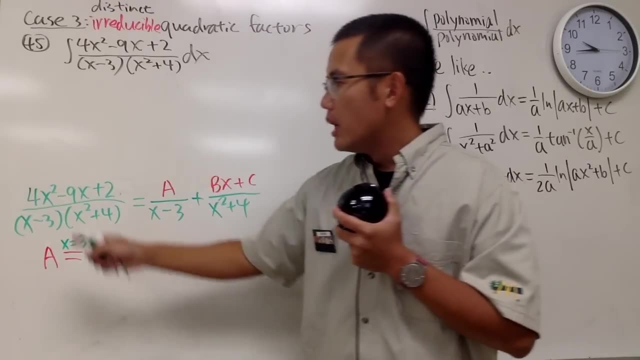 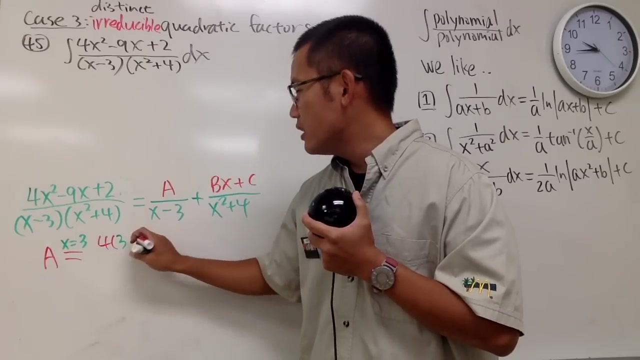 So we can do cover-up for a. Let's go ahead and take advantage of that. a is equal to when x is positive 3.. Put it here, Put it here. Put it here, All right. So we get 4 times 3 squared minus 9 times 3.. 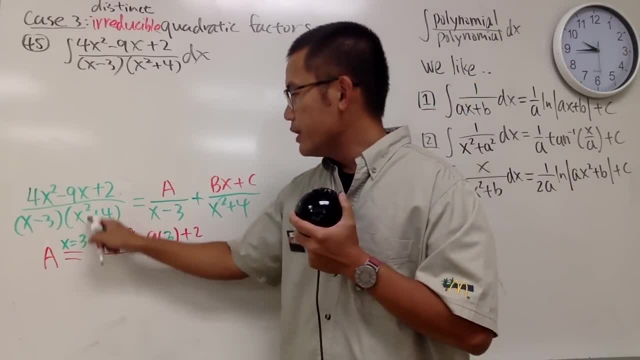 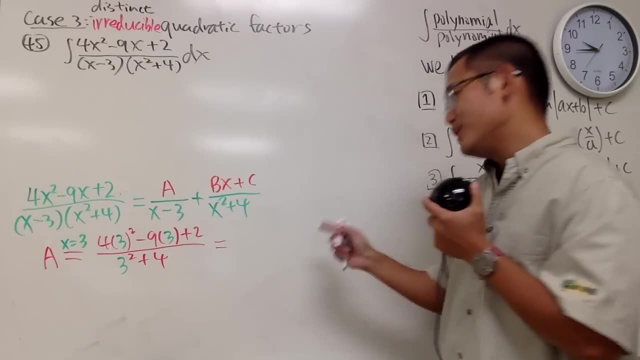 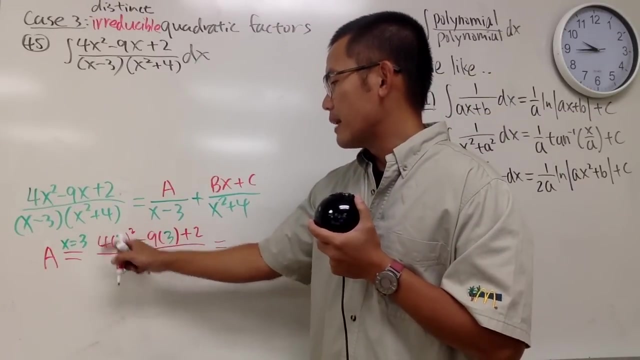 And then plus 2 all over. Putting 3 into here, we get 3 squared plus 4.. And now I'm kind of tired So I have to see if I can really do the computation correctly or not. This is 9 times 9 is 36.. 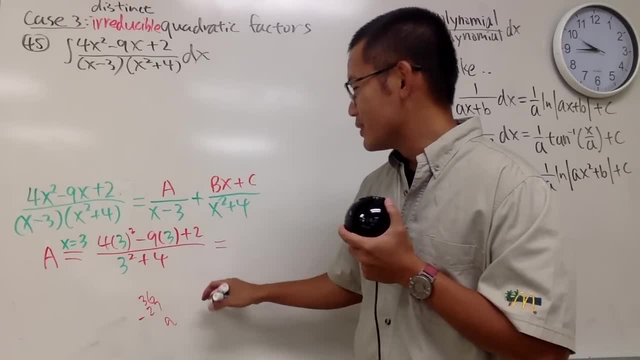 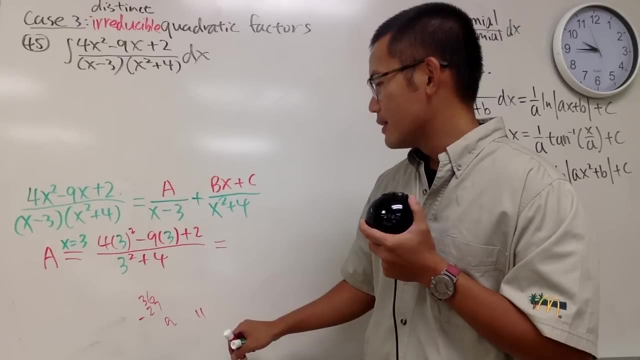 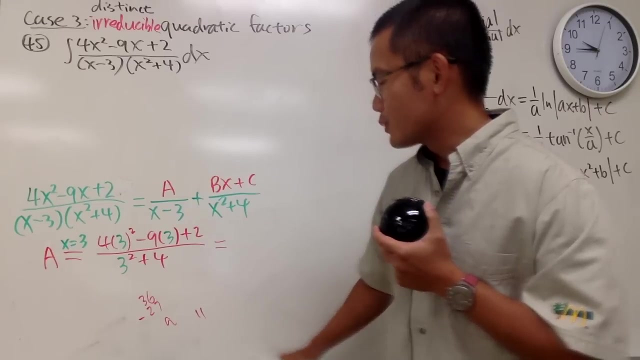 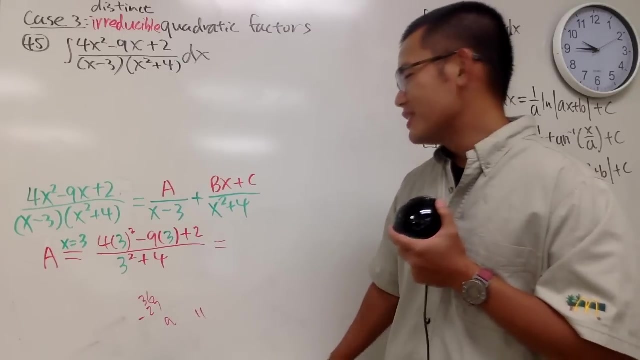 Minus 27 is 9.. Plus 2 is 11.. 36 minus 27 is 9. 9.. Man, I have 11 over 13.. I don't think I have the equation that hard, though, to be honest. 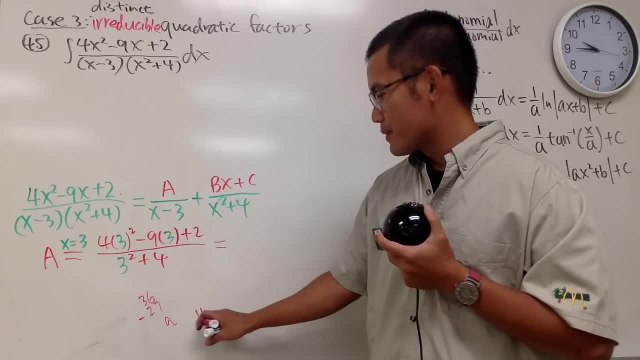 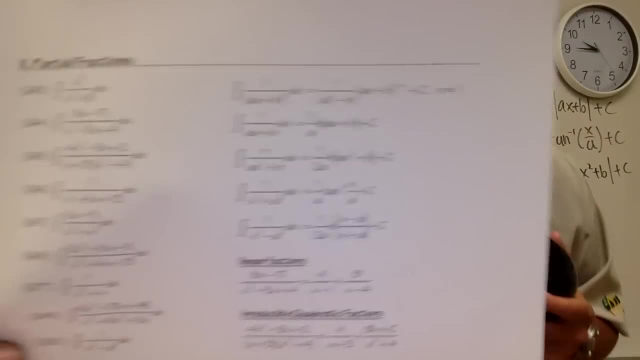 I think I set that, so the number actually worked out pretty nice. Let me see I have. Sorry, Sorry, Sorry, Sorry, Sorry. I copied down the wrong question. I knew something was wrong. My bad, This right here. 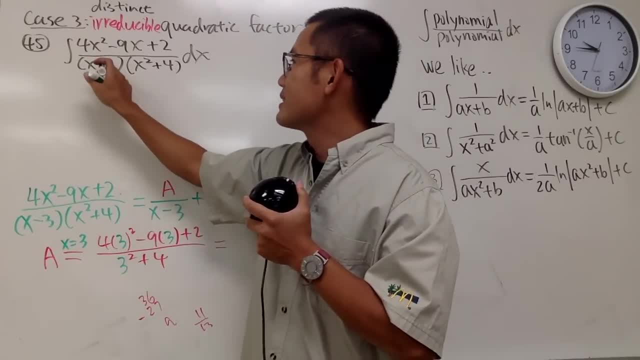 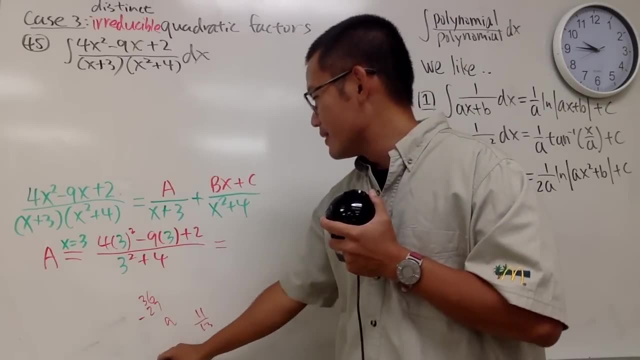 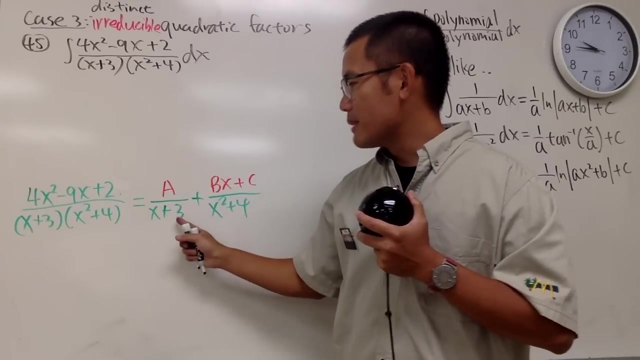 It's meant to be x, What here? it's meant to be x plus 3, okay, And then x plus 3, x plus 3.. So let me do this again, All right. second case: this right here is the setup. So a over x plus 3, and. 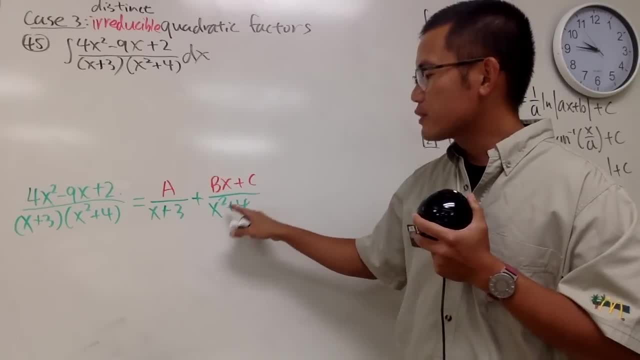 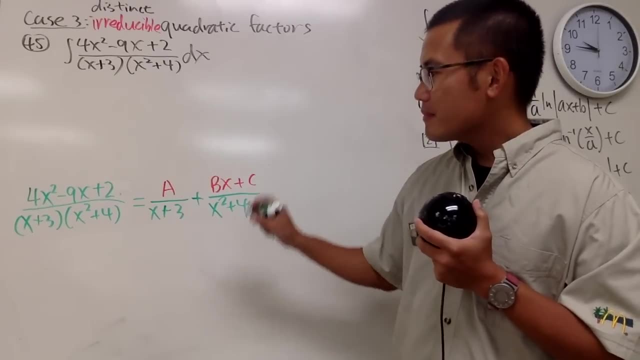 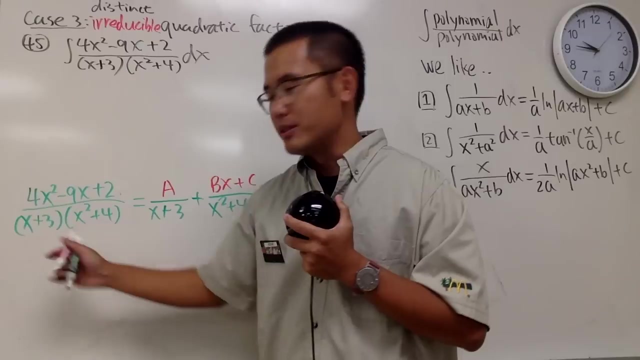 then bx plus c over x, squared plus 4, because the top has to be one degree less than the bottom, like this right. So maybe I'll just do a timestamp right here. All right, a right here. we are going to do the cover-up, because we can cover this up and make it equal to. 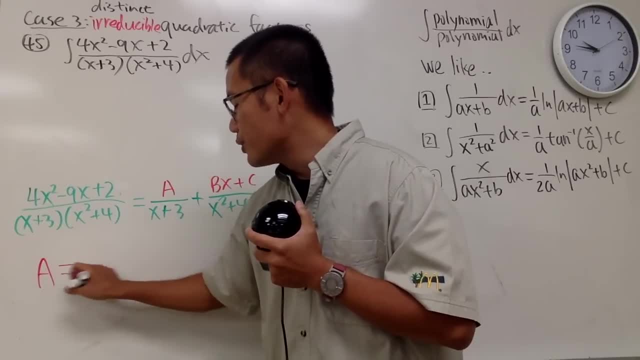 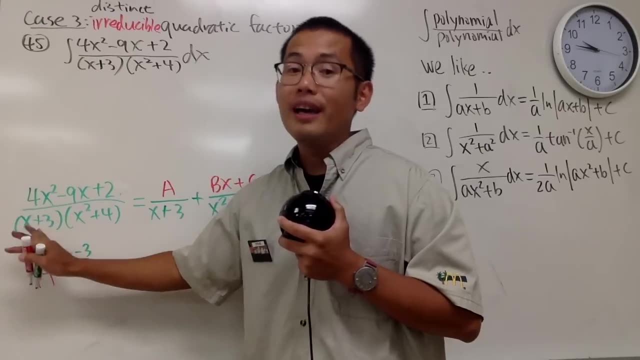 0.. Well, for a, this is going to be when x is equal to negative 3, because when we cover this up, to make x plus 3 equal to 0, x has to be negative 3.. Put negative 3 into all. 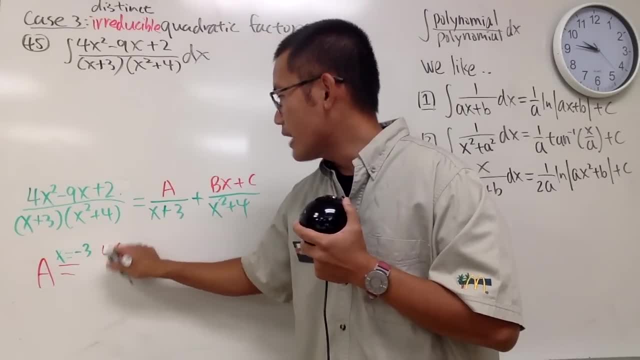 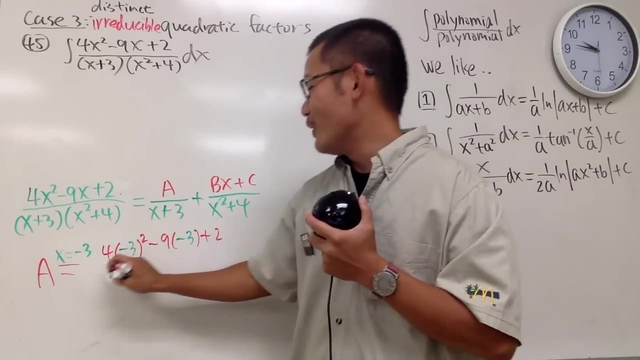 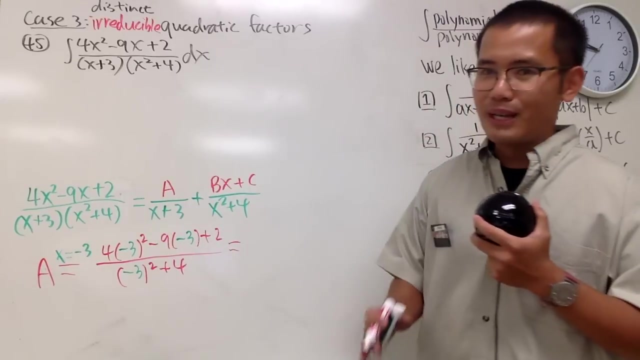 the x, this, this and that. So we get 4 times negative 3 squared minus 9 times negative 3, and then plus 2, all over, So negative 3 and squared plus 4, like that. Now let me try again: This is 9 times that. 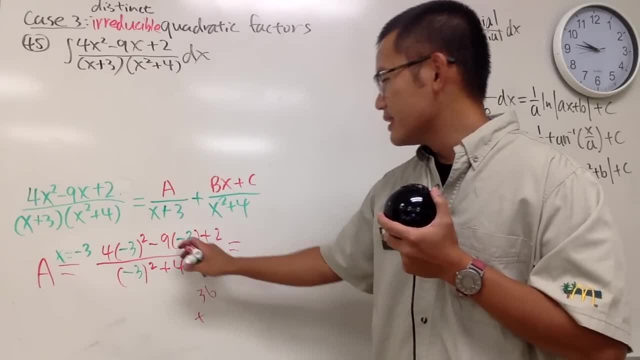 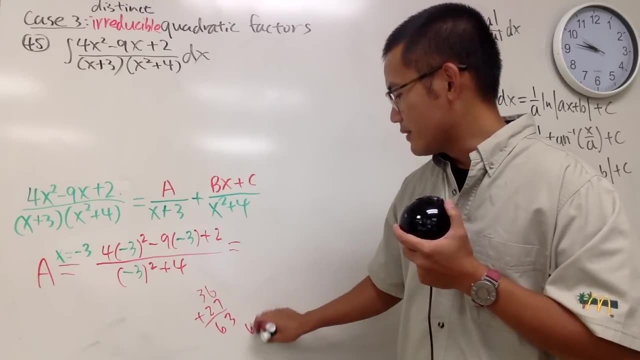 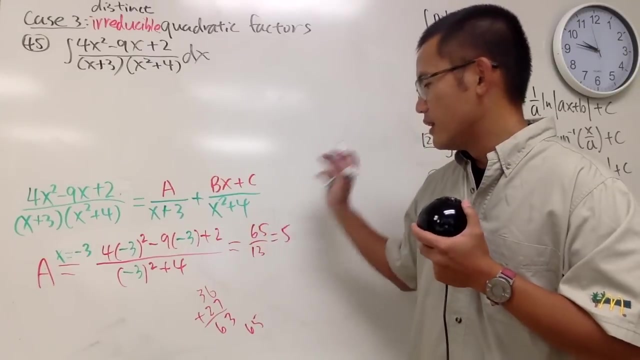 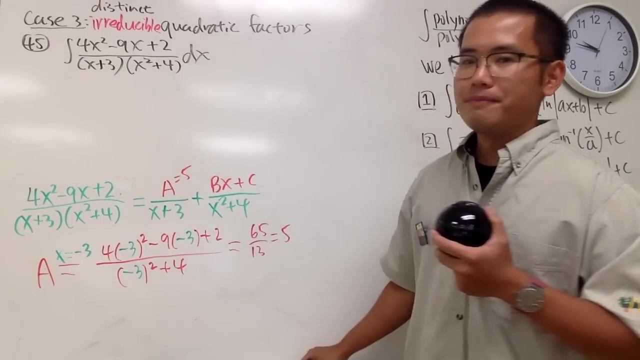 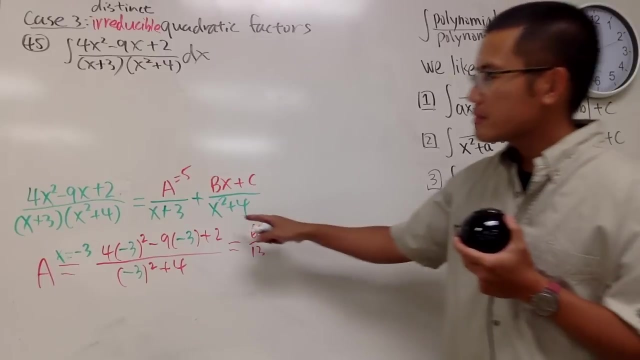 is 36, plus. this is plus 27,, which is 3, and then 6, plus, or 65,, and then divided by so it's 65 over 13,, which is 5.. Okay, much better. This is 5. Good, But how can we do b and c though? Well, in this case can we do cover-up. 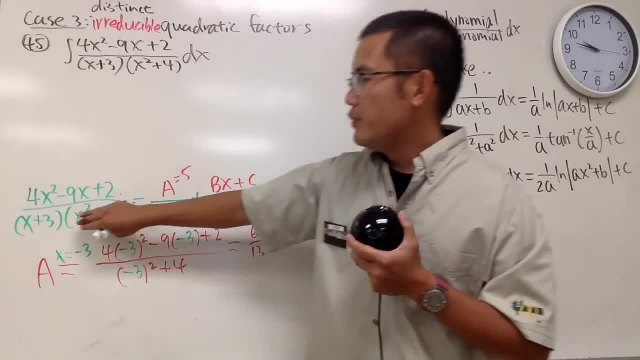 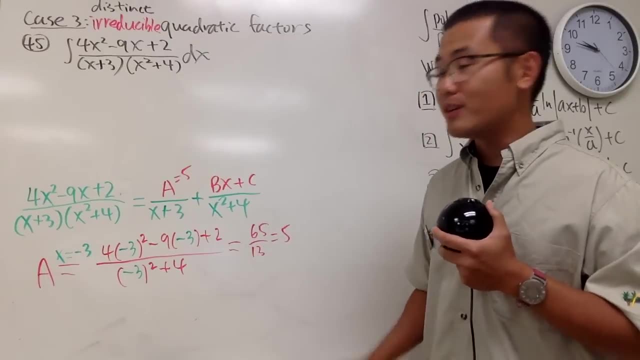 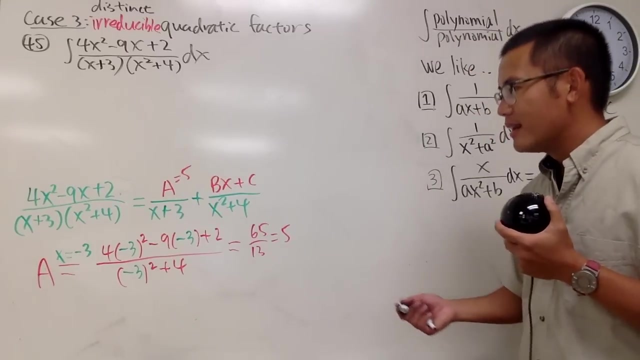 for b or c. No, One reason is because if you cover x squared plus 4, how can you make x squared plus 4 equal to 0? We cannot. And again, we are not using complex number whatsoever, so cannot In this case. we just have to do the dirty algebra right. We just have to. 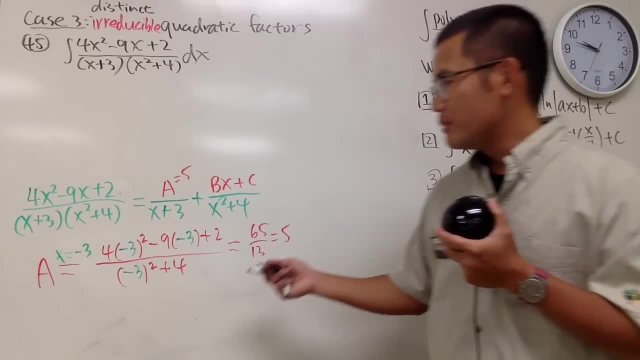 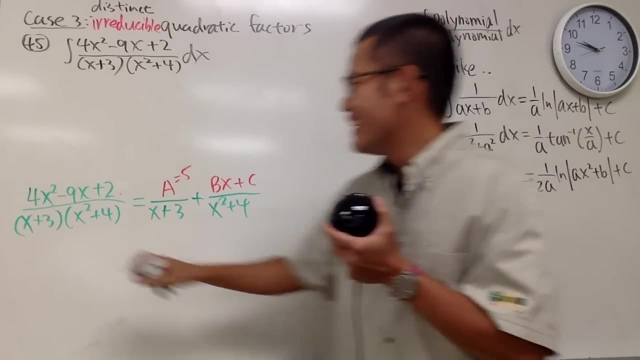 do the dirty algebra. Dirty algebra, And because we got the a already, so let me just clean this up right, I have to save some space. It's dirty algebra series. you see Meaning we are going to multiply everybody by the lowest common denominator, so that 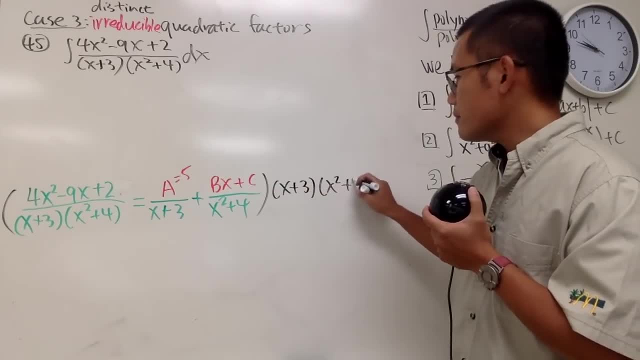 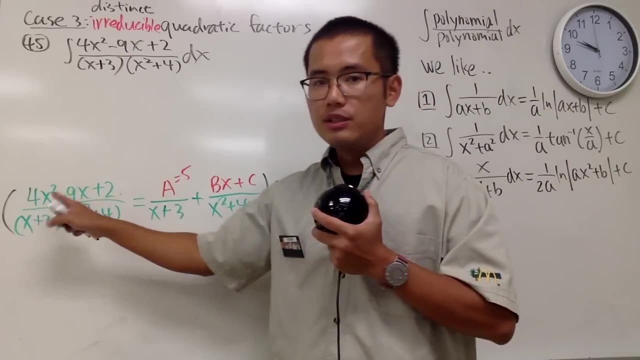 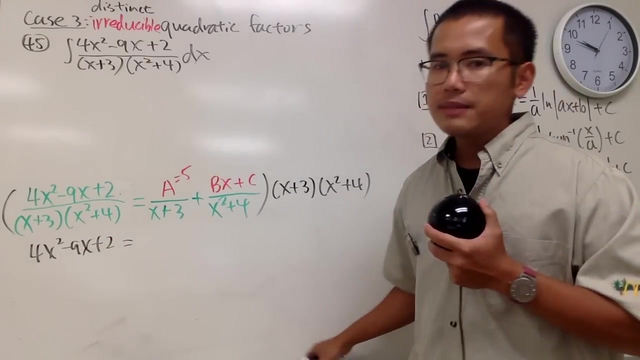 we don't have to deal with fractions anymore, just how we did the explanation of why the cobra method worked. Anyway, this times this just the top left, which is 4x squared minus 9x plus 2, and this is going to give us we have 5 times this. You see, This is 5.. We. 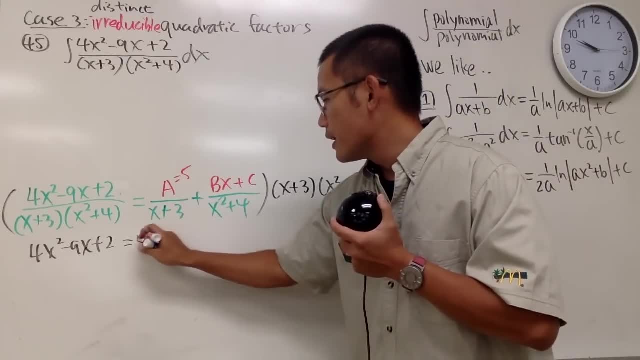 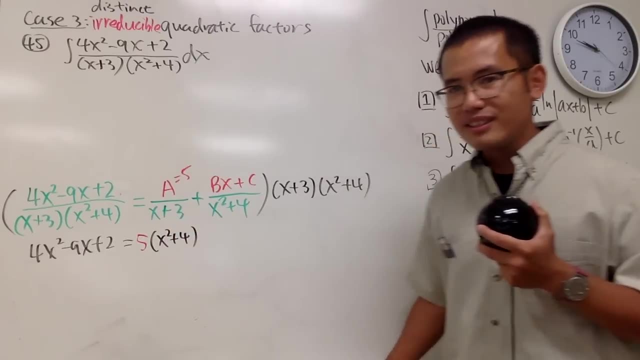 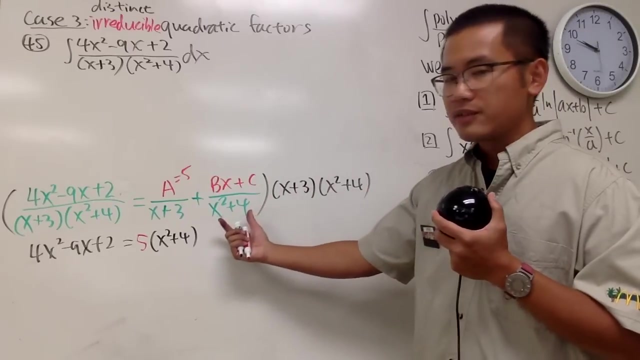 know a already and this, and that will cancel. so we'll just have 5 times that, namely x squared plus 4, like this, Isn't it? Yeah, Then we are going to do this times that, and the x squared plus 4 cancel each other out, so we will say plus. 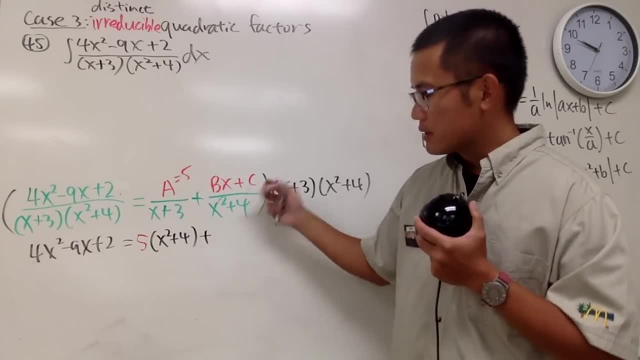 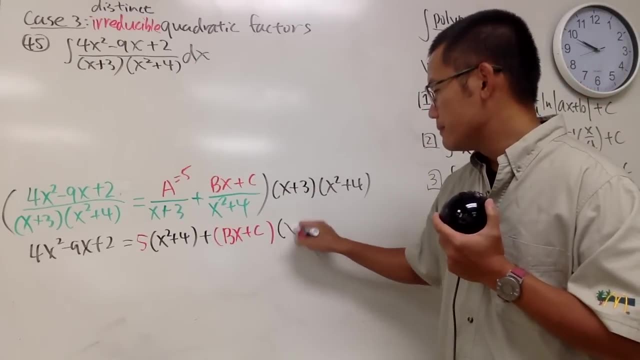 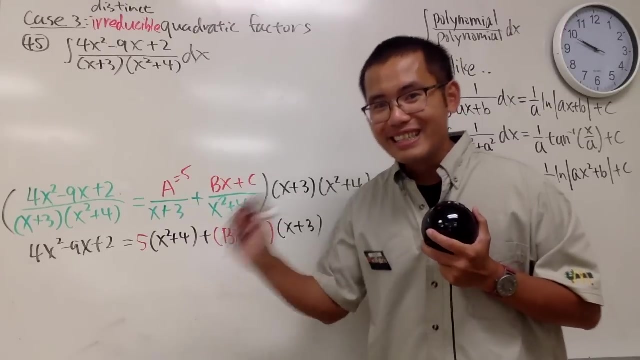 This right here should be put in parentheses, right, Because the whole top Bx plus c and we multiply by x plus 3, like this. And now we are going to focus on the right-hand side and we are going to multiply things out and combine the terms: Here is 5x squared plus. 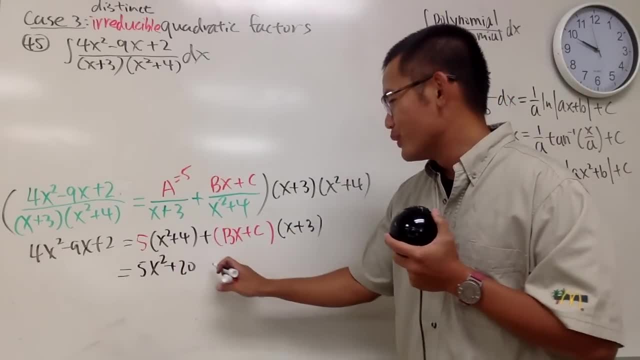 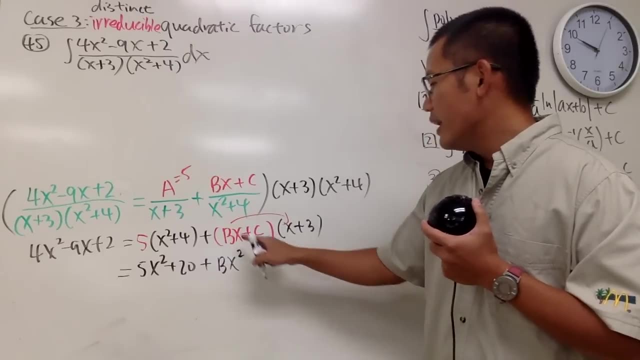 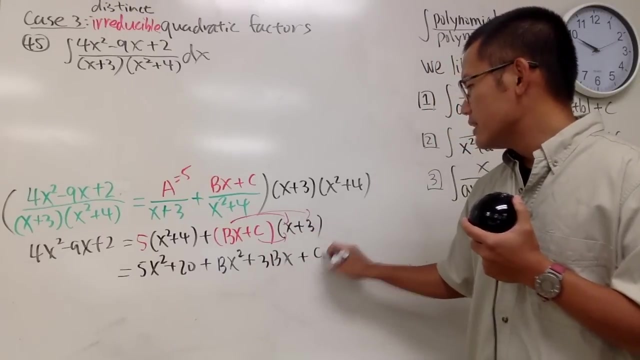 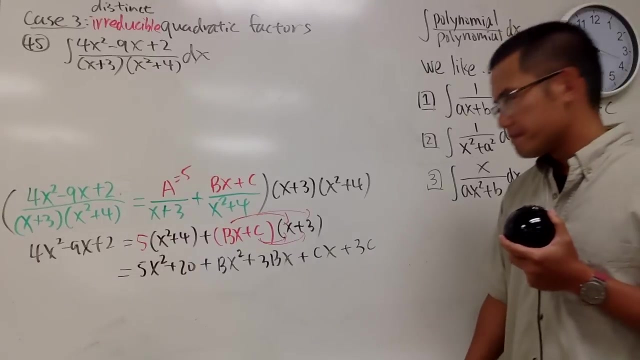 20.. And of course, right here, just distribute another good old day business: Bx times x is bx squared, and then bx times 3 is plus 3bx, and then this is going to be plus cx and lastly, is plus 3c like this. All right, pretty good, huh? Now combine the terms. 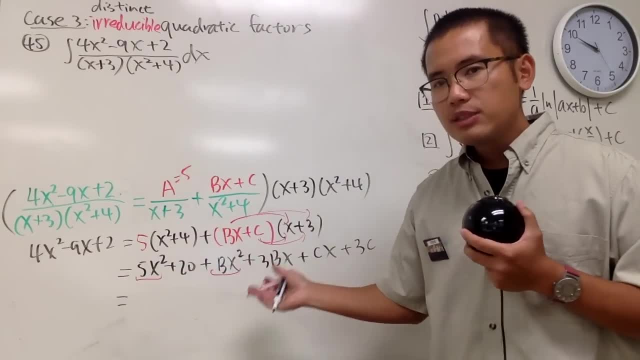 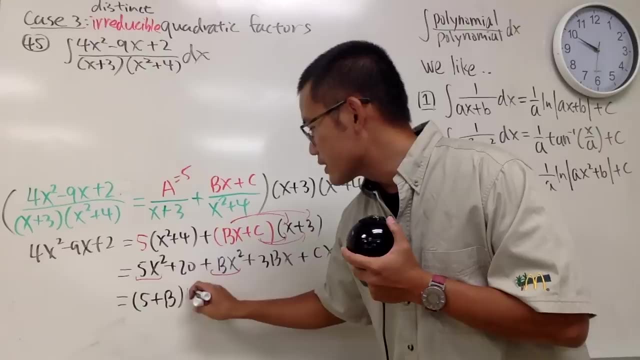 Notice, we have the x squared terms right here and right here and let's just combine it like this way: Open the parentheses with 5 and plus b inside, And then we are going to put the x squared outside, just factor it. put the x squared at the end, like that. 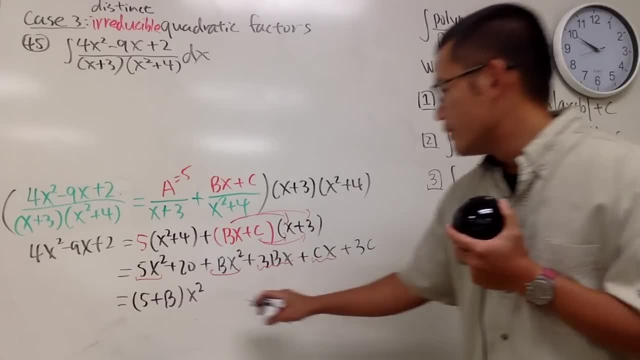 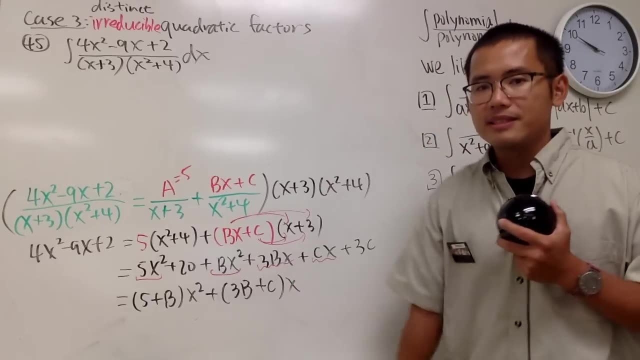 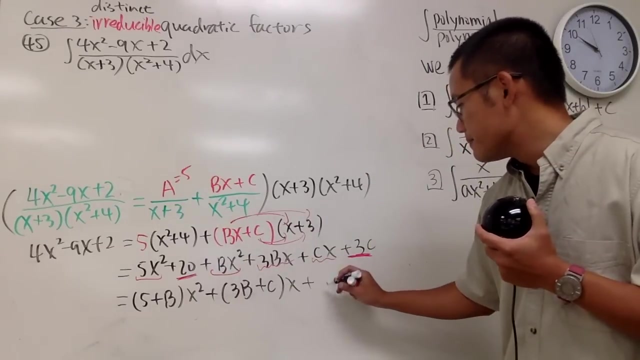 And then the x terms. we have this and that and we have, plus parentheses, 3b and then plus c and put the x at the end like this. Lastly, we have the 20 and the 3c, so plus 20 plus 3c, And these two guys, unfortunately, 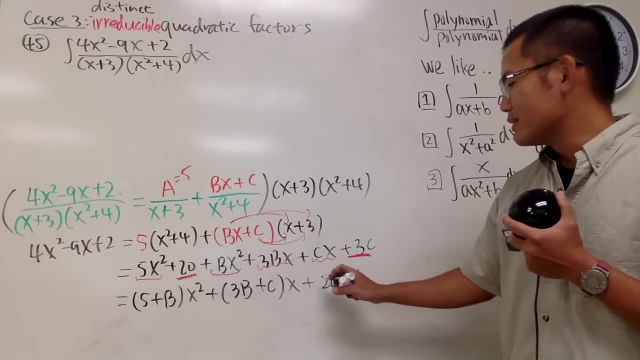 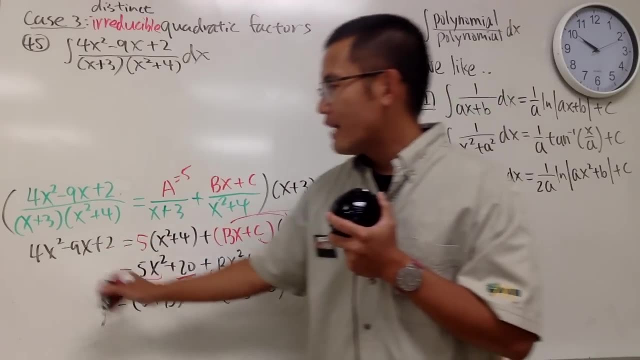 they don't have a number. They don't have a number, They don't have a number, They don't have the x. so that's just pretty much by itself like this. And now, what do we do next? Well, look at the left-hand side. Notice that we have 4x. 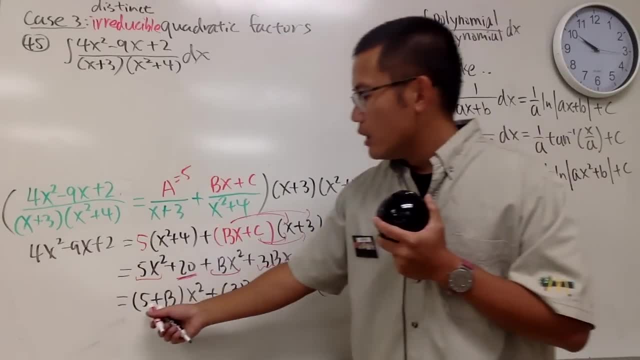 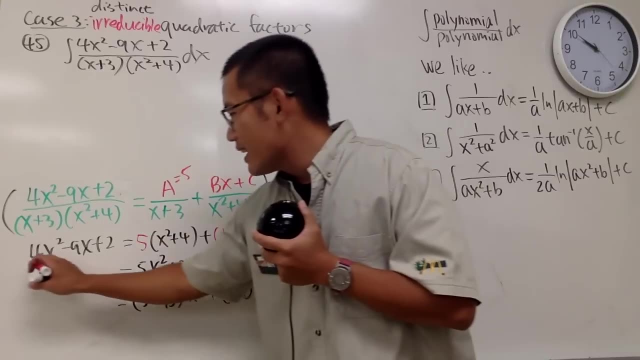 squared On the right-hand side. the coefficient of x squared is 5 plus b. So play, miss and match. In this case, 4 has to be 5 plus b, isn't it? So perhaps I'll do this in greens. 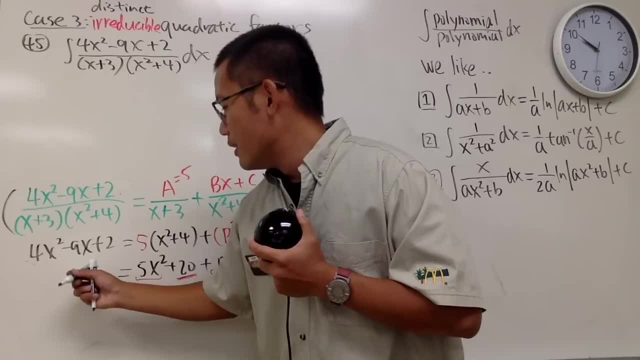 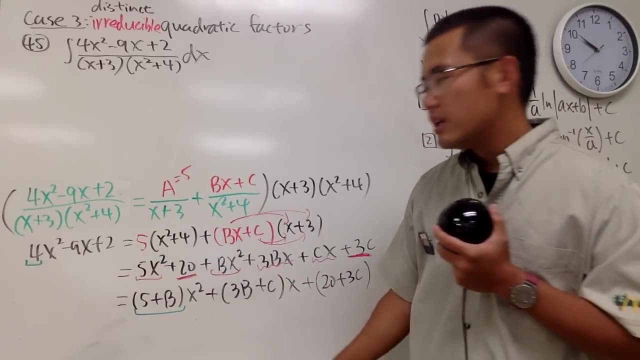 because I used red earlier. 4 has to be the same as this coefficient, Otherwise the left-hand side cannot be the same as the right-hand side. So in this case, we know 4 plus 3.. In this case, we know let. 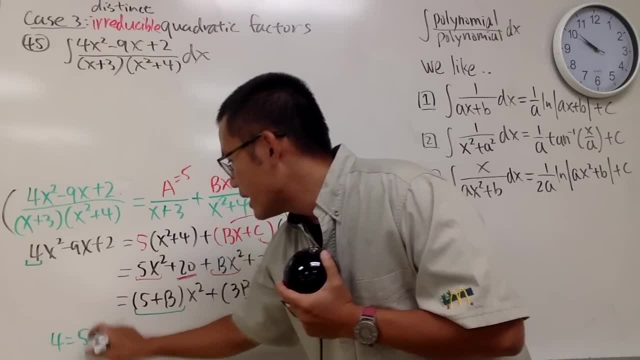 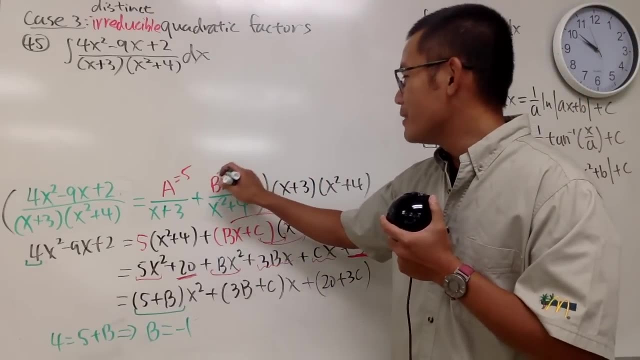 me put it down here: 4 has to be 5 plus b. In another word, b has to be negative 1. So we can come back here and be happy because b is negative 1. And in fact you can just 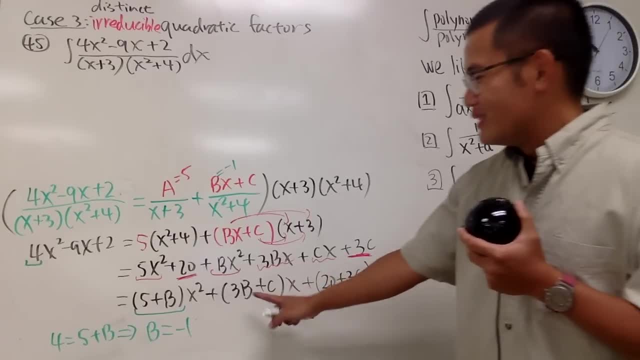 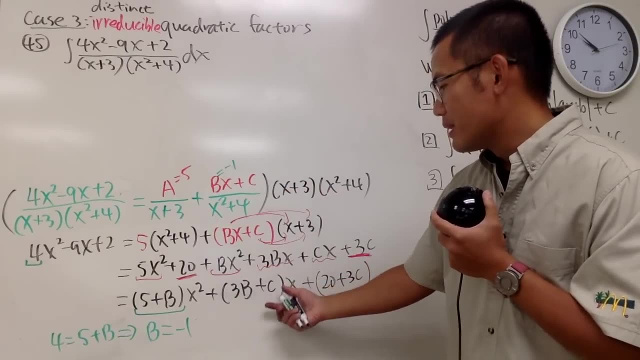 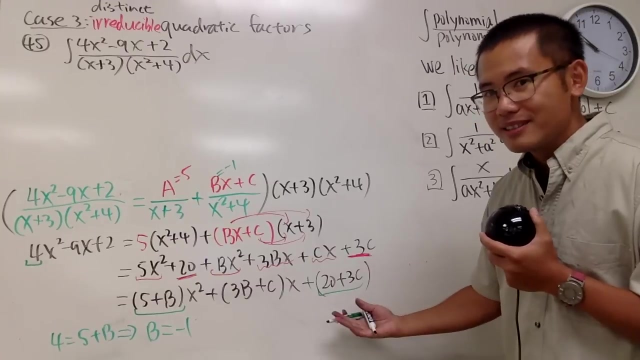 pick down the other ones. whichever one is easy to do. You can use the middle to get the c. b is negative 1, you can put it here: 3b with negative 3 plus c has to be negative 9.. But I will just use this, because 20 plus c- this is the constant term, It has no x. 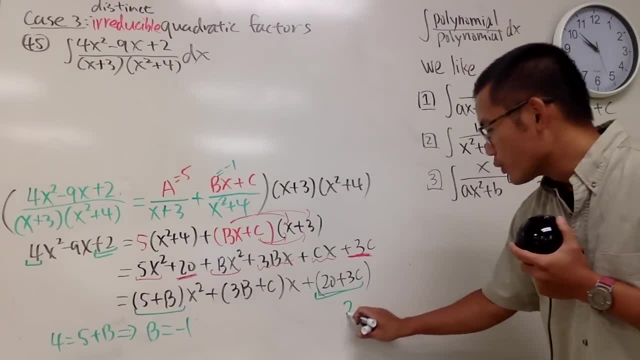 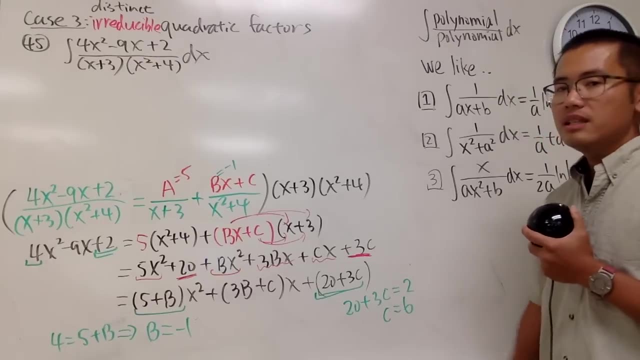 It has to be 2.. So I will just tell you, we know, 20 plus 3c is equal to 2.. And, of course, solve this in your head- c is equal to positive 6.. Well, does it work? if you want to use the middle term, Sure it. 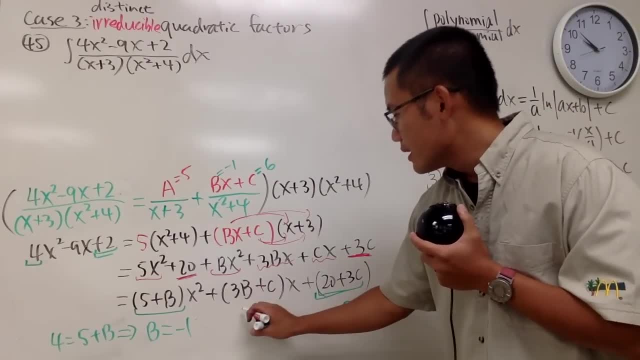 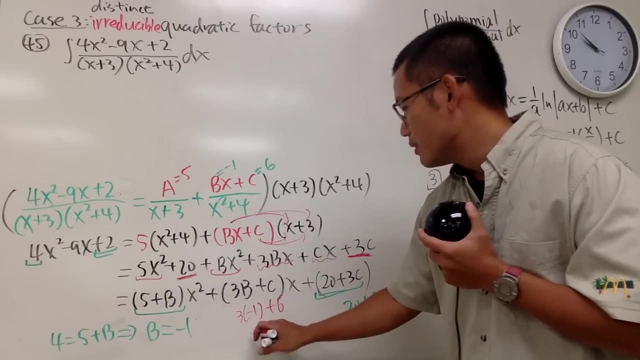 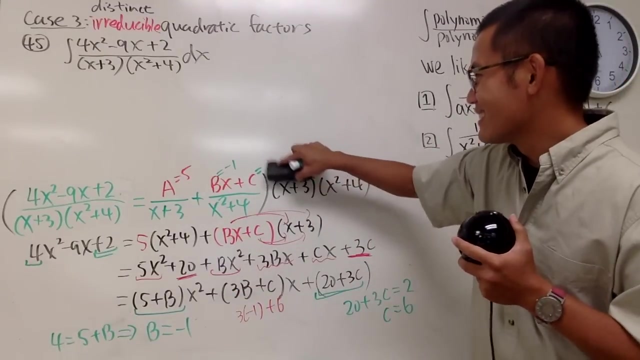 does, because if you do this real quick, you get 3 times negative, 1 plus 6. And that's going to be, oh sorry, negative 6.. Good that I checked. Good that I checked, Because this is 20 plus 3c is equal to 2.. 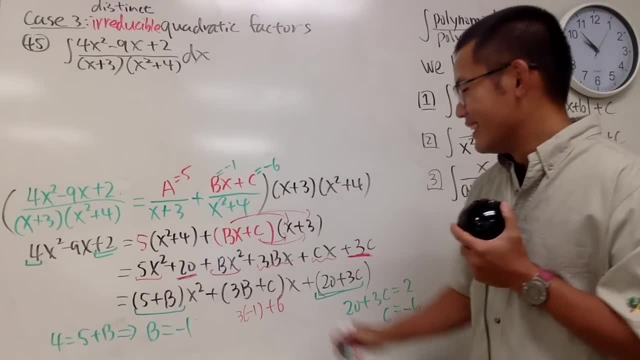 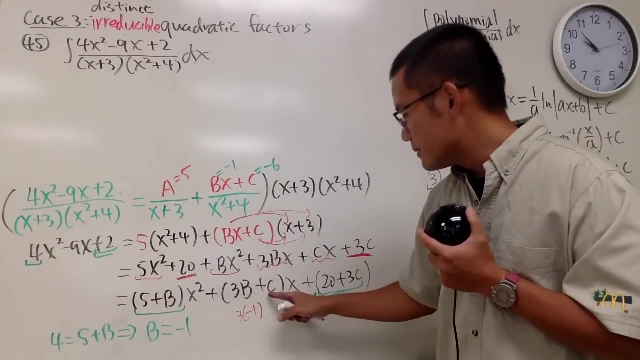 So c has to be negative 6.. So c is negative 6.. And if we plug in this and that into here, well, 3 times negative 1 and c is negative 6.. When we work this out, this is negative. 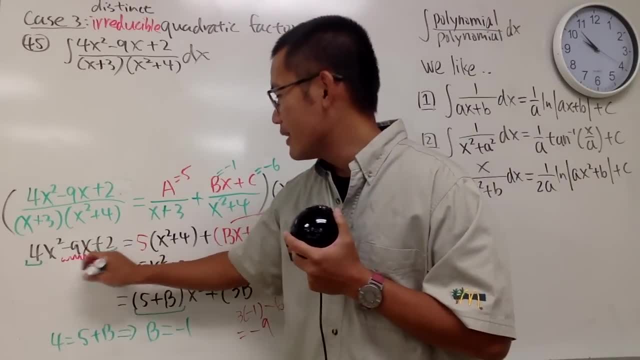 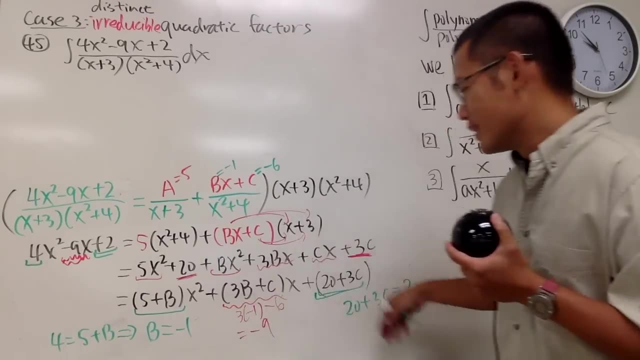 9. And that works out right here. That's negative 9x as well, So it just makes it match the coefficients. I think this is the easier way to. this is the how should I say more consistent way to do it. 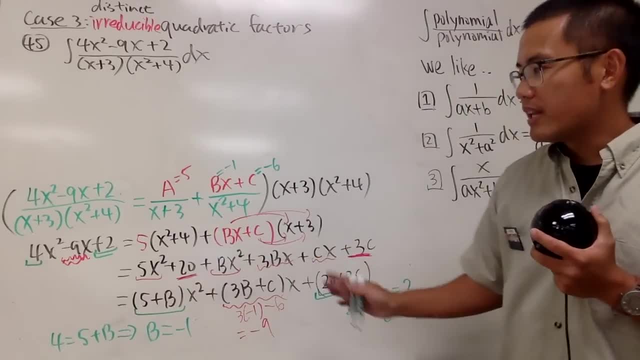 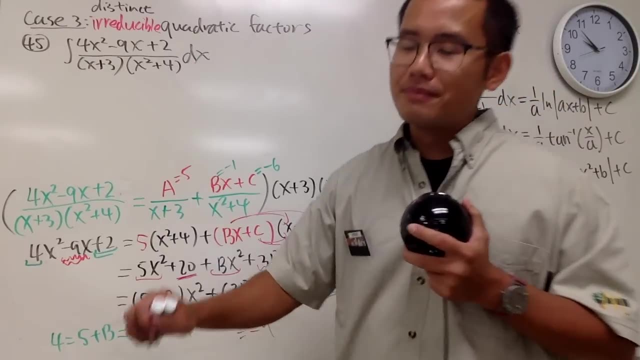 Do the cover-up whenever we can. For the rest, when we cannot just multiply it out and equate coefficients Just like that, Okay, We did a lot of work already, But so far we haven't done any integration yet. 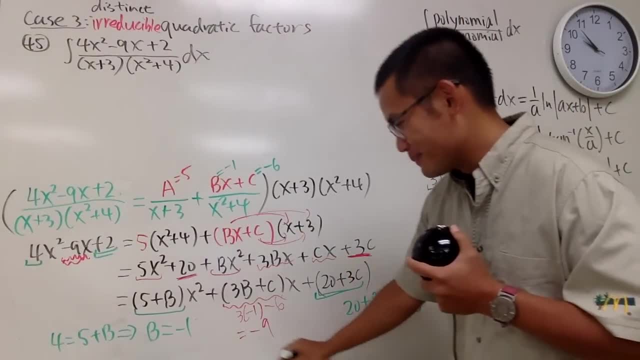 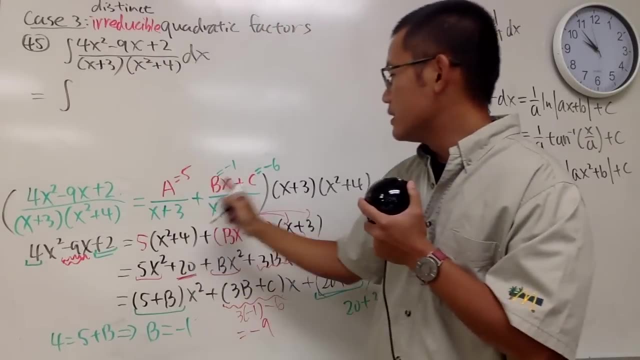 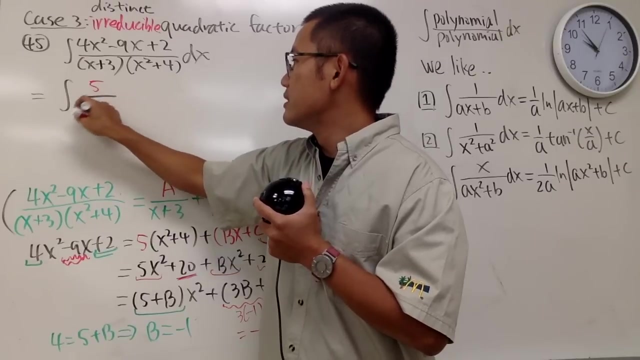 Well, it's about time to do the integrals, So we will. Here's the deal: Integral: All this is equal to this, this, that First thing. first, we have 5 over x plus 3. This is the innocent one, This is the cute one, the one that people like the most. Next, 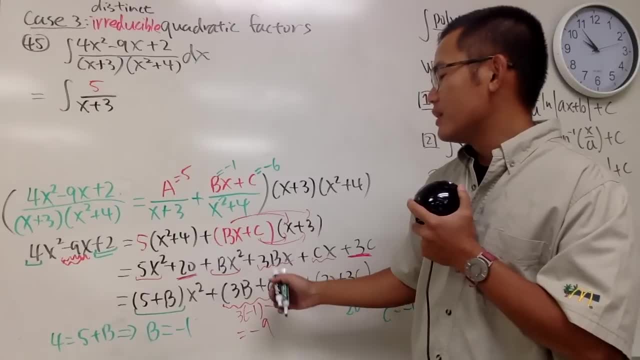 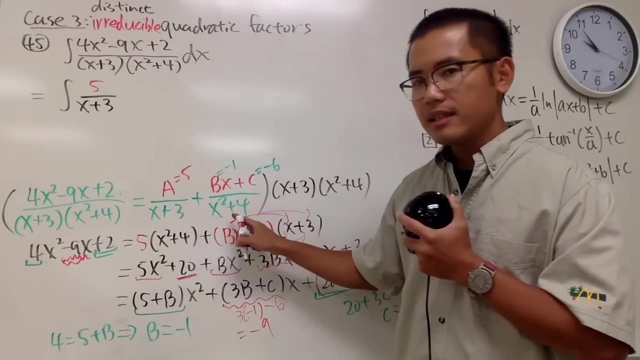 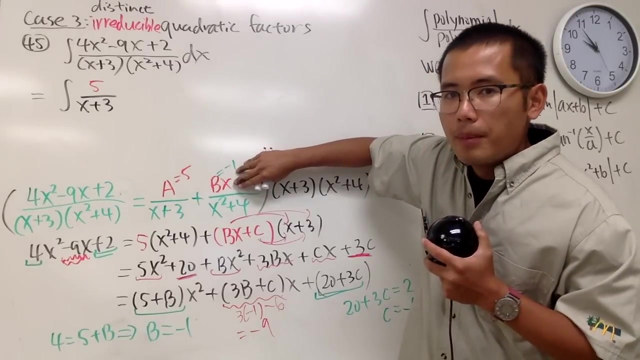 we have. Next, we have negative 1x over that And you see, we like to have this to be integrated. So I'm just going to split the fraction Bx over this and then c over that when I integrate. right. So the whole thing is the same thing. All the 된 and the then and the then, the same thing. Yes, we have the integral, This is the integral over them right, And we can take it And we take the integral, and we can take the integral right And we take. 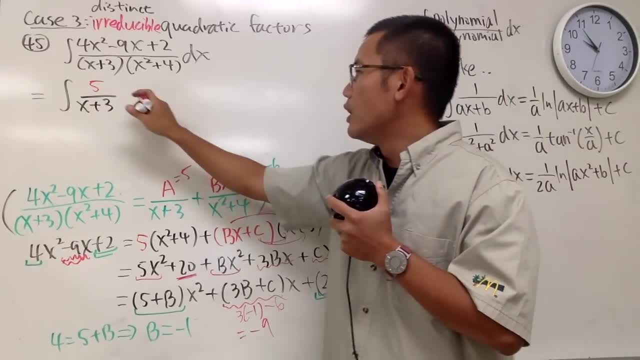 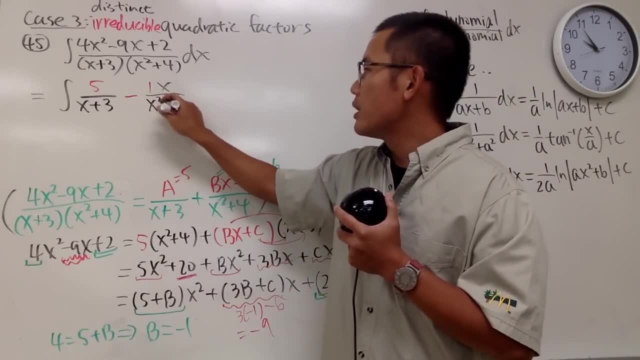 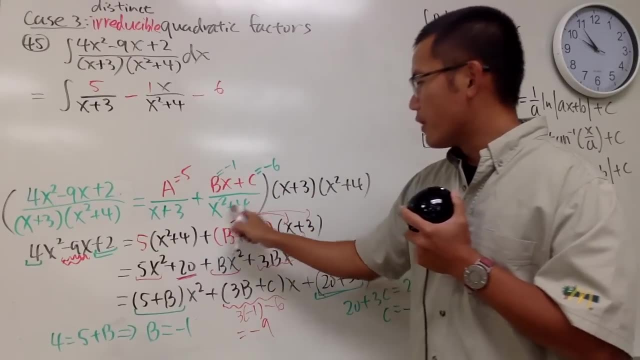 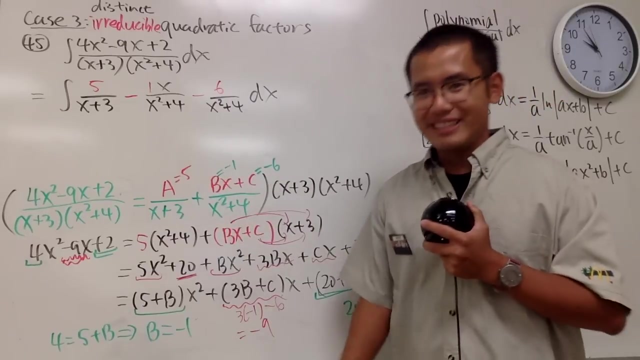 over this denominator, which is x squared plus 4.. And lastly, we have the minus 6 over this guy. We have the over x squared plus 4, like this. That's the idea. Now for the first one, of course. that's the natural law situation. 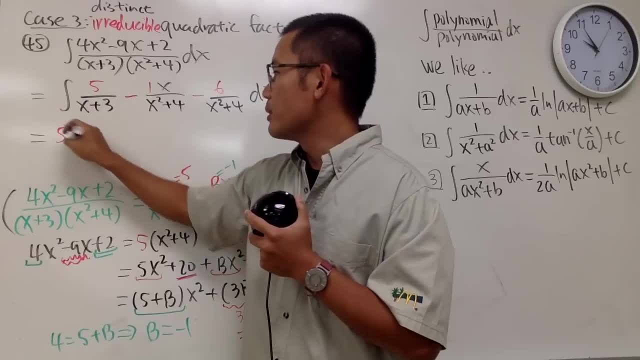 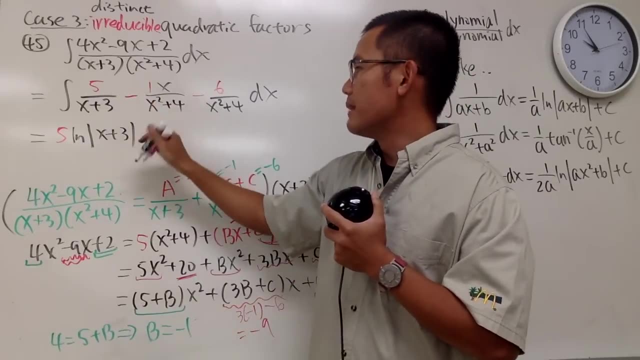 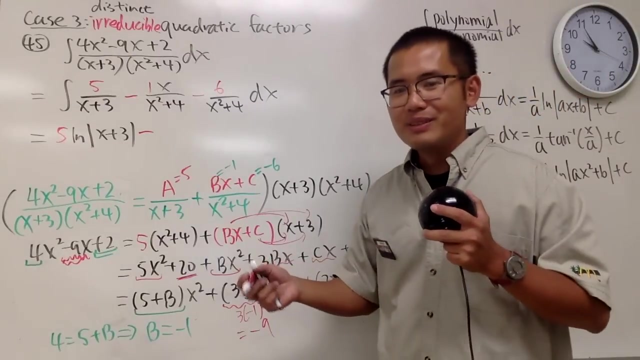 because the bottom is just linear and we will have a constant multiple of 5, natural log absolute value of x plus 3, like this: Next, this is minus. keep it. Use this formula if you would like, or you can just do this in your head. use substitution. 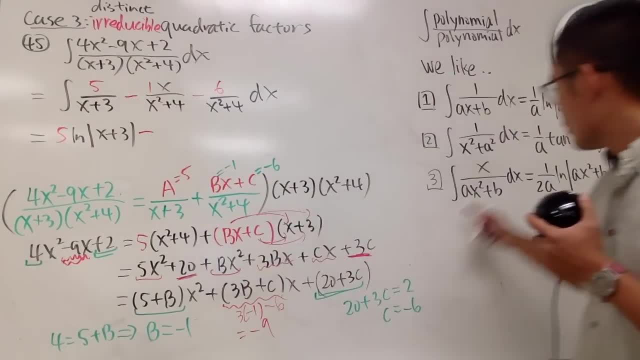 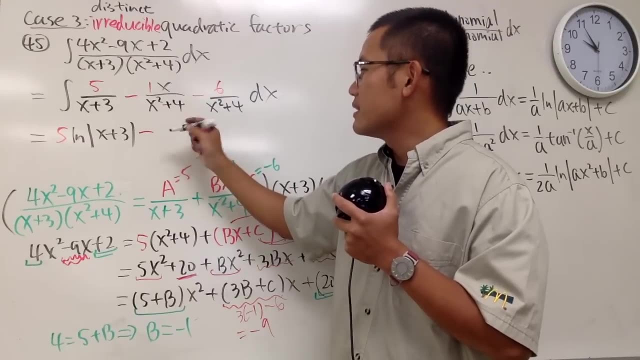 But only all. the 1 doesn't really matter. And then, don't forget, divide it by 2a, and then the a right here is 1, so it's just 1 half. So the part in black is just 1 half. 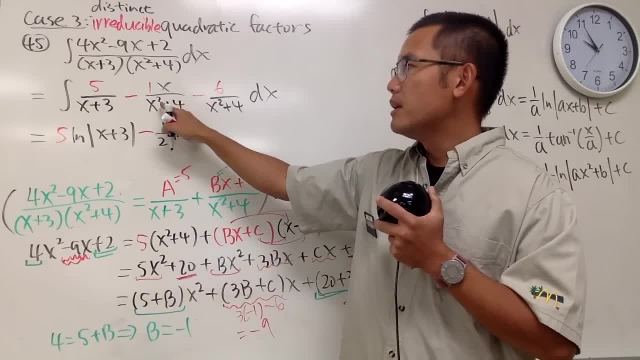 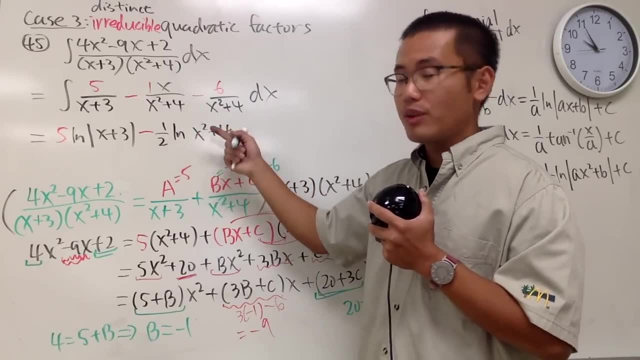 This is also a natural law situation, because we have the x on the top and this is x squared plus 4.. Here we have x squared plus 4, but this is always positive because we have the plus 4.. So parenthesis is enough. 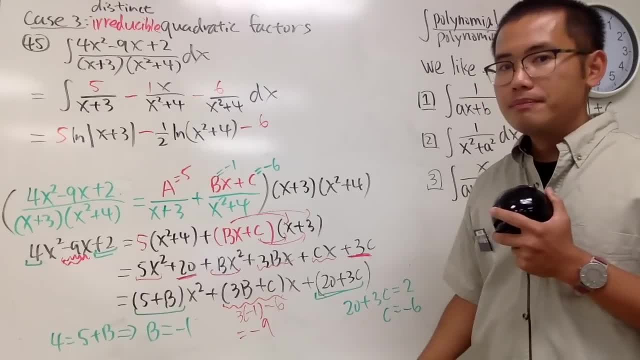 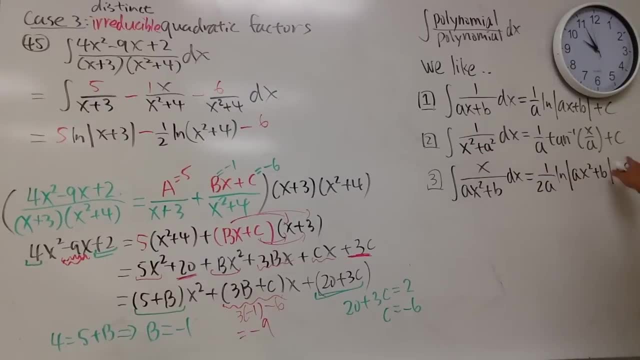 Lastly, let me write down the minus 6 right here. But if you look at this as just a constant 1 over x, squared plus 4, that's fine. That's this situation. So we have to look at the 4 as what. 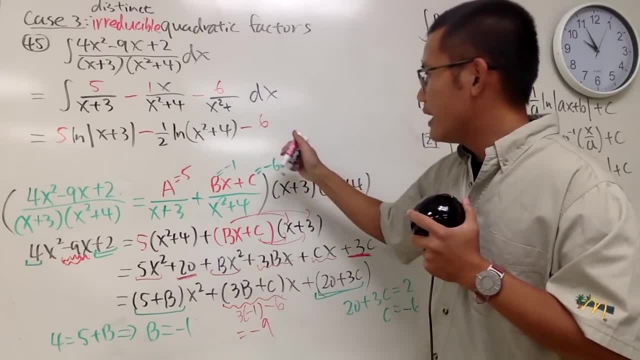 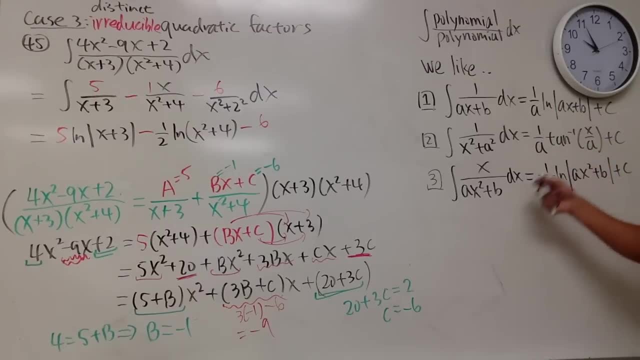 2 squared. So let me just rewrite this and I'll just put this as 2 squared. Well, to integrate this part, we do 1 over a, so 1 over 2, so we have the over 2 right here. 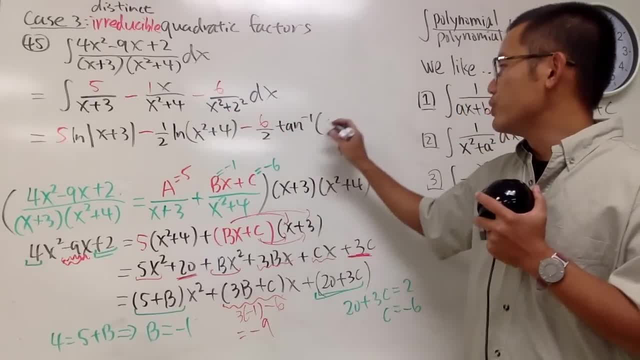 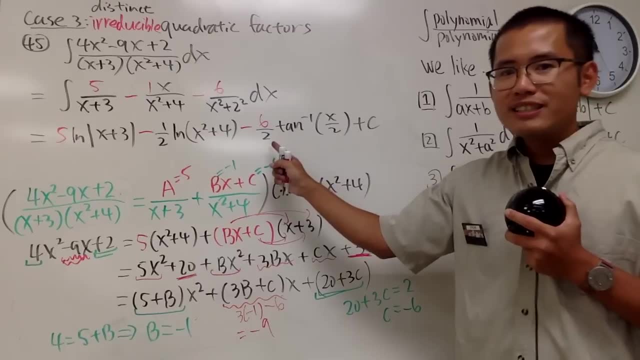 and then inverse tangent x over 2, like that, And then in the end we are done plus c. But seriously, are you serious, Are you serious If you leave negative 6 over 2 on the test? seriously, don't do that. 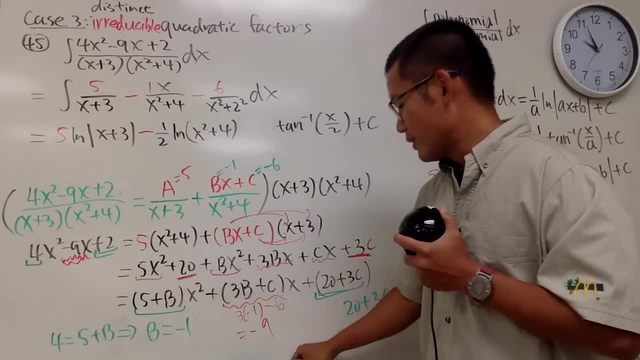 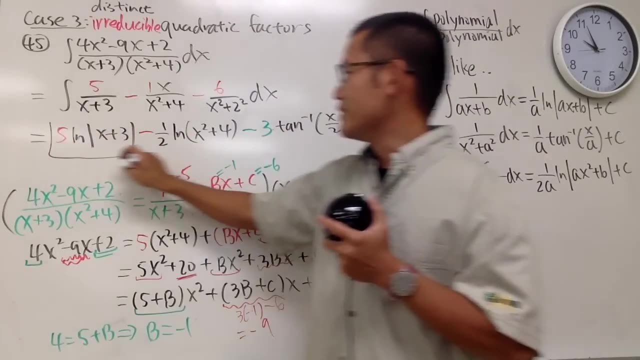 Just change that to be minus 3, right? So hopefully you guys are actually watching me doing this step by step, so I'll just change this because I don't want to write down the other things over again. So this, right here is it. 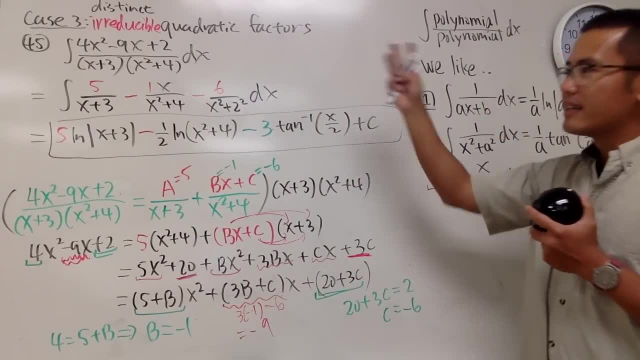 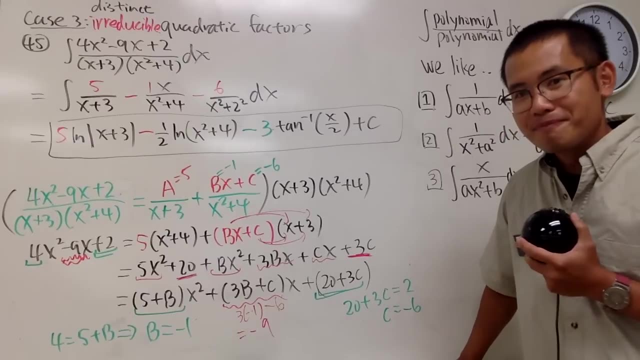 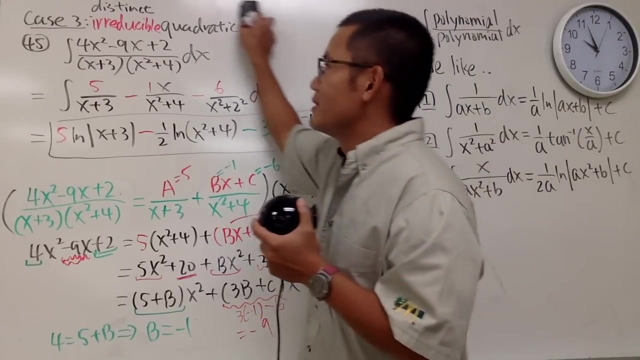 And you can just do that. So that's it, Case 3.. Case 3. Perhaps the longer, the longest case. All right, Seriously, a couple more questions. Okay, I cannot do this before 10 o'clock 11.. 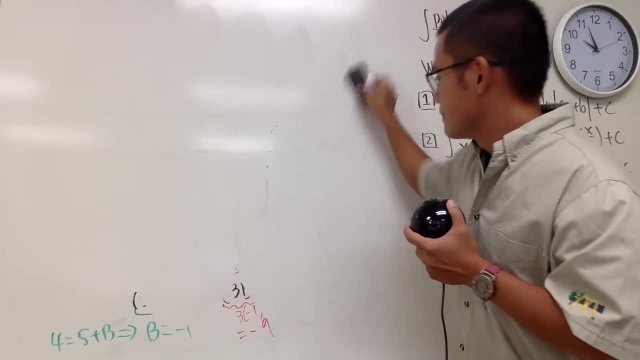 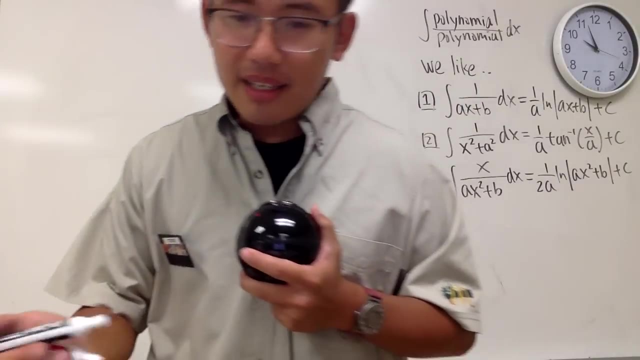 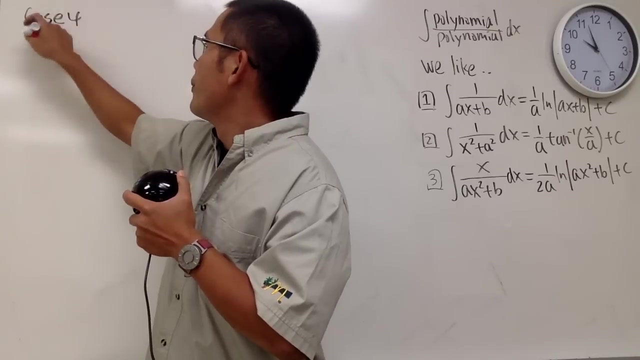 I should be able to finish this by 11.. Okay, So next one. I will tell you guys what the case is, This case 4.. We have the following: We have the following situation: Okay, Let me ask you guys this: 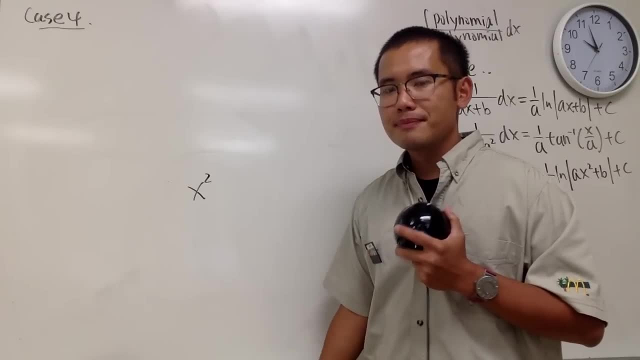 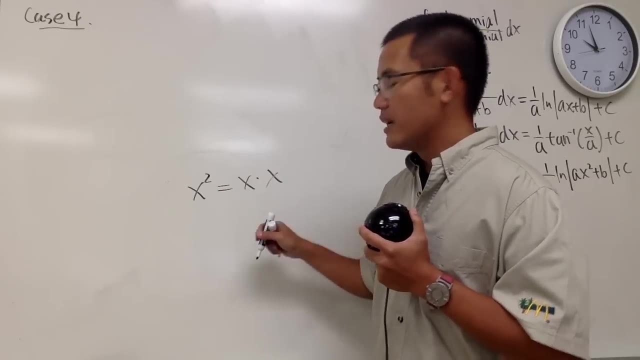 If you see x squared, is this quadratic or not? Sure, it is. You can look at this and how it is, But you should break it apart. If you break this apart, you have x times x. Namely, you have x to the first power times x to the first power. 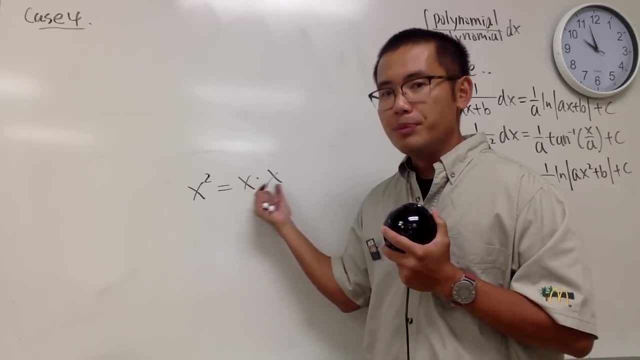 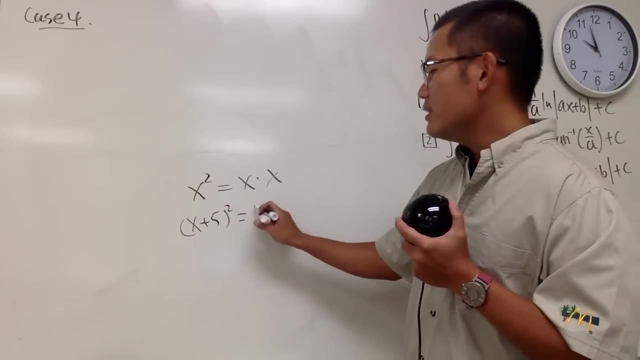 In other words, the linear factor x is being repeated twice, Right? Similarly, when you have x plus 5 squared, look at this as x plus 5 times x plus 5, of course, Sometimes you may have this kind of situation. 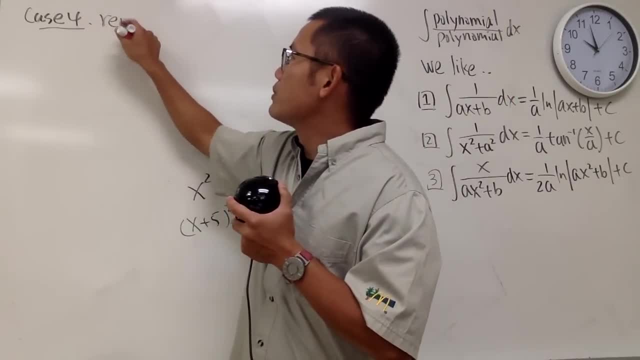 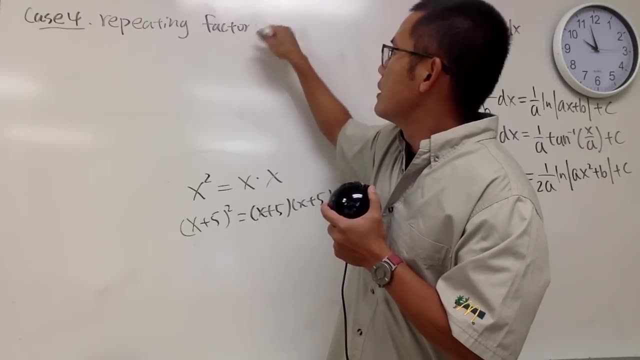 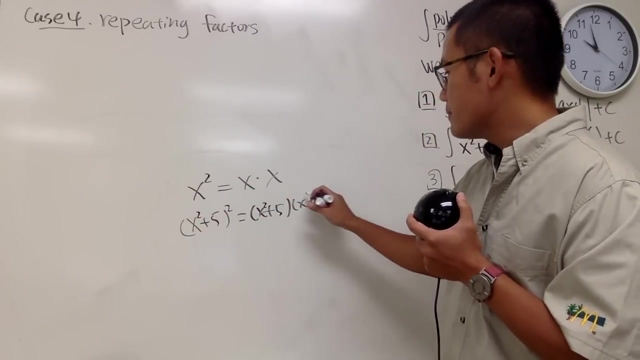 That's case 4.. This right here is- I will just call it the repeating factors. And sometimes, of course, you may have x squared plus 5 squared. That's x squared plus 5 squared. So x squared plus 5 squared is x squared plus 5 times x squared plus 5.. 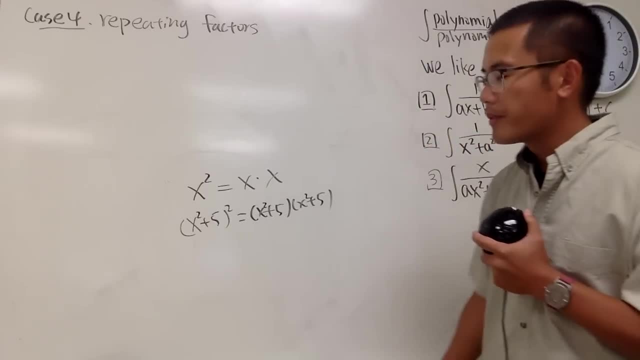 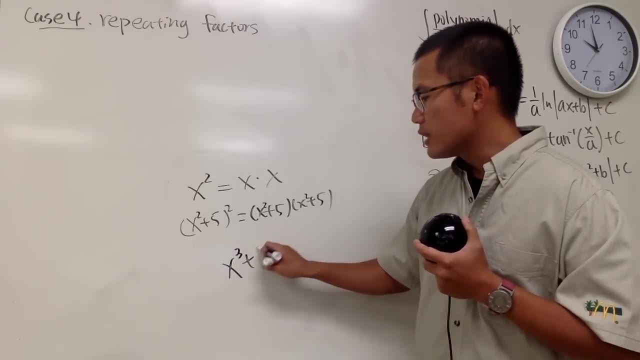 So you can also have the quadratic ones being repeated as well. And if you are thinking about what happened to the cube, well, the truth is, if you have a cubic expression like this, you can always factor it down. It just depends on the difficulty. 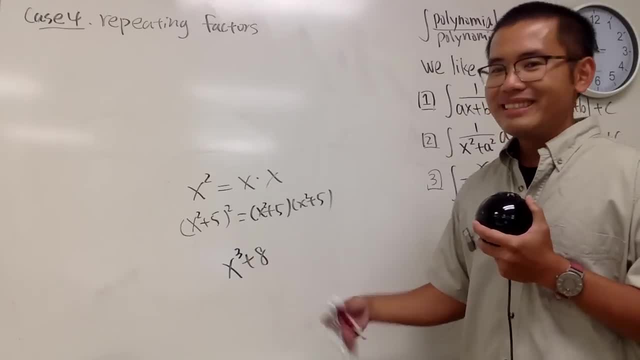 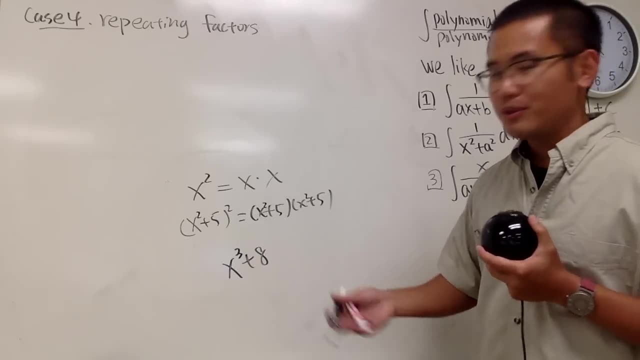 Right. So usually it would be just a nice expression that we deal with by hand in Calc 2.. And if it's like a bizarre cubic, then good luck. That's all I can say. Repeating Factors for this case. 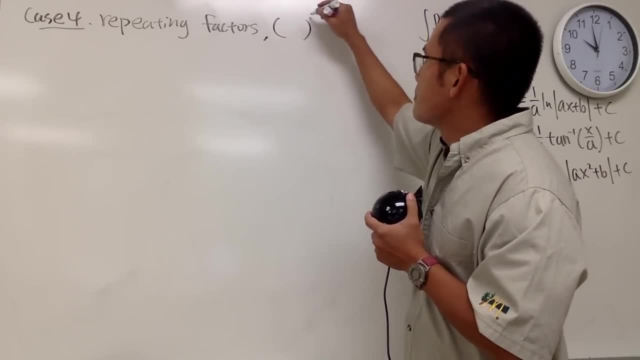 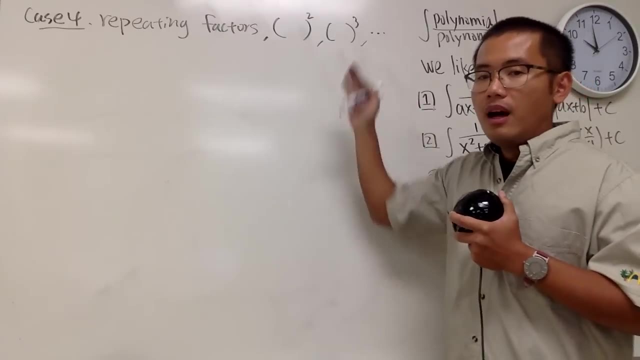 Pay attention to the following form: Pay attention to a parenthesis to some power, And most likely we'll be doing like parenthesis to a second power, parenthesis to a third power, etc. etc. No 2.5,, no 3.5, because again, they will not be polynomials. 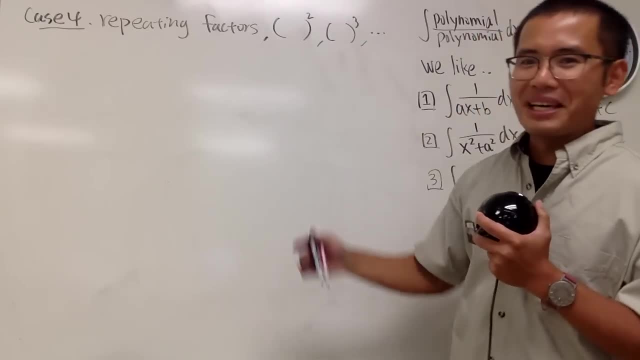 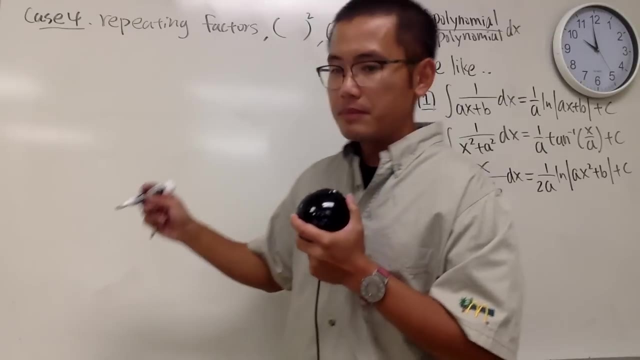 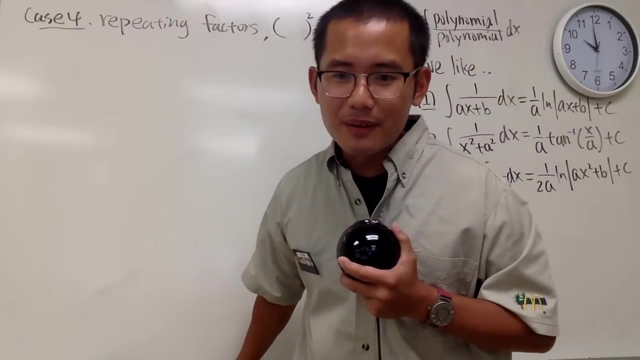 If you have this parenthesis to a first power, that's just the previous cases, right? So that's case 4.. And I have this question for you guys. This is question number. Oh man, I forgot to do the other question earlier. 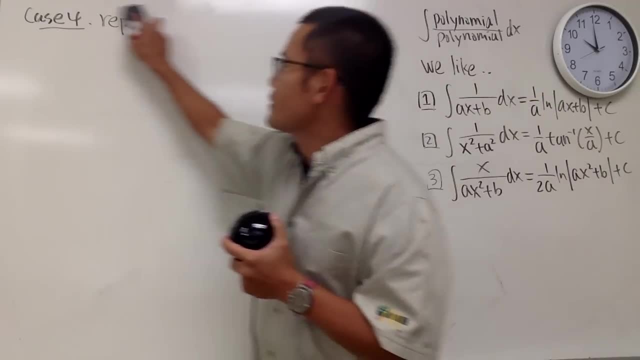 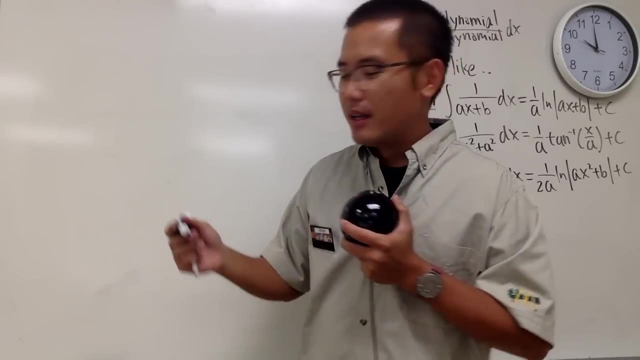 Okay, I will do question number 46 right here. Okay, I will just repeat my little speech earlier. I will just make the timestamp to here. I'll do 46, 45. Okay, So let's take a look of another situation for the irreducible quadratic. 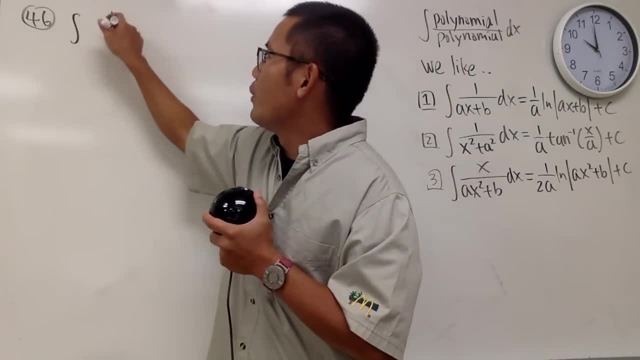 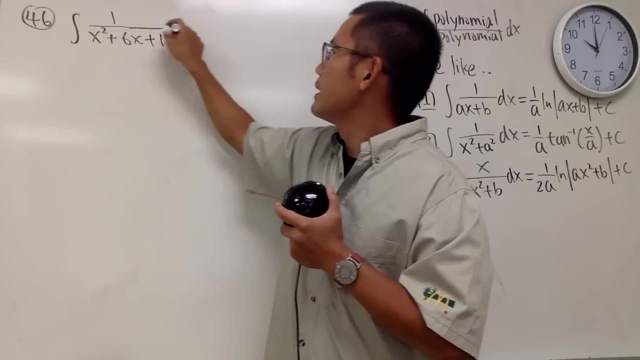 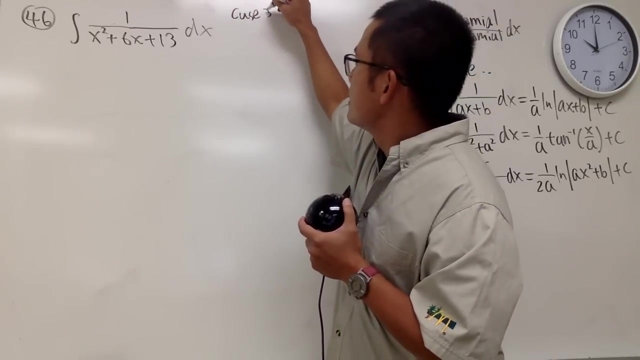 This is question number 46.. Let's look at it: Integral of 1 over x squared plus 6x plus 13.. This is still case 3, right? So still case 3.. Well, look at the bottom here. 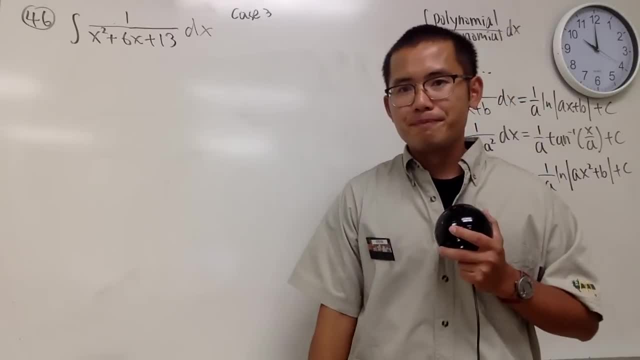 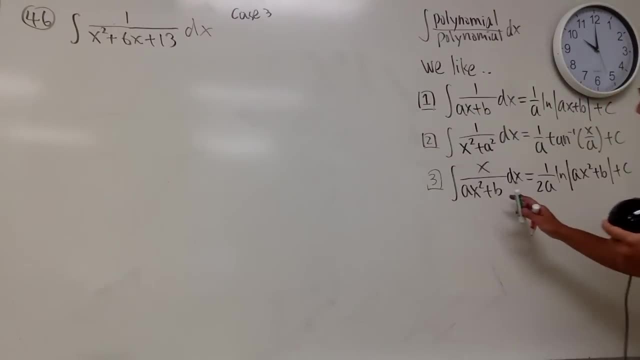 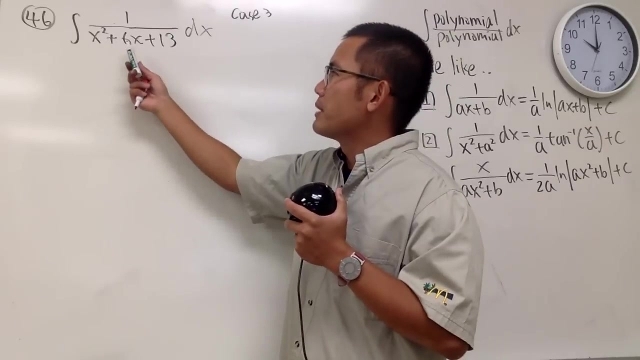 x squared plus 6x plus 13.. Can we factor it? Unfortunately not. Hmm, In this case that's no good. And Notice right here, for example, we only see the x one time, But here we have x squared and then plus 6x. 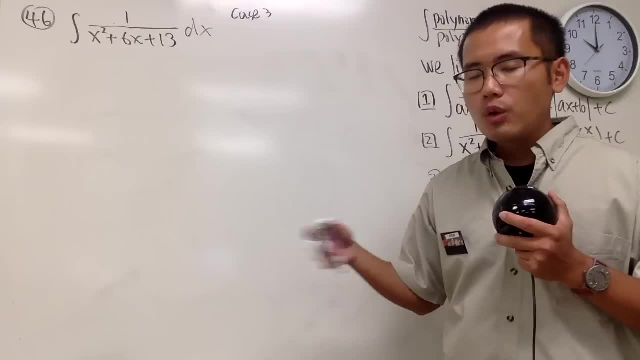 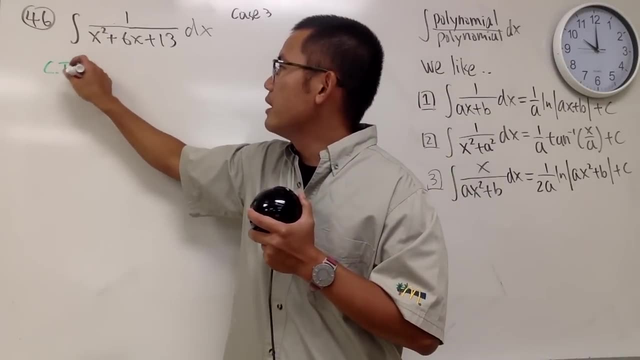 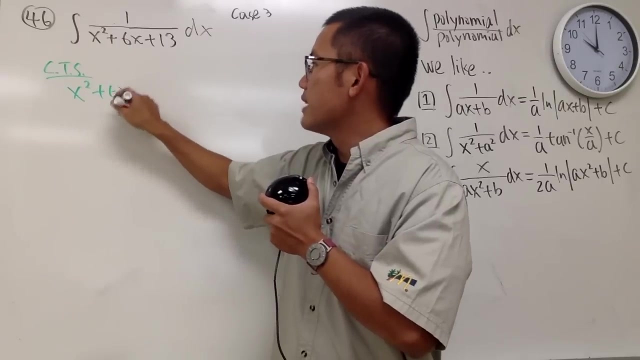 We see the x twice. In such situation, what we can do is just complete the square. So let me show you We are going to complete the square And let me show you, guys, how to do it. right here. Write down the denominator x squared plus 6x. 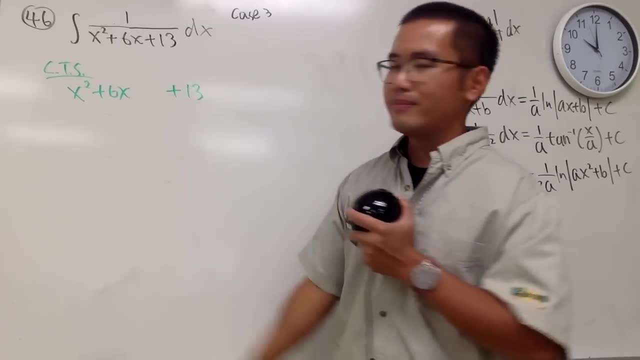 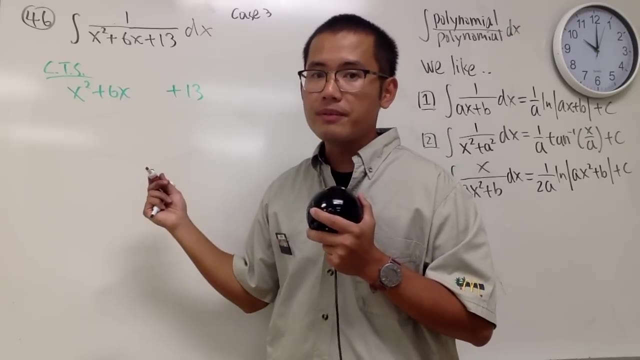 But right here, leave a space because you are going to work out the magic number. The magic number is the following: First, make sure that we have a 1 in front of the x squared, which we do, That's great. Then move to the number in front of the x, which is a 6 in our case. 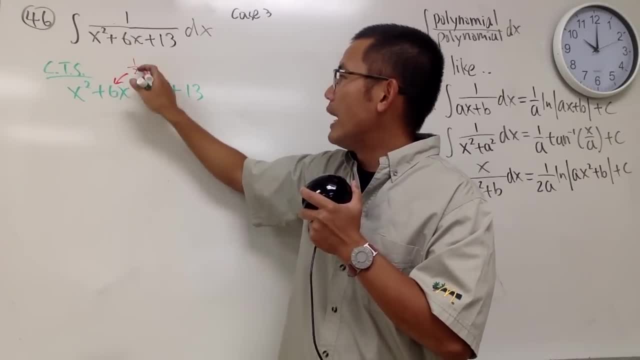 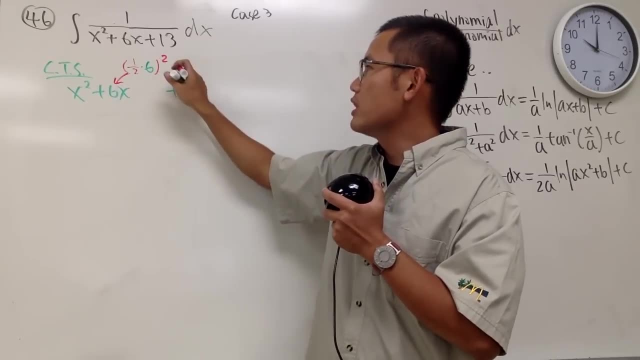 Then multiply this by half. Take half of this, so multiply half with this, And then put in a parenthesis and square that, And this is going to give us 3 inside squared, which is 9.. And we are always going to be adding the matching number right here. 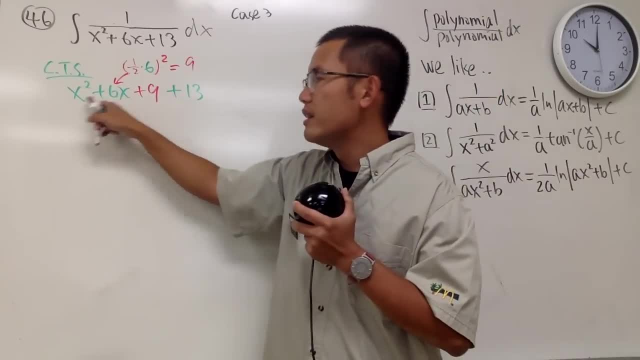 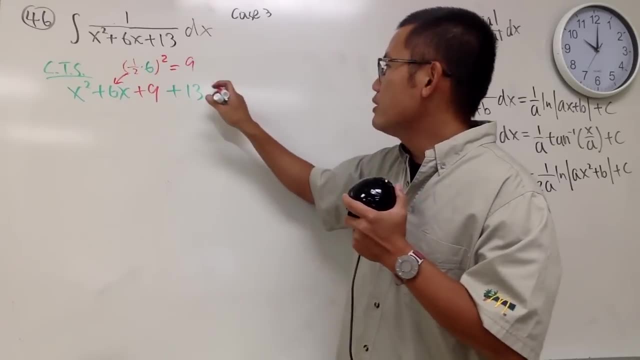 This number is so magical because it's going to make the first three terms a perfect square, But of course, if I add 9 to this, I change the whole thing. That's no good. It's okay, though, because we can just subtract that after that. 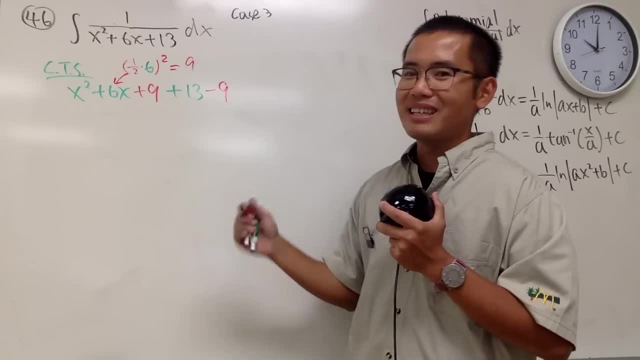 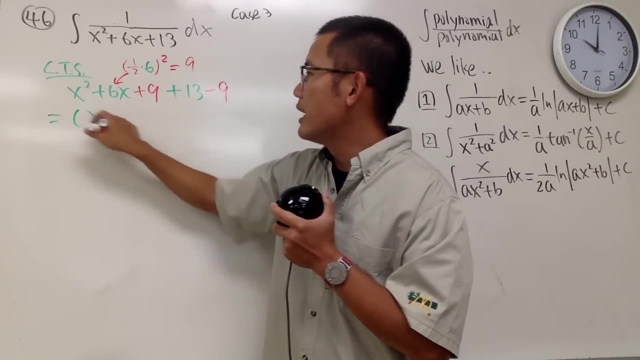 So we still have the same exact expression after we do all this. All right. So you see, this right here is actually just x plus 3 times x plus 3.. So this is x plus 3 squared. So this is x plus 3 squared. 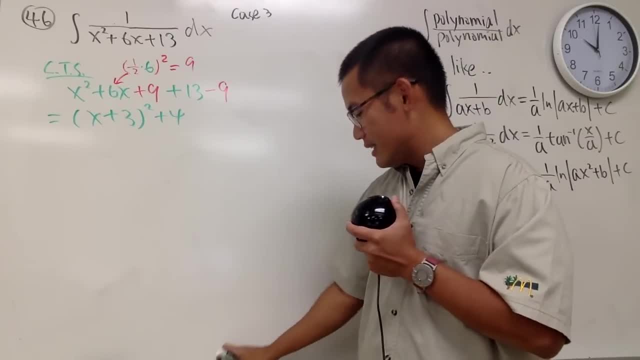 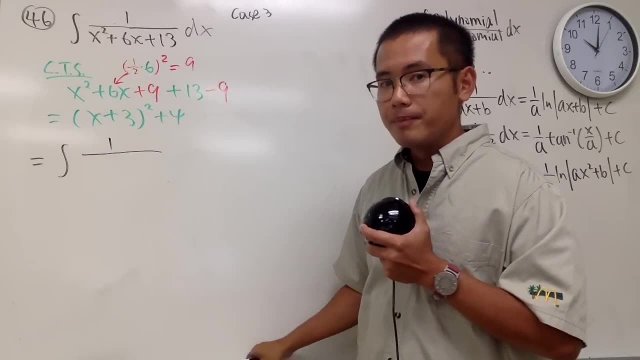 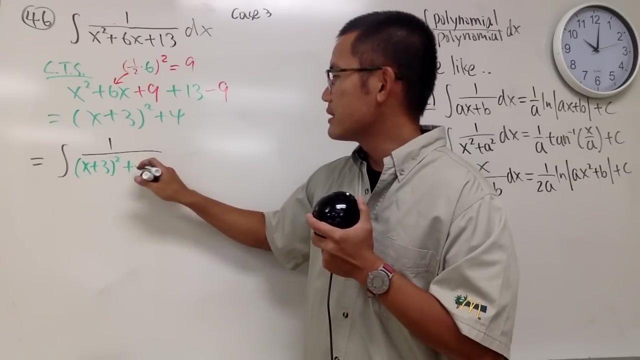 And then this right here is just plus 4, like this: All right, So now look at this as the integral: On the top we have 1. And on the bottom we have this now, which is x plus 3 squared plus 4.. 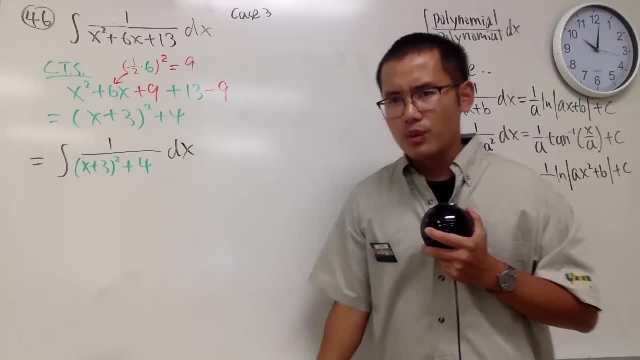 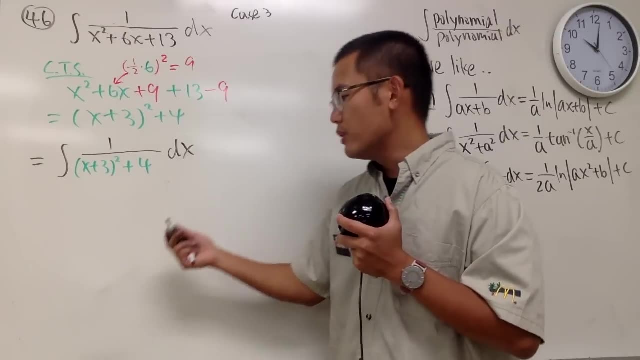 And then, of course, we have the dx like that. Well, what can we do next? Well, when we have x plus 3 squared, this right here will be a good choice for you, And I'll just do a use-out real quick for you guys. 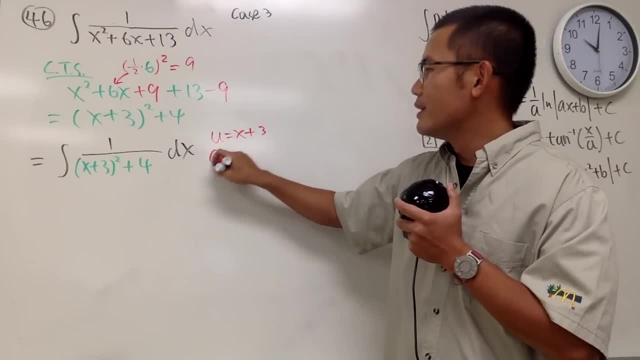 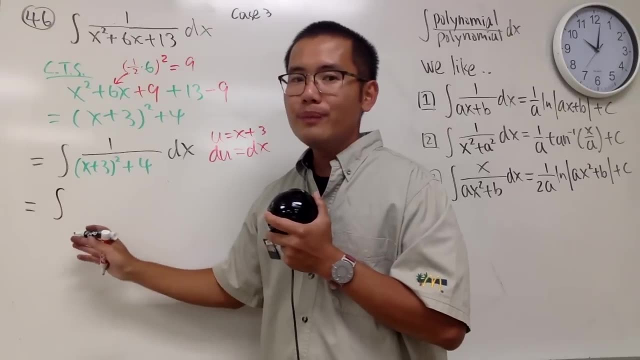 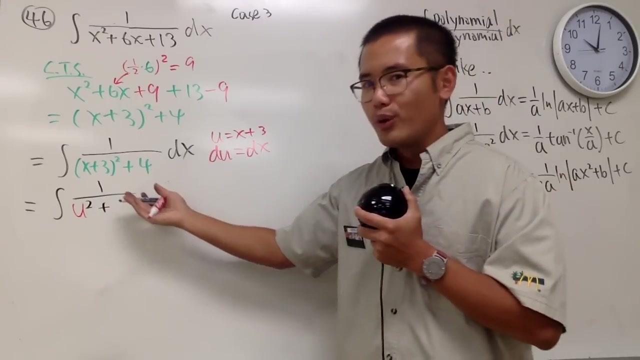 u equals x plus 3.. And yes, du is nicely equal to dx. In another word, you see that after completing a square, we get the integral of 1 over u squared, plus What for the 4?? You guys know I'm about to use this formula. 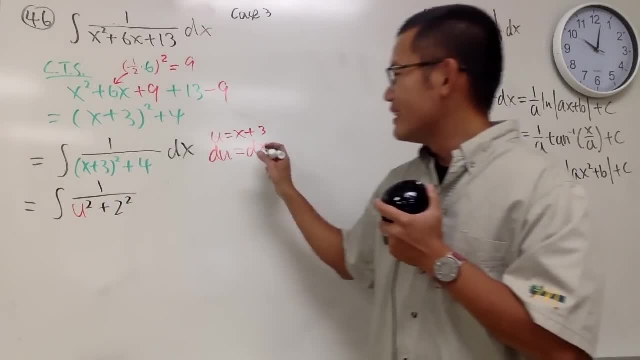 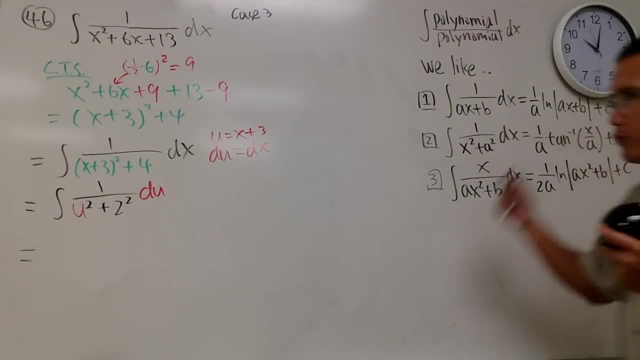 So let's look at this as 2 squared, And then the dx is the same as du, And that's so nice, Yeah, Yeah. So now, by using this formula, we have 1 over a, namely 1 over 2.. 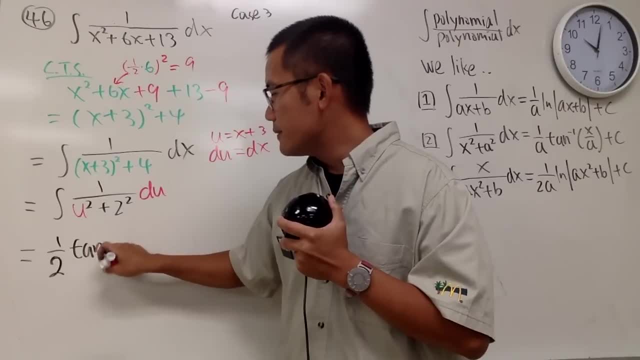 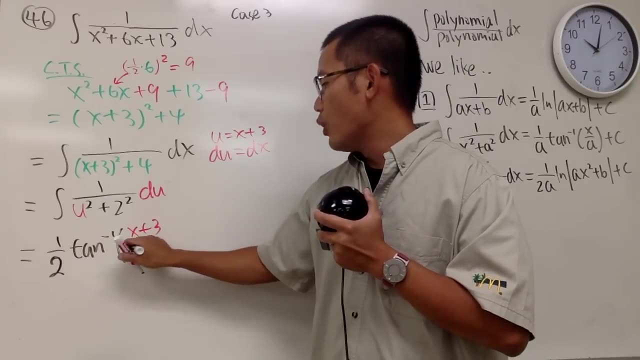 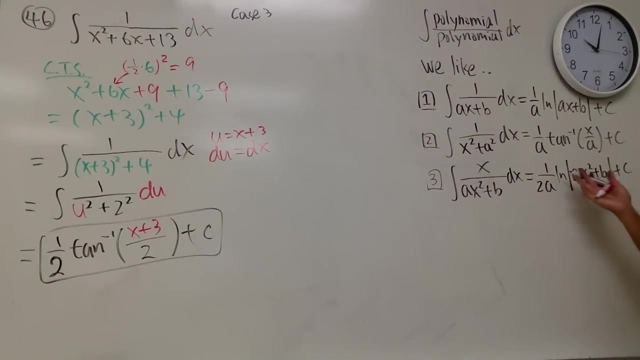 So we have 1 over 2 right here, Inverse tangent of u over 2.. But u is this, So I just put down x plus 3 over 2.. And with that we are done. Okay, The inverse tangent is used whenever the bottom is a quadratic. 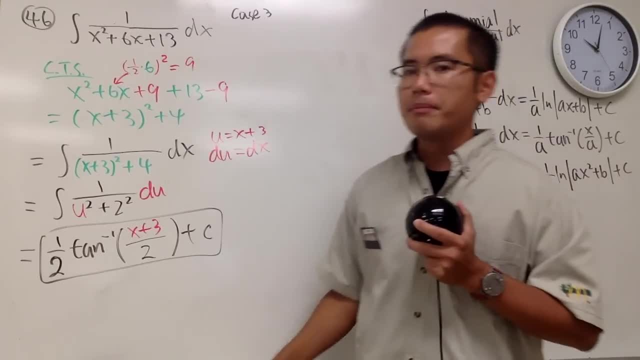 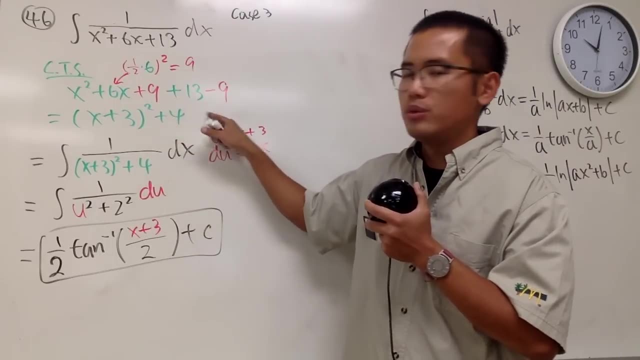 and it does not have any real root. So that's what we mean by irreducible: We cannot have any real root. And if you, The idea is that if you set this equal to 0, you cannot solve x with real numbers. 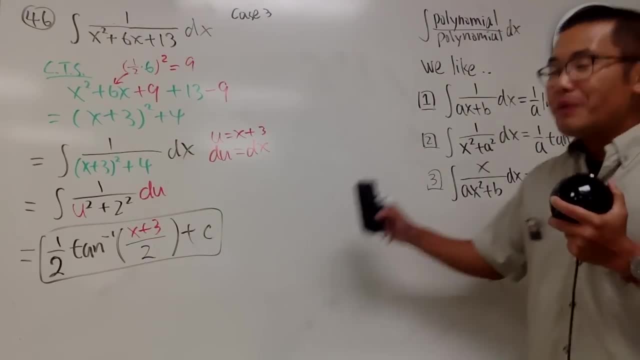 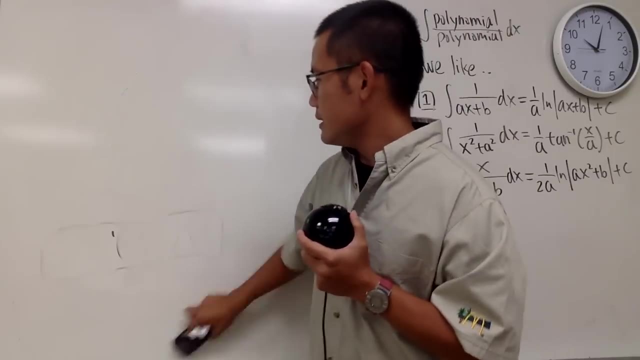 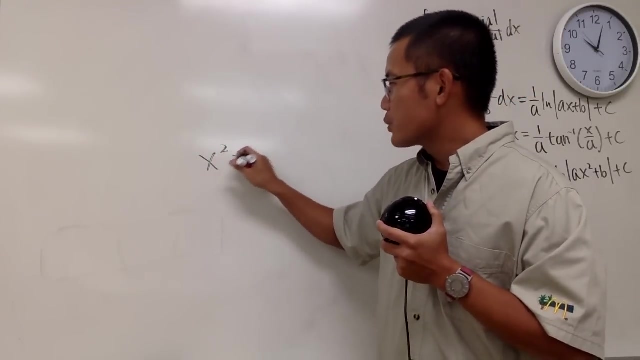 That's what I mean by no real number root. Okay, That was case 3.. And now let's move on to case 4.. Last case: Okay, For this case, let me ask you guys this: If we have x squared, is this quadratic? 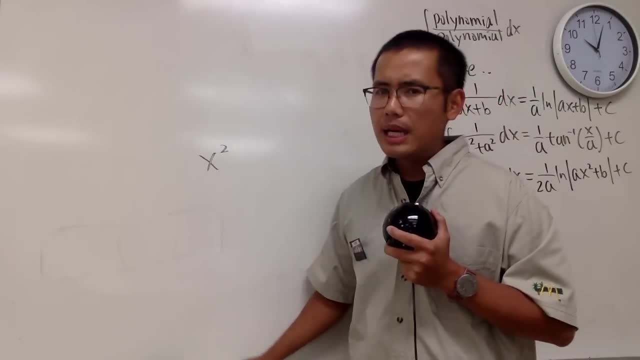 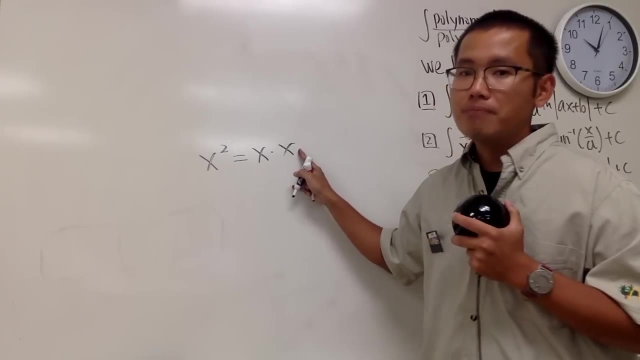 Is this quadratic or not? Sure it is. But can we also look at x squared as x times x, Namely x to the first power times x to the first power? Yeah, So in this case this is just a linear factor repeated twice. 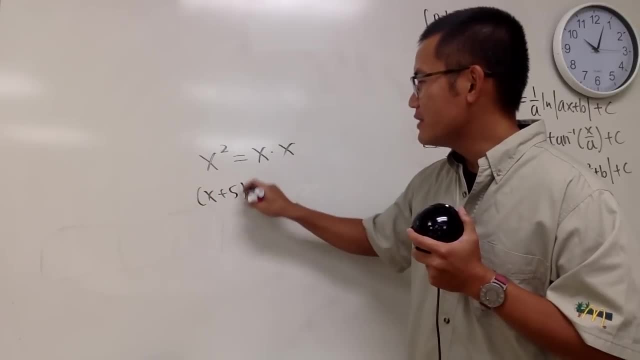 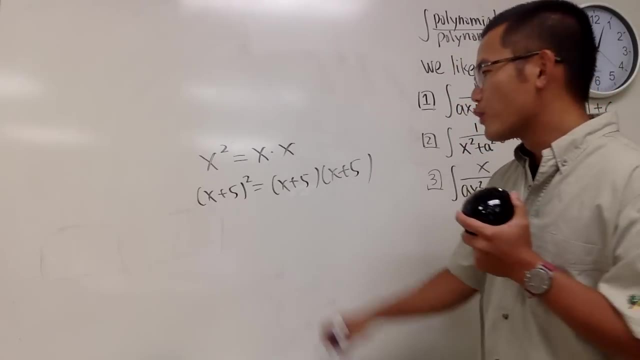 Yeah, Similarly, if we have x plus 5 squared, isn't this just the same as x plus 5 times x plus 5?? Definitely, Of course you can have the same idea. You have the third power. That means you have x plus 5. one more time, right here. 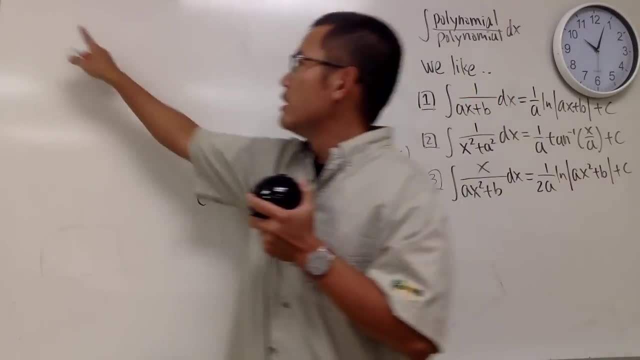 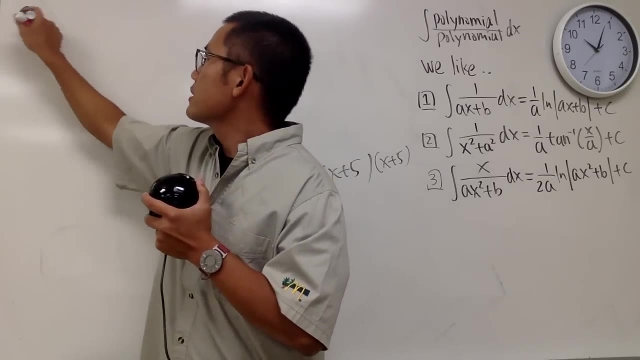 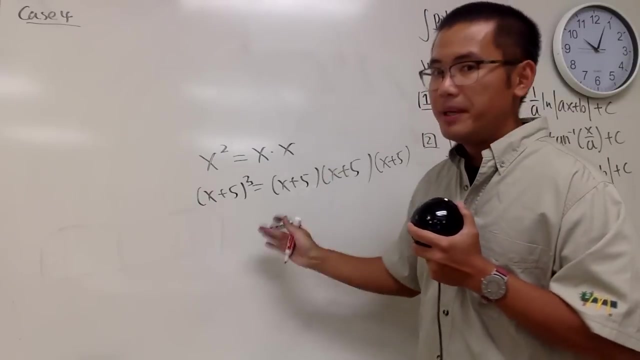 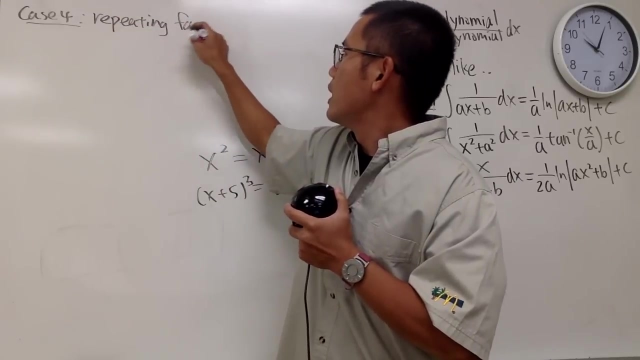 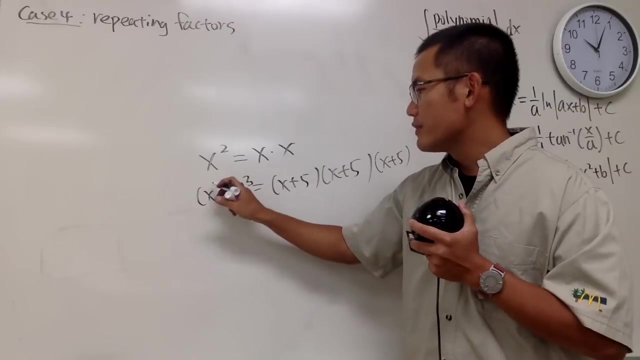 Repeat it three times. So this is the fourth case Right here. right, This is case 4.. This is case 4.. Case 4. We are going to be looking at repeating factors- Right, Repeating factors. And of course, not only we can have the linear being repeated, we can also have the quadratic being repeated. 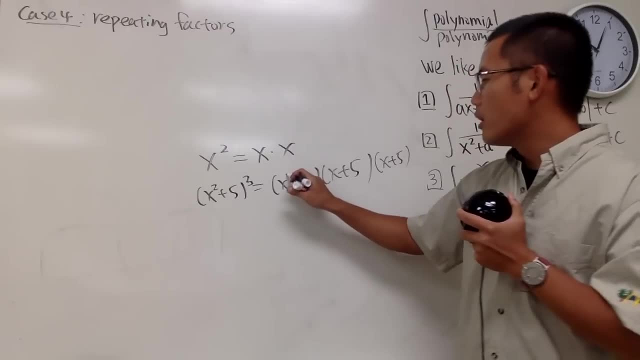 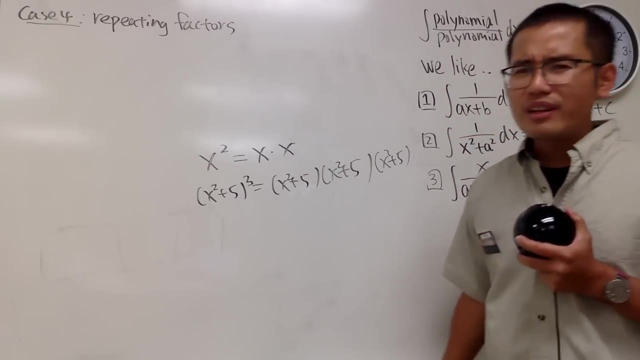 For example, we could have x squared plus 5 to the third power. Of course this is just an irreducible quadratic being repeated three times And you might be wondering what if we have, like a weird cubic, If I have x to the third power plus 8,, for example. 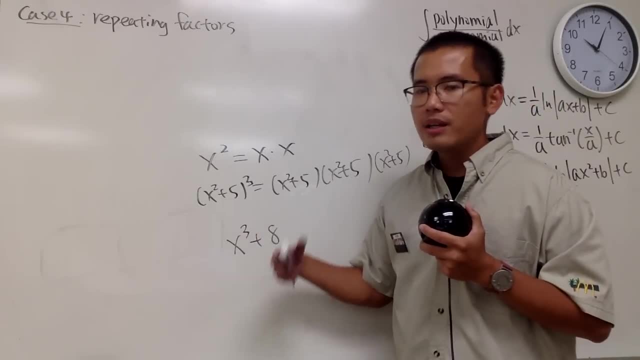 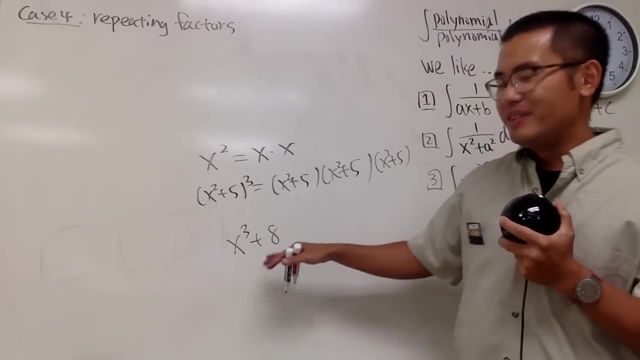 The truth is, we can factor out cubic quadratic and then any higher power. This just depends how difficult it is. And for Calc 2, we'll just be dealing with some nice cubic, like maybe this one, etc. etc. 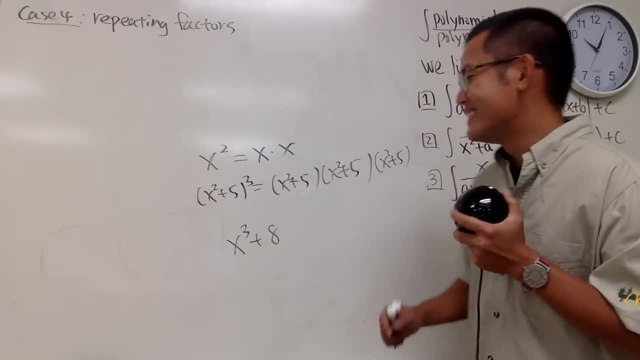 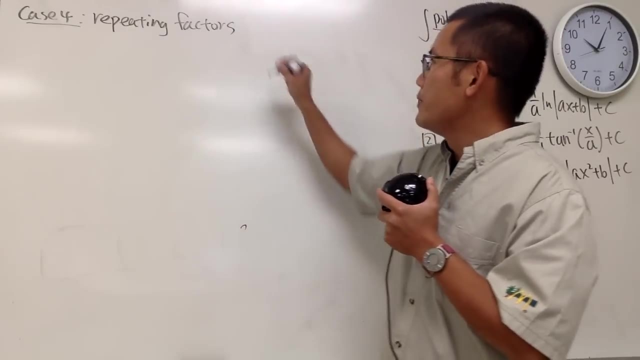 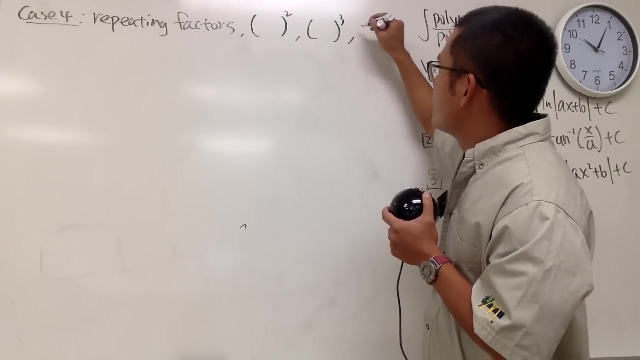 If you have some bizarre cubic or quadratic, then good luck. Yeah, Anyway, for this case, right here, we are going to be focusing on the form of parentheses, some factor to the second power and then something to the second power, Third power, etc. etc. 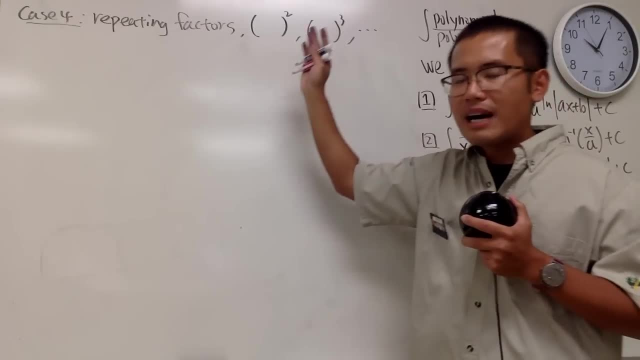 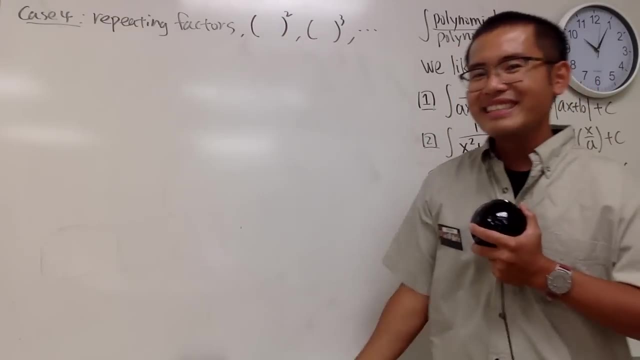 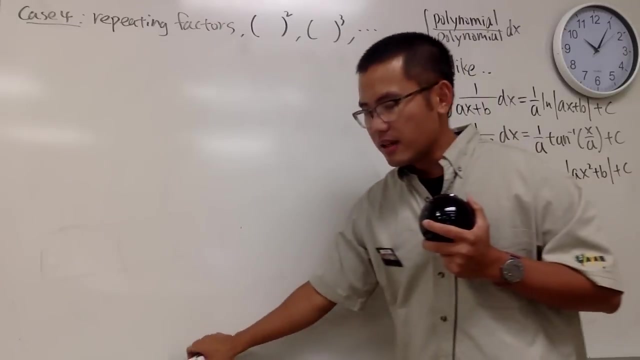 No 2.2,, no 3.5,, no, whatever. I just passed the whole numbers. If you have 1, that's just like the previous cases. If you have 0, that's even better. If you have negative, that's actually another formula, but that's in the notes. 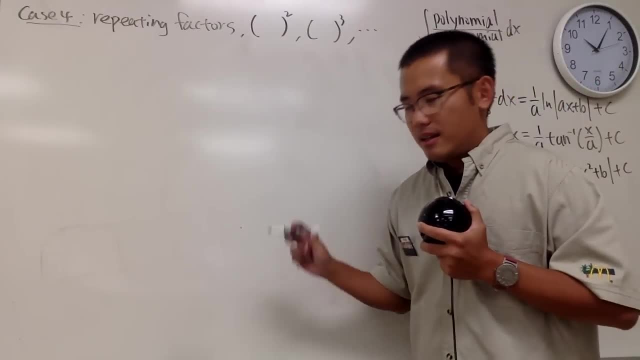 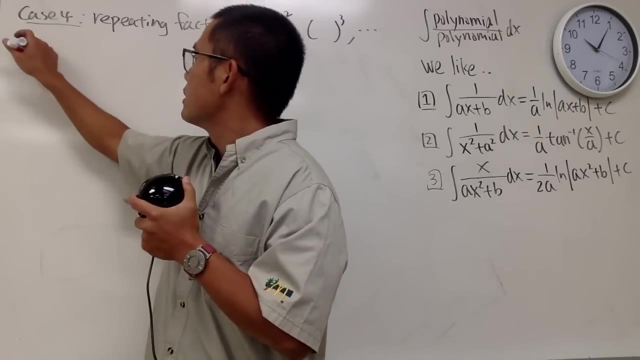 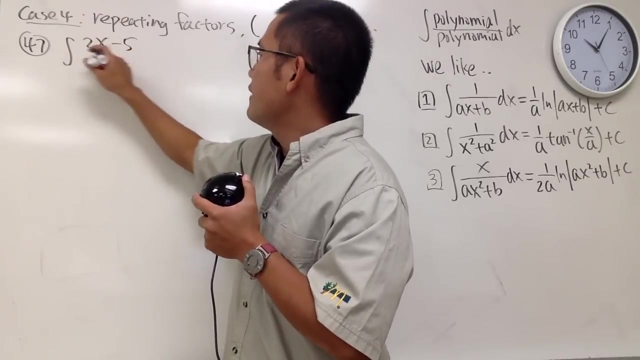 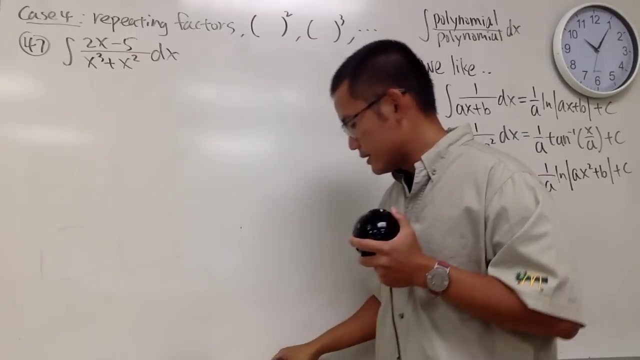 I'm not writing it down because I know we will not be going, It's just yourself. so yeah, Anyway, number 47.. Right here, Let's look at the integral of 2x minus 5 over x cubed plus x squared dx, like this: 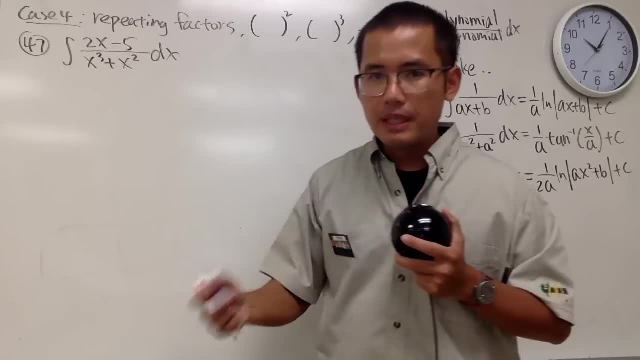 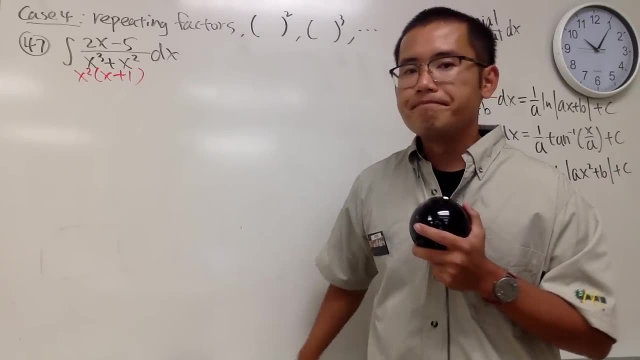 First thing. first, can we factor the bottom? Yes, And to do so, let's factor x squared, and then we get x plus 1, like this, And that's very nice, Good, Well, this is the x squared. 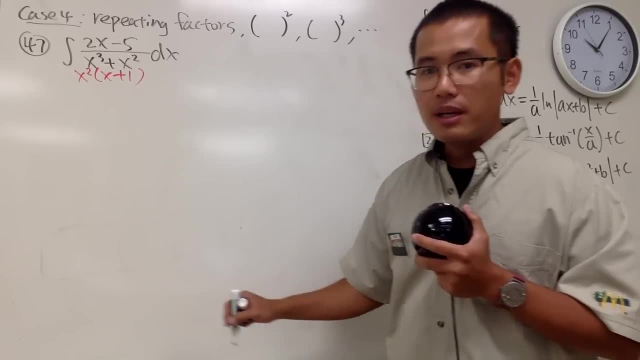 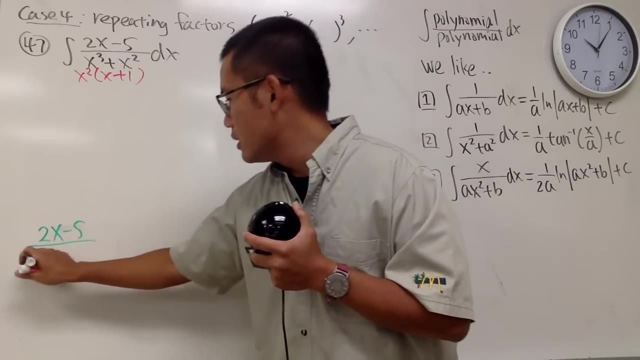 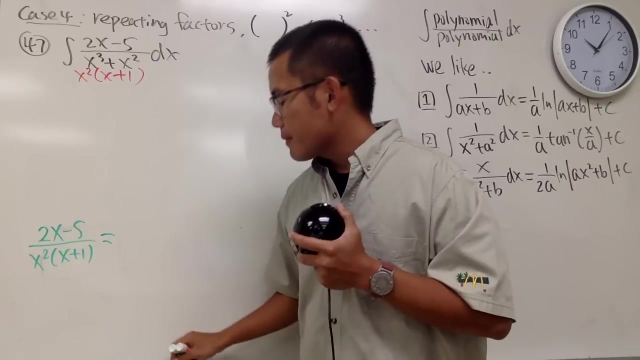 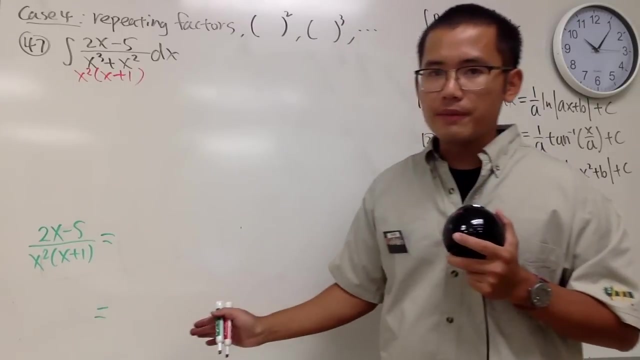 That's the one that I was telling you guys about, And now let me just write this down for you guys. This is how we do the partial fraction. This is how we partial fraction x squared times x plus 1.. In fact, let me tell you guys how you should be dealing with this kind of situation. 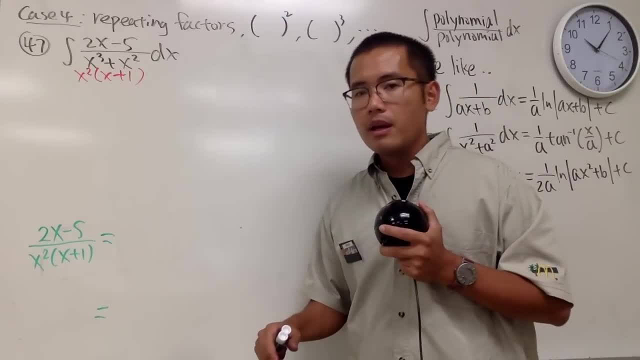 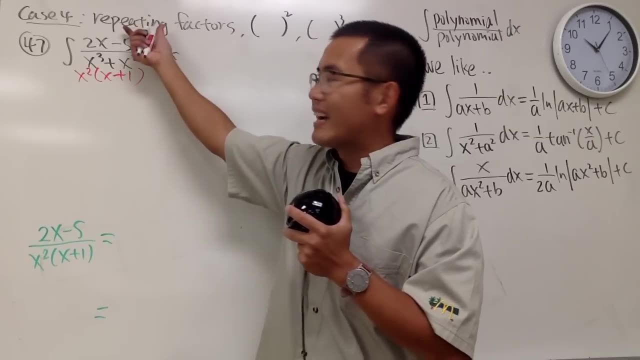 Let me tell you guys how you should be dealing with this kind of situation. When you have x to the second power, notice that this means x times x. This means you have a factor being repeated. When you have a repeating factor, you have to build up the power. 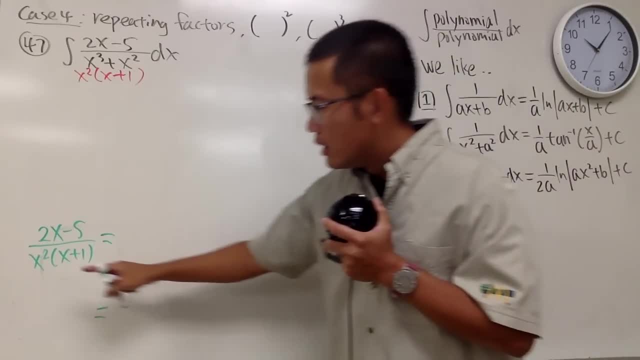 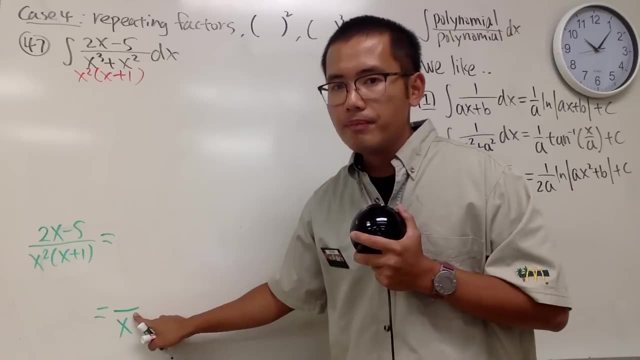 Let me show you What I mean by that is: look at this: x to the second power. right, You're actually going to start off with x to the first power, And because this is x to the first power, then on the top I need to have a constant. 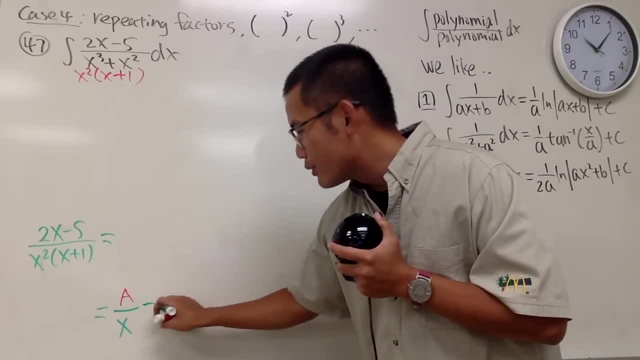 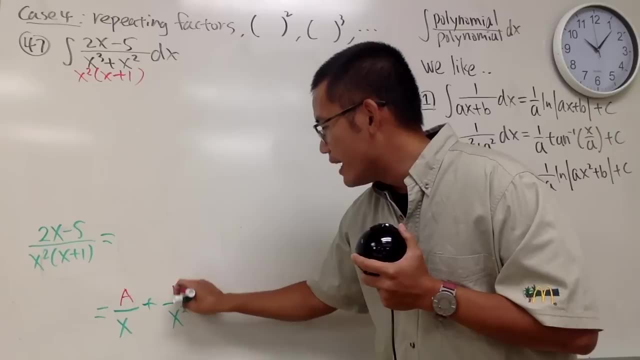 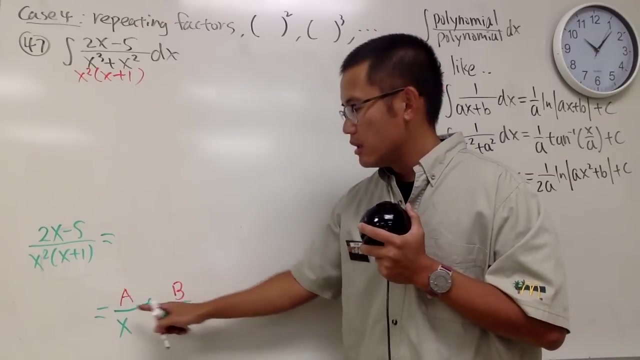 So I'll just put an a for that, And then next I will have to go up to the second power, because right there we have the second power, So we have to go up to x, to the second power, And then when we build up the power we have to make sure the top stays the same kind. 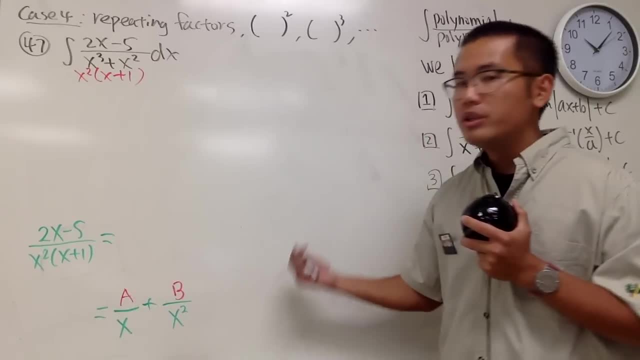 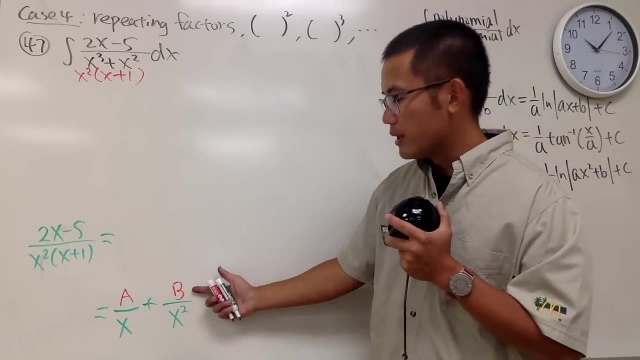 This and that they have to be the same kind when you are building up powers. This is a constant. This is also a constant. Again, we are building up powers. I'm not doing the one degree less than the bottom, because you guys will see why, right? 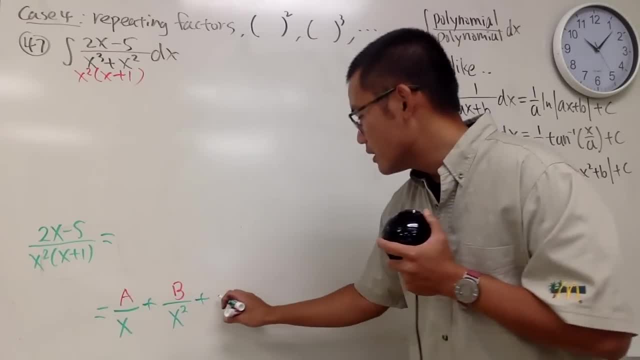 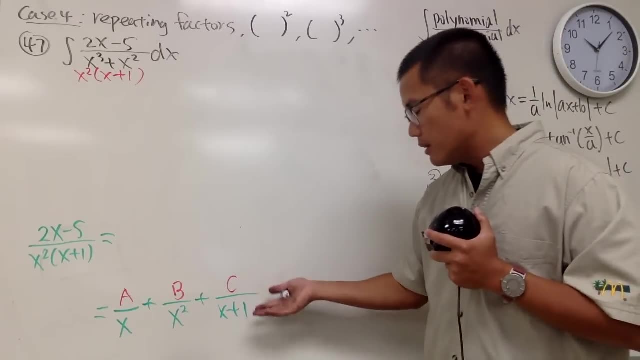 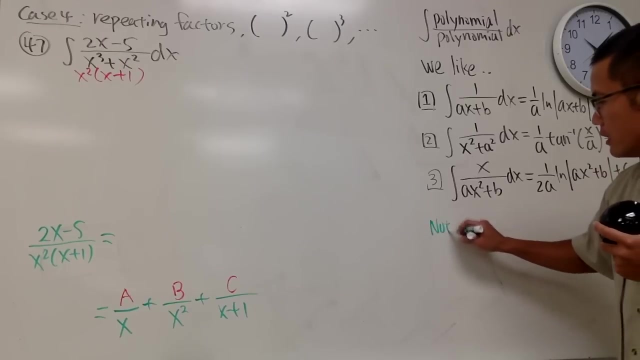 So that's pretty much the idea. And then we have another factor, which is the x plus 1. This is linear, so on the top, I just need to have a constant like this, right? Well, I know, let me just put down some notes on the side. 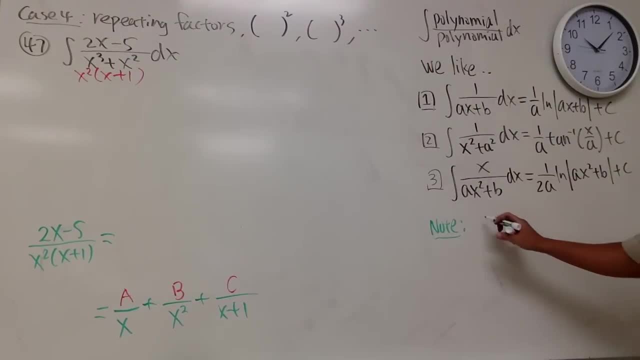 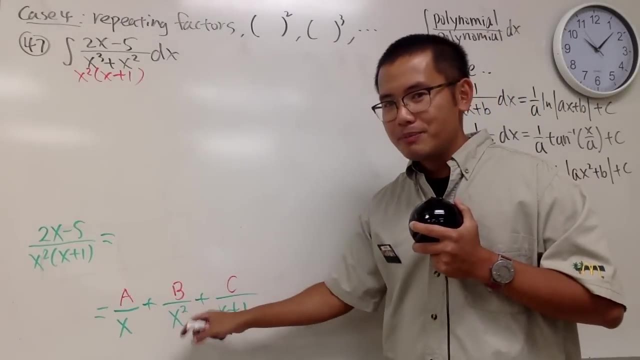 Suppose you have x to the third power. for example, Suppose you happen to have 2x minus 5 over x to the third power. Yeah, you would just go up to, like you know something, x to the third power. 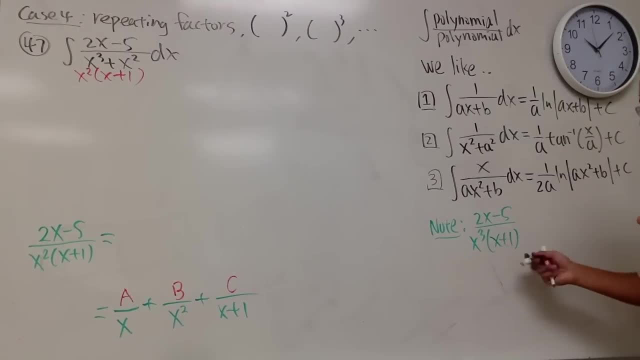 Let's just do this real quick And just to make it slightly more fun, let's say we have x plus 1 to the second power, like this, for example: okay, Let's put it down this way because I may not have enough space. 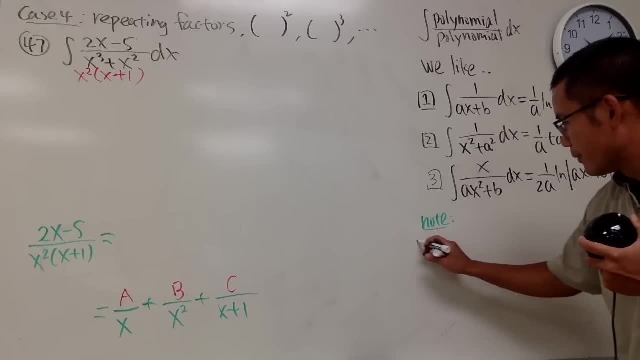 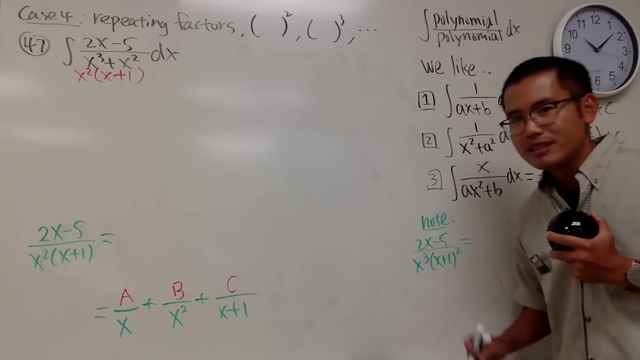 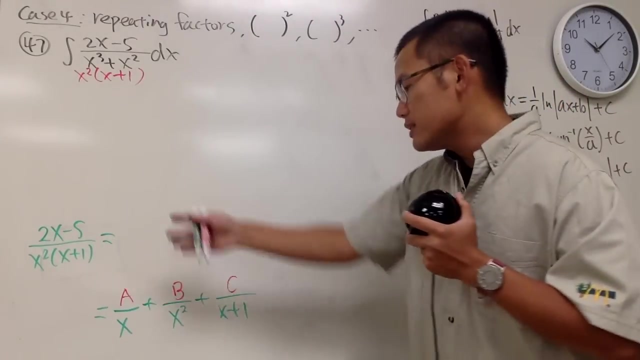 So here, well, maybe just an example: 2x minus 5.. Over x to the third power times, x plus 1 to the second power. yeah, Suppose this is what we have, As long as the top is with lower degree than the bottom, which it is. so let's just do that. 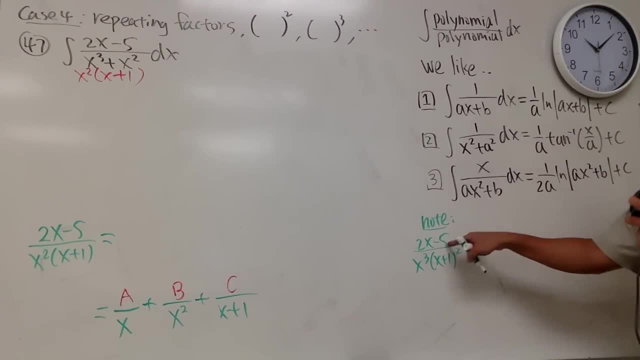 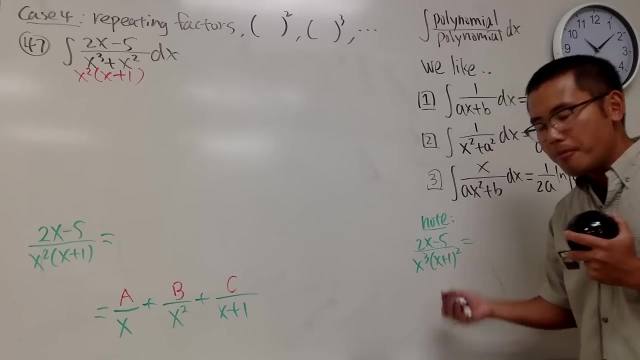 And this is of course it is. You can have like minus 51 for every one, but this is the setup. x to the third power. x is being repeated three times. We have to build up the power. So right here we start off with. 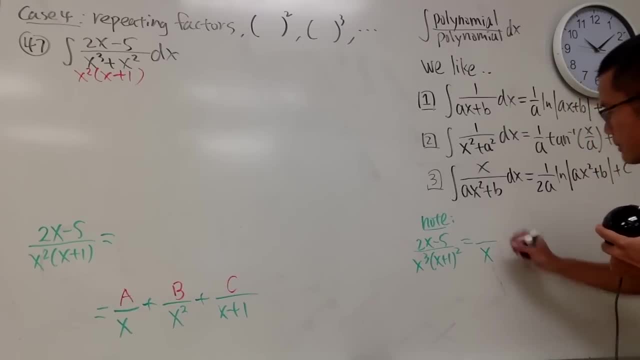 x to the first power and because this is x to the first power, I need to have a. It's just a constant. Next we have to go up to third power, so we have x squared Again. stay the same kind. 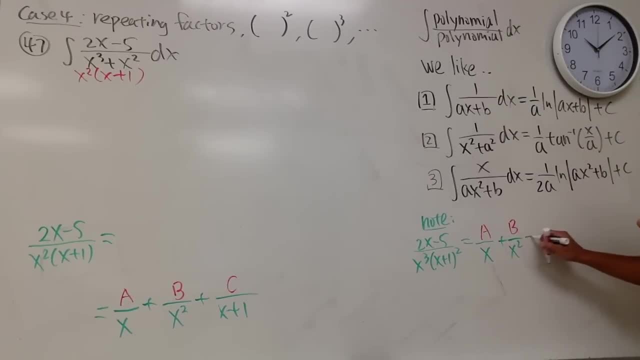 Constant, constant. so we have b. Next we have to have- oops, we have to have- get to the third power. So we have x to the third power right here, and that will be c, like this And: 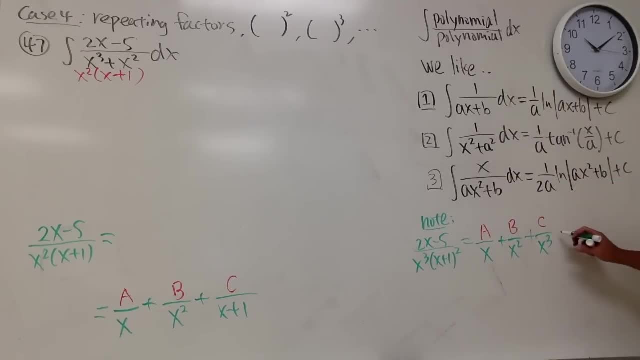 We also have to build up the power for the x plus 1 squared, So start with something over x plus 1.. This is linear On the top. it has to be a constant: a, b, c, d. Lastly, we need a second power, so this is the last one. 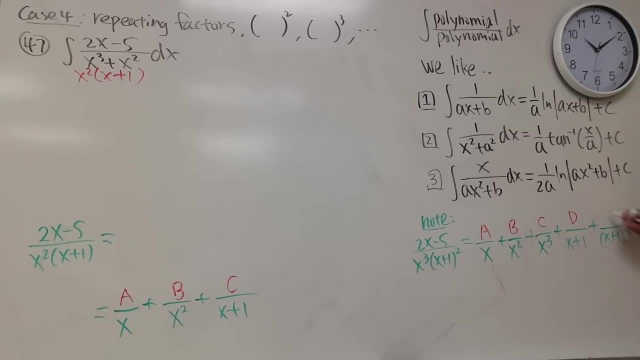 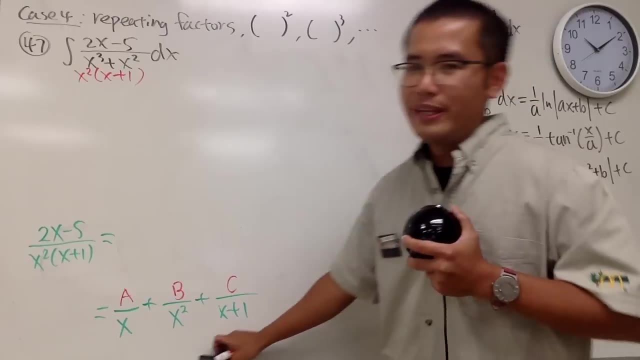 And this is the setup, right, And e like this, And of course you can imagine, if this is x to the 13th, you just go up all the way to the 13th. But of course we are not going to do that. 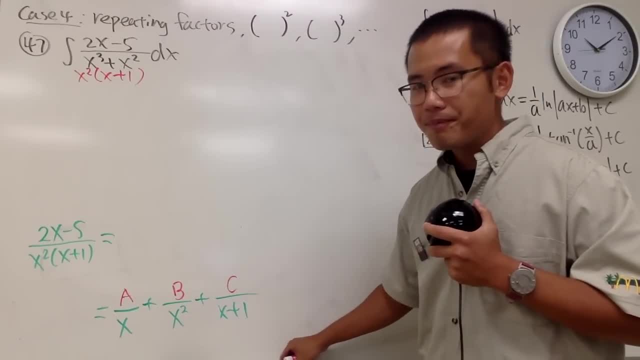 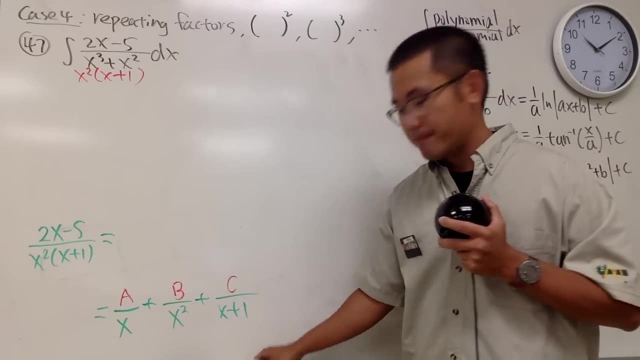 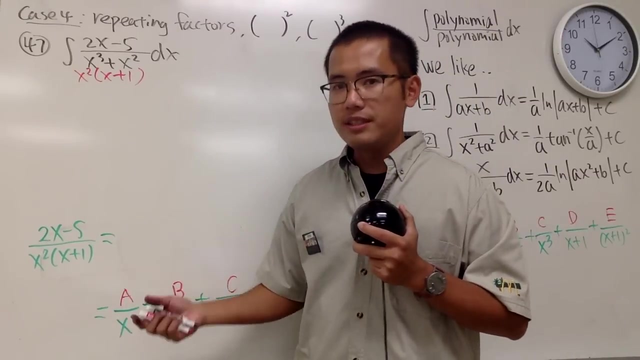 This is the one that we are going to do. Okay, Now you might be wondering why that we need this term. I will explain. Here is the idea. I want you guys to remember, if you are just doing this on the exam. 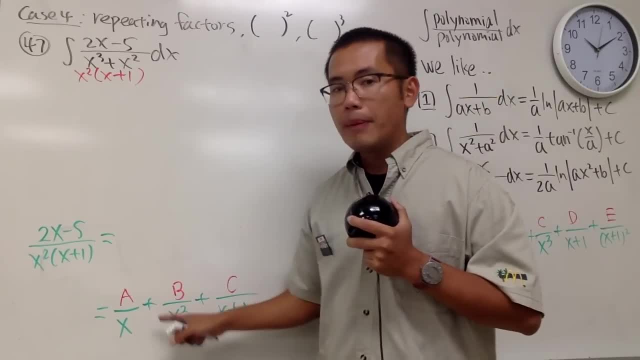 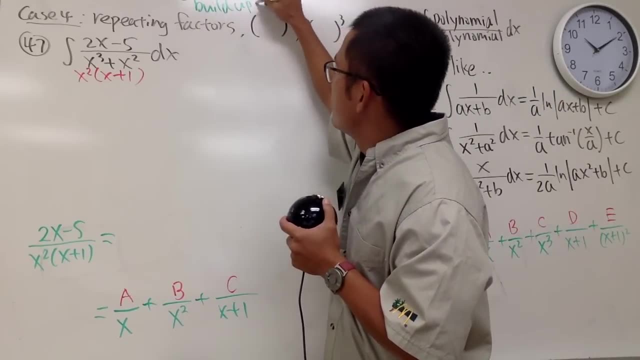 go from here to here and seriously remember to build up the power. And let me just perhaps write this down here. I will tell you guys: Build up the power. It's like playing a video game: You have to build up your power. 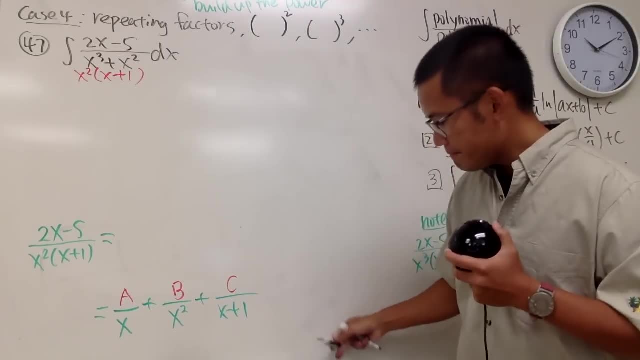 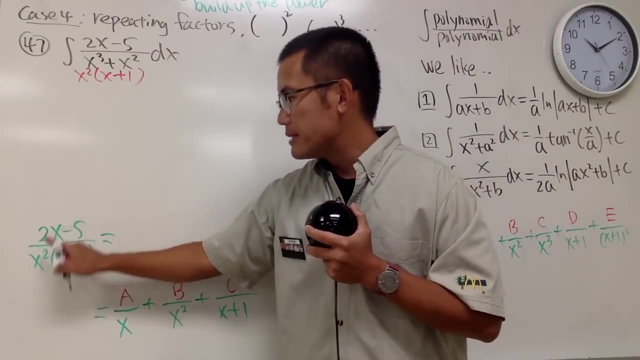 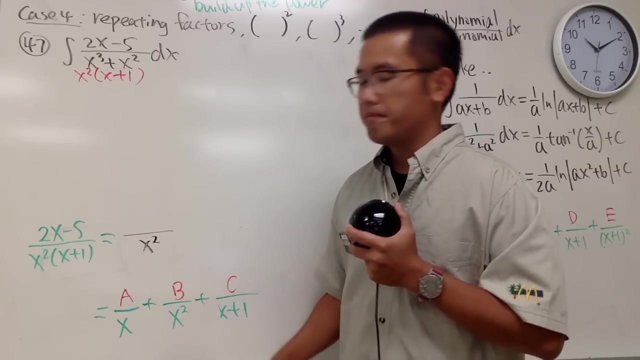 Can you guys see that? Yeah, You have to build up your power. Yeah, Okay, Here is the idea. Ignore that The ground type is less than the bottom. Good, Here we have x squared. If you really want to put it down as something over x squared, that's fine. 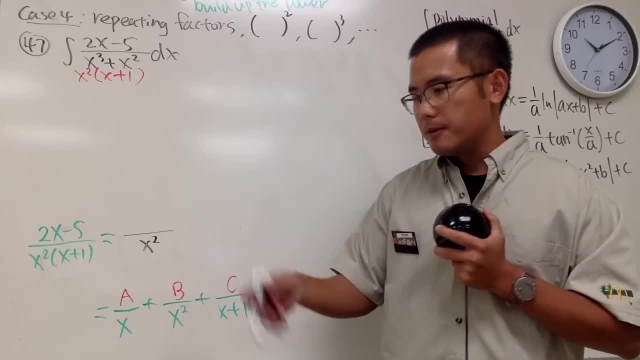 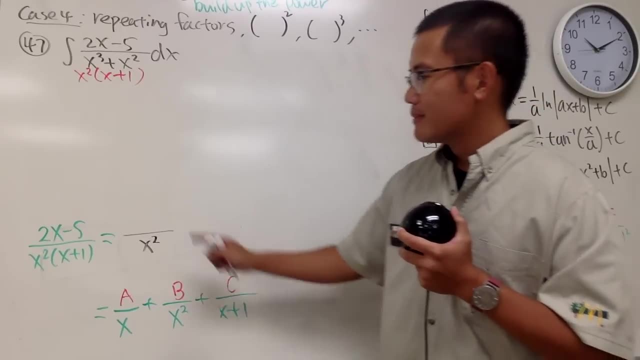 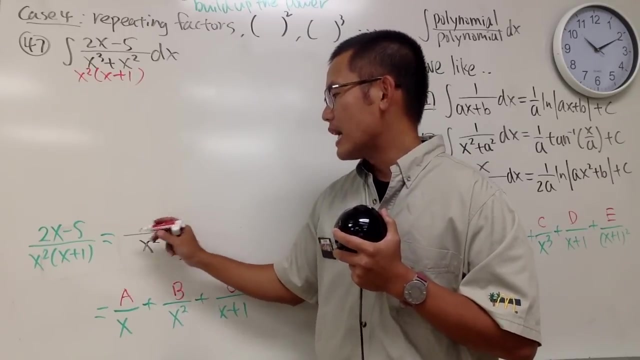 But you will have to go from the very, You will have to start from scratch. The degree on the top in this case has to be one degree lower than the bottom. So this is the second degree On the top. it has to be ax to the first power plus b. 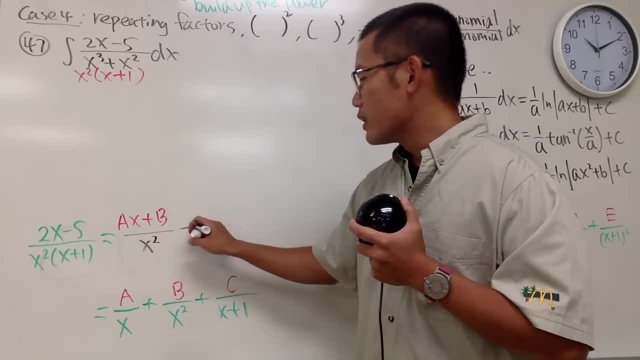 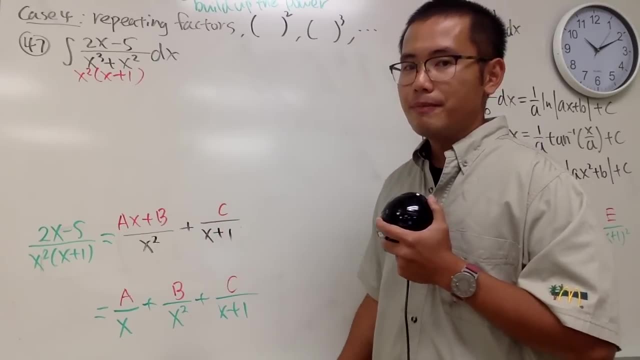 Just like what we talked about in the previous case. Yeah, And then of course we add the width. The next one is x plus 1. And the top is just constant z. And you see, if you set it like this, 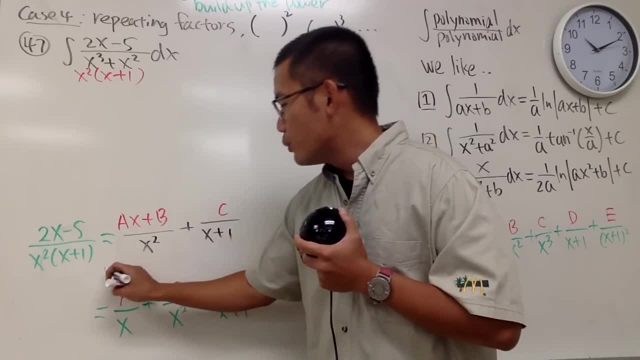 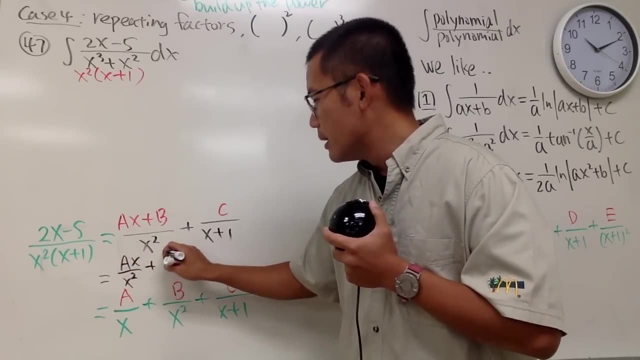 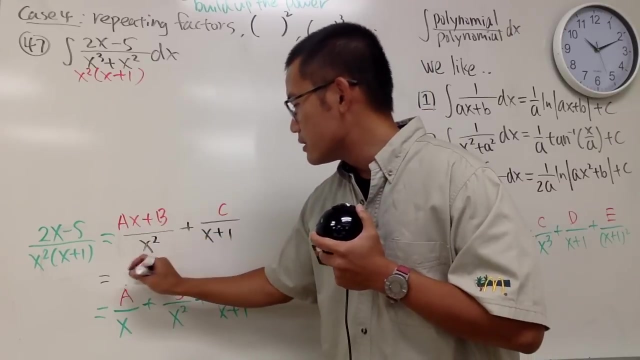 what can we do next? Yes, we can just split the fraction And we see that we will end up with ax over x squared And then plus bx. Sorry, Let me just write it down with the right color, We can split this as ax over x squared. 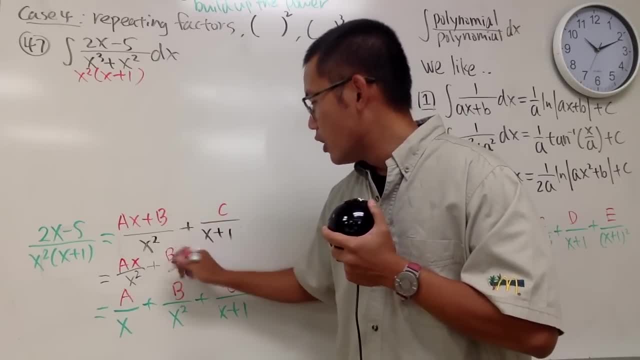 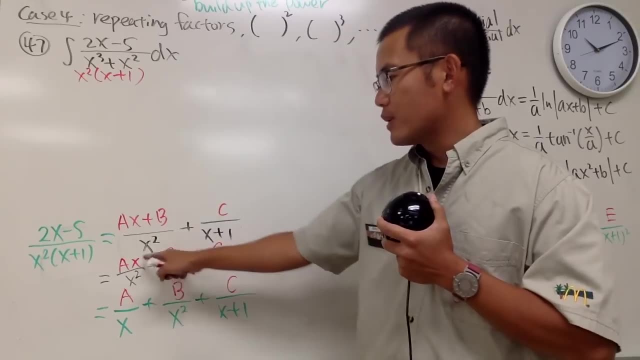 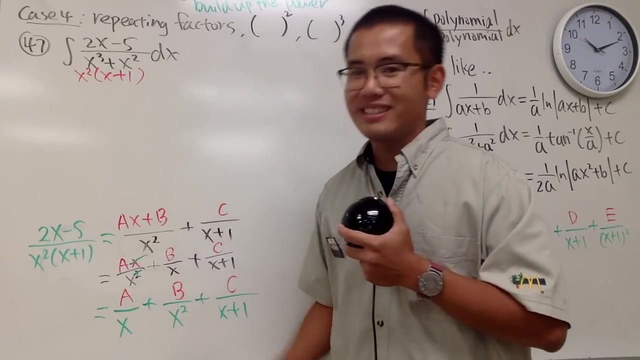 And we will add b over x. And then, of course, this z guy just stays right here. And what can we do, right here? Yes, We cancel things out, Cancel, cancel. So we just have a over x, right here. 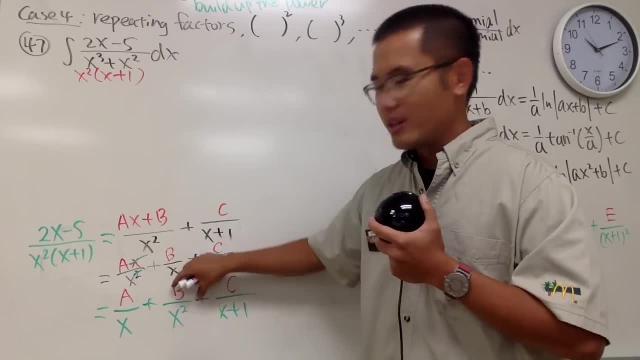 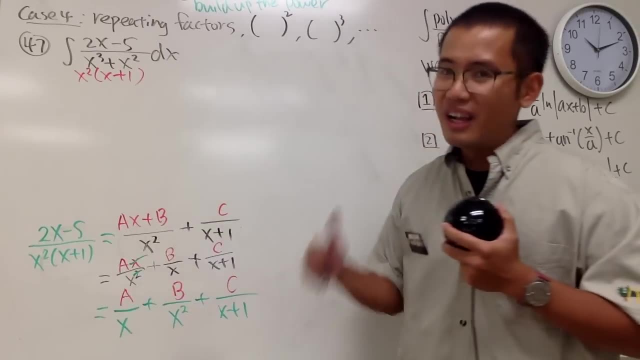 And if you wonder why we didn't do the bx plus z right here as a linear factor, because you can split it and combine it. So remember to just build up the power to go from here to here. That would be the ideal situation, right? 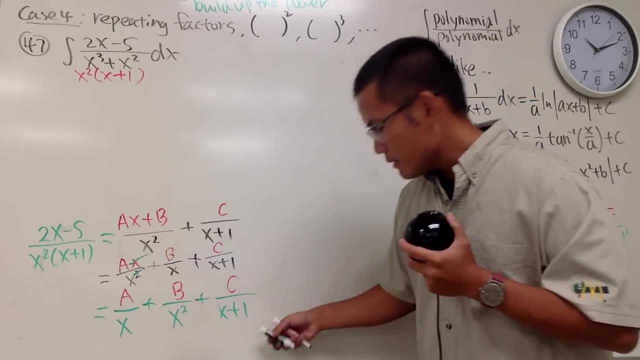 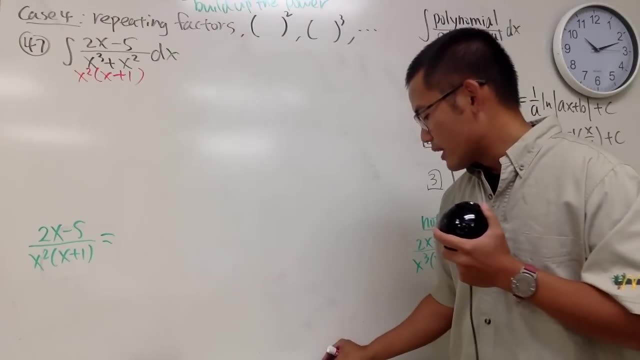 So have a look right here. Okay, Now, of course, I'm just going to work out this for you guys, And I should have enough space to work out the abc for you guys. We'll see. Okay, Here we go. 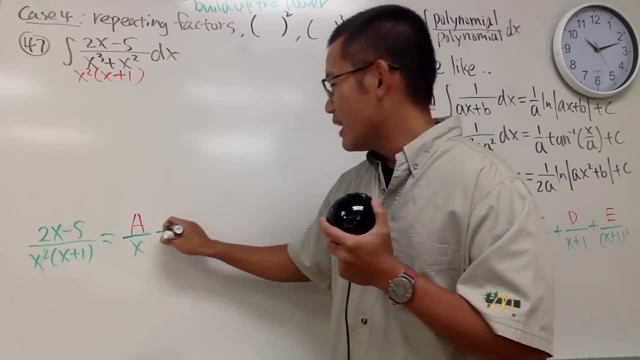 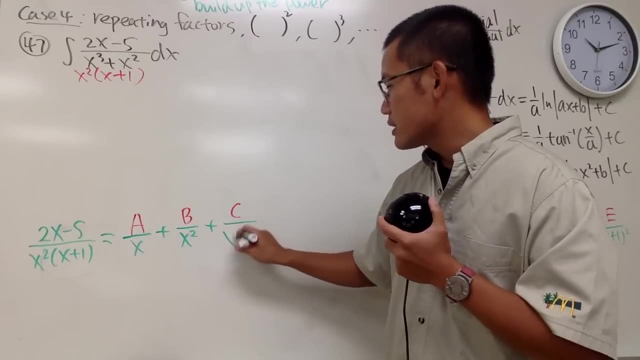 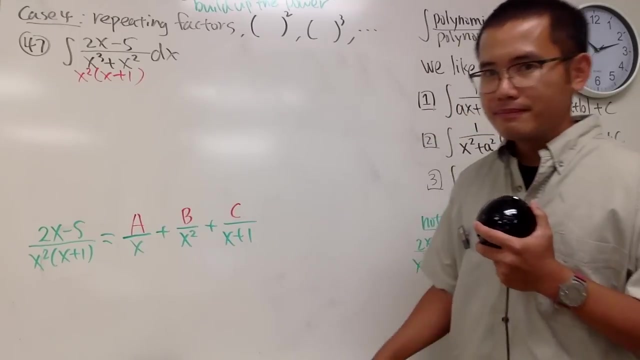 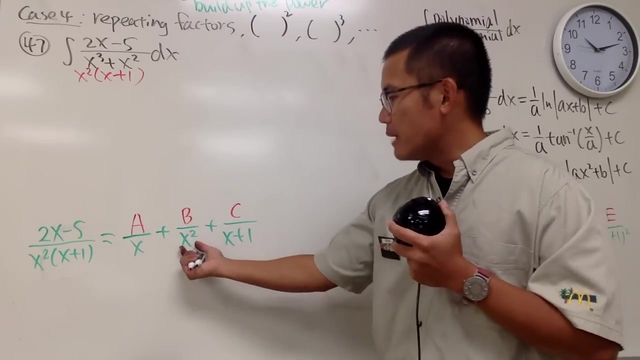 We have a over x to the first power, plus b over x to the second power, And then plus c over x plus 1.. Good news for you guys: This time we can do cover up for two letters. What are they? b and c, because they have the same exact denominator from the original. 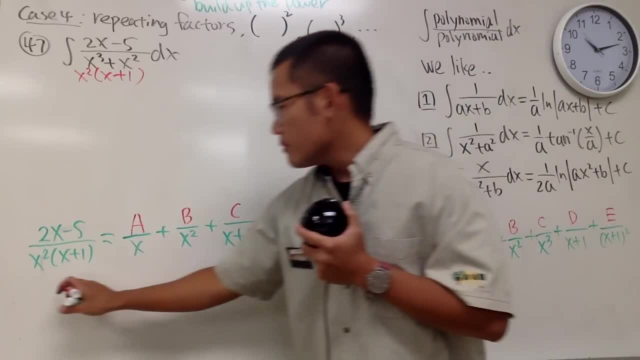 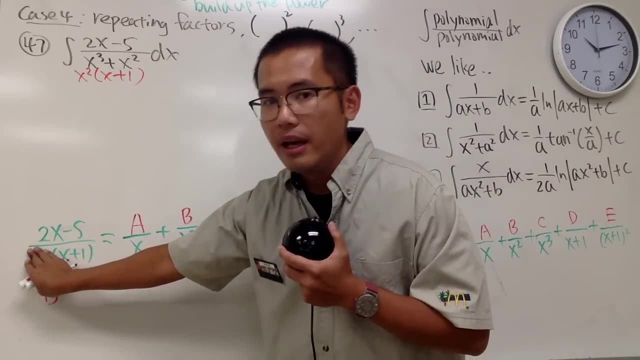 Right, So that's the idea. So let's make that happen. to figure out what b is Again, because b has x squared, we will come back to the original cover up: x squared. And how can we make x squared equal to 0?? 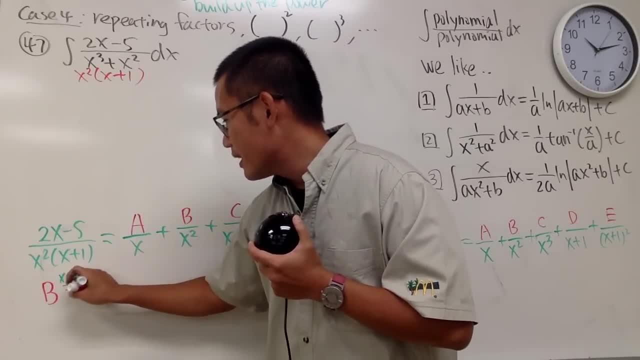 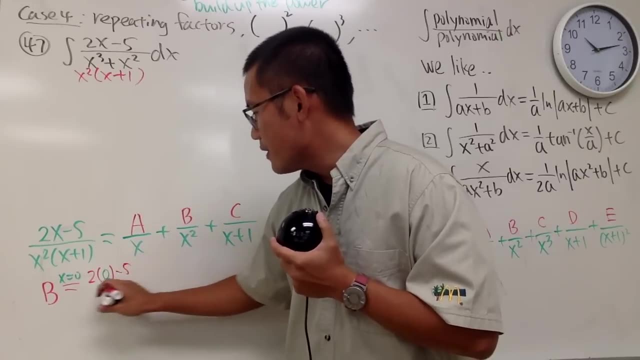 x has to be 0. So right here, make x equal to 0. Put 0 in here and here, So we have 2 times 0, and then minus 5 over putting 0 right here, So we have 0 plus 1.. 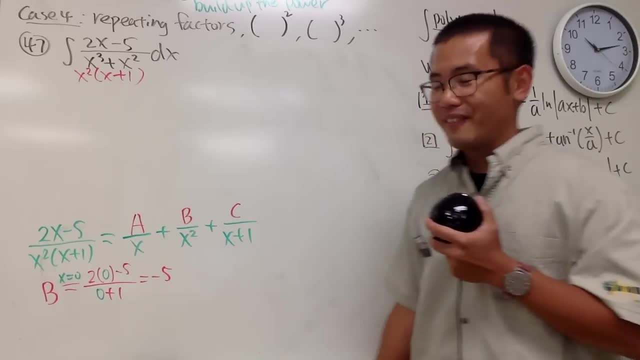 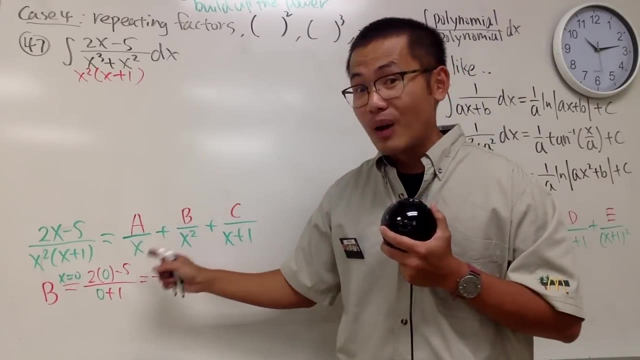 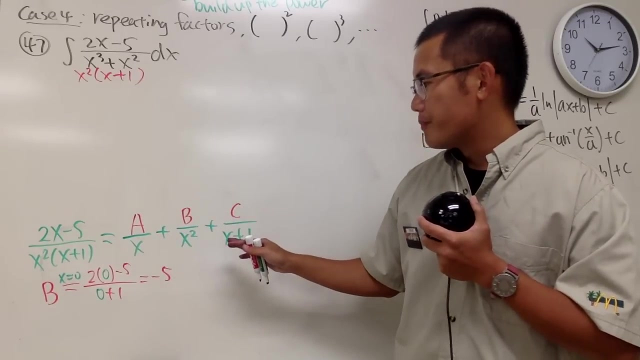 All in all, we get negative 5.. That's it Very neat, huh. And the reason is because we can multiply everybody by x squared. Unfortunately, a does not work with cover up. If you multiply everybody by x, you cannot get rid of the b. 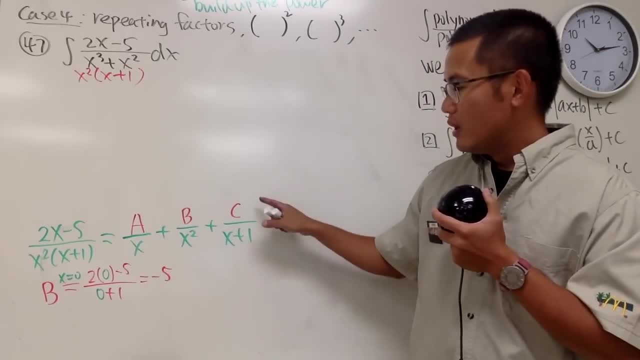 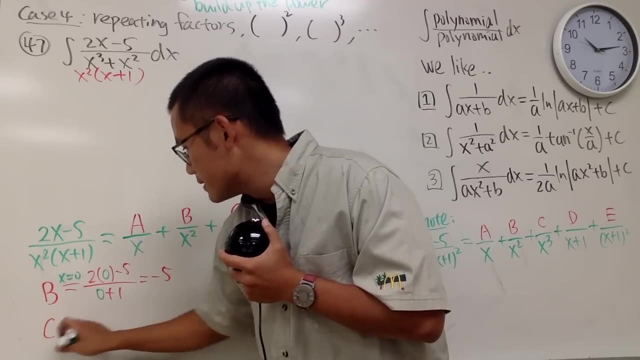 So cover up does not work for a. c can, though. You multiply everybody by x plus 1.. You cover this up. Anyway, I put this down for you guys: c equals. how can we make this equal to 0?? Yes, negative 1.. 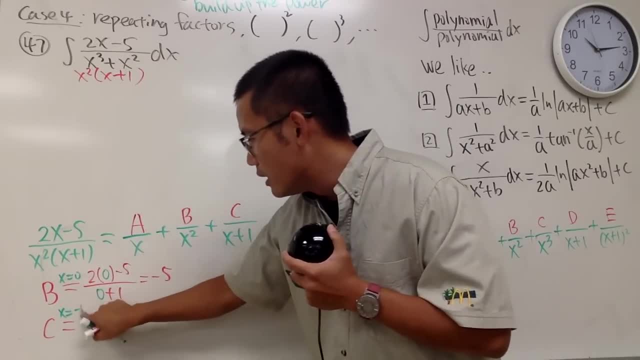 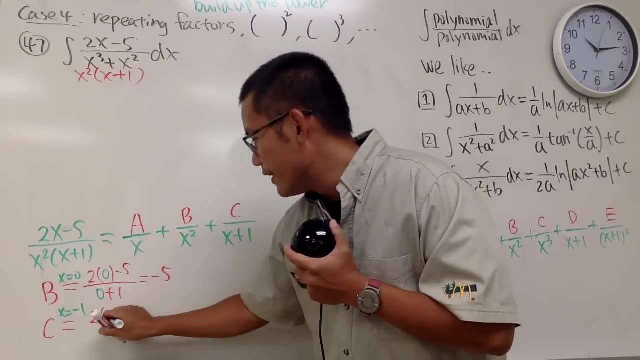 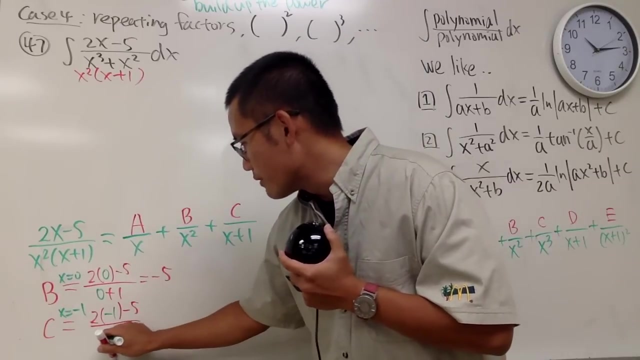 So we put down: x equals negative 1.. And of course, putting negative 1 here and here we get 2 times negative 1 minus 5.. Let me see, Yes, it is correct- Over negative 1 squared, So we have negative 1 squared. 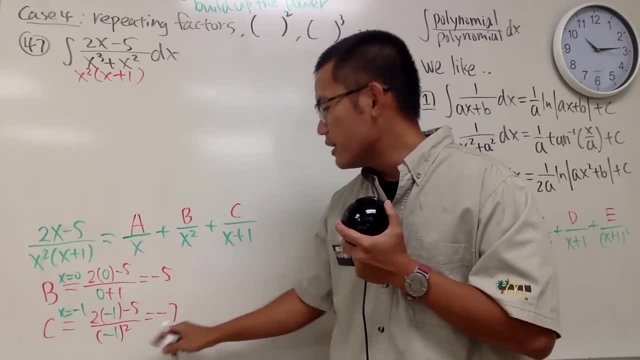 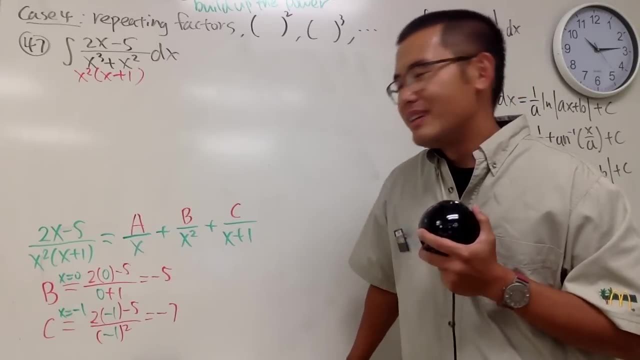 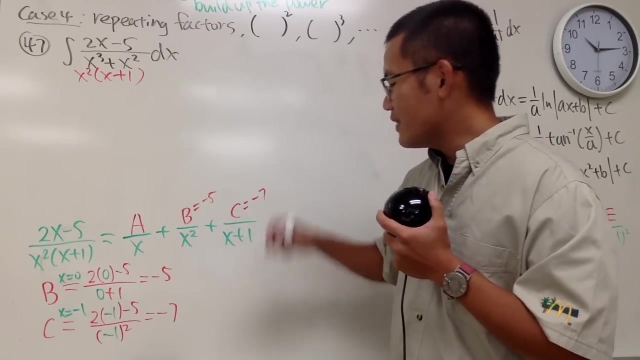 Now this is negative. 2 minus 5 is negative. 7 over 1.. So it's just negative 7.. That's wonderful. Okay, We have this b and c, so that's wonderful. Negative 5, negative 7.. 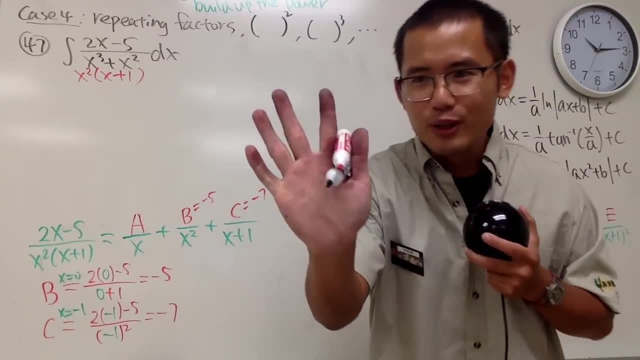 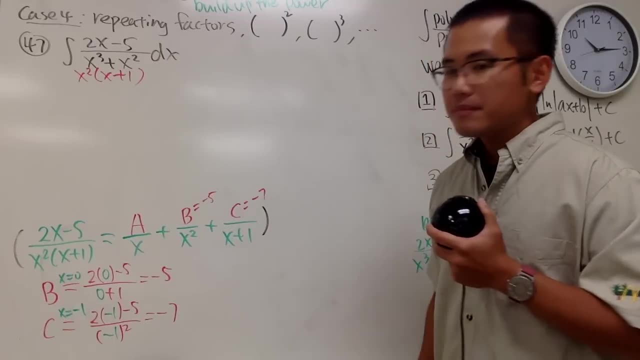 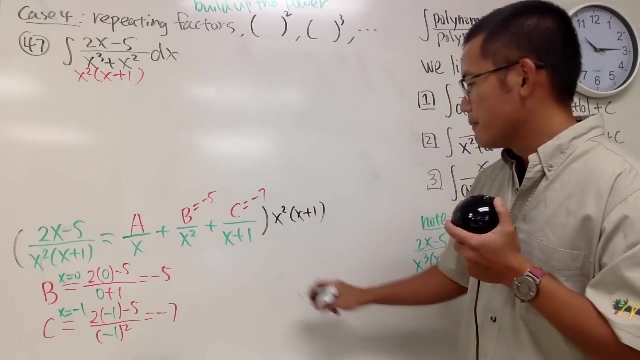 What should we do with a though? Yes, the dirty algebra. seriously, Get your hands dirty to do the dirty algebra right. All right, Multiply everybody by the lowest common denominator, which is just that x squared times x plus 1, right. 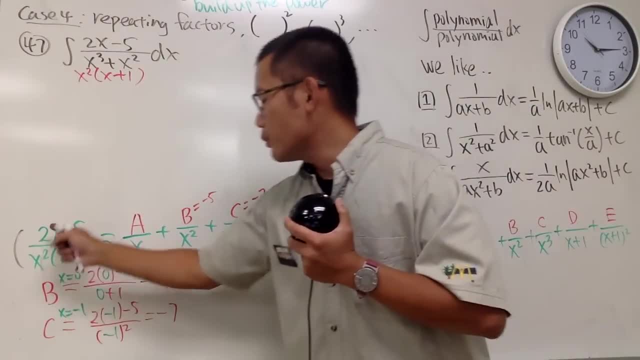 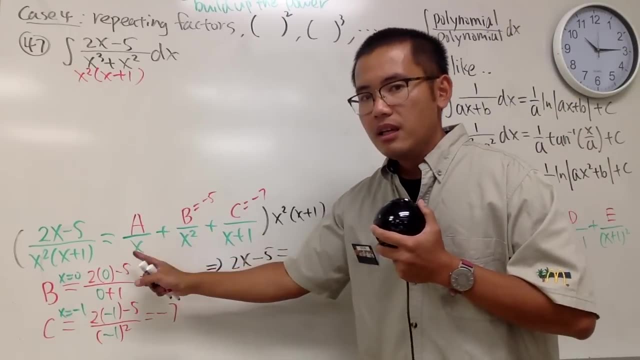 So let's see what we get when we do that This times that we just get this 2x minus 5 equals. Now this times that x and that cancel. So we have a which we don't know at the moment. 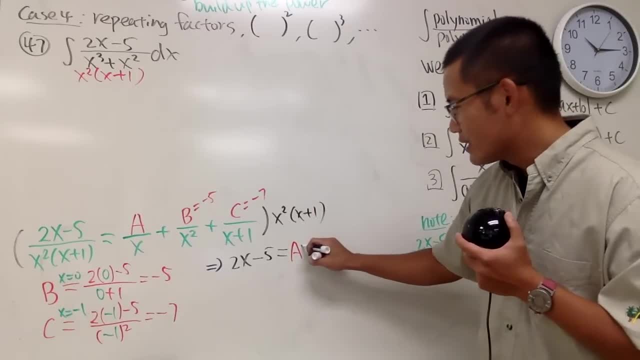 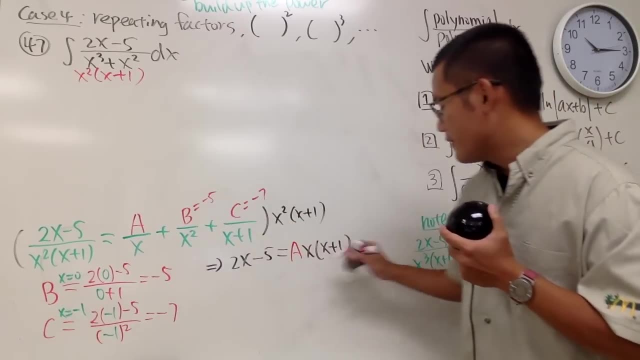 So I just put down a, But we do have another x factor, So I just have x And then x plus 1 right here. yeah, Next this and that will cancel. We have negative 5.. So put down negative 5.. 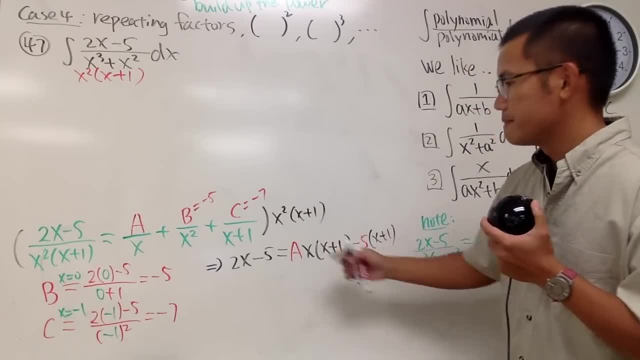 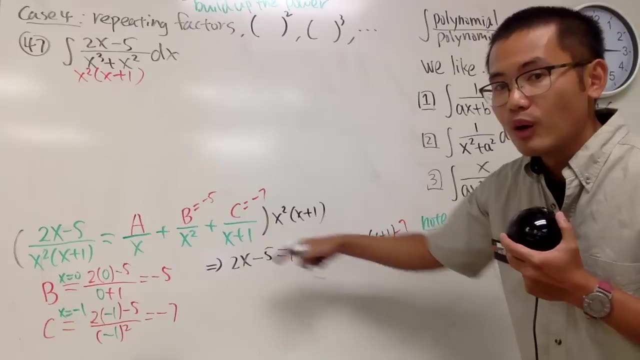 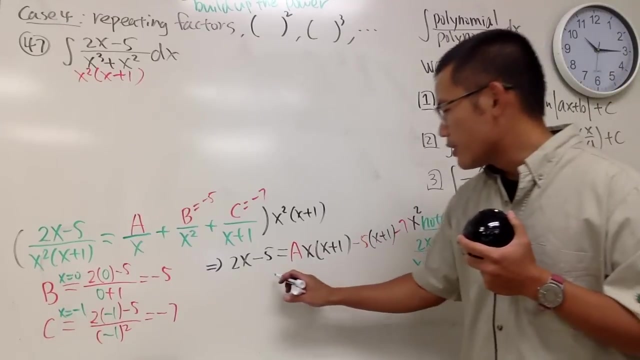 And we have the x plus 1, yeah, Lastly, we have negative 7 for the c And this, and that will cancel. We just have x squared left like this. So that's what we have On the right-hand side. let's go ahead and just multiply things out. 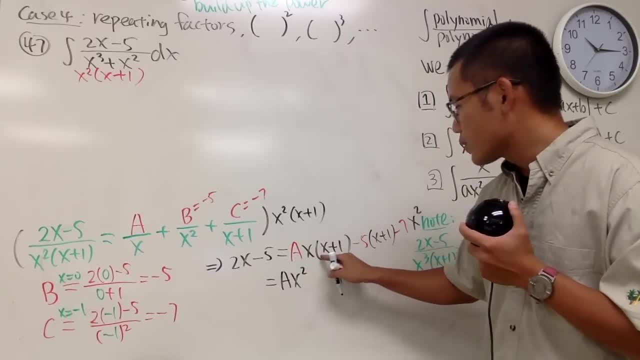 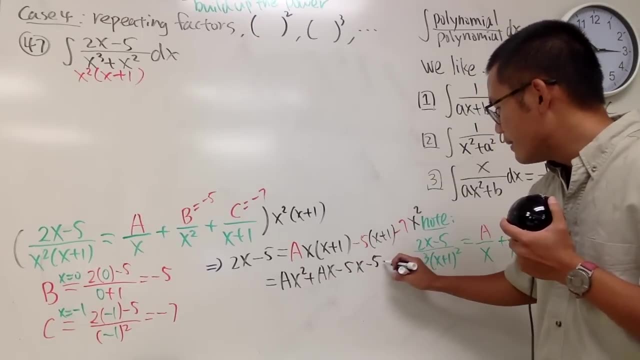 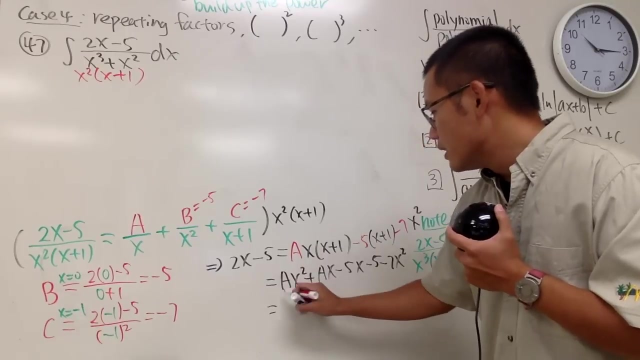 So we get ax squared plus ax, And then we have minus 5x, minus 5.. And then minus 7x squared like this. That's all we have, And then we can combine like terms. You see that we have this and that. 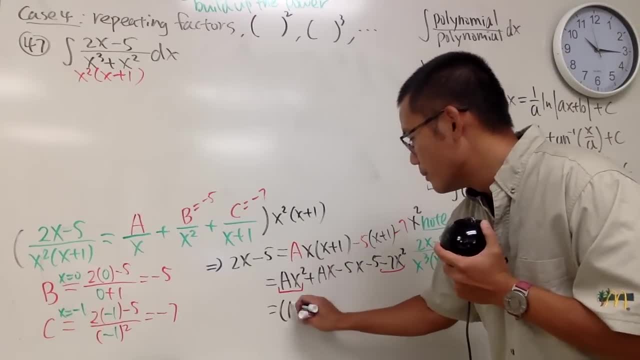 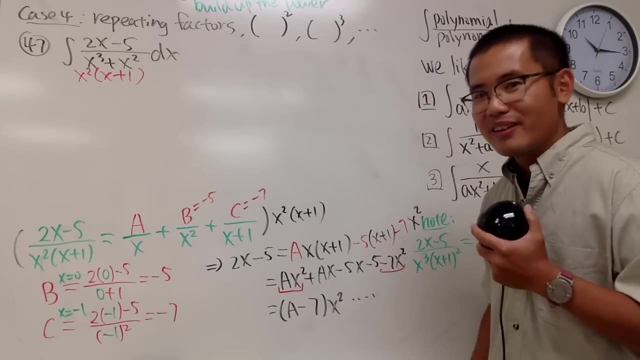 They are the x squared term. We can factor things out, Put it as a minus 7 and then x squared. In fact, this is all I need. I don't care about the other, Because on the left-hand side we happen to just have 2x minus 5.. 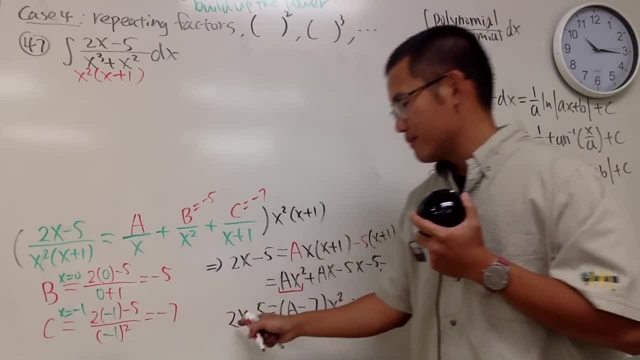 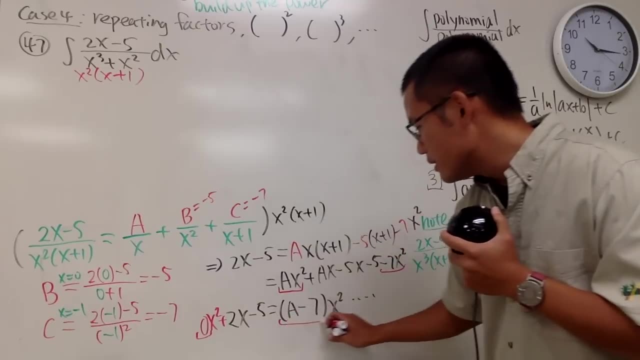 And what's the coefficient of x squared on the left-hand side? 0, because we have nothing here. So this is 0x squared, So 0 has to be this, Namely, a minus 7 has to be 0.. 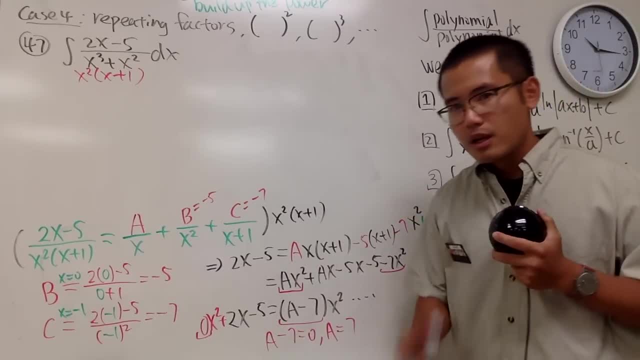 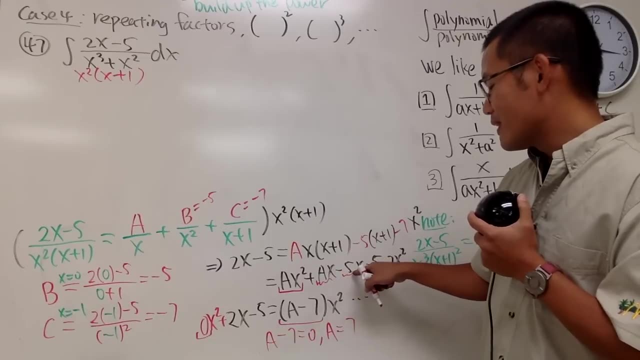 In other words, a has to be 7.. If you want, you can see We can combine this and that A is 7.. Put it here: 7x minus 5x is 2x Done. Same thing too. 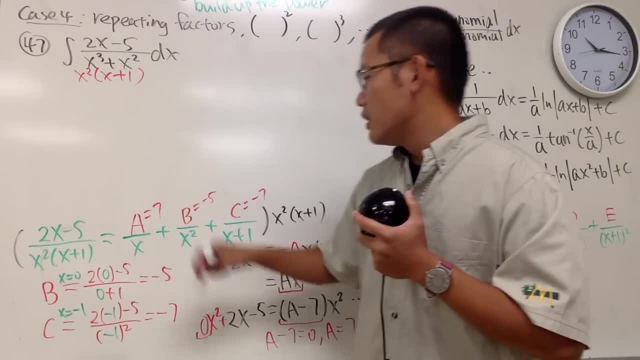 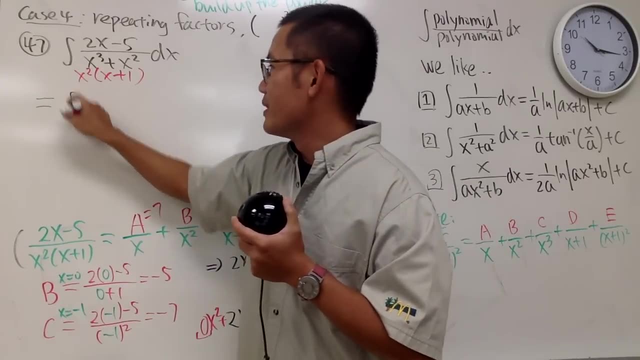 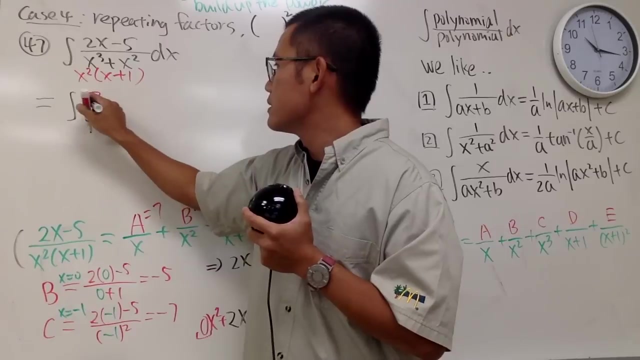 So up to you. Anyway, a is 7.. It's just a partial fraction. That's why I said okay, I know when we are doing it toward the end it will take me the longest. All this is equal to 7 over x. 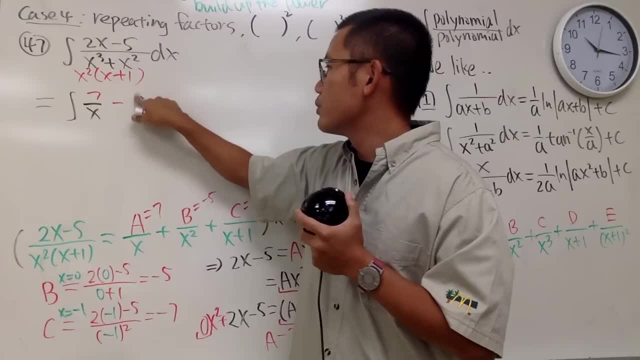 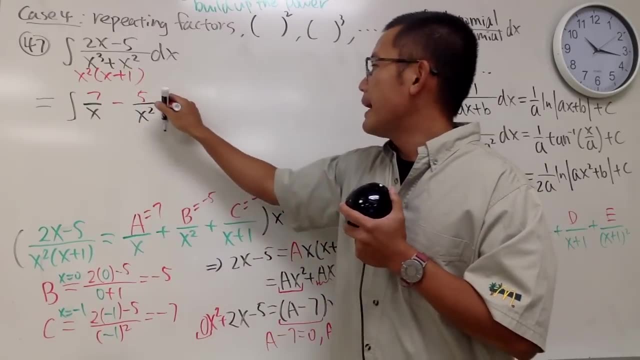 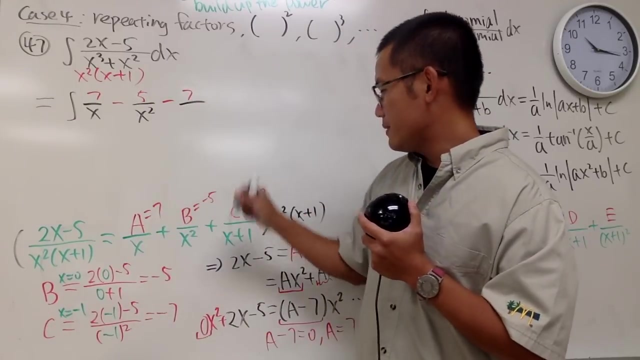 And then minus 5.. Oops, Let's do it Minus 5 over x squared, And then minus 7 over, Sorry, Minus 7.. I know, Minus 7 over x plus 1 dx, Like this: 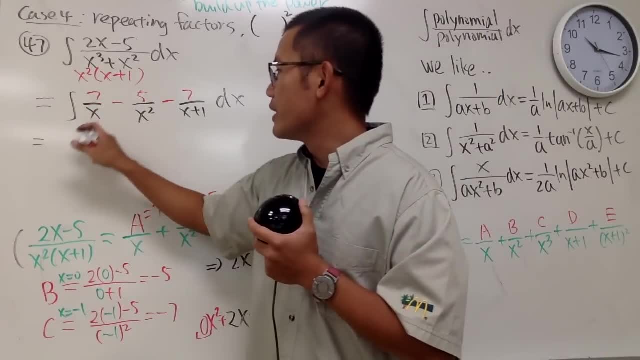 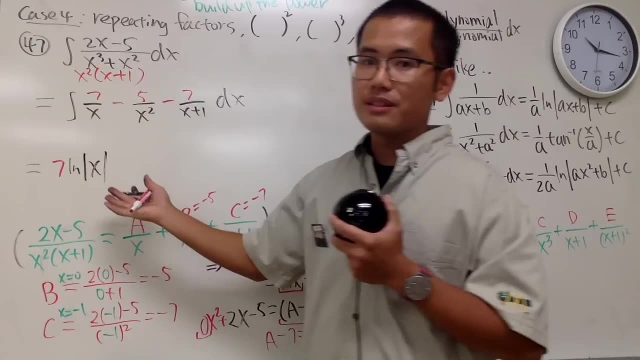 In the end we can just integrate it one by one, right. First one you get, Let me just put it down here, right here. First one: we get 7 natural log of absolute value of x. Like this, Perfect. 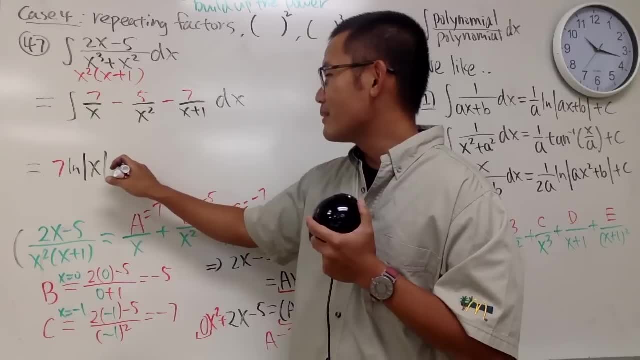 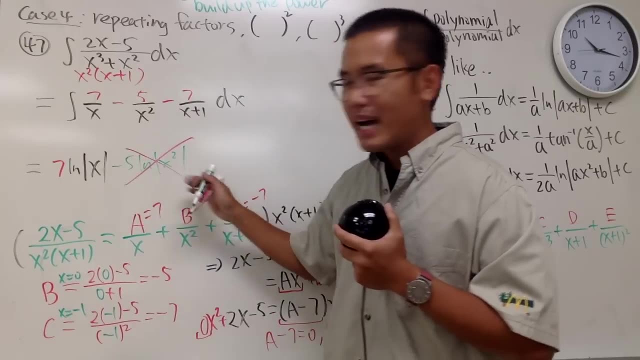 This one is not natural log. Do not put down, Do not put down minus 5 natural log of x squared. Don't do that. No, no, It's not like that. No, No, no, no, no no. 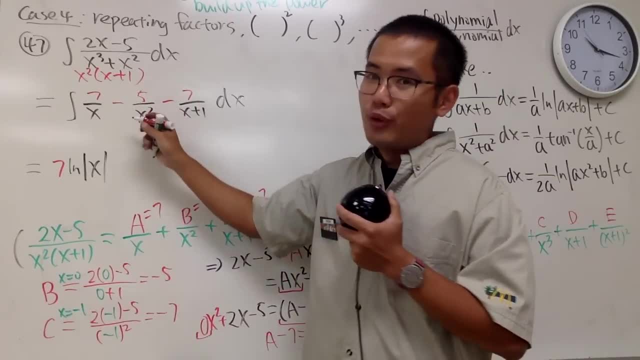 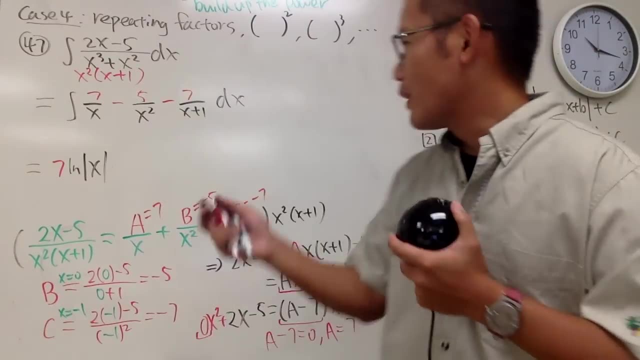 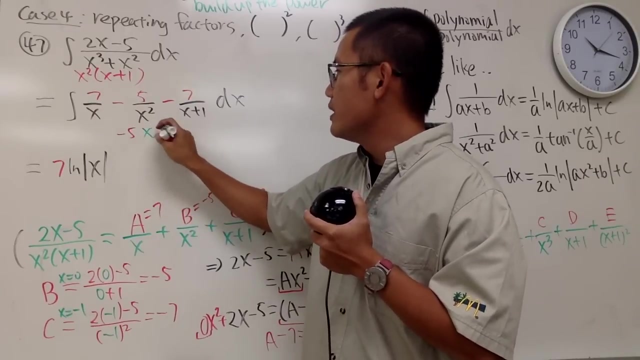 Right, This is how we do it: Reverse power rule all the way to category number 2, which is what Six hours ago- I don't know Five hours ago, something like that. Anyway, this right here. You look at this as negative 5x to the negative 2 power. 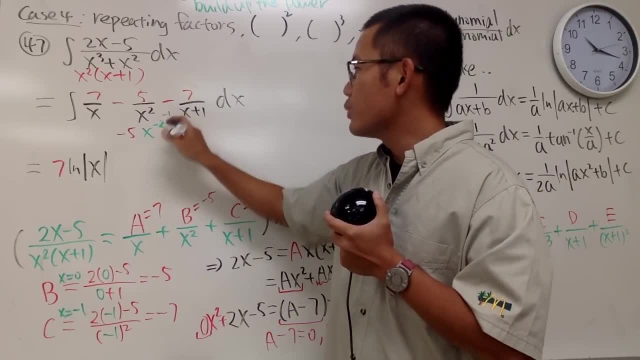 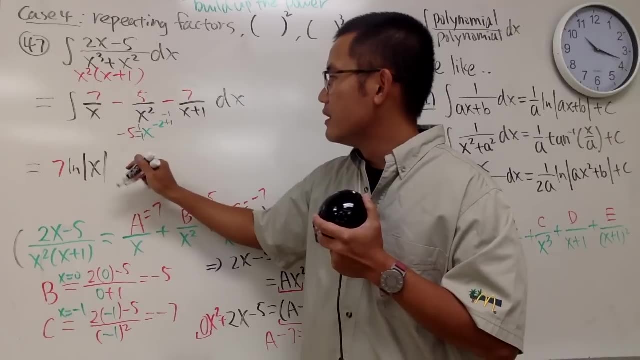 And what we do is you add 1 to the power, which is negative 1, and divide it by negative 1.. Negative 5 times negative 1 is positive 5.. So here let me just put down plus 5.. 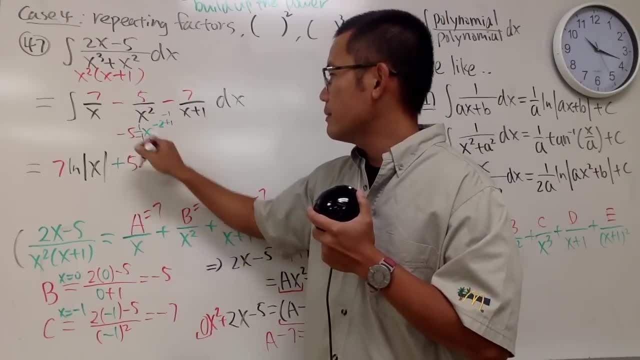 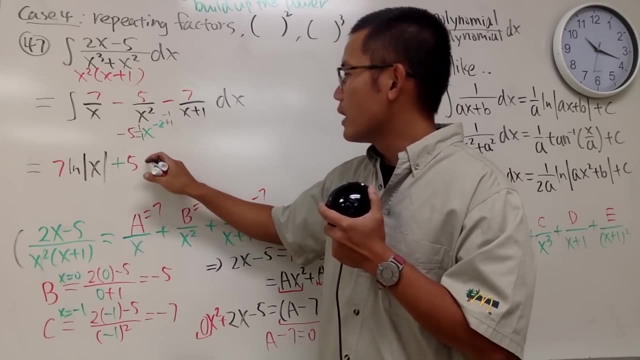 Plus the 5. Positive 5, yeah, And then we have x to the negative 1 power. So we have the 1 over x. So I will just put it as 5 over x. Let's just put it on 5 over x. 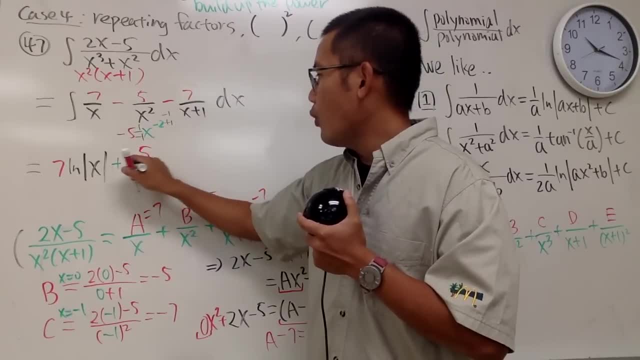 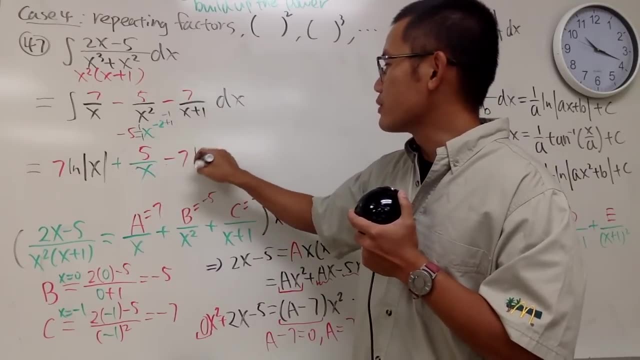 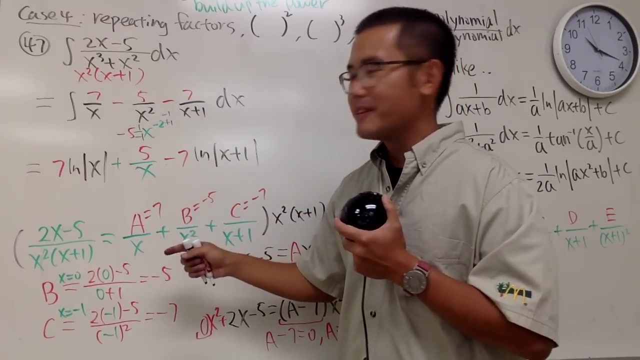 Positive 5 over x, And this is the legit way to do it. Lastly, minus 7.. And we have the natural log And we have absolute value of x plus 1.. Just like this. That is it. That's it. 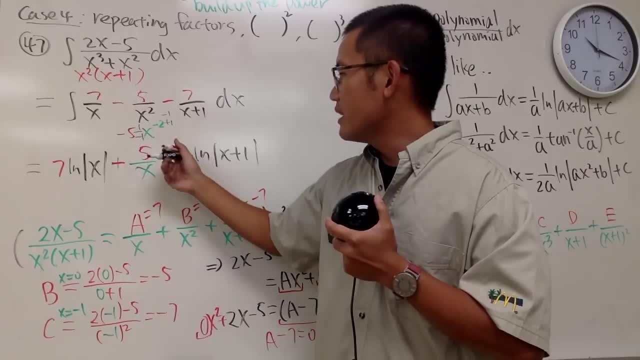 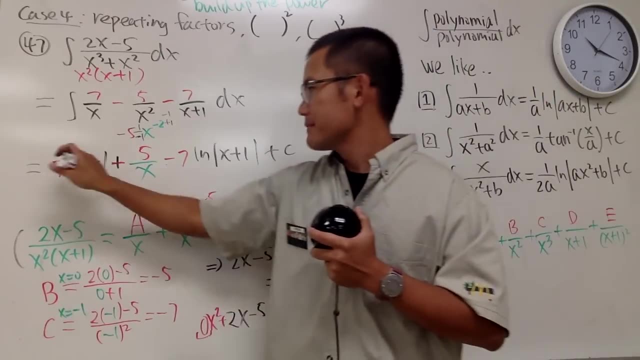 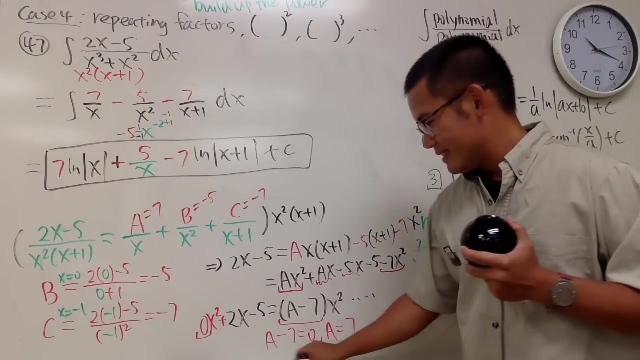 And technically I should have done like this Negative here, But we have another negative. So negative negative becomes positive. Much better, That's it. Put a plus c Done. Honestly, I never thought that I would become a teacher. 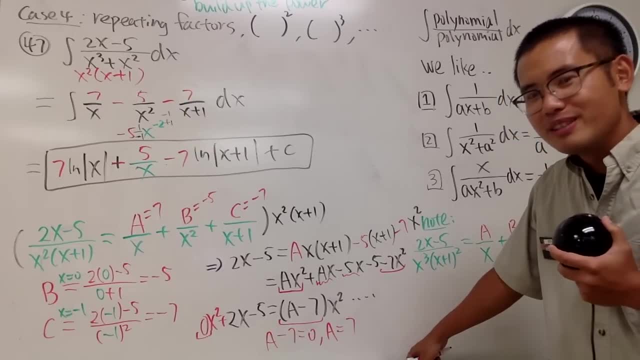 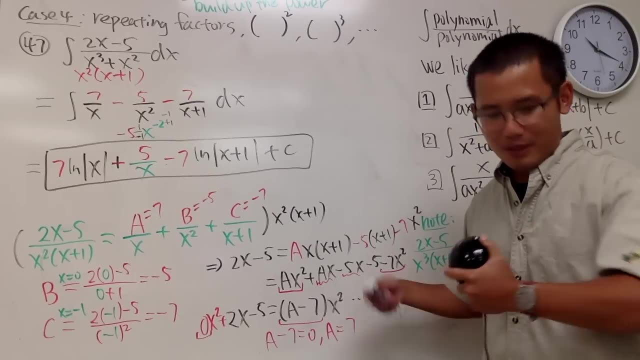 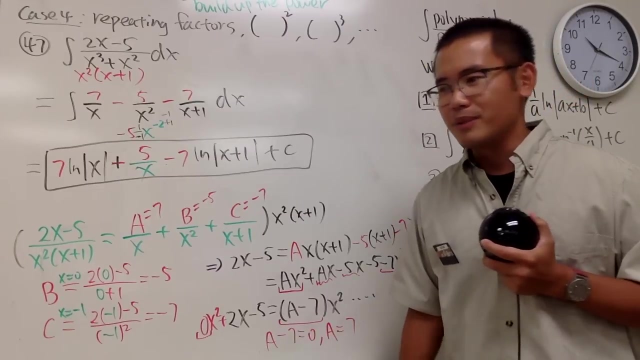 Until the time that my high school teachers inspired me. Of course, big thanks to Mr Sergio Salas, who helped me to get my first part-time job at McDonald's, And that's perhaps my biggest turning point- My first and also my biggest turning point in my life. 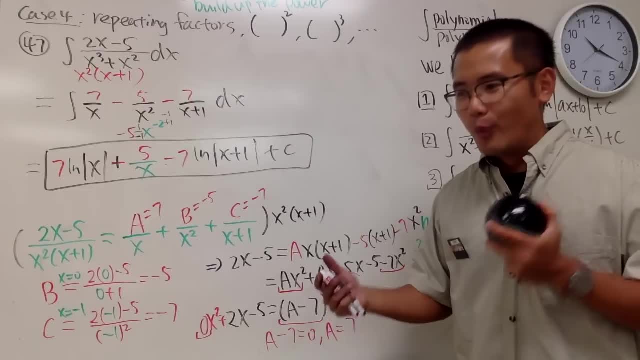 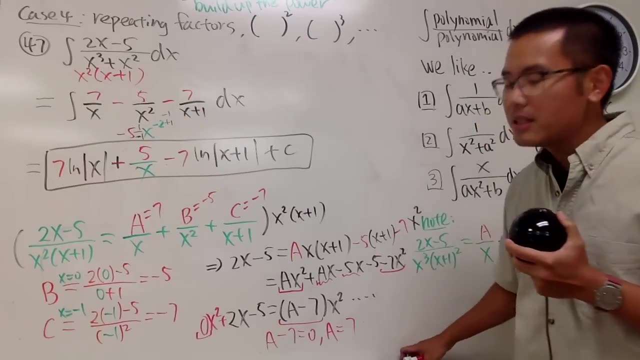 Because that was the first time that I started to go out and talk to people and actually work for my money so I can support myself and also support my parents and all that. Just give them some money and all that, And thanks to Mr Thomas Schneider. 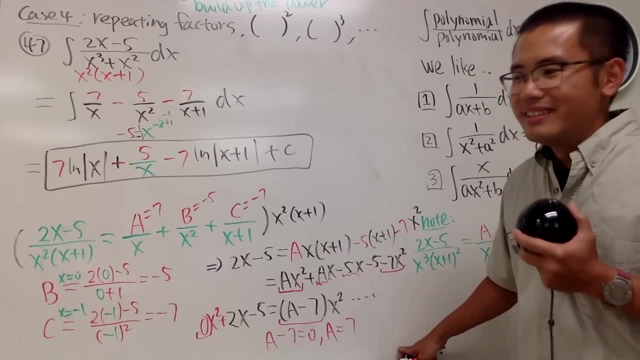 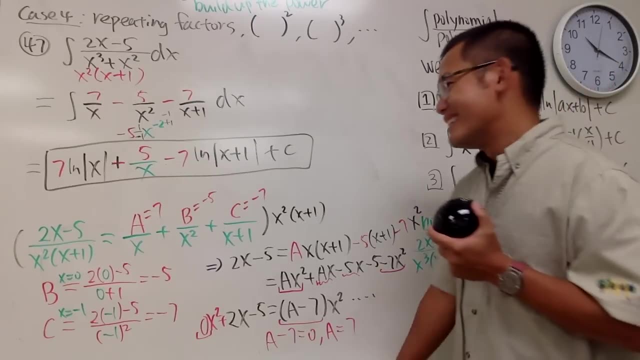 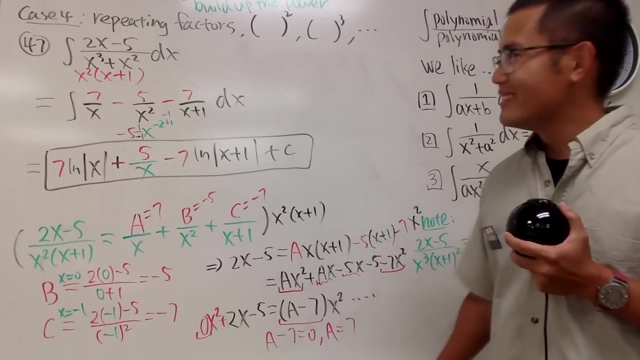 And he was my AP calculus teacher. And, of course, thanks to Mr Dennis Yeo, And they were just my high school teachers. Yeah, They were the ones that made me become. They made me realize that teaching is wonderful, Helping others is wonderful. 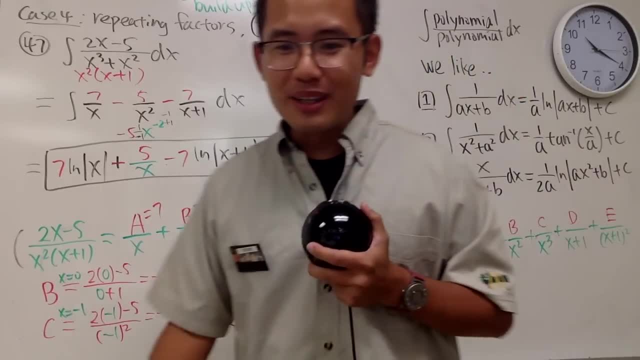 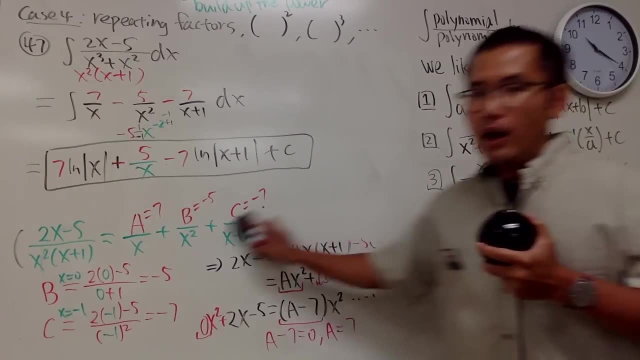 We're not done yet. We have a couple more to go. I just want to tell you guys a few things, That's all All right. A few more questions for you guys, That's all. So we have done all the cases. 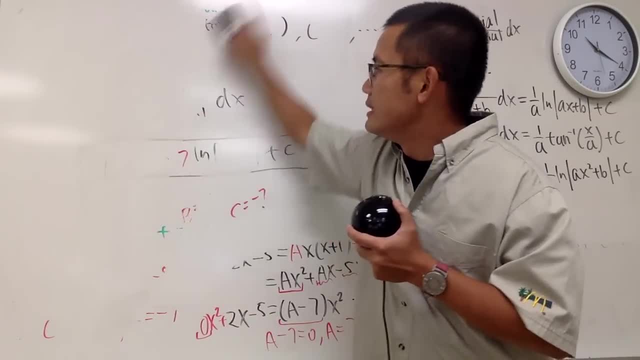 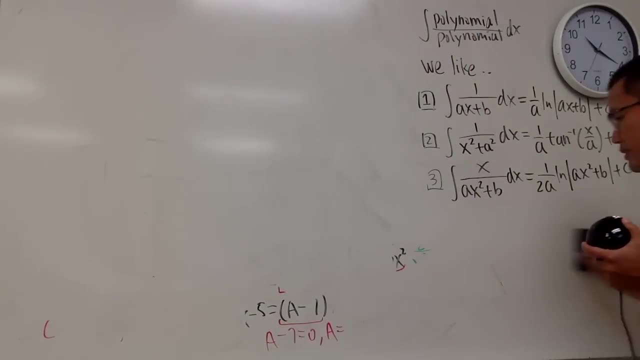 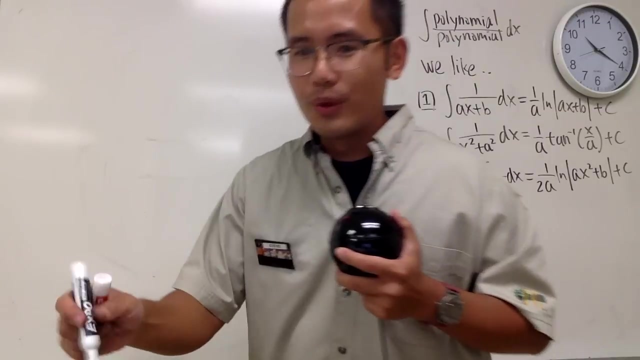 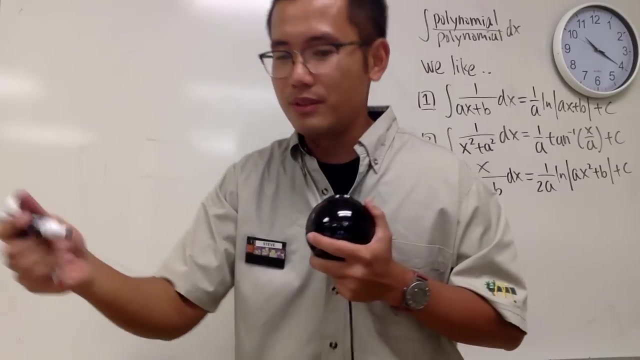 And now I just want you guys to, I just want you guys to work on these questions. Three more questions, Hopefully another 20 minutes or so. I'll try to work it out slightly quicker. I will actually use my older marker. This one here was better and hopefully still better. anyway. 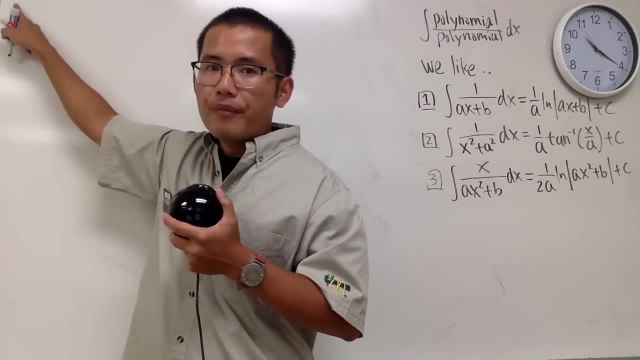 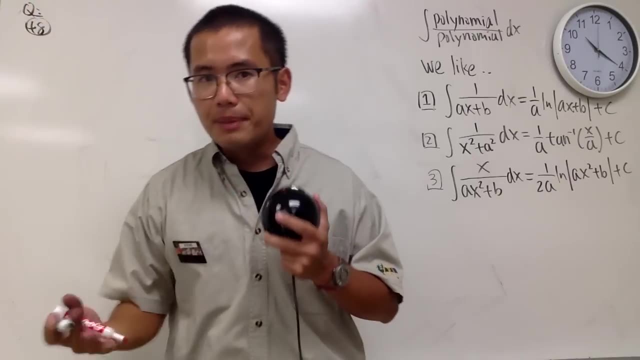 Number 48. So here you don't know what case it is, So just like question okay, Just question okay, So 48. It depends on the situation. So just think about how you are going to do this, this and that. 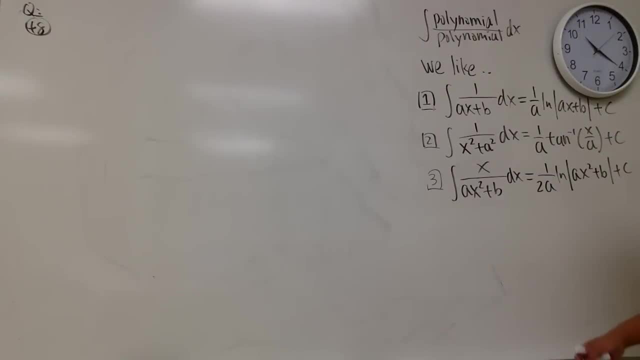 Oh, by the way, Oh man, I erased this. Serious Anyway. so this is how you set up the repeating situation, right? Repeating factors: Again. the example was 2x minus 5 over x squared. If you have the 2x. 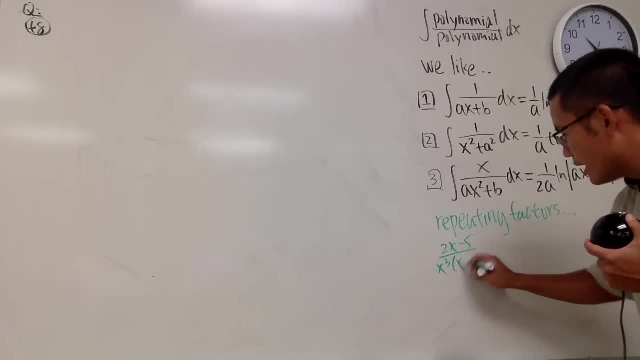 minus 5 over x to the third power, x plus 1 to the second power. This right here is a over x plus b over x, squared, plus z over x, cubed, plus d over x plus 1 to the first, plus e over x plus 1 to the second. 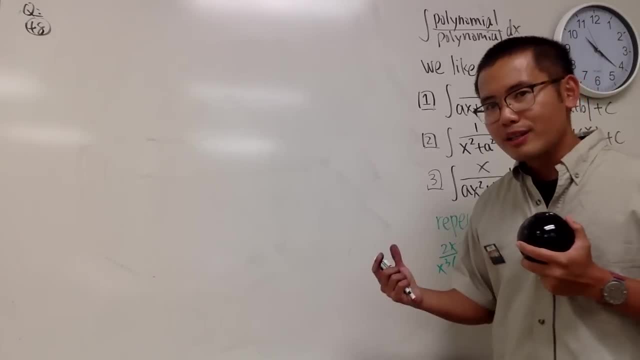 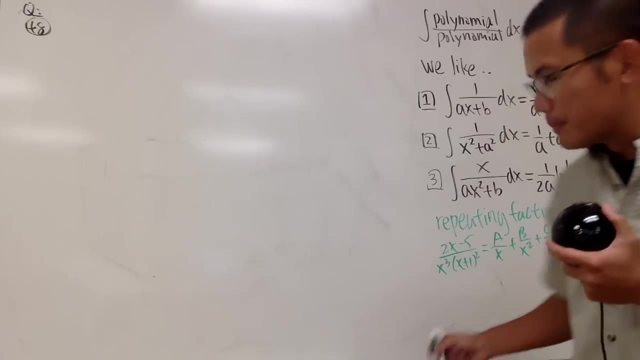 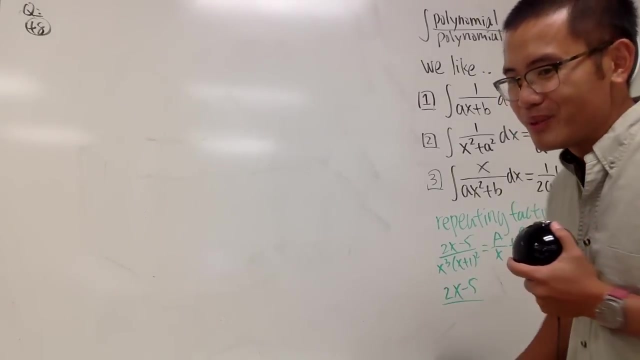 Right? Well, again you might have quadratic factors being repeated, So let me just give you a quick example to have one. So suppose you have this: 2x minus 5.. Again, the top doesn't matter. As long as the degree is lower than the bottom, you are good to go. 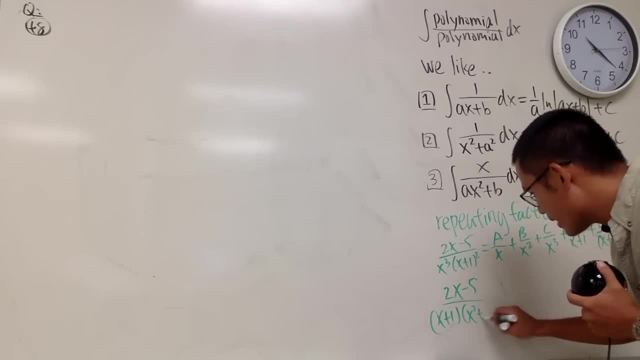 Anyway, suppose you have x plus 1, and you have x squared plus 4 squared. Well, this, right here you see, the first factor is x plus 1, and you have constant on the top. That's good, This is quadratic and it's being repeated. 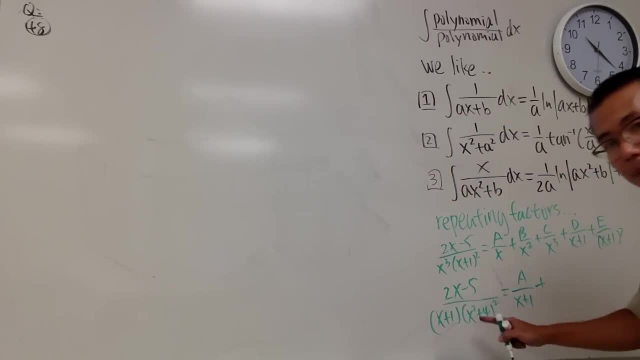 I erased it, unfortunately, But we are going to build up the power like what we talked about earlier. First, you put down x squared plus 4.. Well, this is a quadratic. so what should we do on the top Linear? So be sure, you put down bx plus c. 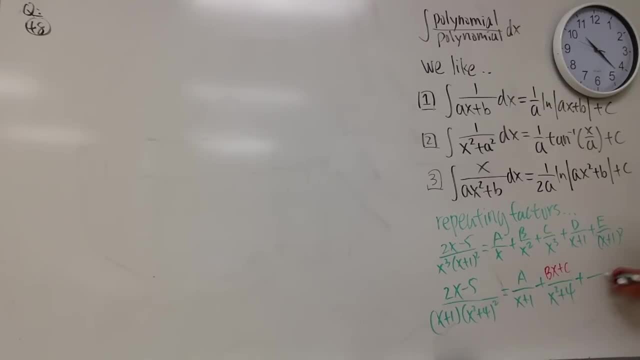 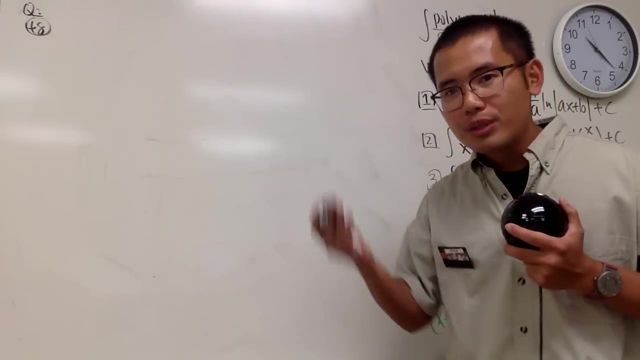 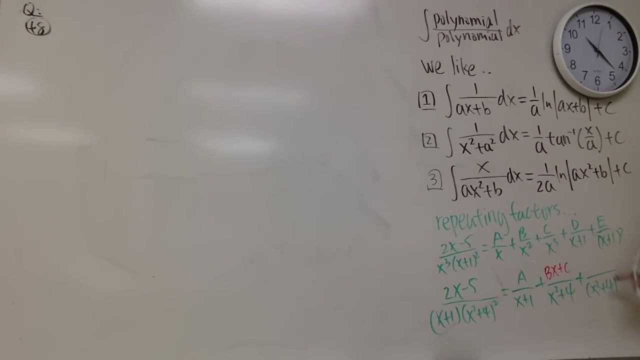 Next, we are going to build up the power to parentheses: x squared plus 4 squared. And what did we talk about earlier? When we build up the power, the top has to stay the same. Same kind, same kind, same kind. constant all that, and then same kind, same kind. 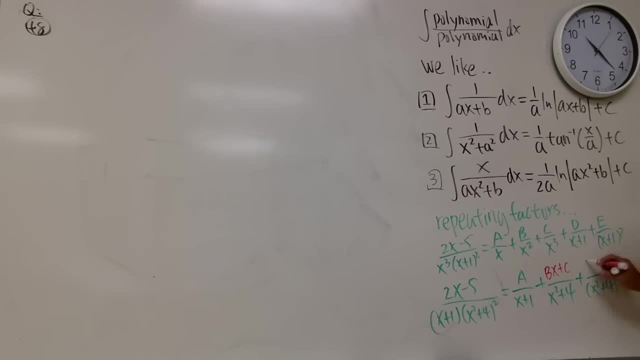 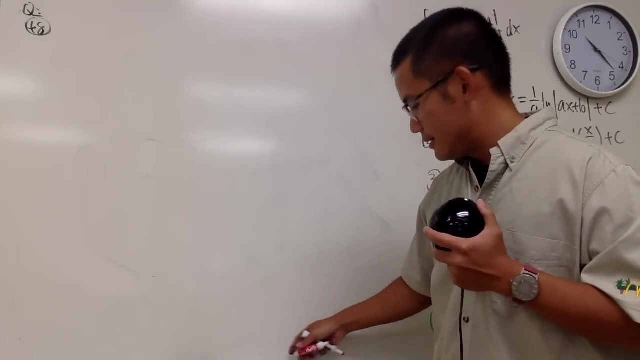 This right here, linear earlier. This right here, still linear. Oops, no, but you have to be different letters, So abc, dx plus e. So that's just some ideas. Okay, so we have a few more to go, That's all. 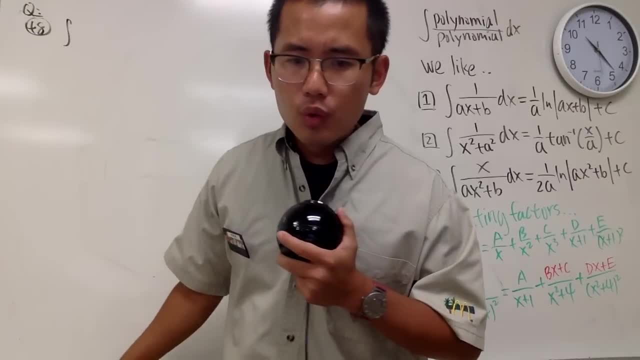 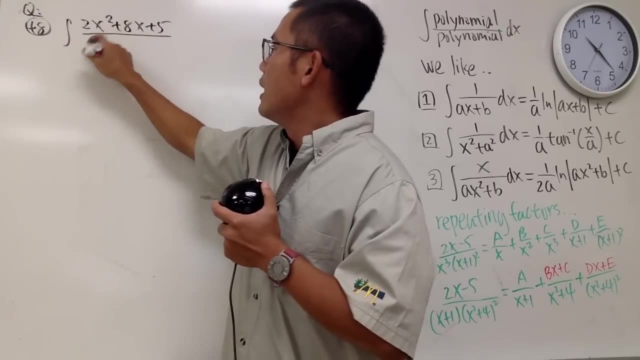 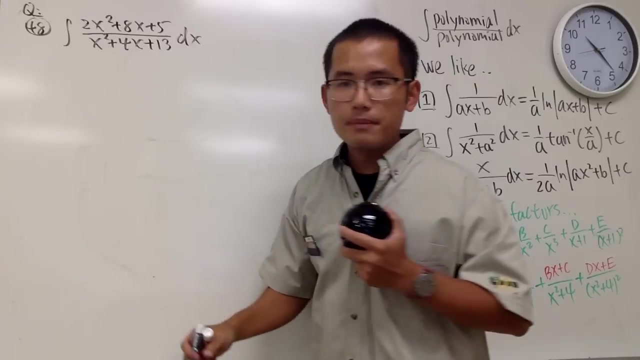 Not too bad, Integral, and we have 2x plus 2x, squared plus 8x plus 5 over x squared plus 4x plus 13.. Right, And I may have a big one over there. and I have a last one. 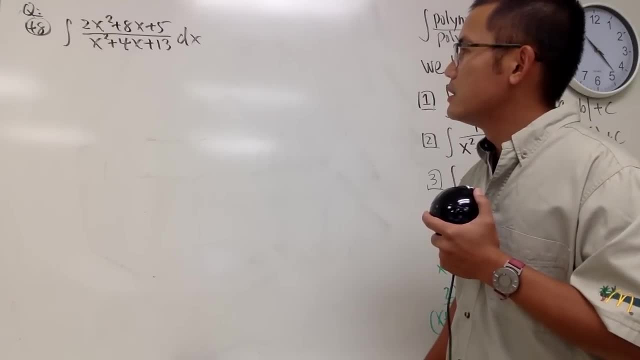 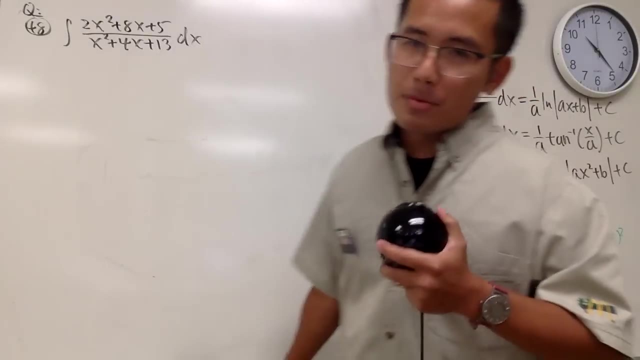 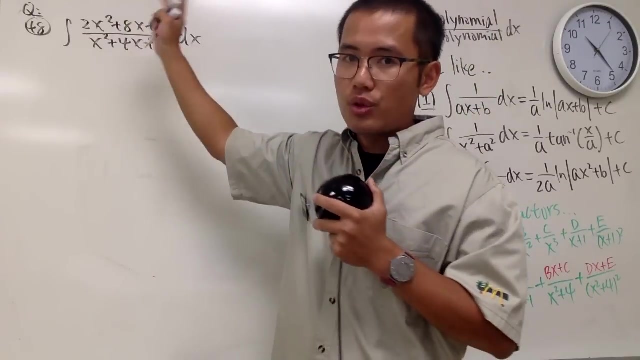 Hmm, All right, let's do this, And let's just do this one by one, Because I need to have this on the board. Okay, What should we do? Check the degree. Degree on the top is 2.. Degree on the bottom is 2.. 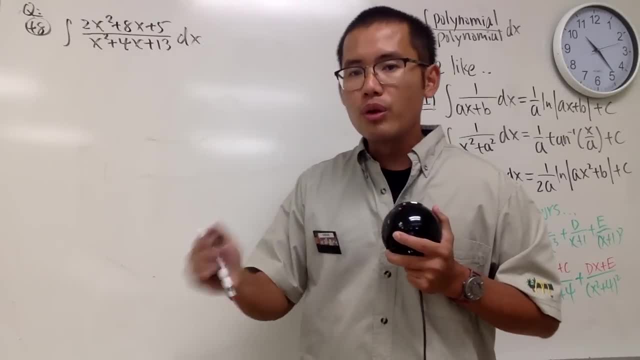 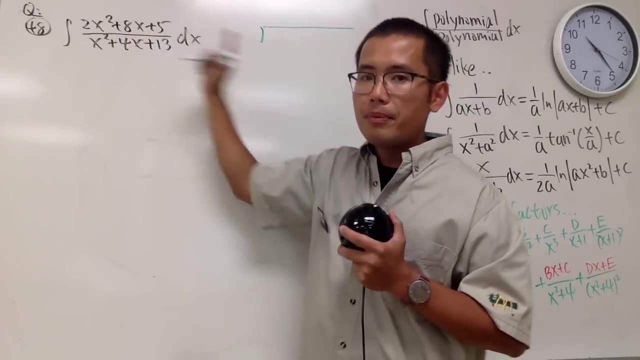 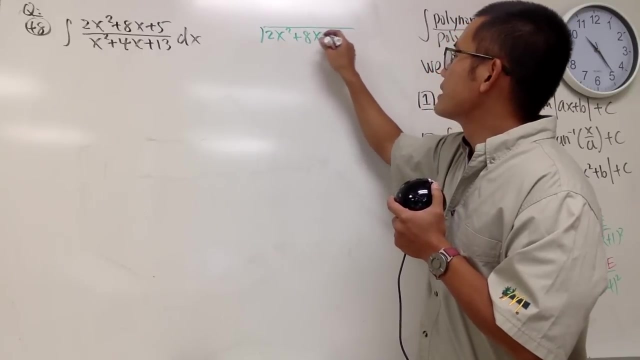 So go ahead and do long division. when the degrees are equal, Do long division. That is the key. So perhaps I will put down the long division right here on the side, The top inside. Namely, we have 2x squared plus 8x plus 5.. 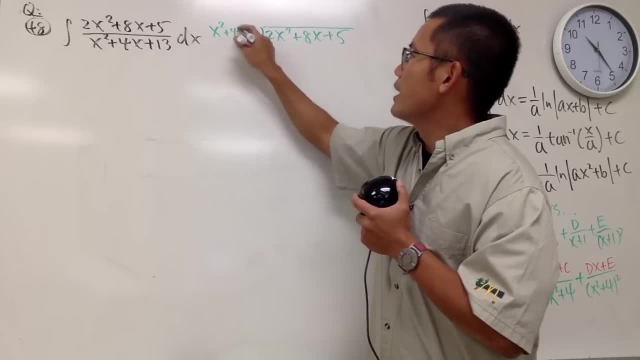 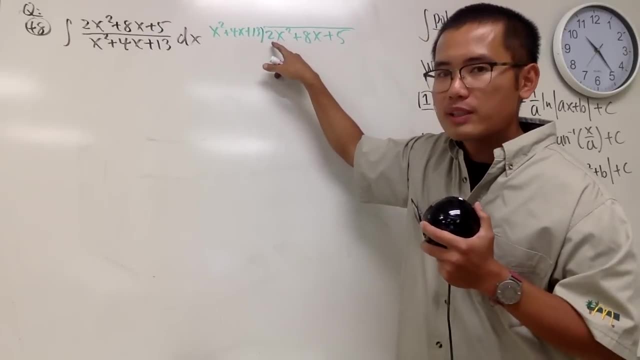 And then x squared plus 4x plus 13 on the whole side. Now I have x squared here. What times x squared will give us 2x squared? We need 2.. So 2 right here. 2 times this is 2x squared. 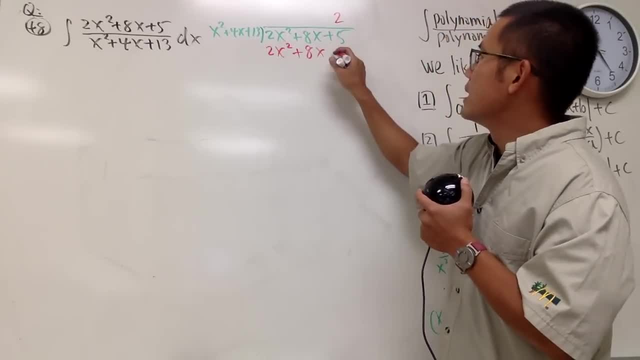 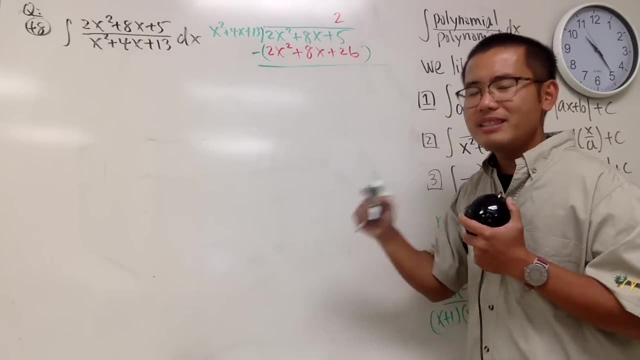 2 times that is plus 8x. 2 times that is plus 26.. Subtract: Nicely canceled it, Nicely canceled it: 5 minus 26 is negative 21.. So here we have minus 26.. Minus 21.. 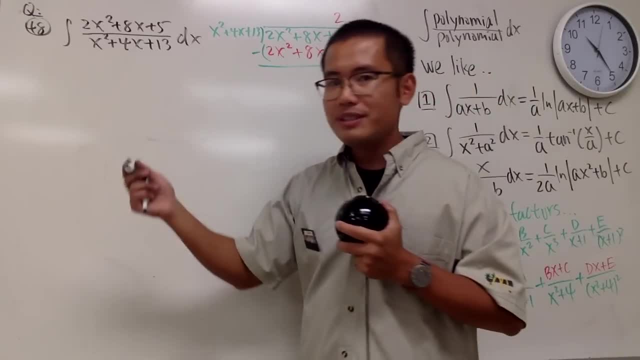 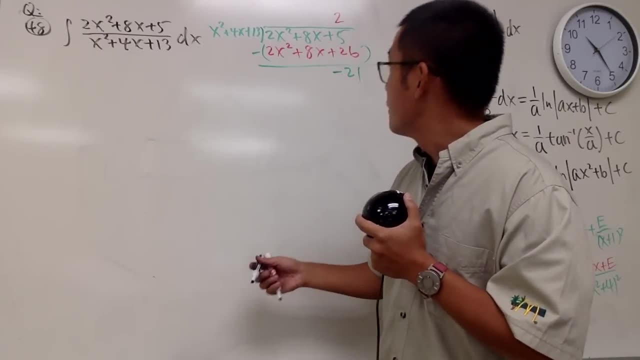 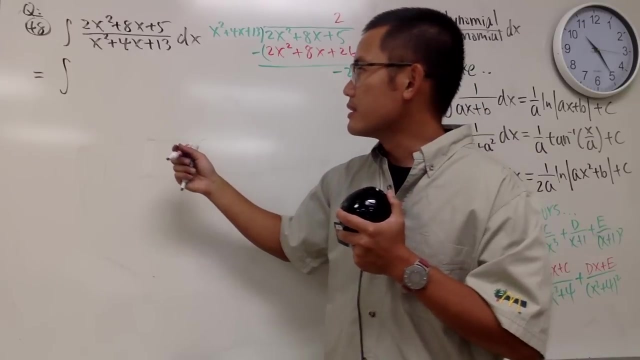 Now we are going to put this down right here. Here we have Oh wrong color, Here we go. Here we have the integral, And let's put it down like this. Let's just put it down like this: What color should I use? 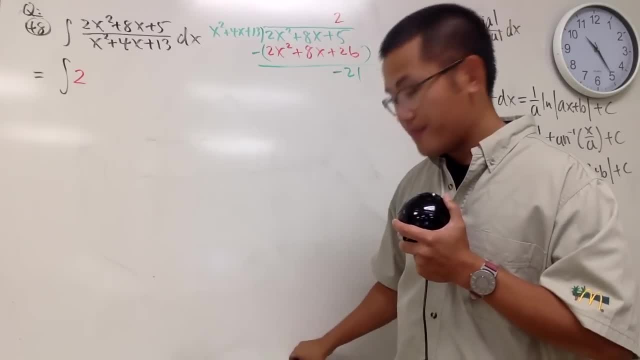 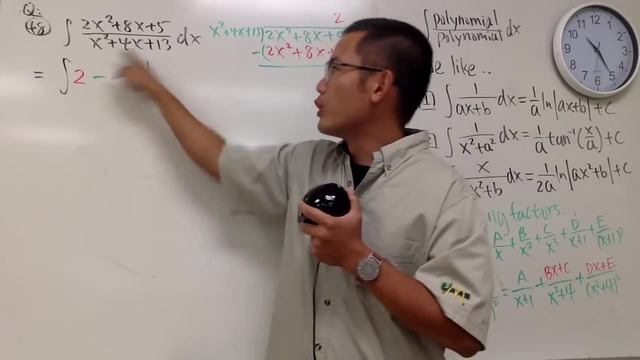 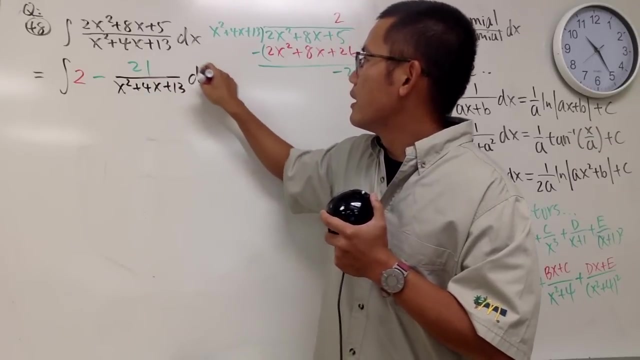 Let's just put it down like this: 2. We have minus 21. So we have minus 21 over the original denominator x squared plus 4x plus 13. And you see how we didn't care to factor this at the moment. 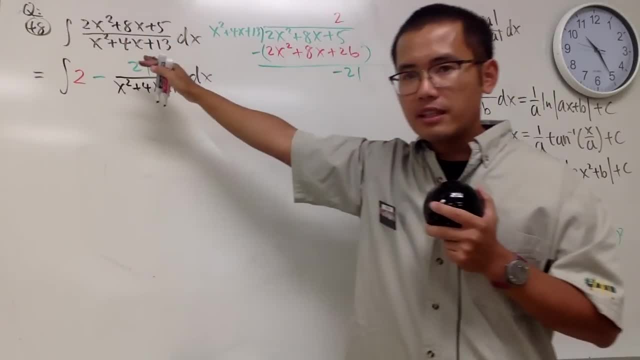 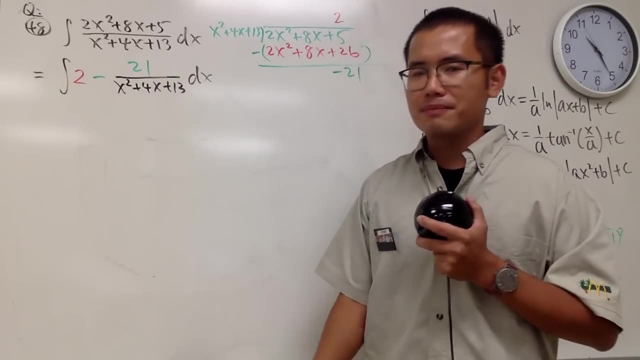 because we noticed that the degree on the top is the same as the degree on the bottom. So go ahead and do long division. That's the deal Now. we don't care about to see if we can factor this or not, But we can't. 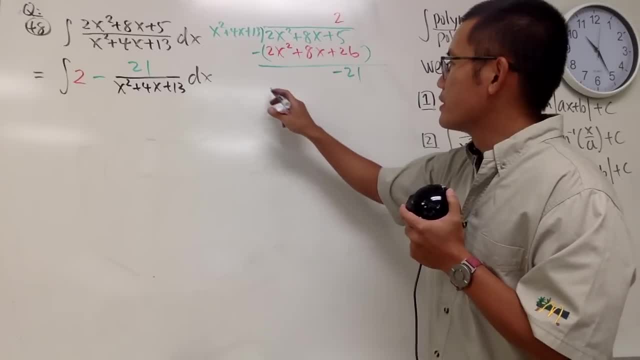 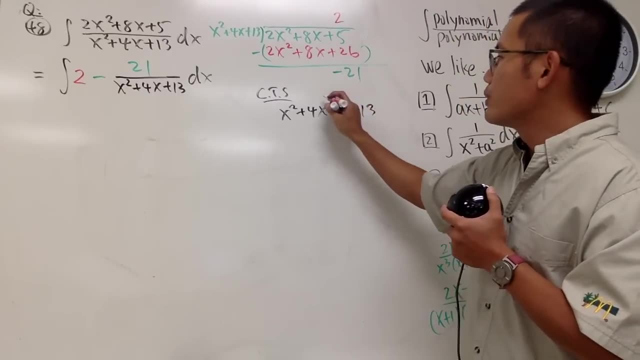 Complete the square. Yes, So right here, let's complete the square. So, CTS, I have x squared plus 4x. Leave a space plus 13.. Well, look at this number, because this is 1 already. So that's good. 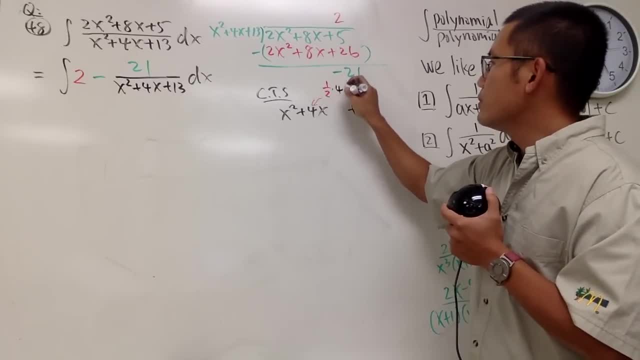 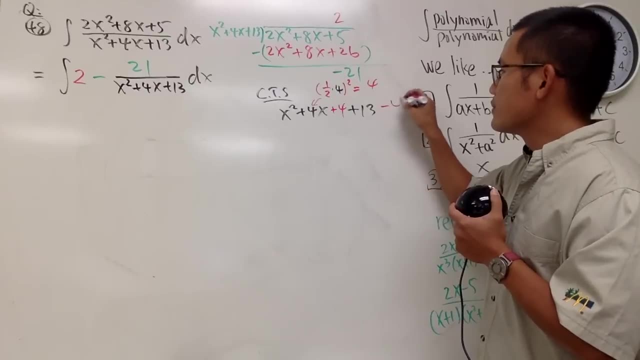 Take half of it. Half of 4 is 2.. But don't forget we have to square that. This is 2.. Square is 4.. We have to add 4 to it and minus 4 after that. This is the perfect square. 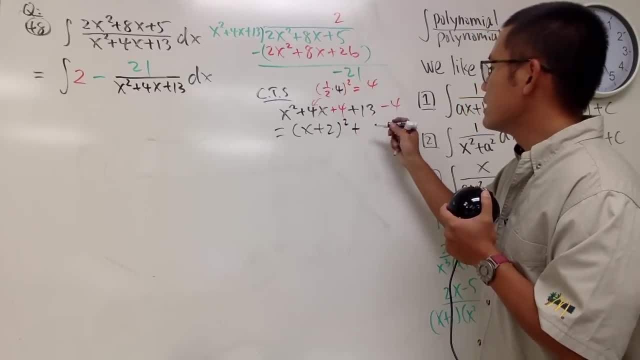 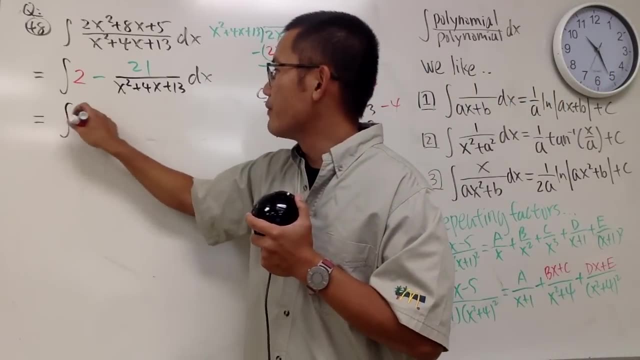 CX plus 2 squared, And this right here is just plus 9.. And let me just put on 9.. Now we'll come back here. This is the integral of 2. And let me just keep the minus. Let me do this. 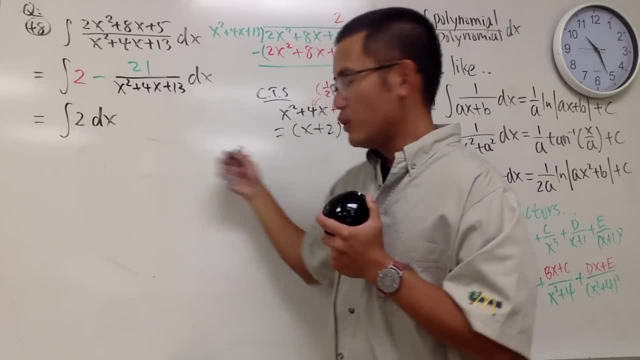 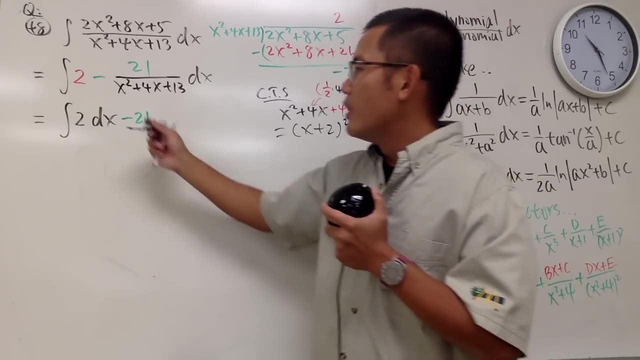 I'll close the integral: yeah And then minus 21.. Just put that in the front. And this is still in green: Minus 21.. Then we have the integral. Now we just have a 1 on the top, yeah. 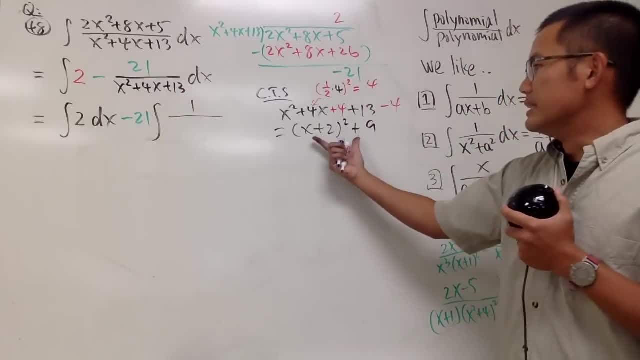 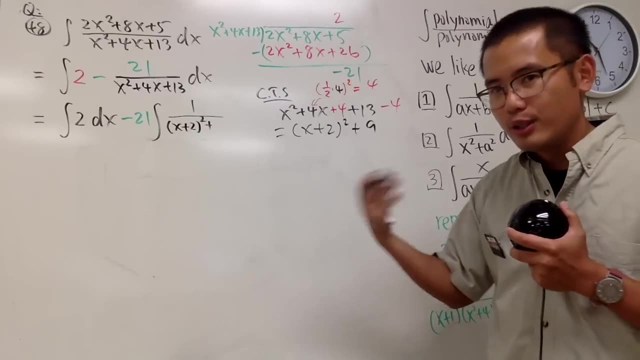 Over. Well, in this case it's this: X plus 2 squared plus 9 is the same as 3 squared, So I put down 3 squared like this dx. Well, for this one we can just do a use-up real quick. 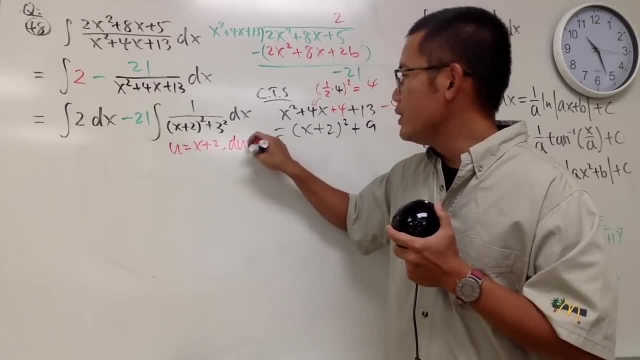 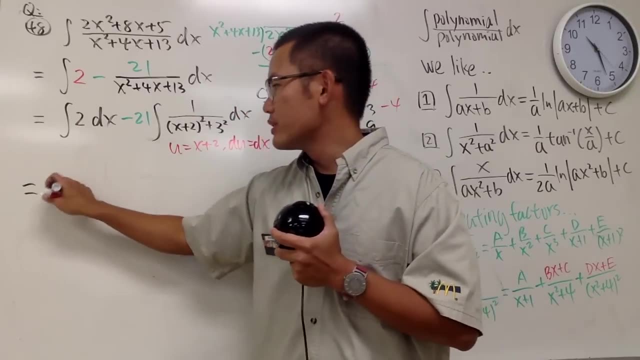 Let u equal to x plus 2.. And you notice du is the same as dx, So you can actually do this in your head. Anyway, the integral of 2 in the x-world is just 9 squared, So it's actually equal to 2x. 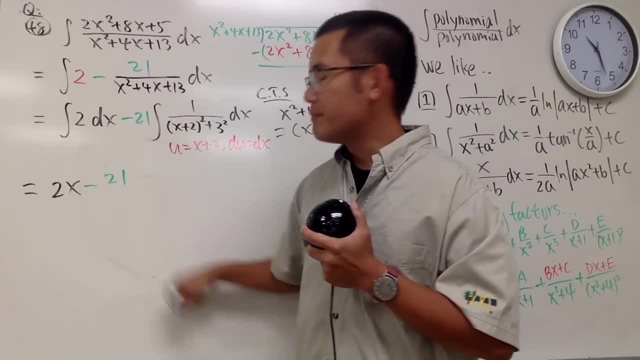 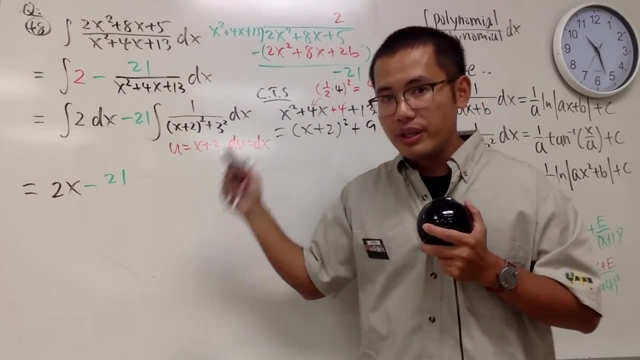 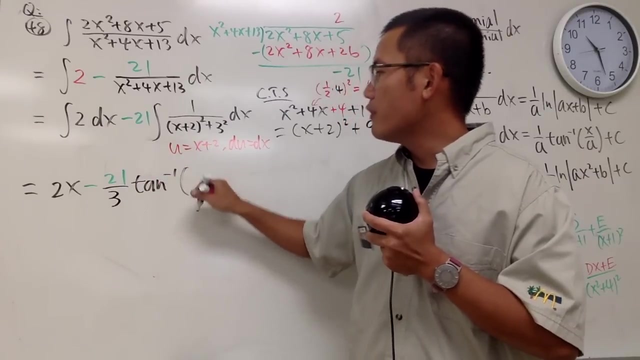 Nice. Now this is the constant multiple, So we have minus 21.. And the integral right here is 1 over 8.. And the 8 right here is 3.. So we have negative 21 over 3.. And multiply by the inverse tangent of u. 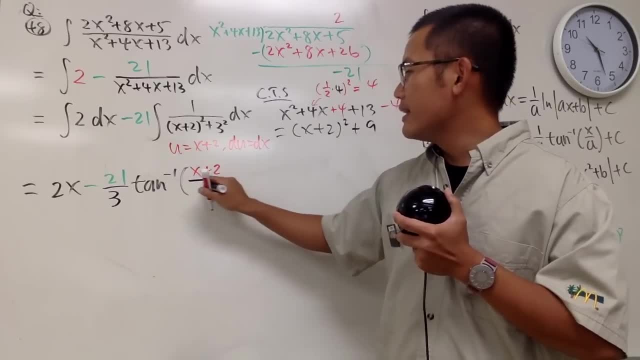 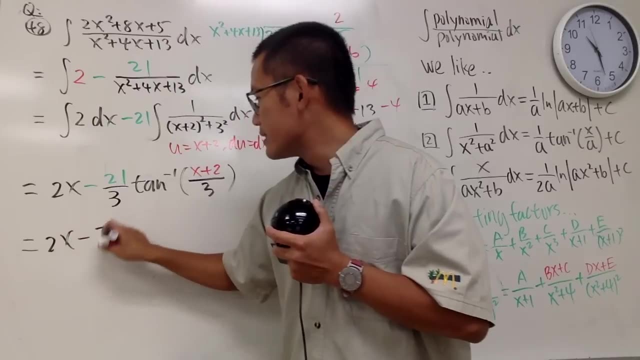 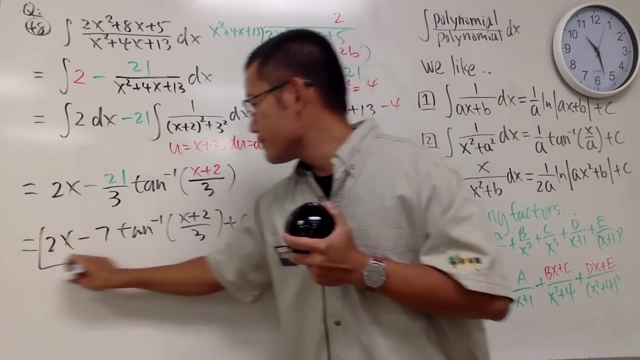 which is just that X plus 2.. And then divided by 3, like this: Seriously, yeah, Simplify this. 2x minus 7, inverse tangent of x plus 2 over 3, like this: So that's it. 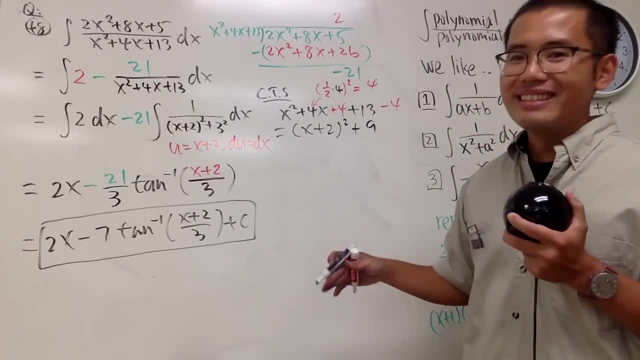 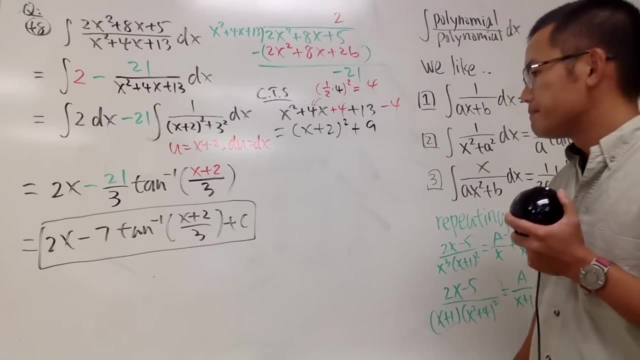 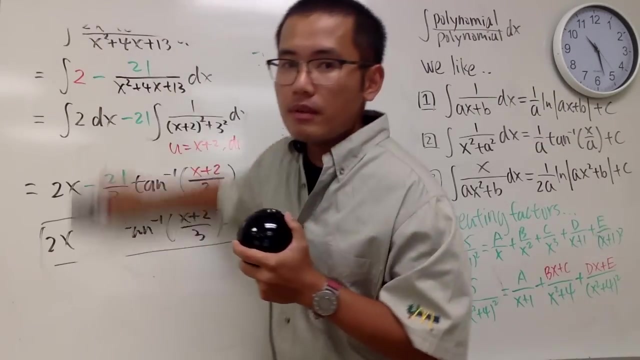 So this is the combination of the first case and also the third case. You have to complete the square because you have irreducible quadratic, And you also have to do long division in the beginning. All right, Two more to go. Yeah, this is making me really happy too. 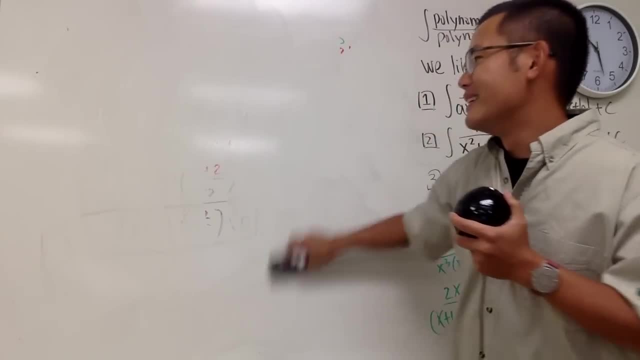 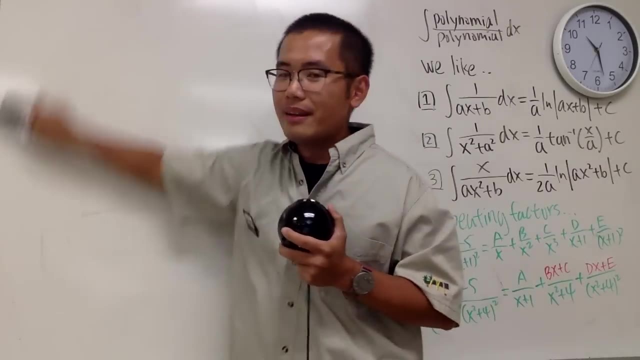 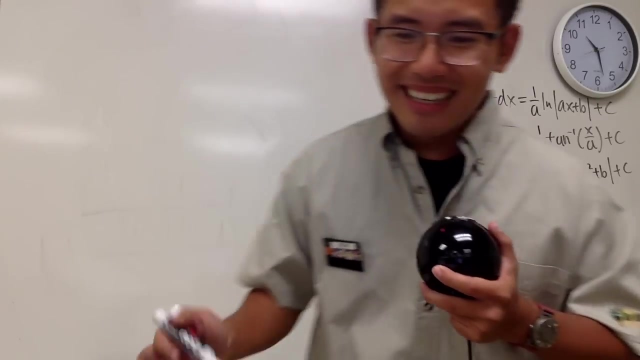 Again, this right here is meant to be, And the truth is, yeah, it takes me three weeks to go over this right here and also practice with my students and all that, And I'm giving you guys this in like six hours, Yeah. 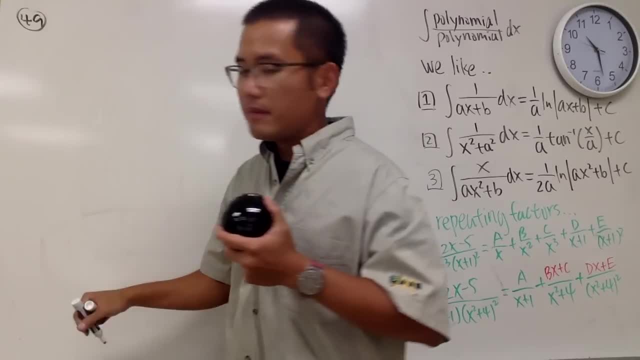 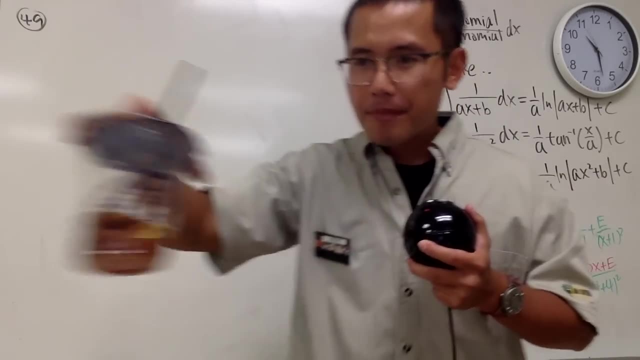 So this right here, let's see 49.. Yeah, Usually I will do this in like six hours. I will do this in like two, three weeks for my Cal 2 class, But we're doing this in like six hours for all the methods that you have to know for Cal 2.. 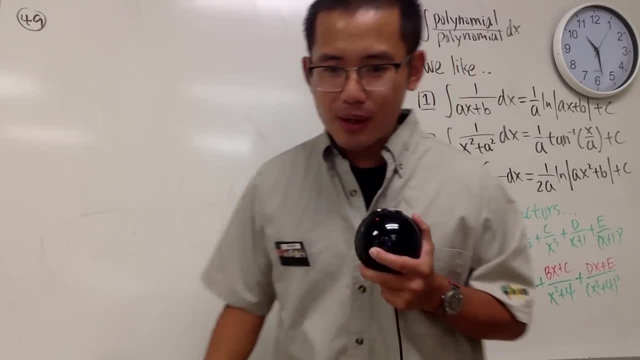 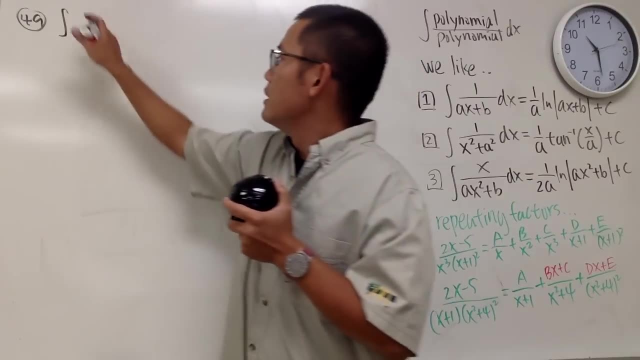 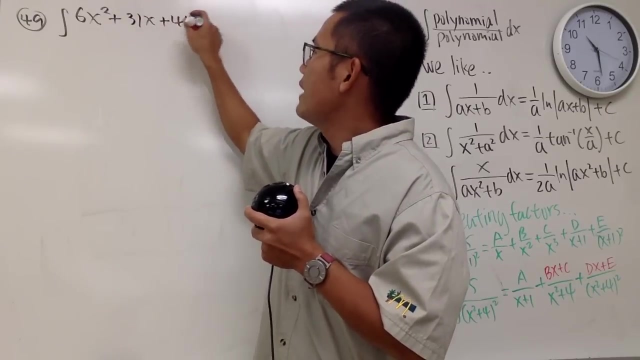 So hopefully this helps you for your practice right, For your Cal 2 and all that stuff. All right, 49.. Let's look at the integral of 6x squared plus 31x plus 45.. All over x cubed. 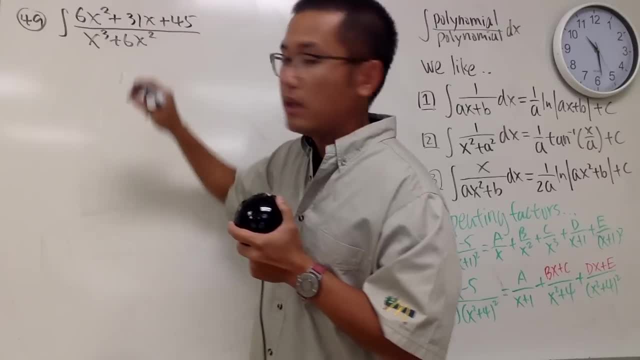 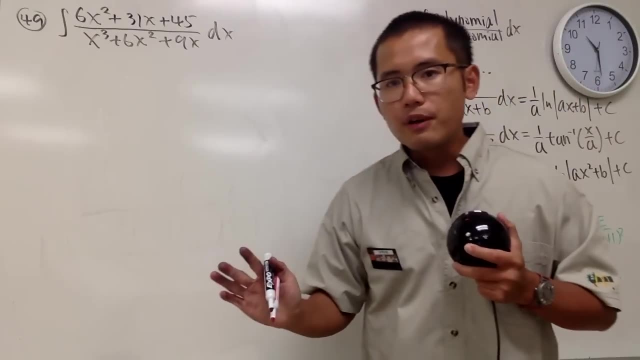 Oh my God, x cubed plus 6x squared plus 9x dx, Like that. First thing first. The degree on the top is 2.. The degree on the bottom is 3. So we don't need long division. 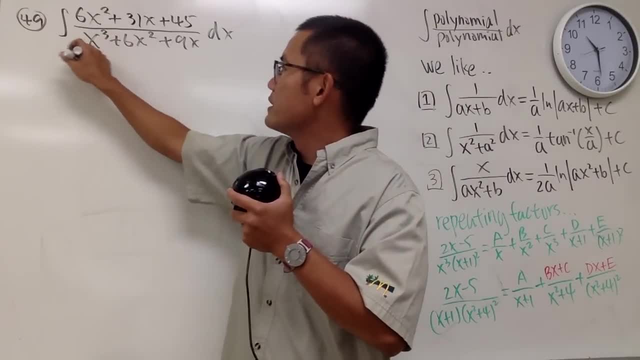 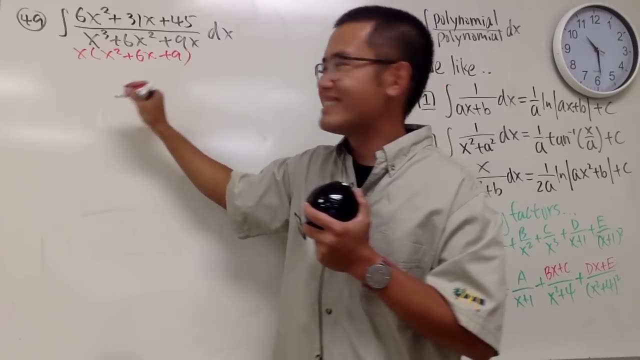 Let's factor out the bottom For this one. we can first take on x. We have x squared plus 6x plus 9.. Can we keep going? Yes, So we have x times x plus 3 squared. Oh my God. 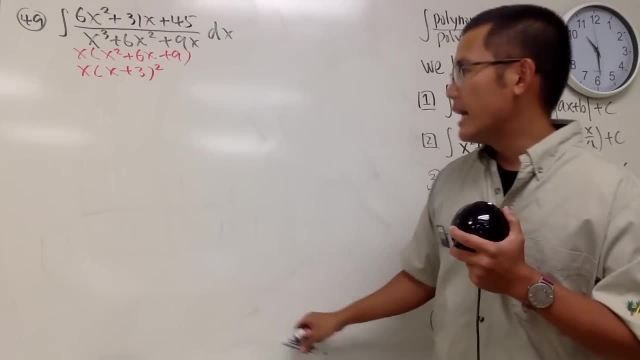 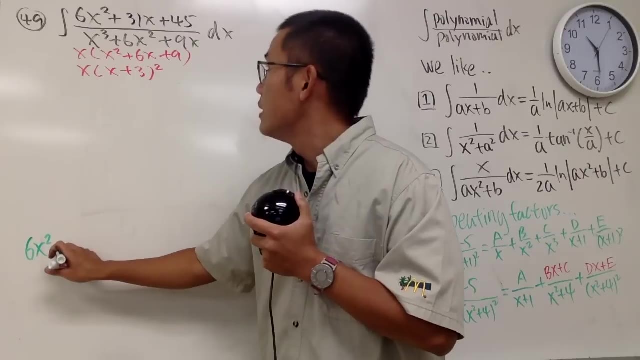 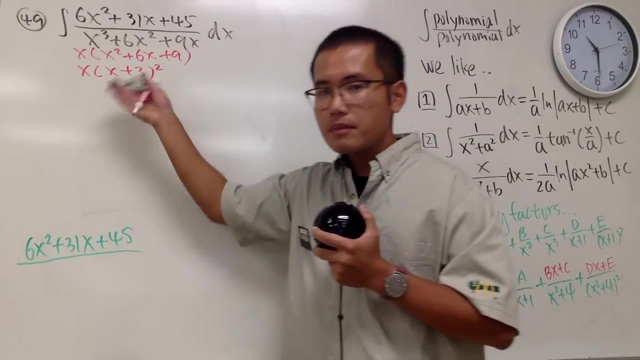 This is a repeating situation, So we have to build out the power. And let's do the partial fractions down here again. So I'll put it down: 6x squared plus 31x plus 45, over x times x plus 3 squared. 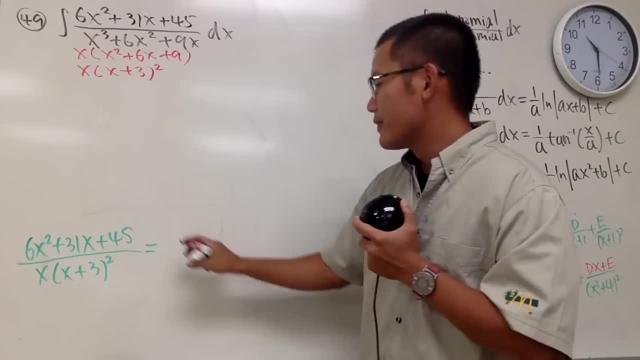 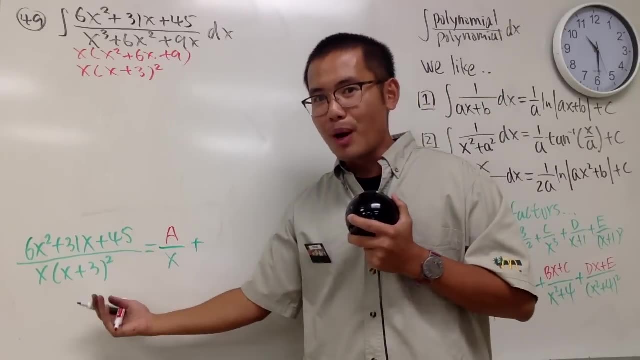 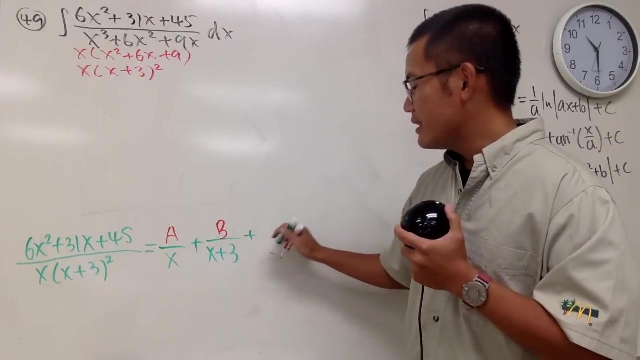 Here we go. x is by itself. That's nice. So we have a over x. Then we have to build out the powers. now This is linear, Not so bad: x plus 3.. And then the top is b. And then build out the power to x plus 3 squared. 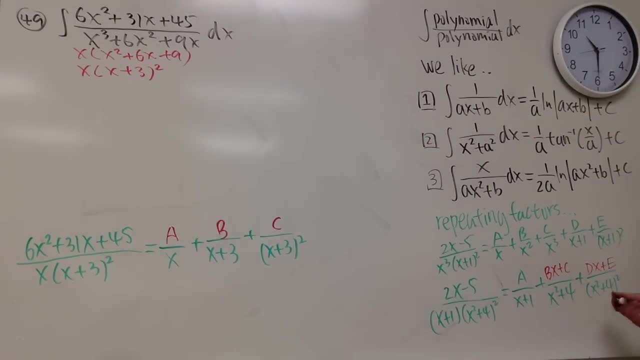 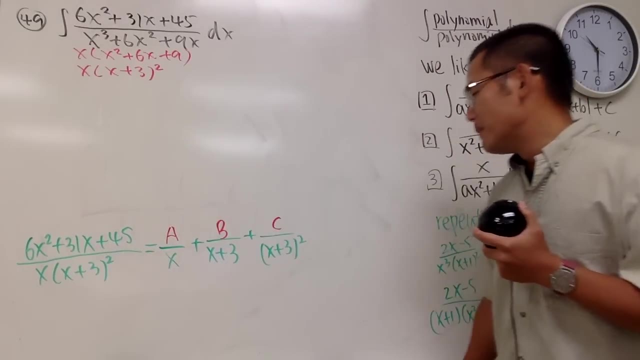 And we need a- c. You might be wondering: why don't I do this? Well, a, b, c, d, e, Come on Seriously, Maybe once in a while, but I don't know. It's just rather tedious. 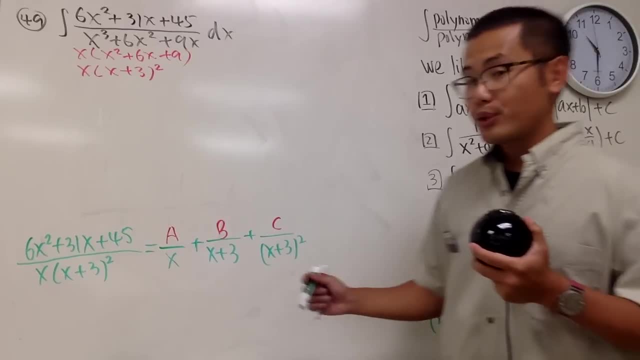 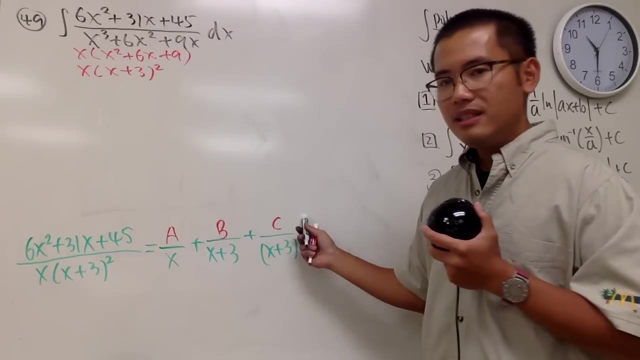 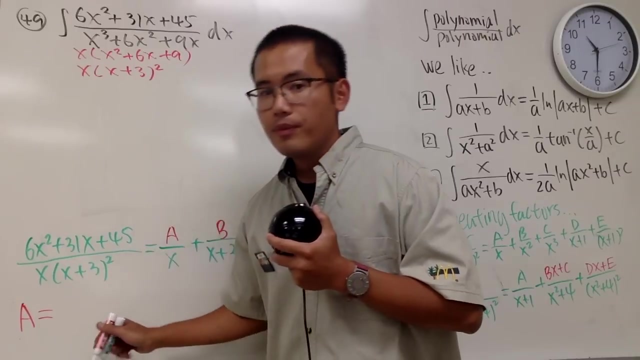 That's why- OK, Good news, We can do couple up for two letters. What This case? a and c, Because a has a denominator right here. So let's go ahead and find that out: a equals when x is equal to 0. 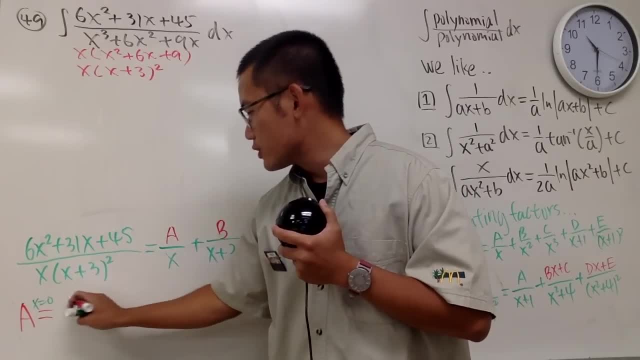 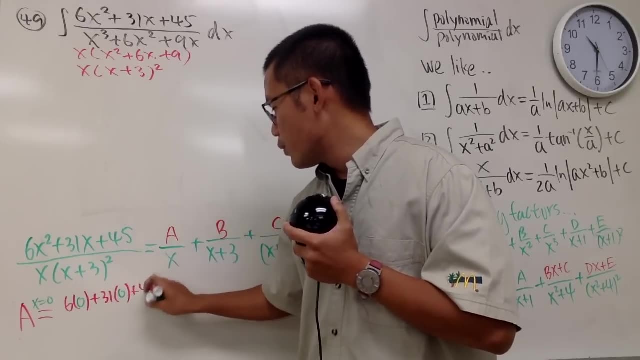 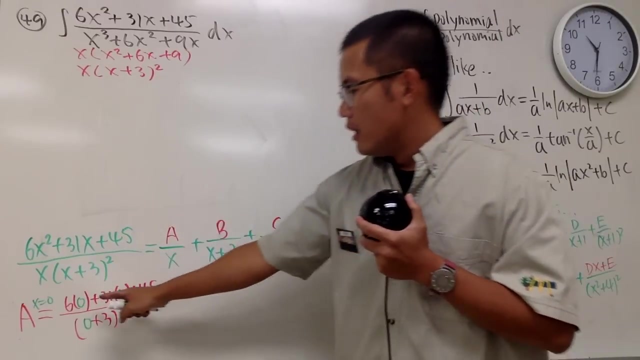 Let's do this up already. Put in 0, 0, 0, right? So I'll show you guys all the work: 6 times 0 plus 31 times 0 plus 45.. All over, 0 plus 3, squared like this: 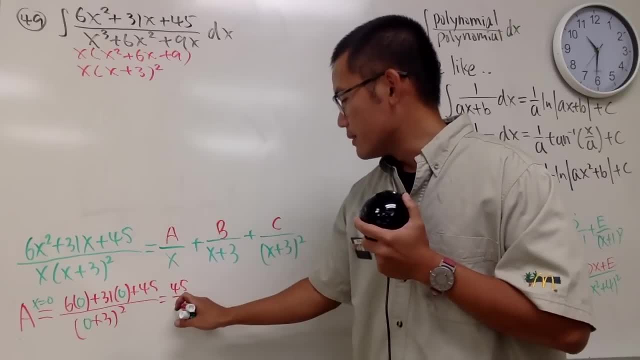 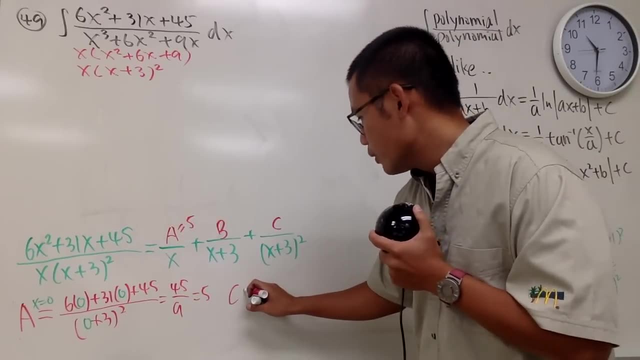 On the top is 45.. On the bottom is 3 squared, which is 9.. So all in all, it's 5.. Good, Now for c. We can also do couple up. This is the time when x is equal to negative 3.. 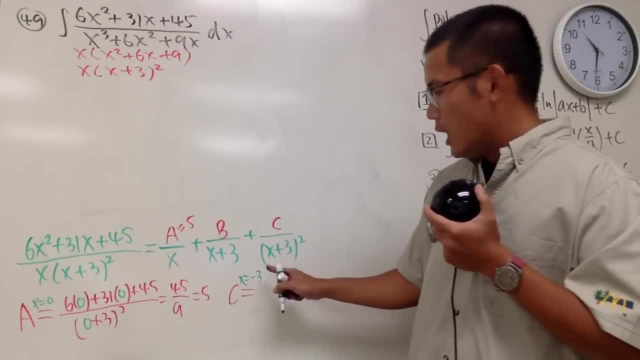 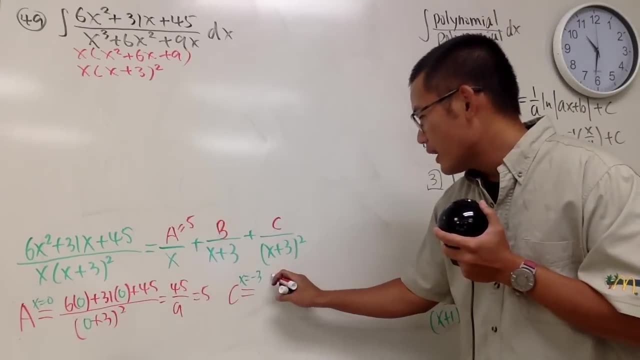 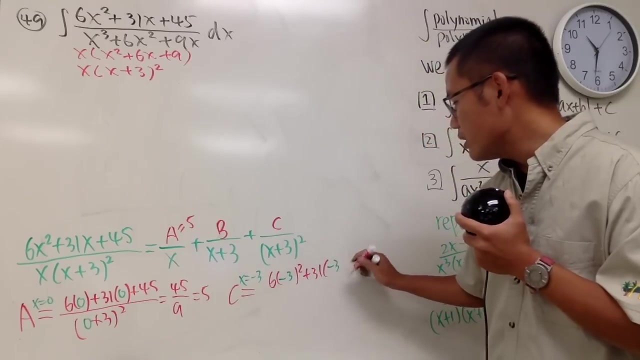 This time I didn't write down the wrong question. Yeah, Put in negative 3.. Man, I picked a big number, didn't I? I did Big expression, but it's OK. OK, 6 times negative 3 squared plus 31 times negative 3 plus 45.. 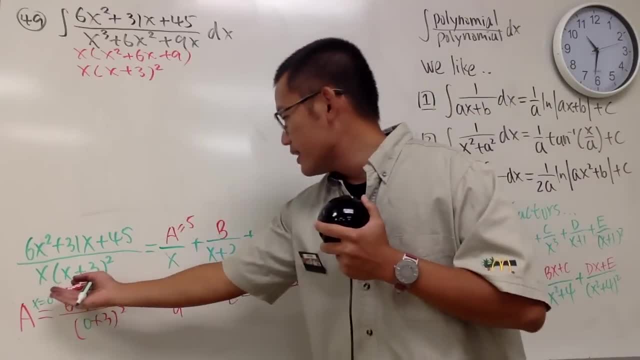 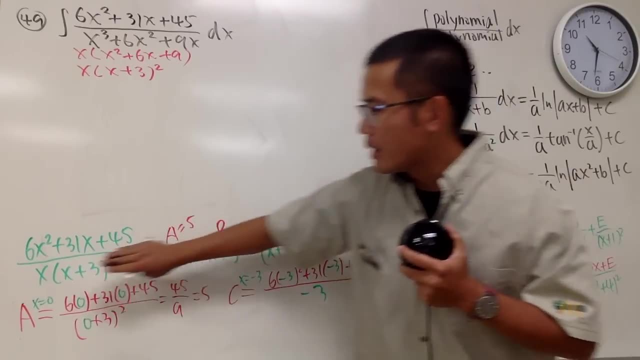 All over And on the bottom we have negative 3 right there. And remember, you have to couple up the same exact denominator, right, Couple up the same exact denominator so we don't have the other part. This is it, Yeah. 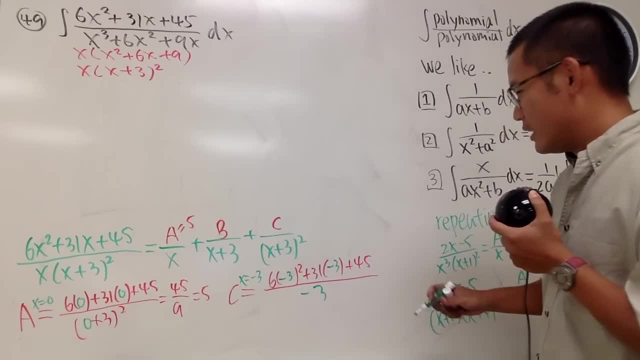 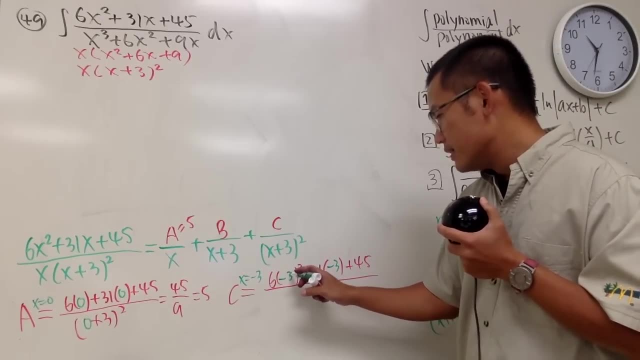 Good, Just want to make sure that microphone still works. All right, Man, this number is pretty big, so we'll see The top wise. this is 9 times 9 is 54.. And then this is minus 93.. 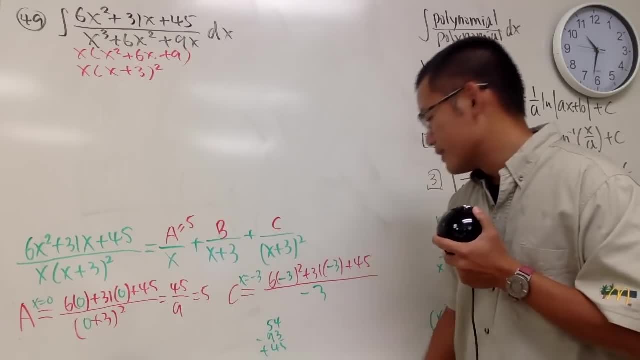 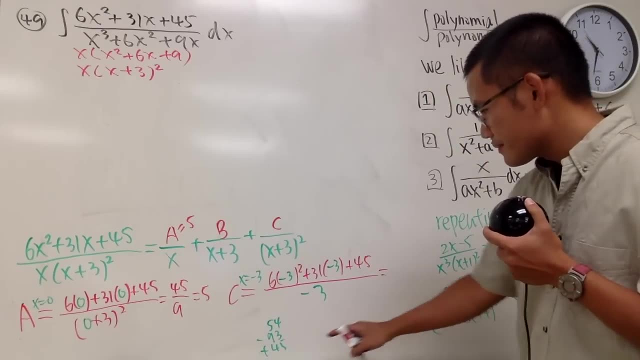 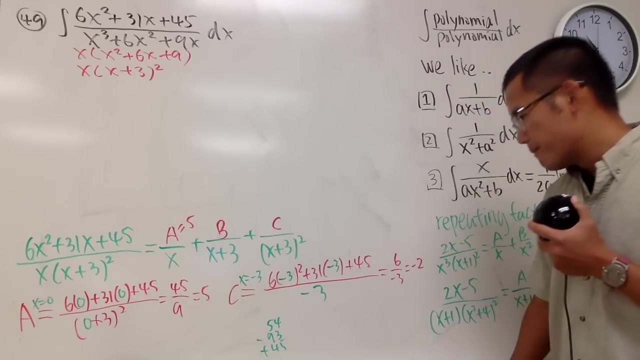 And then plus 45. Man, I think, OK, This is 99.. Yeah, 99.. So 99 minus that is 6 over negative 3.. So all you know is negative 2.. Yeah, Why not Negative 2.? 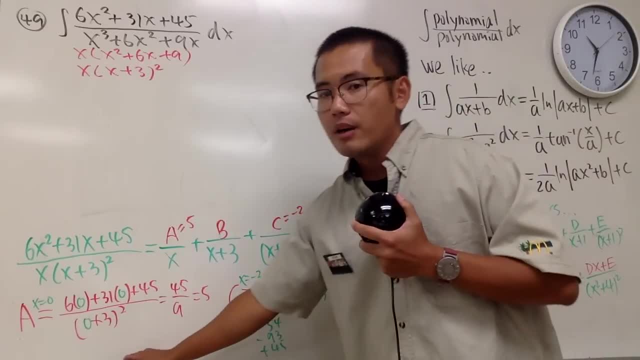 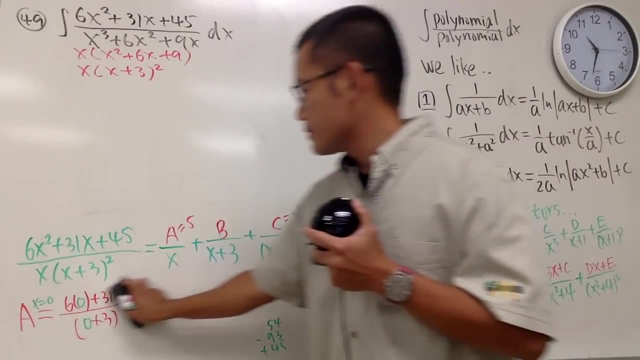 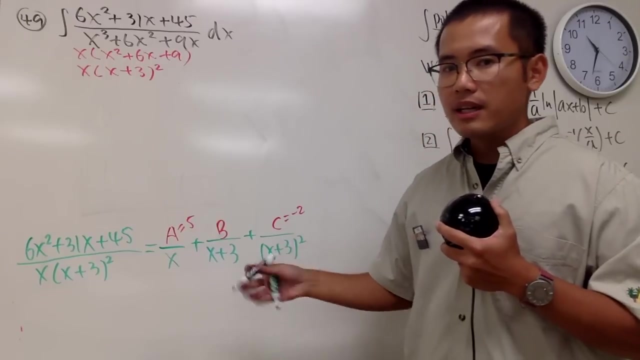 Still works out pretty nicely, So that's good, All right. So to save space, I'm going to erase this right here for the couple up, And now we'll do the dirty algebra right here, All right? Well, again for b. let's just clean up this right here. 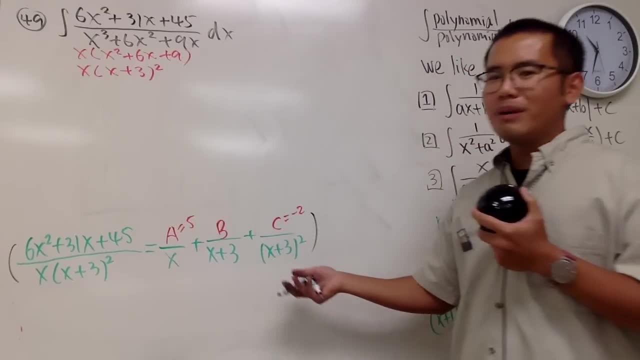 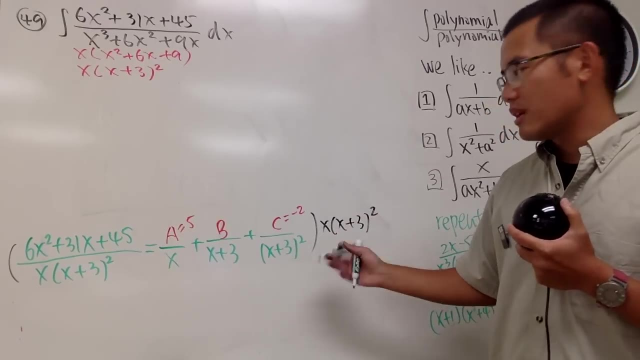 And another way to do it is you could have x equal to 1 or so, but I think it's just consistent. Let's just do the dirty algebra. I think my students like this And from experience my teaching, I think this is easier. 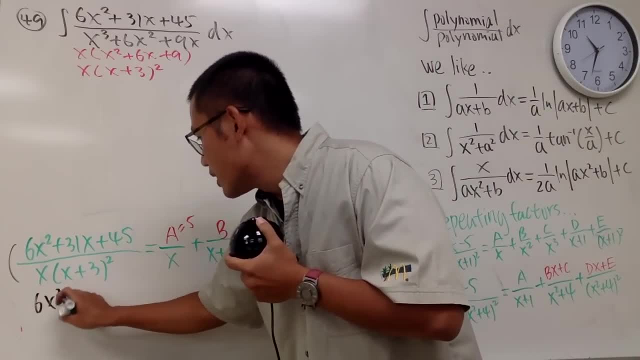 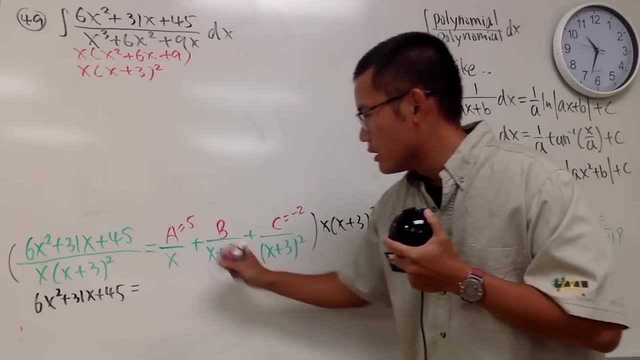 Anyway, this times that we get this, which is 6x squared plus 31x plus 45.. This times that we get 5.. This is 5.. x cancels out already. So we have parentheses x plus 3 squared. 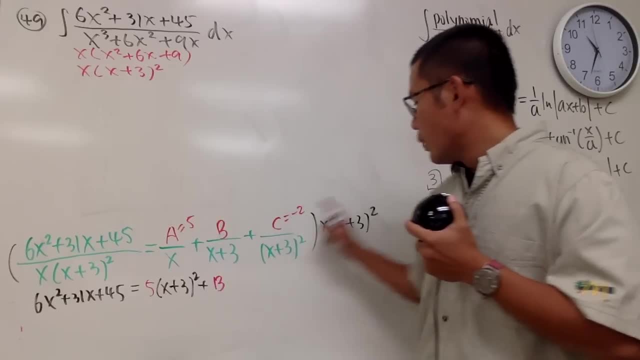 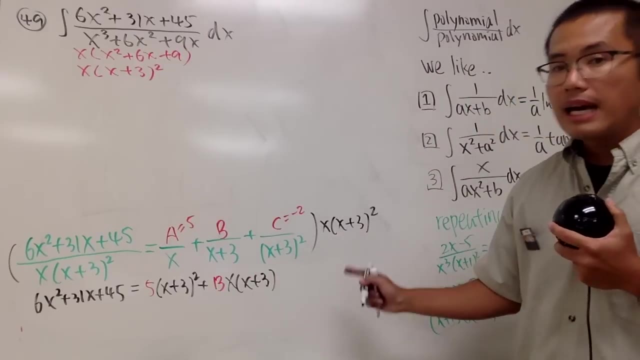 And b, we don't know. so plus b, One of the x plus 3 cancels out. And don't forget the x. So we have x times x plus 3.. Lastly, this and that cancel out, So we have minus 2 times x, just like this. 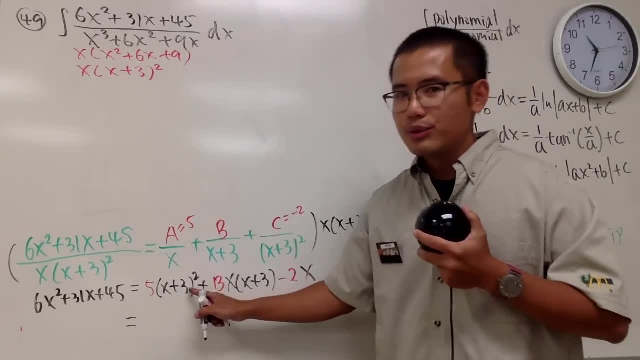 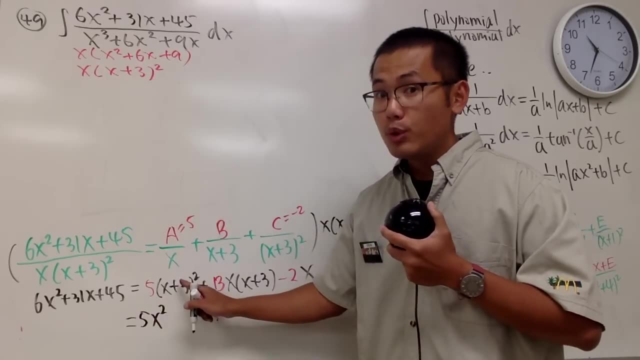 Now do more right here. OK, Let's do this in your head: This is going to be x squared, yeah, So we have 5x squared, And then, when you multiply this out, you will get 6x times the 5.. 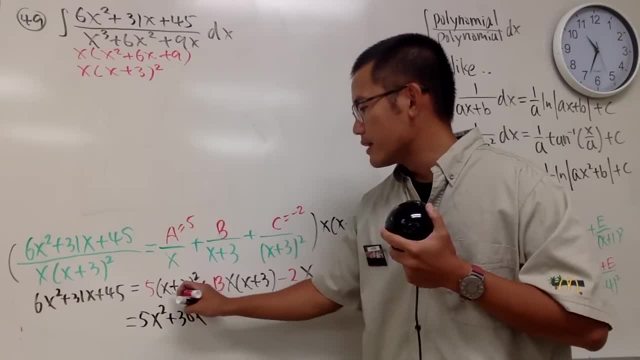 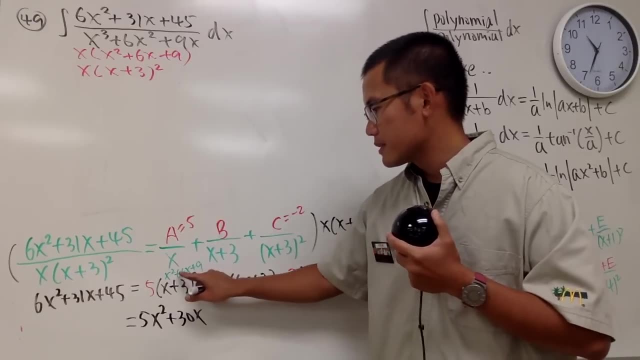 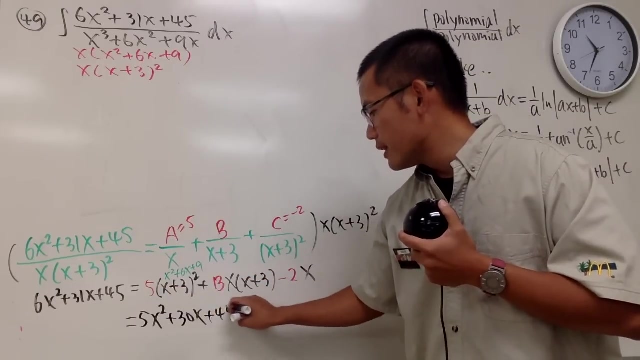 It's going to be plus 30x. Again, let me just show you, guys, all the work. This is x squared plus 6x plus 9.. So this is 30x, and then this is plus 45,, like that. 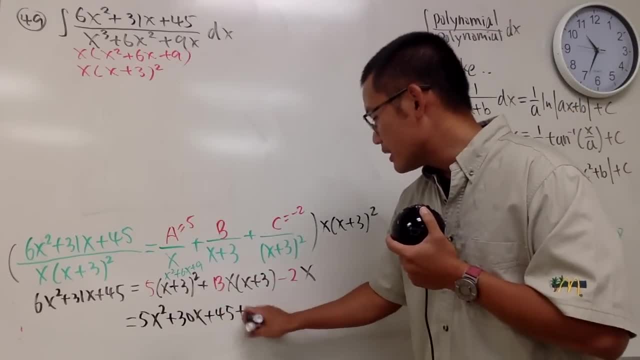 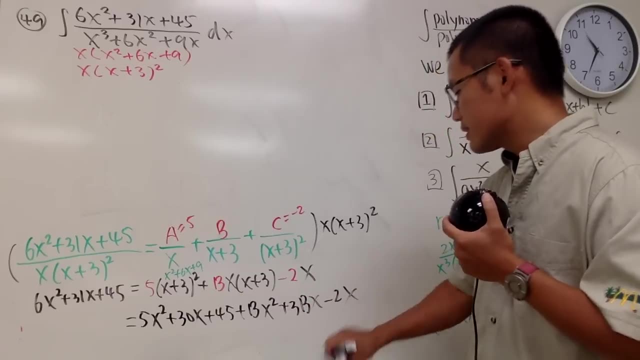 OK, Then you just distribute so we get plus bx squared And then plus 3bx And then minus 2x, And you can guess it. Just look for the x squared term, because we have the b right here. 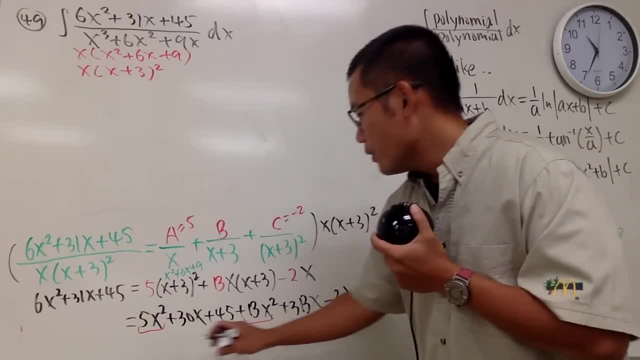 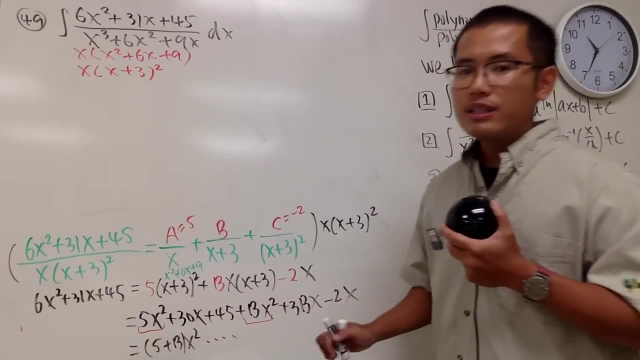 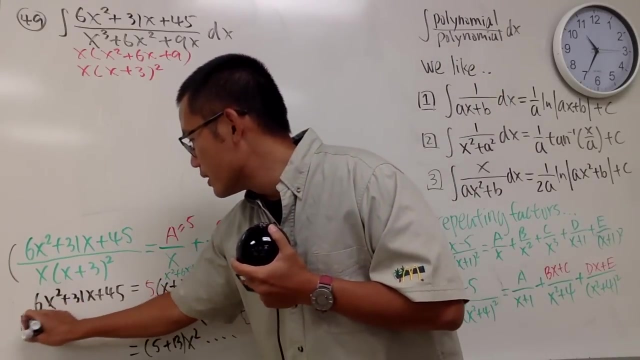 and that's in the front of the x squared. Well, here we get 5 plus b, and then the x squared term and then, da-da-da, Notice- on the left-hand side we have 6x squared. Let's do this thing green again, because I used the red earlier. 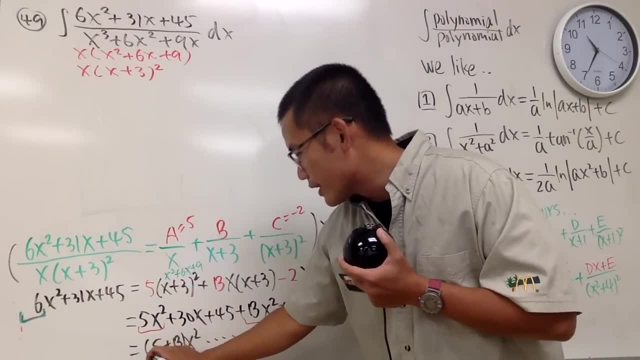 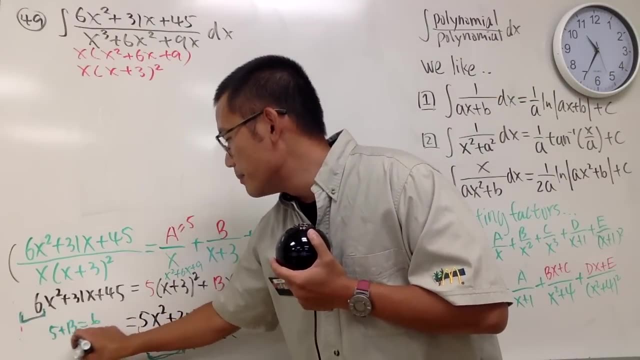 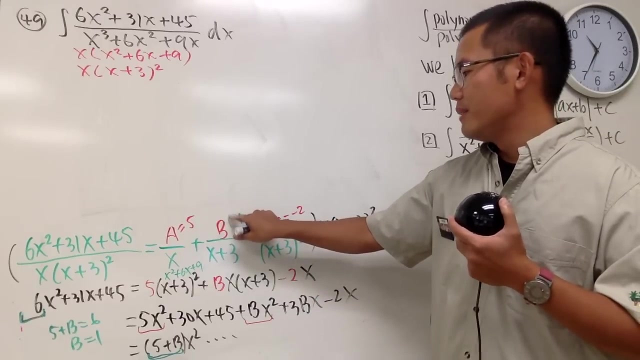 So this is the 6x squared, And this right here is 5 plus b. In another word, 5 plus b has to be 6.. b has to be positive: 1. Done, Whew, Man, It's not. people don't like calculus. 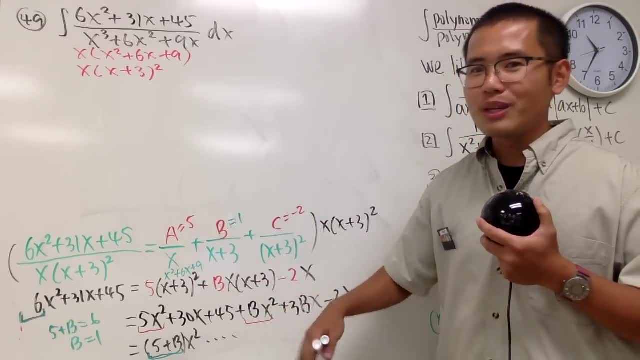 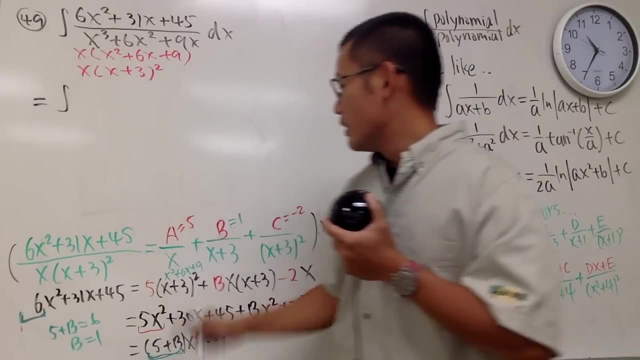 It's people don't like the algebra or the trick in calculus. That's what makes them say they don't like calculus. OK, So here we have the integral This, this and that. For this one we have 5 over x. 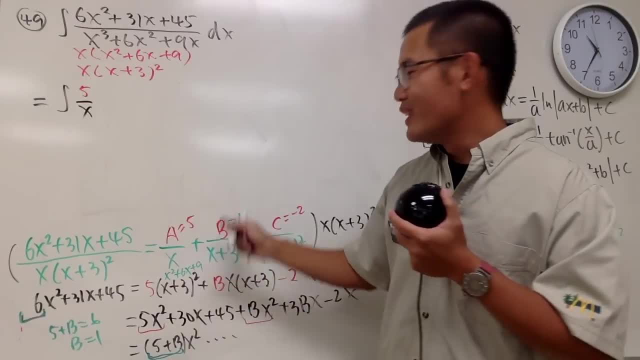 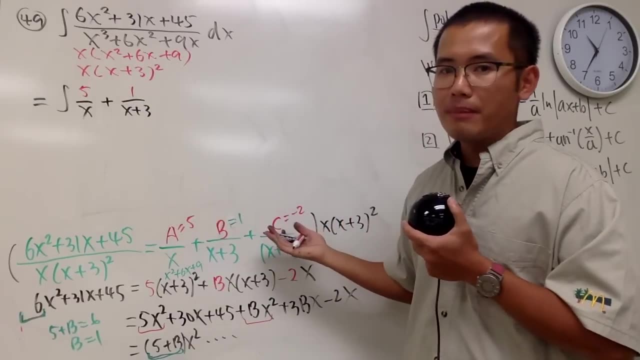 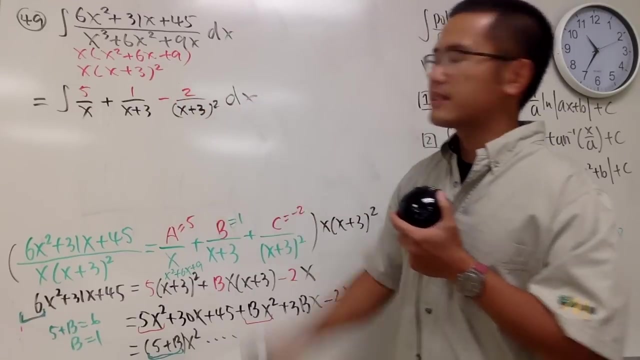 So let's put that down. And then for the next one, we have 1 over that. So let's put down plus 1 over x plus 3.. And lastly, we have the minus 2.. So we have the minus 2 over x plus 3 squared dx. 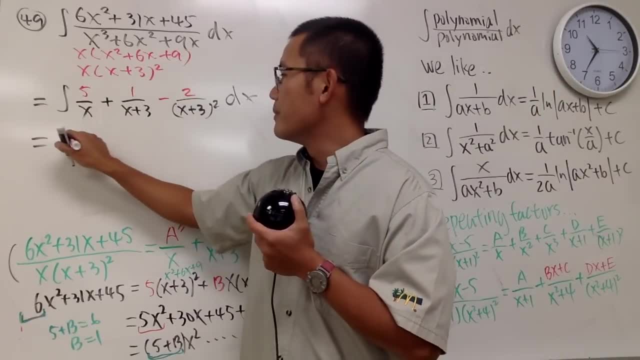 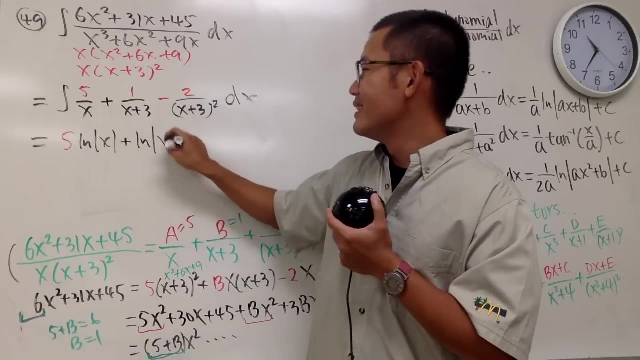 Now integrate this term by term. 5, natural log: absolute power of x Next plus 1, which you don't have to write down- x plus 3, like that. This is something to the second power, So do the reverse power rule. 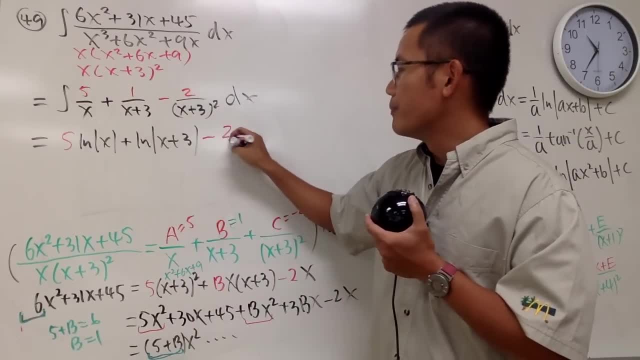 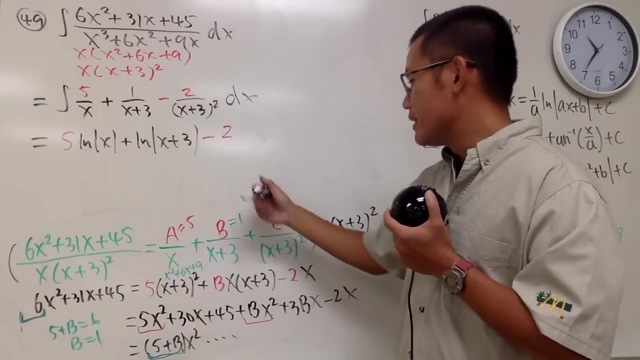 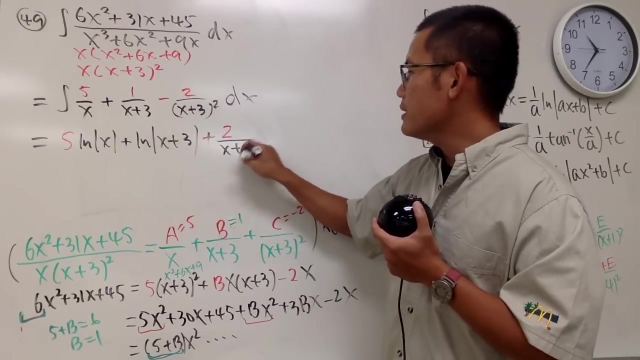 Well, originally we have negative 2. But this is negative. 2 power Plus 1 is negative 1. divided by that It becomes positive. And then this is x plus 3 to the negative 1 power. So it's 2 over x plus 3, like this: 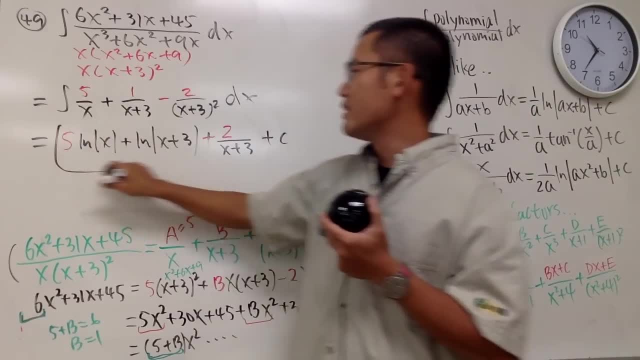 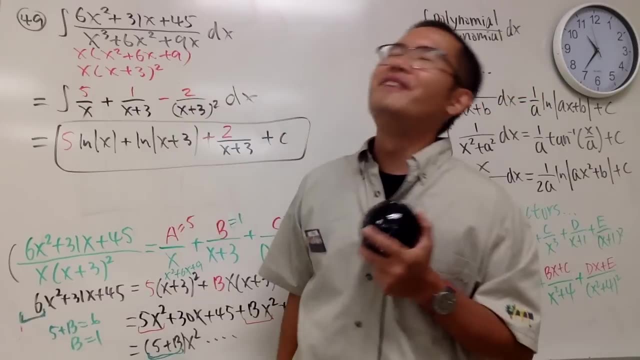 So, just like the similar example earlier- So I'll leave the detail for you guys- That's what we have. OK, Yeah, Number 50.. Oh my god, Last question, And for the last question, in fact, it's really really great. 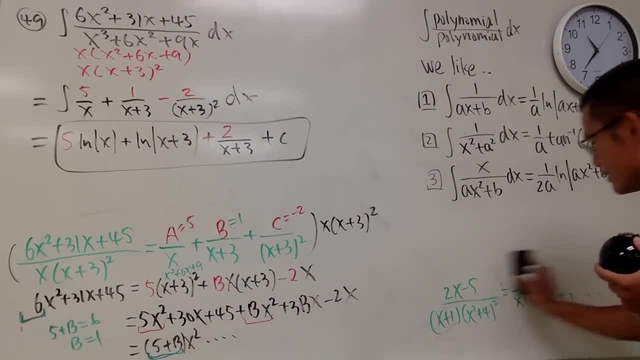 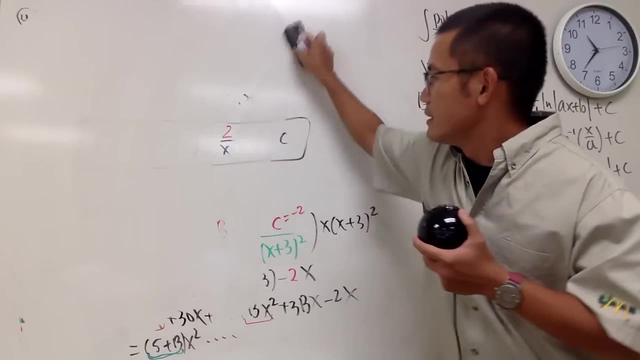 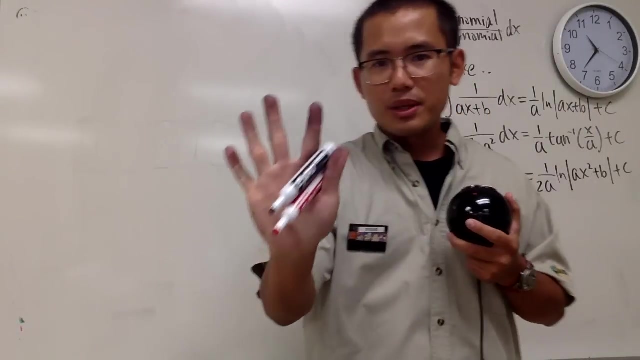 Because I will give you guys another formula, So I don't need this anymore. All right, So I know the question, Of course, And I'm going to just give you guys Seriously dirty algebra, Dirty algebra, Anyway, Number 50.. 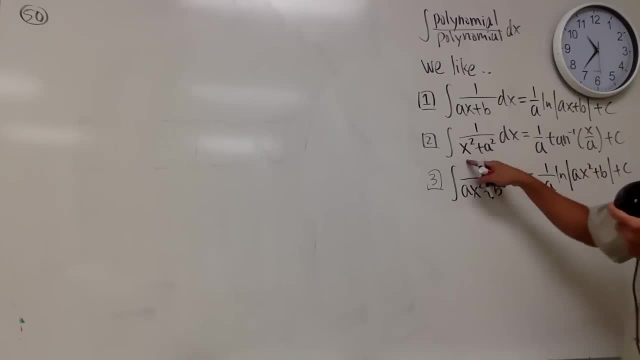 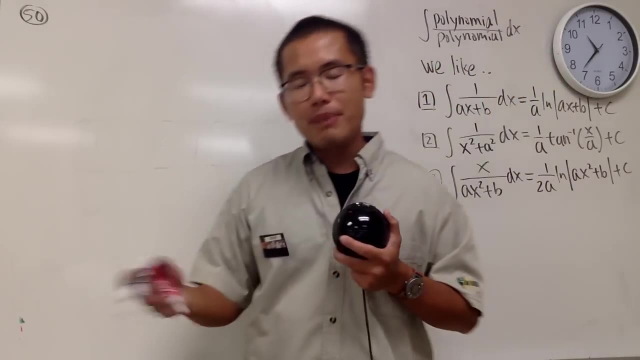 OK, You might notice, here we have integral 1 over x squared plus a squared. Well, what if we have a subtraction instead? Yes, you can do tricks up for it, But no, Let's do partial fractions. Let's do a partial fraction for this. 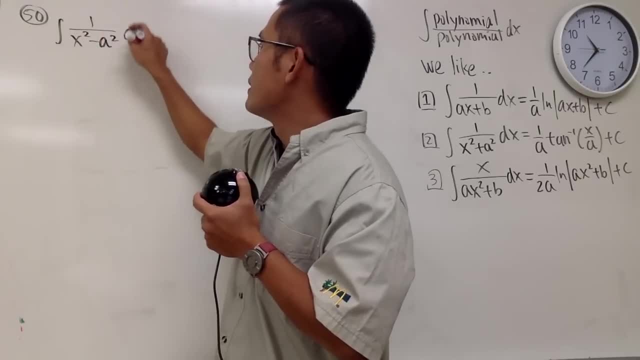 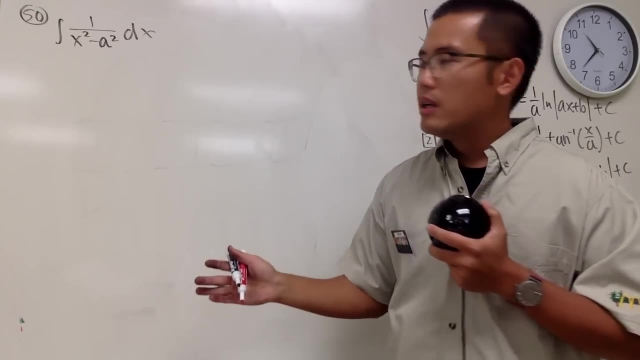 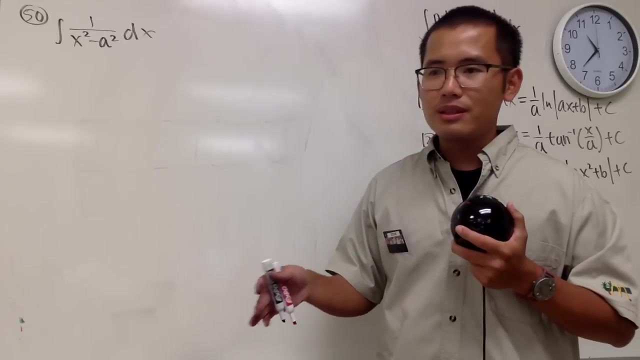 Here we go: Integral 1 over x squared minus a squared dx. I will show you guys how to do partial fraction for this one. Because this one, when you do partial fraction, the answer is actually more universal. I would say: Don't use the hyperbolic tangent or hyperbolic cotangent inverse. 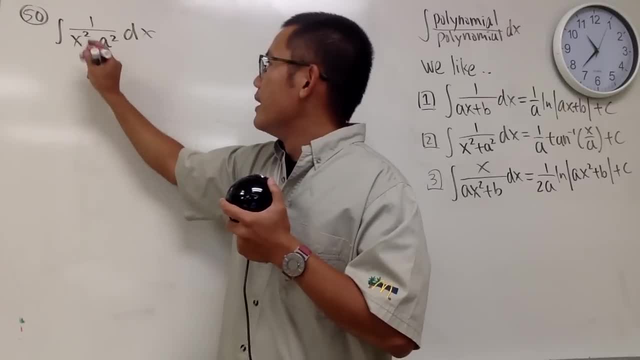 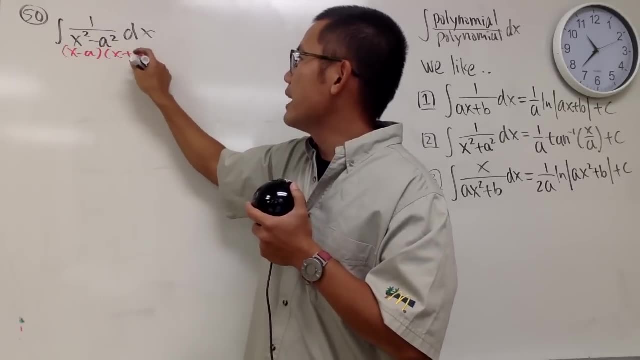 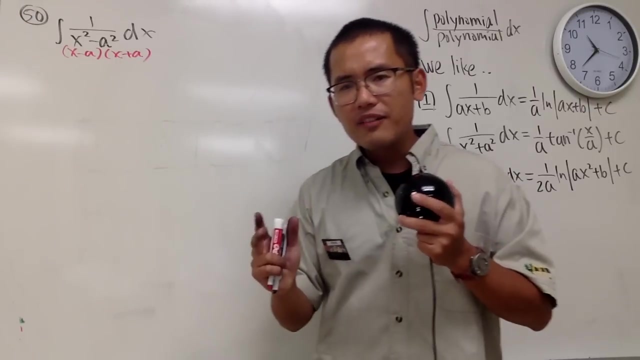 Just do this. Anyway, Here we go. Let's factor this And keep in mind we have a. This is just x minus a times x plus a. Good, And this is the nice case because we have distinct linear factors And for the Kappra method, if you have like 3 or 4, it works the same too. 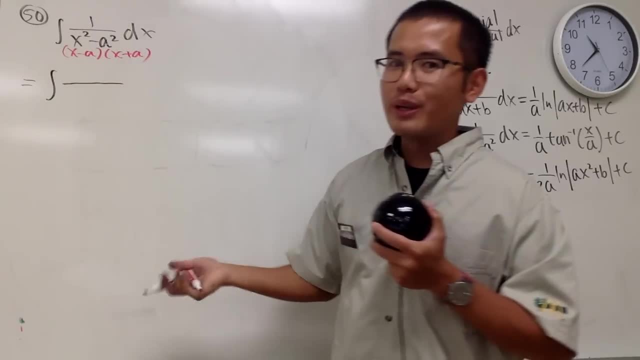 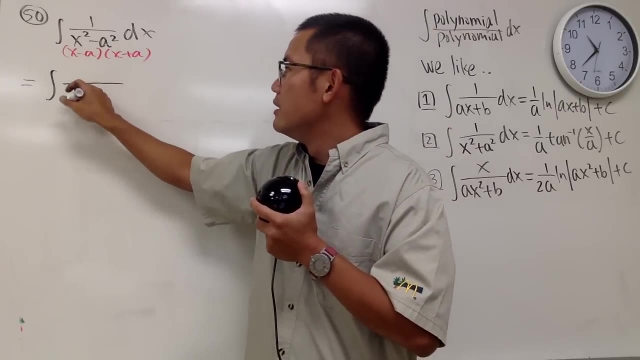 Anyway, Here we go. This time I'll just show you guys how we can do it real quick And let's see if we can get used to this. For the first one, I must have something over x minus a and then plus with something over x plus a. 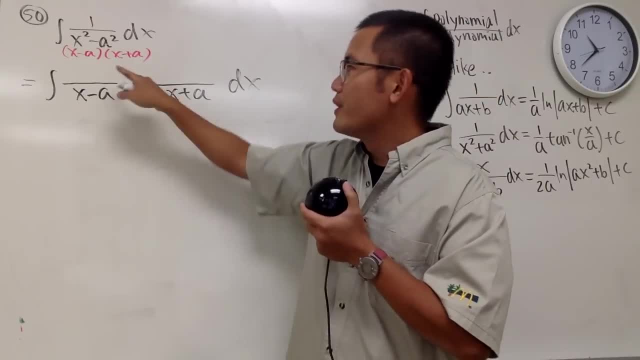 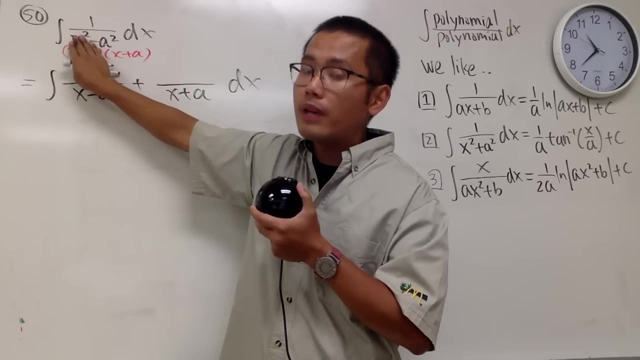 Yeah, Now to figure this out, I go back to the original. I have to couple this up, And I want x minus a to be 0. How can I make that happen? x has to be what s has to be a. 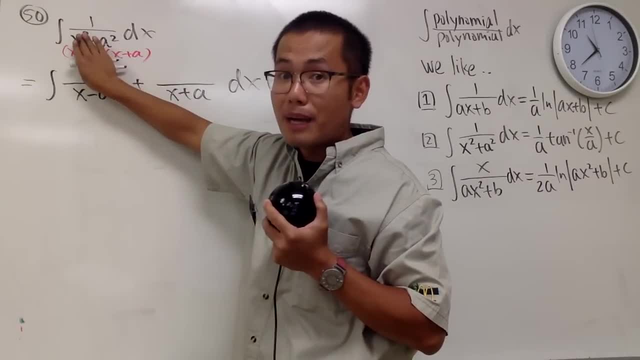 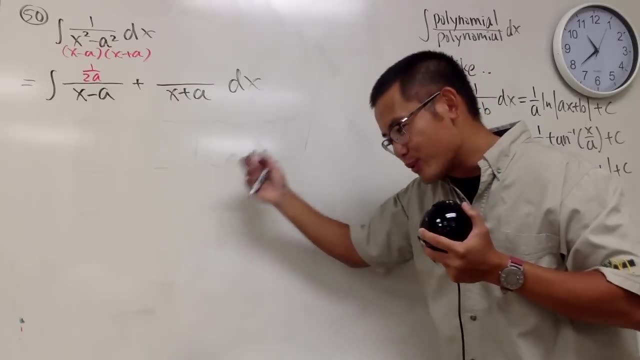 Put the a right here And you have a plus a which is 2a on the bottom, 1 over 2a. then That's the constant here And that's the quicker way to do it if you don't have to show work. 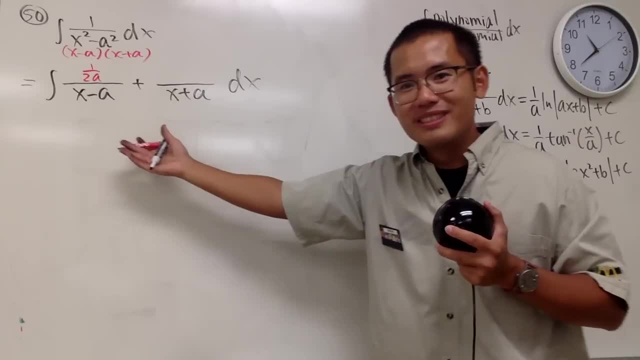 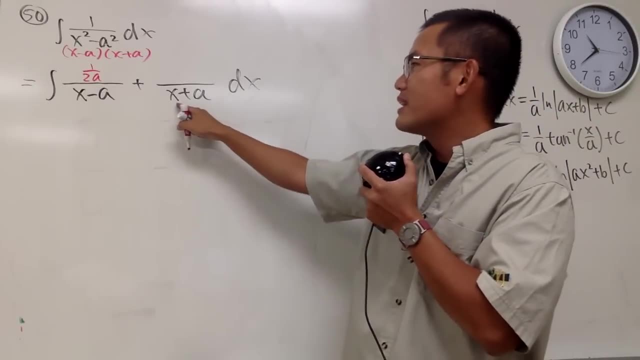 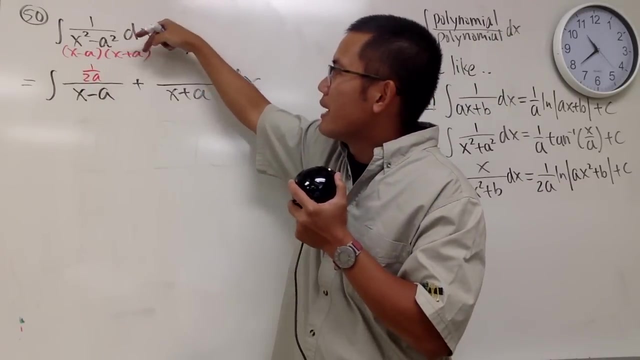 Guys, learn this. You can impress girls, And girls learn this so you can show off to guys. Right, Let's practice another one. Here we have x plus a. We go back to here. Couple this up: How can we make x plus a equal to 0?? 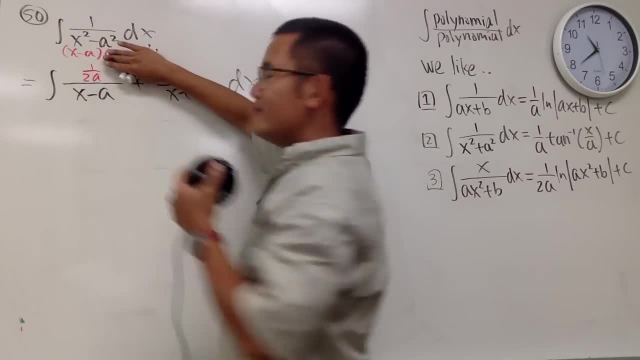 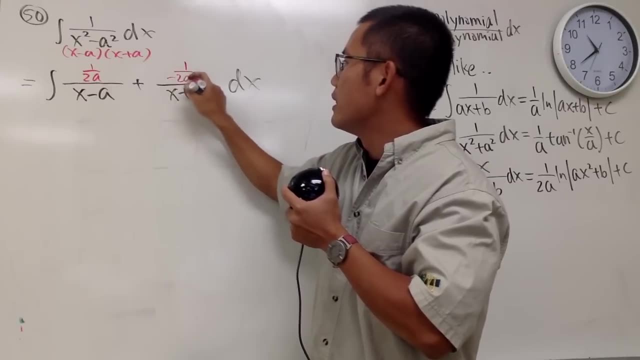 x has to be negative a. Put it here: Negative a minus a is negative 2a. So we have 1 over negative 2a, Like this, And that's just constant multiple. Now we are ready to integrate First one. 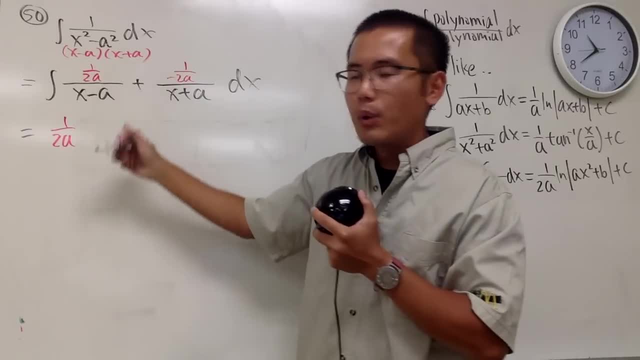 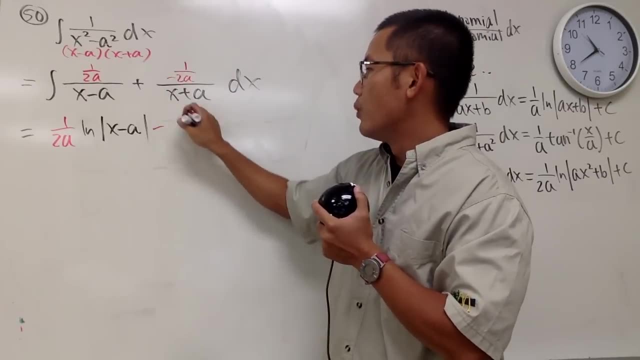 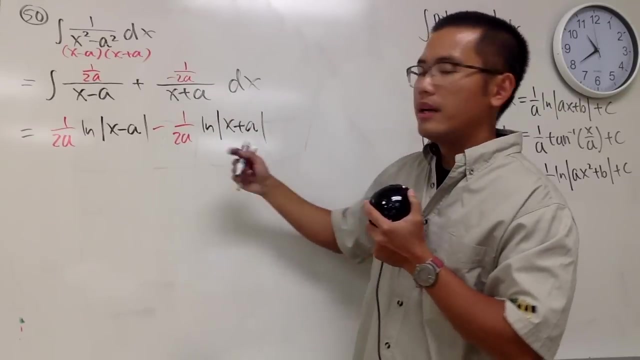 1 over 2a And that will give us natural log absolute value x minus a Like this: Secondly, this is minus 1 over 2a And we have natural log absolute value of x plus a, And again the coefficient here is 1.. 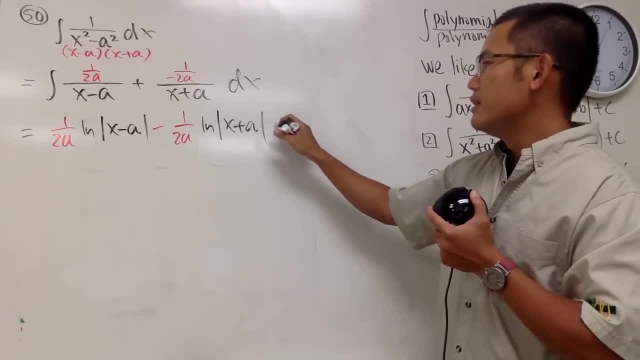 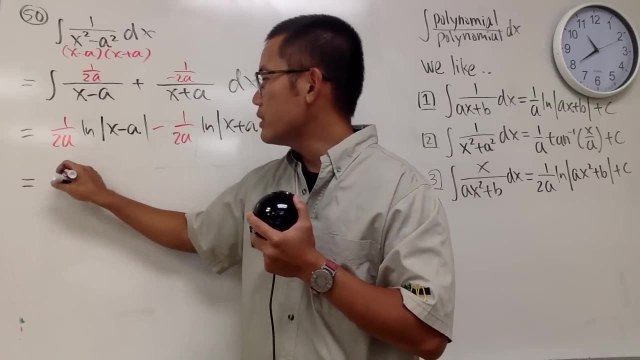 So you don't have to worry about dividing by 1.. This is pretty much it, But not yet, Because- notice- both of them have 1 over 2a, So we can factor that out: 1 over 2a. 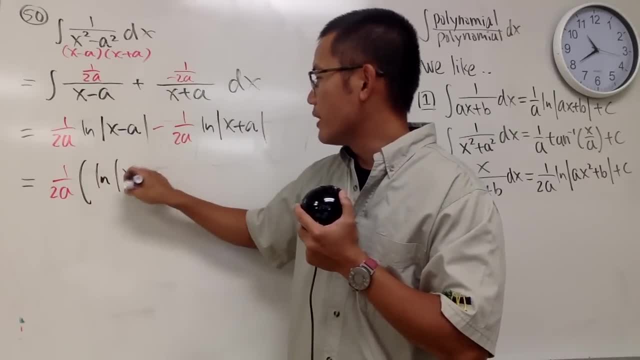 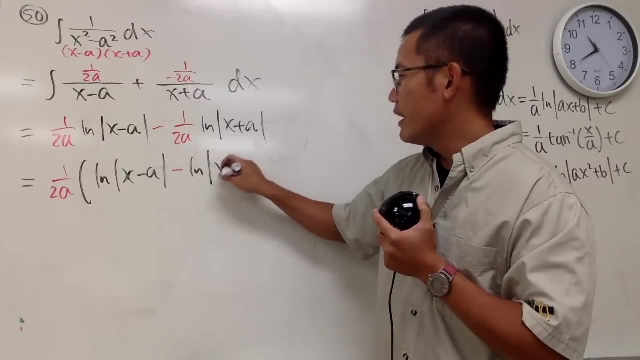 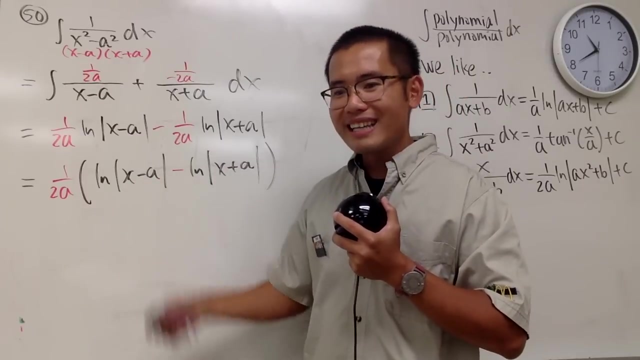 And we will get natural log absolute value of x minus a Minus natural log absolute value of x plus a, Like this In the end, by the log property. we can put this over that, So we end up with a really nice formula. 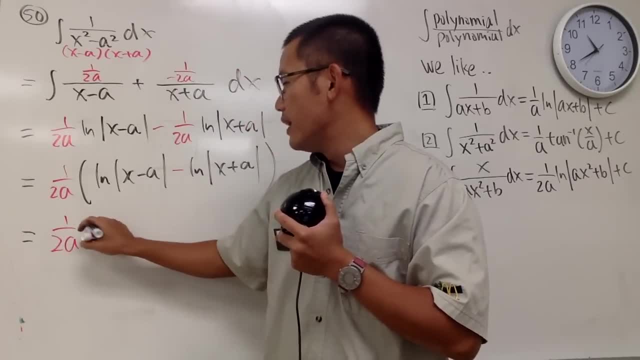 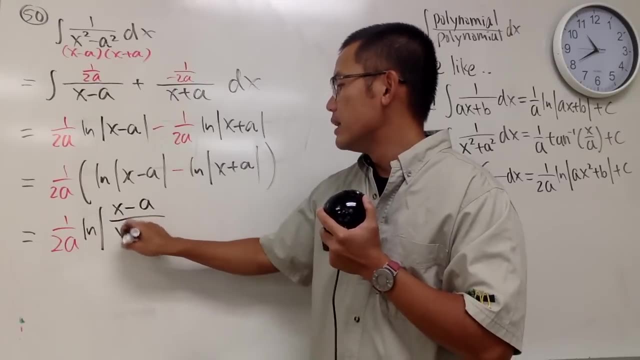 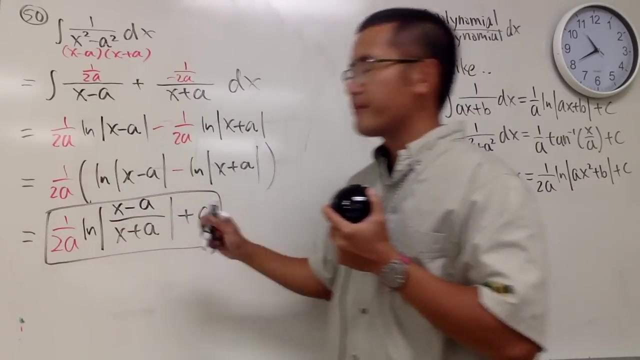 1 over 2a. Natural log: absolute value: x minus a over x plus a. Like this, And we are all done The end Of course. put down the plus c. This is it, And perhaps I'll just write down another formula right here for you guys. 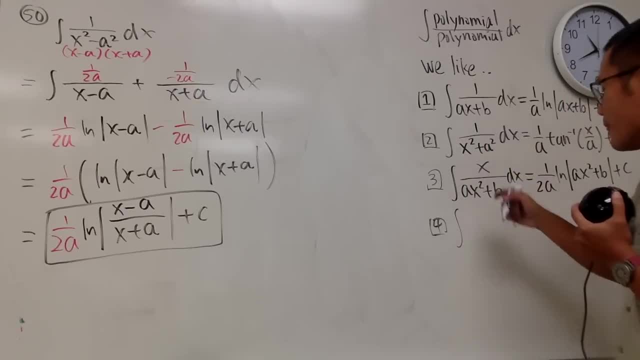 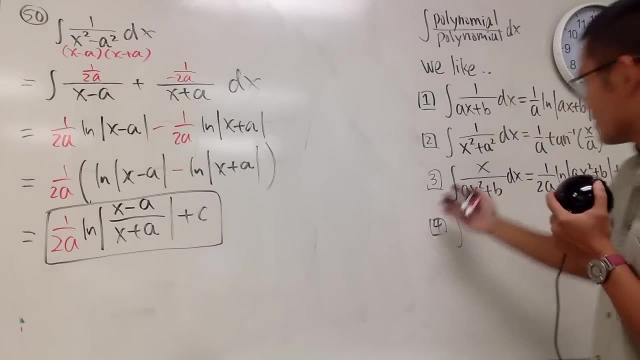 It's pretty much like a complement of the formula number 2.. Imagine if this is stick, then this is the lobster tail. So that's the idea. 1 over x squared minus a squared dx gives us that, Which is 1 over 2a. ln. absolute value of x minus a, x plus a plus c. 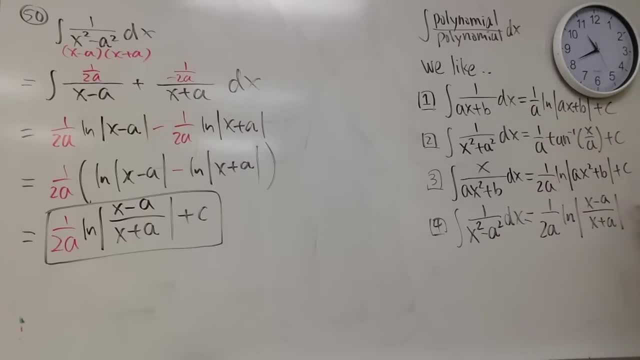 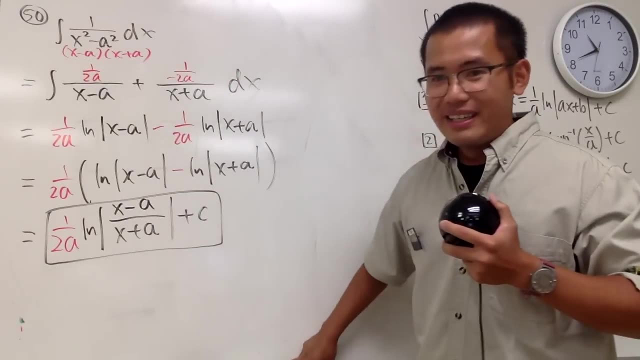 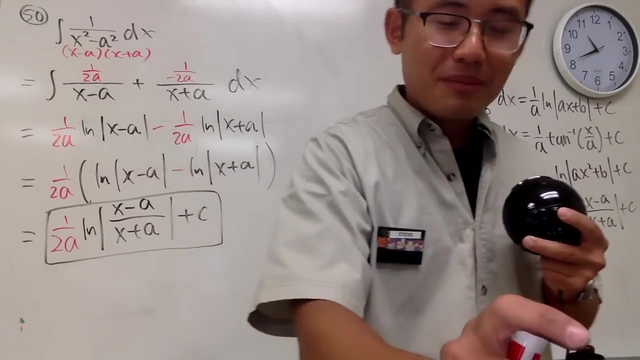 Of course you have other forms for this formula, But again, I will just show you guys this right here, And that's it. Yes, Man, This is so wonderful. Okay, 554.. So it's not exactly 6 hours. 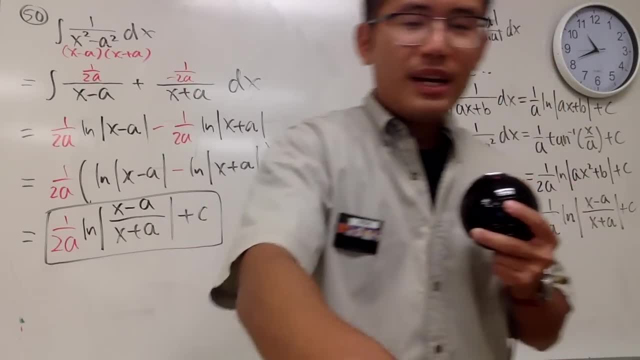 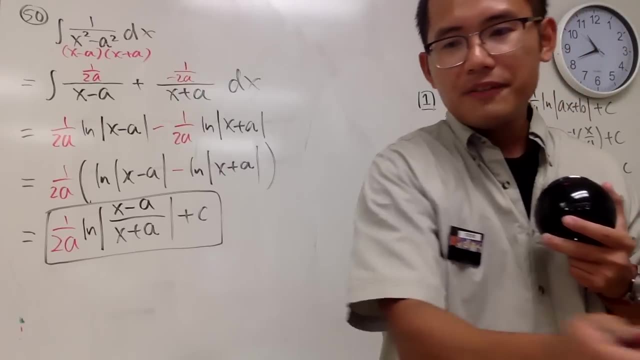 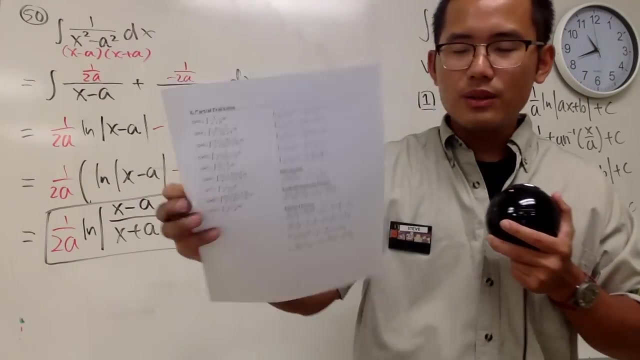 Pretty good, Pretty good, pretty good, All right. Thank you guys, so much for watching And again, hopefully this helps And go download the PDF, Because I typed out all the notes right here for you guys, including the formulas and including other things. 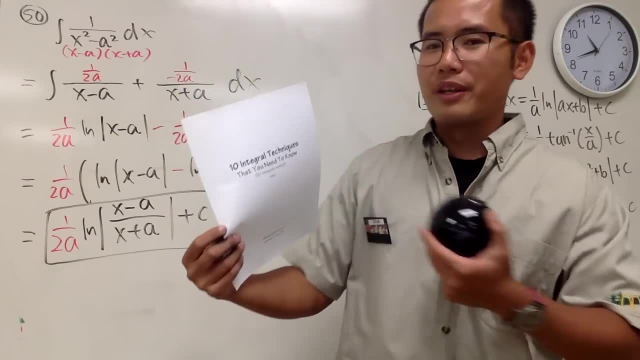 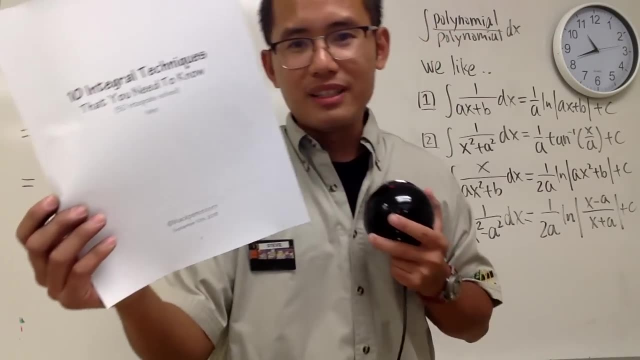 So go download it And if you have a better title for this right here, you can also let me know to give me some suggestions. But I think this is pretty okay. In fact, I came up with this last week, but I didn't have the time to actually work this out. 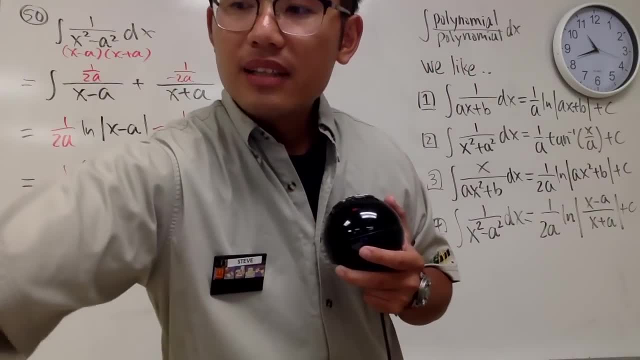 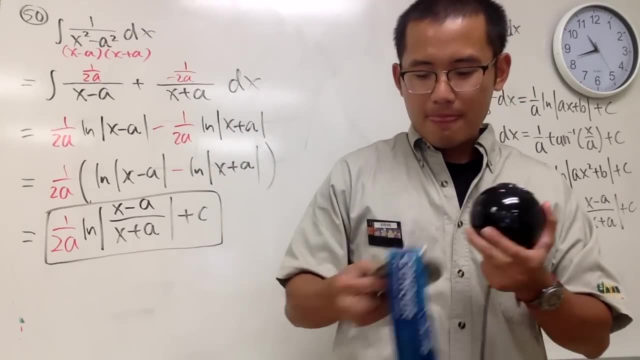 So I'm doing this today And, as always, you guys know that I will show you guys a marathon. Sorry, I will show you guys a marathon battle. This is the one from this year, Look 2019.. And it has two sides actually. 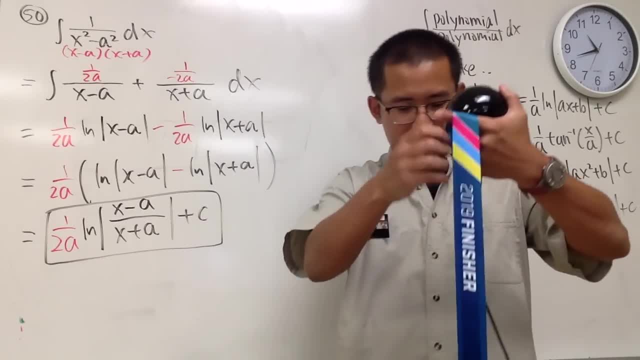 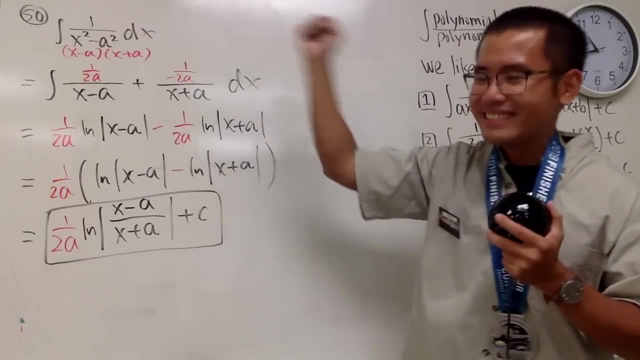 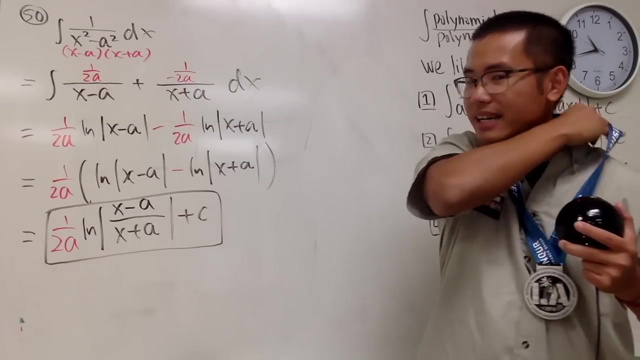 Like this. I'll put this up. It's only 6 hours, so not so bad. Yes, Yes, yes. So this right here covers all the integration techniques that you have to know, And well, I think I did my work. 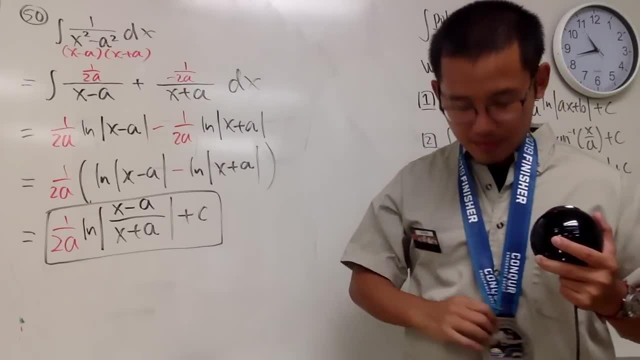 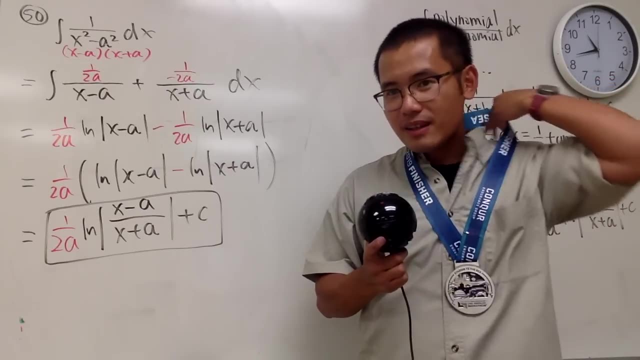 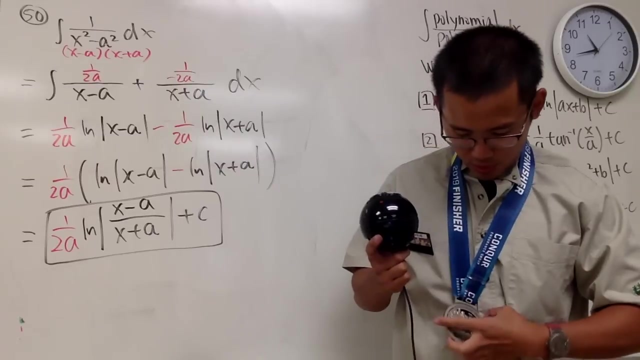 I did my job, So the rest is you guys. You have to put in effort to actually do a lot more practice and all those things, All right. So let me just put this down, Whew, So I can maybe take a screenshot like this for the thumbnail.